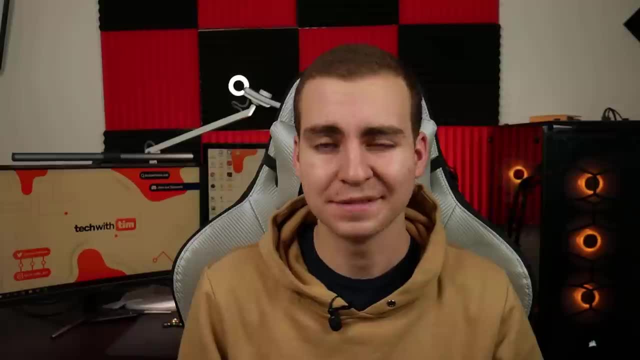 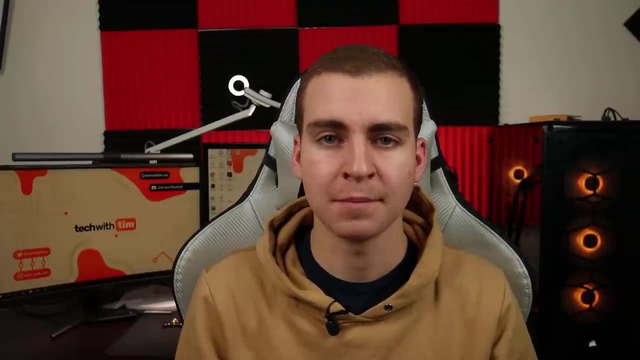 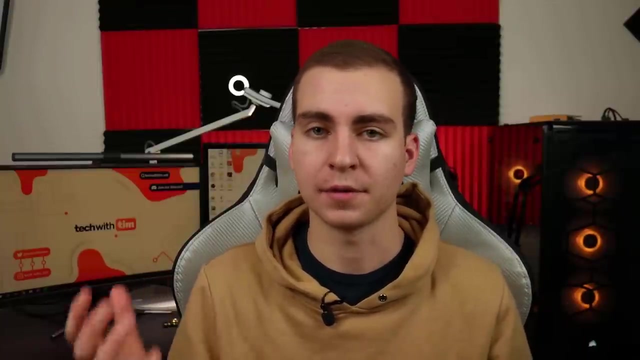 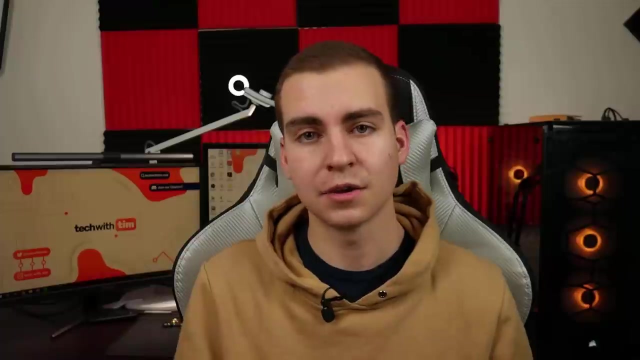 Hello everybody and welcome to an absolutely massive tensorflow slash machine learning, slash artificial intelligence course. Now please stick with me for this short introduction, as I am going to give you a lot of important information regarding the course content, the resources for the course and what you can expect after going through this. Now, first, I will tell you who this course is aimed for. So this course is aimed for people that are beginners in machine learning and artificial intelligence, or maybe have a little bit of understanding but are trying to get better. 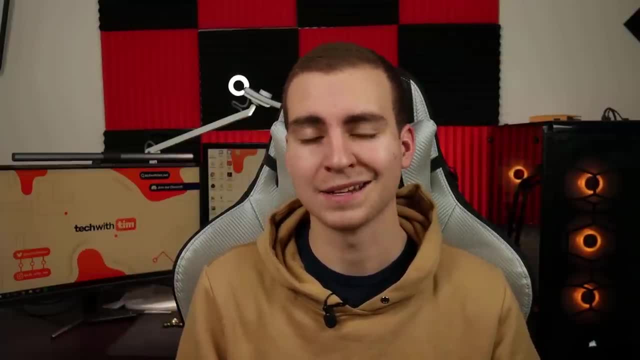 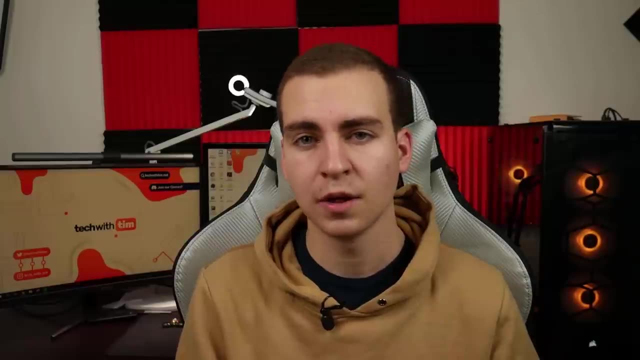 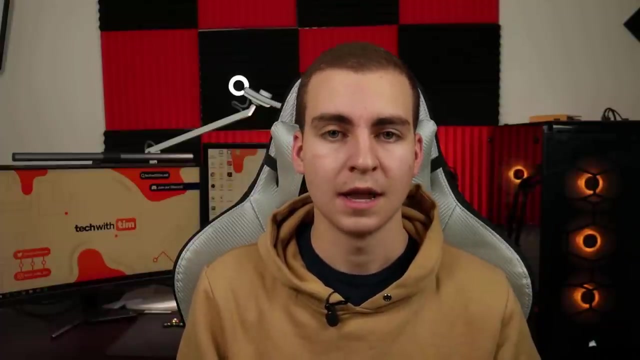 But do have a basic, fundamental knowledge of programming and Python. So this is not a course you're going to take if you haven't done any programming before or if you don't know any Python syntax in general. It's going to be highly advised that you understand the basic syntax behind Python. as I'm not going to be explaining that throughout this course. Now, in terms of your instructor for this course, that is going to be me. My name is Tim. Some of you may know me as tech with Tim from my YouTube channel where I teach all kinds of different programming topics, and I've actually been working with free code camp and posted some of my 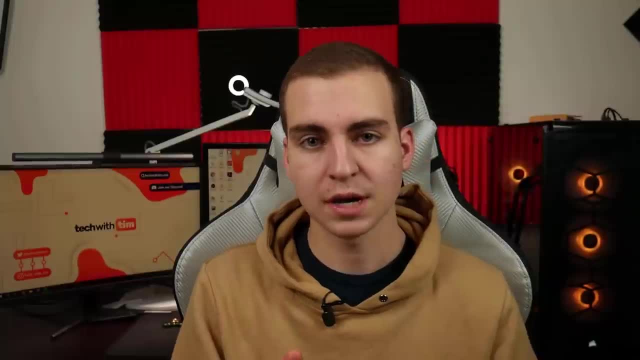 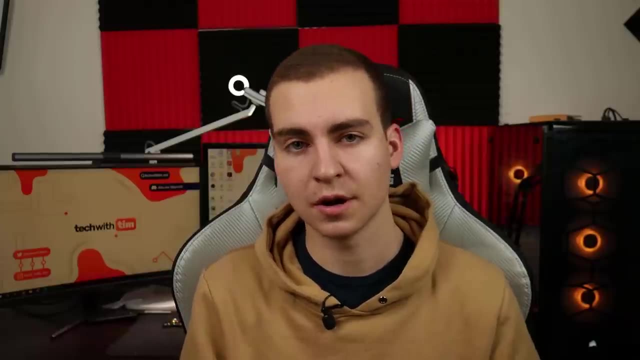 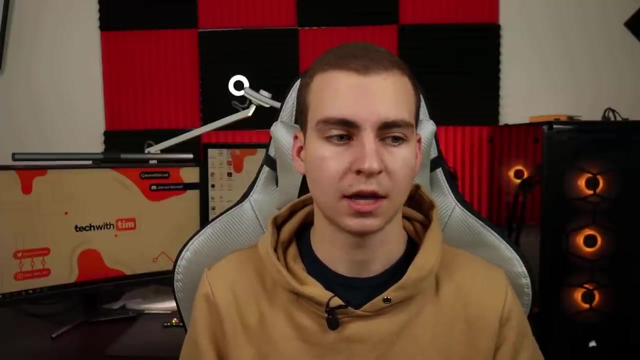 series on their channel as well. Now let's get into the course breakdown and talk about exactly what you're going to learn and what you can expect from this course. So, as this course is geared towards beginners and people just getting started in the machine learning and AI world, we're going to start by breaking down exactly what machine learning and artificial intelligence is, So, talking about what the differences are between them, the different types of machine learning- reinforcement learning, for example, versus neural networks, versus simple machine learning. We're gonna go through all those different differences And then we're going to get into 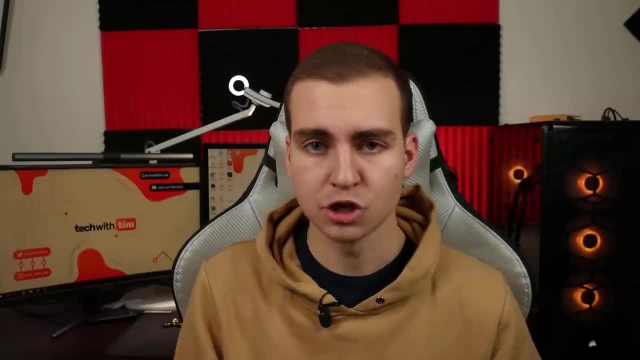 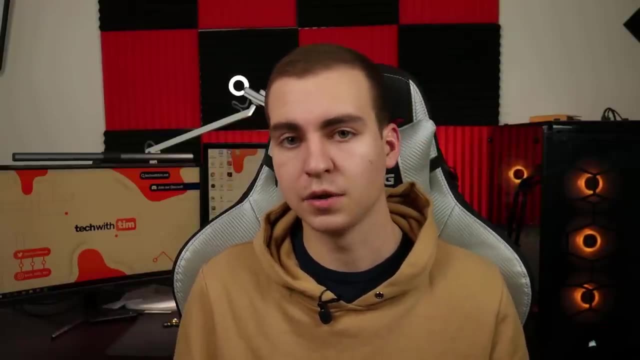 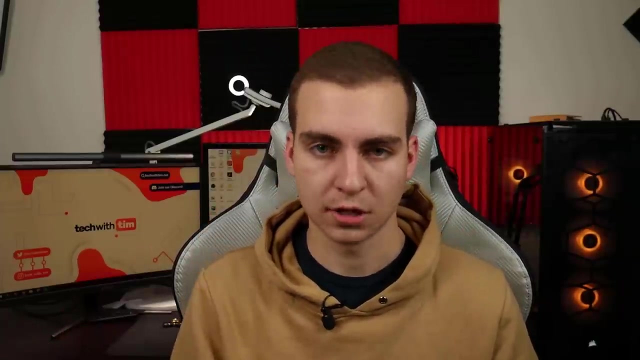 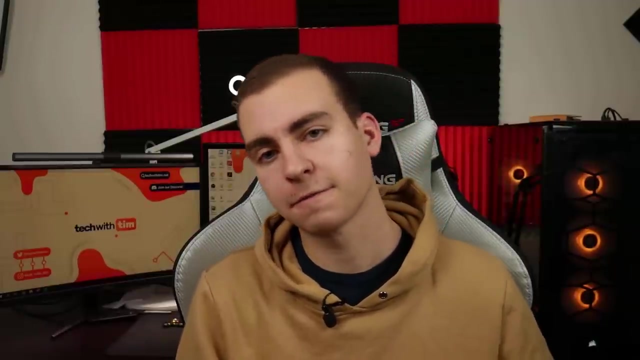 a general introduction of TensorFlow Now. for those of you that don't know, TensorFlow is a module developed and maintained by Google which can be used within Python to do a ton of different scientific computing, machine learning and artificial intelligence applications. We're gonna be working with that through the entire tutorial series And after we do that general introduction to TensorFlow, we're going to get into our core learning algorithms. Now these are the learning algorithms that you need to know before we can get further into machine learning. They build a really strong foundation. They're pretty easy to understand and implement. 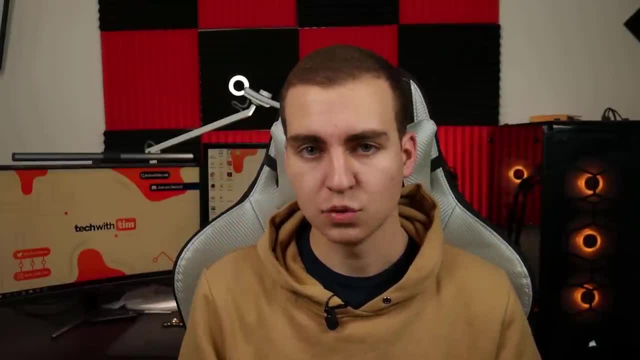 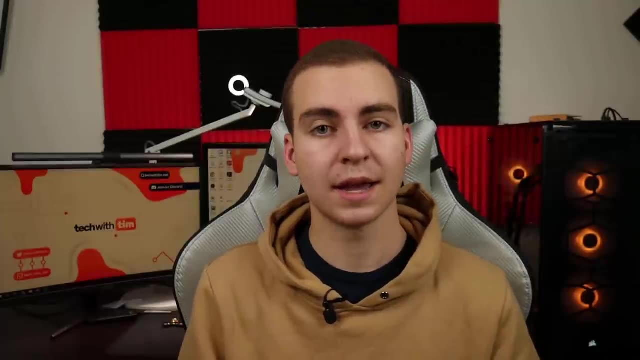 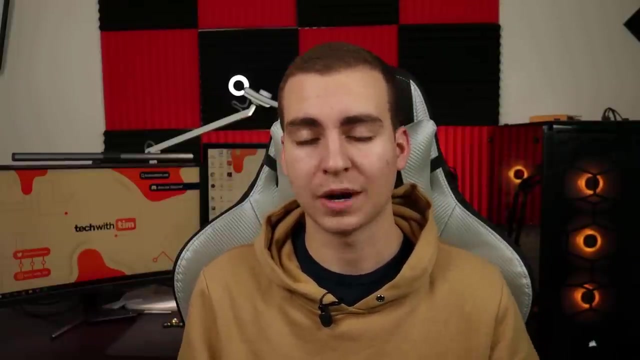 And they're extremely powerful. After we do that, we're going to get into neural networks, discuss all the different things that go into how neural networks work, how we can use them, and then do a bunch of different examples. And then we're going to get into some more complex aspects of machine learning and artificial intelligence and get to convolutional neural networks which can do things like image recognition and detection. And then we're going to get into recurrent neural networks which are going to do things like natural language processing, chatbots, text processing, all those different kinds of things- And finally ended off with reinforcement learning. 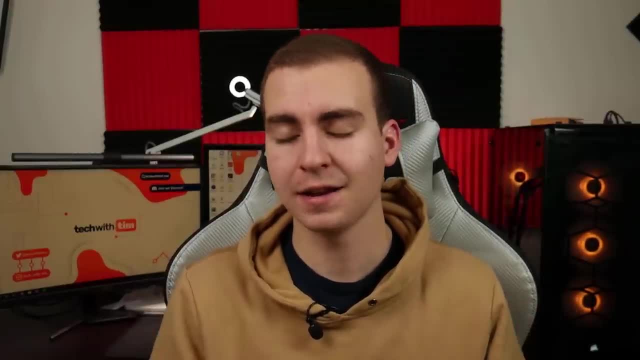 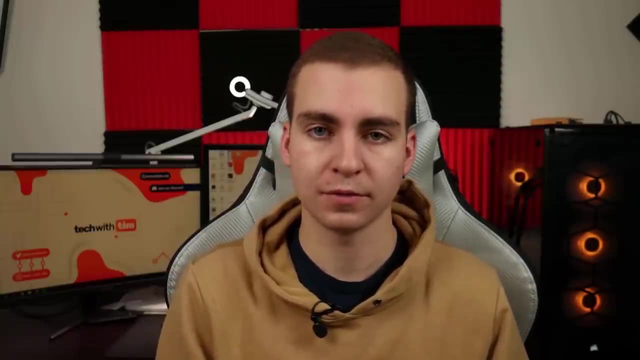 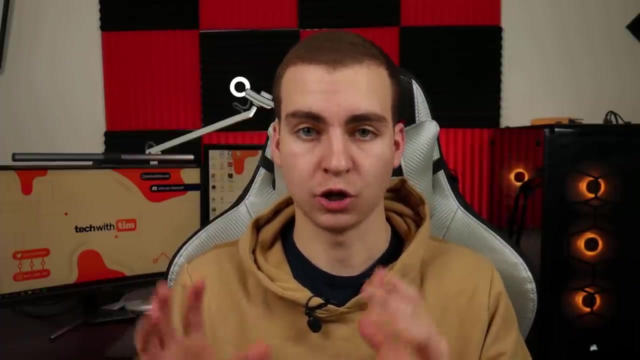 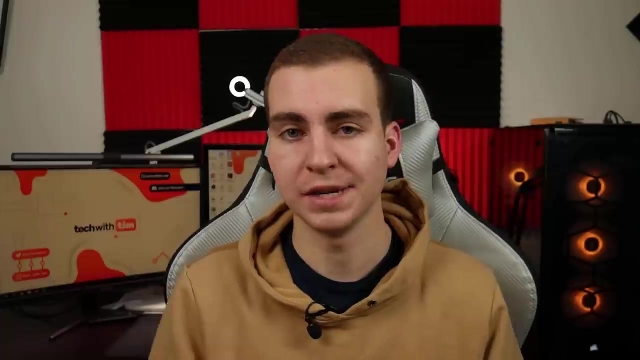 Now, in terms of resources for this course, there are a ton, And what we're going to be doing to make this really easy for you and for me is doing everything through Google Collaboratory. Now, if you haven't heard of Google Collaboratory, essentially it's a collaborative coding environment that runs an iPython notebook in the cloud on a Google machine where you can do all of your machine learning for free. So you don't need to install any packages, you don't need to use pip, you don't need to get your environment set up. all you need to do is open a new Google Collaboratory window and you can start writing code. 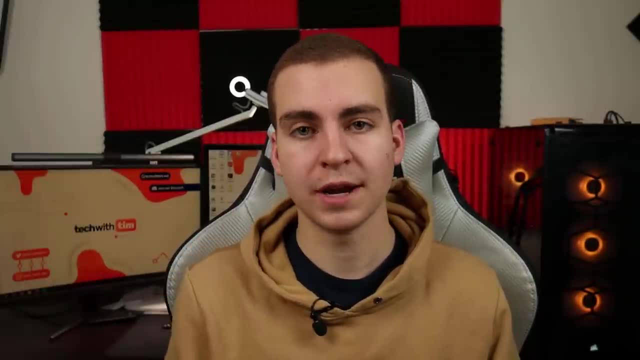 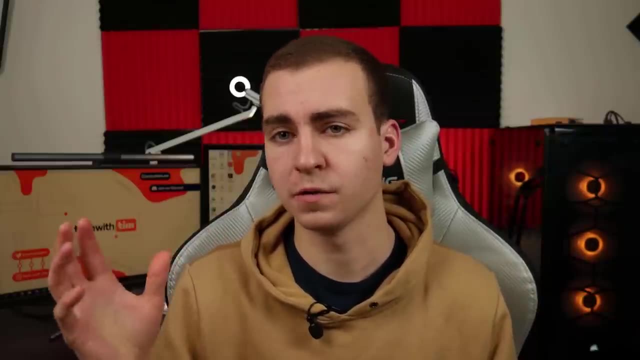 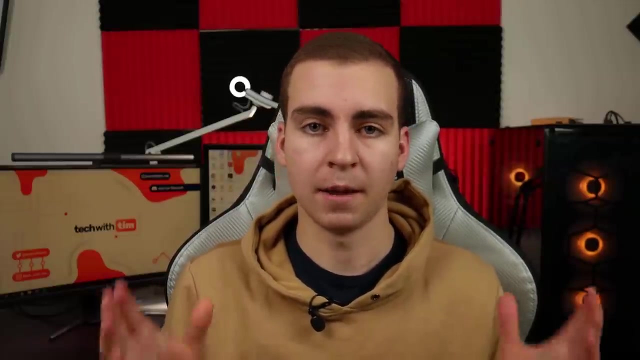 And that's what we're gonna be doing in this series. If you look in the description right now, you will see links to all of the notebooks that I use throughout this guide. So if there's anything that you want to be cleared up, if you want the code for yourself, if you want just text based descriptions of the things that I'm saying, you can click those links and gain access to them. So, with that being said, I'm very excited to get started. I hope you guys are as well, And let's go ahead and get into the content. 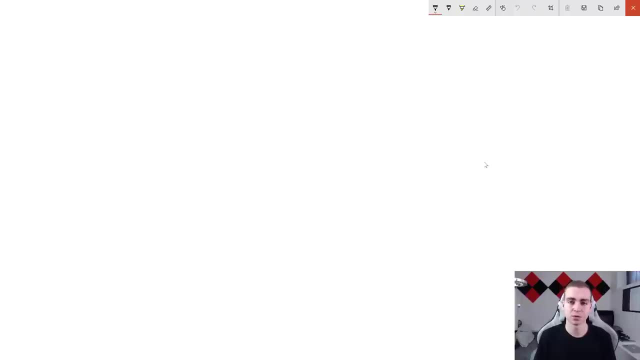 So in this first section I'm going to spend a few minutes discussing the difference between artificial intelligence, neural networks and machine learning, And the reason we need to go into this is because we're going to be covering all of these topics throughout this course. So it's vital that you guys understand what these actually mean And you can kind of differentiate between them. So that's what we're going to focus on now. Now, quick disclaimer here, just so everyone's aware: I'm using something called Windows Ink. this just default comes with Windows. I have a drawing tablet down here And this is what I'm going to be using for some of the explanatory parts where there's no real coding, just to kind of illustrate some concepts and topics. 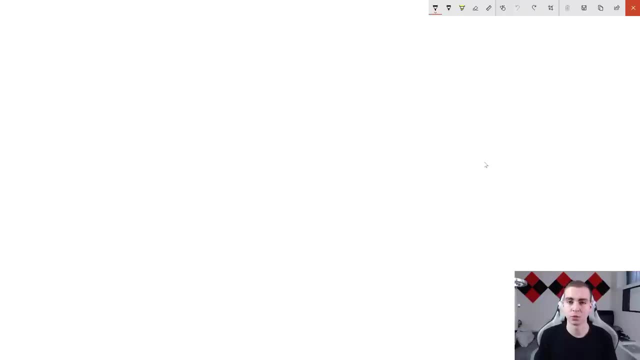 to you Now. I have very horrible handwriting. I'm not artistic whatsoever. programming is definitely more of my thing than you know- drawing and doing diagrams and stuff- But I'm going to try my best And this is just the way that I find I can convey information the best to you guys. So, anyways, let's get started and discuss the first topic here, which is artificial intelligence. Now, artificial intelligence is a huge hype nowadays And it's funny because a lot of people actually don't know what this means, or they try to tell people that what they've created is not artificial. 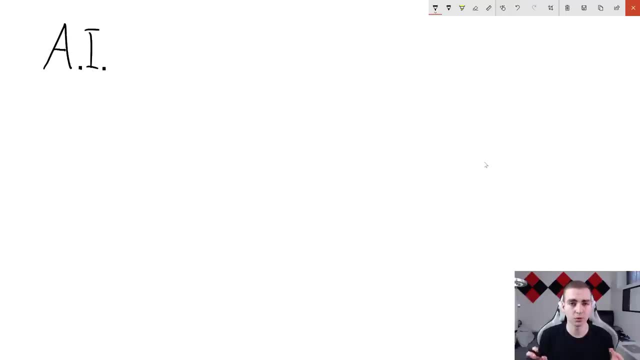 when in reality it actually is. Now, the kind of formal definition of AI- and I'm just going to read it off of my slide here to make sure that I'm not messing this up- is the effort to automate intellectual tasks normally performed by humans. Now, that's a fairly big definition, right? What is considered an intellectual task? And you know, really, that doesn't help us too much. So what I'm going to do is bring us back to when AI was create, first created, to kind of explain to you how AI has evolved and what it really started out being, So back in. 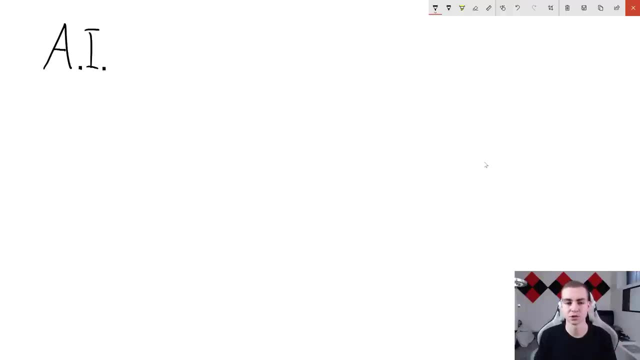 1950, there was kind of the question being asked by scientists and researchers: can computers think? can we get them to figure things out? Can we get away from just hard coding And, you know, having like, can we get a computer to think? can it do its own thing? So that was kind of the question that was asked, And that's when the term artificial intelligence was kind of coined and created. Now, back then AI was simply a predefined set of rules. So if you're thinking about an AI for maybe like tic tac toe or an AI for chess, all they would have had back then. 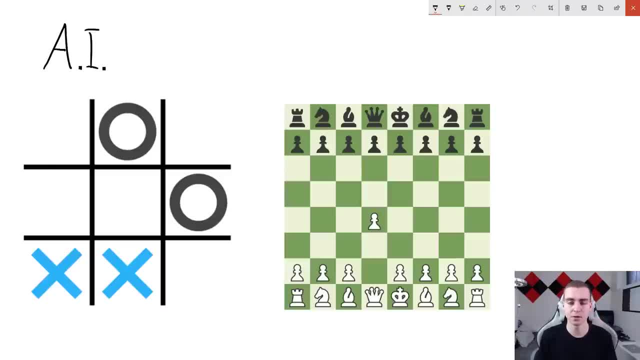 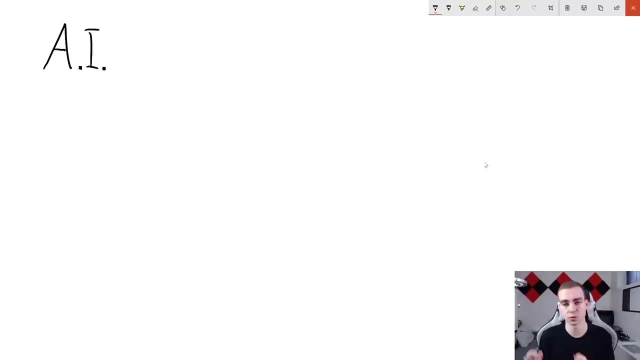 is predefined rules that humans had come up with and typed into the computer in code, And the computer would simply execute those set of rules and follow those instructions. So there was no deep learning, machine learning, crazy algorithms happening. It was simply if you wanted the computer to do something, you would have to tell it beforehand, say you're in this position and this happens, do this. And that's what AI was, And very good. AI was simply just a very good set of rules or a ton of different rules that humans had implemented into some program. you can have AI programs. 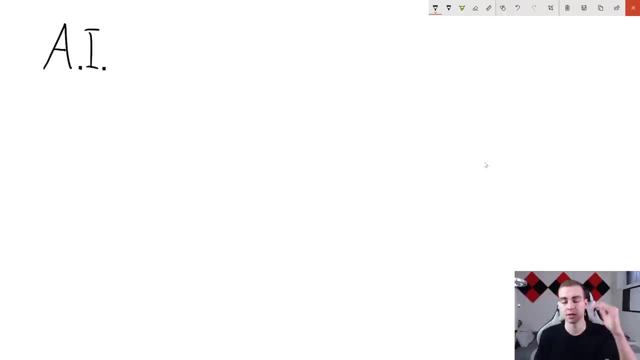 that are stretching, you know, half a million lines of code, just with tons and tons and tons of different rules that have been created for that AI. So just be aware that AI does not necessarily mean anything crazy complex or super complicated, But essentially, if you're trying to simulate some intellectual task like playing a game that a human would do with a computer, that is considered AI. So even a very basic artificial intelligence for a tic tac toe game where it plays against you, that is still considered AI. And if we think of something like 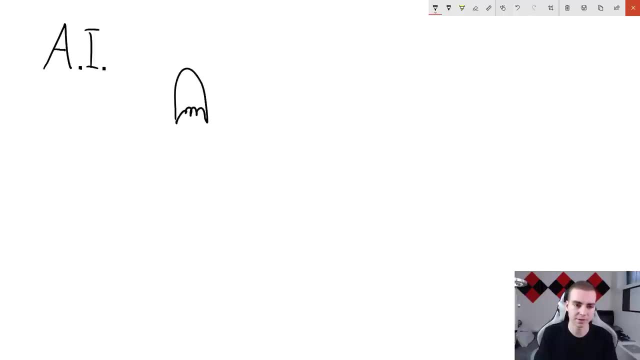 Pac Man right, where we have, you know, our little ghost- and this will be my rough sketch of a ghost- and we have our Pac Man guy, who will just be this. well, would we consider this ghost AI? what it does is it attempts to find and kind of simulate how it would get to Pac Man right, And the way this works is just using a very basic pathfinding algorithm. This has nothing to do with deep learning or machine learning or anything crazy, But this is still considered artificial intelligence. the computer is figuring out how it can kind of play and do something by following an 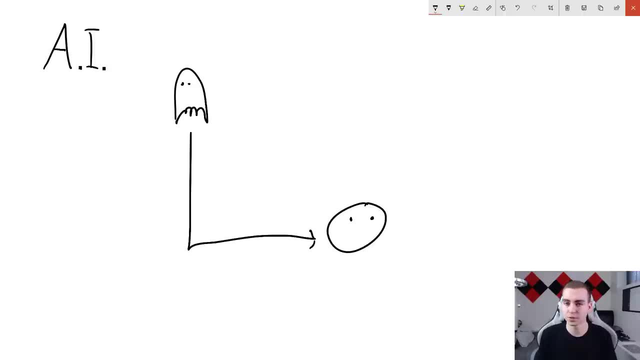 algorithm. So we don't necessarily need to have anything crazy, stupid, complex to be considered AI. it simply needs to just be simulating some intellectual human behavior. That's kind of the definition of artificial intelligence. Now, obviously, today AI has evolved into a much more complex field, where we now have machine learning and deep learning and all these other techniques, which is what we're going to talk about now. So what I want to start by doing is just drawing a circle here, And I want to label this circle and say a I like that. So this is going to define AI. 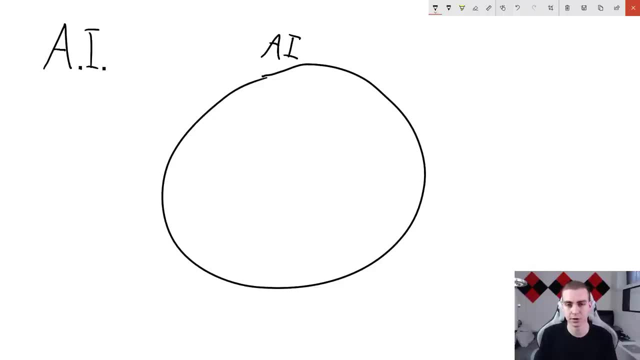 because everything I'm about to put inside of here is considered artificial intelligence. So now let's get into machine learning. So what I'm going to do is draw another circle inside of here And we're going to label this circle ml for machine learning. Now notice, I put this inside of the artificial intelligence circle. This is because machine learning is a part of artificial intelligence. Now, what is machine learning? Well, what we talked about previously was kind of the idea that AI used to just be a predefined set of rules. So what we talked about previously was kind of the idea that AI used to just be a predefined set of rules. 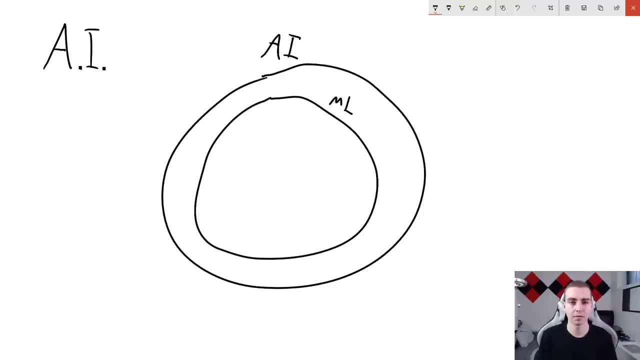 right Where. what would happen is we would feed some data, we would go through the rules by and then analyze the data with the rules And then we'd spit out some output, which would be: you know what we're going to do. So, in the classic example of chess, say we're 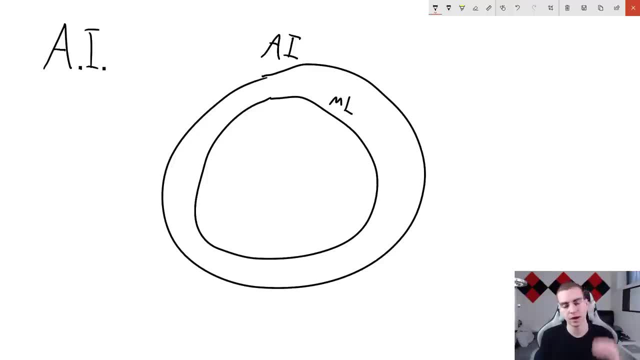 in check. while we pass that board information to the computer, it looks at it, sets of rules, it determines we're in check and then it moves us somewhere else. Now, what is machine learning? in contrast to that? Well, machine learning is kind of the first field, that actually. 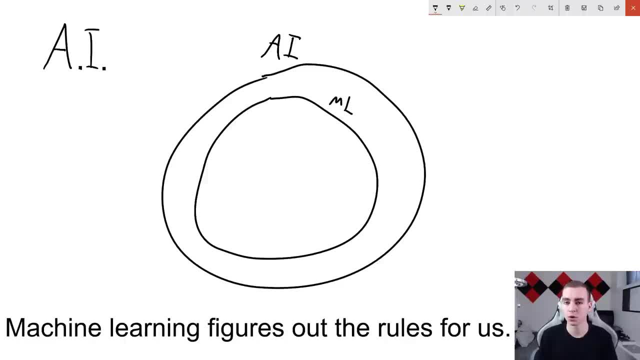 figuring out the rules for us. So, rather than us hard coding the rules into the computer, what machine learning attempts to do is take the data and take what the output should be and figure out the rules for us. So you'll often hear that you know machine learning. 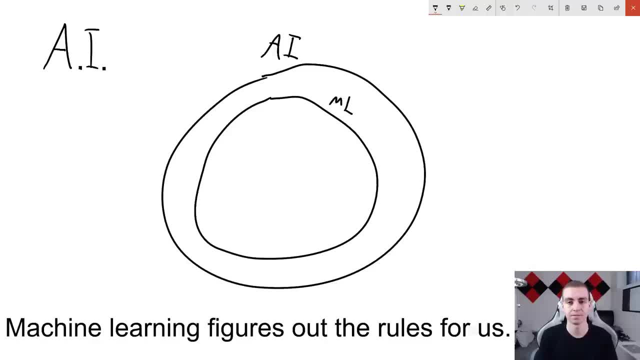 requires a lot of data and you need ton of examples and, you know, input data to really train a good model. Well, the reason for that is because the way that machine learning works is it generates the rules for us. we give it some input data, we give it what the output. 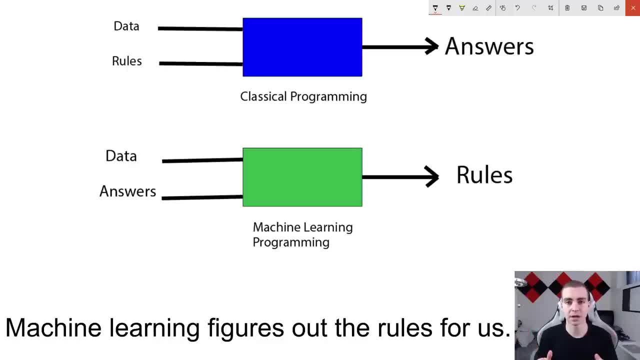 data should be, And then it looks at that information and figures out: what rules can we generate so that, when we look at new data, we can have the best possible output for that? Now, that's also why, a lot of the times, machine learning models do not have 100% accuracy, which means 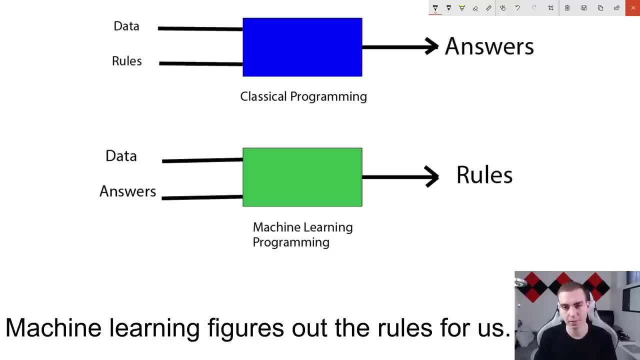 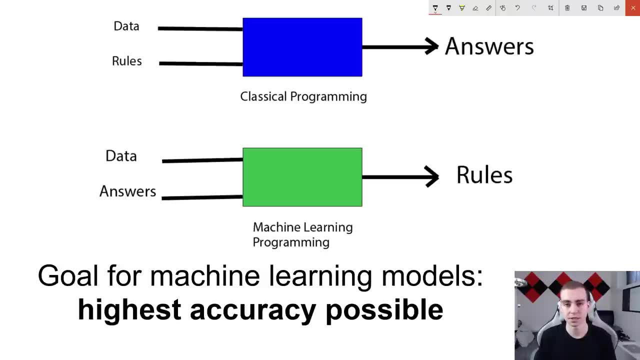 that they may not necessarily get the correct answer every single time, And our goal when we create machine learning models is to raise our accuracy as high as possible, which means it's going to make the fewest mistakes possible because, just like a human, you know our machine. 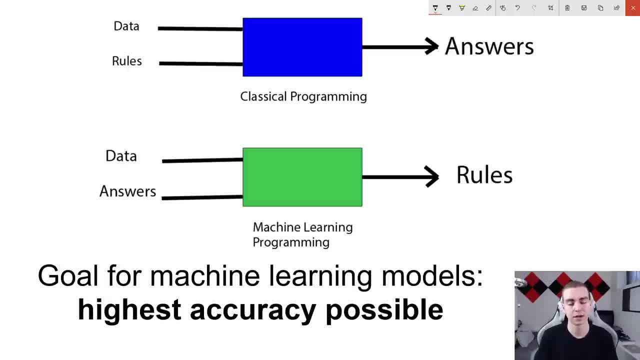 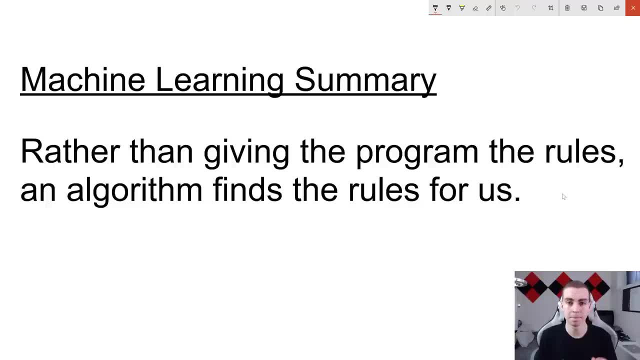 learning models which are trying to simulate. you know, human behavior can make mistakes. But to summarize that, essentially machine learning, the difference between that and kind of, you know, algorithms and basic artificial intelligence is the fact that rather get that, rather than us the programmer giving it the 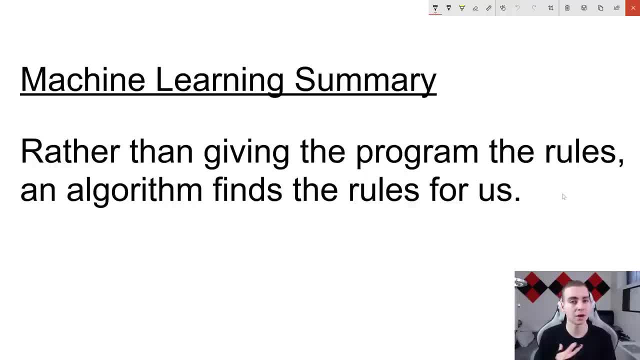 rules. it figures out the rules for us And we might not necessarily know explicitly what those rules are when we look at machine learning and create machine learning models. But we know that we're giving some input data, we're giving the expected output data and then 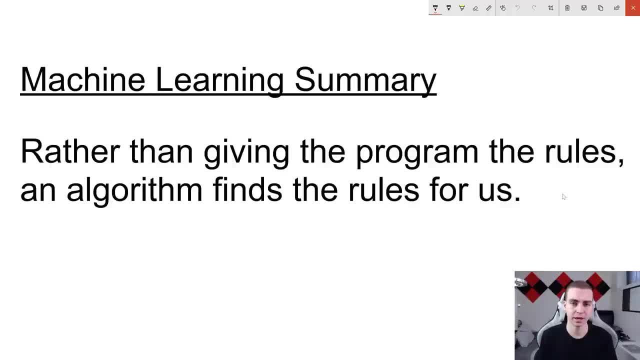 it looks at all of that information. It does some algorithms- which we'll talk about later on that- and figures out the rules for us so that later when we give it some input data and we don't know the output data, it can use those rules that it's figured out from our examples and all that training data. 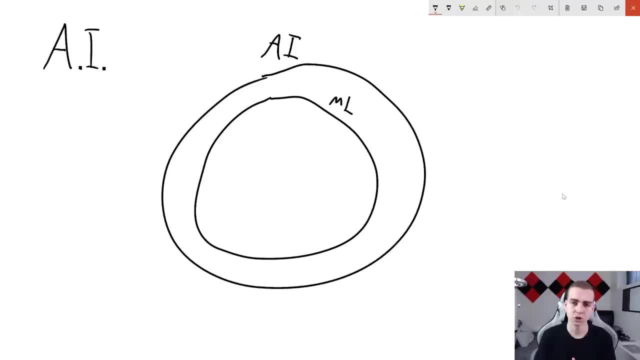 that we gave it to generate some output. Okay, so that's machine learning. Now we've covered AI and machine learning, And now it's time to cover neural networks, or deep learning. Now this circle gets to go right inside of the machine learning. right here I'm just. 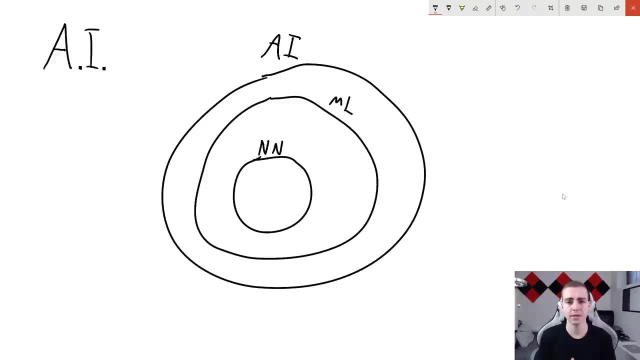 going to label this one nn, which stands for neural networks. Now, neural networks get a big hype. they're usually what the first you know when you get into machine learning. you want to learn neural networks. you're kind of like neural 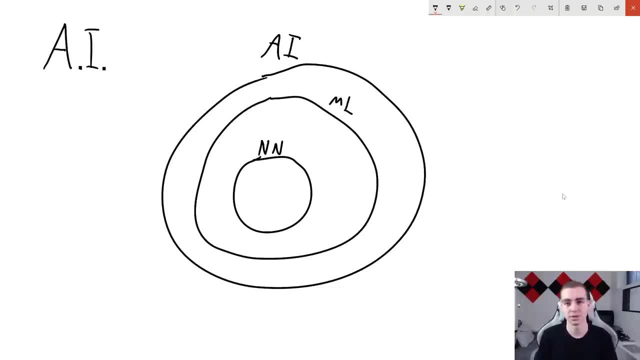 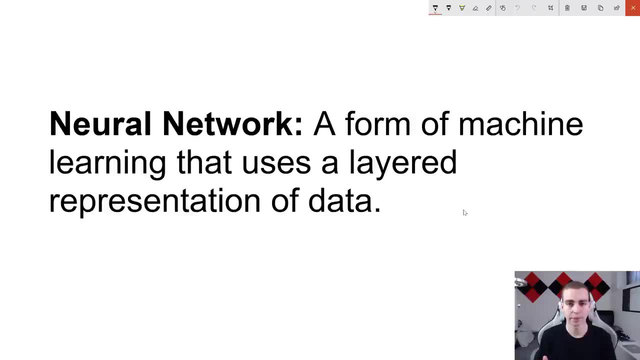 networks are cool, they're capable of a lot, But let's discuss what these really are. So the easiest way to define a neural network is: it is a form of machine learning that uses a layered representation of data. Now we're not going to really understand this completely. 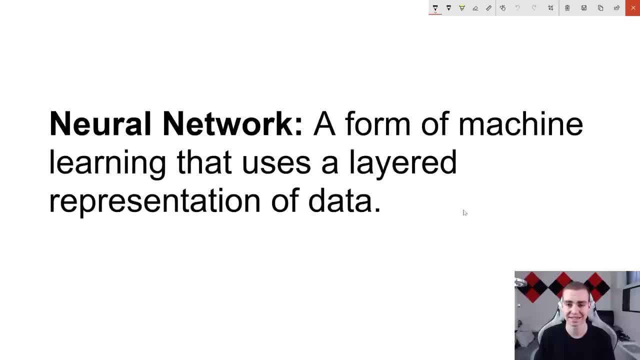 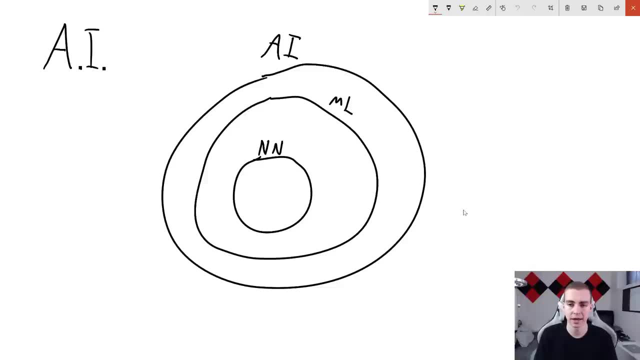 right now, But as we get further in, that should start to make more sense as a definition. But what I need to kind of illustrate to you is that in the previous example we just talked about machine learning. essentially what we had is we had 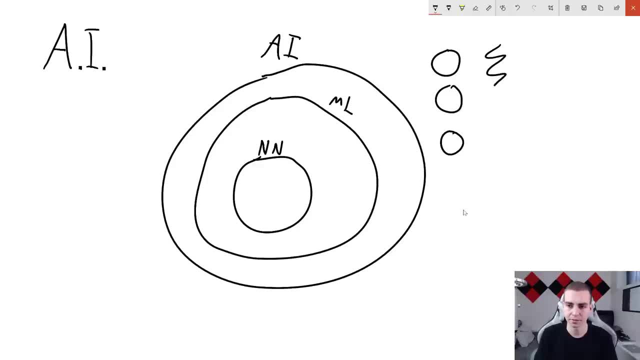 some input bubbles, which I'm going to define as these. we had some set of rules that is going to be in between here, and then we had some output, And what would happen is we feed this input to this set of rules. something happens in here, and then we get some output. 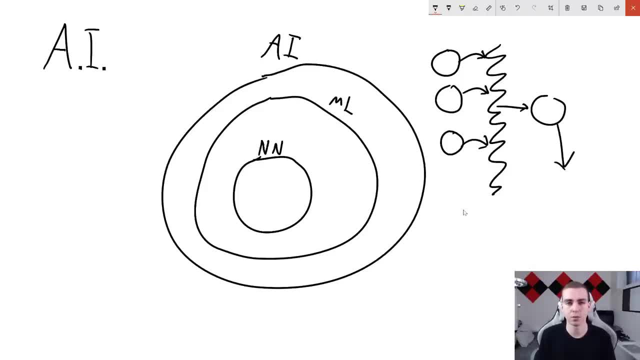 And then that is what you know, our program does. So that's what we get from the model. we pretty much just have two layers. we have kind of the input layer, the output layer, and the rules are kind of just what connects those two layers together. Now in neural. 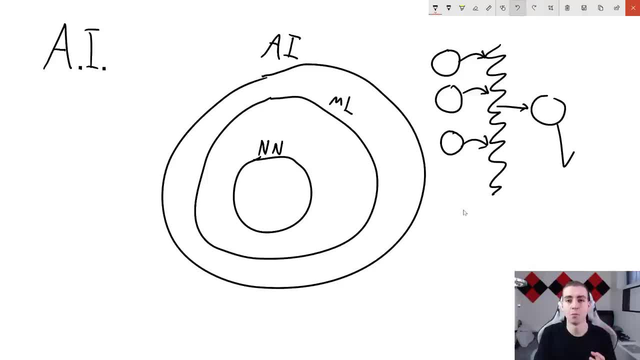 networks and what we call deep learning. we have more than two layers. Now I'm just trying to erase all this quickly so I can show you that. So let's say- and I'll draw this one another color, because why not, if we're talking about neural networks, what? 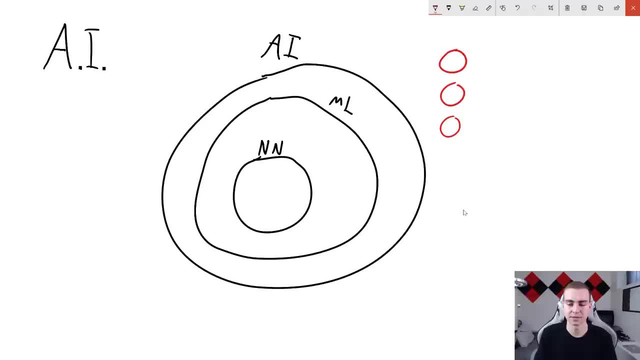 we might have- and this will vary, and I'll talk about this in a second- is the fact that we have an input layer, which will be our first layer of data. we could have some layers in between this layer that are all connected together, And then we could have some output. 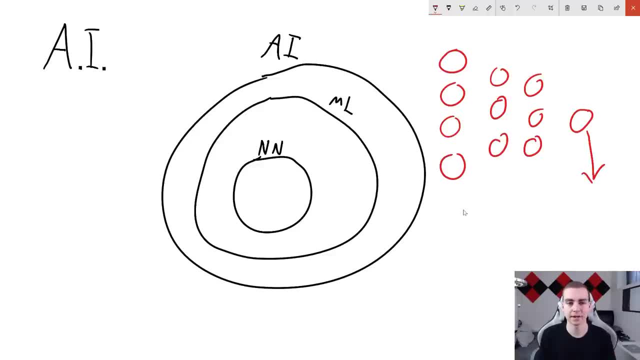 layer. So essentially what happens is our data is going to be transformed through different layers and different things are going to happen. there's gonna be different connections between these layers and then eventually we will reach an output. Now it's very difficult to explain neural networks without going completely. 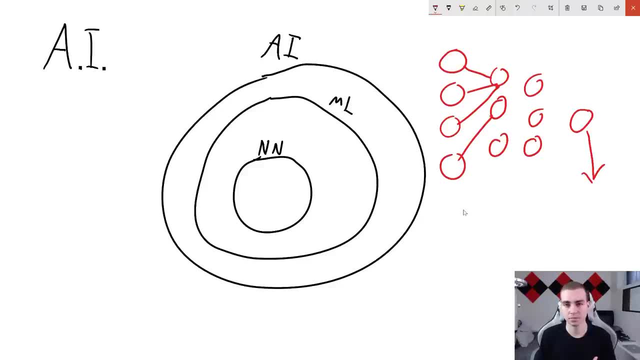 in depth, So I'll cover a few more notes that I have here. Essentially, in neural networks, we just have multiple layers- that's kind of the way to think of them- And as we see machine learning, you guys should start to understand this more. But just understand. 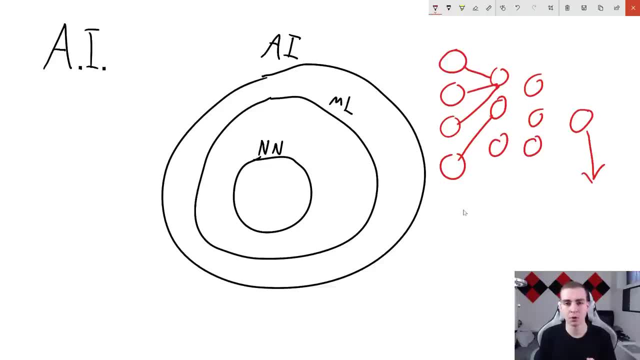 that we're dealing with multiple layers, And a lot of people actually call this a multi stage information extraction process. Now, I did not come up with that term, I think that's from a book or something. But essentially what ends up happening is we have our data at this first layer, which is that input information which 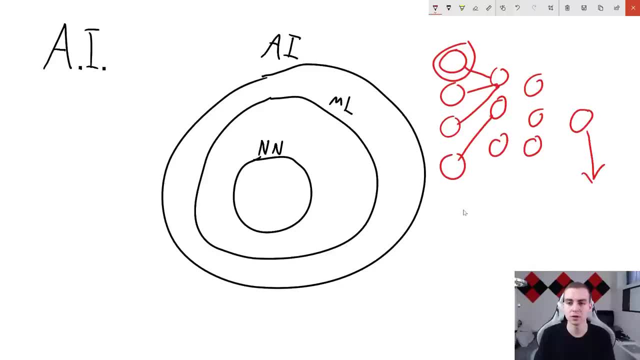 we're going to be passing to the model that we're going to do something with it, then goes to another layer where it will be transformed. it will change into something else, using a predefined kind of set of rules and weights that we'll talk about later. then it will 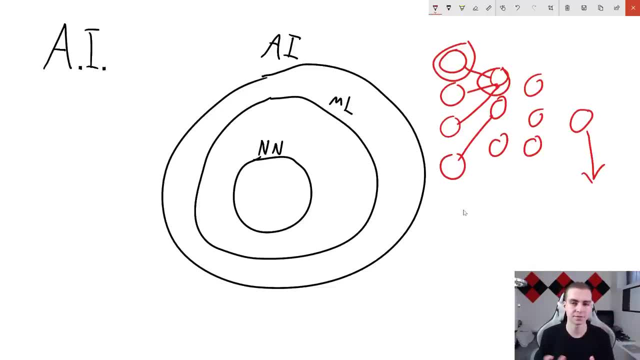 pass through all these different layers. So we're different kind of features of the data, which again we'll discuss in a second, will be extracted, will be figured out, will be found, until eventually we reach an output layer where we can kind of combine everything we've discovered about the data into some. 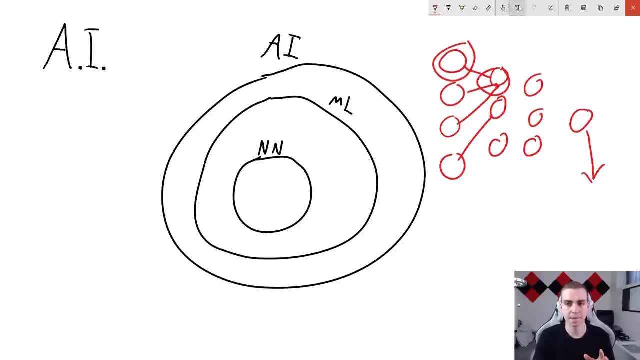 kind of output that's meaningful to our program. So that's kind of the best that I can do to explain neural networks without going on to a deeper level. I understand that a lot of you probably don't understand what they are right now, And that's. 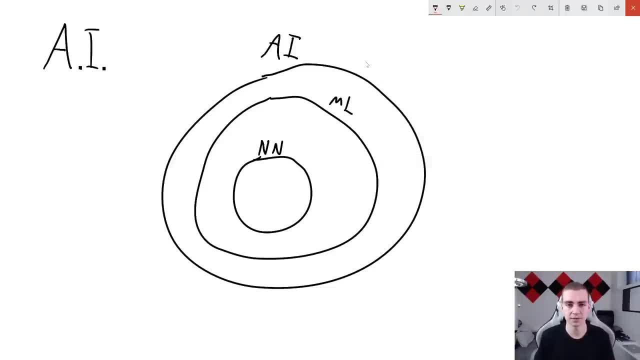 totally fine, But just know that they are layered representation of data. we have multiple layers of information, whereas in standard machine learning we only have, you know, one or two layers, And in artificial intelligence in general we don't necessarily have to have. 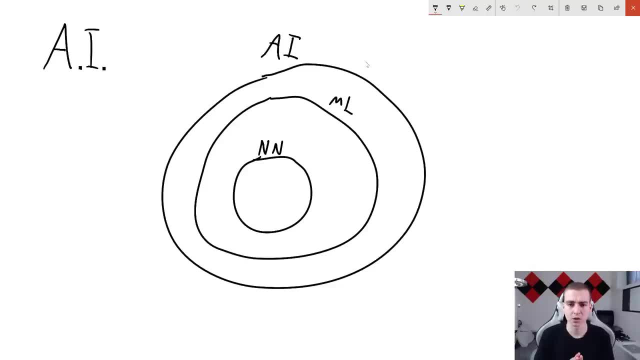 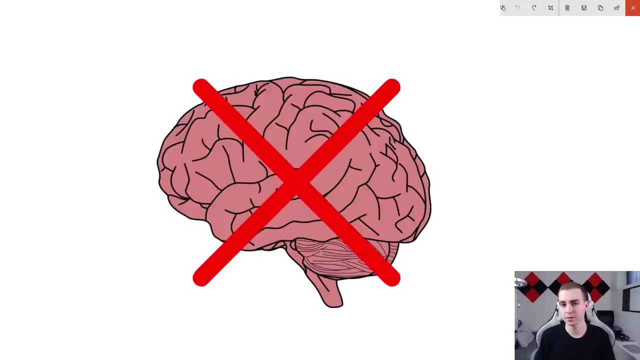 like a predefined set of layers. Okay, so that is pretty much it for neural networks is. one last thing I will say about them is that they're actually not modeled after the brain, So a lot of people seem to think that neural networks are modeled after the brain. 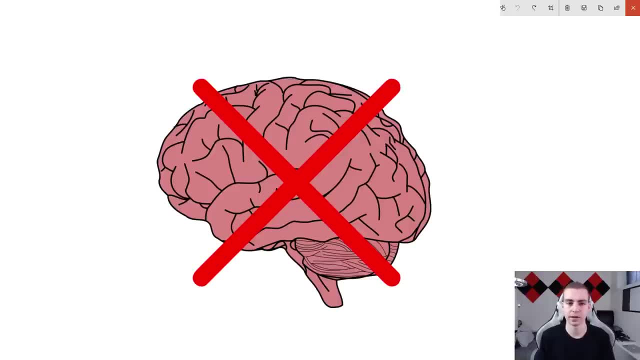 and the fact that you have neurons firing in your brain And that can relate to neural networks. Now there is a biological inspiration For the name: neural networks and the way that they work from. you know human biology but is not necessarily modeled about the way that our brain works And in fact we actually 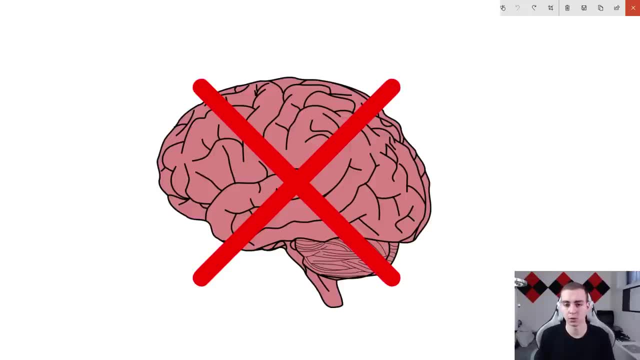 don't really know how a lot of the things in our brain operate and work. So it'd be impossible for us to say that neural networks are modeled after the brain, because we actually don't know how information is, kind of happens and occurs and transfers through our brain. 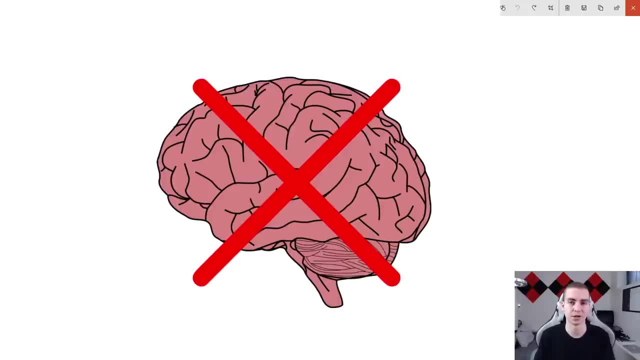 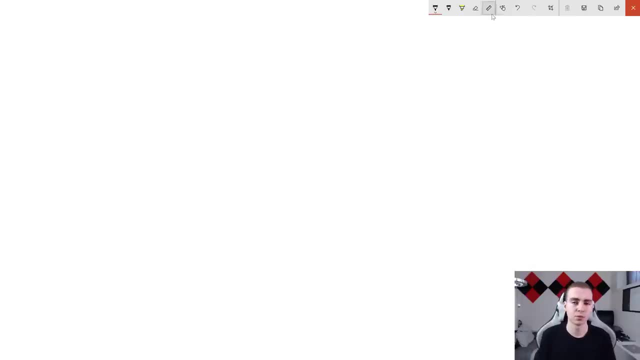 or at least we don't know enough to be able to say: this is exactly what it is: a neural network. So, anyways, that was kind of the last point there. Okay, so now we need to talk about data. Now, data is the most important part of machine learning. 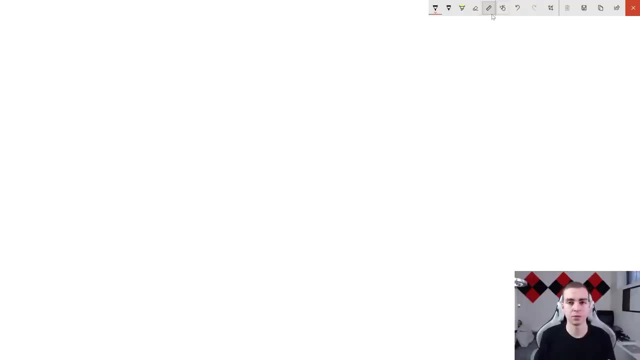 and artificial intelligence, neural networks as well, And it's very important that we understand how important data is and what the different kind of parts of it are, because they're going to be referenced a lot in any of the resources that we're using. Now what I want to do is 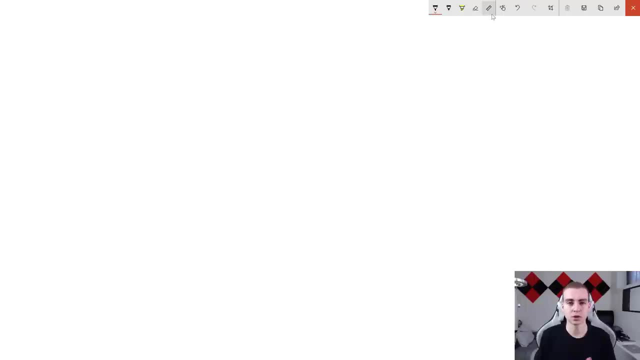 just create an example here where I'm going to make a data set that is about students final grades in like a school system. So essentially we're going to make this a very easy example where all we're going to have for this data set 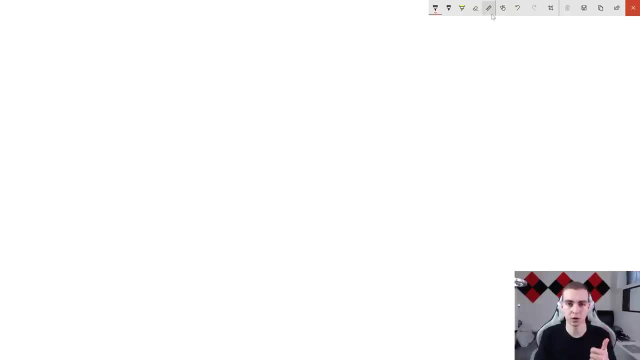 is. we're going to have information about students, So we're going to have their midterm one grade, their midterm two grade and then we're going to have their final grade. So I'm just going to say mid term one and again. excuse my handwriting here, it's not the easiest. 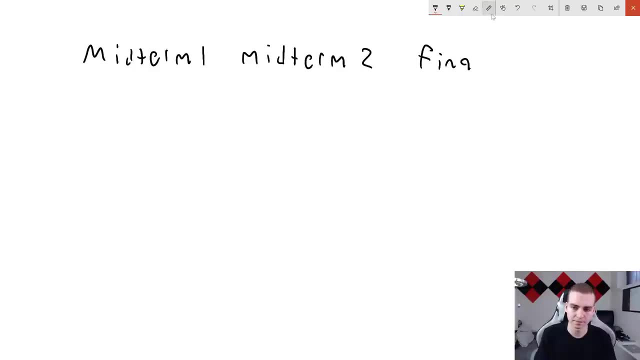 thing to write with this drawing tablet And then I'll just do final. So this is going to be our data set And we'll actually see some similar data sets to this as we go through and do some examples later on. So for student one, which we'll just put, some students here: 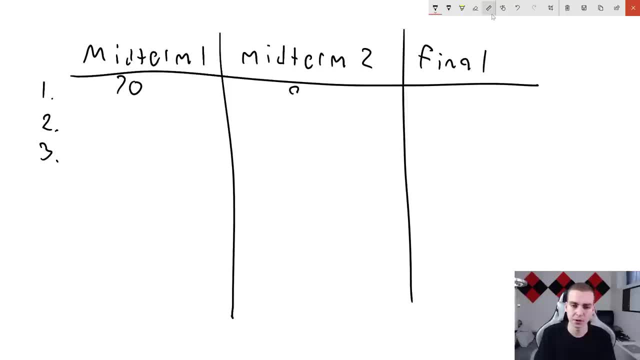 we're going to have their midterm one grade, maybe that's a 70,. their midterm two grade, maybe that was an 80. And then let's say their final was like their final term grade, not just the mark on the final exam. Let's give them a 77.. Now for midterm one, we can give someone a 60,. 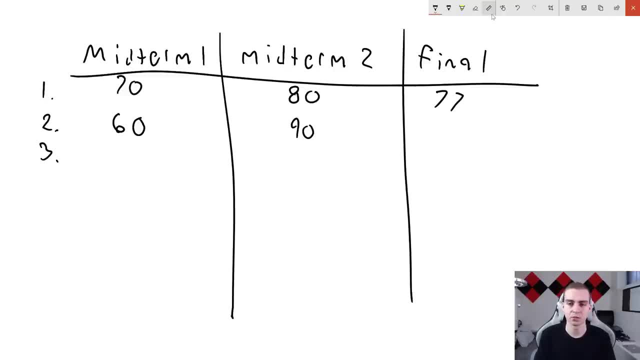 maybe we give them a 90. And then we determined that the final grade on their exam was, let's say, an 84. And then we can do something with maybe a lower grade here, So 4050. And then maybe they got a 38 or something in the final grade. 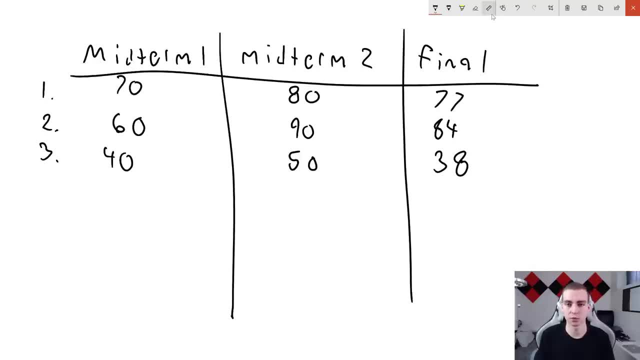 Now, obviously we could have some other information here that we're omitting, Like maybe there was some exams, some assignments, whatever some other things they did that contributed to their grade. But the problem that I want to consider here is the fact that, given our 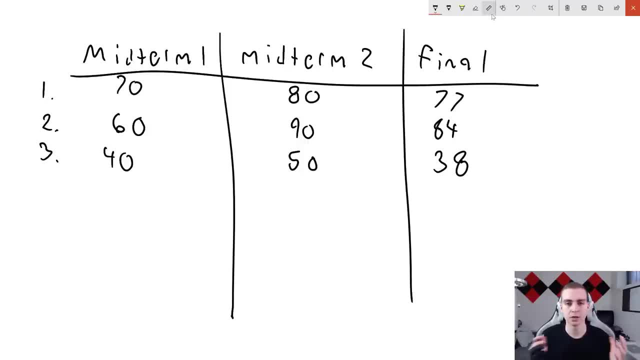 midterm one grade and our midterm two grade and our final grade. how can I use this information to predict any one of these three columns? So if I were given a student's midterm one grade and I were given a student's final grade, how could I predict their midterm two? 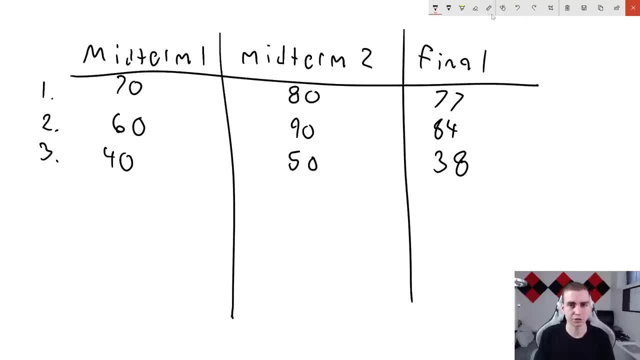 grade relates to midterm one grade. So this is where we're going to talk about the wahrscheinlich. now, obviously, we could have some other information here that we're omitting, like maybe there about features and labels. Now, whatever information we have, that is the input information, which 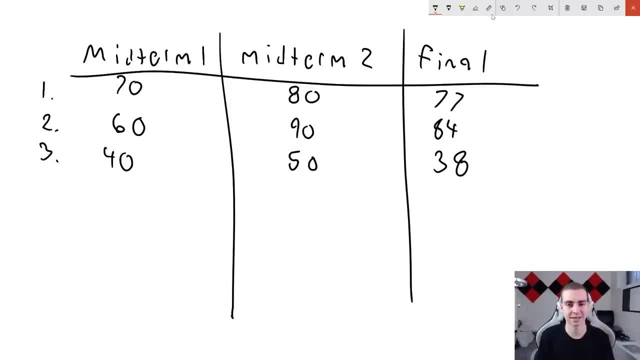 is the information we will always have that we need to give to the model to get some output is what we call our features. So in the example where we're trying to predict midterm two, and let's just do this and highlight this in red so we understand what we would have- 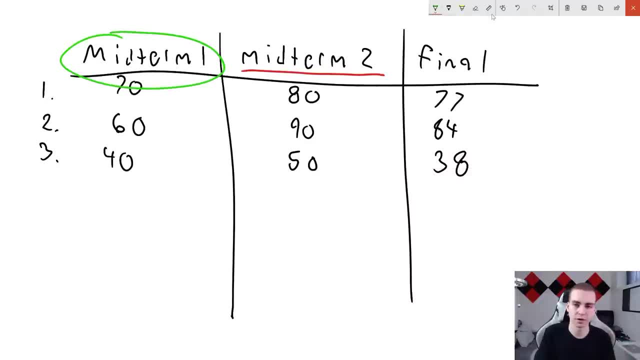 as our features, our input information are going to be midterm one and final, because this is the information we are going to use to predict something. it is the input, it is what we need to give the model And if we're training a model to look at midterm. 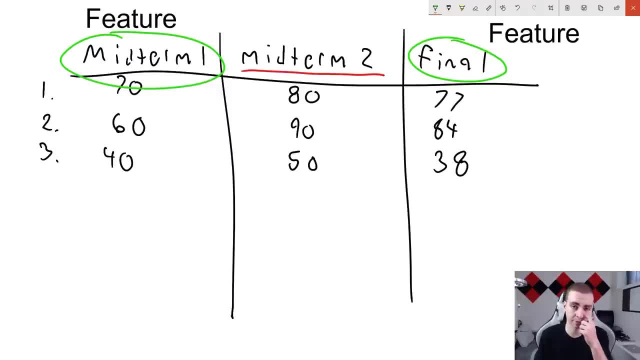 one and final grade. whenever we want to make a new prediction, we need to have that information to do so. Now, what's highlighted in red. so this midterm two. here is what we would call the label, or the output. Now, the label is simply what we are trying to look for or predict. 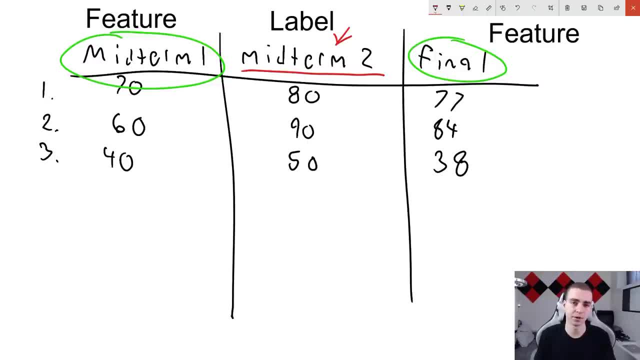 So when we talk about features versus labels, features is our input information, the information that we have that we need to use to make a prediction, And our label is that output information. that is just representing you know what we're looking for. So, when we feed our features to a model, 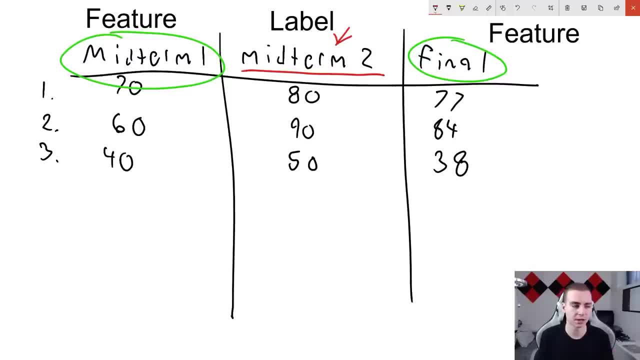 it will give to us a label, And that is kind of the point that we need to understand. So that was the basic here, And now I'm just going to talk a little bit more about data- because we will get into this more as we continue going- and about the importance of it. So the 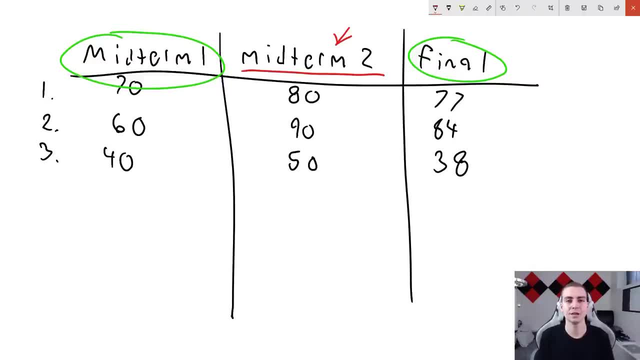 reason why data is so important, as this is kind of the key thing that we use to create models. So whenever we're doing AI and machine learning, we need data pretty much, unless you're doing a very specific type of machine learning and artificial intelligence, which we'll talk about later. Now for most, 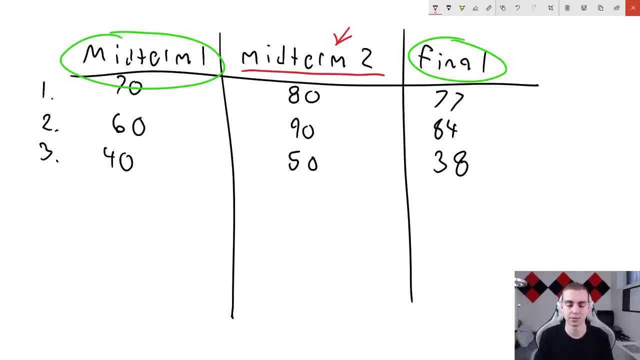 of these models. we need tons of different data, we need tons of different examples, And that's because we know how machine learning works now, which is essentially we're trying to come up with rules for a data set. we have some input information. we have some output. 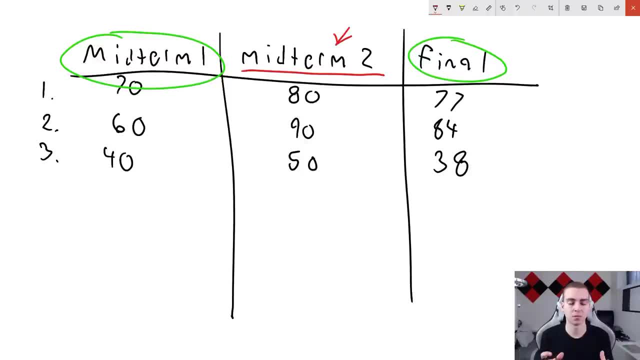 information or some features and some labels. we can give that to a model and tell it to start training, And what it will do is come up with rules such that we can just give some features to the model in the future, And then it should be able to give us a pretty good. 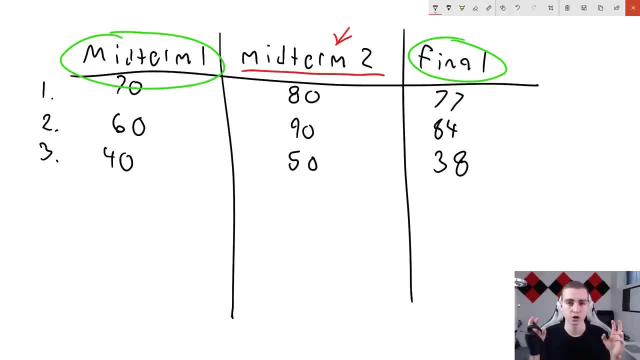 estimate of what the output should be. So when we're training, we have a set of training data And that is data where we have all of the features and all of the labels. So we have all of this information. Then, when we're going to test the model or use the model later, 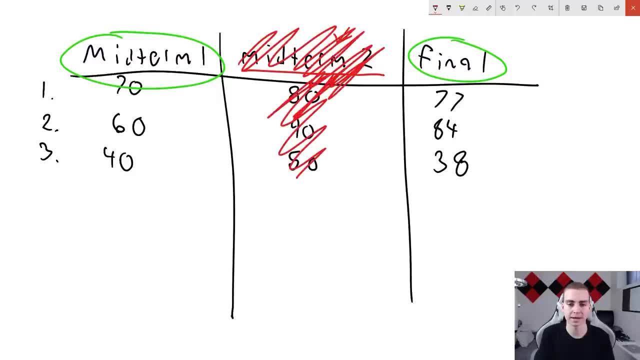 on. we would not have this midterm to information, we wouldn't pass this to the model, we would just pass our features, which is midterm one and final, and then we would get the output of midterm two. So I hope that makes sense. That just means data is extremely important. 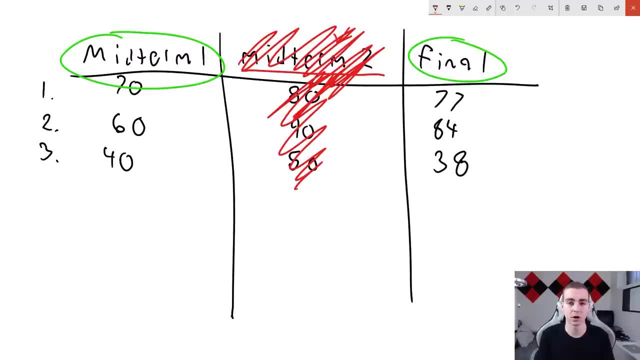 If we're feeding incorrect data or data that we shouldn't be using to the model, that could definitely result in a lot of mistakes. And if we have incorrect output information or incorrect input information, that is going to cause a lot of mistakes as well, Because that is. 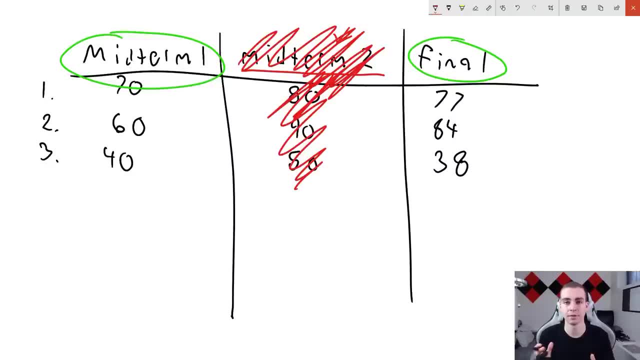 essentially what the model is using to learn and to kind of develop and figure out what it's going to do with new input information. So, anyways, that is enough of data. Now let's talk about the different types of machine learning. Okay, so, now that we've discussed, 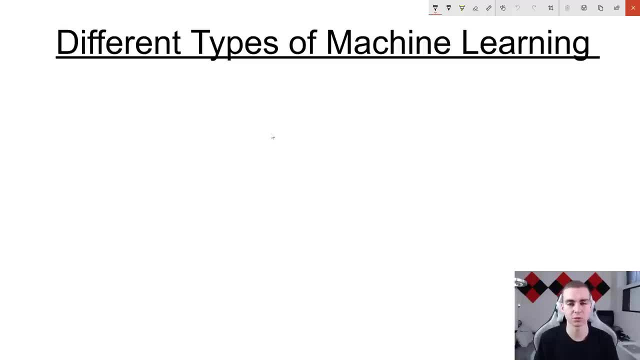 the difference between artificial intelligence, machine learning and neural networks. we have a kind of decent idea about what data is and the difference between features and labels. It's time to talk about the different types of machine learning, specifically, which are: unsupervised learning, supervised learning. 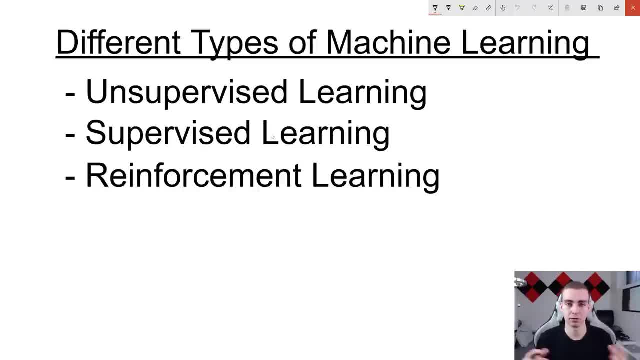 and reinforcement learning. Now, these are just the different types of learning, the different types of figuring things out. Now, different kinds of algorithms fit into these different categories, from within artificial intelligence, within machine learning and within neural networks. So the first one we're going to talk about is supervised learning, which is 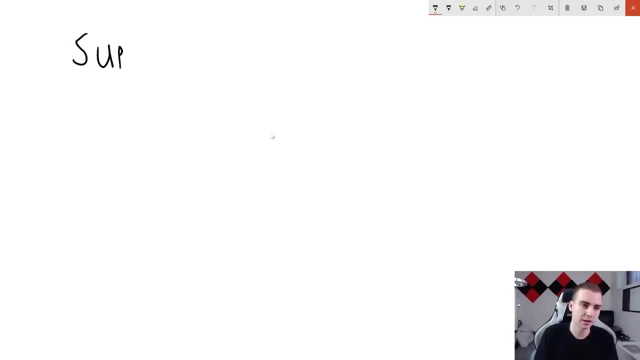 kind of what we've already discussed, So I'll just write supervised up here Again. excuse the handwriting. So supervised learning. Now, what is this? Well, supervised learning is kind of everything we've already learned, which is we have some features. So we'll write our features like this: right, we have some. 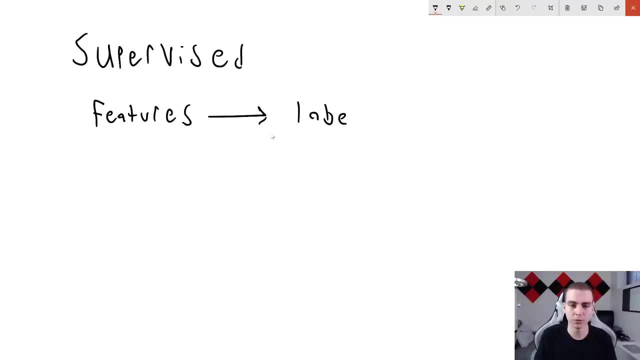 features And those features correspond to some label or potentially labels. sometimes we might predict more than one information. So when we have this information, we have the features and we have the labels. what we do is we pass this information And we pass this information to some machine learning model. it figures out the rules for us And 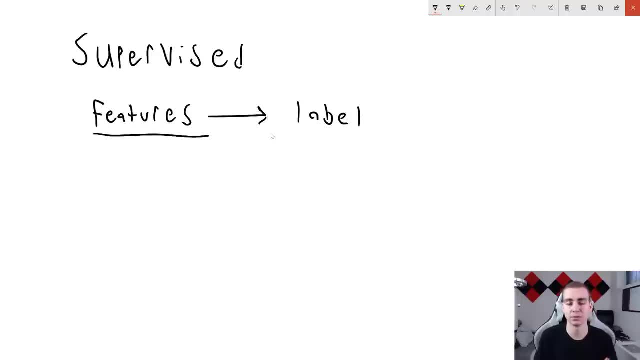 then later on, all we need is the features and it will give us some labels using those rules. But essentially, what supervised learning is is when we have both of this information. The reason it's called supervised is because what ends up happening when we train our machine? 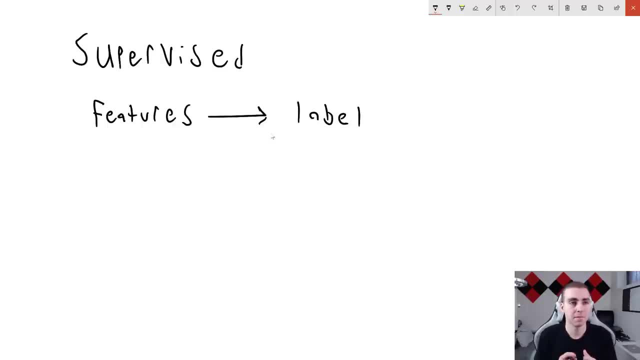 learning model is. we pass the input information, it makes some arbitrary prediction using the rules that already knows, and then it compares that prediction that it made to what the actual prediction is, which is this label. So we supervise the model and we say, Okay, so you predicted that the color was red, but 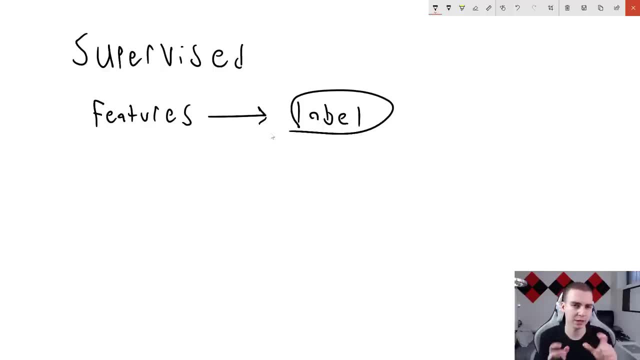 really the color of whatever we passed in should have been blue. So we need to tweak you just a little bit so that you get a little bit better and you move in the correct direction, And that's kind of the way that this works. For example, say, we're predicting, you know? 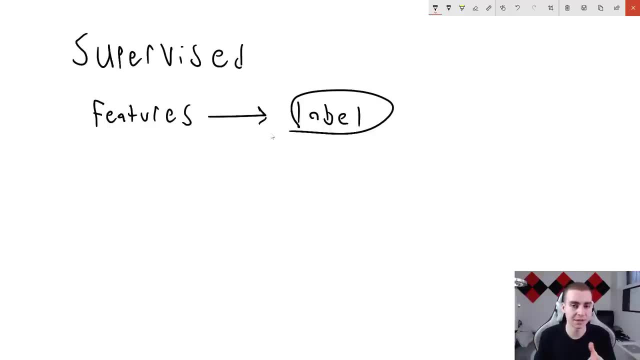 students final grade. well, if we predict that the final grade is 76, but the actual grade is 77,, we were pretty close but we're not quite there. So we supervise the model and we say, Hey, we're going to tweak you just a little bit, move you in the correct. 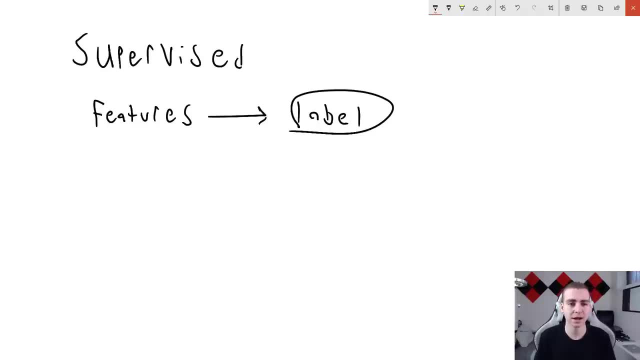 direction and hopefully we get you to 77. And that is kind of the way to explain this. right, you have the features, you have the labels. when you pass the features, the model has some rules that it's already built. it makes a prediction and then it compares that. 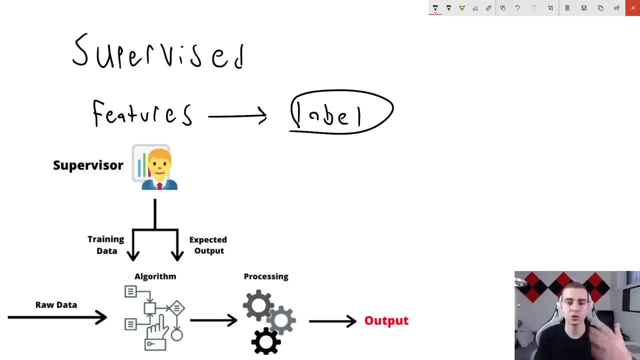 prediction to the label and then retweaks the model and continues doing this with 1000s upon 1000s upon 1000s of pieces of data until eventually it gets so good that we can stop training it. And that is what supervised learning is. it's the most common type of learning. 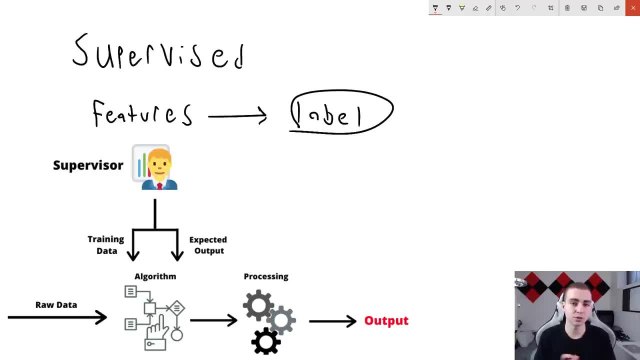 it's definitely the most applicable, And a lot of instances and most machine learning algorithms that are actually used use a form of supervised machine learning. a lot of people seem to think that this is, you know, a less complicated, less advanced way of doing things. That is definitely not true. all of the different 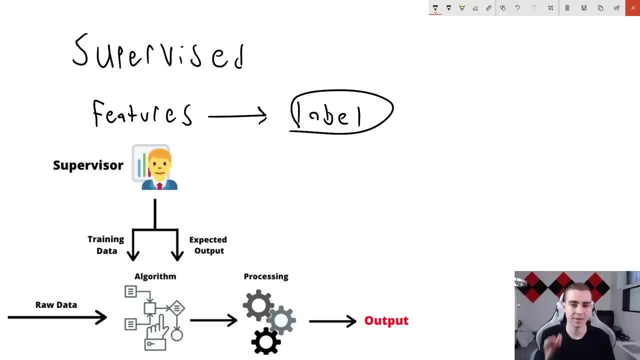 methods I'm going to tell you have different advantages and disadvantages. And this has a massive advantage when you have a ton of information and you have the output of that information as well. But sometimes we don't have the luxury of doing that, And that's. 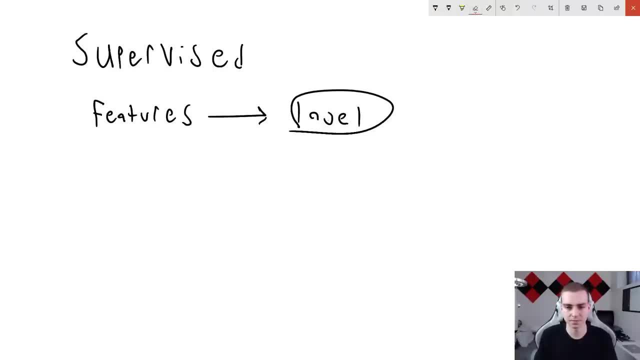 where we talk about unsupervised learning. So hopefully that made sense And I hope that made sense For supervised learning. tried my best to explain that And now let's go into- or sorry for- supervised learning, Now let's go into unsupervised learning. So 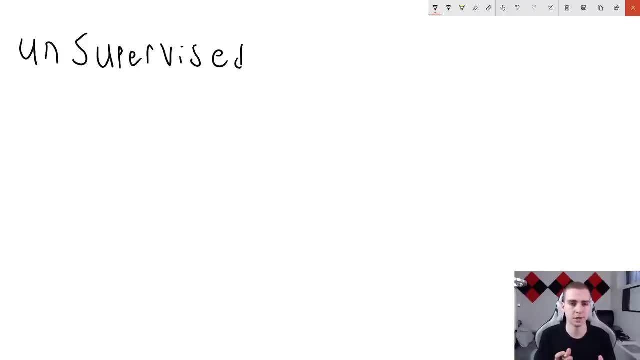 if we know the definition of supervised learning, we should hopefully be able to come up with a definition of unsupervised learning, which is when we only have features. So if given a bunch of features like this and absolutely no labels, no output for these features, what? 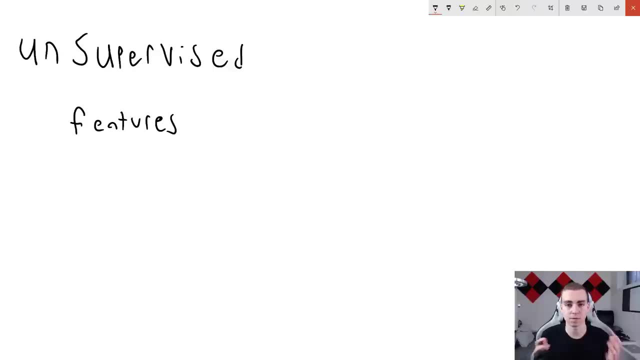 we want to do is have the model come up with those labels For us. Now this is kind of weird. you're kind of like, wait, how does that work? Why would we even want to do that? Well, let's take this for an example. we have some axis. 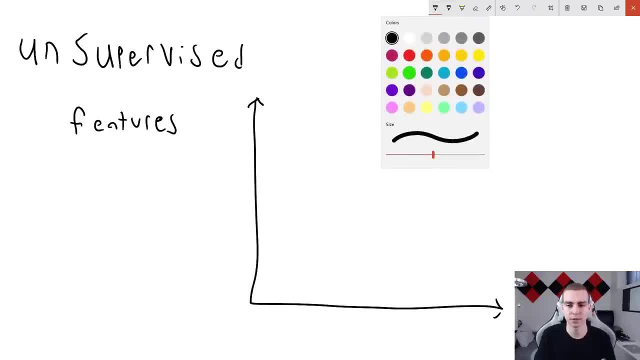 some axes of data, okay, And we have like a two dimensional data point. So I'm just going to call this: let's say x and let's say y, okay, And I'm going to just put a bunch of dots on the screen. that kind of represents like maybe a scatterplot of some of our different 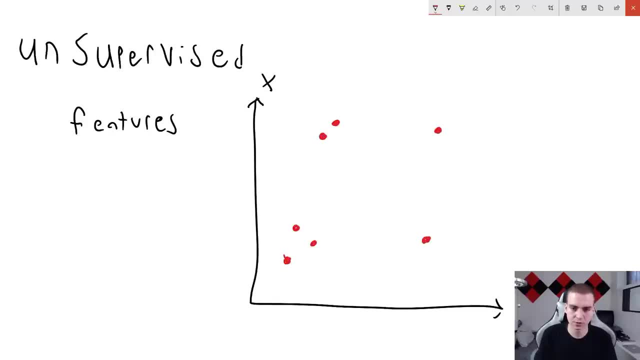 data, And I'm just going to put some dots specifically closer to other ones. just, you guys kind of get the point of what we're trying to do Here, So let's do that. Okay, so let's say: I have this data set, this here is what we're. 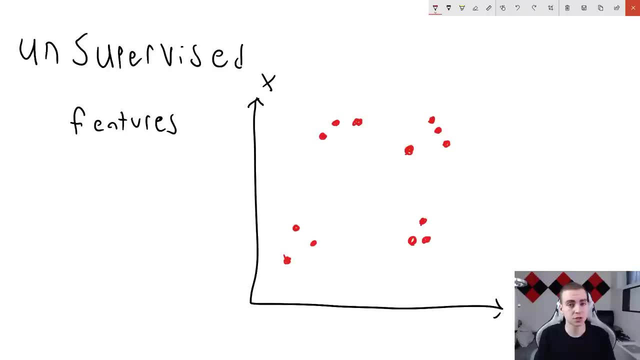 working with And we have these features. the features in this instance are going to be x and y. right, so x and y are my features. Now, we don't have any output specifically for these data points. What we actually want to do is we want to create some kind of model. 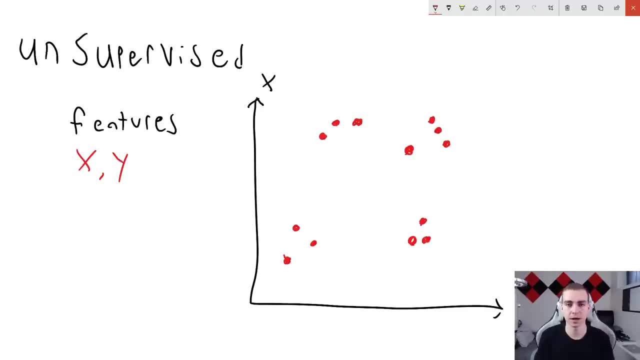 that can cluster these data points, which means figure out kind of you know, unique groups of data and say, Okay, so you're in group one, you're in group two, you're in group three and you're in group four. we may not necessarily. 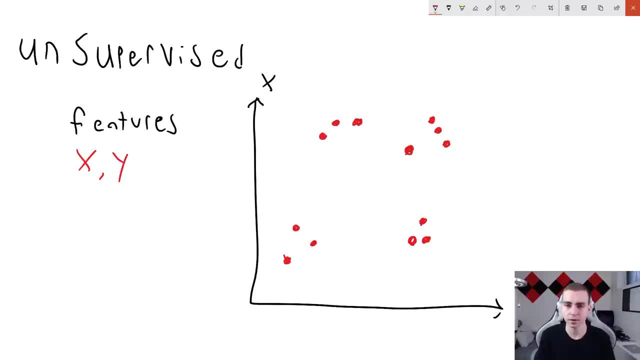 know how many groups we have, although sometimes we do. what we want to do is just group them and kind of say, Okay, we want to figure out which ones are similar and we want to combine those together. So hopefully, what we would do with an unsupervised machine learning model- 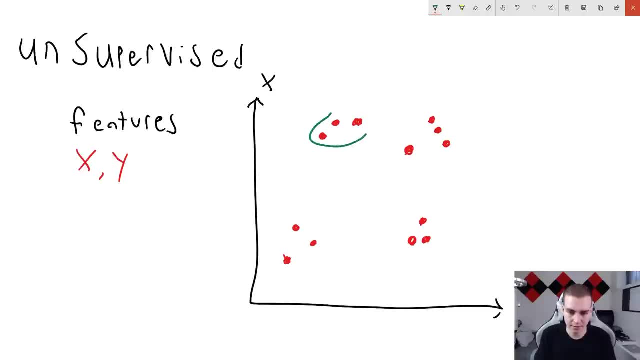 is: pass all of these features and then have the model create kind of these groupings, So like maybe this is a group, maybe this is a group, maybe this is a group if we were having four groupings And maybe if we had two groupings, we might get groupings that look something like this: 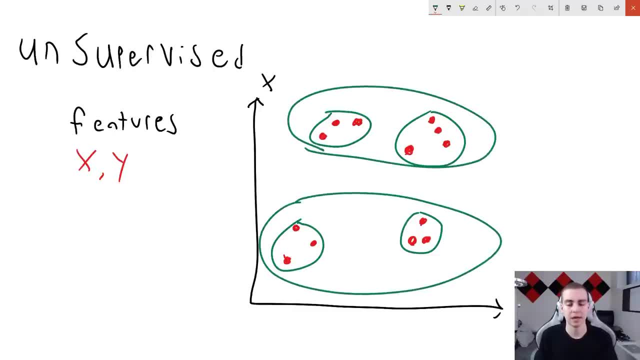 right And then when we pass a new data point in that could, we could figure out what group that was a part of by determining, you know, which one it is closer to. Now this is kind of a rough example. it's hard to again explain all of these without going very in depth into. 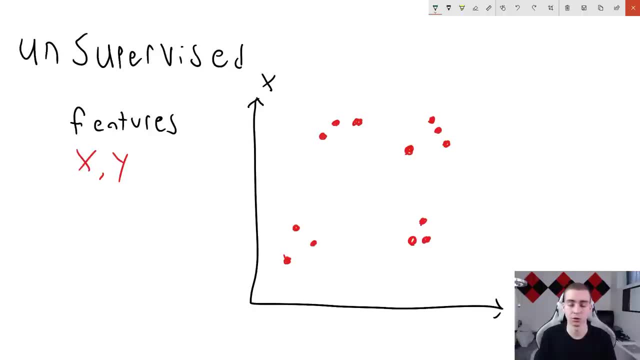 the specific algorithms, But unsupervised machine learning or just learning in general, is when you don't have some output information. you actually want the model to figure out the output for you And you don't really care how it gets there, you just want it to get there. And again, a good example is clustering. 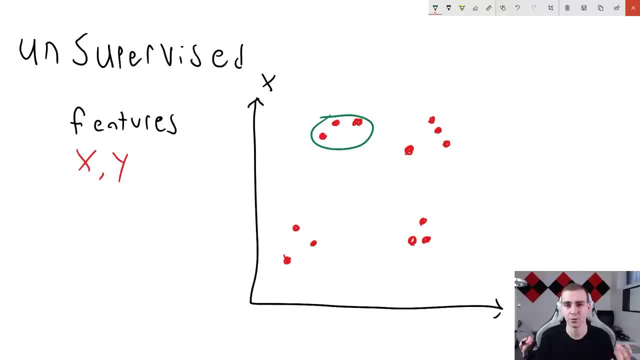 data points And we'll talk about some specific applications of when we might even want to use that later on. just understand: you have the features, you don't have the labels, and you get the unsupervised model to kind of figure it out for you. Okay, so now our last. 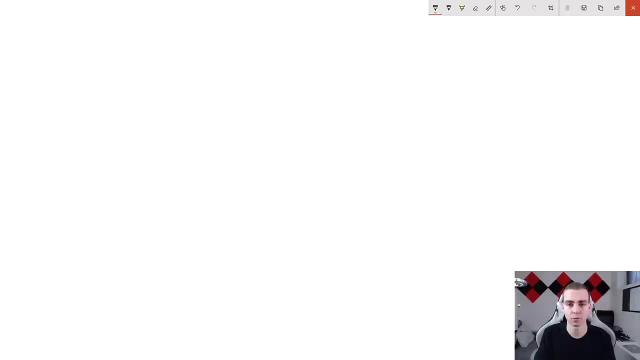 type, which is very different than the two types I just explained, is called reinforcement learning. Now, personally, reinforcement learning- and I don't even know if I want to spell this, because I feel like I'm going to mess it up- Reinforcement learning is the coolest type of machine learning in my opinion, And this 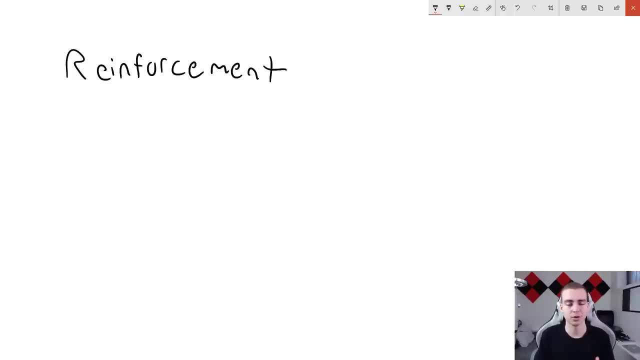 is when you actually don't have any data. you have what you call an agent, an environment and a reward, And I'm going to explain this very briefly with a very, very, very simple example, because it's hard to get too far. So let's say we have a very basic game. you 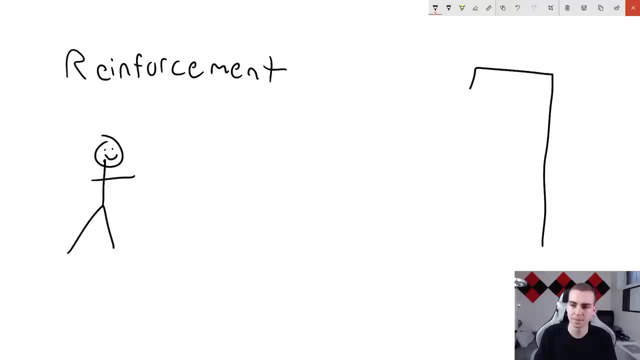 know, maybe we made this game ourselves And essentially, the objective of the game is to get to the flag. Okay, that's all it is. we have some ground, you can move left or right. Get to this flag. Well, we want to train some artificial intelligence, some machine learning. 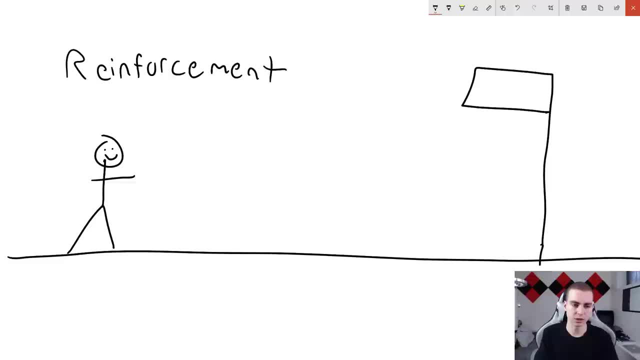 model that can figure out how to do this. So what we do is we call this our agent, we call this entire thing, So this whole thing here, the environment, so I guess I could write that here, So, and by meant think I spelt that correctly. And then we have something. 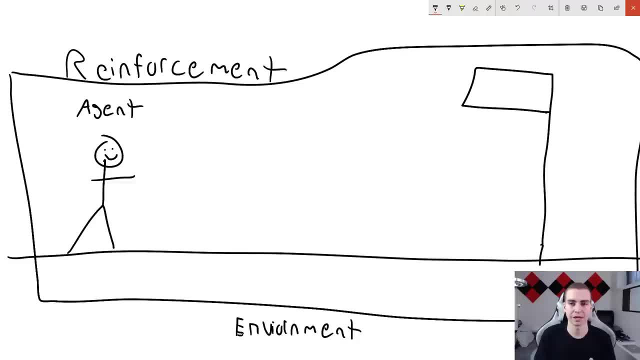 called a reward, And a reward is essentially what the agent gets when it does something correctly. So let's say the agent takes one step over this way. So let's say his new position is here. I just want to keep drawing him, So I'm gonna use a dot. Well, he got closer to. 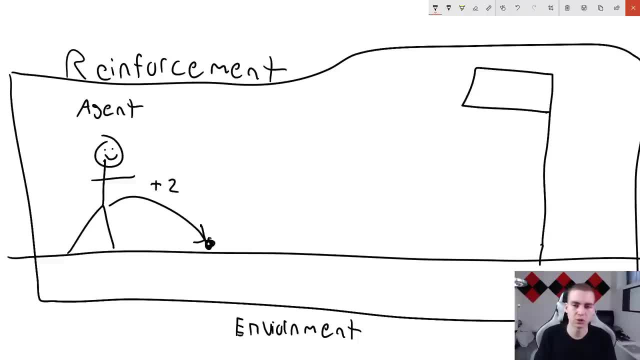 the flag. So what I'm actually going to do is give him a plus two reward. So let's say he moves again closer to the flag. Maybe I give him now plus one. this time he got even closer, And as he gets closer I give him more and more reward. Now what happens if? 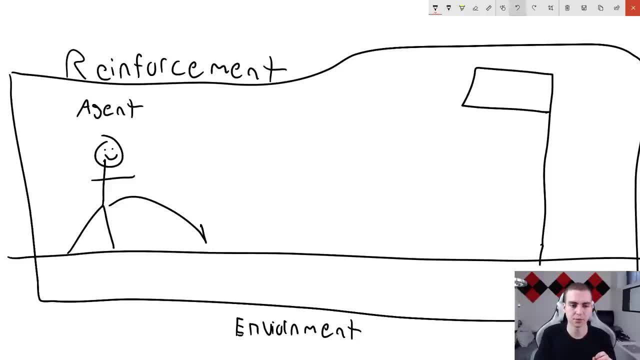 he moves backwards. So let's erase this And let's say that at some point in time, rather than moving close to the threat, the flag, he moves backwards. well, he might get a negative reward. Now, essentially, what the objective of this agent is to do is to maximize its reward. So if 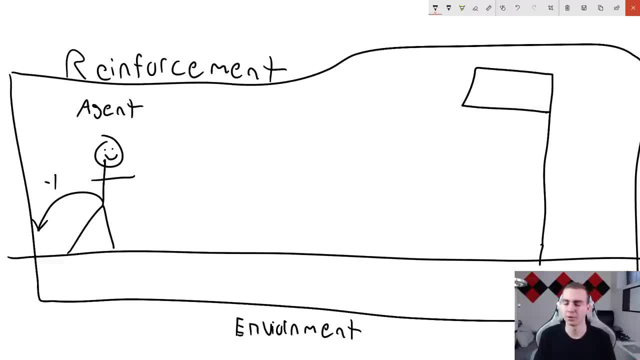 you give it a negative reward for moving backwards. it's going to remember that and it's going to say: okay, at this position here, where I was standing, when I moved backwards, I got a negative reward. So if I get to this position again, I don't want to go backwards anymore. 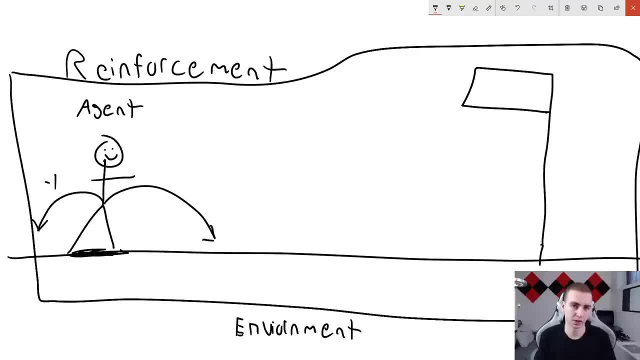 I want to go forwards because that should give me a positive reward, And the whole point of this is we have this agent that starts off with absolutely no idea, no kind of you know knowledge of the environment, And what it does is it starts exploring And it's a. 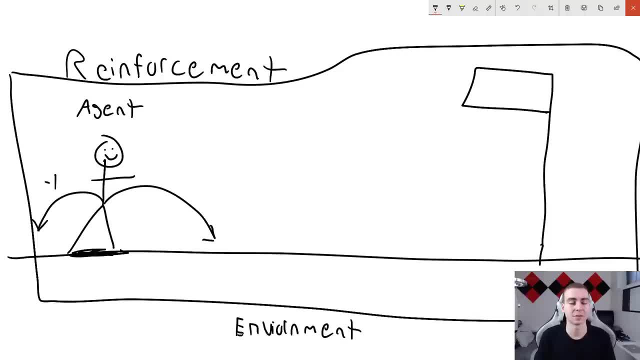 mixture of randomly exploring and exploring using kind of some of the things that's figured out so far to try to maximize its reward. So eventually, when the agent gets to the flag it will have the most, the highest possible reward that it can have. 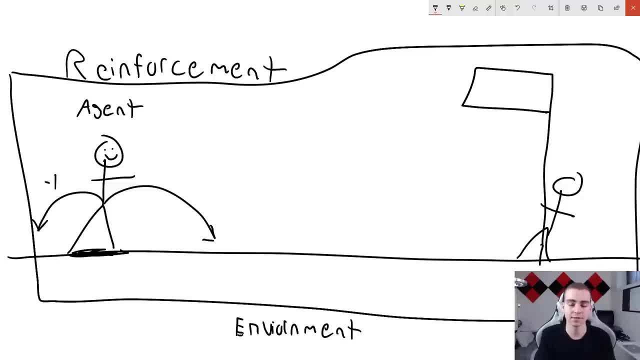 And then next time that we plug this agent into the environment, it will know how to get to the flag immediately, because it's kind of figured that out. It's determined that in all these different positions, if I move here, this is the best place to move. 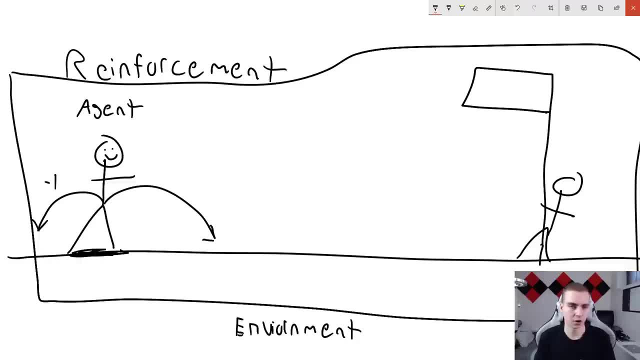 So, if I get in this position, move there. Now this is again hard to explain without more detailed examples and going more mathematically and all that, But essentially just understand. we have the agent, which is kind of what the thing is that's moving around in our environment. 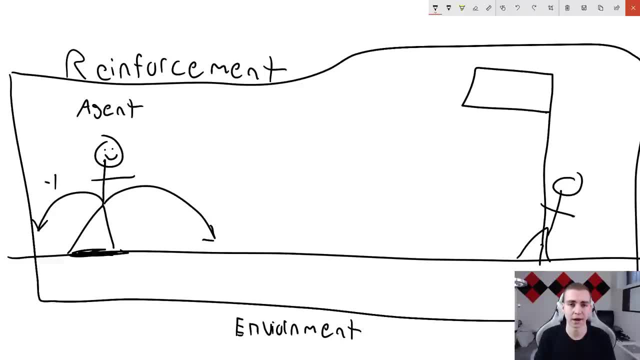 we have this environment, which, which is just what the agent is moving around in our environment. The agent can move around in, and then we have a reward, And the reward is what we need to figure out as the programmer: a way to reward the agent correctly so that it gets. 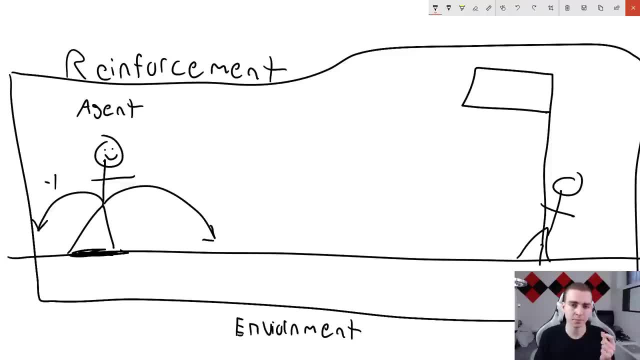 to the objective in the best possible way. But the agent simply maximizes that reward. So it just figures out where I need to go to maximize that reward. It starts at the beginning kind of randomly exploring the environment because it doesn't know any of. 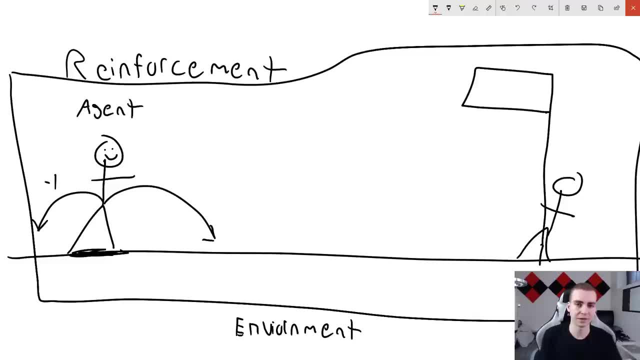 the rewards it gets at any of the positions, And then, as it explores some more different areas, it kind of figures out the rules and the way that the environment works, And then then we'll determine how to reach the objective, which is, whatever it is, that it is, This is: 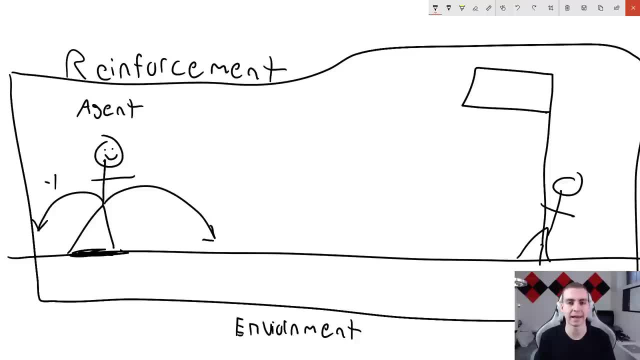 a very simple example. you could train a reinforcement model to do this And you know like half a second right. But there is way more advanced examples And there's been examples of reinforcement learning, like of AI is pretty much figuring out how to play games together, how to it's. 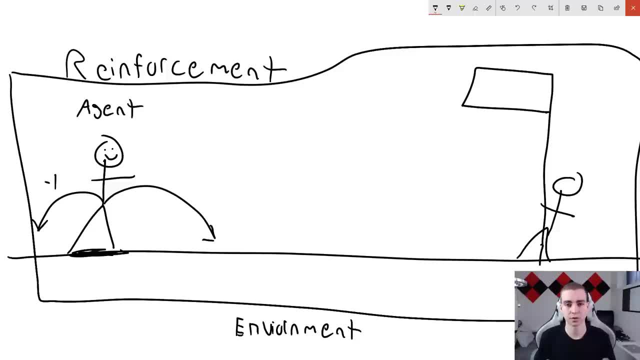 it's actually pretty cool some of the stuff that reinforcement learning is doing, And it's a really awesome kind of advancement in the field because it means we don't need all this data anymore. we can just get this to kind of figure out how to do things for. 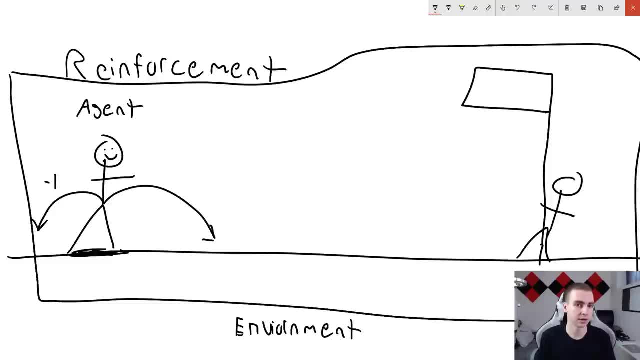 us and explore the environment And learn on its own. Now, this can take a really long time. this can take a very short amount of time. really depends on the environment. But a real application of this is training. AI is to play games, as you might be able to tell by kind of what I was explaining here. 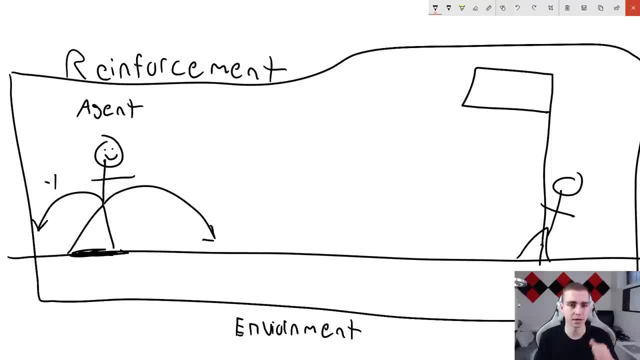 And yeah, so that's kind of the fundamental differences between supervised, unsupervised and reinforcement learning. we're going to cover all three of these topics throughout this course And it's really interesting to see some of the applications we can actually do with this. So, with that being said, I'm going to kind of end what I'm going to call. 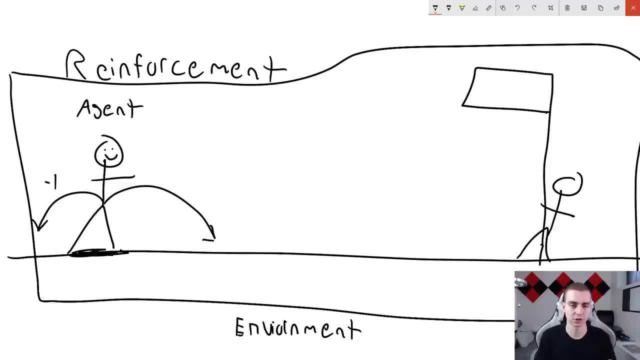 module one, which is just a general overview of the different topics, some definitions and getting a fundamental knowledge. And in the next one, what we're going to be talking about is what TensorFlow is. we're going to get into coding a little bit And we're going to discuss some different aspects of TensorFlow. 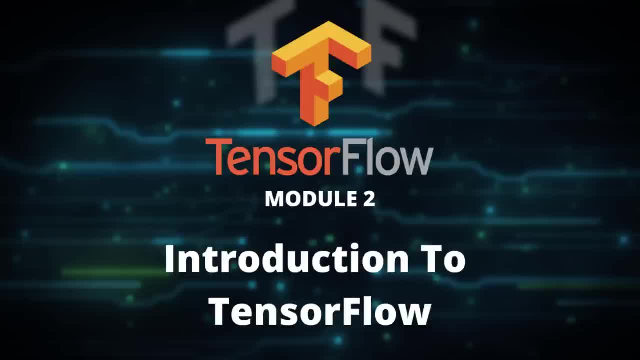 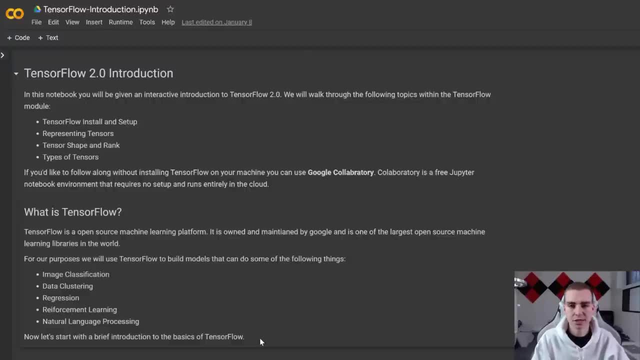 and things we need to know to be able to move forward and do some more advanced things. So now, in module two of this course, what we're going to be doing is getting a general introduction to TensorFlow, understanding what a tensor is, understanding shapes, and. 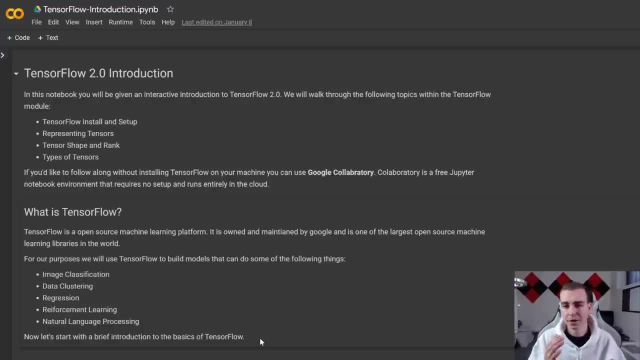 data representation and then how TensorFlow actually works on a bit of a lower level. This is very important because you can definitely go through and learn how to do machine learning without kind of gaining this information and knowledge. But it makes it a lot more difficult to tweak your models and really understand. 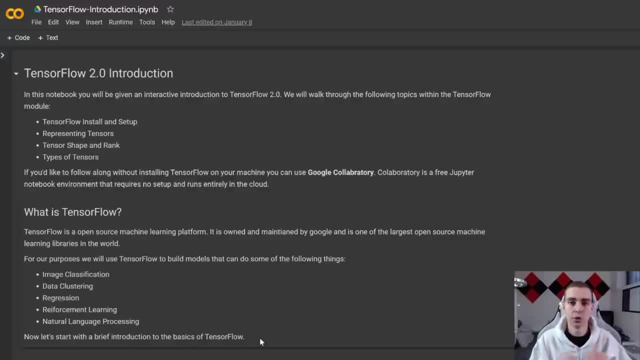 what's going on If you don't. you don't have that fundamental, lower level knowledge of how TensorFlow actually works and operates. So that's exactly what we're going to cover here. Now, for those of you that don't know what TensorFlow is, essentially, this is an 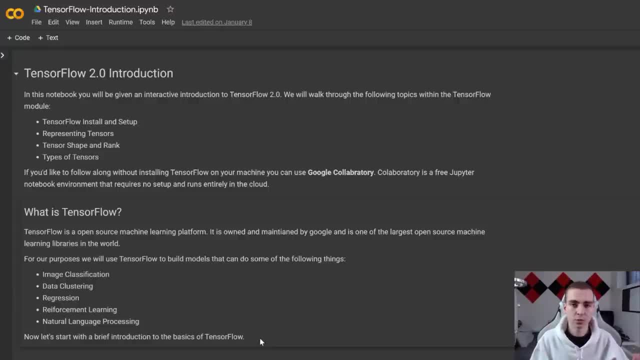 open source machine learning library. it's one of the largest ones in the world, it's one of the most well known and it's maintained and supported by Google. Now, TensorFlow essentially allows us to do and create machine learning models and neural networks, and all of that without 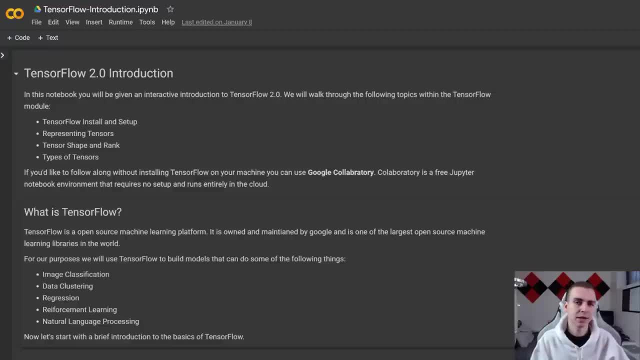 having to have a very complex math background. Now, as we get further in and we start discussing more in detail how neural networks work and machine learning algorithms actually function, you'll realize there's a lot of math that goes into this. Now it starts off being very 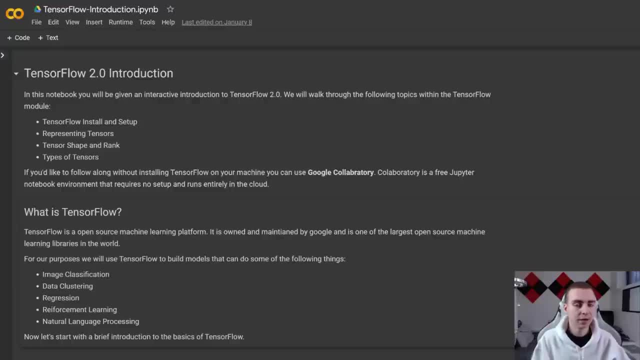 kind of fundamental like basic calculus and basic linear algebra, And then it gets much more advanced into things like gradient descent and some more regression techniques and classification And essentially you know, a lot of us don't know that. And we don't really need to know that So long as we have a basic understanding. 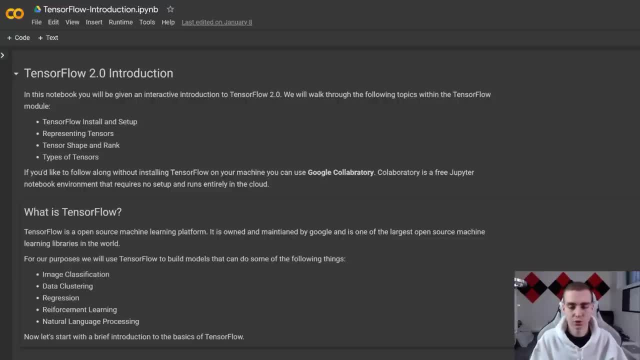 of it. then we can use the tools that TensorFlow provides for us to create models, And that's exactly what TensorFlow does Now. what I'm in right now is what I call Google Collaboratory. I'm going to talk about this more in depth in a second, But what I've done for this whole? 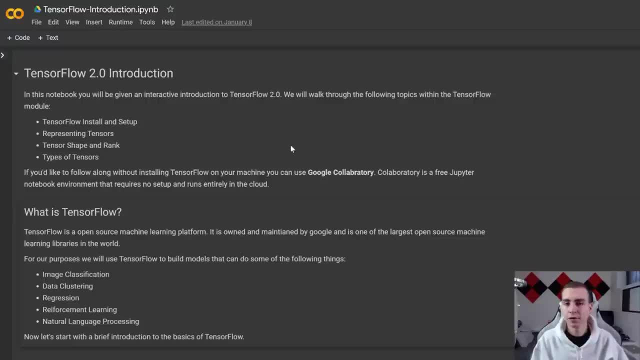 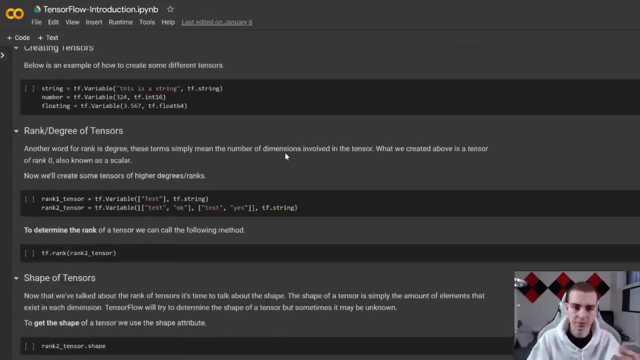 course is, I've transcribed very detailed everything that I'm going to be covering through each module. So this is kind of the transcription of module one, which is the introduction to TensorFlow. you can see it's not crazy long, but I wanted to do this so that any of you can follow along. 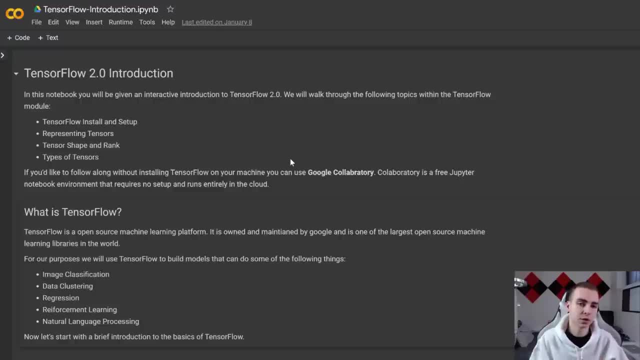 with kind of the text base and kind of my lecture notes. I almost want to call them as I go through the different content. So in the description there will be links to all of these different notebooks. This is in something called Google Collaboratory. 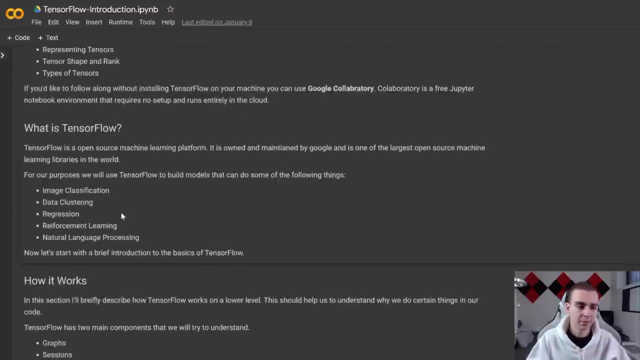 which, again, we're going to discuss in a second. But you can see here that I have a bunch of text and then it gets down to some different coding aspects, And what I'm going to be doing to make sure that I stay on track is simply: 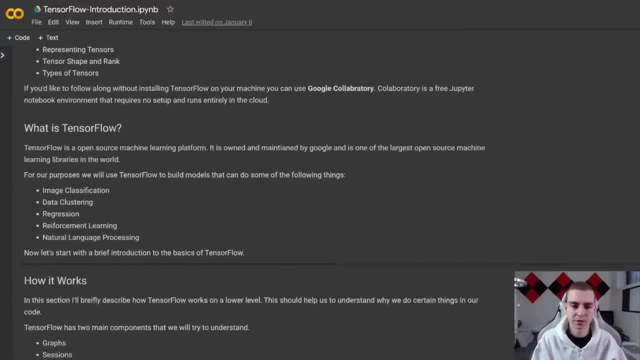 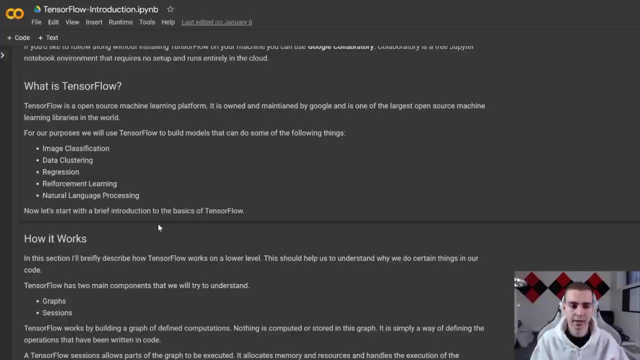 following along through this, I might deviate slightly. I might go into some other examples. this will be kind of everything that I'm going to be covering through each module. So again, to follow along, click the link in the description. Alright, so what can we do with TensorFlow? 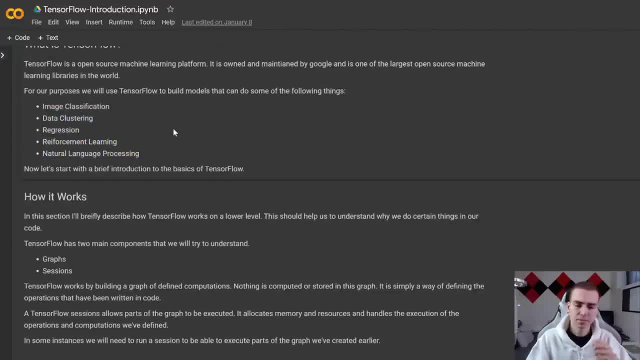 Well, these are some of the different things. I've listed them here, So I don't forget. we can do image classification, data clustering, regression, reinforcement learning, natural language processing and pretty much anything that you can imagine with machine learning. 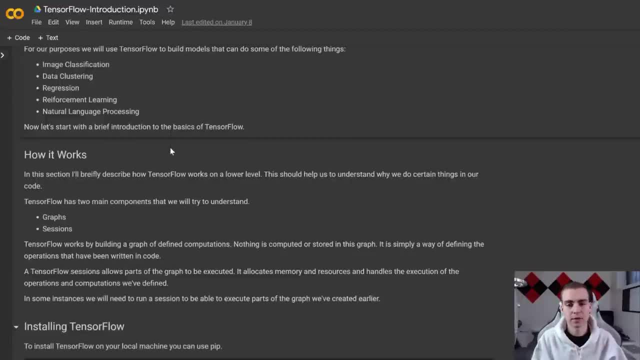 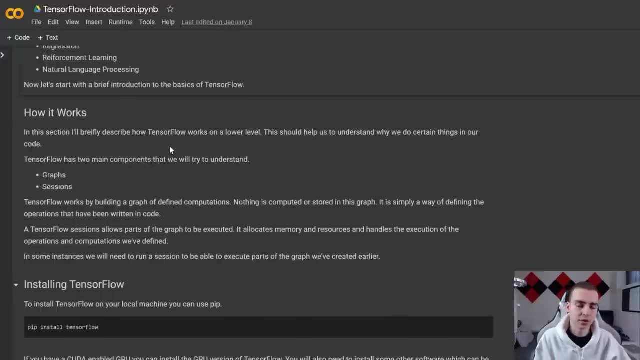 Essentially, what tends to flow does is gives us a library of tools that allow us to omit having to do these very complicated math operations. It just does them for us. Now there is a bit that we need to know about them, but nothing too complex. Now let's talk about how TensorFlow actually works. So TensorFlow? 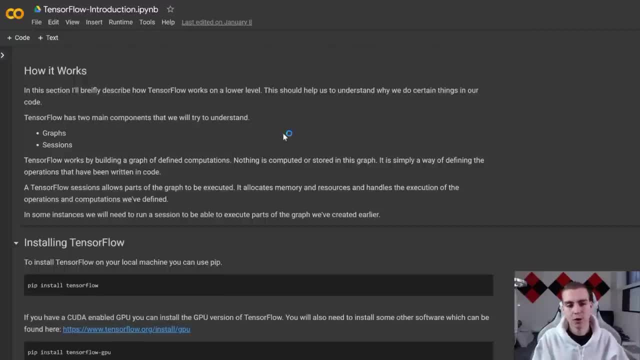 has two main components that we need to understand: to figure out how operations and math are actually performed. Now we have something called graphs and sessions. Now the way the TensorFlow works is it creates a graph of all the things that we need to know about variables in our graduate program. that'sの our curve in our alphabet, for example, And 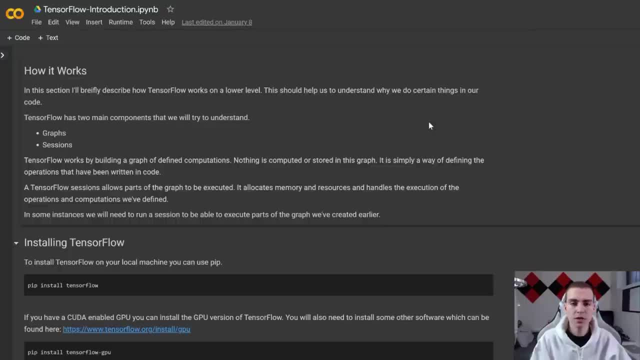 here's where we needed to find out a magic trick to figure out if this is right and perhaps the assumptions that we had out there. and that's the thing that makes sure any of theseotros avoid the experience that we used天使が本格的に strain trunktree. 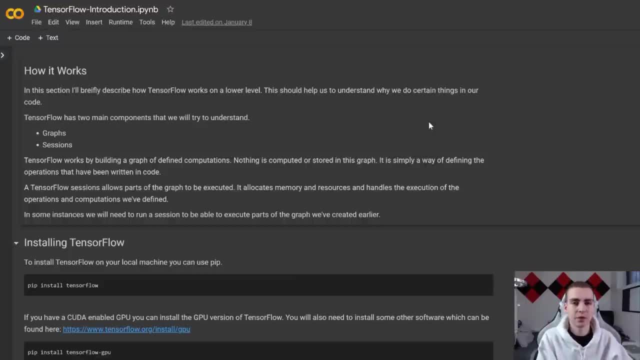 it's all sometimes a good idea to know the nature of table. oh yeah, we've learnt. we've gotten so much into the concepts of table we can't do with senators. you know наход, a lot of others. you know etiquette- to teach you even more Kelvin, and I think that's the. 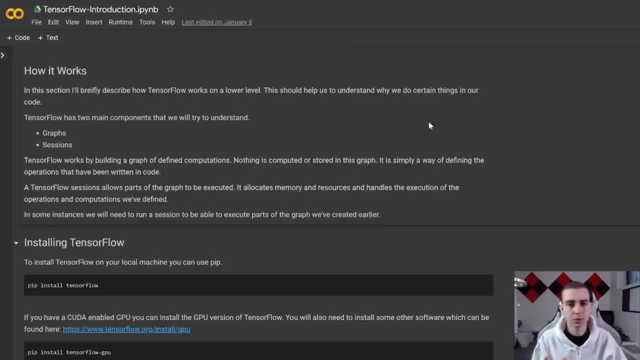 reason that it's super useful and useful again, is that these are the six pit doctors that teach you how to write. some write. they'll give you two choices: ofivi, ssd, 예. this will give you three options, and the following would be to verify your own array. very similarly. 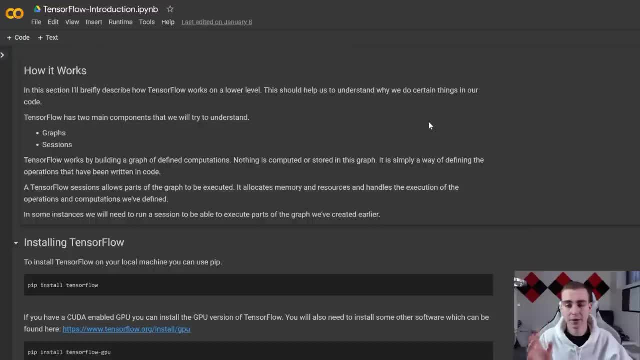 which is equal to the sum of variable two and variable three. But what we need to understand is that it doesn't actually evaluate that. it simply states that that is the computation that we've defined. So it's almost like writing down an equation without actually performing. 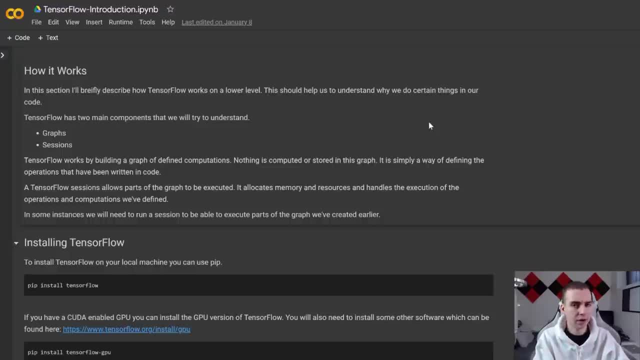 any math. we kind of just you know, have that equation there. we know that this is the value, but we haven't evaluated it, So we don't know that the value is like seven per se. we just know that it's the sum of, you know, vector one and vector two, or it's. 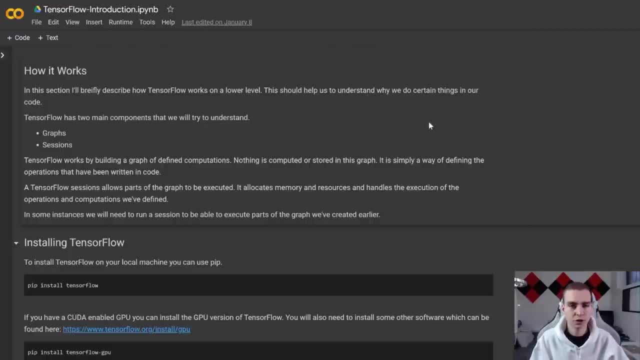 the sum of this, or it's the cross product or the dot product. we just define all of the different partial computations because we haven't evaluated those computation yet And that is what is stored in the graph. And the reason it's called a graph is because 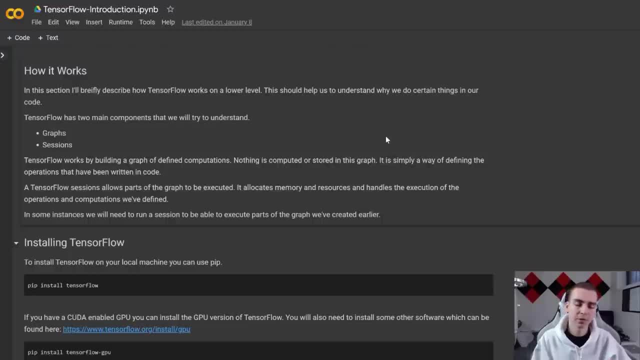 different computations can be related to each other. For example, if I want to figure out the value of vector one, but vector one is equal to the value of vector three plus vector four, I need to determine the value of vector three and vector four before I can do that computation. 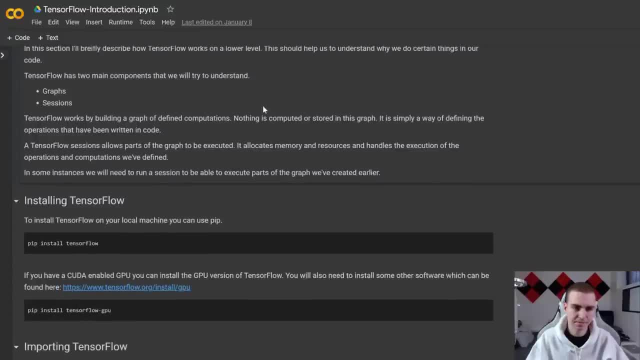 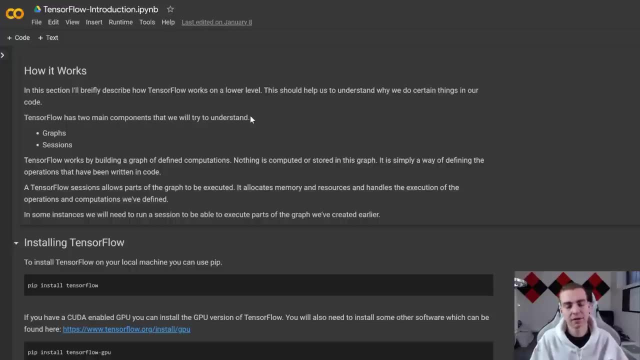 So they're kind of linked together And I hope that makes a little bit of sense. Now, what is a session? Well, session is essentially a way to execute part or the entire graph. So when we start a session, what we do is we start executing different aspects of the 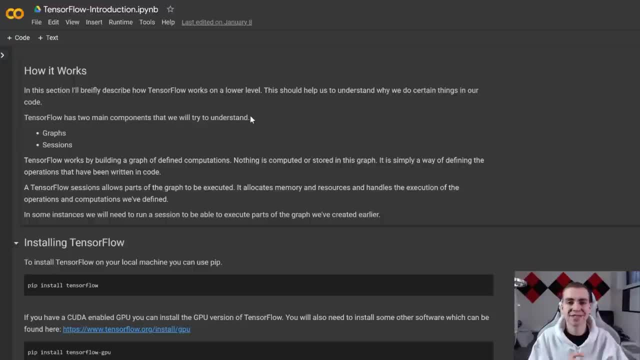 graph. So we start at the lowest level of the graph, where nothing is dependent on anything else. we have maybe constant values or something like that, And then we move our way through the graph and start doing all of the different partial computations that we've defined. Now I hope that this isn't too confusing. I know this. 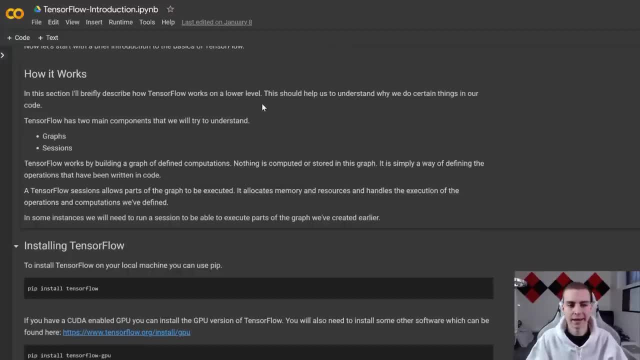 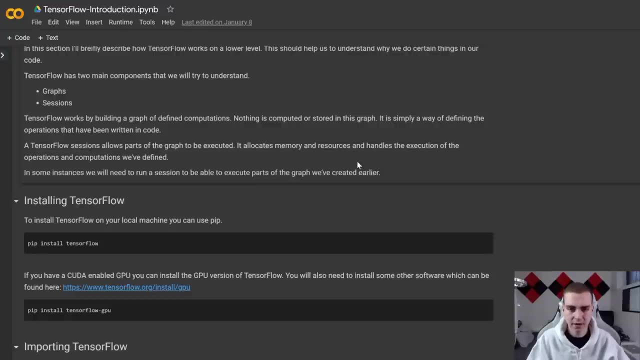 is kind of a lot of lingo. you guys will understand this as we go through. And again you can read through some of these components here that I have in Collaboratory, if I'm kind of skipping through anything or you don't truly understand, but that is the way that. 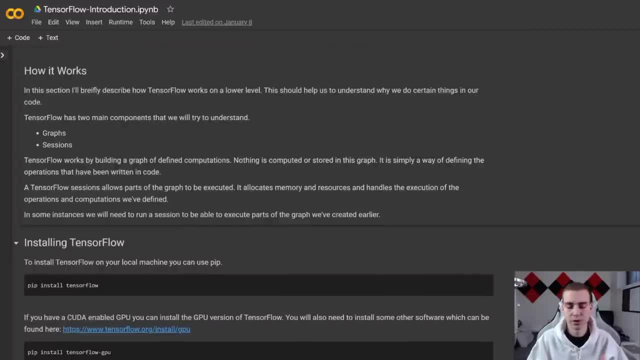 graphs and sessions work. We won't go too in depth with them. we do need to understand that that is the way TensorFlow works, And there's some times where we can't use a specific value in our code Yet because we haven't evaluated the graph, we haven't created a session and gotten the 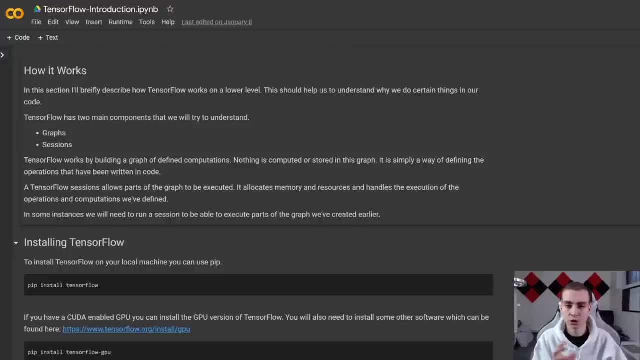 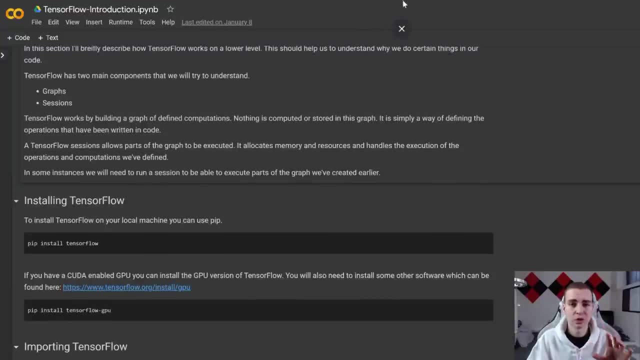 values yet, which we might need to do before we can actually, you know, use some specific value. So that's just something to consider, Alright, so now we're actually going to get into coding, importing and installing TensorFlow. Now, this is where I'm going to introduce. 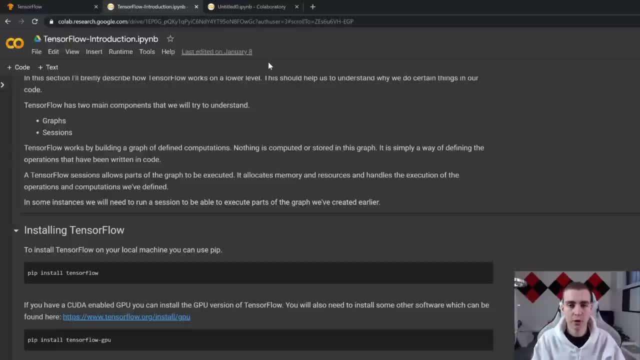 you to Google Collaboratory and explain how you guys can follow along without having to install anything on your computer. And it doesn't matter if you have like a really crappy computer or even if you're on like an iPhone per se. you can actually. 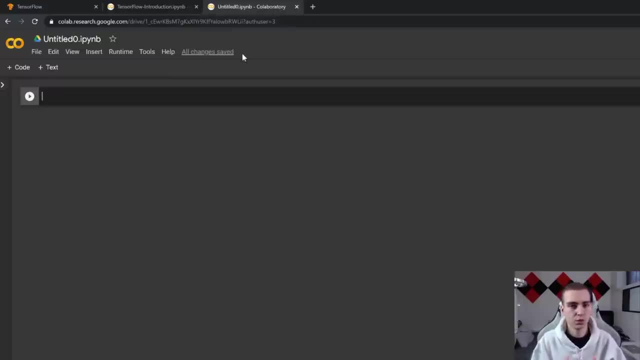 do this, which is amazing. So all you need to do is Google Google Collaboratory and create a new notebook. Now, what Google Collaboratory is is essentially a free Jupyter notebook in the cloud for you. The way this works is you can open up this notebook. you can see. 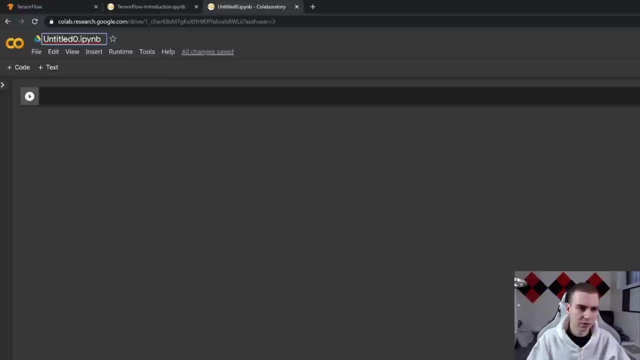 this is called I, pi and B. I- yeah, what is that? I pi and B, which I think just stands for I Python notebook, And what you can do in here is actually write code and write text as well. So this in here is what I called. 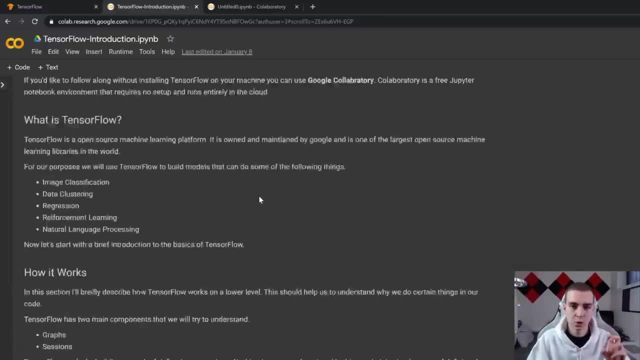 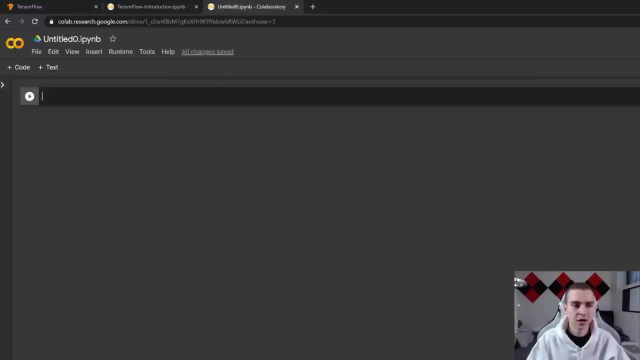 you know Google Collaboratory notebook And essentially why it's called a notebook is because not only can you put code, but you can also put notes, which is what I've done here with the specific titles, So you can actually use markdown inside of this. 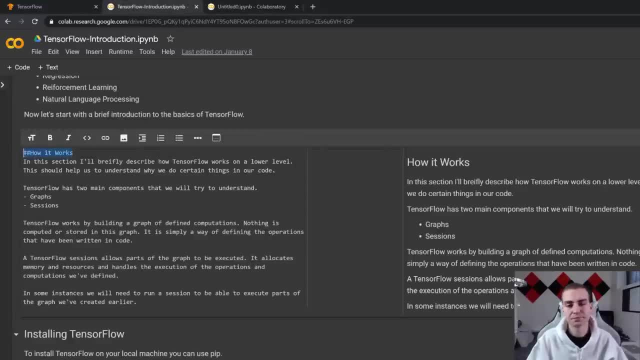 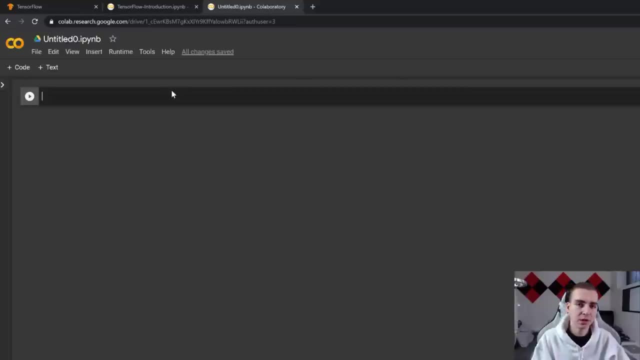 So if I open up one of these, you can see that I've used markdown text to actually kind of create these sections. And yeah, that is kind of how Collaboratory works. But what you can do in Collaboratory is forget about having to install all of these modules. They're 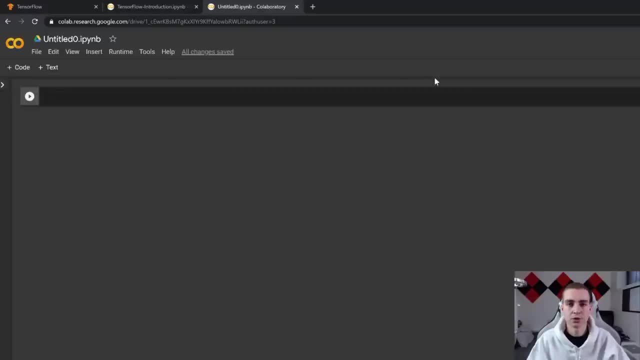 already installed for you. So what you're actually going to do when you open a Collaboratory window is Google is going to automatically connect you to one of their servers or one of their machines that has all of this stuff done and set up for you And you can start writing code and executing. 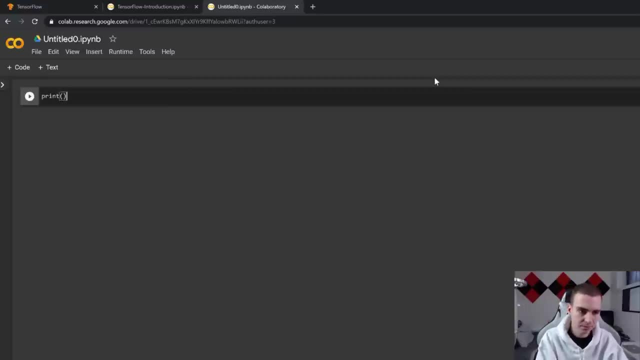 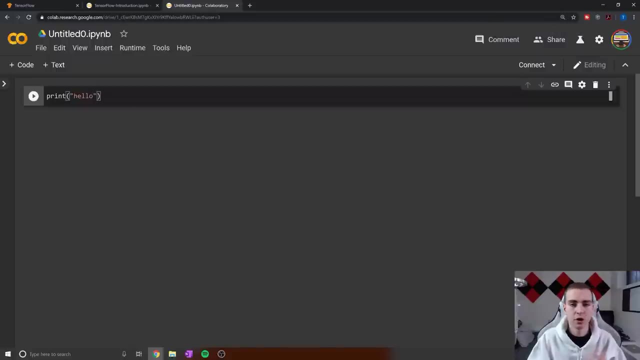 it off their machine and seeing the result. So, for example, if I want to print hello like this- and I'll zoom in a little bit so you guys can read this- all I do is I create a new code block, which I can do by clicking code like that, I can delete one like that. 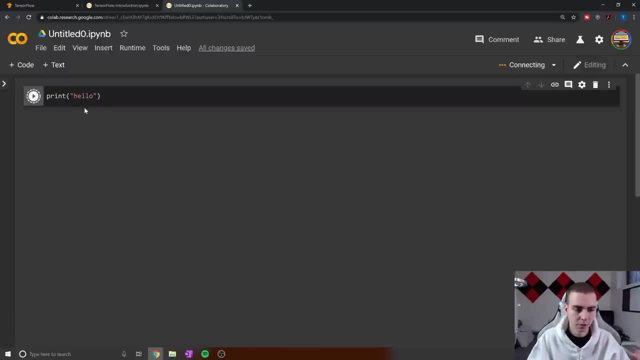 as well, And I hit run Now notice, give it a second. it does take longer than typically on your own machine And we get Hello popping up here. So the great thing about Collaboratory is the fact that we can have multiple code blocks and we can run them in whatever sequence we want. So 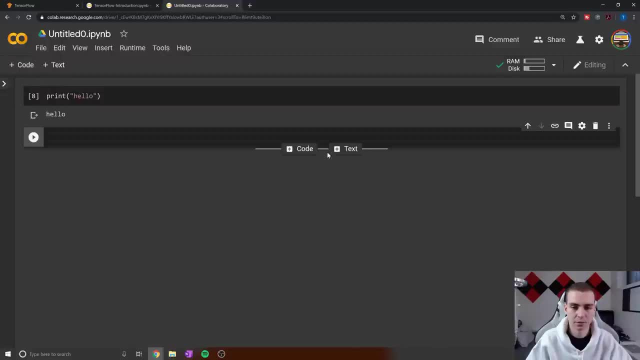 to create another code block. you can just, you know, do another code block from up here or by just by looking down here. you get code and you get text And I can run this in whatever order I want. So I can do like print Yes, for example. I can run Yes and we'll see. 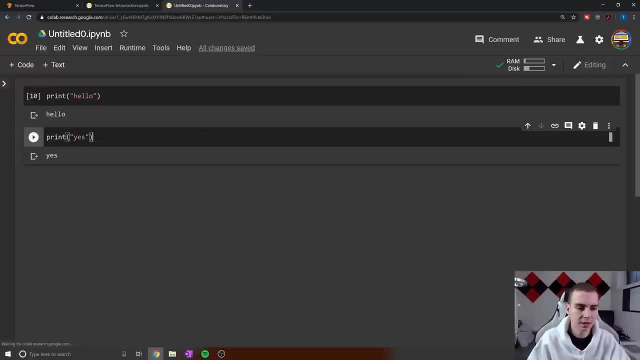 the output of Yes, And then I could print Hello One more time And notice that it's showing me the number on this left hand side here on which these kind of code blocks were run. Now all these code blocks can kind of access. 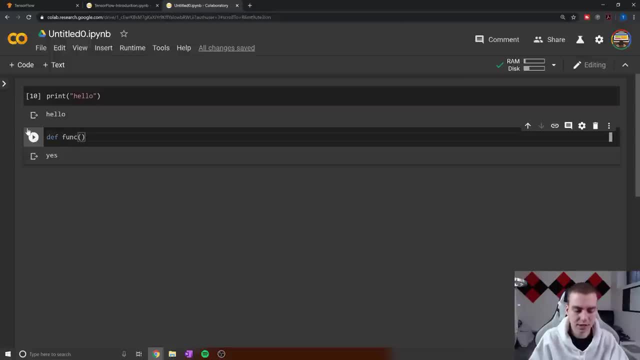 each other. So for example, I do define funk and we'll just take some parameter h And all we'll do is just print h. Well, if I create another code block down here, so let's go code, I can call funk with say: Hello, make sure, I run this block first. So we define: 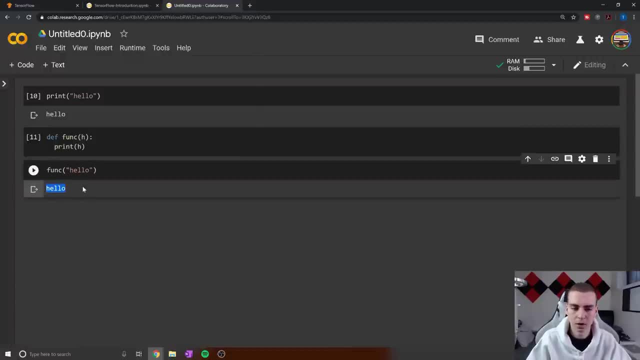 the function. Now. I'll run funk and notice we get the output Hello. So we can access all of the variables, all the functions, anything we've defined in other code blocks, from code blocks that are below it or code blocks that have executed after. 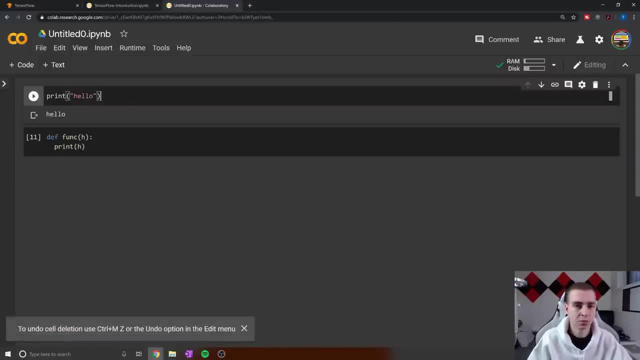 it Now. another thing that's great about Collaboratory is the fact that we can import pretty much any module we can imagine and we don't need to install it. So I'm not actually going to be going through how to install TensorFlow completely. there is a little bit on how to. 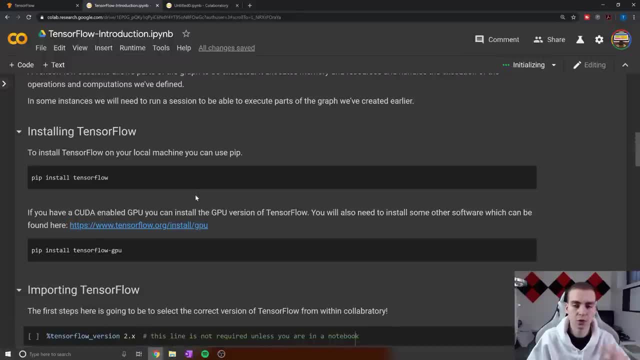 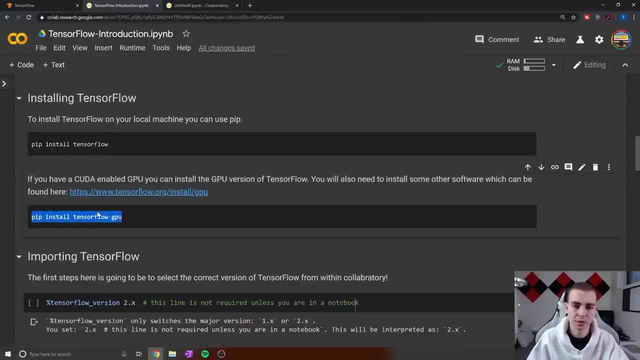 install TensorFlow on your local machine inside of this notebook which I'll refer you to. But essentially, if you know how to use pip, it's pretty straightforward. you can pip install TensorFlow. You can pip install TensorFlow GPU if you have a compatible GPU which you can check. 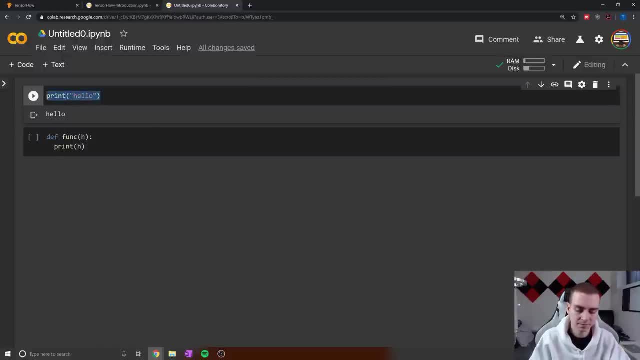 from the link that's in this notebook. Now, if I want to import something, what I can do is literally just write the import, So I can say import NumPy, like this. And usually NumPy is a module that you need to install, But we don't need to do that here, It's already. 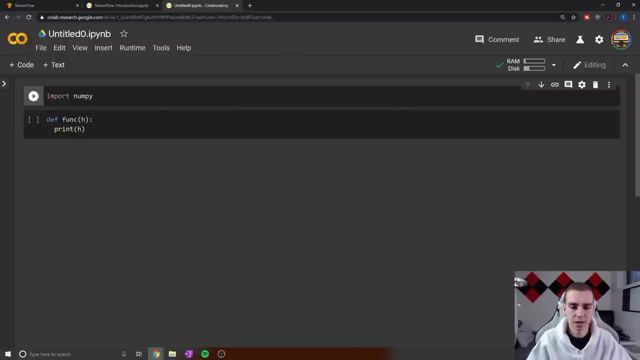 installed on the machine. So again, we hook up to those Google servers, we can use their hardware to perform machine learning, And this is awesome. This is amazing And it gives you performance benefits when you're running on like a lower kind of crappier machine. 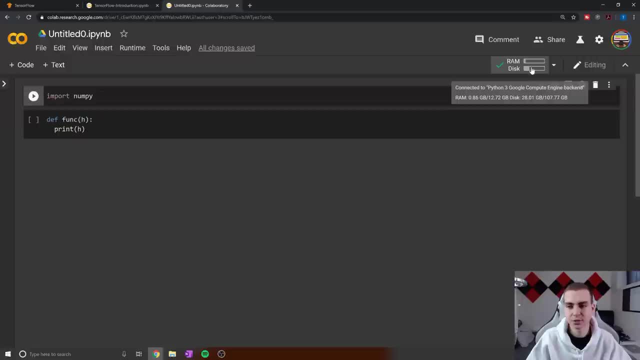 right, We can have a look at the RAM in the disk space of our computer. we can see we have 12 gigs of RAM. we're dealing with 107 gigabytes of data on our disk space And we can obviously- you know- look at that. if we want, we can connect to our local runtime, which I believe. 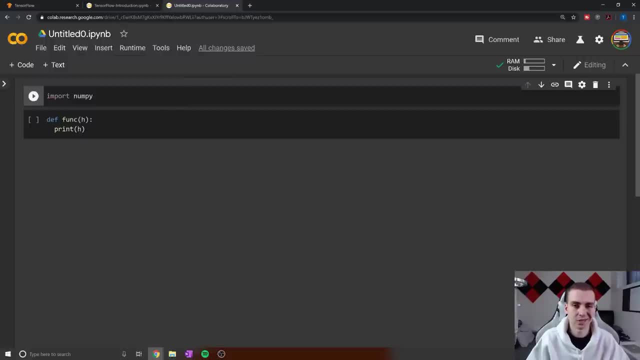 connects to your local machine. But I'm not going to go through all of that. I just want to show you guys some basic components of Collaboratory. Now, some other things that are important to understand is this runtime tab which you might see me use. So restart. 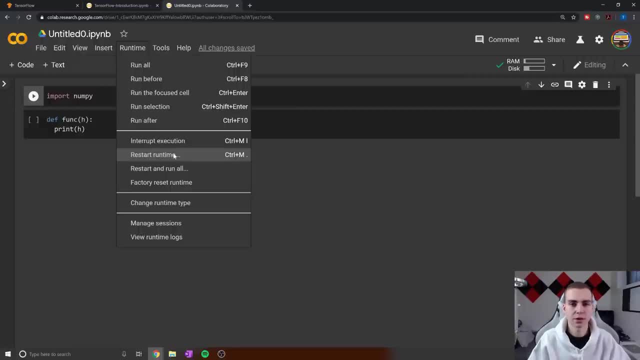 runtime essentially clears all of your output and just restarts whatever's happened. So, first things first, you want to restart everything. In this case, you will be restarting, but then you'll realign everything. And if so, because the great thing with Collaboratory? 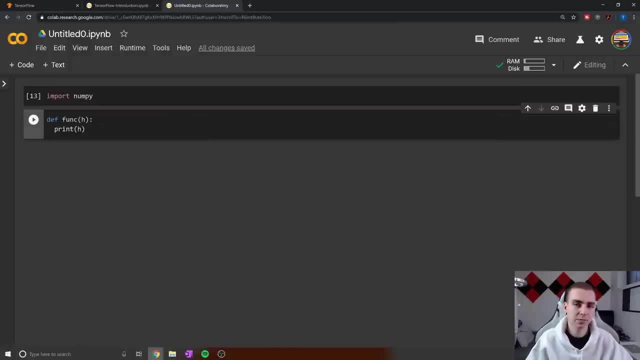 is, since I can run specific code blocks, I don't need to execute the entire thing of code every time I want to run something. If I've just made a minor change in one code block, I can just run that code. Sorry, I can just run that code block. I don't need. 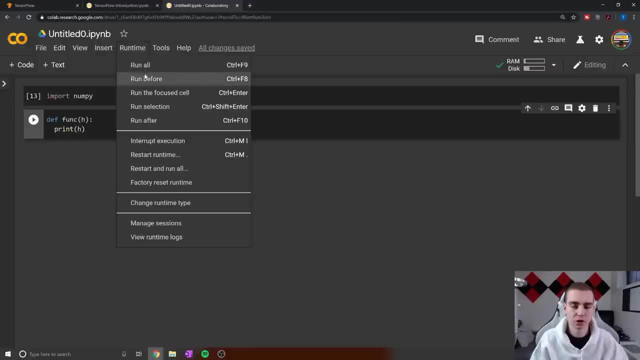 to run everything before or even everything after it, right. But sometimes you want to restart everything and just rerun everything. So to do that you click restart runtime. that's just going to clear everything you have and then restart and run. all will restart. 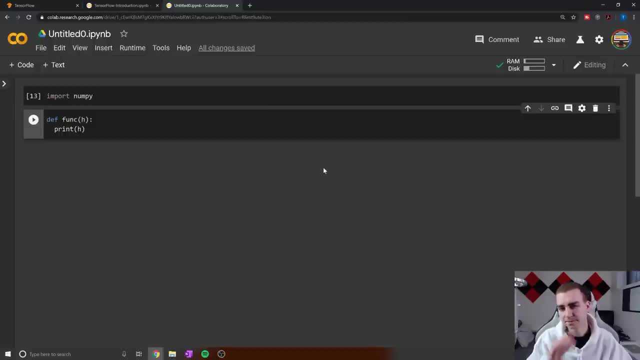 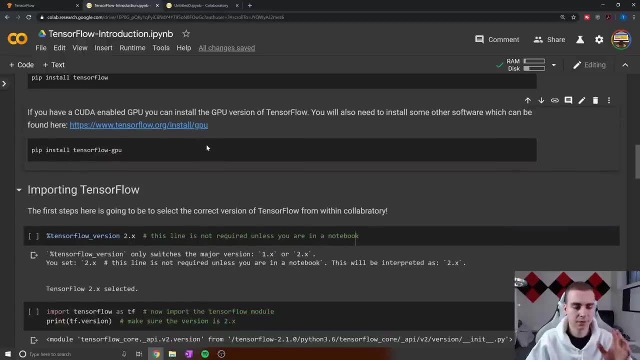 restart the runtime as well as run every single block of code you have in sequential order in which it shows up in the thing. So I'd recommend you guys open up one of these windows. You can obviously follow along with this notebook if you want, but if you want to type it out, 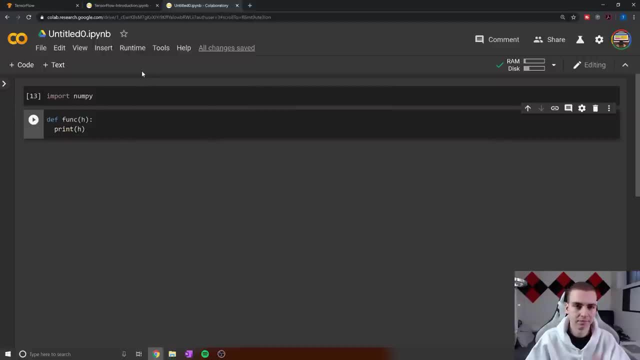 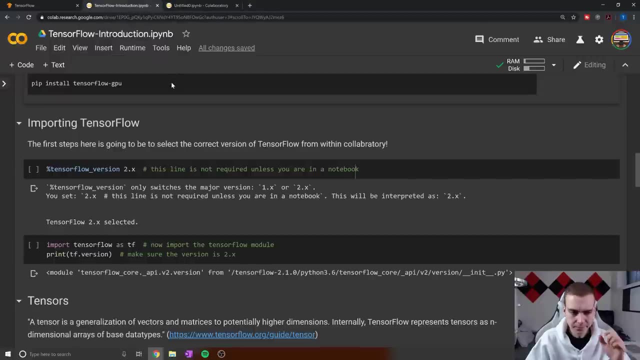 on your own and kind of mess with it. open up a notebook, save it. It's very easy, And these are again extremely similar to Jupiter notebooks. are Jupiter notebooks? They're pretty much the same. Okay, So that is kind of the Google collaboratory aspect: how to use that. 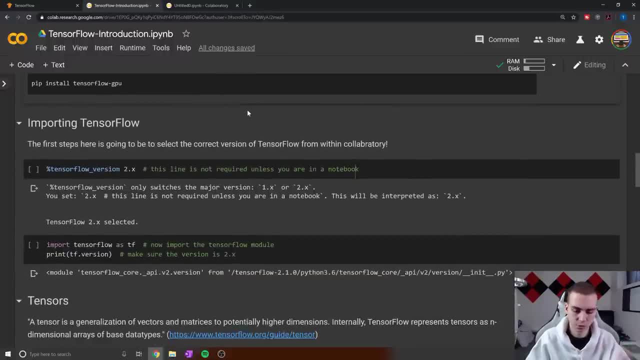 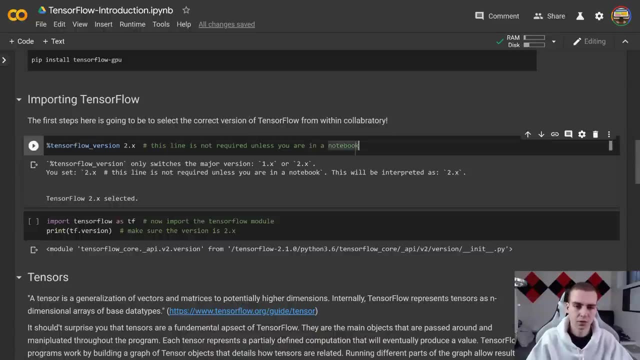 Let's get into importing TensorFlow. Now this is going to be kind of specific to Google collaboratory. So you can see here these are kind of the steps we need to follow to import TensorFlow. So, since we're working in Google collaboratory, they have multiple 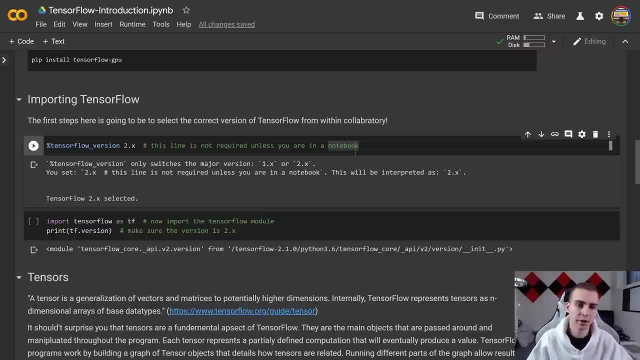 versions of TensorFlow. They have the original version of TensorFlow, which is 1.0, and the 2.0 version. Now, to define the fact that we want to use TensorFlow 2.0, just because we're in this notebook, we need to write this line of code at the very beginning of all of our 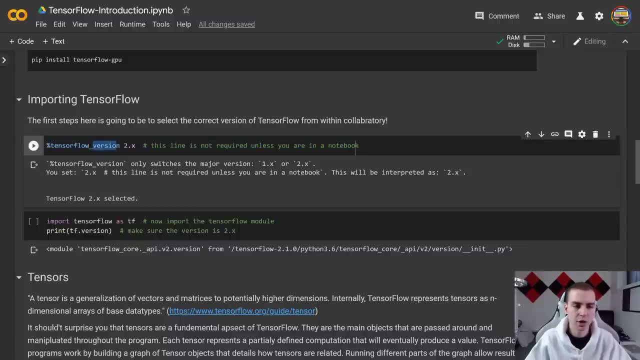 notebooks. So percent TensorFlow underscore version 2.X. Now, this is simply just saying we need to use TensorFlow 2.X. So, whatever version that is- and this is only required in a notebook- If you're doing this on your local machine. 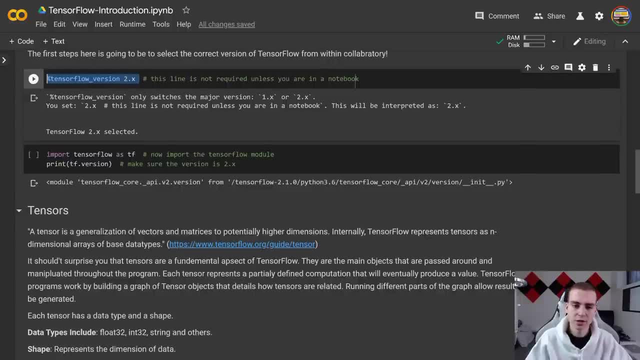 in a text editor. you're not going to need to write this Now. once we do that, we typically import TensorFlow as an alias name of TF. Now, to do that, we simply import the TensorFlow module And then we write as TF. If you're on your local machine, again you're going. 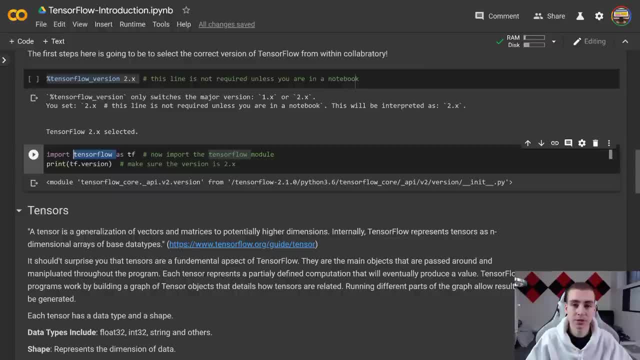 to need to install TensorFlow first to make sure that you're able to do this. But since we're in collaboratory, we don't need to do that Now, since we've defined the fact we're using version 2.X when we print the TensorFlow. 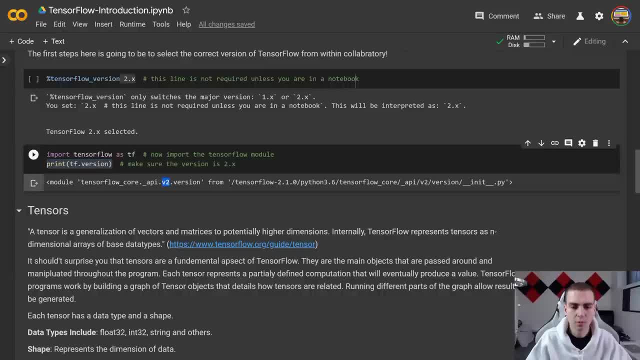 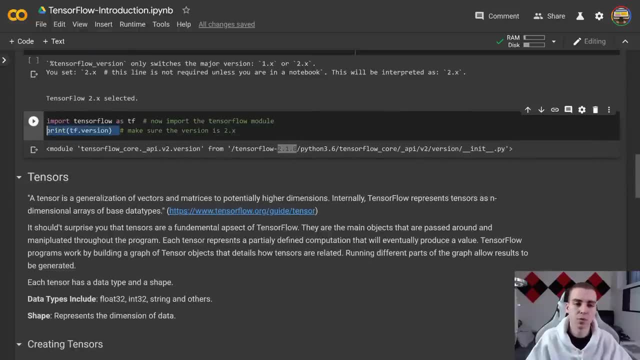 version. we can see here that it says version two, which is exactly what we're looking for, And then it says TensorFlow 2.1.0.. So make sure that you print your version. you're using version 2.0, because there is a lot of what I'm using in this series that is kind of 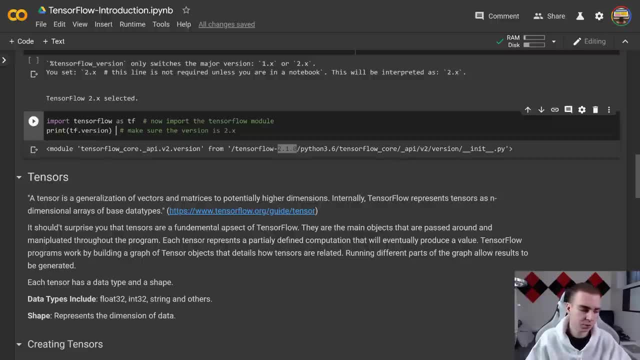 if you're in TensorFlow 1.0, it's not going to work. So it's new in TensorFlow 2.0, or it's been refactored and the names have been changed. Okay, so now that we've done that, 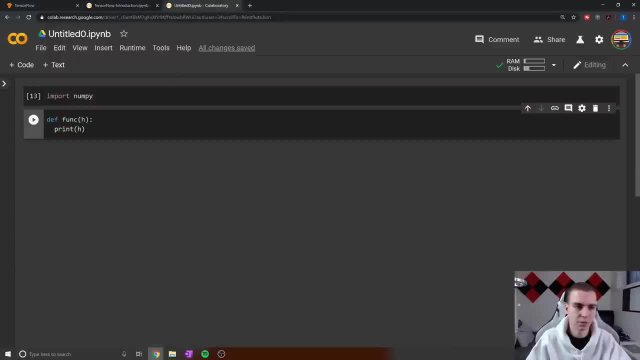 we've imported TensorFlow, we've got this here And I'm actually going to go to my fresh notebook and just do this, So we'll just copy these lines over, just so we have some fresh code And I don't have all this text that we have to deal with. So let's do this, TensorFlow. 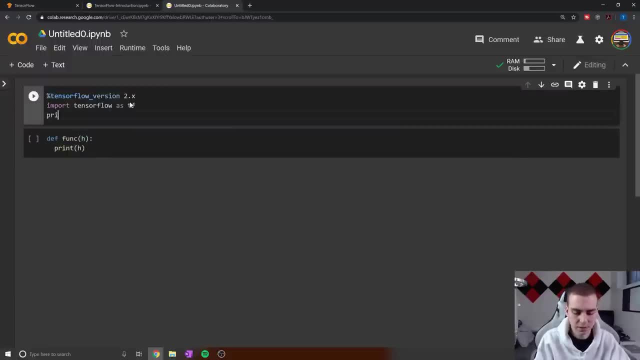 Let's import TensorFlow as TF And then we can print the TF dot version and have a look at that. So version Okay. so let's run our code here. we can see TensorFlow is already loaded. Oh, it says 1.0.. So if you get this error, it's actually good. I ran into this. 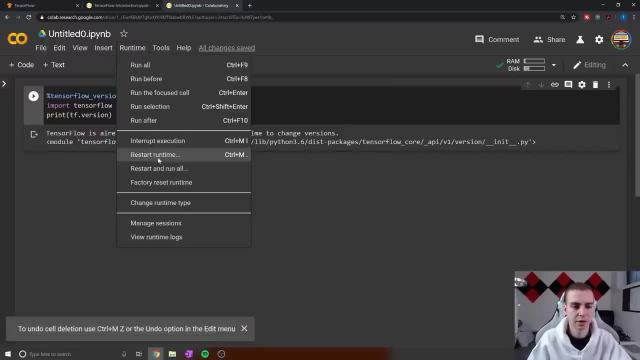 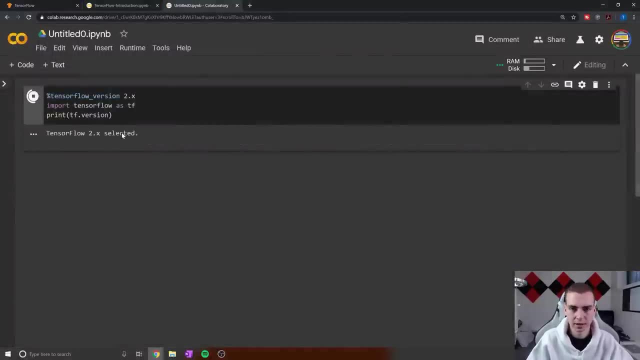 where TensorFlow has already been loaded. All you need to do is just restart your runtime. So I'm going to restart and run all. just click Yes, And now we should see that we get that version 2.0.. Once this starts running. 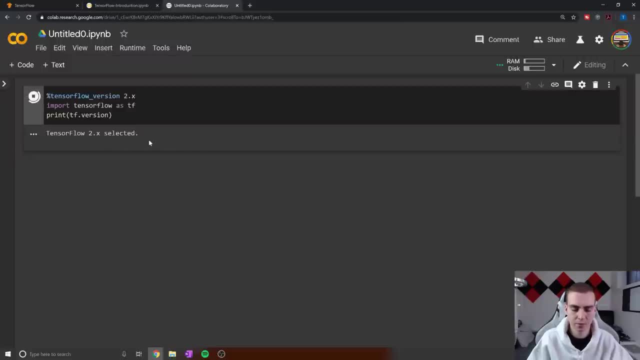 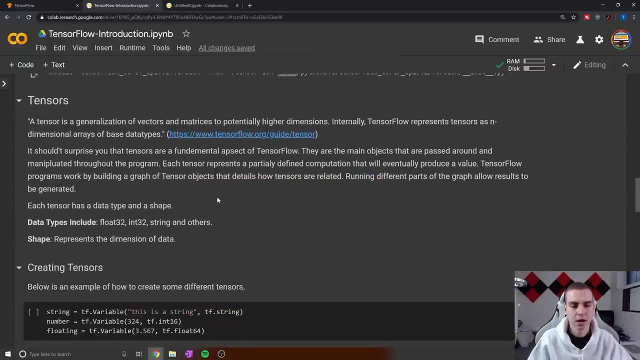 give it a second TensorFlow 2.0, selected. we're going to import that module And there we go, we get version 2.0.. Okay, so now it's time to talk about tensors. Now, what is a tensor? Now, tensor just immediately seems kind of like a complicated name, you're like 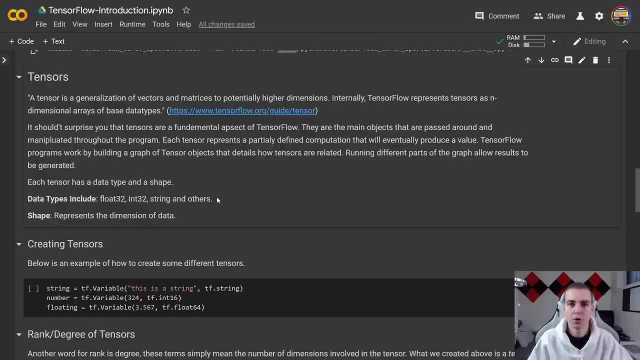 alright, tensor like this is confusing. But what is it? Well, obviously this is going to be a primary aspect Of TensorFlow, considering the name, similarities, and essentially all it is is a vector generalized to higher dimensions. Now, what is a vector? Well, if you've ever done any linear algebra, 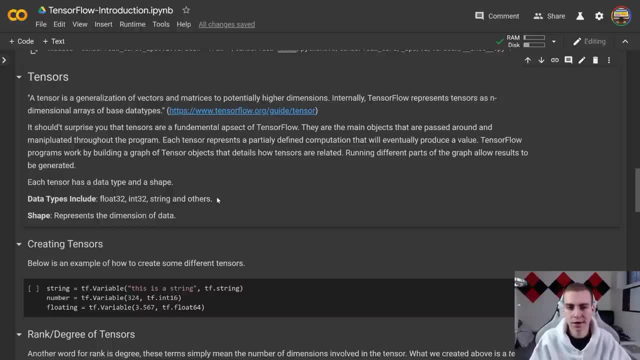 or even some basic kind of vector calculus. you should hopefully know what that is, But essentially it is kind of a data point is kind of the way that I like to describe it, And the reason we call it a vector is because it doesn't necessarily have a certain coordinate. 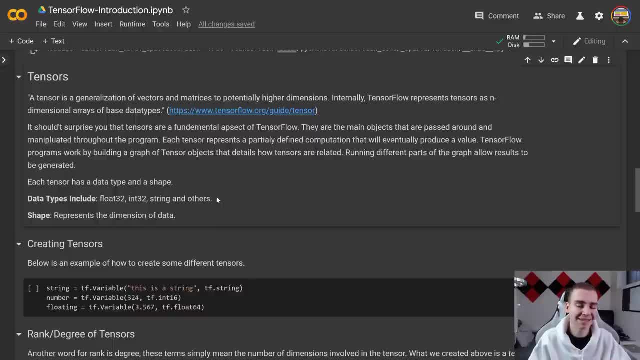 So, like if you're talking about a two dimensional data point, you have, you know, maybe an x and a y value, or like an x one value and an x two value. Now, a vector can have any amount of dimensions in it. it could have one dimension which 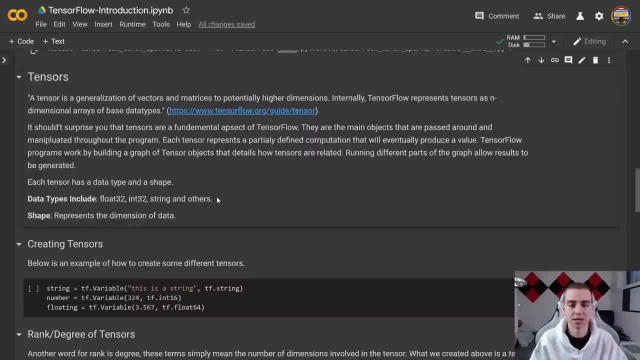 simply means just one number could have two dimensions, which means we're having two numbers, So like an x and a y value. if we're thinking about a two dimensional graph, we'd have three dimensions. if we're thinking about a three dimensional graph, so that would be three. 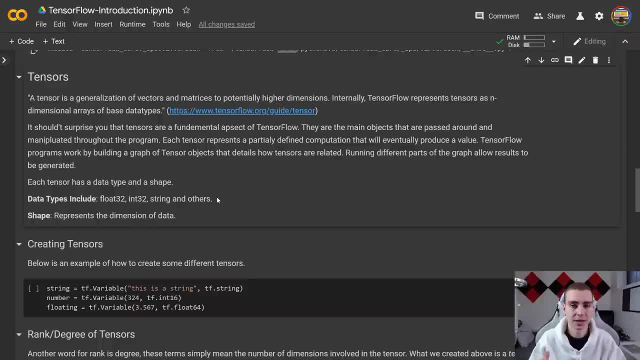 data points. we could have four dimensions if we're talking about sometimes some image data and some video data, And we can keep going, going going with vectors. So essentially what a tensor is, and I'll just read this formal definition to make sure I haven't butchered anything that's from the 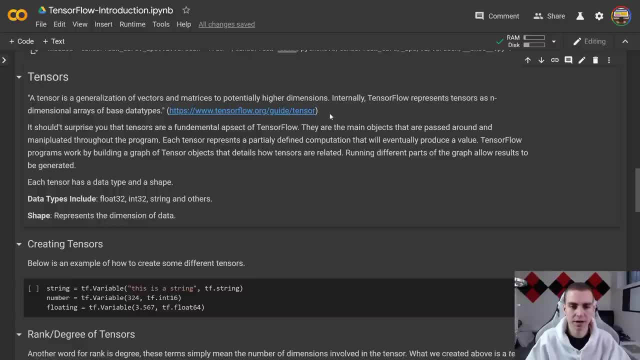 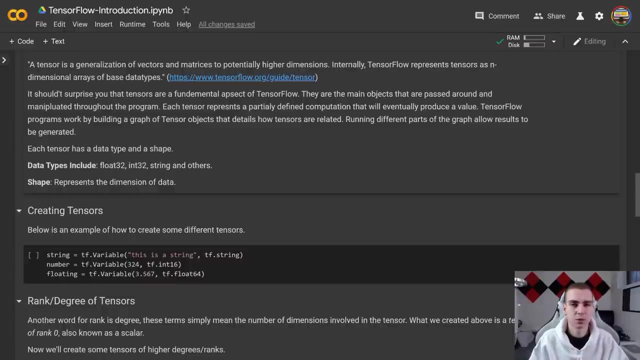 actual TensorFlow website. a tensor is a generalization of vectors and matrices to potentially higher dimensions. Internally, TensorFlow represents tensors as n dimensional arrays of base data types. Now we'll understand what that means in a second, But hopefully that makes sense Now, since tensors are so important to TensorFlow. they're kind of the 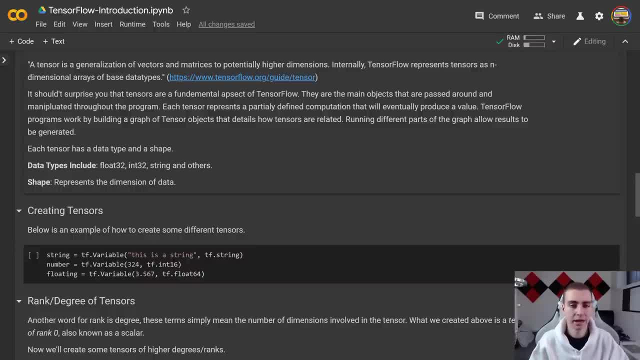 main object that we're going to be working with- manipulating and viewing- And it's the main object that's passed around through our program. Now, what we can see here is each tensor represents a partially defined computation that will eventually produce a value. So, just like we talked about in the graphs and sessions, what 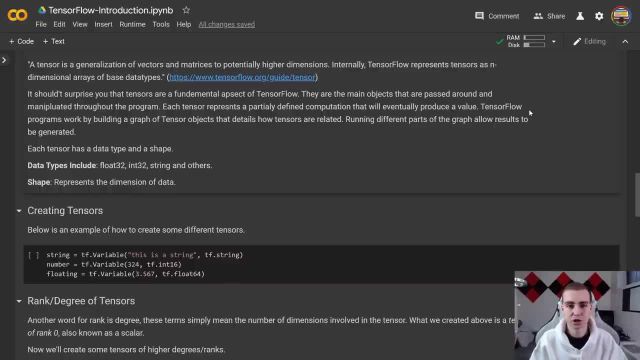 we're going to do is, when we create our program, we're going to be creating a bunch of tensors- and TensorFlow is going to be creating them as well- And those are going to store partially defined computations in the graph. Later, when we actually build the graph and have 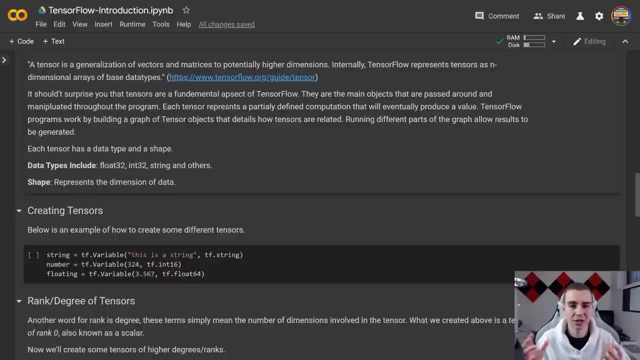 the production running. we will run different parts of the graph, which means we'll execute different tensors and be able to get different results from our tensors. Now, each tensor has what we call a data type and a shape, And that's what we're going to get into now. 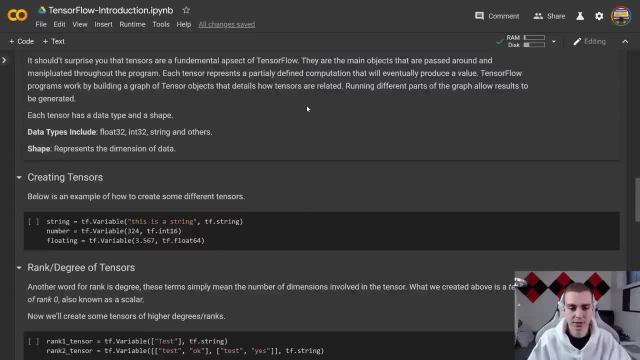 So a data type is simply what kind of information is stored in the tensor. Now, it's very rare that we see any data types different than numbers, although there is the data type of strings and a few others as well, But I haven't included all of them here because they're 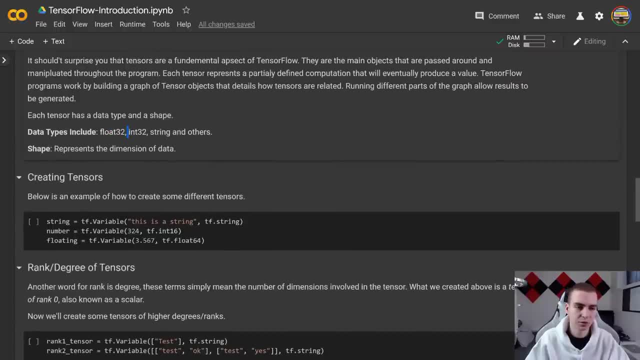 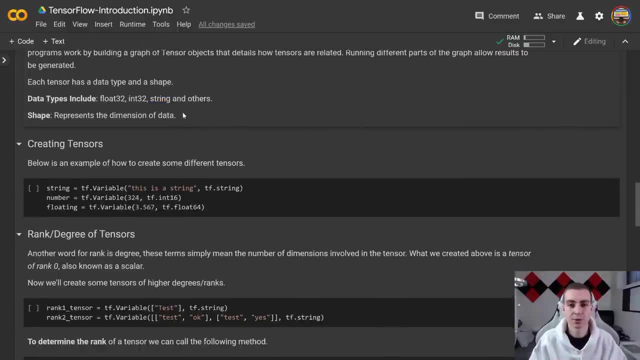 not that important, But some examples we can see are float 32, in 32 string, and we can see string and others. Now, the shape is simply the representation of the tensor in terms of what dimension it is, And we'll get some examples because I don't want to explain the. 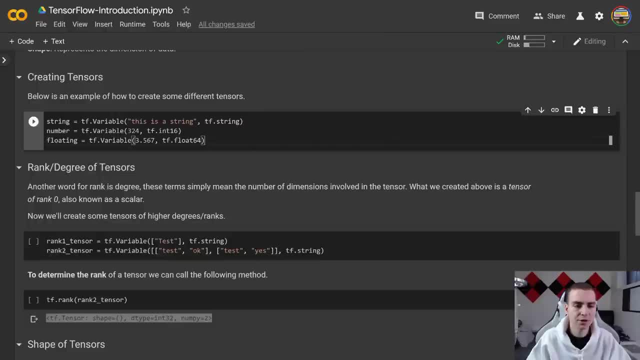 shape until we can see some examples to really dial in. But here are some examples of how we would create different tensors. So what you can do is you can simply do tf, dot variable And then you can do the value and the data type that your tensor is. So in this case, 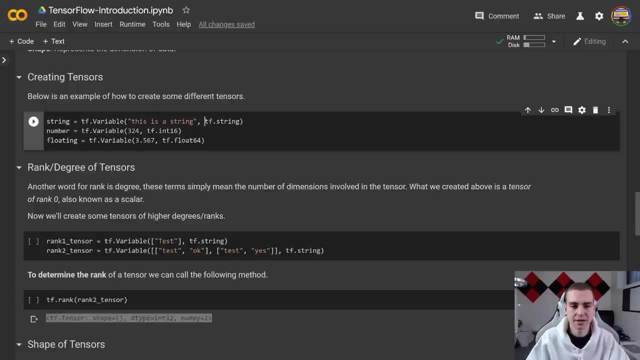 we've created a string tensor which stores one string And it is tf dot strings. we define the data type. Second, we have a number tensor which stores some integer value, And then that is of type tf in 16. And we have a floating. 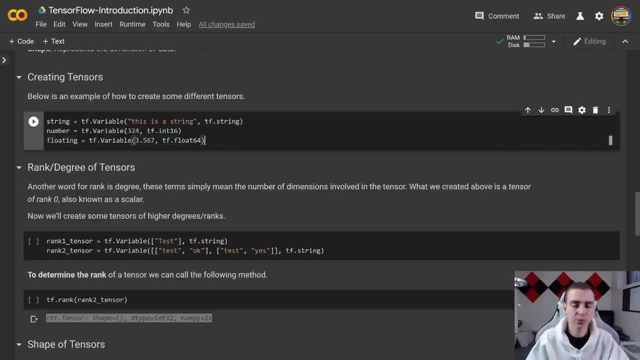 point tensor which stores a simple floating point. Now these tensors have a shape of- I believe it's going to be one, which simply means they are a scalar. Now, a scalar value- and you might hear me say this a lot- simply means just one value. That's all it means. 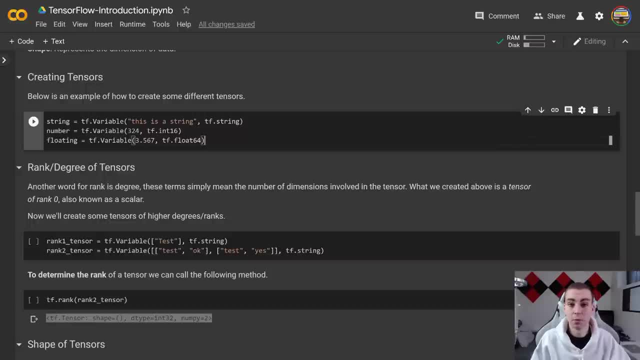 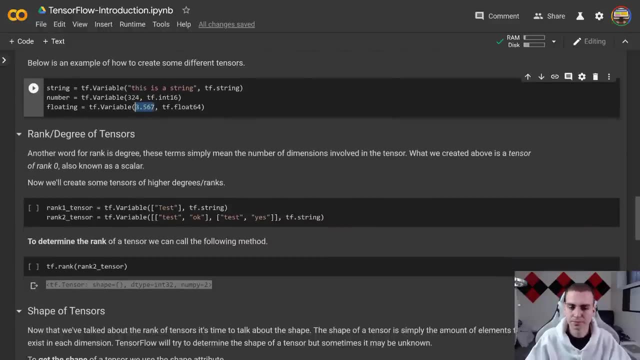 When we talk about like vector values, that typically means more than one value, And we talked about matrices. we're having different. it just it goes up, but scalar simply means one number. So, yeah, that is what we get for the different data types and creating tensors. We're not really. 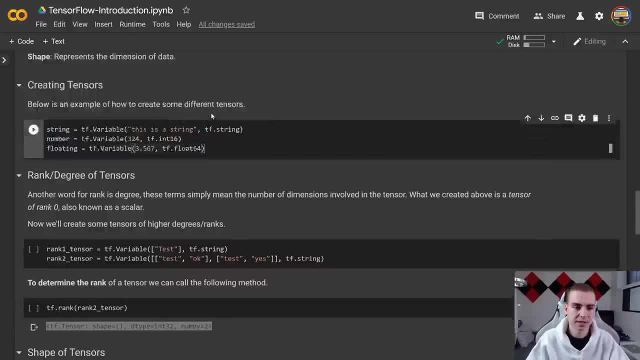 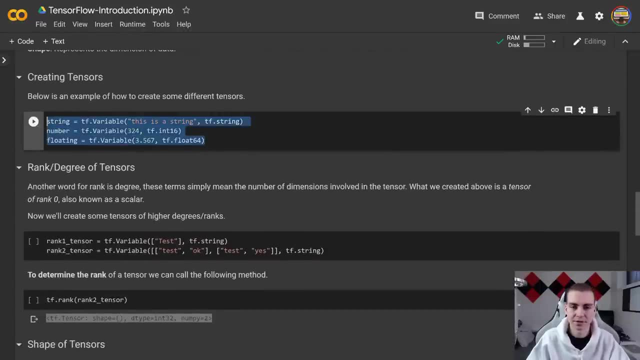 going to do this very much in our program, But just for some examples here, that's how we do it. So we've imported them So I can actually run these. and I mean, we're not going to really get any output by running this code because well, there's nothing to see. But 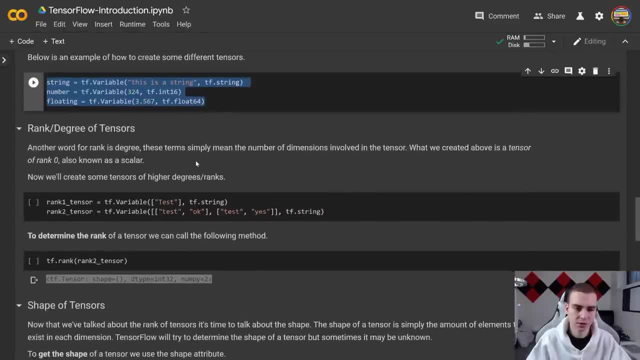 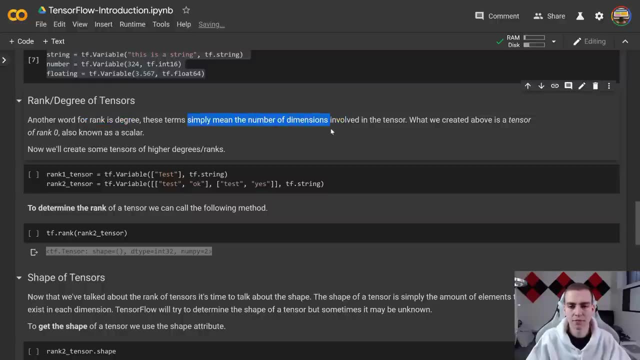 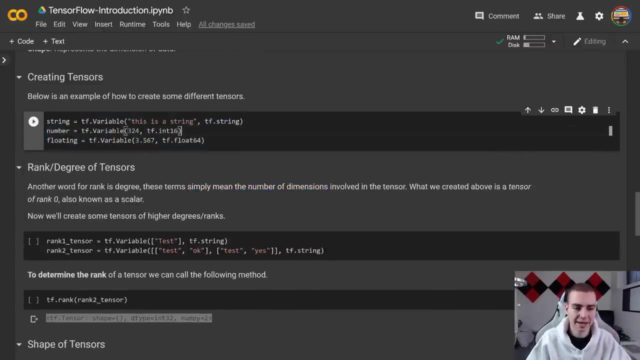 now we're going to talk about the rank slash degree of tensors. So another word for rank is agree. So these are interchangeably, And again this simply means the, the number of dimensions involved in the tensor. So when we create a tensor of rank zero, which is what we've done up here, we call that a scalar. Now the reason. 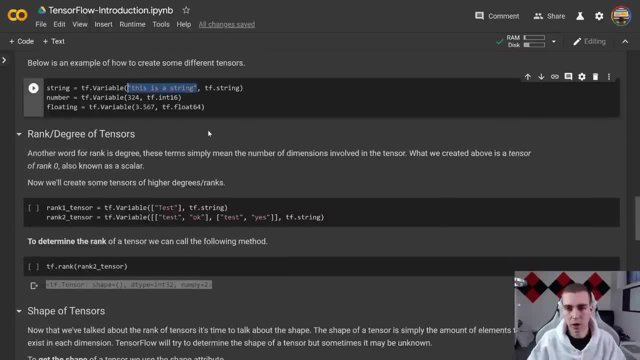 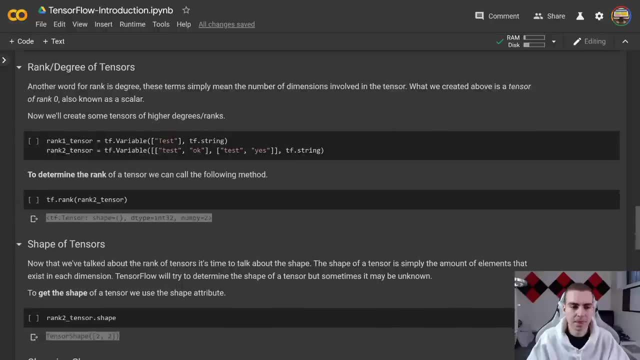 this has rank zero is because it's simply one thing. we don't have any dimensions to this. there's like zero dimensionality. if that is even a word, it's just one value, Whereas here we have an array. Now, when we have an array, we're going to have an array. 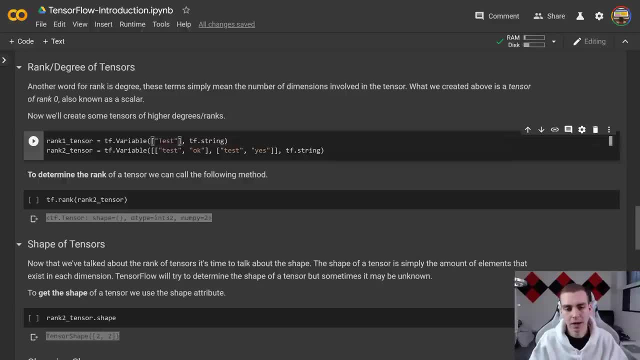 or a list, we immediately have at least rank one. Now, the reason for that is because this array can store more than one value in one dimension, right, So I can do something like test. I can do, okay, I could do Tim, which is my name, And we can run this And we're. 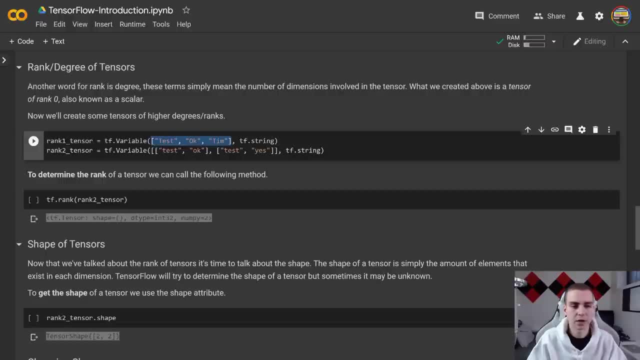 not going to get any output, obviously here. But this is what we would call a rank one tensor, because it is simply one list, one array, which means one dimension, And again, you know that's also like a vector. Now this, what we're looking at here, is a rank two tensor. The reason this is a rank: 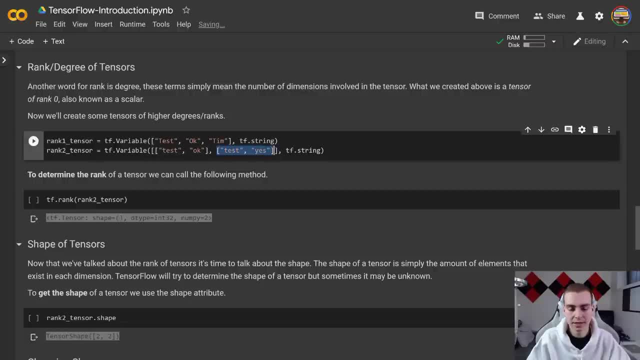 two tensor is because we have a list inside of a list, or, in this case, multiple lists inside of a list. So the way that you can actually determine the rank of a tensor is the deepest level of a nested lists, at least in Python, with our representation that's. 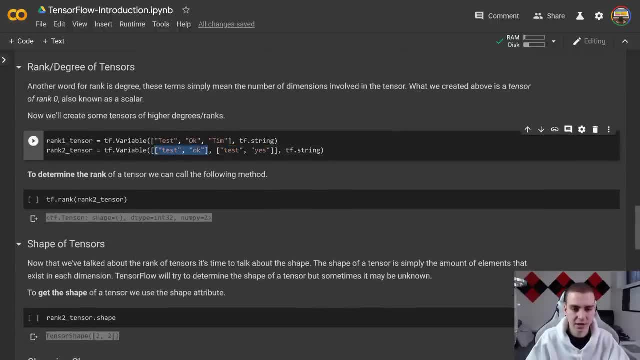 what that is. So here we can see, we have a list inside of a list and then another list inside of this upper list. So this would give us rank two, And this is what we typically call a matrices, And this again is going to be a tf dot string. So that's the data. 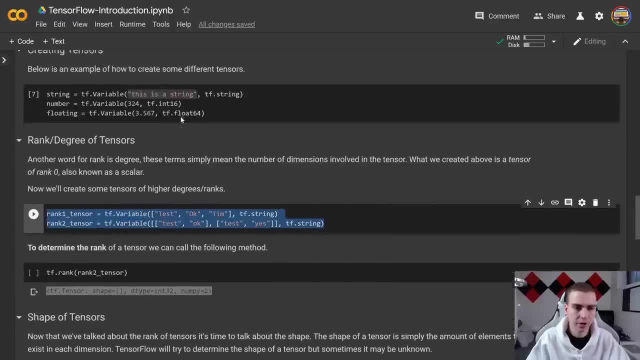 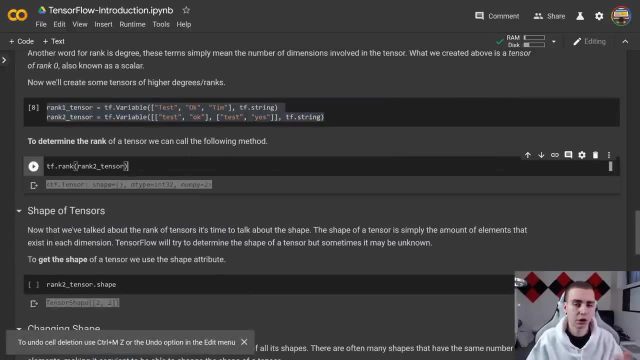 type for this tensor variable. So all of these that we've created are tensors. they have a data type and they have some rank and some shape, And we're going to talk about the shape in a second. So to determine the rank of a tensor, we can simply use the method tf dot. 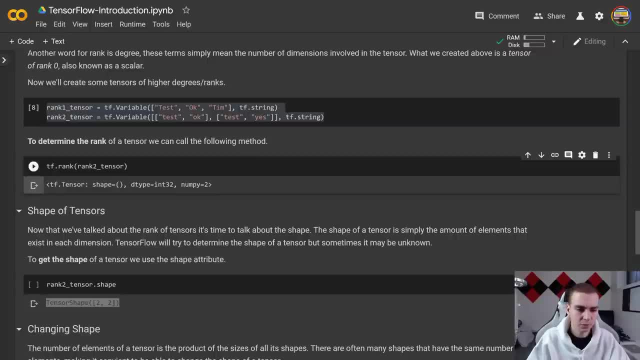 rank. So notice, when I run this, we get the shape, which is blank, of rank two tensor. that's fine. And then we get NumPy two, which simply means that this is a rank two. Now, if I go for that rank one tensor and I print this out, So let's have 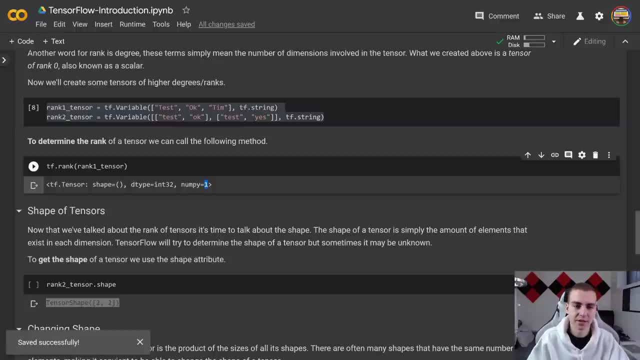 a look at it. we get NumPy one here which is telling us that this is simply of rank one. Now, if I want to use one of these ones up here and see what it is, so let's try it. we can do number. so tf dot rank number, So we'll print that here And we get NumPy zero. 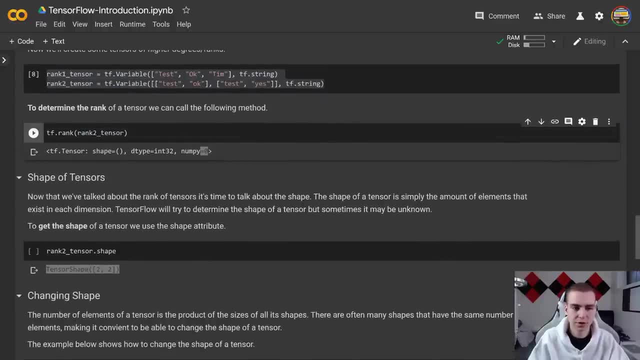 because that's rank zero, right. So we'll go back to what we had, which was ranked to tensor. But again, those are kind of the examples we want to look at. Okay, so, shapes of a tensor. So this is a little bit different now. 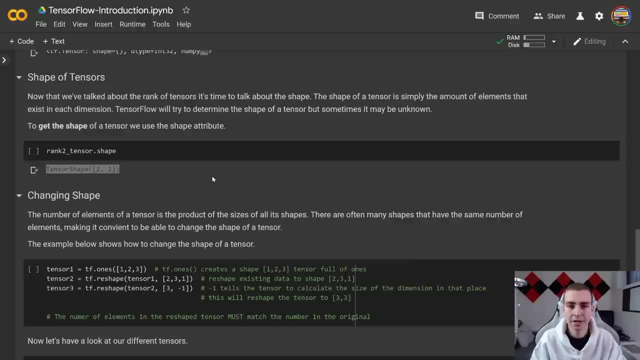 What does shape simply tells us is how many items we have in each dimension. So in this case, when we're looking at rank two, tensor dot shape- so we have dot shape here. that's an attribute of all of our tensors- we get to two. Now let's look up here what we have. 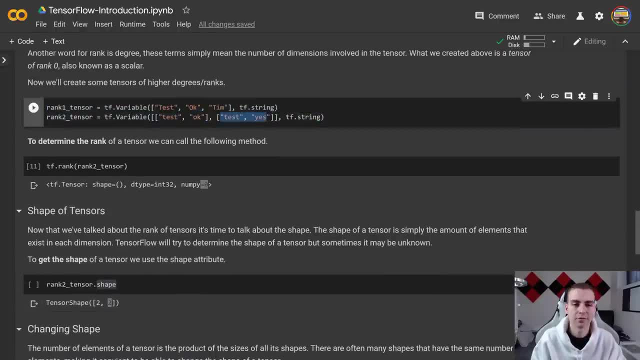 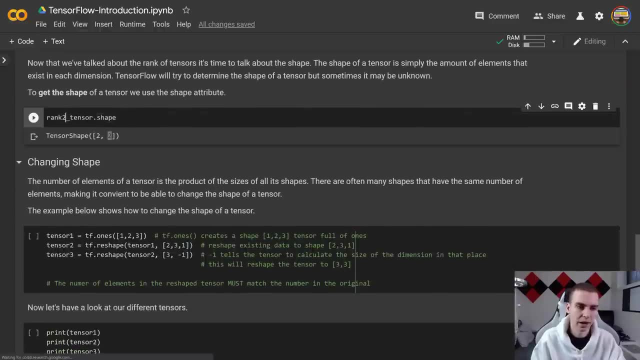 is Whoa. look at this. two and two. So we have two elements in the first dimension, right, and then two elements in the second dimension. That's pretty much what this is telling us. Now let's look at the rank for the shape of rank: one tensor, we get three. 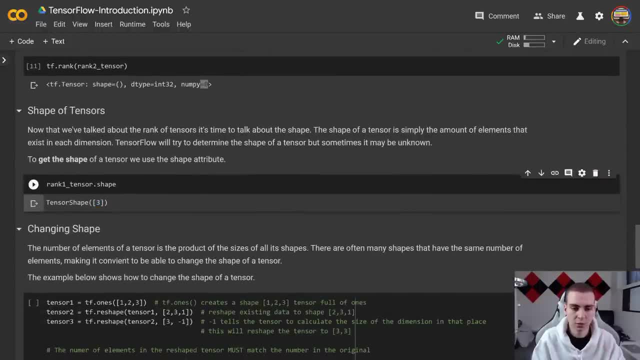 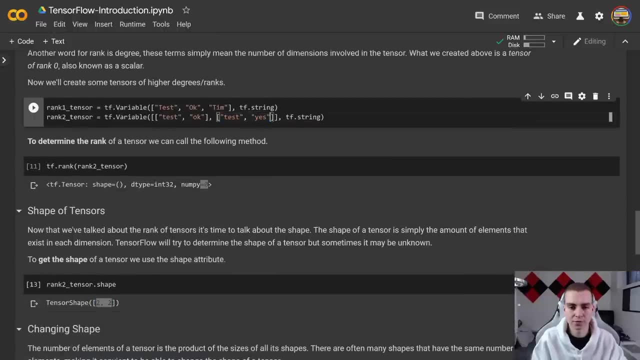 elements. So because we only have a rank one, notice we only get one number, whereas when we had rank two, we got two numbers and it told us how many elements were in each of these lists, right? So if I go and I add another one here like that, and we have a 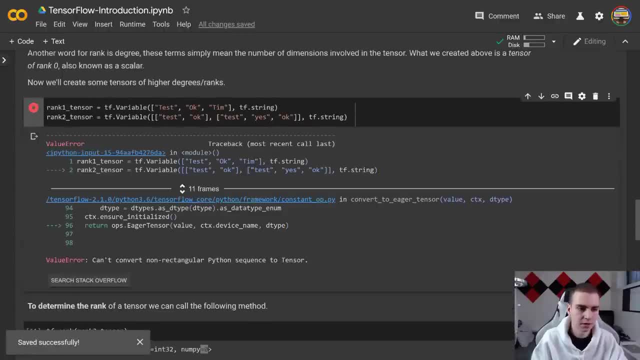 look now at the shape. oops, I got to run this first, So that's something I can't convert non square to tensor, Sorry. so I need to have a uniform amount of elements in each one here. I can't just do what I did there, So we'll add a third element here. Now we'll. 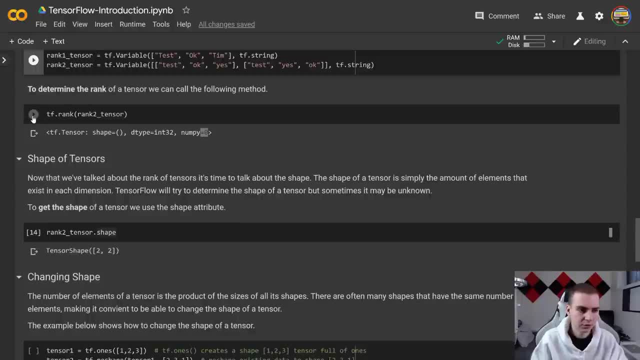 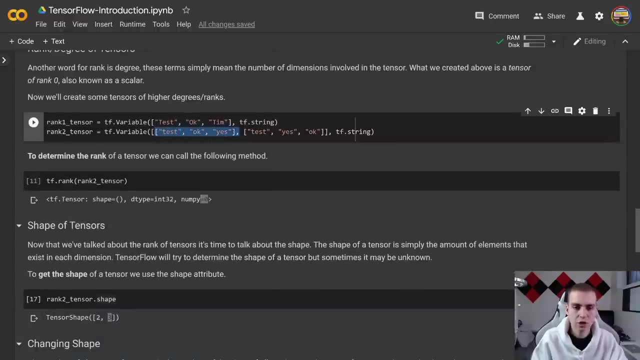 we can do is run. this shouldn't get any issues. Let's have a look at the shape And notice we get now to three. So we have two lists And each of those lists have three elements inside of them. So that's how the shape works. Now I could go ahead and add another list. 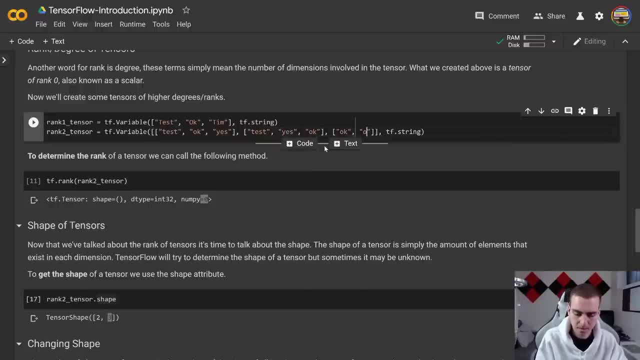 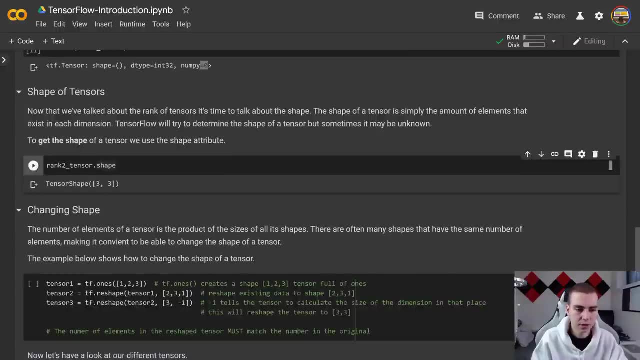 in here if I wanted to And I could say like, okay, Okay, Okay. so let's run this. Hopefully no errors. Looks like we're good. Now let's look at the shape again. And now we get a shape of three. three because we have 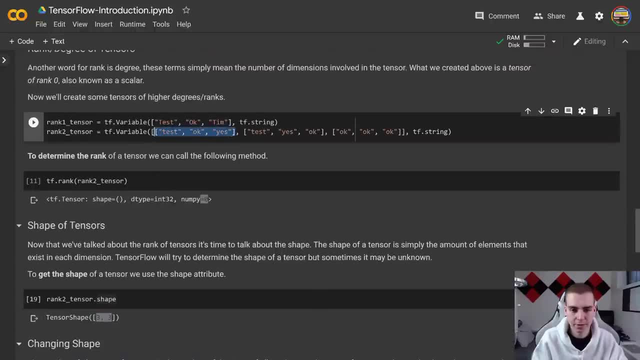 Okay, so let's run this. Hopefully no errors. looks like we're good. Now let's look at the shape again. And now we get a shape of three. three because we have three interior lists And in each of those lists we have three elements, And that is. 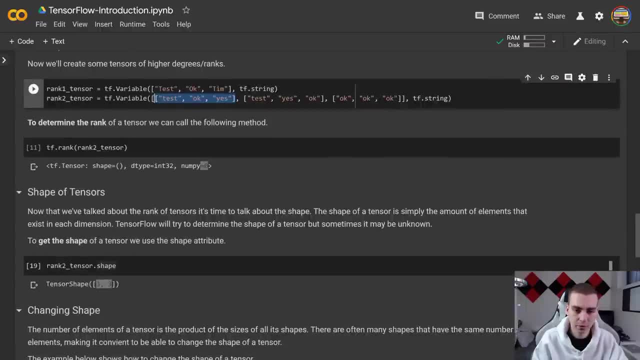 pretty much how that works. Now again, we can go even further here. we can put another list inside of here that would give us a rank three tensor, And we'd have to do that inside of all of these lists, And then what that would give us now would be three numbers. 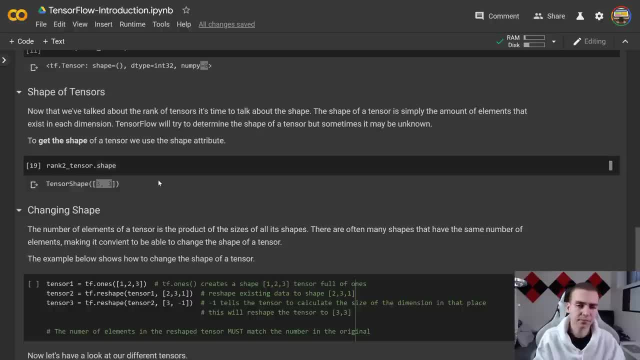 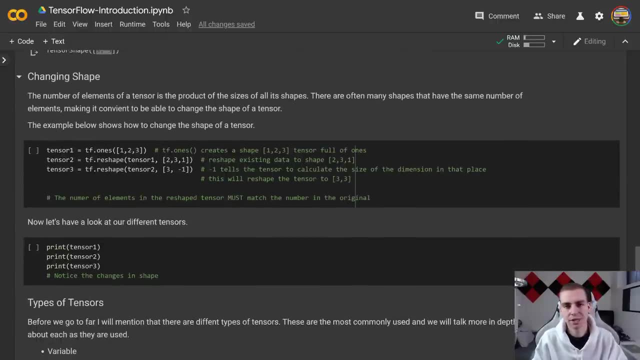 representing how many elements we have in each of those different dimensions. Okay, so changing shape? Alright. so this is what we need to do a lot of times when we're dealing with tensors and TensorFlow. So, essentially, there is many different shapes that can represent the same number of elements. 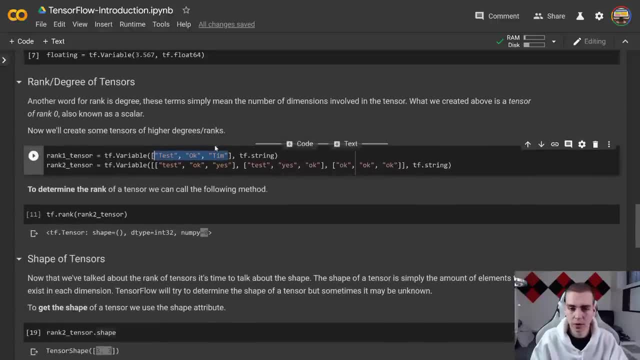 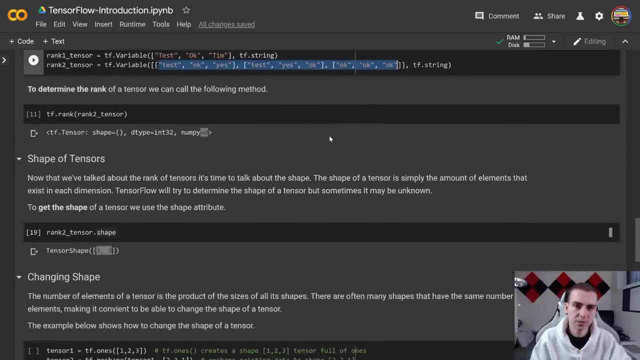 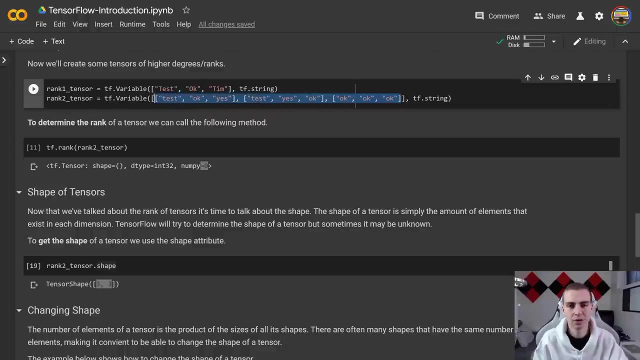 So up here we have three elements in a rank one tensor, And then here we have nine elements in a rank two tensor. Now there's ways that we can reshape this data so that we have the same amount of elements but in a different shape. For example, I could flatten this right. 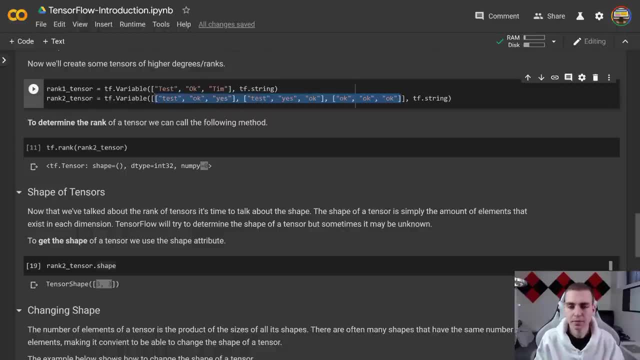 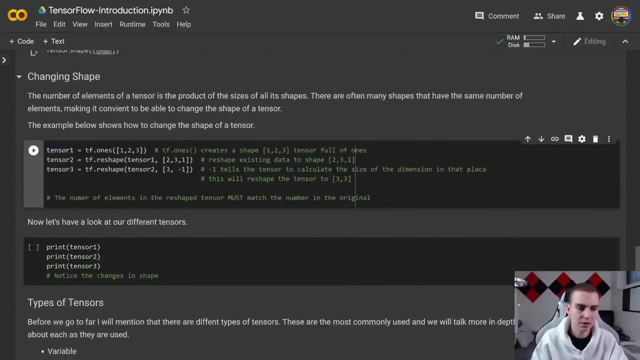 take all of these elements and throw them into a rank one tensor that simply is a length of nine elements. So how do we do that? Well, let me just run this code for us here and have a look at this. So what we've done is we've created tensor one that is tf dot ones. what this stands: 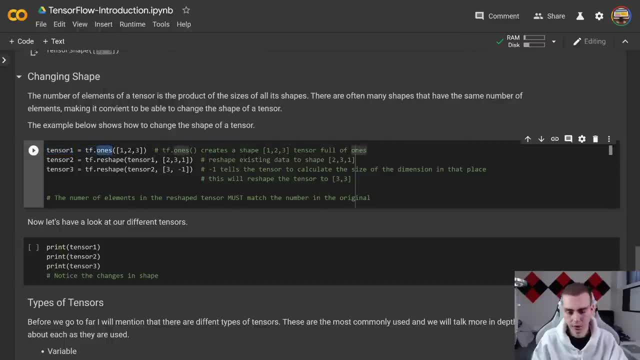 for is we're going to create a tensor that simply is populated completely with ones of this shape, So shape 123, which means you know that's the shape we're going to get. So let's print this out and look at tensor one, just so I can better illustrate this. 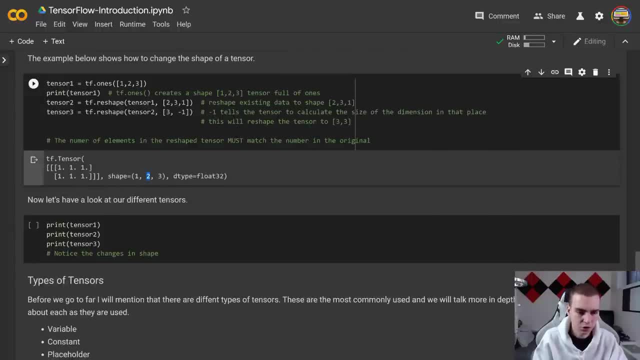 So, tensor one, look at the shape that we have 123.. Right, so we have one interior list which we're looking at here, And then we have two lists inside of that list, And then each of those lists we have three elements. So that's. 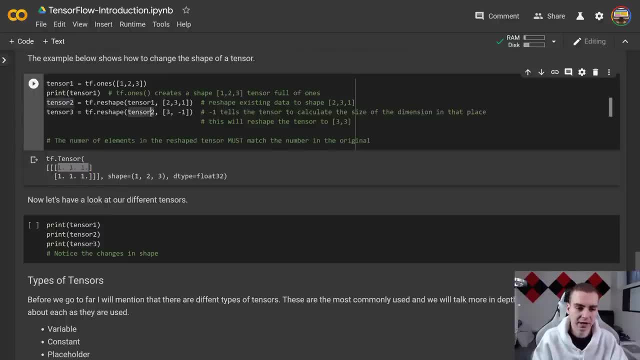 the shape we just defined. Now we have six elements inside of here, So there must be a way that we can reshape this data to have six elements, but in a different shape. In fact, what we can do is reshape this into a 231 shape, where we're going to have two. 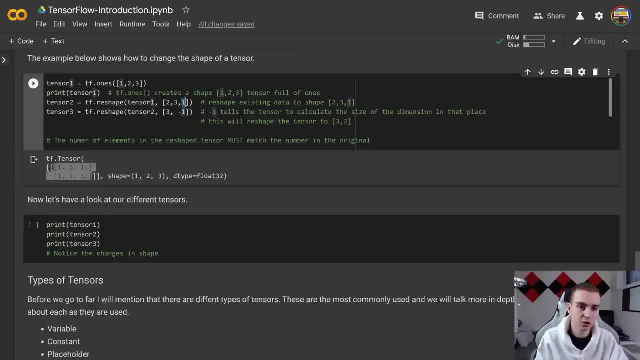 lists, right, we're going to have three inside of those, And then inside of each of those we're going to have one element. So let's have a look at that one. So let's have a look at tensor two. actually, what? 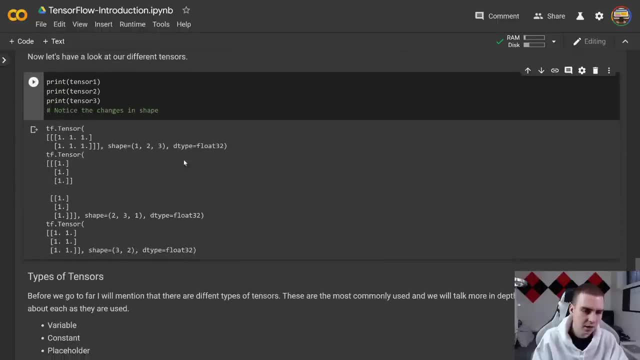 am I doing? we print out. we can print all of them here, So let's just print them and have a look at them. So when we look at tensor one, we saw this was a shape. And now we look at this tensor two, And we can see that we have two lists right Inside of each of those. 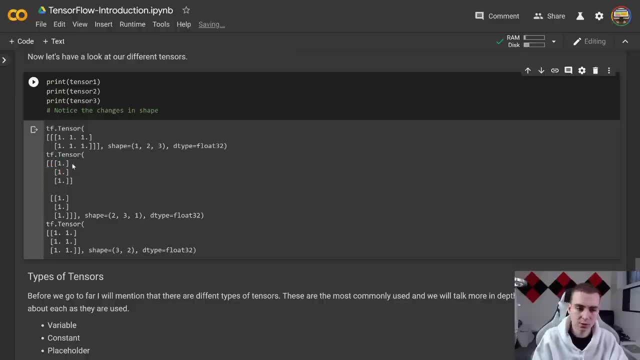 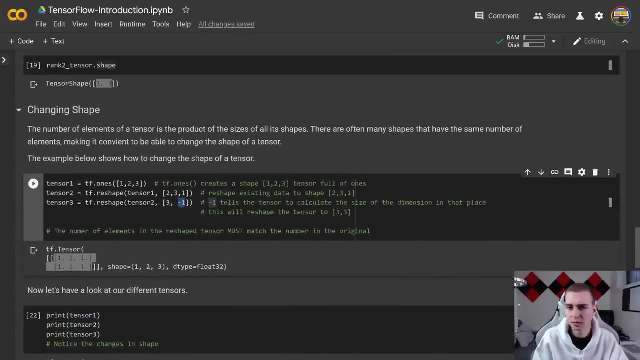 lists. we have three lists And inside of each of those lists we have one element. Now, finally, our tensor three is a shape of three: negative one- well, what is negative one when we put negative one here? what this does? 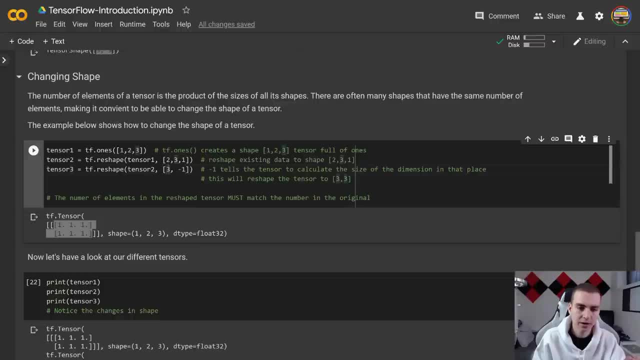 for what this number actually needs to be. So if we define an initial shape of three, what this does is say, okay, we're gonna have three lists, that's our first level, And then we need to figure out based on how many elements we have in this reshape, which is the method. 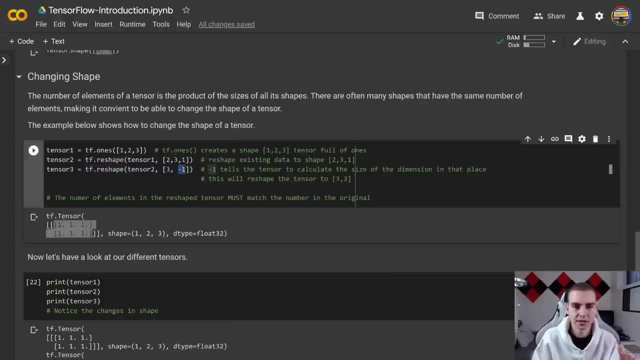 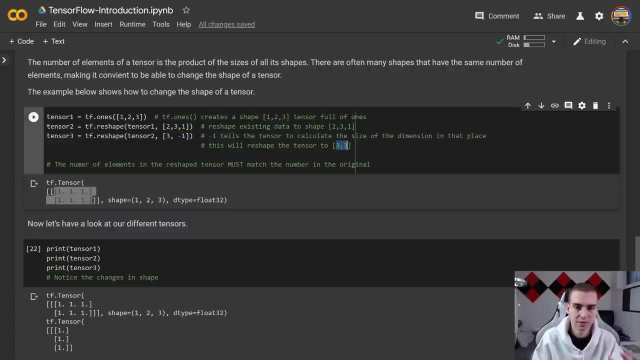 we're using- which I didn't even talk about, which we'll go into a second- what this next dimension should be. Now, obviously, this is going to need to be three. So three, three, right, because we're gonna have three less inside of each of those lists we need to have. 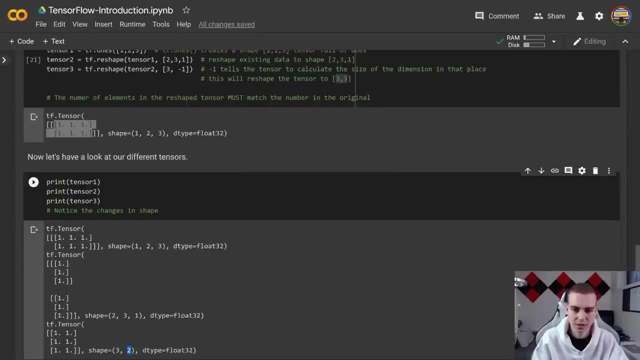 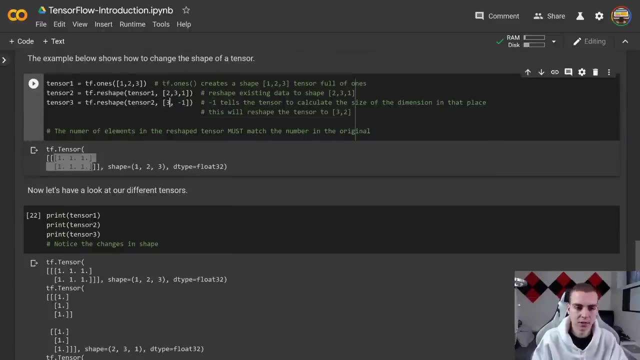 are actually. is that correct? Let's see if that's even the shape Two, my bad. So this actually needs to change to three two. I don't know why I wrote three, three there, But you get the point right. So what this does? we have three lists. we. 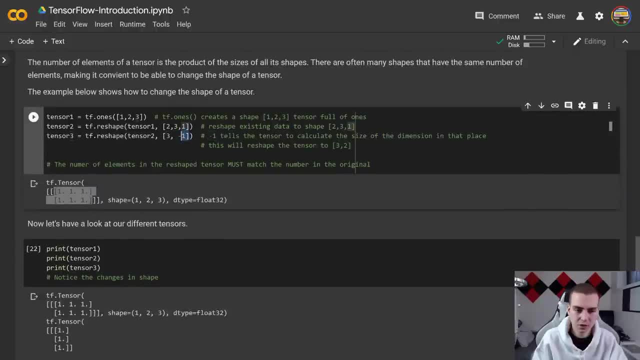 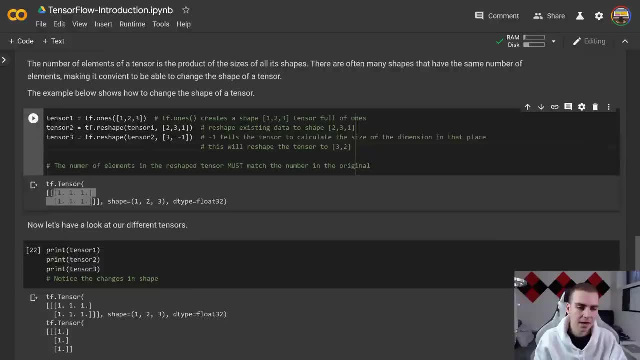 have six elements, this number obviously needs to be two, because, well, three times two is going to give us six. And that is essentially how you can determine how many elements are actually in a tensor: by just looking at its shape. Now, this is the reshape method, where 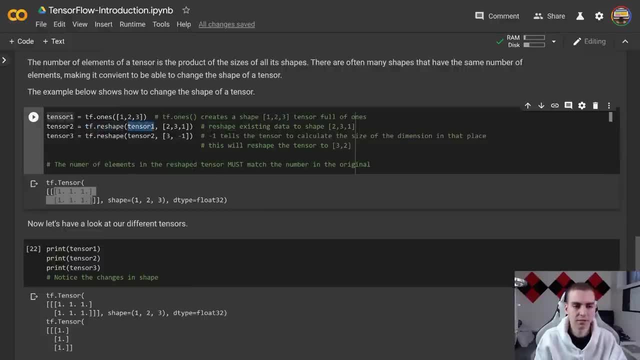 all we need to do is called tf dot reshape- give the tensor and give the shape we want to change it to, So long as that's a valid shape. And when we multiply all of those, all of the numbers in here, it's equal to the number of elements in this tensor. that 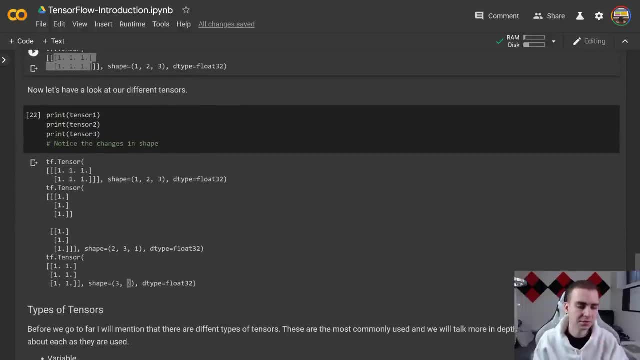 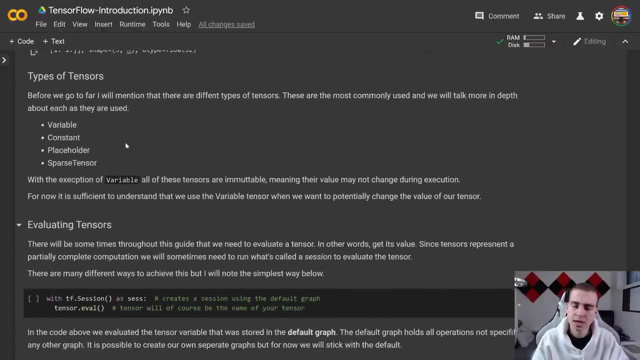 will reshape it for us and give us that new shaped data. This is very useful. We'll use this actually a lot as we go through TensorFlow, So make sure you're kind of familiar with how that works. Alright, so now we're moving on to types of tensors. So there is a bunch. 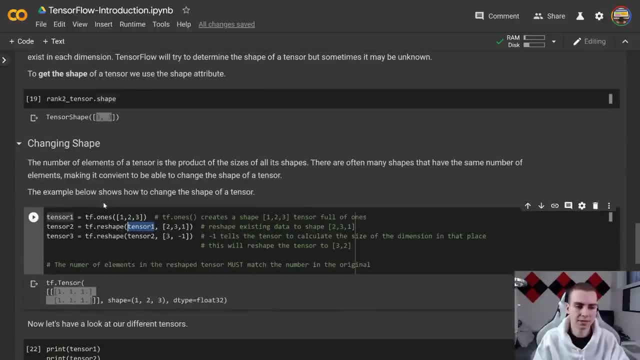 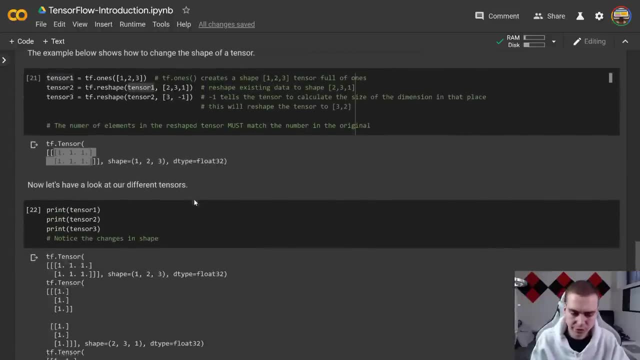 of different types of tensors that we can use. So far the only one we've looked at is variable. So we've created tf, dot variables and kind of just hard coded our own tensors. We're not really going to do that very much. 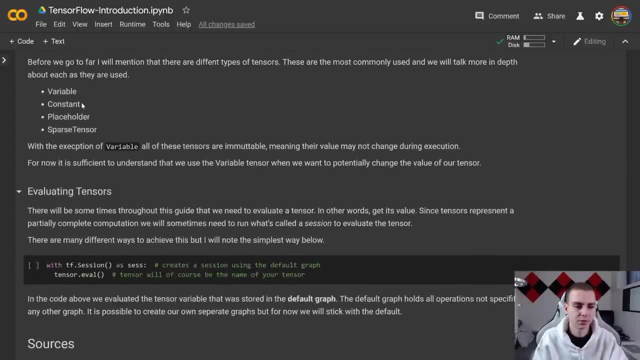 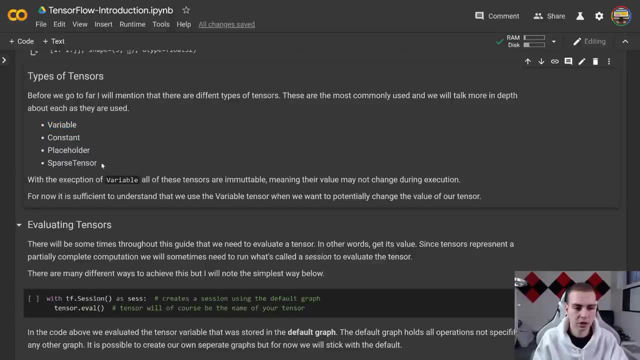 But just for that example. so we have these different types. we have constant, placeholder, sparse, tensor, variable, and there's actually a few other ones as well. Now, we're not going to really talk about these two that much, although constant and variable are important. 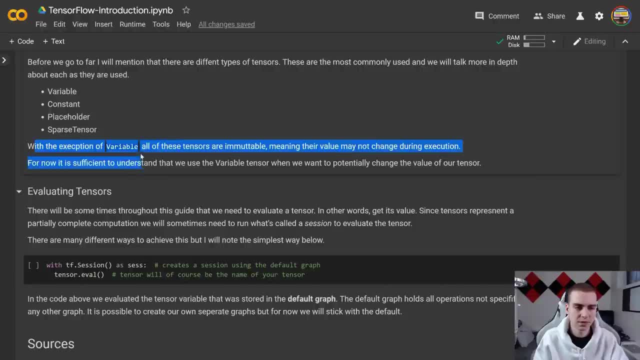 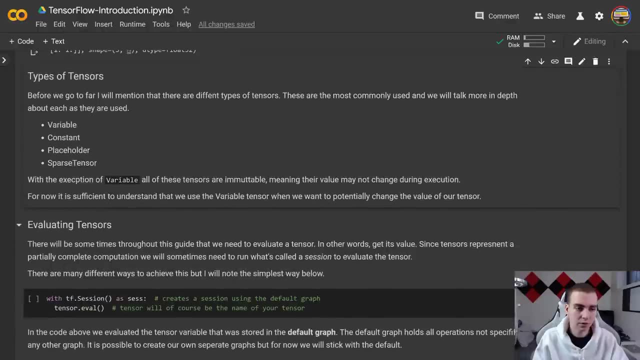 to understand the difference between. So we can read this as, with the exception of variable, all of these tensors are immutable, meaning their value may not change during execution. So essentially all of these, when we create a tensor, mean we have some constant value. 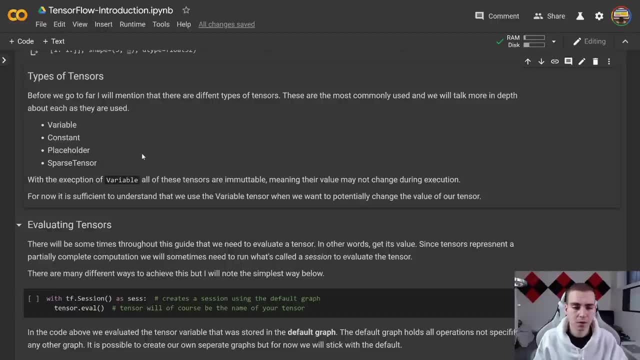 which means that whatever we've defined here, it's not going to change, whereas the variable tensor could change. So that's just something to keep in mind. when we use variable, that's because we think we might need to change the value of that tensor later on, Whereas if 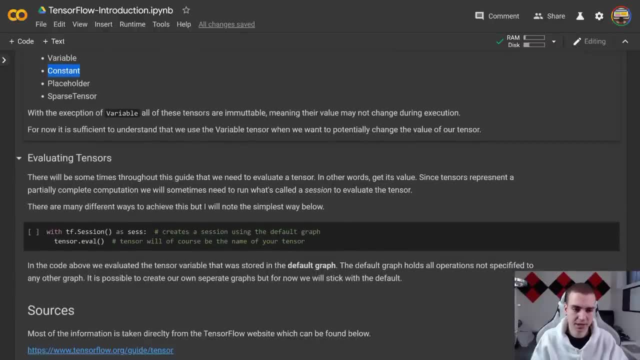 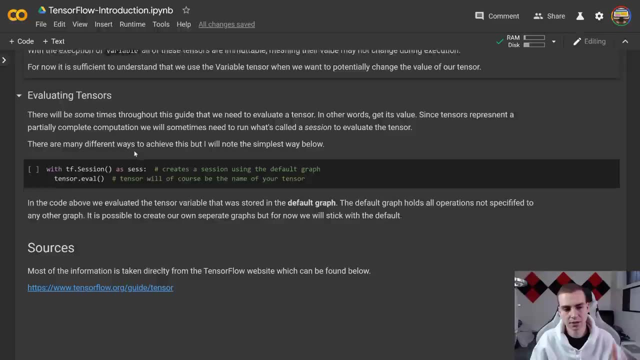 we're using a constant value tensor. we cannot change it. So that's just something to keep in mind. we can obviously copy it, but we can't change it. Okay so, evaluating tensors. we're almost at the end of the section, I know, and then we'll get into some more kind. 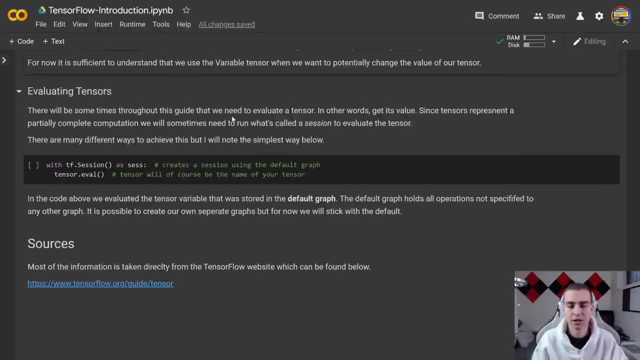 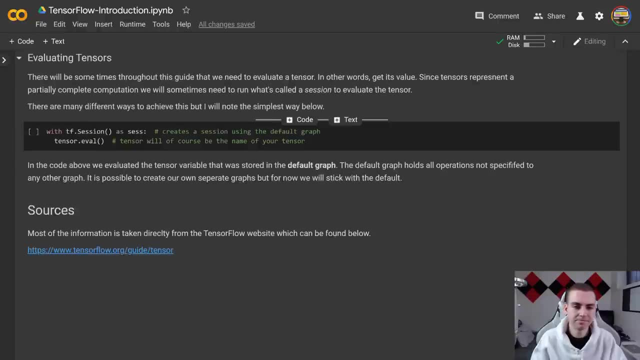 of deeper code, So there will be some times throughout this guide we need to evaluate a tense, of course. So what we need to do to evaluate a tensor is create a session. Now, this isn't really like we're not going to do this that much, But I just figured I'd mention it to make 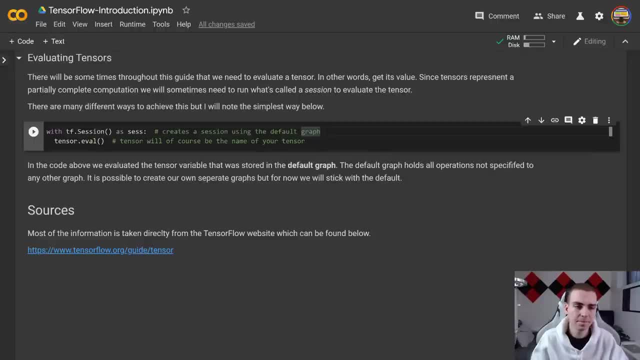 sure that you guys are aware of what I'm doing If I start kind of typing this later on. essentially, sometimes we have some tensor object And throughout our code we actually need to evaluate it to be able to do something else. So to do that, all we need to do is literally just 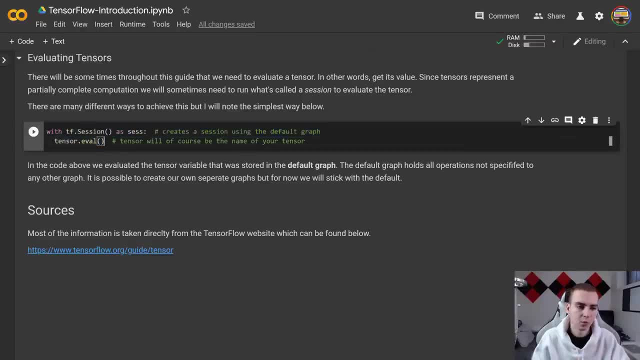 use this kind of default template, a block of code, what we say with tf, dot session as some kind of session, It doesn't really matter what we put here. then we can just do whatever the tensor name is, dot, eval And calling that. we'll actually have TensorFlow, just figure out what it needs. 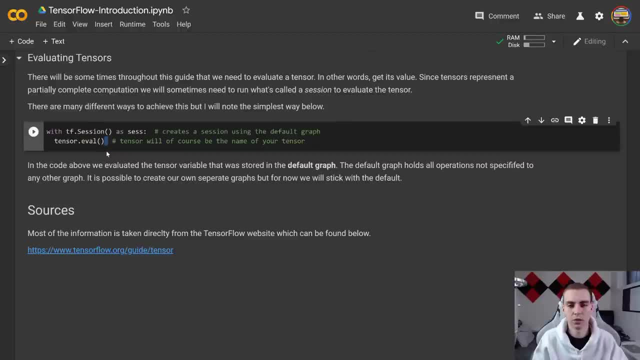 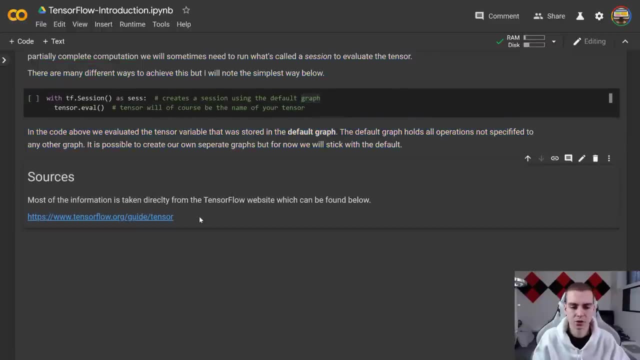 to do to find the value of this tensor. it will evaluate it and then it will allow us to actually use that value. So I've put this in here. you guys can obviously read through this if you want to understand some more in depth on how that works And the source for. 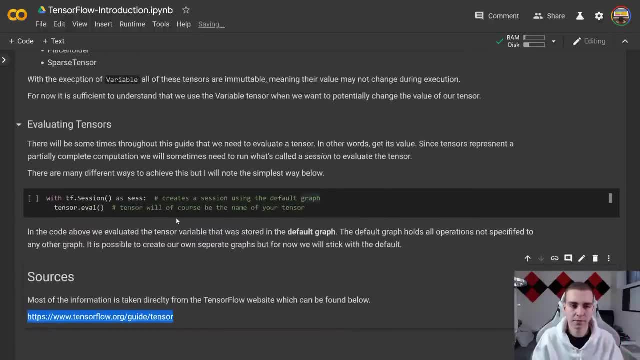 this is straight from the TensorFlow website. a lot of this is straight up copied from there, And I've just kind of added my own spin to it and made it a little bit easier to understand. Okay, so we've done all that, So we're going to go ahead and go ahead, and go ahead, and 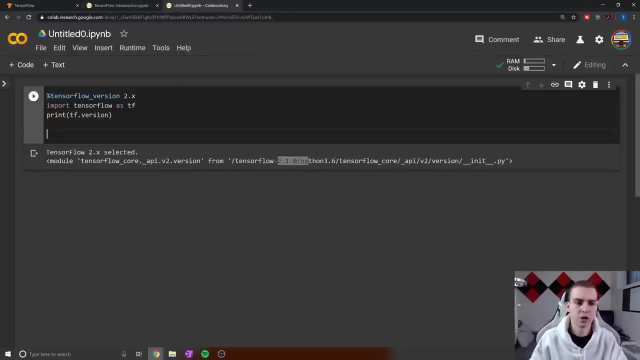 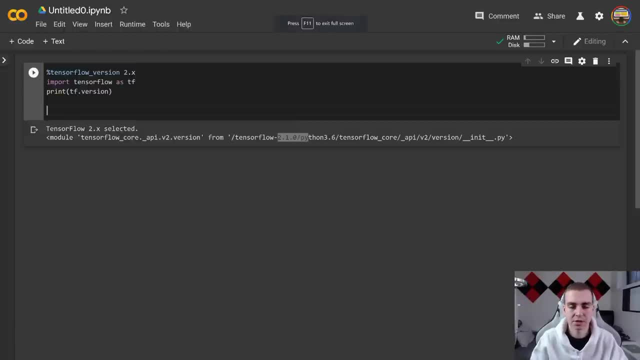 sure that everyone's kind of on the same page, and then we'll move on to actually talking about some simple learning algorithms. So I want to create a tensor that we can kind of mess with and reshape. So what I'm going to do is just say t equals, and we'll say: 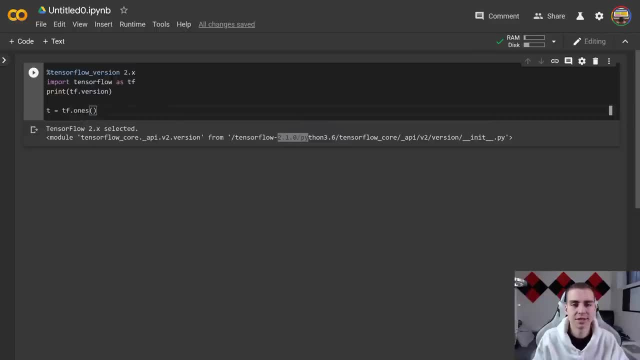 tf dot ones. Now, what tf dot ones does is just create again all of the values to be ones that we're going to have and whatever shape. Now we can also do zeros, and zeros is just gonna give us a bunch of zeros And let's create some like crazy shape and just 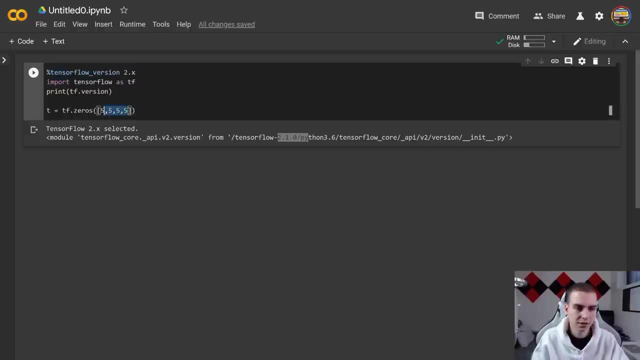 visualize it. let's do like a five by five by five. So obviously, if we want to figure out how many elements are going to be in here, we need to multiply this value. So I believe this is going to be 625, because that should be five to the power of four. So five times five times five. 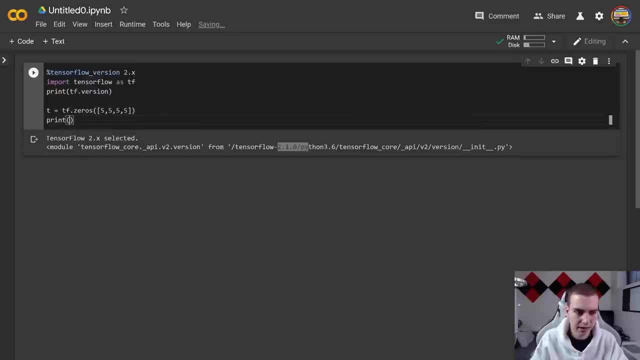 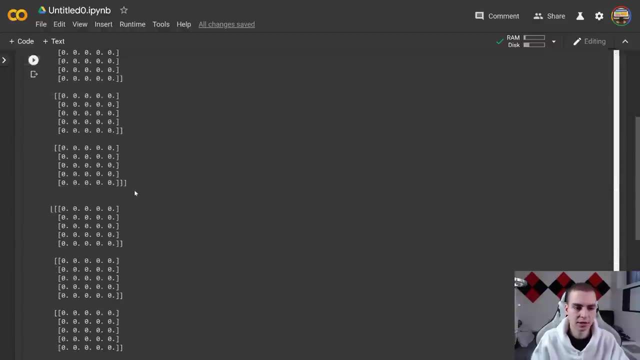 times five And let's actually print T and have a look at that and see what this is. So we run this now And you can see this is the output we're getting. So obviously this is a pretty crazy looking tensor, but you get the point right and it tells us the shape. 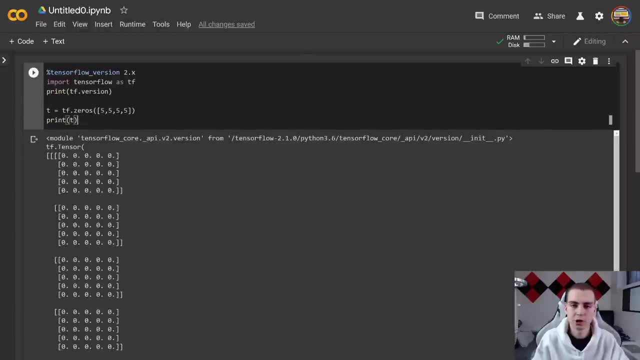 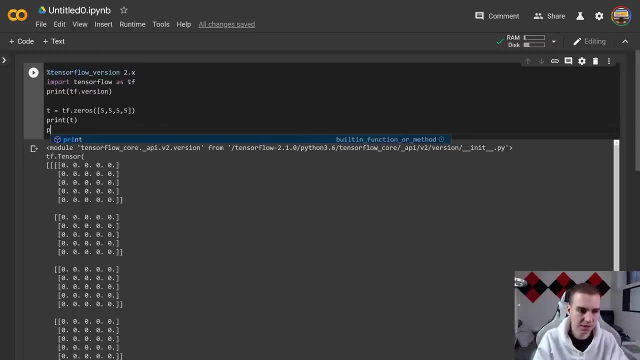 is 55555.. Now watch what happens when I reshape this tensor. So if I want to take all of these elements and flatten them out, what I could do is simply say we'll say t equals t, f, dot reshape. like that, And we'll reshape the tensor T to just the shape 625.. Now if we 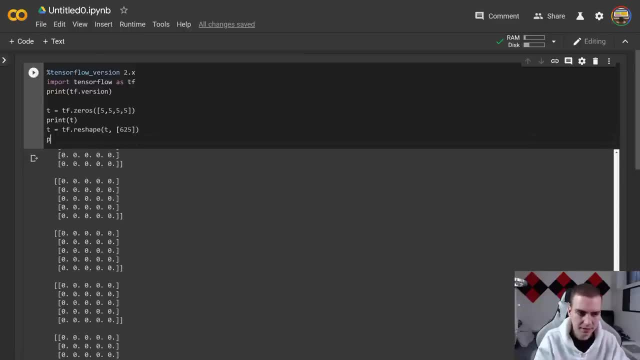 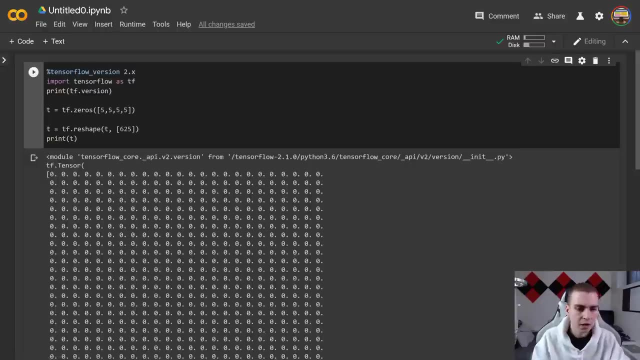 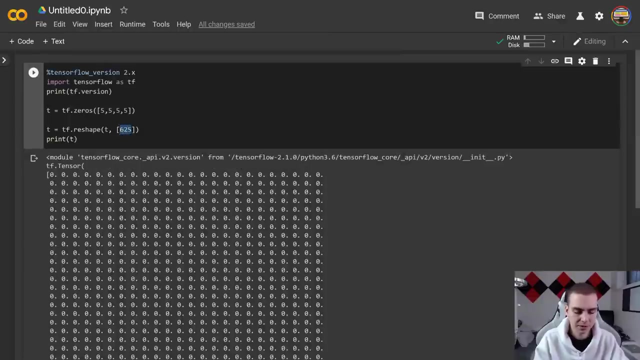 do this and we run here. oops, I got to print T at the bottom after we've done that. if I could spell the print statement correctly, you can see that now we just get this massive list that just has 625 zeros. And again, if we wanted to reshape this to something like 125, and. 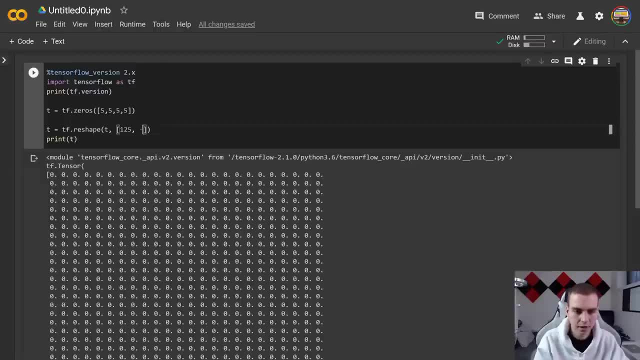 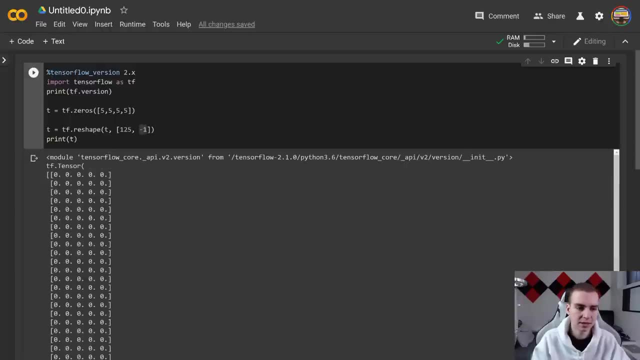 maybe we weren't that good at math and couldn't figure out that this last value should be five. we can put a negative one. this would mean that TensorFlow would infer now what the shape needs to be, And now, when we look at it, we can see that we're what we're going. 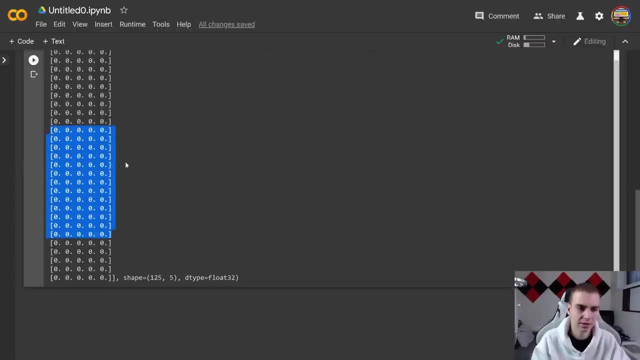 to get is well, just simply five kind of sets of these, I don't know matrices, whatever you want to call them. in our shape Is 125.. Five, So that is essentially how that works. So that's how we reshape, That's how 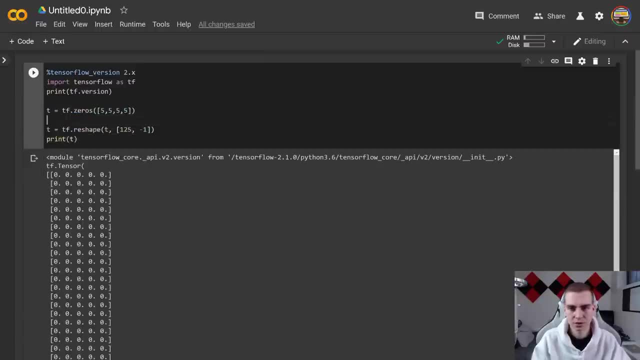 we kind of deal with tensors, create variables, how that works in terms of sessions and graphs, And hopefully with that that gives you enough of an understanding of tensors, of shapes, of ranks, of value, so that when we move into the next part of the tutorial where we're actually 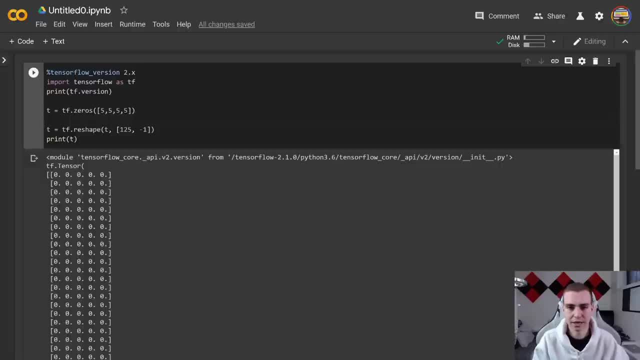 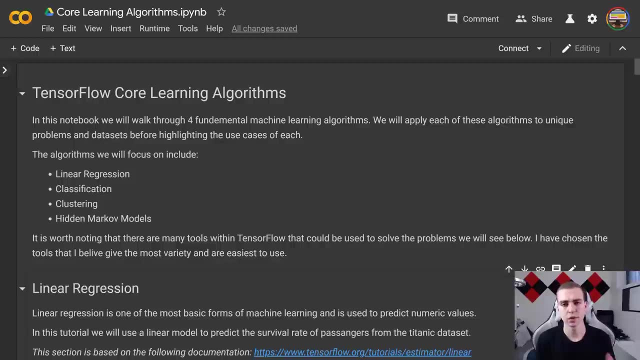 writing code, and I promise we're gonna be writing some more advanced code. you'll understand how that works. So, with that being said, let's get into the next section. So welcome to module three of this course. Now what we're going to be doing in this module. 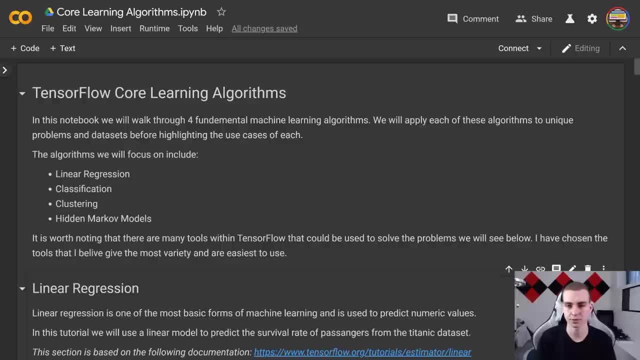 is learning the core machine learning algorithms that come with TensorFlow. Now, these algorithms are not specific to TensorFlow but they are used within there And we'll use some tools from TensorFlow to kind of implement them. But essentially these are the building blocks before moving on to things like neural networks and more advanced machine learning techniques. 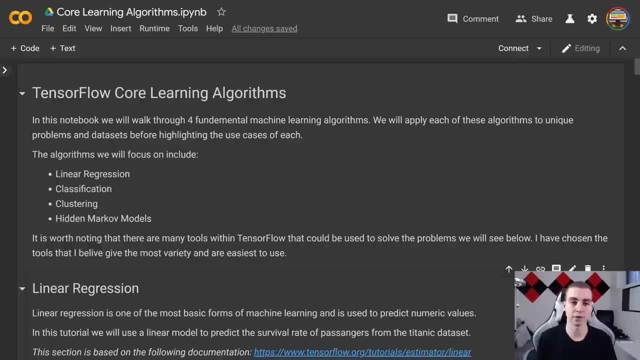 you really need to understand how these work, because they're kind of used in a lot of different techniques and combined together, And what I'm about to show you is actually very powerful If you use it in the right way: a lot of what machine learning actually is and a lot of. 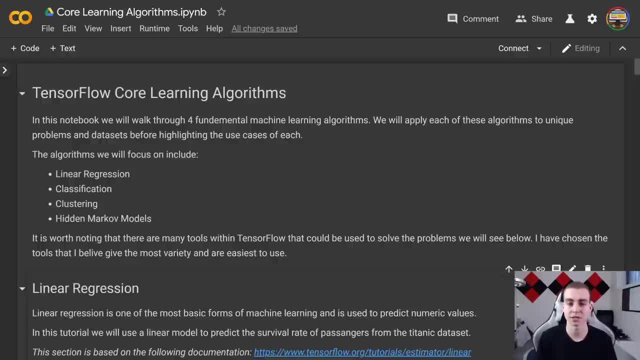 machine learning, algorithms and implementations, and businesses and applications and stuff like that actually just use pretty basic models, because these models are capable of actually doing- you know- very powerful things And when you're not dealing with anything that's crazy complicated, you just need some basic machine learning, some basic classification. 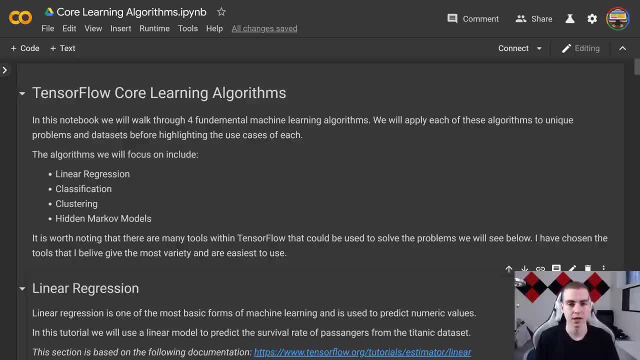 you can use these kind of fundamental core learning algorithms. Now, the first one we're going to go through is linear regression, but we will cover classification and clustering and hidden Markov models And those are kind of going to give us a good spread of the different. 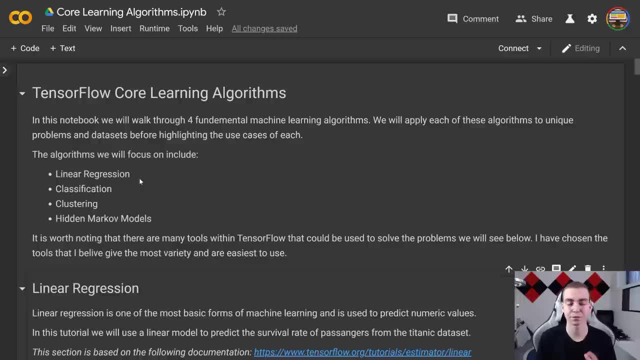 core algorithms. Now there is a ton, ton- like 1000s- of different machine learning algorithms. These are kind of the main categories that you'll cover, But within these categories there is more specific algorithms that you can get into. I just feel like I need to mention 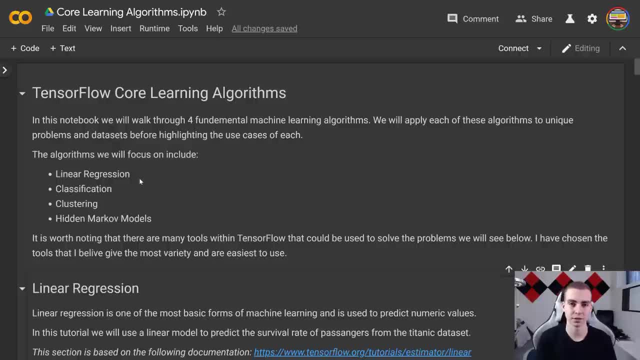 that, because I know a lot of you will have maybe seen some different ways of doing things in this course, might show you, you know, a different perspective on that. So let me just quickly talk about how I'm going to go through this. It's very similar to before. I have this. 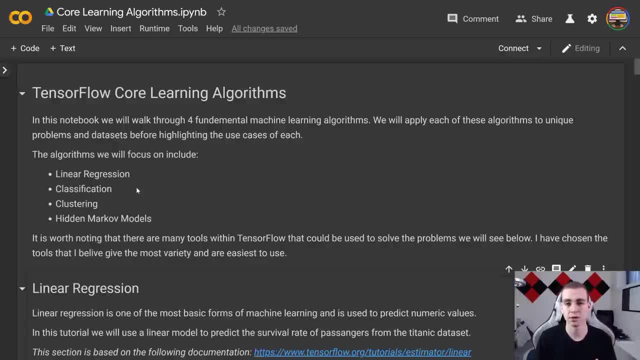 notebook, as I've kind of talked about. there is a link in the description. I would recommend that you guys hit that and follow along with what I'm doing and read through the notebook. But I will just be going through the notebook And then occasionally what I will actually. 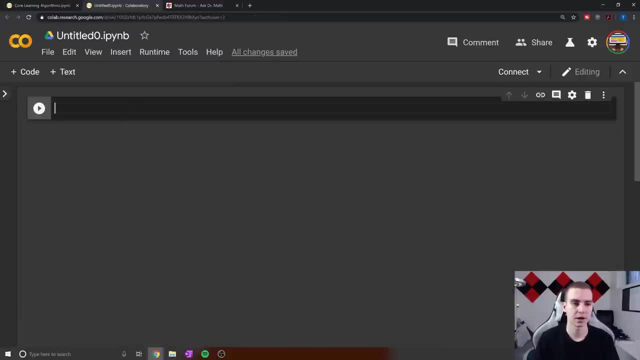 do- oops, I need to open this up here- is go to this kind of untitled tab I have here and write some code in here, Because most of what I'm going to do is just copy code over into here So we can see it all in kind of one block, and then we'll be good to go And the 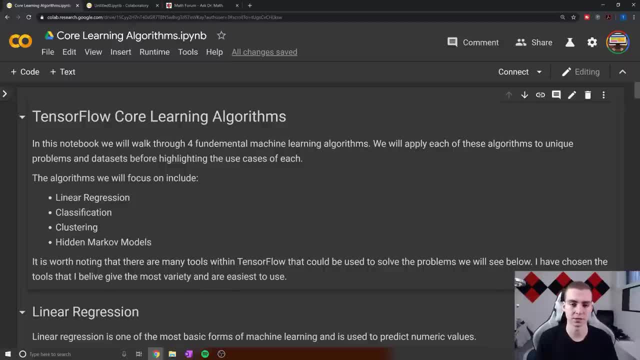 last note before we really get into it, and I'm sorry I'm talking a lot, but it is important to make you guys aware of this. You're going to see that we use a lot of complicated syntax throughout this kind of series and 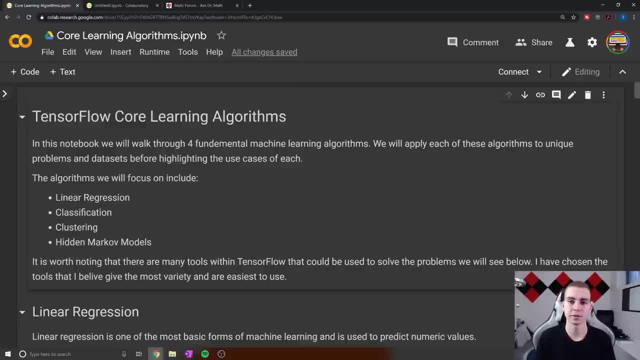 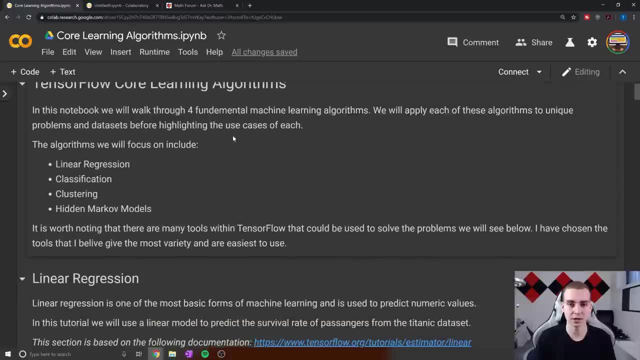 the rest of the course in general. I just want to make it extremely clear that you should not have to memorize, or even feel obligated to memorize, any of the syntax that you see. everything that you see here, I personally don't even have memorized. there's a lot of 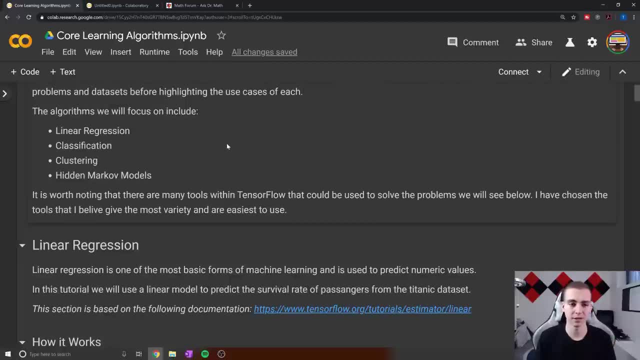 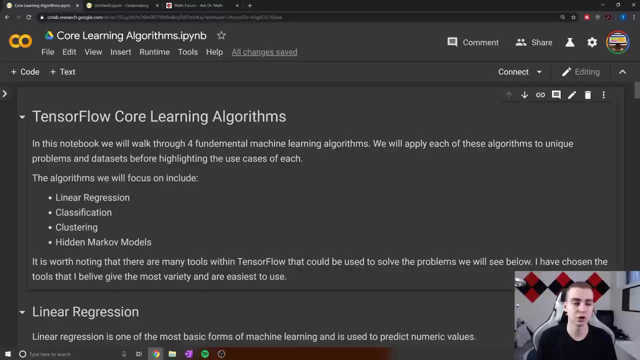 what's in here that I can't just come up with on the top of my head, when we're dealing with kind of a library and module so big that, like TensorFlow, it's hard to memorize all those different components. So just make sure you understand what's happening, But you're 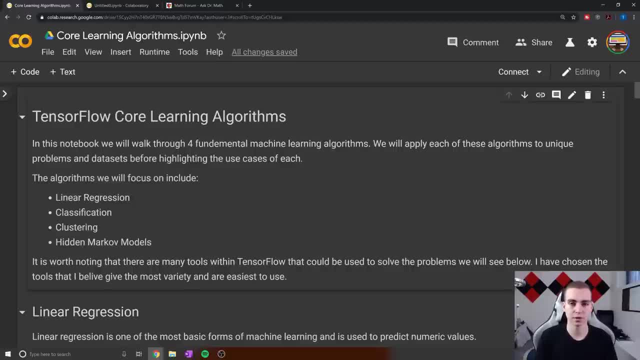 right, you don't need to memorize it. if you're ever going to need to use any of these tools, you're going to look them up, you're going to see what it is. you're like: Okay, I've used this before, you're going to understand it, And then you can go ahead and you know. 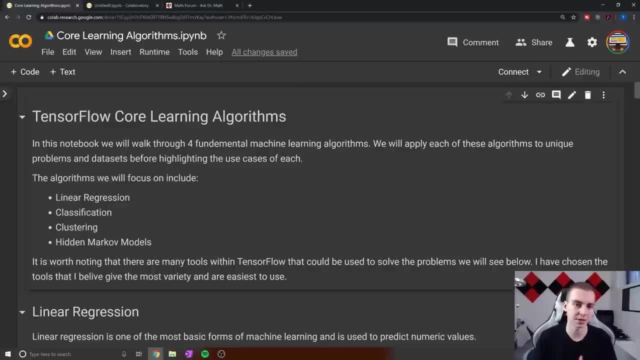 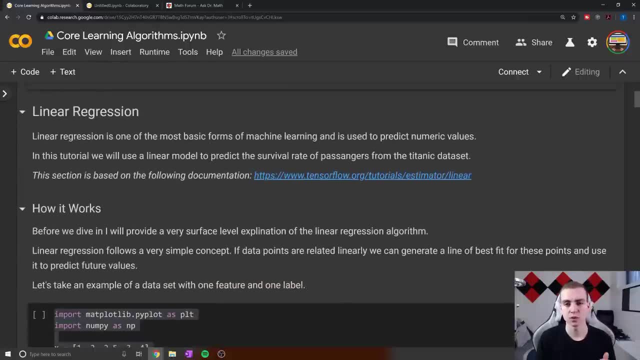 copy that code in and use it in whatever way you need to. you don't need to memorize anything that we do. All right, so let's go ahead and get started with linear regression. So what is linear regression? What's one of those basic forms of machine learning? And essentially, 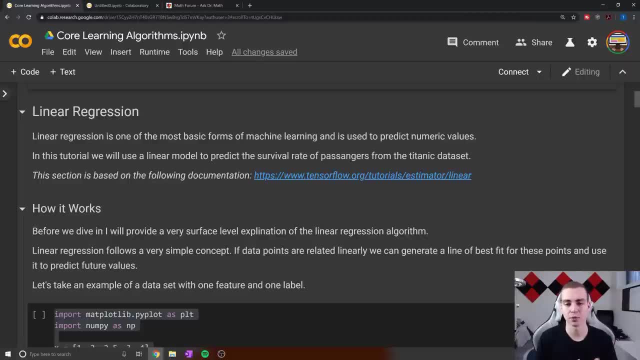 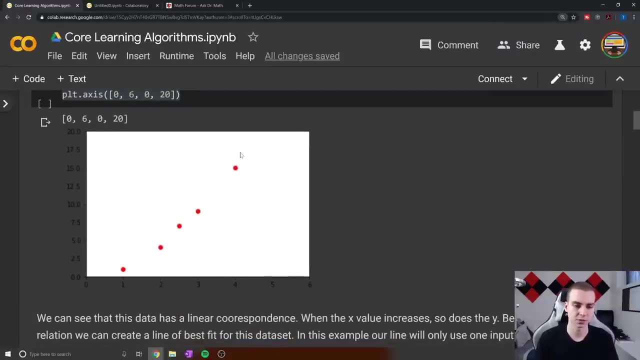 what we try to do is have a linear correspondence between data points. So I'm just going to scroll down here. do a good example. So what I've done is used matplotlibcom And I'm going to use matplotlib just to plot a little graph here So we can see this one right here. 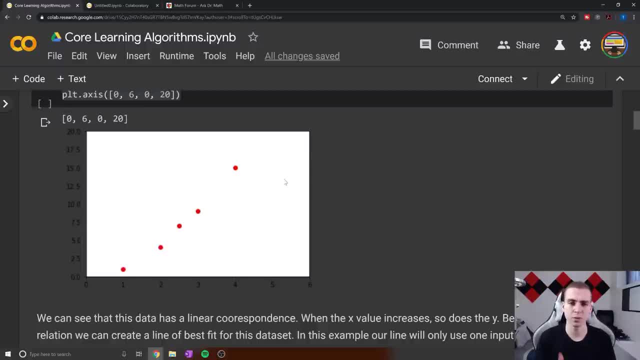 And essentially this is kind of our data set, this what we'll call our data set. what we want to do is use linear regression to come up with a model that can give us some good predictions for our data points. So in this instance, maybe what we want to do is given. 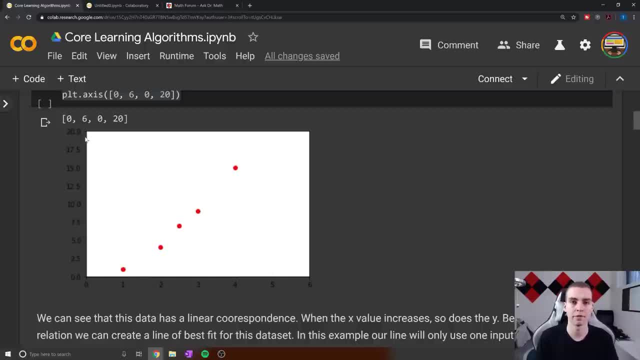 some x value for a data point. we want to predict the y value. Now in this case we can see there is kind of some correspondence linearly for these data points. Now what that means is we can draw something called a line of best fit. 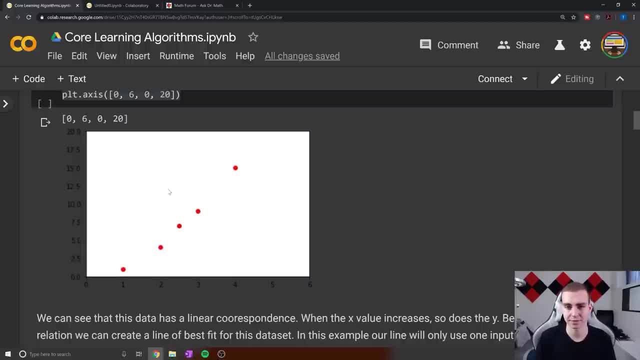 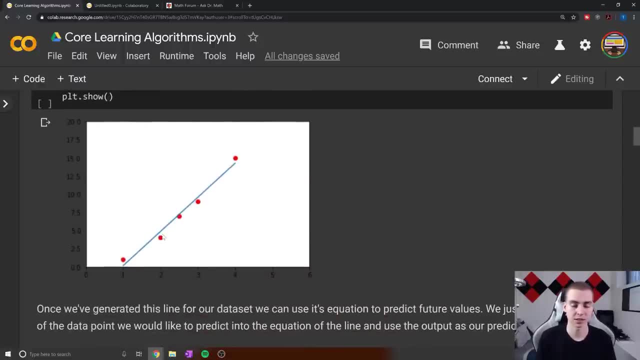 through these data points that can kind of accurately classify them, if that makes any sense. So I'm going to scroll down here and look at what our line of best fit for this data set actually is. we can see this blue line. it pretty much- I mean it is the perfect line. 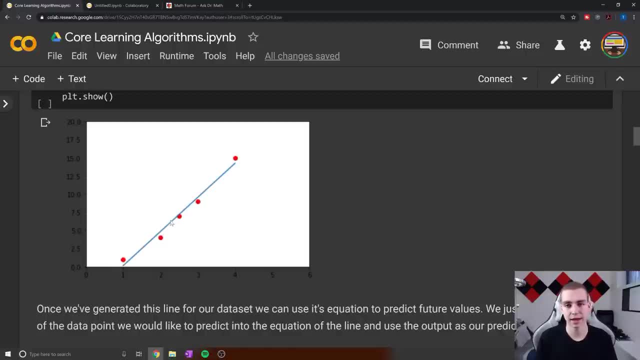 of best fit for this data set And using this line we can actually predict future values in our data set. So, essentially, linear regression is used when you have data points that correlate in kind of a linear fashion. Now, this is a very basic example, because we're doing 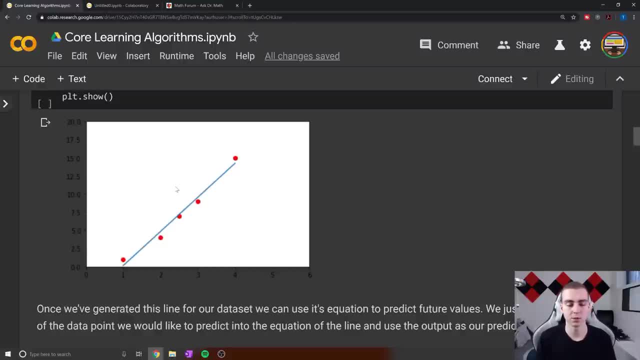 this in two dimensions, with x and y, But oftentimes what you'll have is you'll have data points that have you know eight or nine kind of input values. So that gives us, you know, a nine dimensional kind of data set, And what we'll do is predict one of the 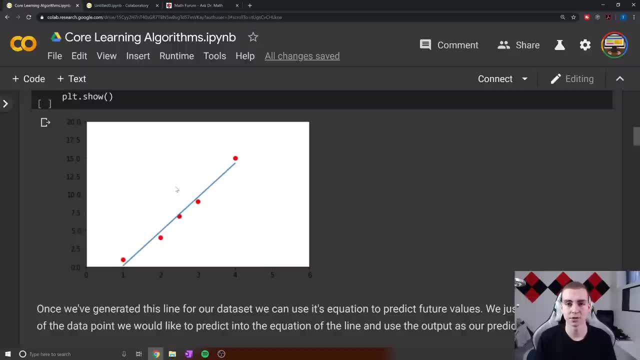 different values. So in the instance where we were talking about students before, maybe we have a student's what is it midterm grade and their second midterm grade and then we want to predict their final grade. what we can do is use linear regression to do that. 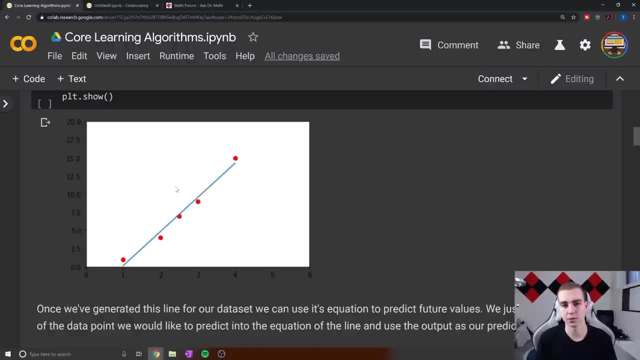 where our kind of input values are going to be the two midterm grades and the output value is going to be that final grade that we're looking to predict. So if we were to plot that, we would plot that on a three dimensional graph and we would draw a three dimensional line that would represent 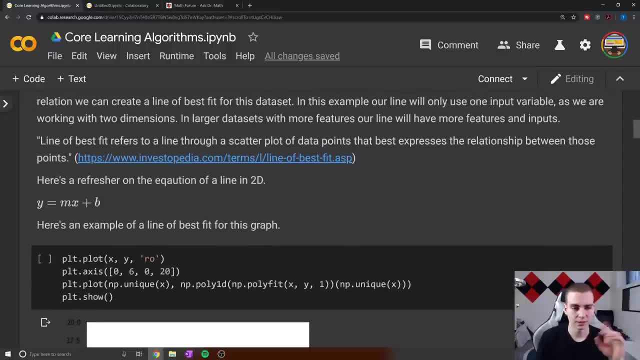 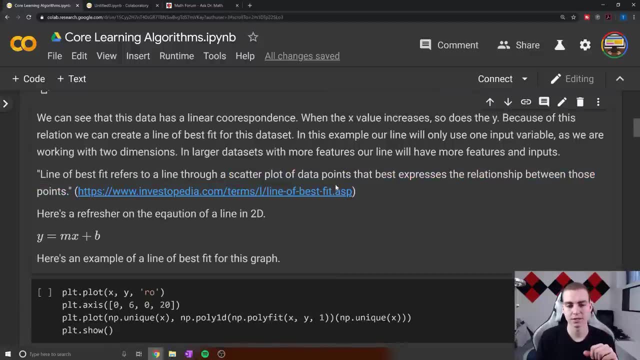 the line of best fit for that data set. Now, for any of you that don't know what line of best fit stands for, it says light, or this is just the definition I got from this website here: line of best fit refers to a line, through a scatterplot of data points, that best expresses 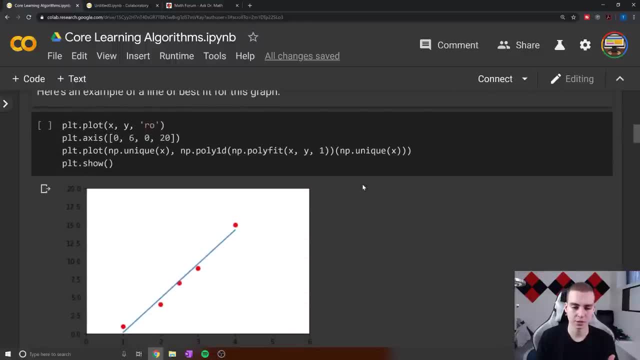 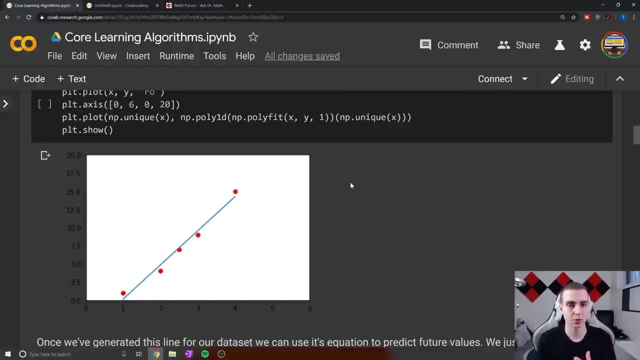 the relationship between those points. So exactly what I've kind of been trying to explain: When we have data that correlates linearly- and I always butcher that word- we're going to use the word. what we can do is draw a line through it And then we can use that. 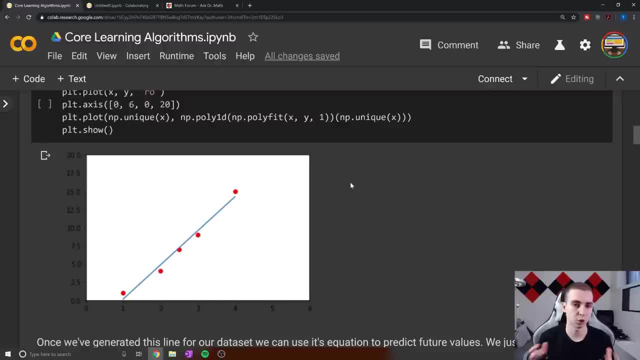 line to predict new data points, Because if that line is good, it's a good line of best fit for the data set. then hopefully we would assume that we can just, you know, pick some point, find where it would be on that line, And that'll be kind of our predicted value. 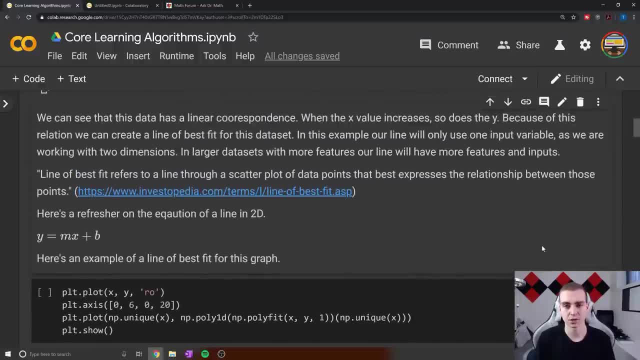 So I'm going to go into an example now where I start drawing and going into a little bit of math So we understand how this works on a deeper level. But that should give you a surface level understanding. So actually I'll leave this up because I was messing with. 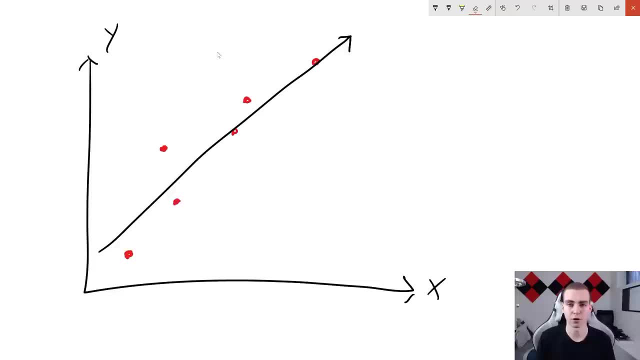 this beforehand. This is kind of a data set that I've drawn on here. So we have our x and we have our y and we have our line of best fit. Now what I want to do is I want to use this line. 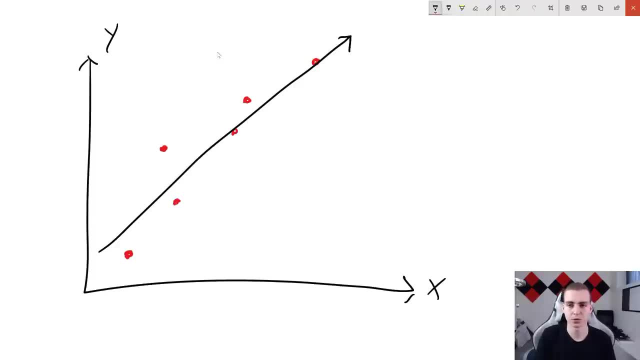 of best fit to predict a new data point. So all these red data points are ones that we've trained our model with their information, that we gave to the model so that it could create this line of best fit, Because essentially, all linear regression really does is look: 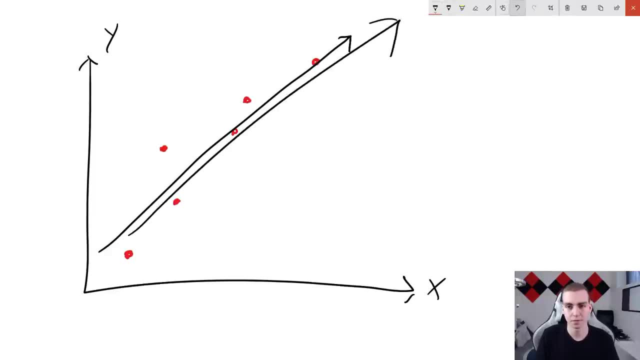 at all of these data points and create a line of best fit for them. That's all it does. It's pretty, I don't know the word for it. it's pretty easy to actually do this. this algorithm is not that complicated, it's not that advanced, And that's. 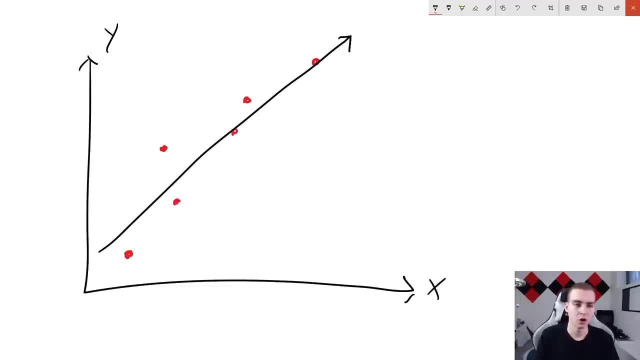 why we start with it here, because it just makes sense to explain. So I hope that a lot of you would know. in two dimensions a line can be defined as follows: So with the equation y equals MX plus B. Now B stands for the y intercept, which means somewhere on this line. 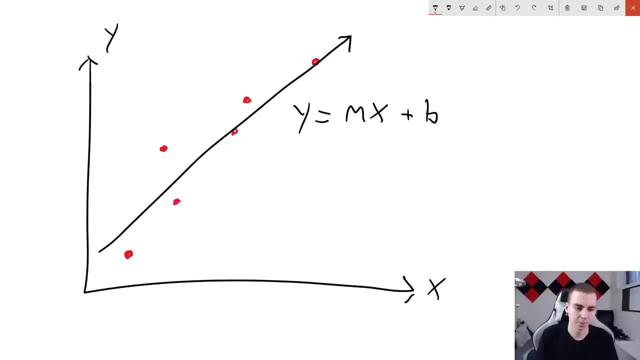 So essentially where the line starts. So in this instance our B value is going to be right here, So this is going to be B because that is the y intercept. So we could say that that's like maybe you know, we go on, we'll do this, we'll say this is like 123, we might. 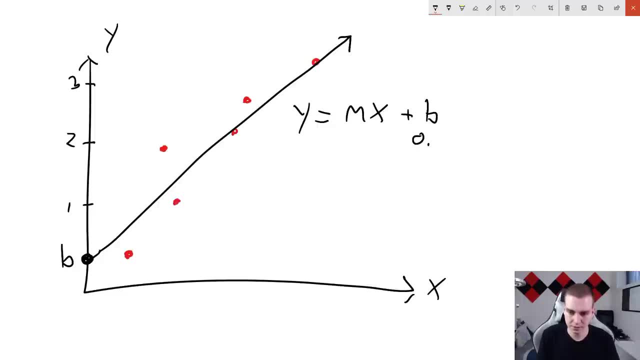 say, B is something like 0.4.. Right, So I could just pencil that into 0.4.. And then what is m, x and y? Well, x and y stand for the coordinates of this data point. So this would have you. 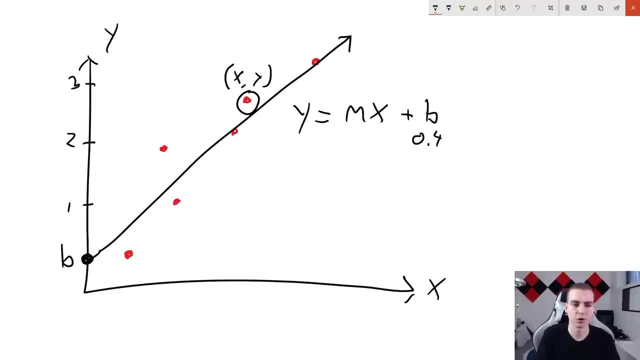 know some x- y value. In this case we might call it. you know, something like what do we want to say to 2.7, that might be the value of this data point. So that's our x and y. 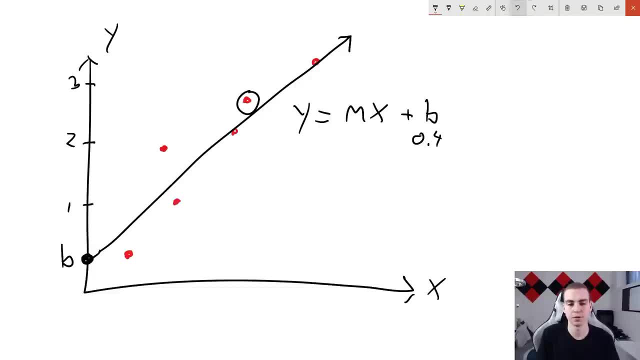 And then our m stands for the slope, which is probably the most important part. Now. slope simply defines the steepness of this line of best fit that we've done here. Now, the way we calculate slope is using rise over run. Now, rise over run essentially just means how much we went. 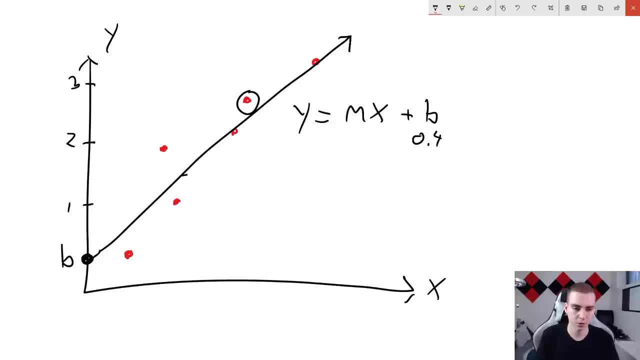 up versus how much we went across. So if you want to calculate the slope of a line, what you can actually do is just draw a triangle, So a right angle triangle, anywhere on the line. So just pick two data points And what you can do is calculate this distance and 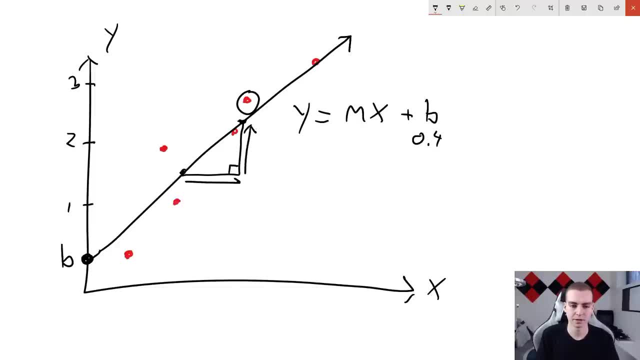 this distance And then you can simply divide the distance up by the distance across and that gives you the slope. I'm not going to go too far into slope because I feel like you guys probably understand what that is, But let's just pick some values for this line, And I want to actually 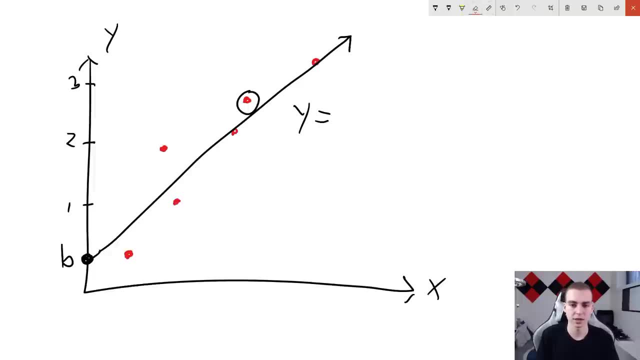 show you some real examples of math and how we're going to do this. So let's say that our linear regression algorithm, you know, comes up with this line. I'm not going to discuss really how it does that, although it just pretty much looks at all these data. 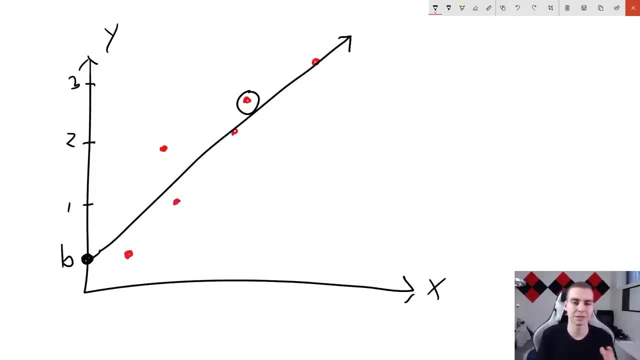 points and finds a line that you know goes, it splits these data points evenly. So essentially, you want to be as close to every data point as possible And you want to have as many data points. you want to have like the same amount of data points on the left side and 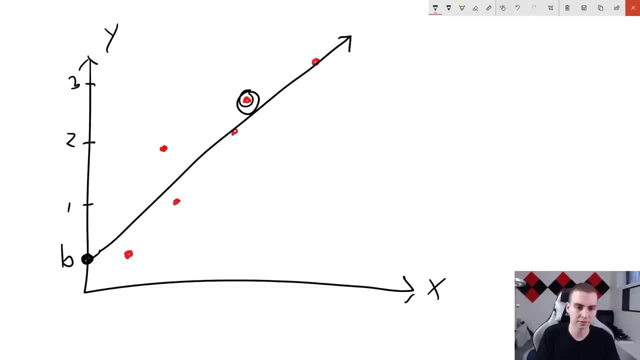 the right side of the line. So in this example we have, you know, a data point on the left, a data Gods left- we have what? two that are pretty much on the line, And then we have two that are on the right. So this is a pretty good line of best fit, because all of the 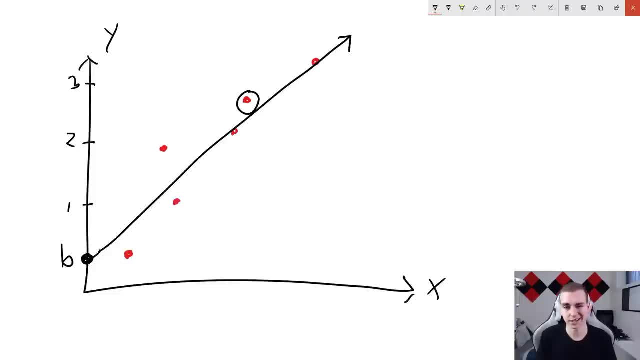 points are very close to the line And they split them evenly. So that's kind of how you come up with the line of best fit. So let's say that the equation for this line is something like Y equals- let's just give it 1.5 and x plus, and let's say that value is just 0.5, to make it easy. So this: 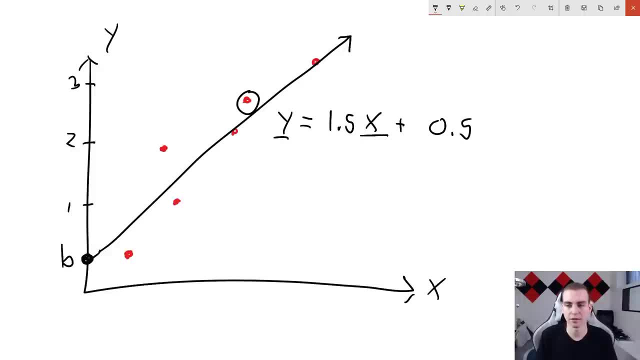 is going to be the equation of our line. Now notice that x and y don't have a value. That's because we need to give the value to come up with one of the other ones. So what we can do is we can say if we have either the y value or we have the x value of some point. 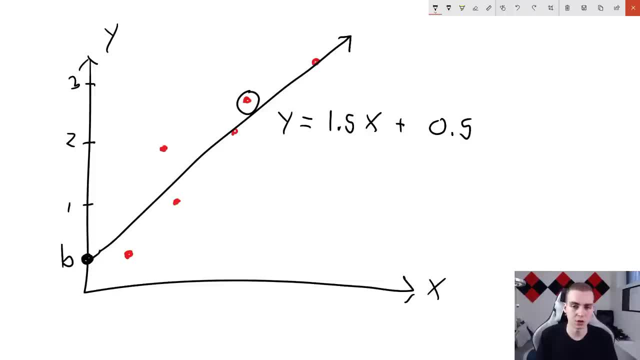 and we want to figure out. you know where it is on the line. what we can do is just feed one in, do a calculation, and that will actually give us the other value. So in this instance, let's say that you know, I'm trying to predict something and I'm given the that, the fact 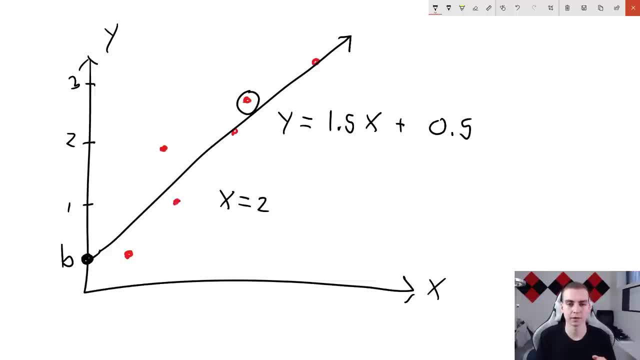 that x equals two. I know that x equals two and I want to figure out what y would be if x equals two. well, I can use this line to do so. So what I would do is I'm going to say: y equals 1.5 times two plus 0.5.. Now, all of you quick math majors out there, give. 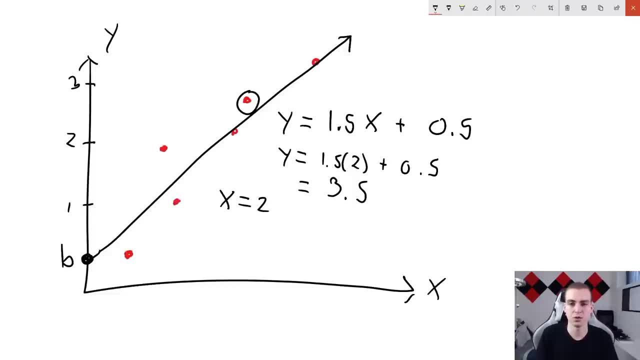 me the value of 3.5.. Which means that if I'm going to say x equals 0.5, I can use this line to do that. So what if x was at two? then I would have my data point as a prediction here on this line. And 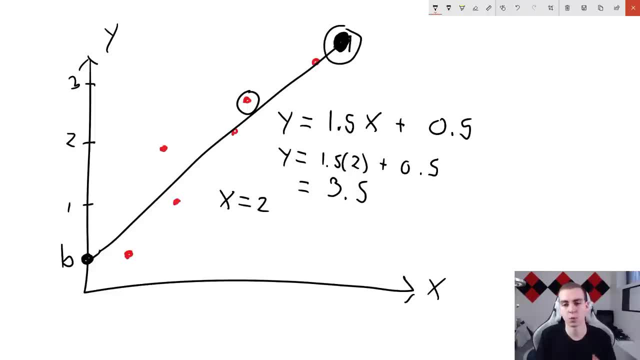 I would say: Okay. so if you're telling me x is two, my prediction is that y is going to be equal to 3.5.. Because, given the line of best fit for this data set, that's where this point will lie, on that line. So I hope that makes sense. You can actually do this. 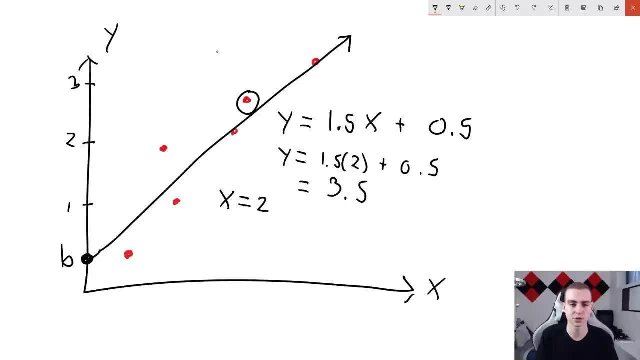 the reverse way as well. So if I'm just given some y values to say I know that you know my y value is at like 2.7, or something I can plug that in, just rearrange the numbers in this equation and then solve for x. Now, obviously this is a very basic example, because 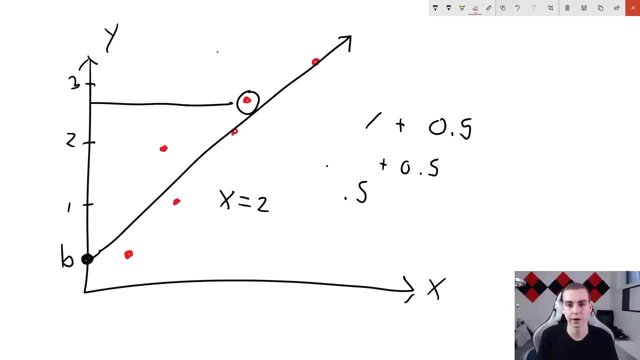 we're just doing all of this in two dimensions, But you can do this in higher dimensions as well. So actually, most times, what's going to end up happening is you're going to have, you know, like eight or nine input variables and then you're gonna have one output variable. 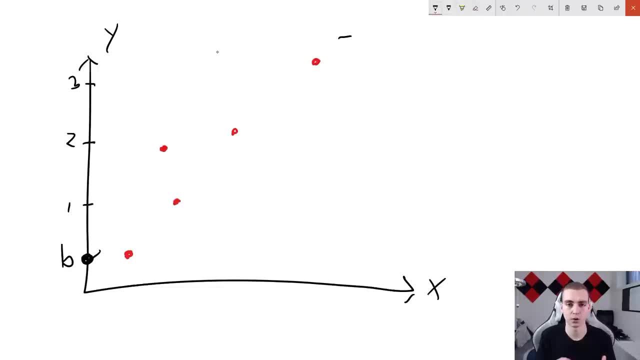 that you're predicting. Now, so long as our data points are correlated linearly in three dimensions, we can still do this. So I'm going to attempt to show you this actually in three dimensions, just to hopefully clear some things up, because it is important to kind of get. 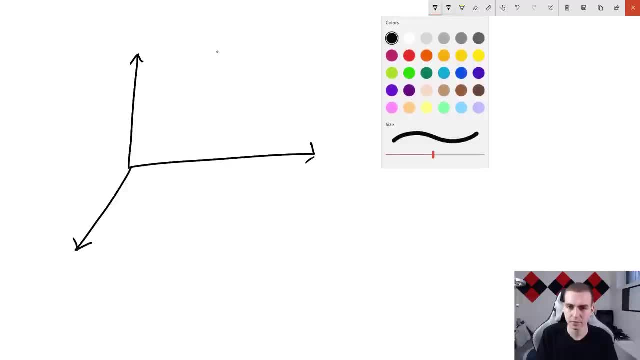 a grasp perspective of the different dimensions. So let's say we have a bunch of data points that are kind of like this and I'm trying my best to kind of draw them in some linear fashion using like all the dimensions here. But it is hard because drawing in three dimensions 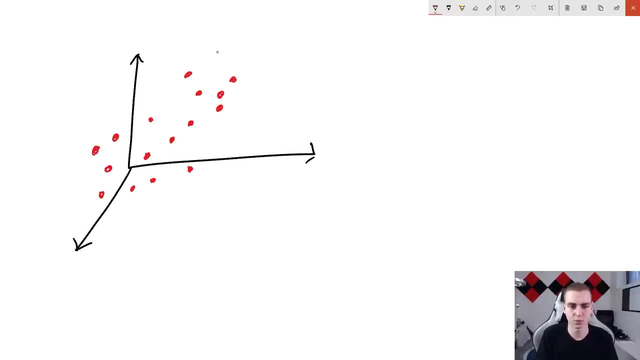 on a two dimensional screen is not easy. Okay, so let's say, this is kind of like what our data points look like. Now I would say that these correlate linearly like pretty pretty well. they kind of go up in one fashion and we don't know the scale of this. So this is. 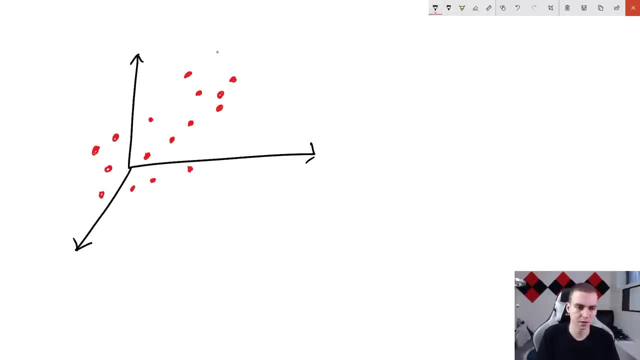 probably fine. So the line of best fit for this data set- and I'll just put my kind of thickness up- might be something like this, right Now, notice that this line is in three dimensions. right, This is going to cross our- I guess this is our- x, y and z axes, So we have a three dimensional 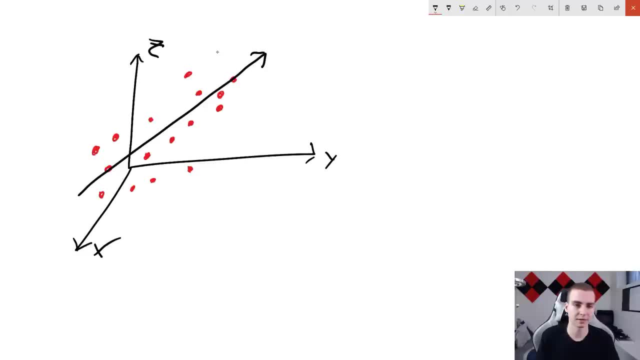 line. Now, the equation for this line is a little bit more complicated. I'm not going to talk about exactly what it is, But essentially what we do is we make this line and then we say, Okay, what value do I want to predict? Do I want to predict y, x or z? Now? so what's? 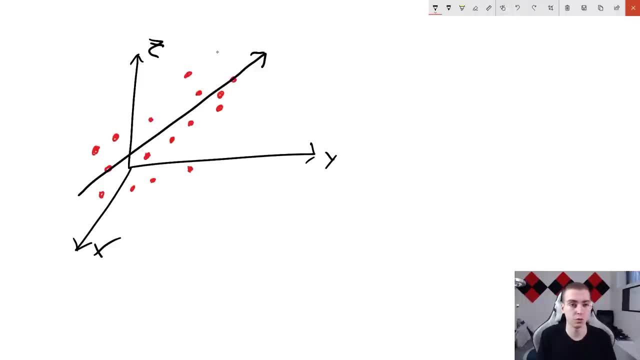 that Now, so long as I have two values, so two values, I can always predict the other one. So if I have, you know, the x- y of a data point, that will give me the Z, And if I have the z- y, that will give me the x. So so long as you have, you know all of the. 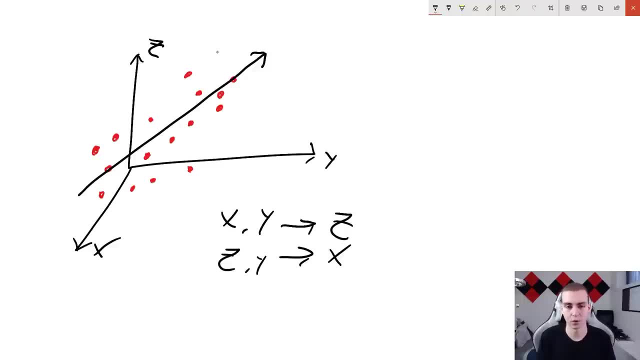 data points, except one. you can always find what that point is based on the fact that you know we have this line and we're using that to predict. So I think I'm going to leave it at that for the explanation. I hope that makes sense. 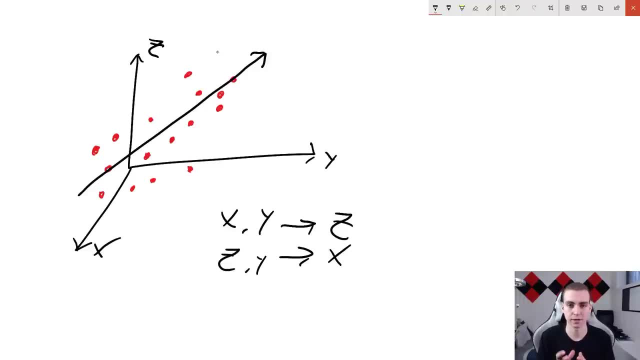 Again understand that we use linear regression when our data points are correlated linearly. Now, some good examples of linear regression were you know, that kind of student predicting the grade kind of thing. you would assume that if someone has, you know, a low grade, 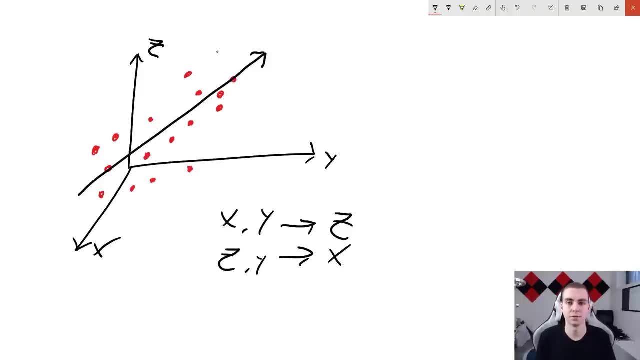 then they would finish with a lower grade and you would assume if they have a higher grade they would finish with a higher grade. Now you could also do something like predicting, you know, future life expectancy. Now this is kind of a darker example, But essentially 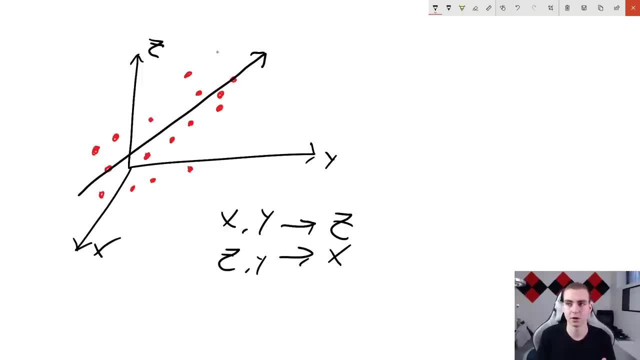 what you could think of here is: if someone is older, they are expected to live, you know, like not as long. or you could look at health conditions. if someone is in critical illness condition they have a critical illness- then chances are their life expectancy is lower, So that's. 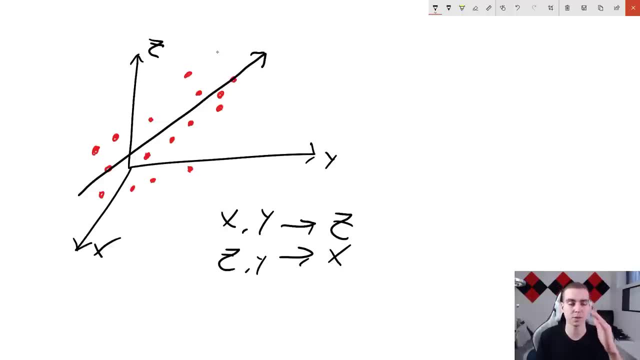 an example of something that is correlated linearly. essentially, something goes up and something goes down, or something goes up, the other thing goes up. that's kind of what you need to think of when you think of a linear correlation. Now, the magnitude of that correlation. 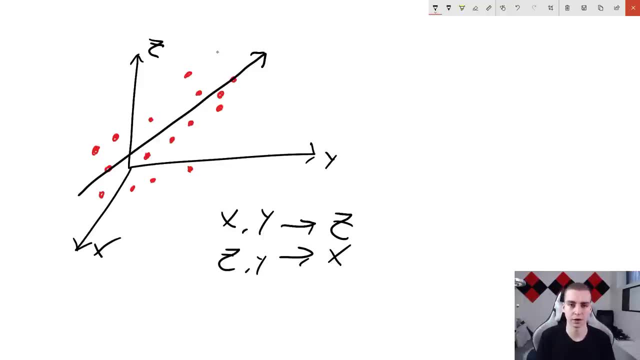 so you know, how much does one go up versus how much one goes down is exactly what our algorithm figures out for us. we just need to know to pick linear regression when we think things are going to be correlated in that sense. Okay, so that is enough of the explanation of linear regression. Now we're going to get. 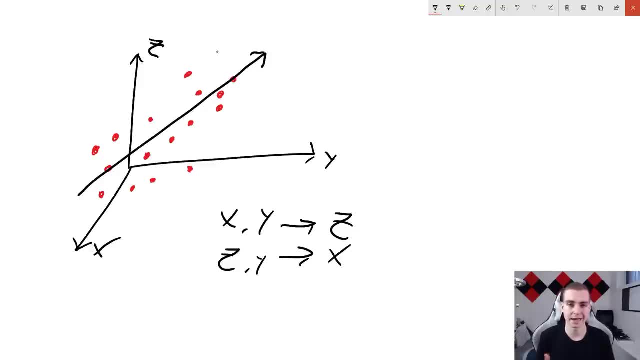 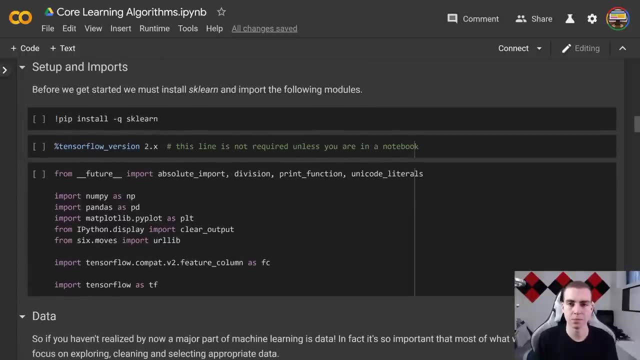 into actually coding and creating a model, But we first need to talk about the data set that we're going to use in the example. we're going to kind of illustrate linear regression with Okay. so I'm here and I'm back in the notebook. Now. these are the imports we need. 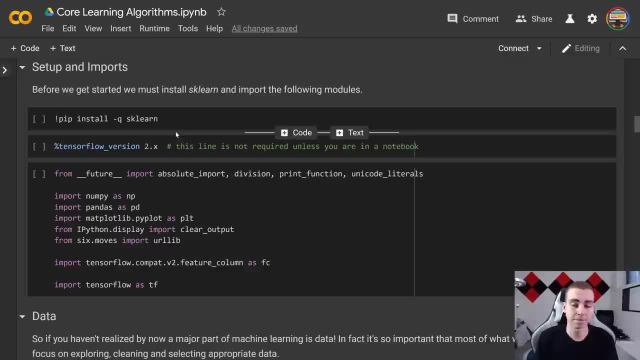 to start with, to actually start programming and getting some stuff done. Now the first thing we need to do is actually install sklearn Now, even if you're in a notebook, you actually need to do this because for some reason it doesn't come by default with the notebook. 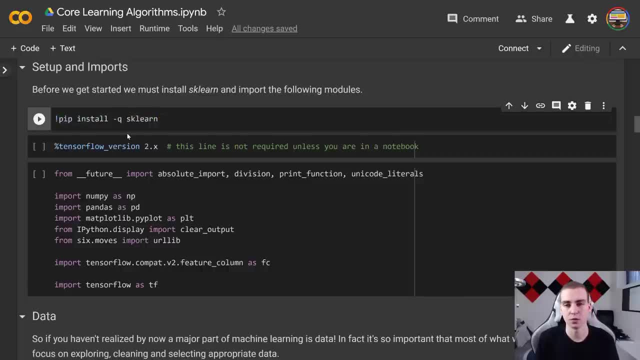 So to do this, we just did an exclamation point: pip install hyphen q sk. learn Now if you're going to be working on your own machine again. you can use pip to install this, And I'm assuming that you know to use pip if you're going. 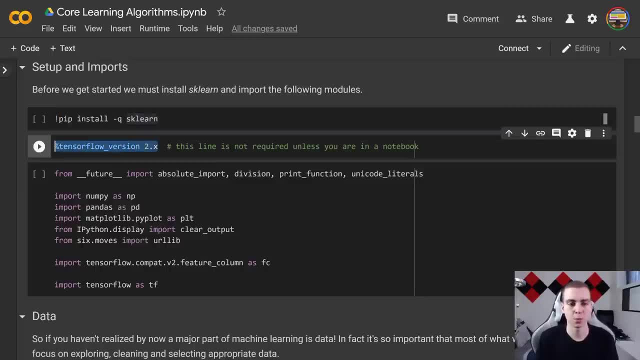 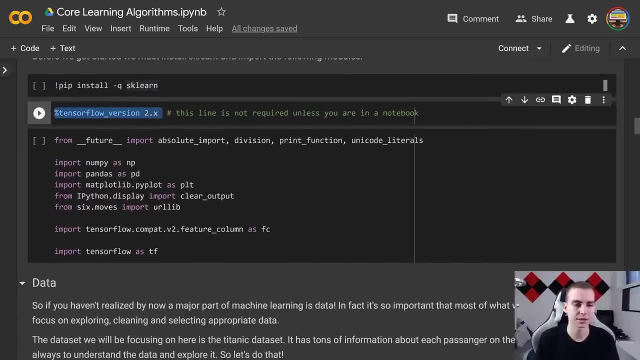 to be going along in that direction. Now, as before, since we're in the notebook, we need to define. we're going to use TensorFlow version 2.x. So to do that, we're going to- just, you know, do that up here with the percent sign, And then we have all these imports. 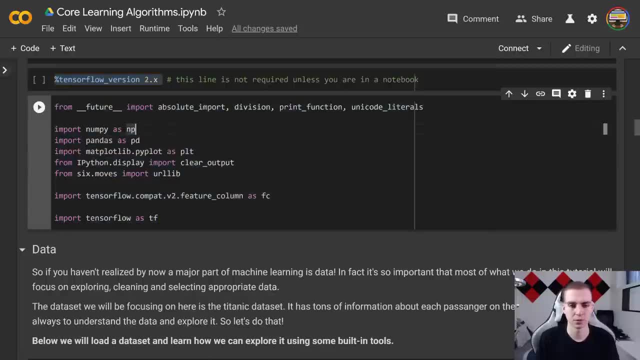 which we're going to be using throughout here. So from future import, absolute import, division, print function, Unicode literals and then obviously the big ones. So NumPy, pandas, matplotlib, we're going to be using I Python, we're gonna be using TensorFlow, And yeah, so I'm actually 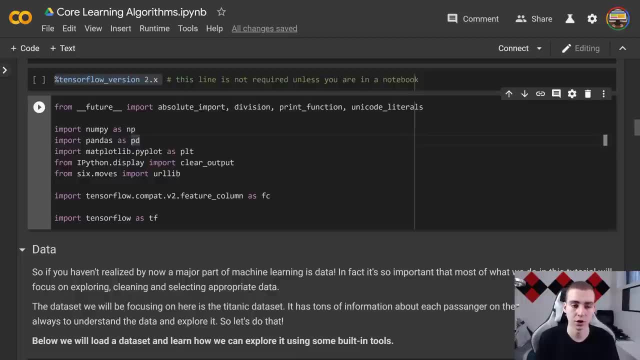 just going to explain what some of these modules are, because I feel like some of you may actually not know. NumPy is essentially a very optimized version of arrays in Python, So what this allows us to do is lots of kind of multi dimensional calculations. So, essentially, if you have 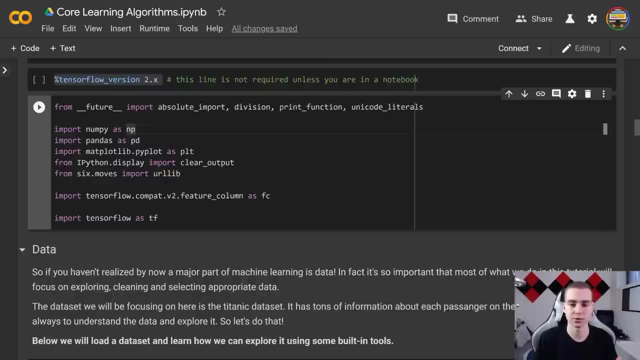 a multi dimensional array which we've talked about before, right when we had, you know, those crazy shapes like 5555,. NumPy allows us to represent data in that form and then very quickly manipulate and perform operations on it, So we can do things like cross product dot. 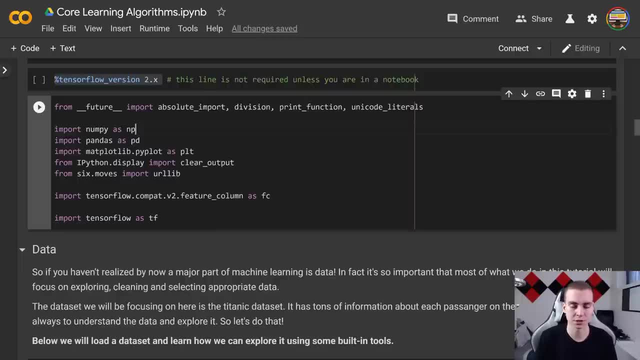 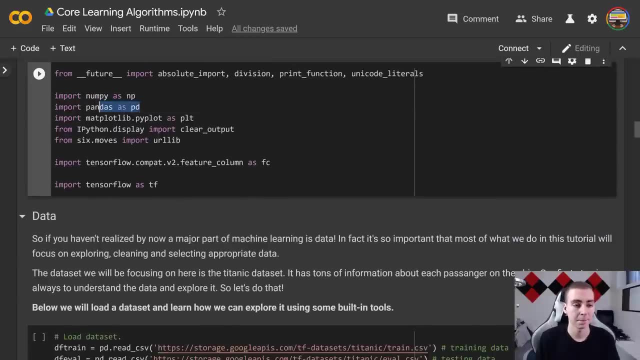 product matrix addition matrix subtraction element wise addition, subtraction. you know, vector operations. that's what this does for us. it's pretty complex, but we're going to be using it a fair amount. Pandas Now what pandas does is it's kind of a data analytics. 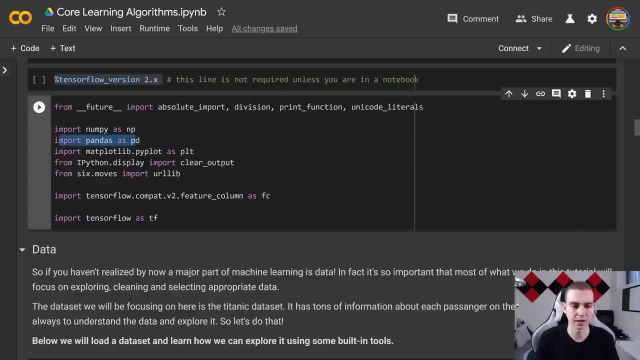 tool. I almost want to say. I don't know the formal definition of what pandas is, but it allows us to very easily manipulate data. So you know: load in data sets, view data sets cut off. Specifically, we're going to be using Pandas. we're going to be using Pandas. 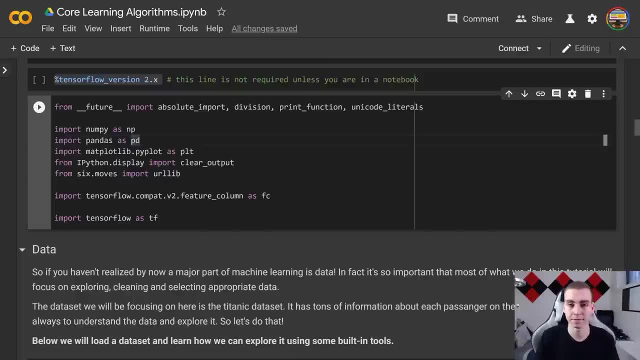 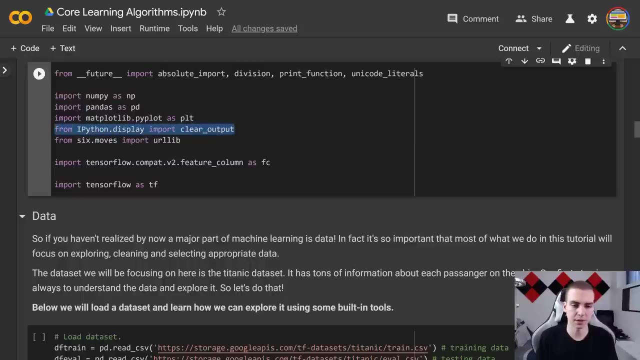 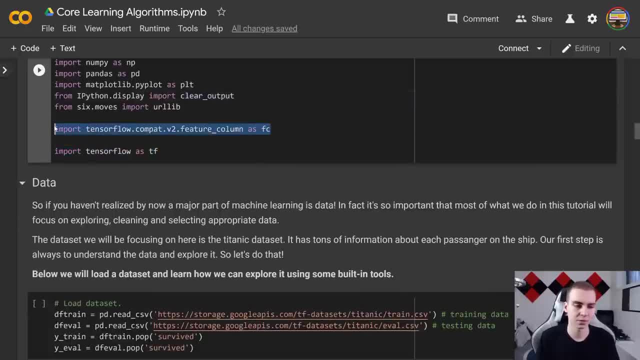 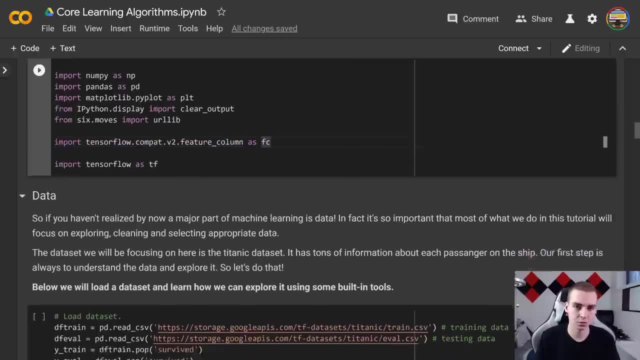 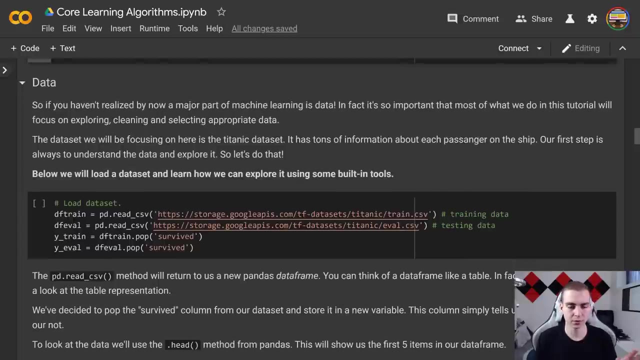 build some data on that data inside a something called a feature column when we create a linear regression algorithm or model and TensorFlow, So we're going to use that, Okay. so now that we've gone through all that, we need to start talking about the data set that we're going to use for linear regression. 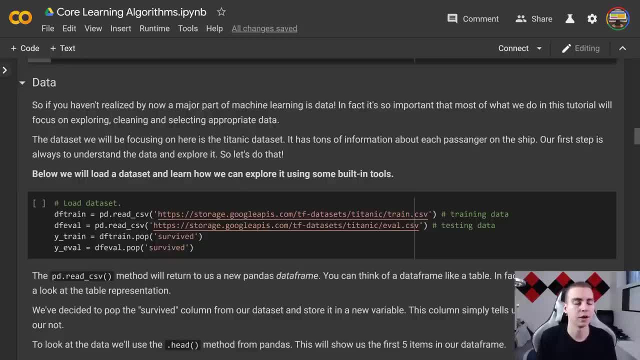 And for this example, because what we're going to do is, you know, actually create this model and start using it to predict values. So the data set that we're going to use actually- I need to read this because I forget exactly what the name of it is- is the Titanic data. 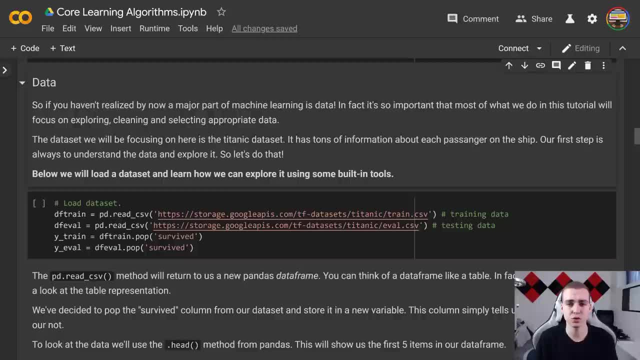 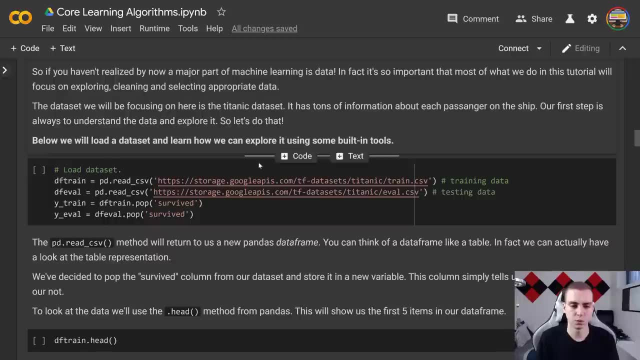 set. That's what it is. So, essentially, what this does is aim to predict who's going to survive or the likelihood that someone will survive being on the Titanic, given a bunch of information. So what we need to do is load in this data set. Now, I know this seems like. 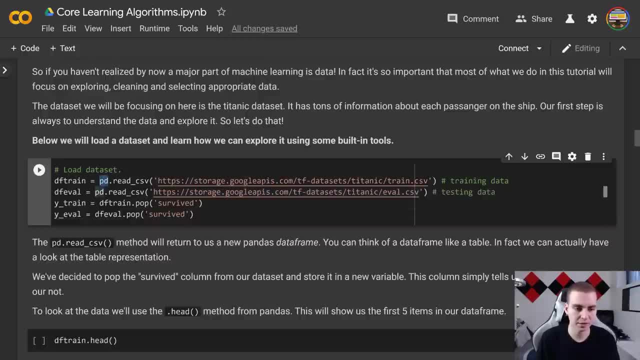 a bunch of gibberish, but this is how we need to load it. So we're going to use pandas. So PD dot read CSV from this URL. So what this is going to do is take this CSV file, which stands for comma separated values, And we can actually look at this if we want. I 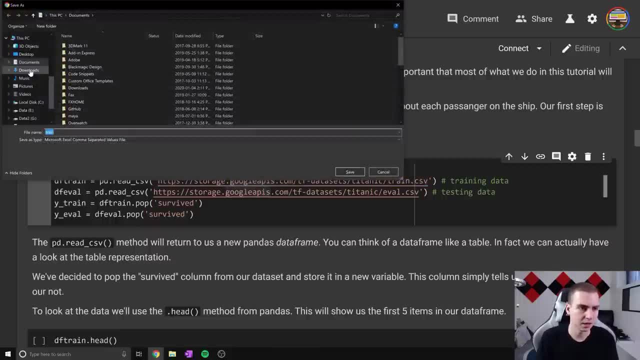 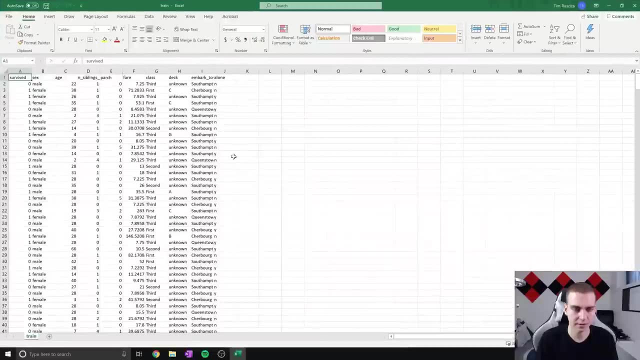 think so. I said it said control, click, let's see if this pops up. So let's actually download this. Let's open this up ourselves and have a look at what it is in Excel. So I'm going to bring this up here. you can see that link And this is what our data set is. So we have our columns. 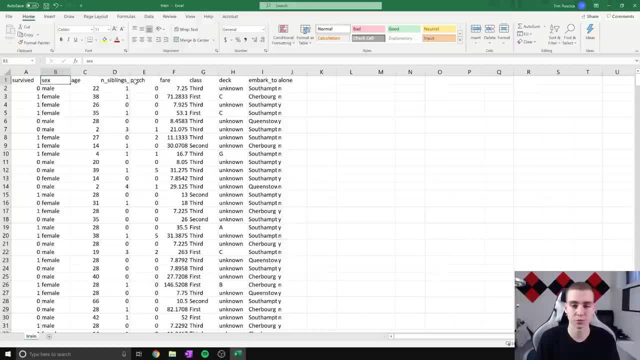 which just stand for you know what is it? the different attributes in our data set, of the different features and labels of our data set. we have survived, So this is what we're actually going to be aiming to predict, So we're going to call this our label, right? 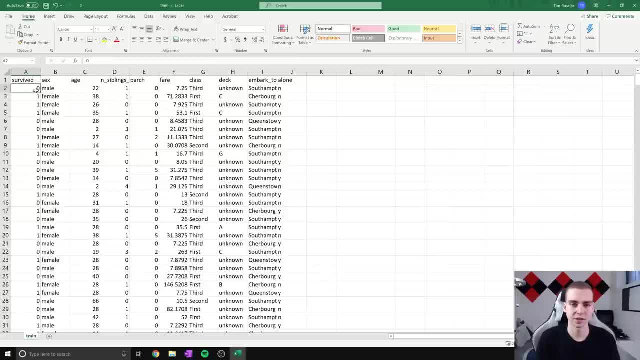 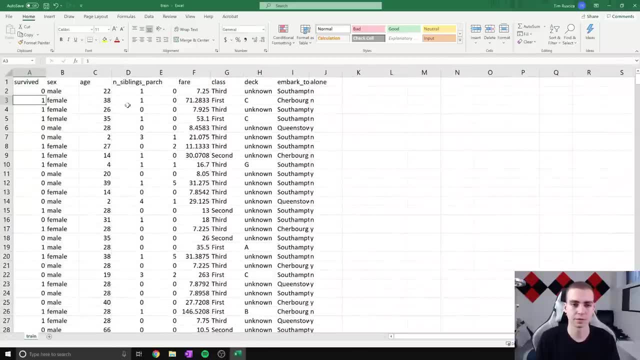 where our output information. So here, a zero stands for the fact that someone did not survive and one stands for the fact that someone did survive. Now, just thinking about it on your own for a second and looking at some of the categories: 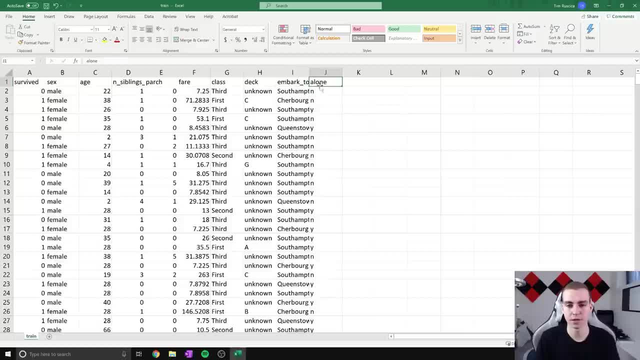 we have up here. can you think about why linear regression would be a good algorithm for something like this? Well, for example, if someone is a female, we can kind of assume that they're going to have a higher chance of surviving on the Titanic, just because of you know. 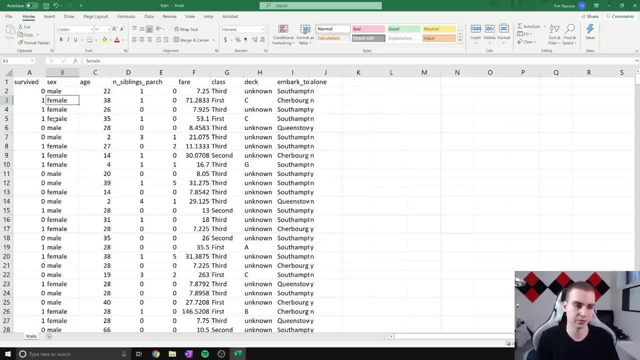 the kind of the way that our culture works, you know, saving women and children first right. And if we look through this data set, we'll see that when we see females, it's pretty rare that they don't survive, Although, as I go through, there is quite a few that didn't. 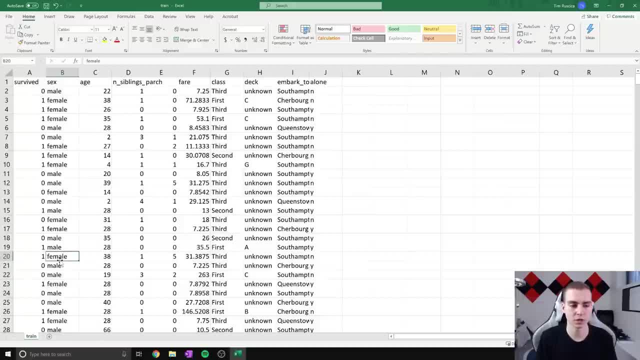 survive. But if we look at it compared to males, you know there's definitely a strong correlation that being a female results in a stronger survival rate. Now, if we look at age right, can we think of how age might affect this? Well, I would assume, if someone's way younger, 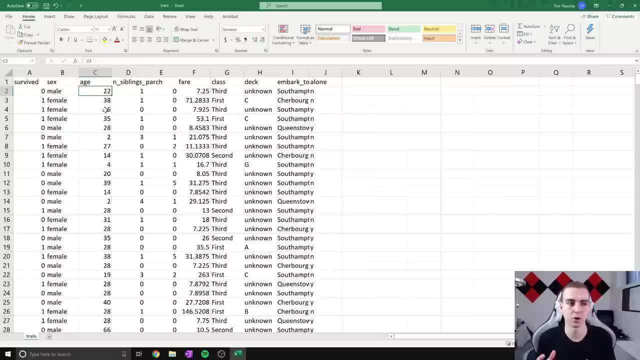 they probably have a higher chance of surviving because they would be, you know, prioritized in terms of lifeboats or whatever it was. I don't know much about the Titanic, So I can't talk about that specifically, But I'm just trying to go through the categories and 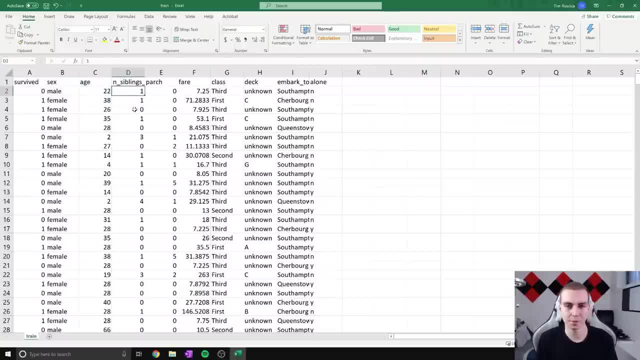 explain to you why we picked this algorithm Now. number of siblings: that one might not be, as you know, influential in my opinion. parche- I don't actually remember what parche stands for, I think it is like what parche. 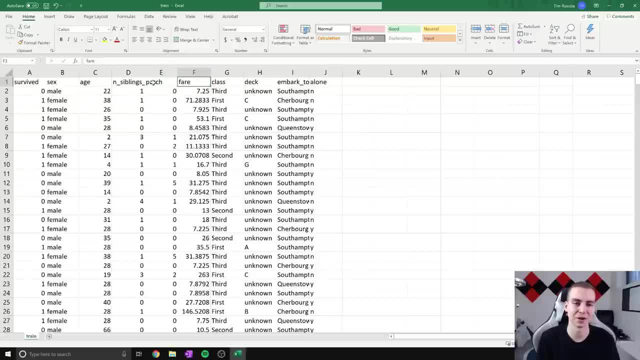 I don't know exactly what this column stands for, So unfortunately I can't tell you guys that one. But we'll talk about some more of the second fair- Again not exactly sure what fair stands for. I'm going to look on the TensorFlow website after this and get back. 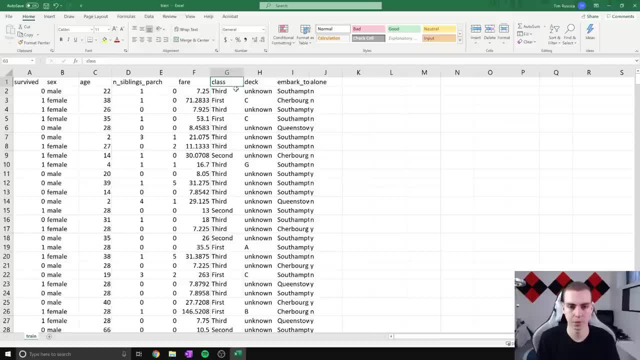 to you guys And we have a class, So class is what class they were. on the boat, right. So first class, second class, third class. So you might think someone that's in a higher class might have a higher chance of surviving. We have deck, So this is what class they were. 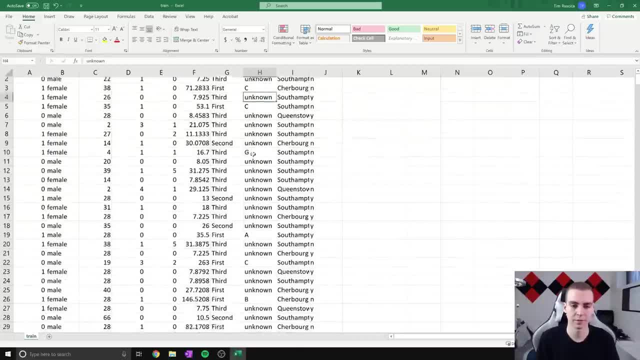 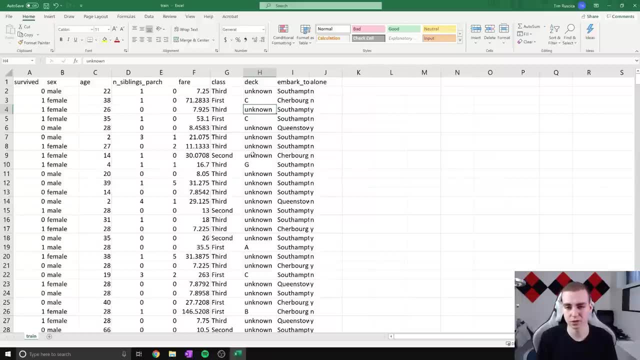 on deck. they were on when it crashed, So unknown is pretty common. And then we have all these other decks. you know, if someone got hit, if someone was standing on the deck that had the initial impact, we might assume that they would have a lower chance of survival. 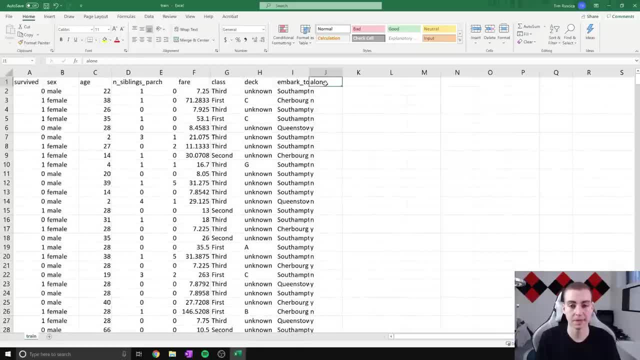 embark to is where they were going. And then, are they alone, Yes or no? And this one, you know this is interesting. we're gonna see. does this make an effect If someone is alone? Is that a higher chance of survival? Is that a lower chance of survival? So this is kind. 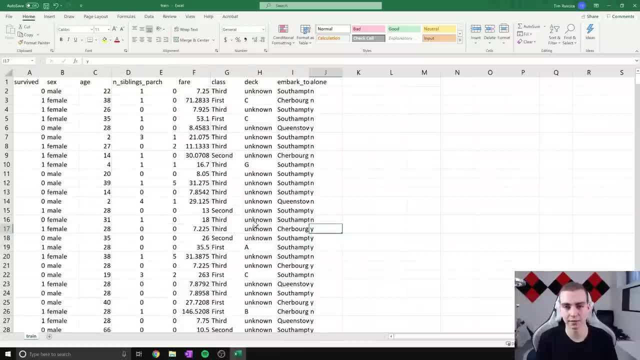 of interesting- And this is what I want you guys to think about- is that when we have information and data like this, We know what correlations there might be, But we can kind of assume there's some linear thing, that we're looking for some kind of pattern, right, Whereas if something is true, 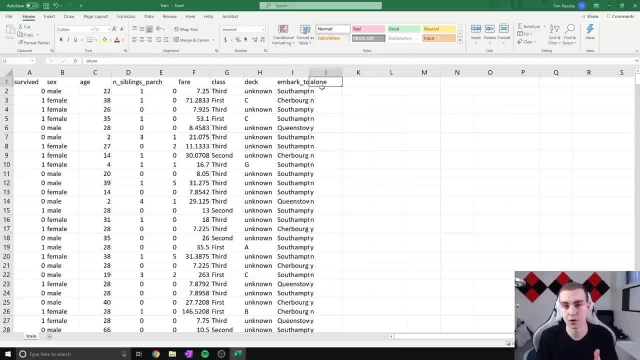 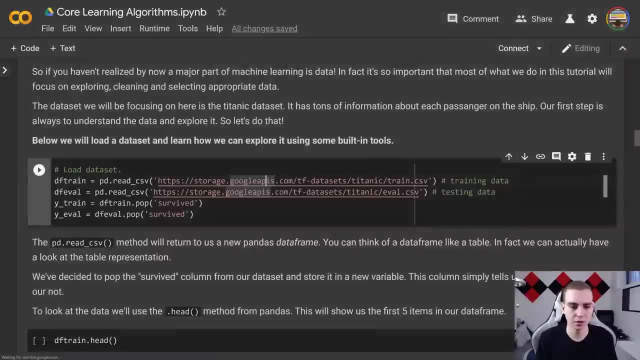 then you know, maybe it's more likely someone will survive, Whereas, like, if they're not alone, maybe it's less likely And maybe there's no correlation whatsoever, But that's where we're going to find out as we do this model. So let me look actually on the TensorFlow. 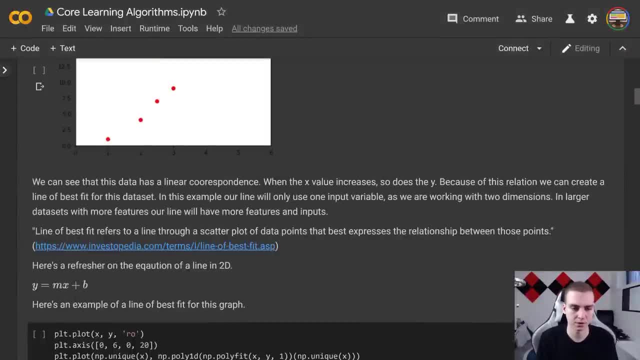 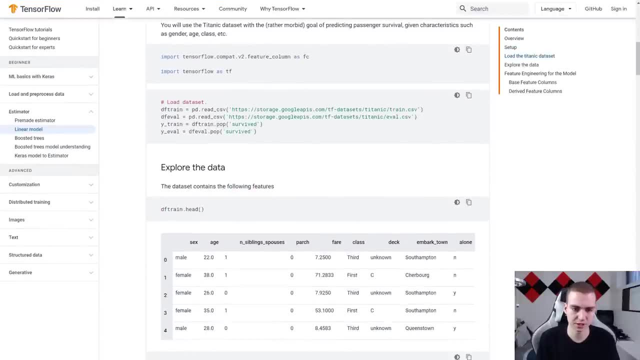 website and see if I can remember what parche and I guess, what fair was. So let's go up to the top here Again. a lot of this stuff is just straight up copied from the TensorFlow website. I've just added my own stuff to it. you can see like I just copied all this. we're just 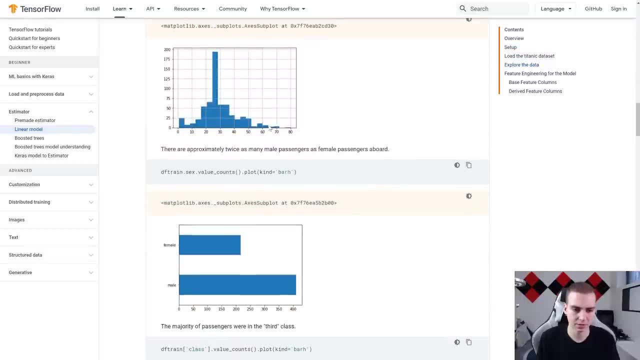 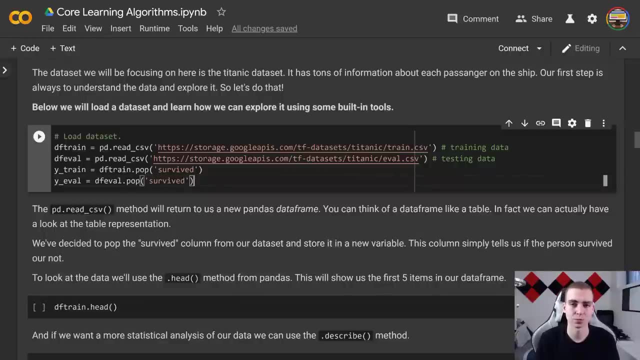 bringing it in there. Let's see what it says about the different columns, if it gives us any exact explanations. Okay, so I couldn't find what parche were fair stands for. for some reason it's not on the TensorFlow website either, And I couldn't really find any information. 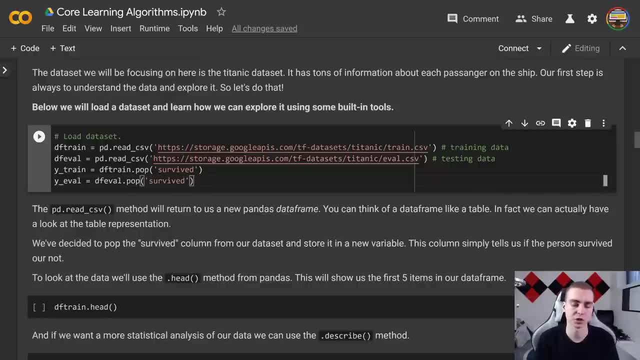 about it. You guys know, you know, leave a comment down below. but it's not that important. We just want to use this data to do a test. So what I've done here: if I've loaded in my data set and notice that I've loaded a training data set in a testing data set and 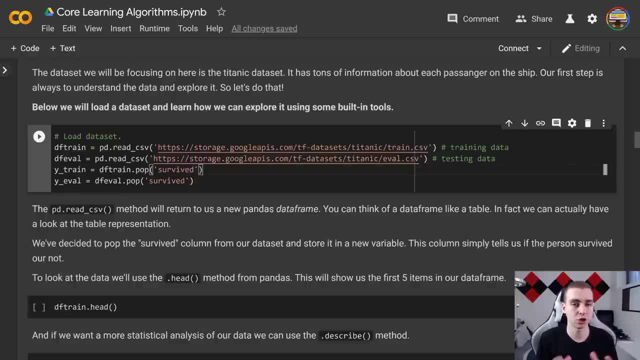 now. we'll talk about this more later, but this is important. I have two different data sets, one to train the model with and one to test the model with now, kind of. the basic reason we would do this is because when we test our model for accuracy, to see how well 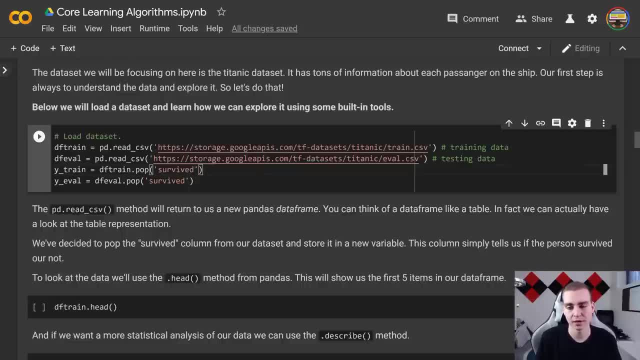 it's doing. it doesn't make sense to test it on data. it's already seen. it needs to see fresh data So we can make sure there's no bias and it hasn't simply just memorize the data. you know that we had Now what I'm doing here at the bottom with this y train. 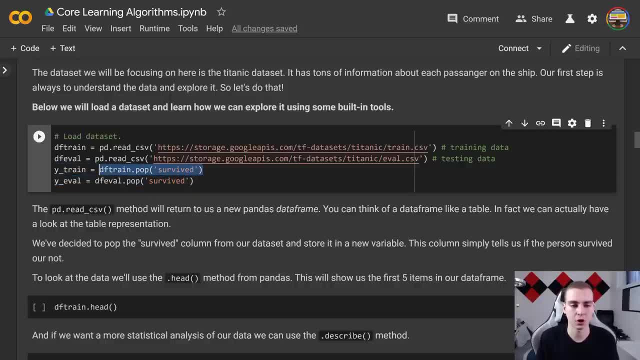 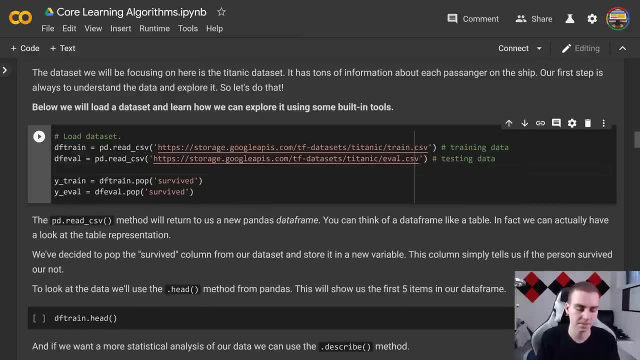 in this y eval is, I'm essentially popping A column off of this data set. So if I print out the data set here- and I'm actually, I'm going to show you a cool trick with pandas that we can use to look at this, So I can. 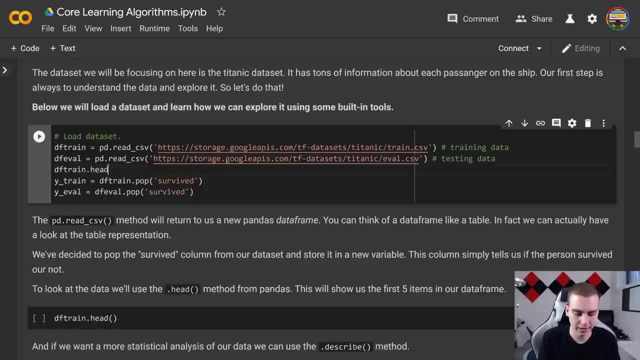 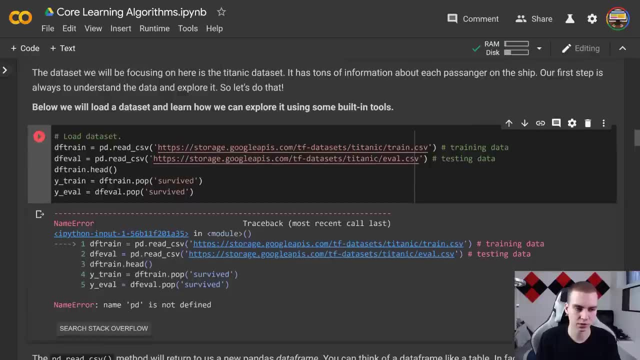 say df train dot head. So if I look at this by just looking at the head and we'll print this out, oh, I may need to import some stuff above. We'll see if this works or not. Yeah, So I need to just do these imports. So let's install And let's do these imports. I'll. 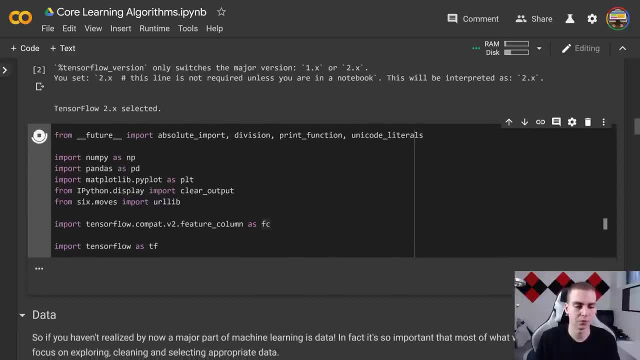 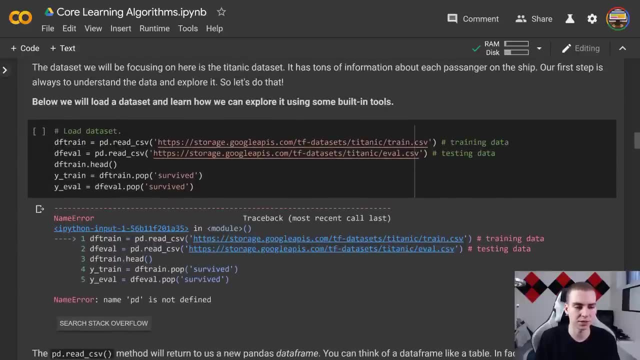 wait for this to run And then okay, so I've just selected TensorFlow 2.0, we're just importing this now should be done in one, One second. And now what we'll do is we'll print out the, the data frame here. So, essentially, 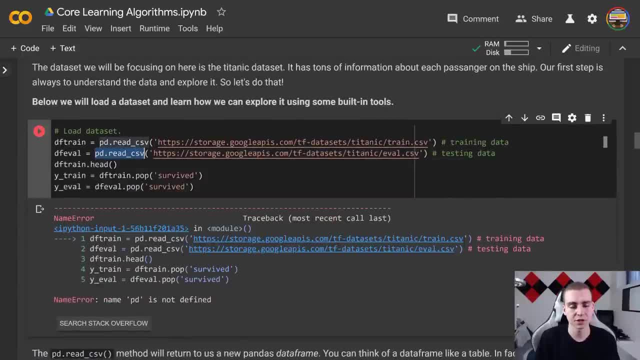 what this does is load this into a pandas data frame, And this is a specific type of object. Now, we're not going to go into this specifically, but a data frame allows us to view a lot of different aspects about the data and kind of store it in a nice form. 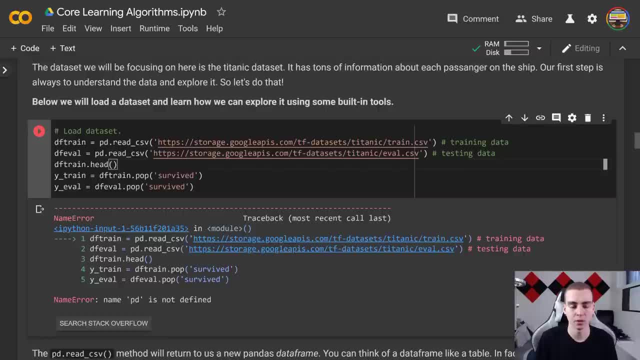 as opposed to just loading it in and storing it in like a list or a NumPy array, which we might do if we didn't know how to use pandas. This is a really nice way to do it. read CSV loaded into a data frame. object: 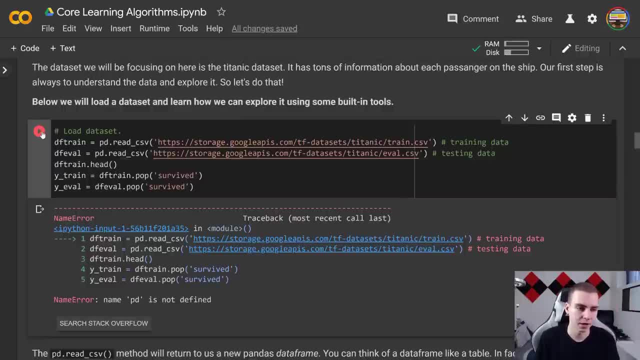 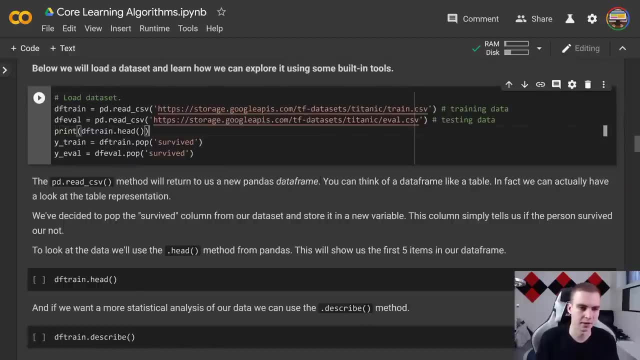 means we can reference specific columns and specific rows in the data frame. So let's run this and just have a look at it. DFO, I got need to print df train dot head. So let's do that And there we go. So this is what our data frame head looks like Now. head. 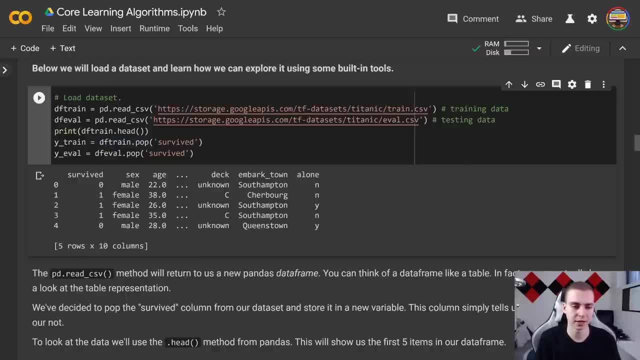 what that does is show us the first five entries in our data set, as well as show us a lot of the different columns that are in it. Now, since we have more than you know, we have a few different columns. it's not showing us all of them, it's just giving us the dot. 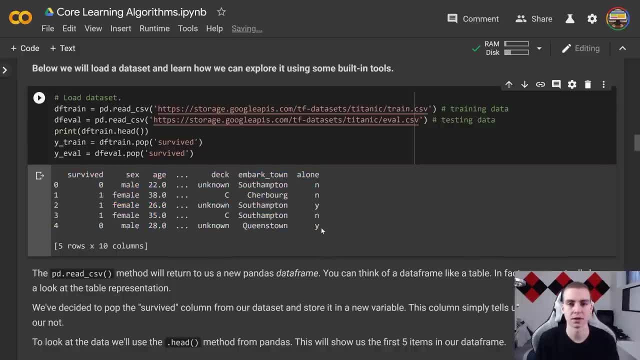 dot dot. So we can see. this is what the data frame looks like And this is kind of the representation internally. So we have entry zero, survived zero, survived one. we have male, female, all that. Now notice that this has the survived column. okay, Because what I'm going to do? 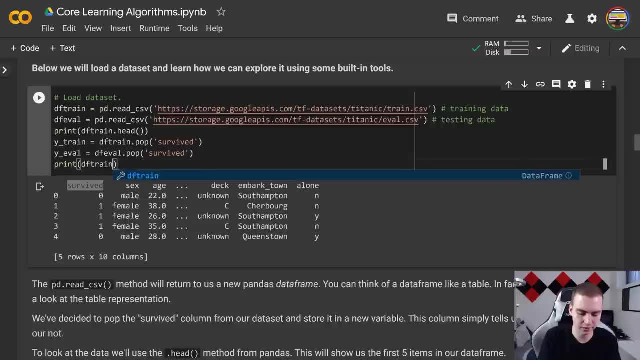 is I'm going to print the data frame head again, so df train dot head, after we run these two lines. Now what this line does is takes this entire survived column, so all these zeros and ones, and removes it from this data frame- So the head data frame- and stores it in the variable y train. The reason we 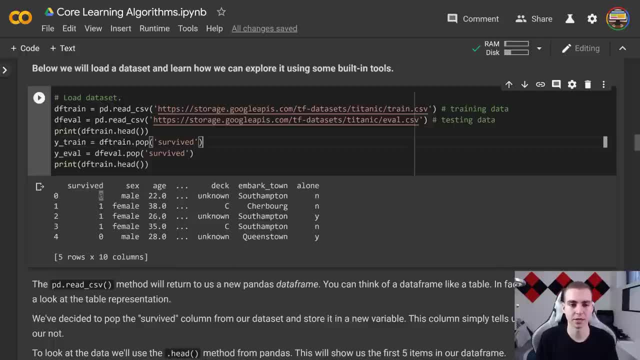 need to do that is because we need to separate the data we're going to be classifying from the data that is kind of our input information or our initial data set right. So since we're looking for the survived information, we're going to put that in its own, you know kind. 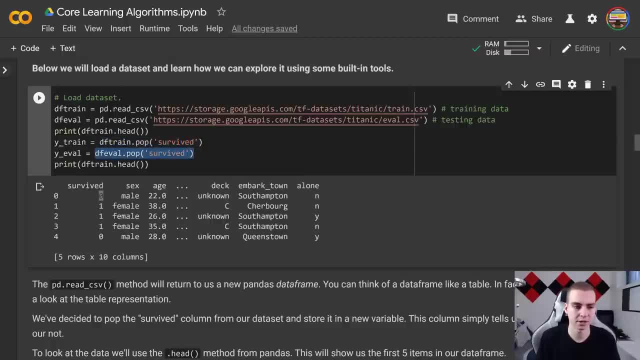 of variable store here. Now we'll do the same thing for the evaluation data set, which is the evaluation or testing data, And notice that here this was trained us CSV and this one was eval dot CSV. Now these have the exact same value, So we're going to put that. 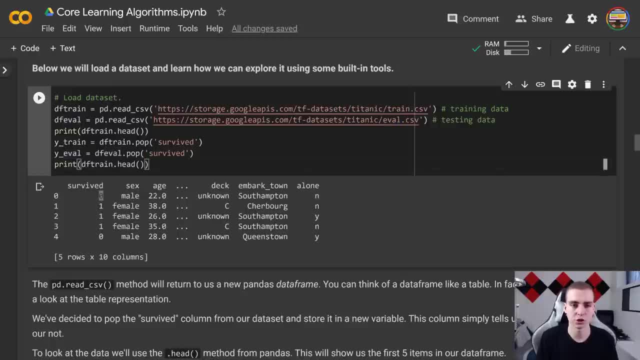 here we're going to put that. here we're going to put that. here we're going to put that in the exact same form. they look like completely identical. it's just that, you know, some entries we've just kind of arbitrarily split them, So we're going to have a lot of entries. 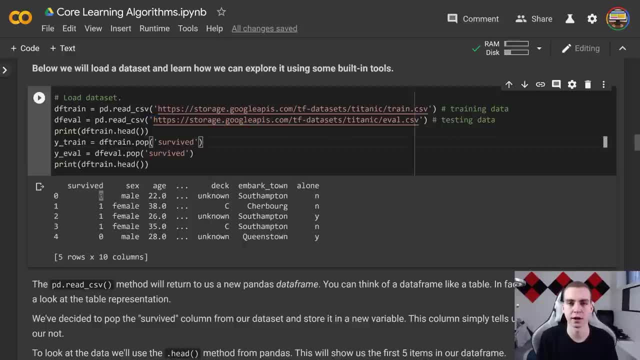 in this training set And then we'll have a few in the testing set that we'll just use to do an evaluation on the model later on. So we pop them off by doing this. pop removes and returns this column. So if I print out y train which are actually, let's look at. 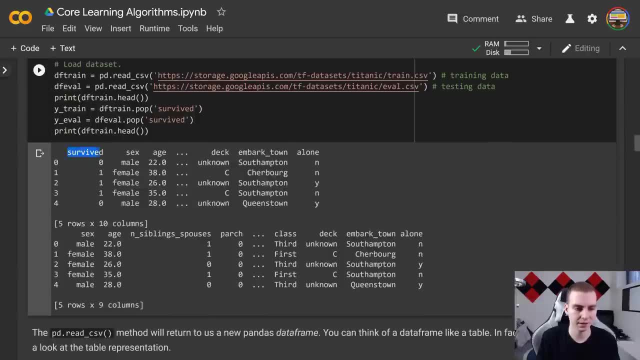 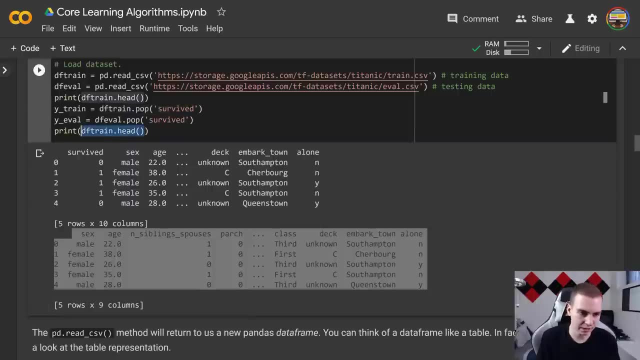 this one first, just to show you how it's been removed. we can see that we have the survived column here. we popped and now the survived column is removed from that data set. So that's just important to understand. Now we can print out some other stuff too, So we can look at the Y train, see what that. 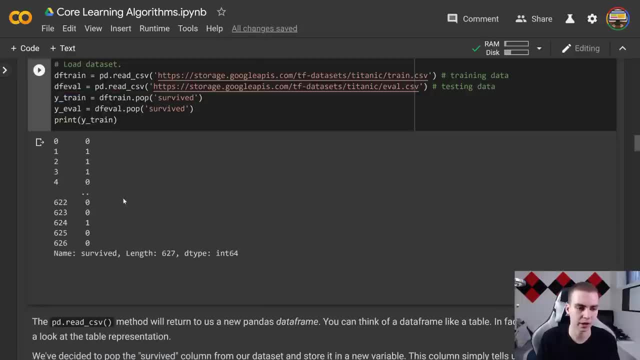 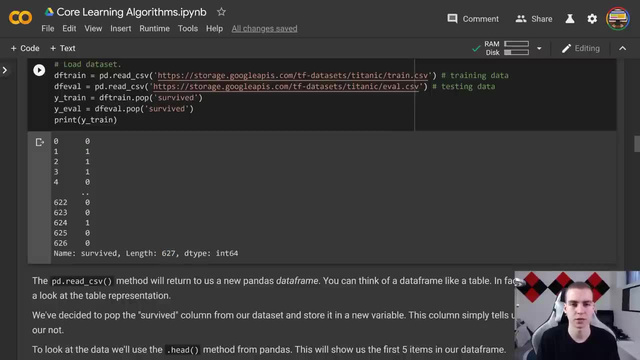 is just to make sure we really understand this data. So let's look at why train And you can see that we have 626, or 627 entries and, just you know, zeros or ones representing whether someone survived or whether they did not. Now the corresponding indexes in this: 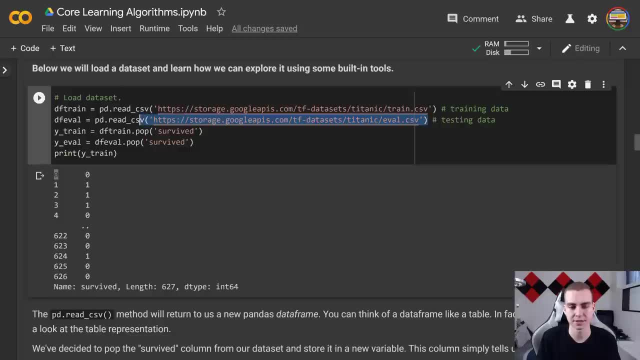 kind of list or data frame correspond to the indexes in the testing and training data frame. What I mean by that is, you know, entry zero in this specific data Data frame corresponds to entry zero in our Y train variable. So if someone survived, 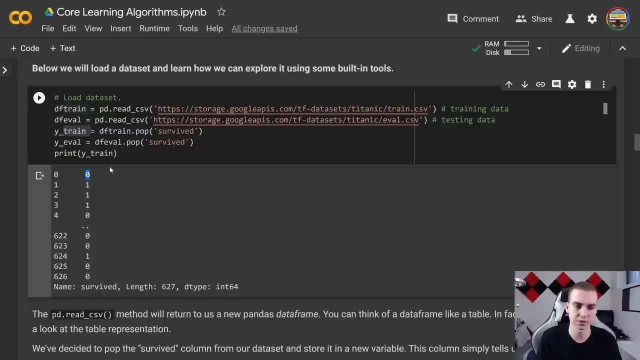 you know, at entry zero it would say one here, right. or in this case entry zero did not survive. Now I hope that's clear. I hope I'm not confusing you with that. But I just want to show one more example to make sure. So we'll say df, train zero. I'm going to print: 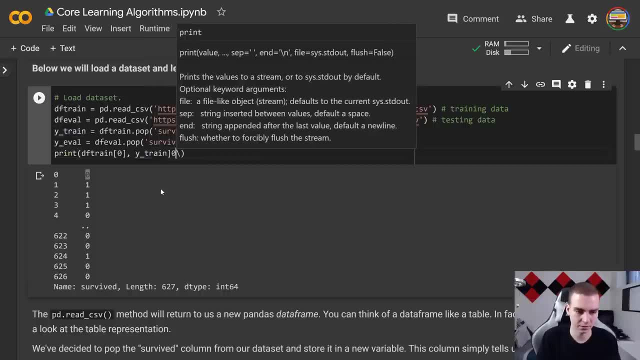 that and I'm going to print y train at index zero- oops, if I didn't mess up my brackets- and we'll have a look at it. Okay, so I've just looked up the documentation because I totally forgot that I couldn't find it. So I'm going to go ahead and go ahead and 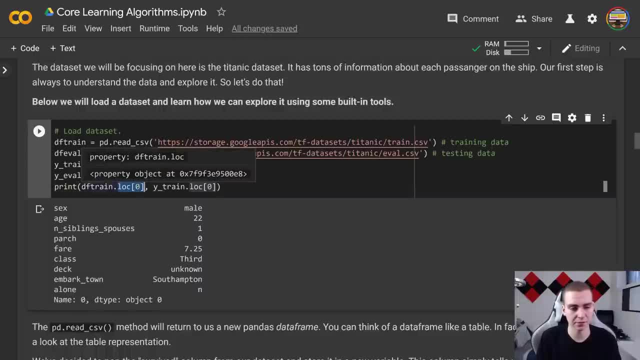 do that. If I want to find one specific row in my data frame, what I can do is print dot loc. So I do my data frame and then dot loc and then whatever index I want. So in this case I'm locating row zero, which is this, And then on the Y train I'm doing the same. 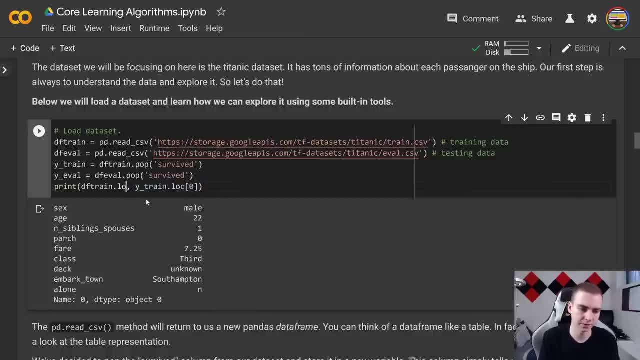 thing. I'm locating row zero Now what I had before. right, if I did df train and I put square brackets inside here, what I can actually do is reference a specific column. So if I wanted to look at, you know, say, the column for age, right, so we have a column for age. 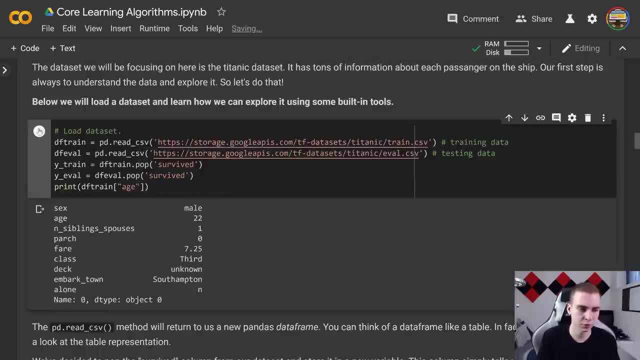 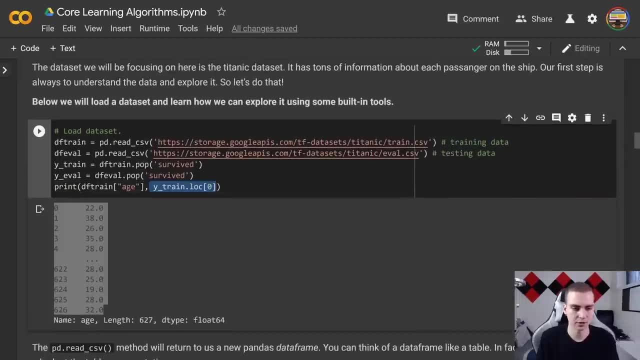 what I can do is do df- train age- And then I can print this out like this And it gives me all of the different age values. So that's kind of how we use a data frame. we'll see that as we go further on. Now let's go back to the other example I had, because I just 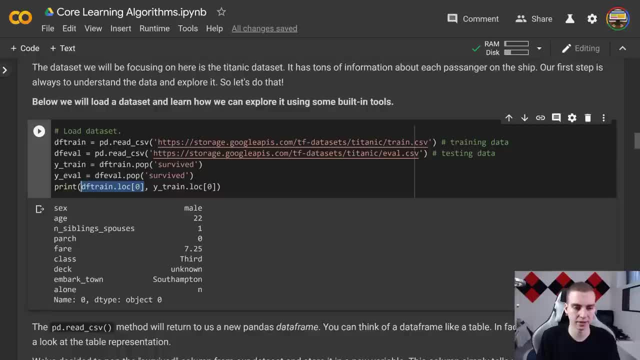 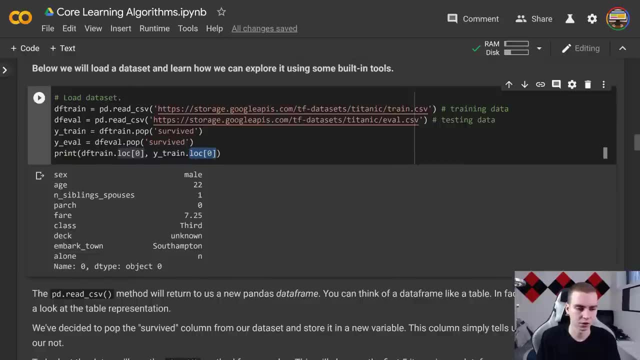 erased it, where I want to show you the row zero in the data frame, that's training, and then in the Y train, you know, output whatever that is, so the survival. So you can see here that this is what we get from printing df train dot loc zero, so row zero, this is all. 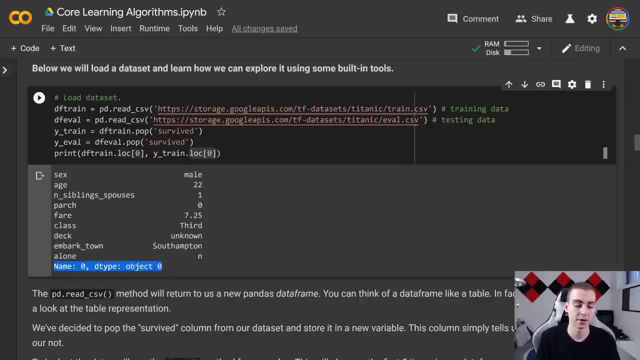 the information Here. this corresponds to the fact that they did not survive at row zero, because it's simply just: the output is value zero. Now I know this is weird. it's saying like: name zero D, type, object zero. don't worry about that, It's just because it's trying to print. 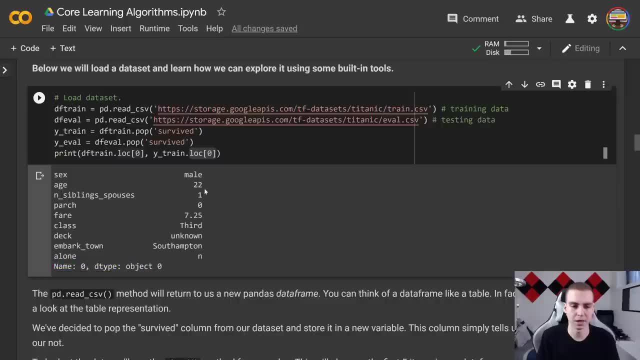 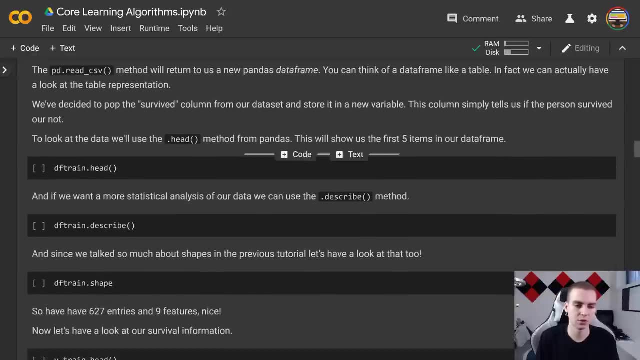 it with some information, But essentially this just means this person, who was male, 22 and had one sibling, did not survive. Okay, so let's get out of this. Now we can close this and let's go to: Oh, we've pretty much already done what I've just have down here. 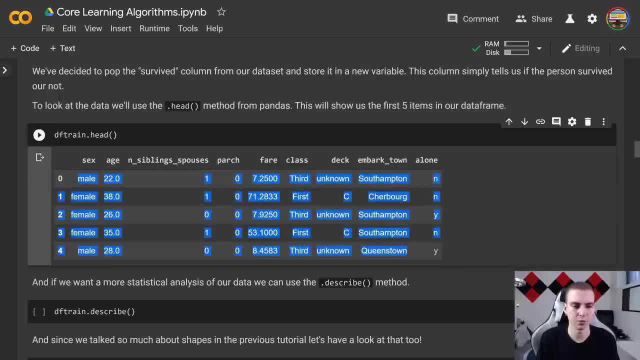 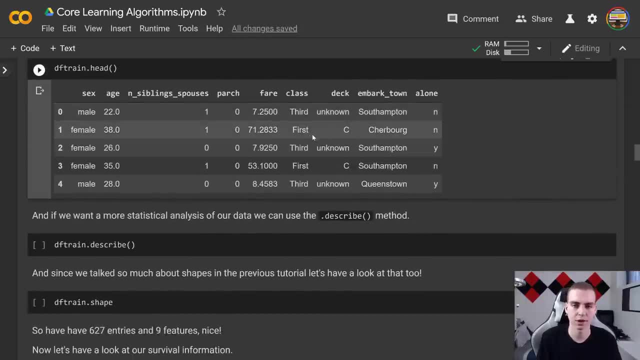 But we can look at the data frame head. this is a little bit of a nicer output. when we just have df, train dot head, we can see that we get kind of a nice outputted little graph. we've already looked at this information So we know kind of some of the attributes. 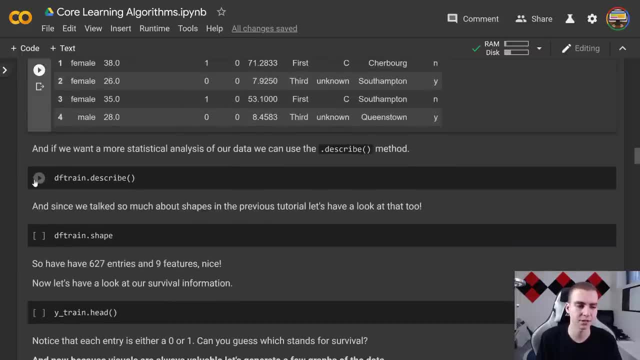 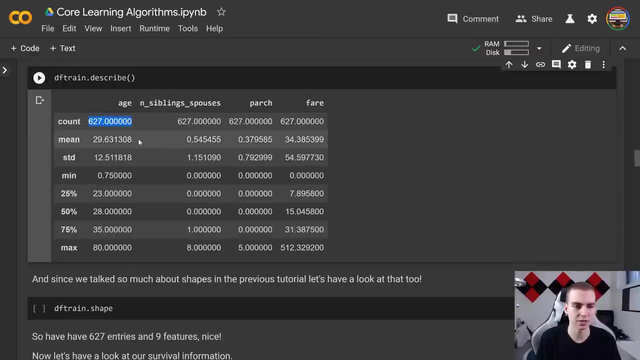 of the data set. Now we want to describe the data set. sometimes, what described as is just give us some overall information. So let's have a look at it here. we can see that we have 627 entries. the mean of age is 29,. the standard deviation is: you know. 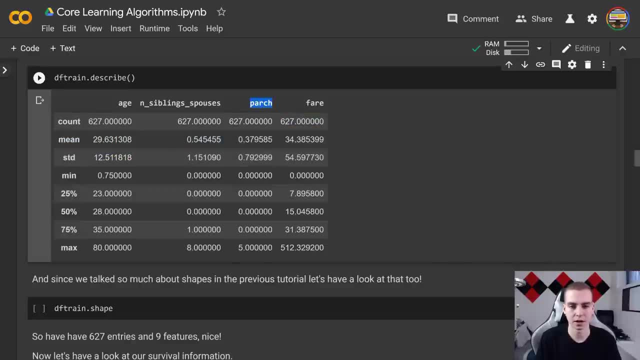 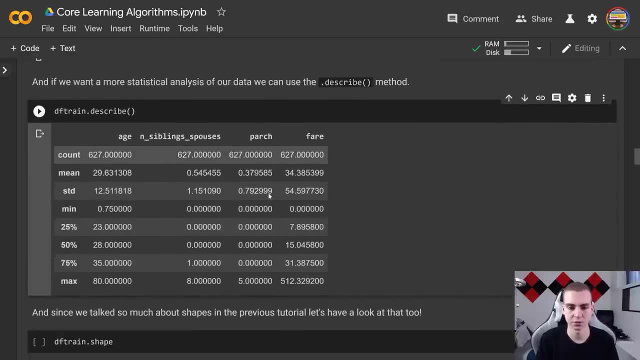 12 point, whatever, And then we get the same information about all of these other different attributes. So, for example, it gives us, you know, the mean fair, the minimum average, minimum fair and just some statistics. If you guys understand this, great. if you don't, 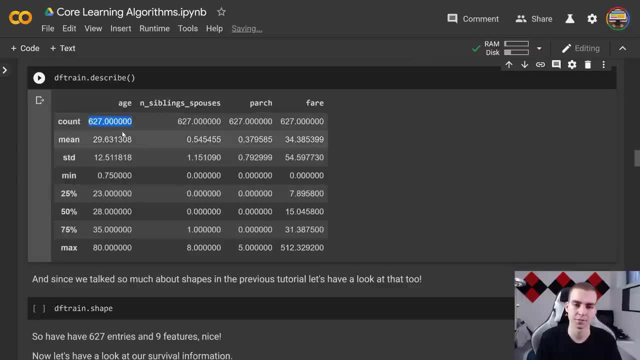 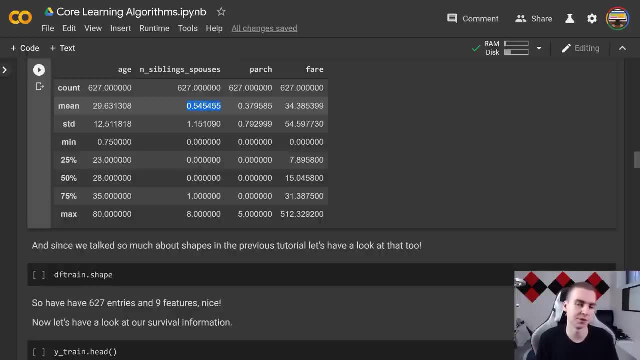 doesn't really matter. The important thing to look at typically is just how many entries we have is. sometimes we need that information, And sometimes the mean can be helpful as well, because you can kind of get an average of like what the average value is in the data. 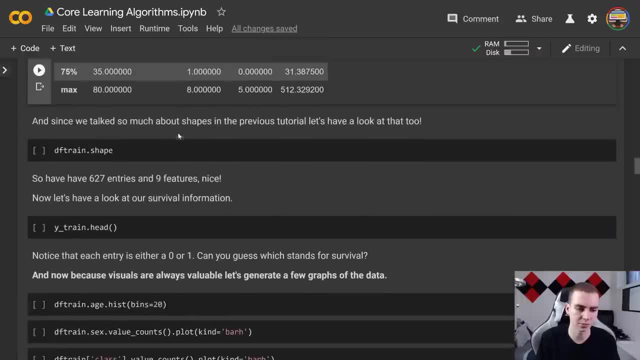 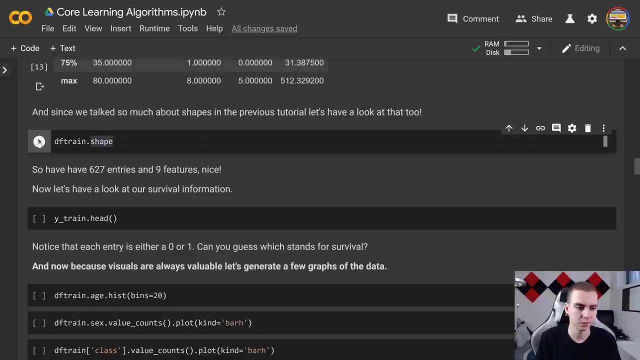 set. So if there's any bias later on you can figure that out. But it's not crazy important, Okay, so let's have a look at the shape. So, just like NumPy arrays and tensors have a shape attribute, So do data frames. So we want to look at the shape. you know we can. 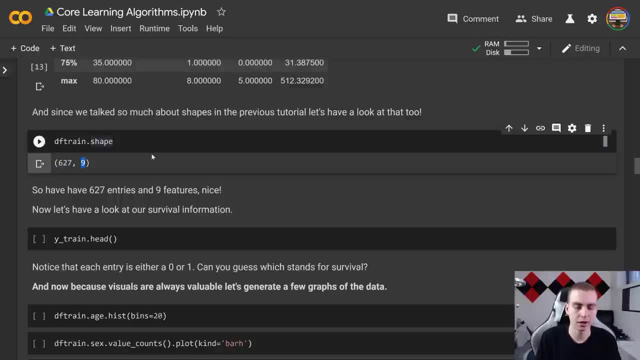 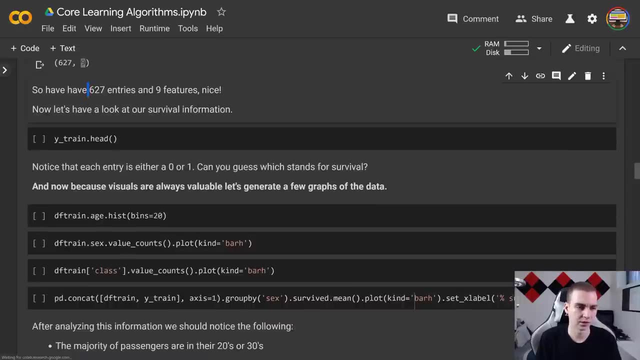 just print out df train dot shape, we get 627.. By nine, which essentially means we have 627 rows and nine columns or nine attributes. So yeah, that's what. it's what it says here. you know, 627 entries, nine features. we can. 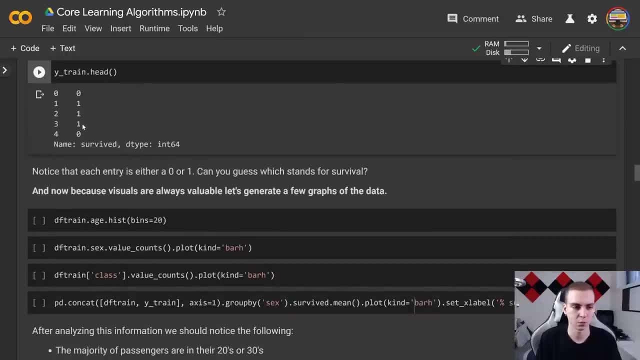 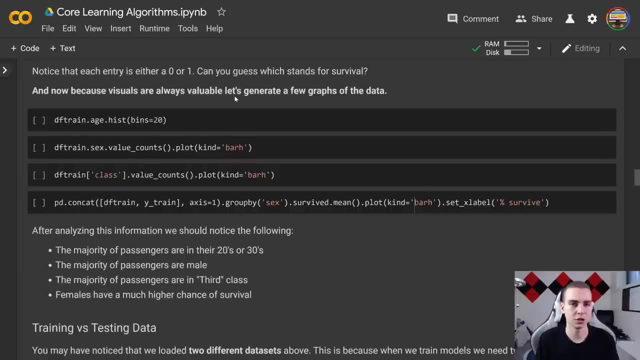 interchange attributes and features And we can look at the head information for why. So we can see that here, which we've already looked at before, And that gives us the name which was survived. Okay, so now what we can actually do is make some kind of graphs about 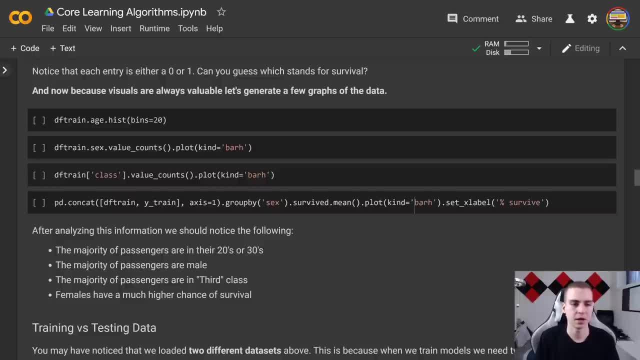 this data. Now, I've just stolen this code, you know, straight up from the TensorFlow website. I wouldn't expect you guys to do any of this. you know like output any of these values, But what we're going to do is create a few histograms. 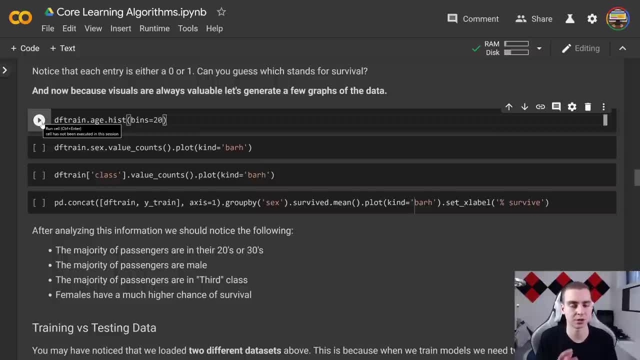 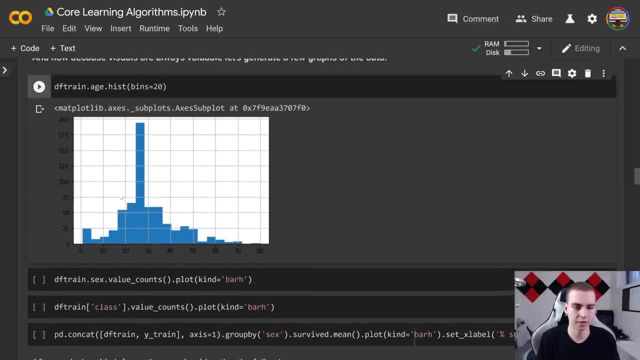 and some plots just to look at kind of some correlations in the data so that when we start creating this model, we have some intuition on what we might expect. So let's look at age. So this gives us a histogram of the age. So we can see that there's about 25 people. 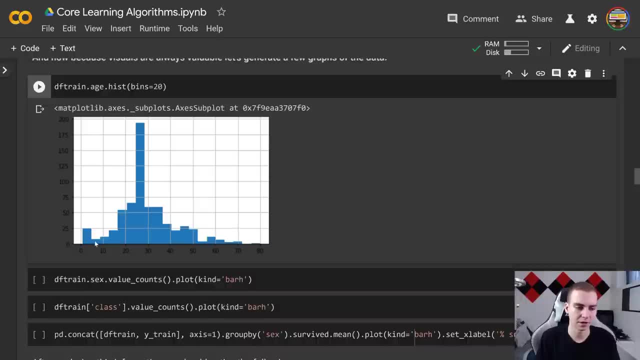 that are kind of between zero and five. there is, you know, maybe like five people that are in between five and 10. And then the most amount of people are kind of in between their 20s and 30s, So in the mid 20s. 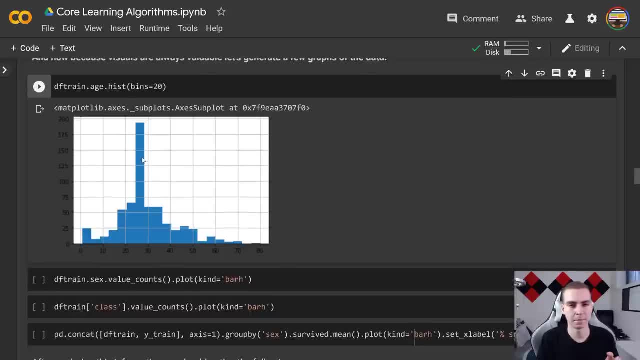 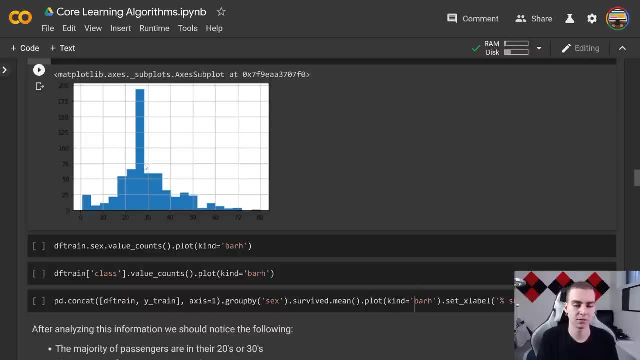 This is good information to know because that's going to introduce a little bit of bias into, kind of our linear correlation graph, right? So, just understanding, you know that we have like a large subset. there's some outliers here, like there's one person, that's. 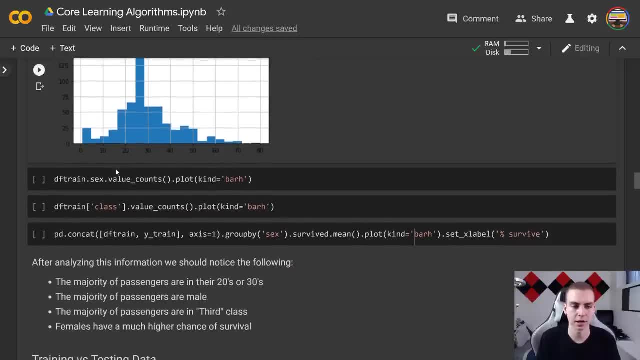 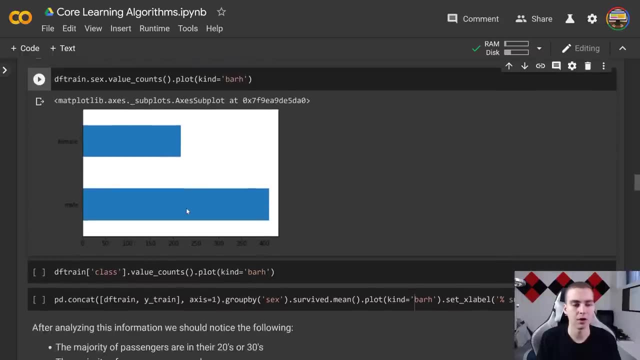 80, right over here, a few people that are 70, some important things to kind of understand before we move on to the algorithm. So let's look at the sex values now. So this is how many female and how many male. we can see that there's many more males than there is. 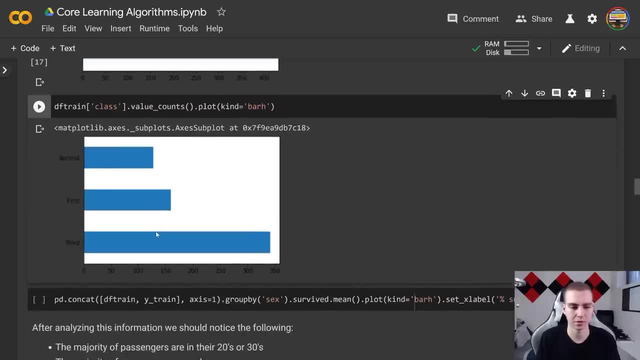 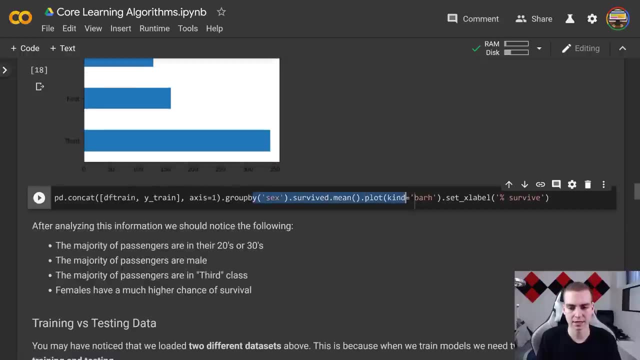 females. we can have a look at the class So we can see if they're in first, second, third class. most people are in third, then followed by first and then second, And then, lastly, we can look at what is this that we're doing? Oh, the percentage survival by sex. 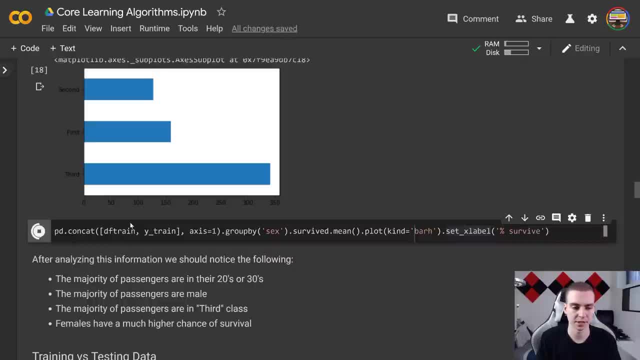 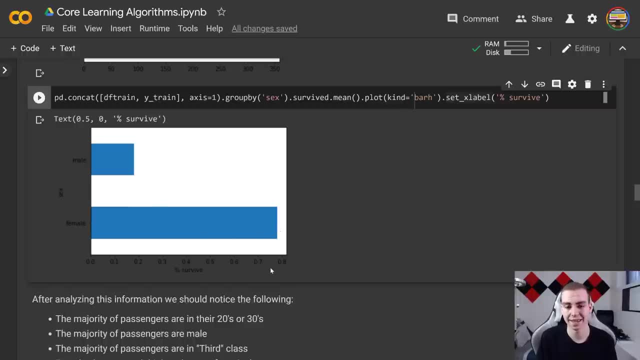 So we can see how likely a specific person or a specific sex is to survive. just by plotting this So we can see that males have about a 20% survival rate, whereas females are all the way up to about 78%. So that's important to understand. that kind of confirms that. 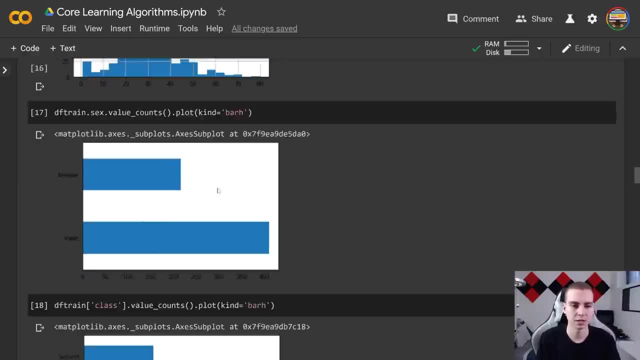 what we were looking at before in the data set when we were exploring it, and you don't need to do this every time that you're looking at it. We're looking at a data set, but it is good to kind of get some intuition about it. So 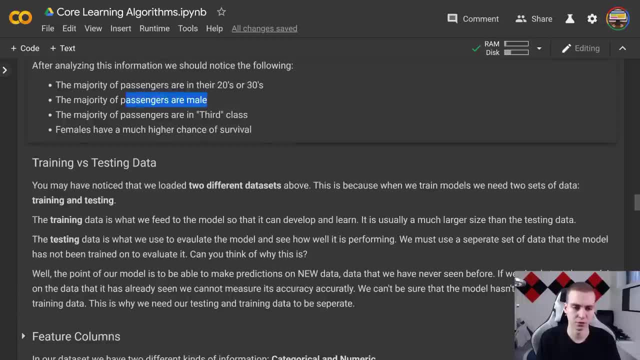 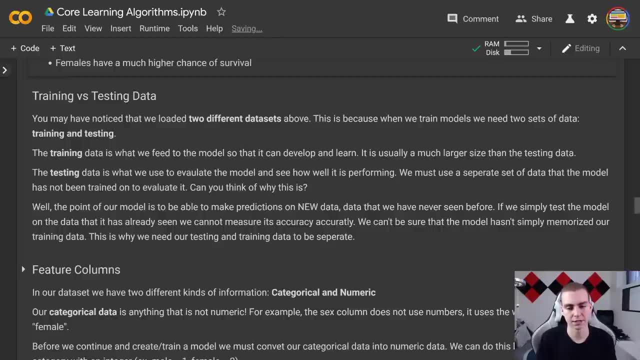 this is what we've learned so far. the majority of passengers are in their 20s or 30s. the majority passengers are male, they're in third class and females have a much higher chance of survival, kind of already knew that. Alright, so training and testing data sets. Now we 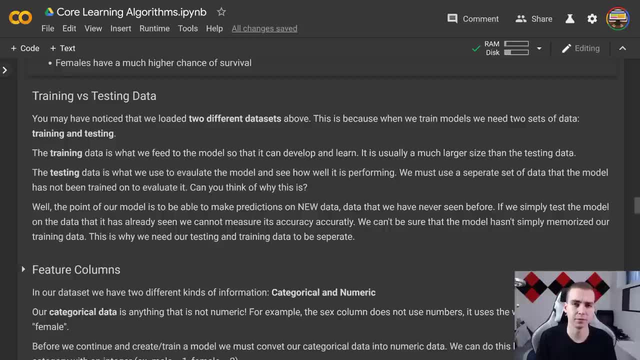 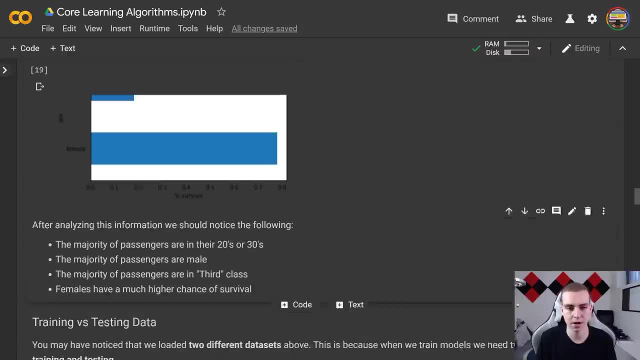 already kind of went through this, so I'll skim through it quickly. Essentially, what we did above is load in two different data sets. The first data set was that training data set which had the shape of 627 by nine, And what I'm actually going to do is create. 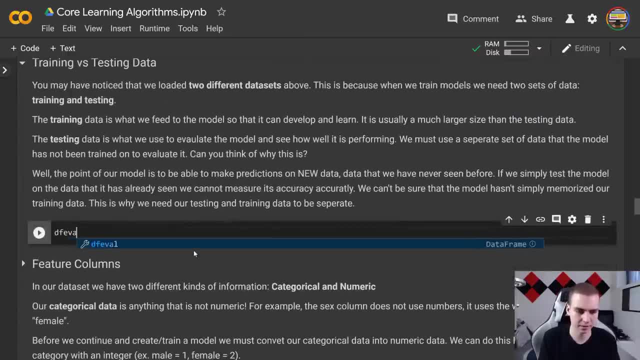 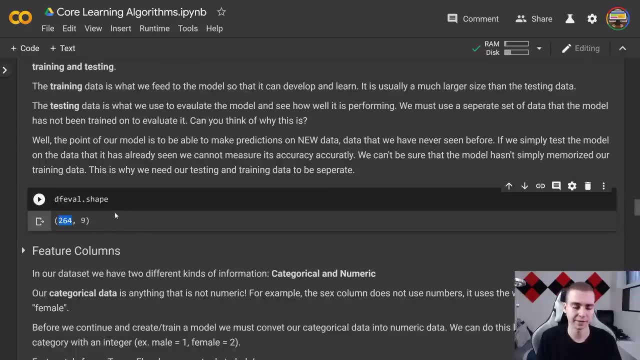 a code block here And just have a look at what was this df eval dot shape to show you how many entries we have in here. So here in our testing data set you can see we have significantly less at 264 entries or rows, whatever you. 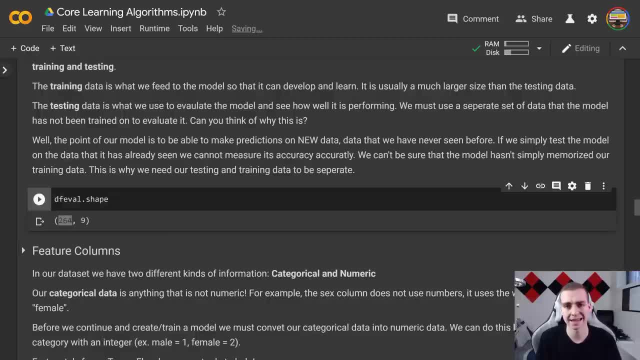 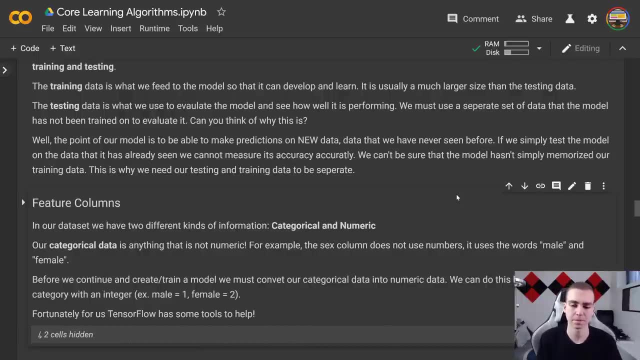 want to call them. So that's how many things we have to actually test our model. So what we do is we use that training data to create the model and then the testing data to evaluate it and make sure that it's working properly. So these things are important Whenever we're. 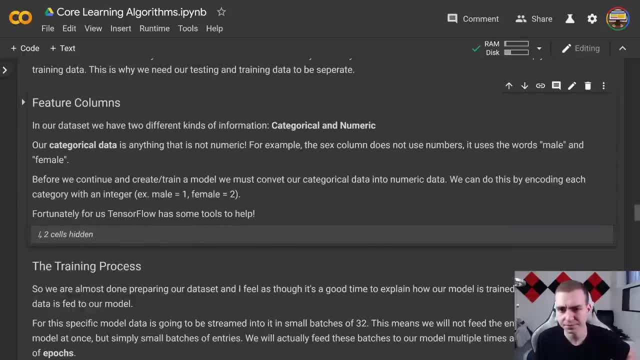 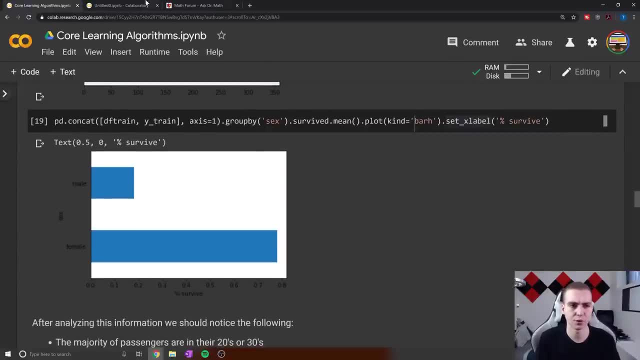 doing machine learning models. we typically have testing and training data, And yeah, that is pretty much it. Now I'm just going to take one second to copy over a lot of this code into the kind of other notebook I have, just so we can see all of it at once, And then we'll be back. 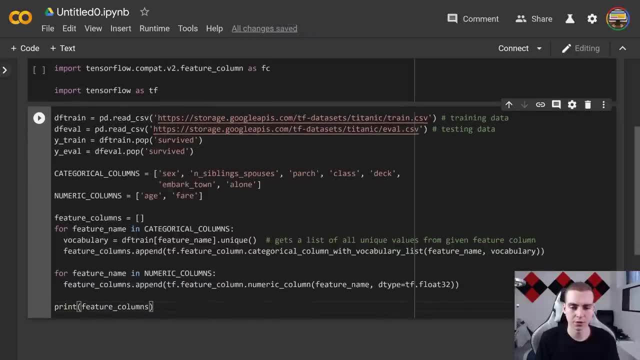 and we'll get into actually making the model. Okay, so I've copied in some code here. I know this seems like a lot of kind of gibberish right now, But I'm going to break down line by line what all this is doing and why we have this here. But we first need to discuss. 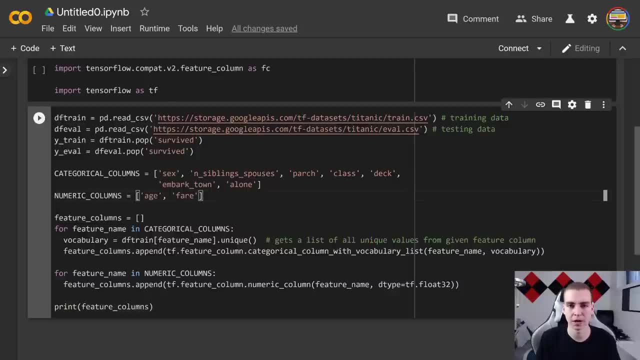 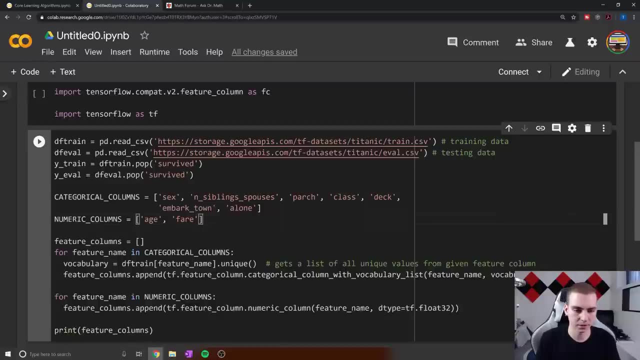 something called feature columns and the difference between categorical and numeric data. So get categorical data is actually fairly common Now when we're looking at our data set and actually I can open, I don't have it open in Excel, So I'm going to go ahead and open. 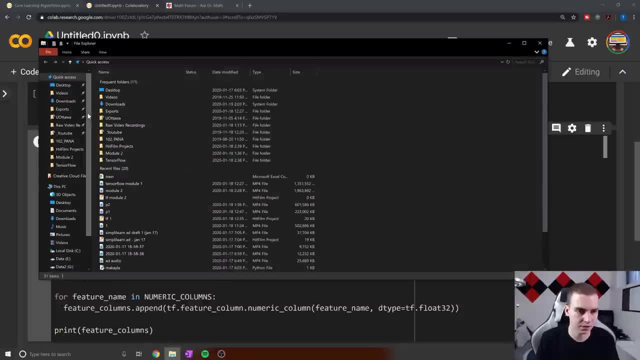 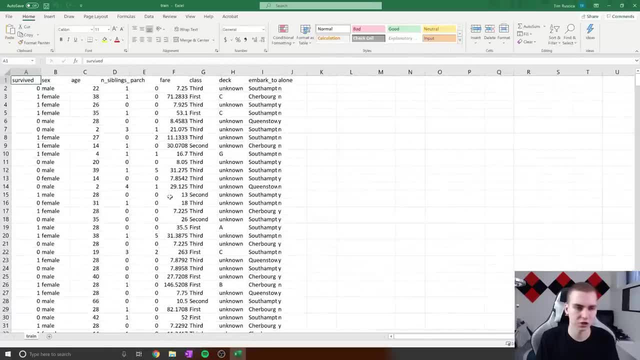 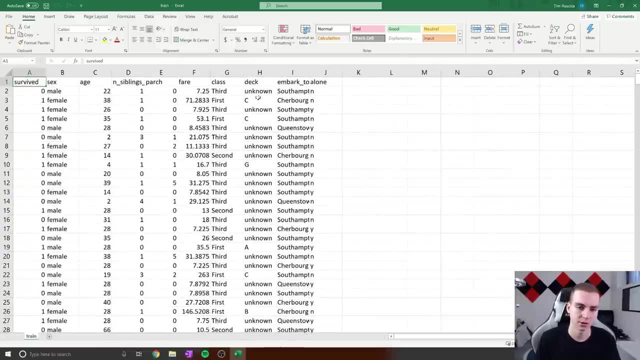 is this Train? Okay, awesome. So we have this Excel data sheet here And we can see what a categorical data or categorical data is, is something that's not numeric. So, for example, unknown, see first third city. And why, Right, So anything that has different. 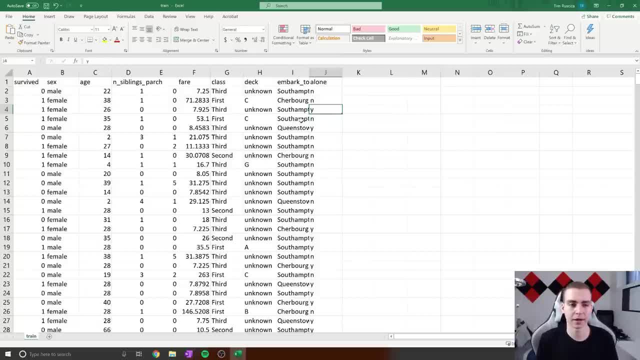 categories. there's going to be like a specific set of different categories there could be. So, for example, for age kind of the set of values we could have for age, we'll look is numeric, So that's different. But for categorical, we can have male or we can have female And 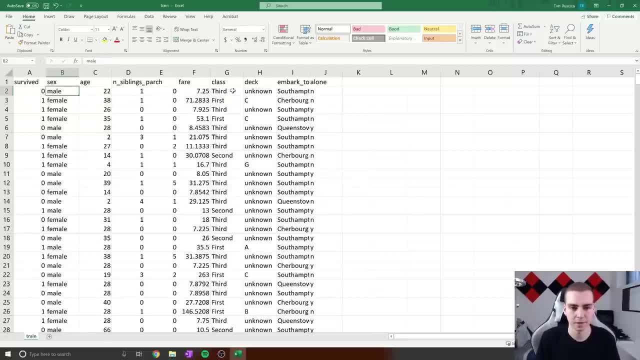 I suppose we could have other, but in this data set we just have male and we just have female. For class we can have first, second, third. for deck, we can have unknown CA, I'm sure through all the letters of the alphabet, but that is still considered categorical. 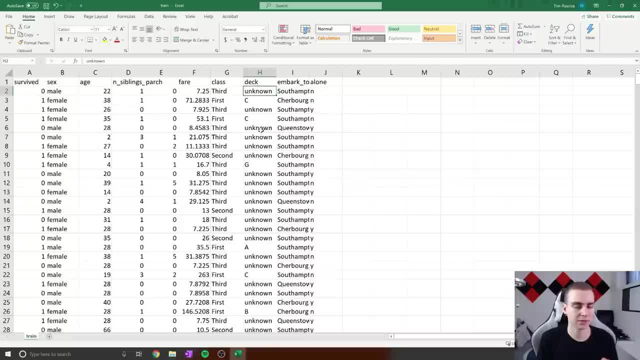 Now, what do we do with categorical data? Well, we always need to transform this data into numbers somehow. So what we actually end up doing is we encode this data using an integer name. So, for the example of male and female, what we might say- and this is what we're- 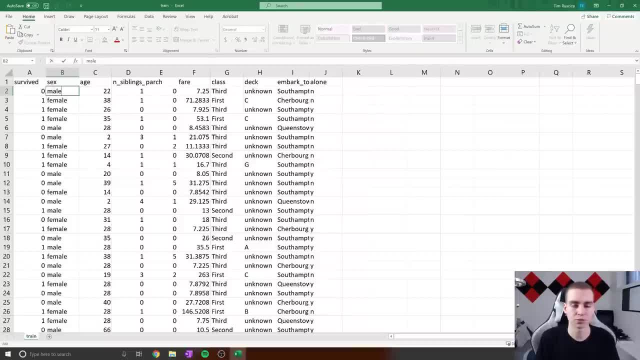 going to do in a second is that female is represented by zero and male is represented by one. We do this because, although it's interesting to know what the actual class is, the model doesn't care right female and male, it doesn't make a difference to it, it just needs to. 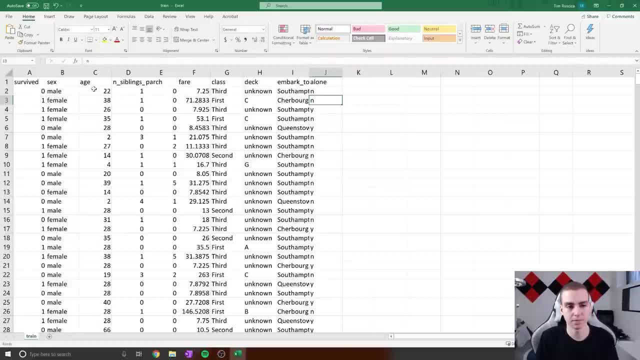 know that those values are, the different are different, or those values are the same. So rather than using strings and trying to find some way to pass that in and do math with that, we need to turn those into integers. So we turn those into zeros and ones, right. 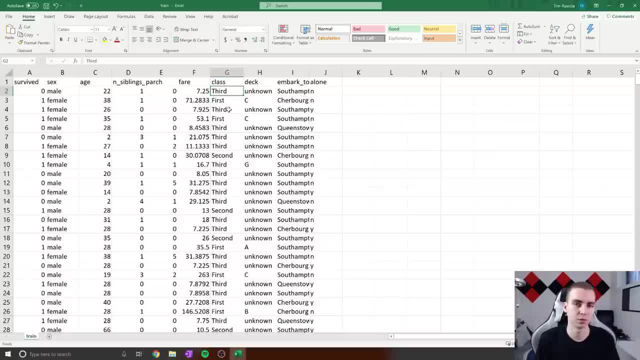 Now for class, right? so first, second, third, you know, you guys can probably assume what we're going to encode this with. we're going to encode it with 012.. Now again, this doesn't necessarily need to be in order. So third could be represented by one and first could. 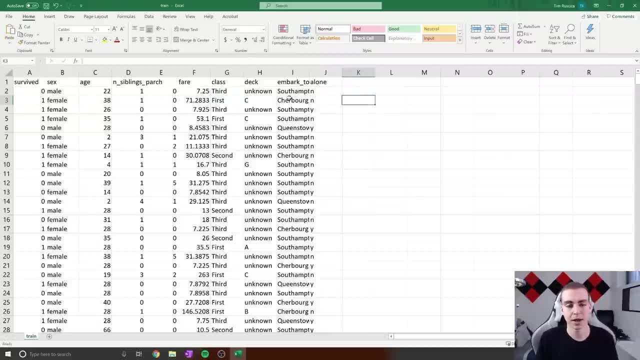 be represented by two right. It doesn't need to be in order, it doesn't matter, So long as every third has the same number, every first has the same number and every second has the same number. And then same thing with that, same thing with embark, and same thing. 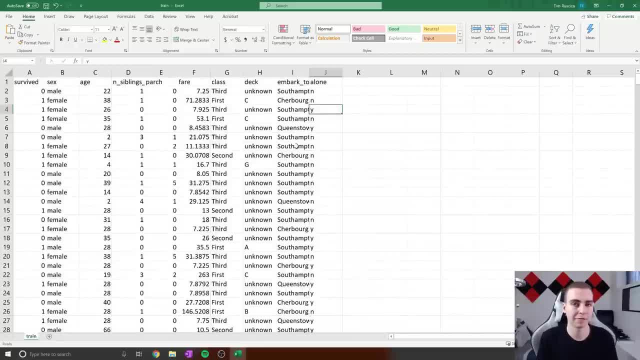 with alone. Now we could have an instance where you know we've encoded every single one of these values with a different value. So in the case, you know, rare occasion- where there's one category that's categorical and every single value in that category is different, then we will have you know 627. In this. 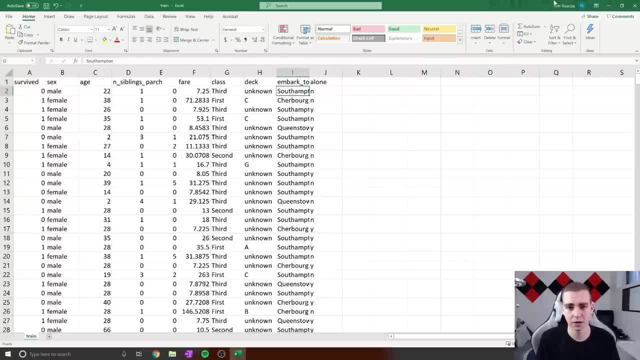 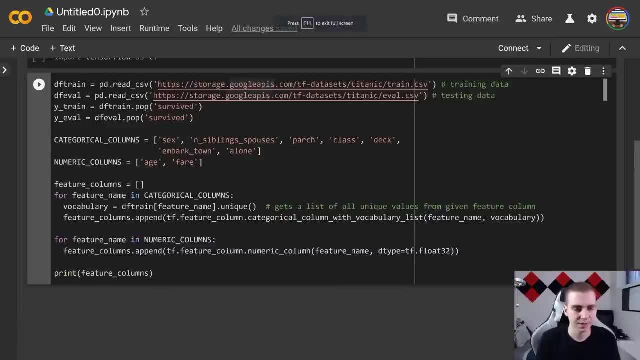 instance, different encoding labels that are going to be numbers. that's fine, we can do that, And actually we don't really need to do that because you're going to see how TensorFlow can handle that for us. So that's categorical data. numeric columns are pretty straightforward. 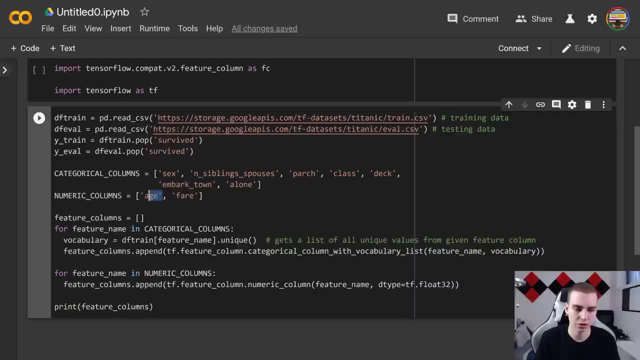 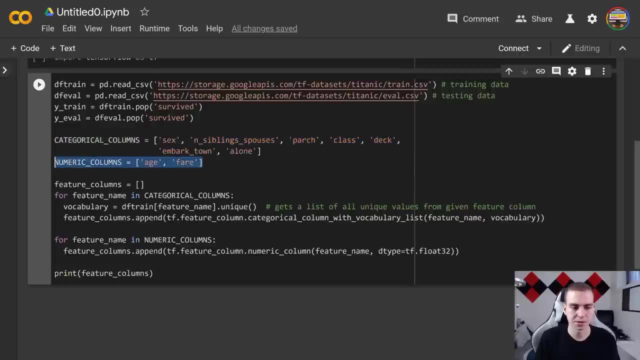 They're anything that just have integer float values already. So in this case, age and fair, And yeah. so that's what we've done. we've just defined our categorical columns here and our numeric columns here. This is important because we're going to loop through them, which we're doing. 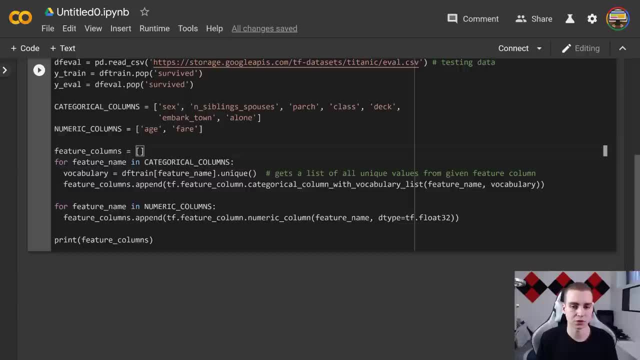 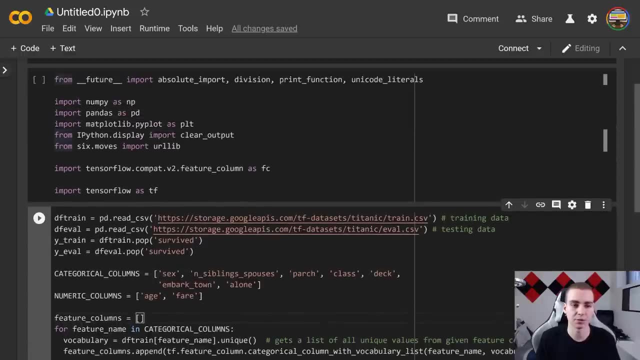 here to create something called feature columns. feature columns are nothing special. they're just what we need to feed to our linear estimator and linear model to actually make predictions. So kind of our steps here that we've gone through so far is: import, load the data set. 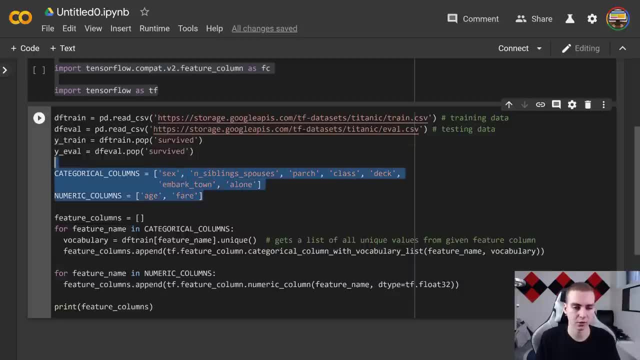 explore the data set, make sure we understand it, create our categorical columns and our numeric columns. So I've just hard coded these in right like sex, parche class, class, class, deck alone, all these ones. And then same thing with the numeric columns, And then 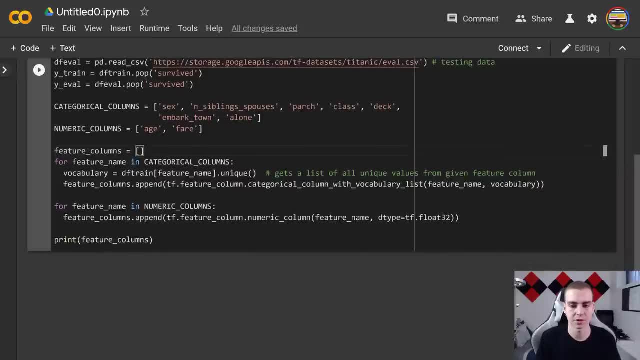 for a linear estimator. we need to create these as feature columns using some kind of advanced syntax which we're going to look at here. So we create a blank list, which is our feature columns, which will just store our different feature columns. we loop through. 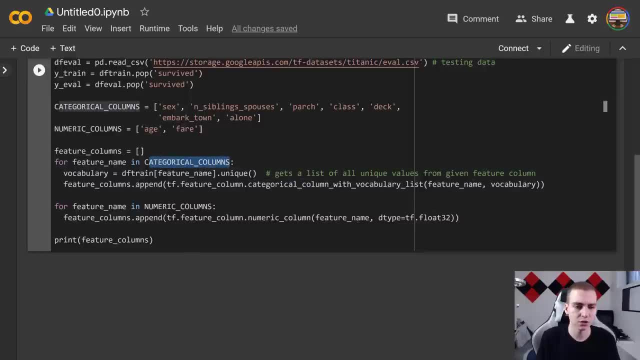 each feature name in the categorical columns And what we do is we define a vocabulary which is equal to the data frame at that feature name. So first we would start with sex, then we go and siblings, then we go parche, then we go class. 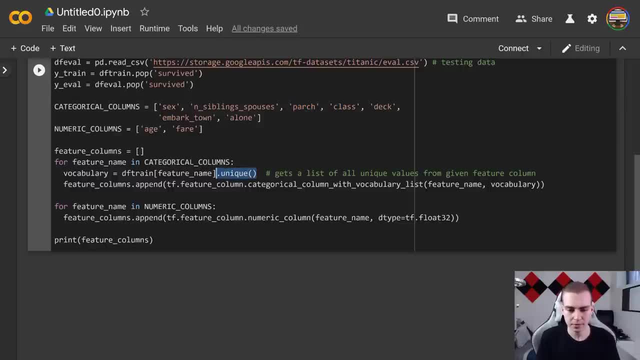 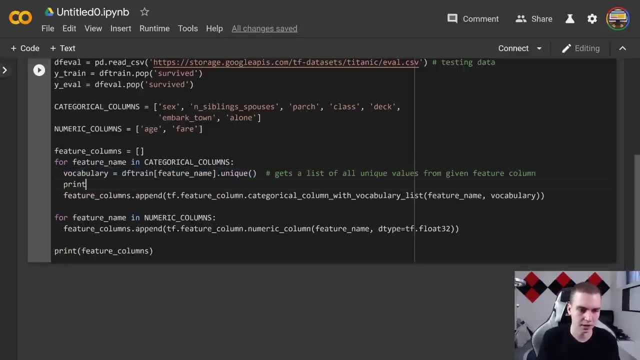 And we get all of the different unique values. So that's actually what this does. dot unique gets a list of all unique values from the feature column And I can print this out. She'll put this in a different line. we'll just take this value and have a look at actually. 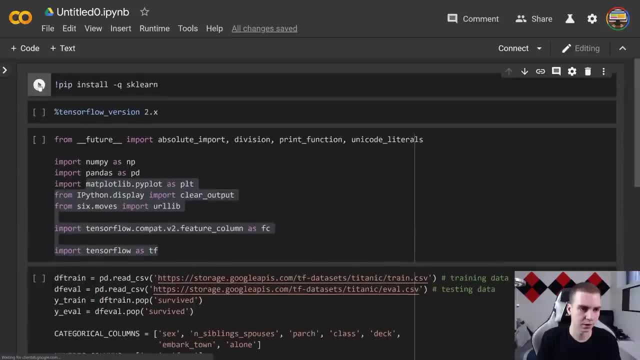 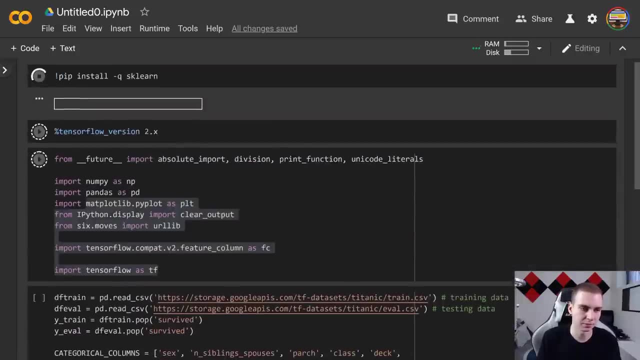 what this is right. So if I run ice, we'll have to run all these in order, And then we'll create a new code block. while we wait for that to happen, Let's see if we can get this installing fast enough. 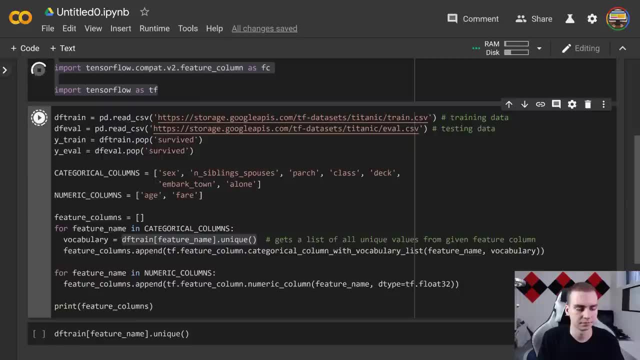 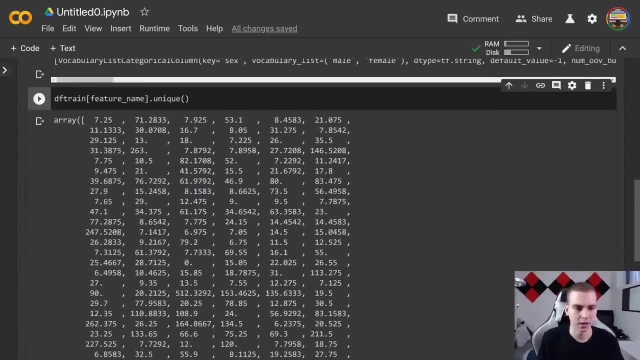 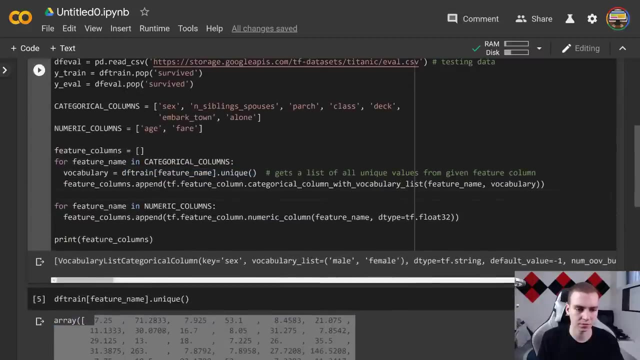 Run, run, run. Okay, now we go to DF train And we can see. this is what this looks like. So these are all the different unique values that we had in that specific feature name. Now, that feature name was: what categorical columns, Oh, what I do- feature name of. sorry, that's going to. 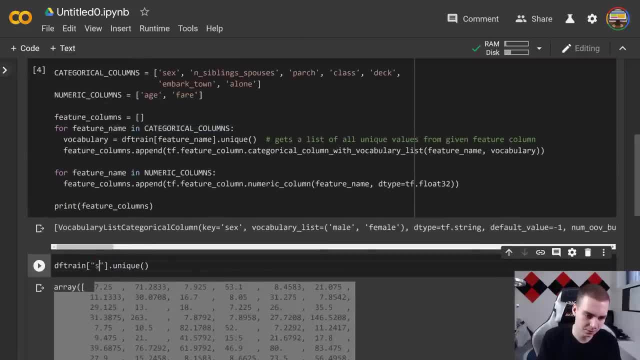 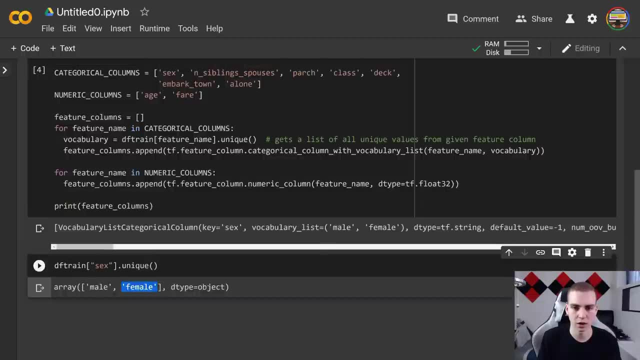 be the unique one. Let's just put, rather than feature name, Let's put sex right and let's have a look at what this is, So we can see that the two unique values are male and female. Now I actually want to do. what is it? 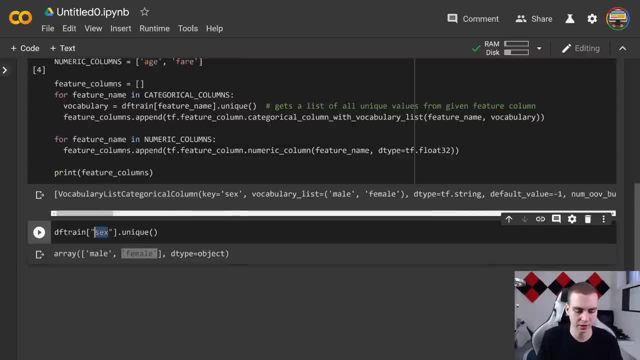 embark town And I want to see what this one is, So how many different values we have. So we'll copy that in And we can see we have Southampton- cannot pronounce that- And then the other cities and unknown, And that is kind of how we get the unique value. So that's. 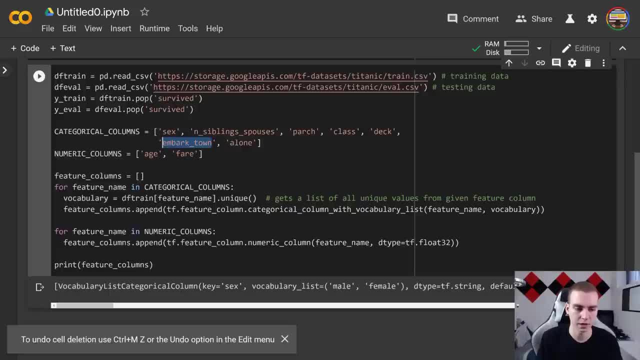 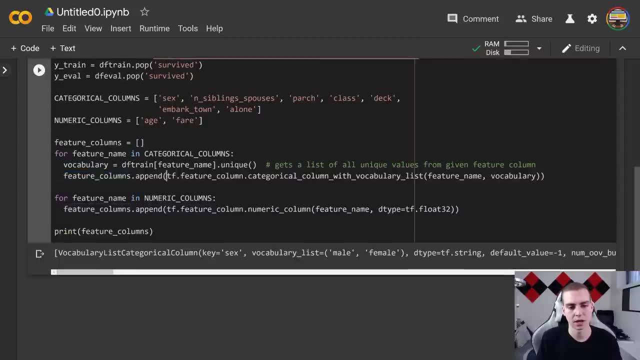 what that method is doing there. Let's actually delete this code block because we don't need it anymore. Alright, so that's what we do. And then what we do down here is we say feature columns, dot append. So just add to this list the TensorFlow feature column dot categorical. 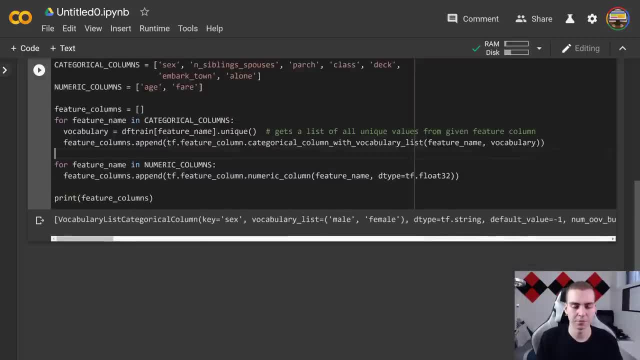 column with vocabulary list. Now, I know this is a mouthful, But this is kind of something again you're just going to look up when you need to use it right. So understand that you need to make feature columns for linear regression. 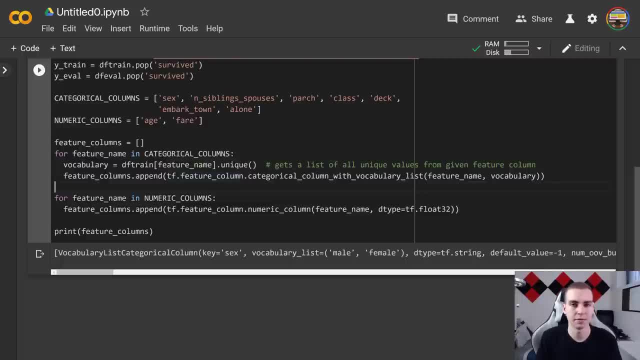 you don't really need to completely understand how, but you just need to know that that's something you need to do, And then you can look up the syntax and understand. So this is what this does. This is actually going to create for us a column. it's going to be. 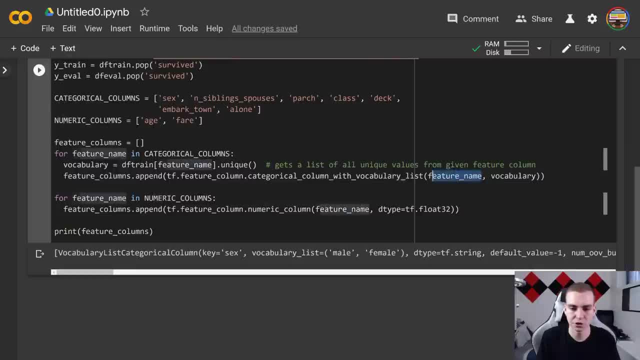 in the form of a like NumPy array kind of that has the feature name, so whatever one we've looped through, and then all of the different vocabulary associated with it. Now, we need this because we just need to create this column So that we 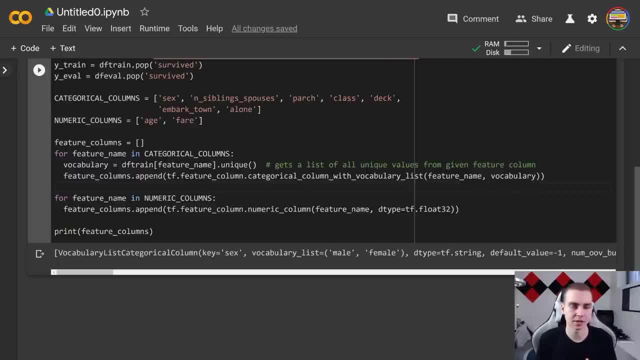 can create our model using those different columns, if that makes any sense or a linear model needs to have you know all the different columns we're going to use. it needs to know all of the different entries that could be in that column and needs to know whether 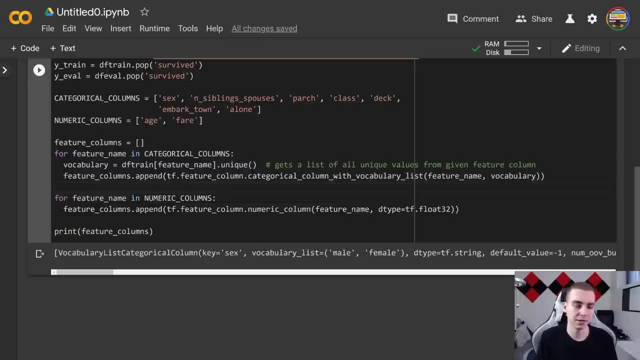 this is a categorical column or a numeric column. In previous examples, what we might have done is actually change the data set manually, So encoded it manually. TensorFlow just can do this for us now in TensorFlow 2.0. So we'll just use that tool, Okay so. 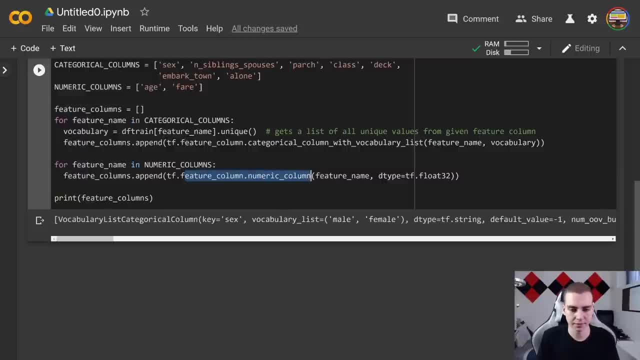 that's what we did with these feature columns. Now for the numeric columns- a little bit different. it's actually easier. All we need to do is give the feature name and whatever the data type is and create a column with that. So notice, we don't, we can omit this unique value, because we know when. 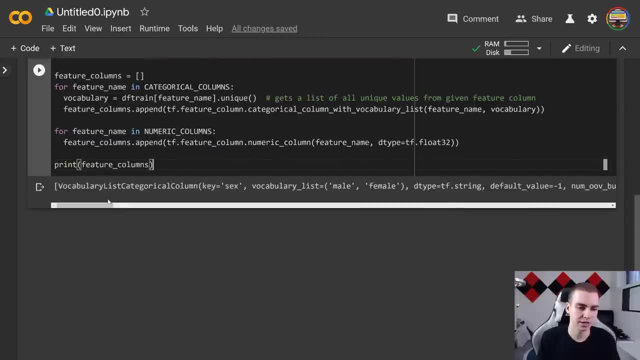 it's numeric, that you know there could be an infinite amount of values. And then I've just printed out the feature columns. you can see what this looks like. So, vocabulary list- categorical column gives us the number of siblings, And then the vocabulary list. 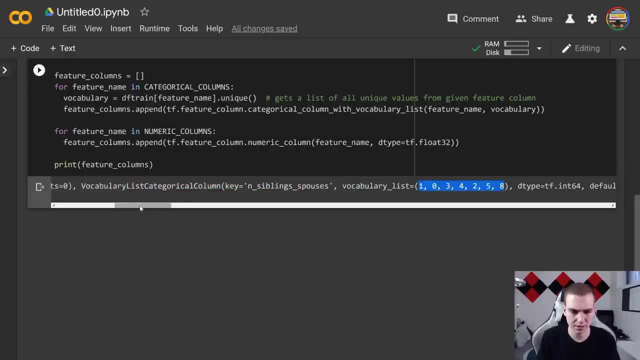 is: these are all the different encoding values that is created And then same thing. you know we could go down here parts. these are different encodings So they're not necessarily in order- is like what I was talking about before. Let's go to a numeric column And 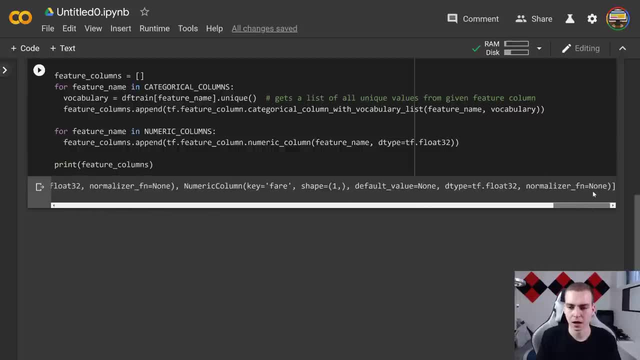 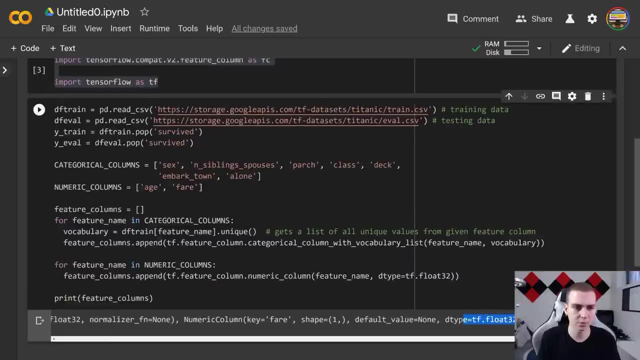 let's do a numeric one. What do we have here? Yeah, so for a numeric column, just as the key, that's the shape we're expecting And this is the data type. So that is pretty much it for actually loading these in. So now it's almost time to create the model. So what we're? 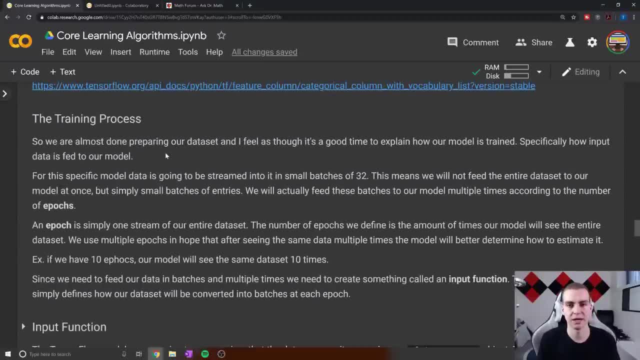 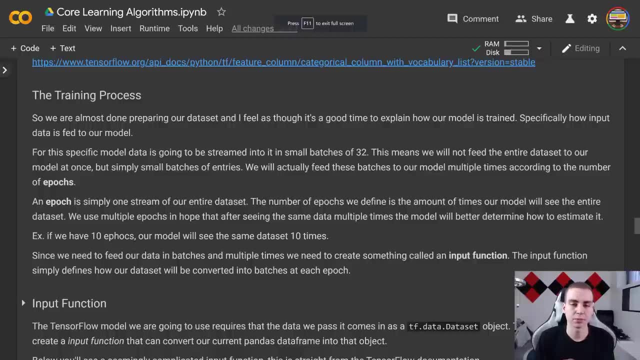 going to do to create the model now is talk about first the training process and training some kind of, you know, machine learning model. Okay, so the training process Now. the training process of our model is actually fairly simple, at least for a linear model, So we're going. 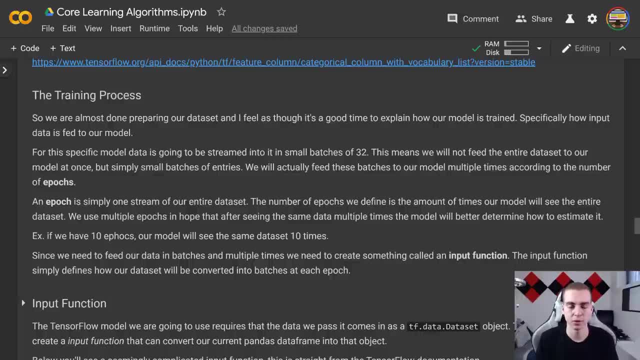 to go ahead and create a model, And we're going to go ahead and create a model, And we're going to go ahead and create a model. Now, the way that we train the model is: we feed it information, right, So we feed it that, those data points from our data set. 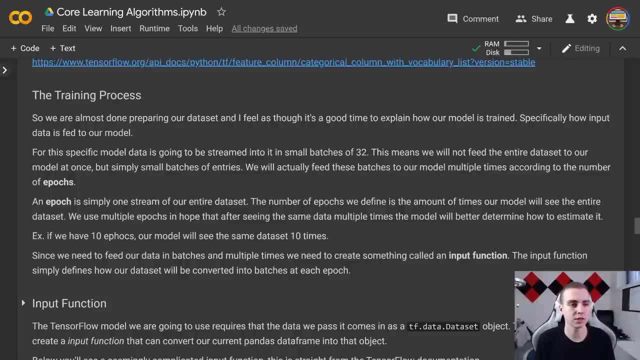 But how do we do that? Right, Like, how do we feed that to the model? Do we just give it all at once? Well, in our case we only have 627 rows, which isn't really that much data like we can fit that in RAM in our computer, right, But what if we're training a crazy? 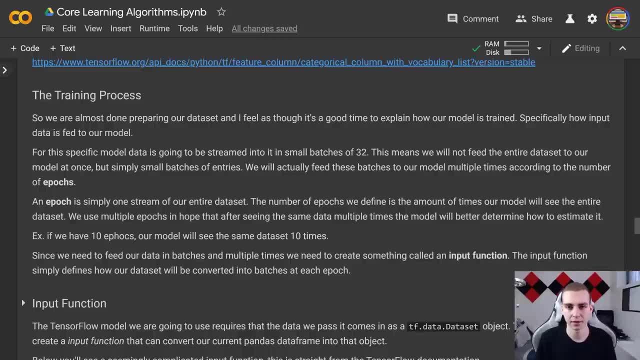 machine learning model and we have, you know, 25 terabytes of data that we need to pass it. we can't load that into RAM- at least I don't know any RAM that's that large- So we need to find a way that we can kind of load that into our computer. So we need to find 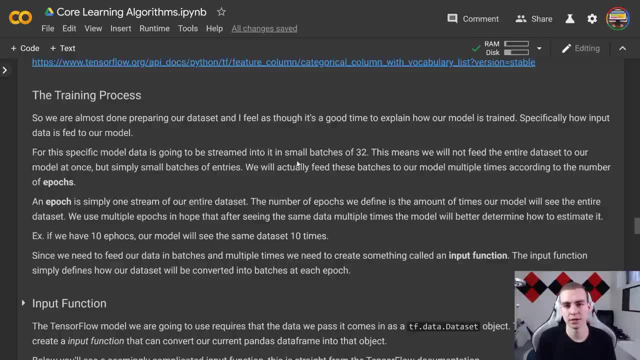 a way that we can kind of load that into our computer. So we need to find a way that we can load it in what's called batches. So the way that we actually load this model is we load it in batches. now we don't need to understand really kind of how this process works and 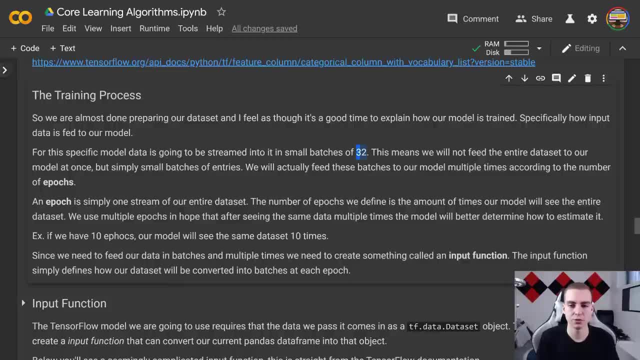 how batching kind of occurs. What we do is give 32 entries at once to the model. Now the reason we don't just feed one at a time is because that's a lot slower we can load, you know, a small batch size of 32 that can increase our speed dramatically, and that's. 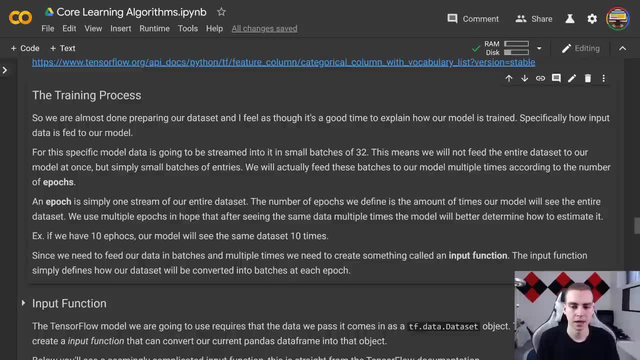 kind of a lower level understanding, So I'm not going to go too far into that. Now that we understand, we kind of load it in batches, right right, so we don't load it entirely all at once, we just load a specific set of kind of elements. 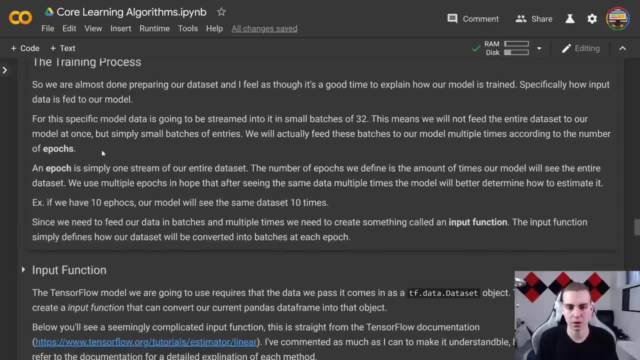 as we go, What we have is called epochs. Now, what are epochs? Well, epochs are essentially how many times the model is going to see the same data. So what might be the case right when we pass the data to our model the first time? it's pretty bad, like it looks at the model. 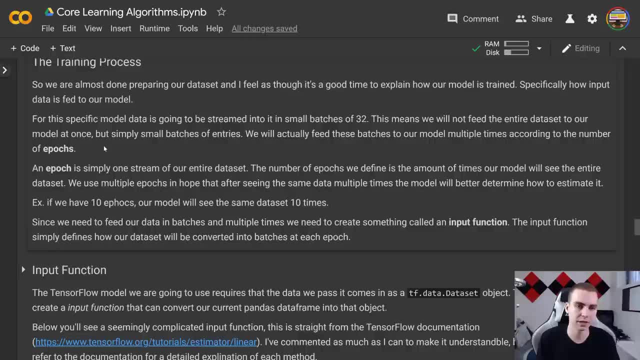 creates our line of best fit. but it's not great, it's not working perfectly. So we need to use something called an epoch, which means we're just going to feed the model, feed the data again, but in a different order. So we do this multiple times so that the model will look at a data. 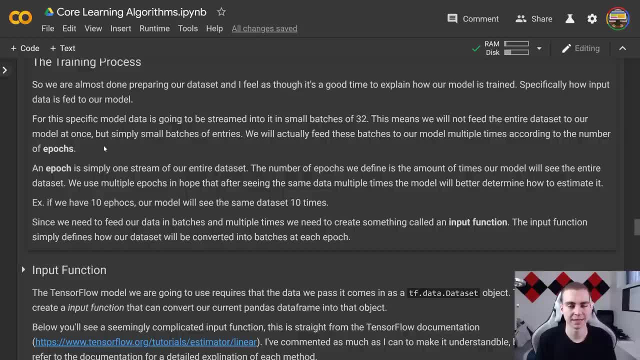 look at the data in a different way, in kind of a different form, and see the same data a few different times and pick up on patterns, because the first time it sees a new data point, it's probably not going to have a good idea how to make a prediction for that. So we can feed it more and 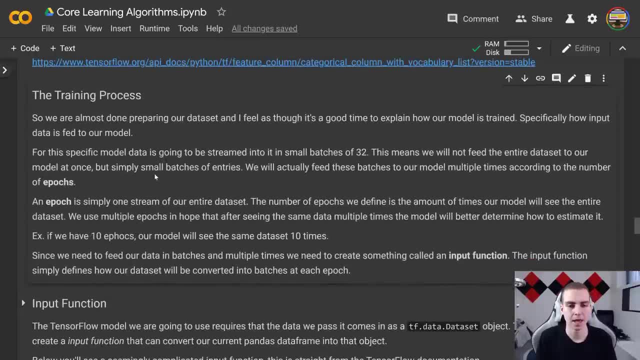 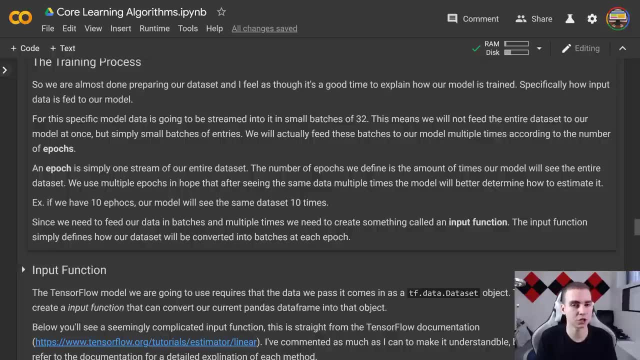 more and more than you know, we can get a better prediction. Now this is where we talk about something called overfitting, though sometimes we can see the data too much. we can pass too much data to our model, To the point where it just straight up memorizes those data points, And it's it's really good at. 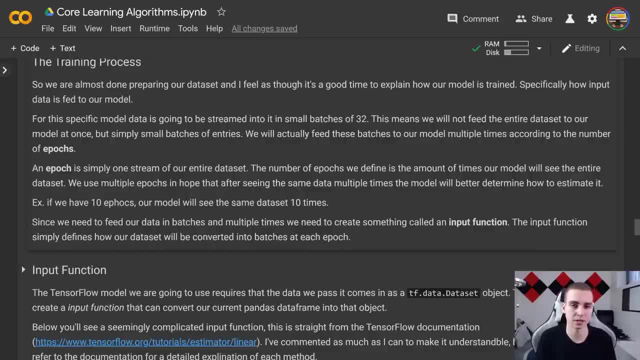 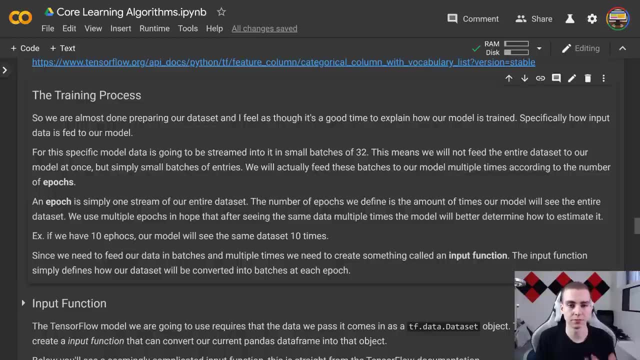 classifying for those data points. But when we pass it some new data points, like our testing data for example, it's horrible at kind of, you know, classifying those. So what we do to kind of prevent this from happening is we just make sure that we start with like a lower amount of epochs. 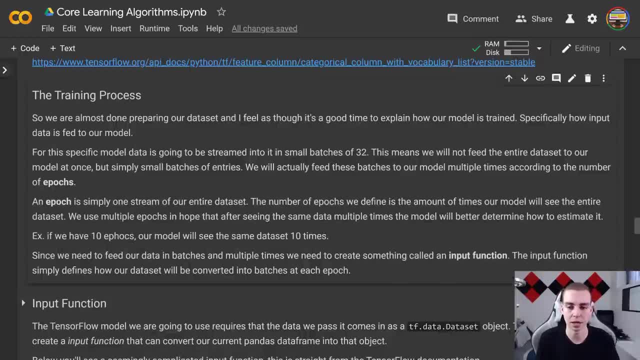 and then we can work our way up and kind of incrementally change that if we need to, you know, go higher. right, we need more epochs, So yeah, so that's kind of it for epochs. Now I will say that this training process kind of applies to all the different- what is it? machine learning models. 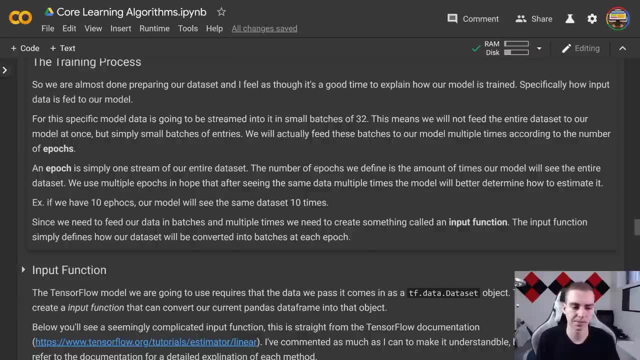 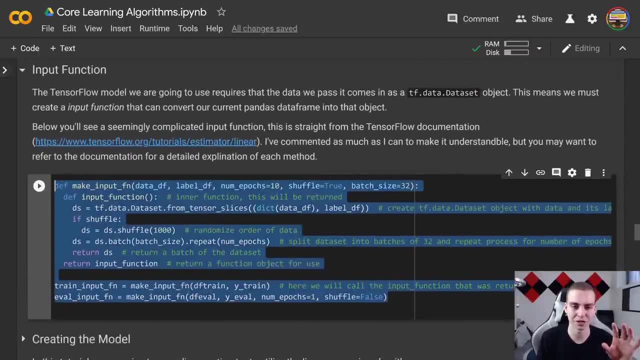 that we're going to look at. we have epochs, we have batches, we have a batch size and now we have something called an input function. Now, this is pretty complicated. This is the code for the input function. I don't like that we need to do this, but it's necessary. So, essentially, what an? 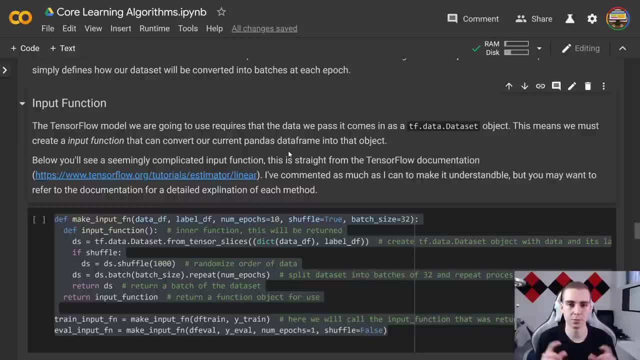 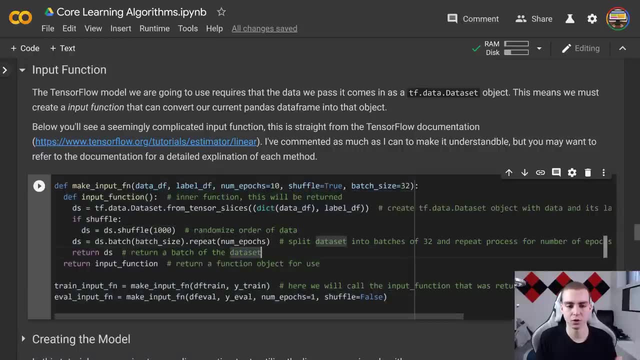 input function is is the way that we define how our data is going to be broke into epochs and into batches to feed to our model. Now, these you probably aren't going to really need to code like from scratch by yourself, But this is the one I've just stolen. 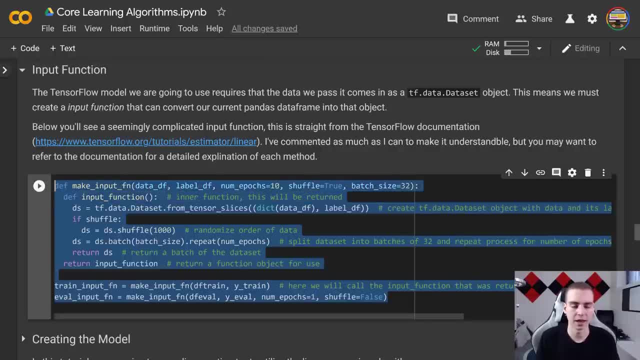 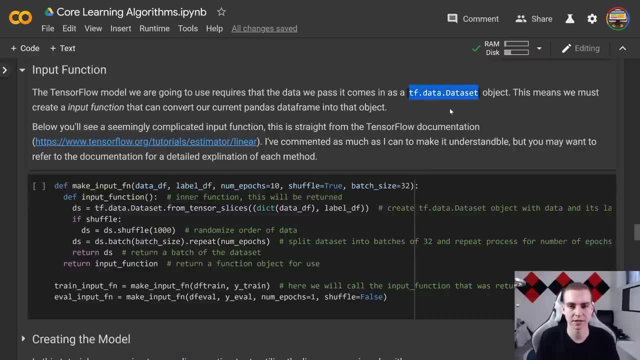 from the TensorFlow website, pretty much like everything else that's in the series, And what this does is it takes our data and encodes it in a tf dot, data dot- data set object. Now, this is because our model needs this specific object to be able to work. it needs to see a data set object to 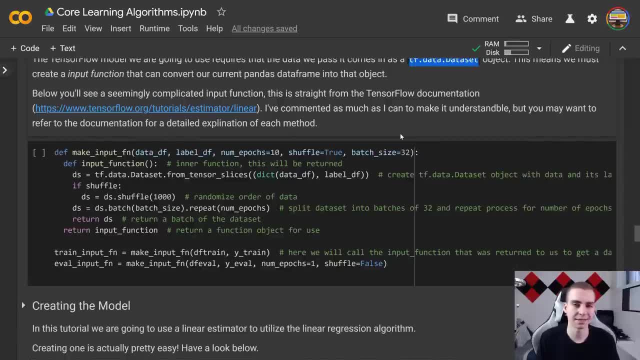 be able to use that data to create the model. So what we need to do is take this pandas data frame. we need to turn it into that object, And the way we do that is with the input function, So we can see that what this is doing here. 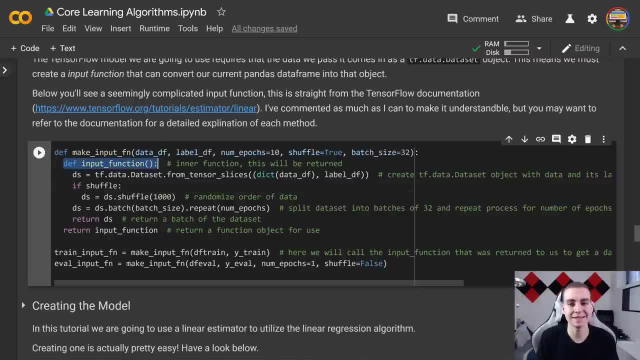 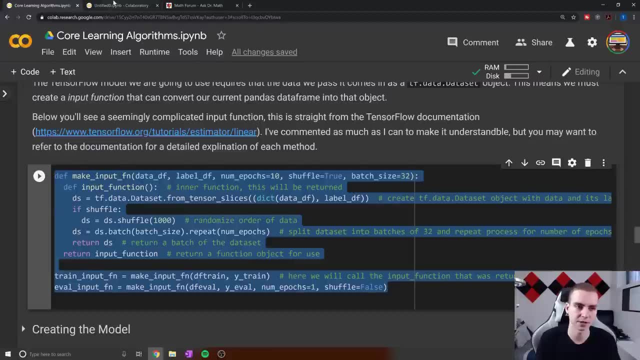 so this is make input function. we actually have a function defined inside of another function. I know this is kind of complicated for some of you guys, but and what I'm actually gonna do? sorry, I'm gonna just copy this into the other page because I think it's easier to explain without. 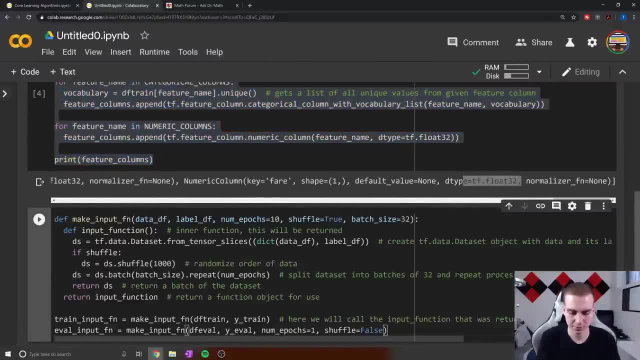 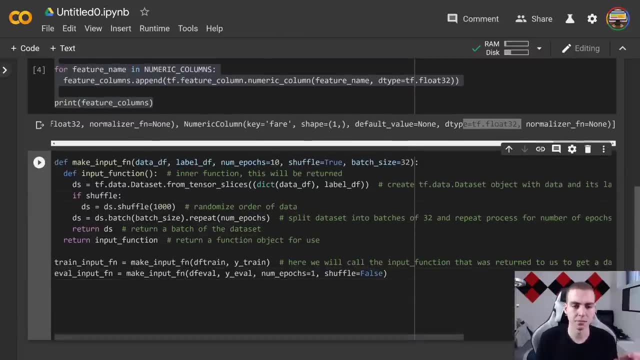 all the text around. So let's create a new code block, Let's paste this in And let's have a look at what this does. So actually let me just tab down. Okay, so make input function. we have our parameters data. 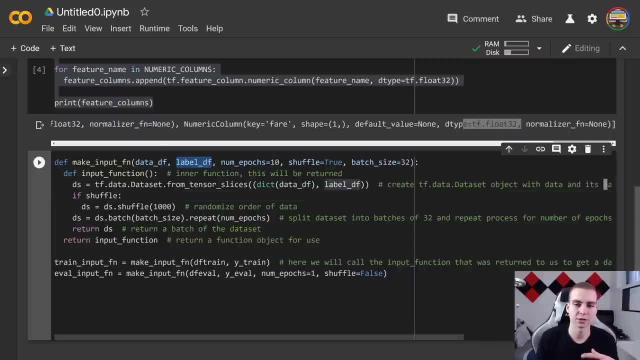 data frame, which is our pandas data frame, our label data frame which stands for those labels, So that, why train? or that eval, Why eval? right, We have a number of epochs, which is how many epochs we're going to do? we set the default 10 shuffle, which means: are we going to shuffle our? 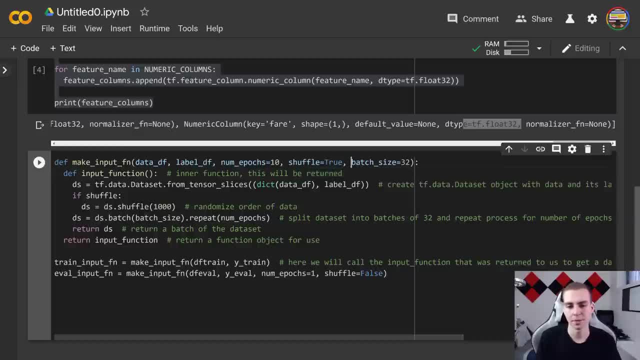 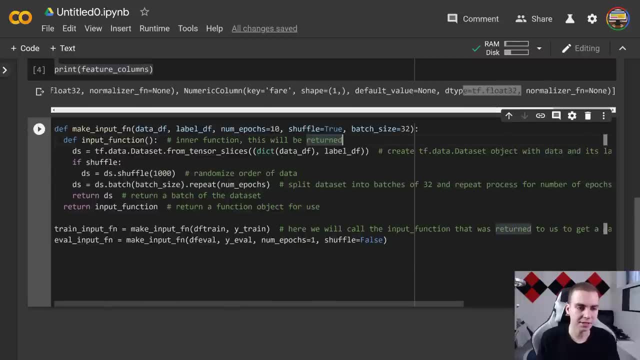 data and mix it up before we pass it to the model. and batch size, which is how many elements are we going to give to the data, to the model, While it's training at once. Now, what this does is we have an input function defined inside of this function. 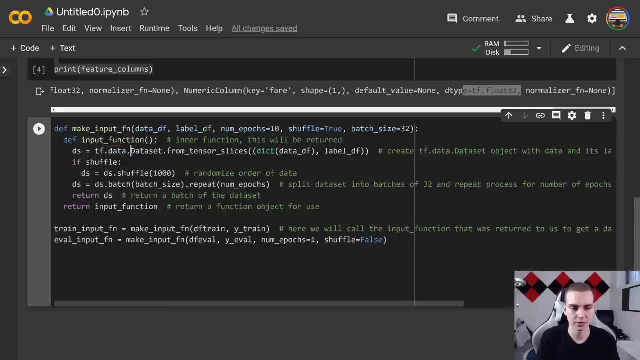 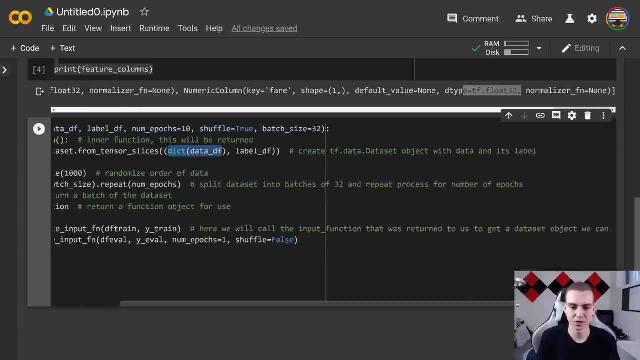 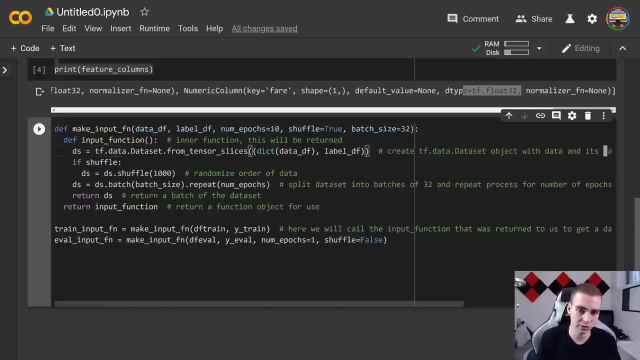 And we say: data set equals tensor frame dot data dot data set from a tensor slices dict data frame label data. Now what this does- and we can read the comment- I mean create a tu f dot data dot data set object with the data and its label. Now I can't explain to you like how this works on a. 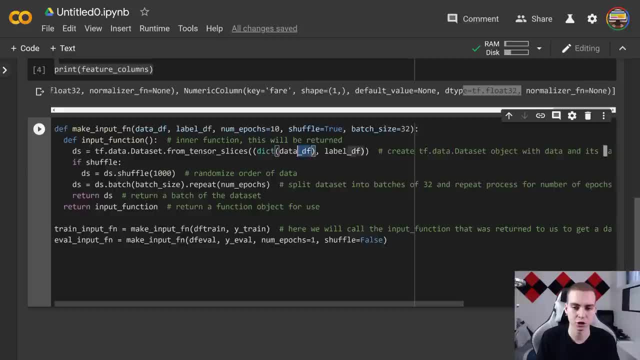 lower level. But essentially we pass a dictionary representation of our data frame, which is whatever we passed in here, And then we pass the label data frame, which is going to be, you know, all those y values, and we create this object And that's what this line of code does. So tf data dot. data set from. 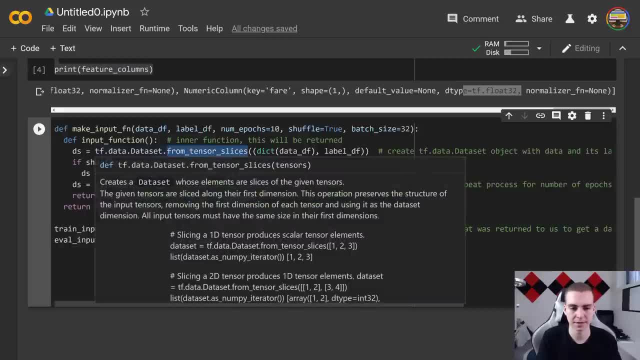 tensor slices, which is just what you're going to use. I mean, we can read this documentation, create a data set whose elements are slices of the given tensors. the given tensors are sliced along their first dimension. this operation preserves the structure of the input tensors. 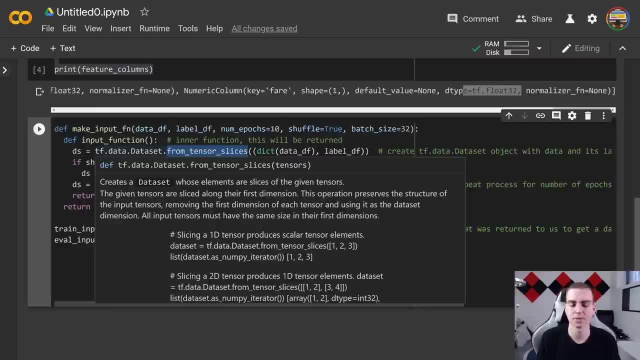 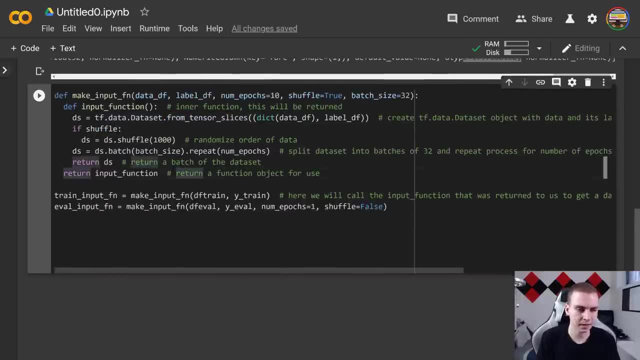 removing the first dimension of each tensor and using it as the data set dimension. So I mean you guys can look at that like, read through the documentation if you want, But essentially what it does is create the data set object for us. Now if shuffle. 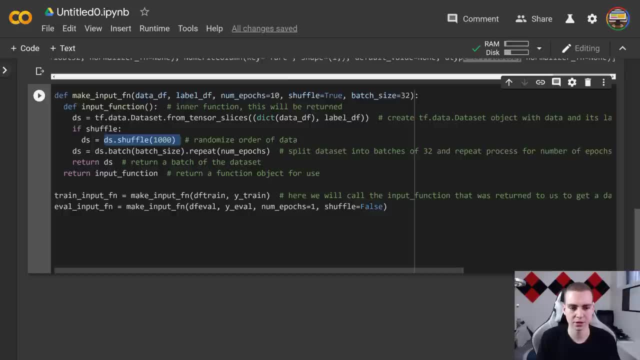 ds equals ds dot shuffle 1000,. what this does is just shuffle the data set. you don't really need to understand more than that. And then what we do is we see data set equals data set dot batch the batch size, which is going to be 32.. And then repeat for the number of epochs. 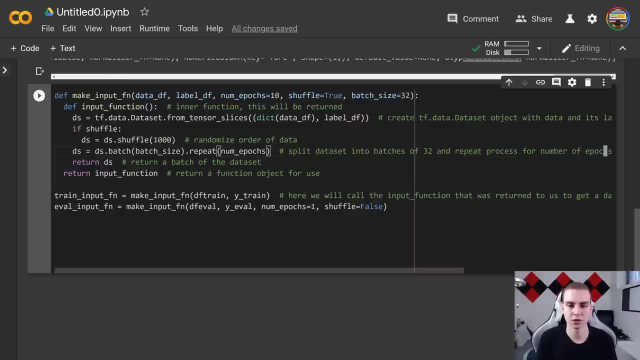 So what this is going to do is essentially take our data set and split it into the number of- I don't want to what do I want to call it like blocks that are going to be passed to our model. So we can do this by knowing the batch size. it obviously knows how many. 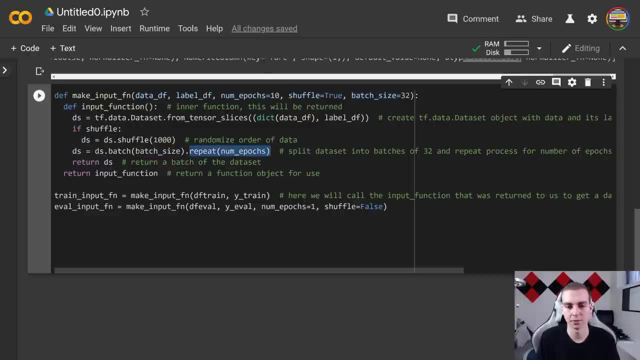 elements, because that's the data set object itself, and then repeat number of epochs. So this can figure out. you know how many one, how many blocks do I need to split it into, to feed it to my model? Now return data set simply from this function here. 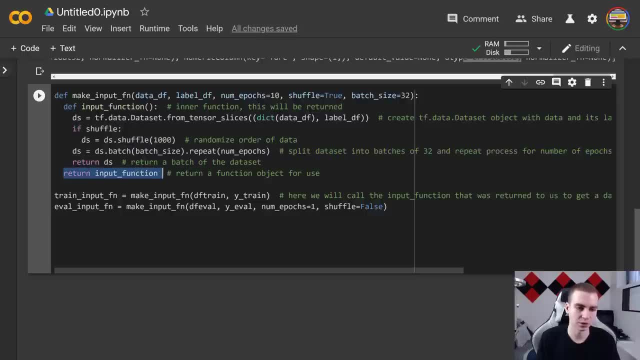 we'll return that data set object And then, on the outside return, we actually return this function. So what this out exterior function does- and I'm really just trying to break this down So you guys understand- is make an input function. it literally makes a function and returns the. 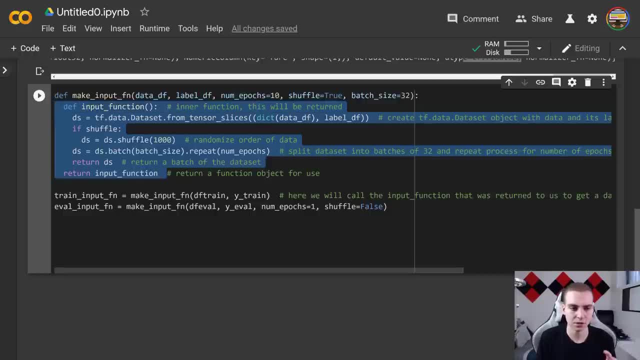 function object to wherever we call it from. So that's how that works. Now we have a train input function and an eval input function, And what we need to do to create these is just use this function that we've defined above. So we say: make input function DF, train. why train? so our data? 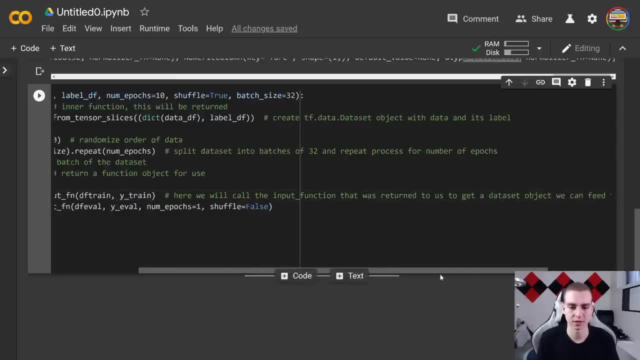 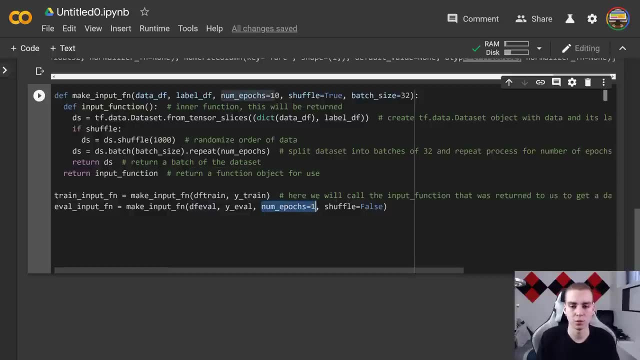 frame for training and our data frame for the labels of that, So we can see the comments. you know, here we will call the input function right and then eval train. So it's going to be the same thing except for the evaluation. we don't need to shuffle the data because we're not training. 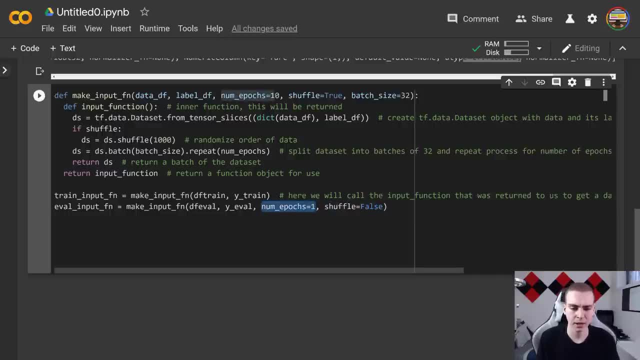 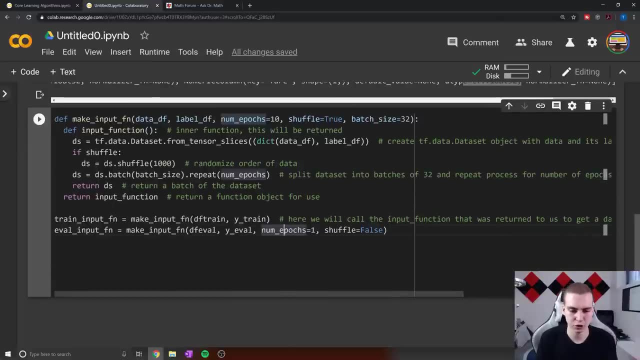 it. we only need one epoch, because, again, we're just training it, And we'll pass the evaluation data set in the evaluation value from Y. Okay, so that's it for making the input function. Now, I know this is complicated, But that's the way we have to do it And, unfortunately, if you don't, 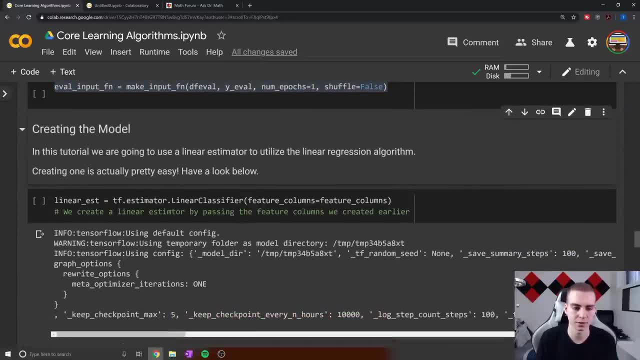 understand. after that, there's not much more I can do. you'd might just have to read through some of the documentation. Alright, creating the model. we are finally here. I know this has been a while, but I need to get through everything. So, linear estimate. so we're going to copy this And I'm 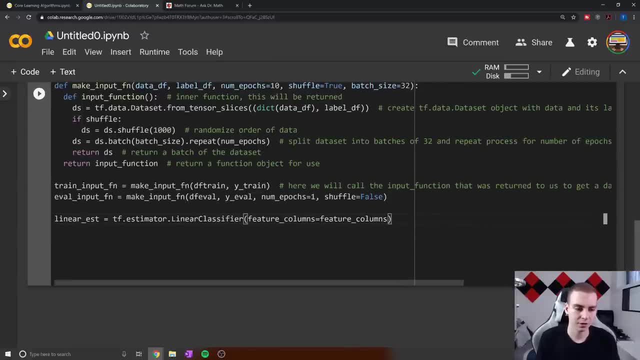 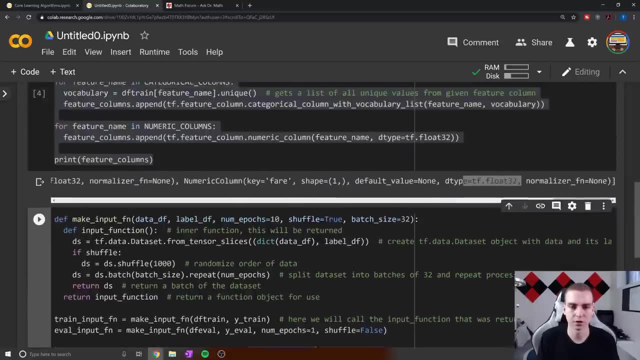 just going to put it in here And we'll talk about what this does. So linear underscore, EST equals tf, dot estimator, dot, linear classifier, And we're giving it the feature columns that we created up here. So this work was not for nothing. we have this feature. 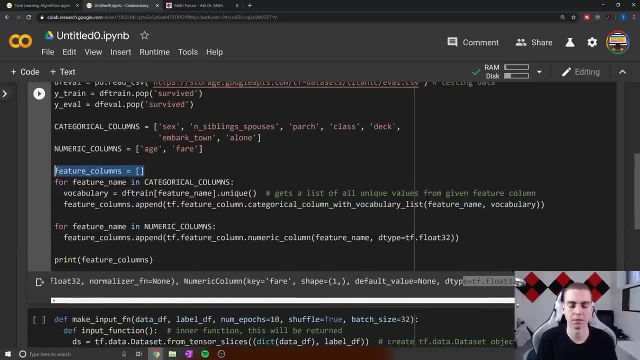 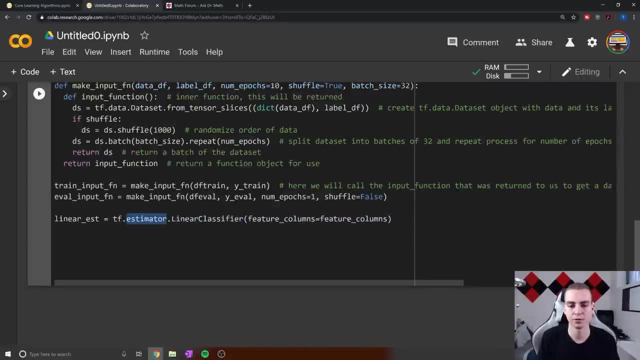 column which defines. you know what is in every single like: what should we expect for our input data? we pass that to a linear classifier object from the estimator module from TensorFlow, And then that creates the model for us. Now, this again is syntax that you don't need to memorize. 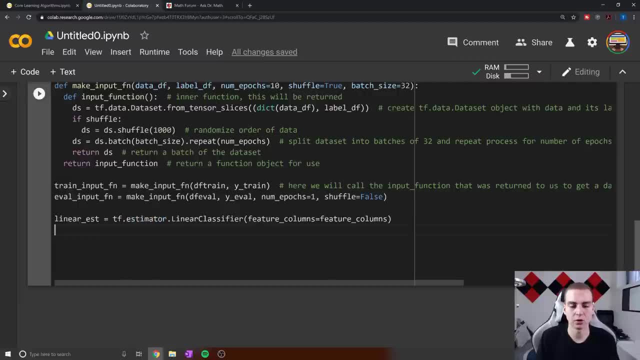 you just need to understand how it works. What we're doing is creating an estimator, all of these kind of core learning algorithms. use what's called estimators, which are just basic implementations of algorithms and TensorFlow, And again pass the feature columns. That's how that works. Alright, so now let's go to training. 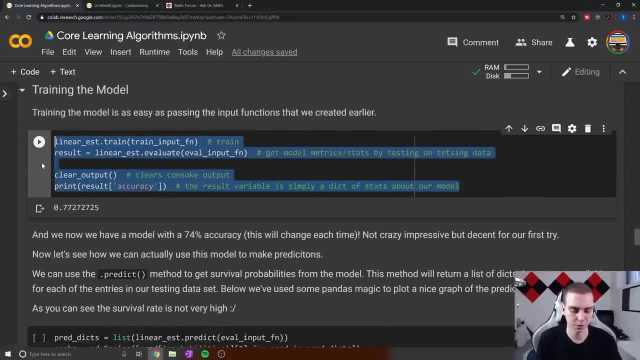 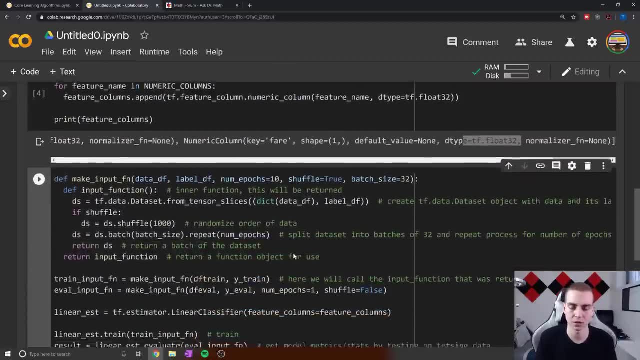 the model. Okay, so I'm just going to copy this again. I know you guys think I'm just copying the code back and forth, But I'm not going to memorize the syntax. I just want to explain to you how all this works. And again you guys will have all this code. you can mess with it, play with it. 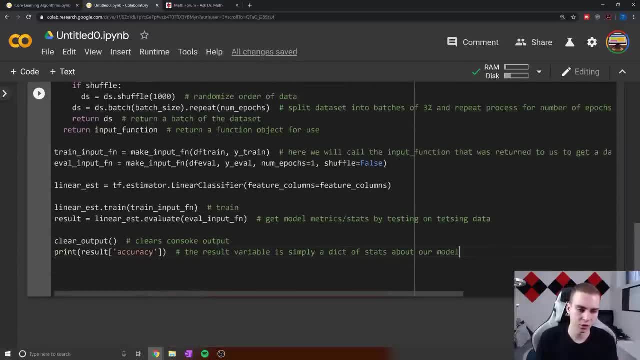 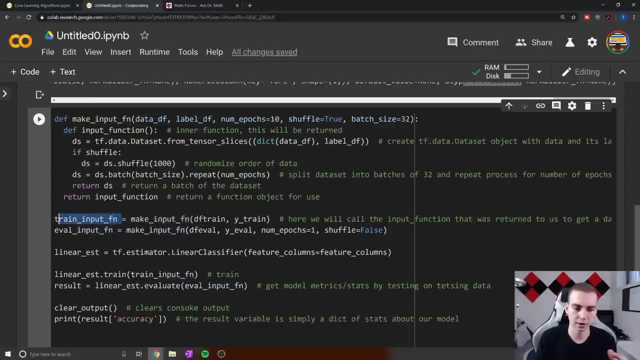 and learn on your own that way. So to train is really easy. all we need to do say linear, EST, dot train and then just give that input function. So that input function that we created up here right, which was returned from, make input function like this train input function. 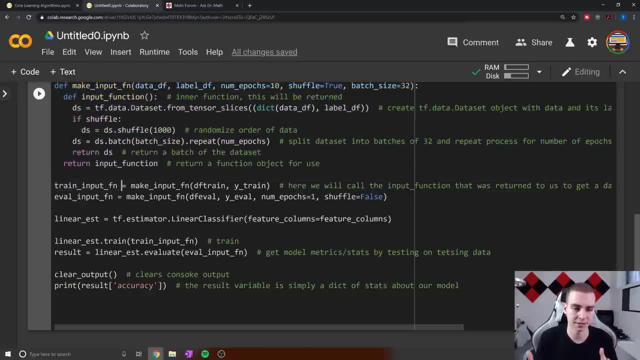 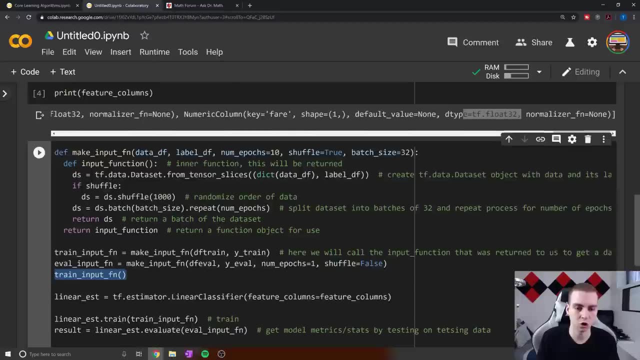 here is actually equal to a function. let's say we'll do a function object itself. If I were to call train underscore input function like this, this would actually call this function. That's how this works in Python. It's a little bit of a complicated syntax, but that's how it works. 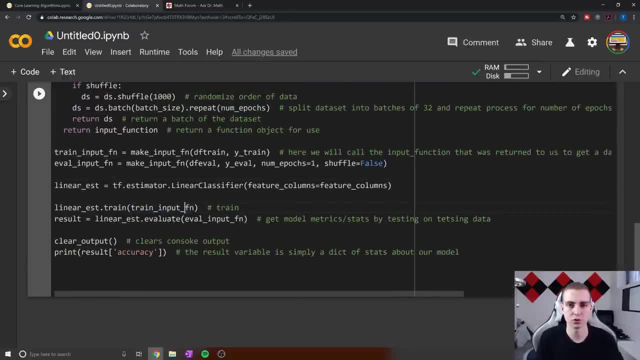 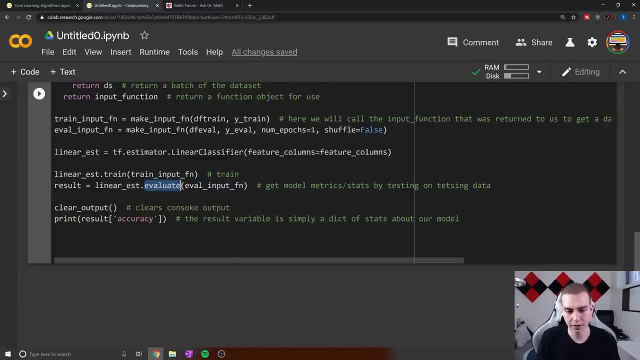 We pass that function here And then we'll use the function to grab all of the input that we need and train the model. Now the result is going to be, rather than trained, we're going to evaluate right and notice that we didn't store. 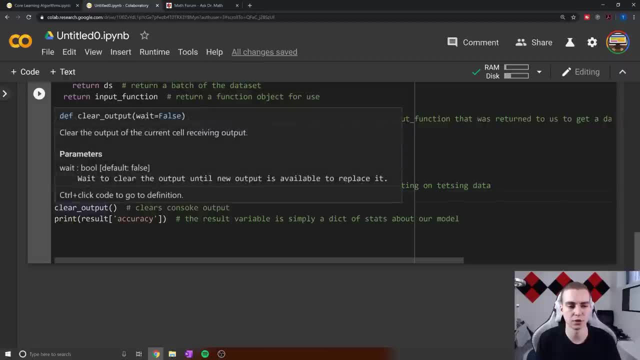 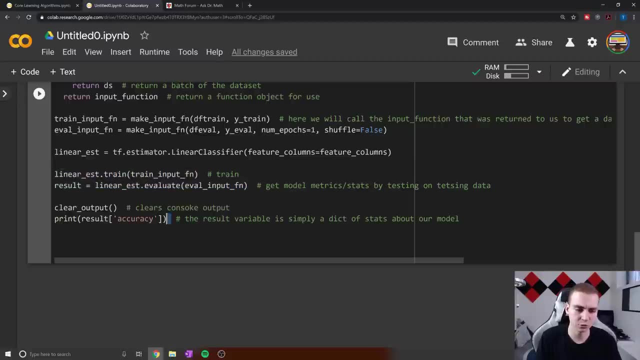 this one in a variable, but we're storing the result in a variable so that we can look at it Now. clear output is just from what we imported above. just going to clear the console output because there will be some output while we're training and we can present print the accuracy. 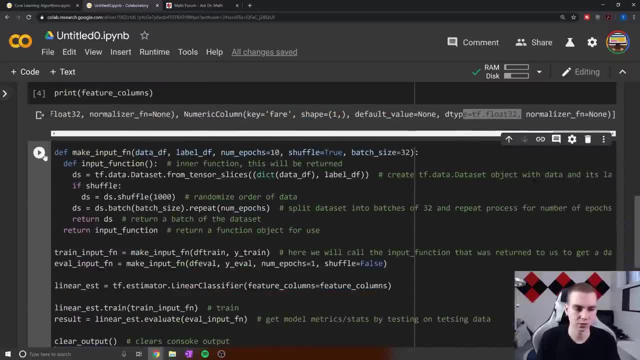 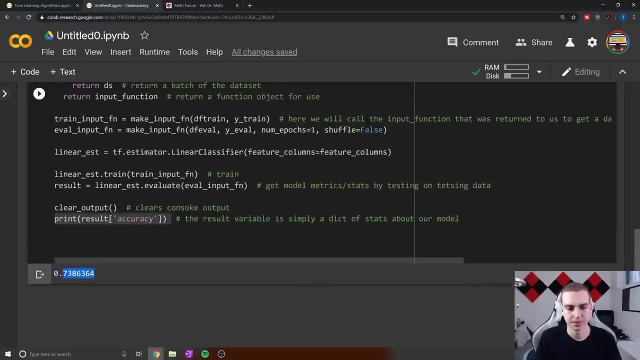 of this model, So let's actually run this and see how this works. This will take a second, So I'll be back once this is done. Okay, so we're back And we've got a 73.8% accuracy. So essentially, what we've done right is we've trained the model. 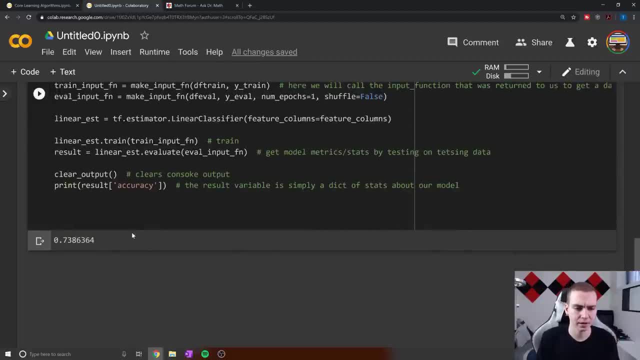 you might have seen a bunch of output while you were doing this on your screen, And then we printed out the accuracy. after evaluating the model, This accuracy isn't very good, But for our first shot this is okay, And we're going to talk about how to improve this in. 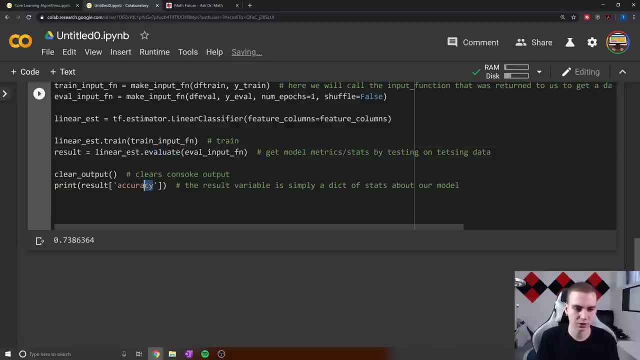 a second. Okay, so we've evaluated the data set. we stored that in result. I want to actually look at what result is, Because obviously you can see we've referenced the accuracy part, like you know, as if this was a Python. 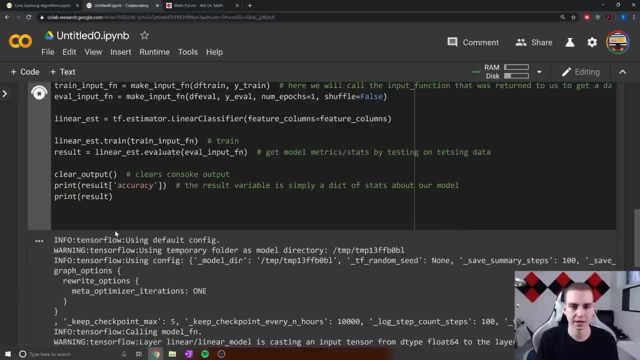 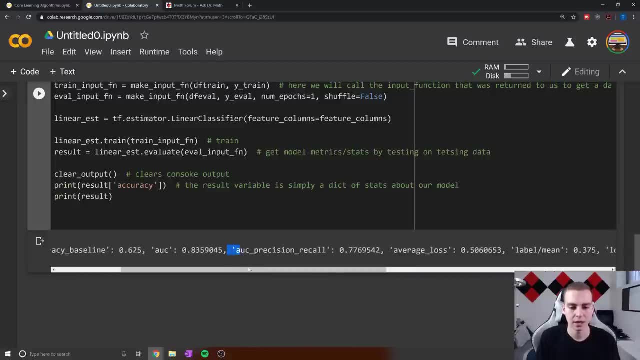 Dictionary. So let's run this one more time of this, going to take a second again, So okay. so we printed out results here And we can see that we have actually a bunch of different values. So we have accuracy, accuracy, baseline, AUC and all these different kind of statistical values. 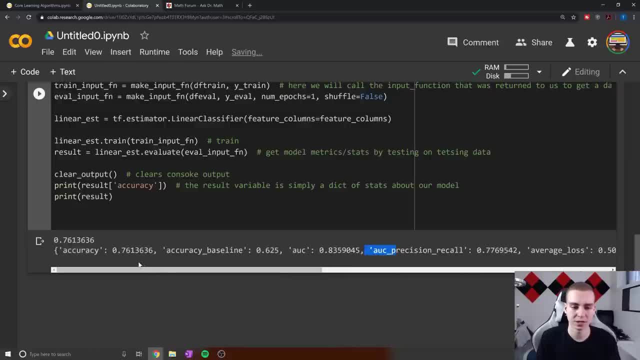 Now, these aren't really going to mean much to you guys, But I just want to show you that we do have those statistics And to access any specific one. this is really just a dictionary object, So we can just reference the key that we want, which is what we did with accuracy. Now notice our accuracy. 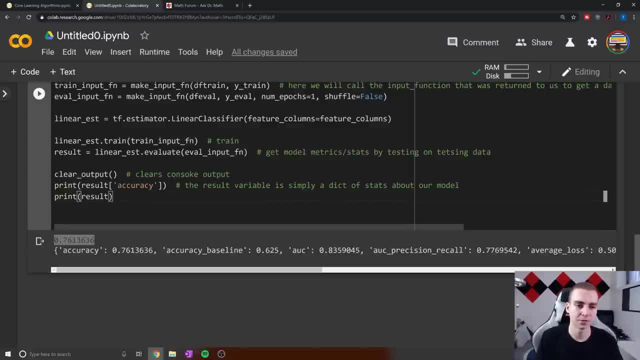 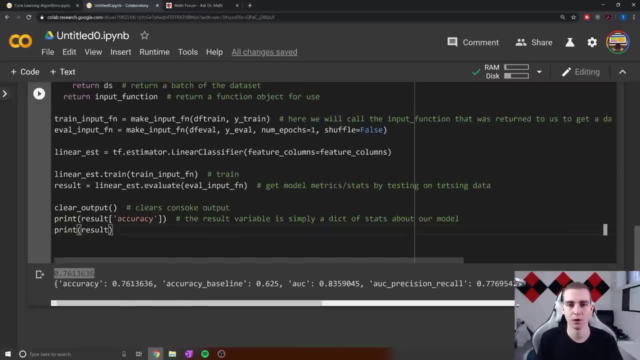 actually changed here we went to 76. Now the reason for this is, like I said, you know, our data is getting shuffled. it's getting put in a different order And based on the order in which we see data- our model, will you know. 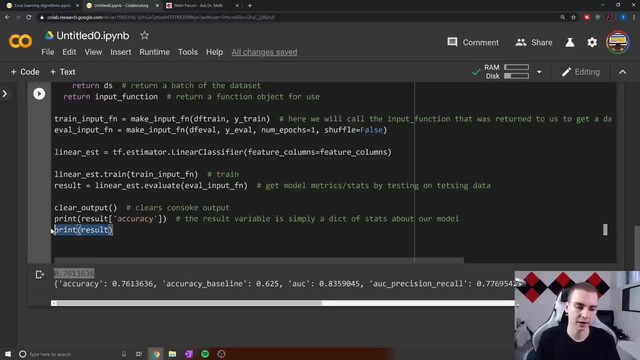 make different predictions and be trained differently. So if we had, you know, another epoch, right? if I change epochs to say 11, or 15, our accuracy will change. Now it might go up, it might go down. that's something we have to play with. as you know, our 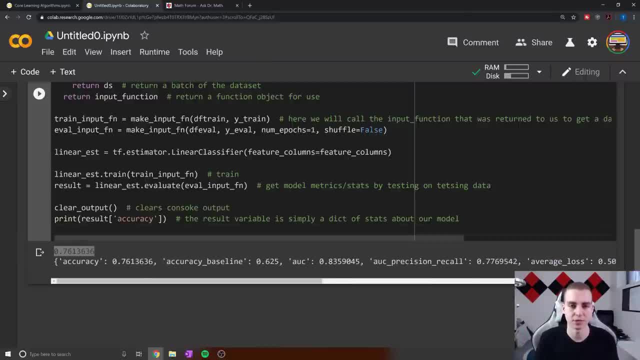 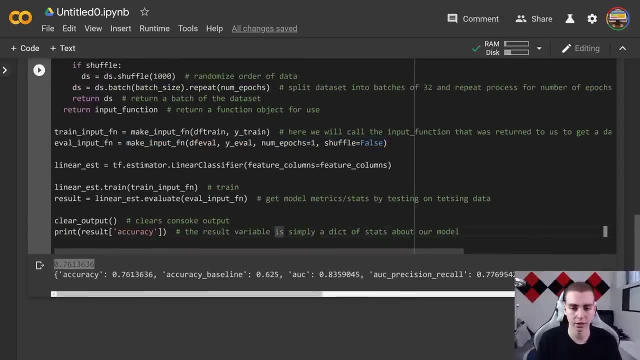 machine learning developer. right, That's what your goal is is to get the most accurate model. Okay, so now it's time to actually use the model to make predictions. So up until this point, we've just been doing a lot of work to understand how to create the model. you know what the model 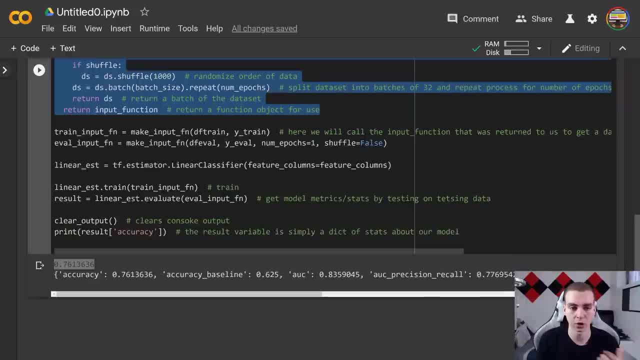 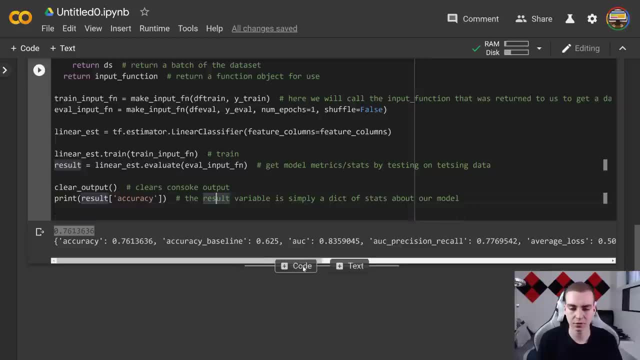 is how we make an input function, training, testing data. I know a lot, a lot, a lot of stuff. Now, to actually use this model and, like, make accurate predictions with it is somewhat difficult, but I'm going to show you how. So essentially, TensorFlow models are built to make predictions. 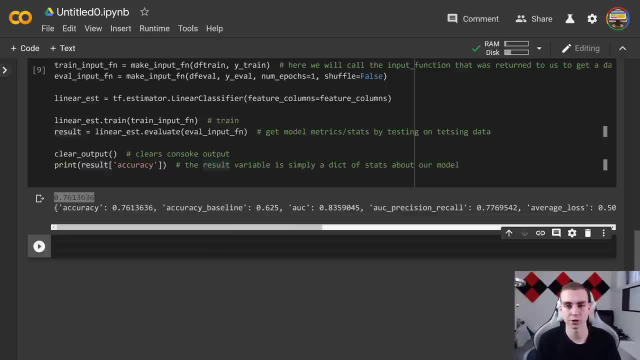 on a lot of things at once. they're not great at making predictions on like one piece of data. you just want like one passenger to make a prediction for. they're much better at working in like large batches of data. Now you can definitely do it with one, but I'm just going. 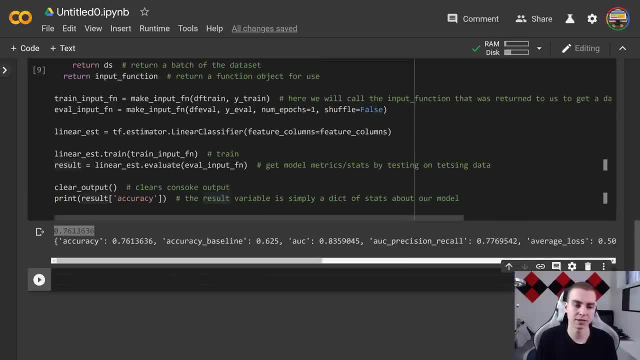 to show you how we can make a prediction for every single point that's in that evaluation data set. So right now we looked at the accuracy And the way we determine the accuracy was by essentially comparing the results that the predictions gave from our model versus what the actual results were. 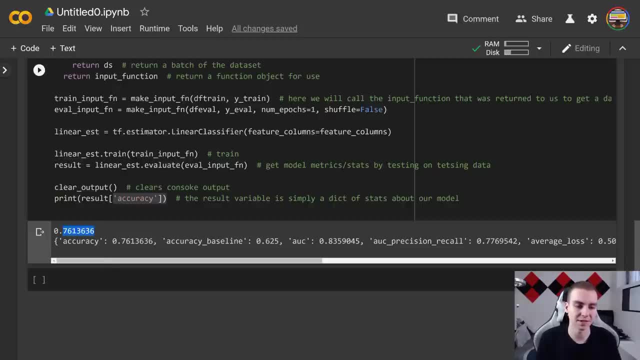 for every single one of those passengers, And that's how we came up with an accuracy of 76%. Now, if we want to actually check and get predictions from the model and see what those actual predictions are, we can do that. So let's go ahead and do that. So we're going to go ahead. 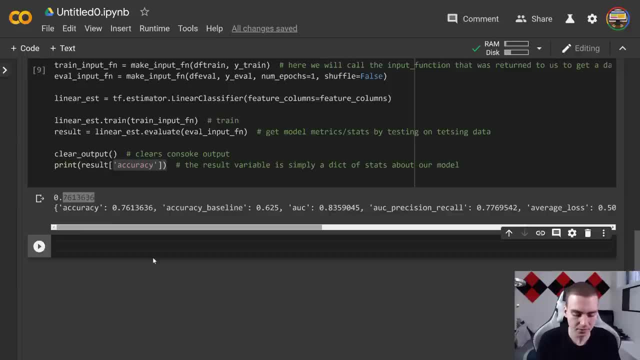 and make a predictionória. One of the nice things about the configuration is that you know what we can do is use a method called dot predict. So what I'm going to do is I'm going to say I guess result like this equals, and in this case we're going to do the model name, which is 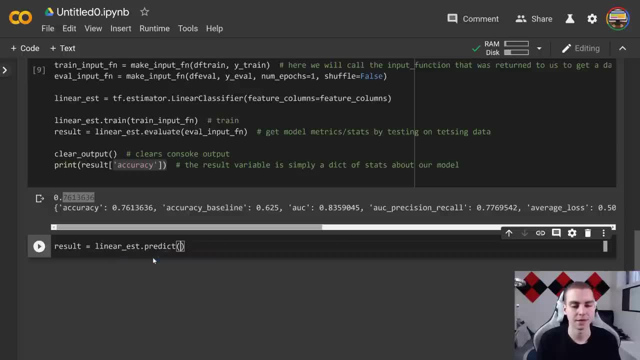 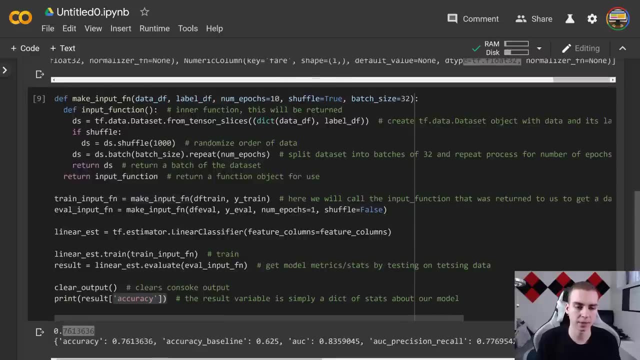 linear est, dot predict. And then inside here, what we're going to pass is that input function we use for the evaluation. So, just like you know, we need to pass an input function to actually train the model. we also need to pass an input function to make a prediction. Now, this input. function could be a function called tp and let me say tp function. tp function, where we have two parameters and this tp function will ask us like a function to predict, toiku, predict tp. now we'll have an input function to predictaremos. we need to capture a prediction that is going to exceed several. 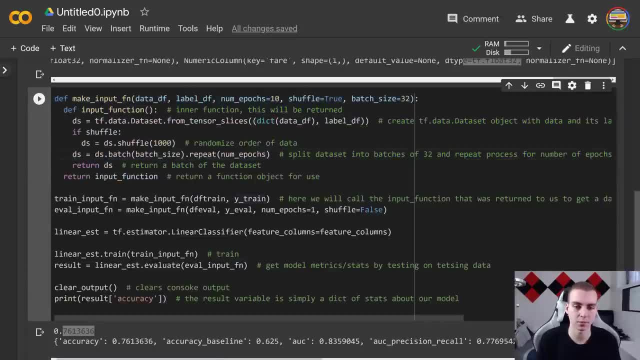 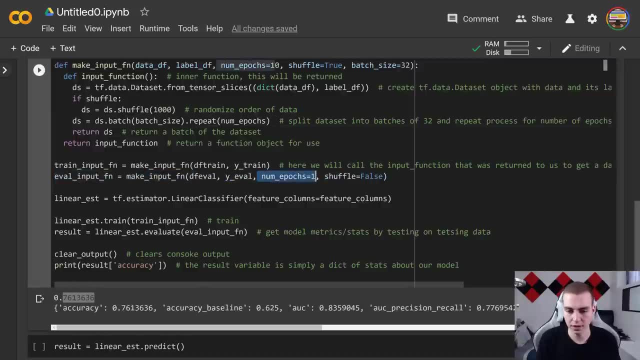 be a little bit different. we can modify this a bit if we wanted to, But to keep things simple, we use the same one for now. So what I'm going to do is just use this eval input function, So the one we've already created where we did, you know, one epoch. we don't need to shuffle because 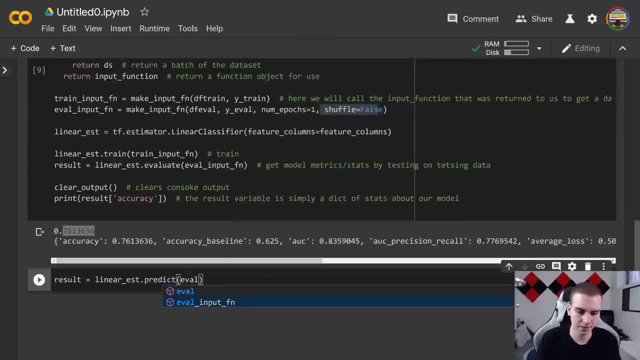 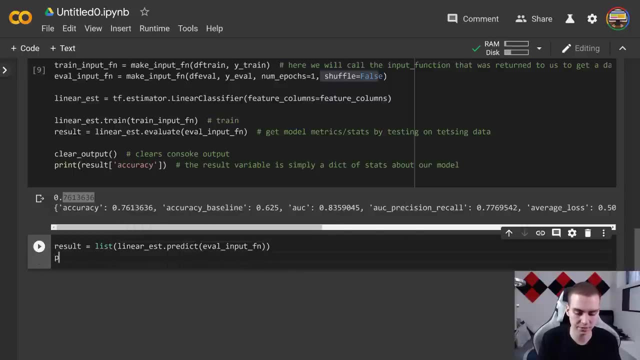 just the evaluation set. So inside here we're going to do eval input function. Now, what we need to do, though, is convert this to a list, just because we're going to loop through it, And I'm actually going to print out this value So we can see what it is before we go to the next step. So 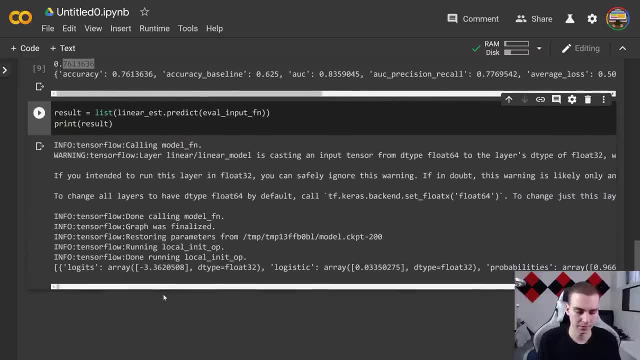 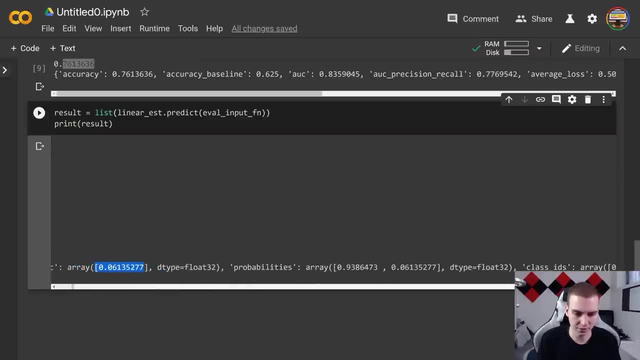 let's run this and have a look at what we get. Okay, so we get logistics array. we can see all these different values. So we have, you know, this array with this value. we have probabilities, this value, and this is kind of what we're getting. So we're getting logistic, all classes. 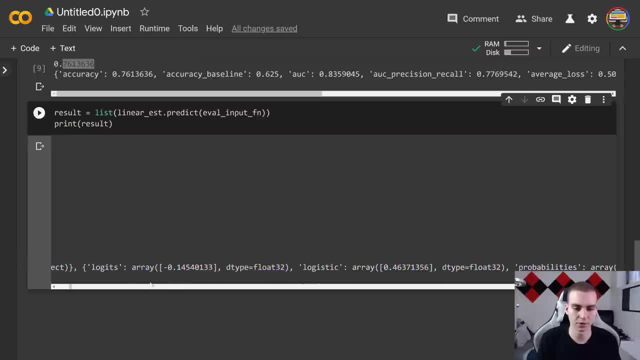 like there's all this random stuff. what you hopefully should notice- and I know I'm just like whizzing through- is that we have a dictionary that represents the predictions, And I'll see if I can find the end of the dictionary here For every single: what is it prediction? 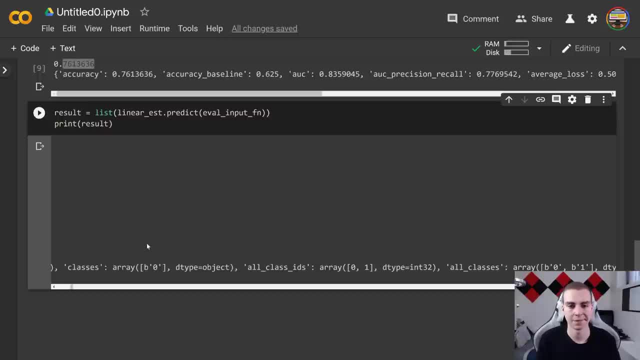 so since we've passed- you know 267, input data from this, you know eval input function. what was returned to us is a list of all of these different dictionaries that represent each prediction. So what we need to do is look at each dictionary so that we can determine what the 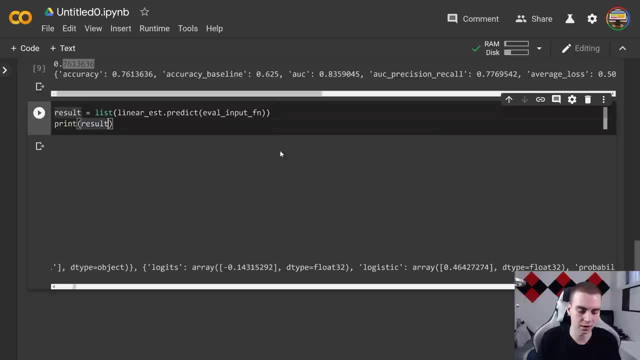 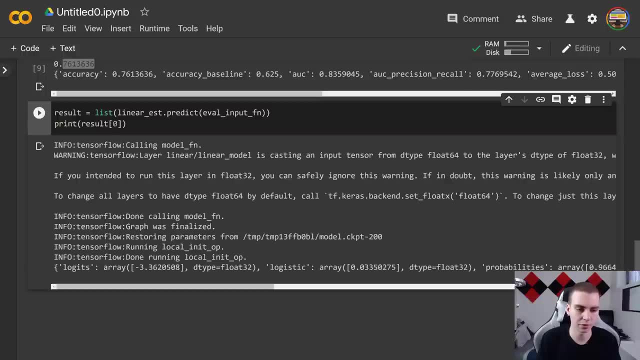 actual prediction was. So what I'm going to do is actually just present do results. When we do, result zero, because this is a list, so that should mean we can index it, So we actually look at one prediction. Okay, so this is the. 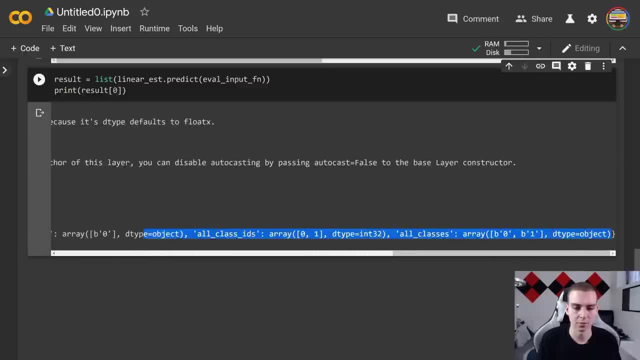 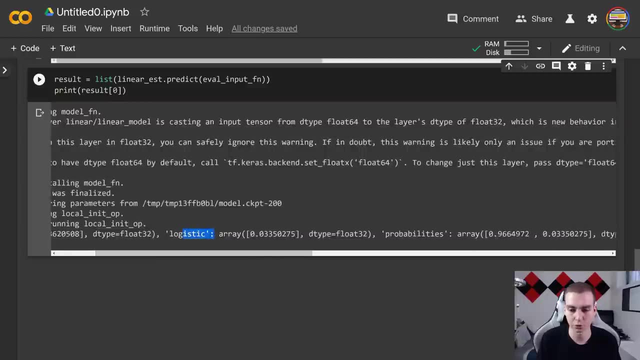 dictionary of one prediction. So I know this seems like a lot, But this is what we have. this is our prediction. So logistics: we get some array. we have logistic in here in this dictionary, and then we have probabilities. So what I actually want is probability. 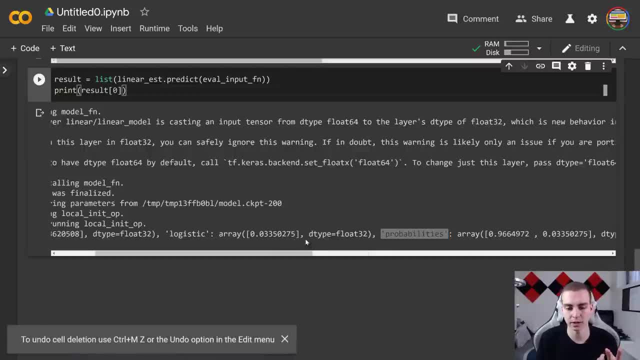 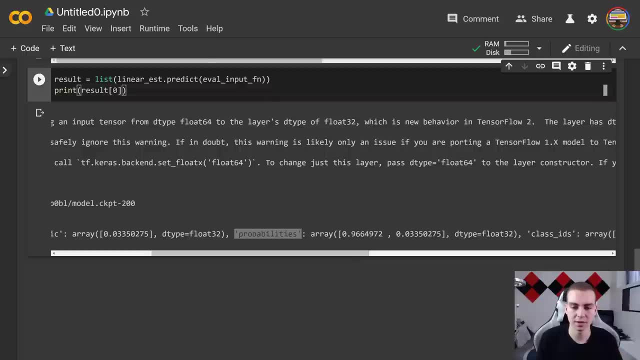 Now, since what we ended up having was a prediction of two classes, right, either zero or one. we're predicting either someone survived or they didn't survive, or what their percentage should be. we can see that the percentage of survival here is actually 96%, And the percentage 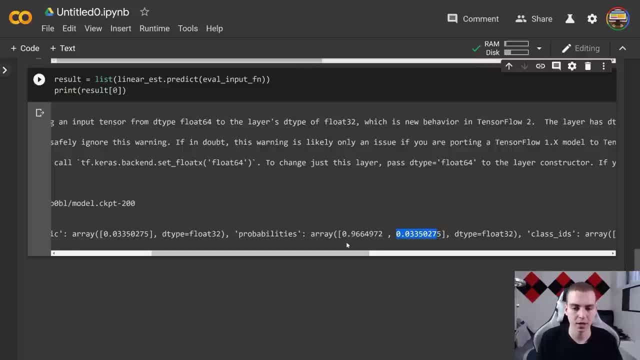 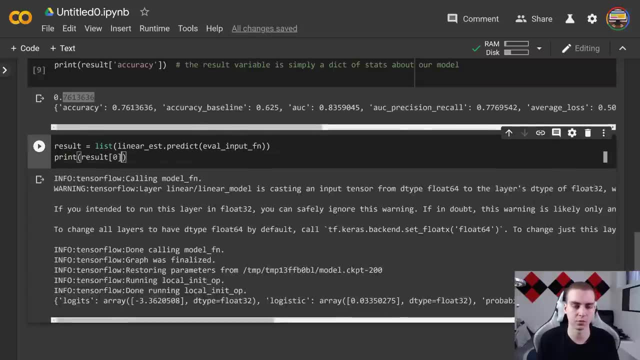 it thinks that it won't survive is, you know, 3.3%. So if we want to access this, what we need to do is click, do result at some index. So whatever you know one we want. So we're gonna say: 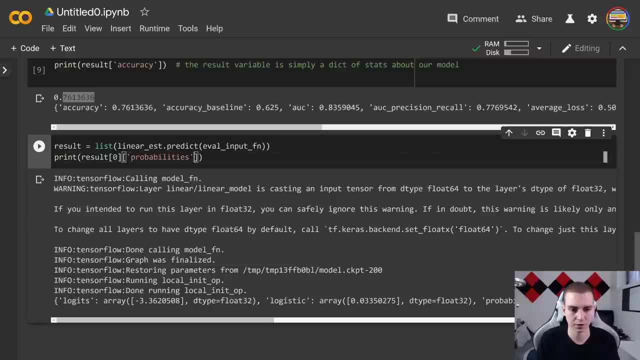 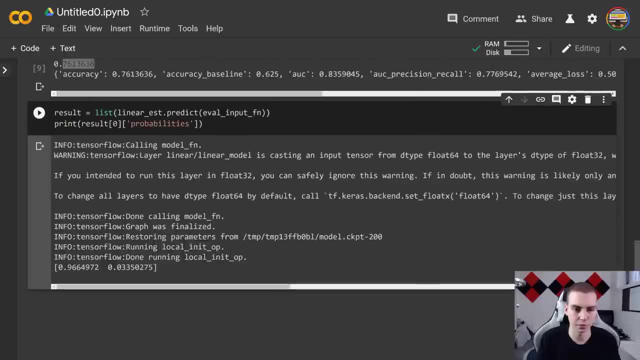 result. And then here we're going to put probabilities. So I'm just going to print that like that, And then we can see the probabilities. So let's run this, And now we see our probabilities are 96 and 33.. Now, if we want the probability of survival, so I think I actually might have. 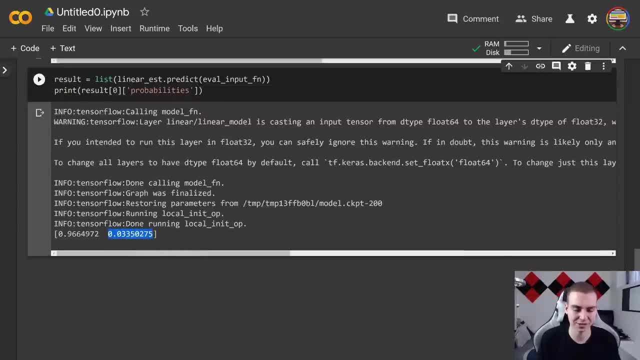 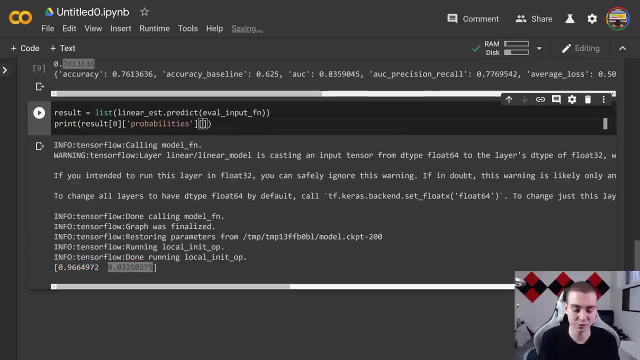 messed this up. I'm pretty sure the survival probability is actually the last one, whereas, like the non survival is the first one, because zero means you didn't survive and one means you did survive. So that's my bad, I messed that up. So I actually want their chance of survival. I'll index one. So if I index one, 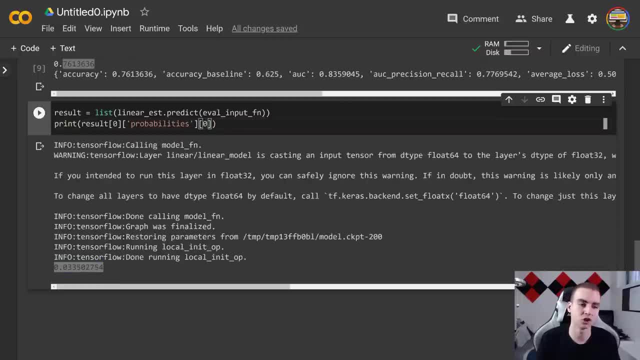 you see we get 3.3%. But if I wanted their chance of not surviving, I would index zero. And that makes sense, because zero is, you know what we're looking like: zero represents they didn't survive, whereas one represents they did survive. So that's kind of how we do that. So 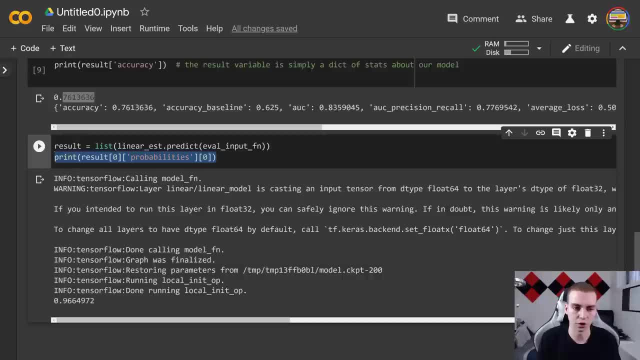 that's how we get them. So that's kind of how we do that. So that's how we get them. If we wanted to loop through all of these, we could. we could loop through every dictionary and we could print every single probability of each person And we can also look at that person's 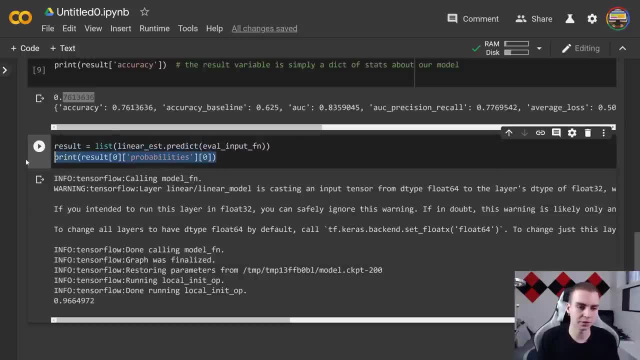 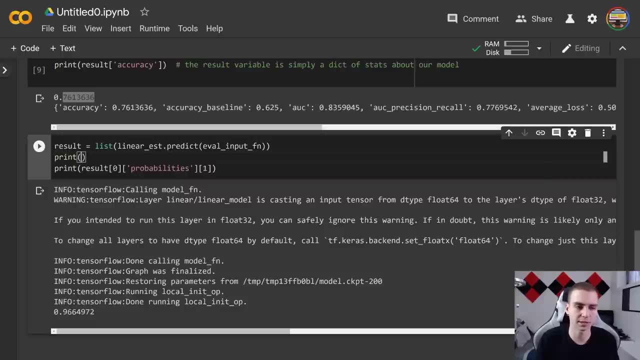 stats and then look at their probability. So let's see, the probability of surviving is, in this case, you know, 3% or whatever, it was 3.3%. But let's look at the person that we were actually predicting them and see if that makes sense. So if I go eval or what was a DF eval? 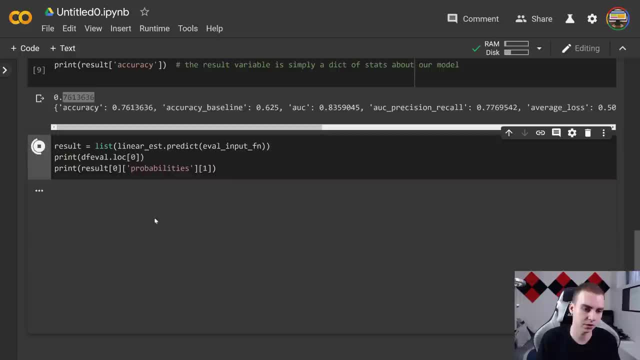 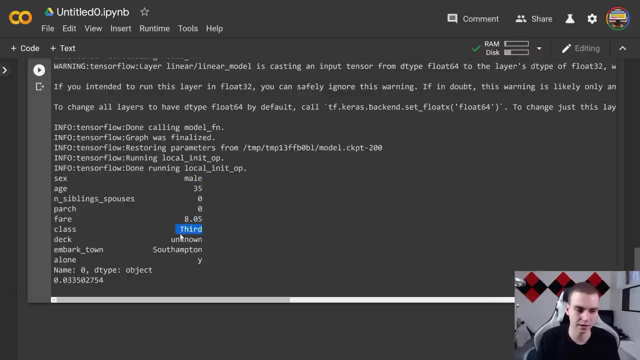 dot loc zero. we print that and then we print the result. What we can see is that for the person who was male and 35, that had no siblings, their fair was this: they're in third class. we don't know what deck they were on, and they were. 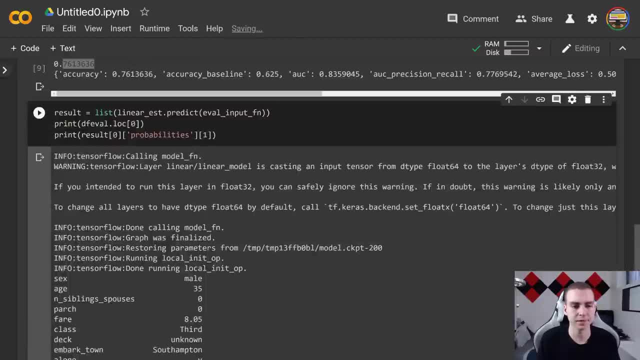 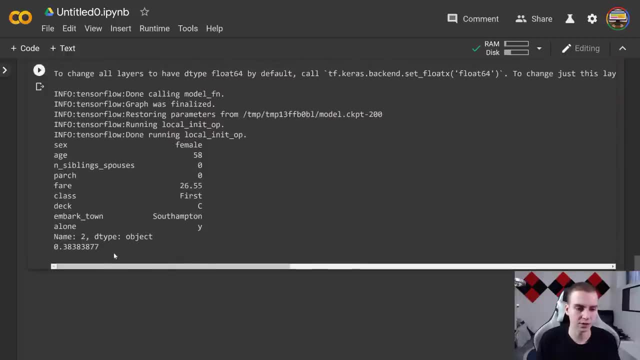 alone, they have a 3.3% chance of survival. Now, if we change this, we could go like two, two. let's have a look at this second person and see what their chance of survival is. Okay, so they have a higher percent chance of 38% chance. they're female, they're a little bit older, So 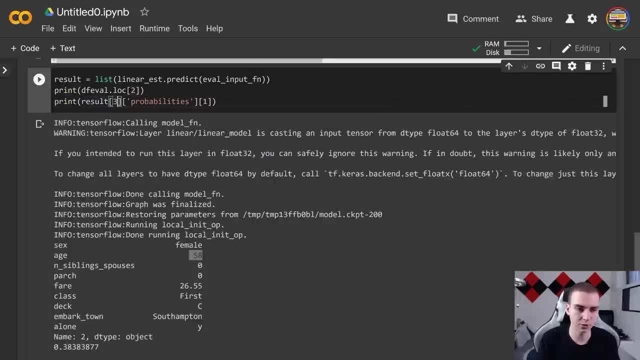 that might be a reason why their survival rates a bit lower. And I mean we can keep doing this and look through and see what it is. So let's look at this second person and see what their chance of survival is. Okay, so they have a higher percent chance of 38% chance. they're female. they're a little. 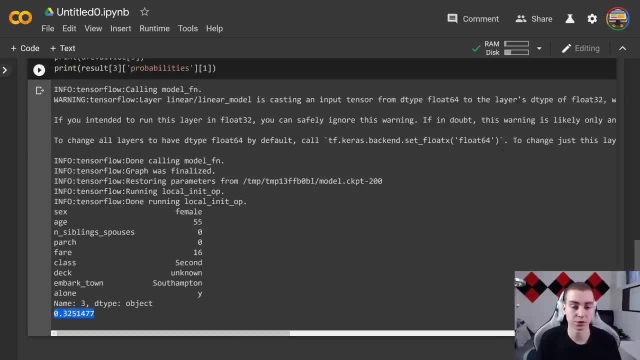 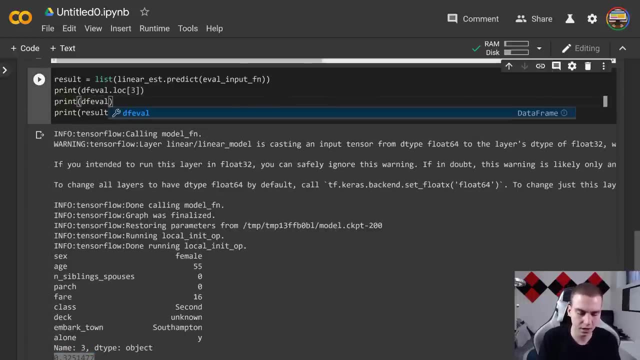 bit older. So let's look at this second person and see what their chance of survival is. Okay, if we want to get the actual value, like if this person survived or if they didn't survive, and what I can do is I can print df eval. Actually, it's not going to be eval, it's going to be. 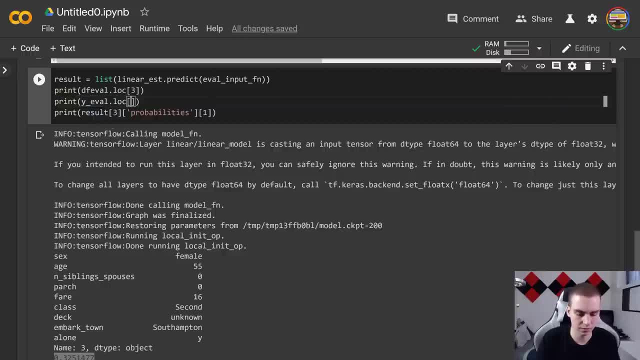 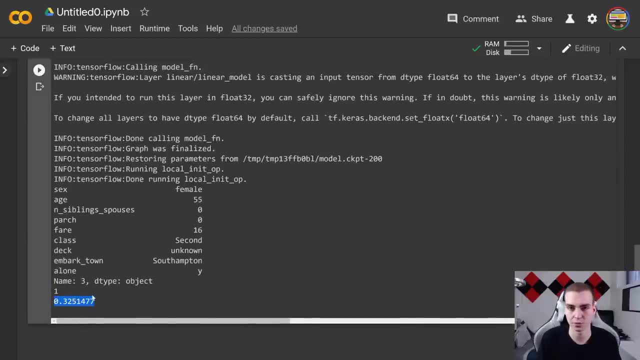 y underscore eval: Yeah, And that's going to be dot loc three. Now, this will give us if they survived or not. So actually, in this case, that person did survive, but we're only predicting a 32%. So you can see that that's, you know, represented in the fact that we only have about a 76% accuracy. 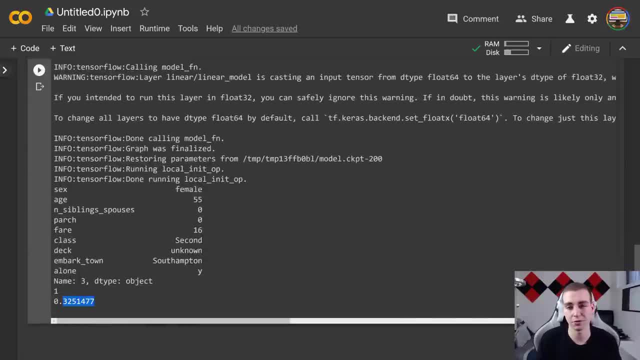 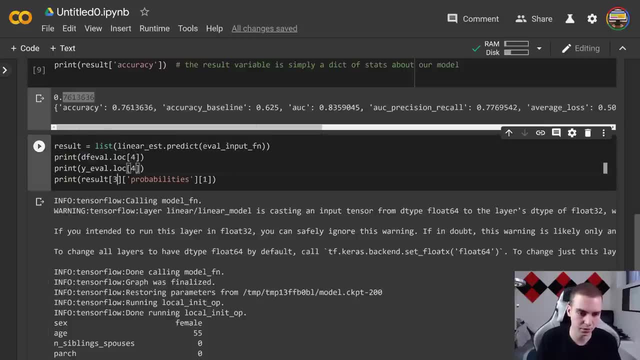 because this model model is not perfect And in this instance it was pretty bad. It's saying they have a 32% chance of surviving, but they actually did survive, So maybe that should be higher, right, So we could change this number. go for four. I'm just messing around and showing you guys. you know how we use this. So 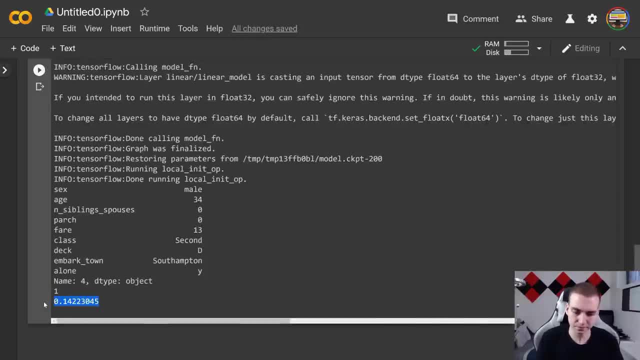 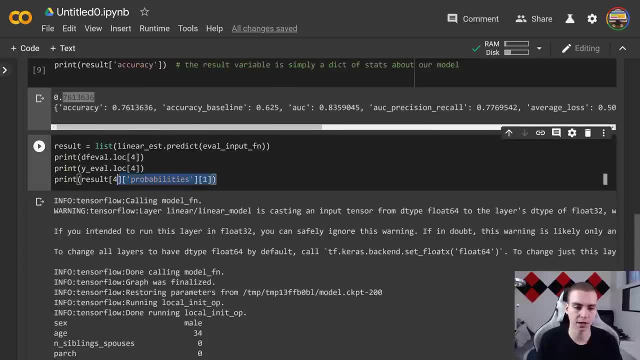 in this one. you know same thing. this person survived, although- what is it? they only were given a 14% chance of survival. So, anyways, that is how that works. This is how we actually make predictions. and look at the predictions. you understand that now. what's happening is: I've 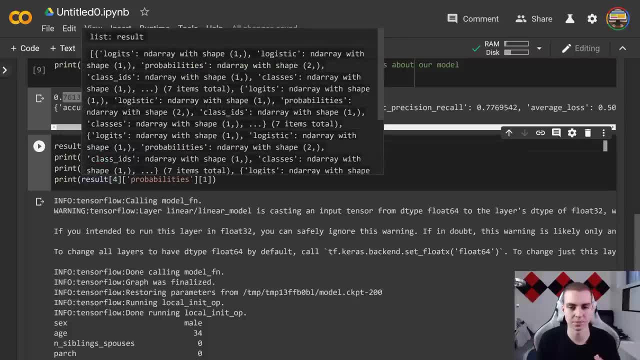 converted this to a list just because this is actually a generator object, which means it's meant to just be looped through rather than just look at it with a list. But that's fine, we'll use a list And then we can just print out you. 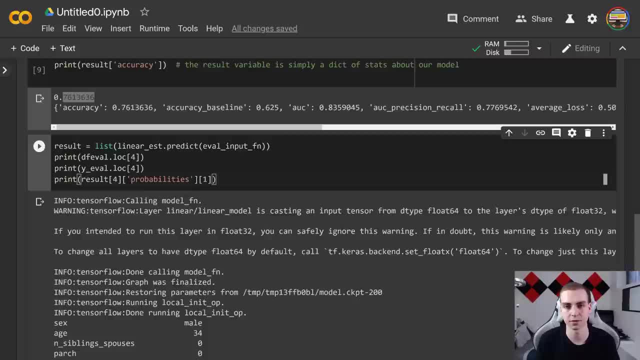 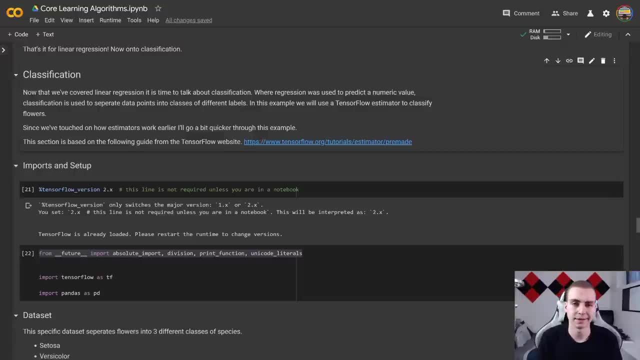 know result at whatever index probabilities, and then one to represent their chance of survival. Okay, so that has been it for linear regression. Now let's get into classification. And now we are on to classification. So, essentially, classification is differentiating between, you know, data points. 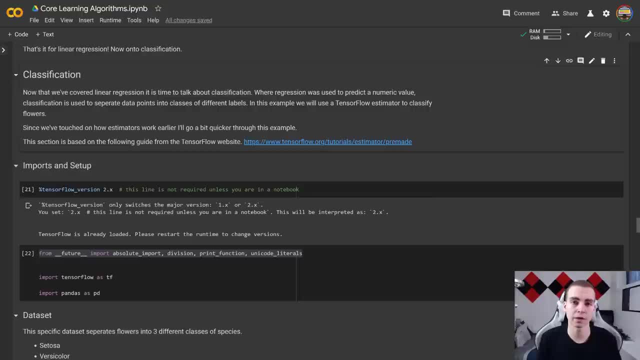 and separating them into classes. So, rather than predicting a numeric value, which is the number of classes, which we did with regression earlier, so linear regression and you know the percentage survival chance, which is a numeric value, we actually want to predict classes. So what we're going to end up? 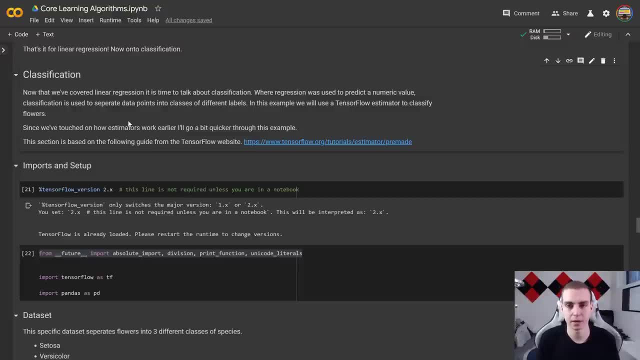 doing is predicting the probability that a specific data point or a specific entry, or whatever we're going to call it, is within all of the different classes. it could be. So, for the example here we're going to use flowers, So it's called the Iris. I think it's the Iris flower data set or something. 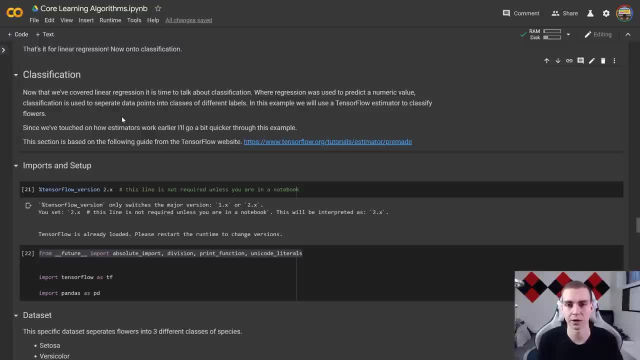 like that, And we're going to use some different properties of flowers to predict what species of flower it is. So that's the difference between classification and regression. Now I'm not going to talk about the specific algorithm we're going to use here for classification, because there's just so many different ones you can. 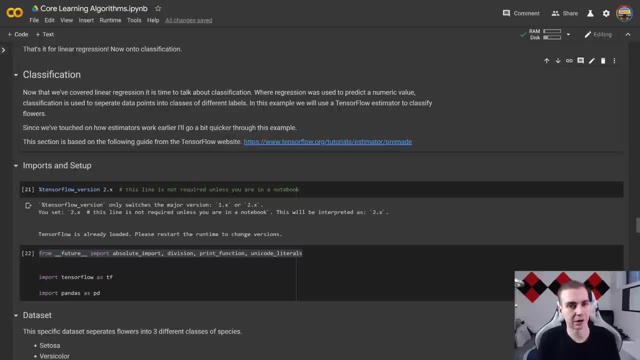 use. But yeah, I mean, if you really care about how they work on a lower mathematical level, I'm not going to be explaining that because it doesn't make sense to explain it for one algorithm when there's like hundreds and they all work a little bit differently. So you guys can kind of look that up And I'll tell. 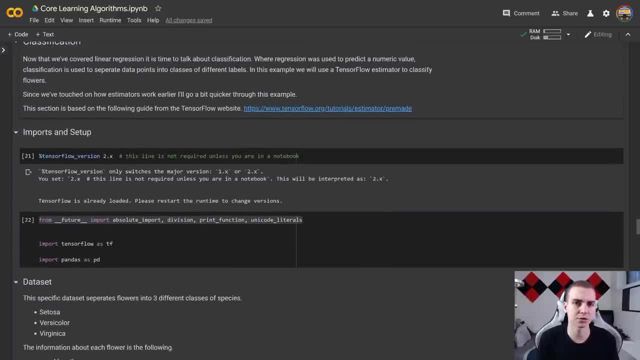 you some resources and where you can find that I'm also going to go faster through this example, just because I've already covered a lot of the fundamental stuff in linear regression, So hopefully we should get this one done a little bit quicker and move on to the next kind of aspects in this series. Alright, so first steps: load. 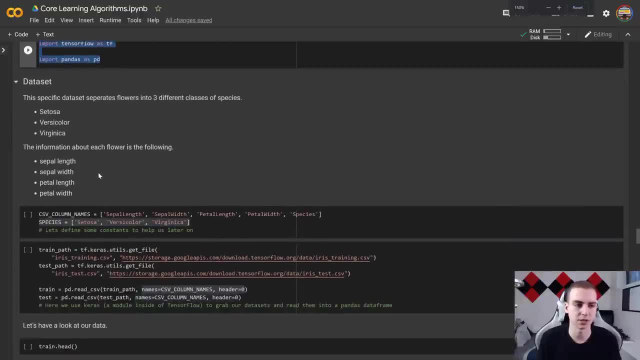 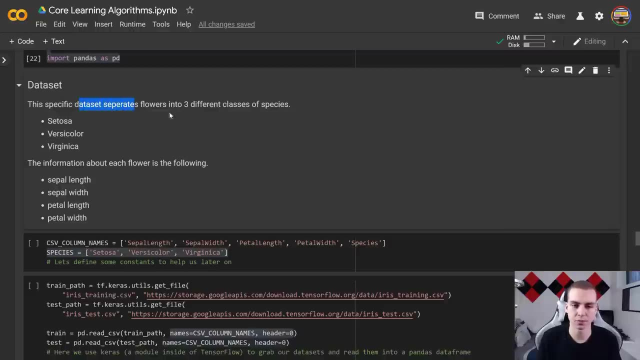 TensorFlow- import TensorFlow. we've done that already. data set- we need to talk about this. So the data set we're using is that Iris flowers data set, like I talked about, and this specific data set separates flowers into three different species, So we have these different species. This is the information we 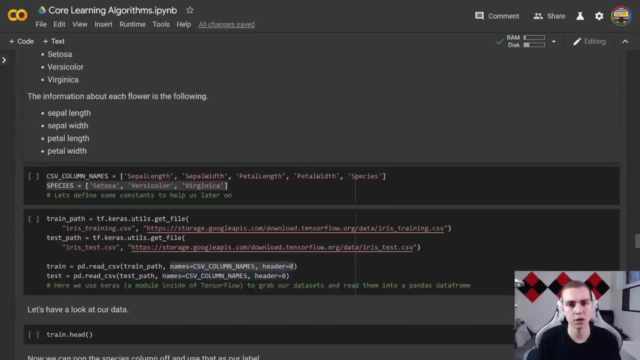 have. So septal length, width, petal length, petal width. we're going to use that information, obviously, to make the predictions. So, given this information, you know, in our final model, can it tell us which one of these flowers it's most likely? 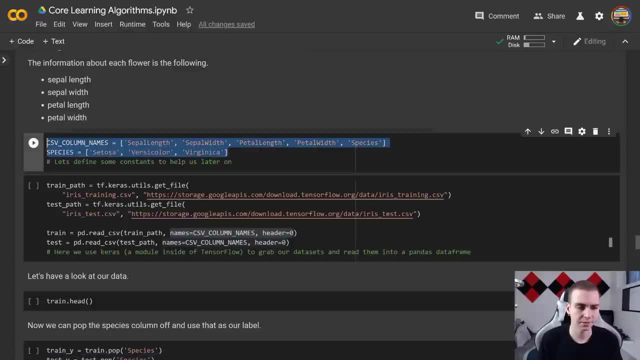 to be Okay. so what we're going to do now is define the CSV column names and species. So the column names are just going to define. what we're going to have in our data set is like the headers for the columns species. obviously it's just the species and we'll throw them there, Alright. so now we're 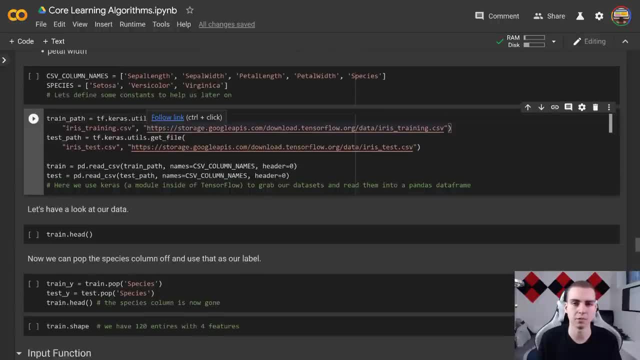 going to load in our data sets, So this is going to be different every time. you're kind of working with models, depending on where you're getting your data from. And our example: we're going to get it from Keras, which is kind of in. 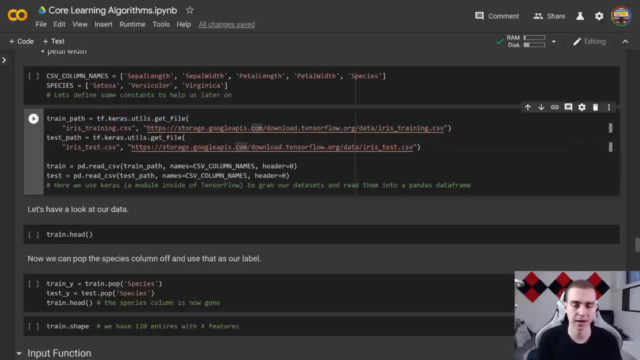 sub module of TensorFlow. It has a lot of useful data sets and tools that we'll be using throughout the series. But Keras dot utils dot get file Again. don't really focus on this. Just understand what this is going to do is save this file onto our computer as iris training dot csv grab it. 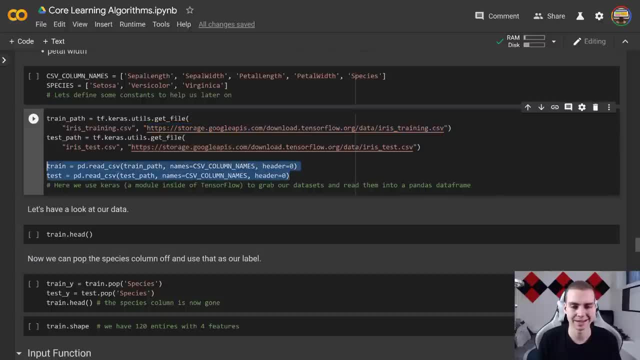 from this link And then what we're going to do down here is load the train and test and again notices his training, And this is testing into two separate data frames. So here we're going to use the names of the columns as the. CSV column names. we're going to use the path as whatever we like, but here from there we're going. So here, one thing that we've dense would need to do here is go to our line base, which is what we used to do on the page. So here we have the subject known as the data frame, And here you can see what that 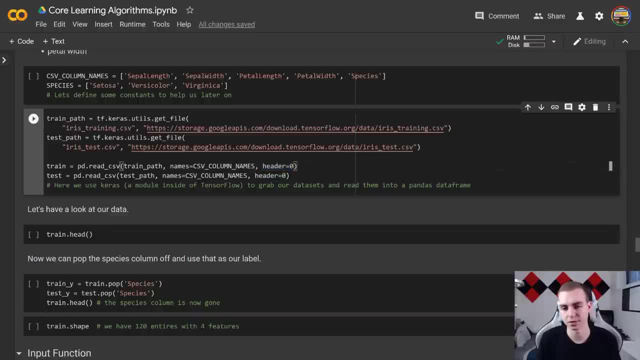 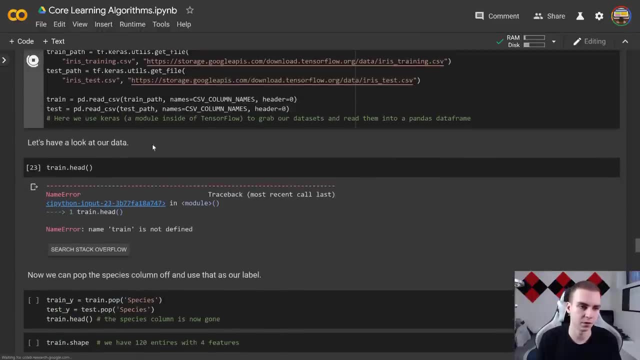 as whatever we loaded here, header equals zero, which just means row zero is the header. Alright, so now we will move down and we'll have a look at our data set. So, like we've done before, oh, I've got to run this code first. CSV, column names. Okay, so we've just, we're just running. 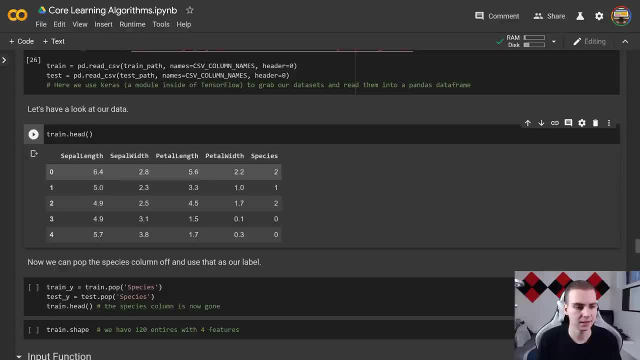 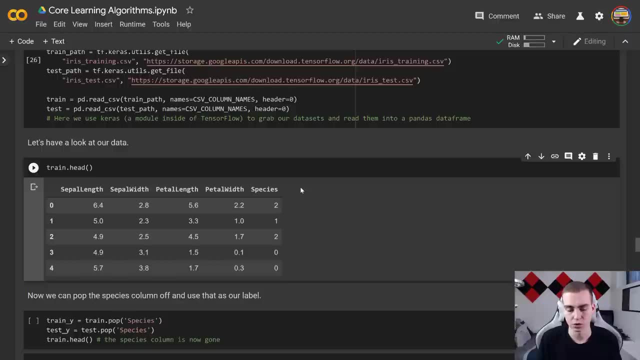 things in the wrong order here, apparently. Okay, so let's look at the head So we can see- this is kind of what our data frame looks like- And notice that our species here are actually defined numerically, So, rather than before, when we had to do that thing where, you know, we made those. 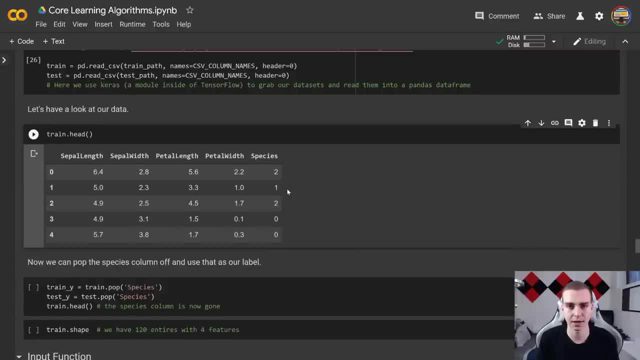 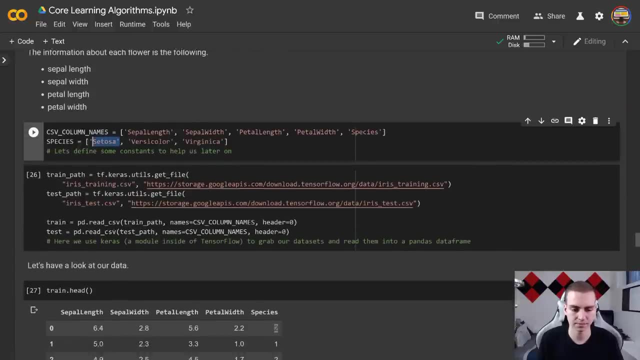 feature columns, and we converted the categorical data into numeric data with those kind of weird TensorFlow tools. this is actually already encoded for us Now. zero stands for satosa, And then one and two obviously stand for these ones respectively, And that's how that works. 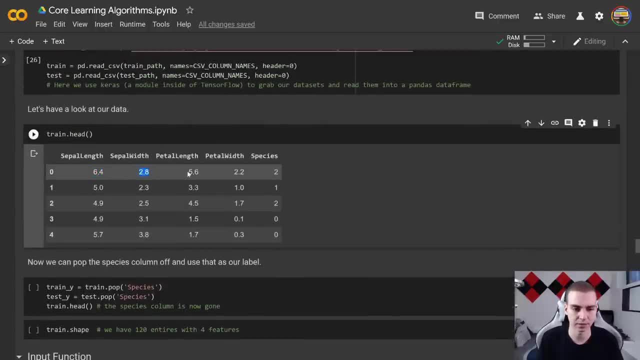 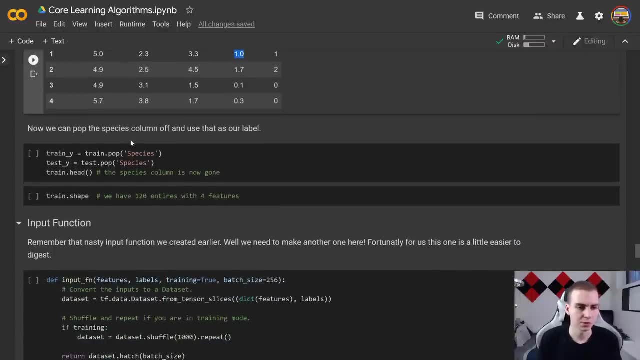 Now these, I believe, are in centimeters: the septal length, petal length, petal width. that's not super important, But sometimes you do want to know that information. Okay, so now we're going to pop off those columns for the species, like we did before, and separate that. 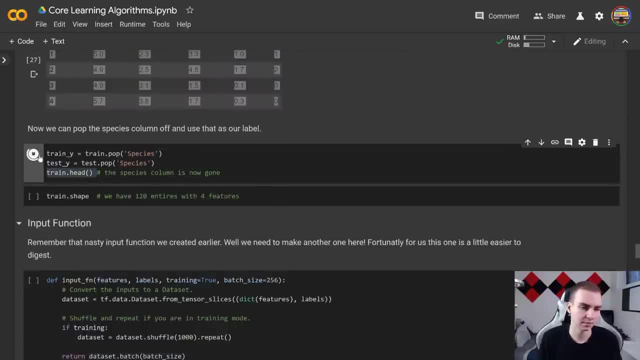 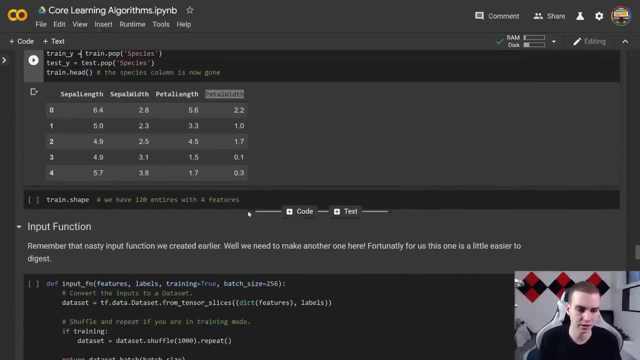 into train y, test y and then have a look at the head again. So let's do that and run this notice that is gone. Again, we've talked about how that works. And then these: if we want to have a look at them, and actually let's do this by just having a new block. let's say, train underscore y. 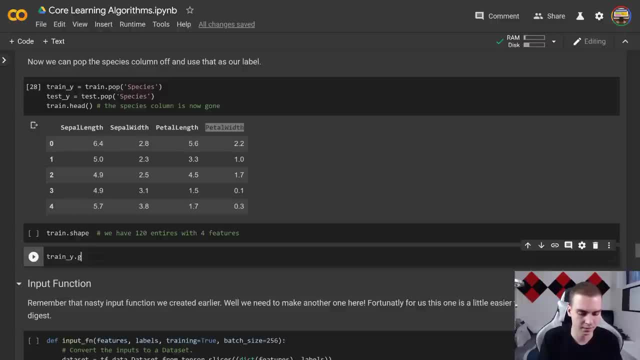 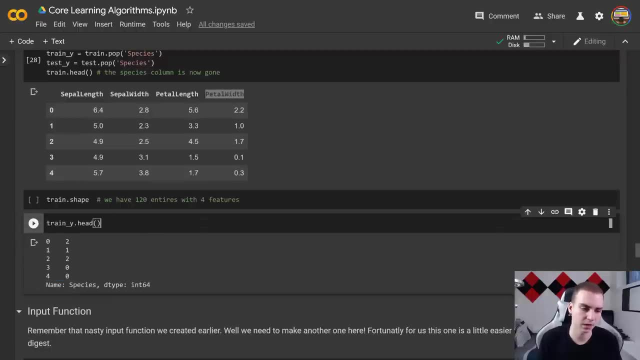 dots. what is it? dot head, If I could spell head correctly. okay, so we run head And we can see. this is what it looks like, nothing special. That's what we're getting, Alright. so let's delete that. Let's look at the shape of our training data. I mean, we can probably guess what it is already. 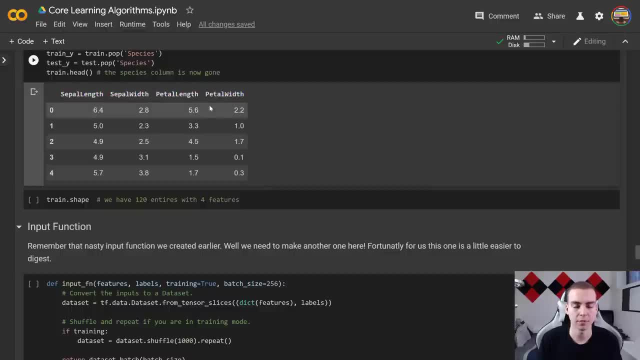 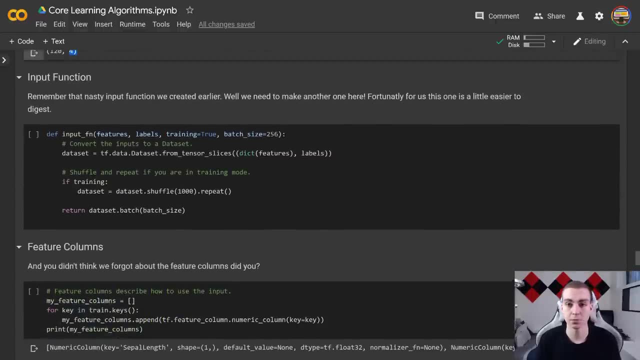 but we're gonna have shape four, because we have four features. And then, how many entries do we have? Well, I'm sure this will tell us. so 120 entries in shape for awesome. that's our shape, Okay input function. So we're moving fast here. already we're getting into a lot of the coding. 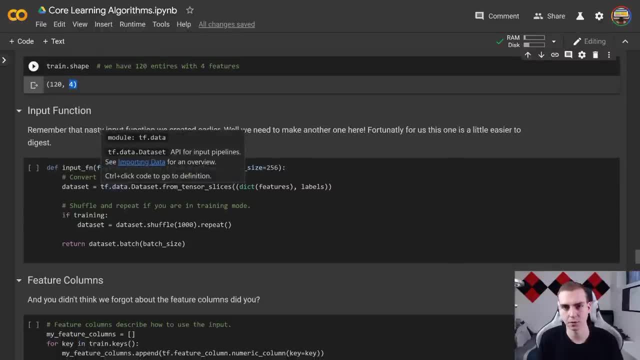 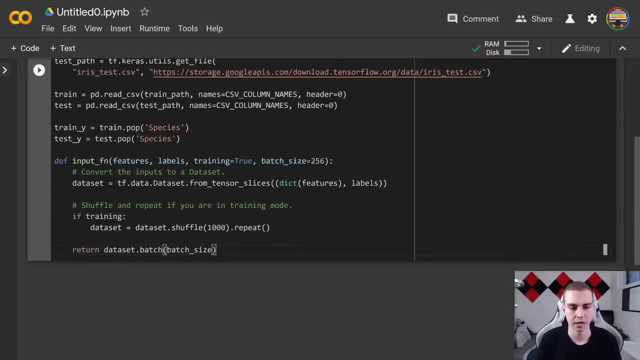 So what I'm actually going to do is again copy this over into a separate document and I'll be back in a second with all that. Okay, so input function time. we already know what the input function does because we used it previously. Now this input function is a little bit different than. 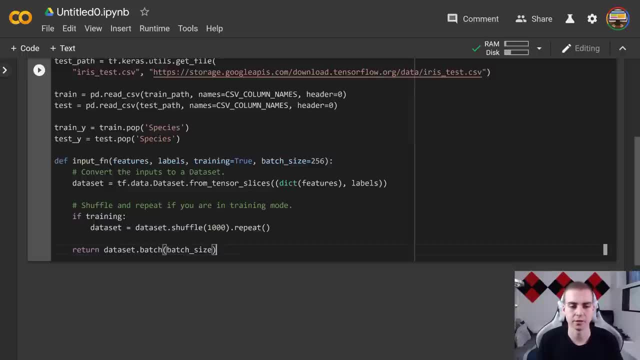 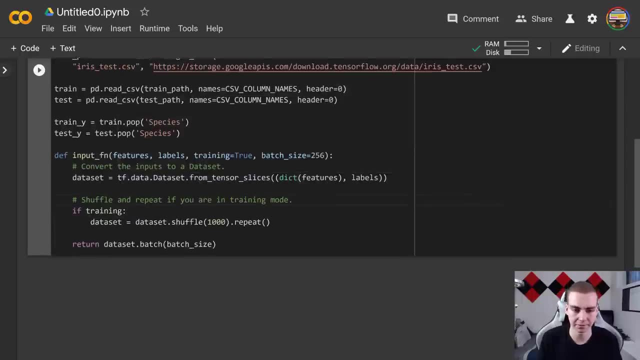 before, just because we're kind of changing things slightly. So here we don't actually have any, What do you call it? we don't have any epochs, and our batch size is different. So what we've done here is, rather than actually, you know, defining like make input function, we just have 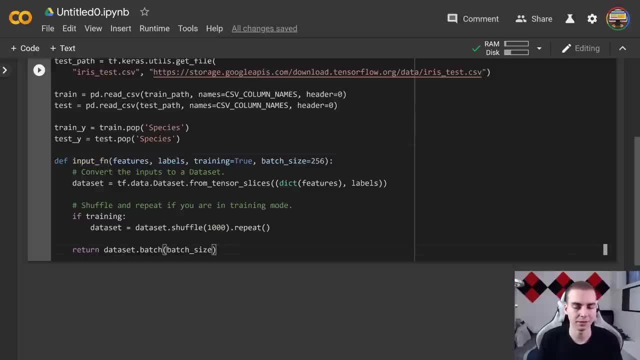 input function like this, And what we're going to do is a little bit different when passes input function. I'll kind of show you. it's a little bit more complicated, But you can see that we've cleaned this up a little bit. So exactly we're doing what we did do before we're converting this. 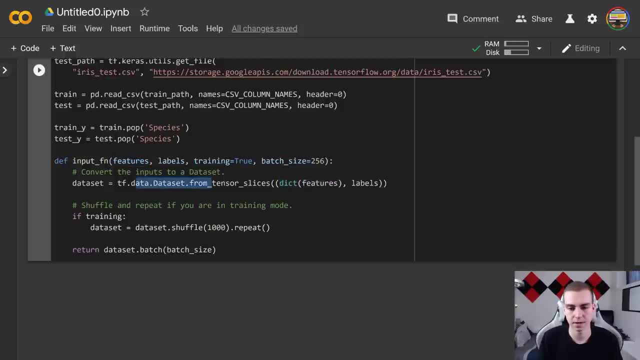 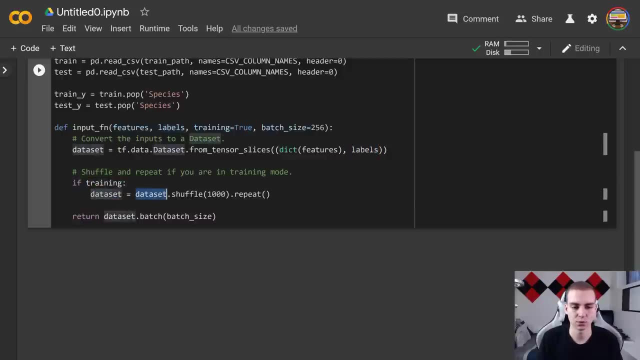 out, which is our features, which we're passing in here into a data set, And then we're passing those labels as well. And then if we're training- so if training is true- what we're going to do is say data set is equal to the data set dot shuffle. So we're going to shuffle that information. 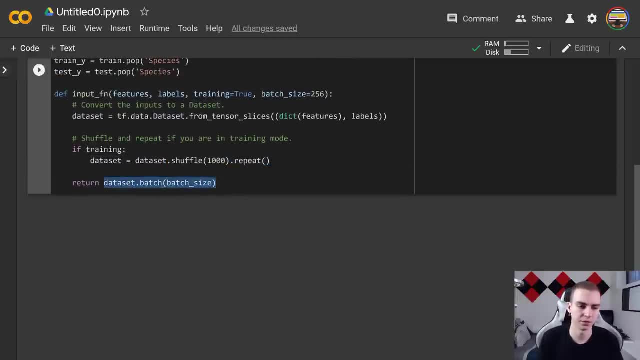 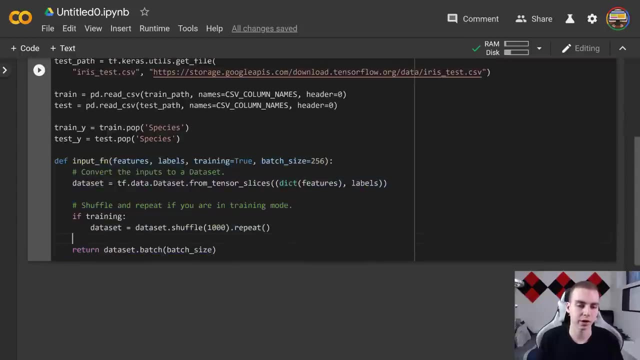 and then repeat that, And that is all we really need to do. we can do data set dot batch at the batch size 256, return that and we're good to go. So this is our input function. Again, these are kind of complicated. you kind of have to just get experience seeing a bunch of different ones to 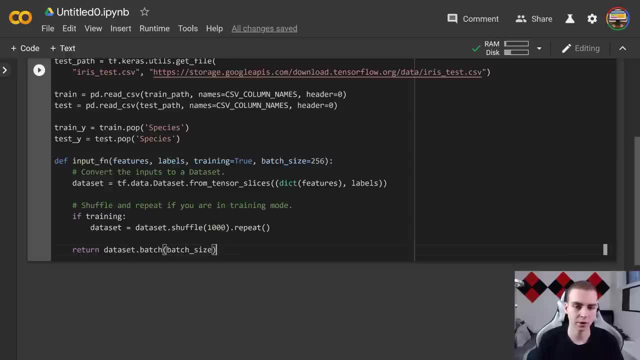 understand how to actually make one on your own. For now on, don't worry about it too much. you can pretty much just copy the input functions you've created before and modify them very slightly if you're going to be doing your own models. But by the end of this you should have a good idea of how these input functions. 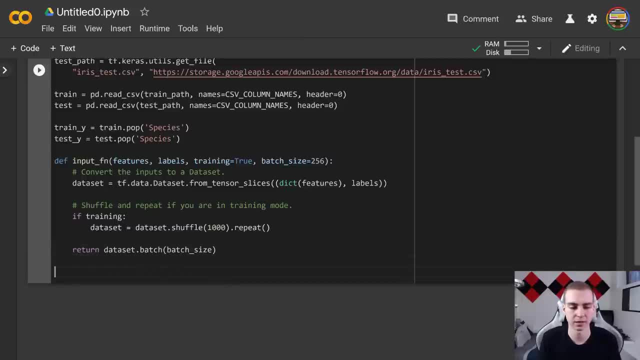 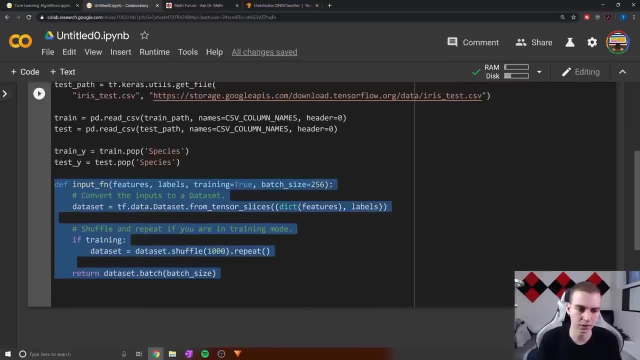 work. we will have seen like four or five different ones, And then you know, we can kind of mess with them and tweak them as we go on, but don't focus on it too much. Okay, so input function, this our input function. I'm not really going to go into much more detail with that. And now our 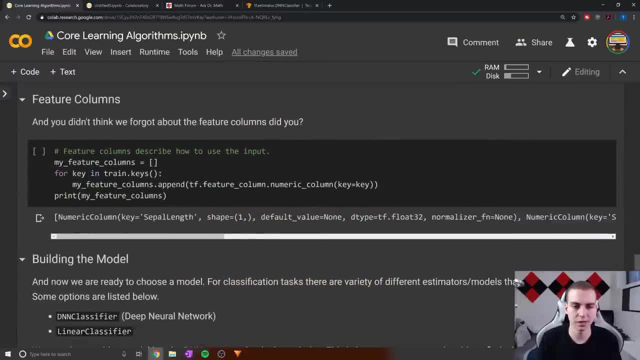 feature columns. So this is again pretty straightforward for the feature columns. all we need to do for this is, since all numeric feature columns is, rather than having two for loops where we were separating the numeric and categorical feature columns before we can just loop through all of the keys in our 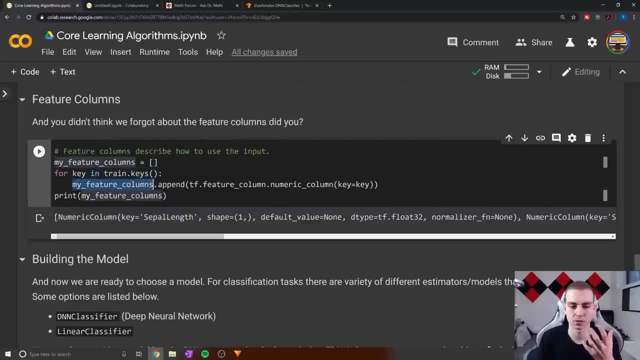 training data set And then we can append to my feature columns blank list the feature column dot numeric column And the key is equal to whatever key we've looped through here. Now I'm going to show you what this means in case anyone's confused. Again, you can see when I print my 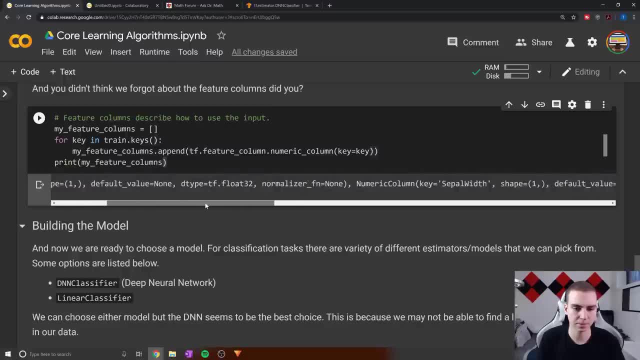 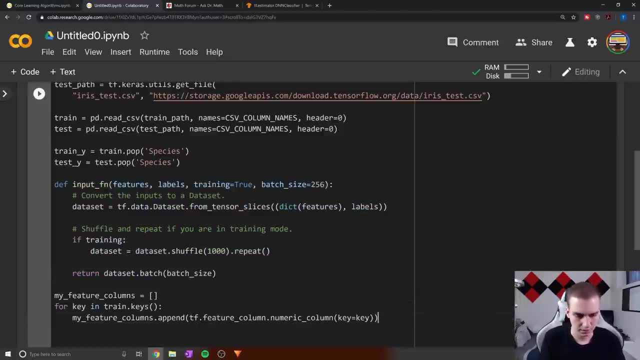 feature columns. we get key equals septal length, we get our shape and we get all of that other nice information. So let's copy this into the other one and have a look at our output after this. Okay, so my feature columns for key and train dot keys. So notice, train is here. train dot keys. 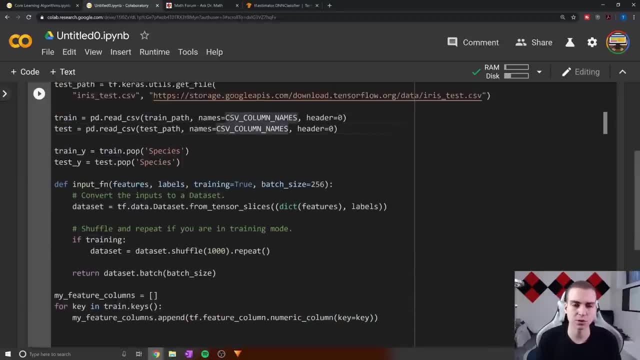 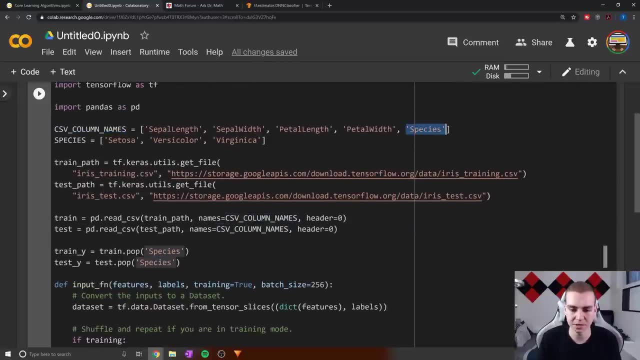 what that does is actually give us all the columns. So this was a really quick and easy way to kind of loop through all the different columns, Although I could have looped through CSV column names and just remove the species column to do that. But again, we don't really. 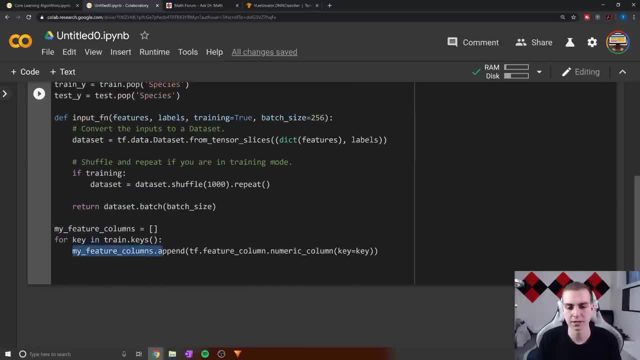 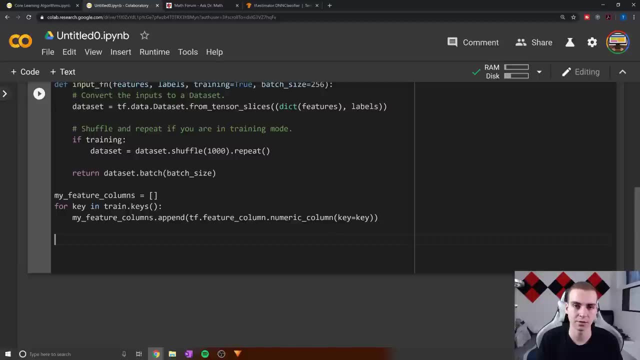 need to. So for key and train dot keys, my feature columns: dot. append TF. feature column: numeric column: key equals key. this was just going to create those feature columns. we don't need to do that vocabulary thing And that dot unique because, again, these are all already encoded for us. Okay. 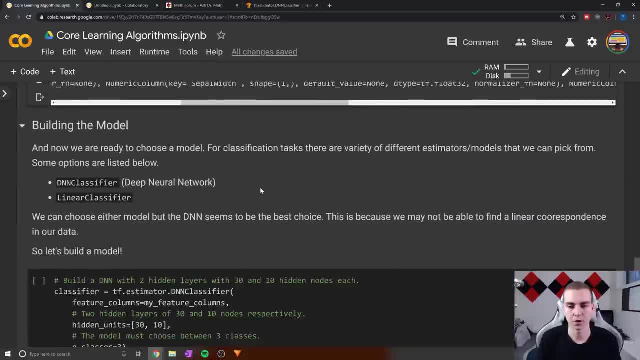 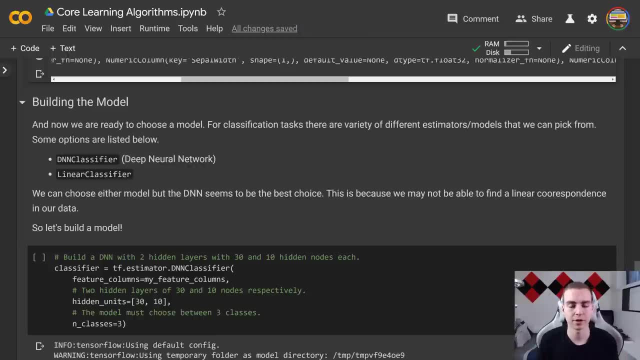 awesome. So that was the next step. So let's go back here building the model. Okay, so this is where we need to talk a bit more in depth of what we're actually going to build. So the model for this is a classification model. Now, there is like hundreds of different classification models we can. 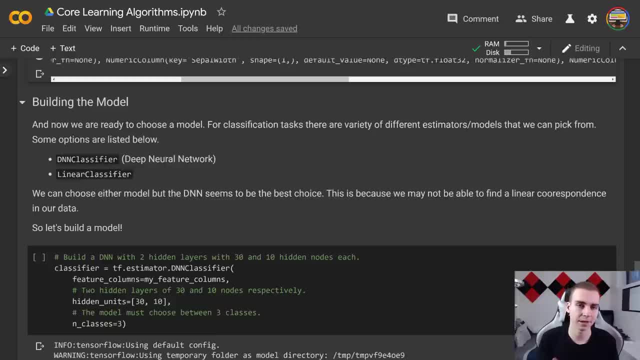 use that are pre made in TensorFlow. And so far what we've done with that linear classifier is that's a pre made model that we kind of just pre made. So we're going to go ahead and create this model and we're going to go ahead and create this model. So we're going to go ahead and create this model. 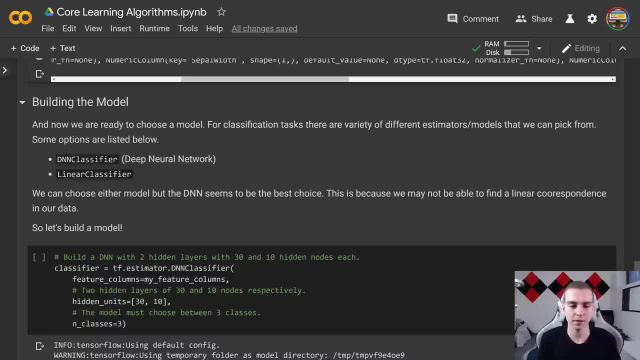 that we kind of just feed a little bit of information to, and it just works for us. Now, here we have two kind of main choices that we can use for this kind of classification task that are pre built in TensorFlow. we have a DNN classifier, which stands for a deep neural network, which 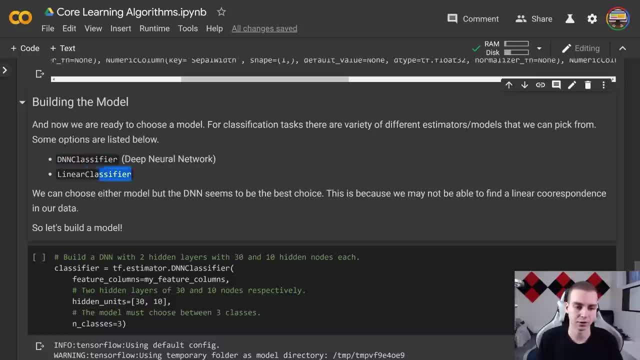 we've talked about very vaguely, very briefly, And we have a linear classifier. Now a linear classifier works very similarly to linear regression, except it does classification rather than regression, So we get actually numeric value or we get- sorry, you know the labels- like: 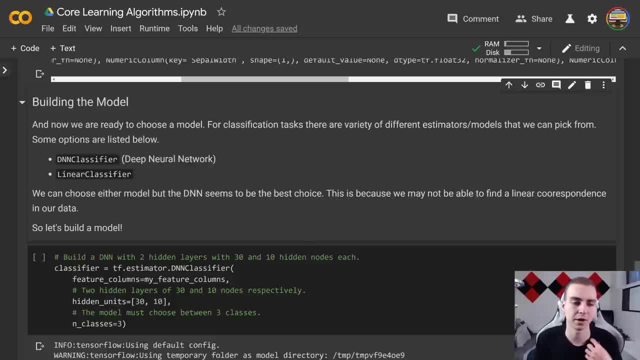 probability of being a specific label rather than a numeric value, But in this instance we're actually going to go with deep neural network. Now that's simply because TensorFlow on their website- like this is all of this- is kind of building off of TensorFlow website, just all the code is very similar And I've just added my own. 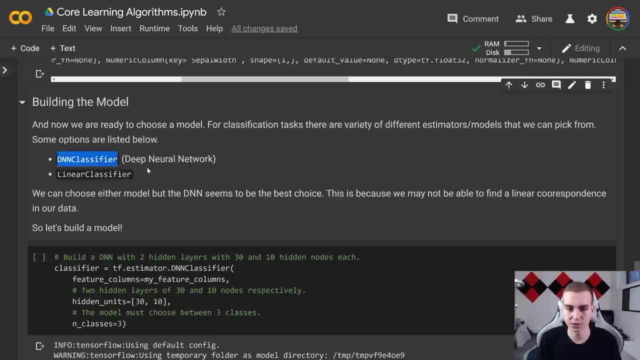 spin and explain things very in depth. They've recommended using that deep neural network, for this is a better kind of choice. But typically when you're creating machine learning apps, you'll mess around with different models and kind of tweak them And you'll notice that it's not. that difficult to change models because most of the work comes from machine learning. And you'll notice that it's not that difficult to change models because most of the work comes from machine learning. And you'll notice that it's not that difficult to change models because most of the work 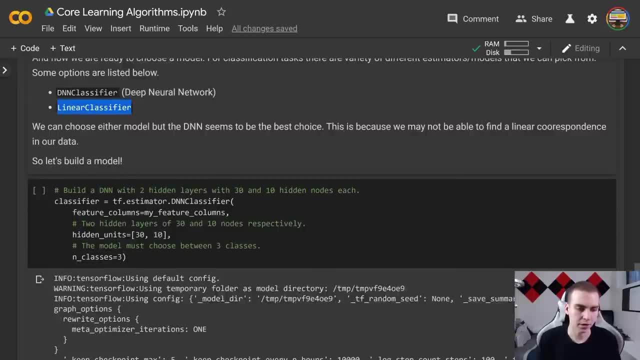 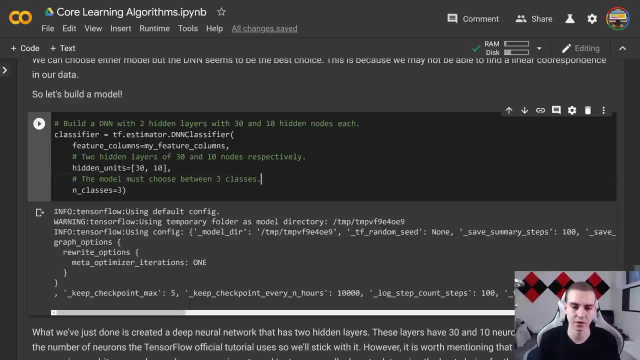 comes from loading and kind of pre processing our data. Okay, so what we need to do is build a deep neural network with two hidden- later two hidden layers with 30 nodes and 10 hidden nodes each. Now I'm going to draw out the architecture of this neural network in just one second, But I 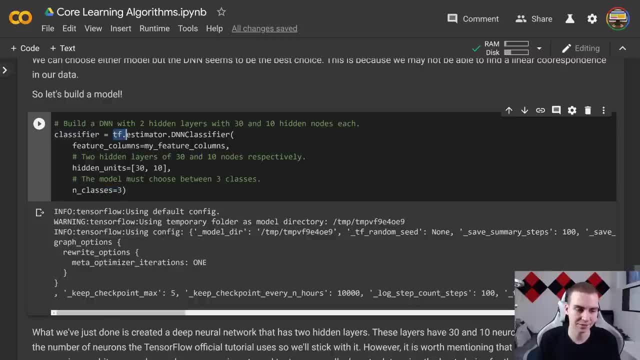 want to show you what we've done here. So we said classifier equals tf dot estimator. So this estimator module just stores a bunch of pre made models from TensorFlow. So in this case, DNN classifier is one of those. what we need to do is pass our feature columns, just like we did to our 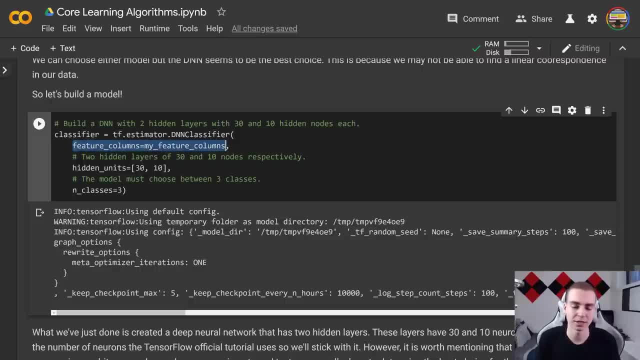 linear classifier. So, in this case, DNN classifier is one of those. what we need to do is pass our feature columns, just like we did to our linear classifier, And now we need to define the hidden units. Now, hidden units is essentially us a building, the architecture of the neural network. 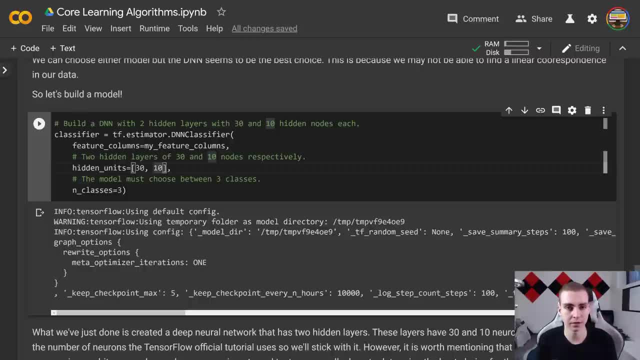 So, like you saw, before we had an input layer, we had some like middle layers, called our hidden layers in a neural network, And then we had our output layer. I'm going to explain neural networks in the next module, So this will all kind of click and make sense. For now we've arbitrarily decided. 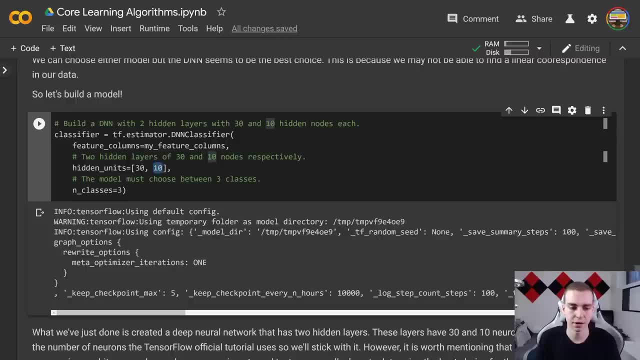 30 nodes in the first, hidden layer, 10 in the second, and the number of classes is going to be three. Now, that's something that we need to decide. we know there's three classes for the flowers, So that's what we've defined. Okay, so let's copy this in. go back to the other page. 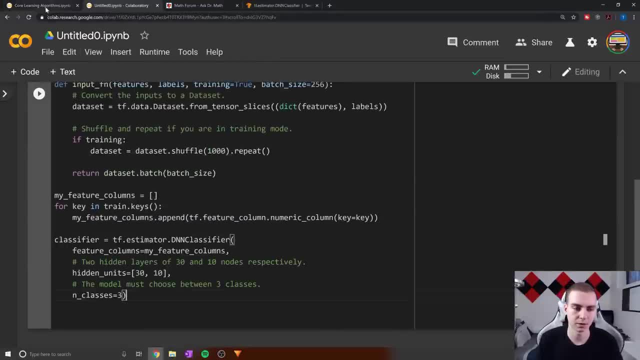 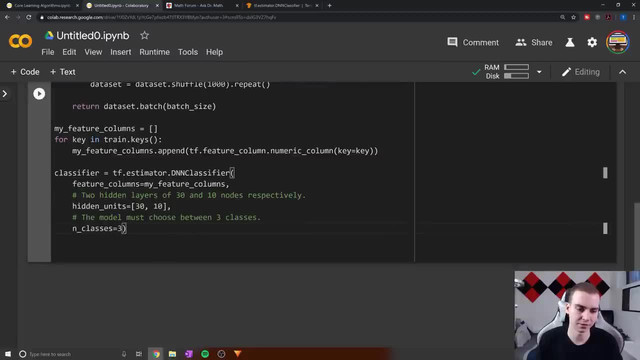 here, And that is now our model. Now it is time to talk about how we can actually train the model which is coming down here. Okay, so I'm going to copy this, I'm going to paste it over here And let's just dig through this, because this is a bit more of a complicated piece of code than we. 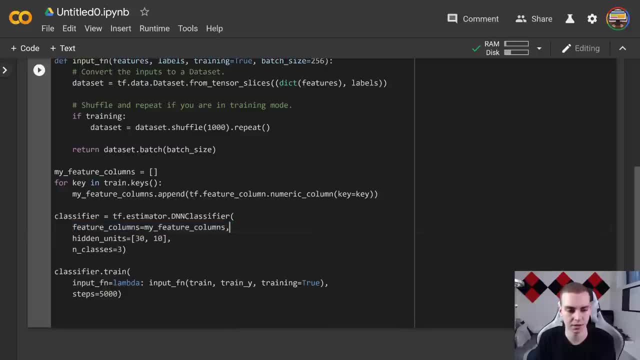 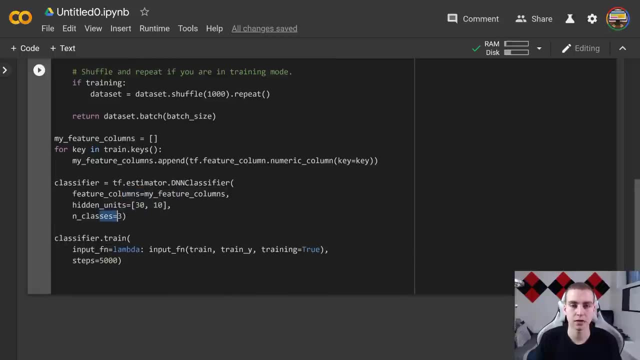 usually used to work with. I'm also going to remove these comments just to clean things up in here. So we've defined the classifier, which is a deep neural network classifier. we have our feature columns, hidden units, classes. Now to train the classifier, So we have this input function here. This input function is: 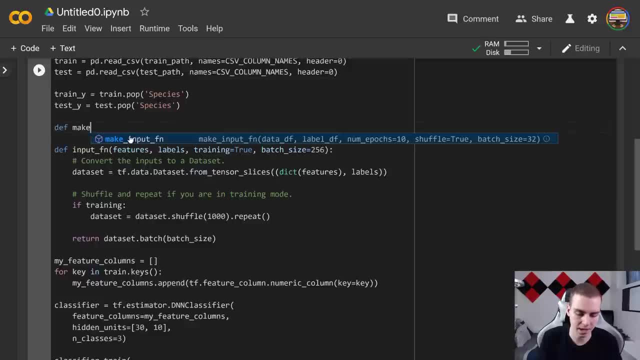 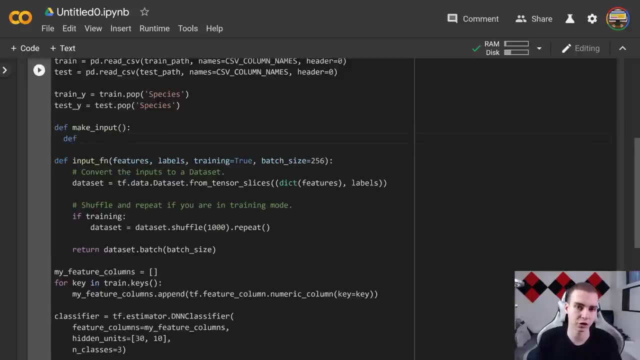 different than the one we created previously. remember when one we had previously was like: make input whatever function, I will continue typing in inside it to find another function, And it actually returned that function from this function. I know complicated if you're not a. 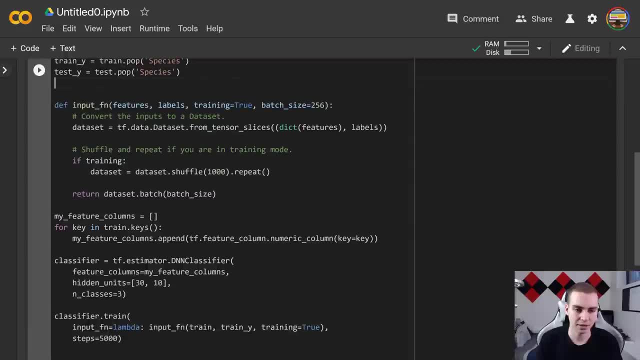 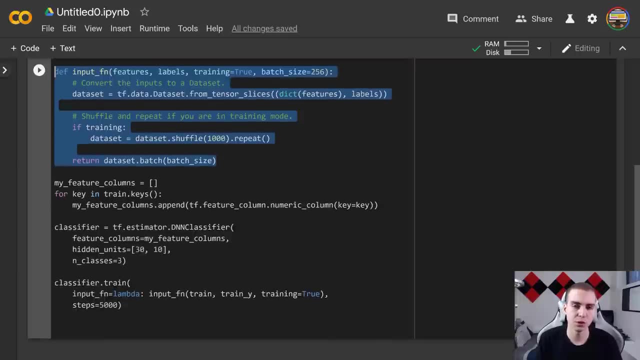 Python kind of pro. I don't expect that to make perfect sense, But here we just have a function right. we do not returning a function from another function, it just one function. So when we want to use this to train our model, what we do is create something called a lambda. Now, a lambda is an. 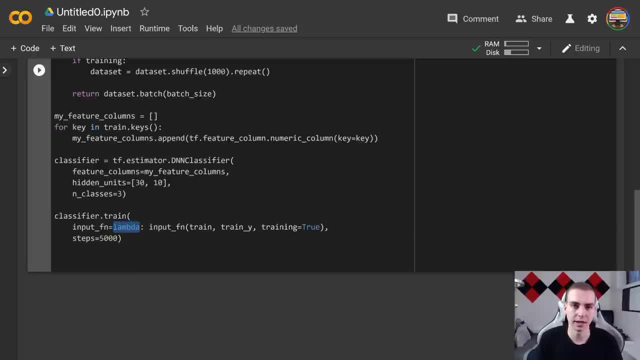 anonymous function that can be defined in one line. When you write lambda, what that means is essentially: this is a function, So this is a function, And whatever's after the colon is what this function does. Now, this is a one line function, So like if I create a lambda here: 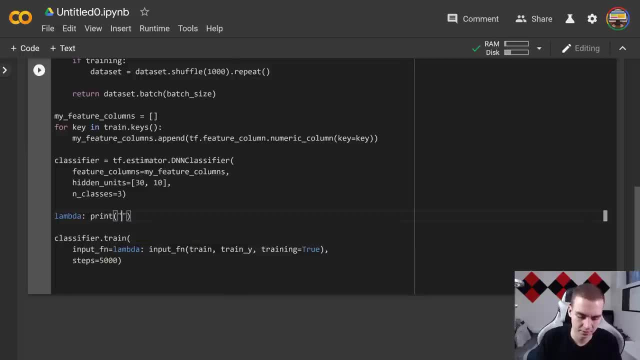 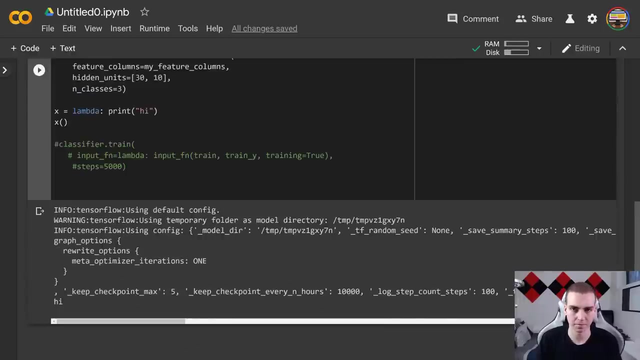 right, and I say lambda, print high, and I said x equals lambda and I called x like that this works. this is a valid line of syntax. Actually, I want to make sure that I'm not just like messing with you And I say that this is actually correct. Okay, so sorry, I just 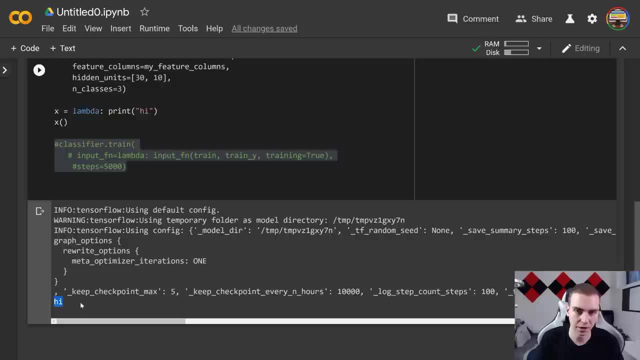 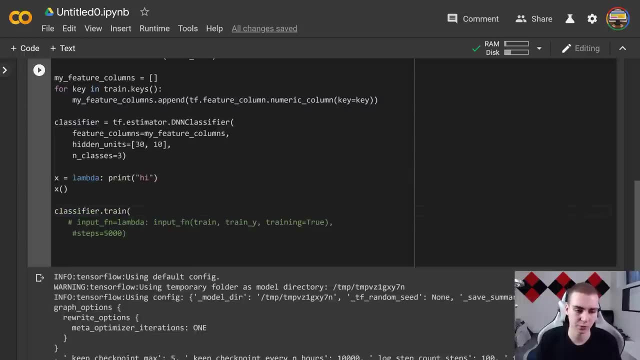 accidentally trained the model, So I just commented that out. You can see we're printing high right at the bottom of the screen. I know it's kind of small, but does say: hi, that's how this works. Okay, so this is a cool thing. If you haven't seen this in Python before, that's what a lambda does. 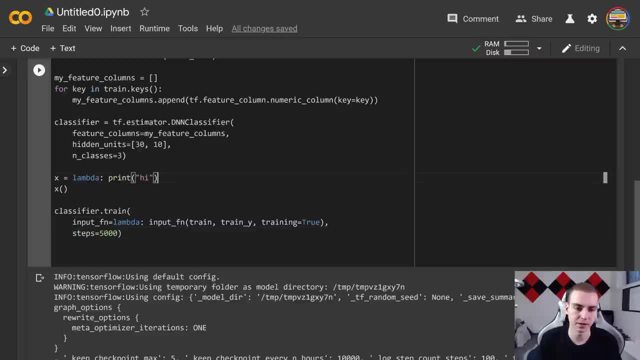 allows you to define a function in one line. Now, the thing that's great about this is that we can say: like you know, x equals lambda, and here put in a lambda, and then we can say: you know x. 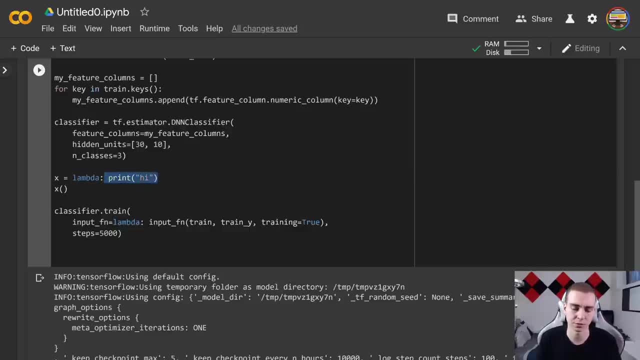 equals lambda, and here put in a lambda. and then we can say, like you know, x equals lambda and here put another function, which is exactly what we've done with this print function, And that means, when we call x, it will, you know, execute this function, which will just execute the other. 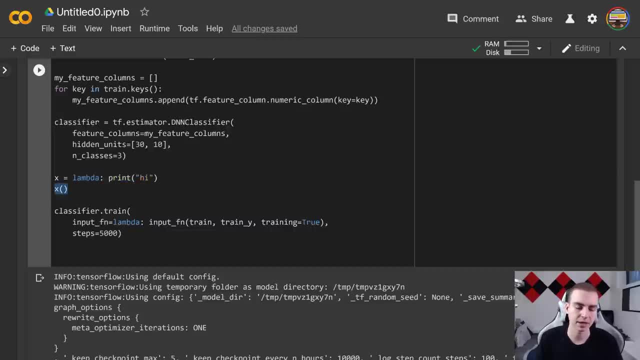 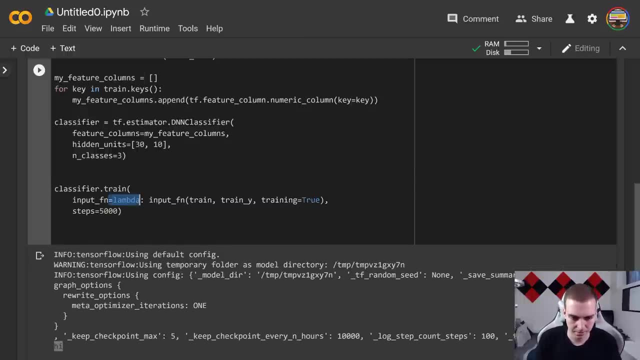 function. So it's kind of like a chain where you call x, x is a function And inside that function it does another function. right, It just like calling a function from inside a function. So what is lambda doing here? Well, since we need the actual function object, what we do is we. 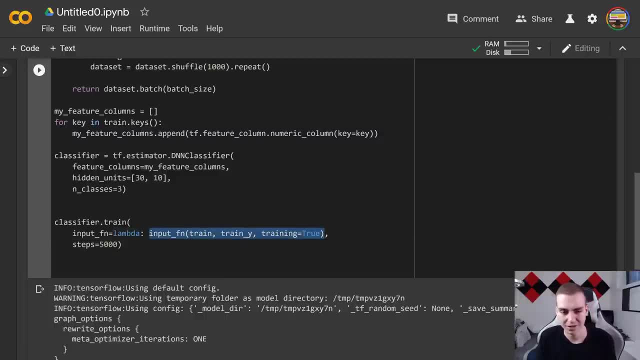 define a function that returns to us a function. So this actually just like it calls this function. when you put this here now there's- no, I can't it's. it's very difficult to explain this if you don't really understand the concept of lambdas And you don't understand the input. 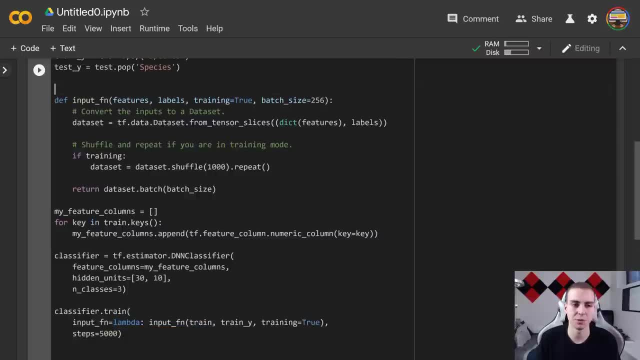 functions. But just know we're doing this because of the fact that we didn't embed another function and return the function object. If we had done that, if we had done that- you know, input function that we had created before where we had the interior function- then we wouldn't need to do. 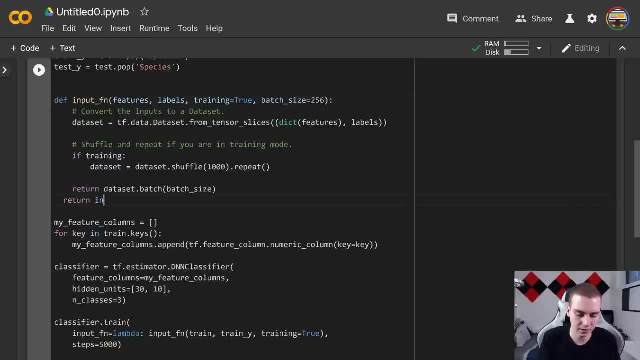 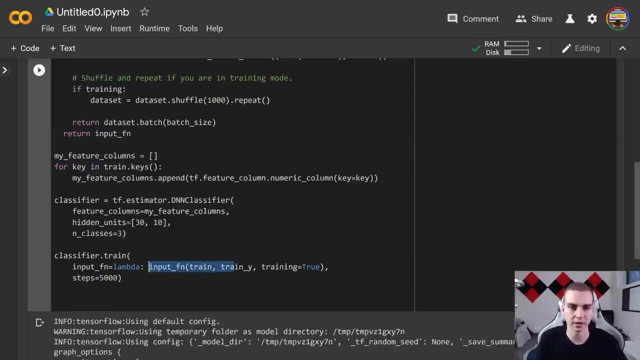 this, Because what would happen is we would return the input function, which is the input function, right like that, which means, when we passed it into here, it could just call that directly. it didn't need to have a lambda, Whereas here, though, since we need to just put a lambda, 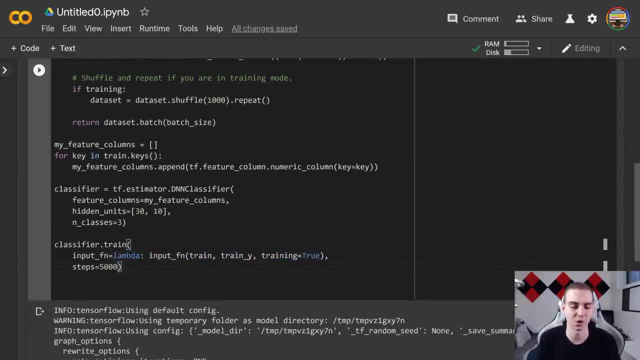 we need to define what this is, And then, and then this works. That's just this. there's no other way to really explain this. So, yeah, what we do is we create this input function, So we pass, we have train, we have train y, and we have training equals true. And then we do steps equals 5000. 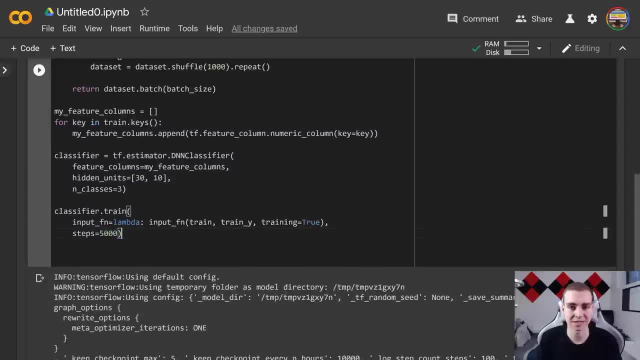 So this is similar to an epoch, except this is just defining a set Of amount of steps we're going to go through. So rather than saying like we'll go through the data set 10 times, we're just going to say we'll go through the data set until we've hit 5000. 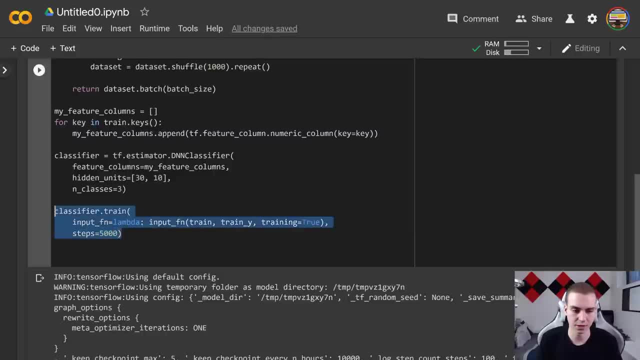 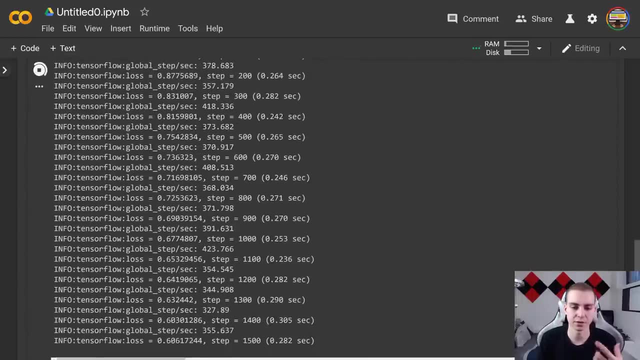 numbers like 5000 things that have been looked at. So that's what this does with that train. Let's run this and just look at the training output From our model. it gives us some like things. here we can kind of see how this is working. Notice that, if I can stop here for 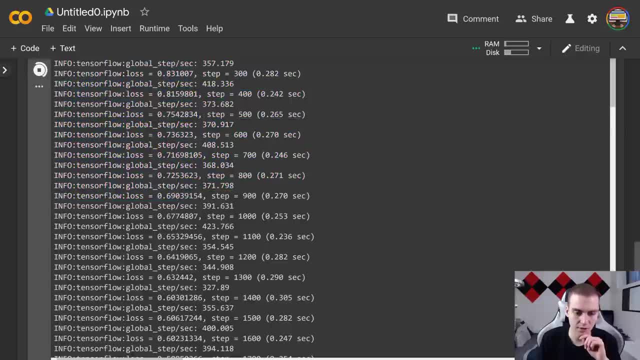 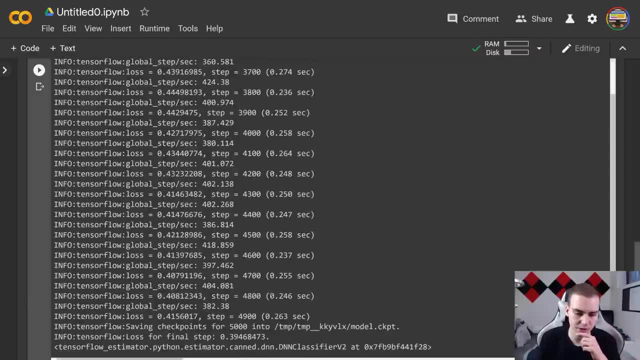 a second. it tells us the current step. it tells us the loss: the lowest, the lower this number, the better. And then it tells us global steps for a second. So how many steps we're completing per second? Now, at the end, here we get final step. 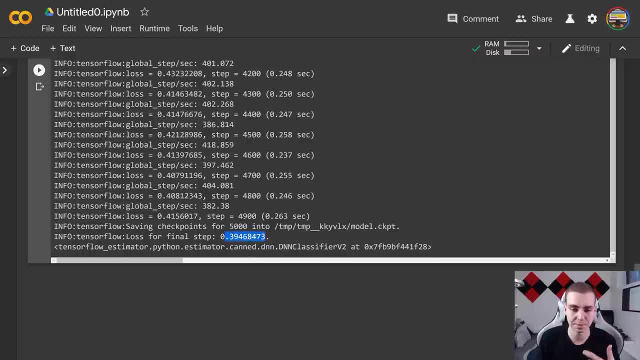 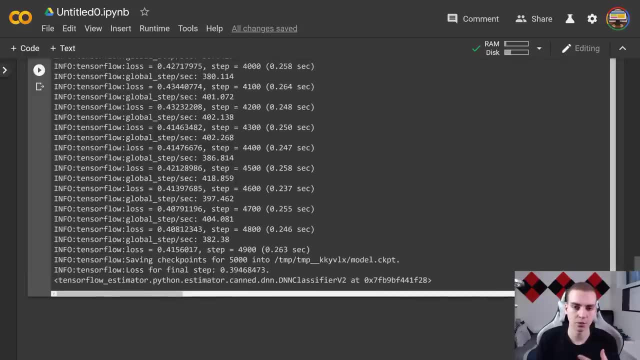 loss of 39,, which is pretty high, which means this is pretty bad, But that's fine. This is kind of just our first test at training a neural network. So this is just giving us output while it's training, to kind of see what's happening. Now, in our case, we don't really care because this 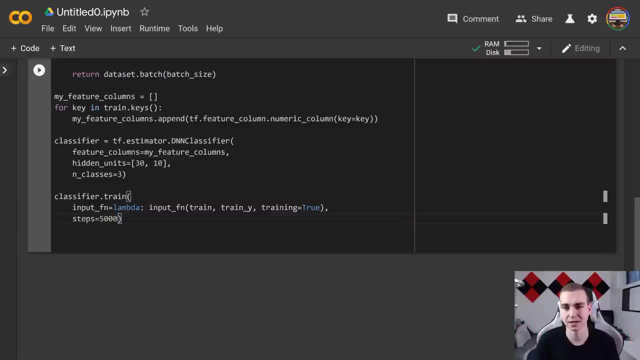 is a very small model. When you're training models that are massive and take terabytes of data, you kind of care about the progress of them. So that's when you would use kind of that output Right And you would actually look at that. Okay, so now that we've trained the model, 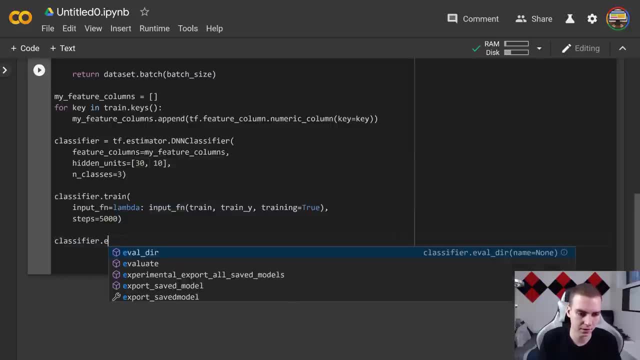 let's actually do an evaluation on the model. So we're just going to say classifier, dot, evaluate, And what we're going to do is a very similar thing to what we've done here is just pass this input function right, like here, with a lambda once again, and reason: we add the lambda when we don't. 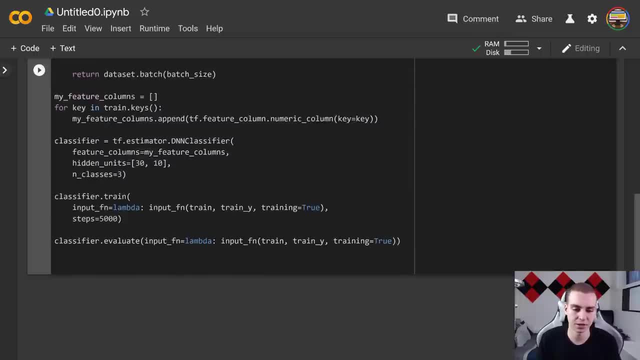 have this like double function going on, like a nested function, we need the lambda. And then here, what we do is, rather than passing train and train, why we're going to pass test. I believe and I think it's. I just called it test. So we're going to pass test, I believe and I think it's. I just 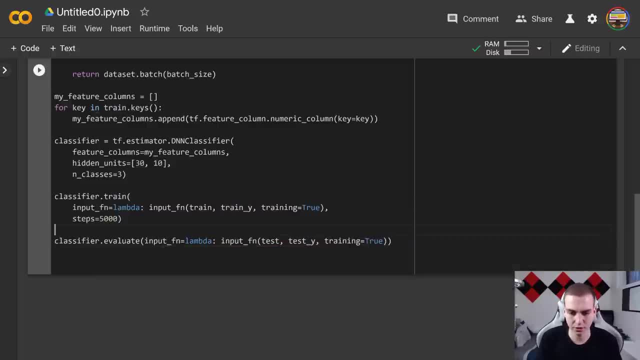 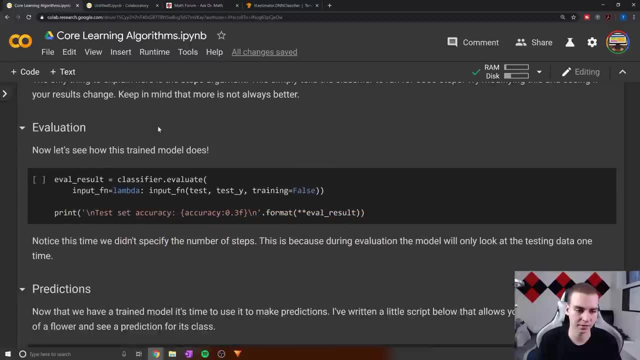 called it test y. Okay, and then for training. obviously this is false, So we can just set that false like that. I'm just going to look at the other screen to make sure I didn't mess this up, Because again I don't remember the syntax. Yeah, so cluster classifier dot. evaluate test test y. 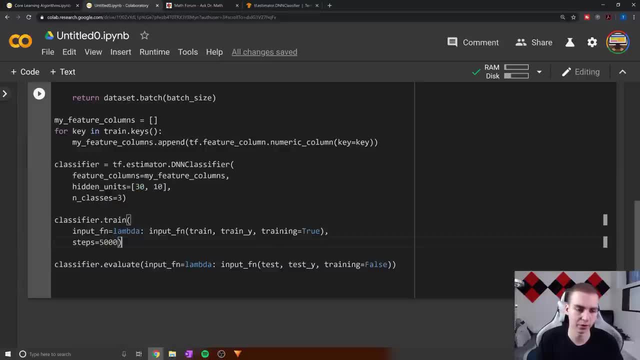 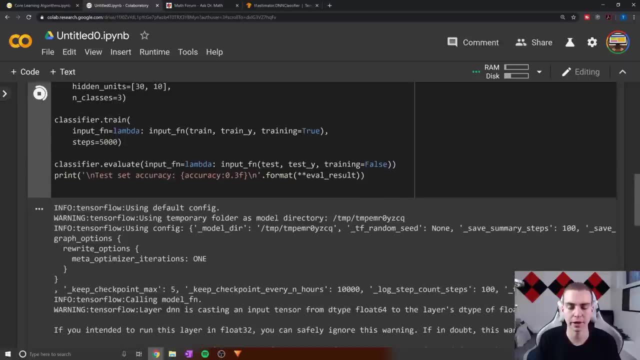 looks good to me. We'll take this print statement just so we get a nice output for our accuracy. Okay, so let's look at this Again. we're gonna have to wait for this to train, But I will show you a way that we don't need to wait for this to train every time in one second. 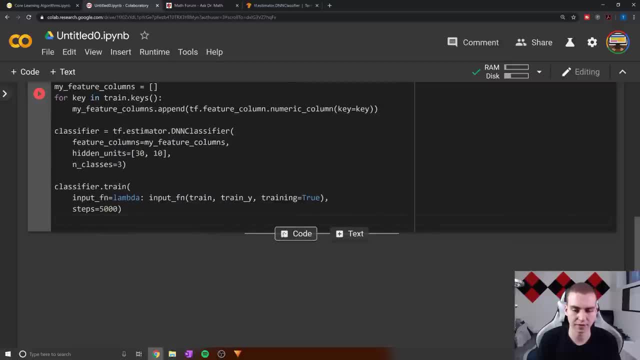 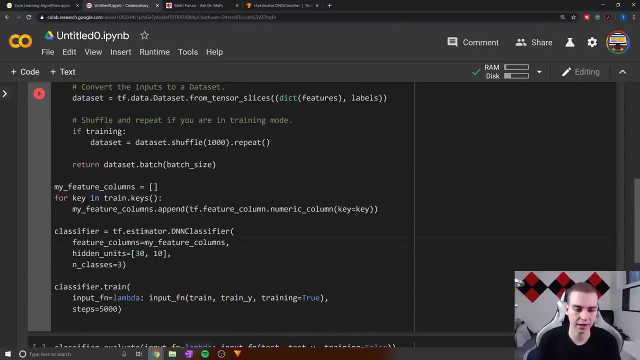 We'll be right back, Okay. so what I'm actually going to do- and I've just kind of pause, like the execution of this code- is throw this in the next block under, because the nice thing about Google Collaboratory is that I can run this block of code. right, I can train all this stuff, which is 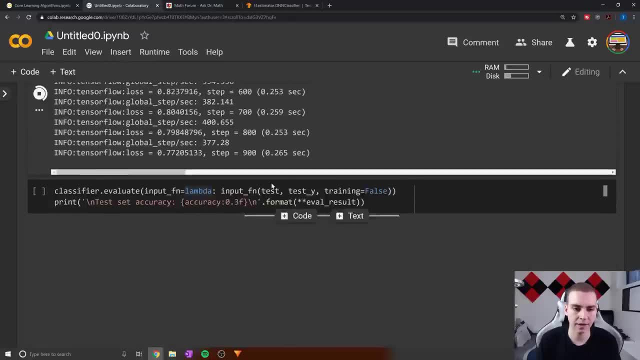 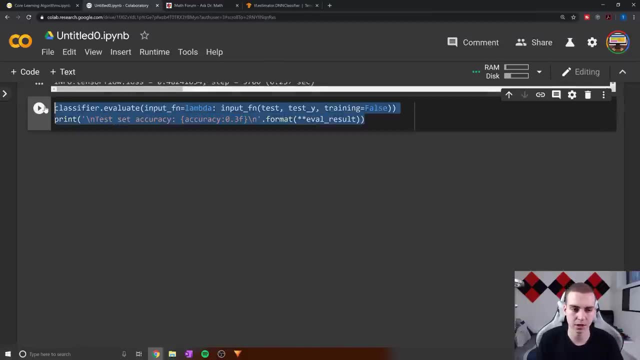 what I'll run now while we're talking, just so it happens. And then I can have another code block kind of below it, which I have here, And it doesn't matter, I don't need to rerun that block every time I change something here. So if I change something in any lower blocks I don't need to. 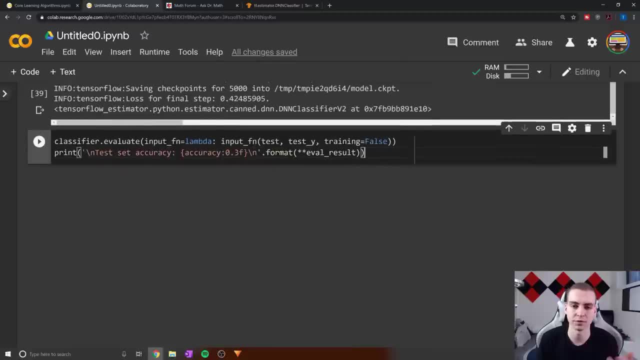 change the upper block, which means I don't need to wait for this to train Every time I want to do an evaluation on it Anyways. so we've done this, we've done tests, we got test. why I just need to change this instead of eval result? Actually, I need to say: 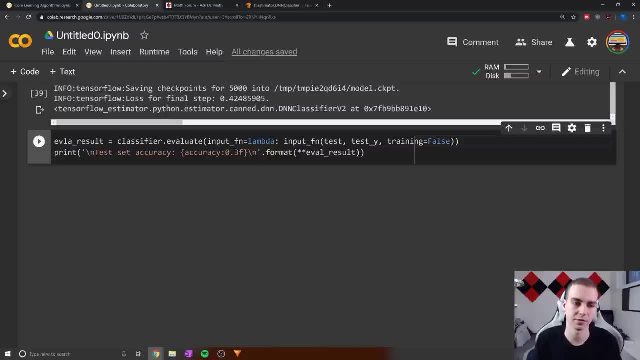 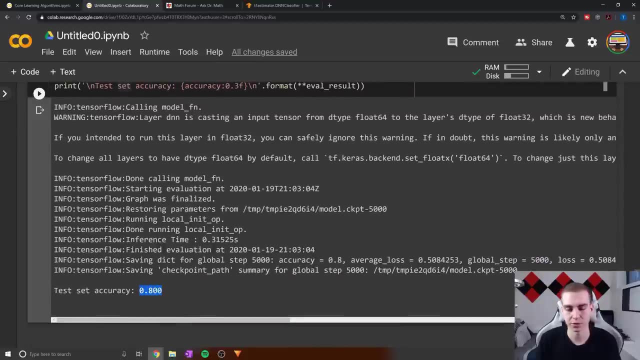 eval underscore results. equals classifier to evaluate so that we can actually store this somewhere and get the answer. And now we'll print this and notice this happens much, much faster. we get a test accuracy of 80%. So if I were to retrain the model, chances are this accuracy. 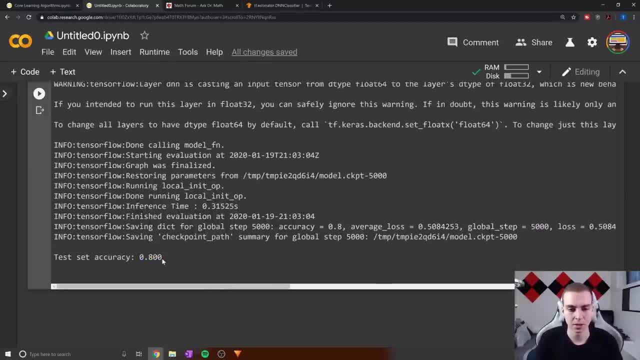 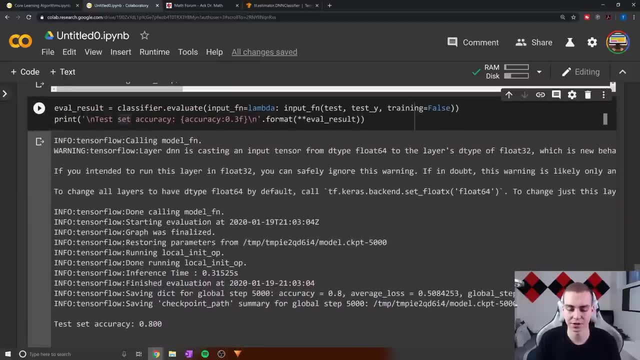 would change again because of the order in which we're seeing different flowers. But this is pretty good. We don't have that much test data And we don't really know what we're doing right. We're kind of just messing around and experimenting for right now. So to get 80% is pretty good, Okay. 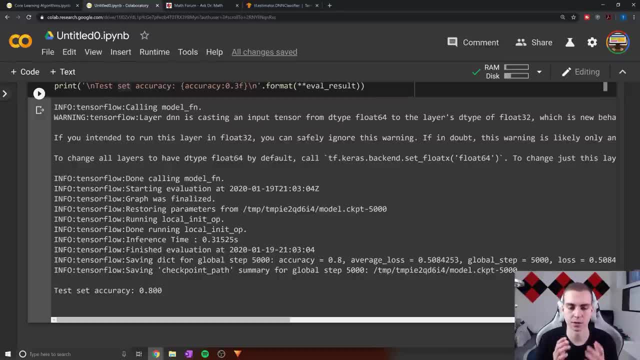 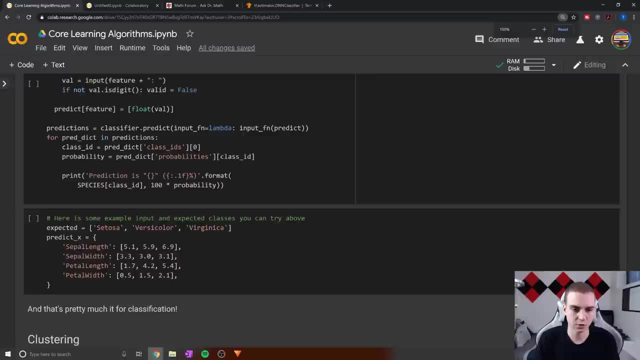 so actually, what am I doing? we need to go back now and do predictions. So how am I going to predict this for specific flowers? So let's go back to our core learning algorithms And let's go to predictions Now. I've written a script already just to save a bit of time that allows. 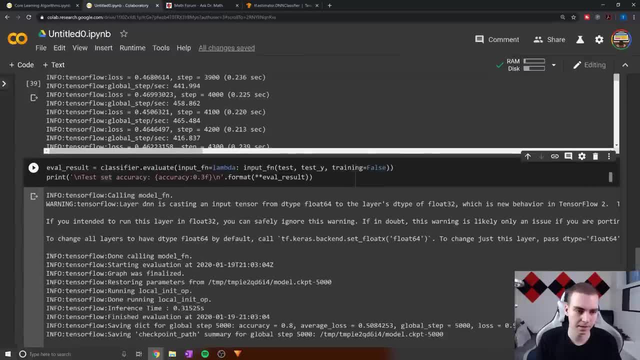 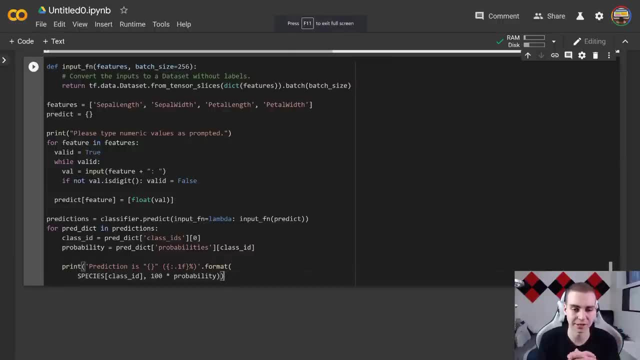 us to do a prediction on any given flower. So what I'm going to do is create a new block down here, this function, And now we're going to digest this and kind of go through this on our own to make sure this makes sense. But what this little script does is allow the user to type in some numbers. So 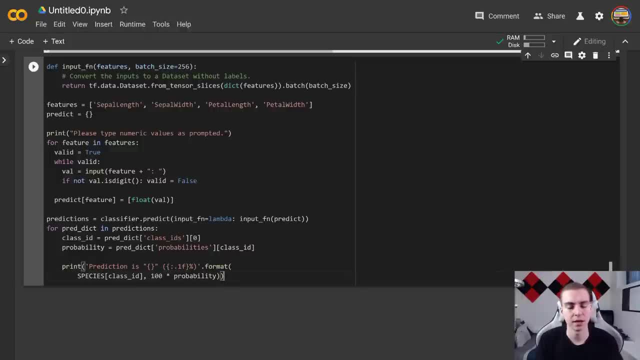 the subtle length, width and, I guess, petal length and width, and then it will spit out to you what the predicted class of that flower is. So we could do a prediction on every single one of our data points, like we did previously, And we already know how to do that. I showed you that with linear. 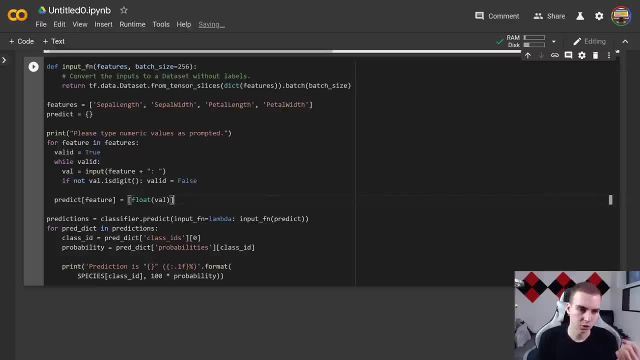 regression. But here I just wanted to do it on one entry. So what do we do? So I start by creating a input function. it's very basic. we have batch size 256.. All we do is we give some features. 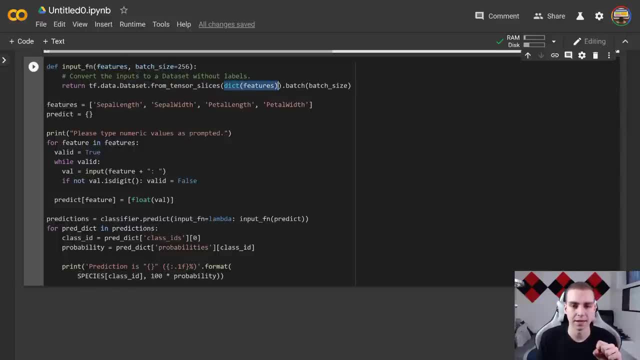 and we create a data set from those features. that's a dict, and then dot batch and the batch size. So what this is doing is notice we don't give any y value. right, we don't give any labels. the reason we do we don't do that is because when we're making a prediction, we don't know the 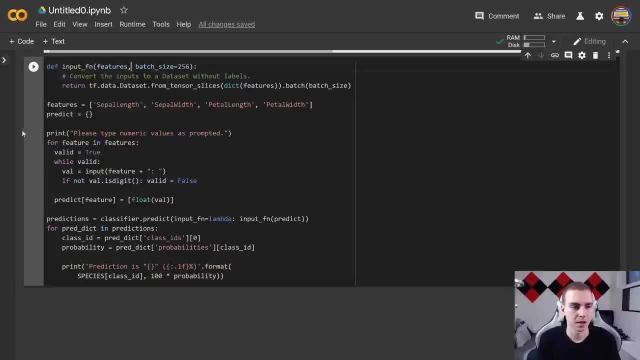 label right, Like we actually want that the model to give us the answer. So here I wrote down the features. I create a predict dictionary just because I'm going to add things to it And then prompt it here With a print statement. please type numeric values. has prompted, So for feature. 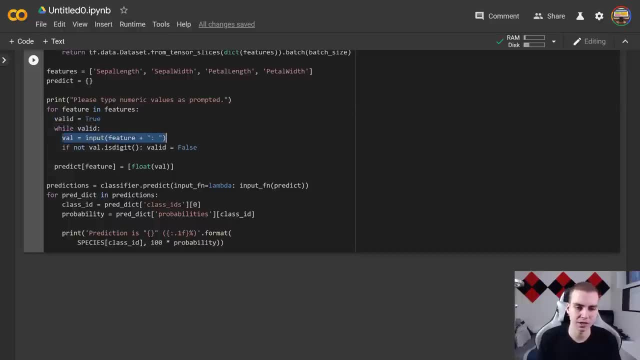 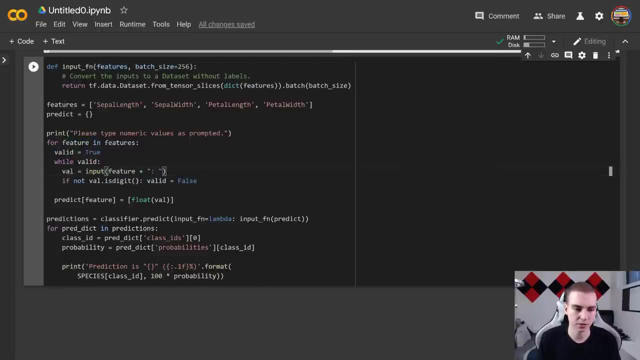 and feature valid equals. true, well, valid valve equals input feature con. So this just means what we're going to do is, for each feature we're going to wait to get some valid response. Once we get some valid response, what we're going to do is add that to our dictionary. So we're going to say: 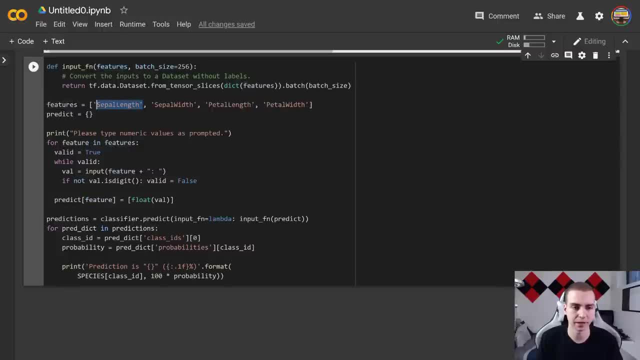 predict feature. so whatever that feature was, so septal length, septal width, petal length or pepped petal width is equal to a list that has, in this instance, whatever that value was. Now, the reason we need to do this is because 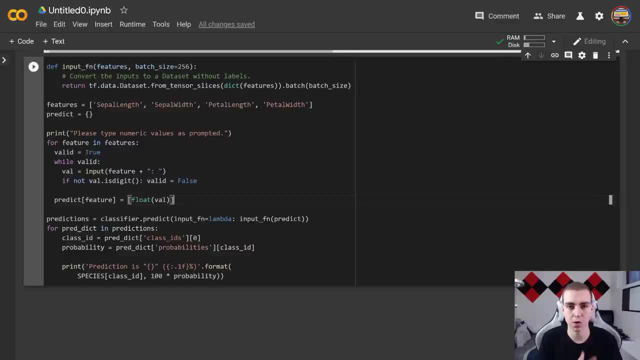 again, the predict method from TensorFlow works on predicting for multiple things, not just one value. So even if we only have one value, we want to predict for it. we need to put it inside of the list because it's expecting the fact that we will probably have. 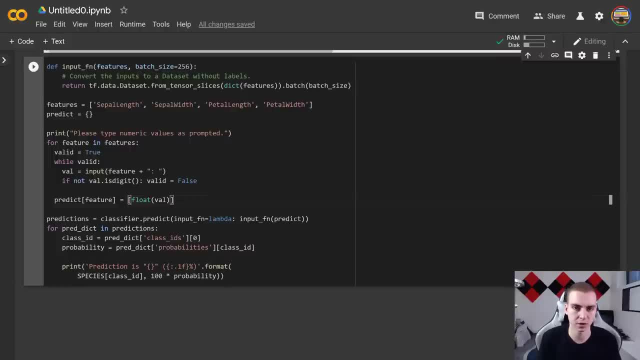 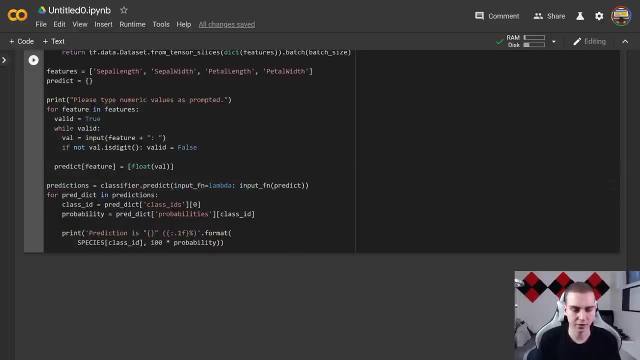 more than one value, in which we would have multiple values in the list right, each representing a different row or a new flower to make a prediction for. Okay, now we say predictions equals classifier, dot predict, And then, in this case, we have input function, lambda input. 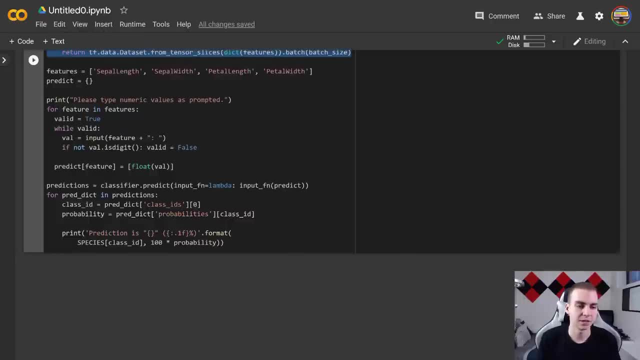 function predict, which is this input function up here. And then we say for prediction dictionaries- because remember every prediction comes back as a dictionary in predictions we'll say the class ID is equal to whatever the class IDs of the prediction dictionary, at zero. 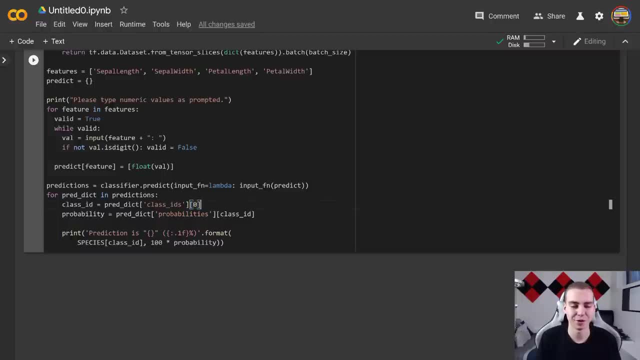 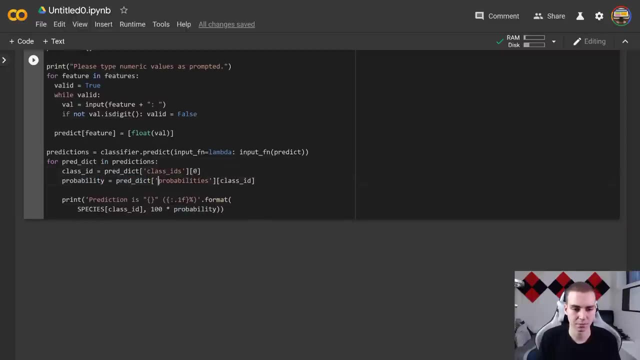 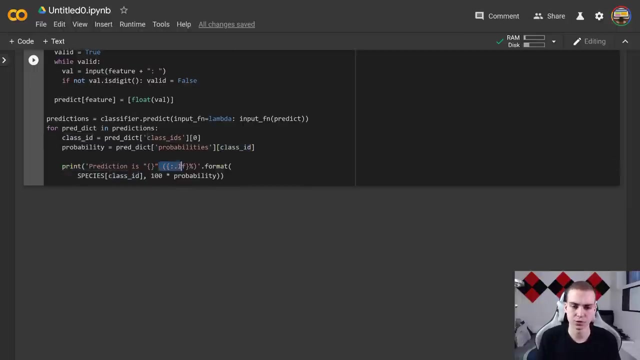 And these are simply what. I don't know exactly how to explain this. We'll look at in a second. I don't go through that. And then we have: the probability is equal to the prediction dictionary probabilities of class ID. Okay, then we're going to say print: prediction is within do. 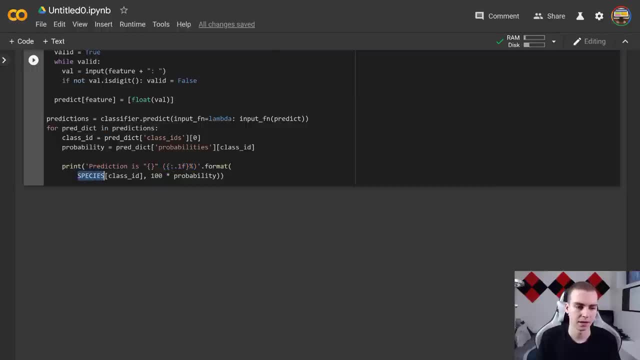 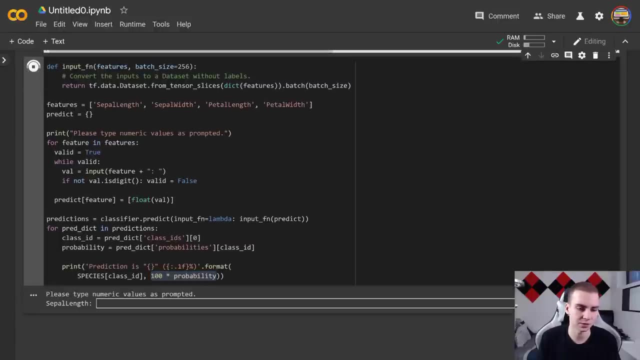 this weird format thing. I just stole this from TensorFlow And it's going to be the species at the class ID and then 100 times probability, which will give us actual integer value. we're going to digest this, but let's run this right now and have a look, So please. 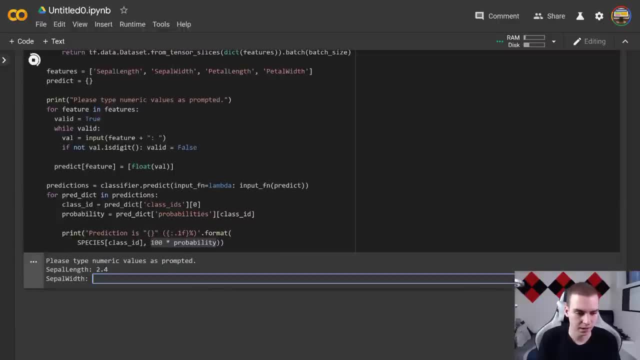 type numeric values as prompted. subtle length: let's type like 2.4, sub the width: 2.6,. pedal width: let's just say that's like 6.5.. And yeah, pedal width like 6.5. And then we're. 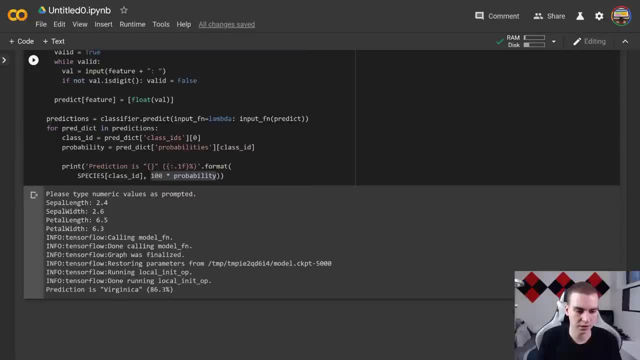 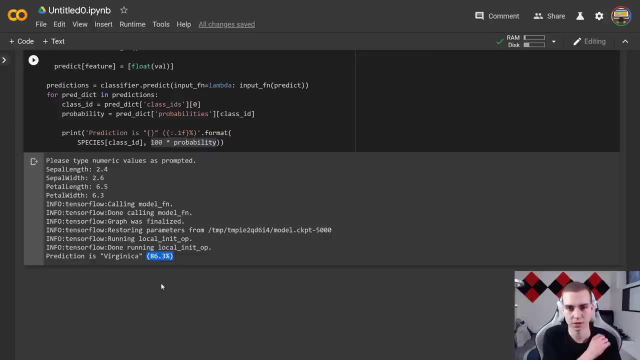 going to have like 6.3.. Okay, so then it calls this and it says: prediction is virginica- I guess that's the the class we're going with- And it says that's an 83 or 86.3% chance that. 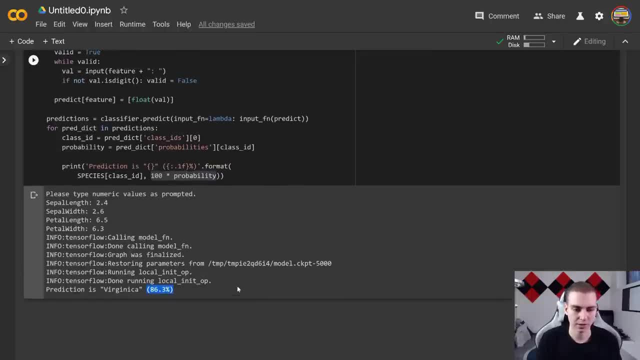 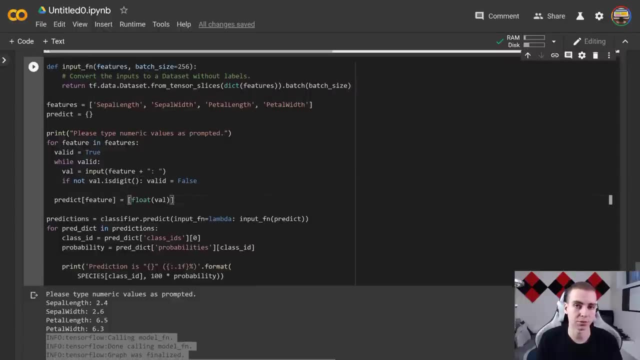 that is the prediction. So yeah, that is how that works. So that's what this does. I wanted to give a little script. I wrote most of this- I mean, I stole some of this from TensorFlow- But just to show you how we can actually predict on one value. So let's look at these prediction. 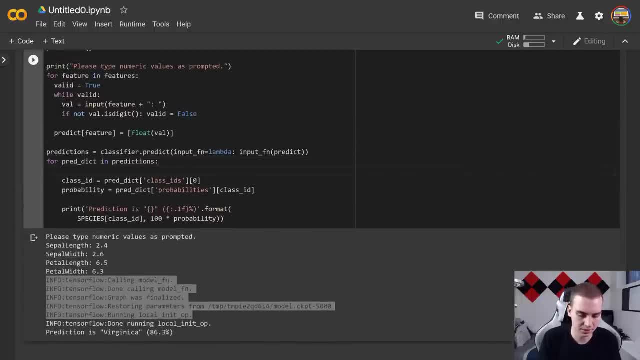 dictionary, because I just want to show you what one of them actually is. So I'm going to say print pred, underscore dict, And then this will allow me to actually walk through what class IDs are, probabilities are and how I've kind of done this. So let's run this up to. 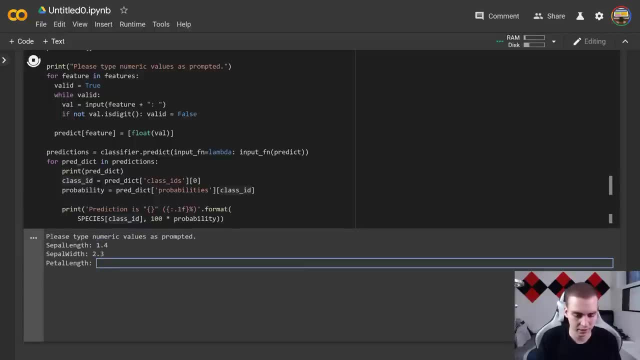 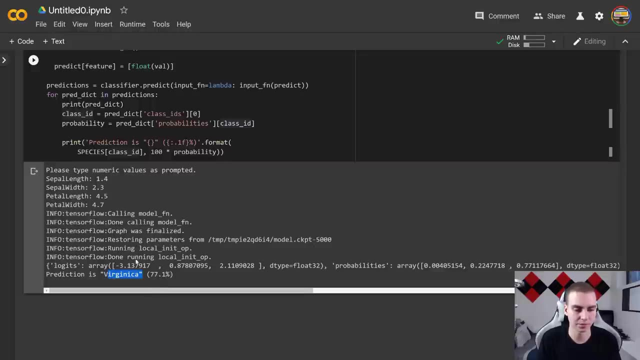 length. let's just go like 1.4, 2.3.. I don't know what these values are going to end up being. And we get- prediction is same one with 77.1%, Which makes sense because these values are similar to, kind of in difference to what I did before. Okay, so this is the dictionary. 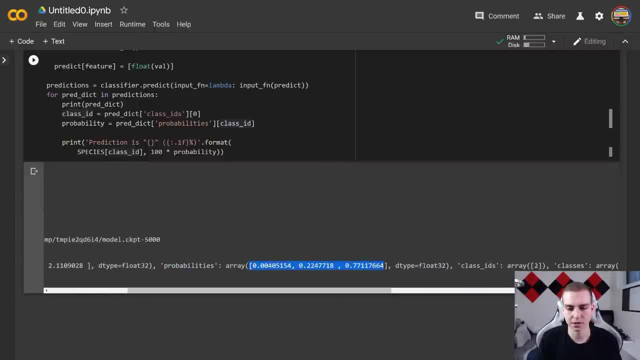 So let's look for what we were looking for. So we're going to go to probabilities. notice: we have three probabilities, one for each of the different classes, So we can actually say what you know, the percentages for every single one of the predictions. then what we have is class IDs. Now, class IDs, what this? 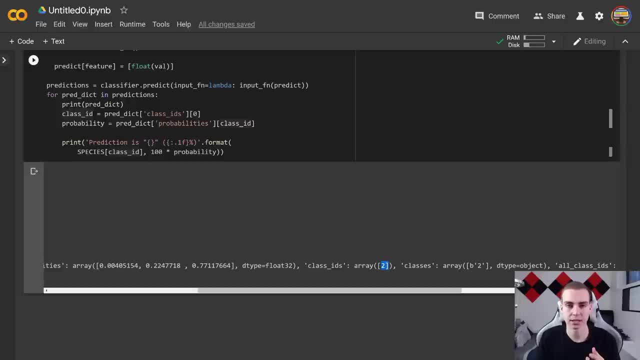 does is tell us what class ID it predicts is actually the flower, right? So here it says two, which means that this probability at 77%, that's that index two in this array right? So that's why this value is two. So it's saying that that class is actually the. 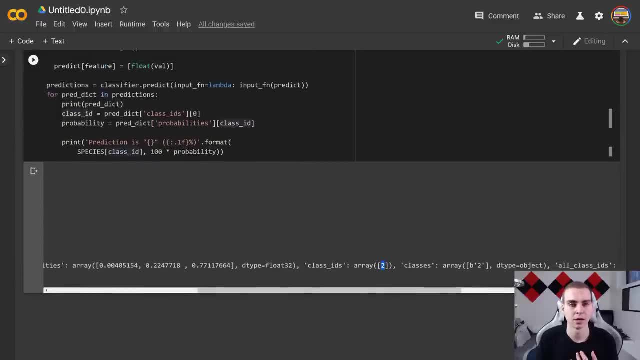 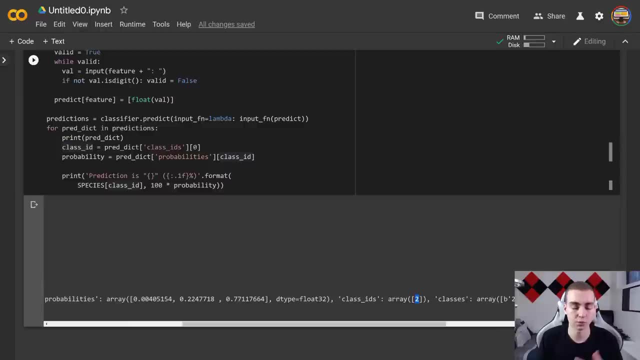 class is to, it thinks it's class two, like that's. whatever was encoded in our system is two And that's how that works. So that's how I know which one to print out is, because this tells me it's class two, And I know from making this list all the way back up here. 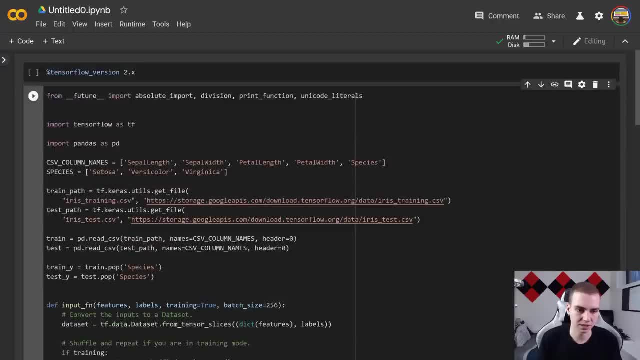 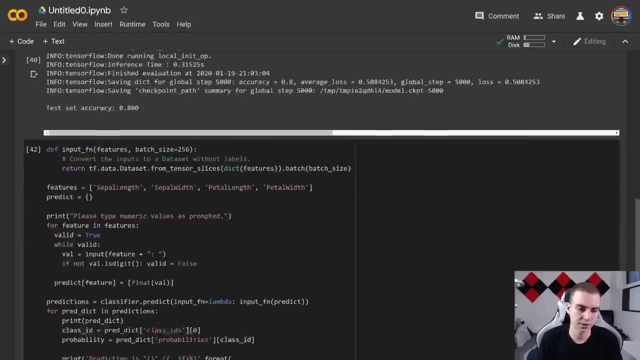 if I can get rid of this output? where is it, when I say species, that number two is a virginica, or I guess that's how you say it. So that is what the classification is And that's what the prediction is. So that's how I do that And that's. 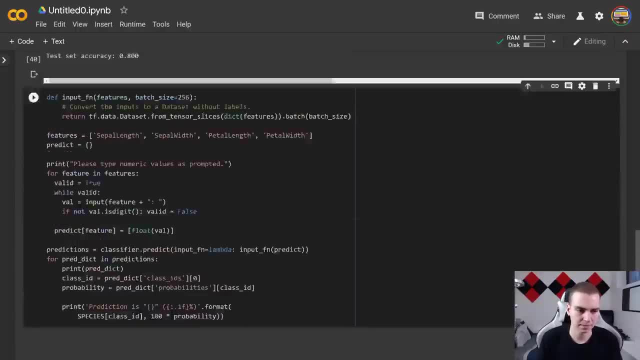 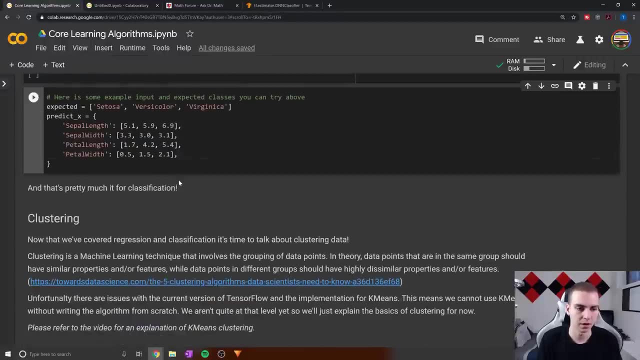 that's how that works, Okay, so I think that is pretty much it for actually classification. So it's pretty basic. I'm going to go and see if there's anything else that I did for classification in here, Okay. so here I just put some examples. So here's some example. 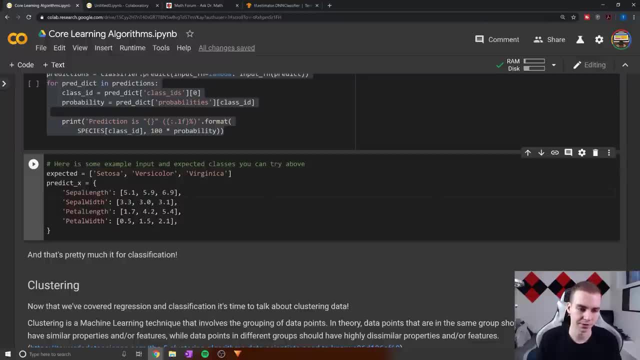 input expected classes. So you guys could try to do these if you want. So, for example, this one septal length, septal width, So for 5.1, 3.3, 1.7 and 0.5, the output should. 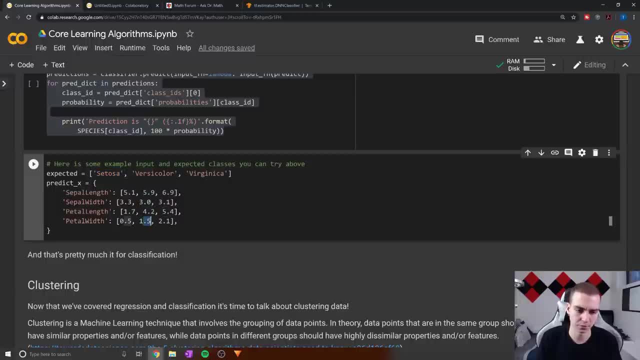 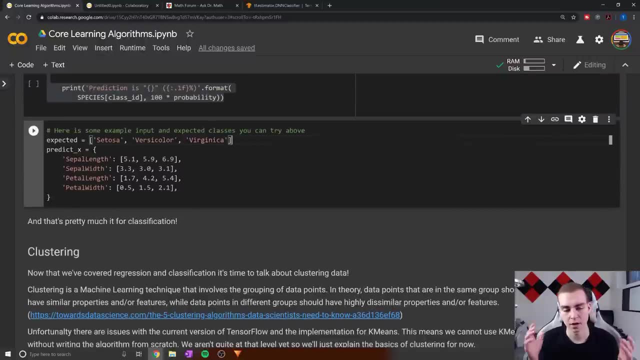 be setosa for 5.9, 3.0, 4.2, 1.5, it should be this one And then obviously this for this, just so you guys can mess with them if you want. but that's pretty much it for classification. 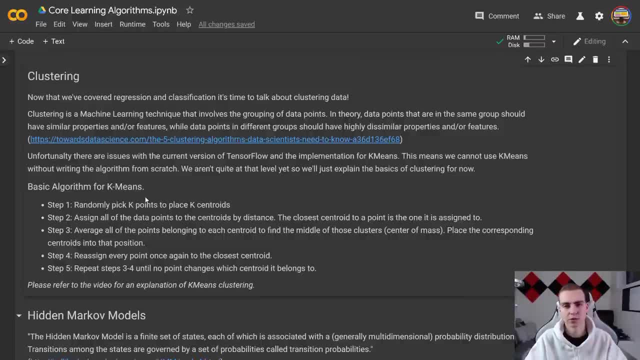 And now on to clustering. Okay, so now we're moving on to clustering. Now, clustering is the first unsupervised learning algorithm that we're going to see in this series, And it's very powerful. Now, clustering only works for a very specific set of problems, And you. 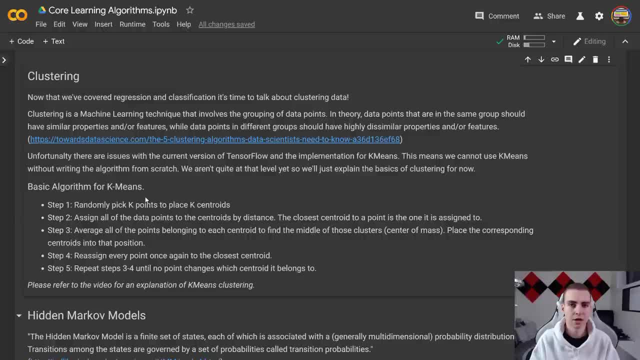 use clustering when you have a bunch of You're going to see in this series and it's very powerful. Now, clustering only works for a very specific set of problems and you use clustering when you have a bunch of input information or features but you don't have any labels or output information. 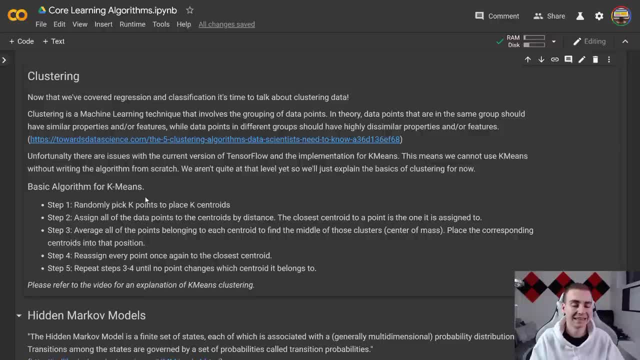 Essentially what clustering does is finds clusters of like data points and tells you the location of those clusters. So you give a bunch of training data. you can pick how many clusters you want to find. So maybe we're going to be classifying digits right handwritten. 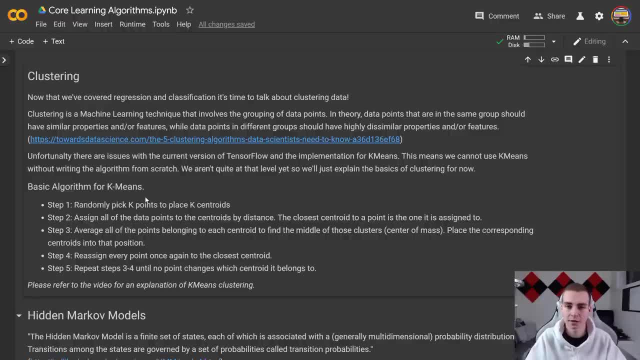 digits. using k means clustering. In that instance we would have 10 different clusters for the digits 0 through nine and you pass all this information and the algorithm actually finds those clusters in the data set for you. we're going to walk through an example. it'll make sense, But 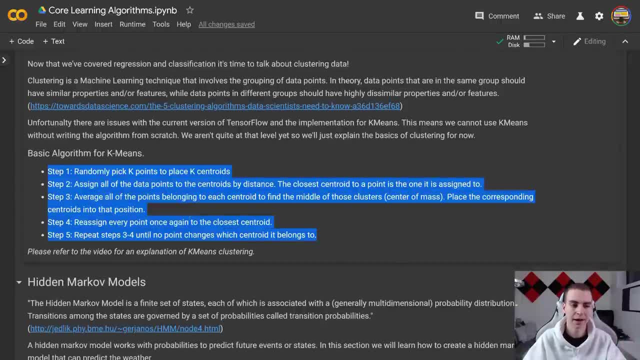 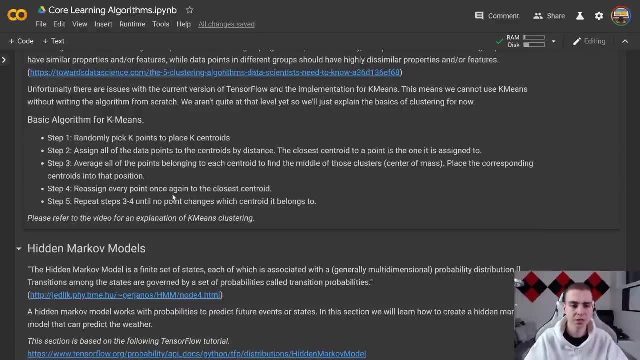 I just want to quickly explain the basic algorithm. behind k means essentially the set of steps, because I'm going to walk you through them and with a visual example. So we're going to start by randomly picking k points to place k centroids. Now, a centroid stands for where 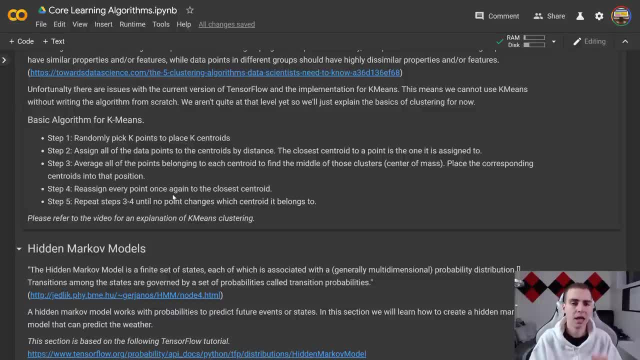 our current cluster is kind of defined and we'll see it in a second. The next step is we're going to assign all of the data points to the centroids by distance. So actually, now that I'm talking about this, I think it just makes more sense to get right. 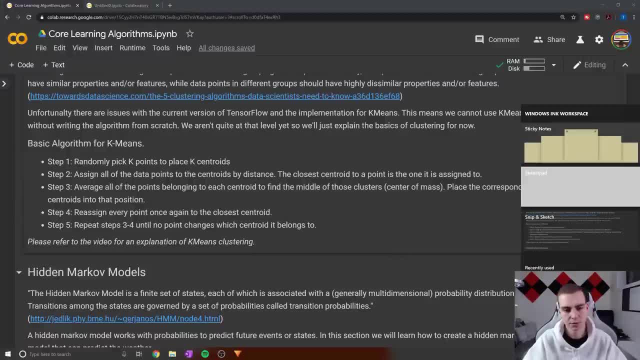 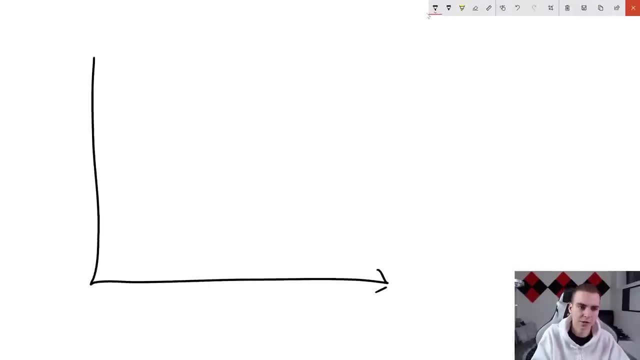 into the example, Because if I keep talking about this, you guys are probably just going to be confused, Although I might come back to this just to reference those points. Okay, so let's create a little graph like this in two dimensions for our basic example, And 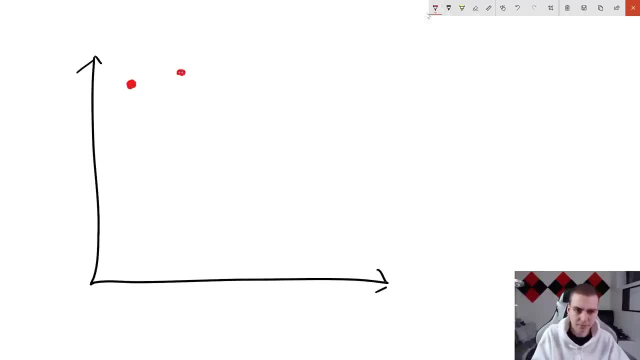 let's make some data points here. So I'm just gonna make them all red And you're gonna notice that I'm gonna make this kind of easier for ourselves by putting them in like their own unique little group, Right? So actually we'll add one up here And we can add some down here and down here. 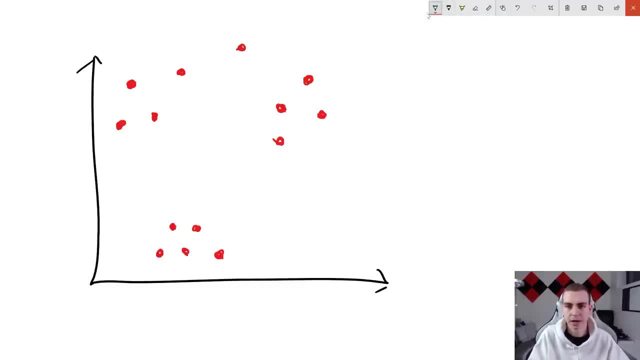 Now the algorithm starts, for k means clustering And you guys understand how this works as we continue by randomly picking k centroids. I'm going to denote a centroid by little filled in triangle like this, And essentially what these are is where these different clusters. 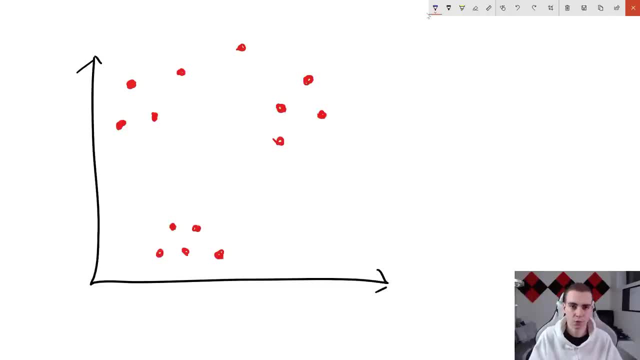 currently exist. So we start by randomly picking k, which is what we've defined. So let me in this instance, say: k equals three k centroids wherever. So maybe we put one, you know, somewhere, like here, And you know what. I might not bother filling these in because they're going to 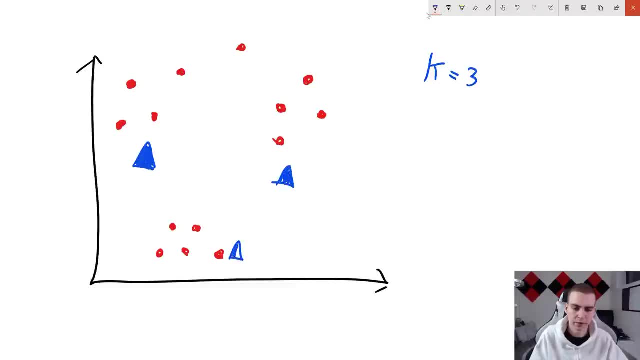 take a while. maybe we pull in here And maybe we end up putting one over here. Now I've kind of put them close to where clusters are, But these are going to be completely random. Now what happens next is each group or each data point is assigned to a cluster by distance. 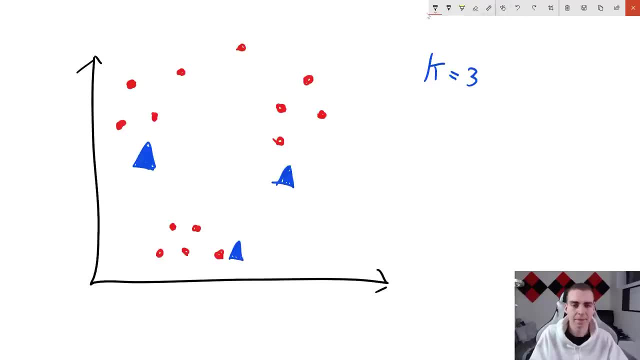 So essentially what we do is, for every single data point that we have, we find what's known as the Euclidean distance, or actually could be a different distance you'd use like Manhattan distance, if you guys know what that is- to all of the centroids. 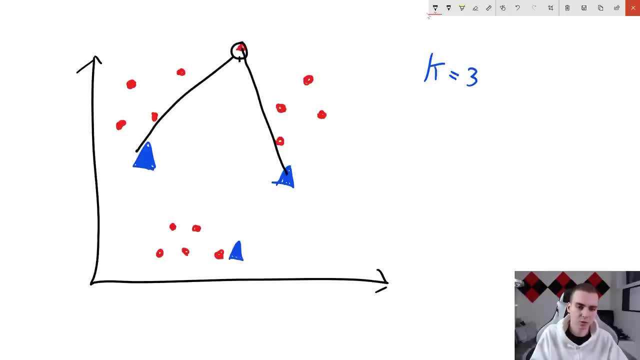 So let's say we're looking at this data point here. what we do is find the distance to all of these different centroids And we assign this data point to the closest central. so the closest one by distance Now in this instance, is looking like it's going to be. 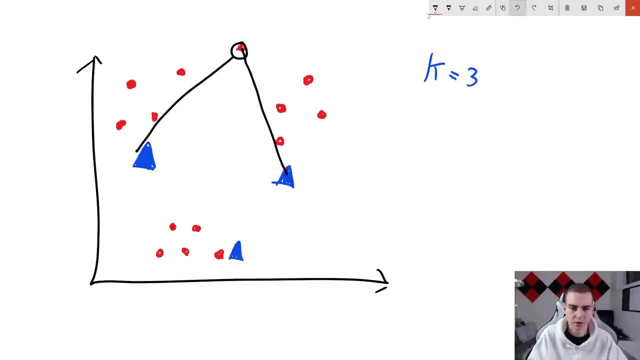 a bit of a tie between this centroid and this centroid, but I'm going to give it to the one on the left. So what we do is we're going to say this is now a part of this centroid. So if I'm calling this like, let's just say this is centroid one, this is centroid two. 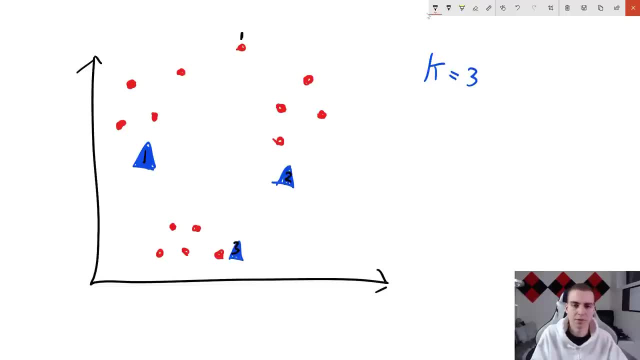 and this is centroid three. then this now is going to be a part of centroid one, because it's closest to centroid one, And we can go through and we do this for every single data point. So obviously we know all of these are going to be our ones, right, And we know. 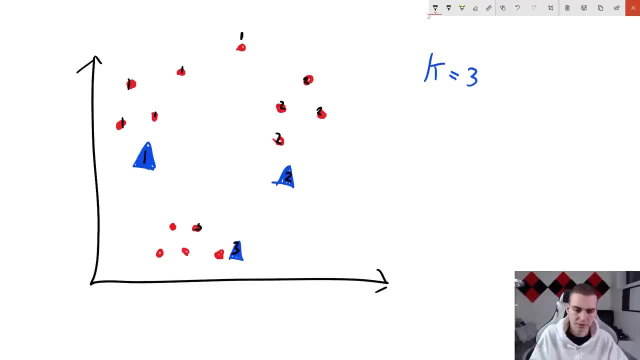 these are going to be our two. so two, two, two, and then these are obviously going to be our three. Now I'm actually just going to add a few other data points, because I want to make this a little bit more sophisticated, almost. 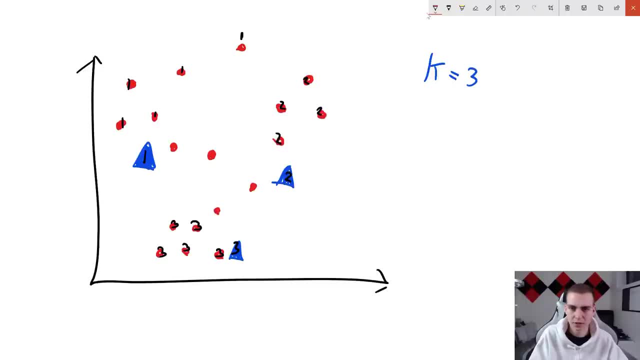 If that makes any sense. So I'll add those data points here. we even add one here and I will give these labels. So these ones are close. So I'm going to say this one's one, I'm going to say this one's two. I know it's not closest to it, But just because I want. 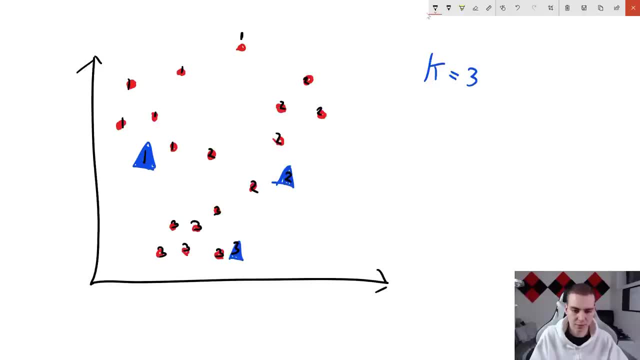 to do that for now. we'll say two for that And we'll say three here. Okay, so now that we've done that, we've labeled all these points, what we do is we now move these centroids that we've defined into the middle of all of their data points. So what I do is I essentially 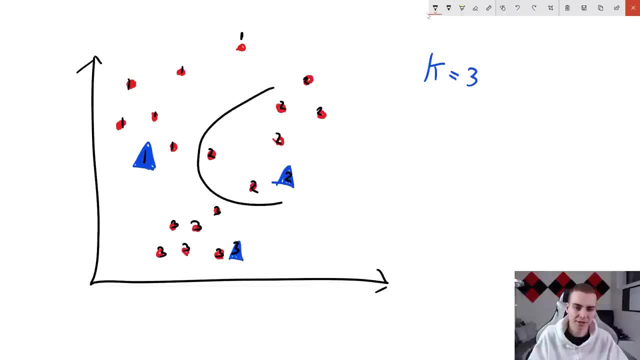 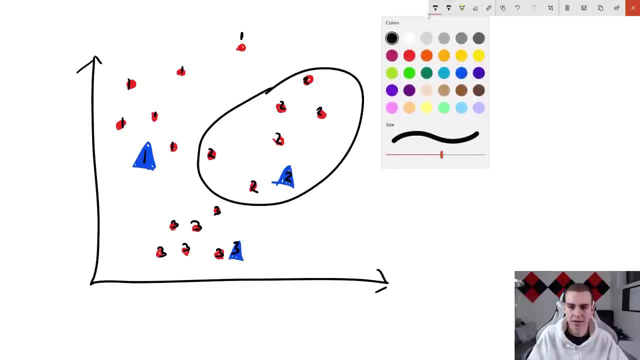 data points that are labeled the same. So in this case, these will be all the ones that are labeled the same, And I take this centroid, which I'm going to have to erase, get rid of it here, And I put it right in the middle. So let's go back to blue And let's say the. 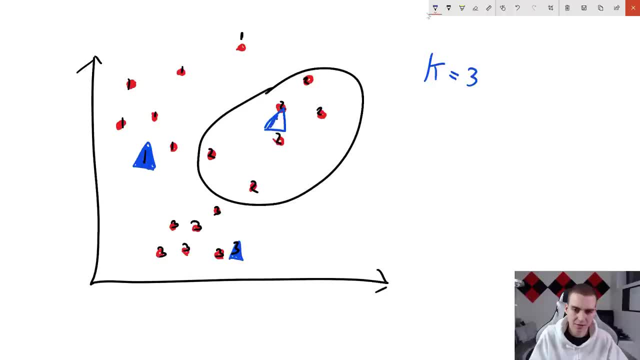 middle of these data points ends up being somewhere around here, So we put it in here And this is what we call center of mass And this again it'd be centroid two. So it's just erase this, And there we go. Now we do the same thing with the other centroid, So 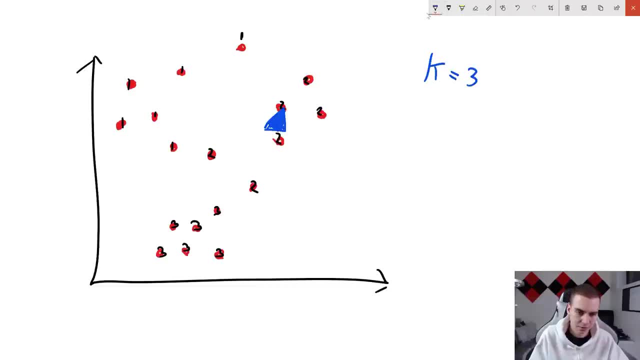 let's remove these ones, let's remove these ones. So for three, I'm saying it's probably going to be somewhere in here, And then for one, our center of mass is probably going to be located somewhere about here. Now, what I do is I repeat the. 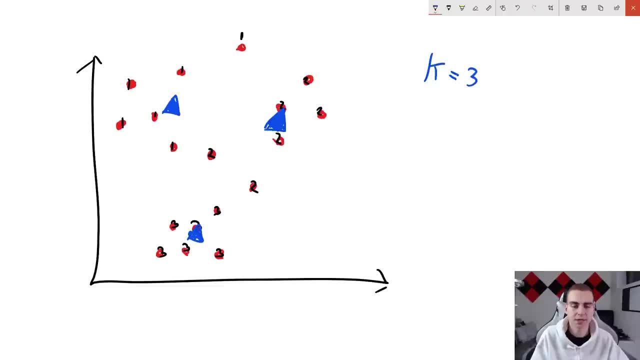 process that I just did And I reassign all the points now to the closest centroid. So all these points are labeled one to all. that you know, we can kind of remove their labels And this is just going to be great me trying to erase the labels I shouldn't have wrote. 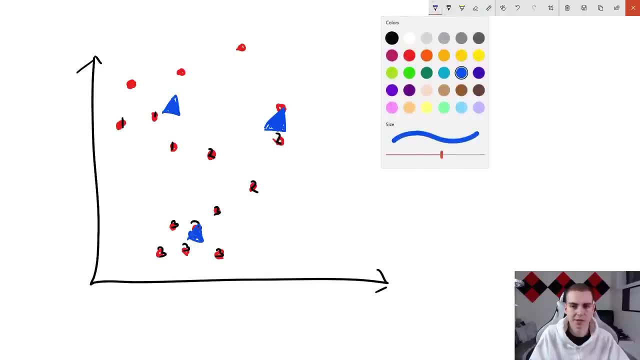 them on top. But essentially what we do is we're just going to be like reassigning them. So I'm going to say, Okay, so this is two. and we just do the same thing as before: find the closest distance. So we'll say, you know, these can stay in the same cluster maybe. 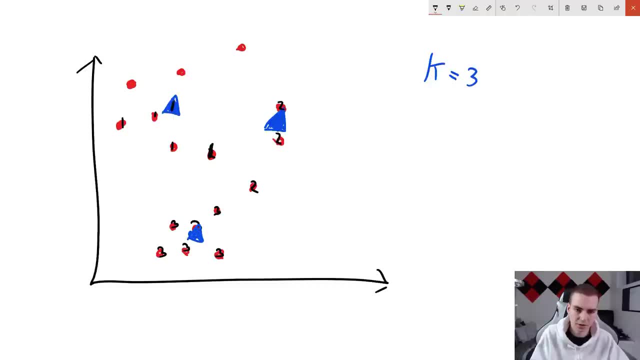 this one actually here gets changed to one now because it's closest to centroid one, And we just reassign all these points, And maybe you know this one now, if it was two before, let's say like this one's one, and we just reassign them Now. we repeat this. 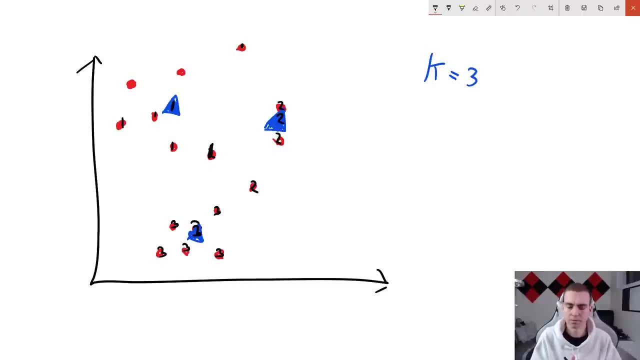 process of finding the closest, or assigning all the points that are closest centroid, moving the centroid into the center of mass, And we keep doing this until eventually we reach a point where none of these points are changing which centroid they're a part of. So eventually we reach a point where I'm 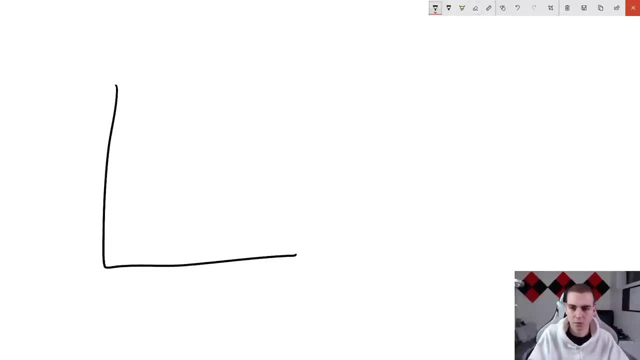 just going to erase this and draw like a new graph, because it'll be a little bit cleaner. But what we have is, you know, like a bunch of data points. So we have some over here, some over here. maybe we'll just put some here And maybe we'll do like a k equals four. 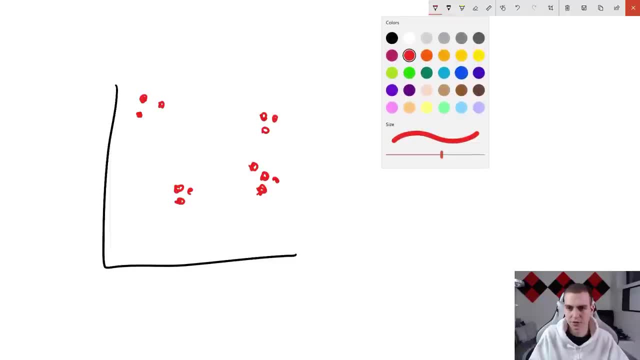 example for this one. And we have all these centroids- And I'll just draw these centroids with blue again- that are directly in the middle of all of their data points. they're like as in the middle, as they can get. none of our data points have moved And we call. 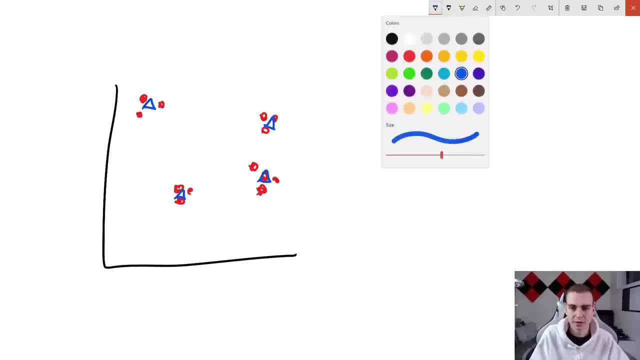 this now our cluster. So now we have these clusters, we have these centroids, right, we know where they are, And what we do is we have a new data point that we want to make a prediction for or figure out what cluster it's a part of what we do is: we will plot. 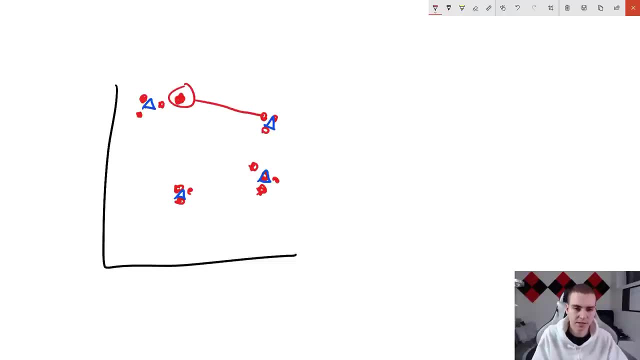 that data point. So let's say it's this new data point. here we find the distance to all of the clusters that exist and then we assign it to the closest one. So obviously it would be assigned to that one, And we can do this for any data point, right? So even if I have 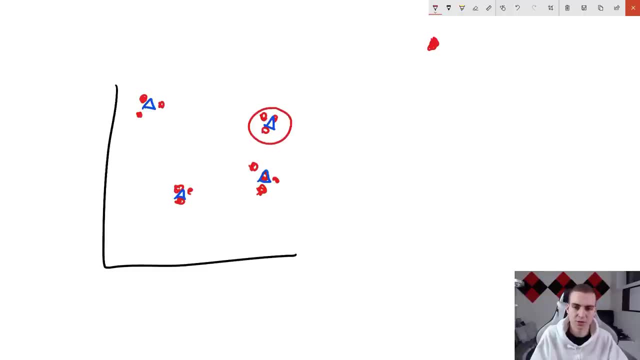 this put a data point all the way over here. well, its closest cluster is this, so it gets assigned to this cluster and my output will be whatever this label of this cluster is, And that's essentially how this works. you're just clustering data points, figuring out. 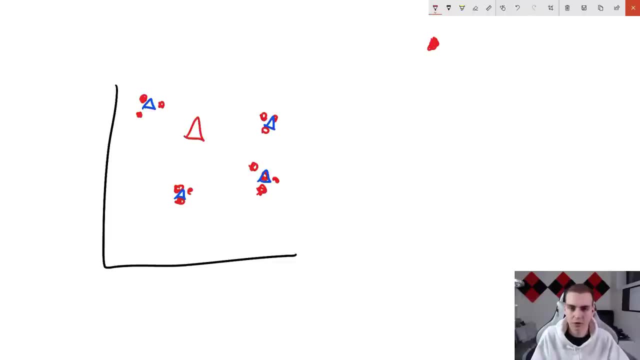 which ones are similar, And there's a pretty basic algorithm. I mean, you draw your little triangle, you find the distance from every point to the triangle, or to all of the triangles actually, And then what you do is just simply assign those values to that centroid you. 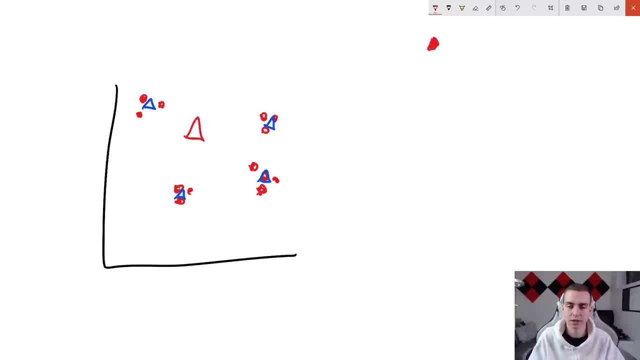 move that centroid to the center of mass and you repeat this process constantly And until eventually you get to a point where none of your data points are moving. that means you've found the best clusters that you can. essentially Now the only thing. 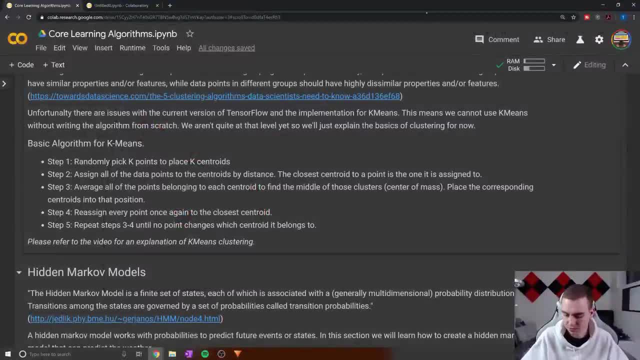 with this is you do need to know how many clusters you want, for cave means clustering, because K is a variable that you need to define, Although there is some algorithms that can actually determine the best amount of clusters for a specific data set. But that's a little. 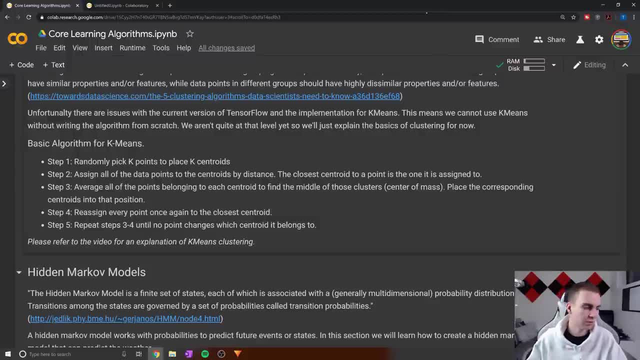 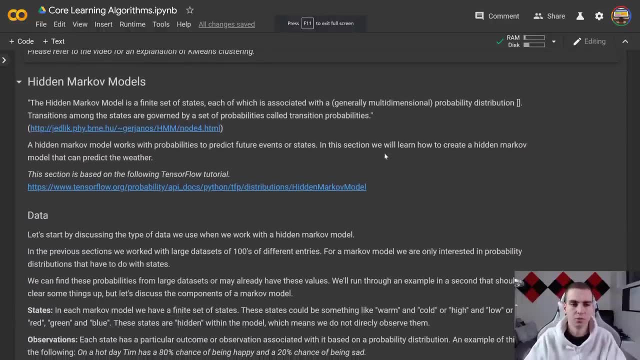 bit beyond what we're going to be focused on focusing on right now. So that is pretty much clustering. There's not really much more to talk about it, especially because we can't really code anything for it now. So we're going to move on to hidden Markov models. Now, hidden Markov models are way different. 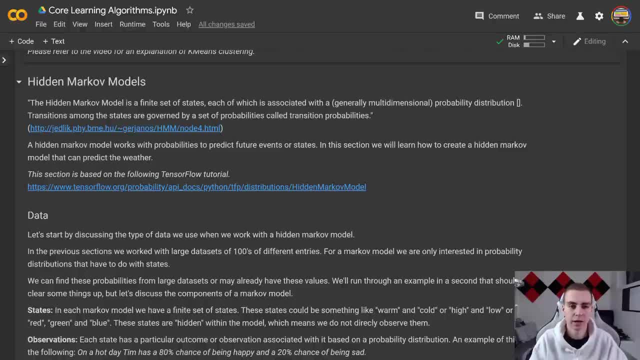 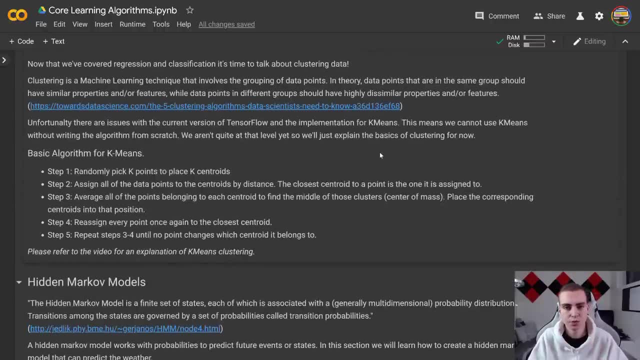 than what we've seen so far. we've been using kind of algorithms that rely on data. So like k means clustering. we gave a lot of data and we know clustered all those data points found those centroids. use those centroids to find where new data points should be Same. 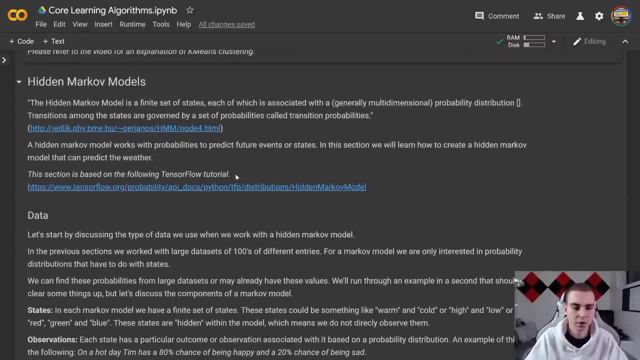 thing with linear regression and classification, Whereas hidden Markov models we actually deal with probability distributions. Now the example we're going to go into here- and it's kind of- I have to do a lot of examples for this because it's a very, very complex- 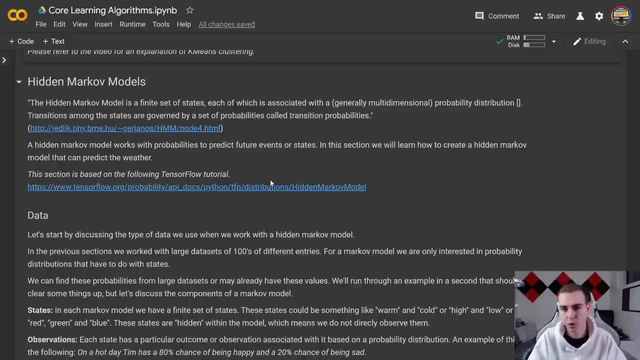 model. But we're going to go into here- and it's kind of- I have to do a lot of examples for this because it's a very abstract concept- is a basic weather model. So what we actually want to do is predict the weather on any given day, given the probability of different events occurring. So let's say: 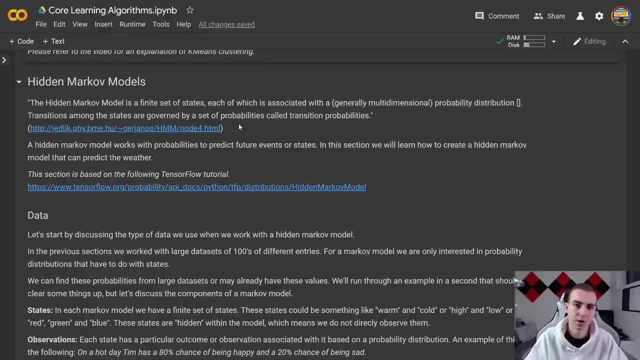 we know- you know, maybe in like a simulated environment or something like that, this might be an application- that we have some specific things about our environment. like we know, if it's sunny, there's an 80% chance that the next day it's going to be sunny again. 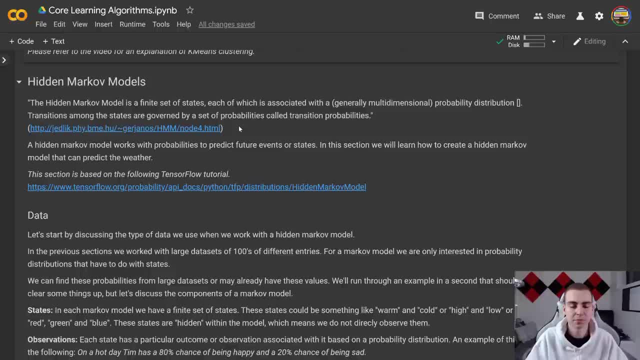 and a 20% chance that it's going to rain. Maybe we know some information about the weather on that day. Maybe we know some information about sunny days and about cold days, And we also know some information about the average temperature on those days. Using this information, 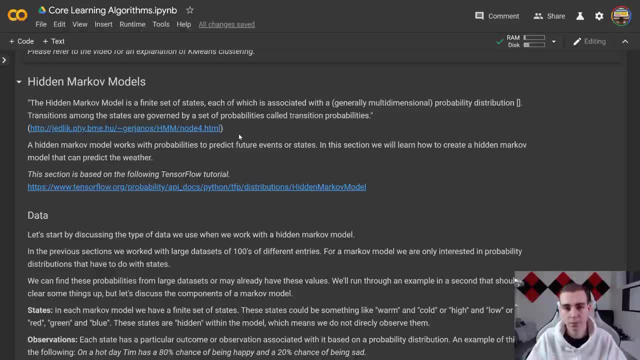 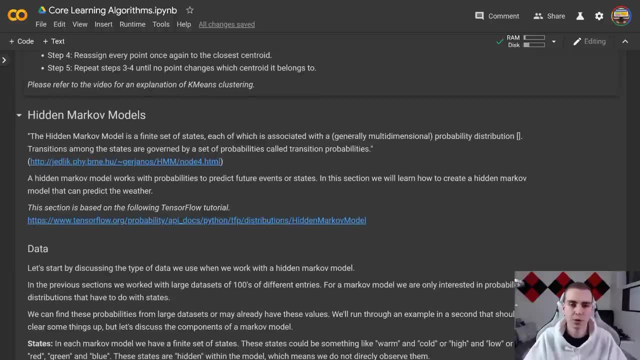 we can create a hidden Markov model that will allow us to make a prediction for the weather in future days, given kind of that probability that we've discovered. Now you might be like: well, how do we know this? Like, how do I know this probability? a lot of the times, 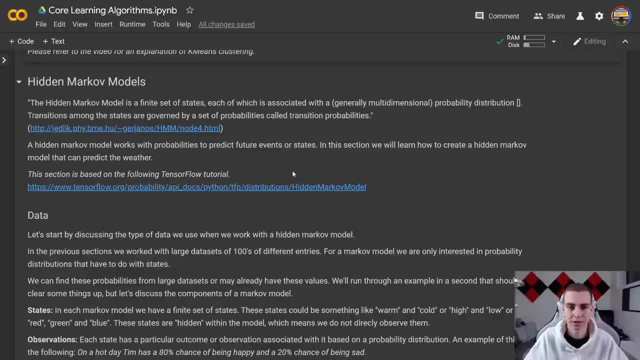 you actually do know the probability of certain events occurring or certain things happening, which makes these models really good. But there's some times where what you actually do is you have a huge data set and you calculate the probability of things occurring based on that data set. So we're not going to do that part, because that's just kind of going. 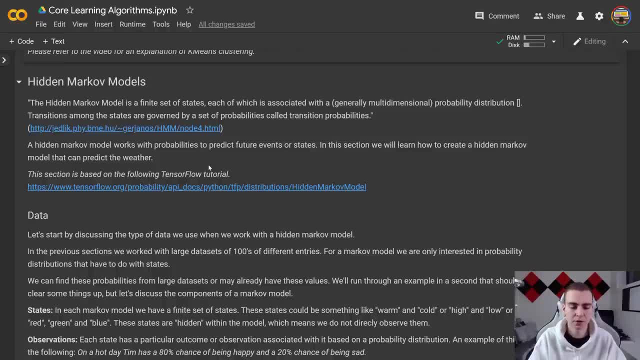 a little bit too far, And the whole point of this is just to introduce you to some different models. But in this example, what we will do is use some predefined probability distributions. So let me just read out the exact definition of a hidden Markov model. we'll start going. 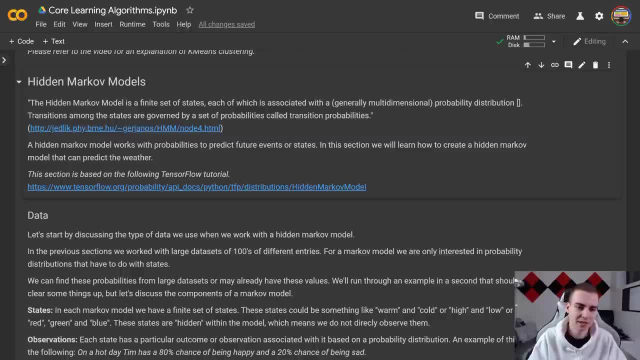 more in depth. So the hidden Markov model is a finite set of states, each of which is associated with a generally multi dimensional probability distribution. transitions among states are governed by a set of probabilities called transition probabilities. So in a hidden Markov model we have a bunch of states. Now in the example that was just talking. 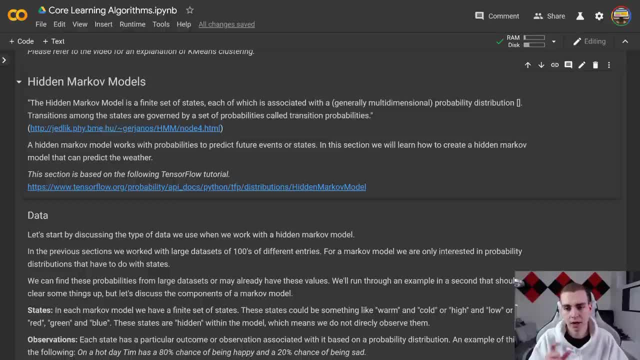 about with this weather model. the states we would have is hot day and cold day. Now, these are what we call hidden, because never do we actually access or look at these states while we interact with the model. In fact, what we look at is something called observations. 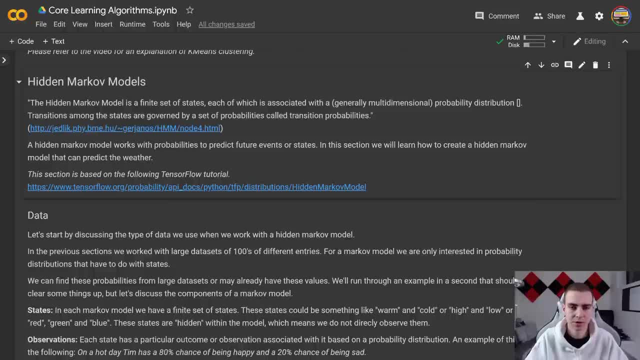 Now, at each state we have an observation. I'll give you an example of an observation. if it is hot outside, Tim has an 80% chance of being happy. If it is cold outside, Tim has a 20% chance of being happy. That is an observation. So at that state we can observe. 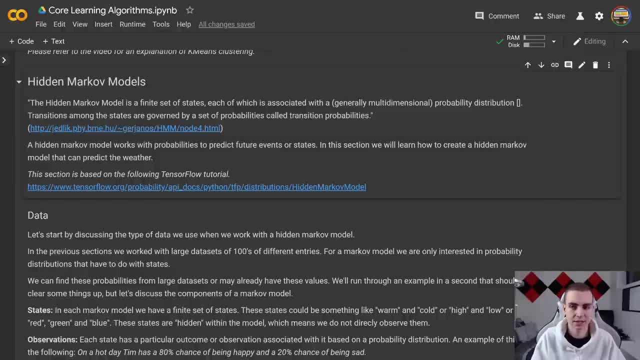 the probability of something happening during that state is x right, or is y or whatever it is. So we don't actually care about the states in particular, we care about the observations we get from that state. Now, in our example, what we're actually going to do is we're going. 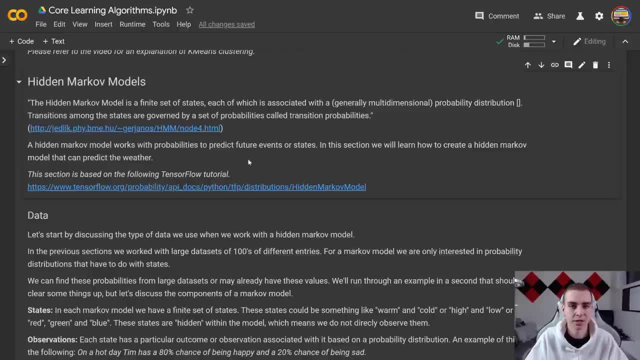 to look at the weather as an observation for the state. For example, on a sunny day, the weather has, you know, the probability of being between five and 15 degrees Celsius, with an average temperature of 11 degrees. That's like that's. 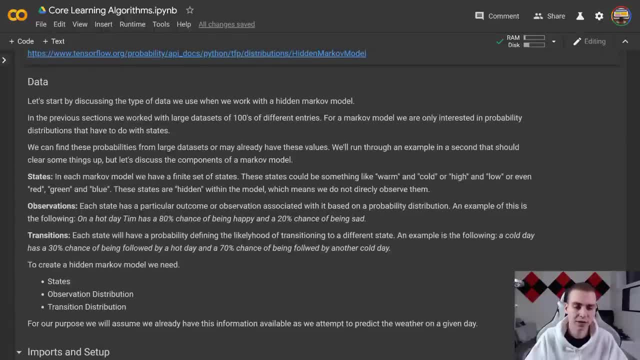 a probability we can use. Now I know this is slightly abstract, but I just want to talk about the data we're going to work with here. I'm going to draw out a little example, go through it and then we'll actually get into the code. So let's start by discussing the 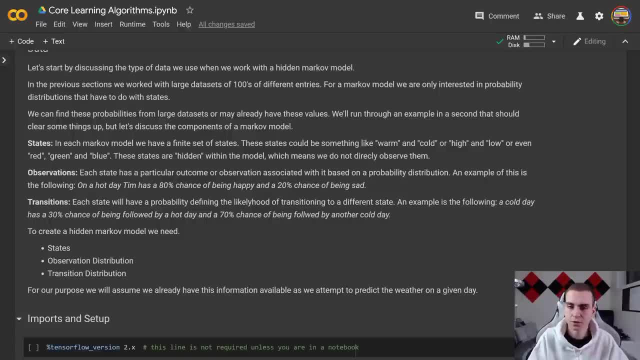 type of data we're going to use So typically in previous ones. right, we use like hundreds, if not like 1000s, of entries or rows or data points for our models to train. For this we don't need any of that, In fact. all we need is just constant values. 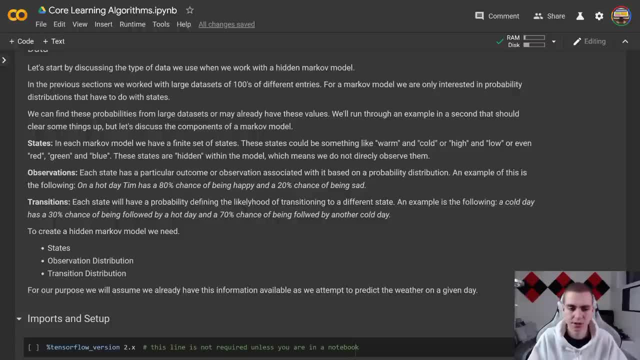 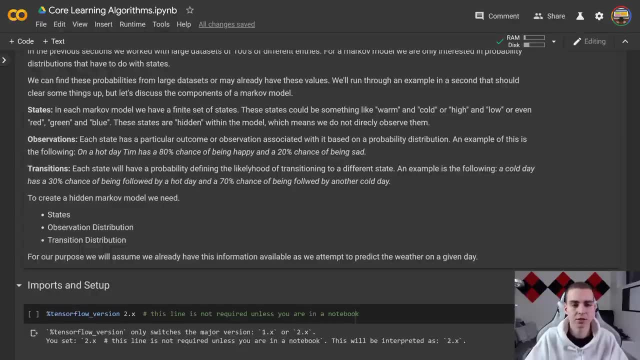 for probability and or what is it? transition distributions and observation distributions. Now, what I'm going to do is go in here and talk about states, observations and transitions. So we have a certain amount of states. Now we will define how many states we have, but 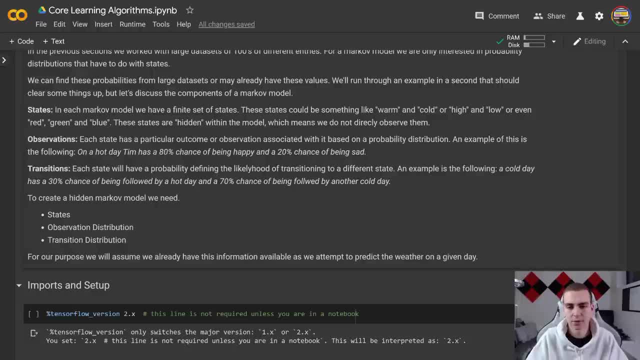 we don't really care what that state is. So we could have states, for example, like warm, cold, high, low, red, green, blue. you have as many states as we want. we could have one state to be able to get rid of, And then we can just go ahead and go ahead and do that. 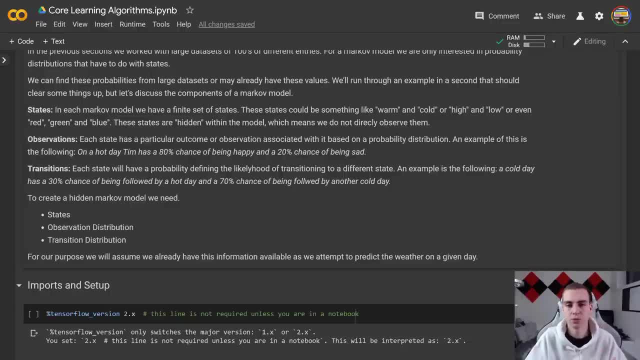 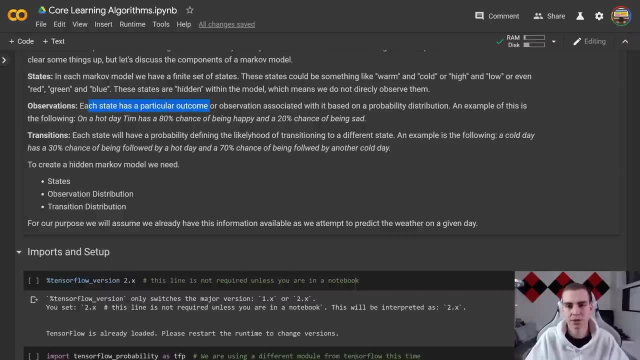 To be honest, although that would be kind of strange to have that- And these are called hidden because we don't directly observe them. Now observations: So each state has a particular outcome or observation associated with it, based on a probability distribution. So it 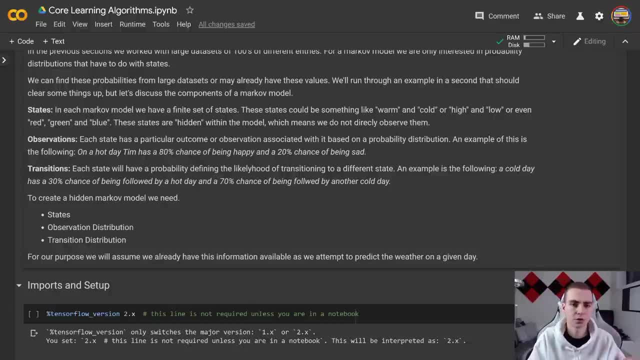 could be the fact that during a hot day, it is 100% true that Tim is happy, Although in a hot day we could observe that 80% of the time Tim is happy And 20% of the time he is sad. right, Those are observations we make about each state and each state will have. 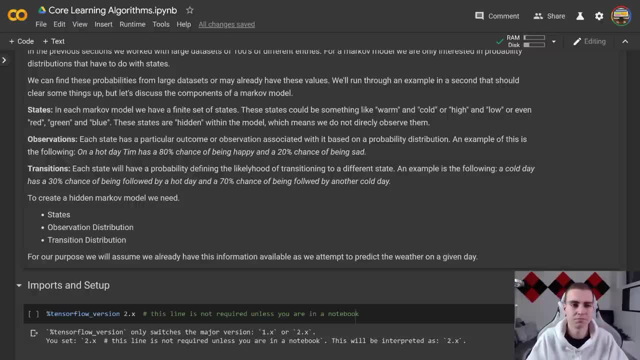 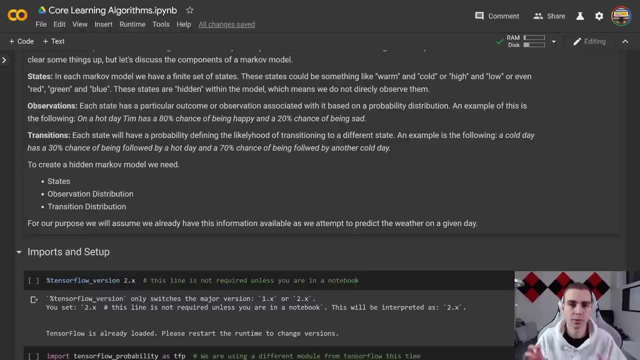 their different observations And different probabilities of those observations occurring. So if we were just gonna have like an outcome, for the state that means it's always the same, there's no probability that something happens, And in that case that's just called an outcome, because the probability 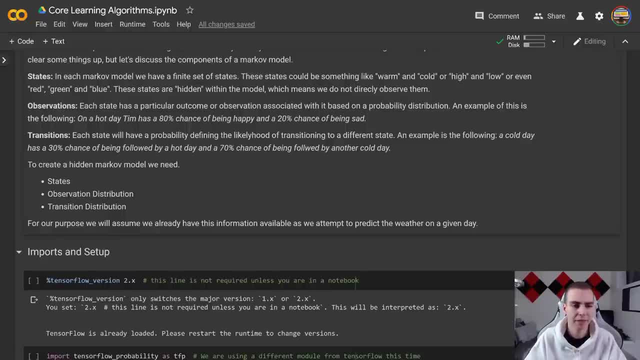 of the event occurring will be 100%. Okay, then we have transitions, So each state will have a probability defining the likelihood of transitioning to a different state. So, for example, if we have a hot day, there will be a percentage chance. the next day will be. 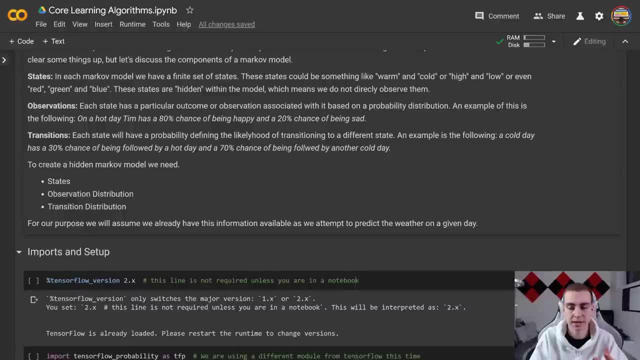 a cold day, we have a cold day. there will be a percentage chance of the next day is either a hot day or a cold day. So we're going to go through like the exact what we have for our specific model below, But, just understand, there's a probability that we could transition into a different state. 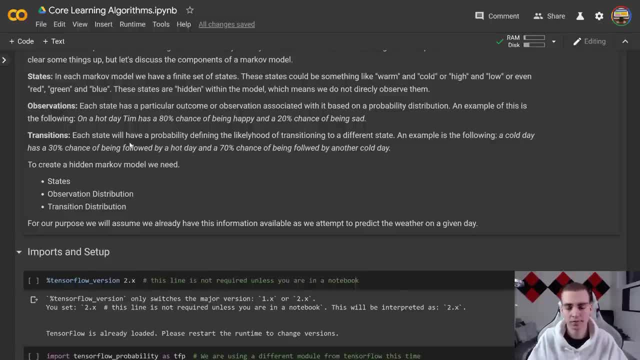 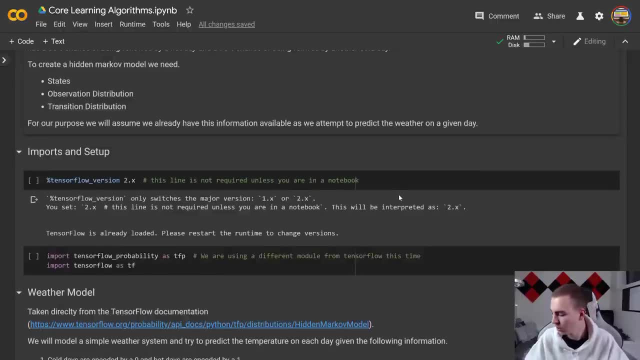 And for each state we can transition into every other state or a defined set of states, given a certain probability. So I know it's a mouthful, I know it's a lot, But let's go into a basic drawing example, Because I just want to illustrate like graphically a little bit kind of how this 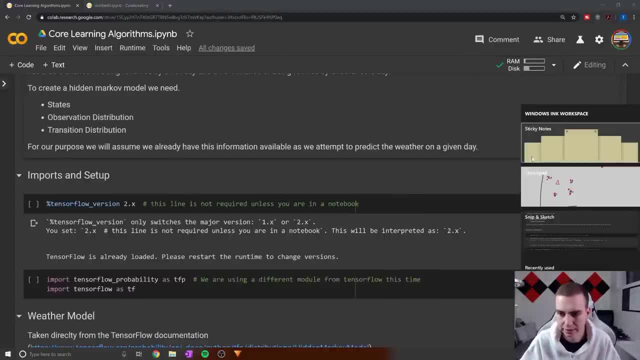 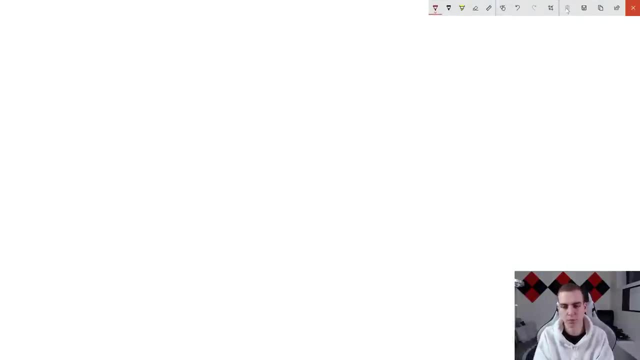 works In case, these are ideas are a little bit too abstract for any of you. Okay, I'm just pulling out the drawing tablet, just one second here, And let's do this basic weather model. So what I'm going to do is just simply draw two states. Actually, let's do it with some colors, because 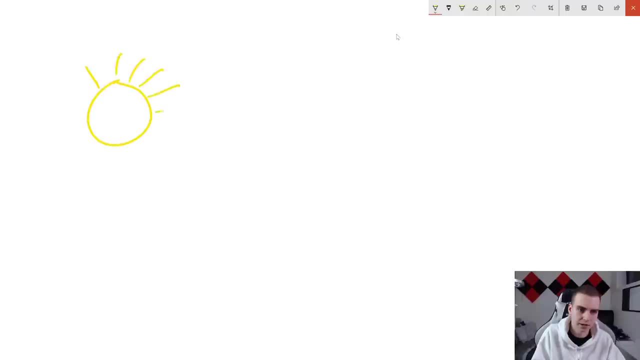 why not? So we're going to use yellow, and this is going to be our hot day. okay, this is going to be our sun, And then I'm just going to make a cloud. we'll just do like a gray cloud. this will. 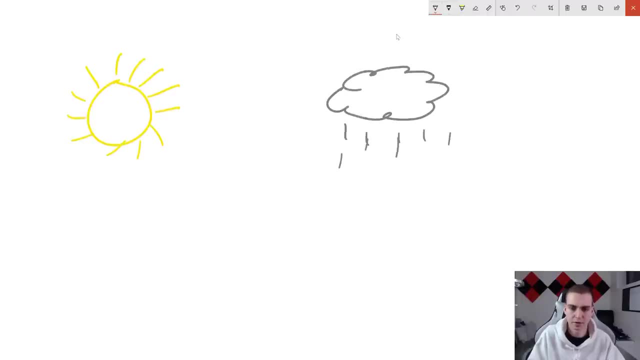 be my cloud And we'll just say it's going to be a raining over here. Okay, so these are my two states. Now, in each state there's a probability of transitioning to the other state. So, for example, in a hot day we have a, let's say, 20%. 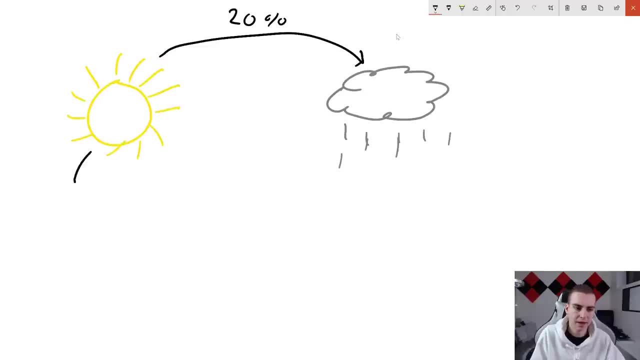 chance of transitioning to a cold day And we have a 80% chance of transitioning to another hot day, like the next day right Now, in a cold day, we have, let's say, a 30% chance of transitioning to a hot day, And we have, in this case- what is that going to be? a 70% chance of transitioning to. 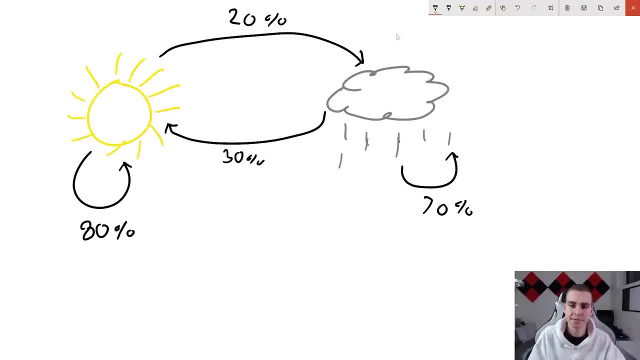 another cold day Now. on each of these days we have a list of observations, So these are what we call states. right, So this could be s1. And this could be s2, it doesn't really matter, like if we. 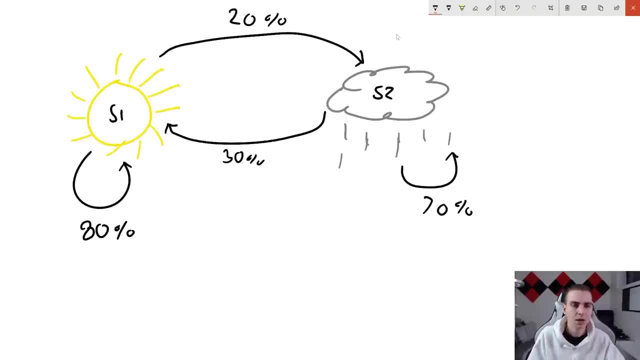 name them or anything. we just we have two states, that's what we know. We know the transition probability, that's what we've just defined. Now we want the observation probability or distribution for that. So essentially, on a hot day, our observation is going to be that the temperature 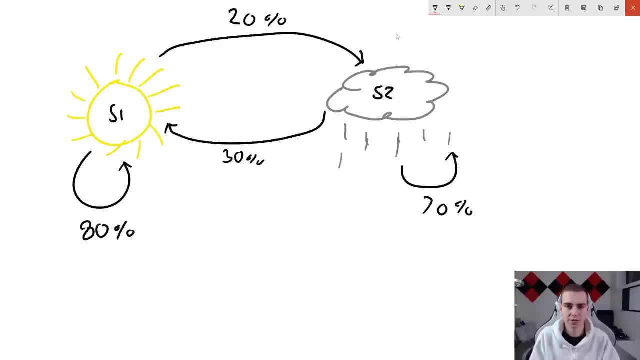 could be between 15 and 25 degrees Celsius, And then we're going to be able to see the temperature, with an average temperature of, let's say, 20.. So we could say: observation, right, so say observation. and we'll say that the mean, so the average temperature is going to be 20.. And then 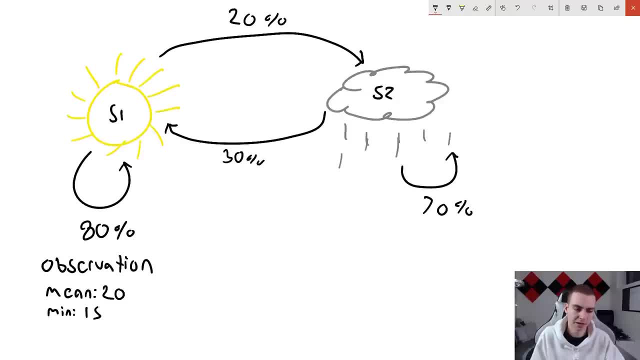 the distribution for that will be like the minimum value is going to be 15. And the max is going to be 25.. So this is what we call actually like a standard deviation. I'm not really going to explain exactly what standard deviation is, although you can kind of think of it as something. 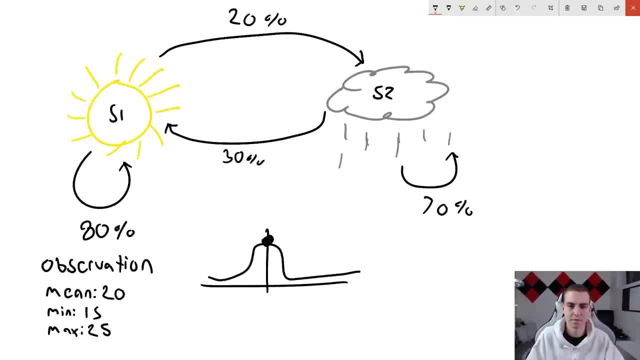 like this. So essentially, there's a mean, which is the middle point, the most common event that could occur, And, at different levels of standard deviation- which is going into statistics which I don't really want to mention that much because I'm definitely not an expert- we have a probability of hitting 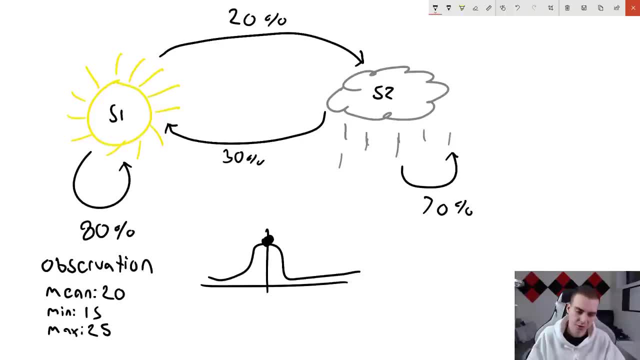 different temperatures as we move to the left and right of this value. So on this curve, somewhere, we have 15.. And on this curve to the right, somewhere, we have 25.. Now we're just defining the fact that this is where we're going to kind of end our curve. So we're 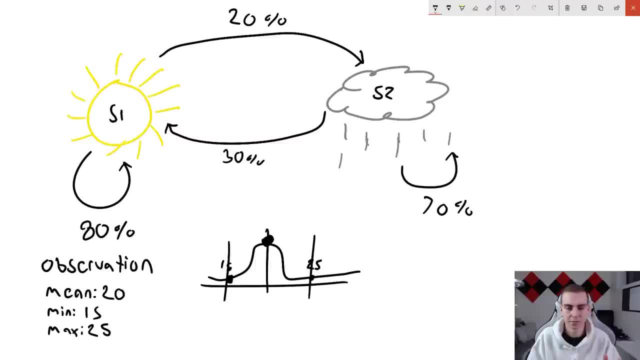 going to say that, like, the probability is in between 15 and 25 degrees Celsius, And between these numbers it's gonna be in between 15 and 25, with an average of 20.. And then our model will kind of figure out some things to do with that. That's as far as I really. 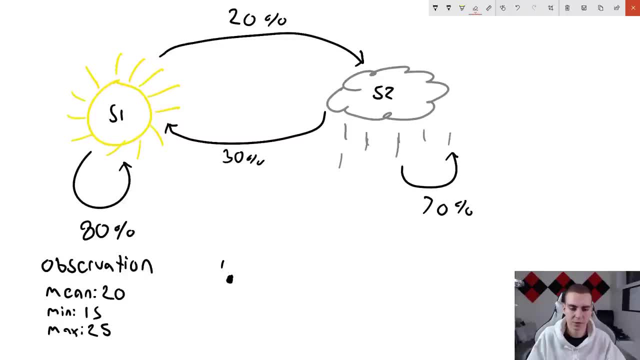 want to go in standard deviation, And I'm sure that's like a really horrible explanation, But that's kind of the best I'm going to give you guys for right now. Okay, so that's our observation here. Now our observation over here is going to be similar, So we're going. 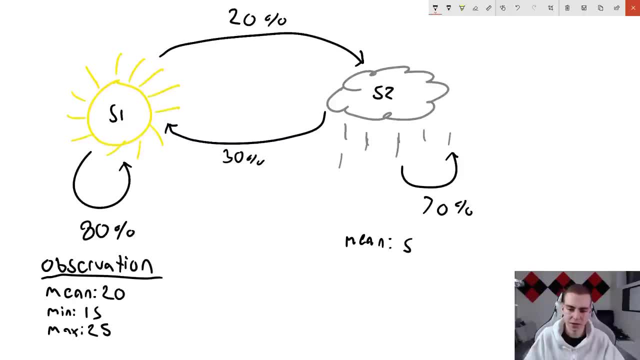 to say: mean, on a cold day temperature is going to be five degrees. we'll say: the minimum temperature maybe is going to be something like negative five and the max could be something like 15.. Or like: yeah, I'm gonna say 15.. So we'll have some distribution. that's just what we. 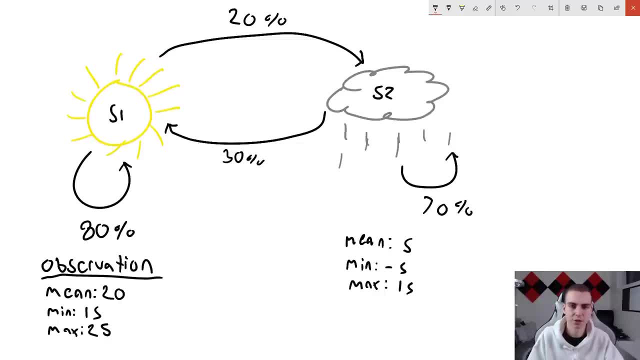 want to understand right. And this is kind of a strange distribution because we're dealing with what is it? standard deviation, although we can just deal with like straight percentage observations. So, for example, you know, there's a 20% chance that Tim is happy, or there's 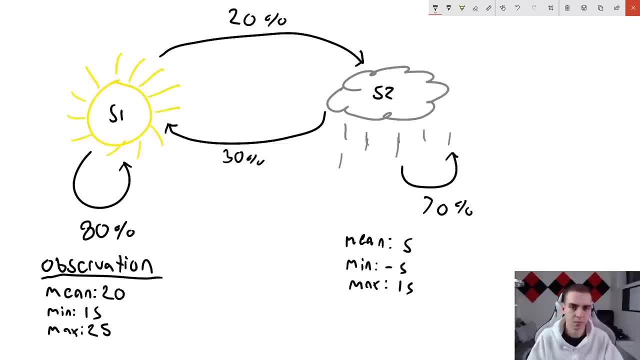 an 80% chance that he is sad like. those are probabilities that we can have as our observation probabilities in the model. Okay, so there's a lot of lingo, there's a lot going on And we're going to get into like a concrete example now. So hopefully this should make more sense. 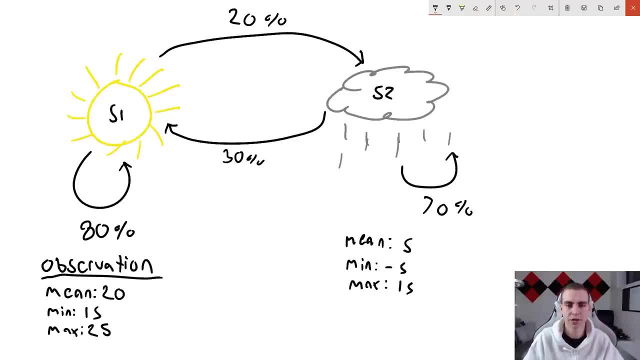 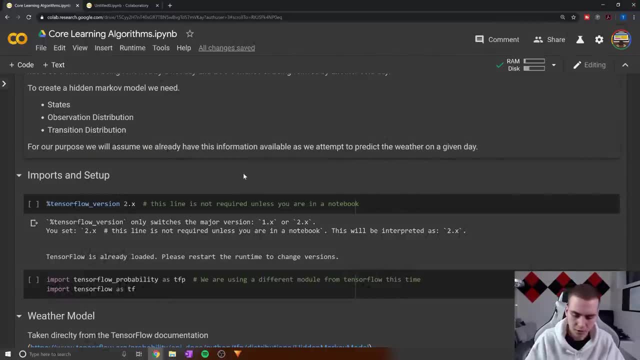 But, again, just understand states, transitions, observations. we don't actually ever look at the states, we just have to know how many we have and the transition probability and observation probability in each of them. Okay, So what I want to say now, though, is what: 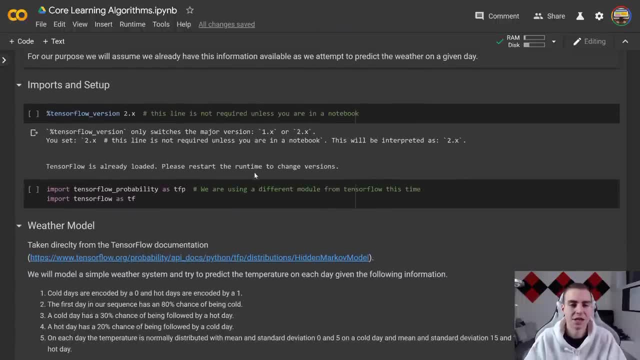 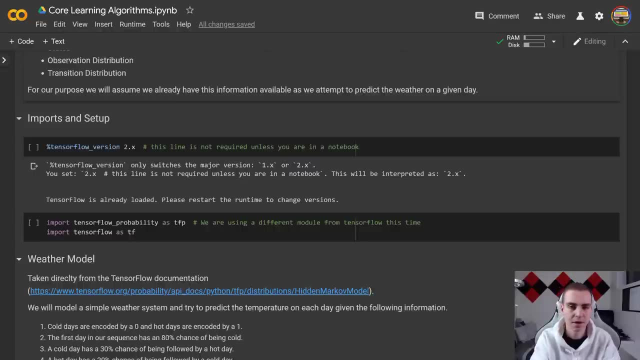 do we even do with this model. So, once I make this right, once I make this hidden Markov model, what's the point of it? Well, the point of it is to predict future events based on past events. So we know that probability distribution And I want to predict the way we're going. 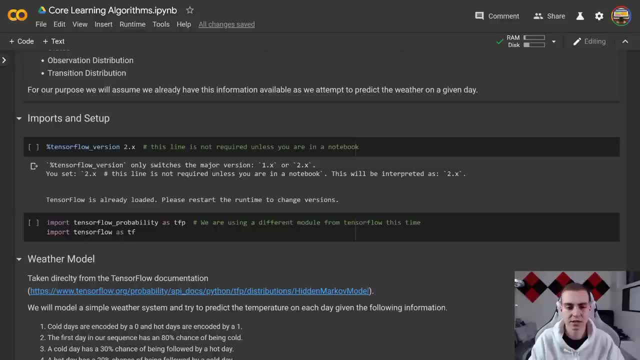 to weather for the next week. well, I can use that model to do that, because I can say: well, if the current day today is warm, then what is the likelihood that the next day, tomorrow, is going to be cold? right, And that's what we're kind of doing with this model. we're 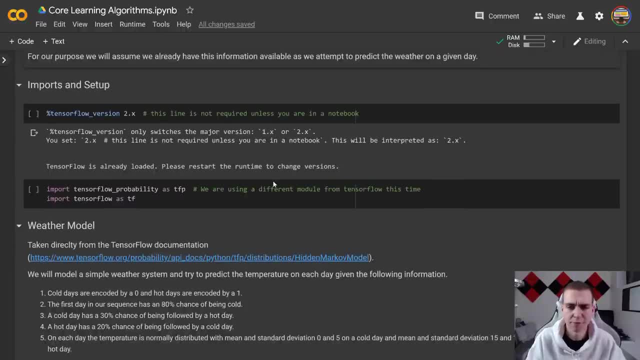 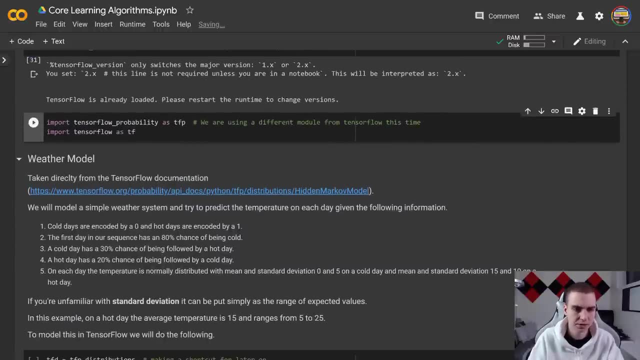 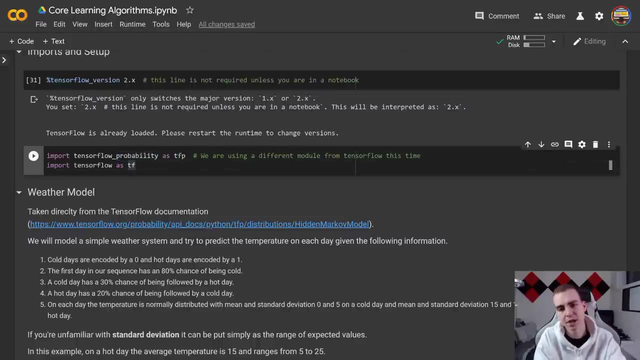 making predictions for the future based on probability of past events occurring. Okay, so imports and setup. So let's just run this already loaded import TensorFlow And notice that here I've imported TensorFlow probability is TF P. This is because this is a separate module from TensorFlow that deals with probability. 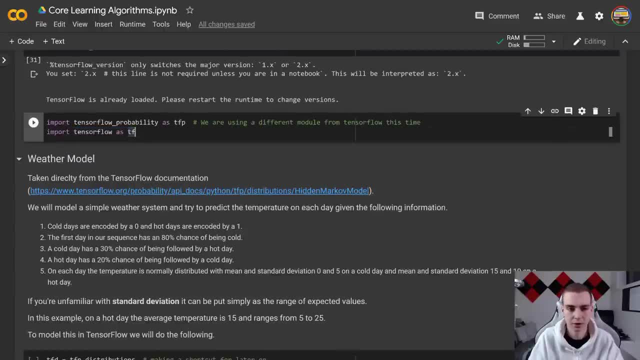 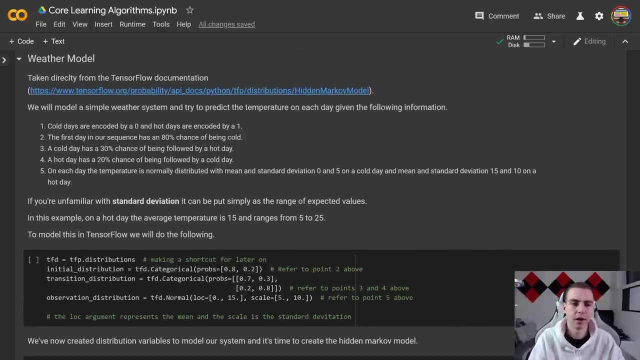 Now we also need TensorFlow to before this hidden Markov model. we're going to use the TensorFlow probability module. not a huge deal, Okay. so weather model. So this is just going to define what our model actually is, So the different parts of it. So this is taken. 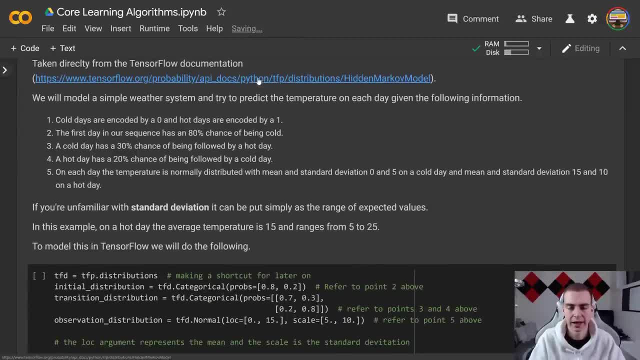 directly from the documentation of TensorFlow. you guys can see. you know where I have all this information from, like I've sourced all of it. But essentially what the model we're going to try to create is that cold days are encoded by zero and hot days are encoded by. 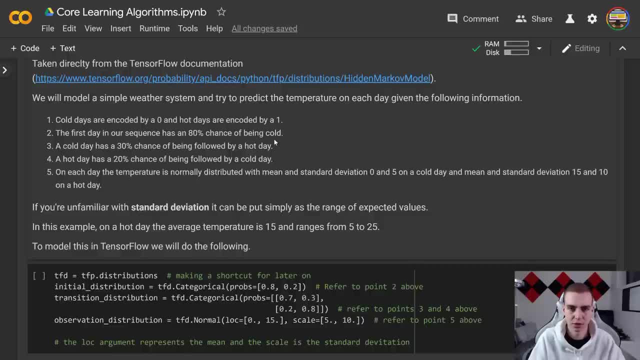 one. the first day in our sequence has an 80% chance of being cold. So whatever day we're starting out at has an 80% chance of being cold, which would mean 20% chance of being one. a cold day has a 30% chance of being followed by hot day, and a hot day is 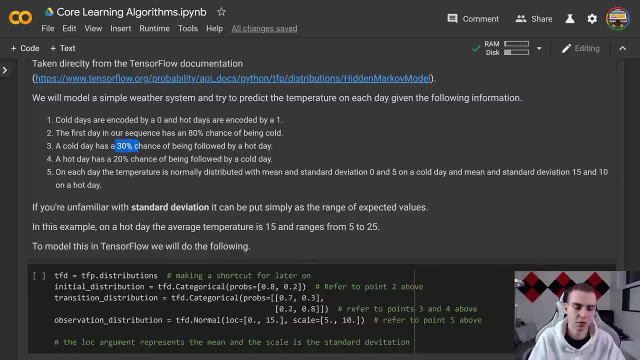 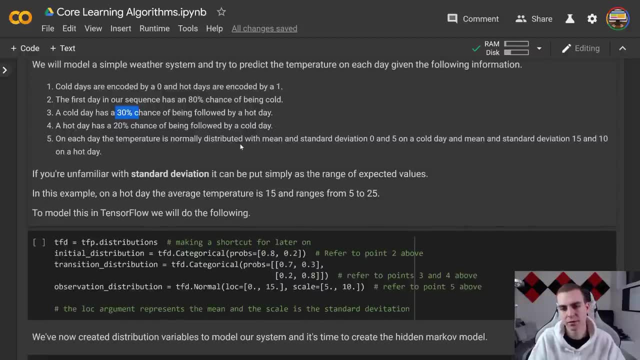 a 20% chance of being followed by a cold day, which would mean, you know, 70% cold to cold and 80% hot to hot On each day. the temperature is normally distributed with mean and standard deviation zero and five on a cold day and mean and standard deviation 15 and 10 on a. 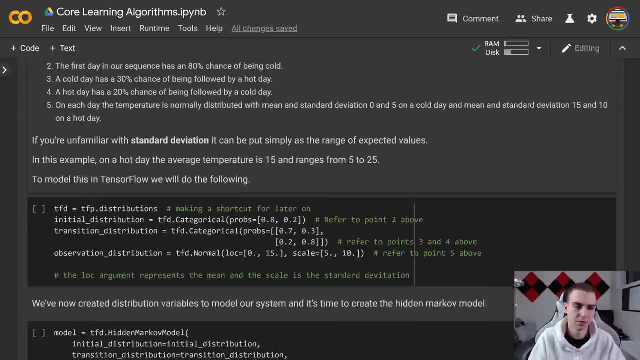 hot day. Now, what that means, standard deviation is essentially- I mean we can read this thing here- is that on a hot day, the average temperature is 15.. That's mean and ranges from five to 25.. Because the standard deviation is 10 of that which 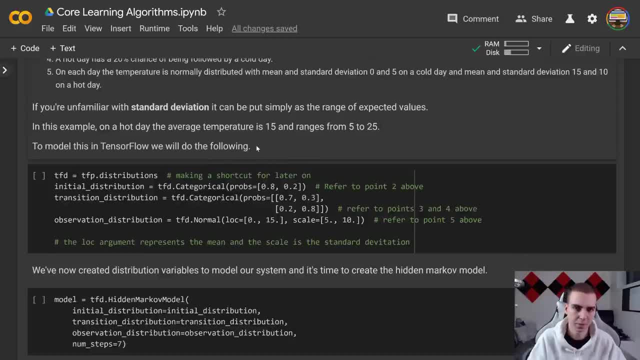 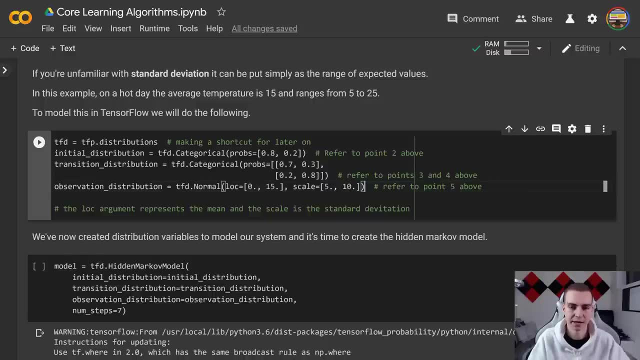 just means 10 on each side, kind of the min max value. Again, I'm not in statistics, So please don't quote me on any definitions of standard deviation. I just trying to explain it enough so that you guys can understand what we're doing here. Okay, so what we're. 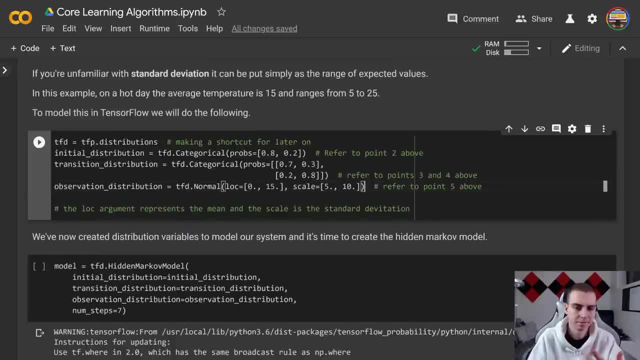 going to do to model this and I'm just kind of going through this fairly quickly because it's pretty easy to really do. this is I'm going to load the tensorflow probability distributions kind of module and just save that as TFD And I'm just going to do that So I don't need to write TFP, dot distributions, dot all. 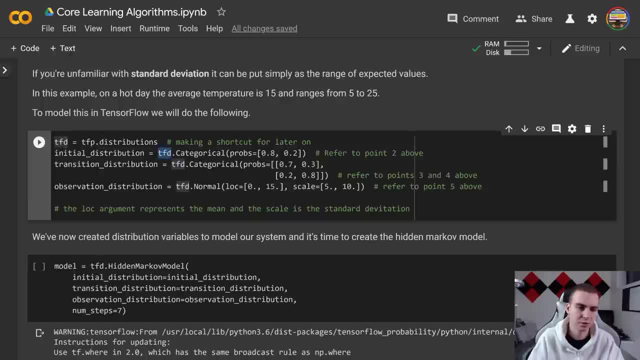 of this. I can just kind of shortcut it So you'll notice I'm referencing TFD here, which just stands for TFP, dot distributions, and TFP is TensorFlow probability. Okay, so my initial distribution is TensorFlow probability distributions, dot categorical. This is probability. 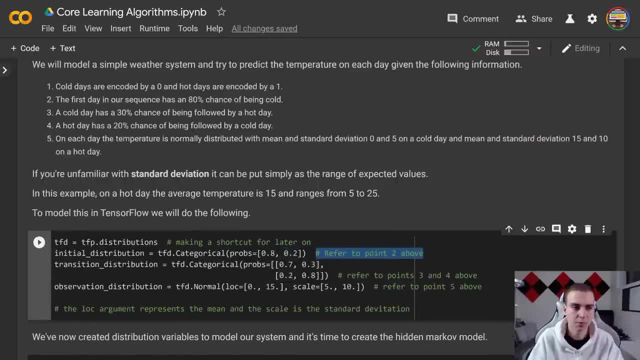 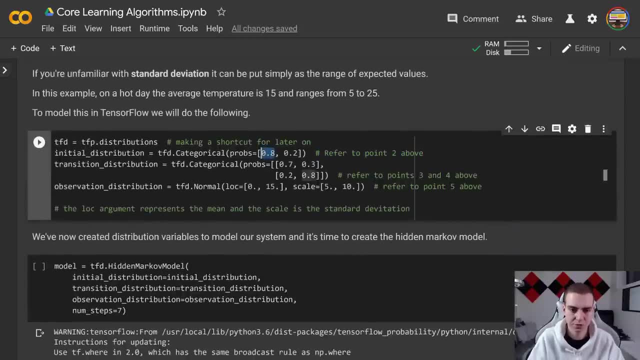 of 80% and 20%. Now this refers to point two. So we got point two. the first day in our sequence has an 80% chance of being cold. So we're saying that that's essentially what this is: the initial distribution of being. 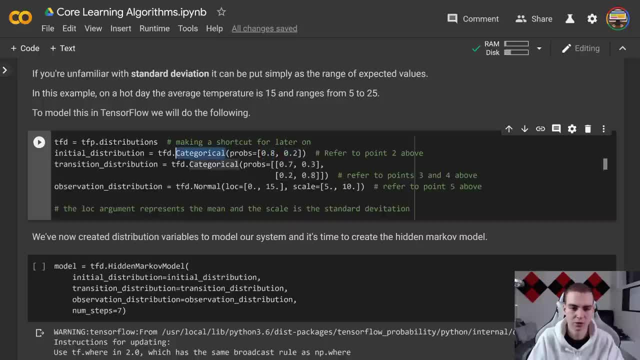 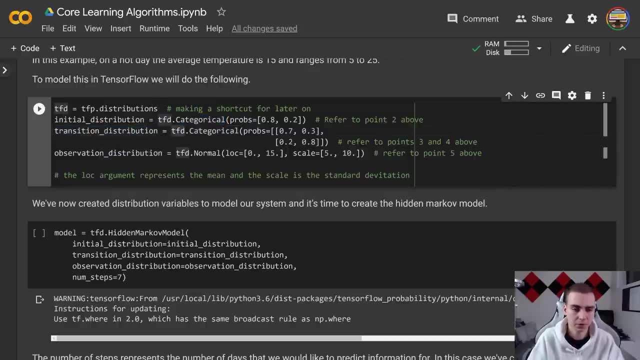 cold is 80% And then 20% after. categorical is just a way that we can do this distribution. Okay, so transition distribution was a TensorFlow probability. categorical, the probability is 70% and 30% and 20%- 80%. Now notice that since we have two states, we've defined two. 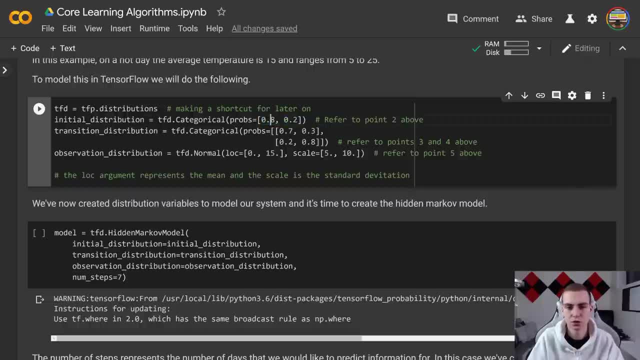 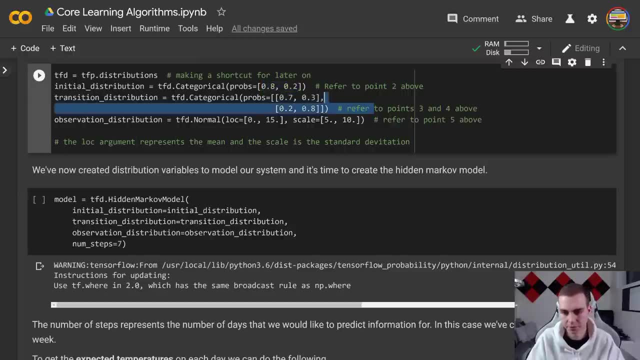 probabilities. Notice: since we have two states, we have defined two probabilities: the probability of landing on each of these states at the very beginning of our sequence. This is the transition probability referred to points three and four above. So this is what we have. 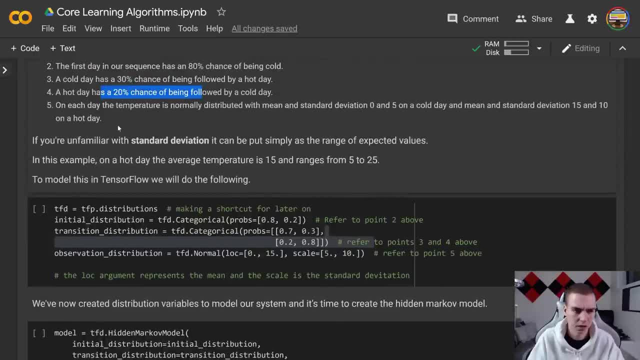 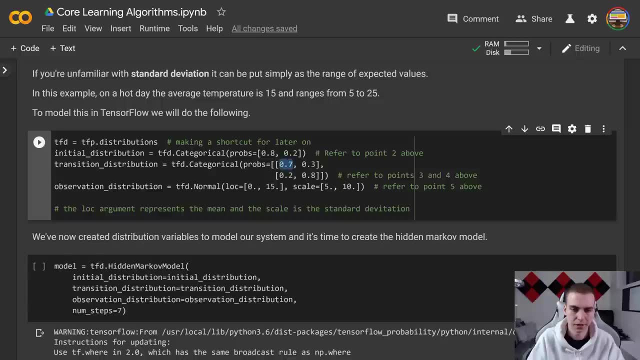 here. So cold is 30% chance, 20% chance for a hot day, And that's what we've defined. So we say: this is going to be cold day, state one. we have 70% chance of being cold day. again we have 30% chance of going hot day, and then you know reverse here. Okay so, 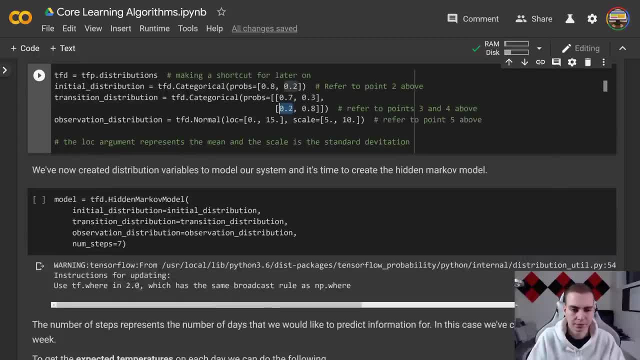 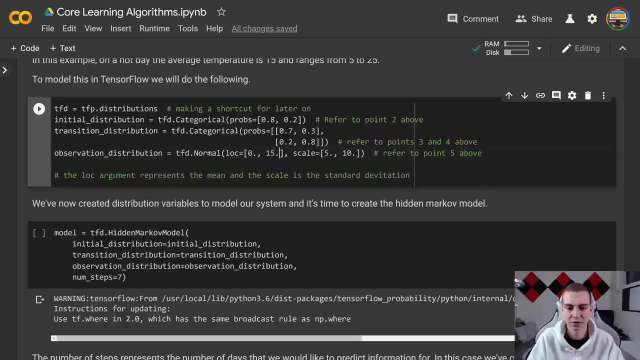 observation distribution. Now this one is a little bit different, But essentially we do tf, D, dot, normal. Now I don't know it's. I'm not gonna explain exactly what all this is, But when you're doing standard deviation, you're gonna do it like this: we're gonna say loke, which stands for your average. 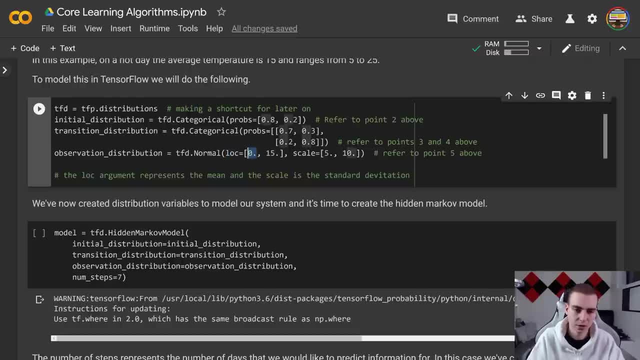 or your mean right. So that was their average. temperature is going to be zero. on a hot day, 15. on a cold day, the standard deviation on the cold days: five, which means we range from five or negative five to five degrees, And on a hot day it's 10.. So that is going to 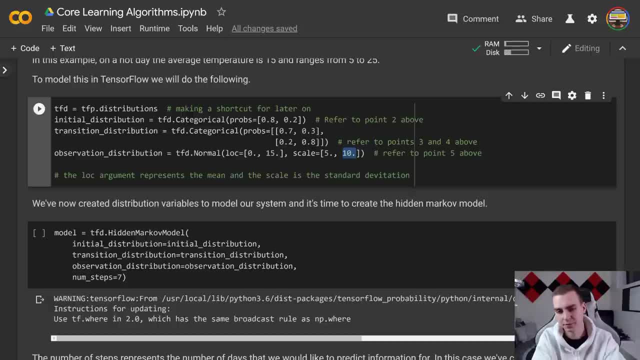 be. we go range from five to five degrees, We range from three to five degrees, And so five to 25 degrees, and our average temperature is 15.. Now the reason we've added dot here is because these just need to be float values. So rather than inserting integers here and having 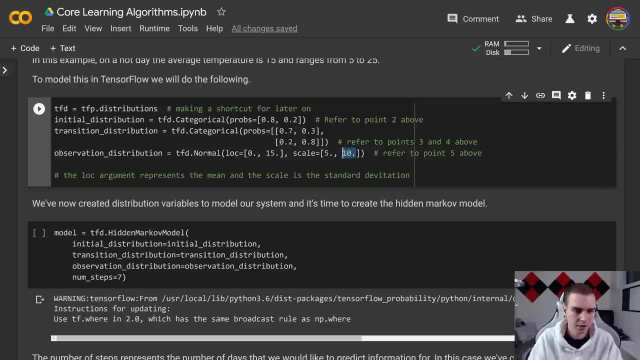 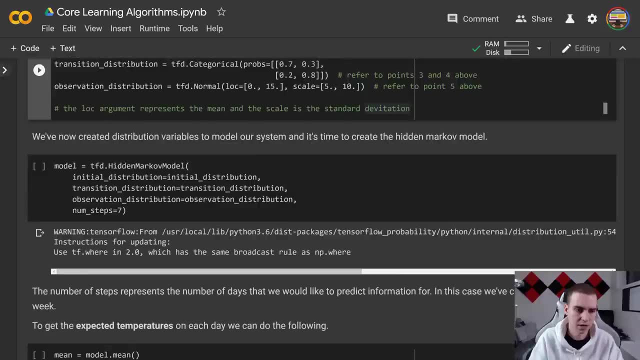 potentially type errors later on. we just have floats. Okay, so the local argument represents the mean and the scale is a standard deviation. Yeah, exactly what we just defined there. Alright, so let's run this. I think we actually already did, And now we can create our model. So 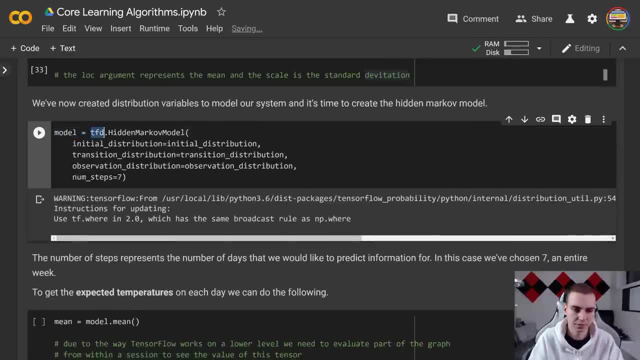 to create the models pretty easy. I mean, all we do is say: model equals TensorFlow distribution. dot hidden Markov model. give it the initial distribution, which is equal to initial distribution, transition distribution, observation distribution and steps. Now what is steps? Well, 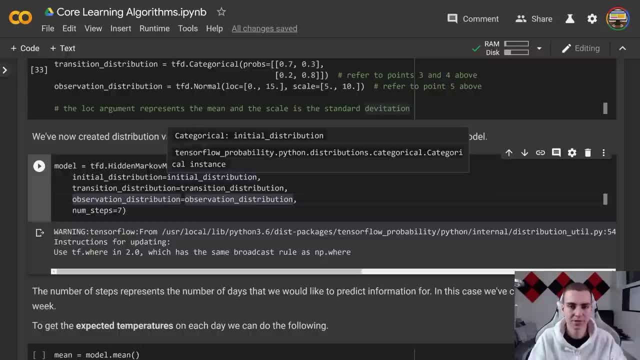 steps is how many days we want to predict for. So the number of steps is how many times we're going to step through this probability cycle and run the model. essentially, Now, remember, what we want to do is we want to predict the average temperature on each day. right, Like that's what the goal of 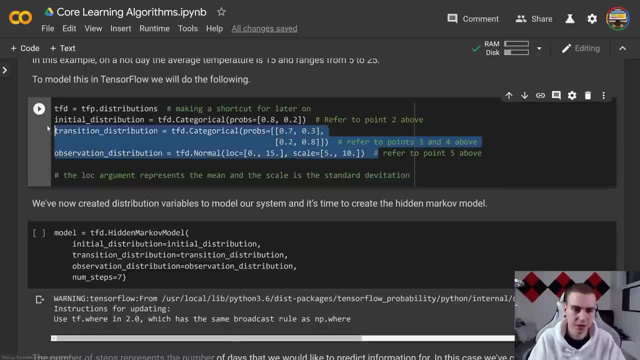 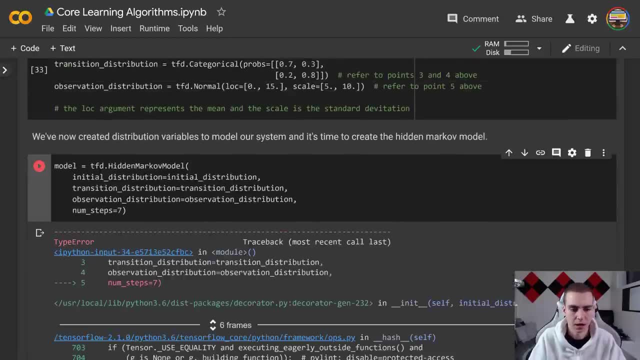 our example is is to predict the average temperature. So, given this information, using these observations and using these transitions, what we'll do is predict that. So I'm going to run this model. What is the issue here? tensor is unhashable of tensor is. okay, give me one sec. 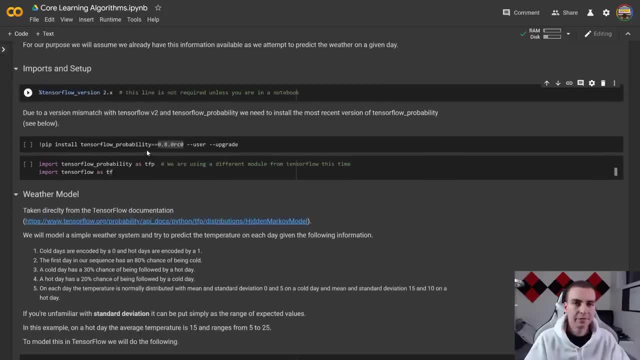 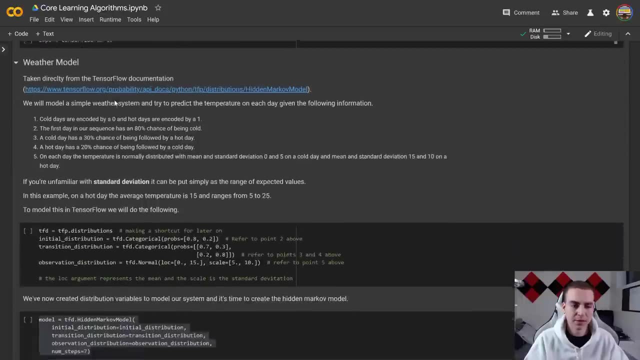 look here, though I haven't had this issue before. Okay, so after a painful amount of searching on Stack Overflow and Google, and actually just reading through more documentation on TensorFlow, I have determined the issue. So remember the error was we were getting on. 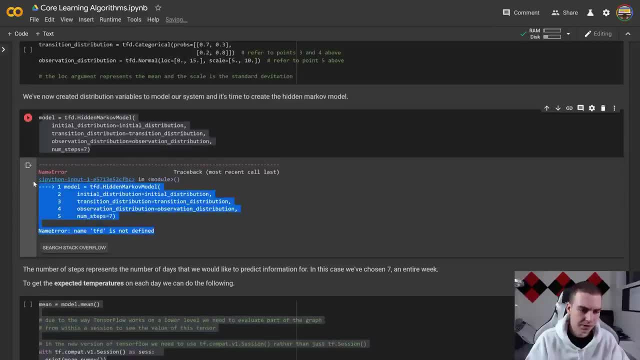 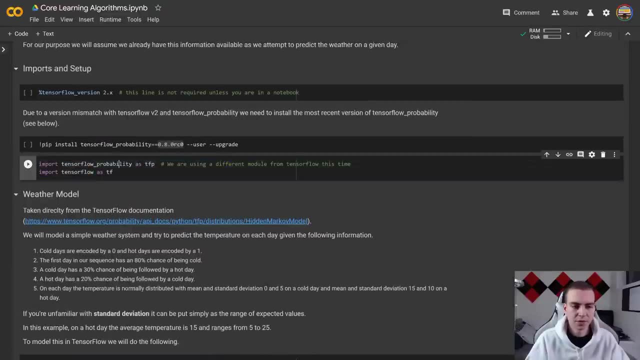 actually this line. here I think I can see what the output is. Oh, this, Okay. well, this is a different error, But anyways, there was an error at this line. essentially, what was happening is we have a mismatch between the two versions here, So the most recent version of TensorFlow is not compatible. 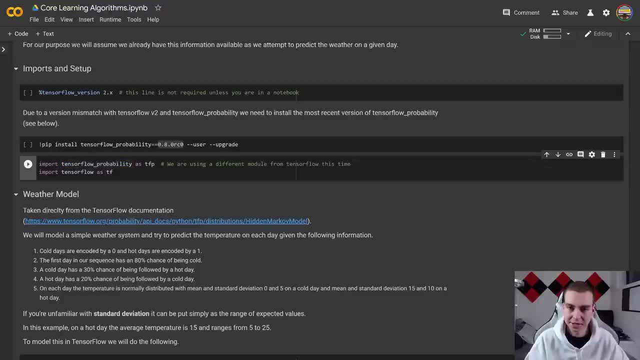 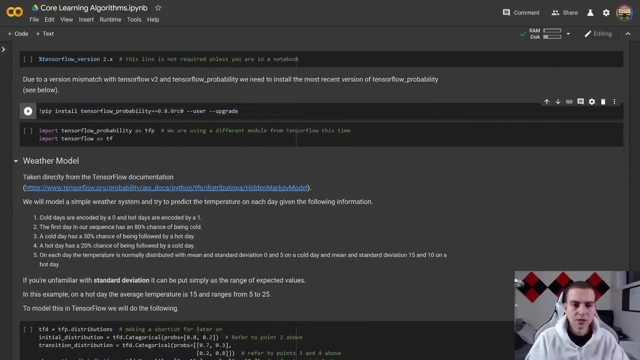 with the older version of TensorFlow probability, at least in the sense that the things that we're trying to do with it. So I just need to make sure that I installed the most recent version of TensorFlow probability. So what you need to do if this is in your notebook and this should actually 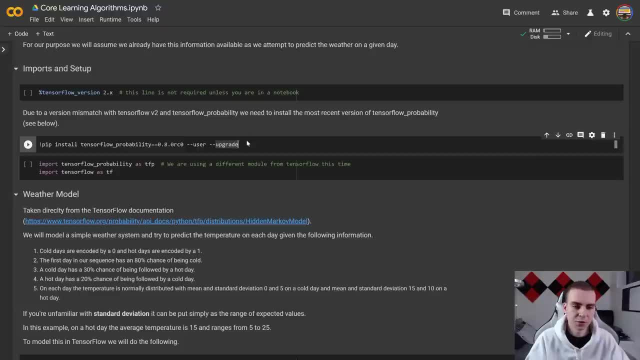 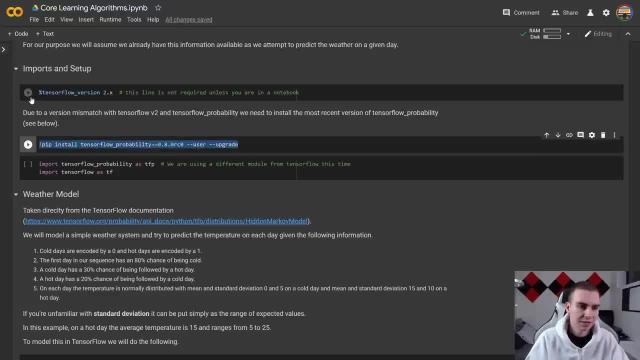 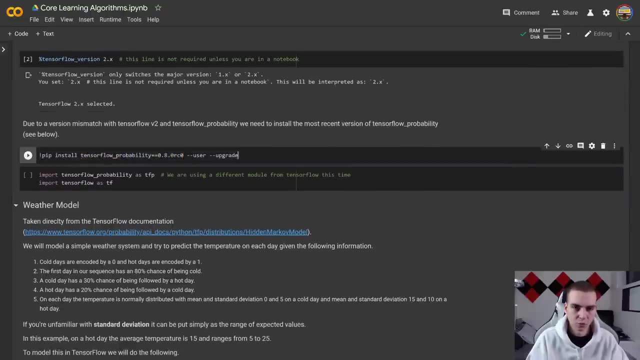 the issue. I'll, you know, deal with it. But essentially we're going to do select version two, point x of TensorFlow. you're going to run this install commands. you're going to install TensorFlow probability, just run this command. then, after you run this command, you're going to 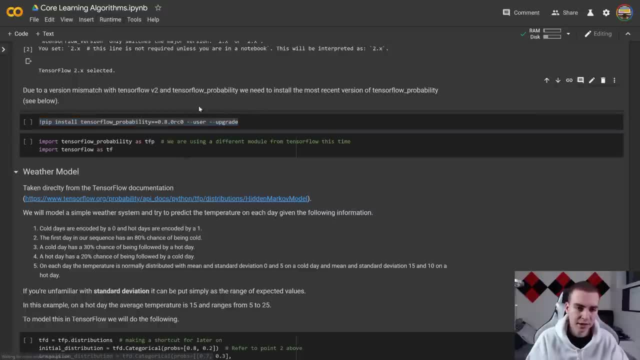 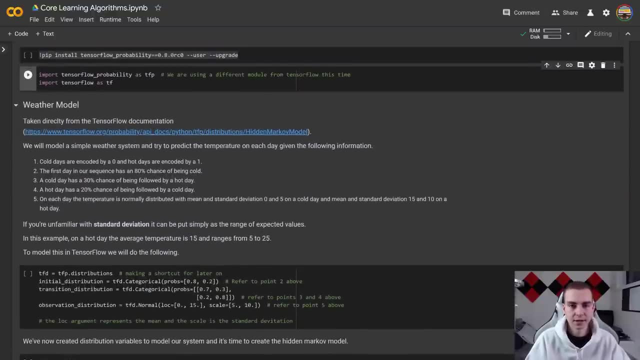 need to restart your runtime. So go to runtime and then restart runtime And then you can just continue on with the script. select TensorFlow 2.x. Again, do your imports And then you know we'll test if it's actually going to work for us here. run our distributions. create the model. 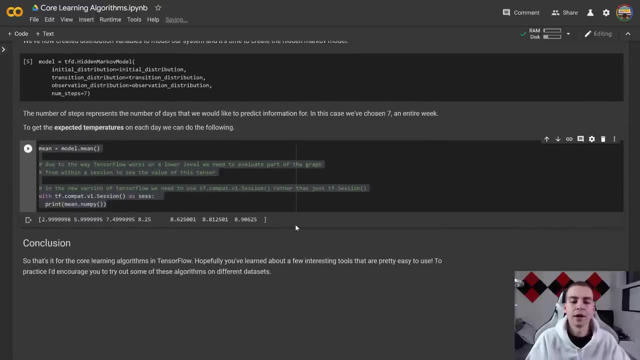 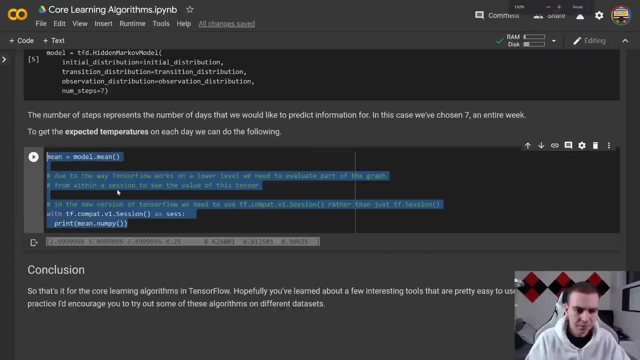 without any issues. this time, notice no red text and then run this final line, which will give you the output. Now, this is what I wanted to talk about here, that we didn't quite get to because we were having some bugs, But this is how we can actually kind of run our model and see the output. So what you can do, 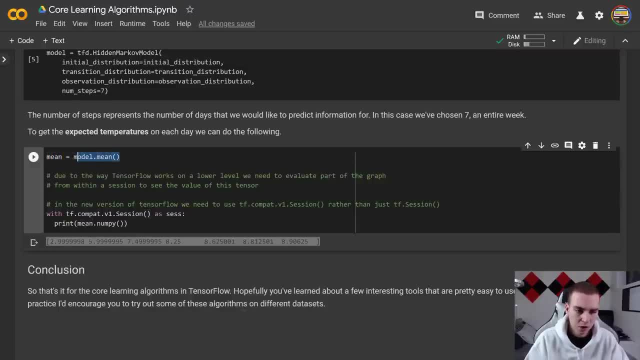 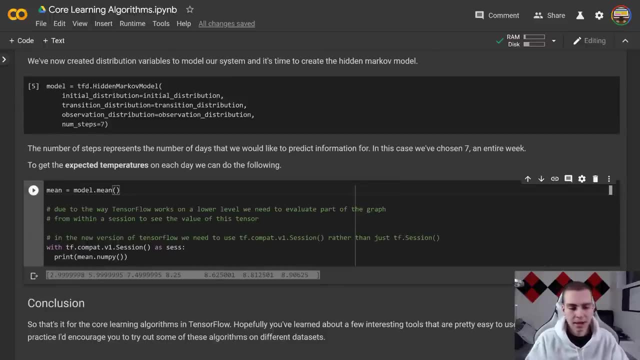 is: do model dot mean? so you say, mean equals? model dot mean, And what this is going to do is essentially just calculate the probability, is going to essentially take that from the model. Now, when we have model dot mean, this is what we call, you know, a partially defined 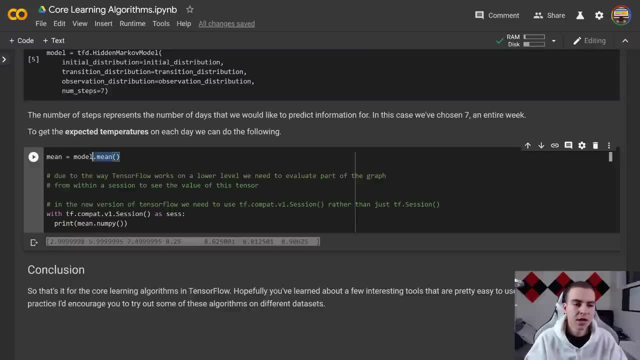 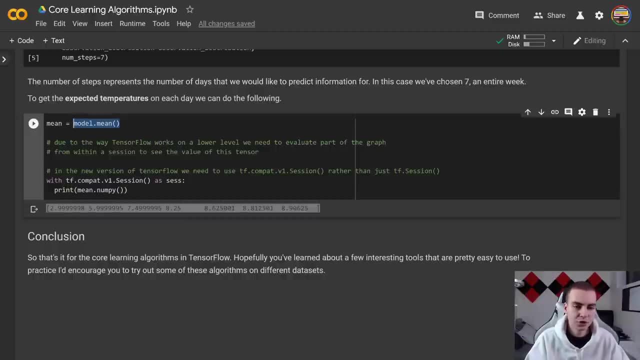 tensor. So remember, our tensors were like partially defined computations. Well, that's what model dot mean actually is that's what this method is. So if we want to get the value of that we actually need to do is create a new session in TensorFlow, run this part of the graph. 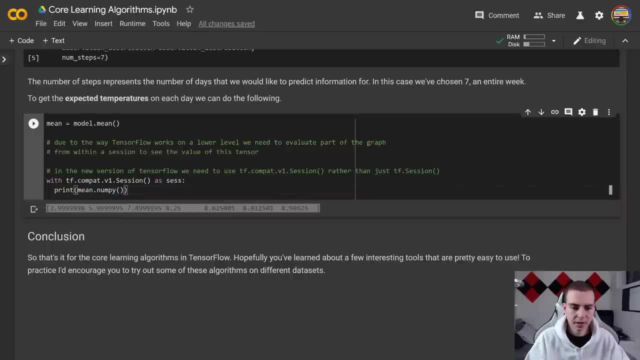 which we're going to get by doing mean dot numpy And then we can print that out. So I know this might seem a little bit confusing, but essentially to run a session in the new version of TensorFlow. so two point x or 2.1, or whatever it is you're going to type with tf dot compact. 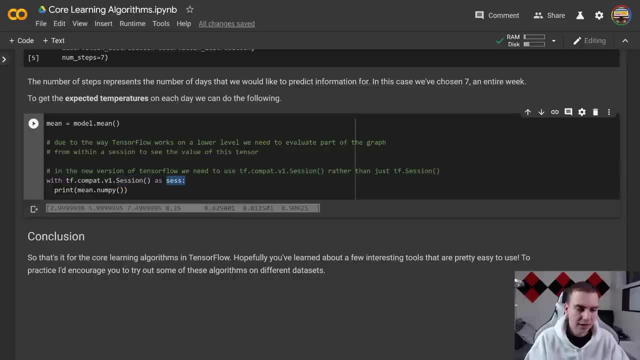 dot v, one dot session as sesh, And then I mean this doesn't really matter what you have here, but whatever you want. and then what I'm doing is just printing mean dot numpy So to actually get the value from this. here, this variable I call dot numpy, And then what it does is print. 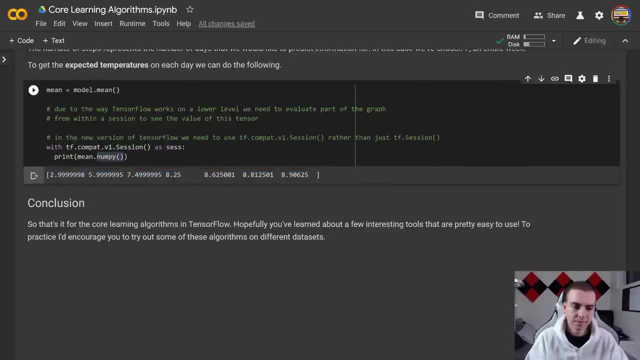 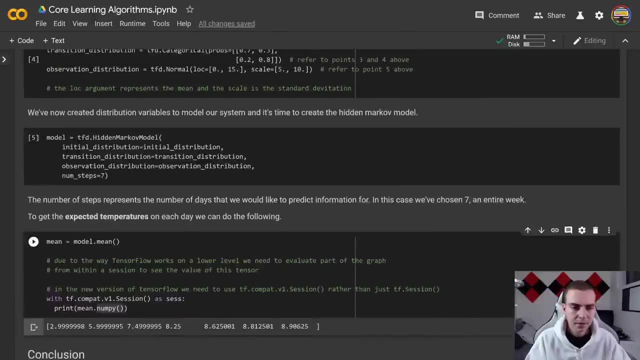 out this array that gives me the expected temperatures on each day. So we have, you know, three, six, essentially 7.5, 8.25.. And you can see, these are the temperatures based on the fact that we start with an initial probability of starting on a cold day. 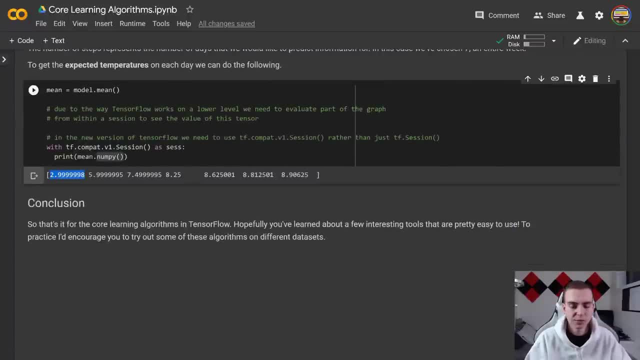 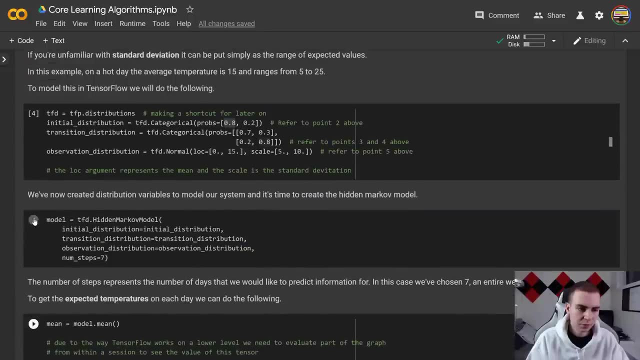 So we kind of get that here right. we're starting at three degrees, that's what it's determined we're going to start at, And then we have all of these other temperatures as predicting for the next days. Now notice if we recreate this model. so just rerun the distributions, rerun. 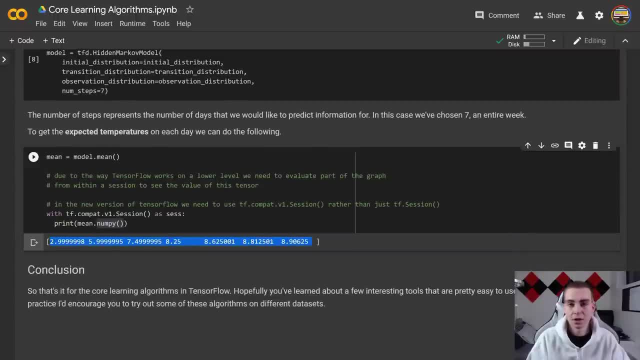 them and go model dot mean again, this stays the same, right? Well, because our probabilities are the same. this model is going to do the calculation, the exact same. there's not really any training that goes into this, So we get you know: very similar, if not the exact. 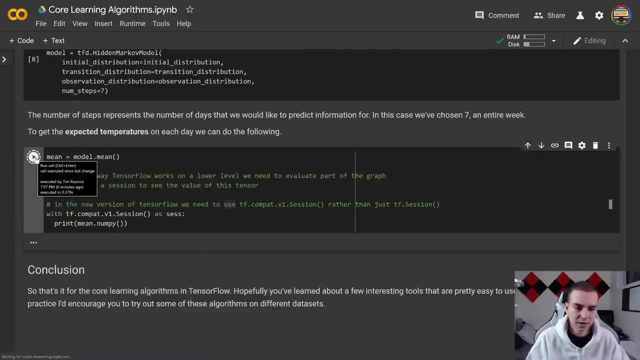 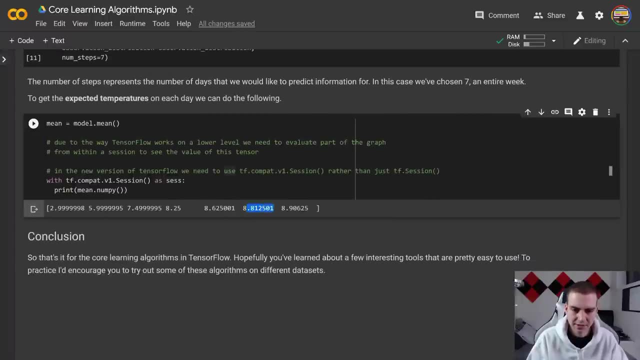 same values. I can't remember if these are identical, But that's what it looks like to me. I mean, we can run this again. see, we get the same one And we'll create the model one more time. And let me just check these values here to make sure I'm not lying to us. Yes, they're the exact same. 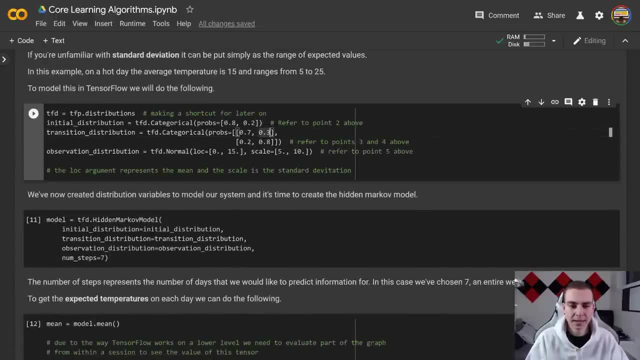 Okay, so let's start messing with a few probabilities and see what we can do to this temperature and see what changes we can cause. So if I do 0.5 here- and I do 0.5, for the categorical probability, remember this refers to points three and four above. 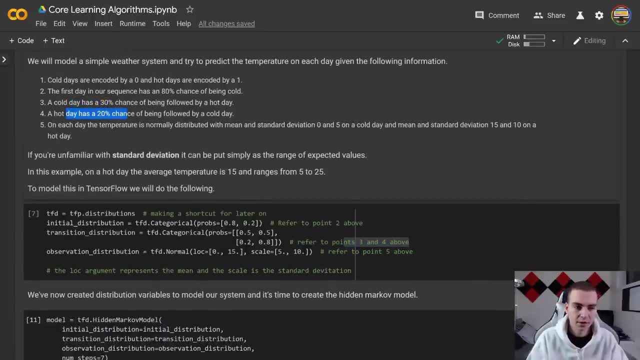 So that's, a cold day has a 30% chance of being followed by hot day, and then a hot day is 20% chance of being followed by cold day. So what I've just done now is change the probability to be 50%, So that a cold day now has a 50% chance of being followed by hot day and a 50% chance of 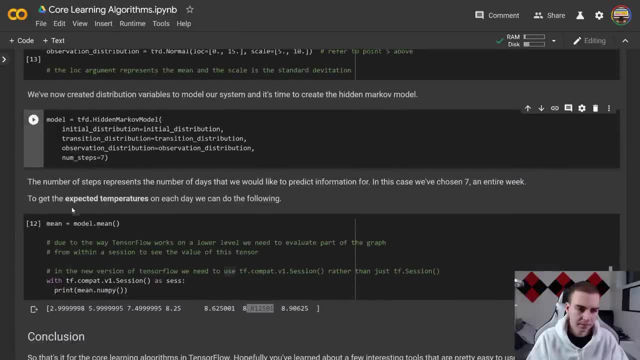 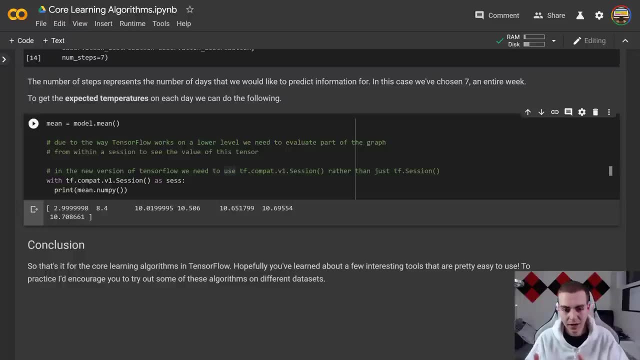 being followed by a cold day, And let's recreate this model, Let's rerun this And let's see if we get a difference. Oh, we do notice this. the temperature now has been is going a little bit higher. Now notice that we get the same starting temperature, because that's just the average. 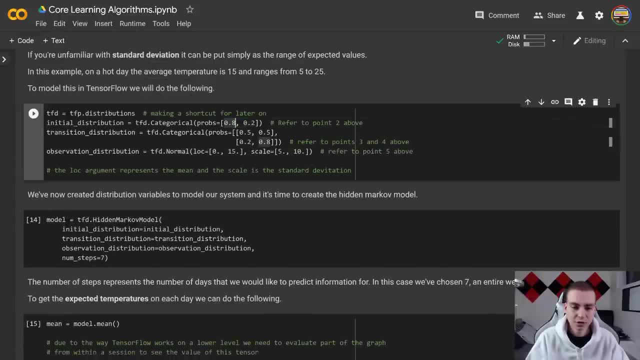 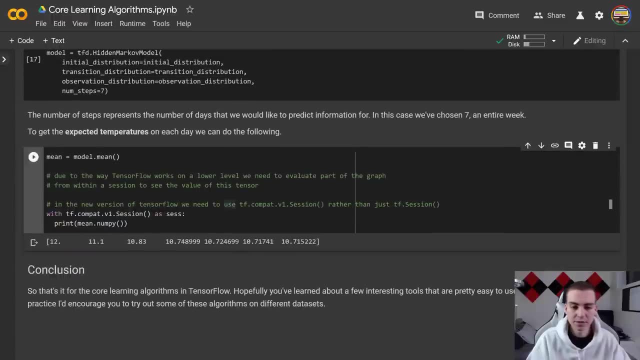 based on this probability that we have here. But if we wanted to potentially start, you know, hotter, we could reverse these numbers. we go 0.2- 0.8.. Let's rerun all of this And now look at this: what our temperatures are. we start at 12. And 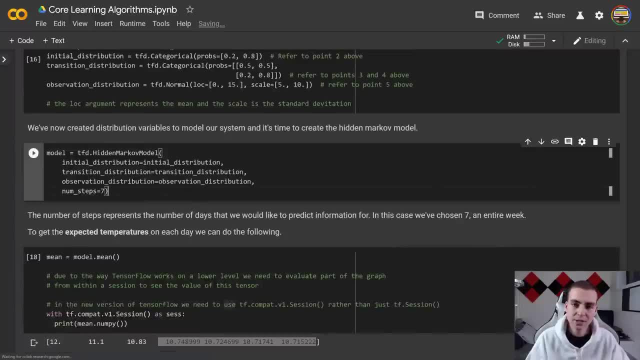 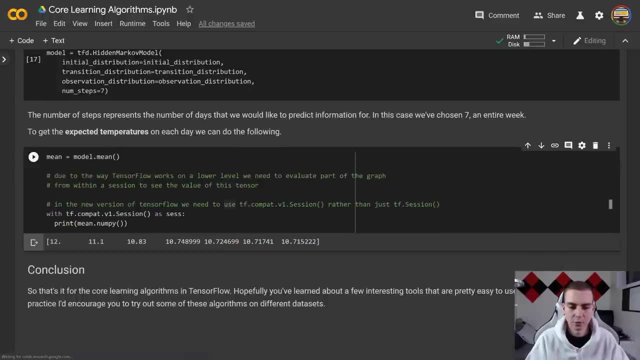 then we actually drop our temperature down to 10.. So that's how this hidden Markov model works. Now, this is nice because you can just tweak the probabilities. this happens pretty well instantly And we can have a look at our output very nicely. So obviously this is representing the temperature. 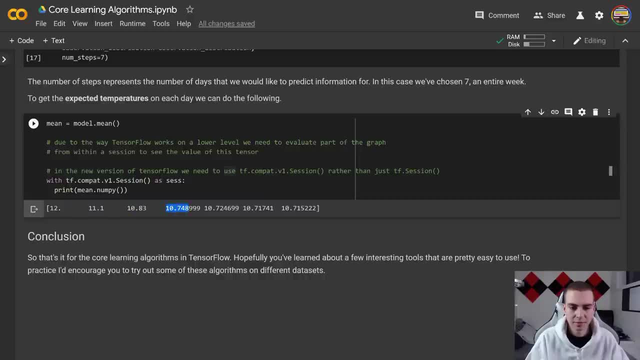 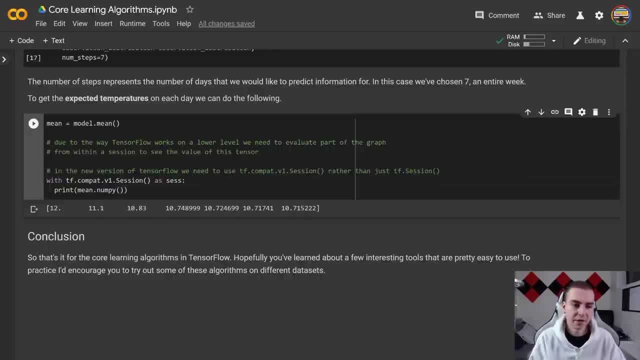 going to try to predict. you know a year in advance and you're using the weather that you have from, I guess, the previous year. you're probably not going to get a very accurate prediction, But anyways, these are hidden Markov models. they're not like extremely useful. 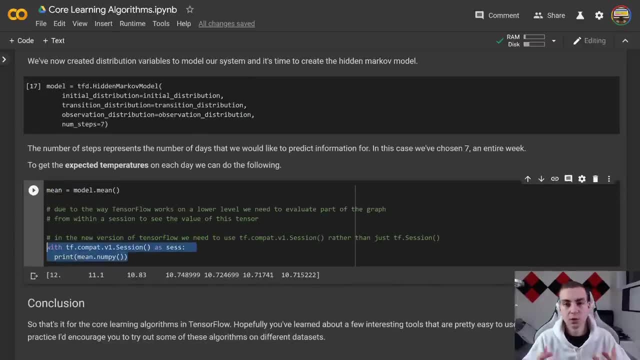 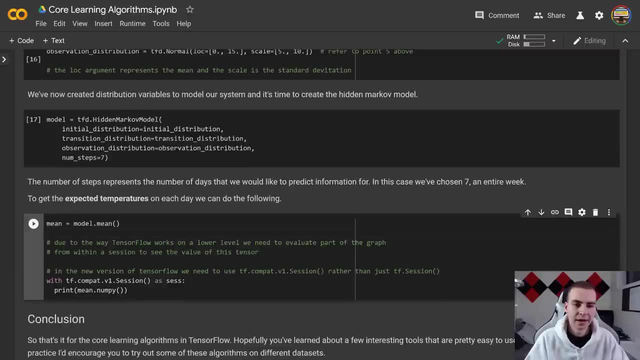 there's some situations where you might want to use something like this, So that's why we're implementing them in kind of in this course and showing you how they work. It's also another feature of TensorFlow that a lot of people don't talk about or see, And you know personally. 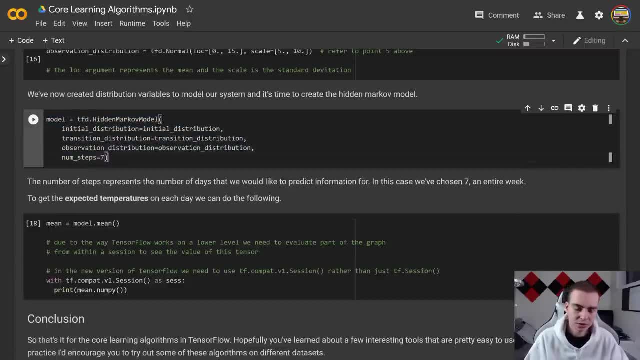 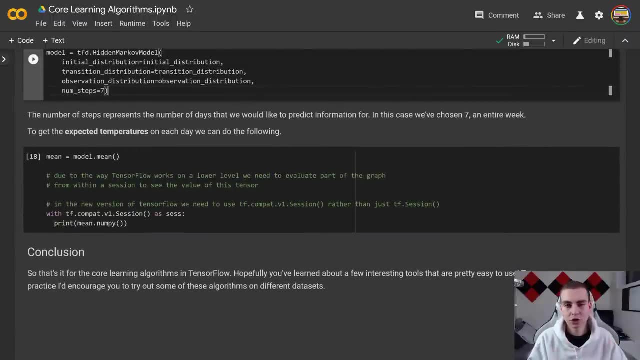 I hadn't really heard of hidden Markov models until I started developing this course. So, anyways, that has been it for this module. Now, I hope that this kind of gave you guys a little bit of an idea of how we can actually implement some of these machine learning algorithms, a little bit of idea of how to work with data. 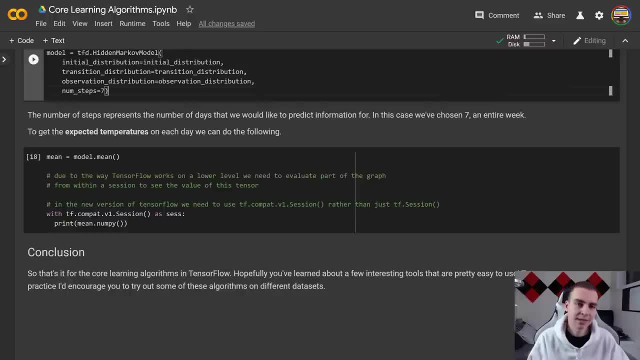 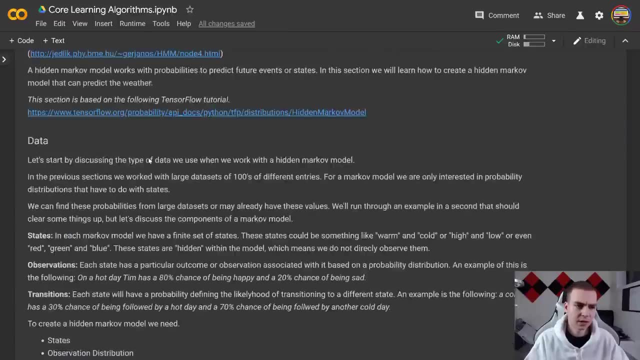 how we can feed that to a model, the importance between testing and training data, And then, obviously, linear regression is one we focused a lot on, So I hope you guys are very comfortable with that algorithm. And then, what was the last? the second one we did- I got to go up. 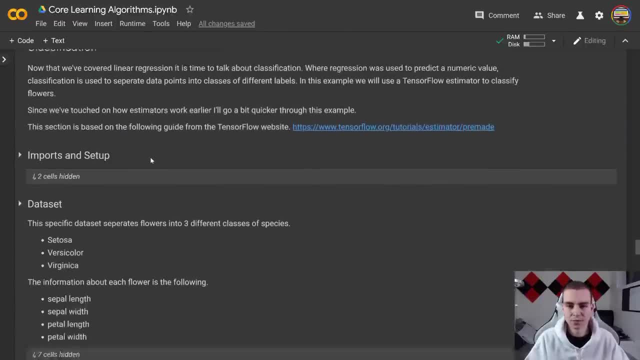 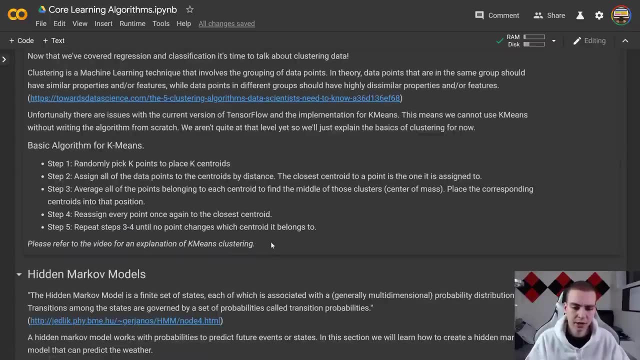 to remember exactly the sequence we had here. So classification- that one was important as well. So I hope you guys really understood that. clustering- we didn't go too far into that. Again, this is an interesting algorithm And if you need to do some kind of clustering, 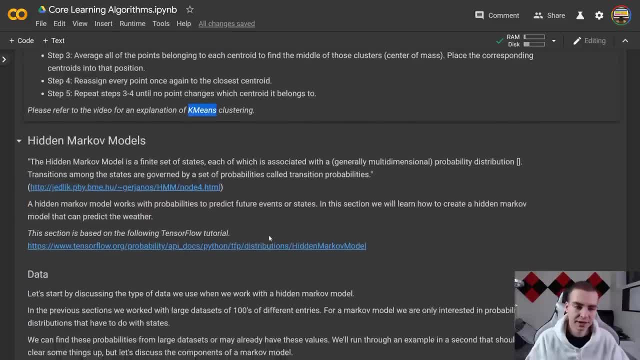 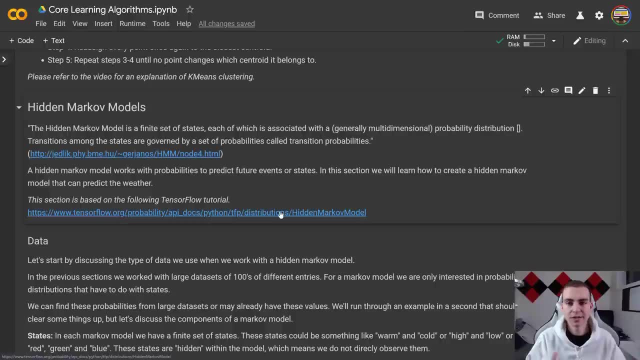 you now know of one algorithm to do that, called k means clustering, and you understand how that works. And now you know hidden Markov models. So in the next module we're going to start covering neural networks. we now have the knowledge we need to really dive. 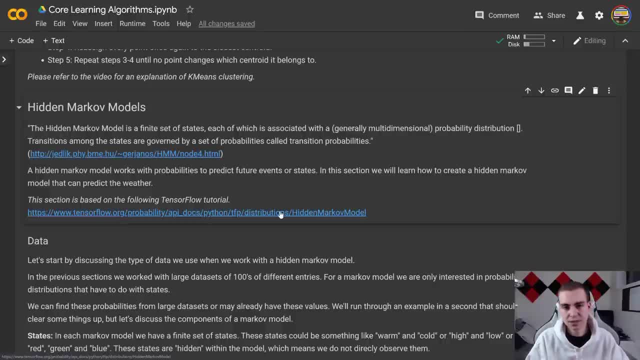 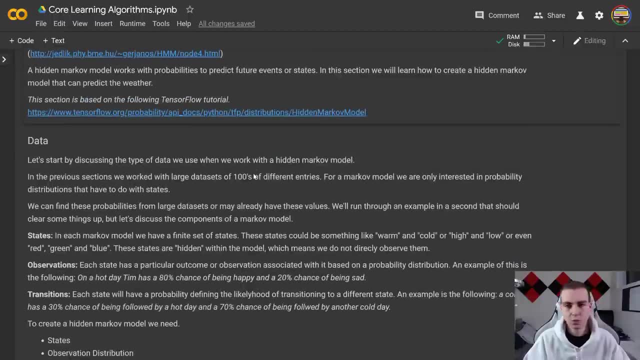 in there and start doing some cool stuff, And then, in the future modules, we're going to do deep computer vision. I believe we're going to do chat bots with recurrent neural networks and then some form of reinforcement learning at the end. So, with that being said, 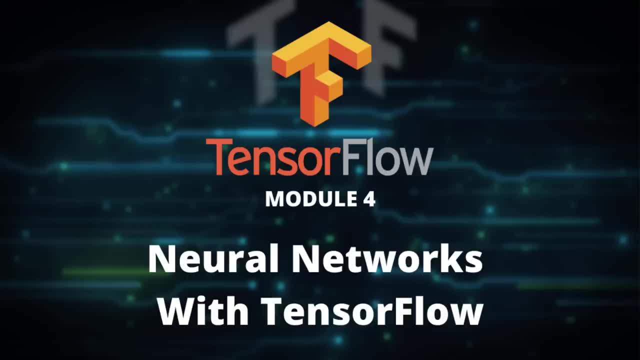 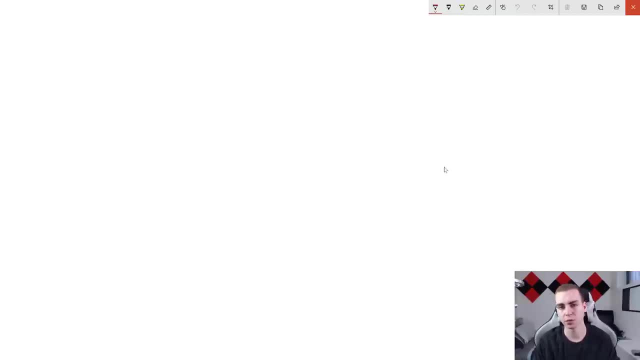 let's go to the next module. Hello everybody and welcome to module four. Now in this module of this course, we're gonna be talking about neural networks, discussing how neural networks work, a little bit of the math behind them, talking about gradient descent and back propagation and how information 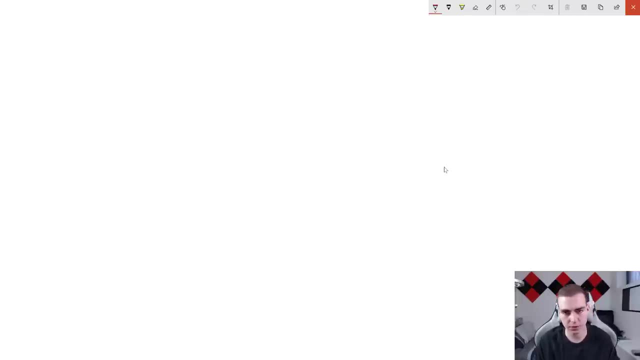 actually flows through the neural network And then getting into an example where we use a neural network to classify articles of clothing. So I know that was a lot, But that's what we're gonna be covering here Now. neural networks are complex. there's kind. 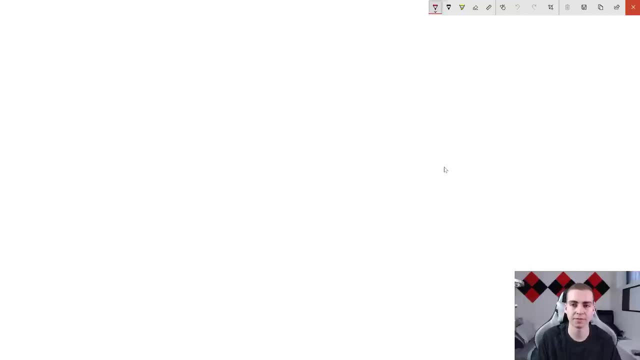 of a lot of components that go into them, And I'm going to apologize right now because it's very difficult to explain it all at once. what I'm going to be trying to do is kind of piece things together and explain them in blocks And then at the end you know. 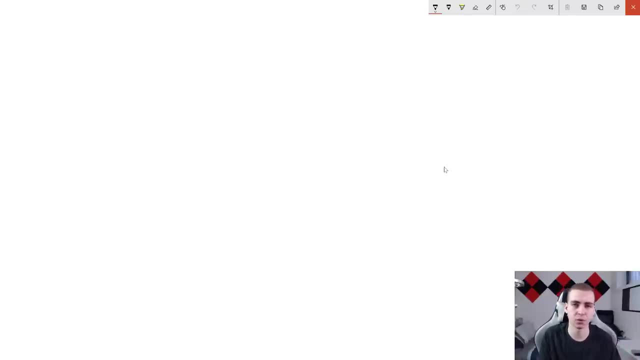 kind of combine everything together. And I will say, in case any of you didn't watch the beginning of this course, I do have very horrible handwriting, But this is the easiest way to explain things to you guys. So bear with me, you know, I'm sure you'll be able to understand. 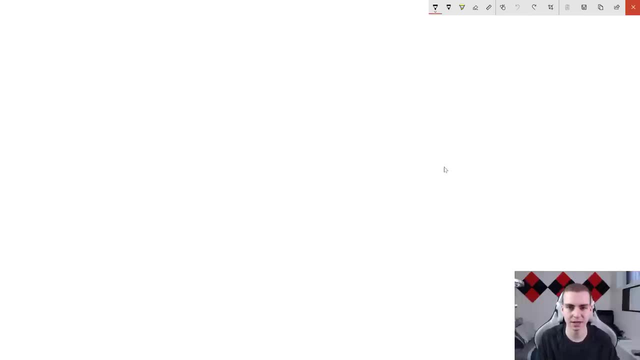 what I'm saying, But it might just be painful to read some of it, Alright, so let's get into it right away and start discussing what neural networks are and how they work. Well, the whole point of this course is to explain how neural networks work, And I'm going to 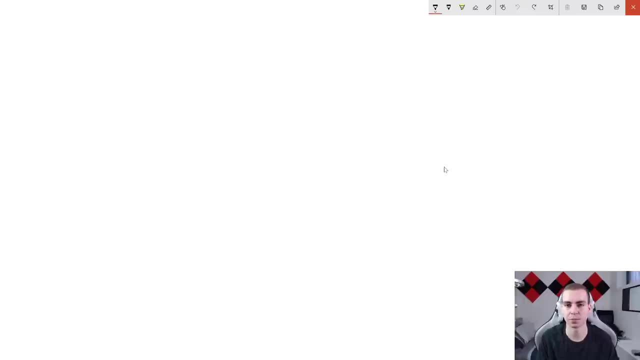 start with, the first point of a neural network is to provide, you know, classification or predictions for us. So we have some input information, we feed it to the neural network and then we want it to give us some output. So if we think of the neural network as this, 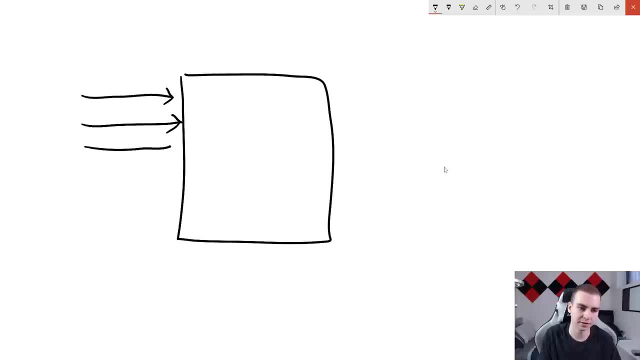 black box. we have all this input right. we give all this data to the neural network. maybe we're talking about an image, maybe we're talking about just some random data points, maybe we're talking about a data set- and then we get some meaningful output. This: 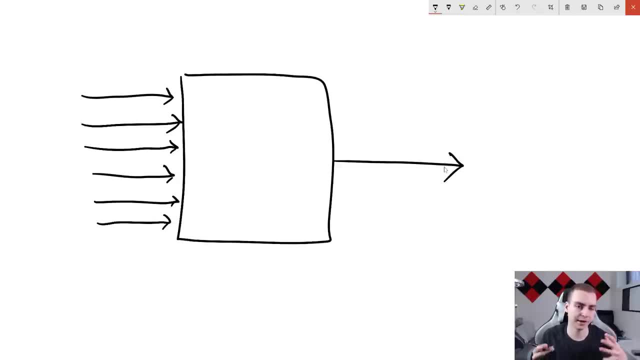 is what we're looking at. So if we're just looking at a neural network from kind of the outside, we think of it as this magical box. So we have this black box, we give some input, it gives us some output, And I mean we could. 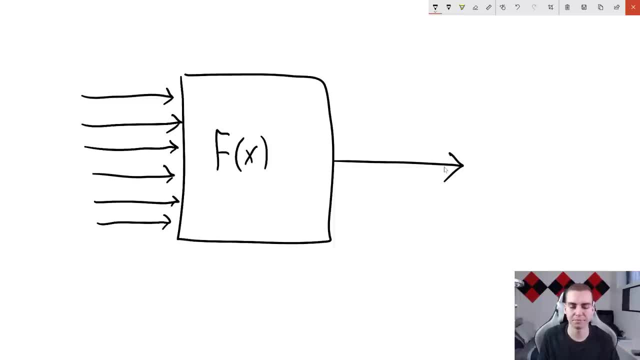 call this black box. just some function right, where it's a function of the input, maps it to some output. And that's exactly what a neural network does: It takes input and maps that input to some output, just like any other function right, Just like if you had a straight. 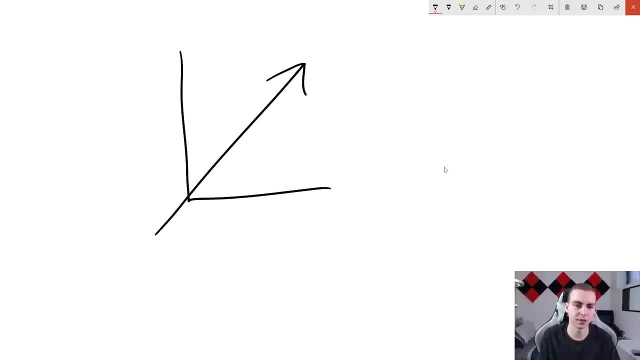 line like this. this is a function. you know, this is your line. you know, whatever it is, you're gonna say: y equals like four x. maybe that's your line. you have some input x and it gives you some value y. this is a. 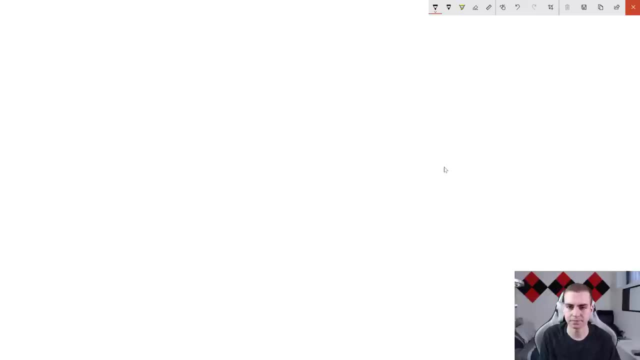 m mapping of your input to your output. Alright, so now that we have that down, what is a neural network made up? Well, a neural network is made up of layers, And remember, we talked about the layered representation of data when we talk about neural networks. So I'm going 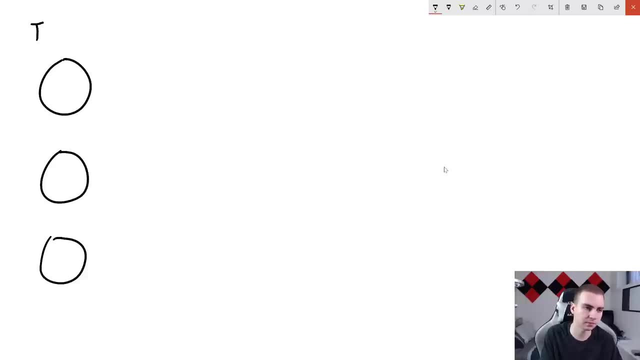 to draw a very basic neural network. we're going to start with the input layer. Now, the input layer is always the first layer in our neural network And it is what is going to accept our raw data. Now, what I mean by raw data is: 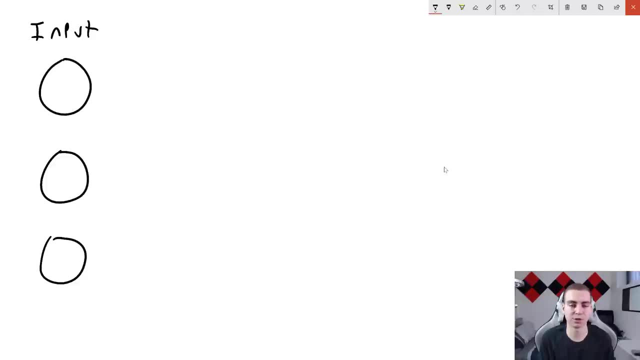 whatever data we like want to give to the network, whatever we want to classify, whatever our input information is, that's what this layer is going to receive in the neural network. So we can say: you know, these arrows represent our input and they come to our first input. 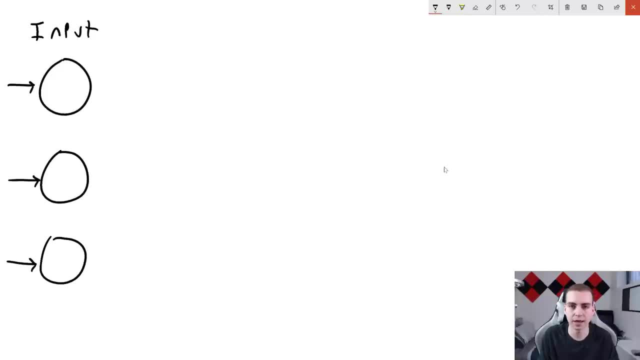 layer. So this means, for example, if you had an image, and this image, and I'll just draw like one- like this, let's say this: our image and it has all these different pixels, right, all these different pixels in the image, and you want to make a classification on this. 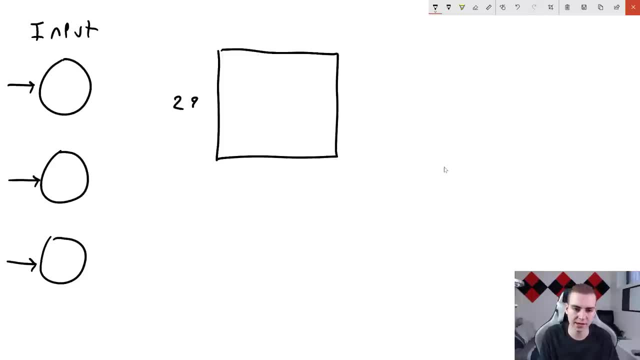 image. well, maybe it has a width and a height, And a classic width and height example is 28 by 28.. If you had 28 by 28 pixels and you want to make a classification on this image, how many input neurons you think you? 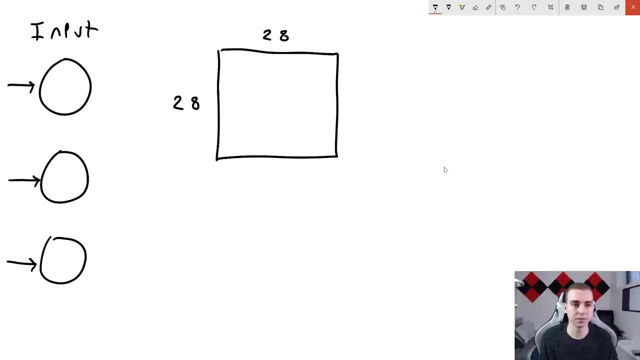 would need in your neural network to do this. Well, this is kind of, you know, a tough question if you don't know a lot about neural networks. If you're predicting for the image, if you're going to be looking at the entire image to make a prediction, you're going to need every 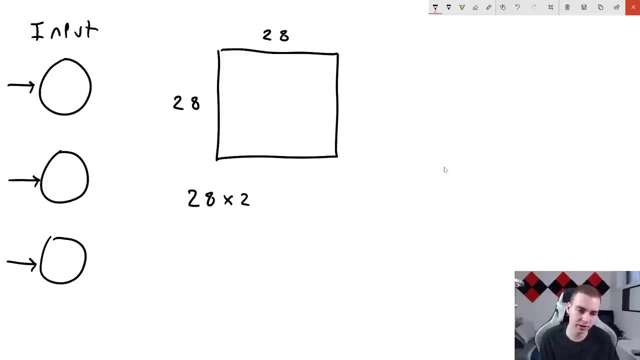 single one of those pixels, which is 28 times 28 pixels, which I believe is something like 700.. 84, I could be wrong on that number, but I believe that's what it is. So you would need 784 input input neurons. Now, that's totally fine. that might seem like a big number, but 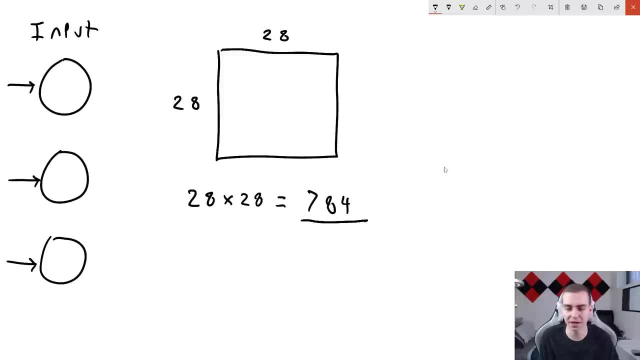 we deal with massive numbers when it comes to computers, So this really isn't that many, But that's an example of you know how you would use a neural network input layer to represent an image. you would have 784 input neurons and you would pass one pixel to every. 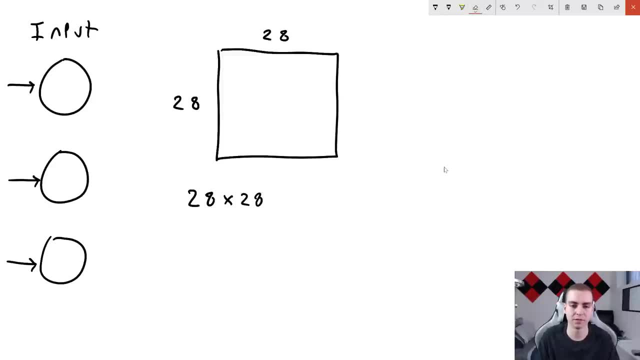 single one of those neurons. Now, if we're doing an example where maybe we just have one piece of input information, maybe it's literally just one number, well then all we need is one input neuron. If we have an example where we have four pieces of information, we would need four input neurons. 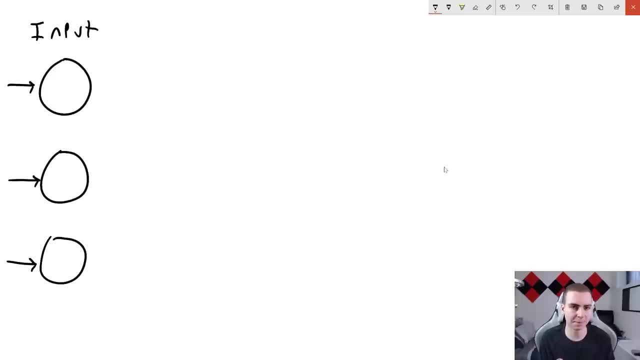 right Now this can get a little bit more complicated, But that's the basis that I want you to understand is that you know the pieces of input you're going to have, regardless of what they are, you need one input neuron for each piece of that information, unless 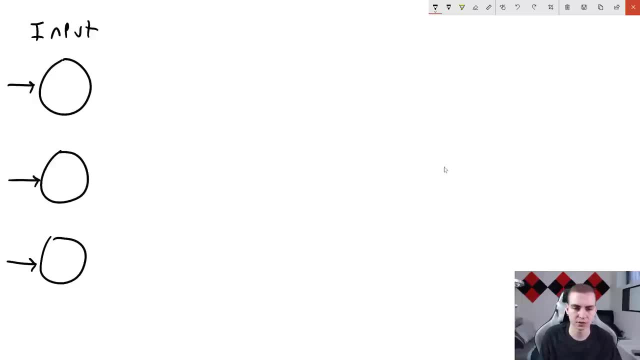 you're going to be reshaping or putting that information in different form. Okay, so let's just actually skip ahead and go to now, our output layer. So this is going to be our output. Now, what is our output layer? Well, our output layer. 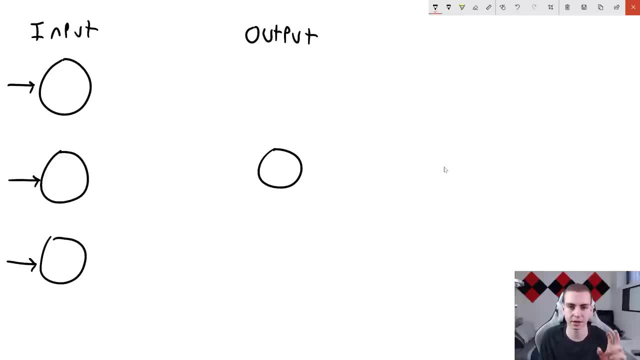 is going to have as many neurons And again the neurons are just representing, like a node in the layer as output pieces that we want. Now let's say we're doing a classification for images, right, And maybe there's two classes that we could represent. Well, there's a few. 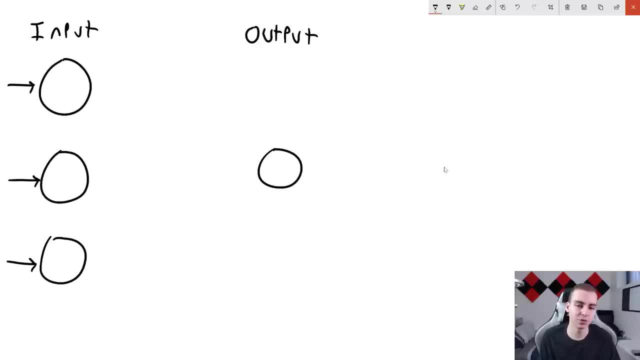 different ways we could design our output layer. what we could do is say, okay, we're going to use one output neuron. this output neuron is going to give us some value, And we want this value to be between zero and one, And we'll say: that's inclusive. Now, 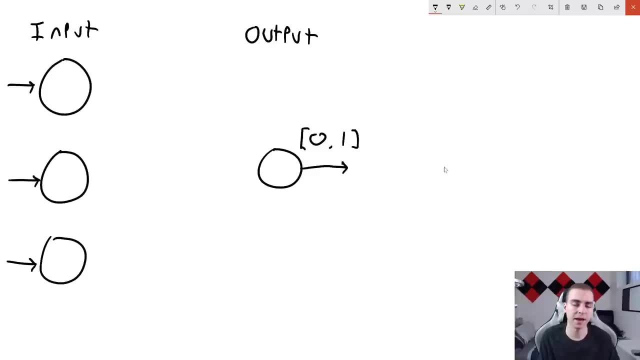 what we can do now. if we're predicting two classes, say: Okay, so if my output neurons going to give me some value, if that value is closer to zero, then that's going to be class zero. If this value is closer to one, it's going to be class one. right, And that? 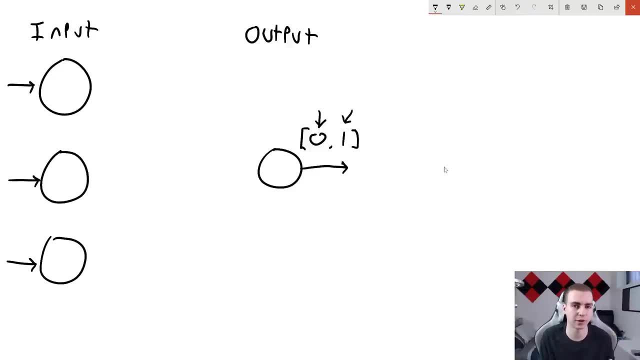 would mean when we have our training data- and we talked about training and testing data- we'd give our input and our output would need to be the value of our output. So we have a value zero or one, because it's either the correct class, which is zero, right, or 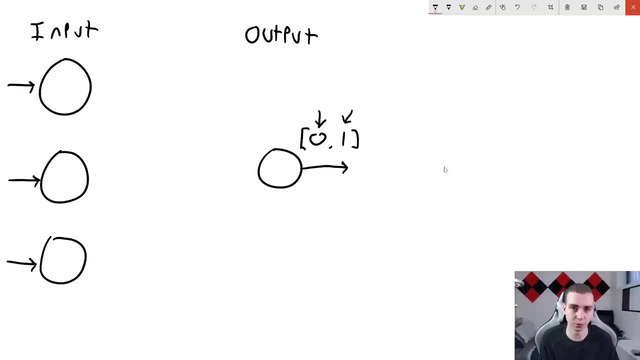 the correct class, which is one. So, like our- what am I saying? our labels for our training data set would be zero and one, and then this value on our output neuron will be guaranteed to be between zero and one, based on something that I'm going to talk about a little bit. 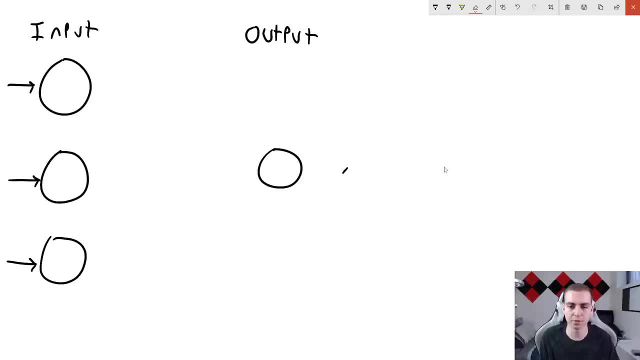 later. That's one way to approach it right. we have a single value. we look at that value And, based on what that value is, we can determine. you know what class we predicted not work sometimes, But in other instances, when we're doing classification, what makes more sense. 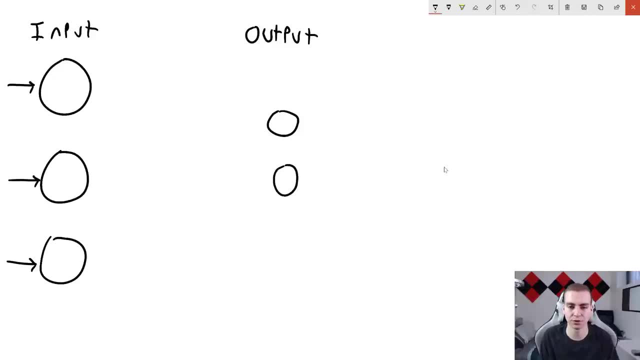 is to have as many output neurons as classes you're looking to predict for. So let's say we're going to have, you know, like five classes that we're predicting for, and maybe these three pieces of input information are enough to make that prediction. well, we'd actually. 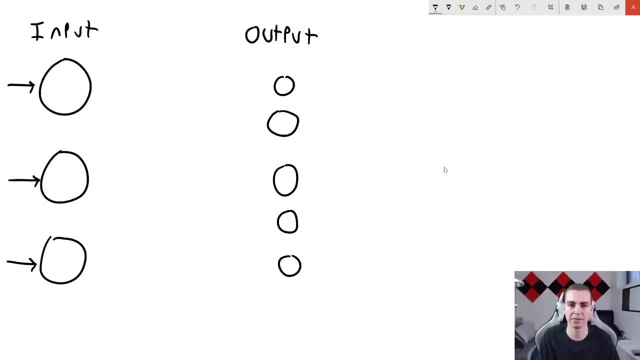 have five output neurons, And each of these neurons would have a value between zero and one And the combination, so the sum of every single one of these values would be equal to one. Now can you think of what this means if every single one of these neurons has a? 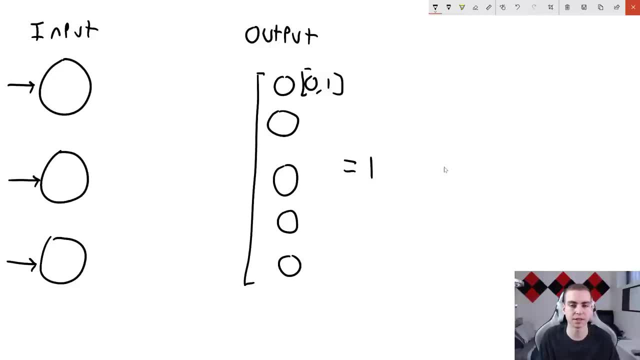 value of one, and we're going to have a value of zero, and then we're going to have a value between zero and one, and their sum is one. what does this look like to you? Well, to me this looks like a probability distribution, And essentially, what's going to happen is we're going to make 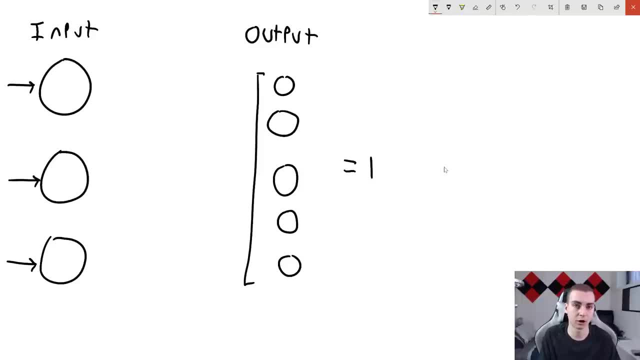 predictions for how strongly we think each our input information is each class. So if we think that it's like class one- maybe we'll just label these like this- then what we would do is say, okay, this is going to be 0.9, representing 90%. Maybe this is like 0.001.. Maybe this is 0.05- 0.0.. 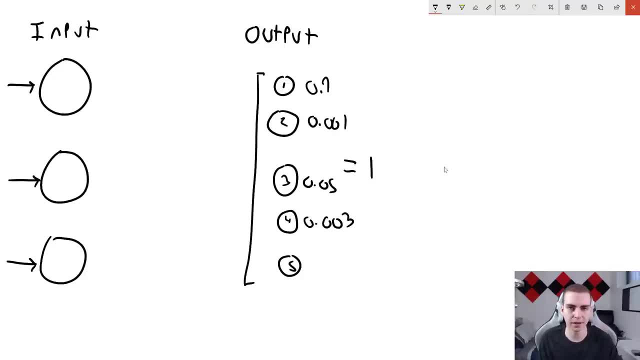 Three. right, you get the point. it's going to add up to one, And this is a probability distribution for output layer. So that's a way to do it as well. And then, obviously, if we're doing some kind of regression task, we can just have one neuron and that will just predict some value. And 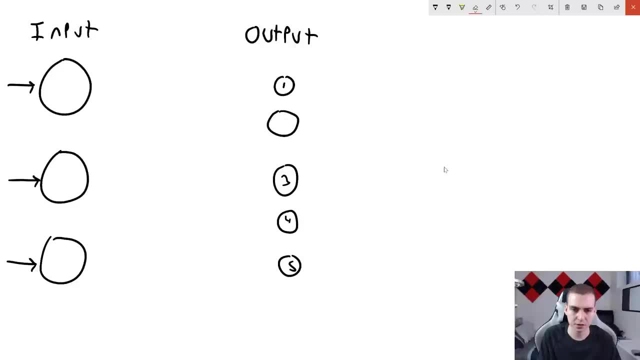 we'll define. you know what we want that value to be. Okay, so that's my example for my output. Now let's erase this And let's actually just go back to one output neuron, because that's what I want to use for this example. Now we have something in between these layers Because obviously you know, 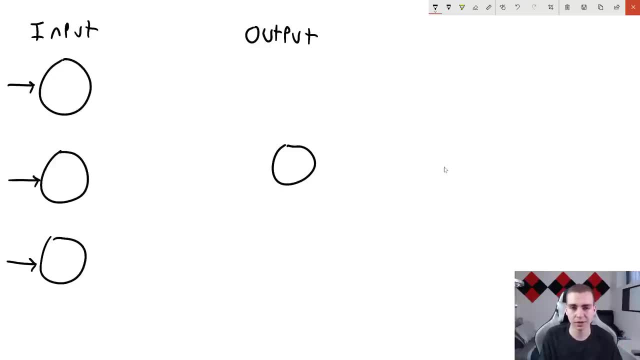 we can't just go from input to output with nothing else. What we have here is called a hidden layer. Now, in neural networks we can have many different hidden layers. we can have, you know, hidden layers that are connecting to other hidden layers, And like we could have hundreds, 1000s if we wanted to, for this. 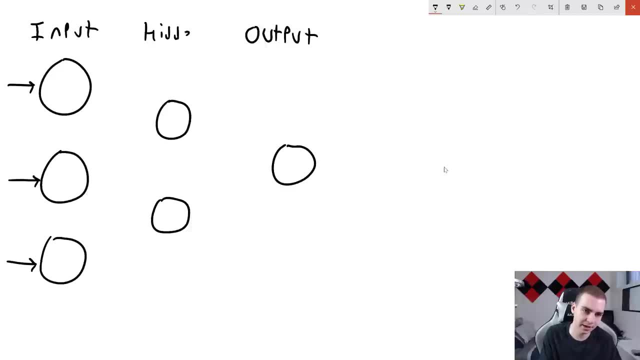 basic example, we'll use one And I'll write this as hidden. So now we have our three layers. Now why is this called hidden? The reason this is called hidden is because we don't observe it when we're using the neural network. we pass information to the input layer. we get information from the output. 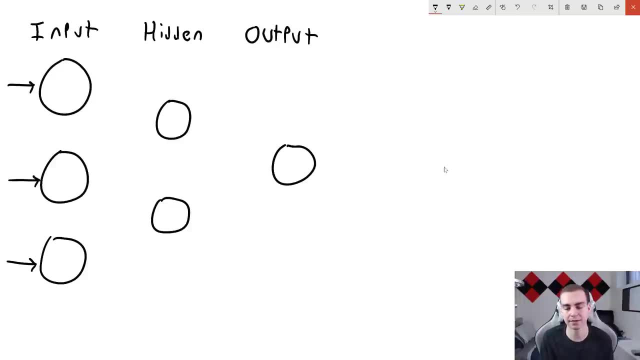 layer. we don't know what happens in this hidden layer or in these hidden layers. Now, how are these layers connected to each other? How do we get from this input layer to the hidden layer, to the output layer and get some meaningful output? Well, every single layer is connected to another layer with something. 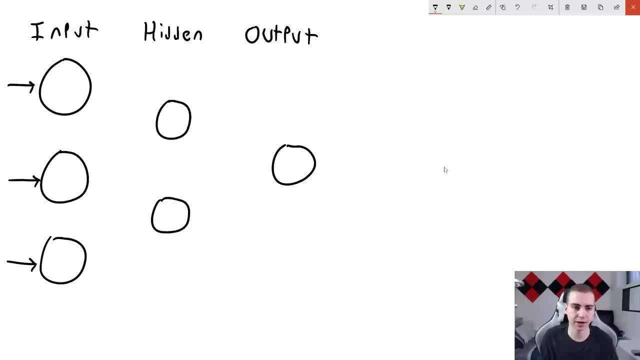 called weights. Now we can have different kinds of architectures, of connections, which means I could have something like this: can one connects to this, this connects to this, this connects to this, And that could be like my connection kind of architecture. right, We could have another one. 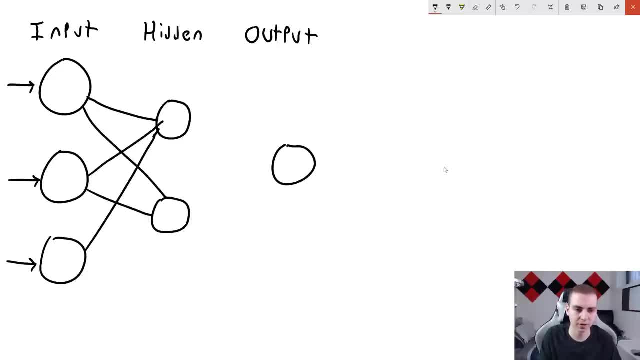 where this one goes here And you know, maybe this one goes here And actually, after I've drawn this line, now we get what we're going to be talking about: a lot which is called a densely connected neural network, Now a densely 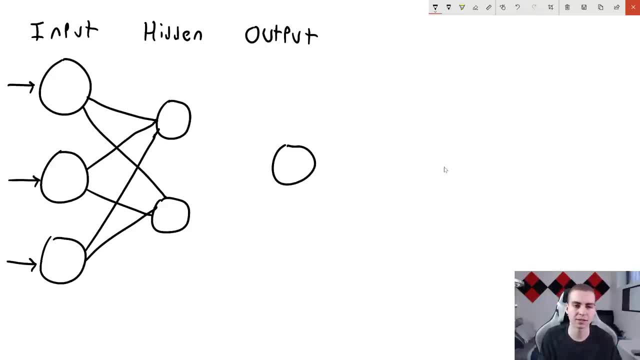 connected neural network or a densely connected layer essentially means that is connected to every node from the previous layer. So in this case you can see every single node in the input layer is connected to every single node in the output layer or in the hidden layer. my bad And these? 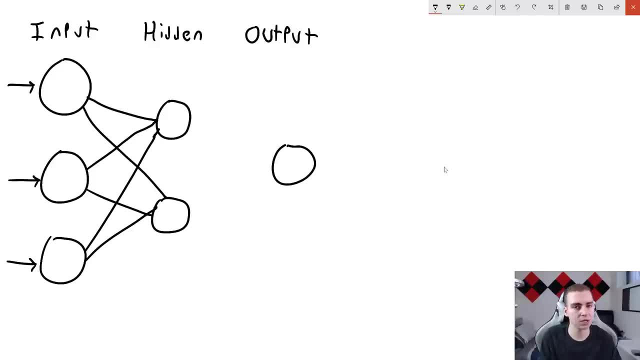 connections are what we call weights. These weights are actually what the neural network is going to change and optimize to determine the mapping from our input to our output. Because, again, remember, that's what we're trying to do. we have some kind of function: we give some input, it gives us some output. how do we get that input and 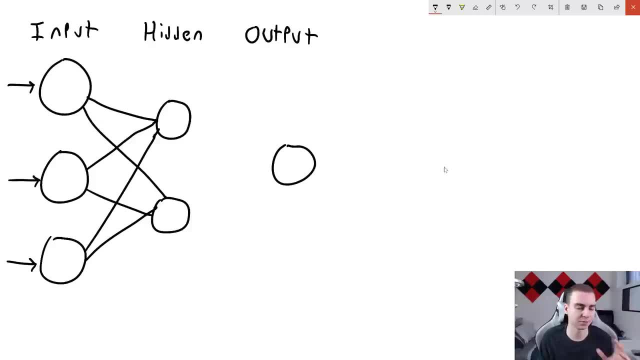 output. Well, by modifying these weights it's a little bit more complex, but this is the starting. So these lines that I've drawn are really just numbers, And every single one of these lines is some numeric value. Typically these numeric values are between zero and one, but they can be large. they 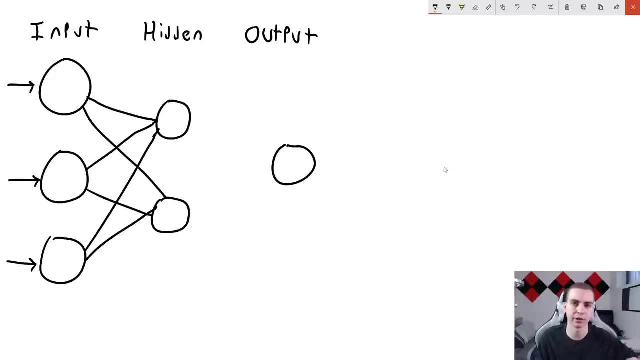 can be negative On what kind of network you're doing and how you've designed. Now let's just write some random numbers. we'd have like 0.1,. this could be like 0.7,. you get the point right. we just have numbers. 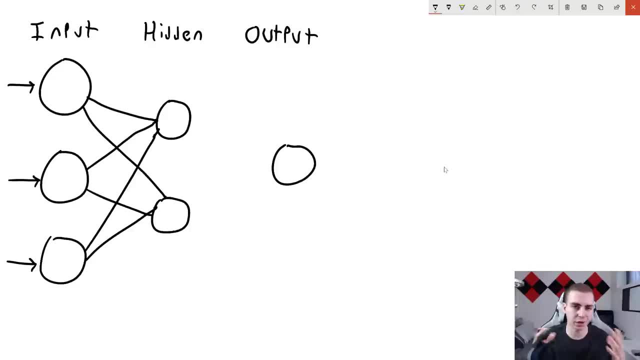 for every single one of these lines- And these are what we call the trainable parameters- that our neural network will actually tweak and change as we train to get the best possible result. So we have these connections Now. our hidden layer is connected to our output layer as well. This is again. 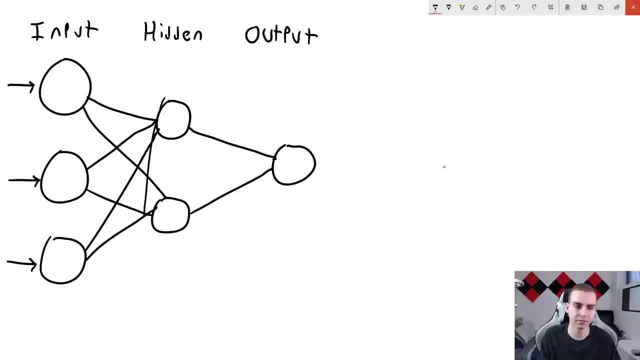 another densely connected layer, Because every layer or every newer on from the previous layer is connected to every neuron from the next layer. you would like to determine how many connections you have. what you can do is say there's three neurons here. there's. 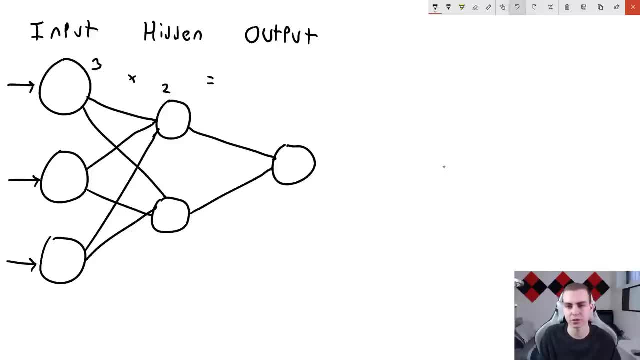 two neurons here. three times two equals six connections. That's how that works from layers, And then obviously you can just multiply all of the neurons together as you go through and determine what that's going to be. Okay, so that is how we connect these layers. we have these weights. So 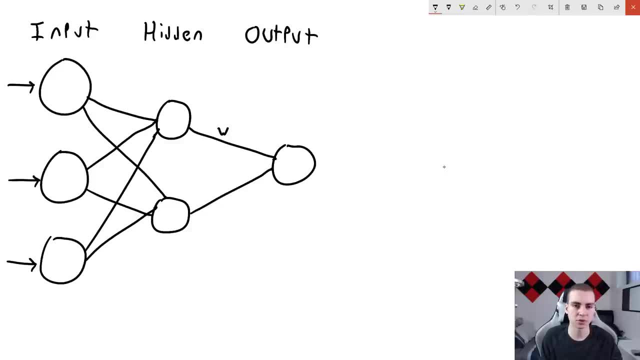 let's just write a W on here, So remember that those are weights. Now we also have something called biases, So let's add a bias here. I'm going to label this B Now. biases are a little bit different than these nodes we have. regularly. there's only one bias and a bias exists in the previous layer. 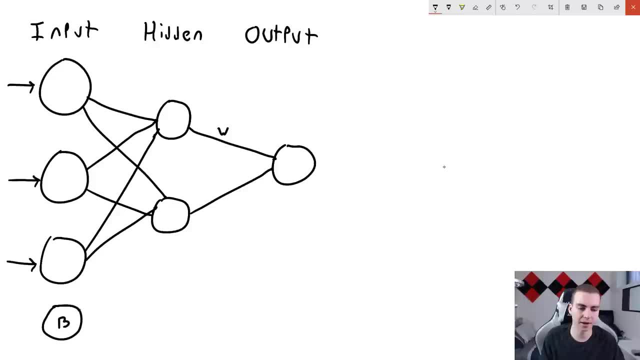 to the layer that it affects. So in this case, what we actually have is a bias that connects to each neuron in the next layer from this layer, right. so it's still densely connected, But it's just a little bit different. Now notice that this bias doesn't have an arrow beside it, because this: 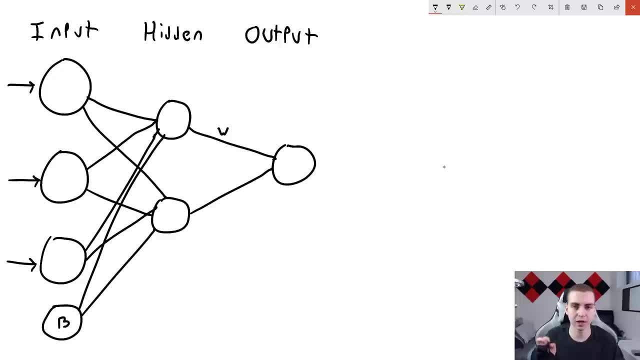 doesn't take any input information. This is another trainable parameter for the network, And this bias is just some constant numeric value that we're going to connect to the hidden layer, So we can do a few things with it. Now, these weights always have a value of one. we're going to talk about why they have a value. 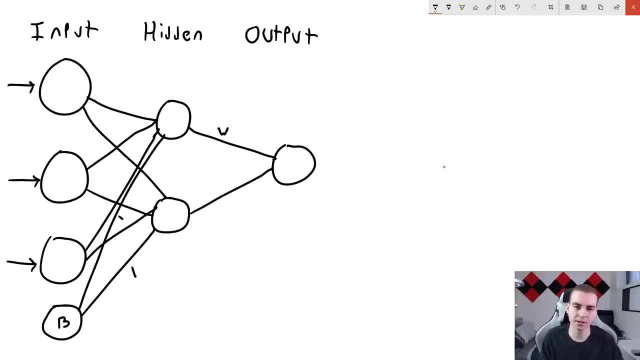 of one in a second. But just know that whenever a bias is connected to another layer or to another neuron, its weight is typically one. Okay, so we have that connected, we have our bias And that actually means we have a bias. So we have a bias that connects to another layer. So we have a bias. 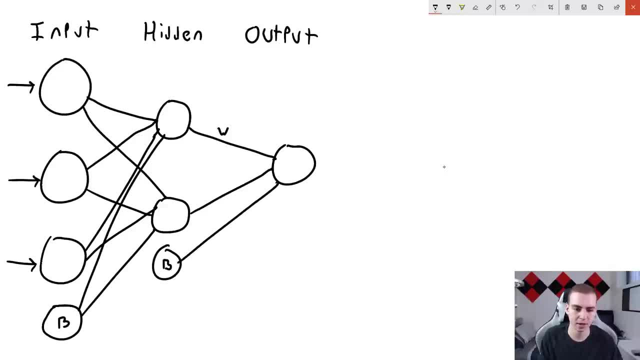 here as well, And this bias connects to this. notice that our biases do not connect with each other. The reason for this, again, is they're just some constant value And they're just something we're kind of adding into the network as another trainable parameter that we can use. Now let's 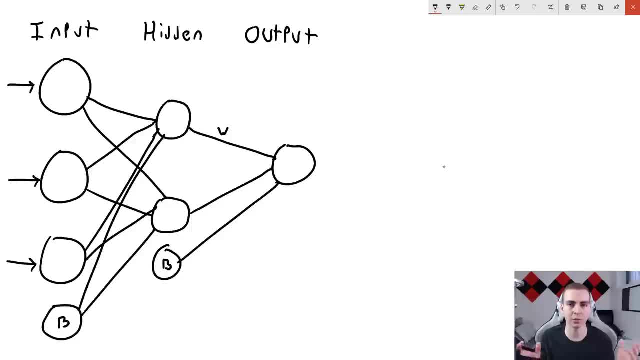 talk about how we actually pass information through the network and why we even use these weights and biases of what they do. So let's say we have. I can't really think of a good example, So we're just gonna do some arbitrary stuff. Let's say we have like a data, points right, x, y, z and 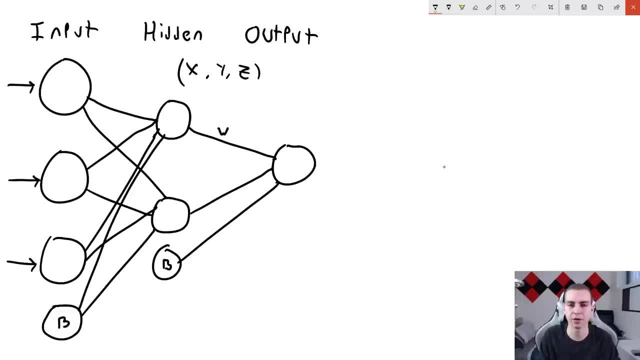 z, And all of these data points have some mapped value right. There's some value that we're looking for for them or there's some class we're trying to put them in. maybe we're clustering them between, like, red dots and blue dots, So let's do that. Let's say an x, y, z is either a part of the red 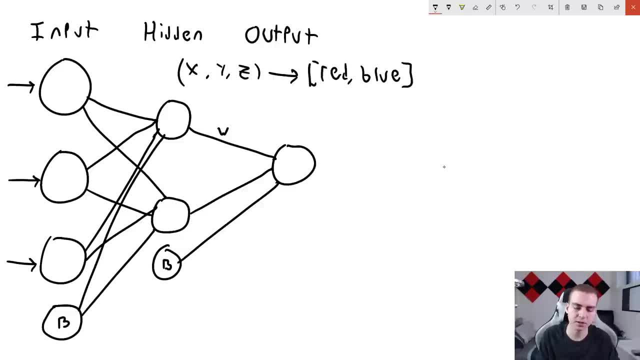 class or the blue class. let's just do that. So what we want this output neuron to give us is red or blue. So what I'm going to do is say, since it's just one class, we'll get this output neuron in. 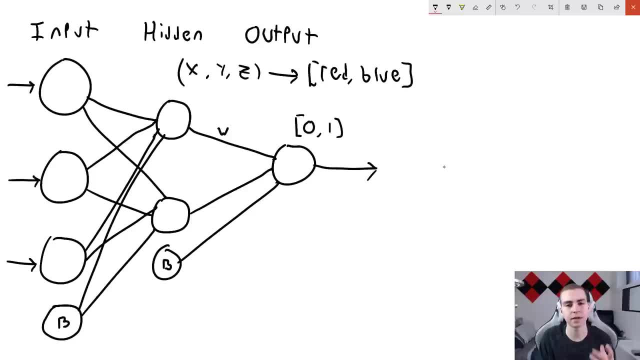 between the range is your own one. we'll say, okay, we're going to give this output neuron a value. Okay, if it's closer to zero, that's red, if it's closer to one, that's blue. And that's what. 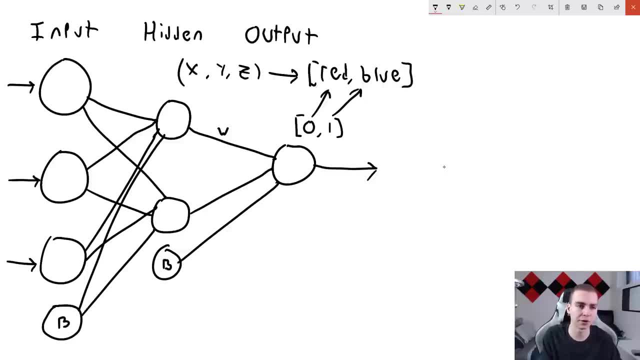 we'll do for this network And for this example. now our input neurons are going to obviously be x, y and z. So let's pick some data point And let's say we have, you know, the value two, two. 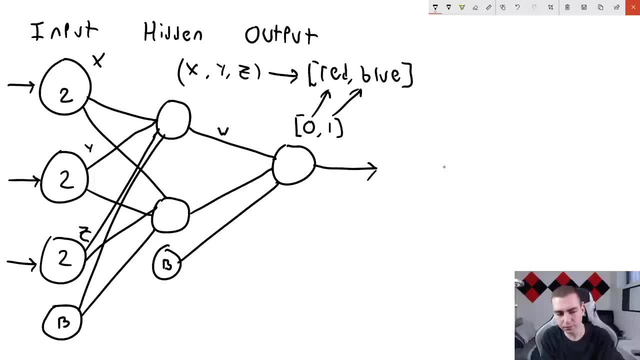 two. that's our data point, And we want to predict whether it's red or blue. How do we pass it through? Well, what we need to do is determine how we can- you know, find the value of this hidden layer. note: we already know the value. 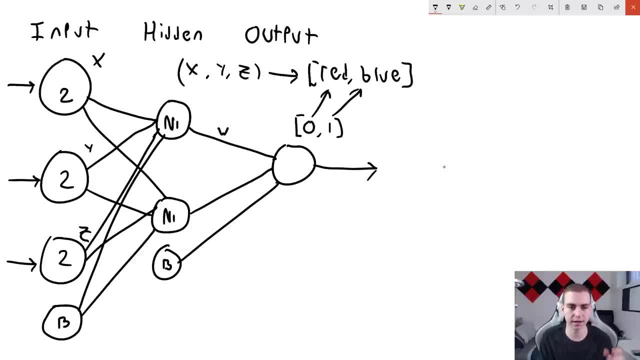 This input node. but now we need to go to the next layer, using these connections, and find what the value of these nodes are. Well, the way we determine these values is, I'm going to say, and I've just said n one just to represent: like this is a node, like this is node one, maybe this one? 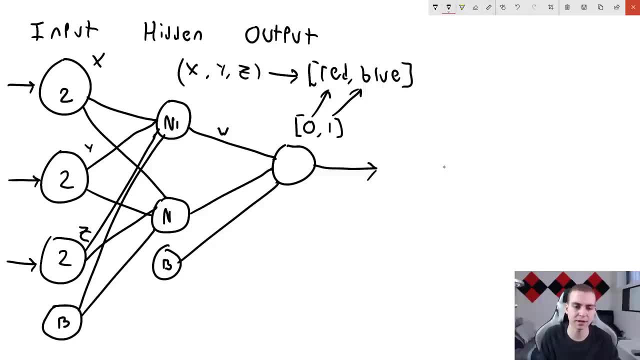 should be. node two is equal to what we call the weighted sum of all of the previous nodes that are connected to it, if that makes any sense to you guys. So a weighted sum is something like this. So I'm just going to write the equation. I'll explain it. I'm gonna say n one is: 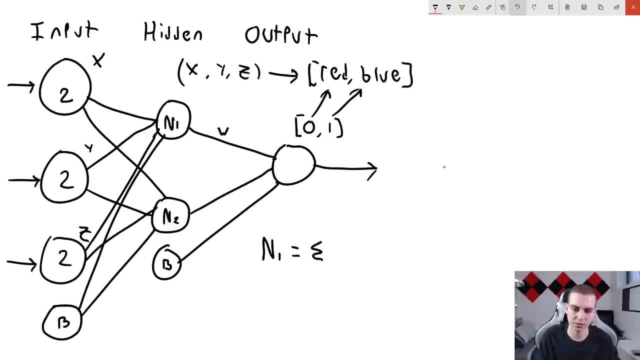 equal to the sum of. let's not say n equals zero. let's say i equals zero to n of. in this case we're going to say wi times x, i plus b. Now I know this equation looks really mathy and complicated. 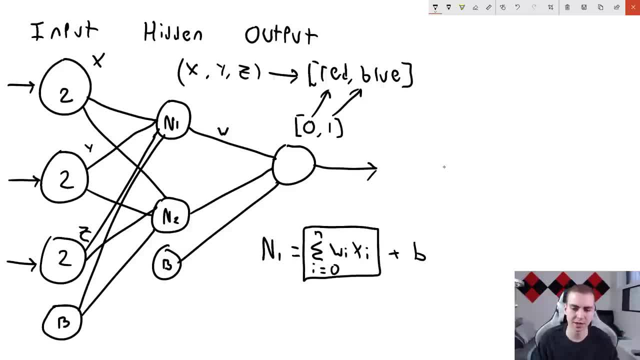 it's really not. what this symbol and this equation here means is take the weighted sum of all the neurons that are connected to this neuron. So in this case we have neuron x, neuron y and neuron z connected to n one. So when we take the weighted sum or we calculate this, what this is really equal to is the weight. 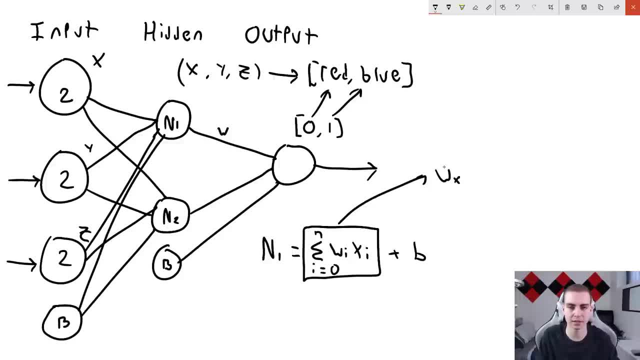 at neuron x, we'd say w? x times the value at neuron x, which in this case is just equal to two right Plus whatever the weight is at neuron y. So in this case this is w? y and then times two. 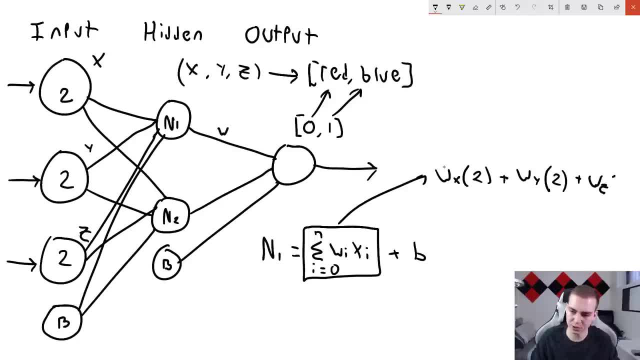 And then you get the point where we have w, z and I'm trying on the edge of my drawing tablet to write this times two. Now, obviously, these weights have some numeric value. Now, when we start our neural network, these weights are just completely random. They don't make any sense. 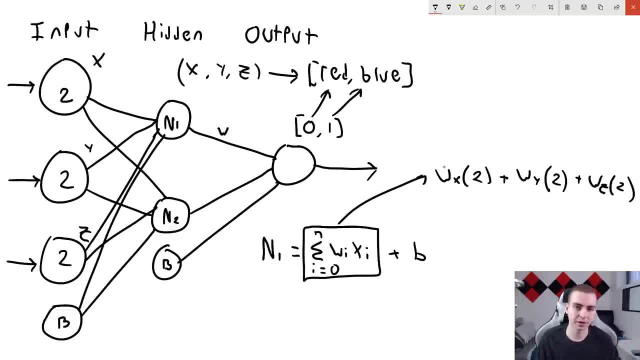 or just some random values that we can use. As the neural network gets better, these weights are updated and changed to make more sense in our network. So right now we'll just leave them as w, x, w, y, w, z. But no, these are some numeric values, So this returns to a. 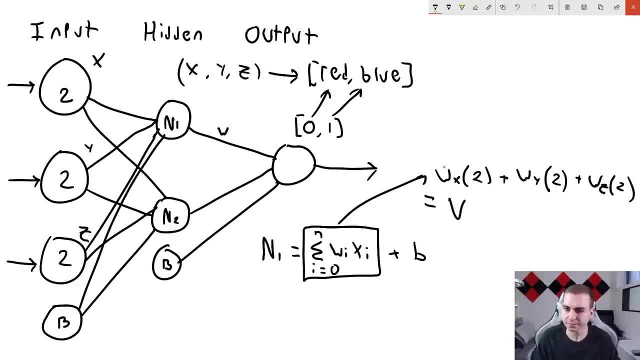 some value, right, some value. let's just call this value v, And that's what this is equal to, So v. then what we do is we add the bias. Now remember, the bias was connected with a weight of one, which means if we take the weighted sum of the bias right, all we're. 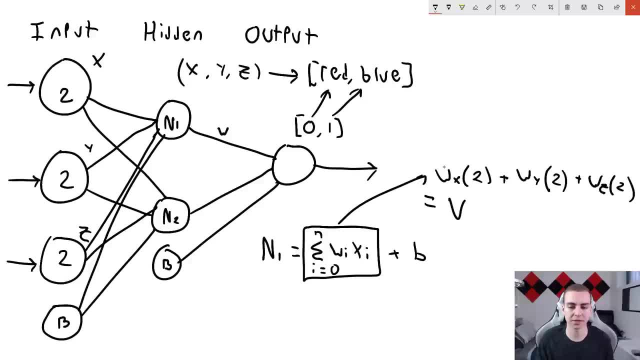 doing is adding whatever that biases value was. So if this bias value was 100, then what we do is we add 100.. Now I've just written the plus b to explicitly state the fact that we're adding the bias, although it could really be considered as a part of the summation equation. 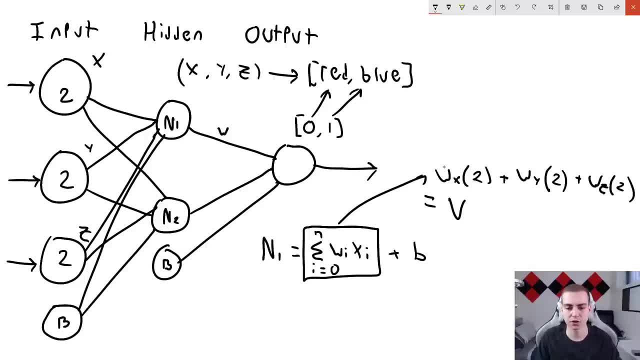 because it's another connection to the neural. Now let's just talk about what this symbol means for anyone that's confused about that. Essentially, this stands for some: I stands for an index and M stands for what index will go up to now and means how many. 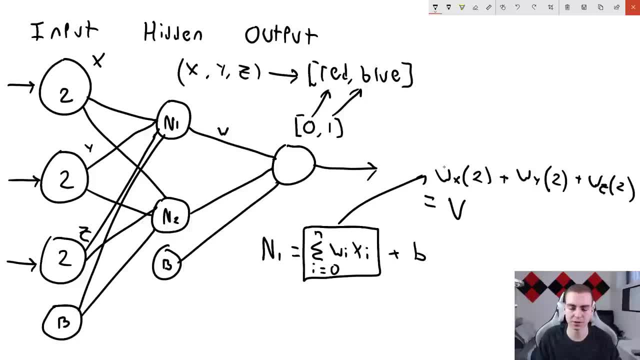 neurons we had in the previous layer. And then what we're doing here, saying wi x i. so we're gonna say weight zero x zero, plus weight one x one plus weight two x two. it's almost like a four loop. we're just adding them all together And then we add the B. 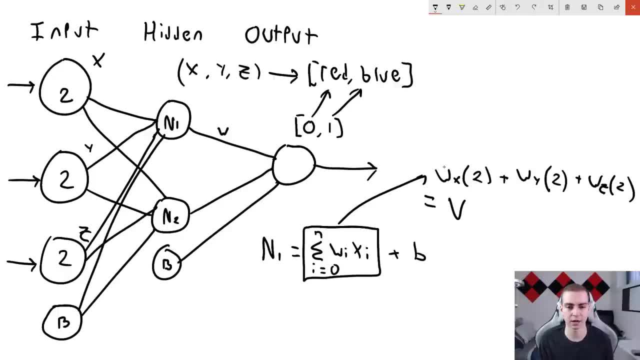 And I hope that makes enough sense so that we understand that. so that is our weighted sum and our bias. So essentially what we do is we go through and we calculate these values. So this gets some value. Speaker 1. this value is like 0.3, maybe this value seven, whatever it is, and we do the same thing now. 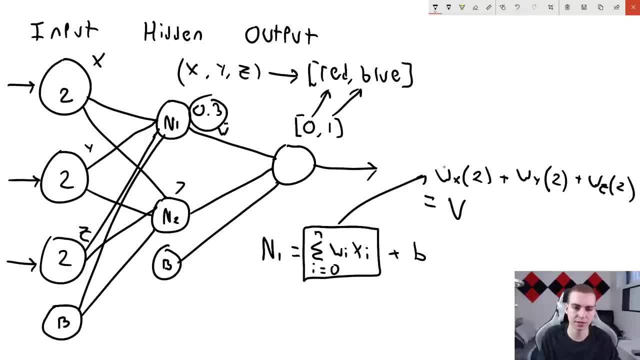 at our output neuron. So we take the weighted sum of this value times its weight. And then we take the weighted sum So this value times its weight plus the bias. this is given some value here And then we can look at that value and determine what the output of our neural 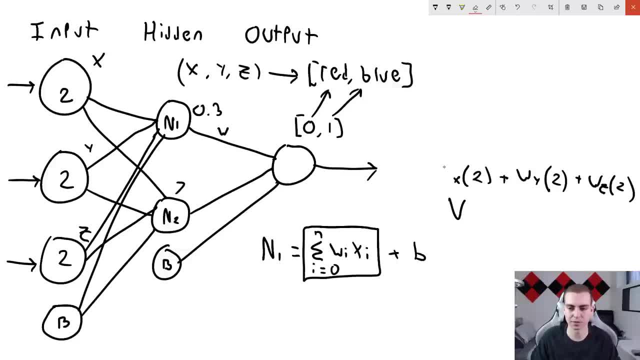 network is. So that is pretty much how that works in terms of the weighted sums, the weights and the biases. Now let's talk about the kind of the training process and another thing called an activation function. So I've lied to a little bit because I've said I'm just 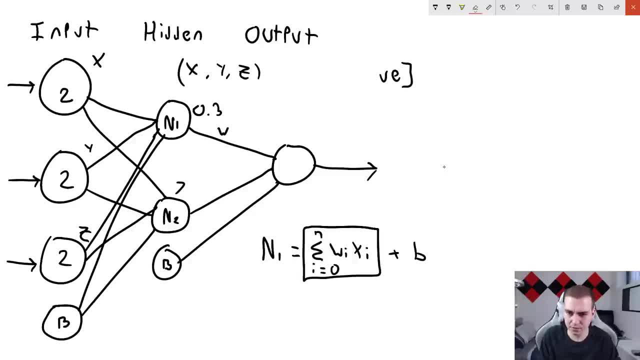 going to start erasing some stuff, So we have a little bit more room on here. So I've lied to you And I've said that this is completely how this works. Well, we're missing one key feature that I want to talk about, which is called an activation function. Now, remember, 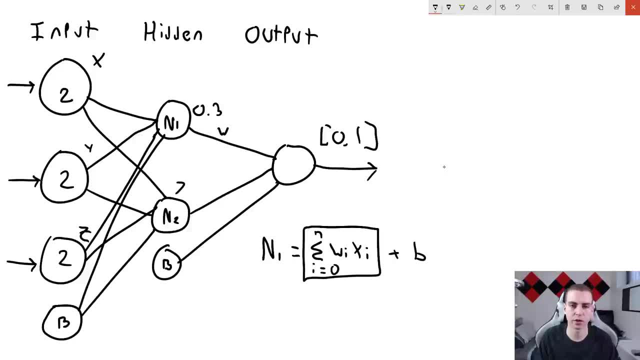 how we want this value to be in between zero and one right at our output layer. Well, right now we can't really guarantee that that's going to happen. I mean especially for starting with random weights and random biases in our neural network and we're passing this information. 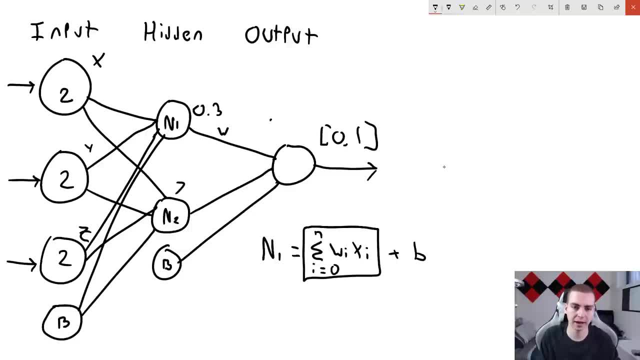 through. we could get to this point here: we could have like 700 as our value. That's kind of crazy to me, right? We have this huge value. how do we look at 700 and determine whether this is red or whether this is blue? Well, we can use something called an activation. 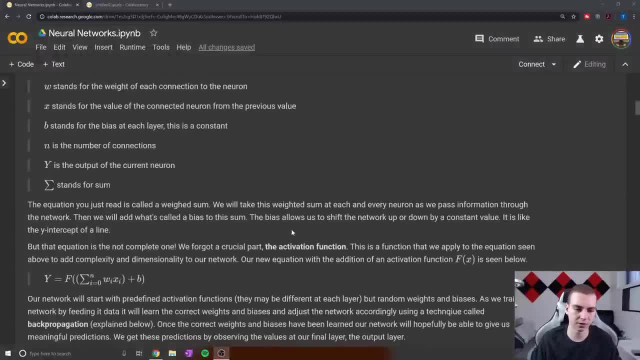 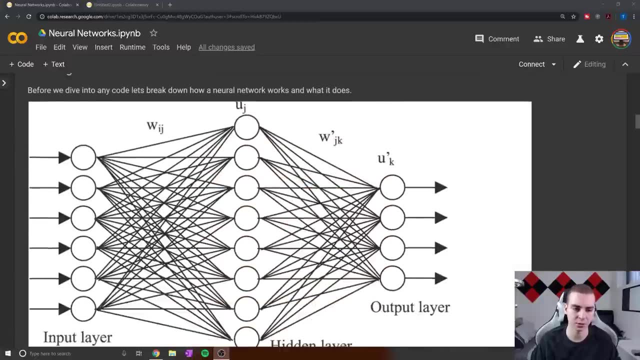 function. Now I'm going to go back to my slides here- whatever we want to call this, this notebook, just to talk about what an activation function is And you guys can see here. you can follow along. I have all the equations kind of written out here as well. So let's go to activation. 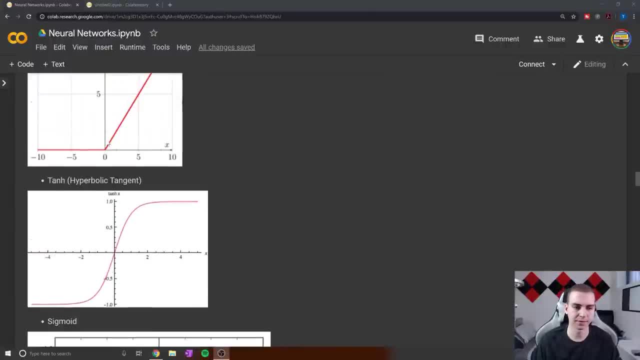 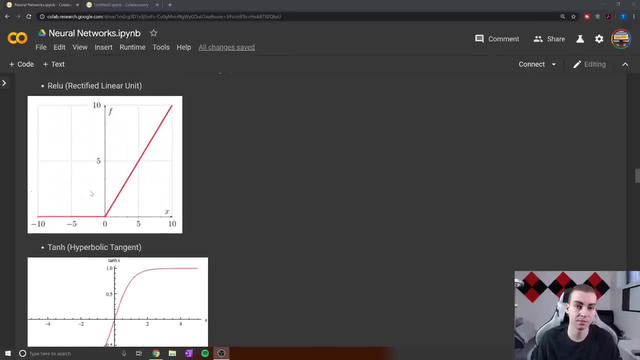 function, which is right here. Okay, So these are some examples of an activation function And I just want you to look at what they do. So this first one is called rectified linear unit. Now notice that essentially, what this activation function does is take any values that are less than zero and just make. 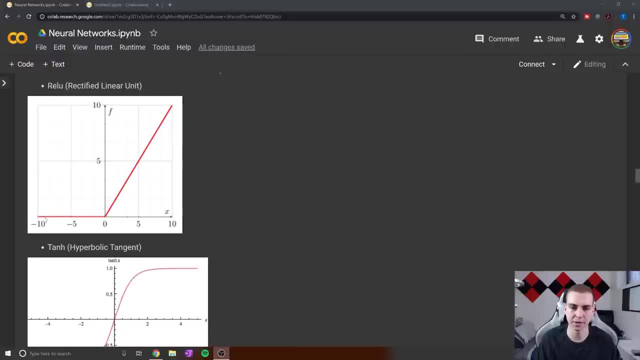 them zero. So any x values that are, you know, in the negative, it just makes their y zero. And then any values that are positive, it's just equal to whatever their positive value is. So if it's 10, it's 10.. This allows us to just pretty much eliminate any negative. 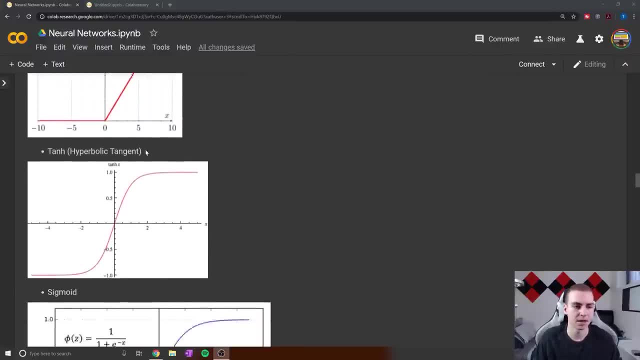 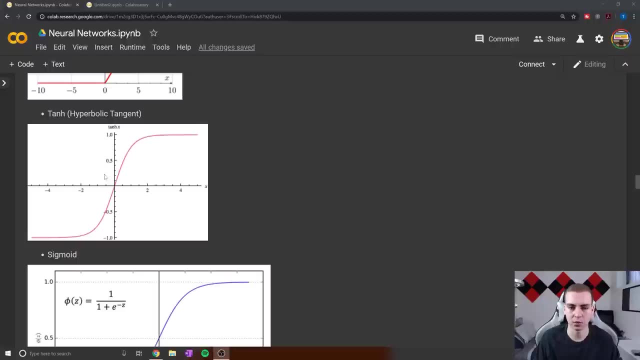 numbers. right? That's kind of what we're rectified. linear unit does Now tan h or hyperbolic tangent. what does this do? This actually squishes our values between negative one and one, So it takes whatever values we have and the more positive. 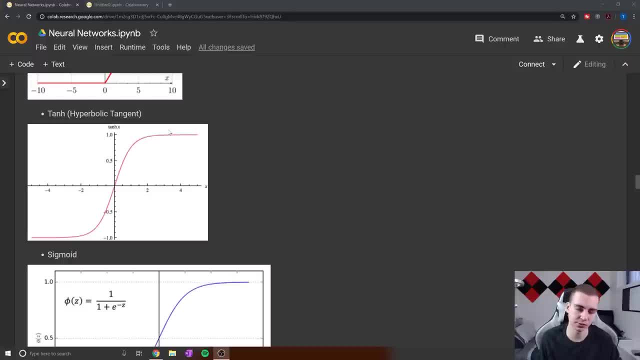 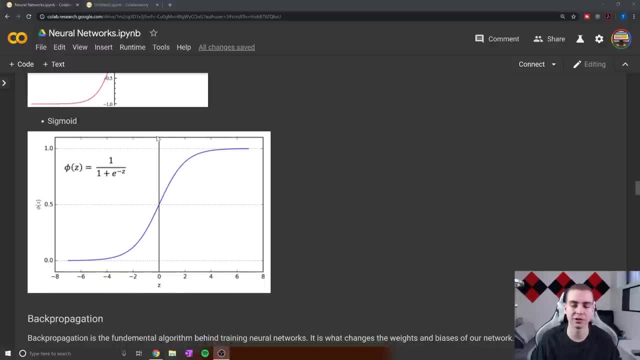 they are. the closer to one they are, the more negative they are, the closer to negative one they are. So can we see why this might be useful right for our neural network? And then last one is sigmoid. What this does is squish our values between zero and one a. 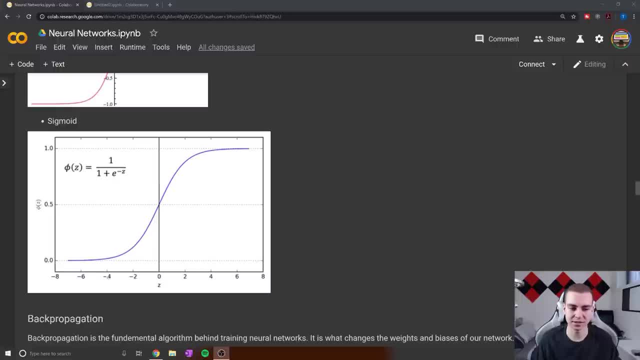 lot of people call it like the squish fire function, because all it does is take any extremely negative numbers and put them closer to zero, And any extremely positive numbers and put them close to one. any values in between, you're going to get some number that's kind of in between that, based on the equation one. 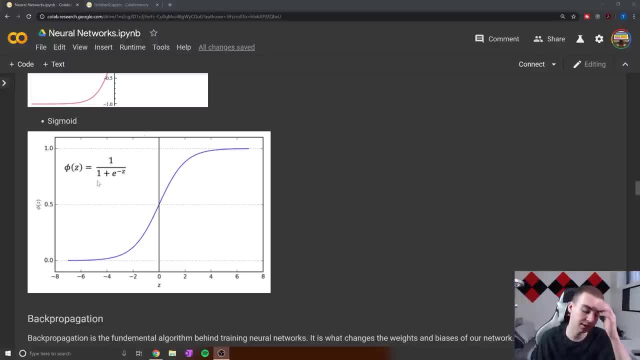 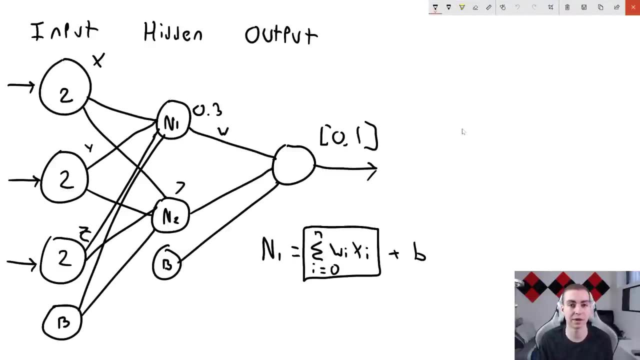 over one plus e to the negative z, And this is theta. z, I guess, is equal to that. Okay, so that's how that works. Those are some activation functions Now. I hope that's not too much math for you, But let's talk about how we use them right. So essentially what we do. 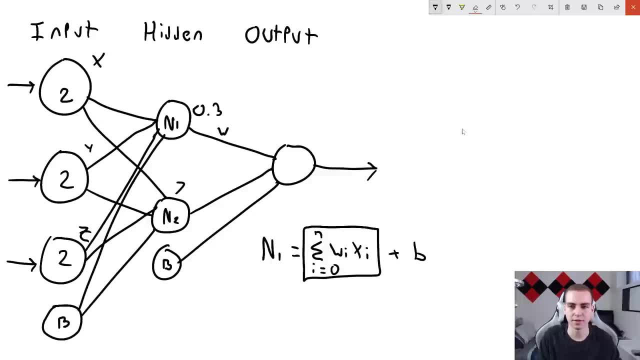 is at each of our neurons, we're going to have an activation function that is applied to the output of that neuron. So we take this, this weighted sum plus the bias, and we're going to have an activation function, And then we apply an activation function to it. 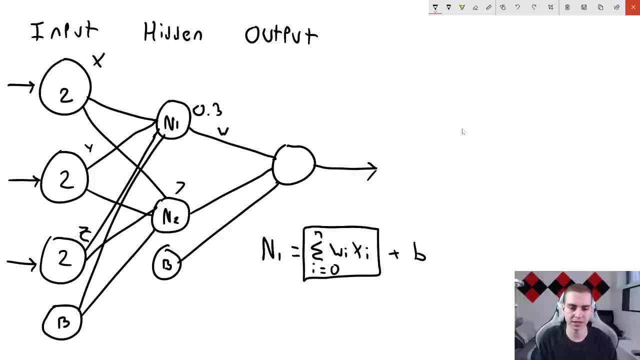 before we send that value to the next neuron. So in this case, n one isn't actually just equal to this. what n one is equal to is n one is equal to f, which stands for our activation function of this equation. right? So say, i equals zero, wi, x, i plus b, And that's what. 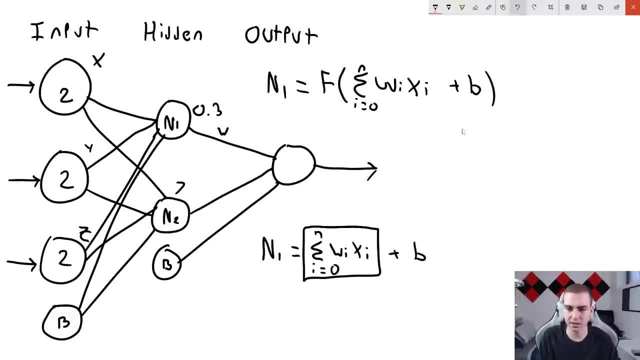 n one's value is equal to when it comes to this output neuron. So each of these have an activation function on them, And two has the same activation function as n one, And we can define what activation function we want to apply at each neuron, Now at our output. 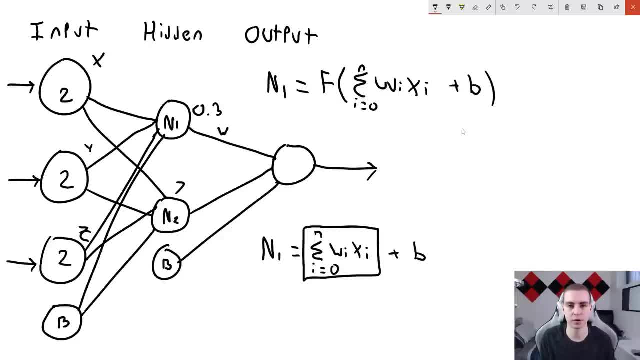 neuron. the activation function is very important because we need to determine what we want our value to look like. do we want it between negative one to one? do we want it between zero and one, Or do we want it to be some massively large number? Do we want it between? 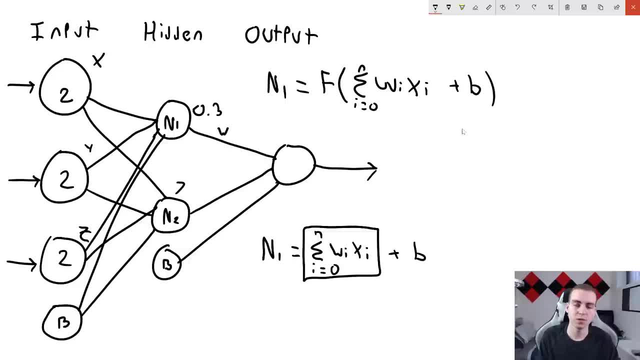 zero and positive infinity. What do we want, right? So what we do is we pick some activation function for our output neuron And, based on what I said, we want our values between zero and one. I'm going to be picking the sigmoid function. 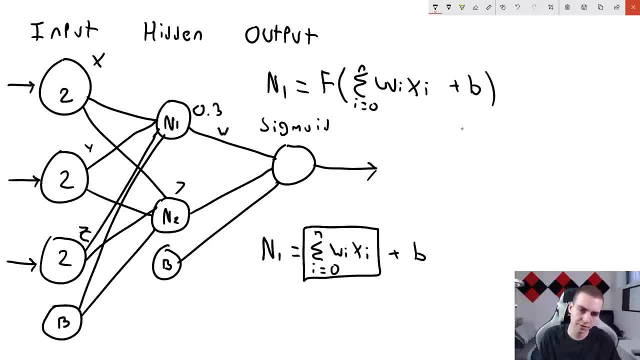 So sigmoid recall squishes our values between zero and one. So what we'll do here is we'll take n, one right, So n one times, whatever the weight is there, So weight zero plus n, two times weight one plus a bias, and apply sigmoid, And then this will give us some value. 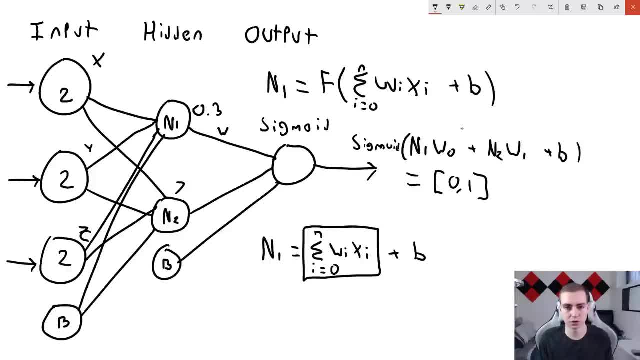 between zero and one. Then we can look at that value And we can determine what the output of this network is. So that's great And that makes sense why we would use that on the output neuron right, So we can squish our value in between some kind of value, So we can actually look. 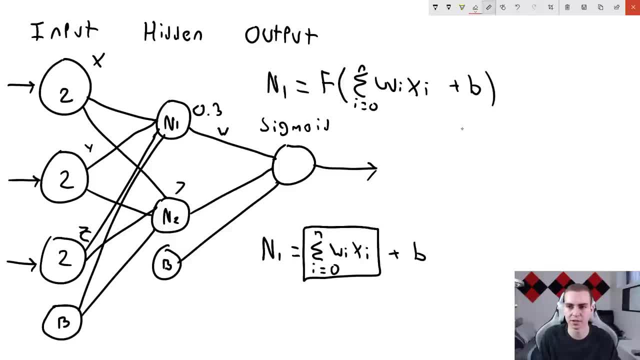 at it and determine you know what to do with it, rather than just having these crazy. and I want to see if I can make this eraser any bigger. Ah, that's much better. Okay, So there we go. Let's just erase some of this. And now let's talk about why we've used the activation. 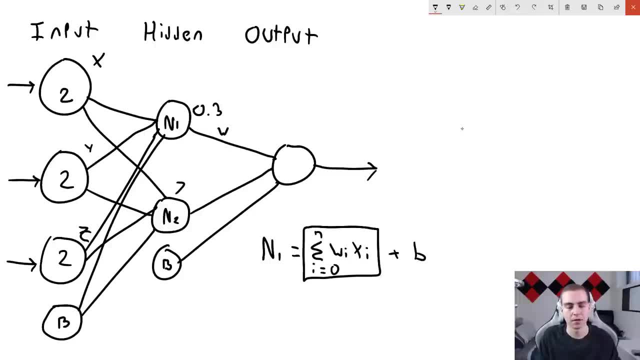 function on like an intermediate layer like this. Well, the whole point of an activation function is to introduce complexity into our neural network. So essentially, you know, we just have these basic weights in these biases And this is kind of just, you know. 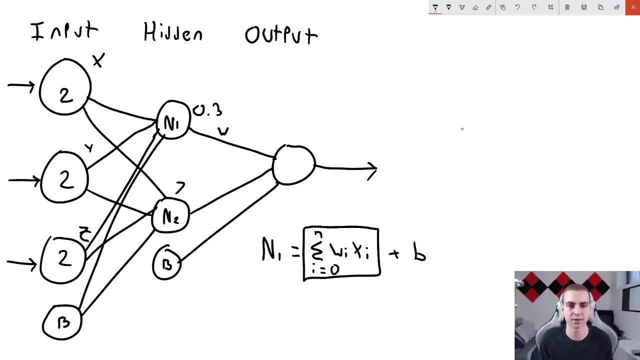 like a complex function At this point. we have a bunch of weights, we have a bunch of biases, And those are the only things that we're training And the only things that we're changing to make our network better. Now, what an activation function can do is, for example, 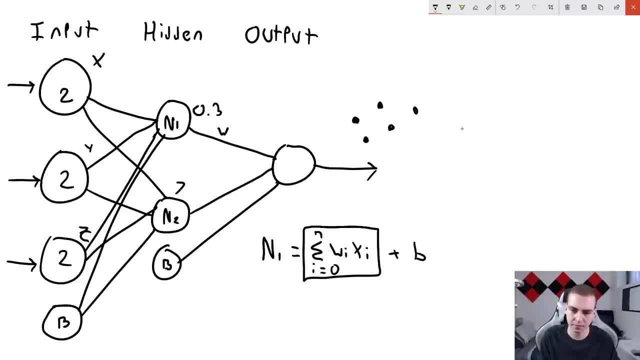 take a bunch of points that are on the same, like plane, right, So let's just say these are in some plane. If we can apply an activation function, function of these where we introduce a higher dimensionality, So an activation function like sigmoid, that is, like a higher dimension function, we can hopefully spread these points. 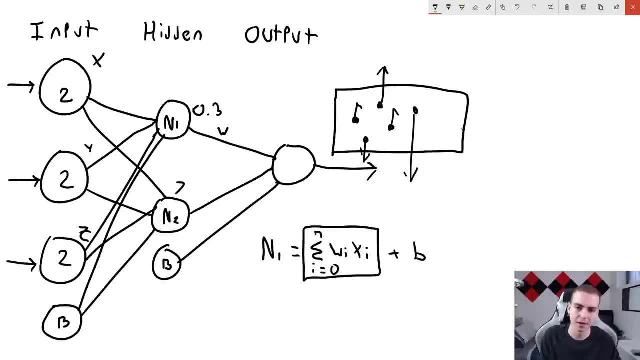 out and move them up or down off the plane In hopes of extracting kind of some different features. Now it's hard to explain this until we get into the training process of the neural network, But I'm hoping this is maybe giving you a little bit of idea, if we can introduce. 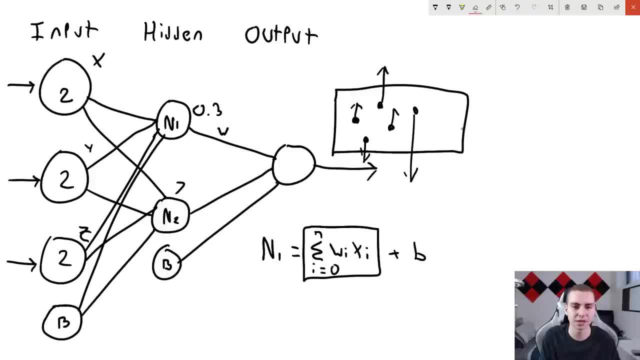 a complex activation function into this kind of process, then it allows us to make some more complex predictions. we can pick up on some different patterns. If I can see that you know, one sigmoid or rectify linear unit is applied to this output. it moves my point up or moves it down or moves. 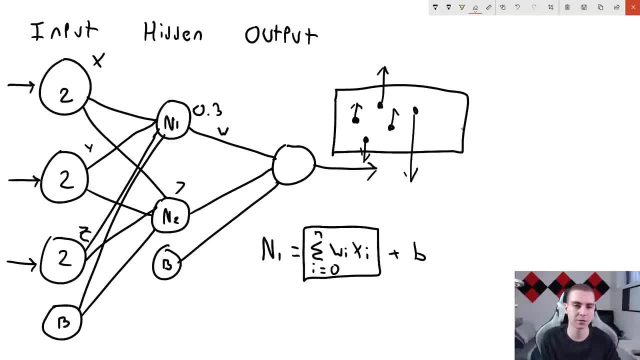 it in like whatever direction and dimensional space. then I can determine specific patterns I couldn't determine in the previous dimension. That's just like if we're looking at something in two dimensions, if I can move that into three dimensions, I immediately see more detail. 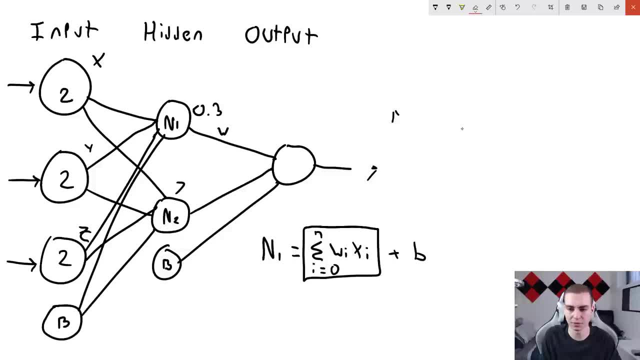 there's more things that I can look at right And I'll try to do a good example of why we might use it like this. So let's say, we have a square right like this right, And I asked you, I'm like tell me some information about this square. Well, 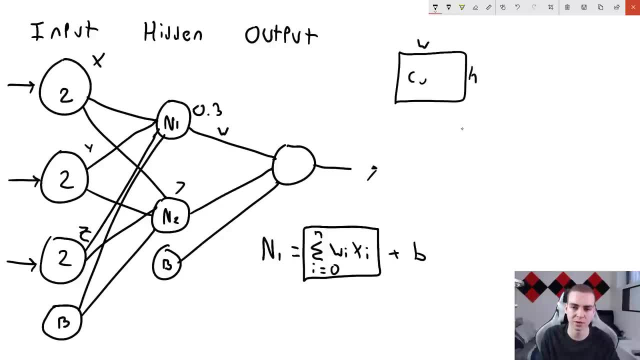 what you can tell me immediately is: you can tell me the width, you can tell me the height and I guess you could tell me the color. right, You can tell me it has one face, you can tell me it has four vertexes and tell me a fair amount about the square. you can tell me its. 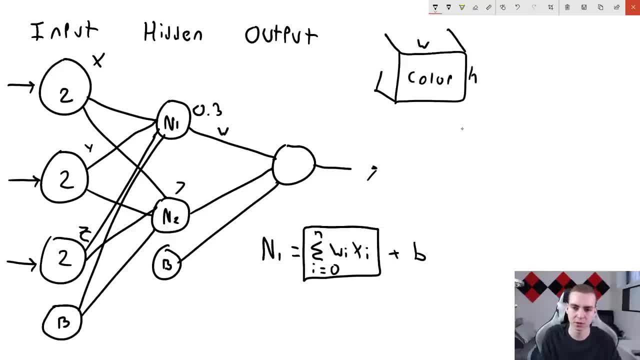 area. Now, what happens as soon as I extend the square and I make it into a cube? Well, now you can immediately tell me a lot more information. you can tell me you know the height or, I guess, the depth with height, depth. 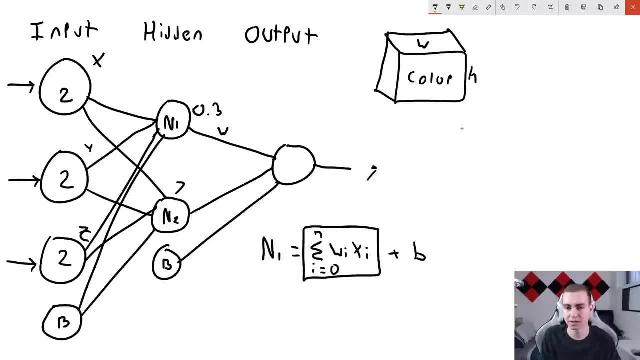 Yeah, whatever you want to call it there. You can tell me how many faces it has. you can tell me what color each of the faces are. you can tell me how many vertexes, you can tell me if this cube or the square, this rectangle, is uniform or not, And you can pick up on. 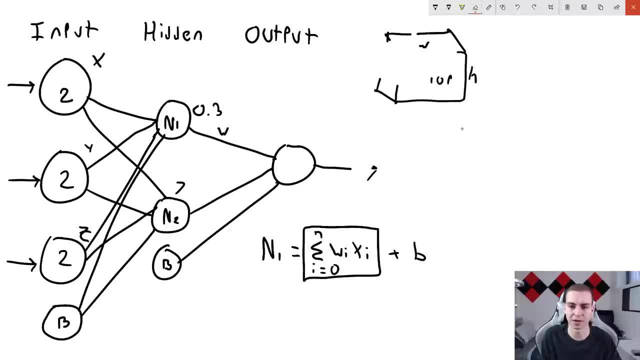 a lot more information. So that's kind of- I mean, this is a very oversimplification of what this actually does, But this is kind of the concept. right is that if we are in two dimensions, if we can somehow move our data points into a higher dimension by applying 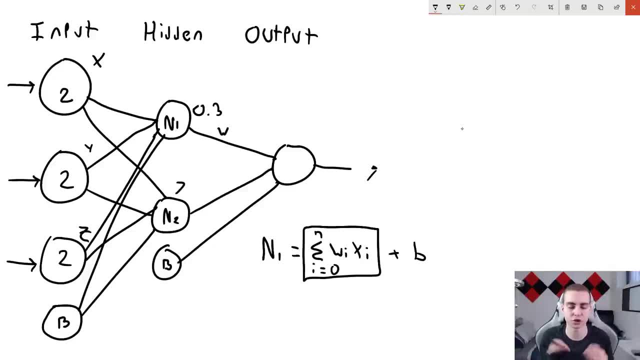 some function to them, then what we can do is get more information and extract more and get more information about the data points, which will lead to better predictions. Okay, so, now that we've talked about all this, it's time to talk about how neural networks train. 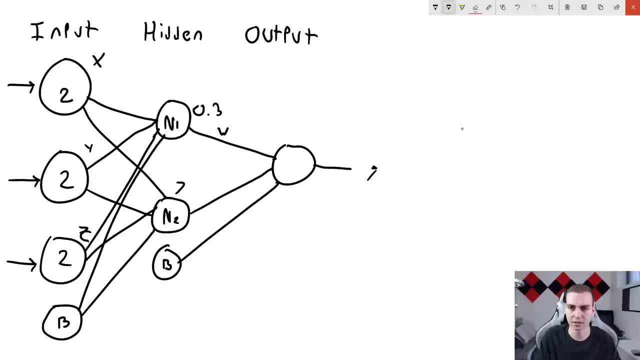 And I think you guys are ready for this. This is a little bit more complicated, But again, it's not that crazy. Alright, so we talked about these weights and biases, And these weights and biases are what our network will come up with and determine to you know like. 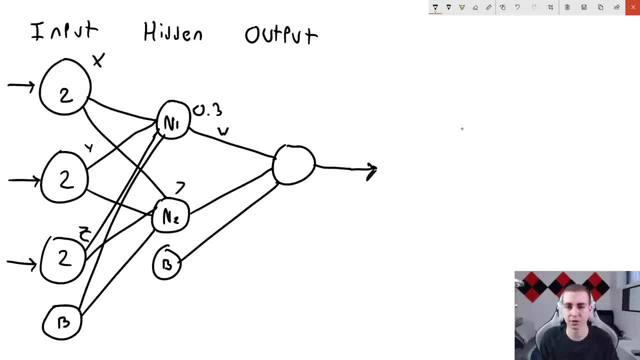 make the network better. So, essentially, what we're going to do now is talk about something called a loss function. So, as our network starts right, the way that we train it, just like we've trained it, we're going to train it in a different way. We're going to train. 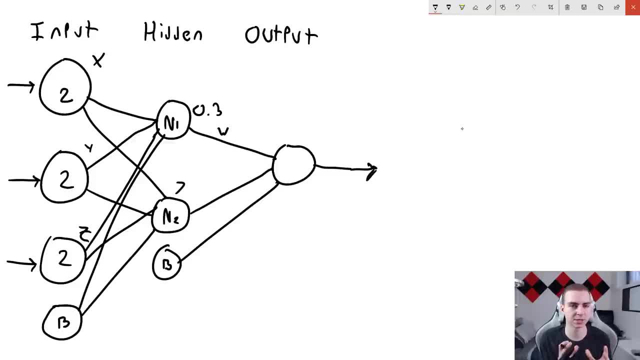 it in a different way while you're changing it. But essentially, what we're gonna do is just take our model and we're going to give it some information. Now what we're gonna do is train other networks or other machine learning models. is we give it some information. 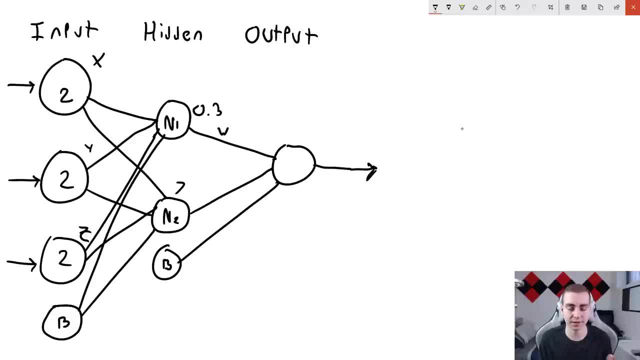 we give it what the expected output is and then we just see what the expected output or what the output was from the network, compare it to the expected output and modify it like that. So essentially what we start with is we say okay, two, two, two. we say this: 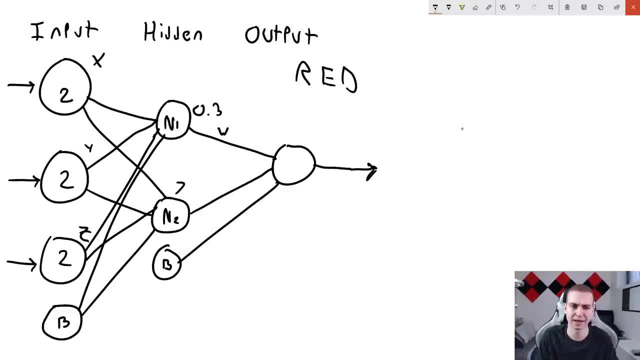 class is red, which I forget what I labeled that was as, but let's just say, like that was a zero. okay, So this class is zero. So I want this network to give me a zero for the point 222.. 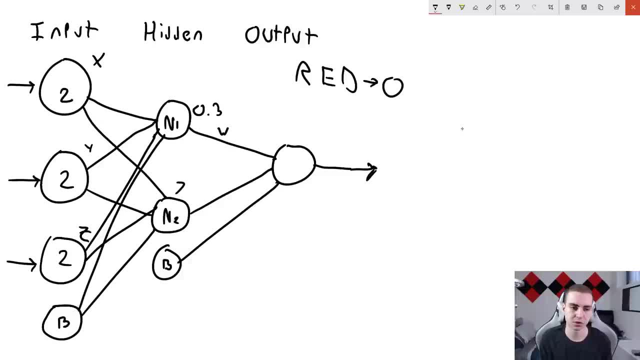 network starts with completely random weights and completely random biases. So chances are when we get to this output here, we're not going to get zero. maybe we get some value after applying the sigmoid function. that's like 0.7.. Well, this is pretty far away from. 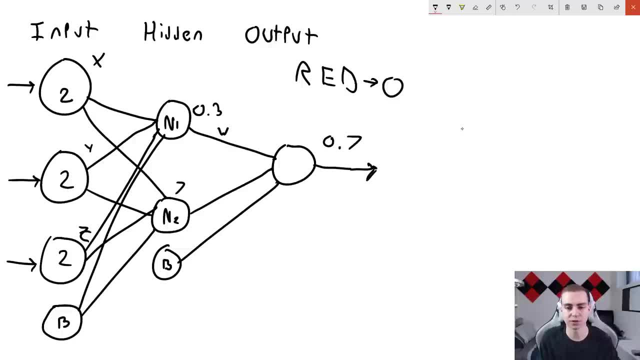 red. But how far away is it? Well, this is where we use something called loss function. Now, what a loss function does is calculate how far away our output was from our expected output. So if our expected output is zero and our output was, your point seven, the loss, 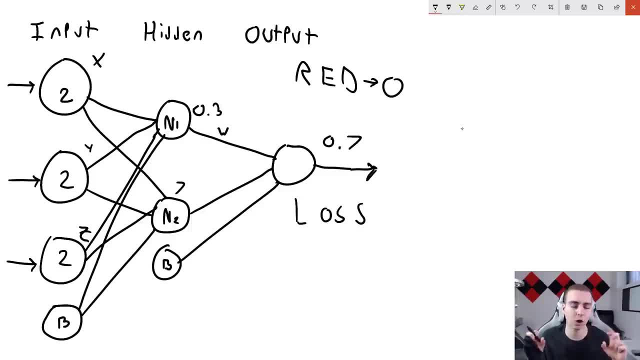 function is going to give us some value. that represents like how bad or how good this network was. Now, if it tells us this network was really bad, it gives us like a really high loss. then that tells us that we need to tweak the weights and biases more and move the network. 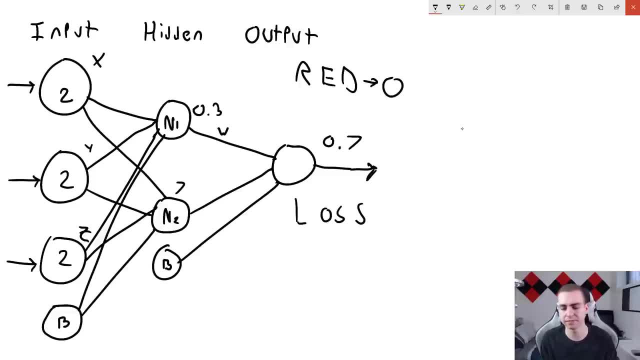 in a different direction. We're starting to get into gradient descent. But let's understand the loss function first. So it's going to say: if it was really bad, let's move it more, let's change the weights more drastically, So let's move it more, let's change the weights more drastically, So let's move it more drastically. 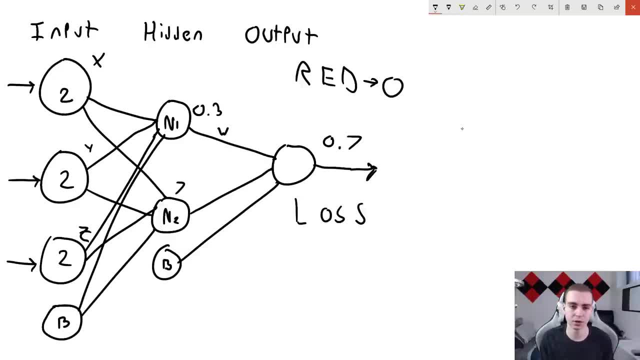 Let's change the biases more drastically, Whereas if it was really good, it'll be like: okay, so that one was actually decent. you know, you only need to tweak a little bit, and you only need to move this, this and this. So that's good And that's the point of this. 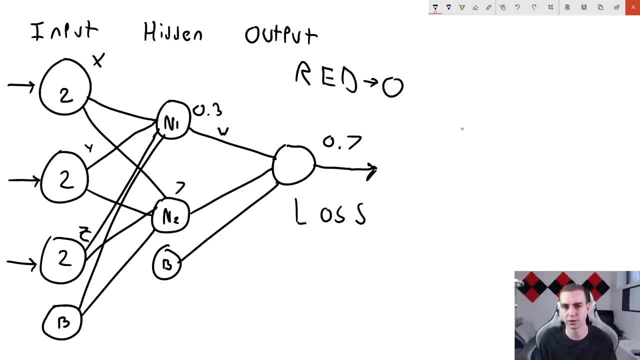 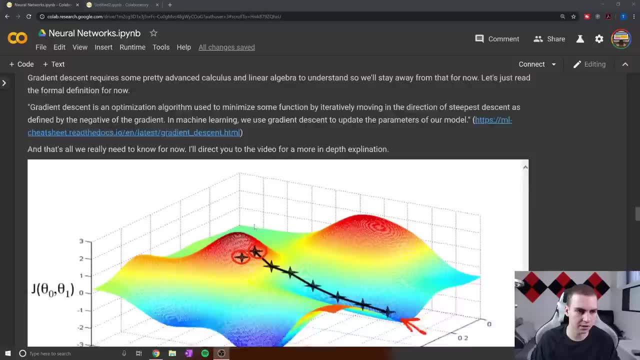 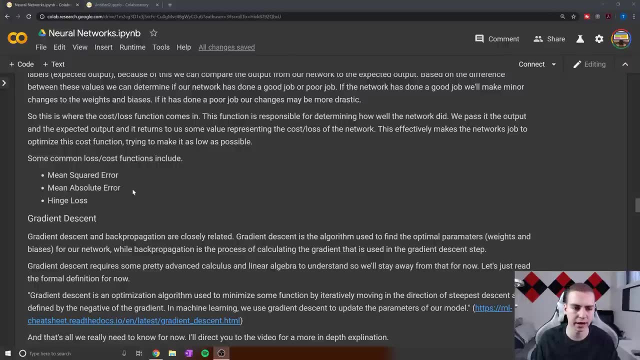 loss function. you just calculate some value. the higher the value, the worse. our network was a few examples of loss function. Let's go down here because I think I had a few optimizer. loss here mean squared error, mean absolute error and hinge loss Now mean absolute error. 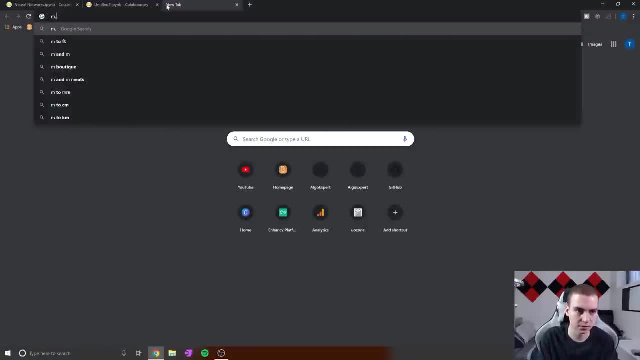 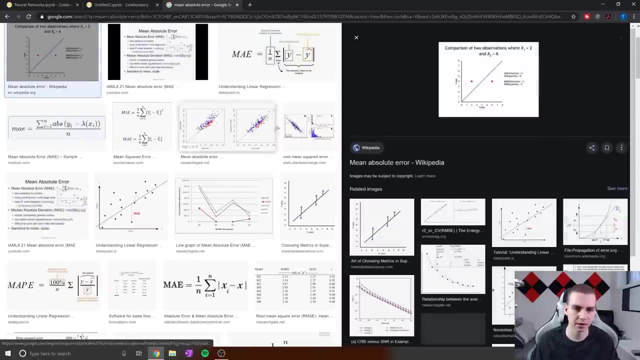 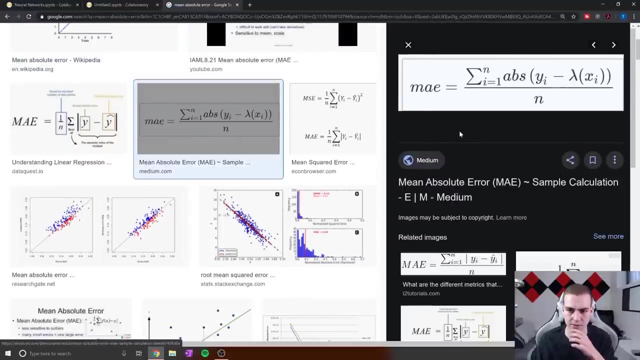 error. You know what? let's actually just look one up here So mean absolute error and have a look at what this is. So images, let's pick something. This is mean absolute error. This is the equation for mean absolute error. Okay, so the summation of the absolute. 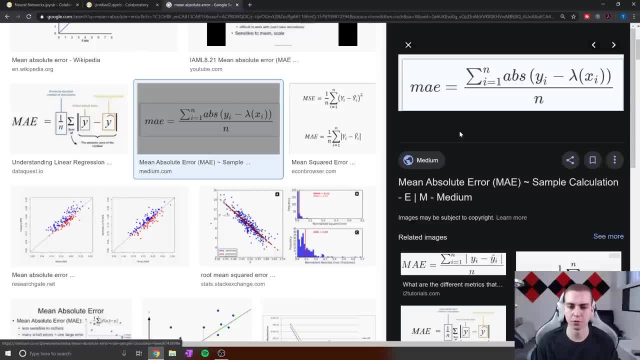 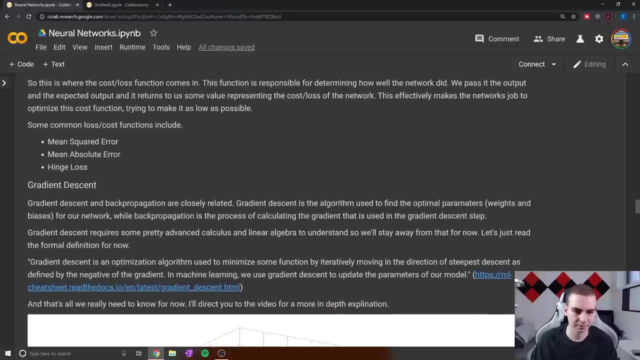 value of y- i minus lambda of x- i over n. Now this is kind of complicated. I'm not going to go into it too much. I was expecting. I was hoping I was going to get like a better example for mean squared error. Okay, so these are the three loss functions here. So 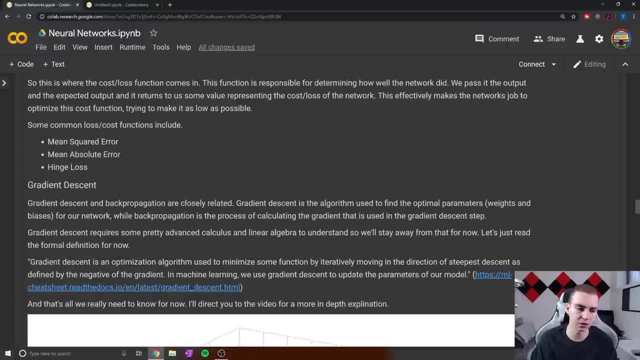 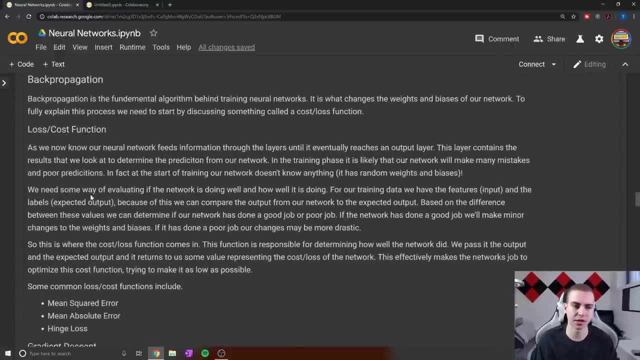 mean squared error, mean absolute error, hinge loss. obviously there's a ton more that we could use. I'm not going to talk about which, how each of these work specifically. I mean, you can look them up pretty easily And also, so you know, these are also referenced as: 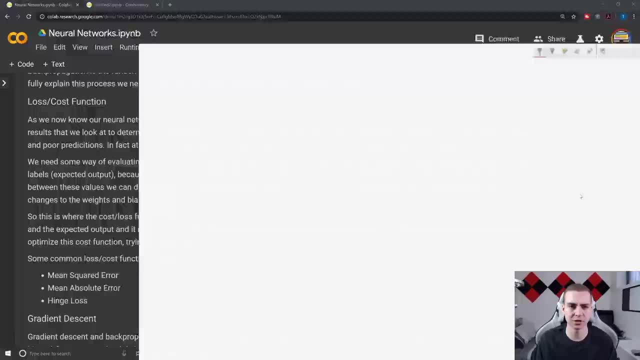 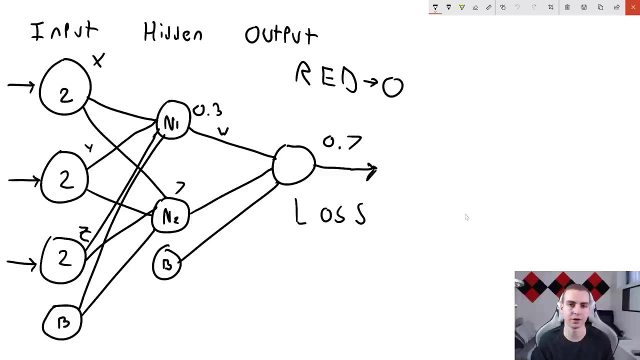 cost functions. So cost or loss- you might just hear these, these terms kind of interchanged- cost and loss essentially mean the same thing: You want your network to cost the least. you want your network to have the least amount of loss. Okay, so now that we have talked about the loss function, we need to talk about 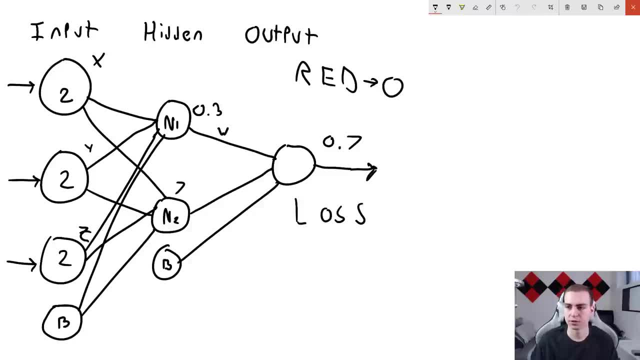 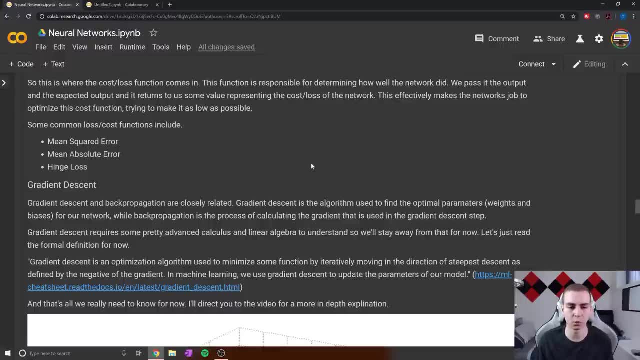 how we actually update these weights and biases. Now, actually, let's go back to here, because I think I had some notes on it. This is what we call gradient descent. So essentially, the parameters for our network are weights and biases, And by changing these weights, 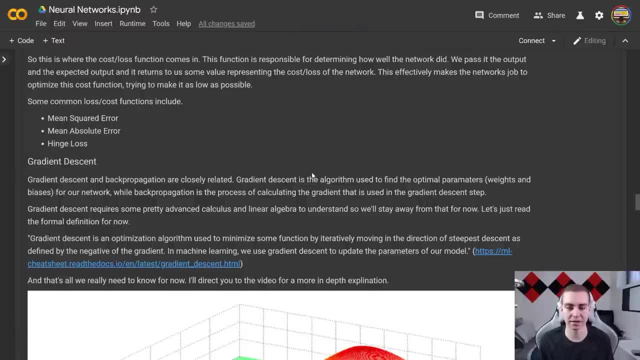 and biases. we will, you know, either make the network better or make the network worse. the loss function will determine if the network is getting better, if it's getting worse, and then we can determine how we're going to move the network to change that. So this is now gradient descent, where the math gets a little bit. 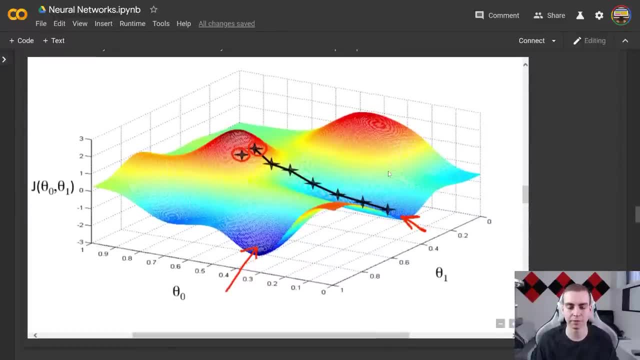 more complicated. So this is an example of what your neural network function might look like. Now, as you have higher dimensional math, you have, you know, a lot more dimensions, a lot more space to explore when it comes to creating different parameters and creating 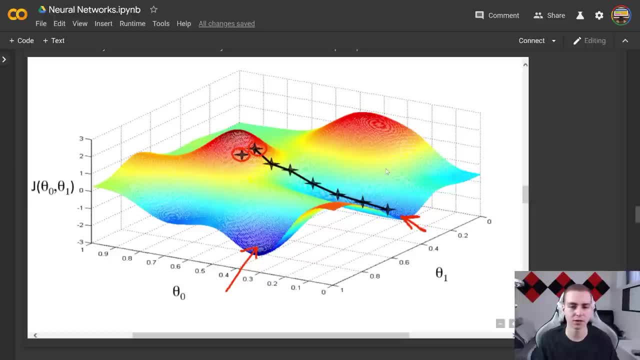 different biases and activation functions and all that. So as we apply our activation functions, we're kind of spreading our network into higher dimensions, which just makes things much more complicated. Now, essentially, what we're trying to do with the neural network is optimized this loss. 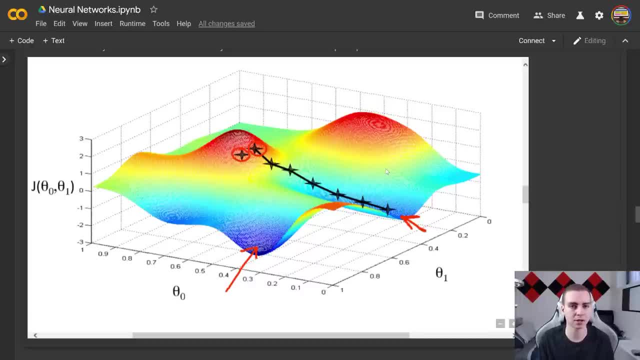 function. this loss function is telling us how good it is or how bad it is. So if we can get this loss function as low as possible, then that means we should technically have the best neural network. So this is our kind of loss functions, like mapping or whatever. 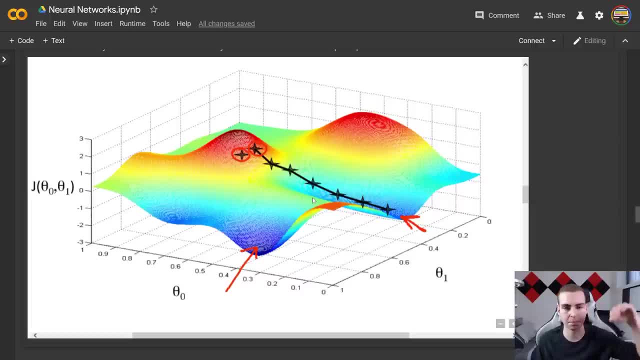 what we're looking for is something called a global minimum. we're looking for the minimum point where we get the least possible loss from our neural network work. So if we start where these red circles are right- and I've just stole this image- 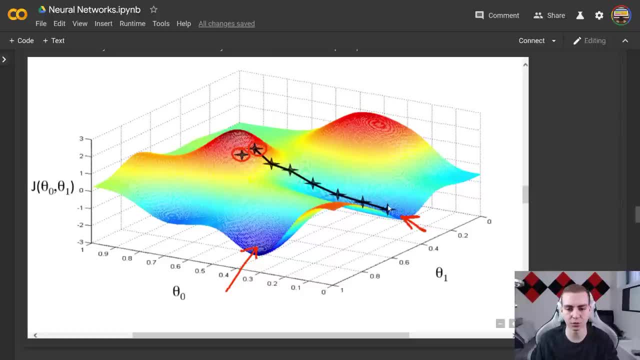 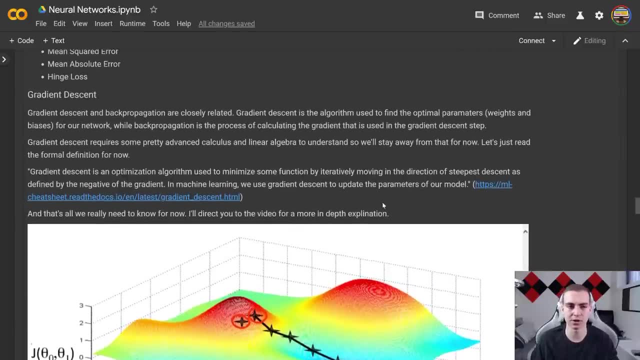 off Google Images. what we're trying to do is move downwards into this global, global minimum, And this is what the process of called gradient descent. So we calculate this loss and we use an algorithm called gradient descent which tells us what direction we need to move. 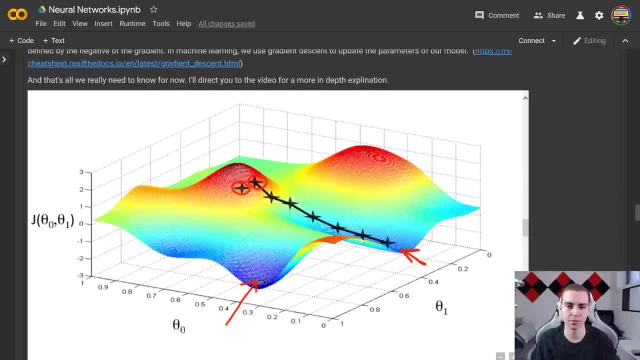 our function to determine or to get to this global minimum. So it essentially looks where we are. It says this was the loss and it says, Okay, I'm going to calculate what's called a gradient, which is literally just a steepness or a direction, And we're going to move in. 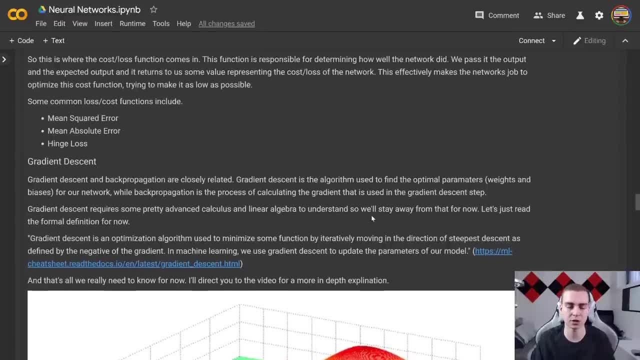 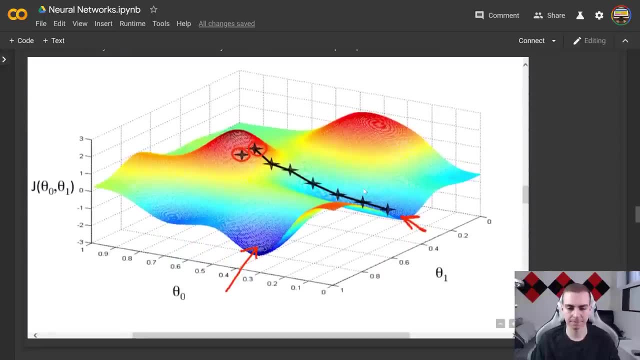 that direction And then the algorithm called brought back propagation will go backwards through the network and update the weights and biases so that we move in that direction. I think this is as far as I really want to go, because I know this is getting more complicated. 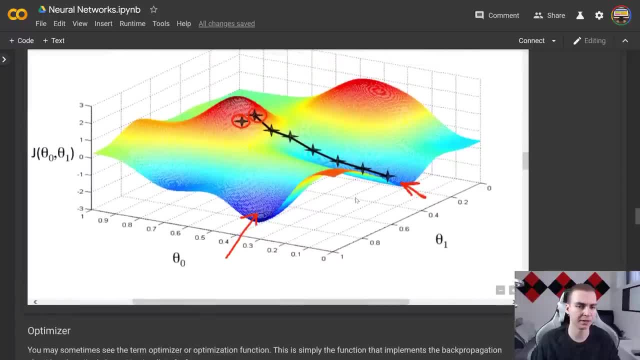 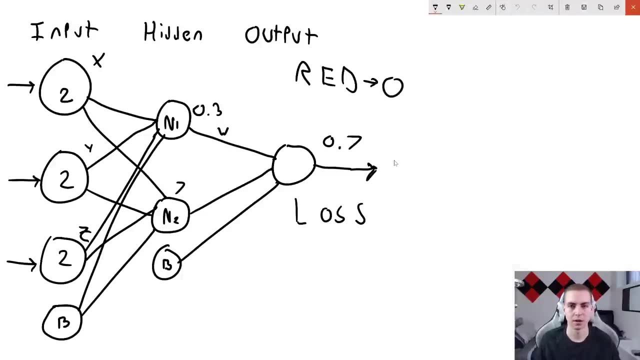 already than some of you guys probably can handle and that I can probably explain. But that's kind of the basic principle. We'll go back to the drawing board And we'll do a very quick recap before we get into some of the other stuff- neural networks, So let's. 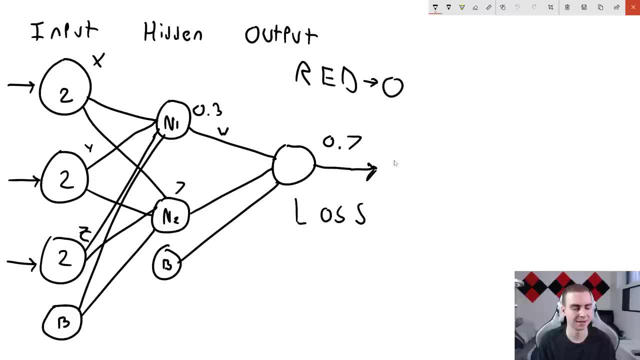 start with input output, hidden layers connected with weights. there's biases that connect to each layer. these biases can be thought of as y intercepts. they'll simply move completely up or move completely down that entire. you know activation function. right, we're shifting. 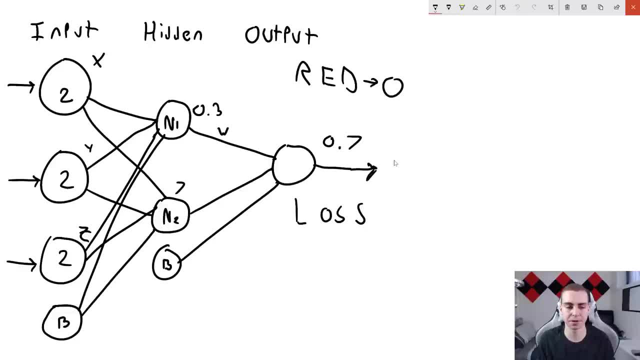 things left or right, because this will allow us to get a better prediction and have another parameter that we can train and add a little bit of complexity to our, you know, neural network model. Now, the way that information is passed through these layers is we take 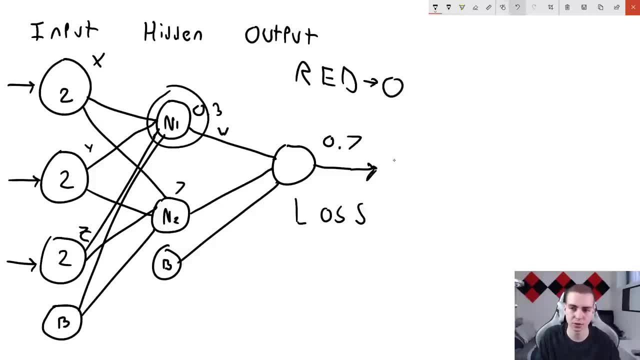 the weighted sum at a neuron of all of the connected neurons to it. we then add this bias neuron and we apply some activation function that's going to put this- you know these values in between two set values. So, for example, when we talk about sigmoid, that's going to. 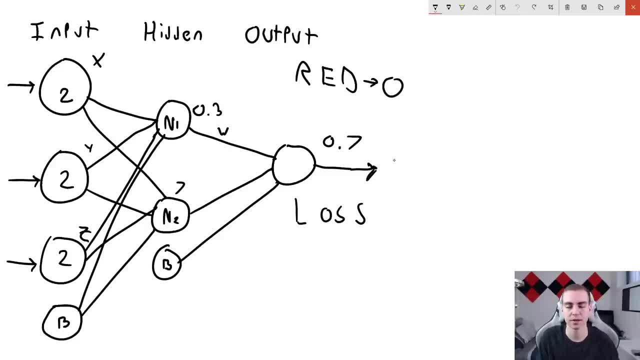 squish our values between zero and one. when we talk about hyperbolic tangent, that's going to squish our values between negative one and one. And when we talk about rectify linear unit, that's going to squish our values between zero and positive infinity. So we apply those. 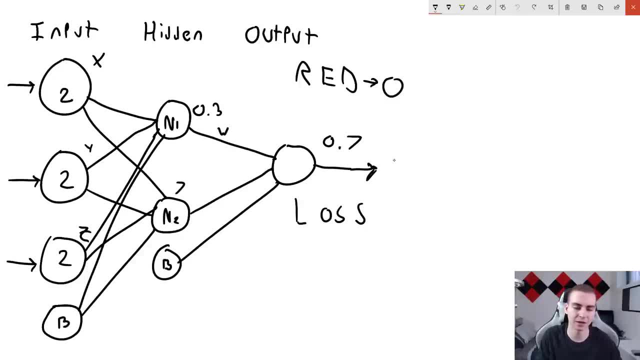 activation functions, and then we continue the process, So n one gets its value and two gets its value, And then, finally, we make our way to our output layer. we might have passed through some other hidden layers before that. And then we do the same thing. we take the weighted sum, we add the bias, we apply an activation. 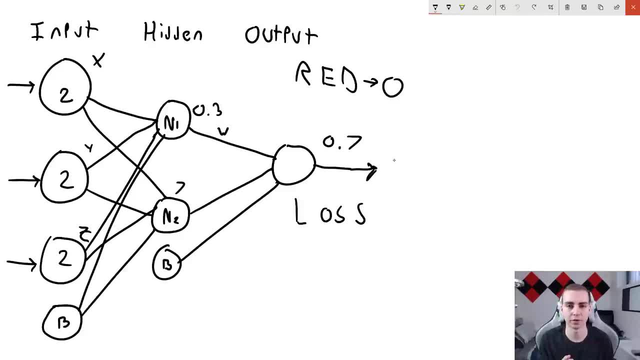 function. we look at the output And we determine whether we know we are class Y or we are class Zed, or whether this is the value we're looking for, And that's how it works. Now we're at the training process, right, So we're doing this now. that's kind of how this worked when. 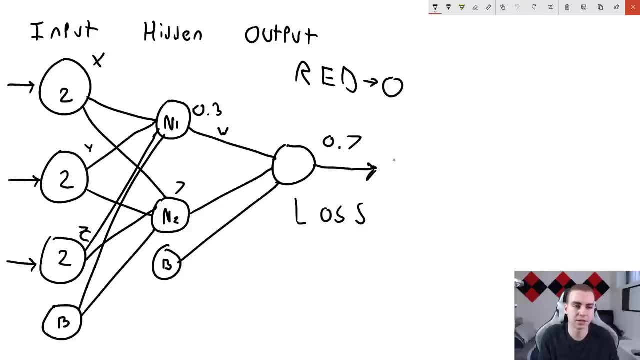 we were making a prediction. So when we're training, Essentially what happens is we just make predictions. we compare those predictions to whatever these expected value should be using this loss function. then we calculate what's called a gradient. a gradient is the direction we need to move to minimize this. 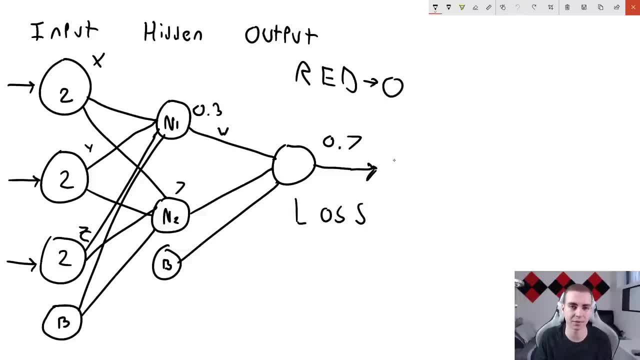 loss function, And this is where the advanced math happens and why I'm kind of skimming over this aspect. And then we use an algorithm called back propagation, where we step backwards through the network and update the weights and biases according to the gradient that. 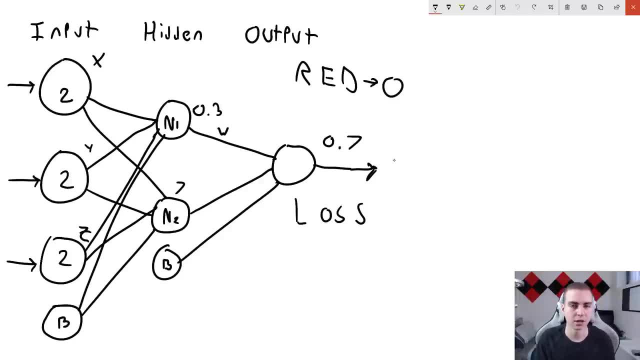 we calculated. Now that is pretty much how this works. So you know, the more info we have, likely, unless we're overfitting. but you know, if we have a lot of data, if we can keep feeding the network, it starts off being really horrible: having no idea what's going on. And then, as 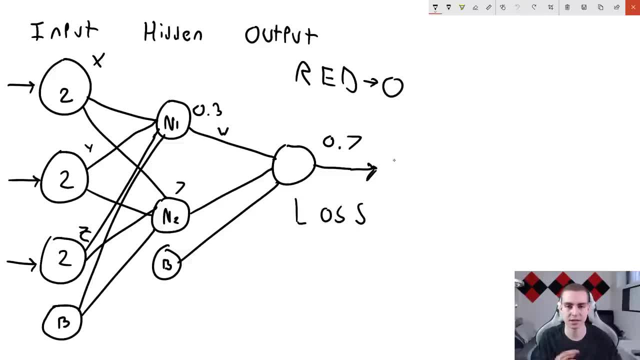 more and more information comes in. it updates these weights and biases, gets better and better, sees more examples And, after you know certain amount of epochs or certain amount of pieces of information, our network is making better and better predictions and having a lower and lower loss. 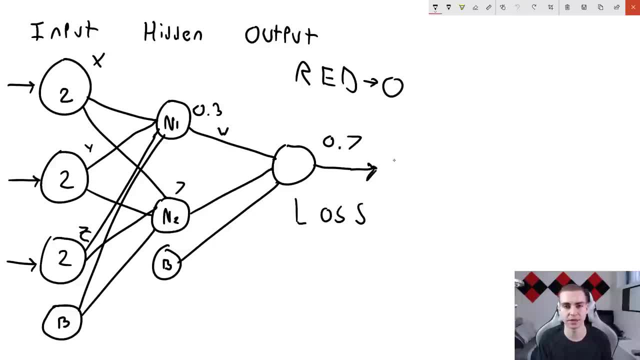 And the way we will calculate how well our network is doing is by passing it. you know our validation data set where it can say: okay, so we got an 85% accuracy on this data set. we're doing okay, you know. 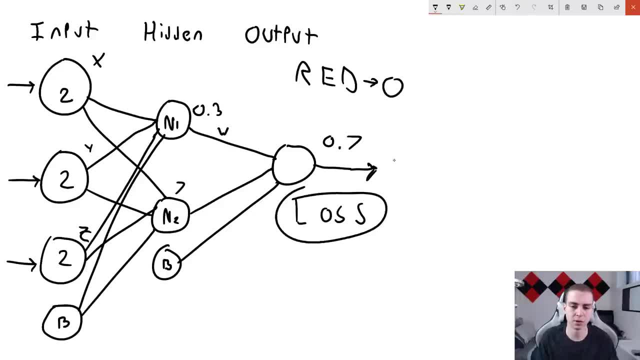 let's tweak this, let's tweak that, let's do this. So the loss function: the lower this is the better, also known as the cost function, And that is kind of neural networks in a nutshell. Now, I know this wasn't really in a nutshell because it was 30 minutes long, But that is. 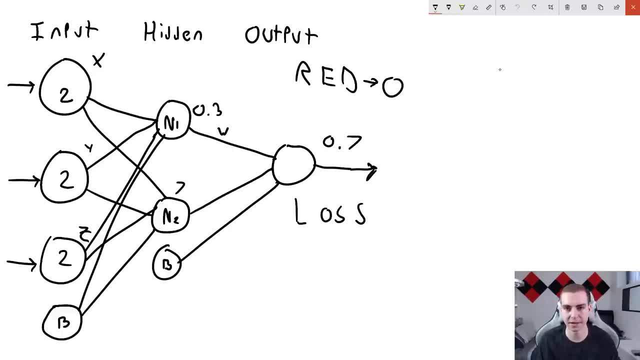 you know as much of an explanation as I can really give you without going too far into the mathematics. And again, remember, the activation function is to move us up in dimensionality. the bias is another layer of complexity and a trainable parameter for our network allows us to shift. 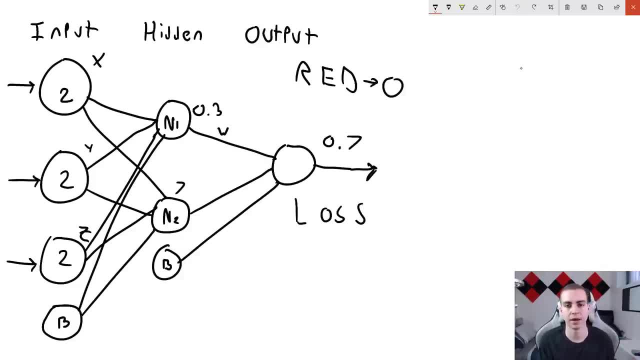 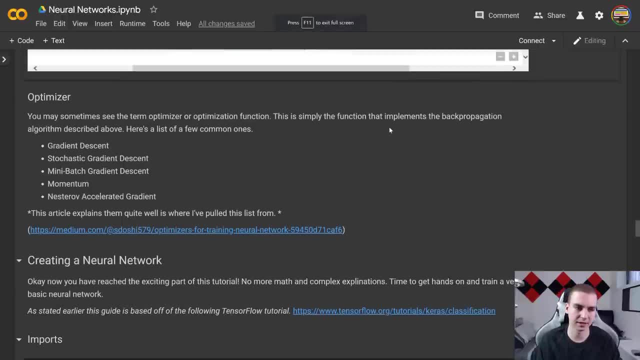 this kind of activation function left, right, up down, And yeah, that is how that works. Okay, so now we have an optimizer. This is kind of the last thing on how neural networks work. Optimizer is literally just the algorithm that does the gradient descent and back propagation. 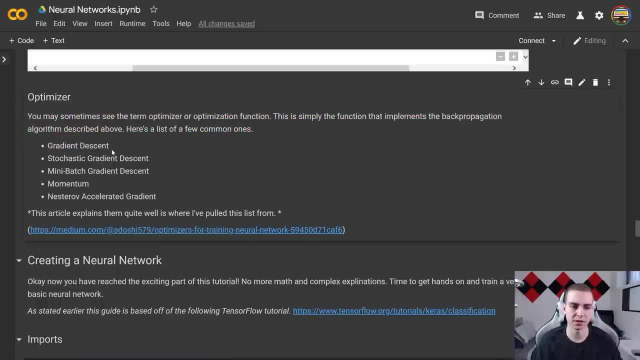 for us. So I mean you guys can read through some of them here. we'll be using, you know, using probably the atom optimizer for most of our examples, although there's, you know, lots of different ones that we can pick from Now the this optimization technique again. 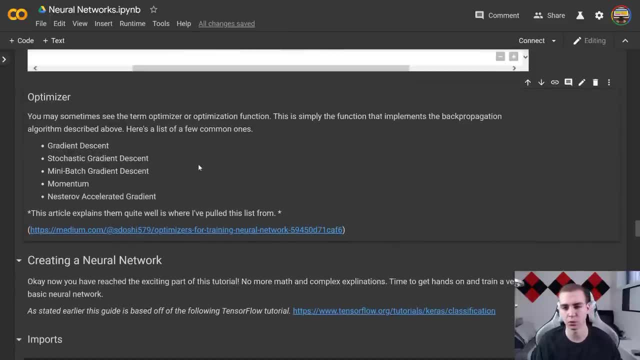 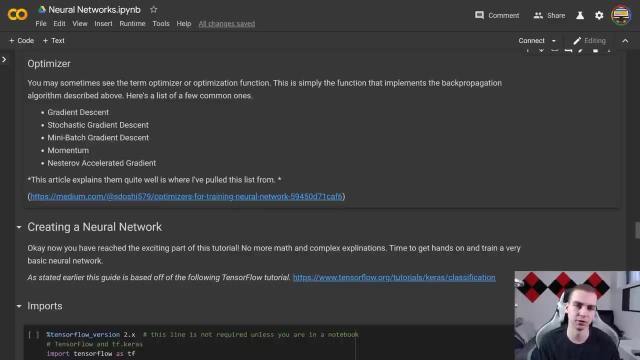 is just a different algorithm there's. some of them are faster, some of them are slower, some of them work a little bit differently And we're not really going to get into picking optimizers in this course, because that's more of an advanced machine learning technique. 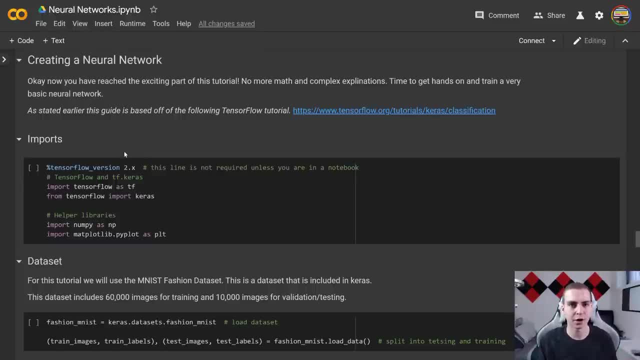 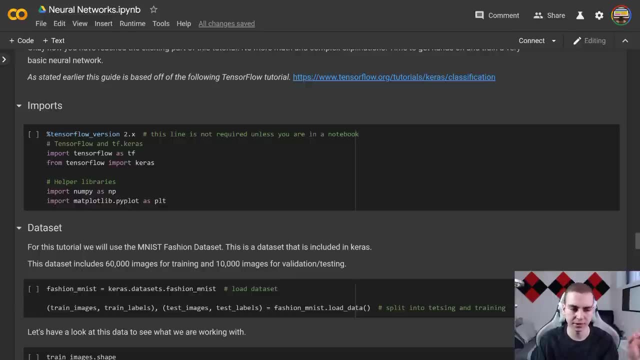 Alright. so enough explaining, enough math, enough drawings, enough talking. now it is time to create our first official neural network. Now these are the imports we're going to need. So import TensorFlow: is TTF from TensorFlow. import Keras again. so this does actually come with TensorFlow. I forget if I said you. 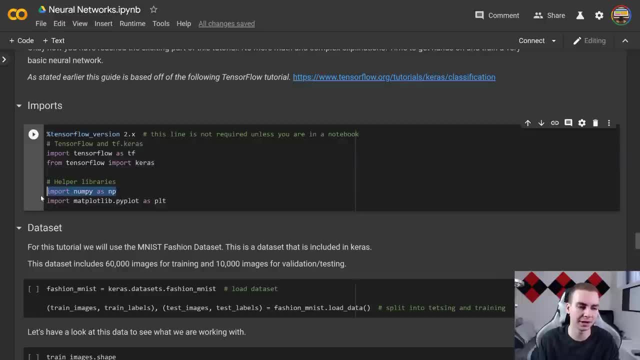 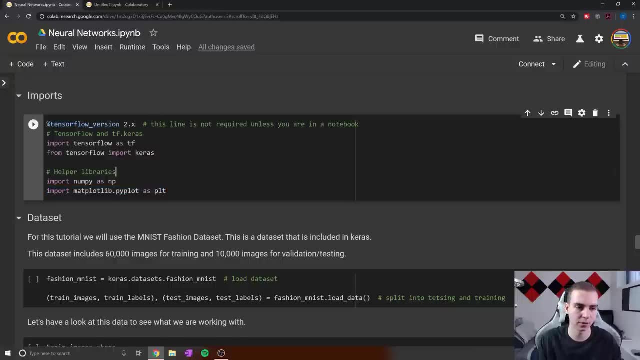 need to install that before, my apologies- and then import NumPy as NP, import matplotlib dot pi plot as PLT. Alright, so I'm going to do actually similar thing to what I did before. I'm kind of just going to copy some of this code into another notebook, just to. 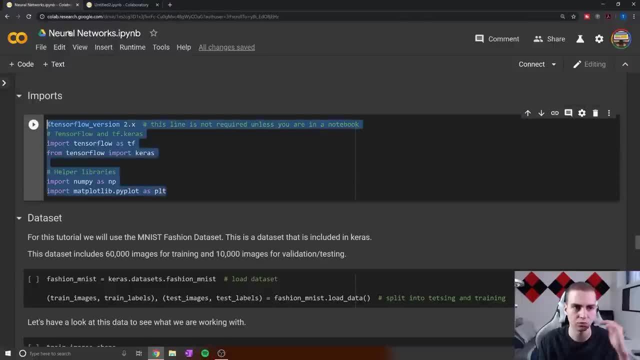 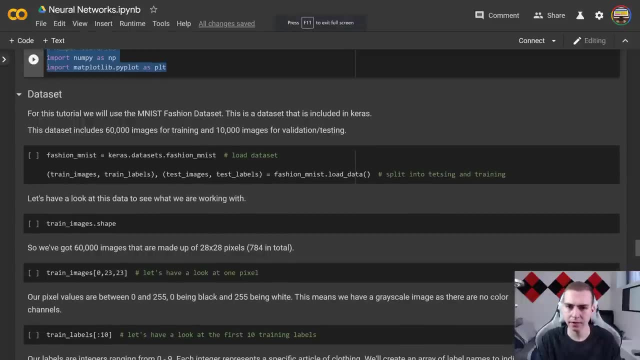 make sure that we can look at everything at the end and then kind of step through the code step by step, rather than all the text kind of happening here. Alright, so the data set and the problem we are going to consider for our first neural 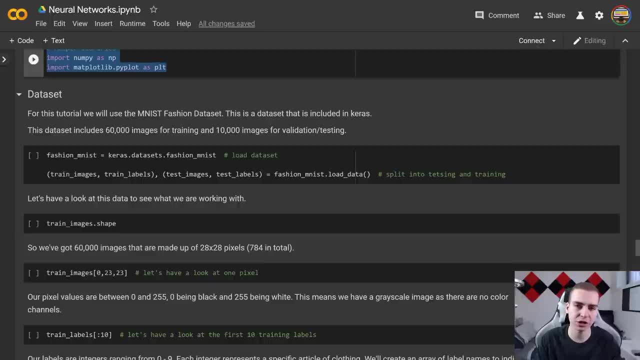 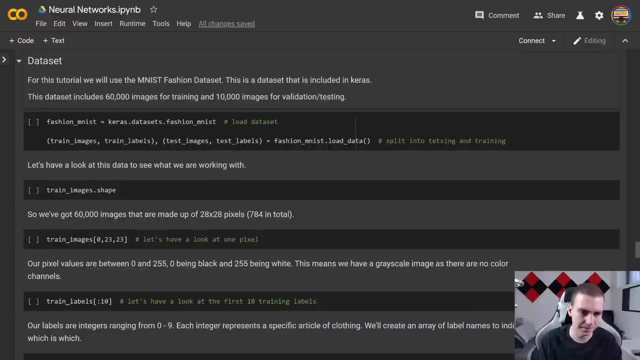 network is the fashion MNIST data set. Now the fashion MNIST data set contains 60,000 images for training and 10,000 images for validating and testing. 70,000 images- And it is essentially pixel data- of clothing articles. So what we're going to do to load in this? 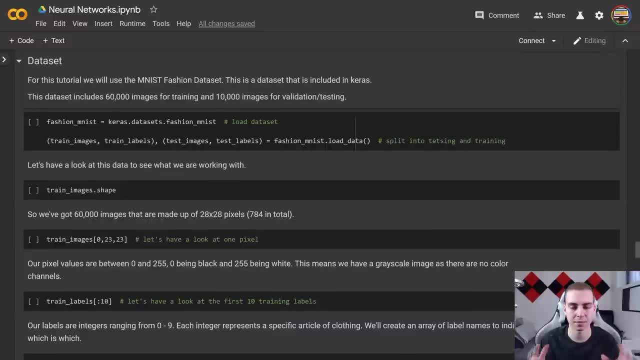 data set from Keras. this actually built into Keras. it's meant as like a beginner, like testing, training, data set. we're going to say fashion underscore MNIST equals Keras dot data sets dot fashion MNIST. Now this will get the data set object and then we can load that object. 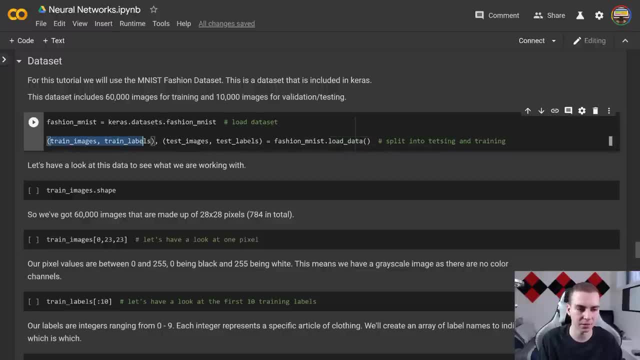 by doing fashion, MNIST, dot load data. Now, by doing this, by having the tuples, train images, train labels, test images, test labels- equals this. this will automatically split our data into the sets that we need. So we need the training and we need the testing. And again, 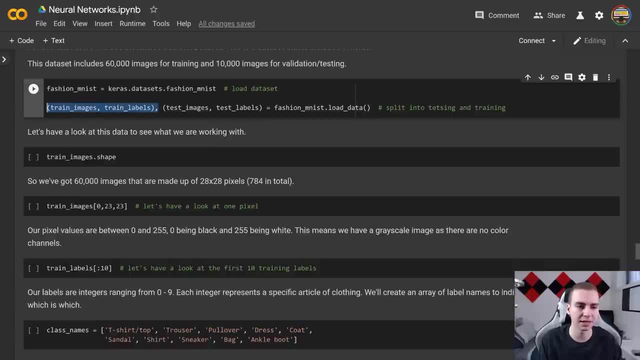 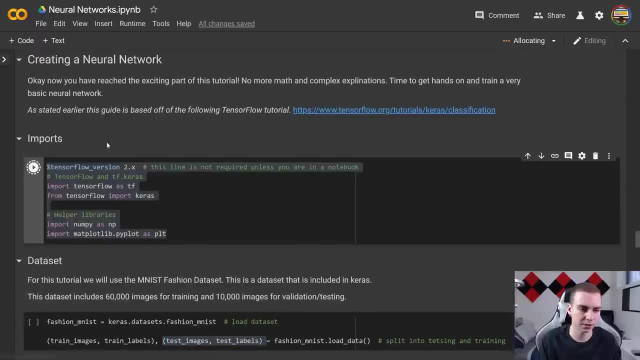 we've talked about all that, So I'm going to kind of skim through that. And now we have it in all of these kind of tuples here. Alright, so let's have a look at this data set to see what we're working with. Okay, so let's run some of this code. Let's. 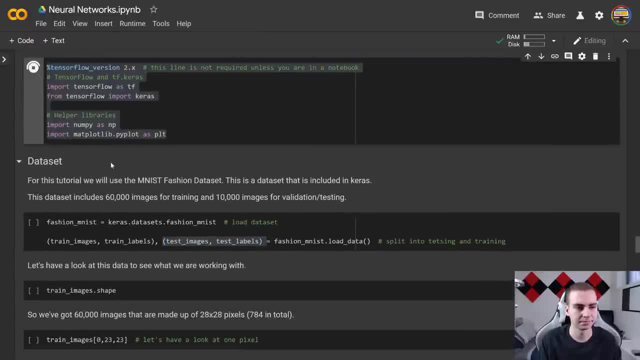 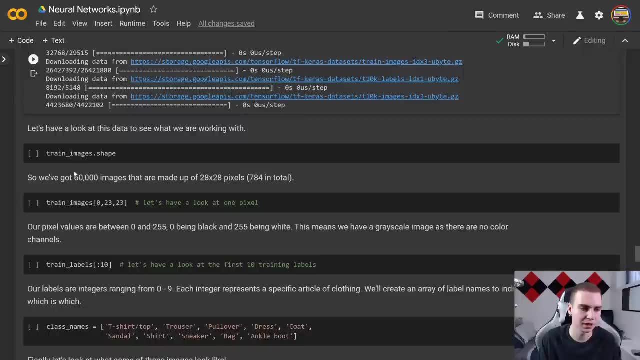 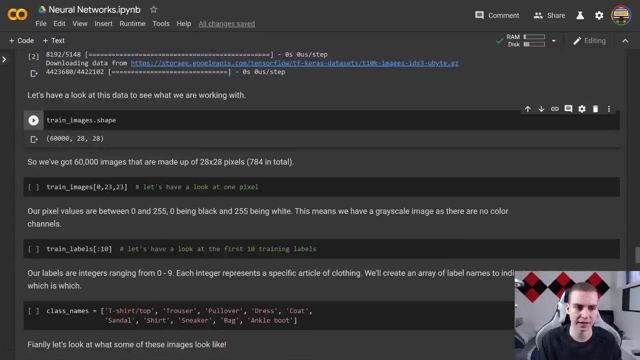 get this import going If it doesn't take forever. Okay, let's get the data set. Yeah, this will take a second to download for you guys, if you don't already have it cached. And then we'll go train images, dot shape, And let's look at what one of the images looks like Or, sorry, what our data set. 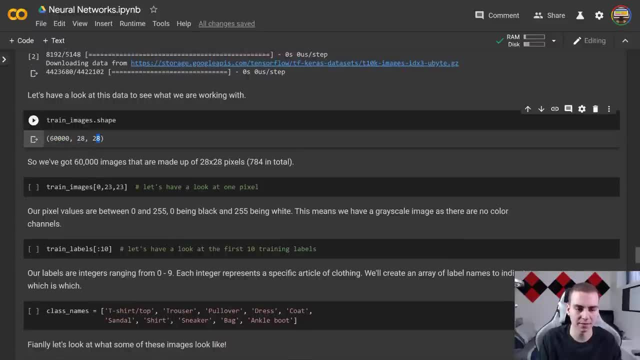 looks like. So we have 60,000 images that are 28.. By 28.. Now, what that means is we have 28 pixels, or 28 rows of 28 pixels, right? So that's kind of what our- you know- information is. So we're going to have in total 784 pixels, which I've denoted. 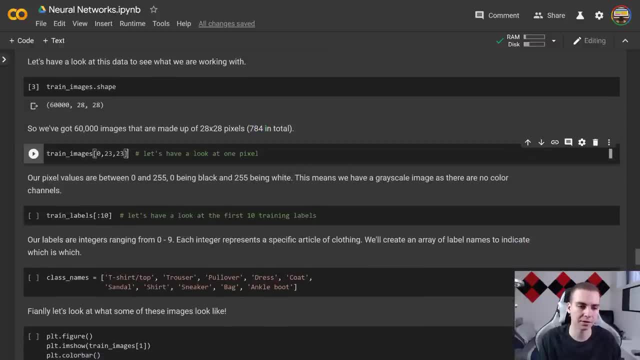 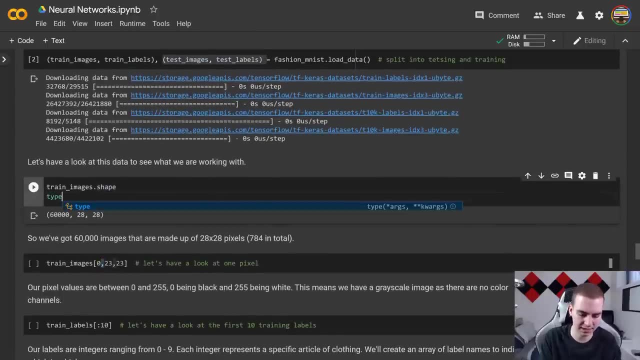 here. So let's have a look at one pixel. So, to reference one pixel, this is what I, what I'm doing. this comes in as a- actually I'm not sure what type of data frame this is, But let's have a look. 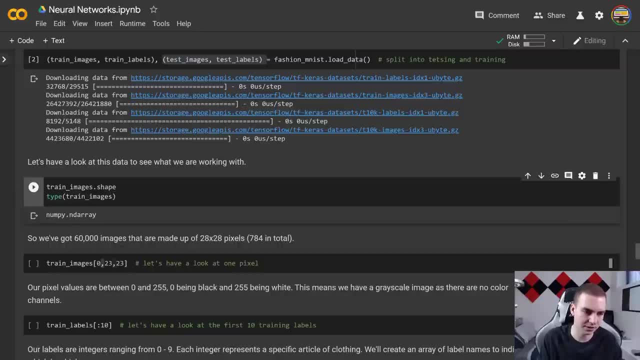 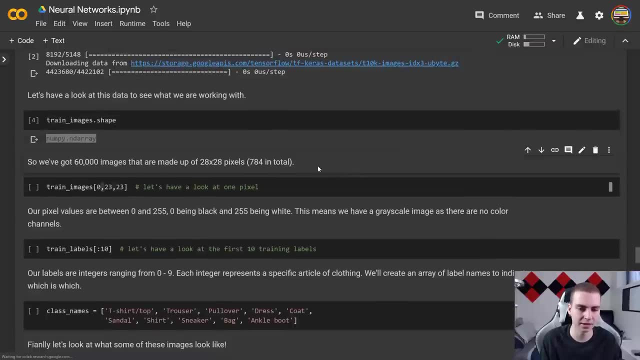 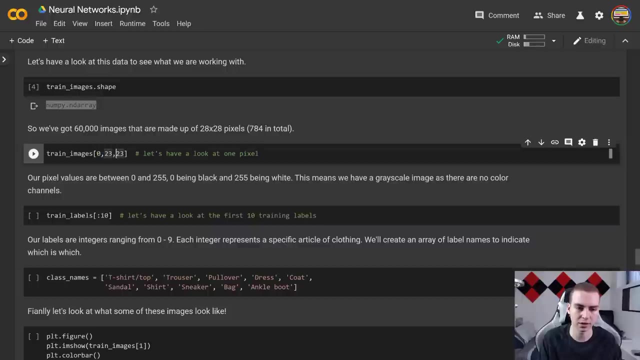 at it. So let's say: type of train underscore images, because I want to see that. So that's a numpy array, So to reference the different indexes in this. it's similar to pandas. we're just going to do zero, comma 23, comma 23, which stands for, you know, image 023, and then 23.. And this gives us 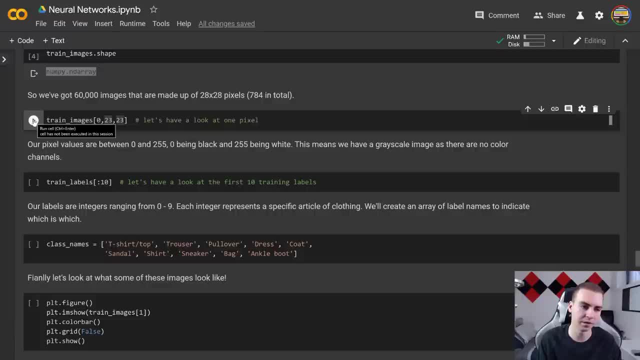 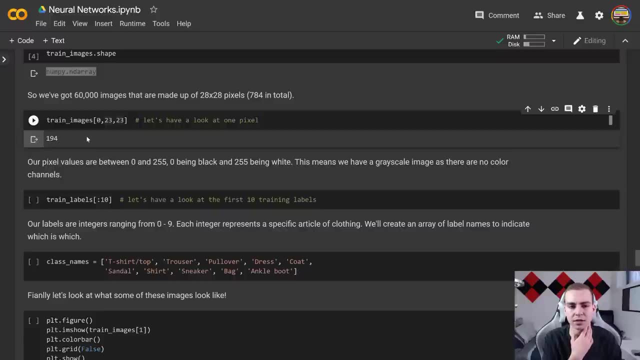 one pixel, So row 23,, column 23,, which will be that. Okay, so let's run this And let's see: this value is 194.. Okay so, that's kind of interesting. That's what one pixel looks like. So let's look at. 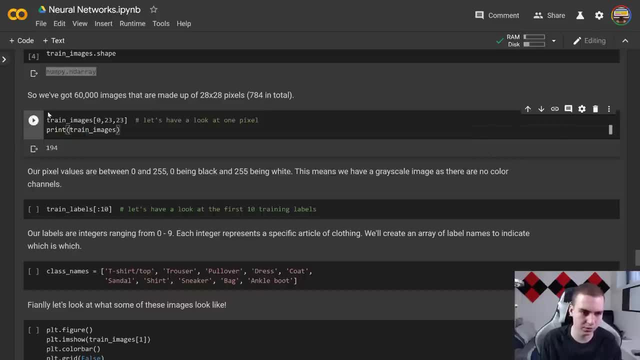 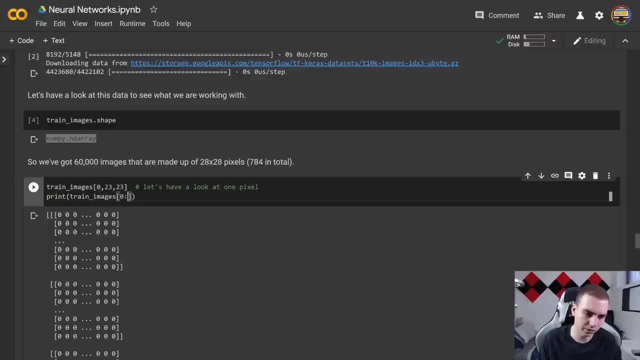 what multiple pixels look like. So we'll print train underscore images And, okay, so we get all these zeros. let's print train images, zero colon. that should work for us And we're getting all these zeros. Okay, so that's the border of the picture. That's okay. I can't. 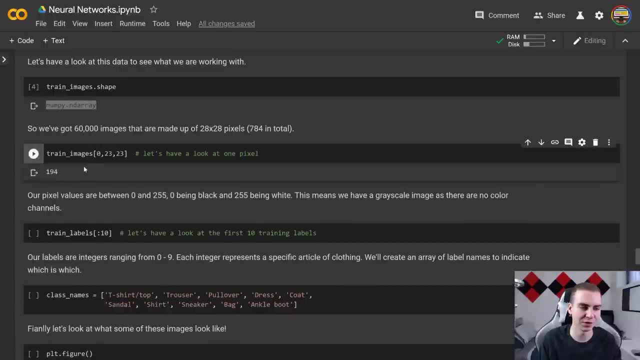 show you what I wanted to show you. Anyways, one pixel, and I wanted to have you guys guess. it is simply just represented by a number between zero and 255.. Now what this stands for is the grayscale value of this pixel. So we're dealing with grayscale images, although we can deal with you. 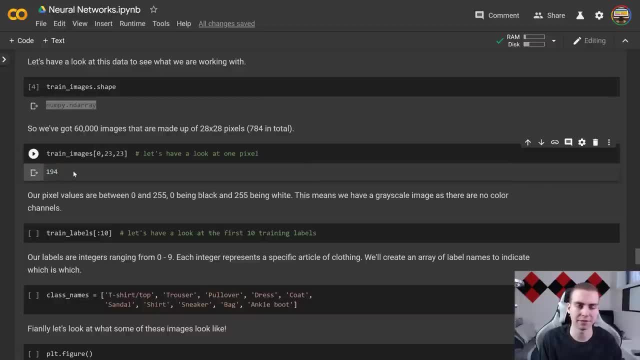 know 3d, 5d images as well or not 5d images, but we can deal with images that have like RGB values first, So, for example, we could have a number between 02- 55,, another number between zero and 255, and. 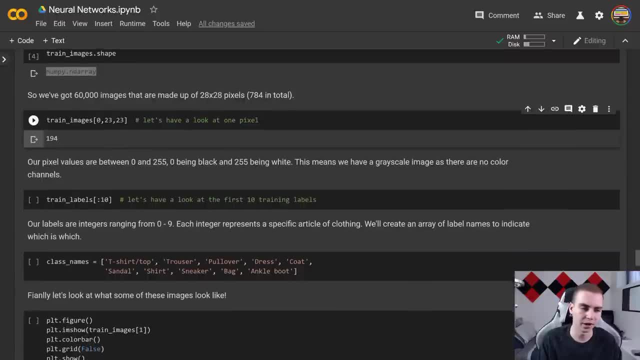 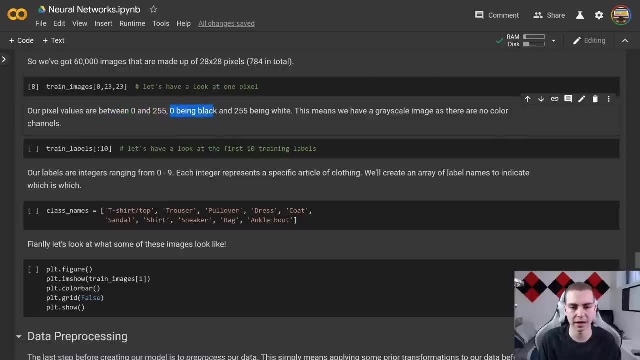 another number between zero and 255 for every single pixel, right, whereas this one is just one simple static value. Okay, so it says like here, our pixel values: between zero and 255.. Zero being black and 255 being white. So essentially, you know, if it's 255, that means that this is white. 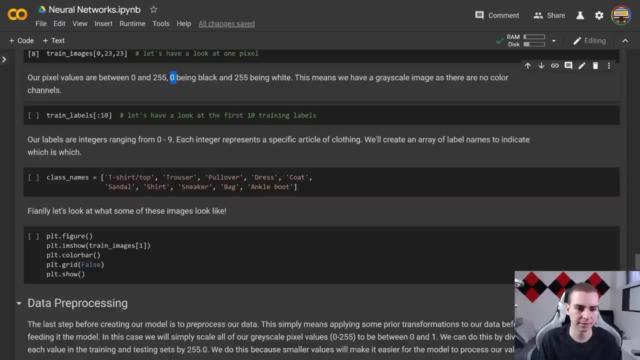 If it's zero, that means that it's white is black. Alright, so let's have a look at the first 10 training labels. So that was our training images. Now, what are the training labels? Okay, so we have an array and we get. 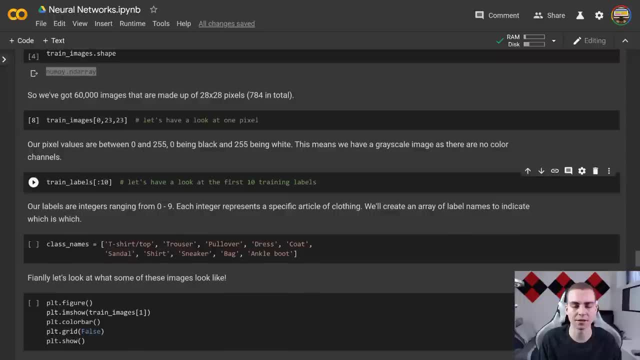 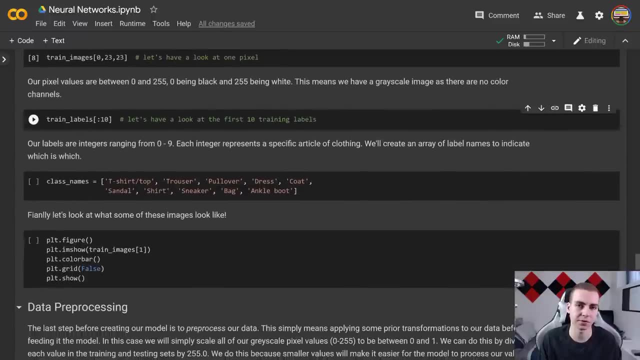 values from zero to nine. Now, this is because we have 10 different classes that we could have for our data set, So there's 10 different articles of clothing that are represented. I don't know what all of them are, although they are right here. So T shirt, trouser. 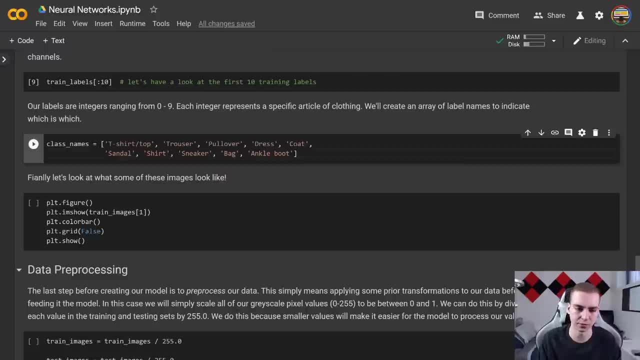 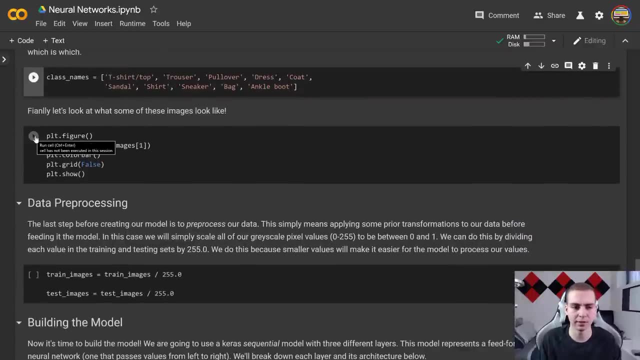 pullover, dress, coat, sandal shirt, sneaker bag, ankle boot. Okay so let's run this class names, Just so that we have that saved. And now what I'm going to do is just use matplotlib to show you what one of the images looks like. So, in this case, this is a shirt. I know this. 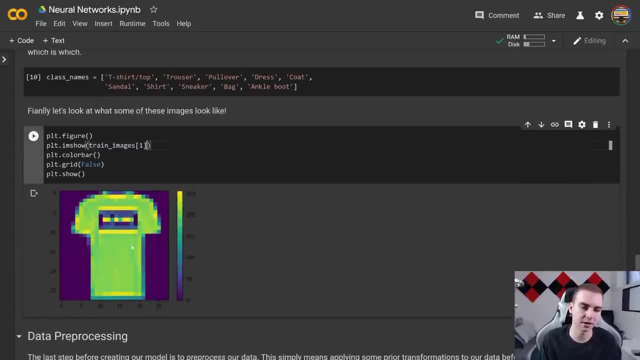 is printing out kind of weird, but I'm just showing the image. I know it's like different colors, But that's because if we don't define that we're drawing a grayscale, it's going to do this, But anyways, that is what we get for the shirt, So let's go to another image. 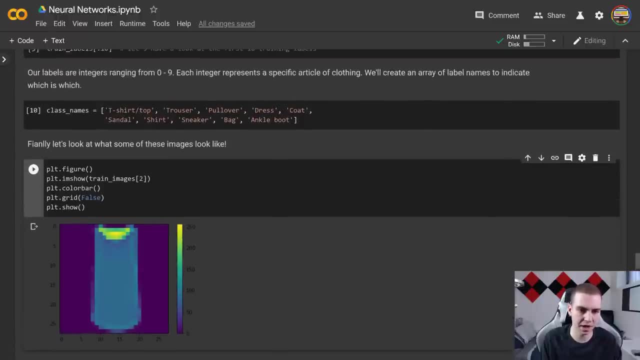 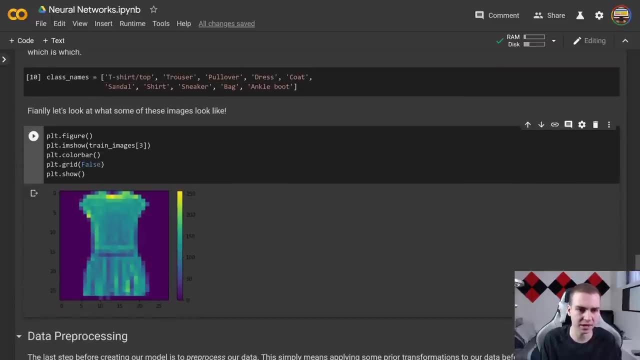 And let's have a look at what this one is. I actually don't know what that is. I don't know what that is, So we'll skip that. Maybe that's a, what is it? T shirt or top? This, I guess, is going to be like a dress. Yeah, so we do have dress there. Let's go for have. 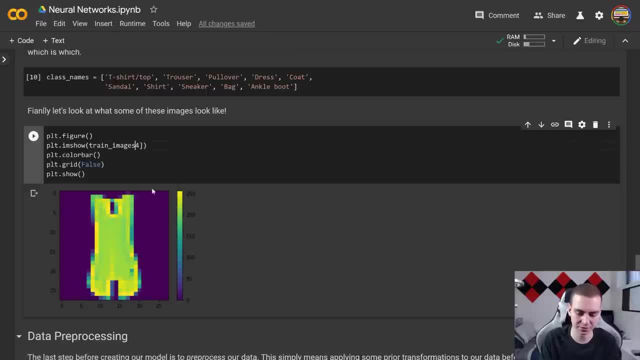 a look at this And some of these are like hard to even make out when I'm looking at them myself. And then I guess this will be like a hoodie or something. I'm trying to get one to sandal to show you guys a few different ones. There we go. So that is a sandal, or 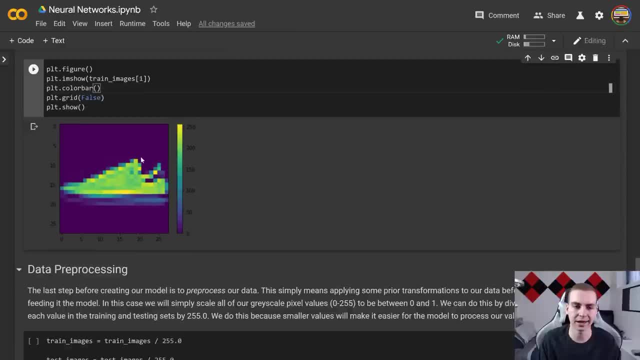 a sneaker. Okay, so that is kind of how we do that and how we look at the different images. So if you want to just draw it out, all you do is just make a figure. you just show the image. do the color bar? 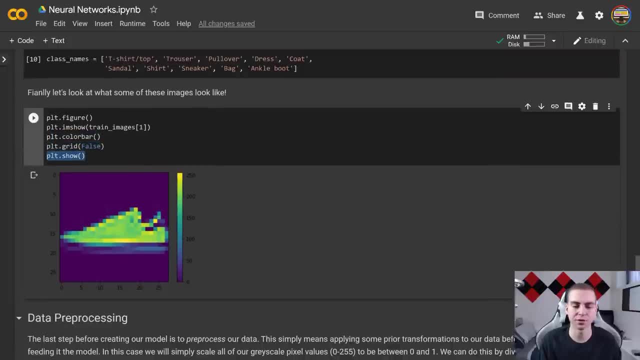 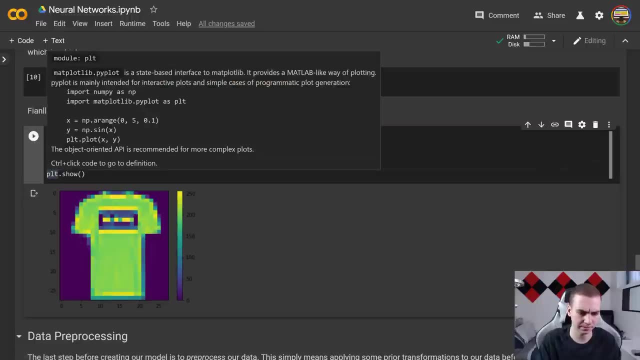 which is just giving you this. then you're going to say I don't want to grid, and then you can just show the image right, Because if you don't have this line here and you show with the grid, oh, it's actually not showing the grid. That's interesting, Although. 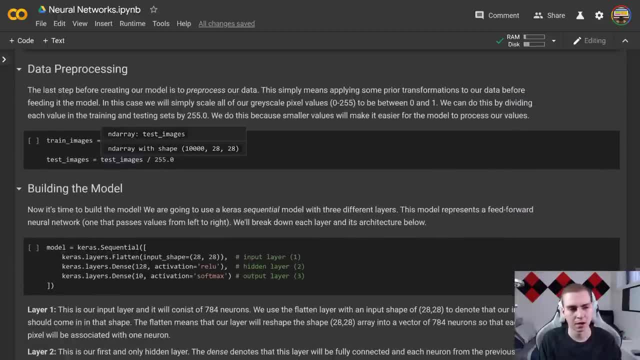 I thought it was going to show me those pixelate grid, So I guess you don't need that line, Alright. so data pre processing: Alright. so this is an important step in neural networks And a lot of times when we have our data, we have it in these like random forms or 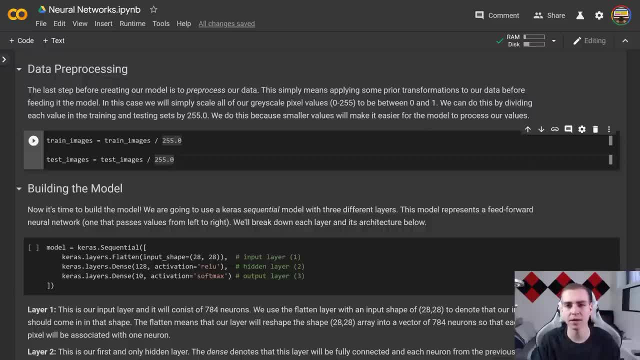 we're missing data. there's information we don't have, There's information we don't know or that we haven't seen, And typically what we need to do is pre process it. Now, what I'm going to do here is squish all my values between. 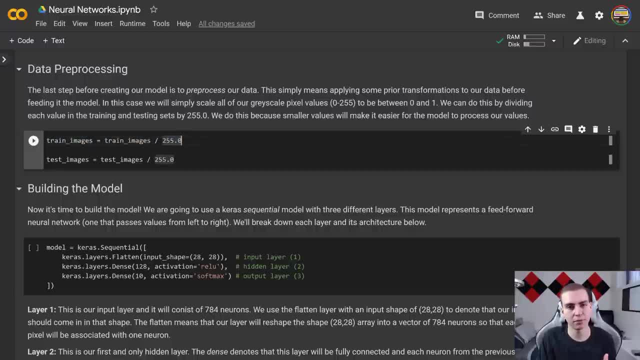 zero and one. Typically, it's a good idea to get all of your input values in a neural network in between, like that range in between, I would say negative, one and one is what you're trying to do. you're trying to make your numbers as small as possible to feed to the neural. 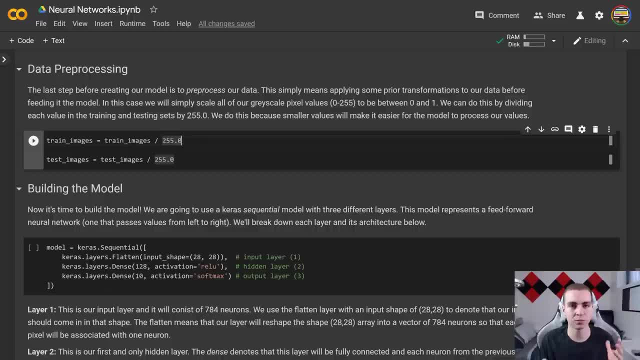 network. The reason for this is your neural network starts out with random weights and biases that are in between the range zero and one, unless you change that value. So if you have massive input information and tiny weights, then you're kind of having a bit of a mismatch. 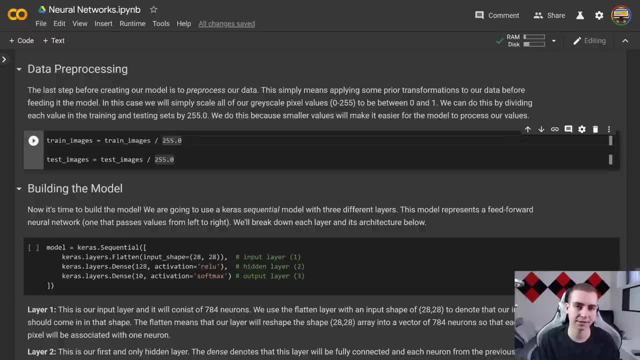 and you're going to make it much more difficult for your network to actually classify your information because it's going to have to work harder to update those weights and biases to reduce how large those values are going to be. if that makes any sense, So it usually. 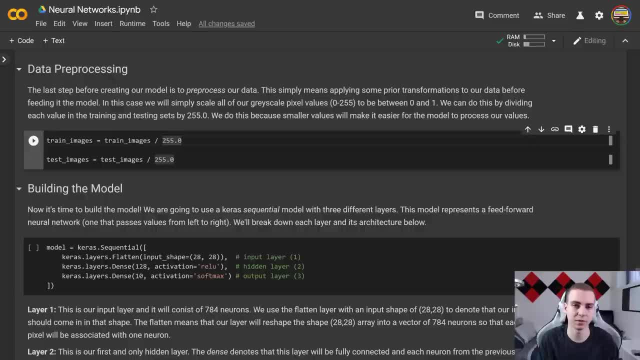 is a good idea to pre process these and make them in between the value of zero and one. Now, since we know that we're just going to have pixel values that are in the range of 255, we can just divide by 255. So we can actually scale it down for us, Although it is extremely important that we do this. 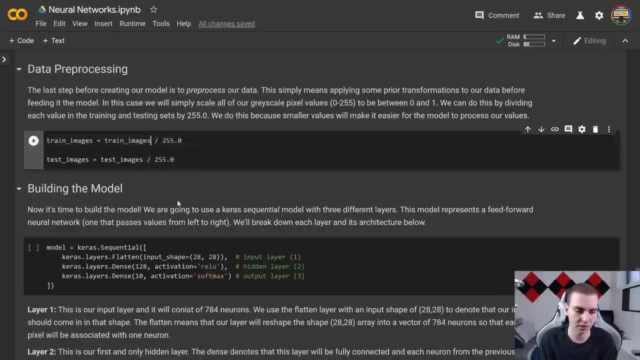 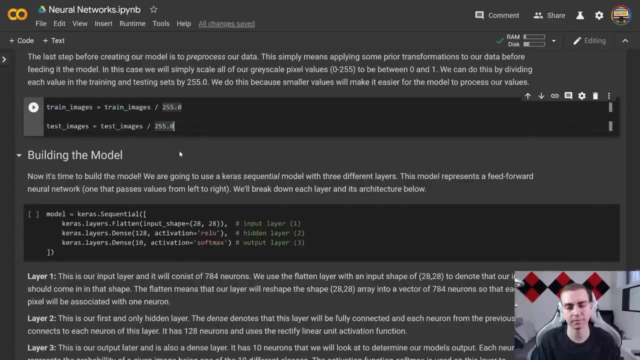 to not only the training images but the testing images as well. If you just pre process your training images and then you pass in, you know, new data that's not pre processed, that's going to be a huge issue. you need to make sure that your data comes in the same form. 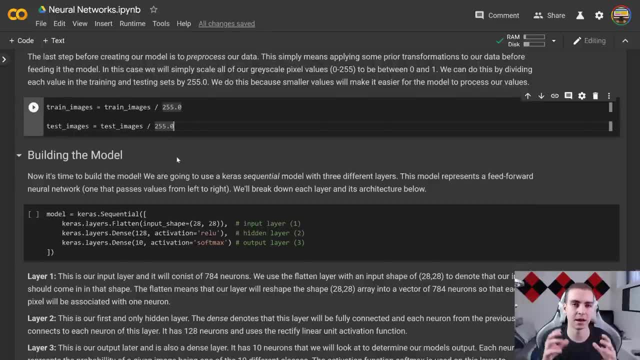 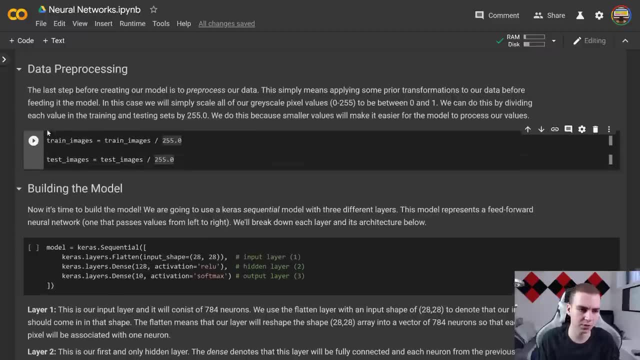 And that means when we're using the model to, to make predictions. whatever you know, I guess at pixel data we have, we need to pre process in the same way that we pre processed our other data. Okay, so let's pre process that. So train images and test images, and I'm just going 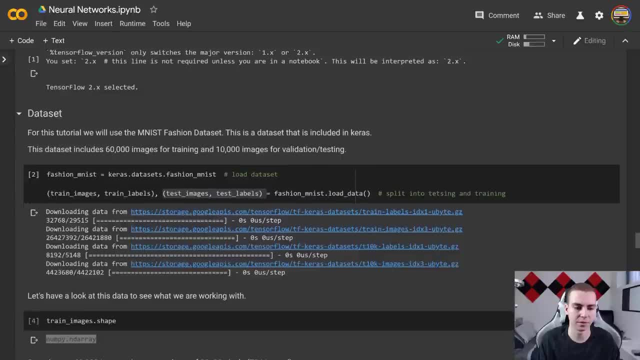 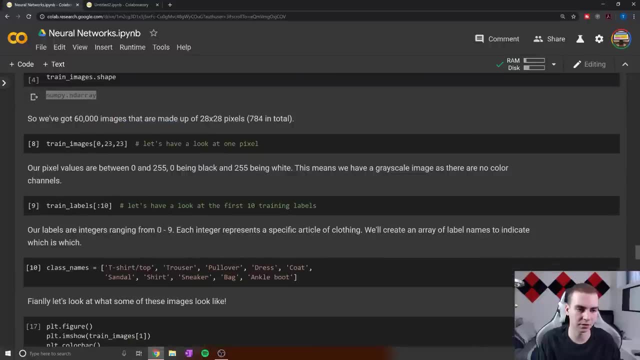 to actually steal some of the stuff here and throw it in my other one before we get too far. So let's get this data set And let's throw it in here, just so we can come back and reference all of this together. Let's go class names. We don't actually need the 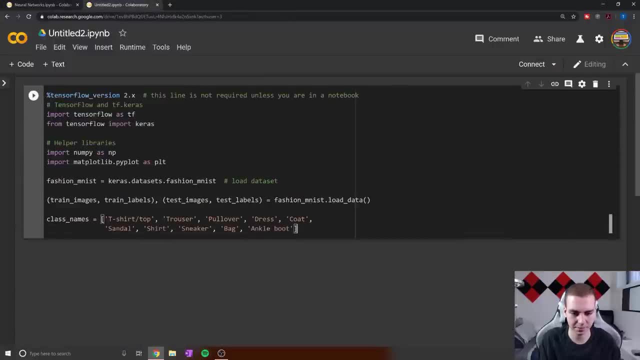 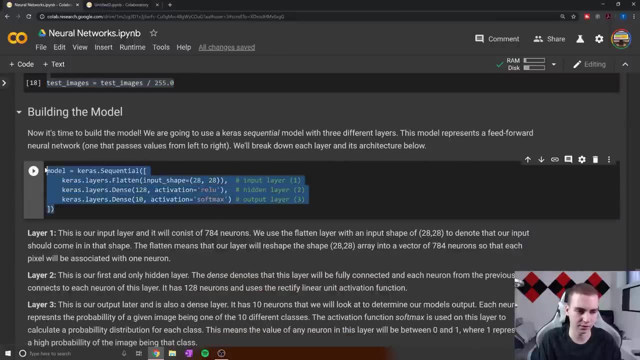 figures- a few things I can skip. we do need this pre processing step like that. if I could go over here. and then, what else do we need? we're going to need this data set, Okay. so let's actually just copy the model into this and just make it a little bit cleaner. 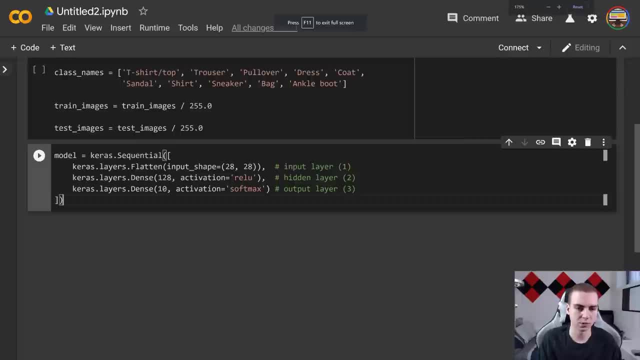 we can have a look at it. So new code: block model. Okay, so model creating our model. Now creating our model is actually really easy. I'm hoping what you guys have realized so far is that data is usually the hardest part of machine learning and neural networks. 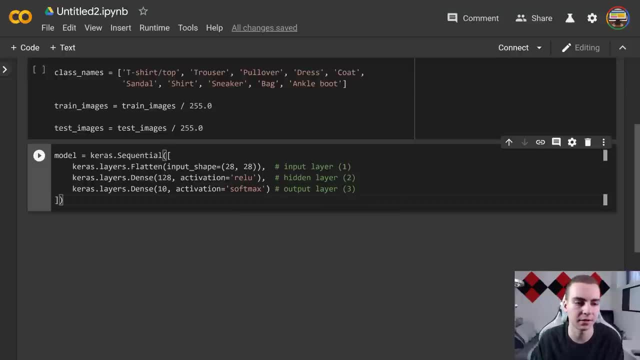 getting your data in the right form, the right shape And you know pre process correctly. building the model is usually pretty easy because we have tools like tensor loan, Keras that can do it for us. So we're gonna say: model equals Keras, dot sequential. Now let's. 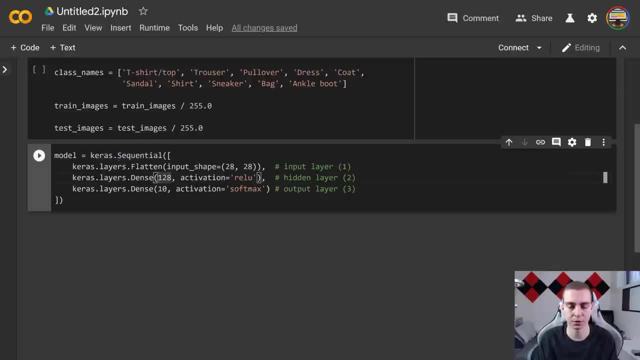 do that Now. sequential simply stands for the most basic form of neural network which we've talked about so far, which is just information going from the left side to the right side, passing through the layers sequentially, right called sequential we have not talked about. 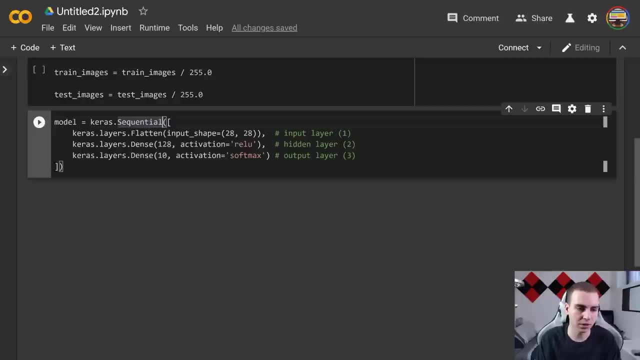 recurrent or convolutional neural networks. yet Now what we're going to do here is go Keras, dot, layers, dot, flat, So sorry. inside. here we're going to define the layers that we want in our neural network. This first layer is our input layer. And what flatten? 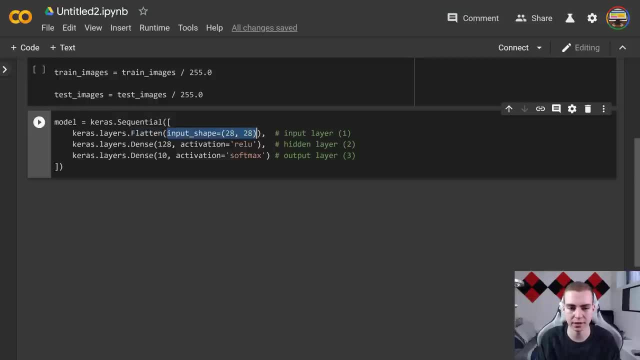 does is allows us to take in a shape of 28 by 28,, which we've defined here, and flatten all of the pixels into 784 pixels. So we take this 28 by 28, kind of matrix, like structure, and just flatten it out And Keras. 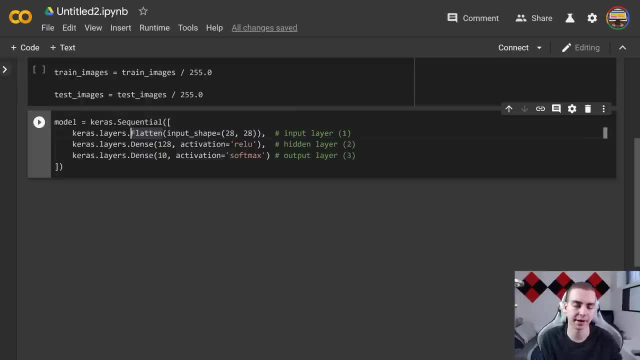 will do that for us. we don't actually need to take our- you know- matrix data in transform before passing, So we've done that. Next we have Keras dot layers, dot. dense 128. activation equals rectify linear unit. This is our first hidden layer, layer two: right, that's what I've denoted here, And 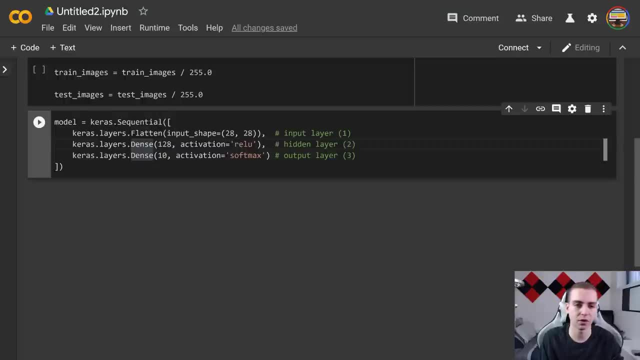 this is a dense layer. Now, dense again means that all of the- what is it? the neurons in the previous layer are connected to every neuron in this layer. So we have 828 neurons here. how do we pick that number? We don't know, we kind of just came up with it Usually. 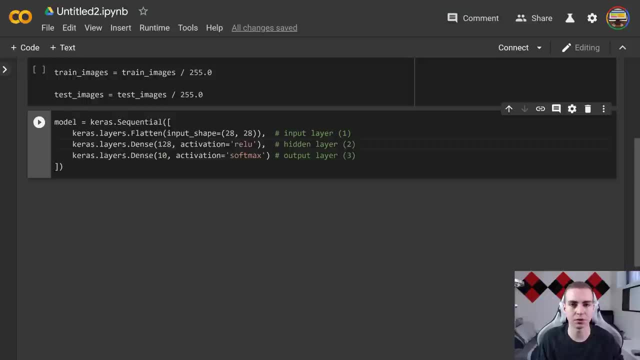 it's a good idea that you're going to do this as, like, a little bit smaller than what your input layer is, although sometimes it's going to be bigger, you know, sometimes it's going to be half the size. it really depends. 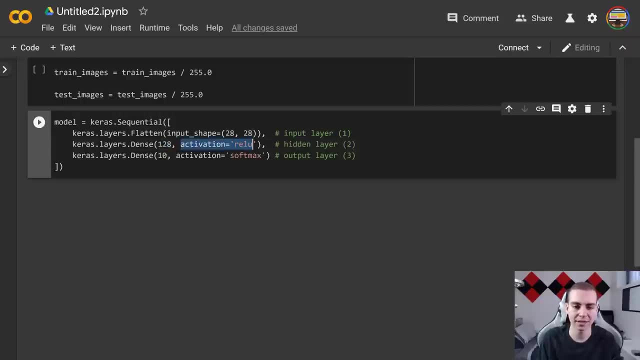 On the problem- I can't really give you a straight answer for that- And then our activation function will define as rectify linear unit. Now we could pick a bunch of different activation functions. there's time. we can pick sigmoid, we can pick tan h, which is hyperbolic tangent. 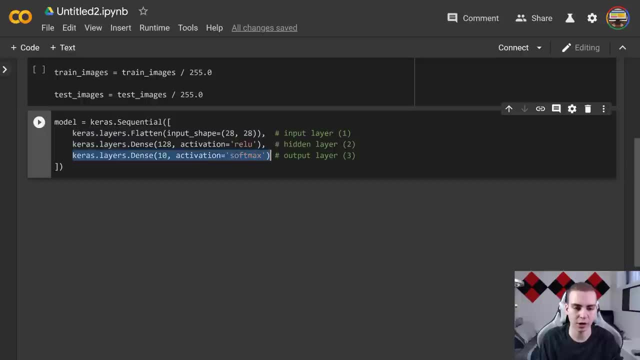 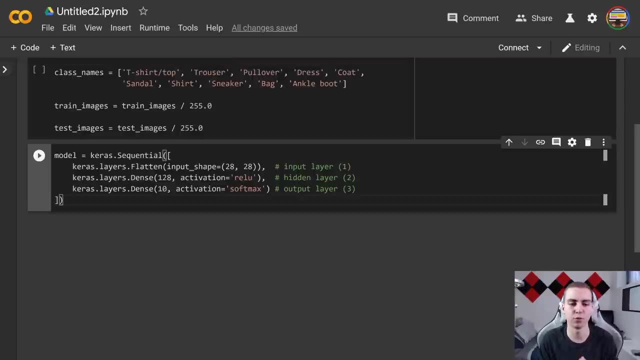 doesn't really matter. And then we're going to define our last layer, which is our output layer, which is a dense layer of 10 output neurons with the activation of softmax. Okay, so can we think of why we would have picked 10 here? right, I'll give you guys a second. 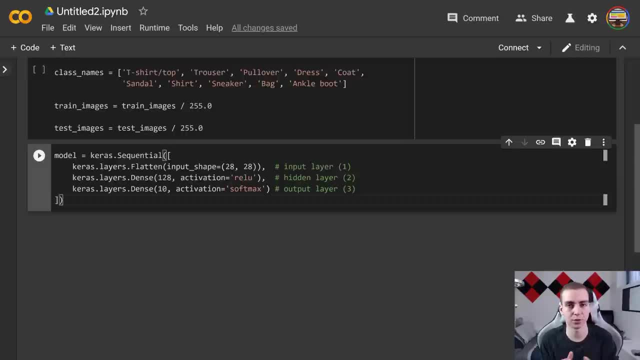 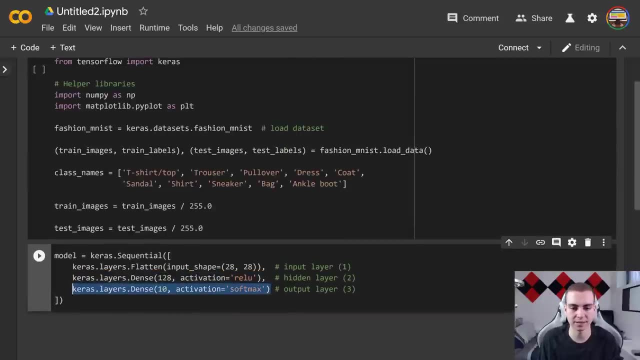 to think about it, Based on the fact that our output neurons are 10.. Our output layer, you know, is supposed to have as many neurons as classes we're going to predict for. So that is exactly what we have: 10.. If we look, we have 10 classes here. 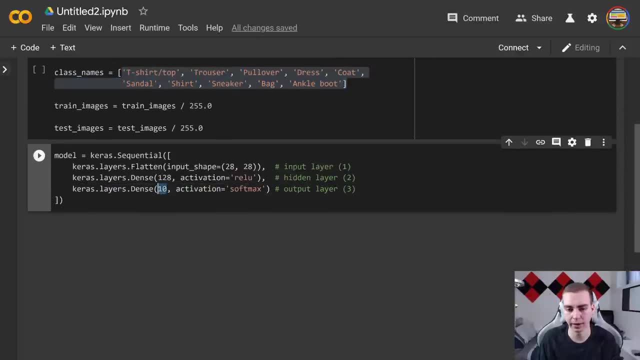 So we're going to have 10 output neurons in our output layer And again we're going to have this probability distribution. And the way we do that is using the activation function softmax. So softmax, we'll make sure that all of the values of our neurons add up to. 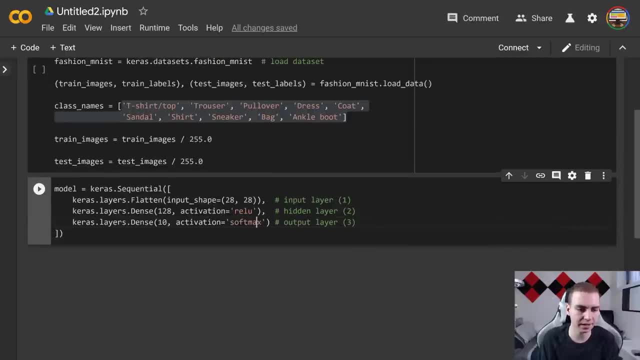 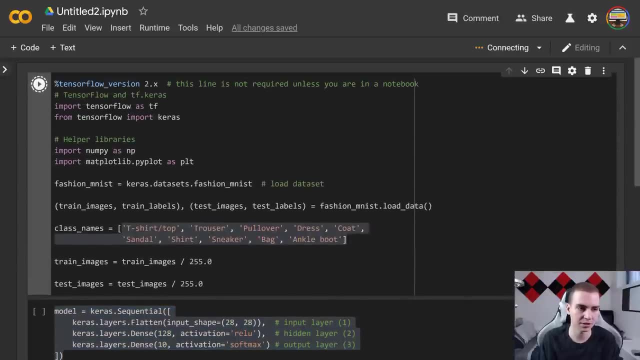 one and that they're between zero and one. So that is our, our model. we've created the model now, So let's actually run this. See, are we going to get any errors here? Is this going to run? and then we'll run the model, And then we'll. 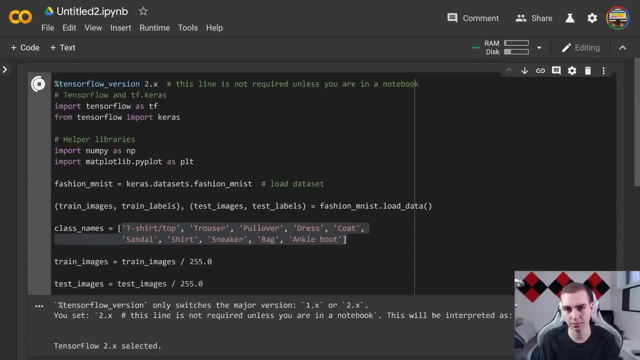 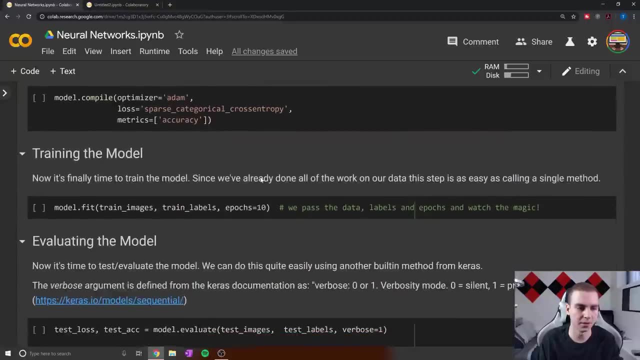 go on to the next step, which actually going to be training and testing the model. Okay, so, let's create the model now, shouldn't get any issues and we're good, And now let's move on to the next step. I'm forgetting what it is, though, which is training the model of. 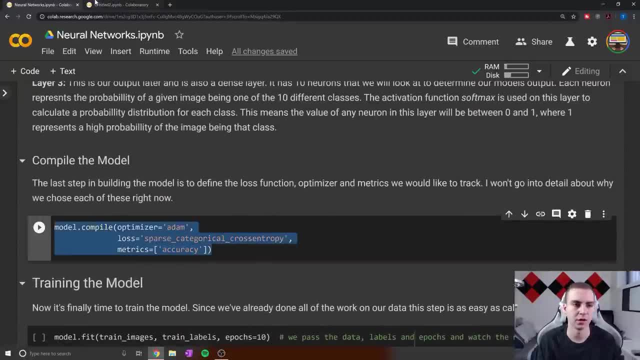 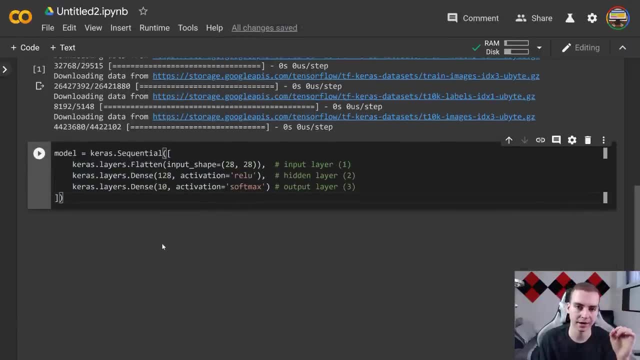 sorry, compiling the model. Okay, so compiling the model. So we've built now what we call the architecture of our neural network. So we've built now what we call the architecture of our neural network. So now we've built right. we've defined the amount of neurons in each layer, we've defined the activation. 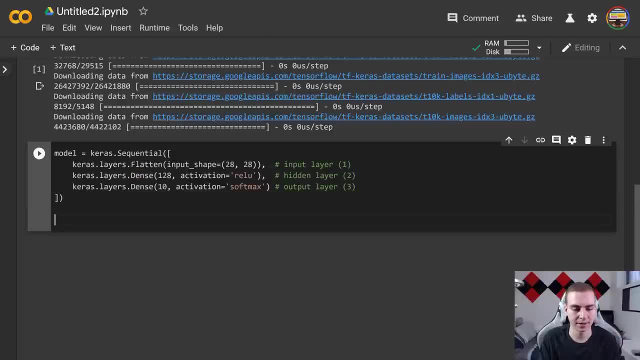 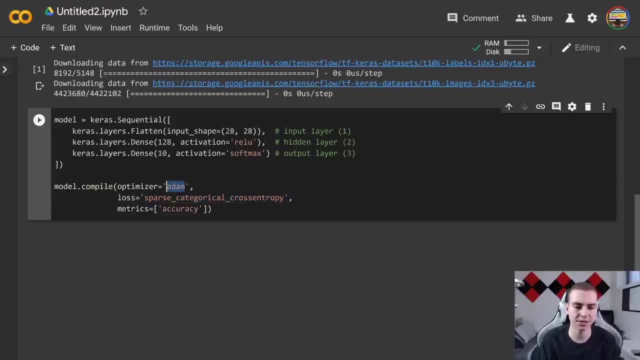 function and we define the type of layer and the type of connections. The next thing we need to pick is the optimizer, the loss and the metrics we're going to be looking at. So the optimizer we're going to use is Adam. this is again just the algorithm that. 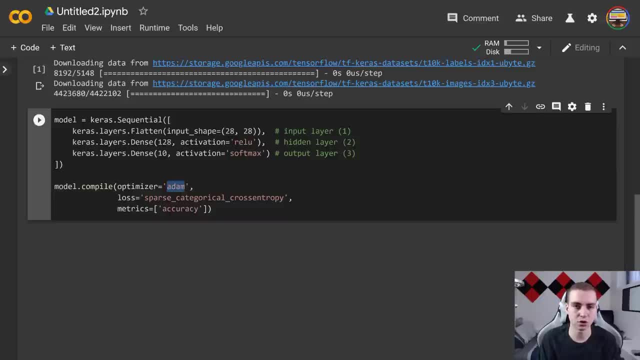 performs the gradient descent. you don't really need to look at these too much. you can read up on some different activation functions or, sorry, optimizers, if you want to kind of see the difference between them. but that's not crazy, we're going to pick a loss. So 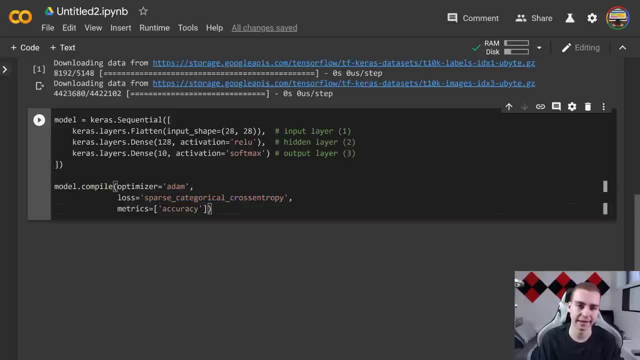 in this case, sparse, categorical cross entropy- again not going to go into depth about that, you guys can look that up if you want to see how it works. And then metrics. So what we're looking for, the output that we want to see from the network, which is accuracy Now, from 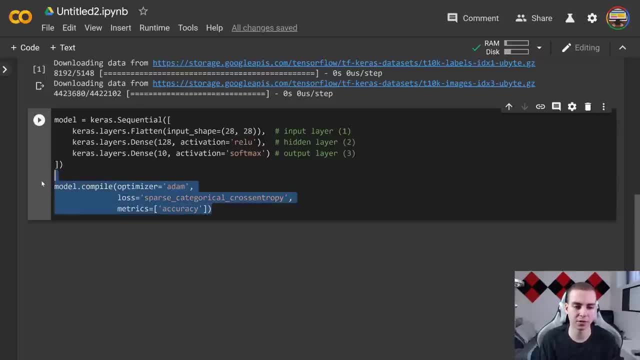 you know, kind of right now, with our current knowledge, we're just going to stick with this as what we're going to compile our neural networks with. we can pick different values if we want, And these are what we call. what is it? 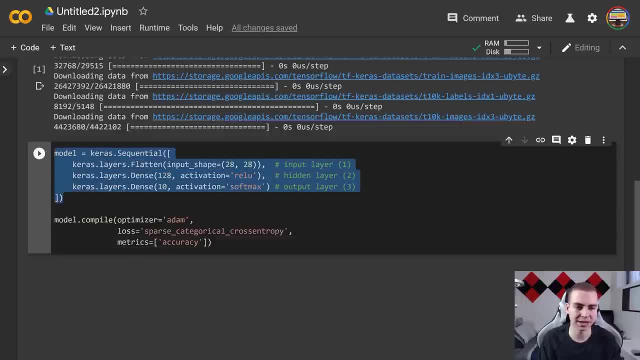 Hyper parameter tuning. So the parameters that are inside here, so like the weights and the biases, are things that we can't manually change, But these are things that we can change right: the optimizer, the loss, the metrics, the activation function. we can change that. 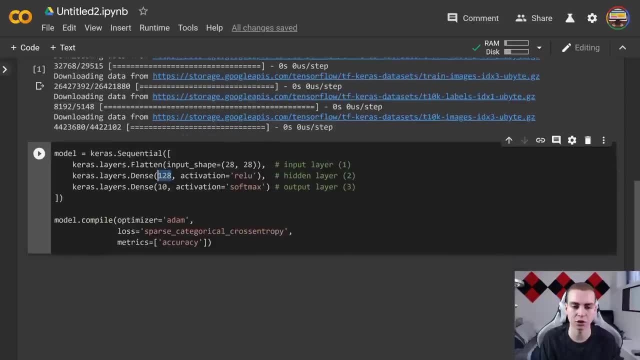 So these are called hyper parameters, same thing with the number of neurons in each layer. So hyper parameter tuning is a process of changing all of these values and looking at how models perform with different hyper parameters change. So I'm not really going to talk about. 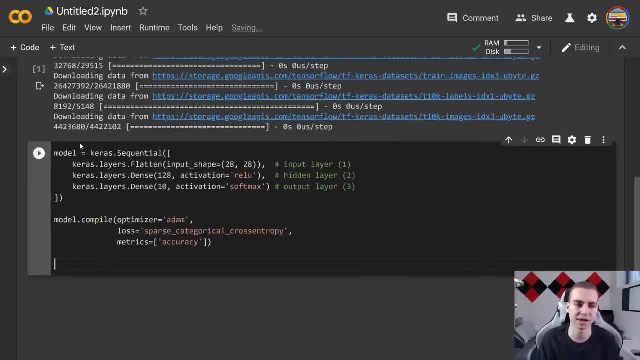 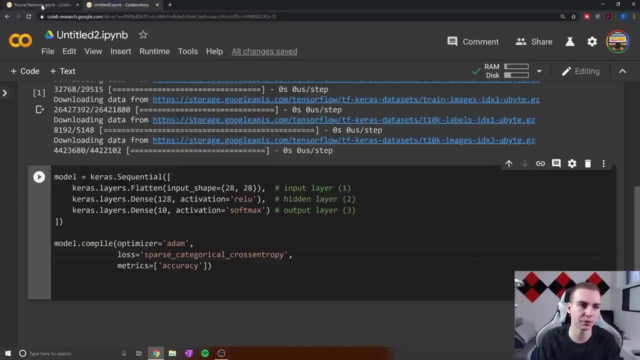 that too Much, but that is something to note, because you'll probably hear that you know this hyper parameter kind of idea. Okay, so we've compiled the model now using this, which just means we've picked all the different things that we need to use for it. And now on to 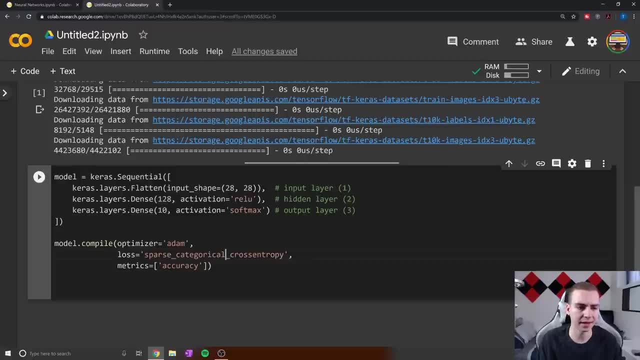 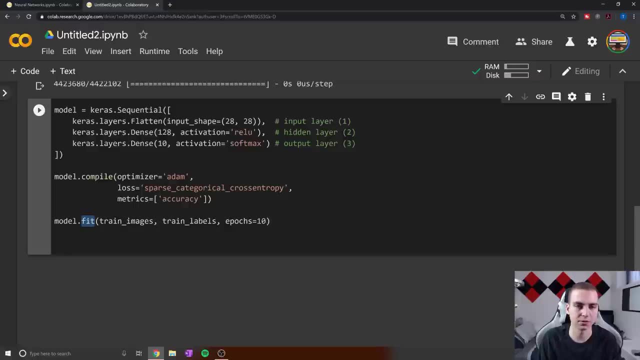 training the model. So I'm just going to copy this in Again. remember this: these parts are pretty syntax, actually heavy, but fairly easy to actually do. So we're going to fit the model. So fit just means we're fitting it to the training data. It's another word. 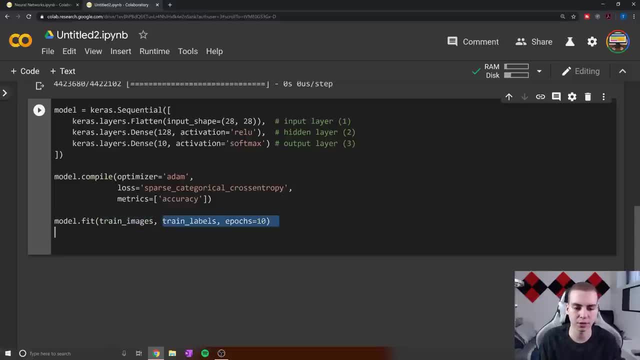 for training, essentially. So we're going to pass it- the training images, the training labels- and notice how much easier it is to pass this Now. we don't need to do this input function. we don't need to do all of that because Keras can handle it for us, And 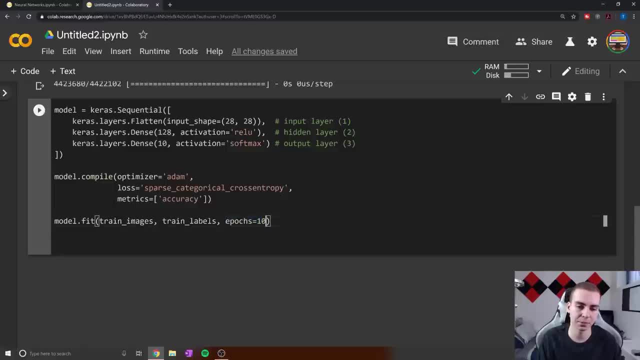 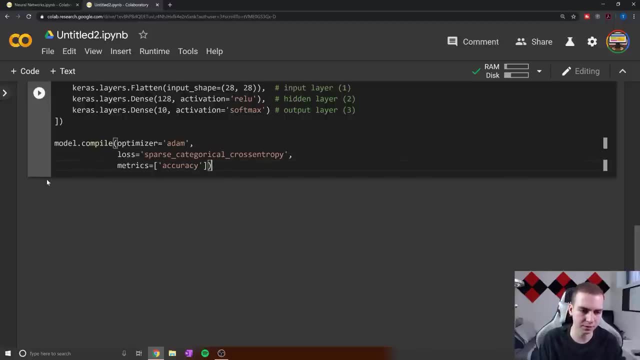 we define our epochs as 10.. epochs is another hyper parameter that you could tune and change if you wanted to. Alright, so that will actually fit our model. So what I'm going to do is put this in another code block, So I don't need to keep retraining this. So we'll go. 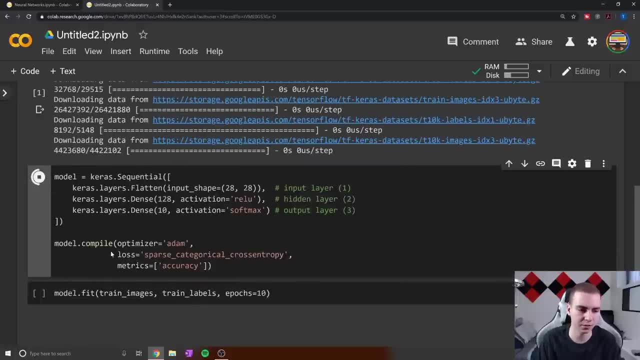 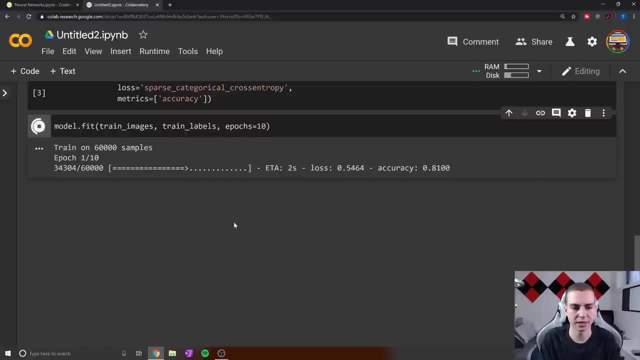 like that And let's actually look at this training process. So we've run the model this should compile And now let's fit it And let's see what we actually end up getting. Alright, so epoch one, and we can see that we're getting a loss and we're getting accuracy. 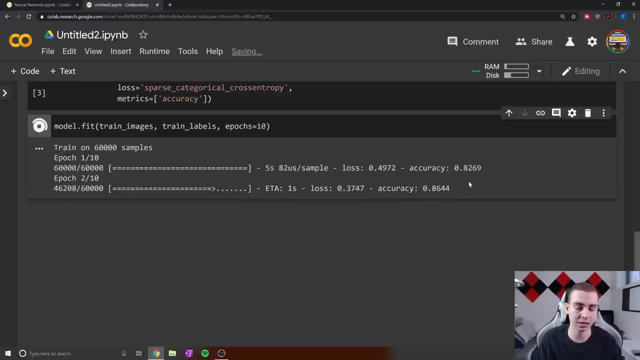 printing out on the side here. Now, this is going to take a second like this is going to take a few minutes, as opposed to our other models that we made are not a few minutes, but, you know, a few seconds when you have 60,000 images and you have a network. that's. 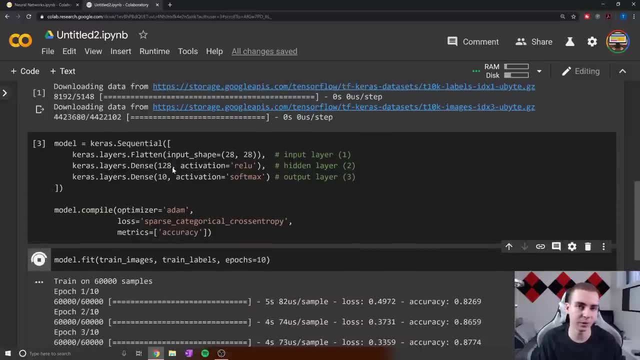 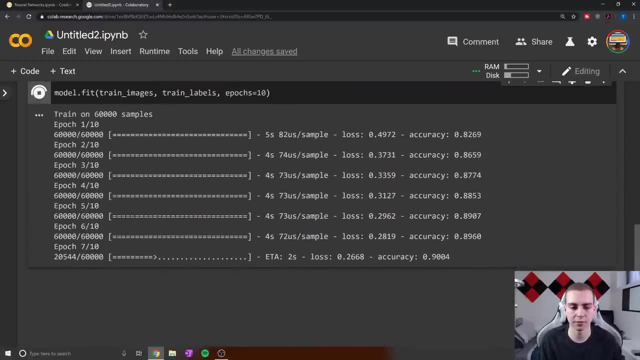 comprised of 784 neurons, 128 neurons and then 10 neurons. you have a lot of weights and biases and a lot of math that needs to go on, So this will take a few seconds to run. If you have a much faster computer, you'll probably be faster than this, But this is. 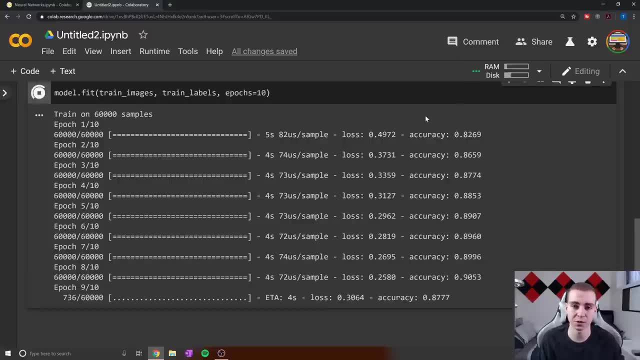 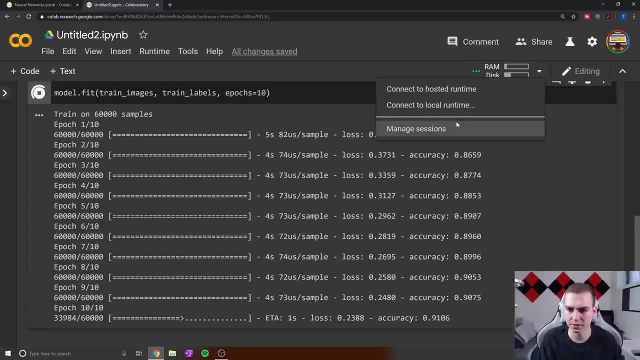 why I like Google Collaboratory, Because you know this isn't using any of my computer's resources to train. it's using this And we can see, like the RAM and the disk. How do I look at this In this network? Oh, is it gonna? let me look at this now. Okay, I don't. 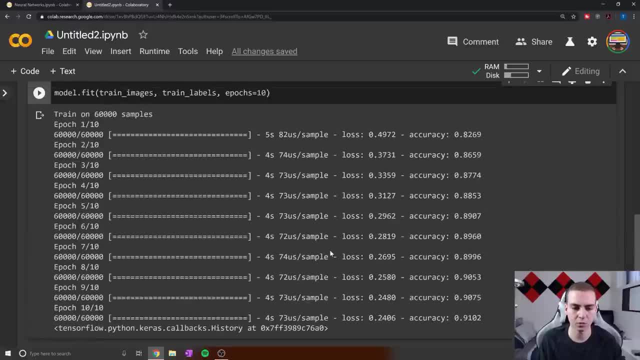 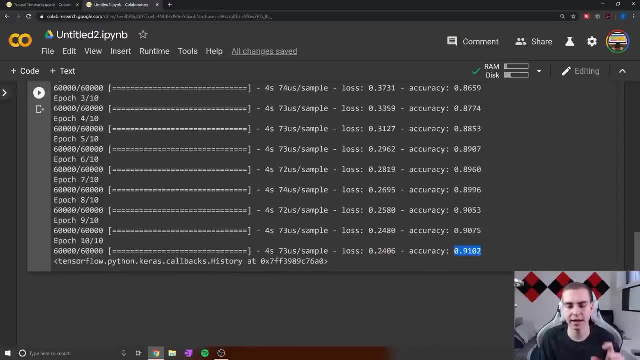 know why it's not letting me click this, But usually you can have a look at it, And now we've trained and we've fit the model, So we can see that we have an accuracy of 91%. But the thing is this is the accuracy. 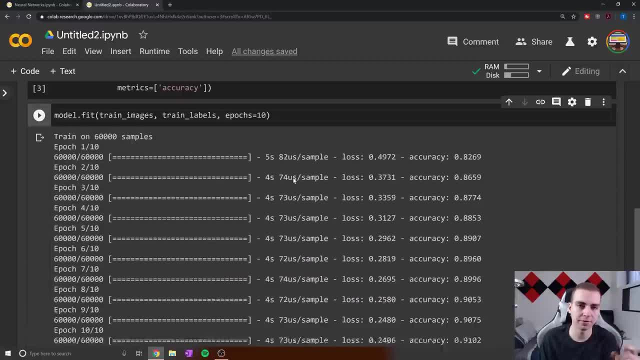 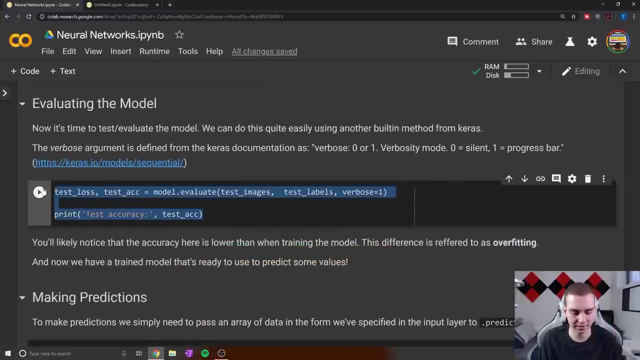 On, or testing or our training data. So now, if we want to find what the true accuracy is, what we need to do is actually test it on our testing data. So I'm going to steal this line of code here. This is how we test our model. Pretty straightforward, I'll just 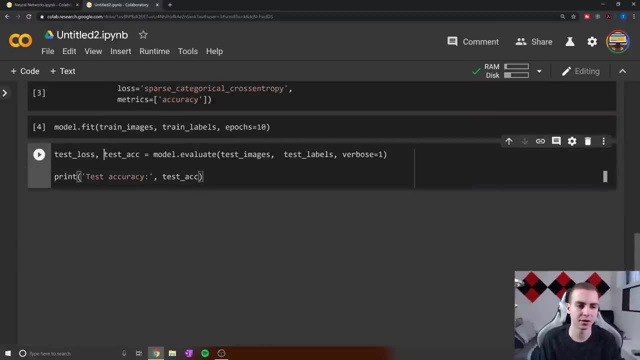 close this, So let's go into code block. So we have test loss. test accuracy is modeled on evaluate test images, test labels. verbose equals one. Now, what is verbose? I was hoping it was going to give me the thing so I could just read it to you guys, But verbose essentially. 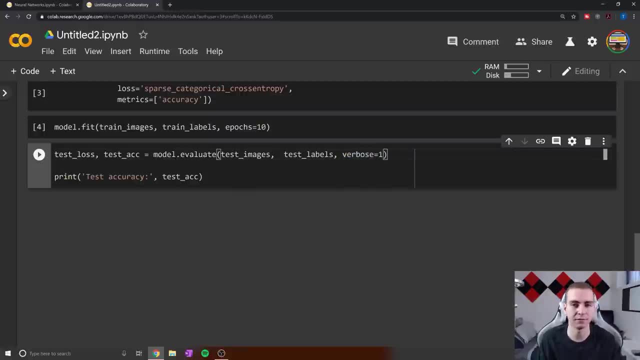 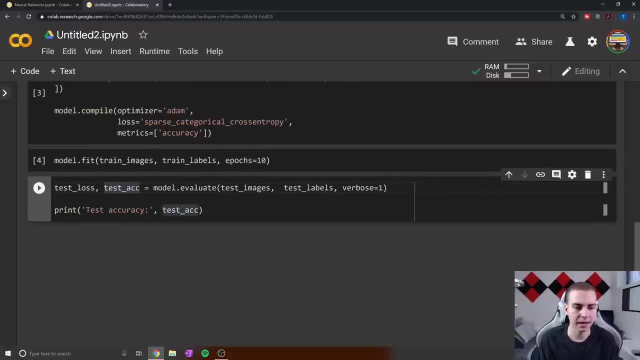 is just: are we looking at output or not? So like, how much information are we seeing as this model evaluates? It's like how much is printing out to the console? That's what that means And, yes, this will just split up kind of the metrics that are returned to. 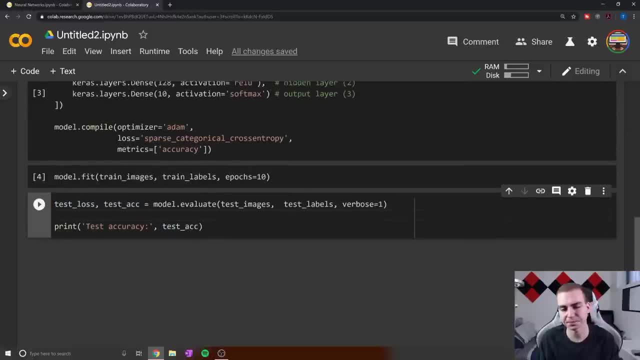 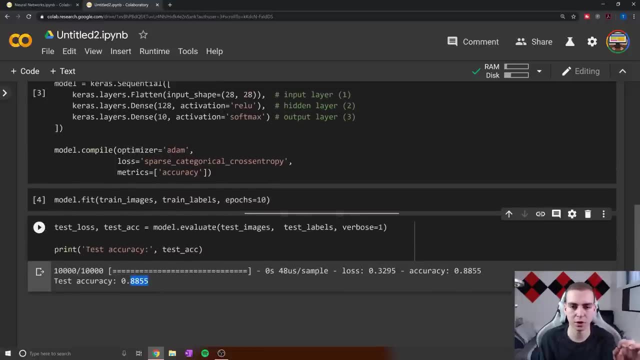 this into test loss and test accuracy So we can have a look at it Now. you will notice when I run this that the accuracy will likely be lower on this than it was on our model. So actually the accuracy we had from this was about 91. And now we're only getting 88.5.. 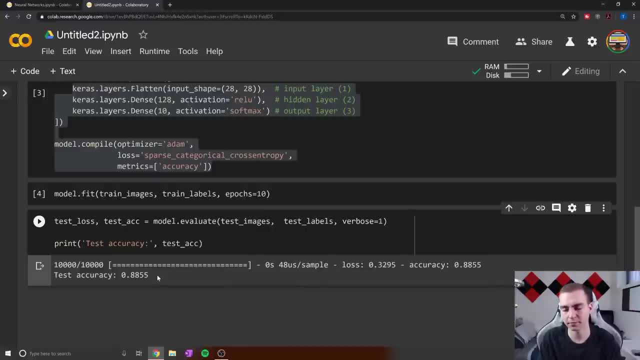 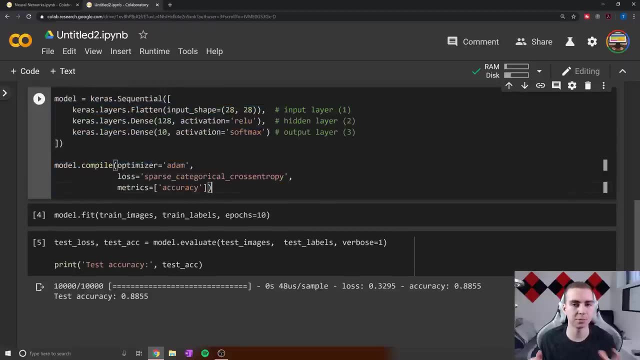 So this is an example of something we call overfitting. Our model seemed like it was doing really well on the testing data, or sorry, the training data, But that's because it was seeing that data so often. right with 10 epochs, it started to just kind of memorize that data. 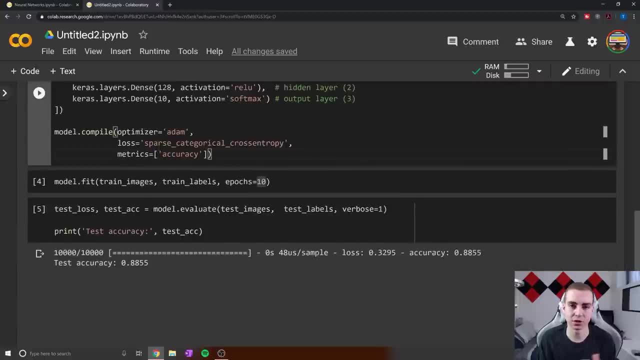 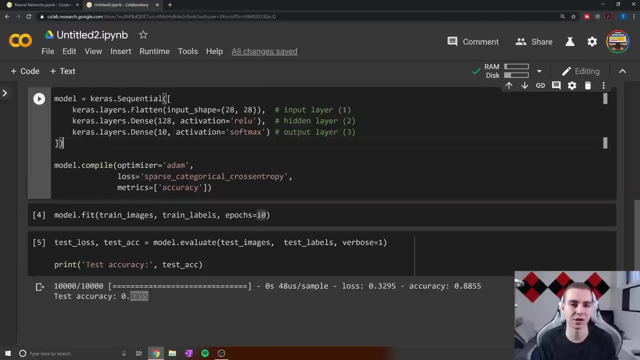 and get good at seeing that data, Whereas now, when we pass it new data that it's never seen before, it's only 88.5% accurate, which means we overfit our model, And it's not as good at generalizing for other data. 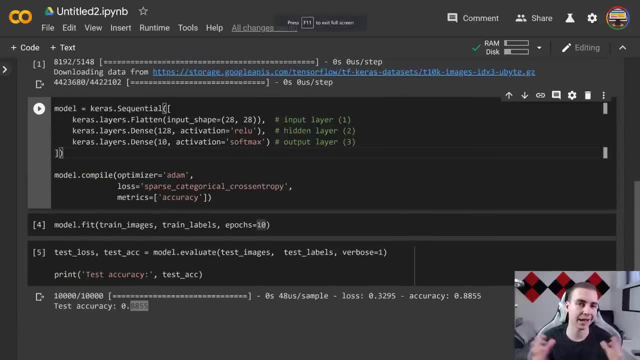 data sets, which is usually the goal right When we create a model. we want the highest accuracy possible. But we want the highest accuracy possible on new data, So we need to make sure our model generalizes properly. Now in this instance- you know we like it's. 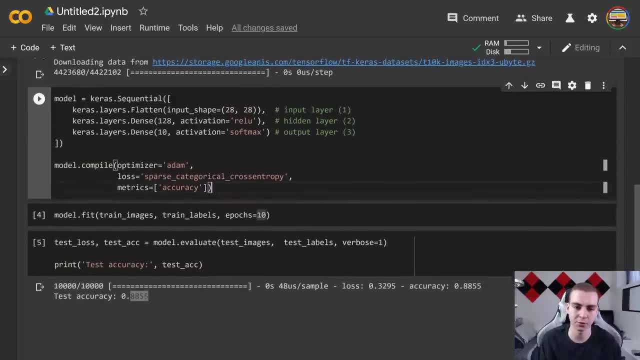 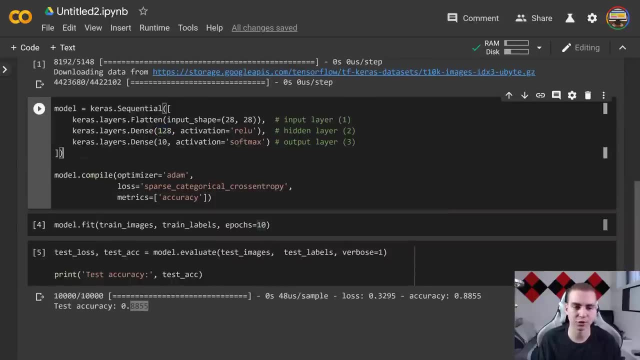 it's hard to figure out how do we do that, because we don't know that much about neural networks, But this is the idea of overfitting and of hyper parameter tuning right. So if we can start changing some of this architecture and we can change maybe the optimizer, the 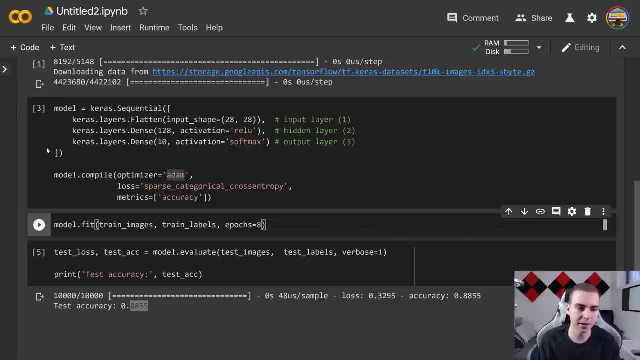 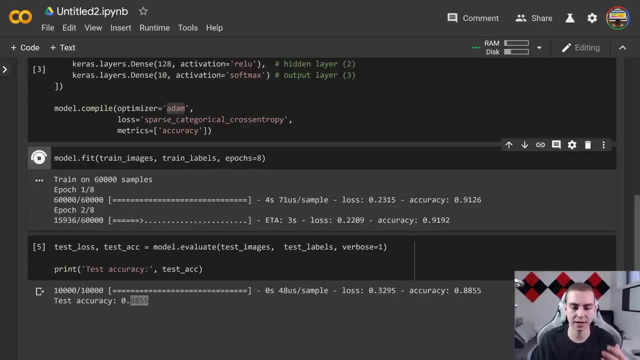 loss function. maybe we go epochs eight. let's see if this does any better, right? So let's now fit the model with eight epochs. we'll have a look at what this accuracy is And then we'll test it and see if we get a. 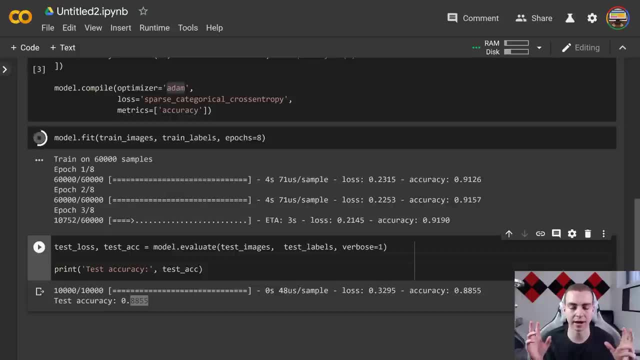 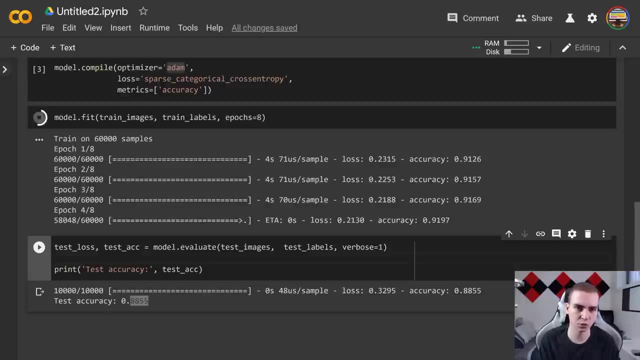 higher accuracy on the testing data set, And this is kind of the idea of that hyper parameter tuning right. Well, we just look at each epoch- or not each epoch- we look at each parameter, we tweak them a little bit And usually we'll like write some code that automates. 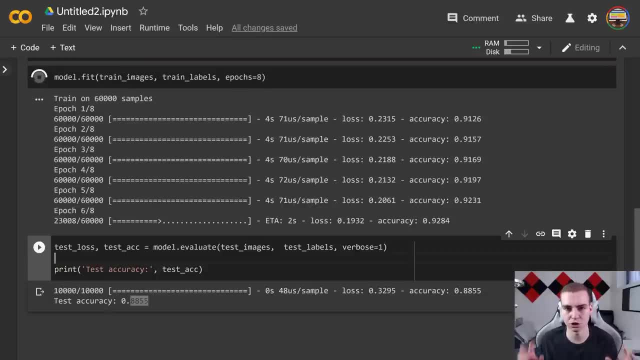 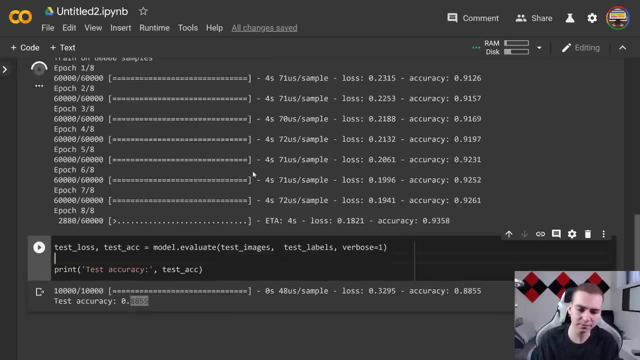 this for us. But that's the idea is, we want to get the most generalized accuracy that we can, So I'll wait for this to train. We're actually almost done, So I won't even bother cutting the video, And then we'll run. 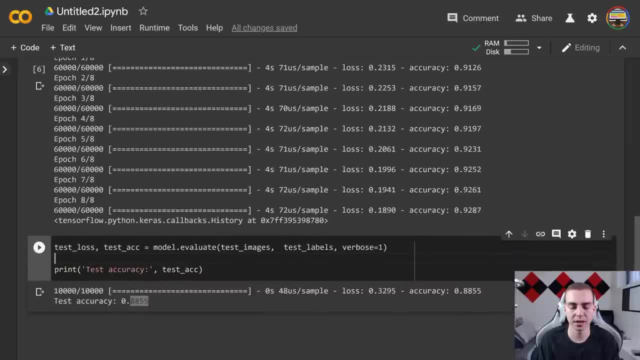 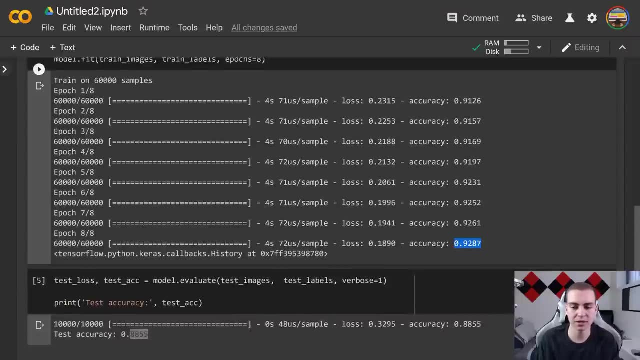 at this evaluation And we'll see now if we got a better accuracy. Now I'm getting a little bit scared because the accuracy is getting very high here And sometimes you know like you want the accuracy to be high on your training data, But when it gets to a point where it's 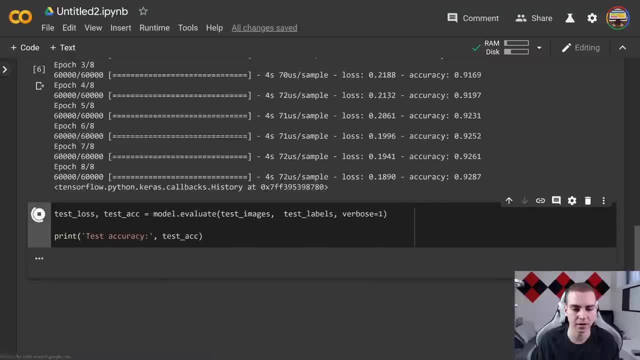 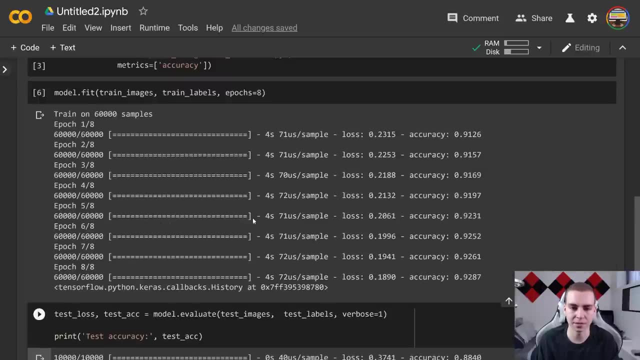 very high. you're in a situation where it's likely that you've overfit. So let's look at this now And let's see what we get. So 88.4.. So we actually dropped down a little bit And it seemed like those epochs didn't make a big difference. So maybe, if I train 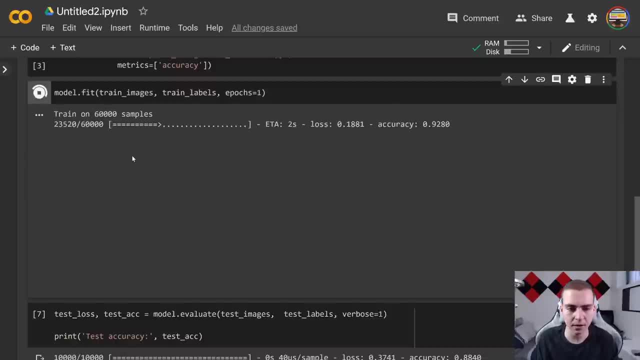 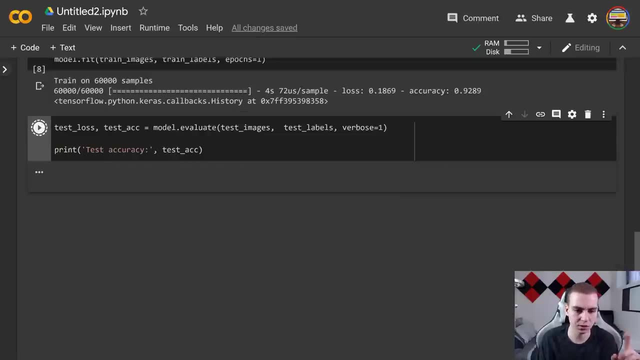 it on one epoch. let's have an idea and see what this does. You know, make your prediction. You think we're going to be better? Do you think we're going to be worse? It's only seen the training data one time. Let's run this. 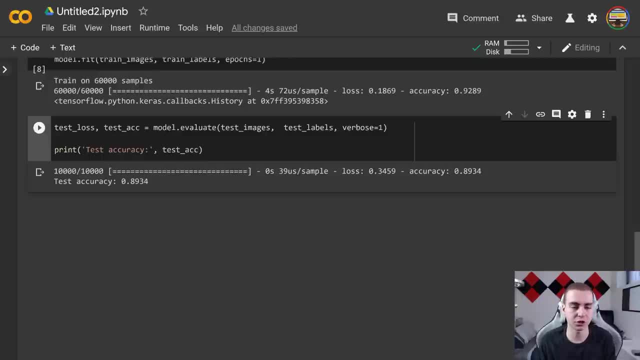 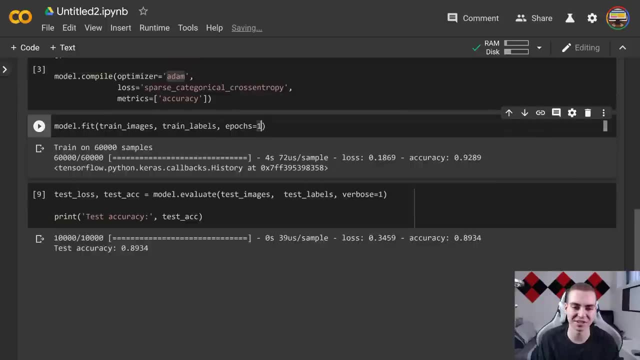 And let's see 89.34.. So in this situation, less epochs was actually better. So that's something to consider. You know a lot of people I see just go like 100 epochs and just think their model is going to be great. That's actually not good to do A lot of the times. 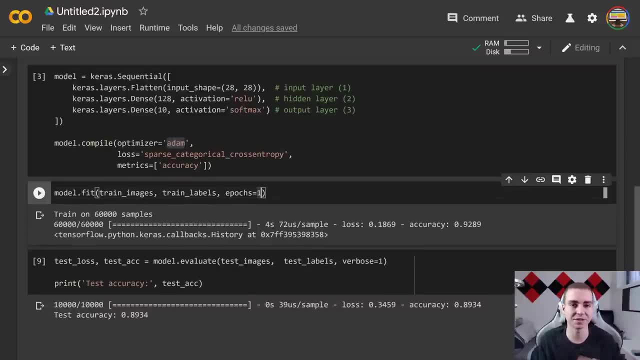 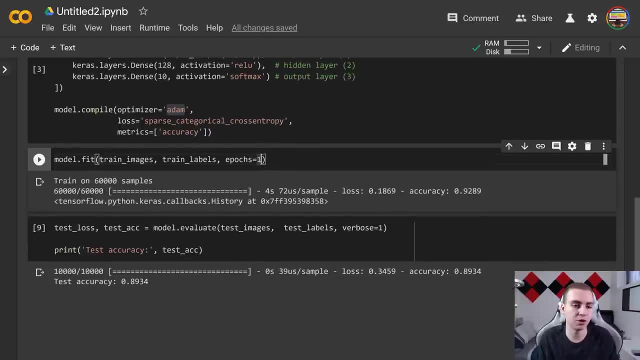 you're going to have a worse model, because what's going to end up happening is it's going to be seeing the same information, Much tweaking. so specifically to that information that it's seen that when you show it new data, it can't actually, you know, classify and generalize on that. Alright, so let's go back. 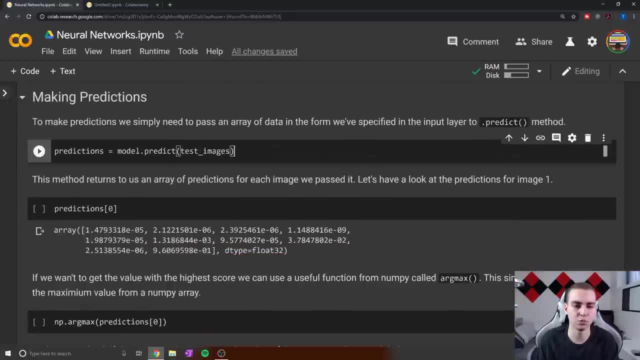 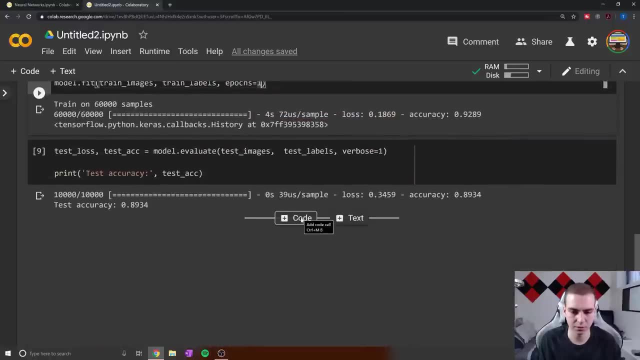 and let's see what else we're doing now with this. Okay, so now that we've done that, we need to make predictions. So to make predictions is actually pretty easy. So I'm actually just going to copy this line in: we'll go into a new code block down here. So all you have. 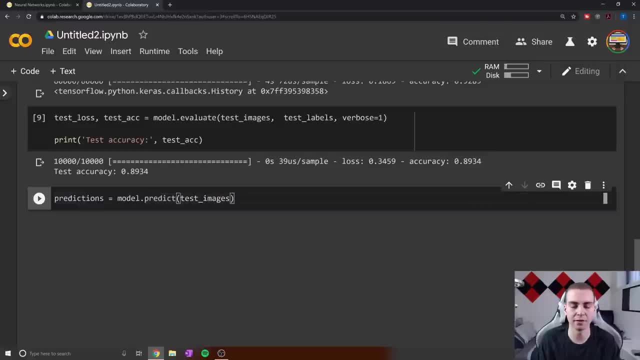 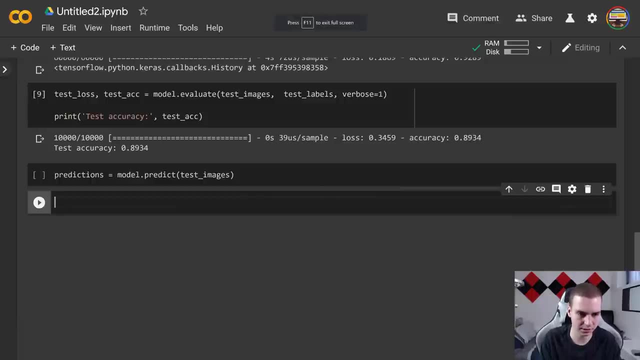 to do is say model dot, predict, and then you're going to give it an array of images that you want to predict on. So in this case, if we look at test images shape, so actually let's make a new code block And let's go here. So let's say test underscore images dot shape. Alright, give. 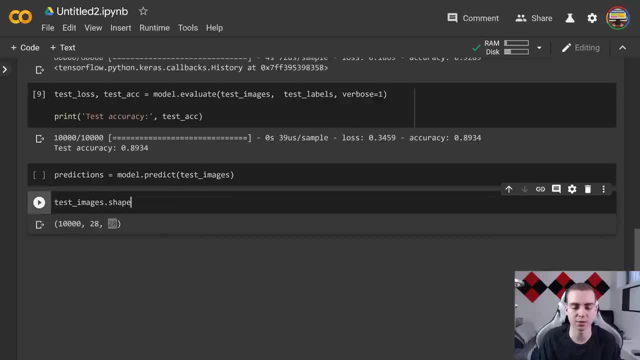 me a second. So we have 10,000 by 28 by 28.. So this is an array of 10,000 entries of images. Now, if I just wanted to predict on one image, what I could do is say: test images zero and 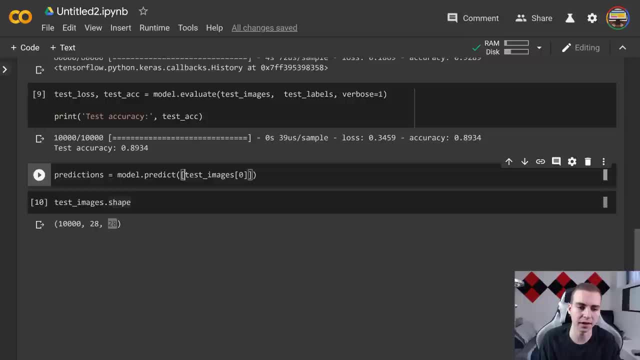 then put that inside of an array. The reason I need to do that is because the data that this model is used to seeing is an array of images to make a prediction on. That's what this predict method needs, And it's much better at making predictions on many things at once. 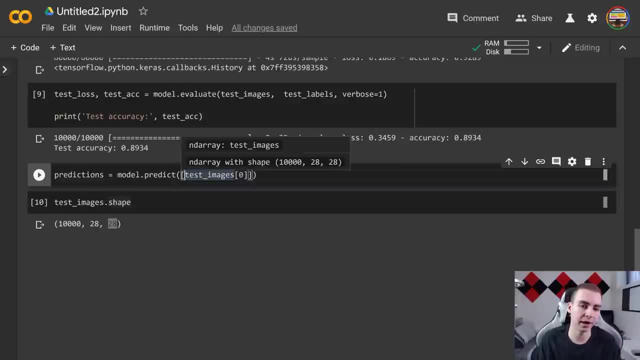 than just one specific item. So if you are predicting one item only, you do need to put it in an array, because it's used to seeing that form. So we could do this. I'm I mean, I'm just going to leave it. So we're just going to predict on every single one of the 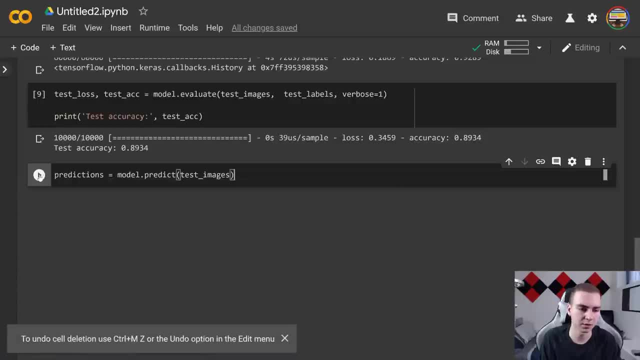 test images, because then we can have a look at a cool function I've kind of made. So let's actually do this. predictions equals model dot- predict test images. I mean that's pretty, that's pretty cool, So let's go ahead and do that. So let's go ahead and do that. So 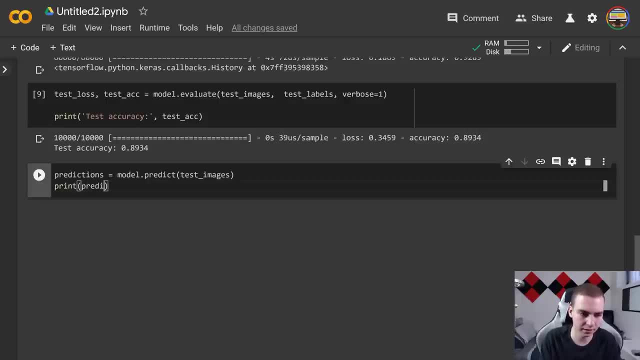 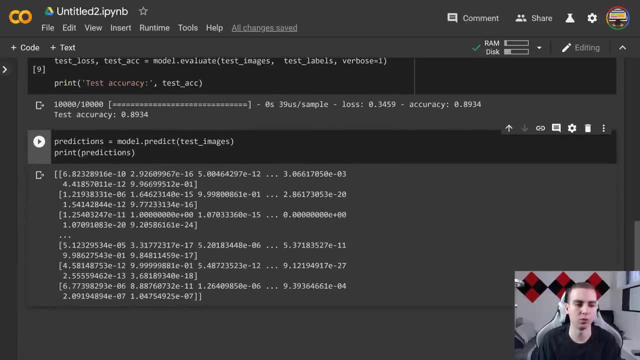 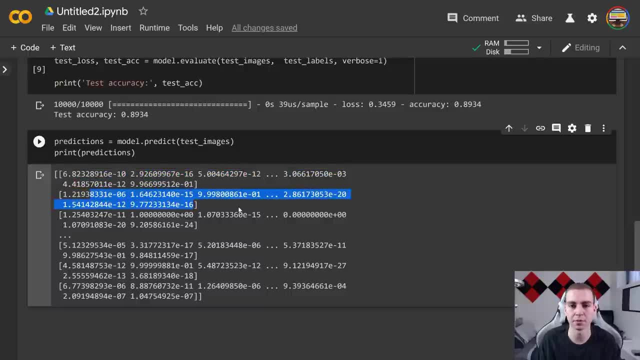 of arrays That looks like we have some like really tiny numbers in them. So what this is is essentially every single you know prediction, or every single image has a list that represents the prediction for it, just like we've done with kind of the linear models. 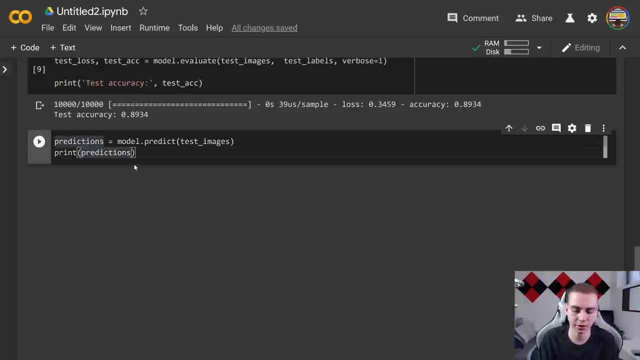 and stuff like that. So if I want to see the prediction for test image zero, I'm going to say prediction zero. right, Let's print this out. And this is the array that we're getting these. this is the probability distribution that was calculated on our output layer for. 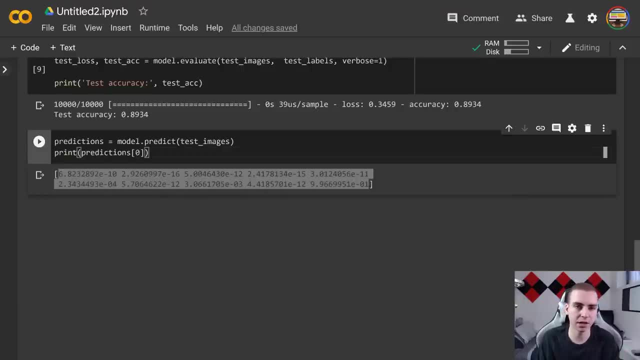 you know these? what is it for that image? So if we want to figure out what class we actually think that this is predicting for, we can use a cool function from NumPy called arg max, which essentially is just going to take the index this is going to return to. 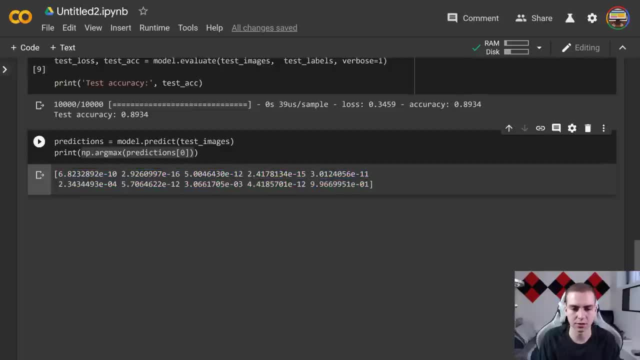 us the index of the maximum value in this list. So let's say, Say that it was. I'm looking for the least negative, which I believe is this: So this should be nine, This should return to us nine, because this is the index of the highest value. 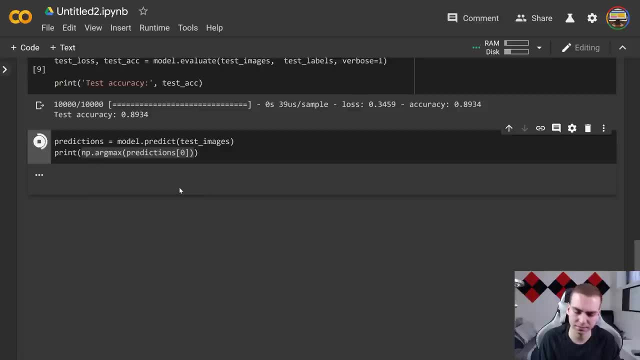 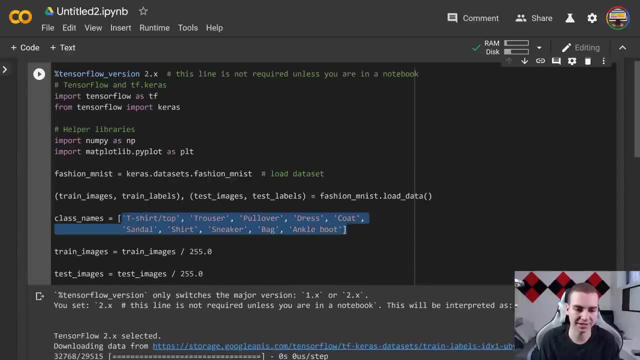 in this list, unless I'm just wrong when I'm looking at the negatives here. So nine, that's what we got. Okay. So now, if we want to see what the actual class is, well, we have our class names up here, So we know class nine is actually ankle boot, So let's see if this. 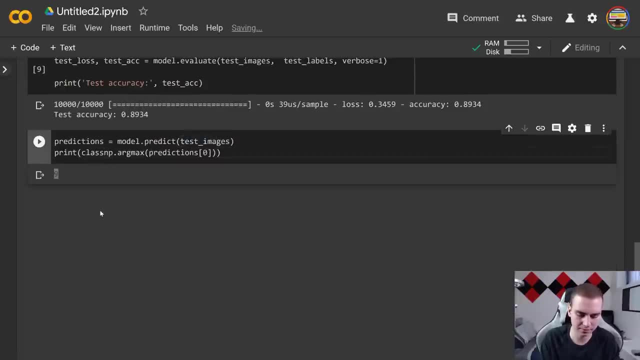 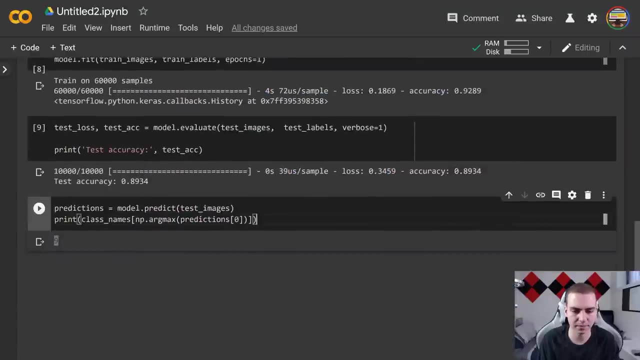 is actually an ankle boot, So I'm just going to do class underscore names. I think it's what I called it like this. So that should print out what it thinks it is. Yeah, class underscore names. But now let's actually show the image of this prediction. So to do. 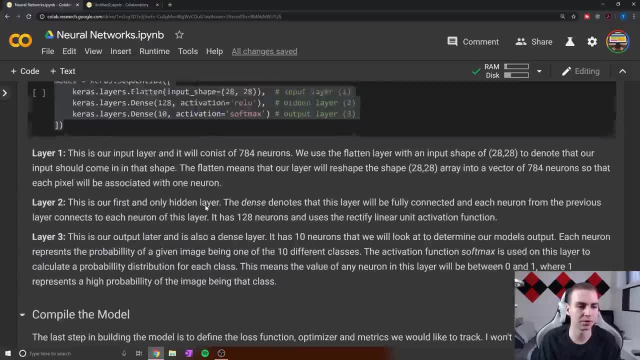 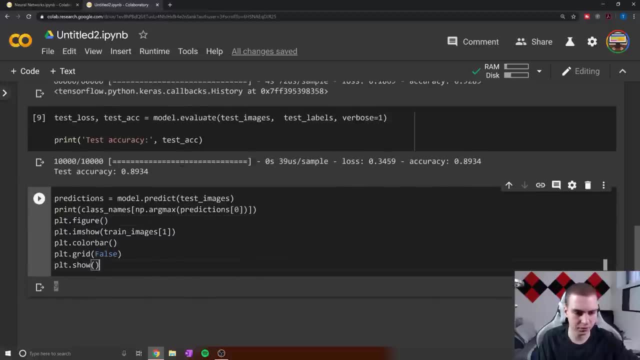 that I'm just going to steal some code from here because I don't remember all the syntax off the top of my head. So this: So let's steal this figure, Let's show this and let's see if it actually looks like an ankle boot. So to do that, we're going to say test underscore. 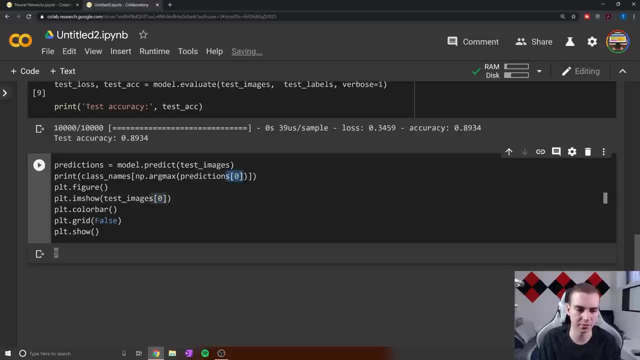 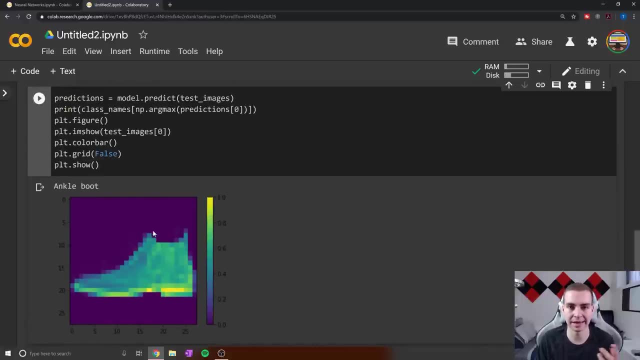 images zero, because obviously image zero corresponds to prediction. So we're going to say: image zero corresponds to prediction zero. And now we'll show this and see what we get. Okay, so ankle boot, and we'll be looking at the image is actually an ankle. 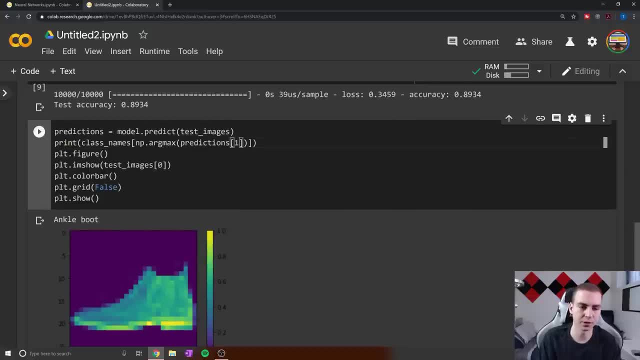 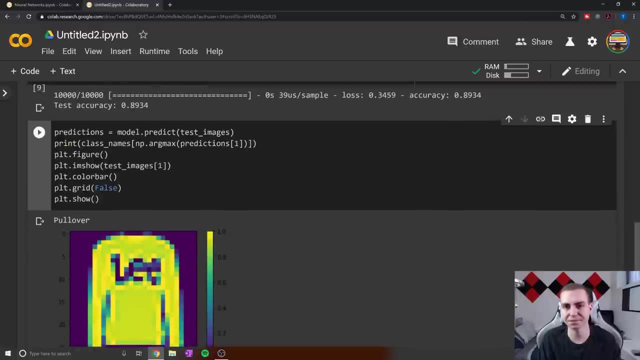 boot, And we can do this for any of the images that we want, Right? So if I do prediction one, prediction one, Now let's have a look pull over, the kind of looks like a pull over to me. I mean, I don't know if it actually is, but that's what it looks like. We do to. 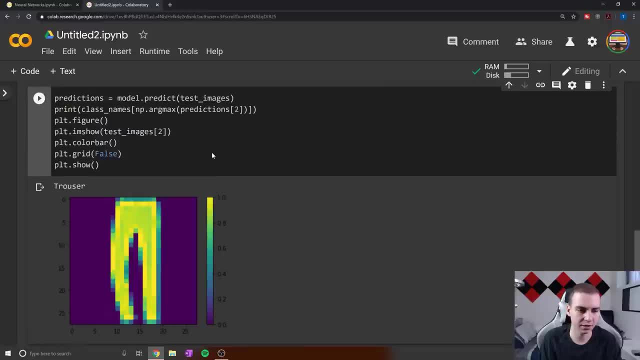 to have a look here. Okay, trouser- Yep, looks like trousers to me And we can see that that is how we get the image. So we're going to do this. So we're going to do this, So we're. 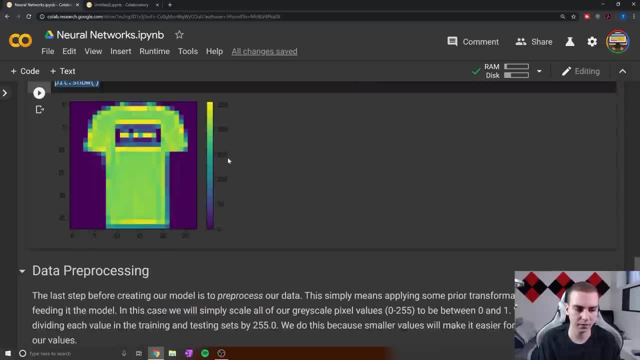 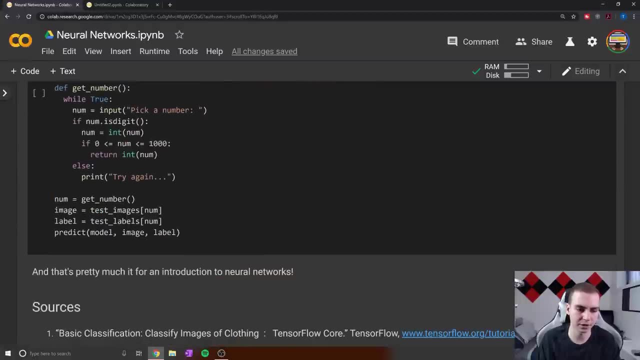 going to get the predictions for our model. we use model dot predict. Alright, so let's move down here now to the next thing that we did. Alright, so we've already done that. So verifying predictions. Okay, so this is actually a cool kind of script that I wrote. 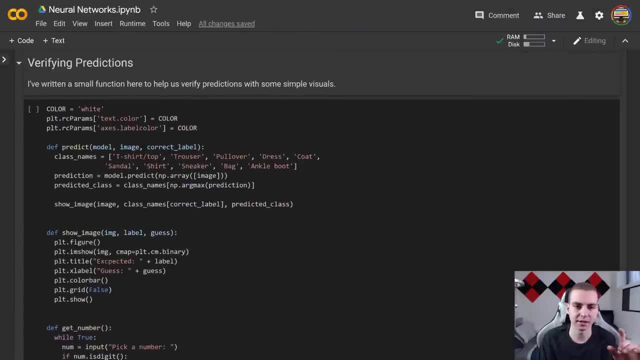 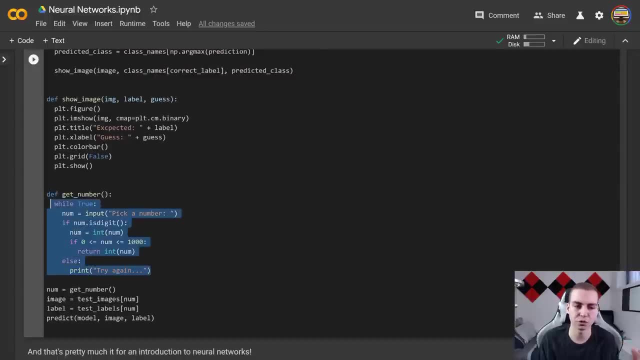 I'll zoom out a little bit so we can read it. What this does is let us use our model to actually make- and I've still some of this from TensorFlow- to make predictions on any entry that we want. So what it's going to do is ask us to type in some number. we're 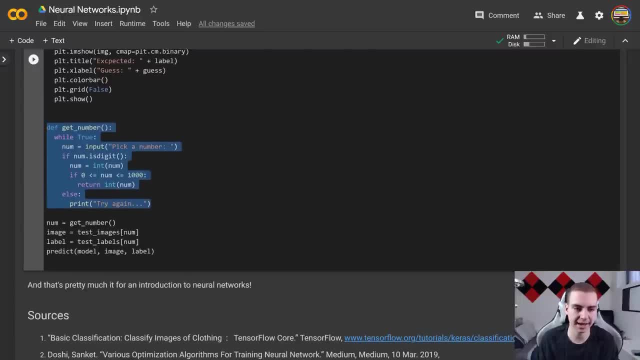 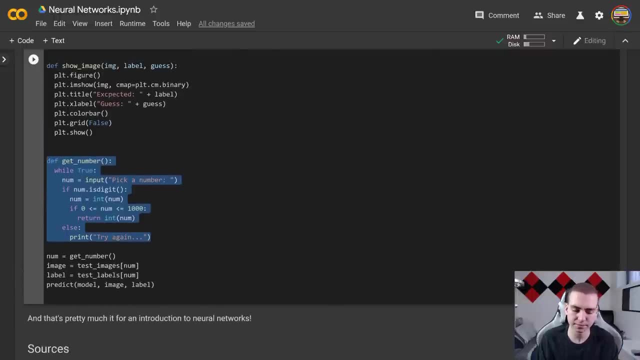 going to type in that number. it's going to find that number And then we're going to find that image in the test data set. it's going to make a prediction on that from the model and then show us what it actually is versus what it was predicted being. Now I 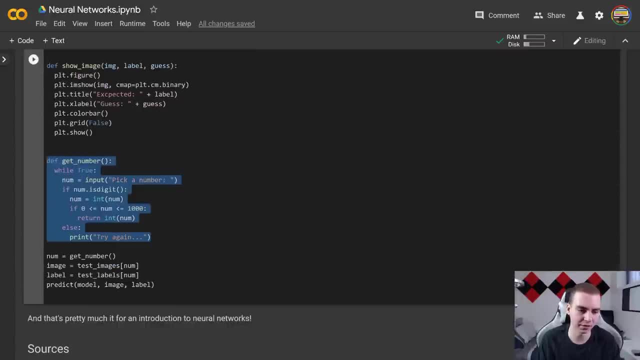 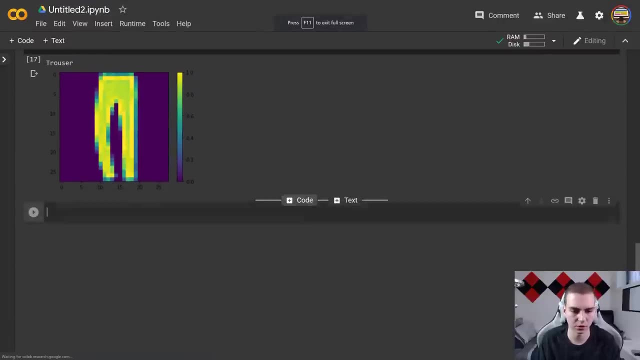 just need to actually run. Actually, let's just steal this code and bring it in the other one. So I've already trained the model there, So we don't have to wait again. So let's go f 11. F 11. Let's go to a new code block and run that. So let's run this script: Have. 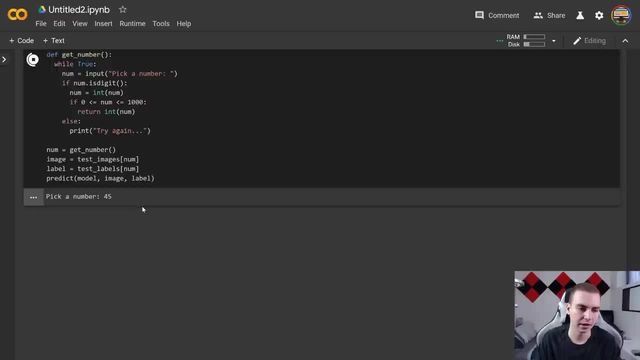 a look down here. So pick a number. we'll pick some number. let's go 45. And then what it's going to do is say: expected sneaker, guess sneaker, and actually show us the image that's there So we can. 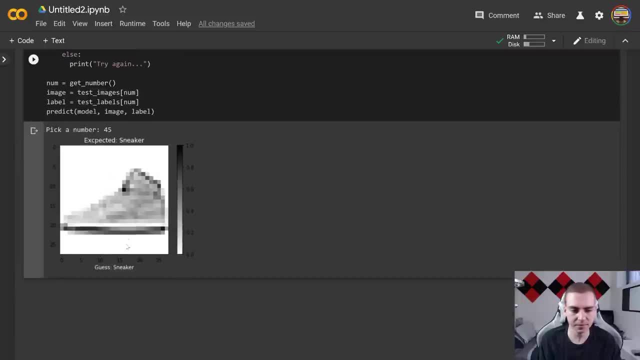 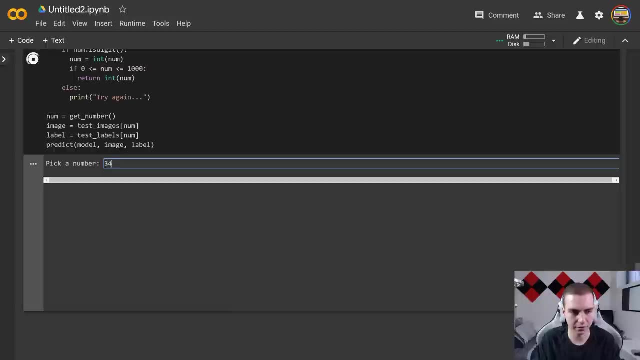 see, this is what you know, our pixel kind of data looks like And this is what the expected was And this is what the guest was from the neural network. Now we can do the same thing if we run it again, pick a number 34.. Let's see here: expected bag, guest bag. So that's. 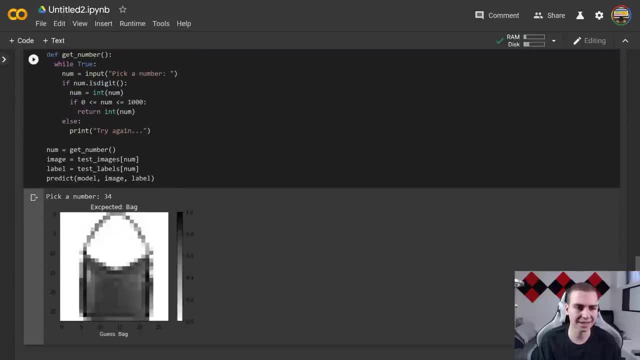 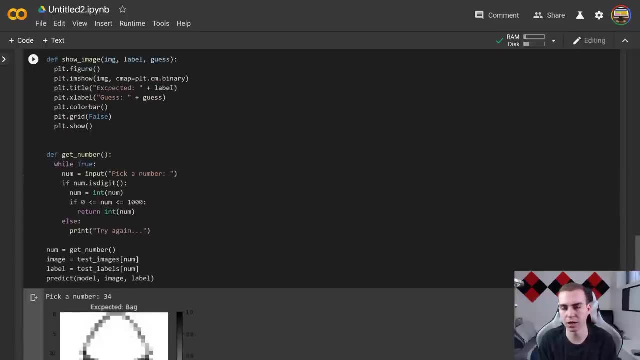 kind of showing you how we can actually use this model. So, anyways, that has been it for this kind of module on neural networks Now. I did this in about an hour. I'm hoping that I explained a good amount, that you guys understand now how neural networks work. In the next, 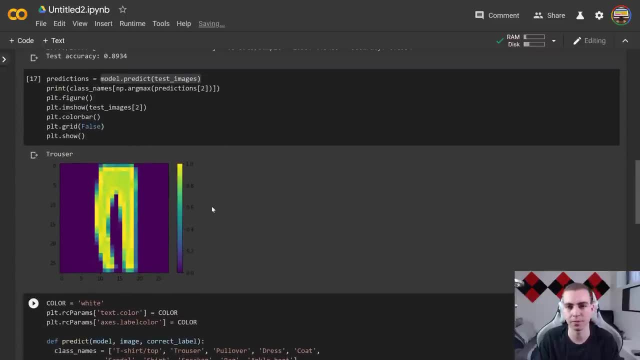 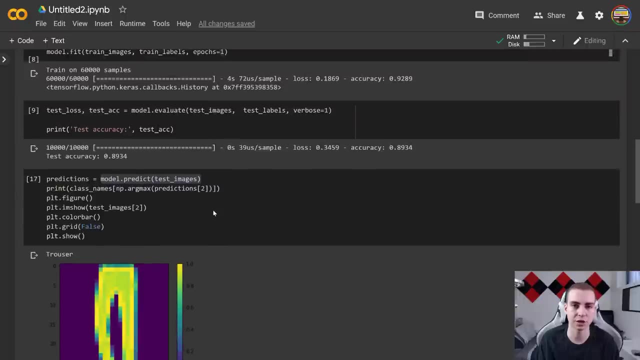 module, we're going to move on to convolutional neural networks, which again should help, you know, kind of get your understanding of neural networks up, as well as learn how we can do deep computer vision, object recognition and detection using convolutional neural networks. 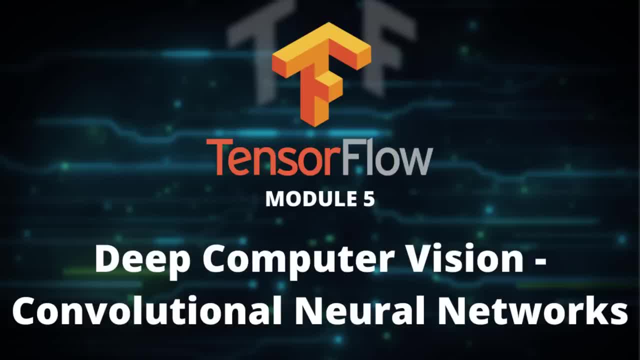 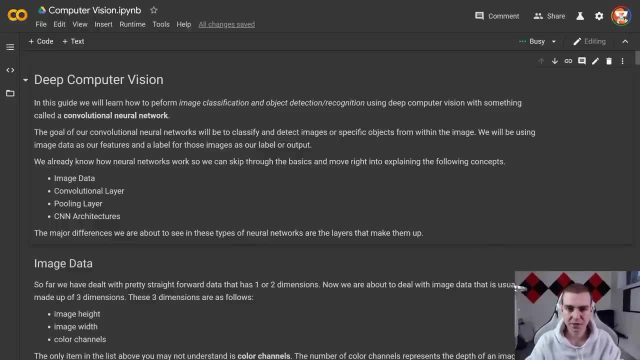 So, with that being said, let's get into the next module. Hello everyone, and welcome to the next module in this TensorFlow course. So what we're gonna be doing here is talking about deep computer vision, Which is very exciting, very cool. This has been used for all kinds of things you ever 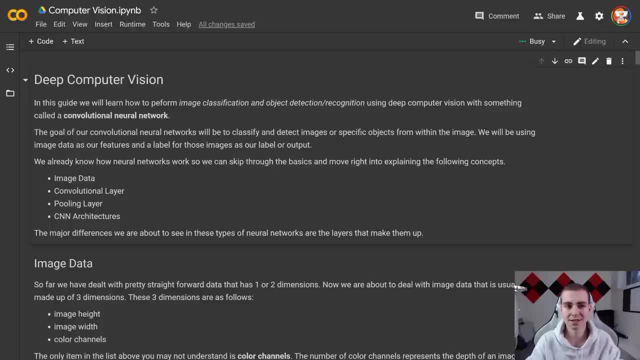 seen the self driving cars, for example Tesla. they actually use a TensorFlow deep learning model, are obviously very complicated- more than I can really explain here- to do a lot of their computer vision for self driving. We've used computer vision in the medicine field. computer vision is actually used in sports a lot for things like goal line technology. 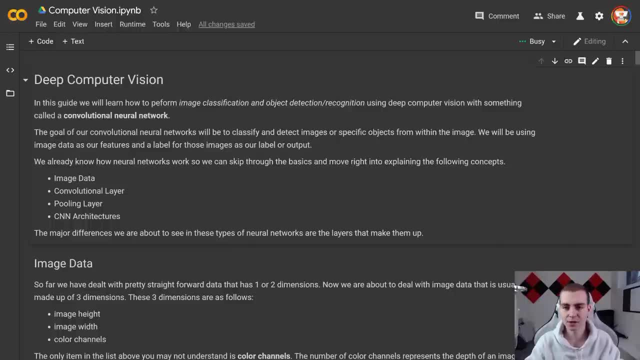 and even detecting images and players on the field doing analysis. there's lots of cool things they're doing with it nowadays And for our purposes. what we're gonna be doing is using this for to perform classification, although it can be used for object detection. 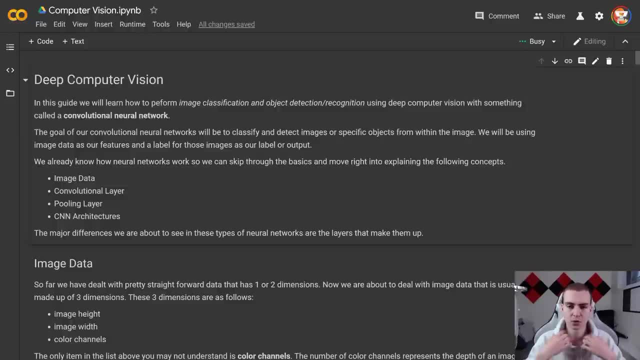 and recognition, as well as facial detection and recognition as well. So all kinds of applications. in my opinion, one of the cooler things in deep learning that we're doing right now And let's go ahead and talk about we're actually going to be focusing on here, So we're going. 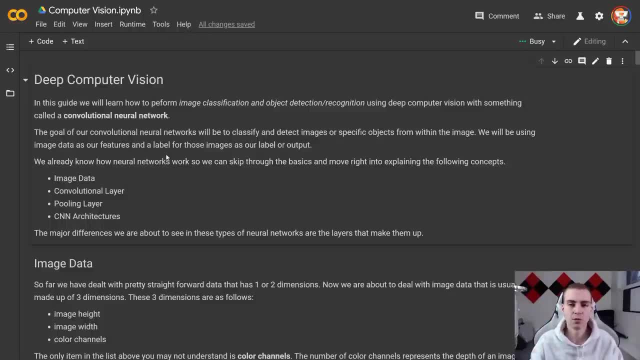 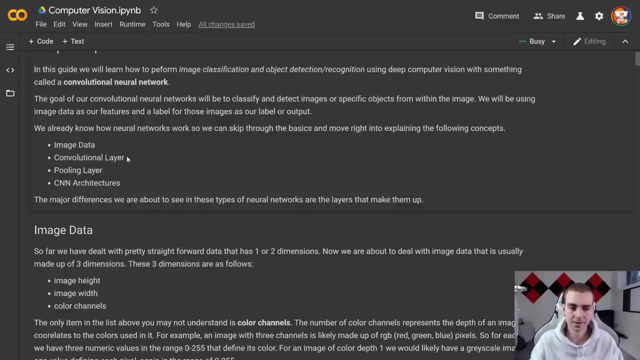 to start by discussing what a convolutional neural network is, which is essentially the way that we do deep learning. we're going to learn about image data, So what's the difference between image data and other regular data? we're gonna talk about convolutional layers. 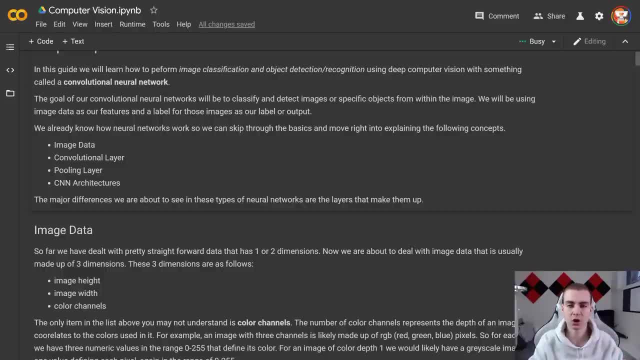 and pooling layers and how stacks of those work together as what we call a convolutional base for our convolutional neural network. And we're going to talk about CNN architectures and get into actually using pre trained models that have been developed by companies such as Google. 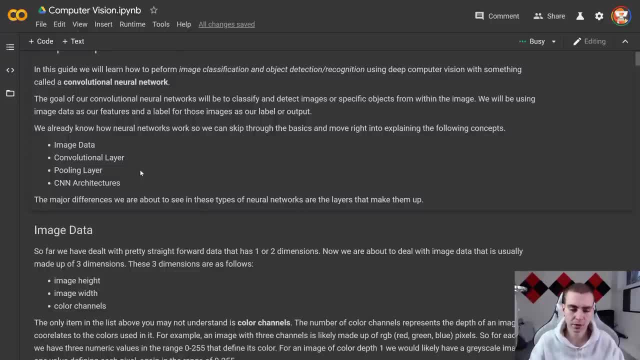 and TensorFlow themselves to perform classification tasks for us. So that is pretty much the breakdown of what we're about to learn. there's quite a bit in this module. it's probably the more difficult one, or the most difficult one we've been doing so far. So if you do get lost at 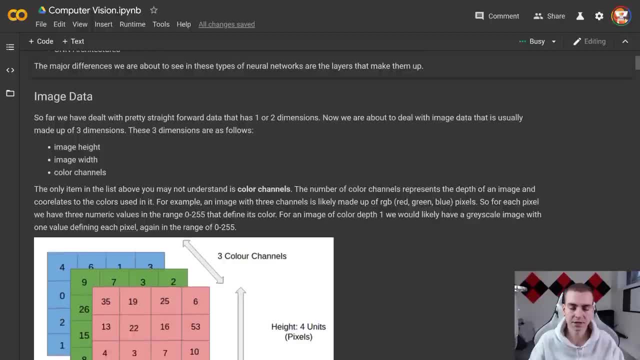 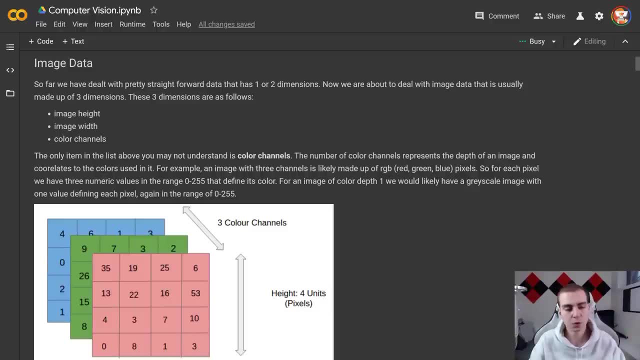 any point or you don't understand some of it. don't feel bad. this stuff is very difficult And I would obviously recommend reading through some of the descriptions I have here in this notebook, which again you can find from the link in the description or looking up some. 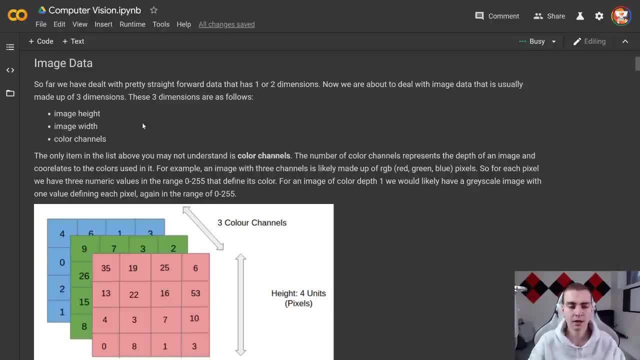 things that maybe I don't go into enough enough depth about in your own time, as I can't really spend, you know, 1011 hours explaining a convolutional neural network. So let's now talk about image data, which is the first thing we need to understand. So, in our previous examples, what 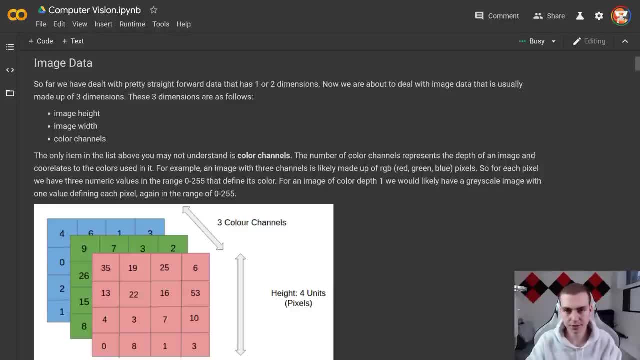 we did with when we had a neural network is we had two dimensional data right, we had a width and a height when we were trying to classify some kind of images, you know, using a dense neural network. And well, that's what we use: two dimensions. well, with an 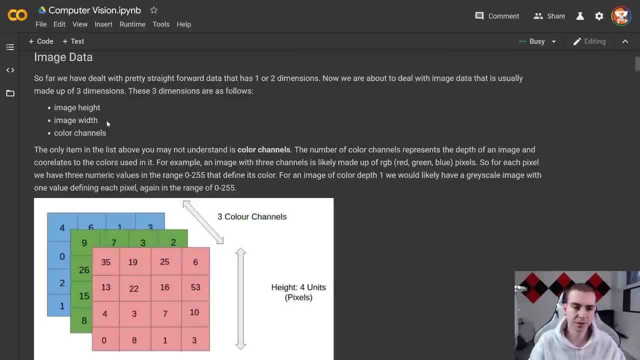 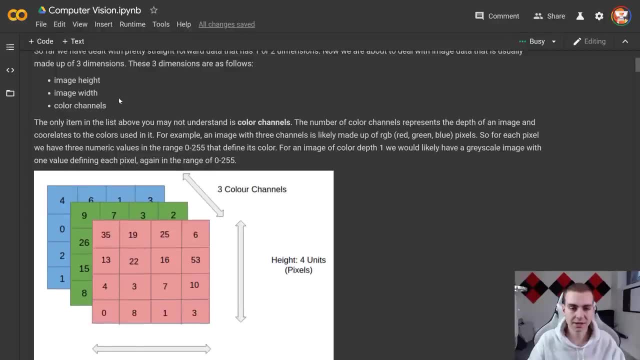 image. we actually have three dimensions, And what makes up those dimensions? Well, we have a height and we have a width, And then we have something called color channels. Now, it's very important to understand this, because we're going to see this a lot as we 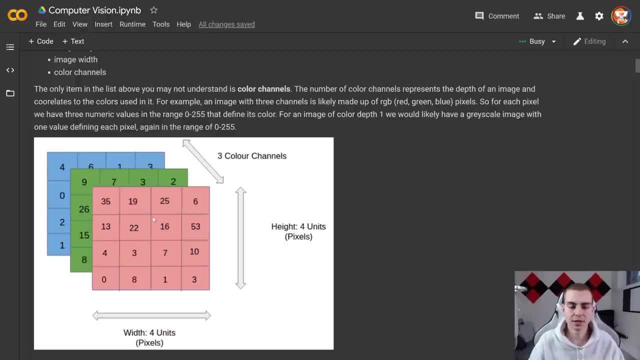 get into convolutional networks, that the same image is really represented by three specific layers. right, We have the first layer, which tells us all of the red values of the pixels, the second layer, which tells us all the green values, And the third layer which tells us all the blue values. So in this case, those are the. 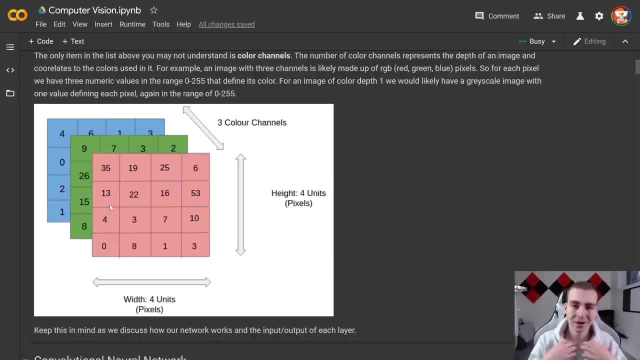 colored channels And we're going to be talking about channels in depth quite a bit in this series. So just understand that although you think of an image as a two dimensional kind of thing and our computer, it's really represented by three dimensions where these channels 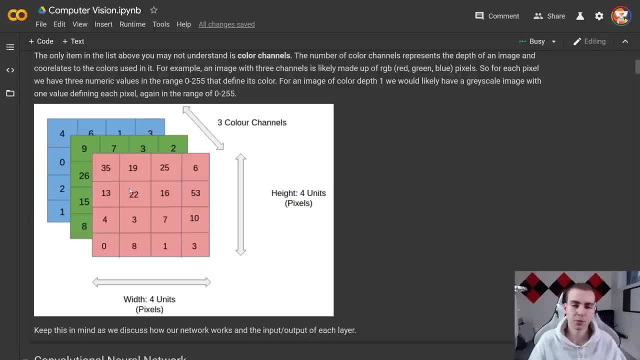 are telling us the color of each pixel, Because, remember, in red, green, blue, you have three values for each pixel, which means that you're going to need three layers to represent that pixel, right? So this is what we can kind of think of it as a 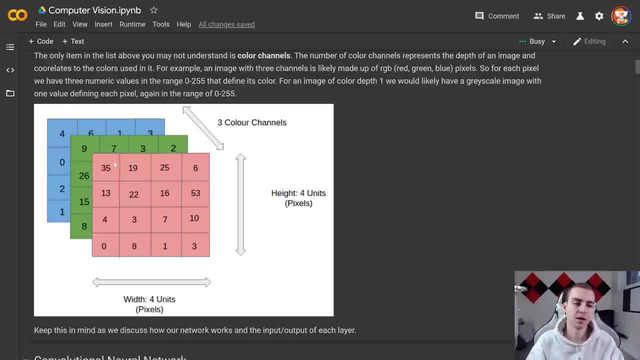 stack Of layers and, in this case, a stack of pixels, right, or stack of colors, really telling us the value for each pixel. So if we were to draw this to the screen, we would get the blue, green and red values of each pixel, determine the color of it and then draw the. 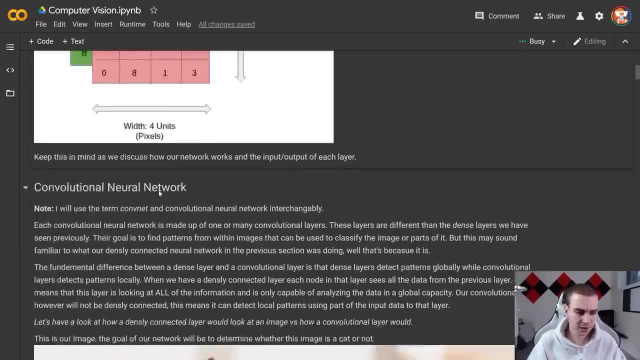 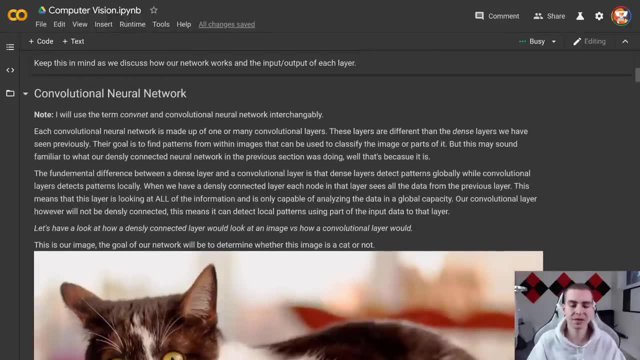 two dimensional image right, based on the width and the height. Okay, so now we're gonna talk about a convolutional neural network and the difference between that in a dense neural network. So in our previous examples, when we use the dense neural network to do some, 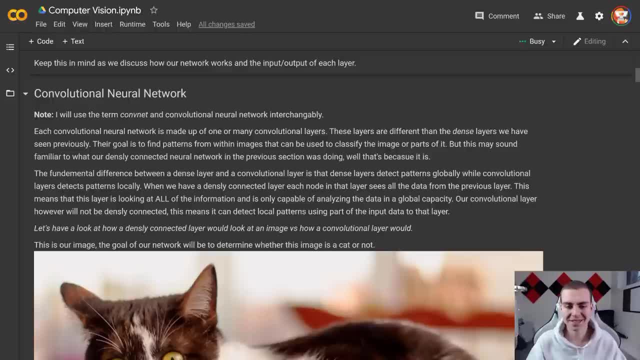 kind of image classification like that fashion MNIST, and then we're going to talk about this data set. what it essentially did was look at the entire image at once and determined, based on finding features in specific areas of the image, what that image was right, Maybe. 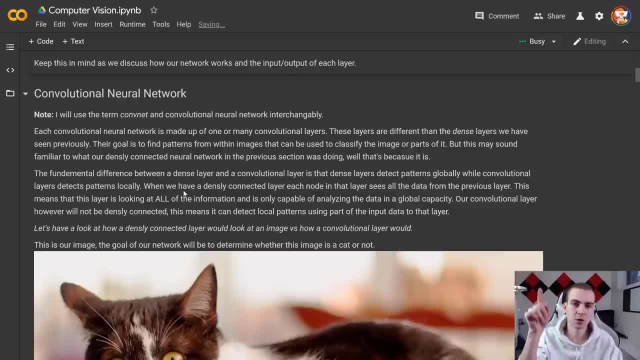 it found an edge here, a line here, maybe it found a shape, maybe it found a horizontal, diagonal line. The important thing to understand, though, is that when it found these patterns and learned the patterns that made up specific shapes, it learns them in specific areas. 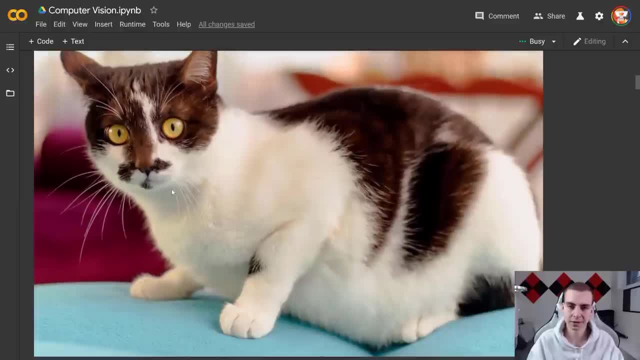 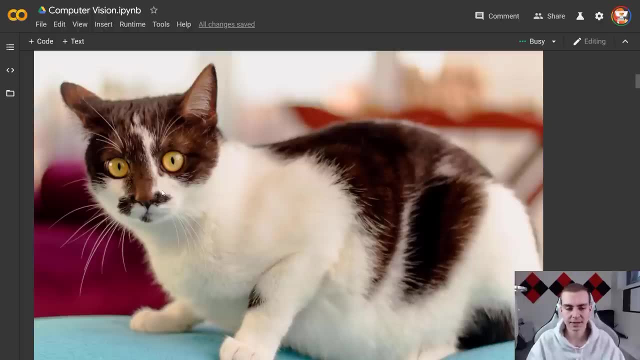 it knew that if we're in between, for example looking at this cat image, we're gonna classify this as a cat. If an eye exists on, you know, the left side of the screen where the eyes are here, then that's a cat. it doesn't necessarily know that if we flip this cat, we did a horizontal. 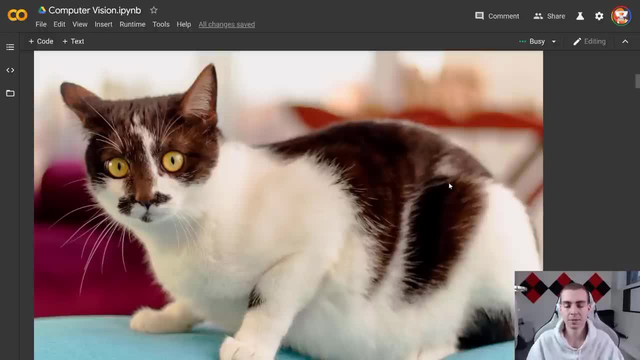 flip of this cat, and the eyes were over here that that is a pattern that makes up a cat. So the idea is that the dense network looks at things globally. it looks at the entire image and learns patterns in specific areas. That's why we need things to be centered. 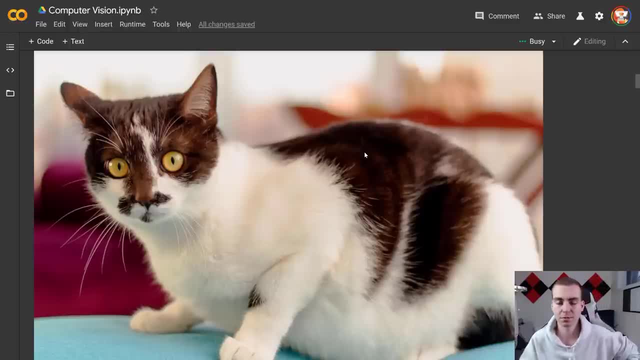 we need things to be very similar when we use a dense neural network to actually perform image classification. Okay so, because you cannot learn local patterns and apply those to different areas of the image. So, for example, some patterns we might look for when we're looking at an image like 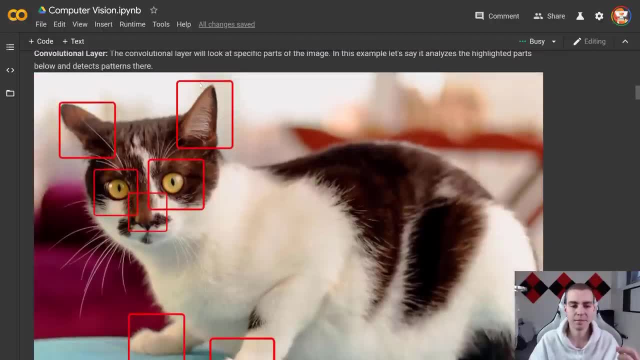 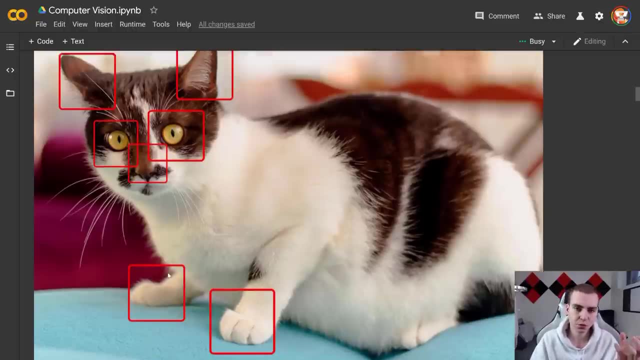 a cat here would be something like this: right, we would hope that maybe we could find a few ears, we could find the eyes, the nose and you know the pause here- And those features would tell us that this makes up a cat Now, with a dense neural network. it would find. 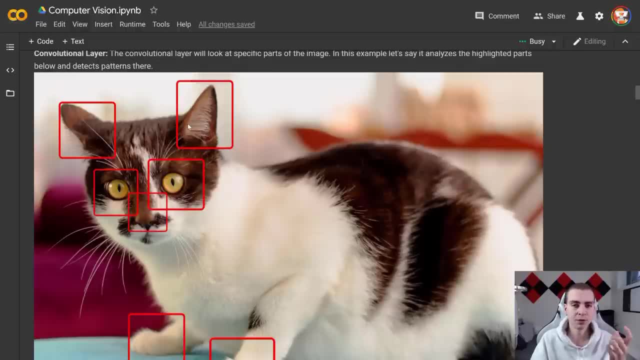 these features, it would learn them, learn these patterns. we're only learning them in this specific area where they're boxed off, which means if I horizontally flip this image right and I go like that, then it's not going to know that that's a cat because it learned that. 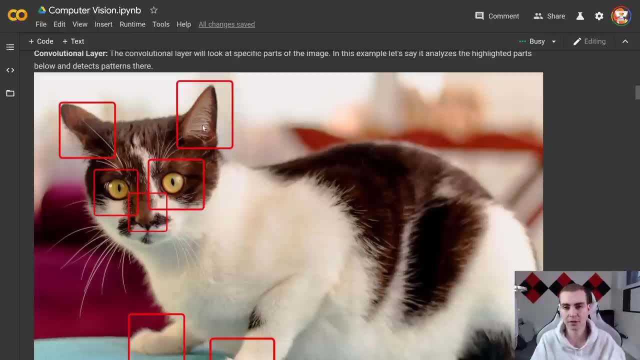 pattern in a specific area, it'll need to relearn that pattern in the other area. Now, a convolutional neural network, on the other hand, learns local patterns. So, rather than learning that the ear exists in you know this specific location, it just learns that. 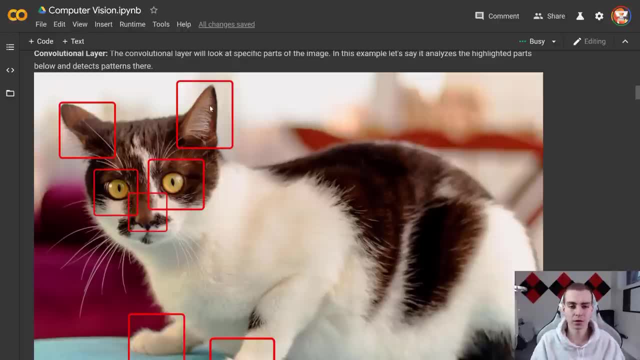 this is what an ear looks like, And it can find that anywhere in the image, And we'll talk about how we do that as we get to the explanation. But the whole point is, you know, the point is that our convolutional neural network will scan through our tire image. 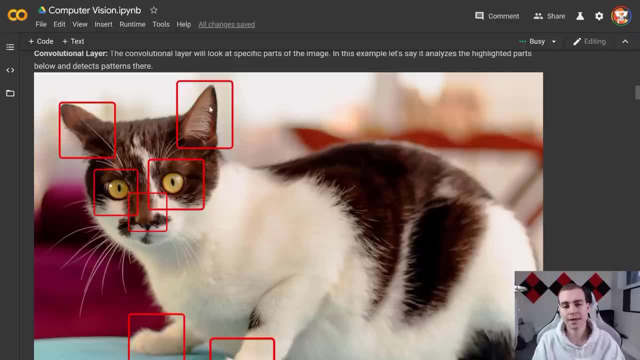 it will pick up features and find features in the image And then, based on the features that exist in that image, will pass that actually to a dense neural network or a dense classifier. it will look at the presence of these features and determine. you know, the combination of 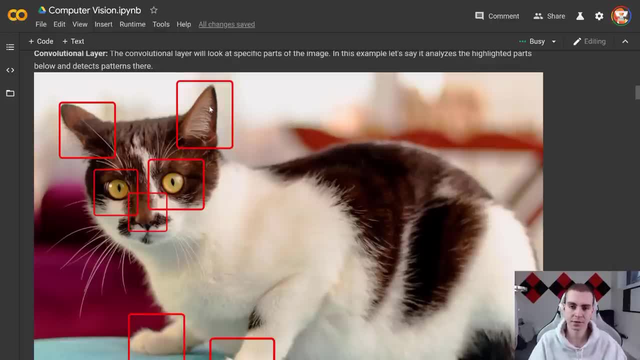 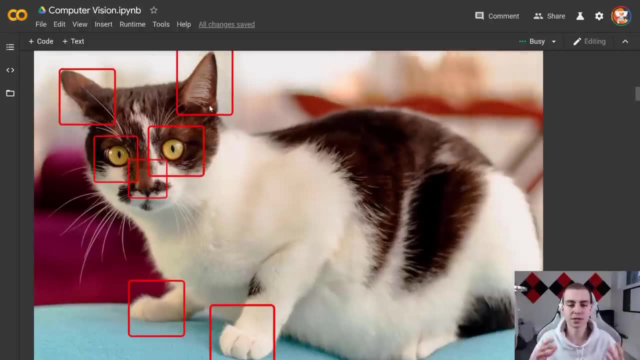 these presences of features that make up specific classes or make up specific objects. So that's kind of the point. I hope that makes sense. The main thing to remember is that dense neural networks work on a global scale, meaning they learn global scale, they learn global scale. 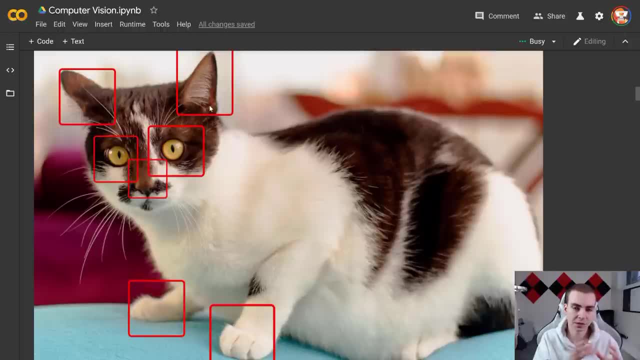 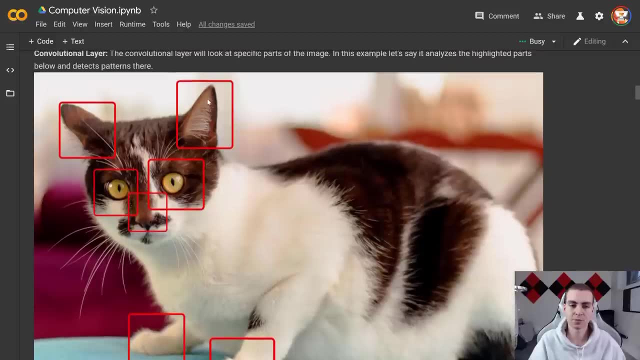 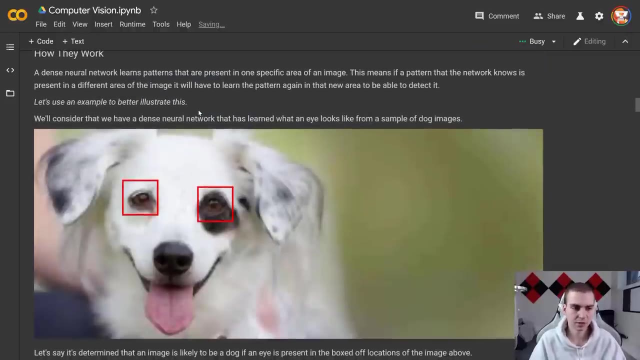 global patterns, which are specific and are found in specific areas, Whereas convolutional neural networks or convolutional layers will find patterns that exist anywhere in the image, because they know what the pattern looks like, not that it just exists in a specific area. Alright, so how they work, right? So let's see what a neural network, regular neural network. 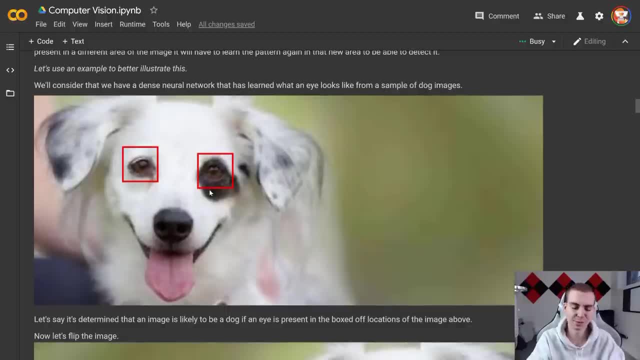 looks at this dog image, this is a good example. I should have been using this before. it will find that there's two eyes that exist here. right, And we'll say, Okay, so I found that these eyes make up a dog. this is its training image, for example, and it's like: okay, so this. 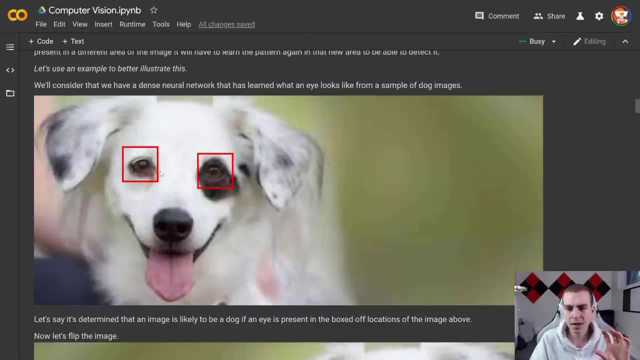 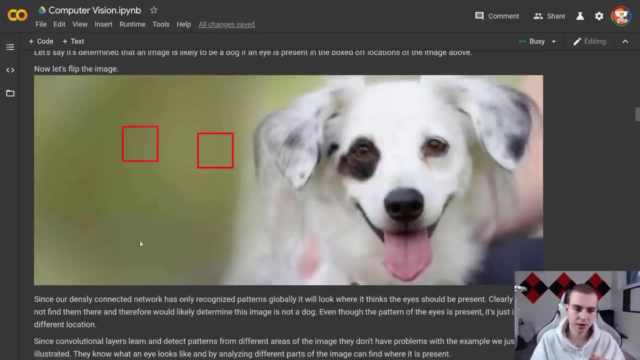 pattern makes up the dog. the eye is in this location. Now, what happens when we do this and we flip the image to the other side? Well, our neural network starts looking for these eyes right on the left side of the image, where it found them previously and where it was. 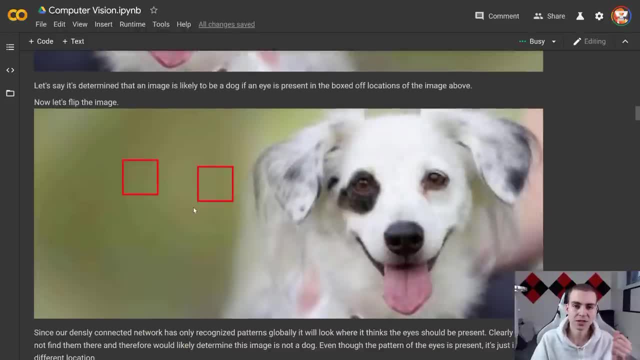 trained on it obviously doesn't find them there, And so it says that our image isn't a dog, although it clearly is a dog. it's just a dog that's orientated differently. In fact, it's just flipped horizontally right, Or actually, I guess I would say vertically. 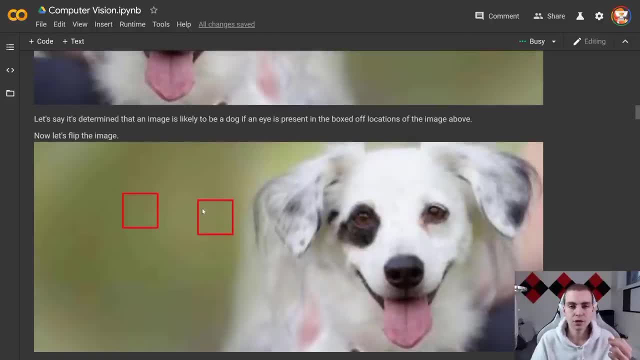 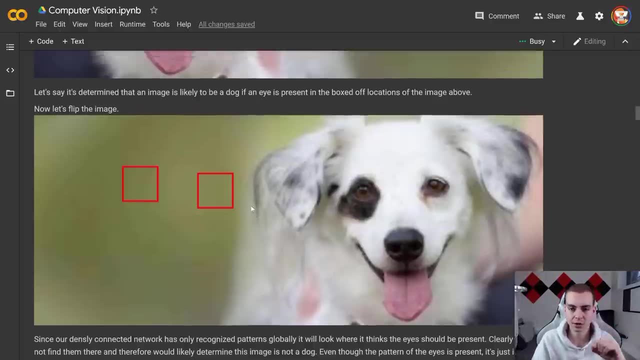 flipped vertically. So, since it doesn't find the eyes in this location and it can only look at patterns that it's learned in specific locations, it knows that this, or it's going to say this, isn't a dog, even though it is, whereas our convolutional layer will find: 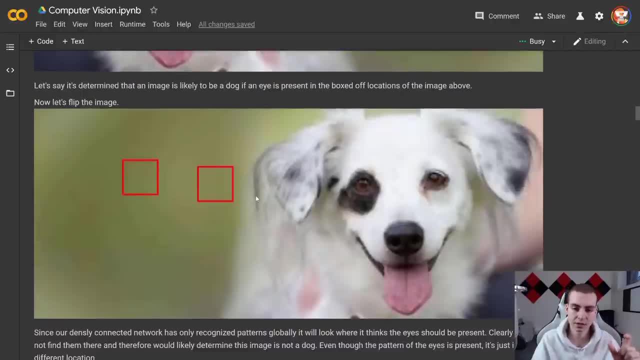 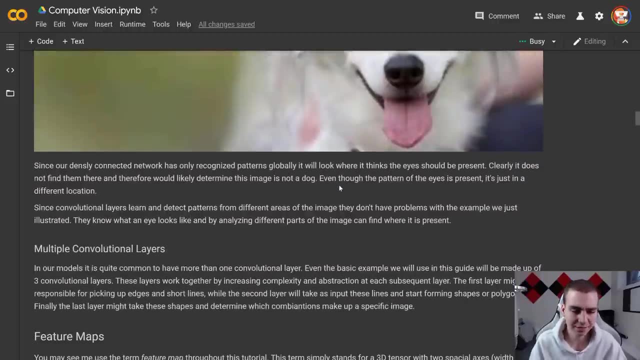 the eyes, regardless of where they are in the image, and still tell us that this is a dog, Because even though the dogs moved over, it knows what an eye looks like, So it can find the eye anywhere in the image. So that's kind of the point of the convolutional neural network. 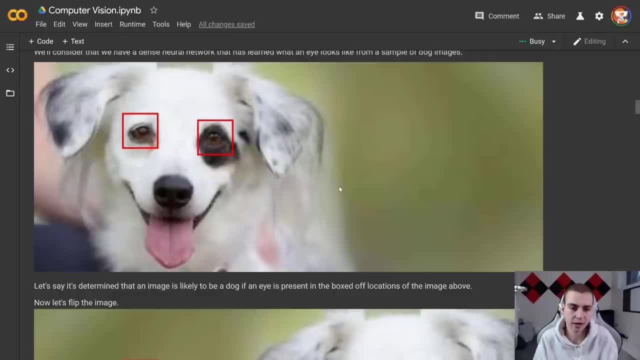 and the convolutional layer. And what the convolutional layer does is it's going to find the eyes in the image. I'm going to find the eyes in the image. So what you're going to find is that the eye will look from the outside up, but the eye is going to look from the inside out. So what? 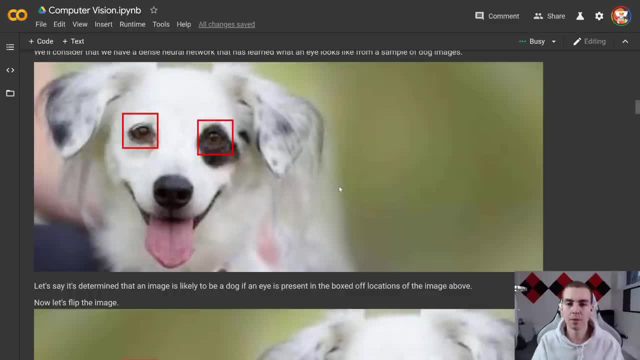 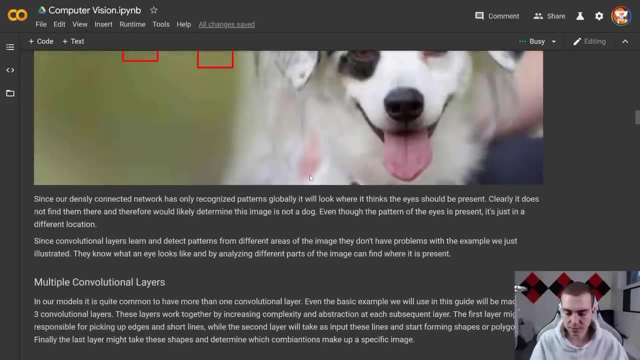 the convolutional layer does is look at our image and essentially feed back to us what we call an output feature map that tells us about the presence of specific features, or what we're going to call filters, in our image. So that is kind of the way that works Now. 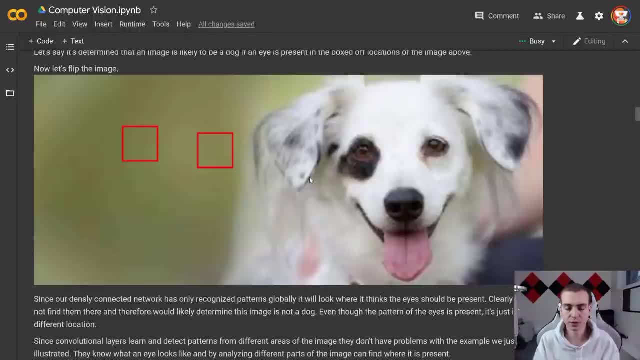 essentially, the thing we have to remember is that our dense neural networks output just a bunch of numeric values, whereas what our convolutional layers are actually going to be doing is outputting what we call a feature map. I'm going to scroll down here to show. 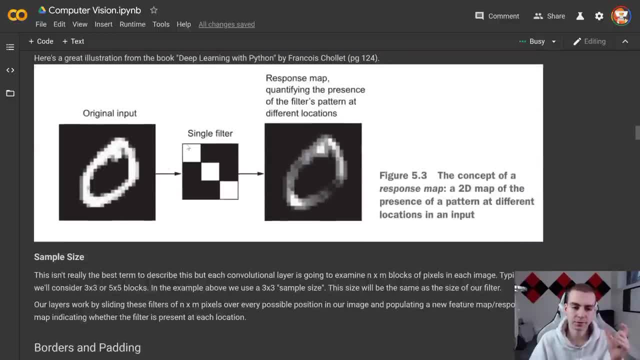 you this example. what we're actually going to do is we're going to have a bunch of workstation unique things that we could literally just import and like we can actually we've is run what we call a filter over our image. we're going to sample the image at all these. 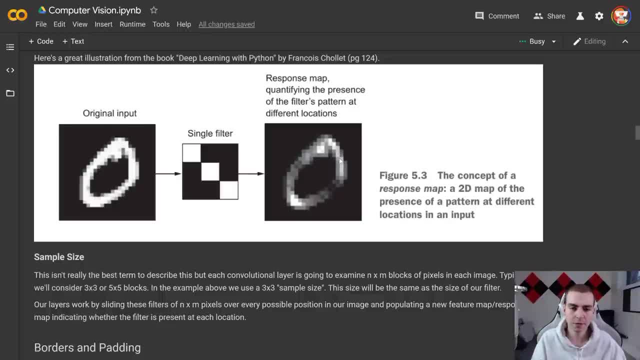 different areas, And then we're going to create what we call an output feature map that quantifies the presence of the filters pattern at different locations, And we'll run many, many, many different filters over our image at a time. So we have all these different feature maps. 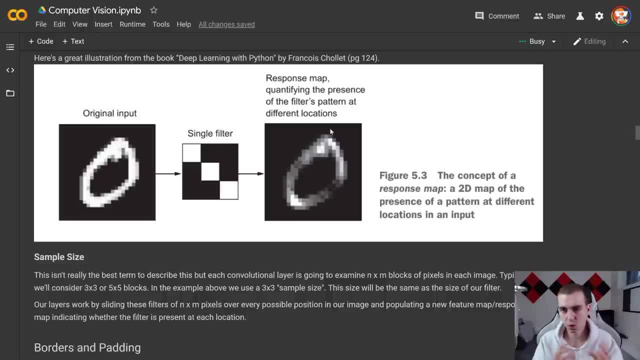 telling us about the presence of all these different features. So one convolutional layer. we'll start by doing that with very small, simple filters, such as straight lines like this, and then other convolutional layers on top of that. right, because it's going. 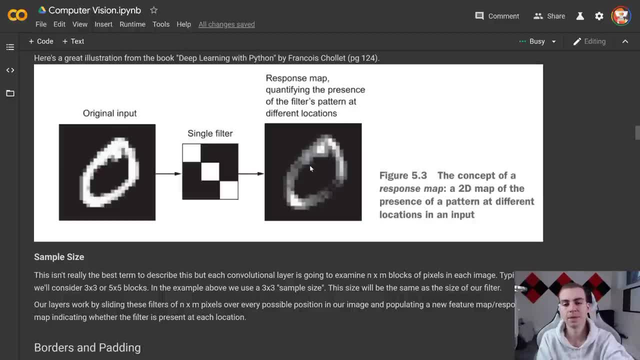 to return a map that looks something like this out of the layer, we'll take this map in now, the one that was created from the previous layer, and say, Okay, well, if this map is representing to me, for example, the presence of these diagonal lines, let me try to look. 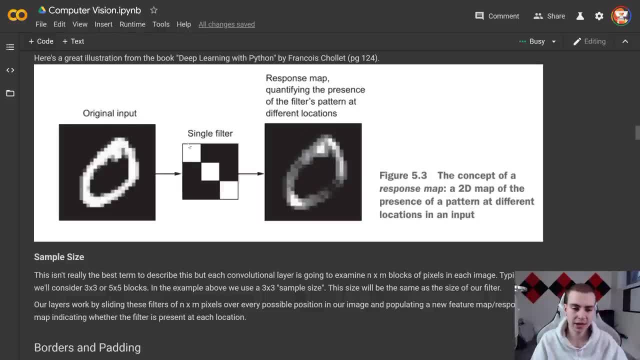 for curves, right. Or let me try to look for edges. So it will look at the presence of the features from the previous convolutional layer and then say, Okay, well, if I have all these lines combined together, that makes up an edge, and it will look for that. And 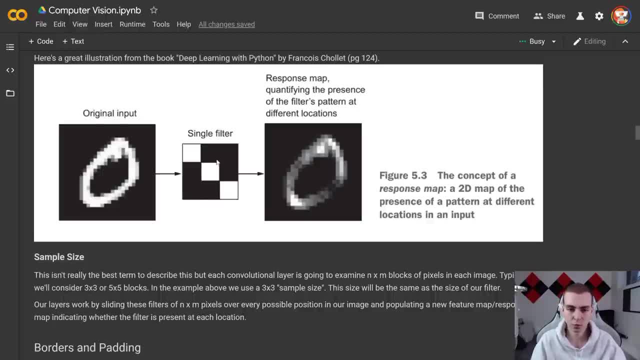 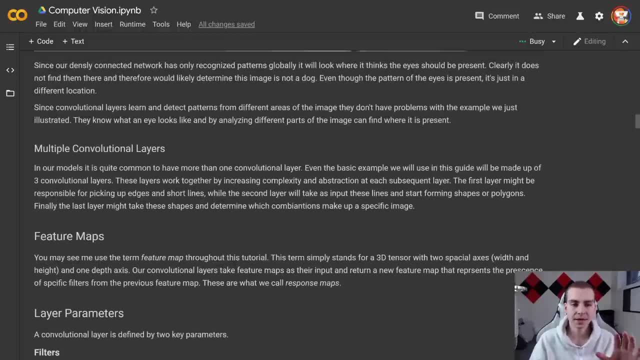 that's kind of the way that a convolutional neural network works and why we stack these different layers. Now we also use something called pooling, And there's a few other things that we're going to get into, But that is the basics. I'm going to go into a drawing. 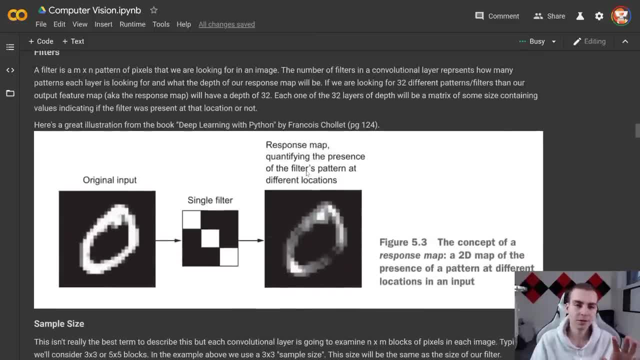 example and show you exactly how that works, But hopefully this makes a little bit of sense- that the convolutional layer returns a feature map that quantifies the presence of a filter at a specific location And this filter. the advantage of it is that we slide. 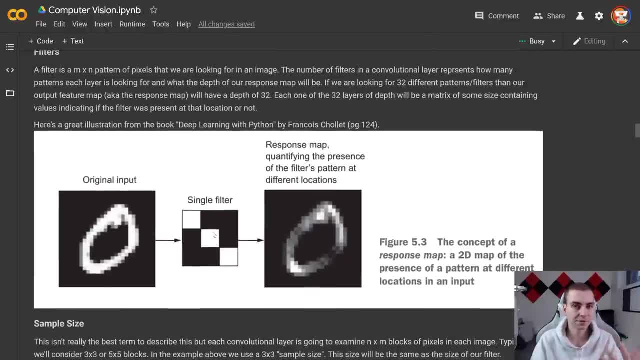 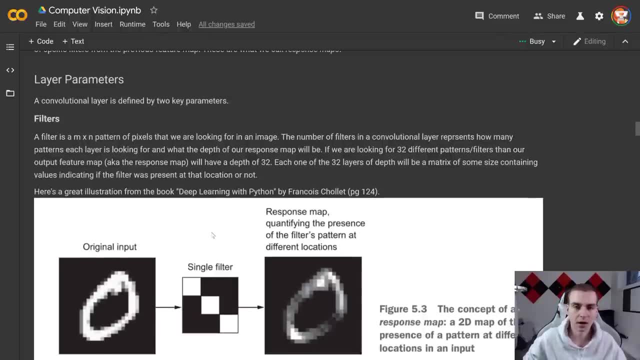 it across the entire image. So if this or this feature is present anywhere in the image, we will know about it, rather than in our dense network, where it had to learn that pattern in a specific global location. Okay, so let's get on the drawing tablet and do a few examples, Alright? so I'm here on my 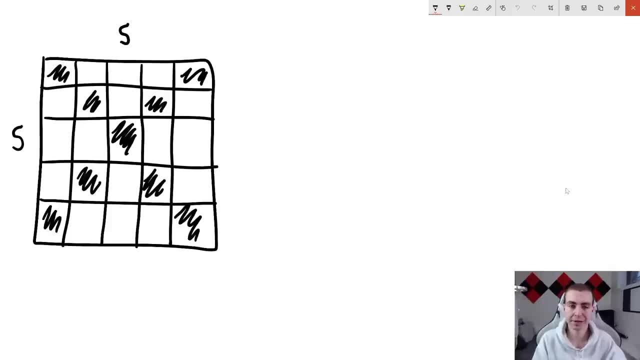 drawing tablet and we're going to explain exactly how a convolutional layer works and how the network kind of works together. So this is an image I've drawn on the left side of our screen here. I know this is very basic. you know this is just an x right. This is 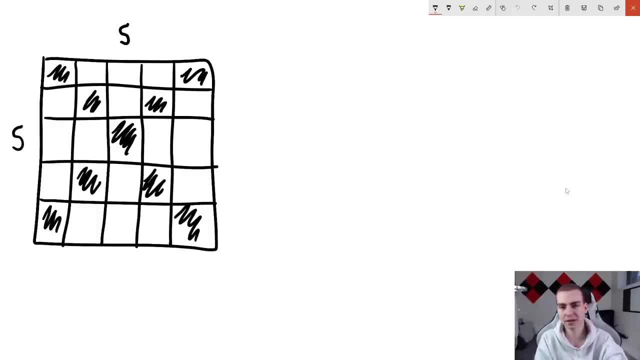 what our images. we're just going to assume this is grayscale. we're going to avoid doing anything with color channels- the second, just because they're not that important. But just understand that what I'm about to show you does apply to color channels as well, and to 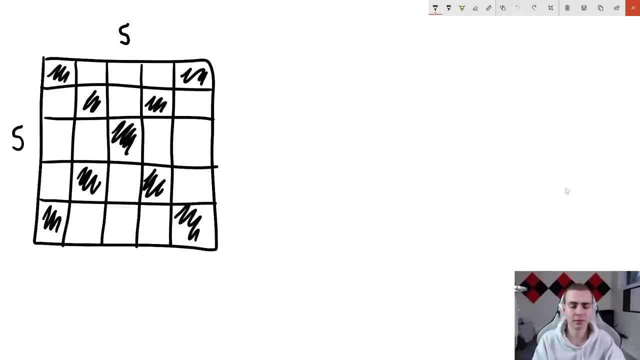 multiple kinds of layers and depth, And then, if we can understand it on a simple level, we should be able to understand it more thoroughly. So what we want essentially is our convolutional layer to give us some output that's meaningful about this image, So we're gonna assume this. 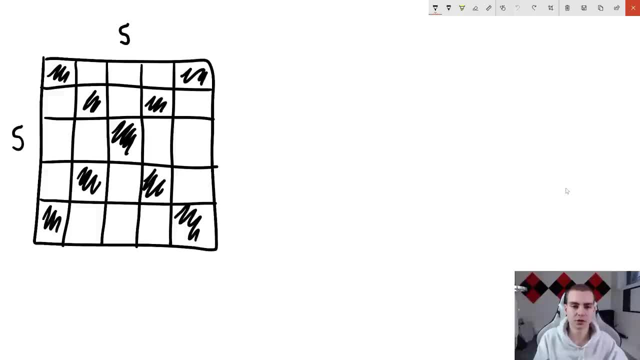 is the first convolutional layer And what it needs to do essentially is return to us some feature matter map that tells us about the presence of specific what we call filters in this image. So each convolutional layer has a few properties to it. The first one is going to be the input. 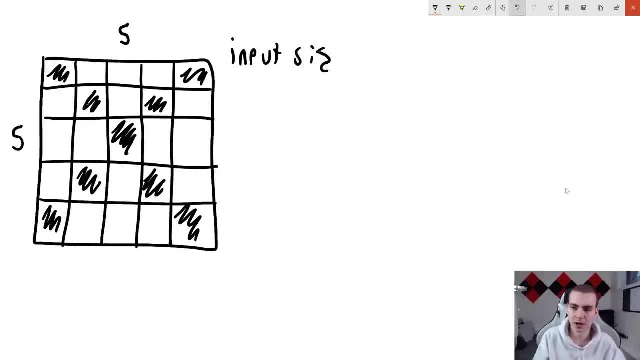 size. So what can we expect? Wow, what is that? that was as the as the input size. How many filters are we going to have? So filters like this, And what's the sample size of our filters? That's what we need to know For each of our convolutional 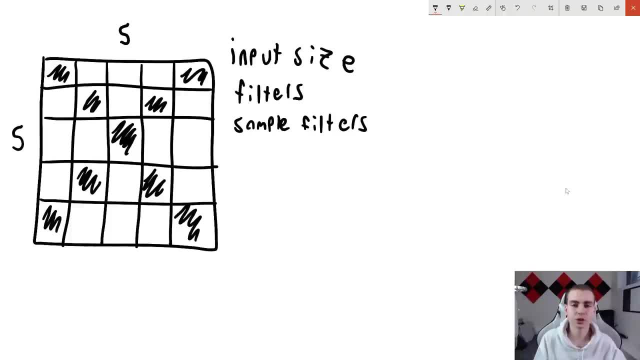 neural networks. So, essentially, what is a filter? Well, a filter is just some pattern of pixels, And we saw them before. we'll do a pretty basic one here as the filter we're going to look for, which will look something like this: This will be the first filter we're. 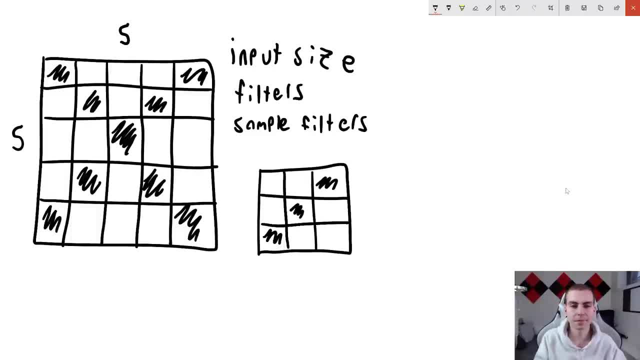 going to look for, just to illustrate how this works. But the idea is that at each convolutional layer we look for many different filters And in fact the number we're typically looking for is actually about times 32 filters. Sometimes we have 64 filters as well, And sometimes 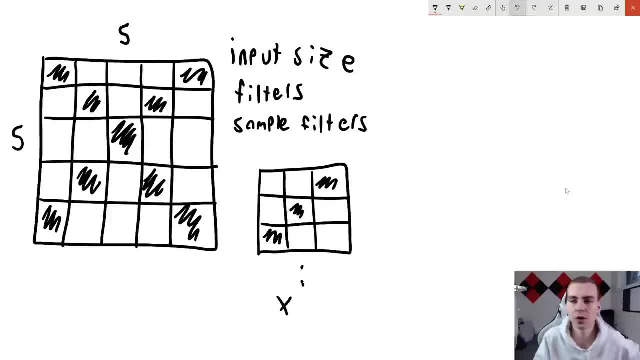 sometimes even 128.. So we can do as many filters as we want, as few filters as we want, But the filters are what is going to be trained. So this filter is actually what is going to be found by the neural network. It's what's going to change. It's you know. this is essentially. 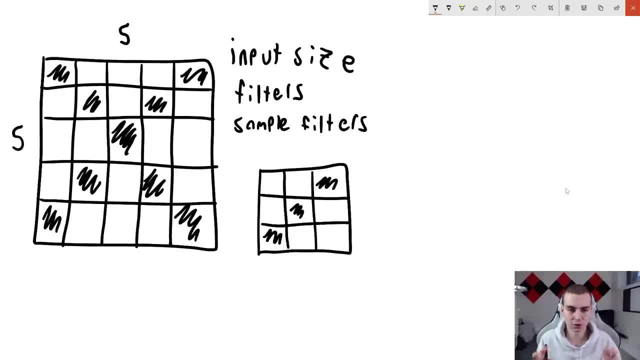 what we're looking for. This is what's created in the program And that's kind of like. the trainable parameter of a convolutional neural network is the filter. So the amount of filters and what they are will change as the program goes on. 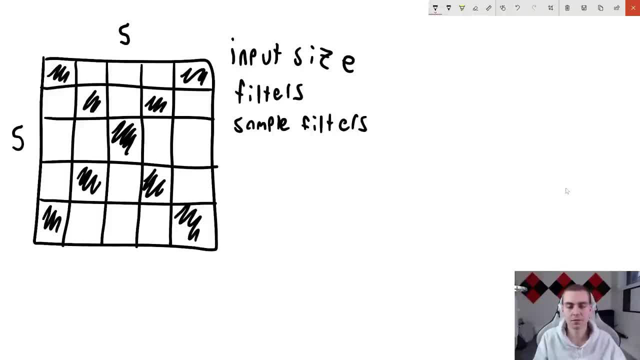 Because we're learning more and figuring out what features that make up, you know, a specific image. So I'm going to get rid of this stuff right now, just so we can draw and do a basic example. But I want to show you how we look for a filter in the image. 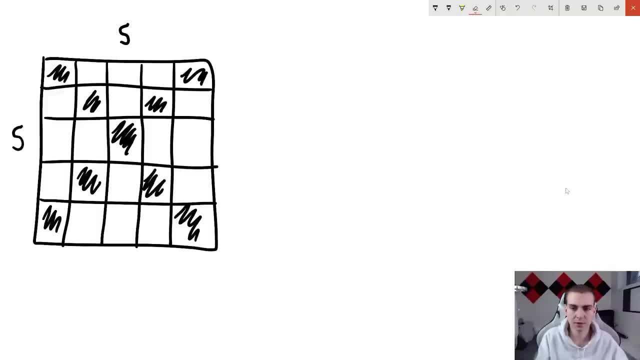 So we have filters, right, they'll come up with them. they're going to start completely random, but they'll change as we go on. So let's say, the filter we're looking for is that one I drew before. I'm just going to redraw it at the top here, a little bit smaller. 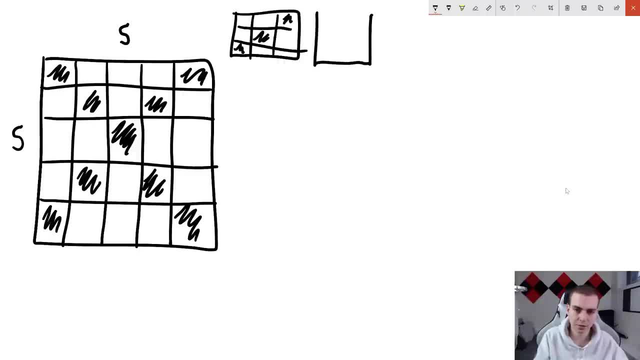 And we'll just say it's a diagonal line, right. But another filter we could look for might be something like you know, a straight line, Just like that all across we could have a horizontal line And in fact we'll have. 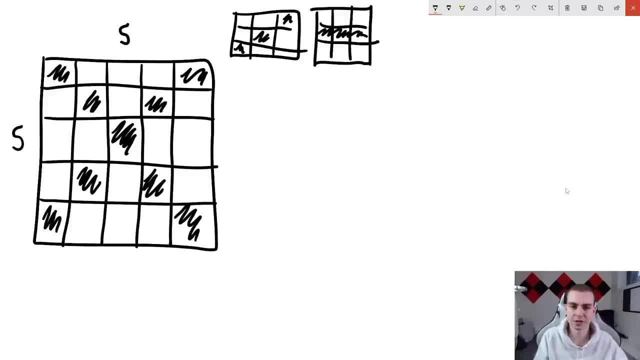 32 of them, And when we're doing just, you know, three by three grids of filters- well, there's not that many. you know combinations. we're going to do at least grayscale wise. So what we'll do is we'll define the sample size, which is how big our filter is going. 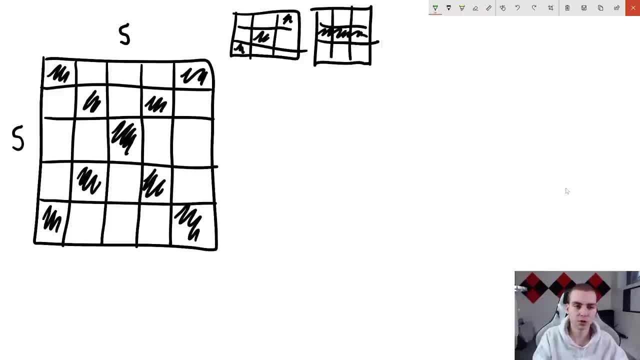 to be three by three, which we know right now, which means that what we're going to do is we're going to look at, three by three, spots in our image and look at the pixels and try to find how closely these filters match. 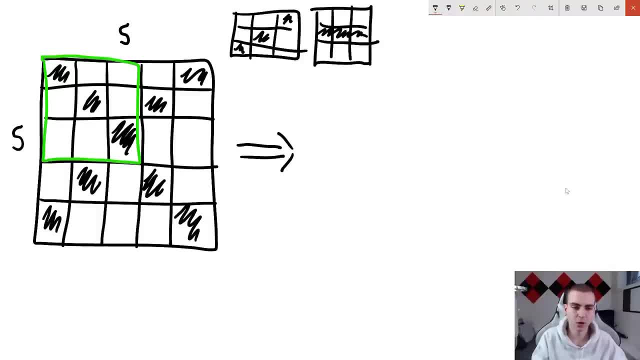 With the pixels we're looking at on each sample. So what this is going to do, this convolutional layer, is going to output to us what we call feature map, which can be a little bit smaller than the original image, and you'll see why in a second, But that tells us about the presence. 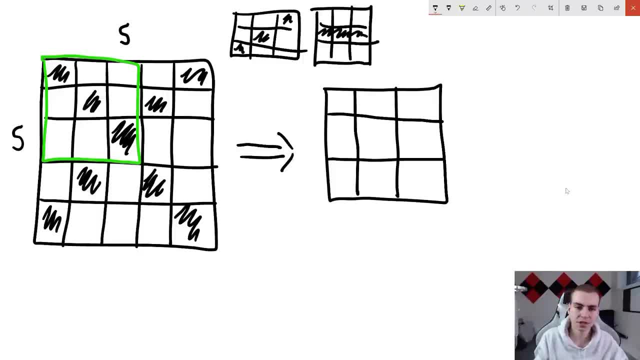 of specific features in areas of the image. So, since we're looking for two filters here, actually we'll do two filters, which means that we're actually going to have a depth to feature map being returned to us, right? Because for two filters, that means we need. 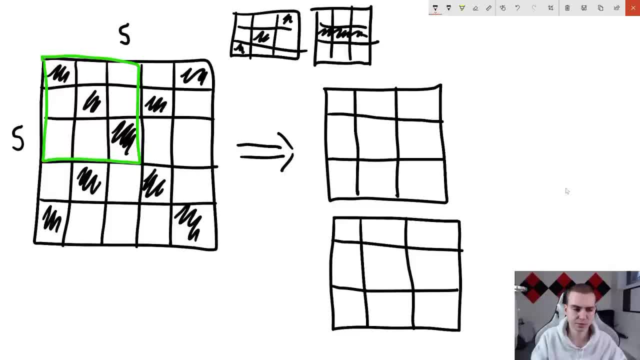 two maps quantifying the presence of both of those filters. So, for this green box that we're looking on the left side here, we'll look for this first filter here, And what do we get? Well, the way we actually do this, the way we look at this filter, is we take the cross product or actually not. 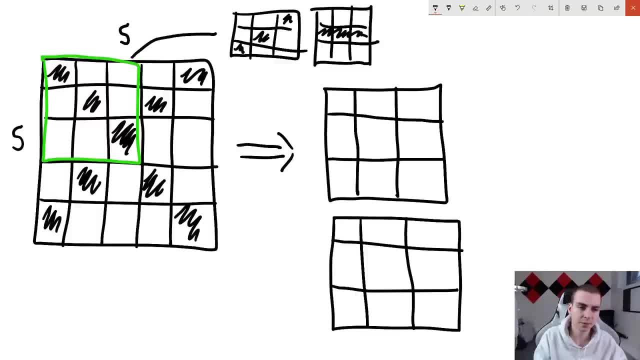 the cross product, the dot product, sorry, between this little green box and this filter. right, because they're both pixels, they're both actually numeric values down at the bottom. So what we do is we take that dot product, which essentially means we're element wise. 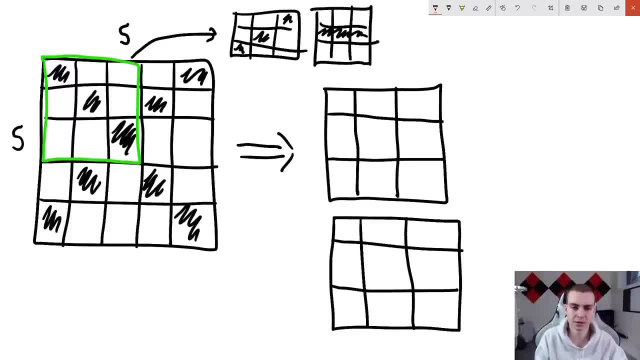 adding or what is it? element wise, multiplying all of these pixels by each other. So if this pixel values is zero, right because it's white, or it could be the other way around. we could say: white is one, black is zero it. 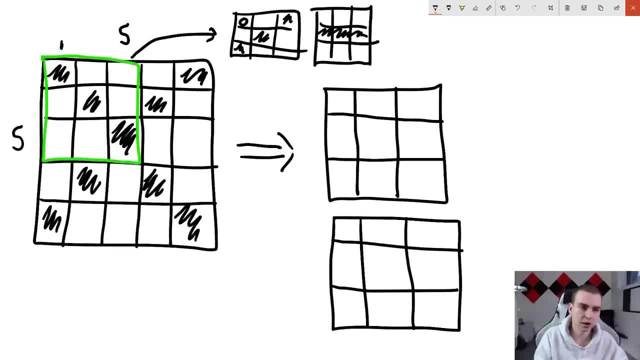 doesn't really matter, right? If this is a zero and this is a one. these are obviously very different, And when we do the dot product of those two, so we multiply them together, then in our output feature we would have a zero, right? That's kind of the way it works. 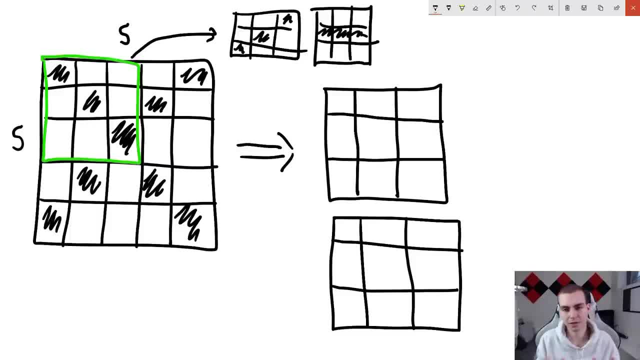 So we do this dot product of this entire thing. If you don't know what the dot product is, I'm not really going to go into that, But we do the dot product And that gives us some value. It's essentially telling us how similar these two blocks are, So how similar this sample. 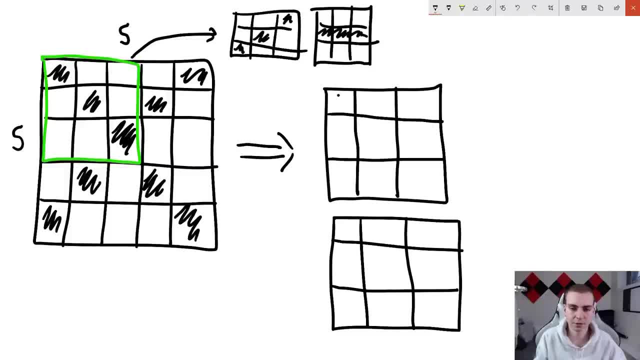 is that we're taking the image and the filter that we're looking for. they're very similar. we're going to likely put a one or something telling us: you know they're very close together, They're not similar at all. we're going to put a zero. So in this case, for our first 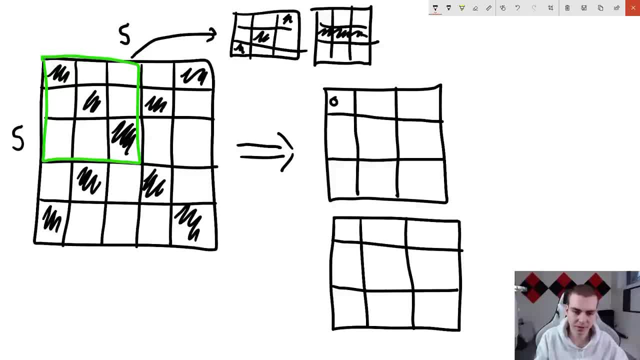 filter. we're probably going to have a value, because this middle pixel is the same as something like 0.1, two, right, but the all the other values are different, So it's not going to be very similar whatsoever. So, then, what we're going to do now is we'll look at the. actually, 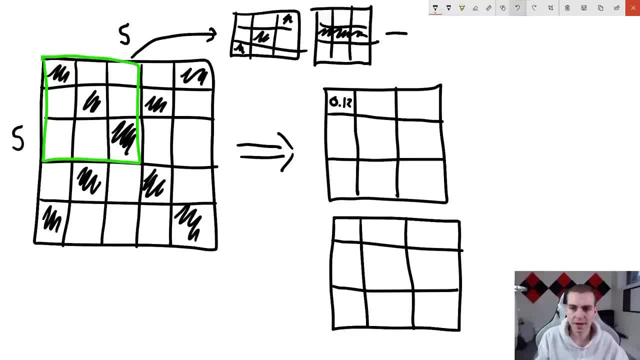 second filter, which is this horizontal line, And in fact we're going to get a very similar output response here, probably something like, you know, 0.1, two, that's going to go in the top left, And again, these are both maps representing each filter, right? So now we'll. 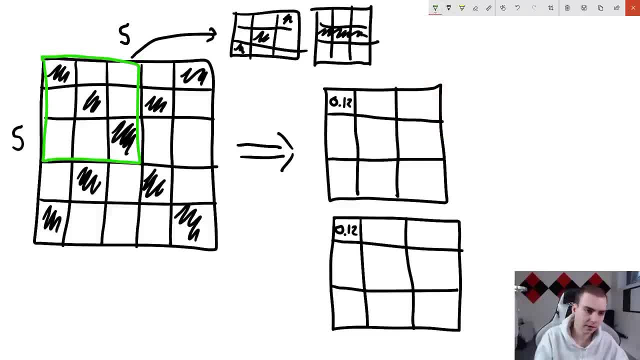 move our green box over one like this. So just shift that over one. And now we'll start looking at the next section, And in fact I'm going to see if I can erase this, just to make it a little bit cleaner here. 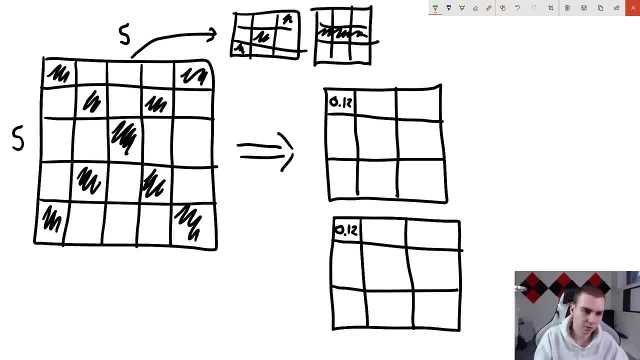 Get rid of the green. Okay, there we go. Okay, so we'll move this box over like this, And now we'll start looking at this one And we'll do the exact same thing we did again before. So we're gonna say, Alright. 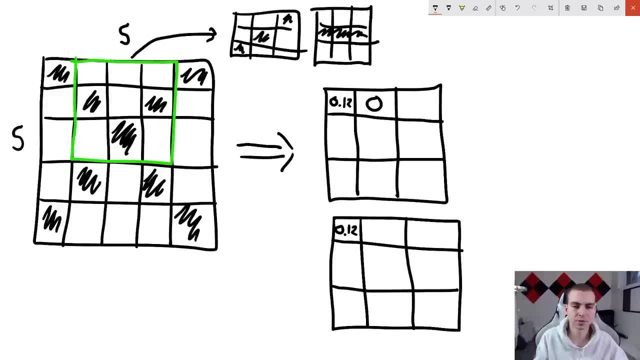 how similar are these? Well, they're not similar at all, So we're gonna get a zero for that first filter. How similar the other ones? Oh, actually, they're like a little bit similar. There's a lot of white that's kind of in the same space, like you know, stuff like that. 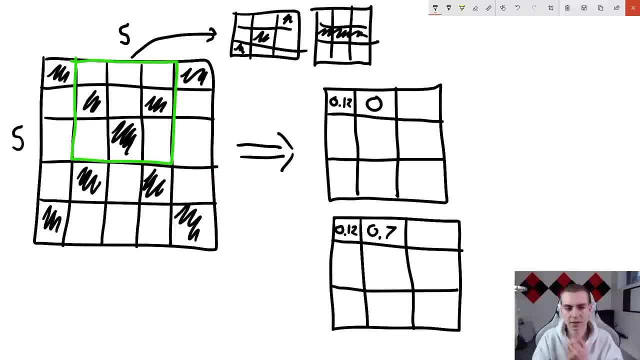 So we'll say maybe this is like 0.7.. Right, I'm just randomly picking these numbers. they are going to be much different than what I'm putting in here, But I'm just trying to get you to understand what's kind of happening, right, And this is completely random the way I'm making the. 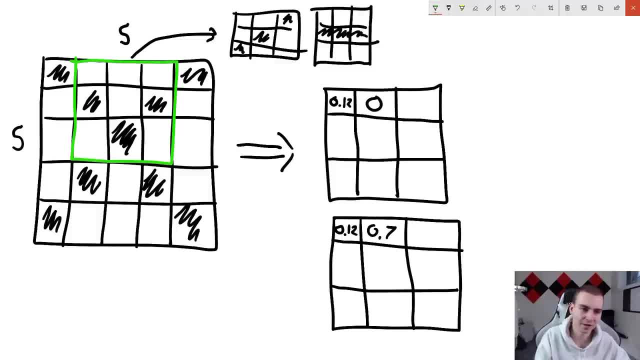 numbers to just make sure you understand that, because this is not exactly what it would look like. Okay, so then we're gonna move the box over one more time. let's just erase this to keep this clean. this will be the last time we do this for the purpose of this. 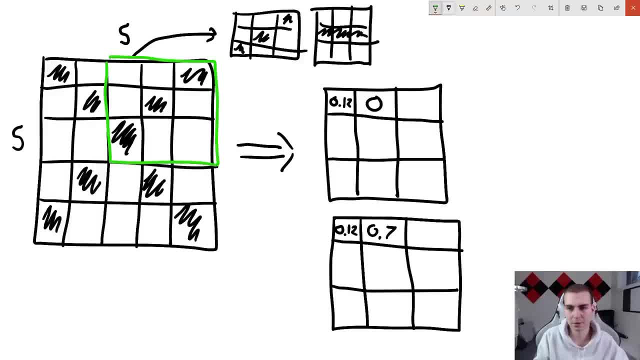 example. And now what we're gonna have is: wow, we have a perfect match for the first filter, So we put one. the other ones, like ads, kind of similar as a few things that are different, So maybe this gets like a 0.4 or something right. Whatever they are, we end. 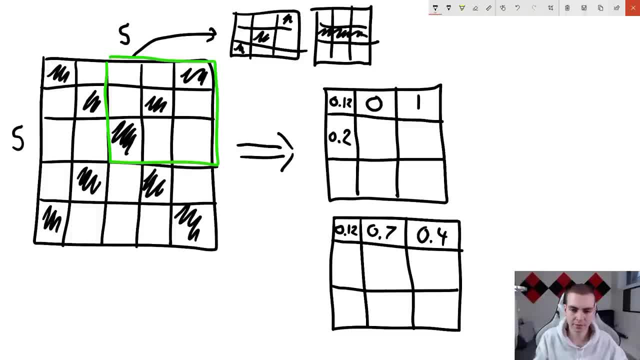 up getting some value, So we'll fill in all these values. let's just put some arbitrary values here for now, just so we can do something with the example: 0.70, 0.12, 0.42, 0.30, 0.9, 2.1.. Again, completely random, 0.40.. Point six: Alright. 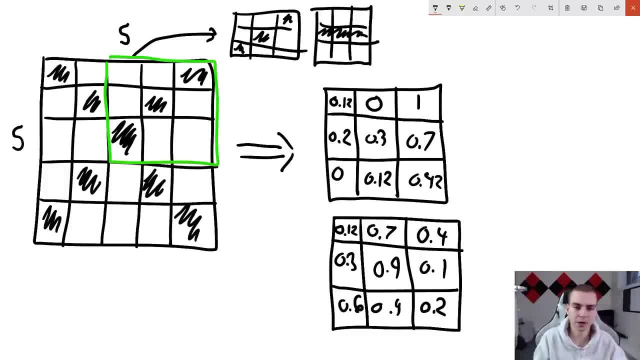 so this is now what we've gotten our response map from: looking at two filters on our original image of five by five. Now notice that the size of these is three by three, And obviously the reason for that is because in a five by five image, when we're taking three by three, 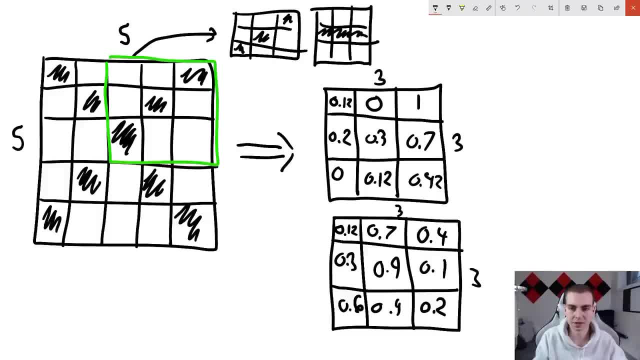 samples. well, we can only take nine three by three samples, because when we go down a row, right, we're going to move down one and we're going to do the same thing we did before. of this, these three by three samples, And if we add the amount of times we can do, 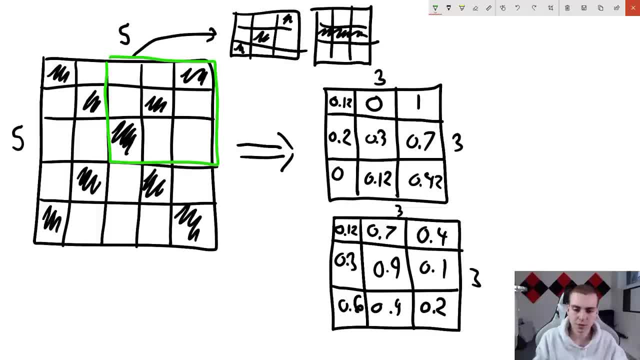 that, well, we just get three by three, which is not So. this, now, is kind of telling us of the presence of features in this original image map. Now, the thing is, though, we're going to do this 64 times right, For 64 filters, or 32 filters are the amount of filters that. 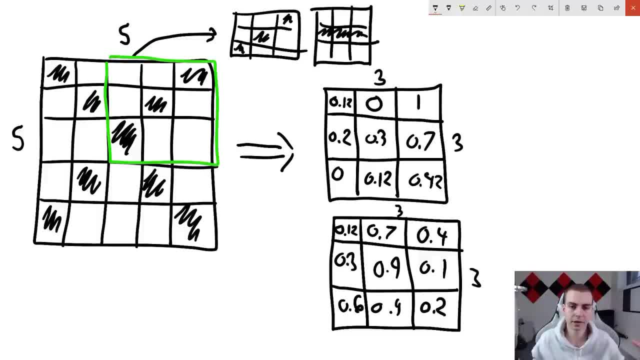 we have. So we're going to have a lot of layers, like a ton of different layers, and we're going to have a lot of layers, which means that we're going to be constantly expanding, as we go through the convolutional layers, the depth of this, this kind of output feature. 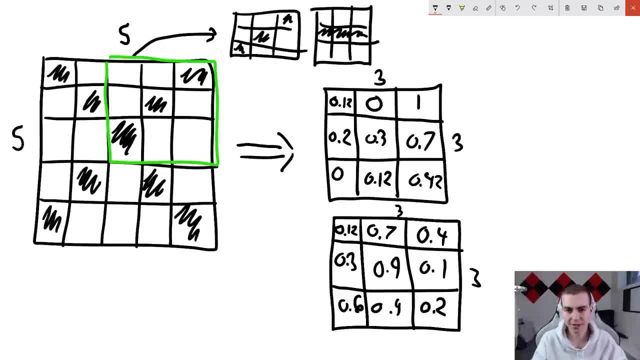 map, And that means that there's a lot of computations that need to be done And essentially that means that this can be very slow. So now we need to talk about an operation called pooling. So I'll backtrack a little bit, but we will talk about pooling in a second. what's? 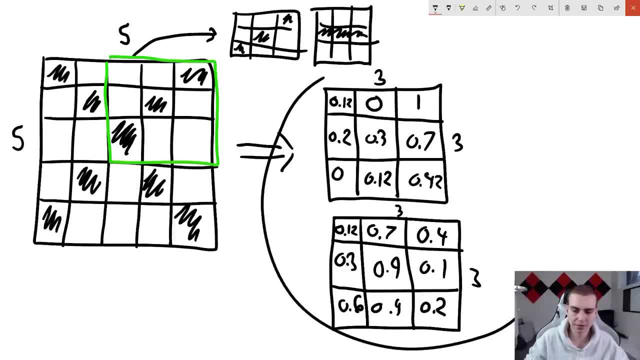 going to happen right is when we have all these layers that are generated. So this is called the output feature map, right From this original image. what we're going to do is the next convolutional layer in the network is now going to do the process we just talked. 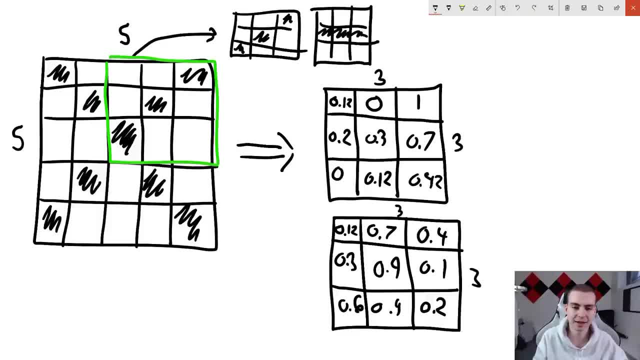 about, except on this output feature map, which means that, since this one was picking up things like lines and edges- right, the next convolutional layer- we'll pick up combinations of lines and edges and maybe find what a curve is right. we'll slowly work our way up from very 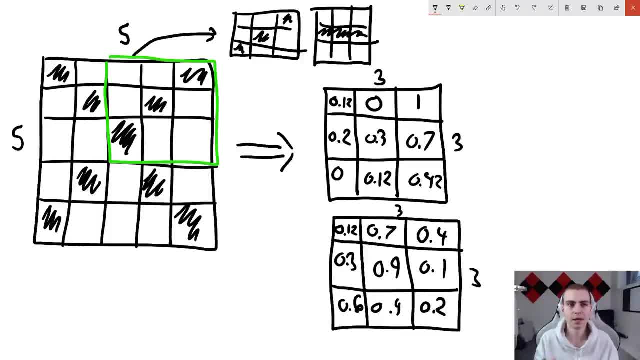 very small amount of pixels, defining more and more- almost- I want to say- abstract- different features that exist in the image. This is what really allows us to do some amazing things with a convolutional neural network. when we have a ton of different layers stacking up on each other, we can pick out all the 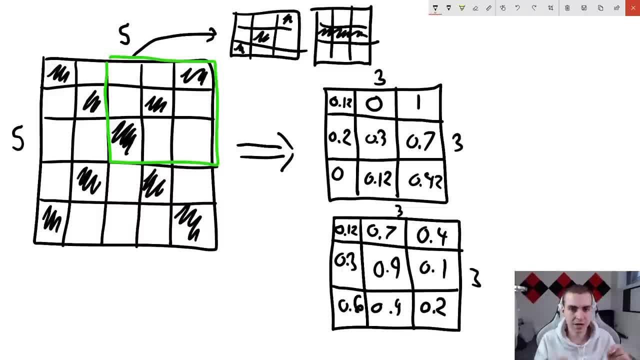 small little edges, which are pretty easy to find, And with all these combinations of layers working together, we can even find things like, say, eyes right or feet or heads or face right. We can find very complicated structures because we slowly work our way. 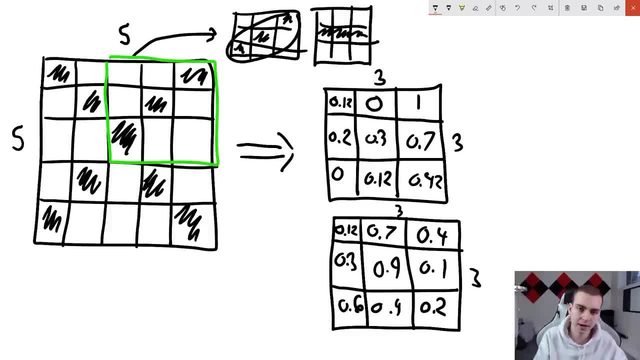 up, starting by solving very easy problem, which are like finding lines and then finding combinations of lines, combination of edges, shapes and like very abstract things. That's how this convolutional network works. So we've done that. now. it's now time to talk about 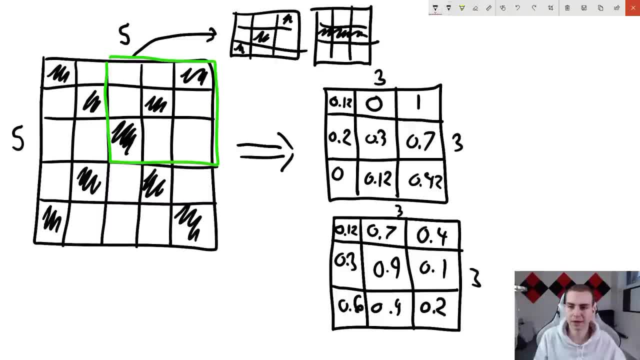 pooling And I will also talk about Pat. actually we'll go padding first before we go pooling. I just it doesn't really matter what order we talk about this in, But I just think padding makes sense based on the way we're going right now. So sometimes we want to make sure that. 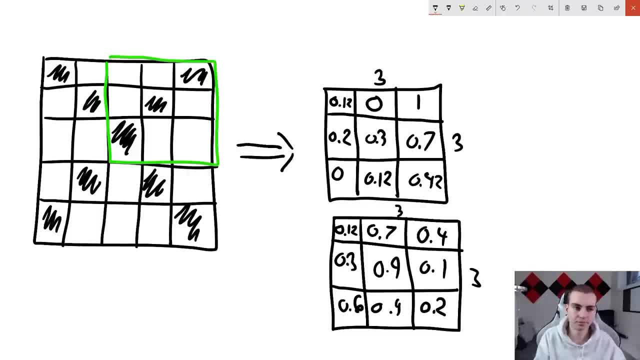 the output feature map from our original image here is the same dimensions or same size as this right. So this is five by five, obviously, And this is three by three. So if we want this to be five by five as an output, what we need to do is add something called padding. 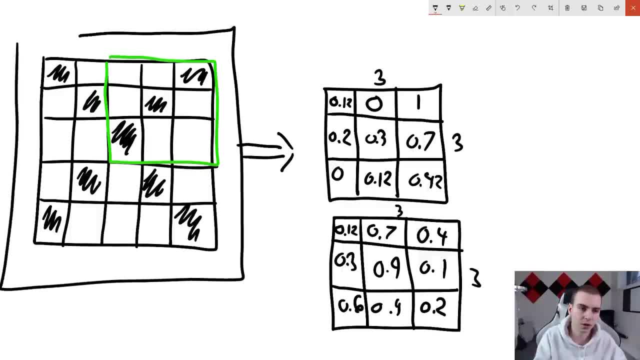 to our original image. So padding is essentially just adding an extra row and column on each side of our image here so that when we and we just fill in all these pixels in like kind of the padded pixels here, I just blank random pixels. they don't mean anything Essentially. 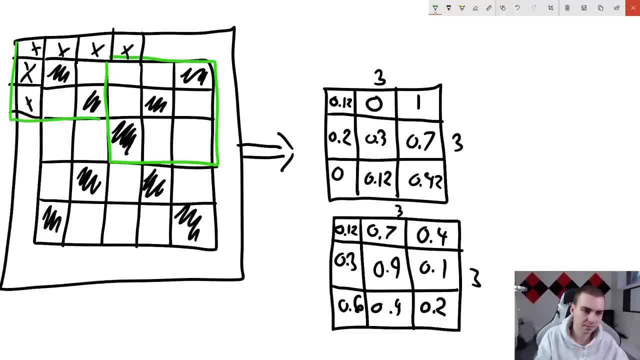 why we do that is so that when we do our three by three sample size here like this, we can take a three by three sample where every single pixel is in the center of that sample, Because right now this pixels not in the center. this pixel can never be in the center. 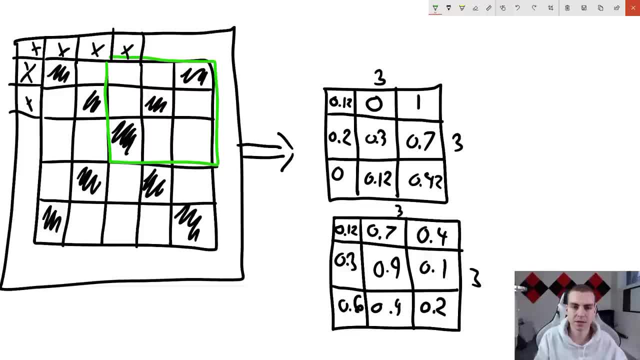 this pixel can never be in the center. only, you know, a few pixels get to be in the center, And what this allows us to do is generate an output map that is the same size as our original input and allows us to look at features that are maybe right on the edges of images. 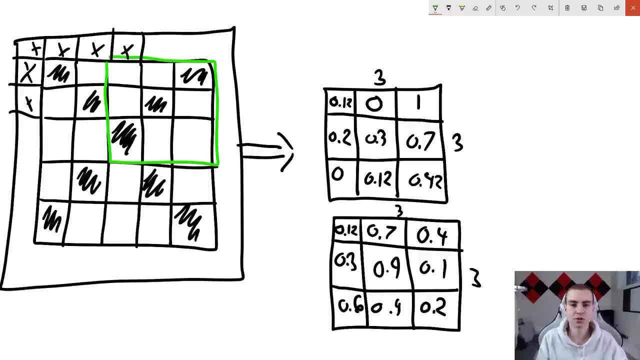 that we might not have been able to see, but see before. Now this isn't super important when you go to like very large images, But it just something to consider. you can add padding. we may do this as we get through our examples, And there's also something called stride which I want to talk about as well. 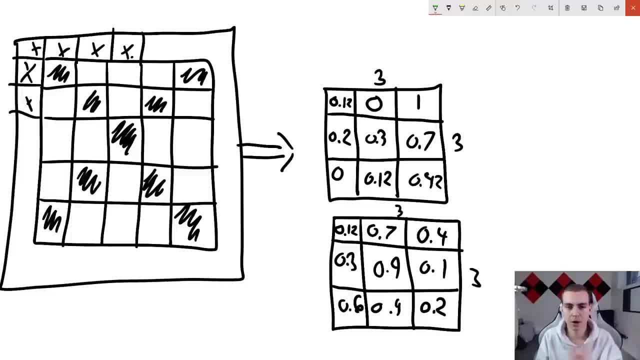 So what a stride is is essentially how much we move this sample box every time that we're about to move it right. So before, like so let's say we're doing example with padding here, right, we are first sample we would take here And again, these pixels are just 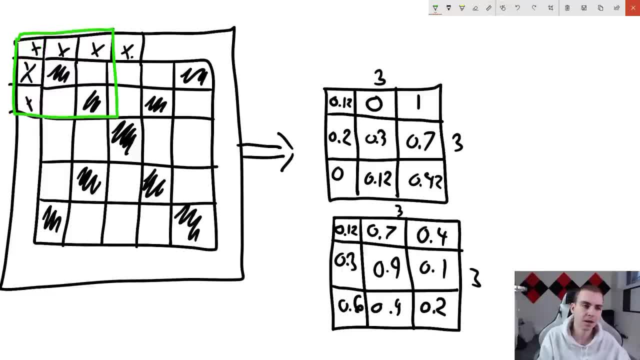 added. we added them in to make this work better for us. you would assume that the next time we move the box, we're going to move that one pixel over. that's called a stride of one. we can do that, But we also can employ a stride of two, which means we'll move over. 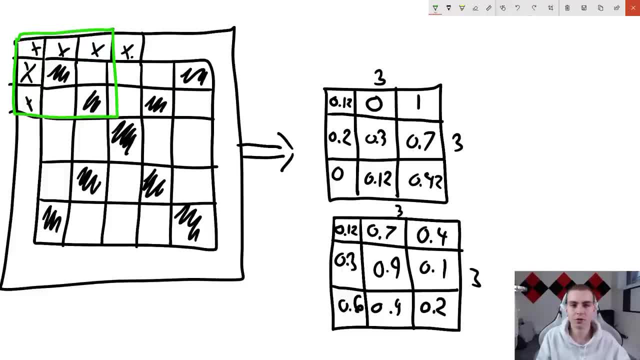 by two. obviously, the larger your stride, the smaller your output feature map is going to be. So you might want to add more padding. well, you don't want to add too much padding, but it's just something to consider, And we will use a stride in different instances. 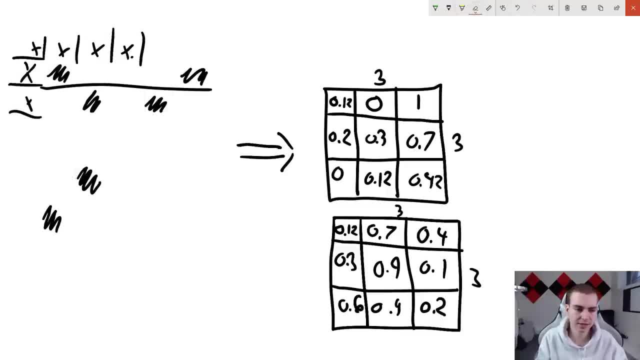 Okay, so that's great. That hopefully makes sense. Let's erase this Now. We don't need this anymore. We talked about padding, we talked about the stride, And now we're gonna talk about a pooling operation, which is very important. So kind of the idea is that we 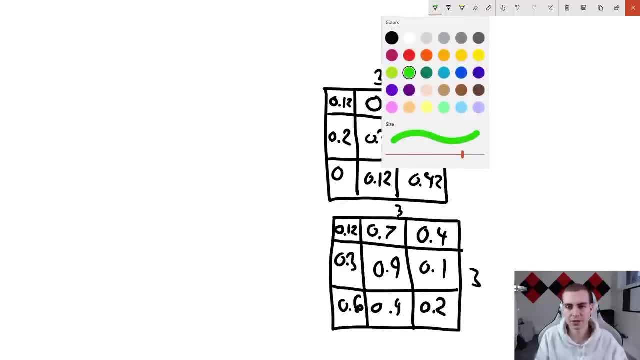 're going to have a ton of layers right for all these filters, And we're just gonna have a lot of numbers, a lot of computations, And there must be some way to make these a little bit simpler, a little bit easier to use. Well, yes, that's true, And there is. 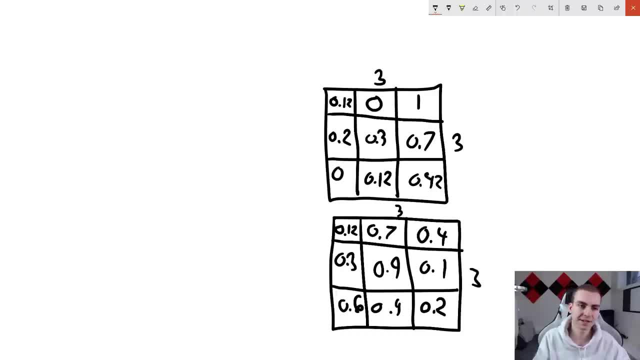 a way to do that And that's called pooling. So there's three different types of pooling. Well, it is more, but the basic ones are min, max and average. And essentially a pooling operation is just taking specific values from a sample of the output feature map. So once 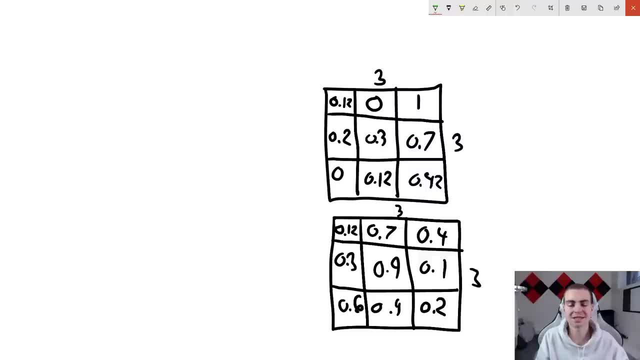 we generate this output feature map. what we do to reduce its dimensionality and just make it a little bit easier to work with is what we sample, typically two by two, areas of this output feature map and just take either the min, max or average value of all the values inside of here and 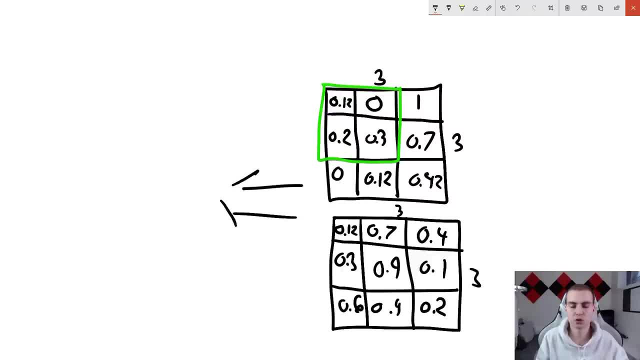 map, these. we're going to go back this way to a new feature map that's twice, like one times, the size, essentially, or not, what am I saying? two times smaller than this original map And it's kind of hard with three, like three by three, to really show you this. But 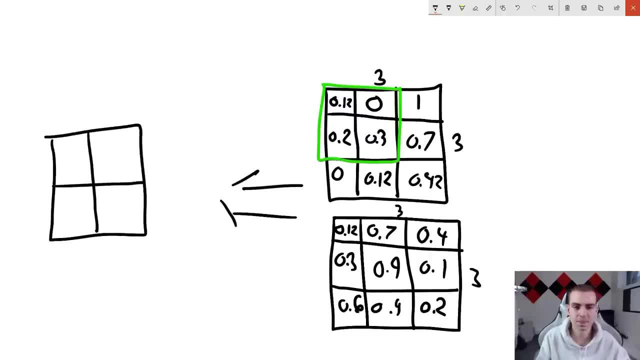 essentially, what's going to end up happening is going to have something like this. So we're going to take the sample here. we're going to say, Okay, what are we doing? min, max or average pooling? for doing min pooling, we're gonna take the smallest value, which means we'll take zero. for doing max, 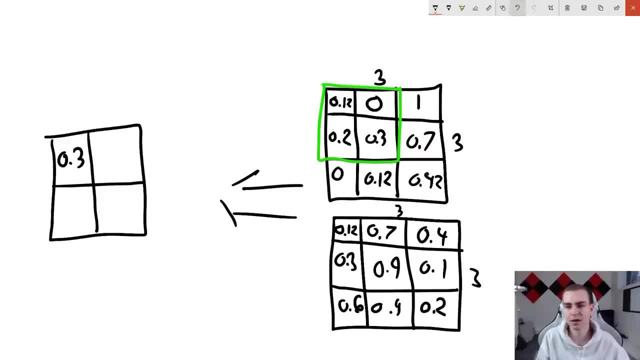 pooling, we'll take the maximum value, which means we'll take 0.3.. If we're doing average, we're probably gonna get an average value of close to what, 0.2, maybe. So let's say 0.2, we'll go there. That's how we do that with pooling. again, just to make this feature, 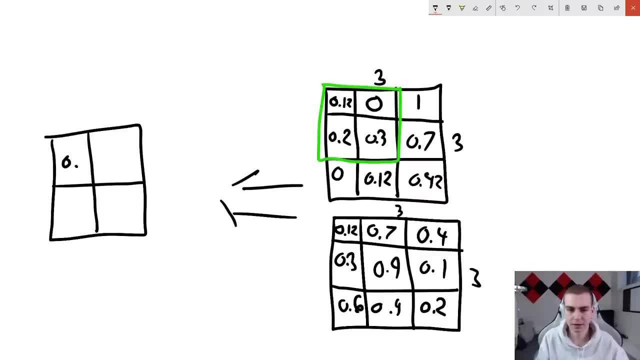 map smaller. So we'll do that for both of the filters. But let's just say this is 0.2.. Let's say this here that I'm blocking off is I don't know what. is this going to be 0.6.. It's hard to do this average with four numbers. let's say this one down here is going. 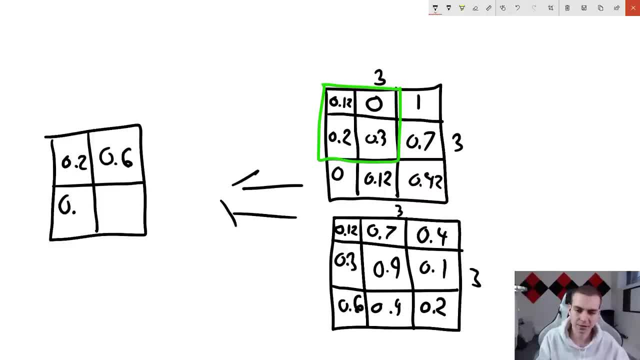 to be zero point. I don't know. let's just do two, one or something. And then this last one. here we Okay, we got some bigger values. maybe this will be like 0.4.. Okay, so that's one. the one down here we'll have some values of its own. we'll just do squiggles to represent. 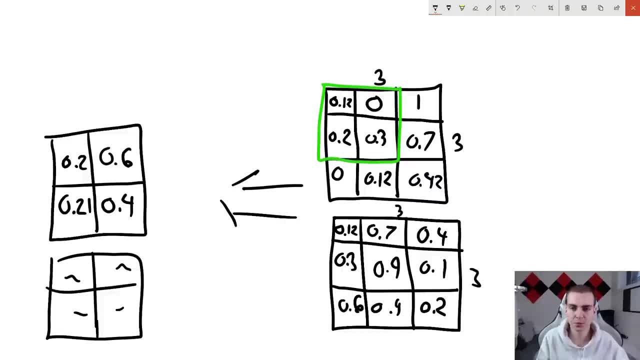 that it has something, And we've effectively done a max pooling operation on this. we've reduced the size of it by about half, And that is kind of how that works. Now, typically, what we do is we use a two by two pooling or like sample size, like that with the stride of two, which actually means 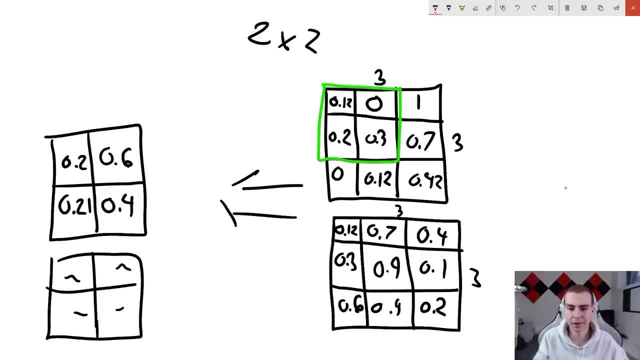 that we would draw it like this, But since we're not going to do padding on this layer right now, we'll just do a stride of one, And this is how we pull it. Now. the different kinds of pooling are used for different kinds of things. The reason we would use a max pooling: 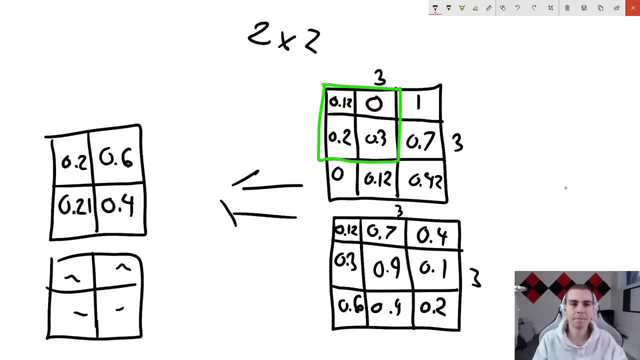 operation is to pretty much tell us about the maximum presence of a feature in that kind of local area. we really only care if the feature exists where. if it doesn't exist, an average pooling is not very often used, Although in this case we did use an average pooling, But you know. 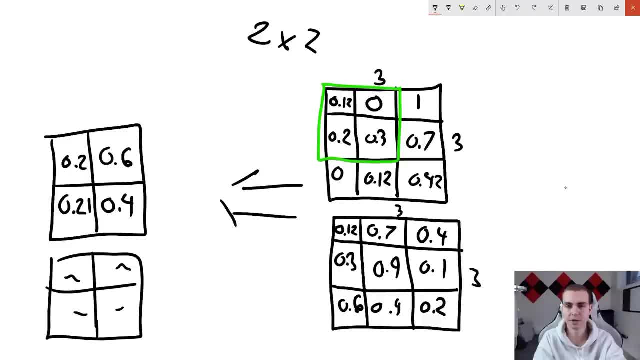 it's just different kinds of pooling: And average tells you about the average presence of the feature in that area, Max tells you about is that feature present in that area at all, And min tells you does it not exist. If it doesn't exist, right, we're just gonna. 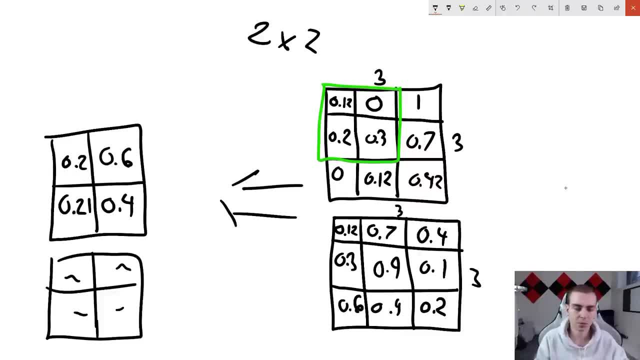 have a zero In that area. So that's the point of pooling, That's the point of convolutional layers. I think I'm done with the whiteboarding For now. we're actually going to start getting into a little bit of code and talking about creating our own convolutional networks, which 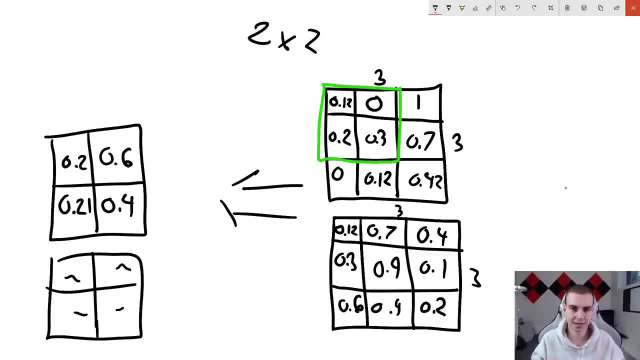 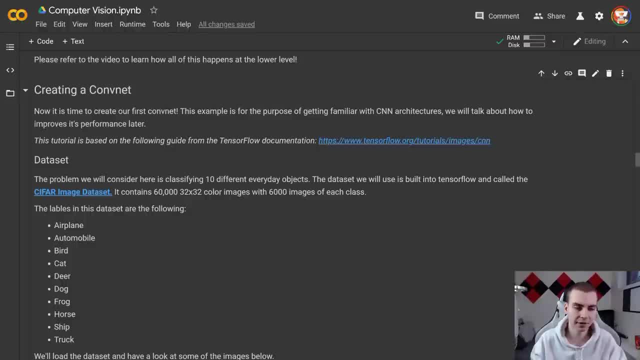 hopefully will make this a lot more clear. So let's go ahead and get into that. Alright, so now it is time to create our first convolutional neural network. Now we're gonna be using Kara's to do this, And we're also going to be using the CIF AR image data set that contains 60,000. 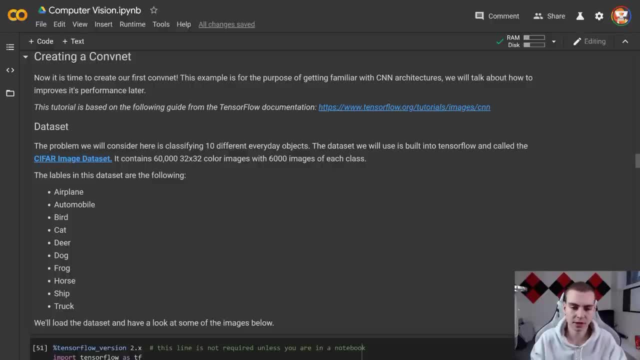 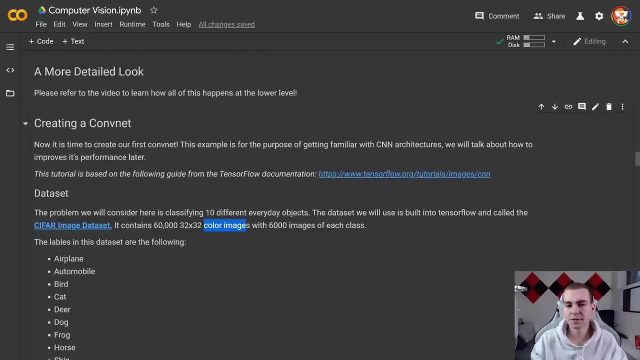 images of 10 different classes of everyday objects. Now, these images are 32 by 32.. And it's actually 32 by 32, which essentially means they are blurs And they are colorful. Now I just want to emphasize, as we get into this, that the reason I'm not typing all of 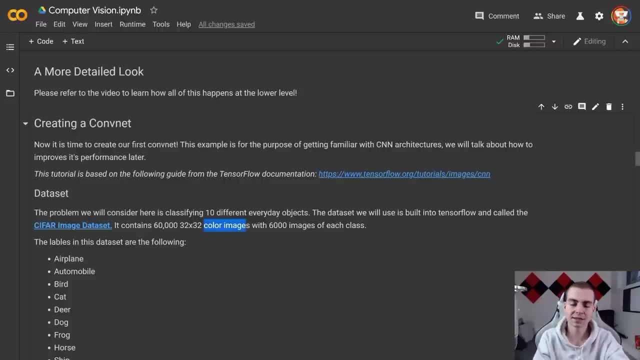 these lines out- and I just have them in here already- is because this is likely what you guys will be using or doing when you actually make your own models. chances are that you are not going to sit, unless you're a pro at TensorFlow- And I am not even there yet either. 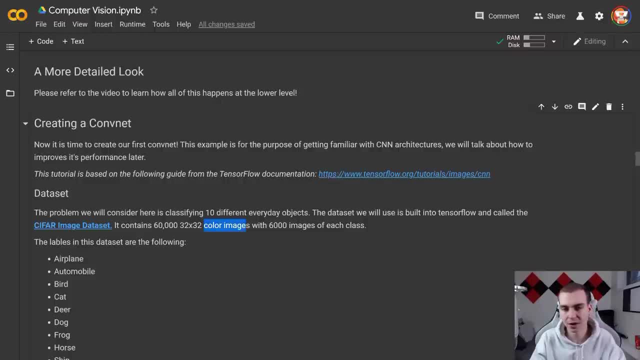 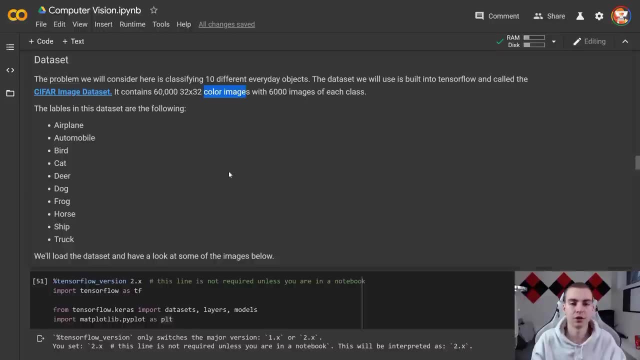 with my knowledge of it and have all of the lines memorized and not have to go reference the syntax. So the point is here. so long as you can understand why this works and what these lines are doing, you're gonna be fine. you don't need to memorize them And 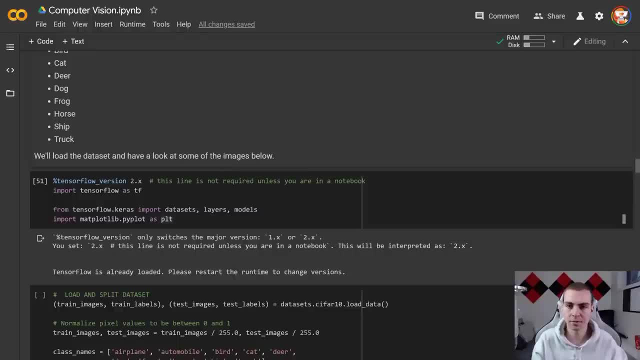 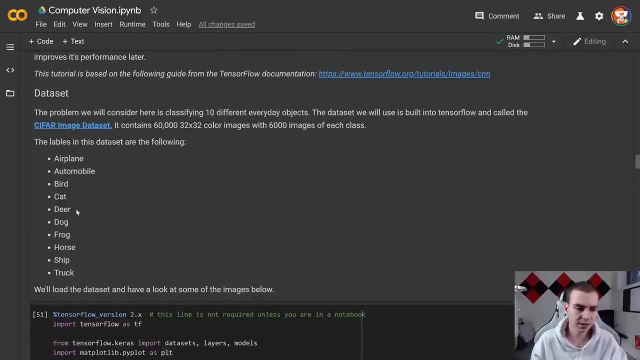 I have not memorized them, And I don't. I look up the documentation, I copy and paste what I need. I alter them, I write a little bit of my own code, But that's kind of what you're going to end up doing, So that's what I'm doing here. So this is the image data set. 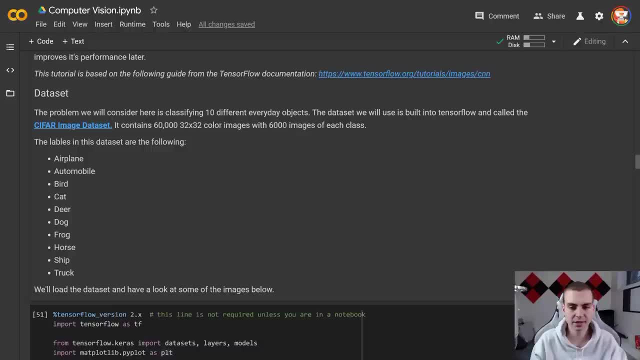 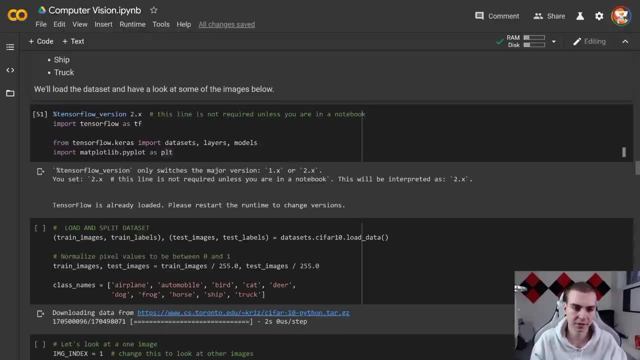 We have truck, horse, ship, airplane, you know just some everyday, regular objects. there is 60,000 images, as we said, and 6000 images of each class, So we don't have too many images of just one specific class. So we'll start by importing our modules, So TensorFlow. 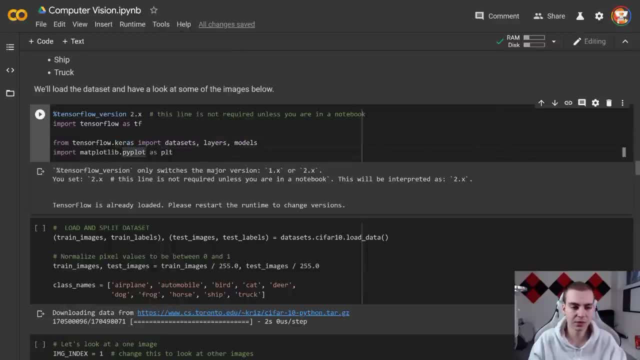 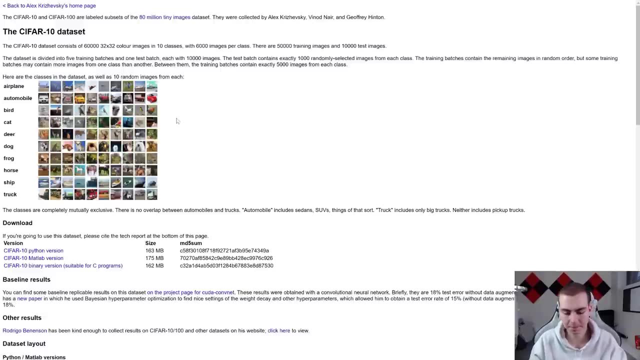 we're going to import TensorFlow dot Keras. we're going to use the data set built into Keras for this. So that's the ci fa r image data set, which you can actually look at just by clicking at this. it'll bring you and give the information about the data set. Although, 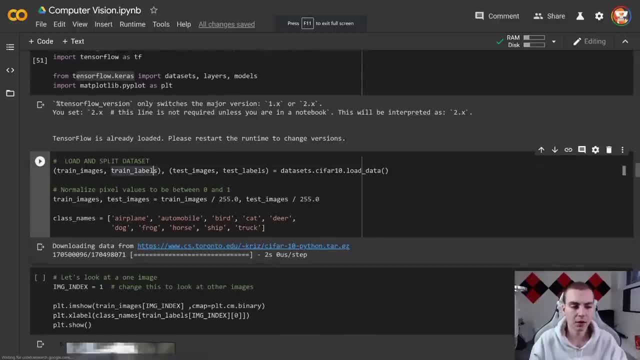 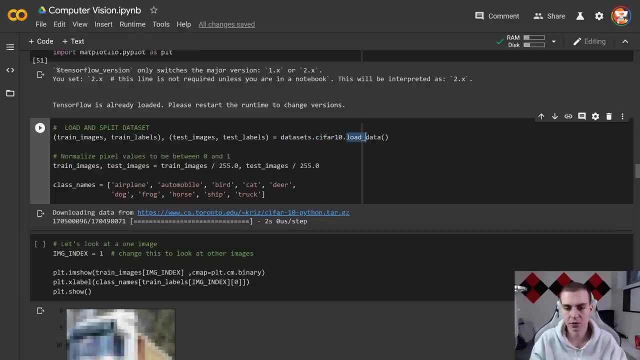 we don't need that right now, because I already know the information about it And now we're just going to load our images in. So again, this stuff, the way this works is you're gonna say data sets: dot, ci, fa, r, 10, dot. load data. 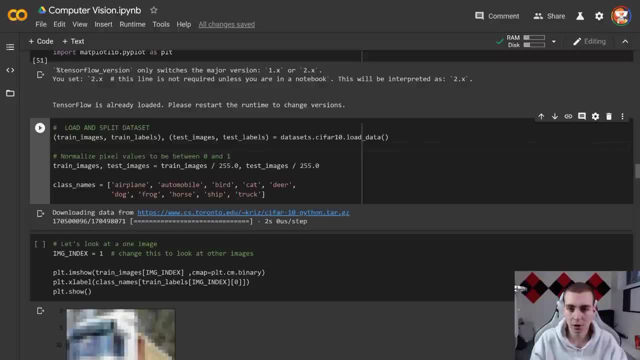 Now this loads it in as like a very strange TensorFlow object, that's like a data set object. So this is different from what we've used before, where some of our objects have actually been like in NumPy arrays where we can look at them better. this is not going. 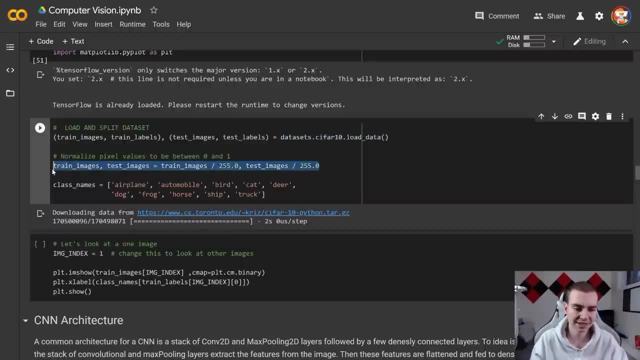 to be in that. So just something to keep in mind here. And we're going to normalize this data into train images and test images by just dividing both of them by 255.. Now again, we're doing that because we want to make sure that our values are between zero and one. 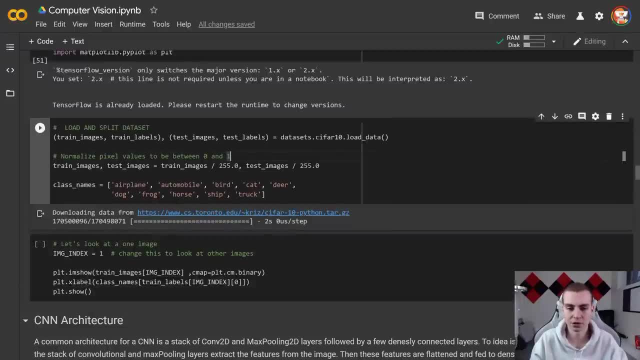 because that's just a lot better to work with in our neural networks rather than large integer values just causes, you know, some things to mess up sometimes. Now, class names: we're just going to define a list here So we have all the class names, so that zero represents. 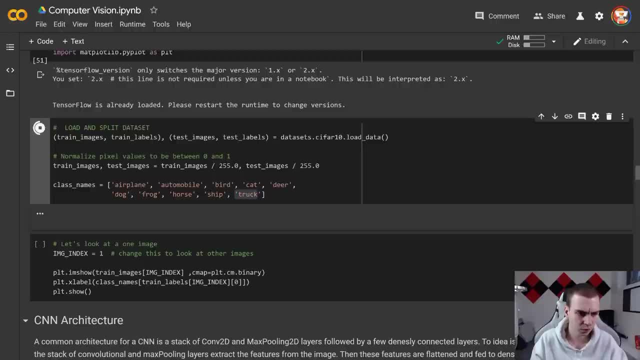 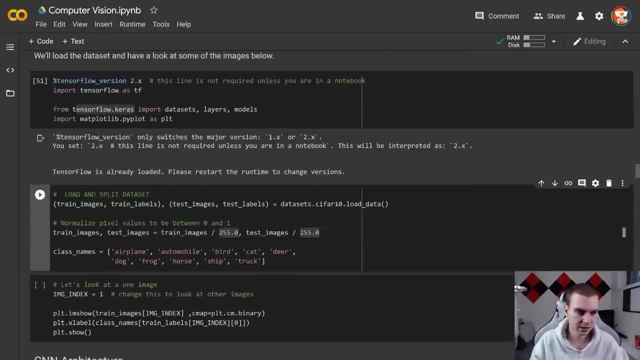 airplane: one auto avail so far until truck run that block of code here. we'll download this data set, although I don't think it takes that long to do that. So Okay, so wait, I guess, Yeah, I guess that's good. I think we're okay there, And now let's just have a look. 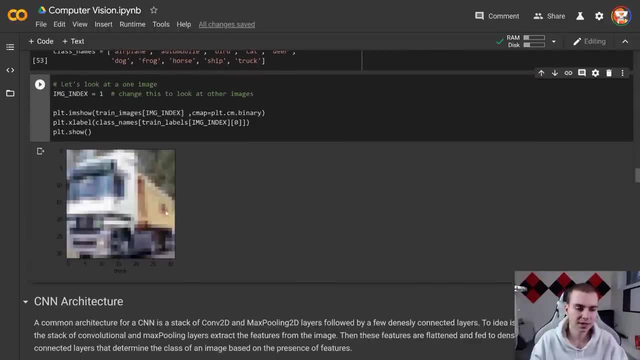 at actually some of the images here. by running this script- So we can see this is a truck- can change the image index to be two. we can see this is another truck. let's go to say six, we get a bird And you can see these are really blurry. 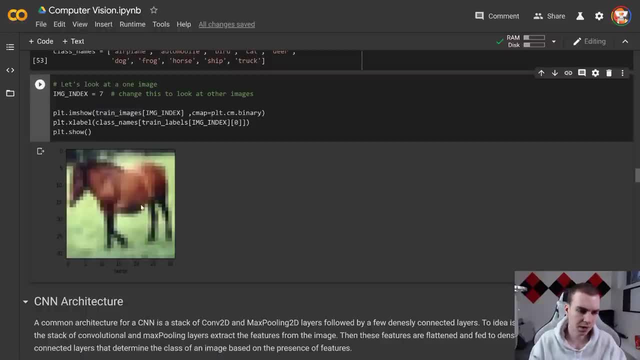 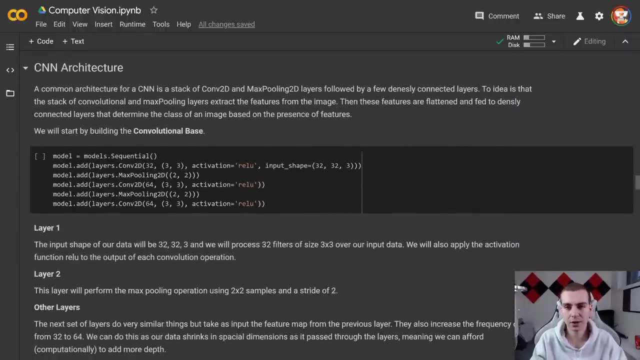 But that's fine For this example. we're just trying to get something that works All right. Okay, so that's a horse, you know, you get the point Alright. so now CNN architecture. So essentially we've already talked about how a convolutional neural network works. 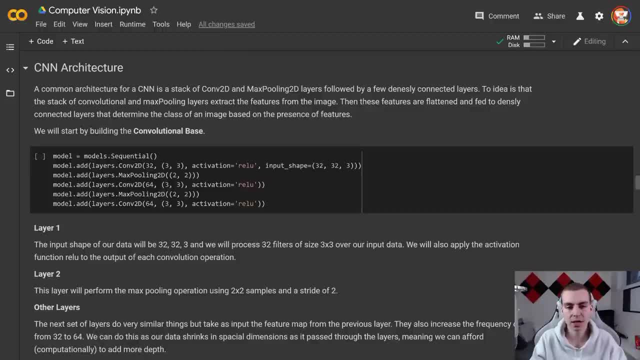 we haven't talked about the architecture and how we actually make one. Essentially, what we do is we stack a bunch of convolutional layers and max pooling, min, pooling our average pooling layers together in something like this right, So after each convolutional layer we have a max pooling layer, some kind of pooling. 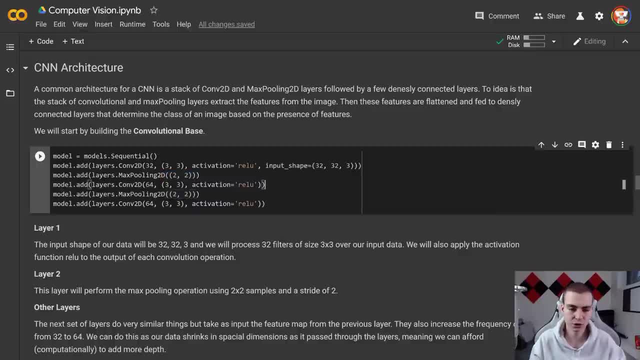 layer, typically to reduce the dimensionality. although you don't need that, you could just go straight into three convolutional layers And on our first layer, what we do is we define the amount of filters, just like here we define the sample size. So how big are those filters? 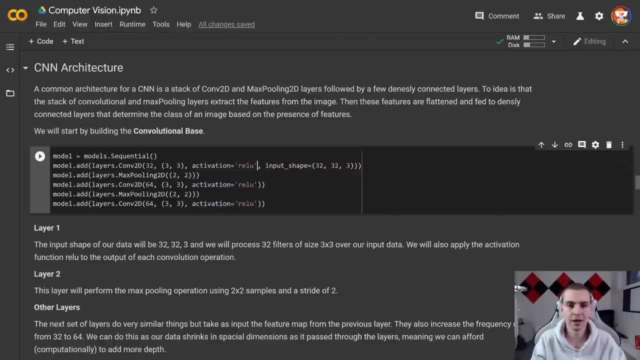 an activation function, which essentially means, after we apply that, what is it that cross, not crossbar dot product operation that we talked about? we'll apply rectifier linear unit to that and then put that in the output feature map. Again, we've talked about activations. 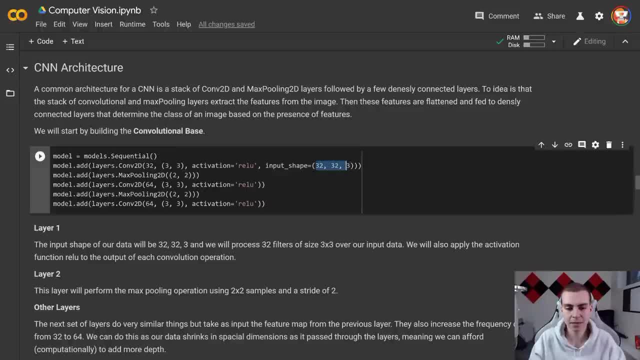 functions before, so I won't go too far into depth with them. And then we define the input shape, which essentially means: what can we expect in this first layer? Well, 32 by 32, by three, these ones. we don't need to do that, because they're going to figure out. 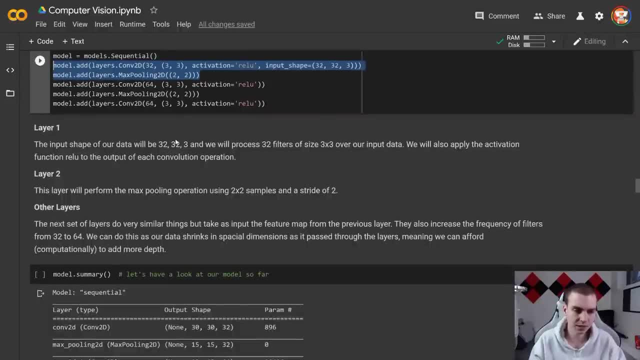 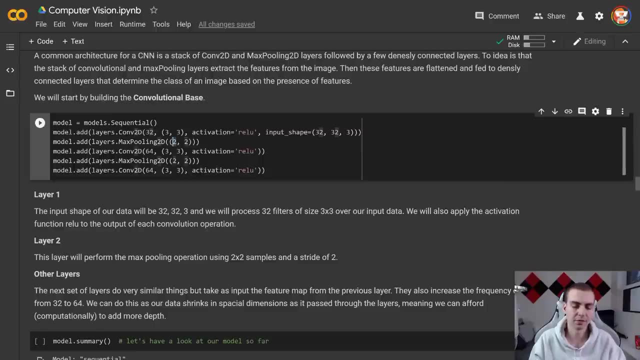 what that is based on the input from the previous layer. Alright, so these are just a breakdown of the layers, the convolution or the max pooling layers here. two by two essentially means that what we're going to do is we're going to have a two by two sample size with 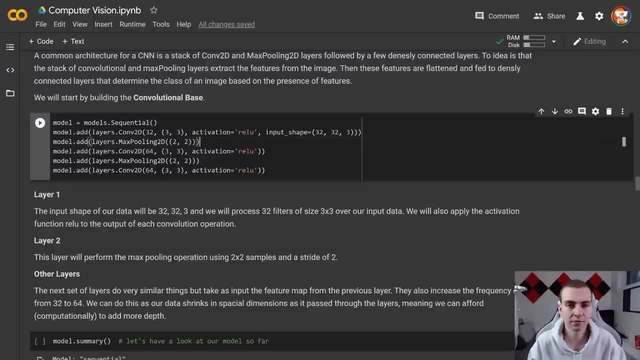 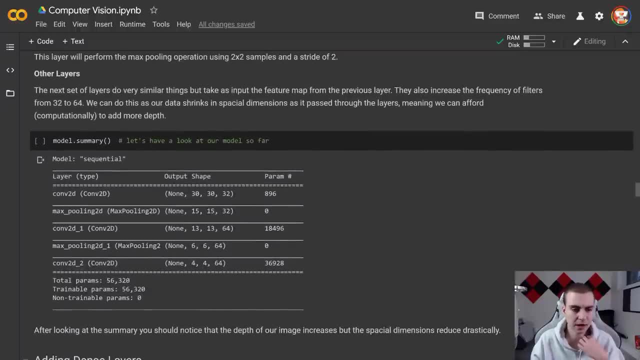 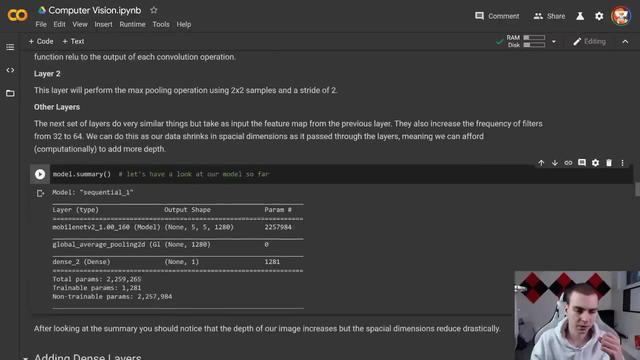 actually a stride of two To actually divide, or, you know, shrink it by a factor of two- how large each of these layers are. Alright, so now let's have a summary. it's already printed out here. we can see that we have- oh wait, is this correct? Mobile net v two. I don't think that's correct. That's. 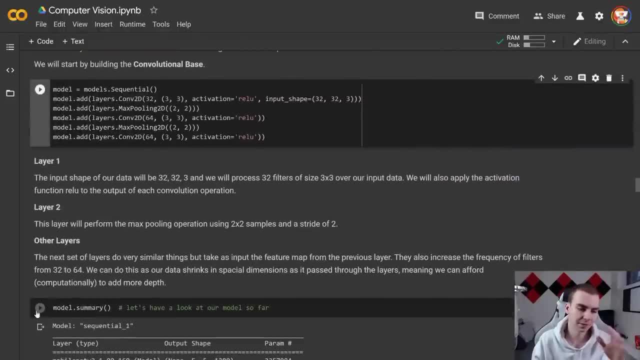 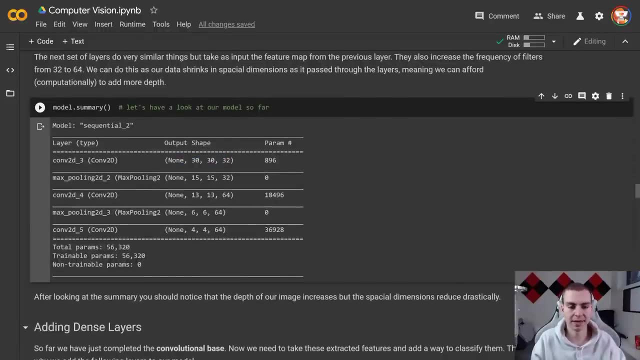 because I haven't run this one. My apologies on that, guys. this is from something later in the tutorial. we can see that we have calm. 2d is our first layer. this is the output shape of that layer. notice that it is not 32 by 32 by 32.. 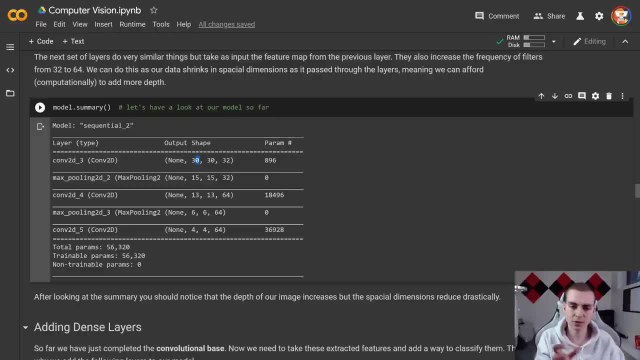 It is 30 by 30 by 32.. Because when we do that sampling without padding, right, that's what we're going to get. we're going to get two pixels less, because the amount of samples we can take, Alright. next we have the max pooling 2d layer. So this now says the output. 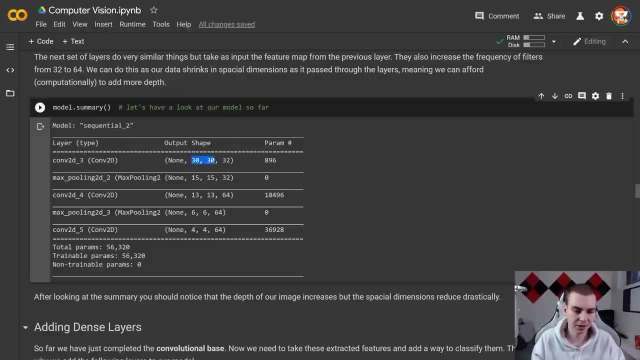 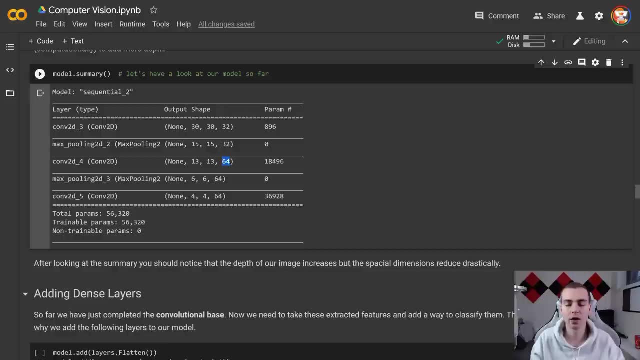 shape is 15 by 15 by 32,, which means we've shrunk this shape by a factor of two. we do a convolution on this, which means that now we get 1313.. And we're doing 64, because we're. 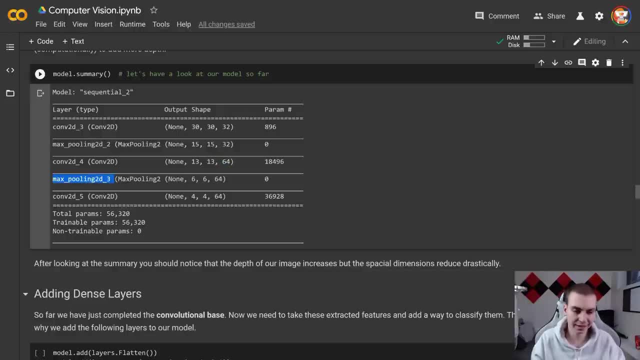 going to take 64 filters this time And then max pooling again. we go six by six by 64. Because we're going to divide this again by a factor of two- notice that it just rounded right- and then calm 2d, So another layer. 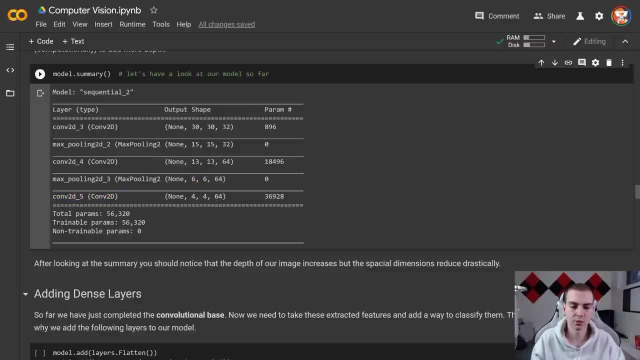 here we get four by four by 64.. Again, because of the way we take those values. So this is what we've defined so far, But this is not the end of our convolutional neural network. In fact, this doesn't really mean much to us, right? This just tells us about the presence. 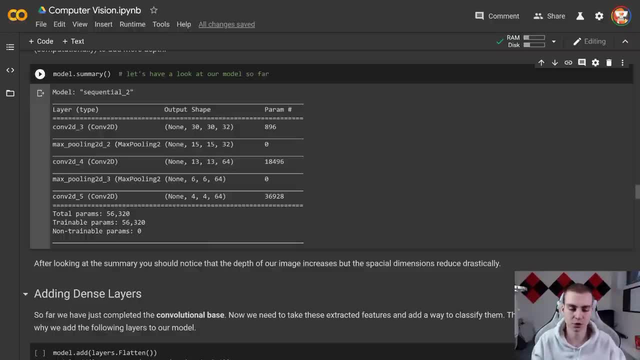 of specific features, as we've gone through this convolution base, which is what this is called, the stack of convolution and max pooling layers. So what we actually need to do is now pass this information into some kind of dense layer classifier, which is actually going to take. 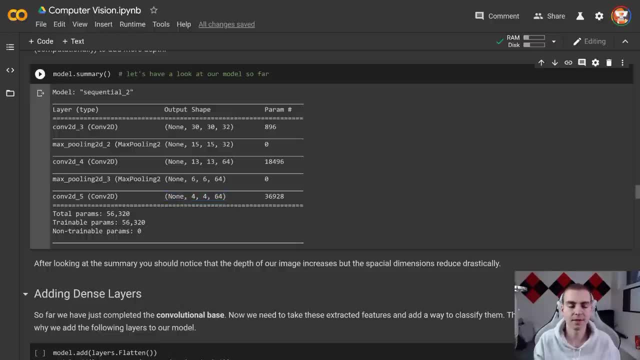 this pixel data that we've kind of calculated and found, So the almost extraction of features that exist in the image and tell us which combination of these features map to either you know what one of these 10 classes are. So that's kind of the point. you do this convolution. 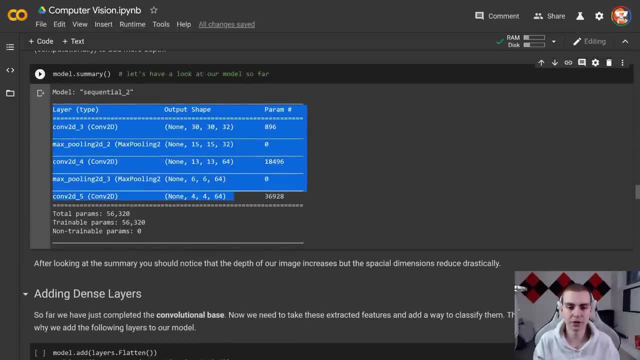 base which extracts all of the features out of your image, And then you use the dense network to say: Okay, well, if these combination of features exist, then that means this image is this, otherwise it's this and that, and so on. 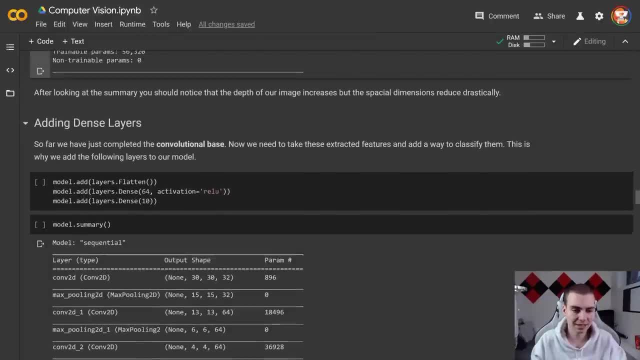 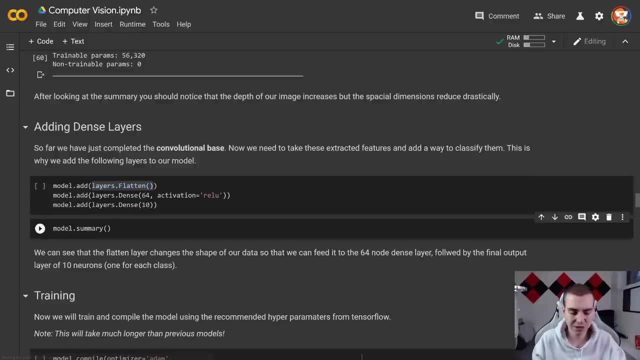 So that's what we're doing here. Alright, so let's say, adding the dense layers. So to add the density is pretty easy. model dot add is just how we add them, right. So we're going to flatten all of those pixels was, which essentially means take the four by four, by 64. And just. 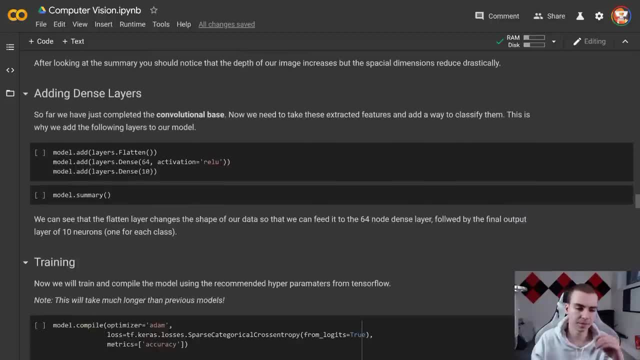 put those all into a straight line like we've done before. So just one dimensional. then we're going to have a 64. 64. Neuron dense layer that connects all of those things to it with an activation function of rectifier linear unit. then our output layer of a dense layer with 10 neurons, obviously. 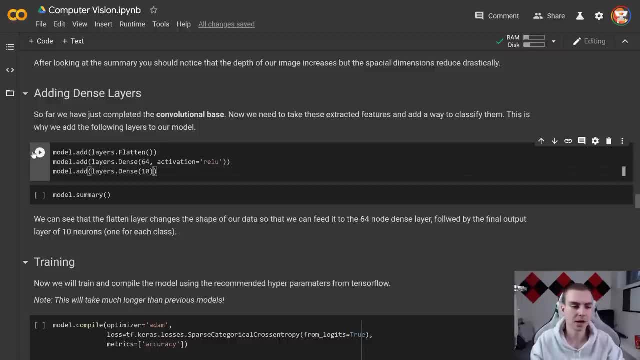 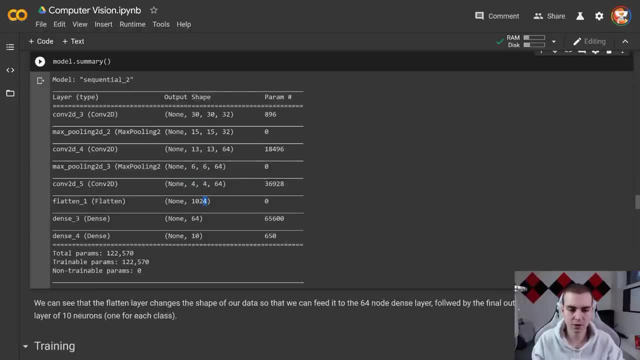 10, because that's the amount of classes we have for this problem. So let's run this here. we'll add those layers. let's look at a summary and see how things have changed now. So we go from four by four by 64: 2024.. Notice that that is precisely the calculation of four. 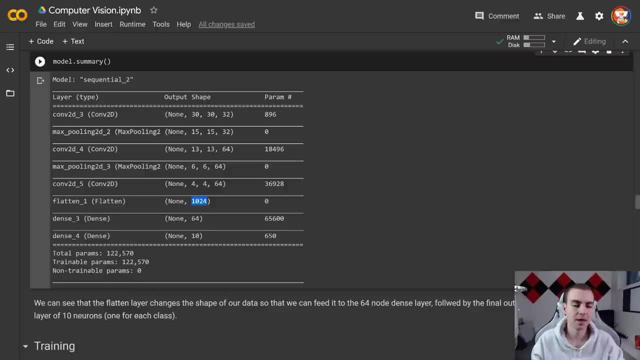 times four times 64.. That's how we get that number here. Then we have a dense layer and another dense layer And this is our output layer. Finally, this is what we're getting: is we're going to get 10 neurons out. So, essentially just. 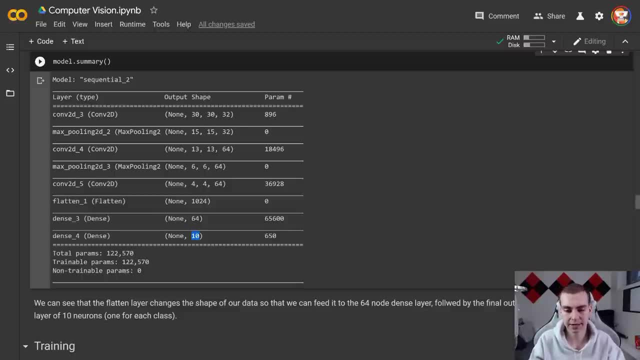 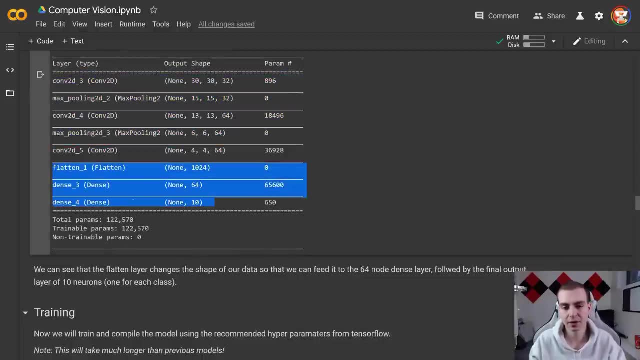 a list of values And that's how we can determine which class is predicted. So this up to here is the convolutional base, this is what we call the classifier, And they work together to essentially extract the features and then look at the features and predict the actual. 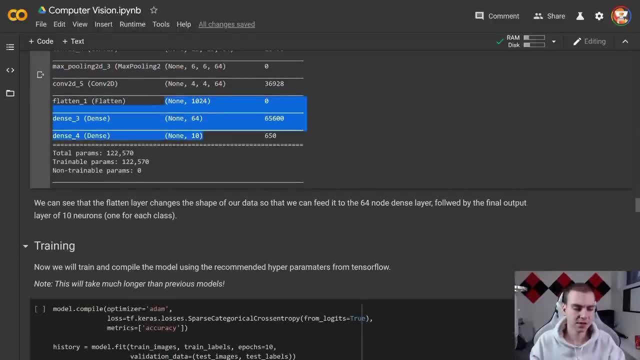 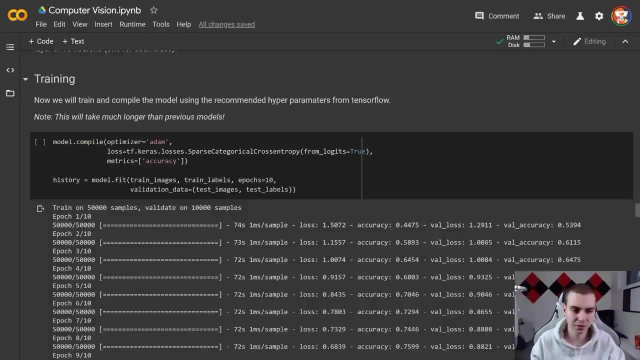 object or whatever it is the class. Alright, so that's how that works. Now it's time to train again. we'll go through this quickly. I believe I've already trained this. this takes a long time to train, So I'm actually going to reduce the epochs here. 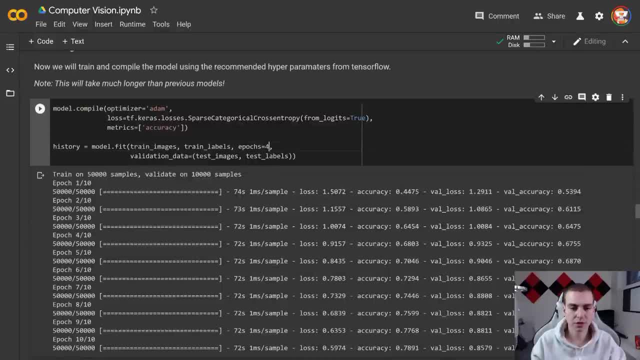 To just be for. I'd recommend you guys train this on higher. So like 10, if you're going to do it does take a while. So for our purposes and for my time, we'll leave a little bit shorter right now, But you should be getting about a 70% accuracy And you can see I've 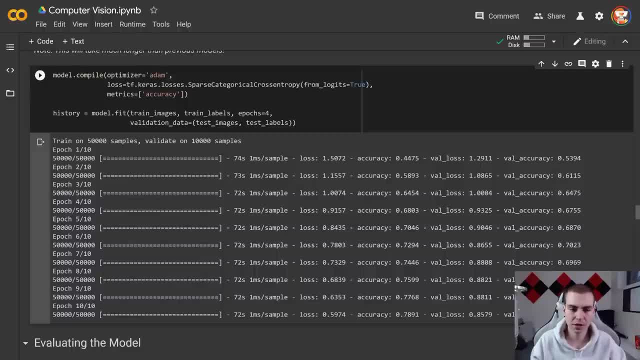 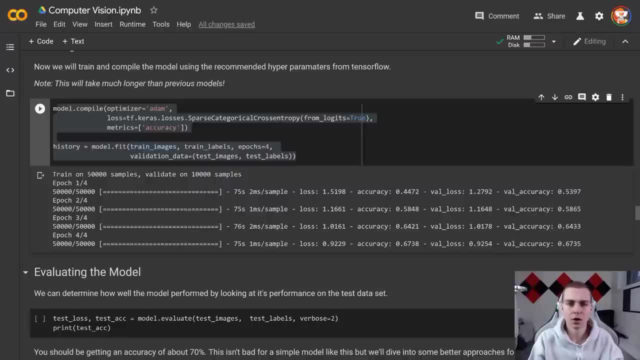 trained this previously. if you train it on 10 epochs- but I'm just going to train up to four- we'll get our 67- 68% And that should be fine. So we'll be back once this is trained. then we'll talk about how some of this works. Okay, so the model is finally finished training. 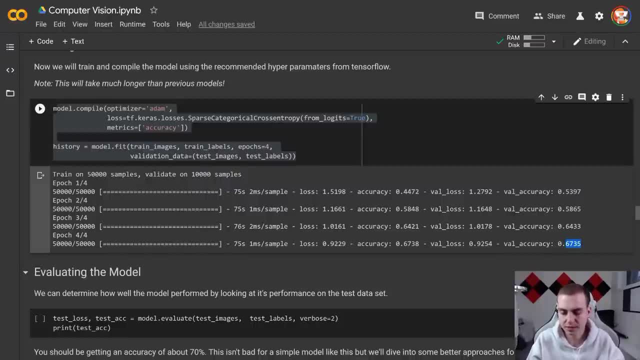 we did about four epochs. you can see we got an accuracy of about 67% On the evaluation. we got about 60% accuracy And then we're going to go ahead and we're going to go ahead and do an evaluation data To quickly go over this stuff. optimizers Adam talked about. 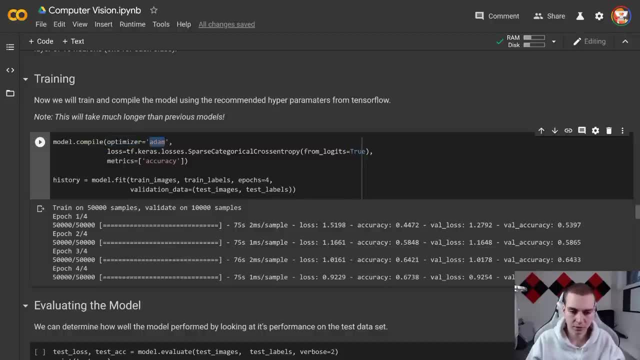 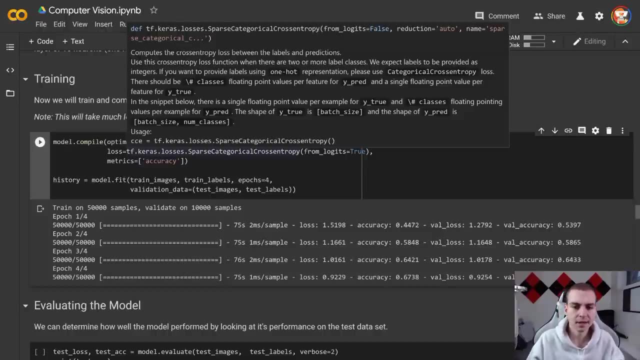 that before loss function is sparse categorical cross entropy. That one, I mean you can read this if you want- computes the cross entropy loss between the labels and predictions, And I'm not going to go into that. But these kind of things are things that you can look up. 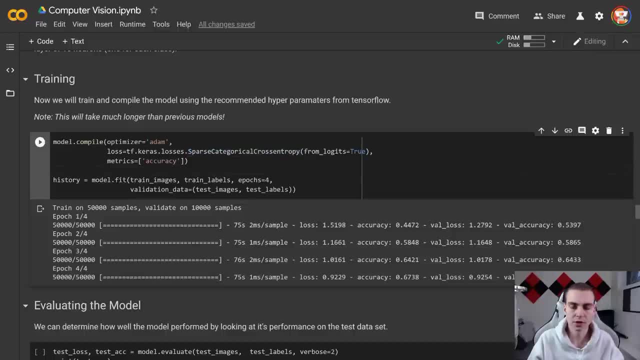 if you really understand why they work. For most problems, you can just. if you want to figure out what you know, loss function or optimizer to use, just use the basics like: use Adam, use a categorical cross entropy. If you're using a classification task you want to do something like this, there's just 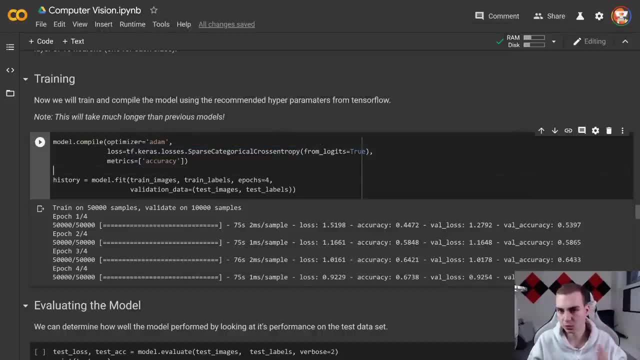 you can go up and look kind of all of the different loss functions and it'll tell you when to use which one, and you can kind of mess with them and tweak them if you want. Now, history equals model dot fit. This is just so we can access some of the statistics. 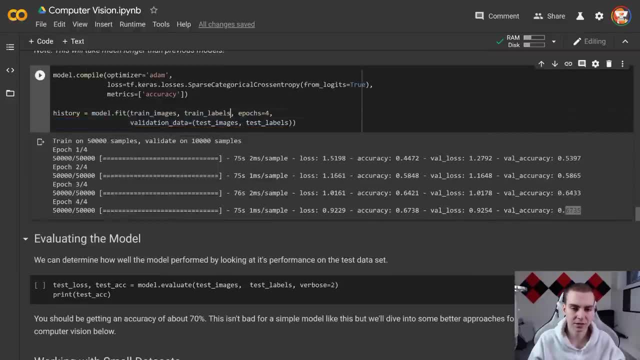 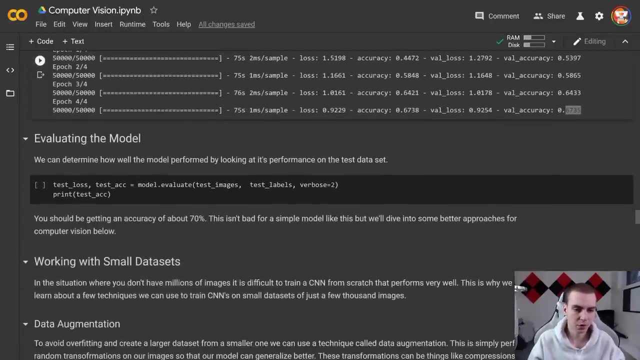 from this model dot fit. obviously it's just training the data to this: test images, test labels and train images and train labels, where this is the validation data suite. So, evaluating the model: we want to evaluate the model, we can evaluate it now on the test. 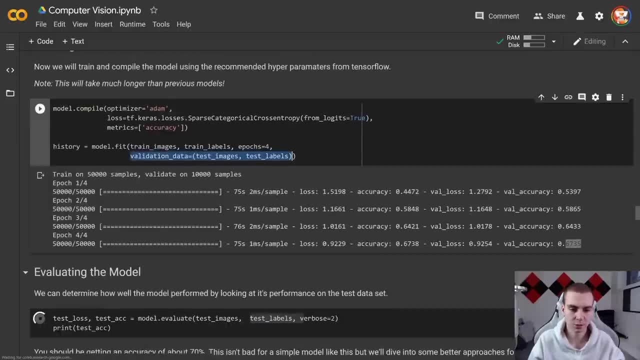 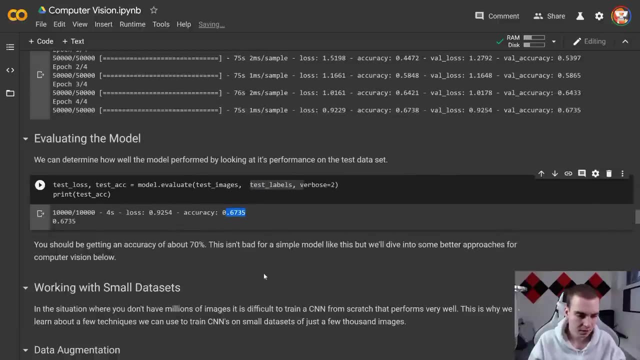 images And test labels. we're obviously going to get the same thing, because the valuation is test images and test labels, So we should get the same accuracy as 6735, which we do right here. Alright, so there we go. we get about 70%. If you guys train this on 10 epochs, you should. 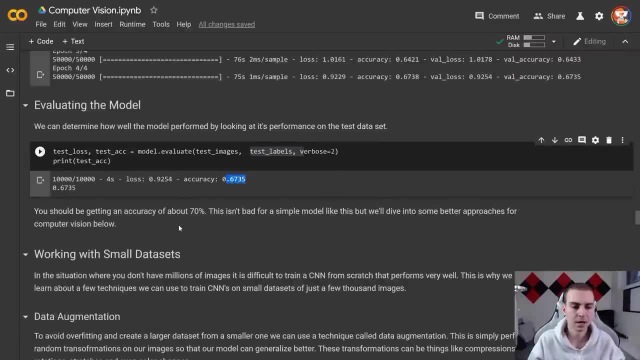 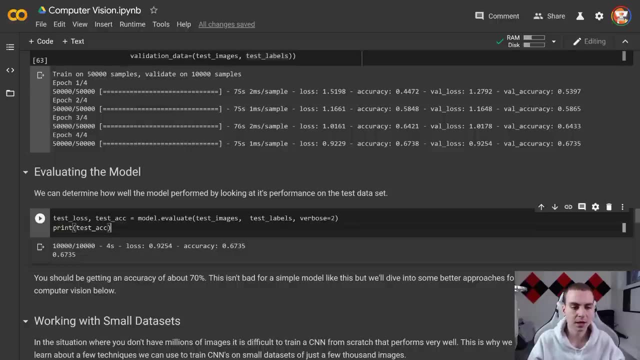 get close to 70, I'm a little bit lower just because I didn't want to go that high, And that is now the model. I mean we could use this if we want. we could use predict, we could pass in some image and we could see the prediction for it. I'm not going to do 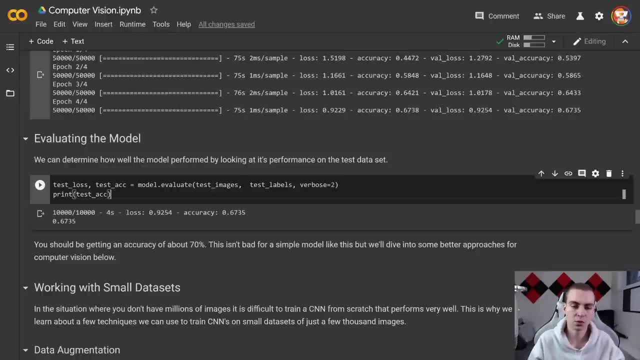 that just because we've already talked about that enough And I want to get into some of the cooler stuff When we're working with smaller data sets. So the basic idea here is: this is actually a pretty small data set, right? we use about 60,000 images And if you think about the amount of different patterns, 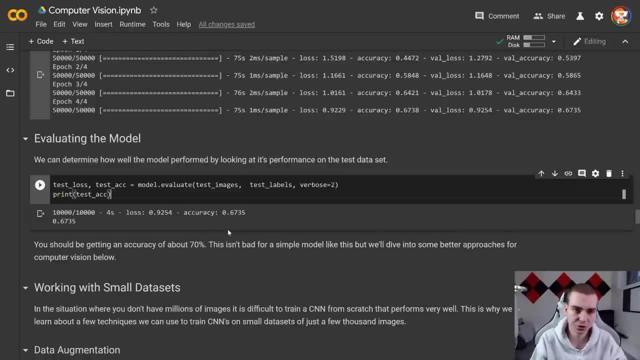 we need to pick up to classify, you know, things like horses versus trucks. that's a pretty difficult task to do, which means that we need a lot of data, And, in fact, some of the best convolutional neural networks that are out there are trained on millions of pieces. 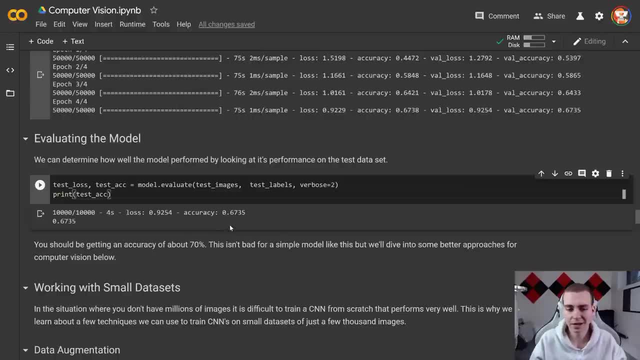 of you know sample information or data, So obviously we don't have that kind of data. So how can we work with? you know a few images, maybe like a few 1000 images, and still get a decent model? Well, the thing is you can't, unless we use 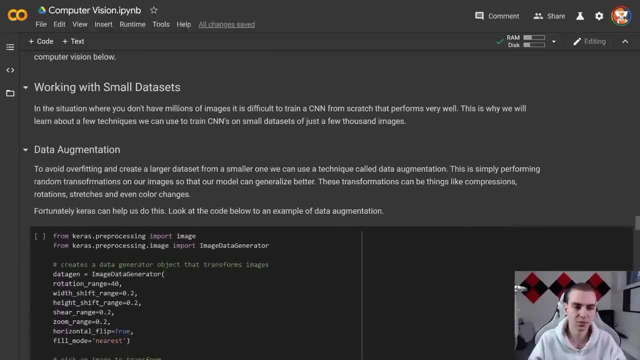 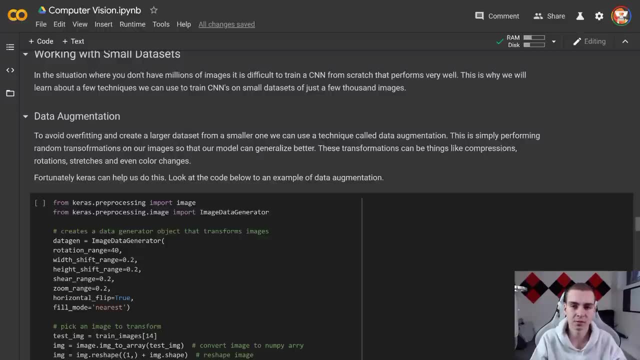 some of the techniques that I've had to show you. So working with small data sets. So, just like I mentioned, it's difficult to create a very good convolutional neural network from scratch if you're using a small amount of data. That is why we can actually employ these. 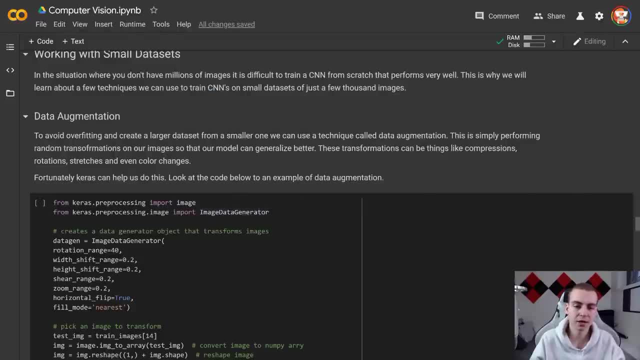 techniques. the first one, data augmentation- but also using pre trained models to kind of accomplish what we need to do, And that's we're going to be talking about now. in the second part of the tutorial, we're going to create another convolutional neural network. 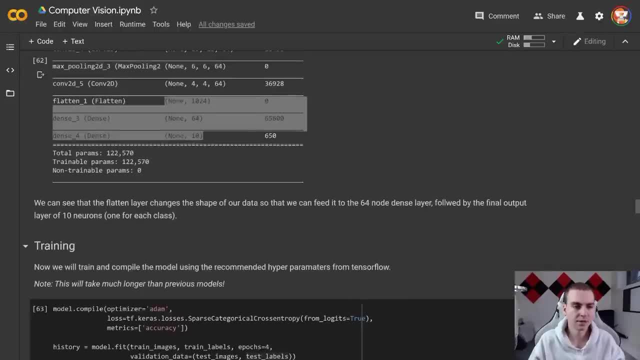 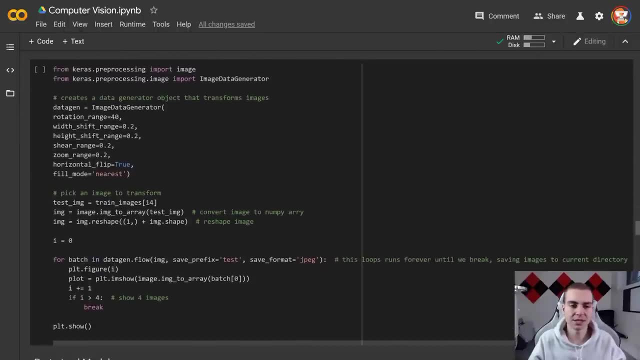 So, just to clarify, this is created. we've made the model up here already. this is all we need to do to do it. This is the architecture And this was just to get you familiar with the idea. So, data augmentation. So this is basically the idea. if you have one image, 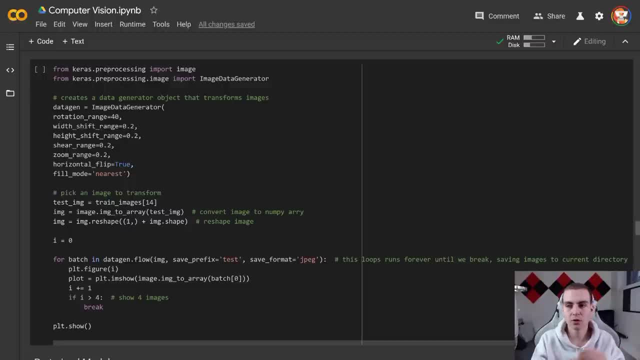 we can turn that image into several different images and train and pass all those images to our, our model. So, essentially, if we can rotate the image, if we can flip it, if we can stretch it, compress it, you know, shift it, zoom it, whatever it is, and pass it to 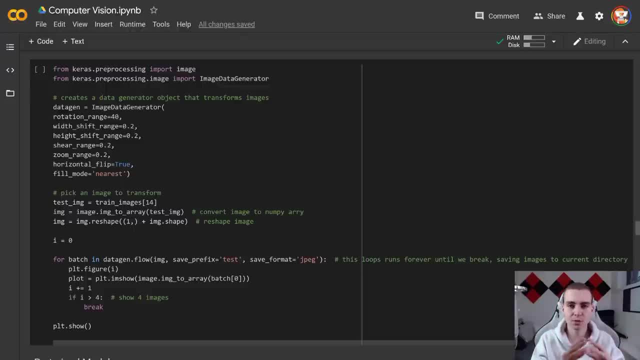 our model. it should be better at generalizing, because we'll see the same image, but modified and augmented multiple times, which means that we can turn a data set, say, of 10,000 images, into 40,000 images by doing four augmentations on every single image. Now, obviously, you 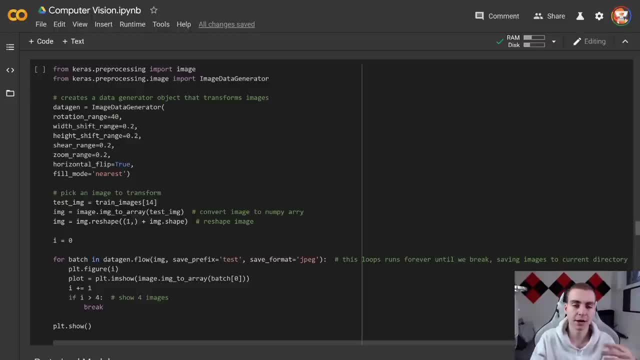 still want a lot of unique images, But this technique can help a lot and is used quite a bit because that allows our kind of model to be able to pick up images that maybe are orientated differently or zoomed in a bit or stretch something different, right. 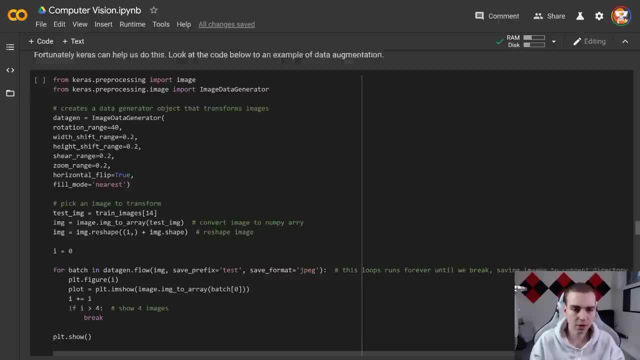 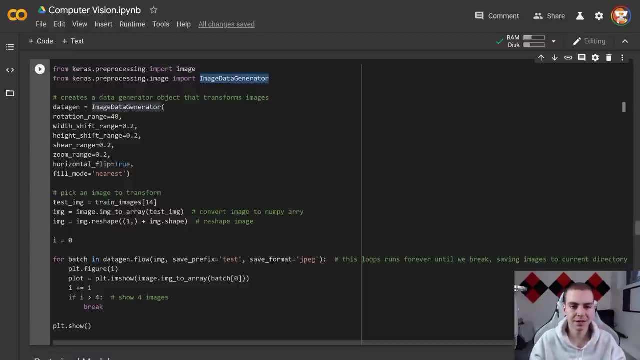 Which is better at generalizing, which is the whole point. So I'm not going to go through this in too depth, too much depth, But this is essentially a script that does data augmentation for you. we're gonna use this image image data generator from the keras dot pre processing. 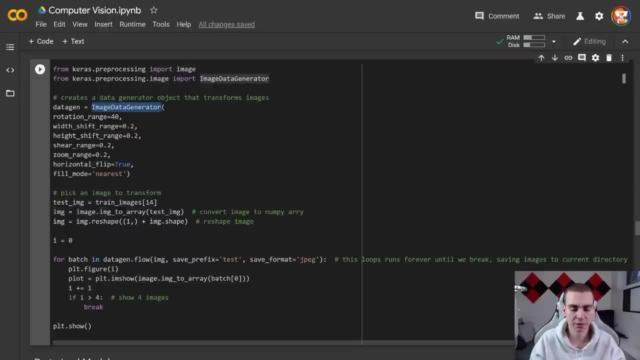 dot image module. we're going to create an image data generator object. Essentially, what this allows us to do is specify some parameters on how we want to modify our image. In this case, we have the rotation range, some shifts, shear, zoom, horizontal flip. 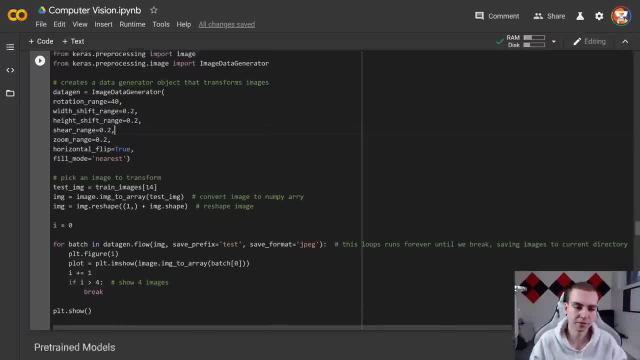 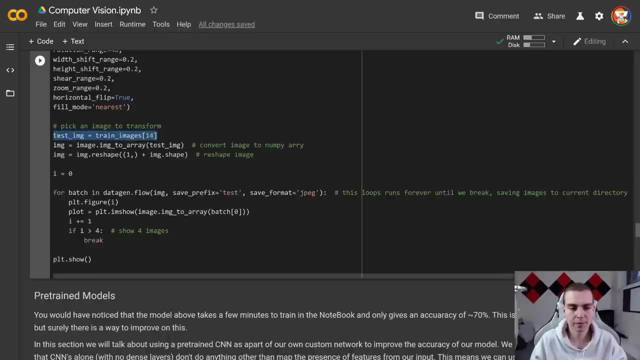 and the mode. Now I'm not going to go into how this works. you can look at the documentation if you'd like- But essentially this will just allow us to augment our images. Now what I'm going to do is pick one arbitrary image from the test image data set, just our test image. 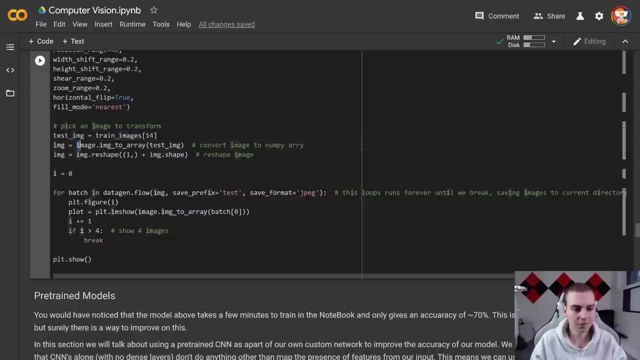 I guess group of photos, whatever you want to call it. I'm going to convert that to an image array which essentially takes it from the weird data set object that it kind of is and turns it into a numpy array. Then we're going to reshape this So it's in the form: 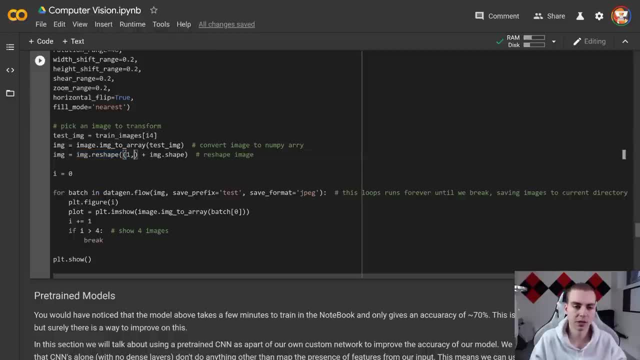 one comma, which essentially means one, and then this will figure out what the rest of the shape should be. Oh, sorry, one. and then plus the image shape, which is whatever this shape is. So we'll reshape that. And then what we're going to do is we're gonna say: 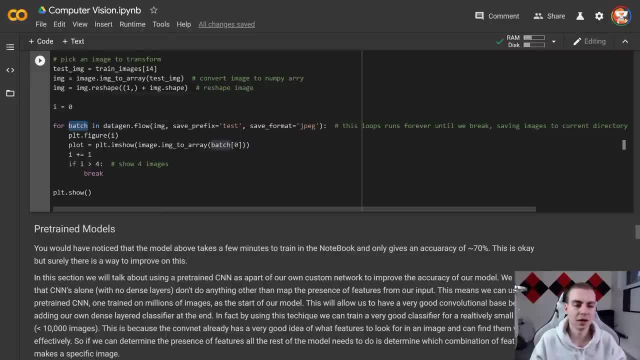 for batch in data flow, Jen dot flow. talk about how that works in a second. Essentially, this is just going to augment the image for us and actually save it onto our drive. So in this instance, what's going to happen is this: data agenda flow is going to take the 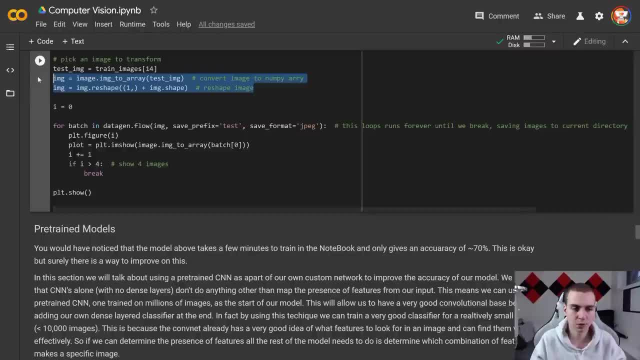 image which we've created here right and we formatted it correctly. by doing these two steps which you need to do beforehand, It's going to save this image as test dot jpeg And this will be the prefix, which means will be some information after, And it will do this as many times until we break. So, essentially, 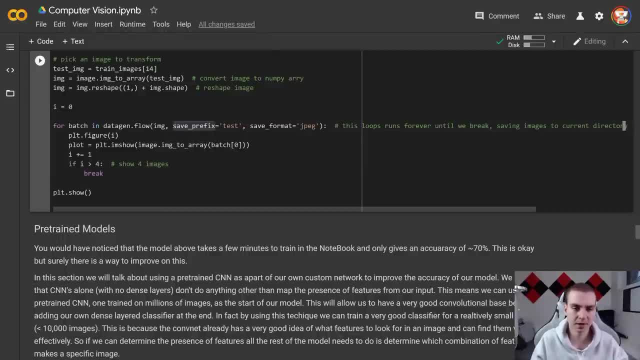 given an image, it will do test one, test two, test three, test four, test five, with random augmentations, using this until eventually. we decided to break out of this. Now, what I'm doing is just showing the image by doing this, and batch zero is just showing us the. 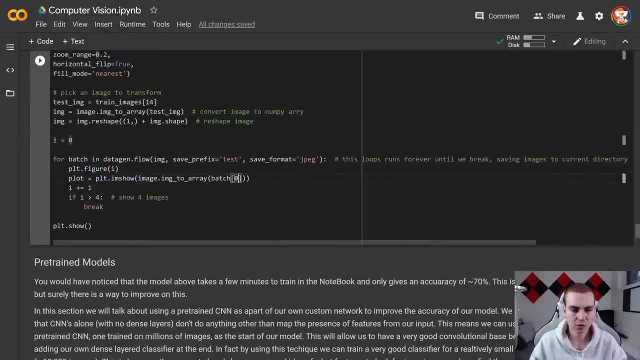 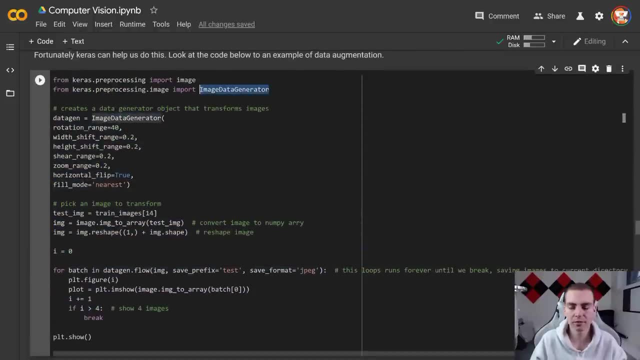 you know that first image in there And that's kind of how this works. So you can mess with the script and figure out a way to use it. But I would recommend, if you want to do data augmentation, just look into image data generator. This is something that I just want to show you. 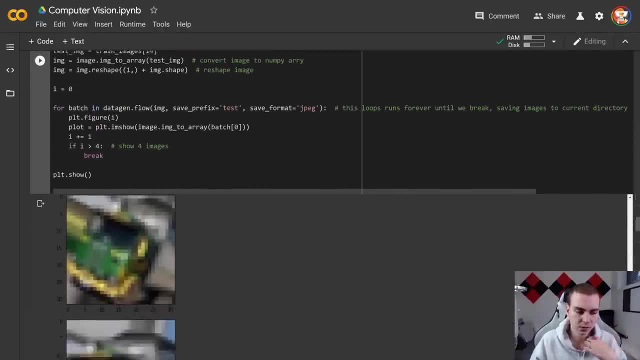 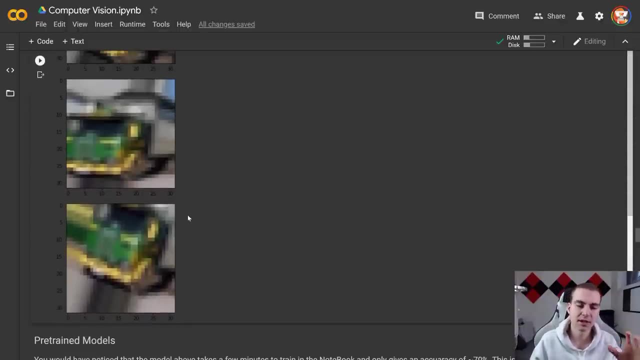 so you're aware of and I'll just run it so you can see exactly how this works. So, essentially, given an image of a truck, what it will do is augmented in these different ways. You can see kind of the shifts, the translations, the rotations, all of that And we'll do actually. 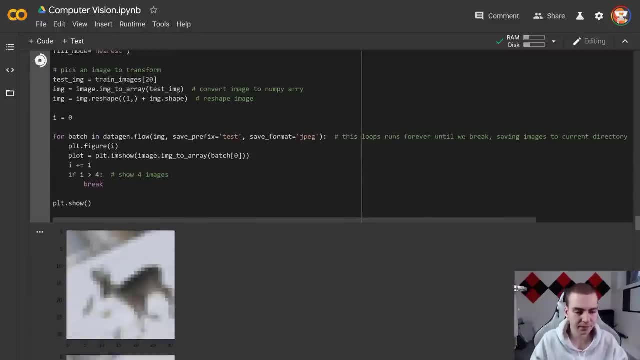 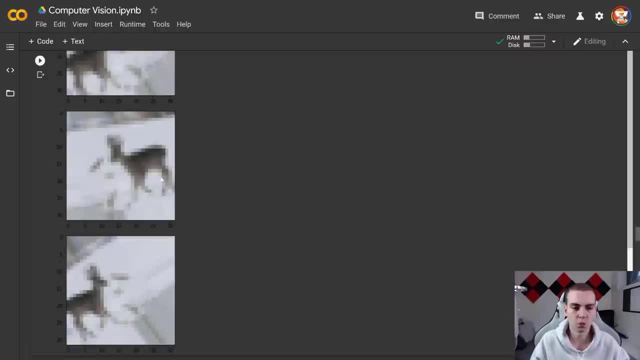 something. I don't really know exactly what it is because it's so blurry, But you can see. that's kind of the shifts we're getting, And it makes sense because you want to have images in different areas so that we have a better generalization. Alright, so let's. 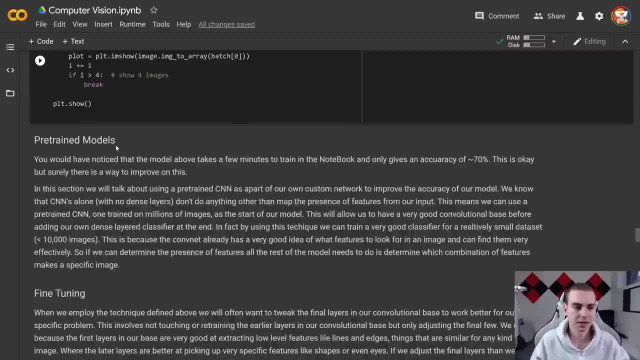 close that, Okay. so now we're gonna talk about using air. Sorry, what is a? pre trained models? Okay. So we talked about data augmentation. That's a great technique if you want to increase the size of your data set, But what if, even after that, we still don't have enough images? 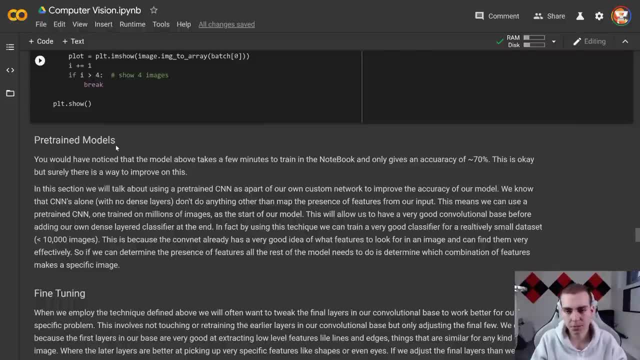 in our data set. Well, what we can do is use something called a pre trained model. Now, companies like Google- and, you know, TensorFlow, which is owned by Google, make their own amazing convolutional neural networks that are completely open source that we can use. So what we're? 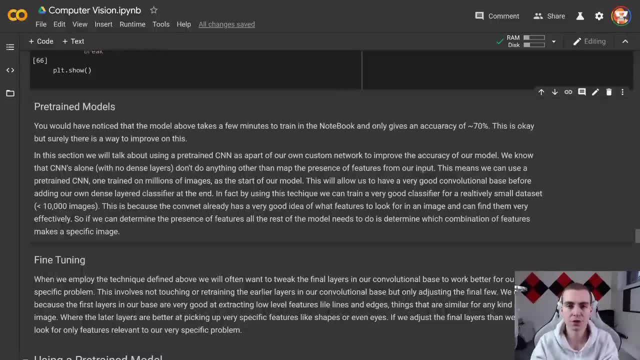 going to do is actually use part of a convolutional neural network that they've trained already on, I believe, 1.4 million images, And we're just going to use part of that model as kind of the base of our models, that we have a really good starting point And all we need to do 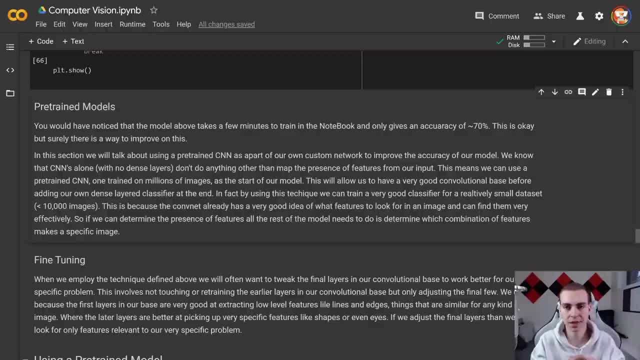 is what's called fine tune, the last few layers of that network so that they work a little bit better for our purposes. So what we're going to do essentially say, Alright, we have this model that Google's trained. they've trained it on 1.4 million images. it's capable. 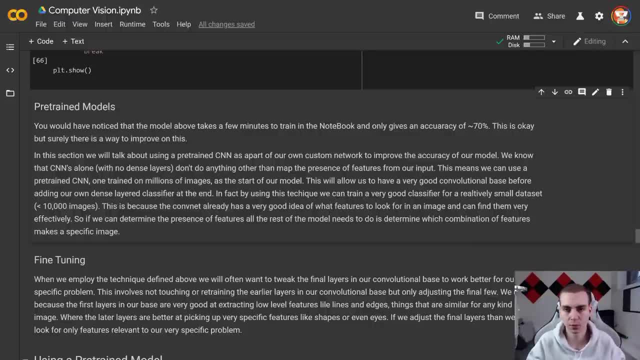 of classifying, let's say, 1000 different classes, which is actually the example we'll look at later. So obviously the beginning of that model is what's picking up on the smaller edges, and you know, kind of the very general things that appear in all of our images. So 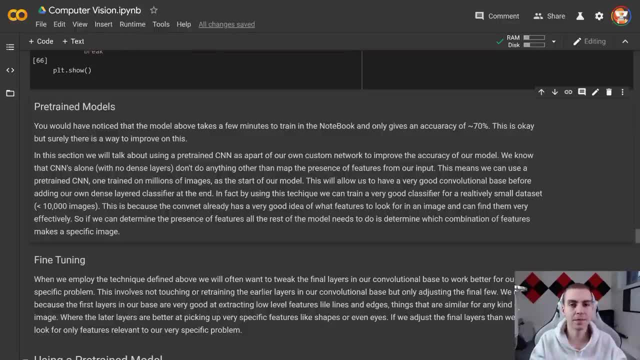 if we can use the base of that model, so kind of the beginning of it, that does a really good job picking up on edges and general things that will apply to any images, then what we can do is just change the top layers of that model a tiny bit or add our own layers to it to classify. 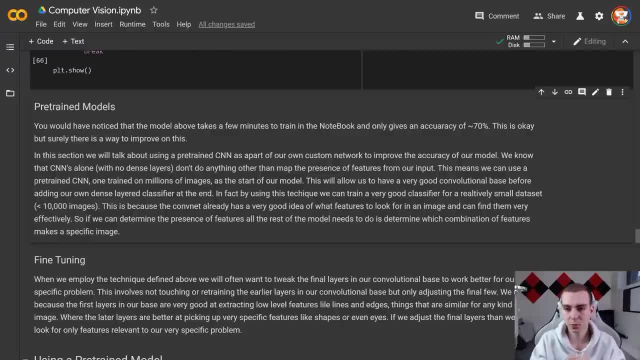 for the problem that we want And that should be a very effective way to use this pre trained model. we're saying we're going to use the beginning part that's really good at kind of the generalization step, then we'll pass it into our own layers. that will do whatever. 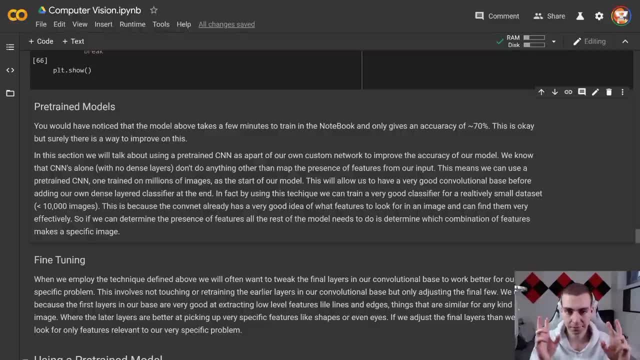 we need to do specifically for our problem, That's what's like the fine tuning step, And then we should have a model that works pretty well. In fact, that's what we're going to do in this example now, So that's kind. 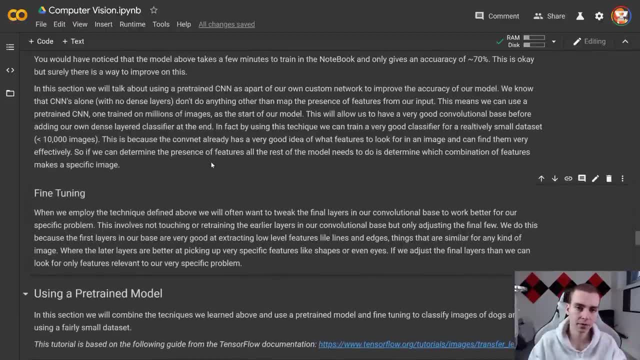 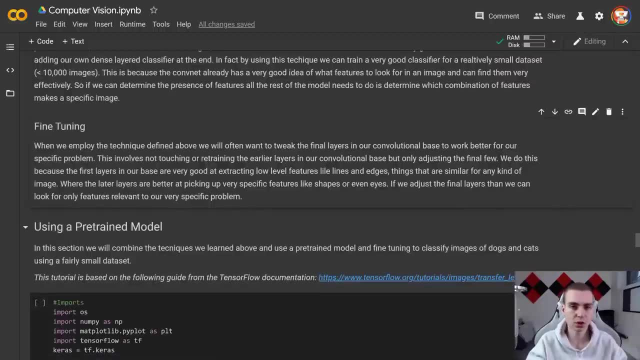 of the point of what I'm talking about here is using part of a model that already exists. that's very good at generalizing and it's been trained on so many different images, And then we'll pass our own training data in. we won't modify the beginning aspect of 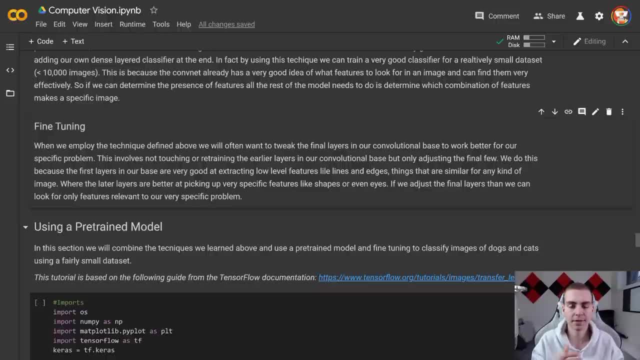 our neural network because it already works really well. we'll just modify the last few layers that are really good at classifying, for example, just cats and dogs, which is exactly the example that we're going to use. So we're going to go ahead and do that. So 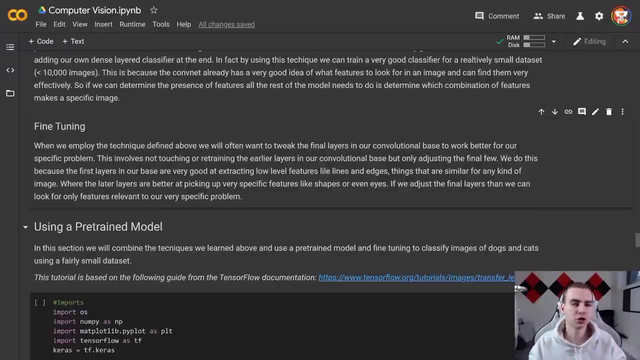 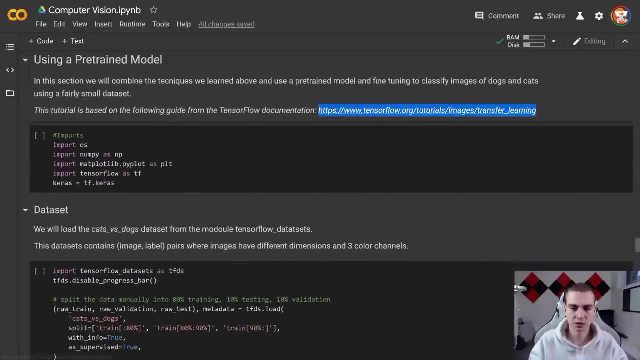 I hope that makes sense. As we get through this should be cleared up a little bit. But using a pre trained model is now the section we're getting into. So this is based on this documentation. As always, I'm referencing everything So you guys can go see that. if 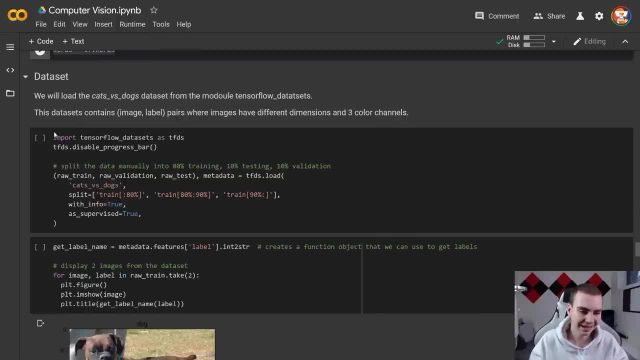 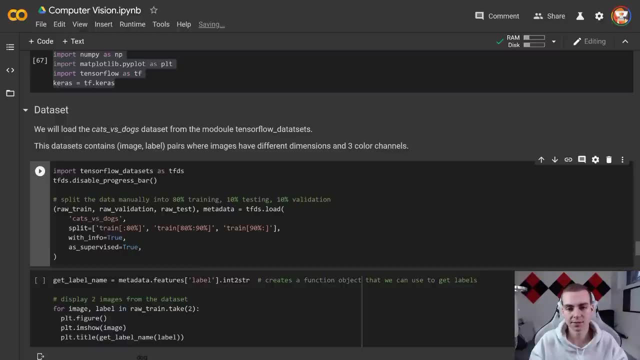 you'd like we do our imports like this: we're going to load a data set. this actually takes a second to load the data set, I believe- oh, maybe not- And essentially the problem we're doing is trying to classify dogs versus cats with a fair degree of accuracy, In fact. 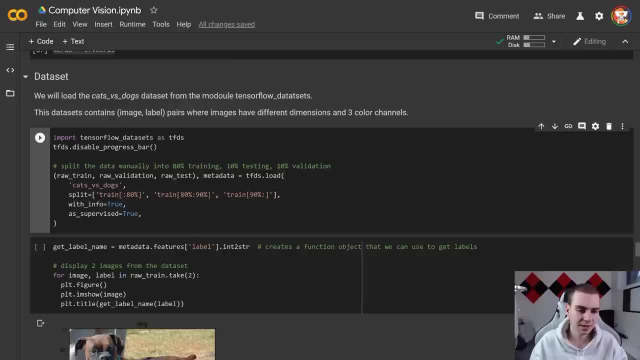 we'd like to get above 90%. So this is the data set we're loading in from TensorFlow data sets as TF DS. This is kind of a weird way to load it in Again stuff like this. you just have to reference the documentation. I can explain it to you. But 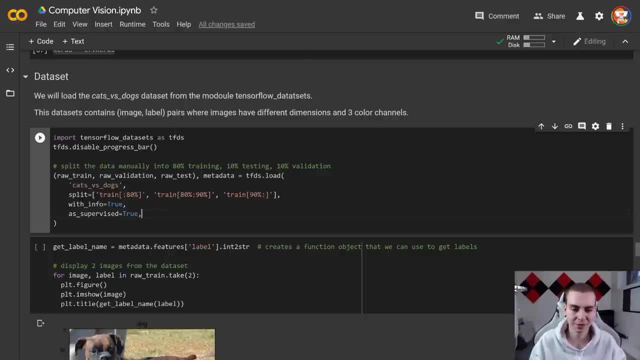 it's not really going to help when the next example is going to be a different way of loading the data right. So so long as you know how to get the data in the correct form, you can get it into some kind of NumPy array. you can split it into training, testing and 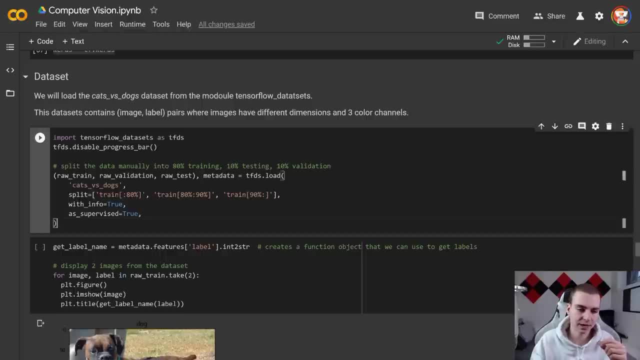 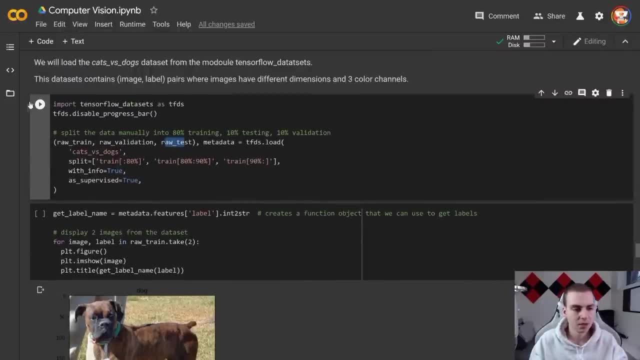 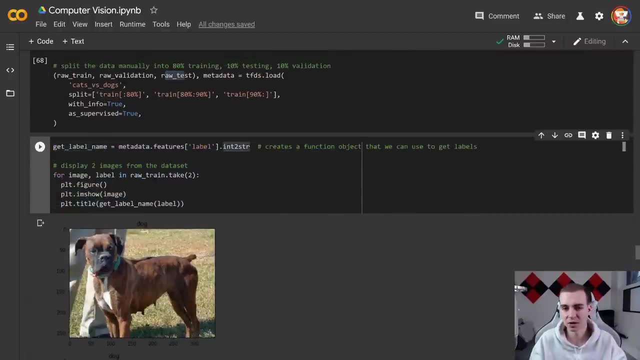 in: 10% for what is it- raw validation- and 10% for the testing data. So we've loaded that, And now what we're doing here is this: we're looking at a few images, So this actually creates a function. I know this is a weird thing. This is pretty unique to this example. 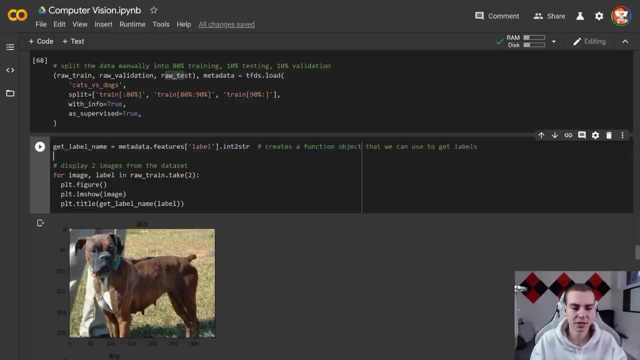 that allows us to call this function with some integer, essentially, and get what the actual string representation of that is. So the label for it And what I'm doing here is just taking two images from our raw training data set and just displaying them And you. 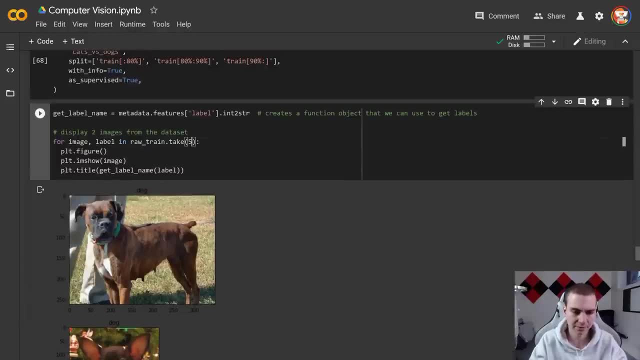 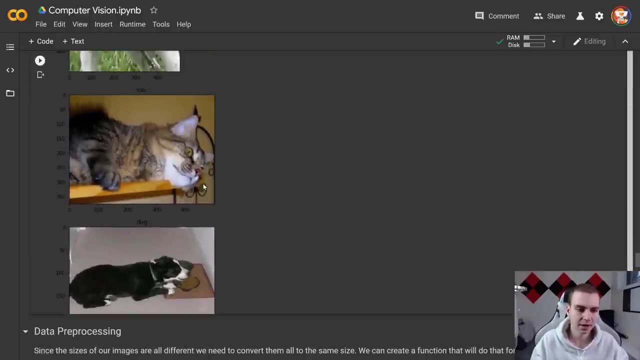 can see. that's what we're getting here: dog and dog. If I go ahead and take five, we'll see. these are what our images look like, Right. So here's an example of a dog. we have a cat right, And so on, so forth. 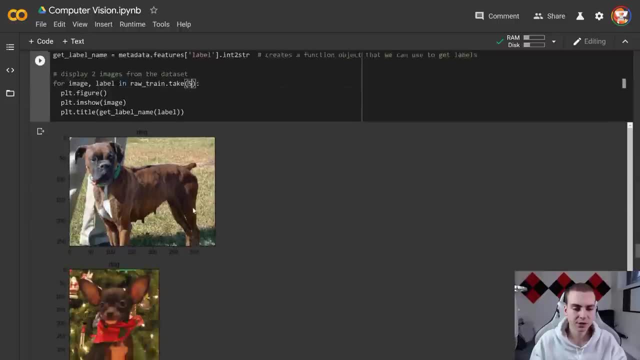 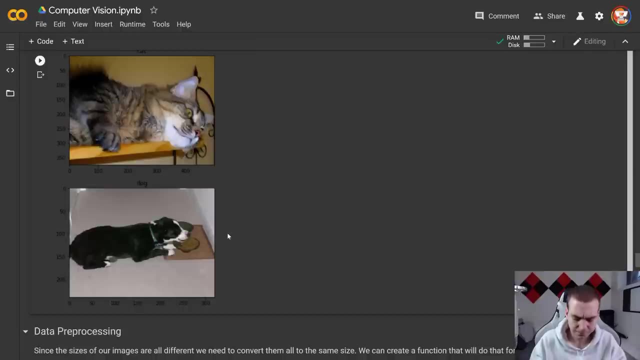 you kind of: you get that. you get the point there. Now notice, though, that these images are different dimensions. In fact, none of these images, other than these two, actually are the same dimension at all. Actually, I don't think these ones are either So obviously. 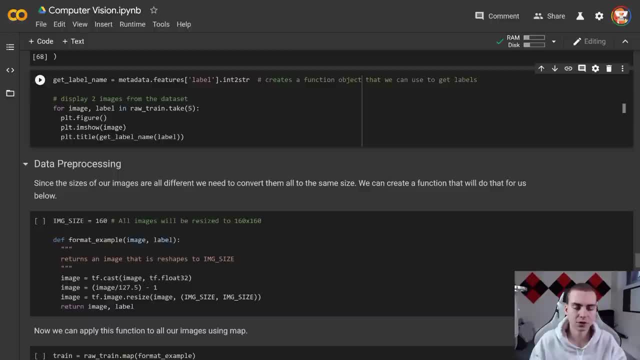 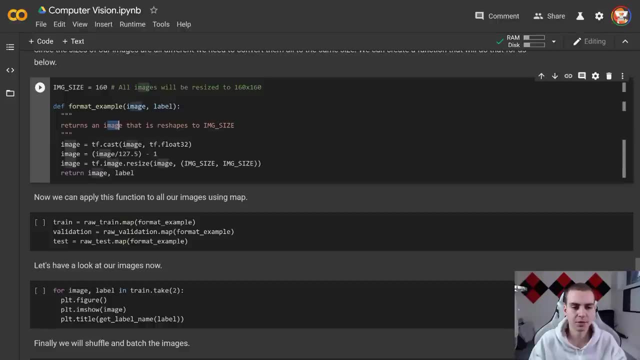 there's a step that we need to do, which is we need to scale all these images to be the same size. So to do that, what we're going to do is write a little function like this that, essentially, will return an image that is reshaped, So I guess that is reshaped to. 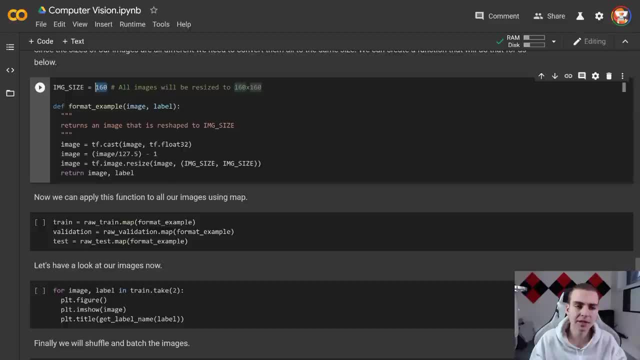 the image size, which I'm going to set at 160 by 160.. Now we can make this bigger if we want, But the problem sometimes if you make an image that is bigger than like, you want to make your image bigger than most of your data set examples, And that means you're. 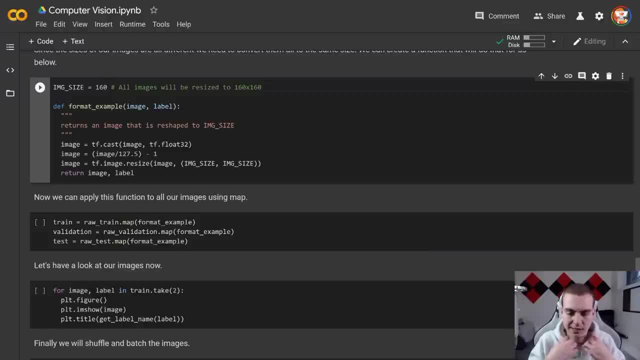 going to be really stretching a lot of the examples out and you're losing a lot of detail. So it's much better to make the image size smaller rather than bigger. You might say: Well, if you make it smaller, you're gonna lose detail too. 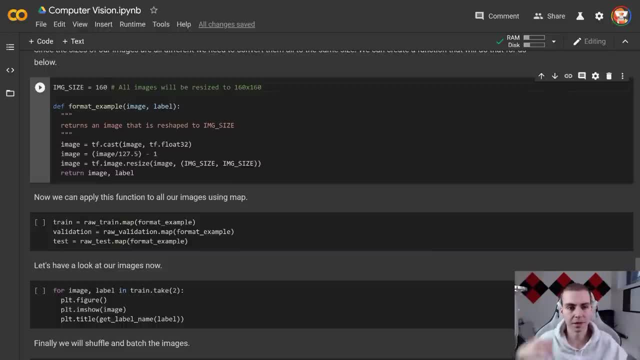 But it's just, it's better to compress it smaller than it is to go really big, even just when it comes to the amount of training time and how complex the network is going to be. So is that something to consider? You can mess around with those when you're making your. 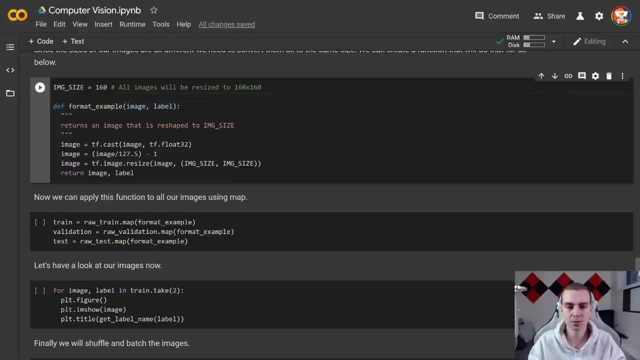 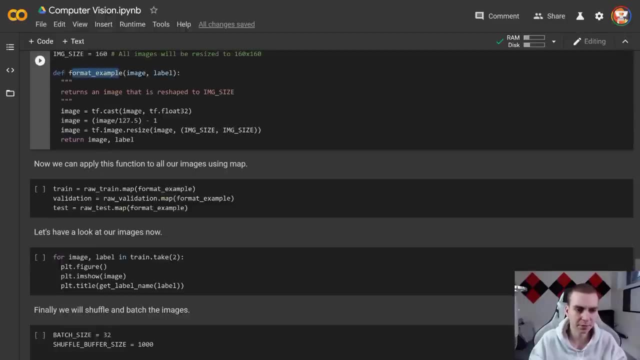 own networks. But again, smaller is typically better, In my opinion. you don't want to go too small, but something that's like you know, half the size of what an average image would be. Alright, so we're gonna go format example, So we're gonna just take an image. 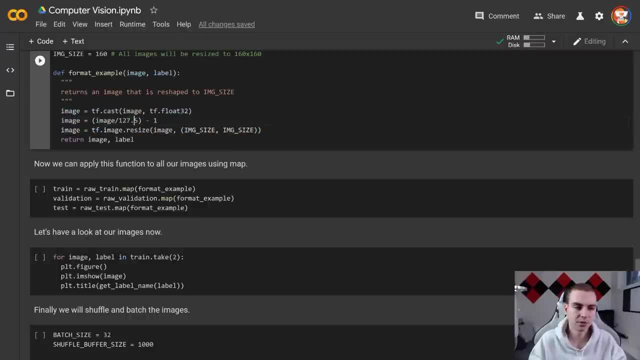 and a label, And what this will do is return to us just the reshaped image and label. So in this case we're going to cast, which means convert every single pixel in our image to be a float 32 value, because it could be integers. we're 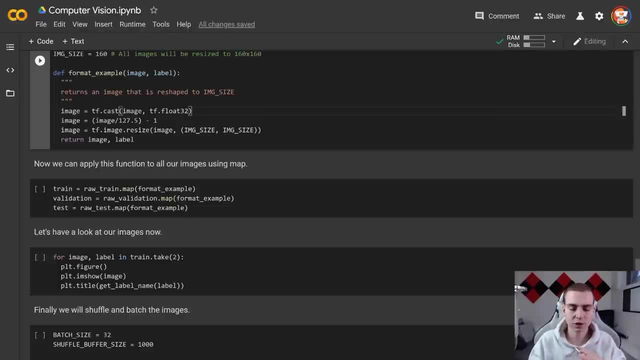 then going to divide that by 127.5, which taken, is exactly half of 255. And then subtract one, then we're going to resize this image to be the image size. So sorry, the image will be resized to the image size, So 160 by 160.. And we'll return the new image and 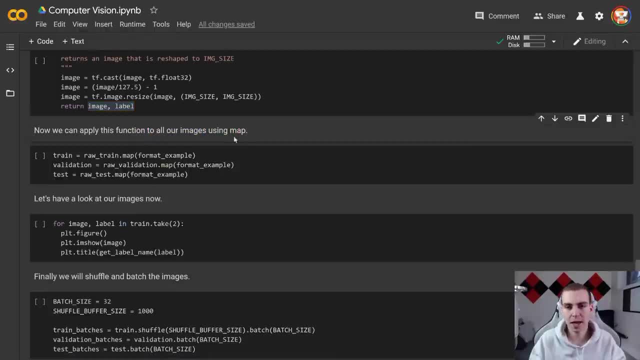 the label. So now we can apply this function to all of our images using map. if you don't know what map is, essentially, it takes every single example in- in this case going to be raw train- and applies the function to it, which will mean that it will convert to raw train into images. 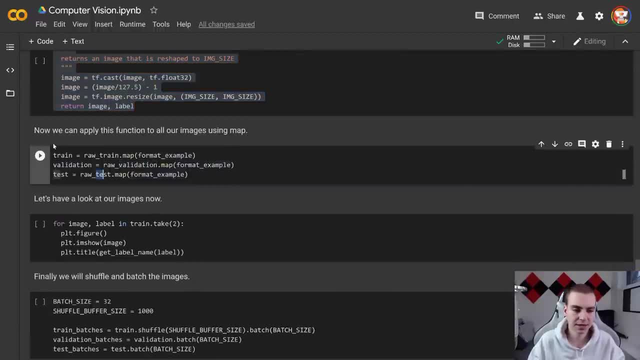 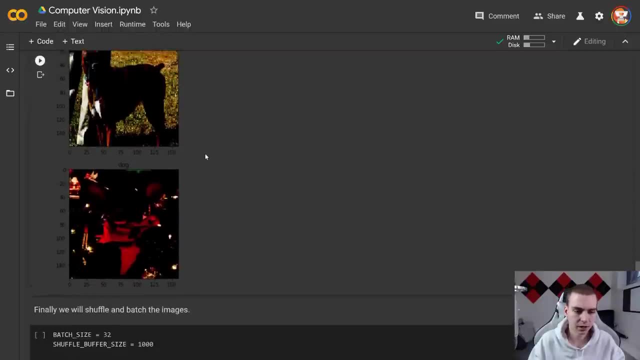 that are all resized to 160 by 160. And we'll do the same thing for validation and test. So run that, no issue there. Now let's have a look at our images and see what we get. And there we are. Now. I've just messed up the color because I didn't add a C map thing. 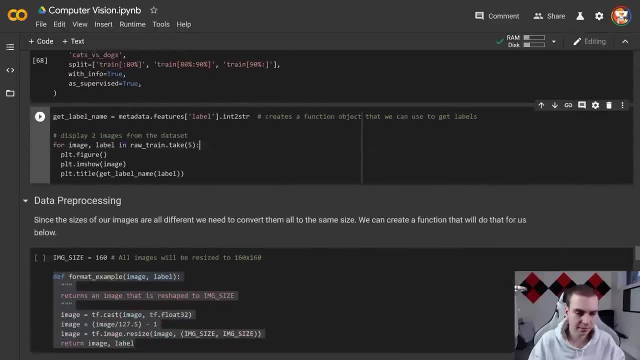 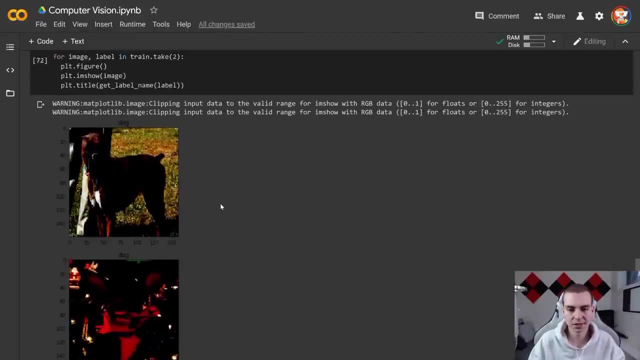 which I think I needed. Where was the C map? Anyways, you know what? that's fine, I'm going to do that. That's fine. For now, This is what our images look like. This is the resize. Now we get all our images 160 by 160. And we are good to go. Alright. so now let's have 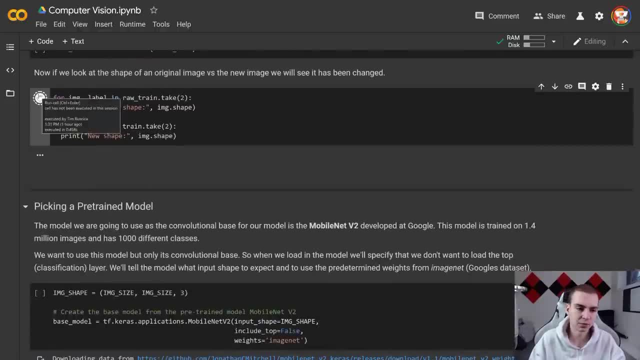 a look at the shape of an original image versus our new image. So I mean, this was just to prove that essentially our original shapes were like 262, 409 by some random values, And they're all reshaped now to 160, 160 by three. three, obviously, is the color channel of the 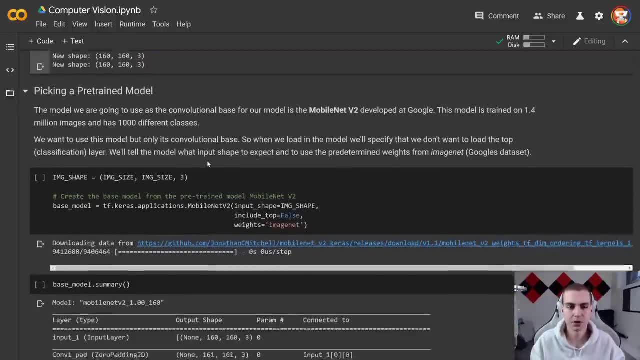 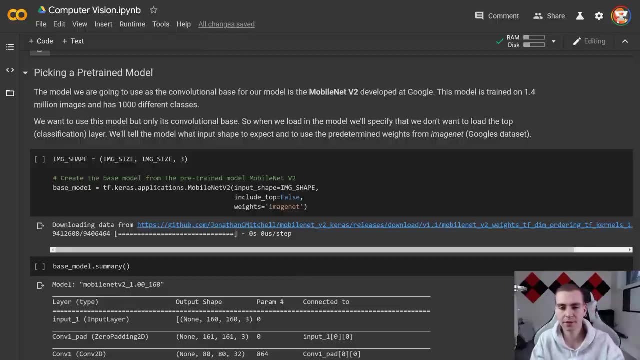 images. Alright, so picking a pre trained model. So this is the next step. This is probably one of the harder steps- Is picking a model that you would actually like to use the base of. Now we're going to use one called mobile net v two, which is actually from Google. it's built into TensorFlow. 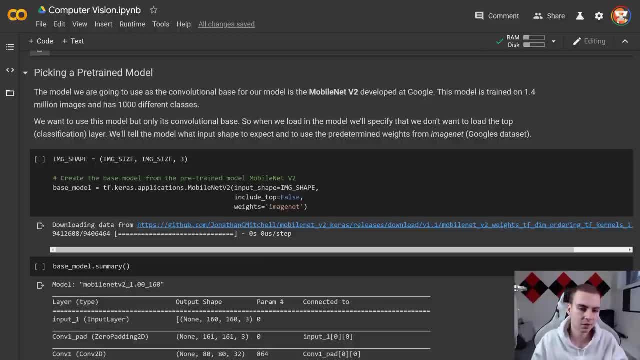 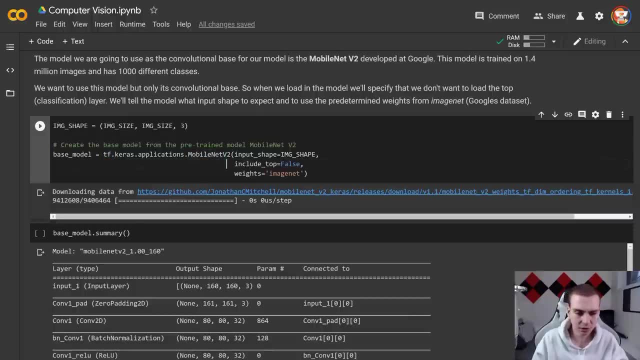 itself. That's why I've picked it And all we're going to do is set this. So essentially, we're gonna say the base model in our code is equal to tf, dot, keras, dot, applications, dot, mobile net, v two, which is just telling us the architecture of the model that we want. 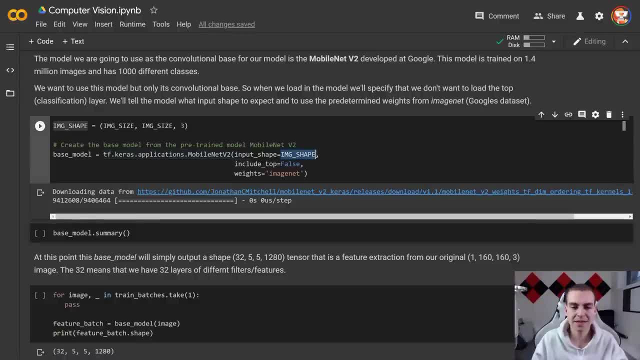 And we'll have a look at it down below here. In just a second we'll define the input shape, which is important because this can take any input shape that we want, So we'll change it to 160, 160 by three. 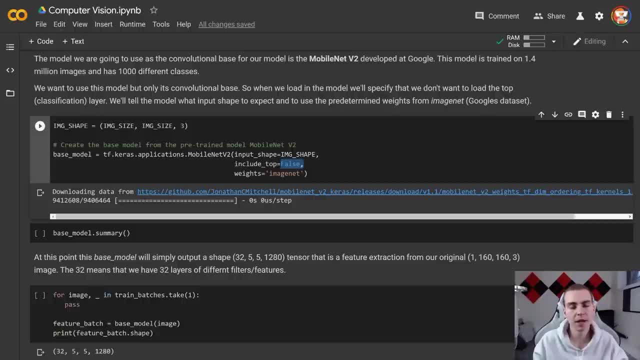 Which we've defined up here include top, very important means. do we include the classifier that comes with this network already or not? Now, in our case, we're going to be retraining parts of this network so that it works specifically for dogs and cats and not for 1000 different. 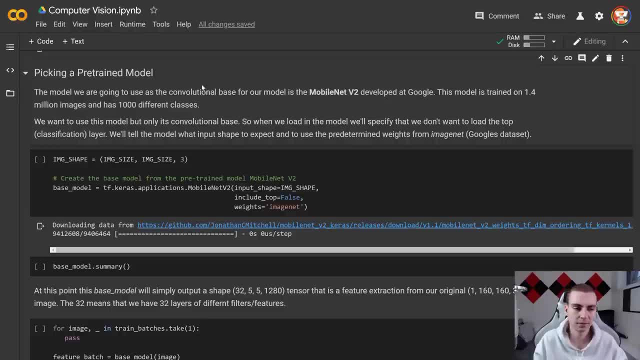 classes, which is what this model was actually aimed to do- is train a 1.4 million images for 1000 different classes of everyday objects. So we're going to not include the top, which means don't include the classifier for these 1000 classes, And we're going to go ahead. 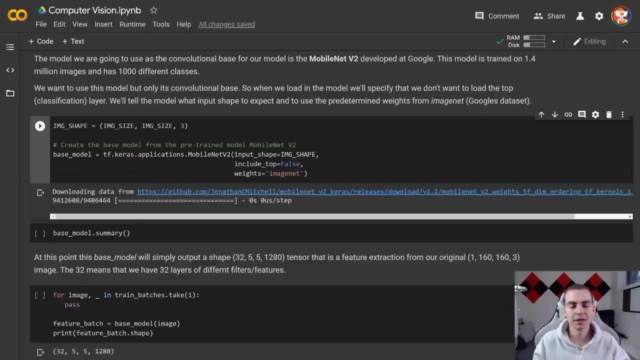 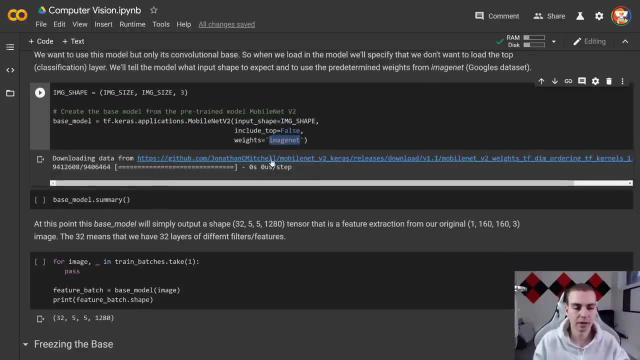 and load the weights from what's called image net, which is just a specific save of the weights. So this is the architecture And this is kind of the data that we're filling in for that architecture, So the weights, and we'll load that in which we have here. 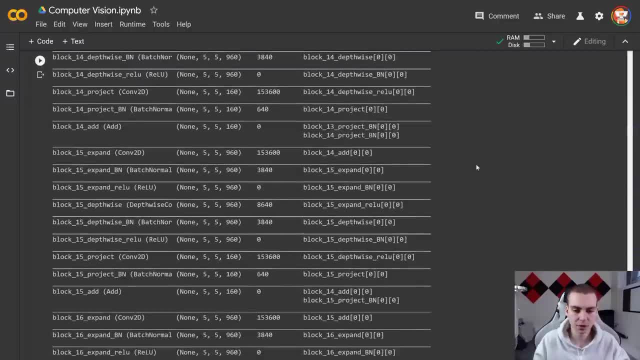 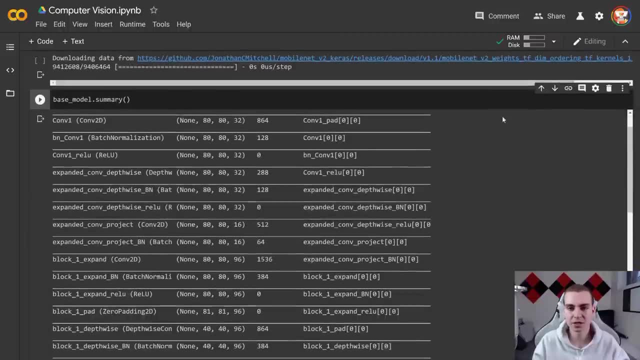 So base model. Now let's look at it. So let's have a summary. you can see, this is a pretty crazy model. I mean, we would never be expected to create something like this by ourself. This is, you know, teams of data scientists, PhD students, engineers, whatever, right. 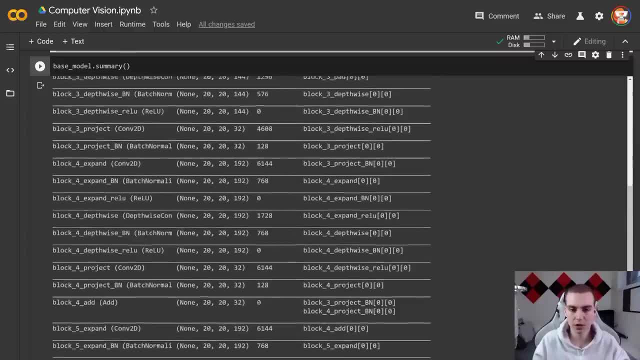 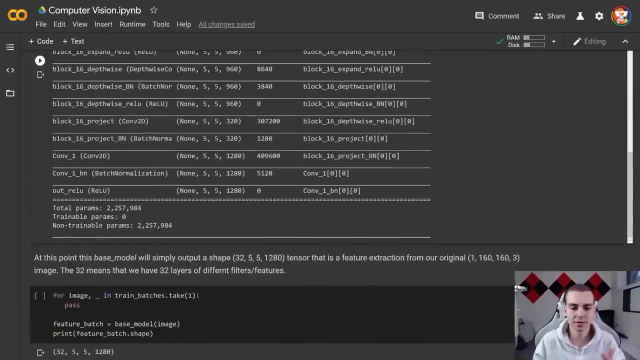 the experts in the field that have created a network like this. So that's why we're going to use it, because it works so effectively For the generalization at the beginning, which is what we want, And then we can take those features that this takes out. So, in five by five, by 1280, which is what I want. 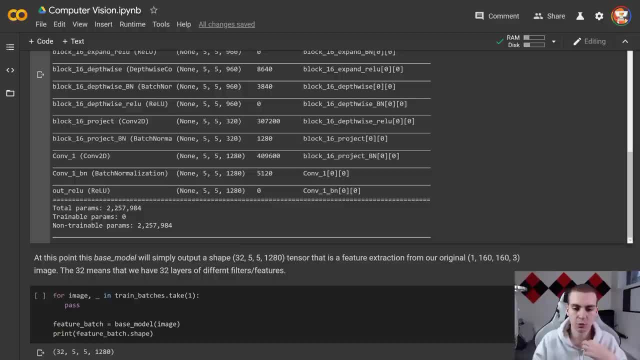 us to focus on the output of this actual network here. So out, really, you can see, this last layer. we're going to take this and, using this information, pass that to some more convolutional layers and actually our own classifier, I believe, and use that to predict versus dogs. 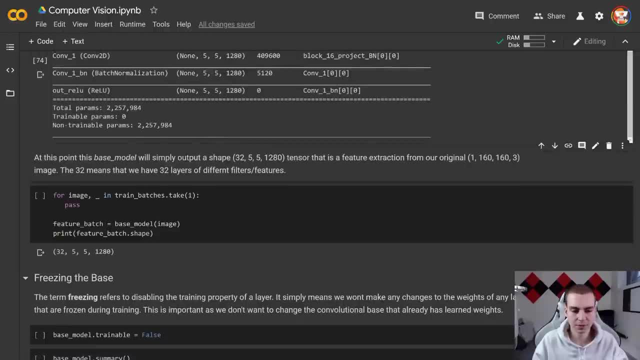 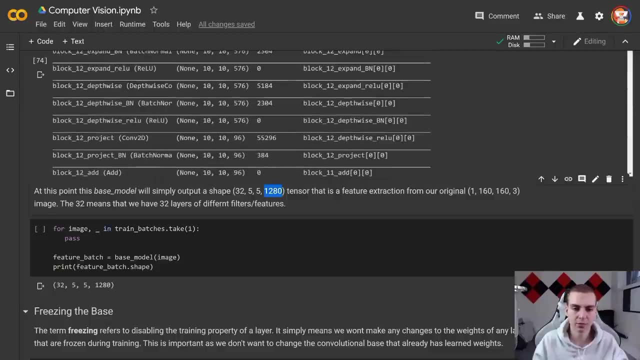 versus cats. So at this point the base model will simply open a shape: 32 by five by five by 1280.. That's the tensor that we're going to get out of this. that's the shape. you can watch how this kind of works as you go through it. And yes, all right, So we can. 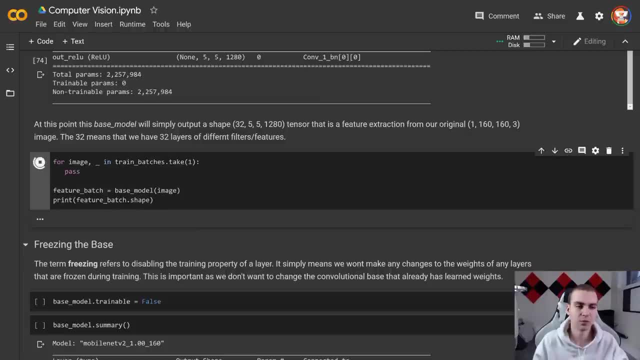 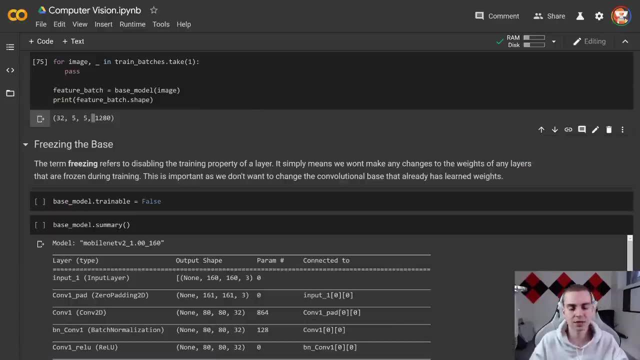 just have a look at this here. This: what I want to do, essentially, was just look at what the actual shape was going to be. So 32, five by five by 1280,. just because this gives us none until it knows what the input is. And now it's time to talk about freezing the base. 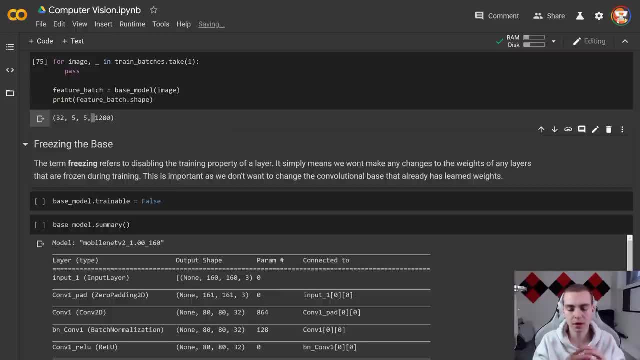 So, essentially, the point is we want to use this as the base of our network, which means we don't want to change it. If we just put this network in right now, is that going to be the base to our neural network? Well, what's going to happen is it's going to start retraining? 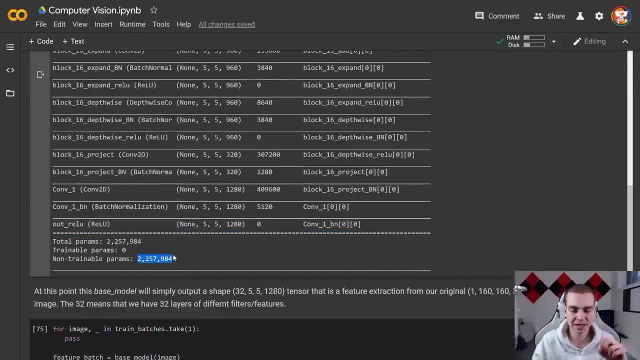 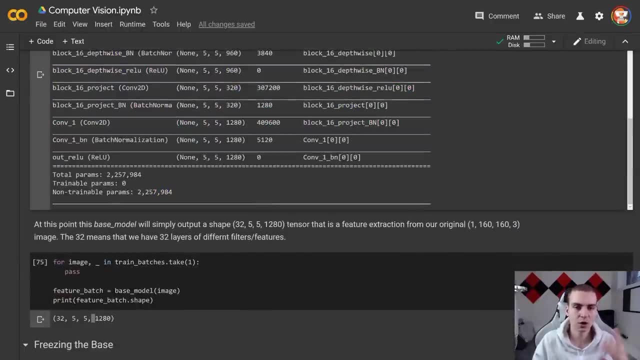 all these weights and biases And in fact it's going to train 2.257 million more weights and biases when in fact we don't want to change these because these have already been defined, they've been set and we know that they work well for the problem already right. 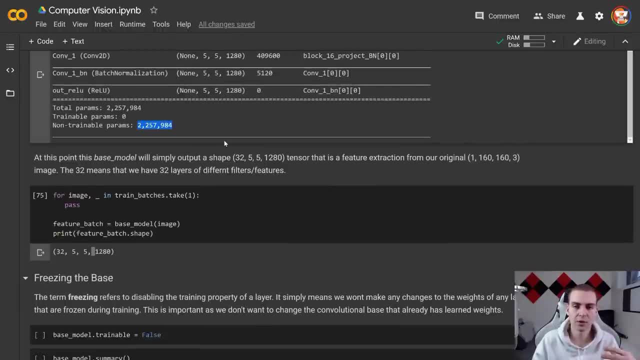 They worked well for classifying 1000 classes. why are we going to touch this now? And if we were going to touch this, what's the point of even using this base? right, We don't want to train this, we want to leave it the same. So to do that, we're just going to freeze. 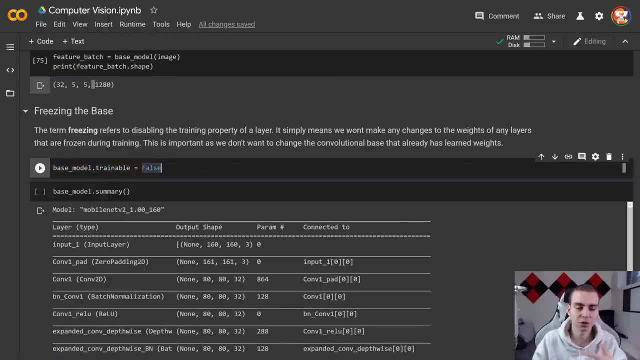 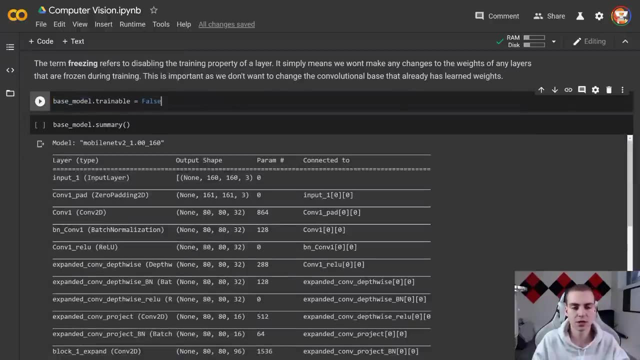 it Now, freezing is a pretty I mean. it just essentially means turning the trainable attribute of a layer off or of the model off. So what we do is we just say base model dot trainable equals false, which essentially means that we are no longer going to be training any aspect of that. I 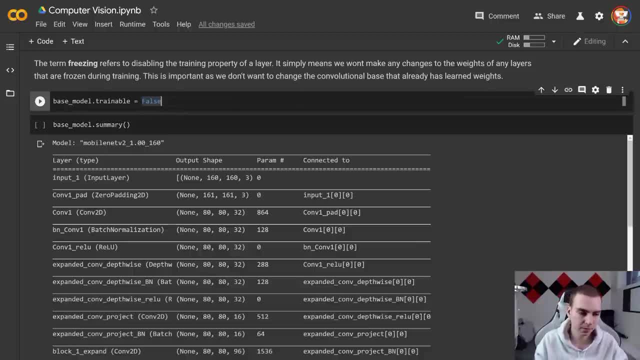 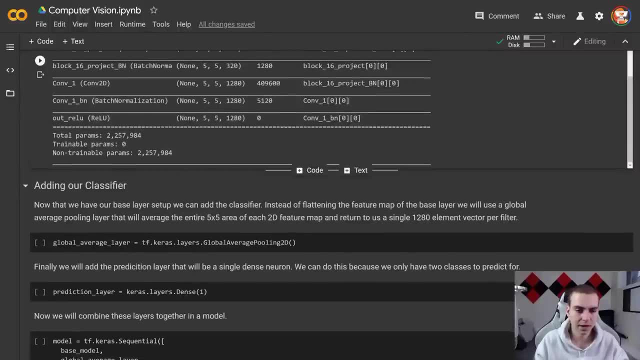 want to say model, although we'll just call it the base layer for now, or the base model. So now, if we look at the summary, we can see, when we scroll down to the bottom, if we get there any day soon- that now the trainable parameters is zero instead of 2.257 million. 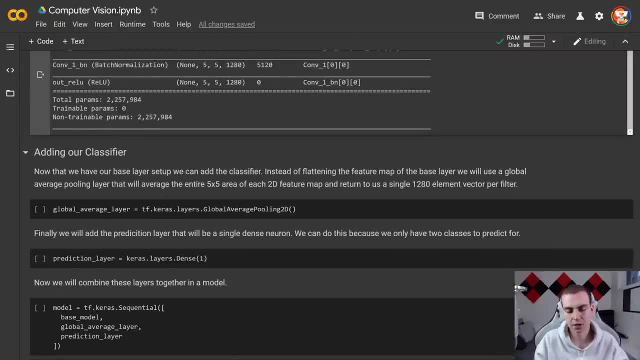 which it was before, And now it's time to add our own classifier On top of this. so essentially, we've got a pretty good network right, five by five, by 1280s, our last output, And what we want to do now is take that and we want to use. 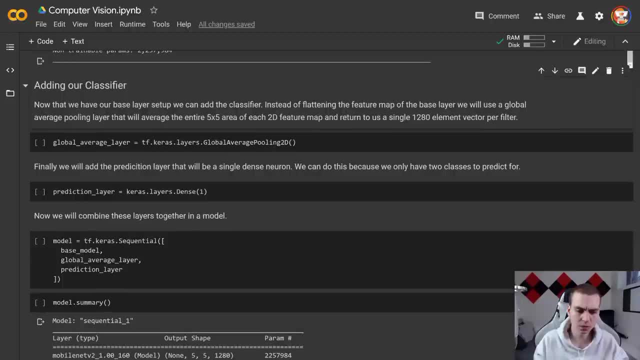 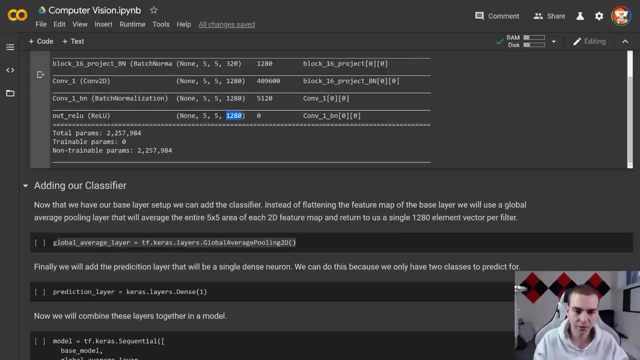 it to classify either cat or either doc, right? So what we're going to do is add a global average layer which essentially is going to take the entire average of every single, so 1280 different layers that are five by five, and put that into a 1d tensor, which. 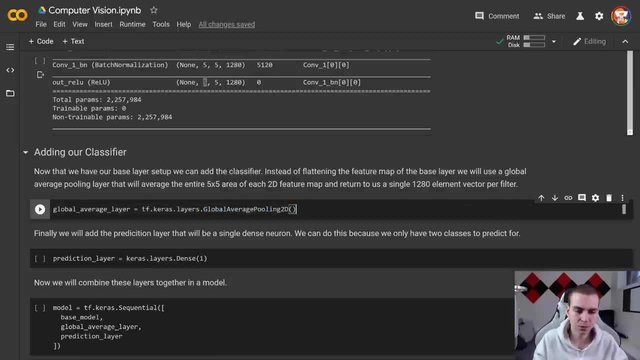 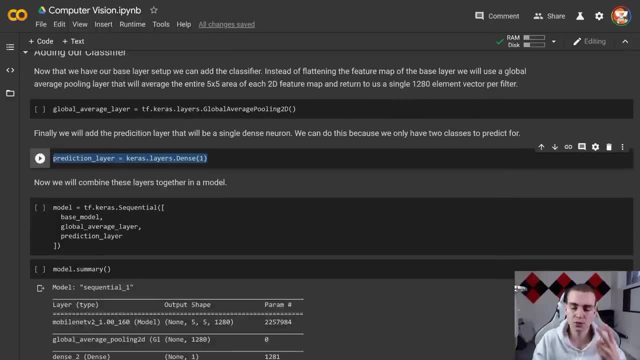 is kind of flattening that for us. So we do that global average pooling And then we're just going to add the prediction layer, which essentially is going to just be one dense node. And since we're only classifying two different classes, right, dogs and cats- 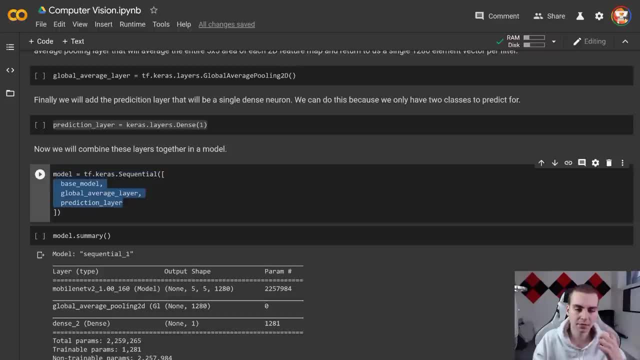 we only need one, then we're going to add all these models together, So the base model and, I guess, layers, the global average layer that we define there, and then the prediction layer to create our final model. So let's do this: global average layer, prediction layer. 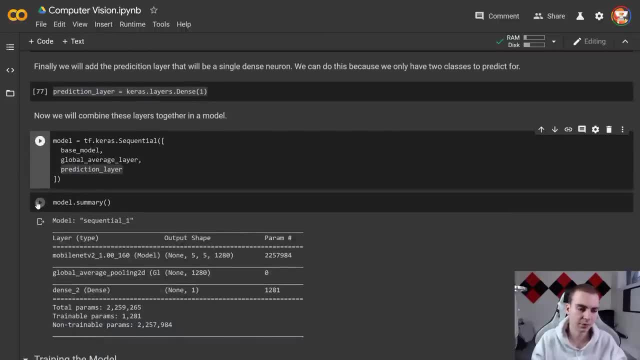 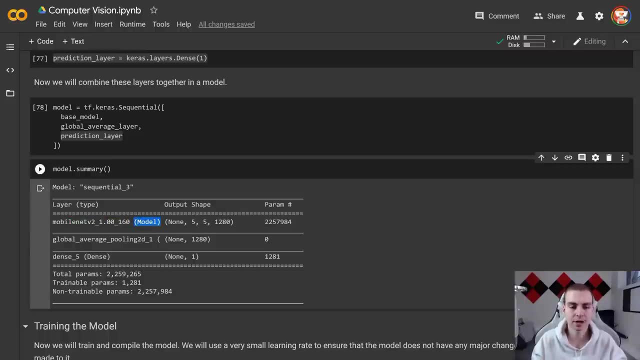 model. give that a second to kind of run there. Now, when we look at the summary, we can see we have mobile average, Mobile net v two, which is actually a model. but that is our base layer And that's fine. 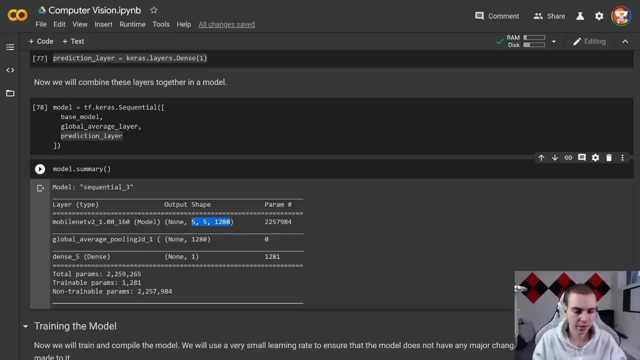 because the output shape is that. then global average pooling, which again just takes this, flans it out, does the average for us, And then finally, our dense layer, which is going to simply have one neuron, which is going to be our output. Now, notice that we have: 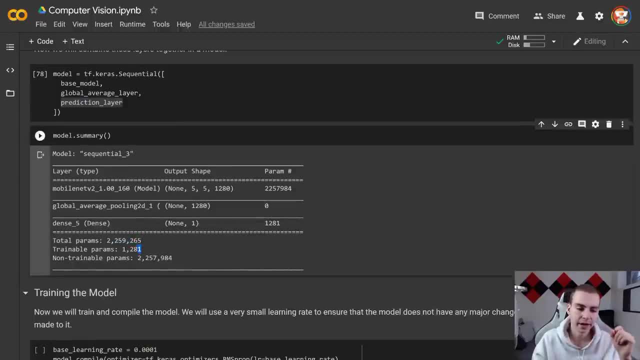 2.259 million parameters in total and only 1281 of them are trainable. That's because we have 1280 connections from this layer to this layer, which means 1280 connections from this layer to this layer, which means 1280 connections from this layer to this layer. 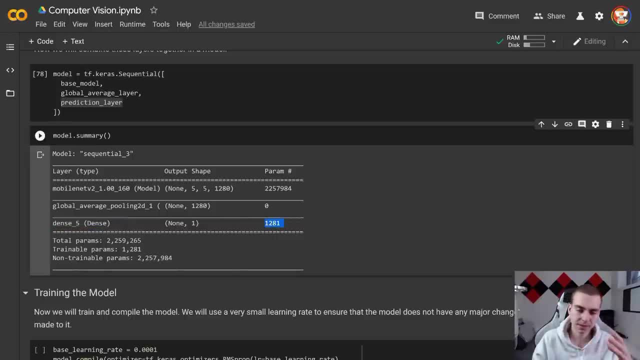 280 weights and one bias. So that is what we're doing. This is what we have created. now, this base, the majority of the network has been done for us, And we just add our own little classifier on top of this. And now we're going to feed some training samples. 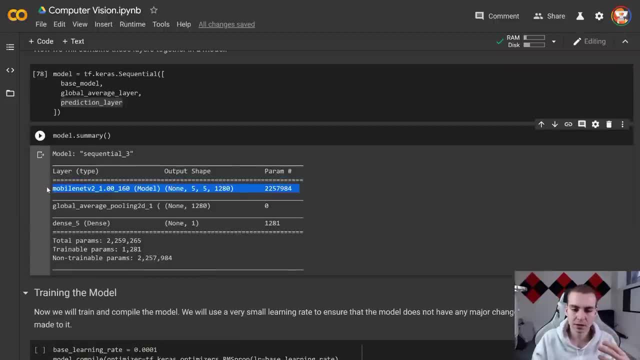 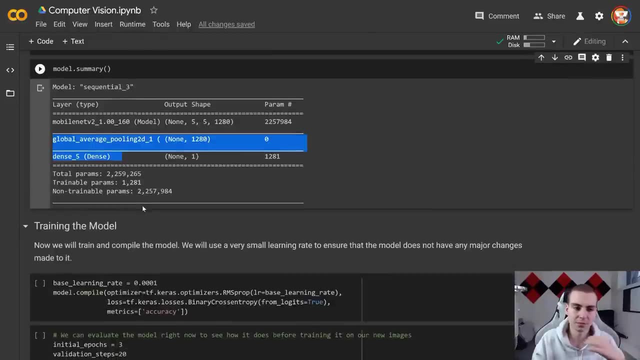 and data to this. Remember, we're not training this base layer whatsoever, So the only thing that needs to be learned is the weights and biases on these two layers here. Once we have that, we should have a decent model ready to go. So let's actually train this Now. 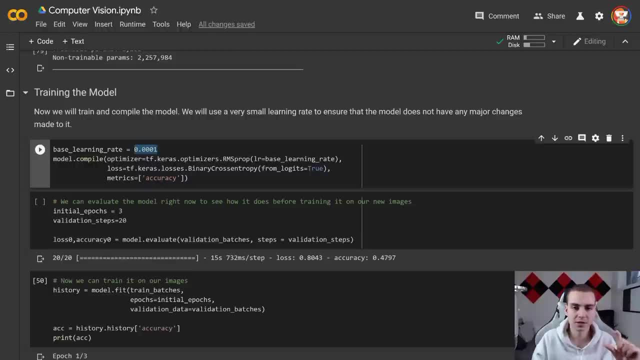 I'm going to compile this here. I'm picking a learning rate. It's very slow. what essentially what the learning rate means is: how much am I allowed to modify the weights and biases of this network, which is what I've done. just made that very. 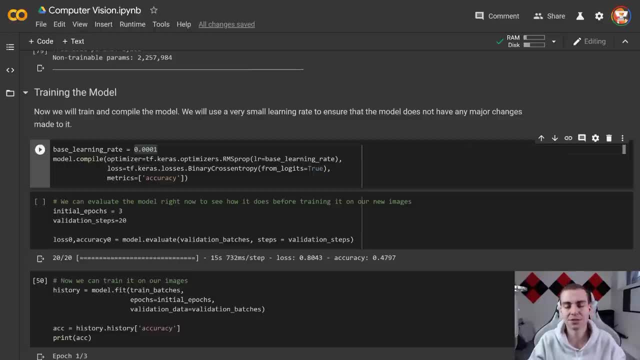 low because we don't want to make any major changes. if we don't have to, because we're already using a base model that exists, right, So we'll set the learning rate. I'm not going to talk about what this does Specifically. you can look that up if you'd like to, And 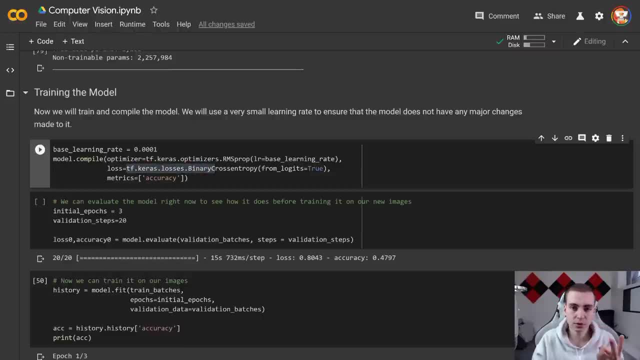 then the loss function. we use binary cross entropy just because we're using two classes. if you're using more than more than two classes, you would just have cross entropy or some other type of cross entropy, And then what we're going to do is actually evaluate the model. 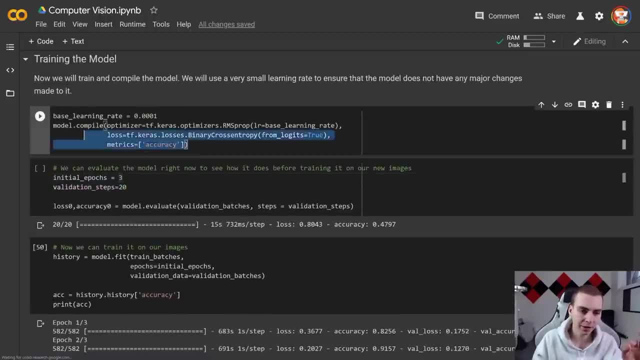 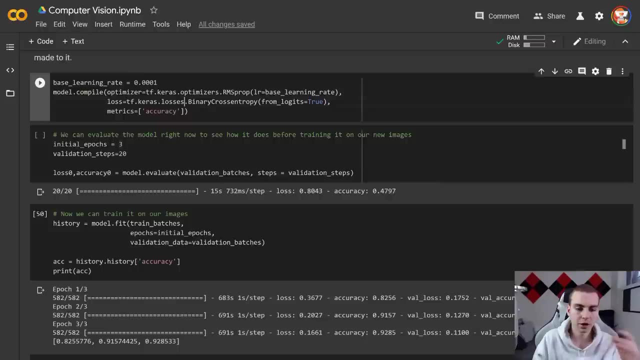 right now, before we even train it. So I've compiled it, I've just set what we'll end up using, but I want to evaluate the model- currently without training it whatsoever- on our validation data or validation batches and see what it actually looks like, what it. 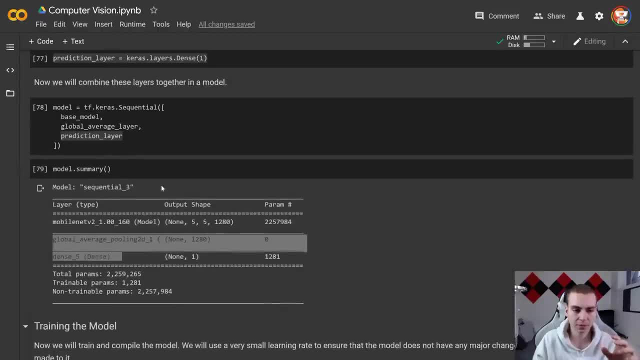 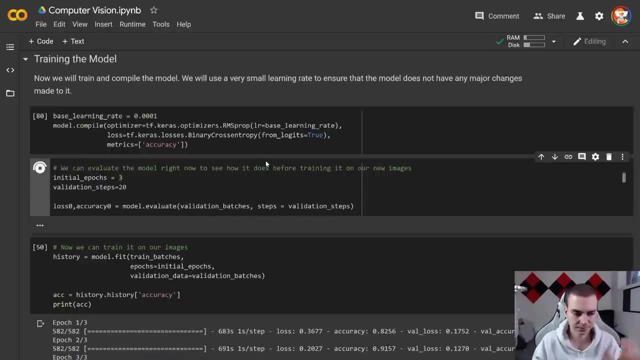 actually, you know what we're getting right now, with the current base model being the way it is and not having changed the weights and biases. they're completely random from the global average pool Cooling in the dense layer. So let's evaluate And let's see what we get as an accuracy. Okay. 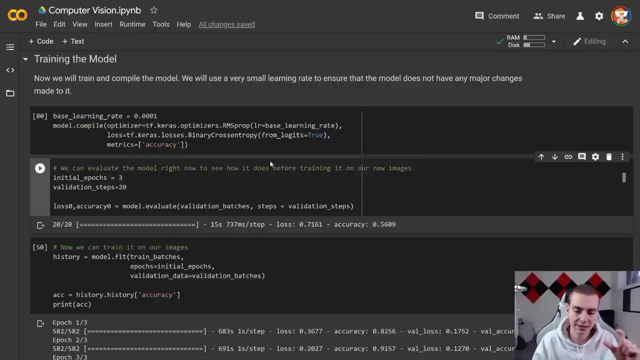 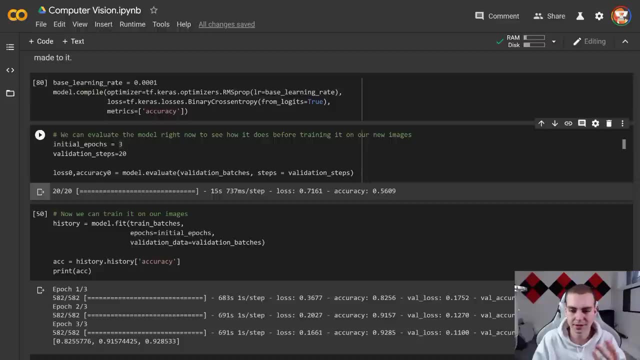 so we can actually see that with the random weights and biases for those last layer that we added, we're getting accuracy of 56%, which pretty much means that it's guessing right. it's, you know, 50% is like two classes. So if we got anything lower than 50, like 50- 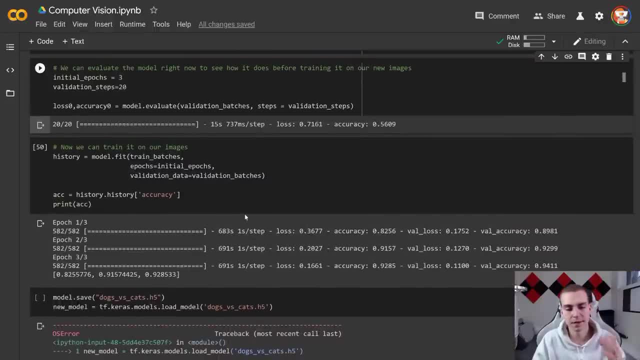 should have been our guests, which is what we're getting. So now, what we're going to do- and I actually I've trained this already, I think, so I might not have to do it again- is a train, this model, on all of our images, so all of our images and cats and cats and dogs that we've loaded. 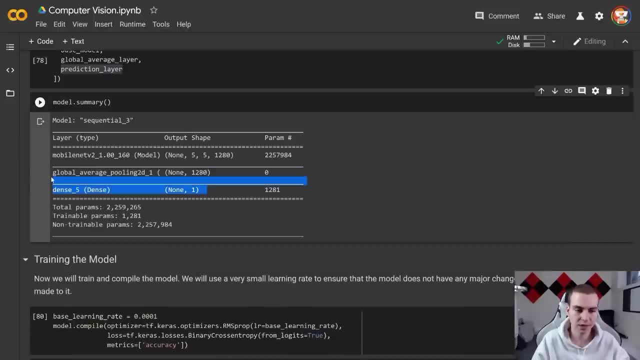 in before, which will allow us now to modify these weights and biases of this layer. So hopefully it can determine what features need to be present for a dog to be a dog and for a cat to be a cat right, And then it can make a pretty good prediction, In fact. 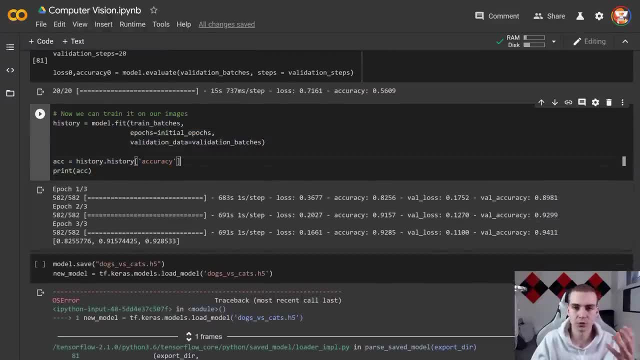 I'm not going to train this in front of us right now, because it actually takes close to an hour to train, just because there is a lot of images that it needs to look at and a lot of calculations that need to happen. But when you do end up training this, you 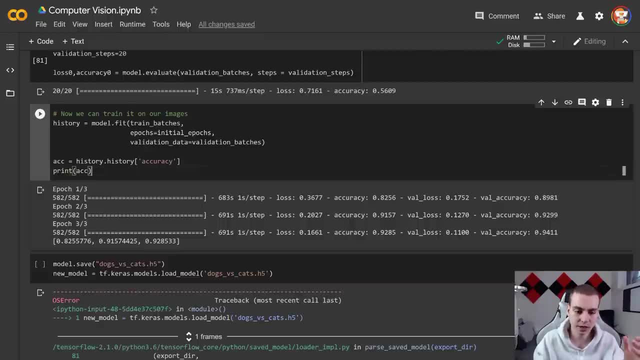 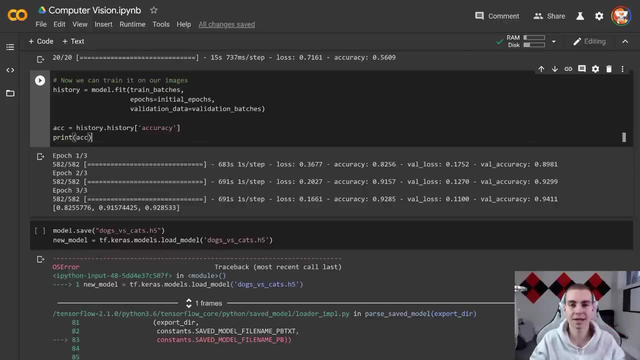 end up getting an accuracy of a close to 92 or 93%, which is pretty good considering the fact that all we did was use an original layer like base layer that classified up to 1000 different images- So very general- and applied that just to cats and dogs by 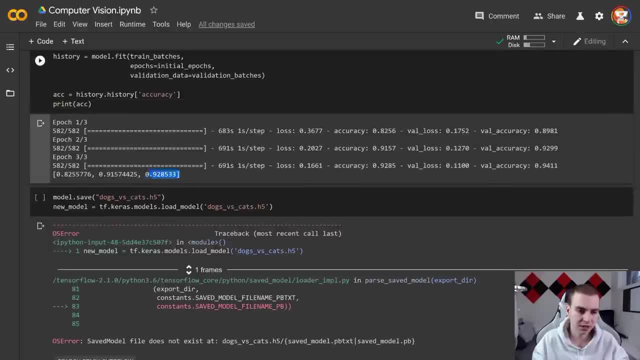 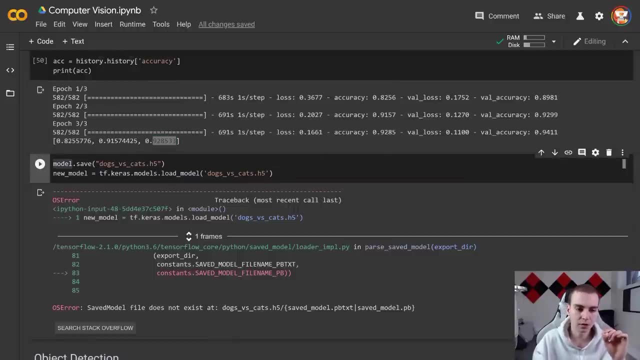 adding our dense layer classifier on top. So you can see this was kind of the accuracy I had from training this previously. I don't want to train again because it takes so long, But I did want to show that you can save a model and load a model by doing this syntax. 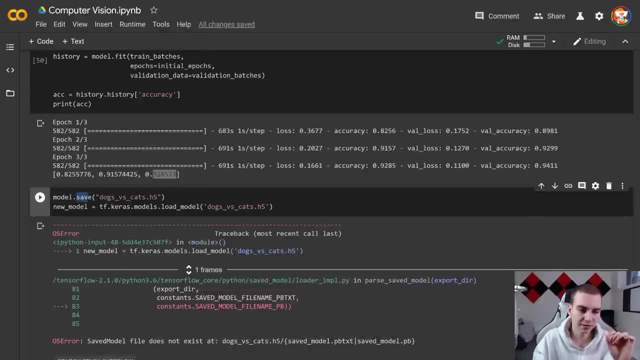 So essentially, on your model object you can call model dot save, save it as whatever name you like, dot h five, which is just a format for saving models and care as specific to care as not TensorFlow, And then you can load the model by doing this. So this is useful. 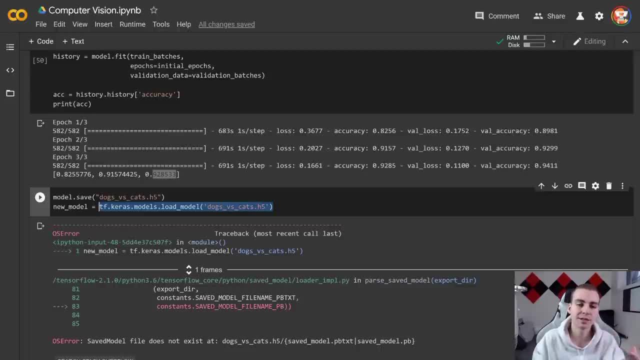 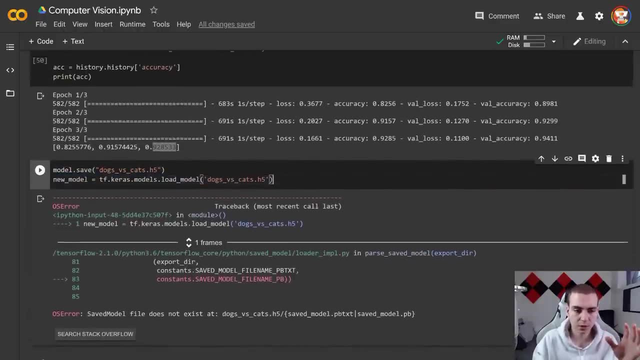 because after you train this for an hour, obviously you don't want to retrain this if you don't have to actually use it to make predictions. So you can just load the model. Now I'm not going to go into using the model specifically. you guys can look up the documentation. 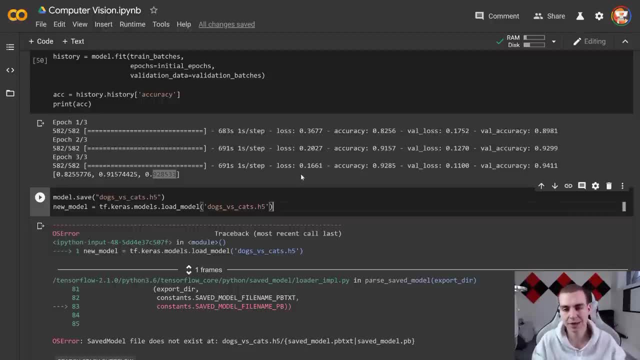 to do that. We're at the point now where I've showed you so much syntax on predicting and how we actually use the models. But the basic idea would be to do model dot predict right, and then you can see that it's even giving me the input. 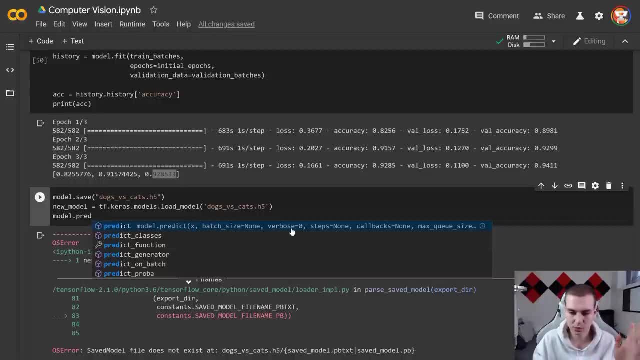 here. So model dot predict. give it some x batch size. we're both right, because it will predict on multiple things And that will spit back to you a class which then you can figure out: okay, this is a cat or this is a dog. you're going to pass this, obviously. 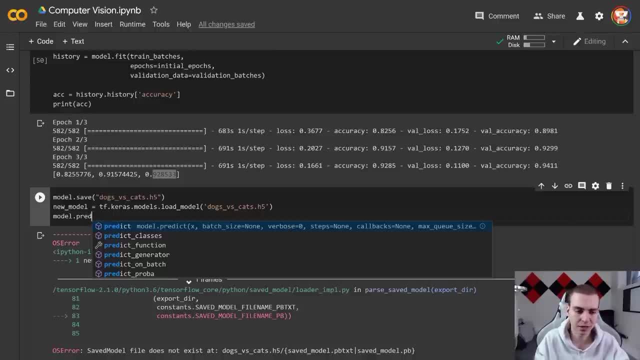 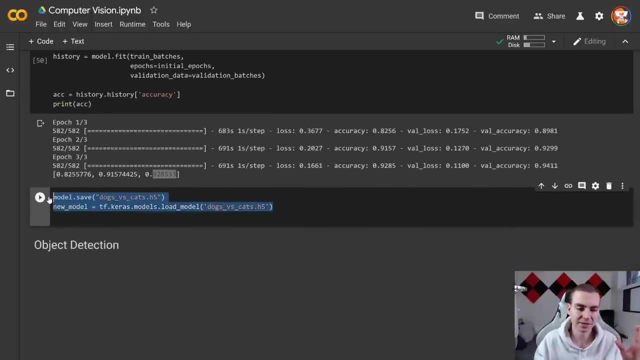 the same input information we have before, which is 160 by 160 by three, and that will make the prediction for you. So that's kind of the thing there. I was getting an OS error just because I hadn't saved this previously, But that's how you save and load models, which I think is important. 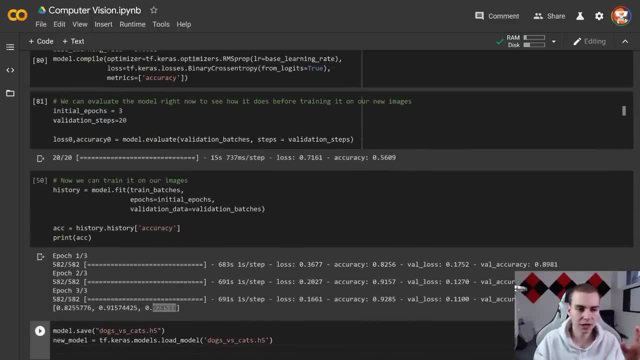 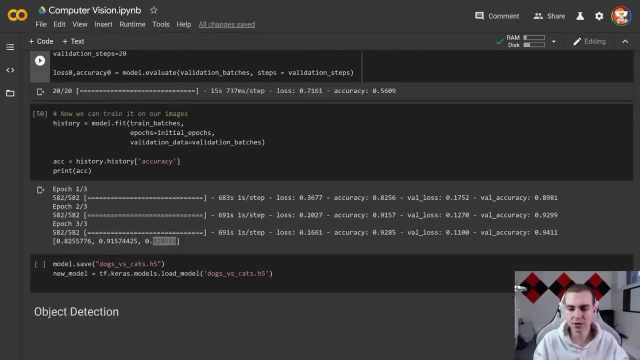 when you're doing very large models. So when you fit this, feel free to change the epochs to be something slower, if you'd like. again, right, this takes a long time to actually end up running, But you can see that the accuracy increases pretty well: exponential, exponentially. 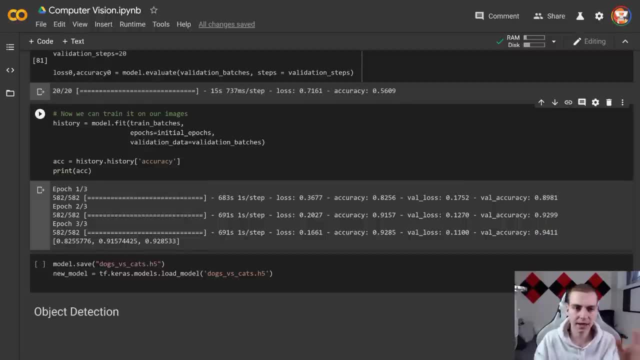 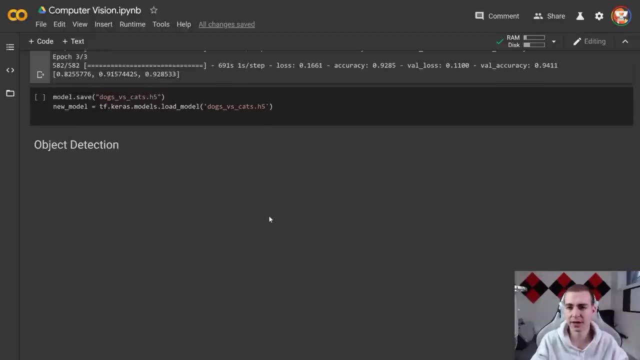 from when we didn't even have that classifier on it. Now, the last thing that I want to talk about is object detection. I'm just going to load up a page. we're not going to do any examples. I'm just going to give you a brief introduction because we're kind of running. 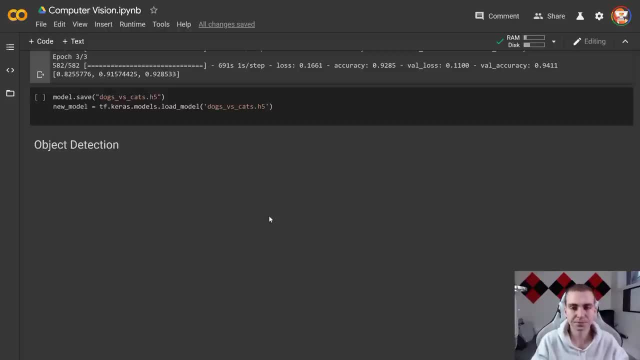 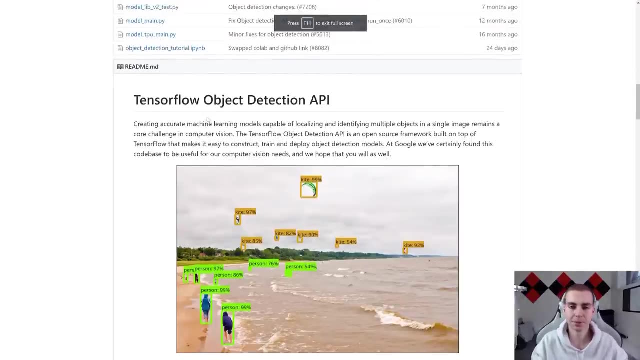 out of time for this module Because you can use TensorFlow to do object detection and recognition, which is kind of cool. So let's get into that now, Okay, so right now I'm on a GitHub page that's built by TensorFlow here. I'm going to leave that link in the notebook where it said: object. 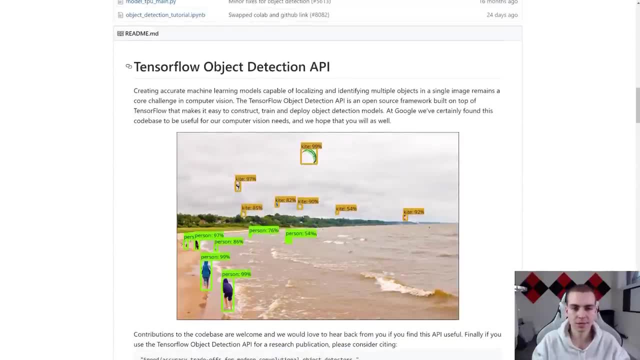 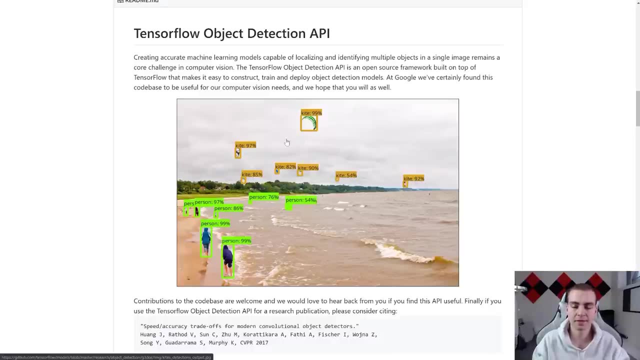 detection. So you guys can look at that. But essentially there is an API for TensorFlow that does object detection for you And in fact it works very well and even gives you confidence scores. So you can see, this is what you'll actually end up getting if you. 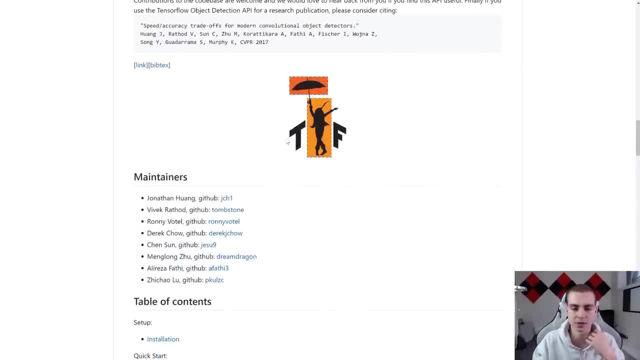 end up using this API Now. unfortunately we don't have time to go through this because this will take a good amount of time to talk about the setup And how to actually use this project properly. But if you go through this documentation, 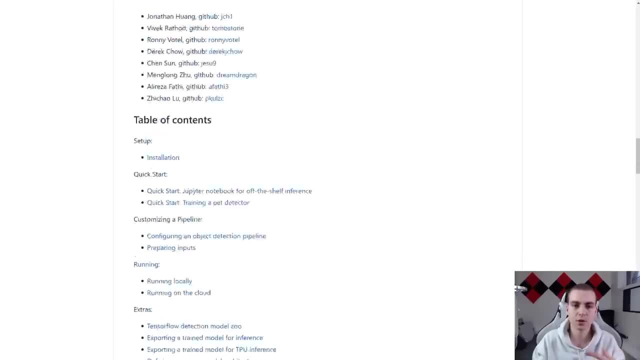 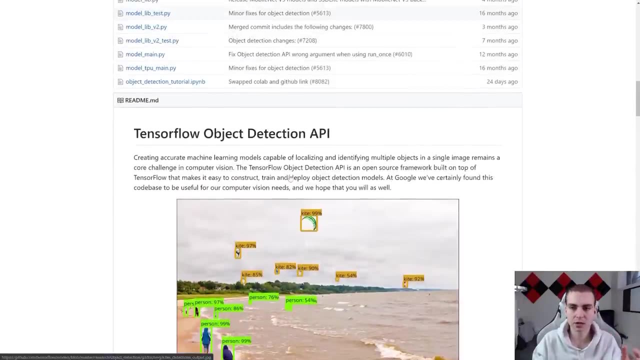 you should be able to figure it out. And now you guys are familiar with TensorFlow And you understand some of the concepts here. This runs a very different model than what we've discussed before. Unfortunately, again, we don't have time to get into it, But just. 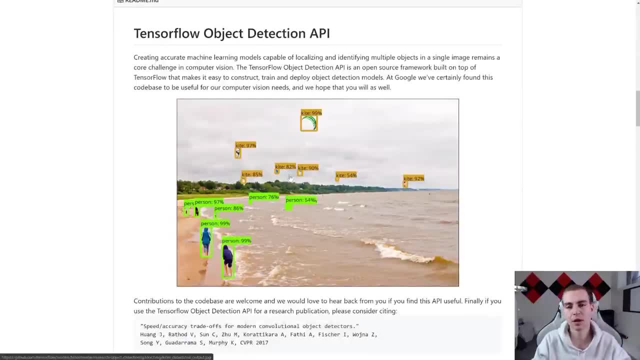 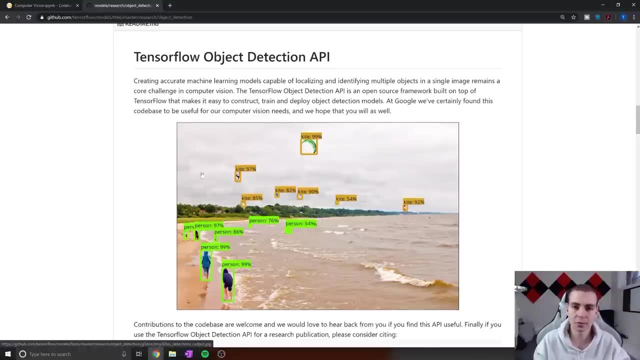 something I wanted to make clear is that you can do something like this with TensorFlow, And I will leave that resource so that if you'd like to check this out, you can use it. There's also a great module in Python called facial recognition. It's not a part. 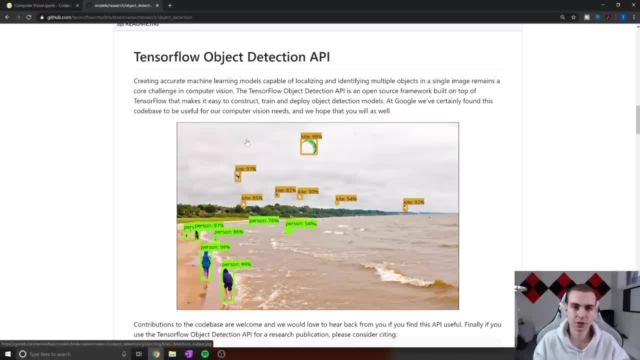 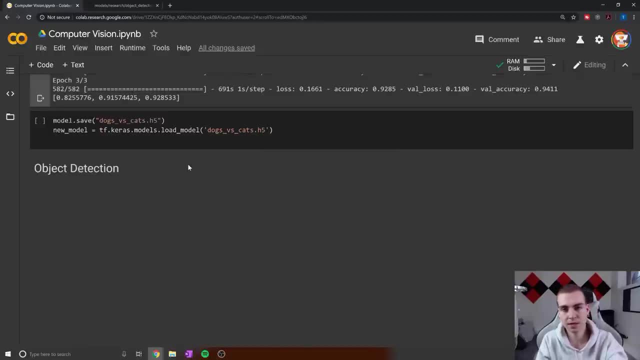 of TensorFlow, But it does use some kind of convolutional neural network to do facial detection and recognition, which is pretty cool as well. So I'll put that link in here. But for that, for now, that's going to be, our was a convolutional neural network kind. 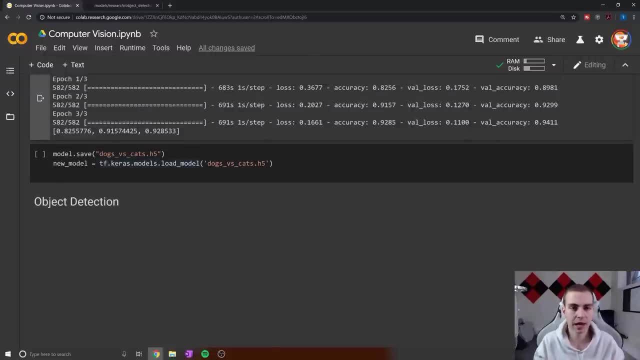 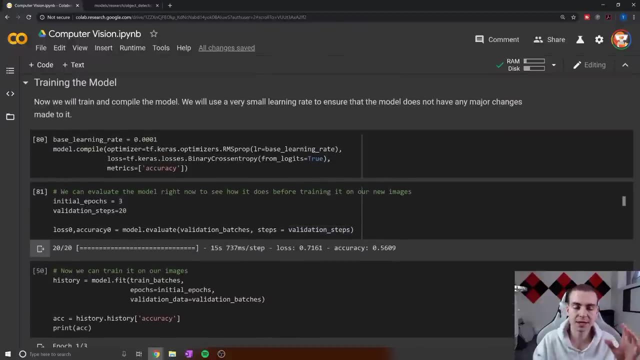 of module. So I hope that says cleared some things up on how deep vision works and how convolutional neural networks work. I know I haven't gone into crazy examples. what I've shown you, some different techniques that hopefully you'll go look up kind of on your own and 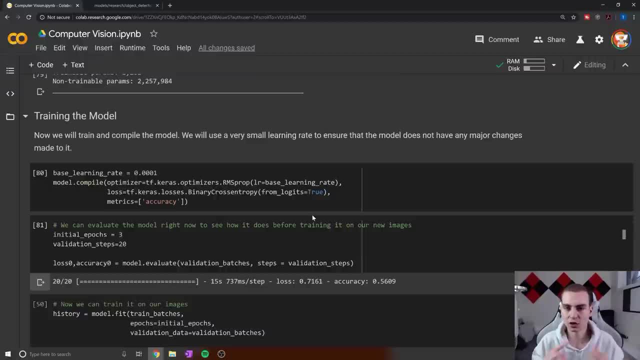 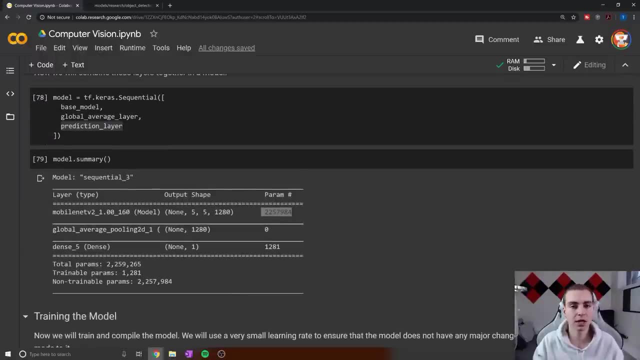 really dive into, because now you have that base kind of domain knowledge where you're going to be able to follow along with the tutorial and understand exactly what you're doing, exactly what to do And, if you want, to create your own model, so long as you can. 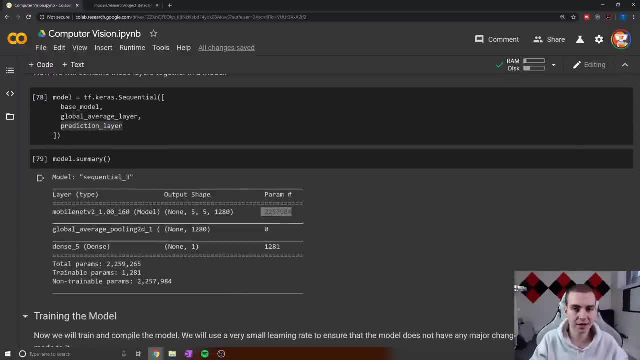 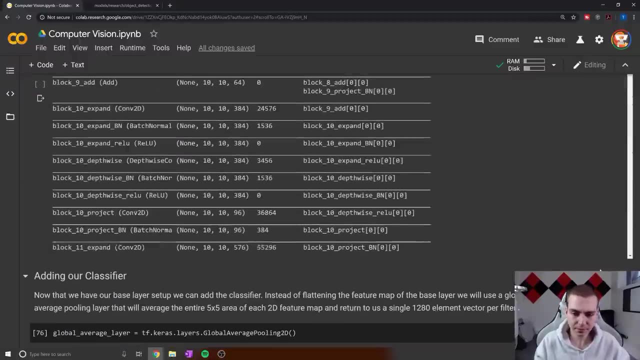 get enough sufficient training data, you can load that training data into your computer, put that in a numpy array. then what you can do is create a model like we've just done, using even something like the mobile nets. what is it? v two that we talked about previously. 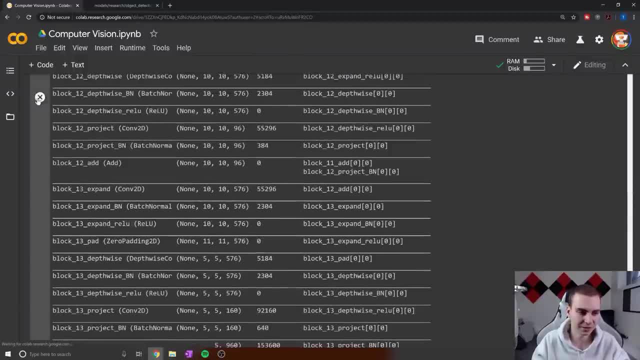 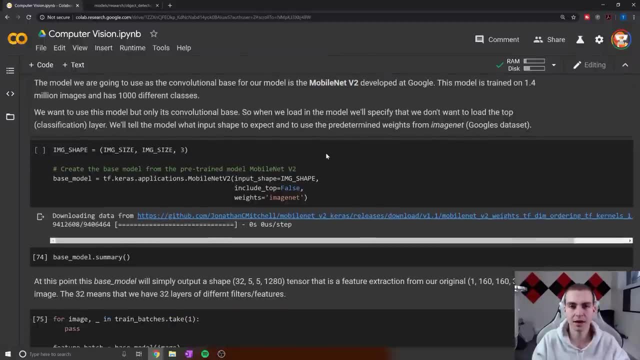 if I could even get up. I need to close this output. Oh my gosh, this is this massive output here. Where is this? We're gonna pre train model. yeah, mobile net v two. you can use the base of that and then add your own classifier on it. 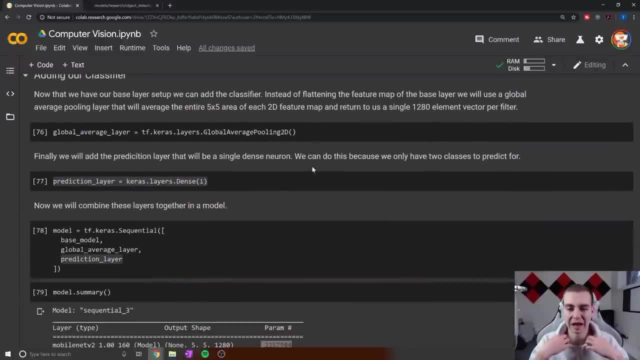 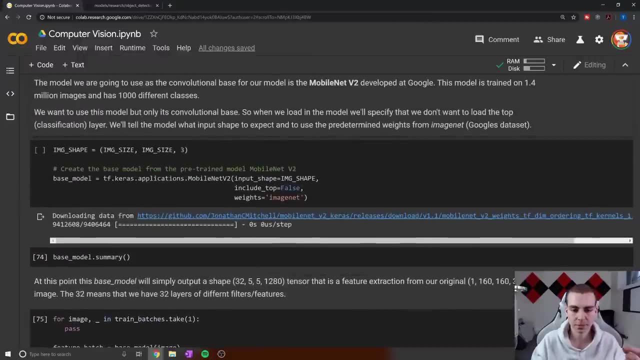 Neuron, do a similar thing to what I've done with that dense neuron and that global average layer, And hopefully you should get a decent result from that. So this is just showing you what you can do. Obviously, you can pick a different base layer depending on what 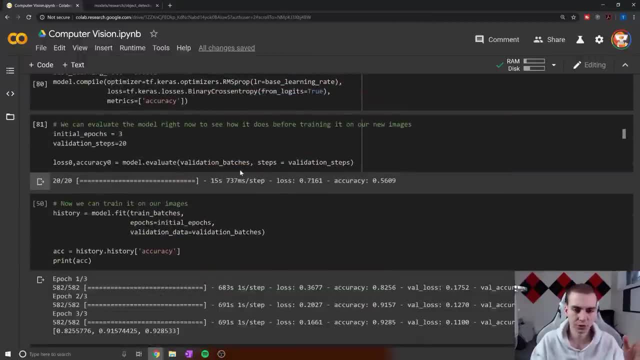 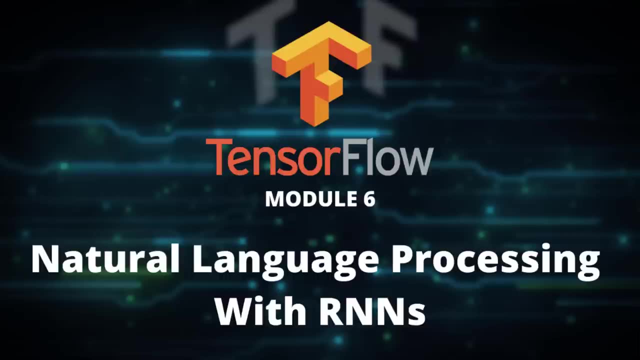 kind of problem you're trying to solve. So, anyways, that has been convolutional neural networks. I hope you enjoyed that module. Now we're on to recurrent neural networks, which is actually gonna be pretty interesting. So I'll see you in that module. Hello everyone. 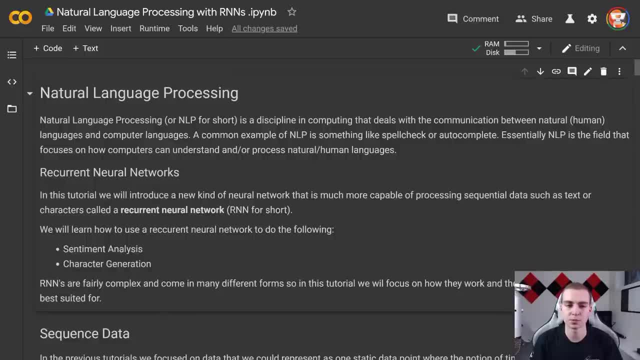 and welcome to the next module in this course, which is covering natural language processing with recurrent neural networks. Now, what we're going to be doing in this module here is, first of all, first off, discussing what natural language processing is, which I guess I'll 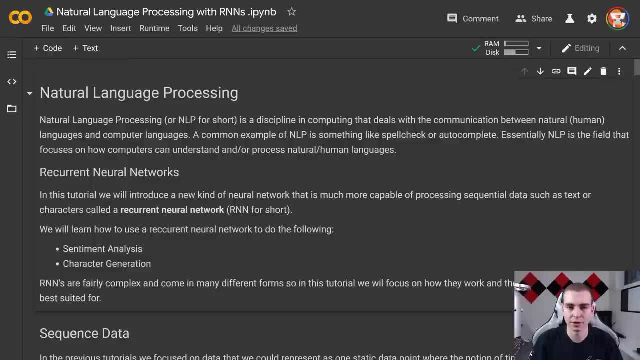 start with here. Essentially, for those of you that don't know, natural language processing, or NLP for short, is the field or discipline in computing or machine learning that deals with trying to understand natural or human languages. Now, the reason we call them natural 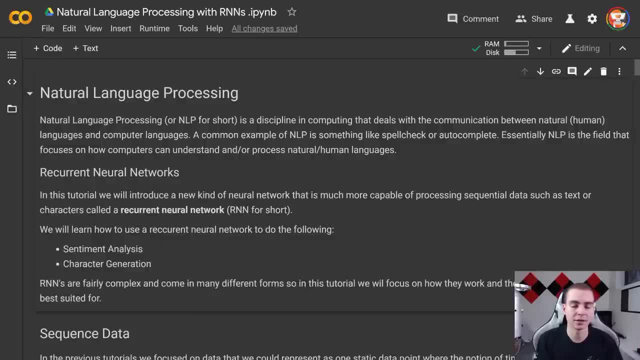 is because these are not computer languages or programming languages per se, and actually computer languages are not computer languages or programming languages per se, And actually computers are quite bad at understanding textual information and human languages, And that's why we've come up with this entire discipline focused on how they can do that. 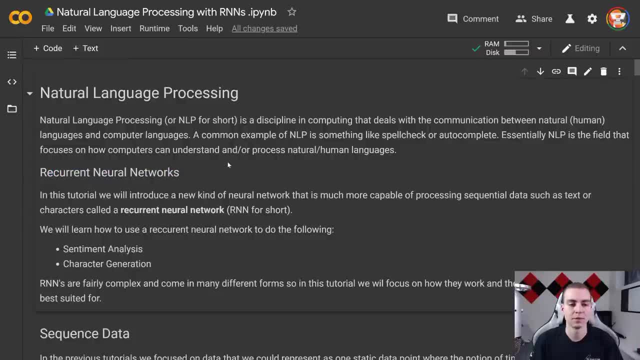 So we're going to do that using something called recurrent neural networks, But some examples of natural language processing would be something like spellcheck, auto complete voice assistance, translation between languages. there's all different kinds of things, chatbots, but essentially anything that deals with textual data. So you like paragraphs, sentences and 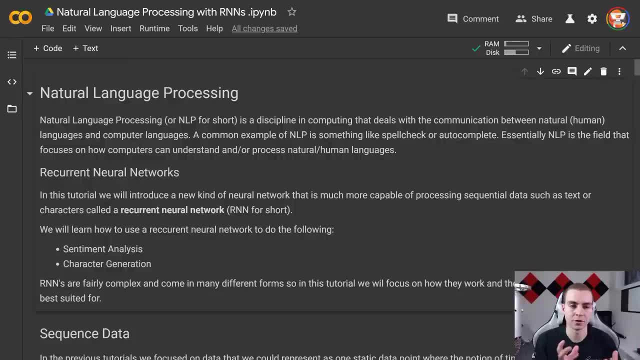 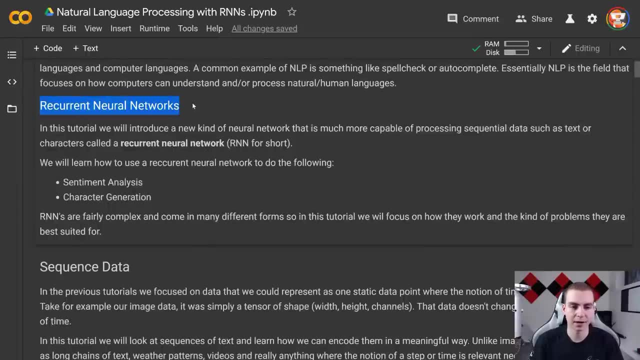 sentences, even words. that is probably going to be classified under natural language processing in terms of doing some kind of machine learning stuff with it. Now we are going to be talking about a different kind of neural network in this series called recurrent neural networks. 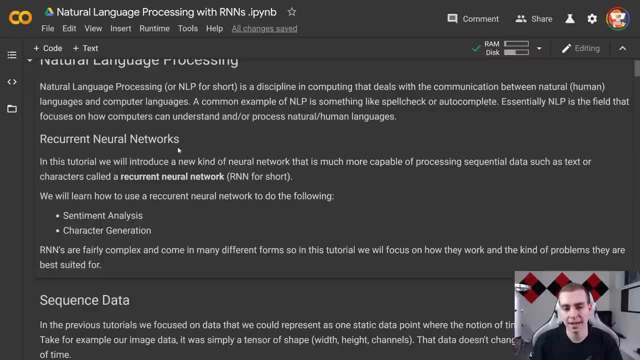 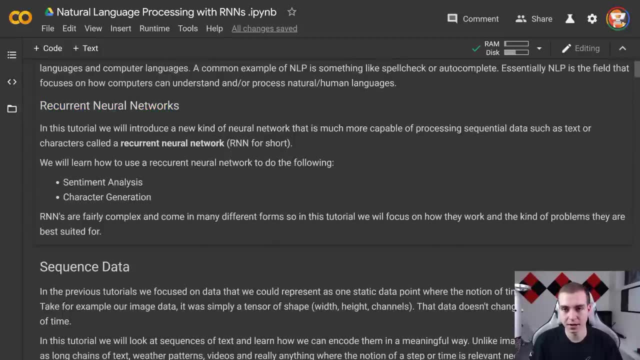 Now, these are very good at classifying and understanding textual data And that's why we'll be using them, But they are fairly complex And there's a lot of stuff that goes into them. Now, in the interest of time and just not knowing a lot of your math background, 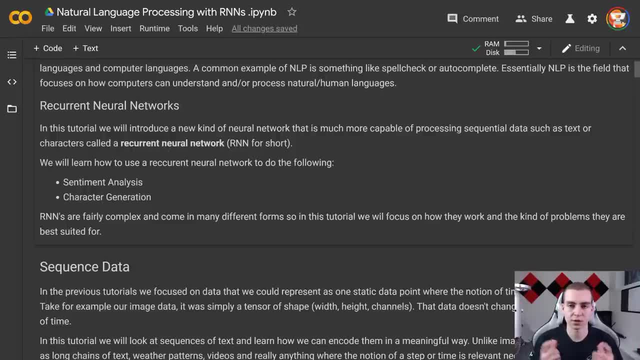 I'm not going to be getting into the exact details of how this works on a lower level, like I did when I explained kind of our, I guess, fundamental learning algorithms which are a bit easier to grasp and even just regular neural networks in general. we're going to be kind of skipping over that and really focusing 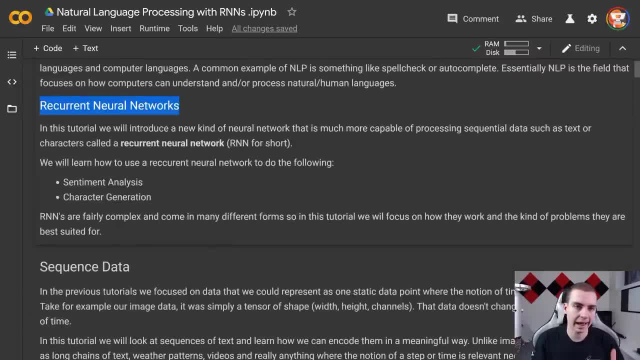 on why this works the way it does, rather than how and when you should use this, And then maybe understanding a few of the different kinds of layers that have to do with recurrent neural networks. But again, we're not going to get into the math. if you'd like to learn, 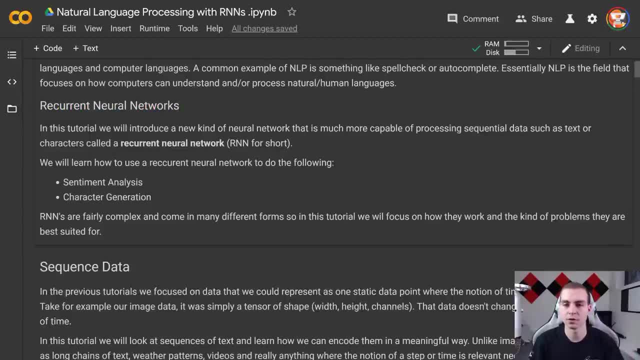 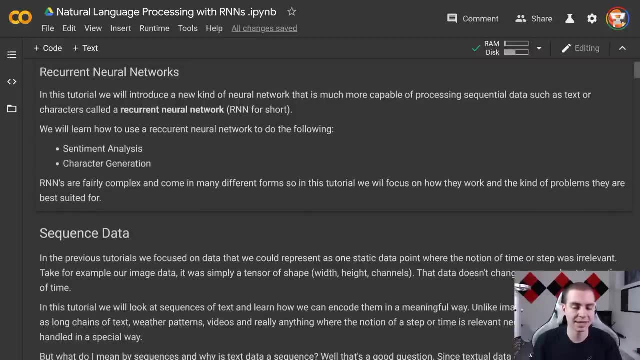 about that. there will be some sources at the bottom of the guide And you can also just look up recurrent neural networks and you'll find lots of resources that explain all of the fancy math that goes on behind them. Now the exact applications and kind. 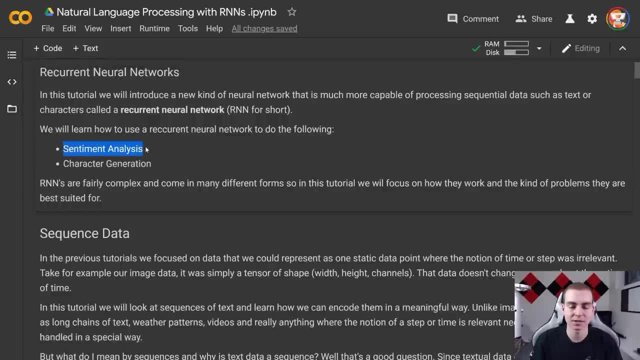 of things we'll be working towards here is sentiment analysis. that's the first kind of task or thing we're going to do. we're actually going to use movie reviews and try to determine whether these movie reviews are positive or negative by performing sentiment analysis on them. Now, if you're unfamiliar with sentiment analysis, we'll talk about. 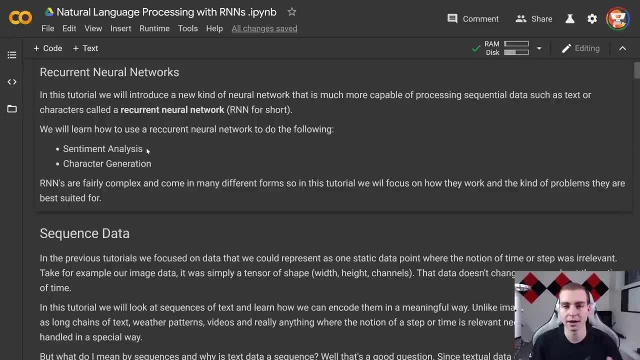 it more later- But essentially means trying to determine how positive or negative the sentence or piece of text is which you can see why that'd be useful for movie reviews. Next, we're going to do character slash, text generation. So essentially we're going to 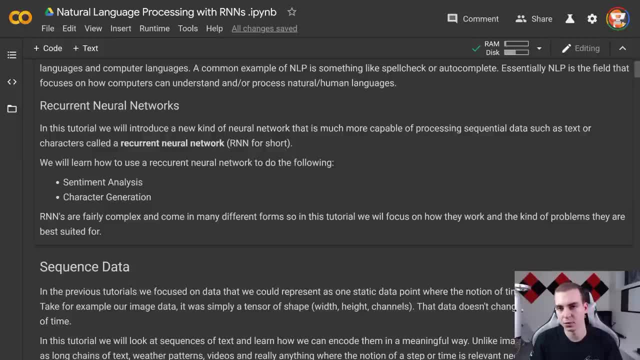 use a natural language processing model, I guess, if you want to call it that, to generate the next character in a sequence of text for us, And we're going to use that model a bunch of times- to actually generate an entire play. Now, I know this seems a little bit ridiculous. 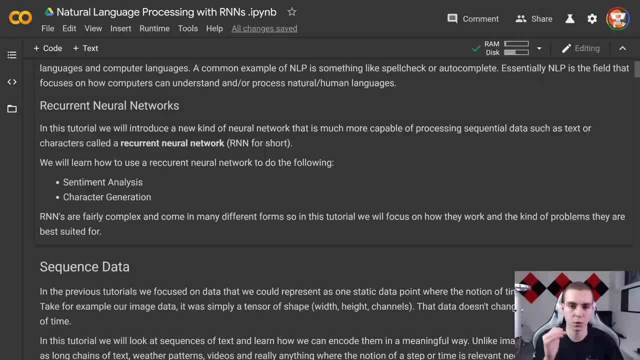 compared to some of the trivial examples we've done before. this will be quite a bit more code than anything We've really looked at yet, But this is very cool because we're going to actually going to train a model to learn how to write a play. that's literally what it's going to do. it's 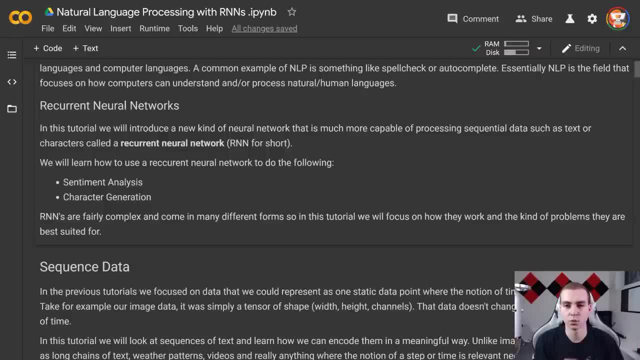 going to read through a play- I believe it's roomy, Romeo and Juliet- And then we're going to give it a little prompt when we're actually using the model, and say, Okay, this is the first part of the play, right the rest of it. and then it will actually go and write. 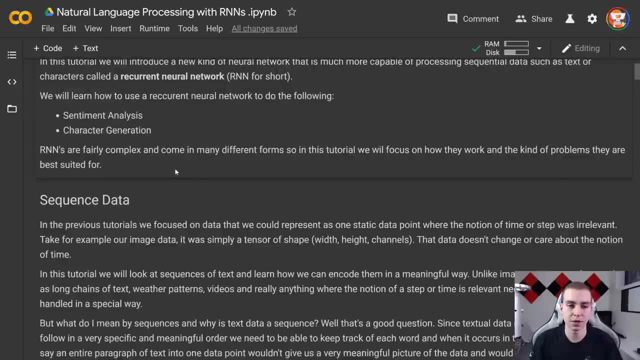 the rest of the characters in the play, And we'll see that we can get something that's pretty good using the techniques that we'll talk about. So the first thing that I want to do is talk about data, So I'm going to hop onto my 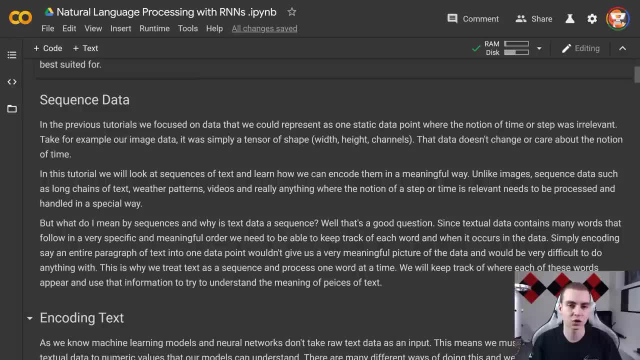 drawing tablet here And we're going to compare the difference between textual data and numeric data, like we've seen before, and why we're going to have to employ some pretty complex and different steps to turn something like this- you know, a block of text- into some. 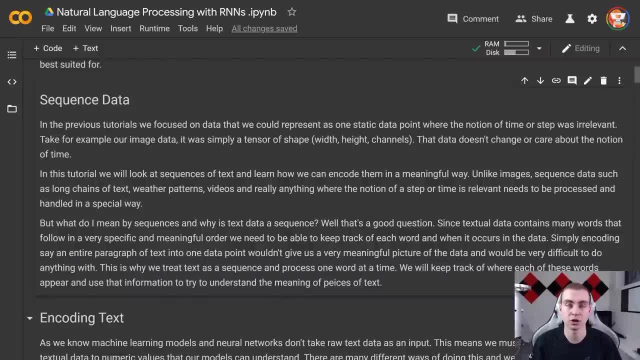 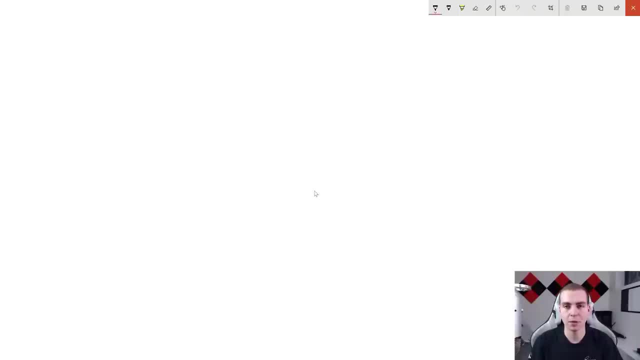 meaningful information that our neural networks actually going to be an actually going to be able to understand and process. So let's go ahead and get over to that, Okay, so now we're going to get into the problem of how we can turn some textual data into numeric. 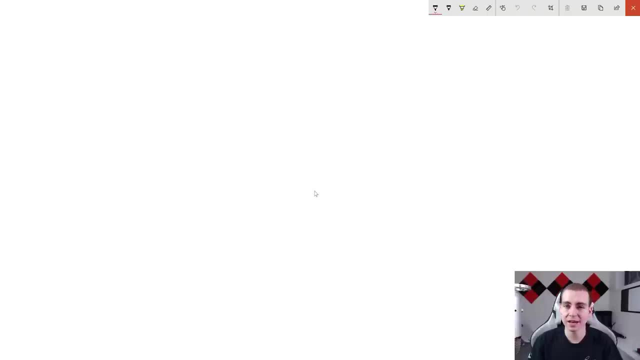 data that we can feed to our neural network. Now this is a pretty interesting problem And we'll kind of go through as we start going through it. you should see why this is interesting and why there's a lot of difficulties with the different methods that we pick. But the first method that I want to talk about is 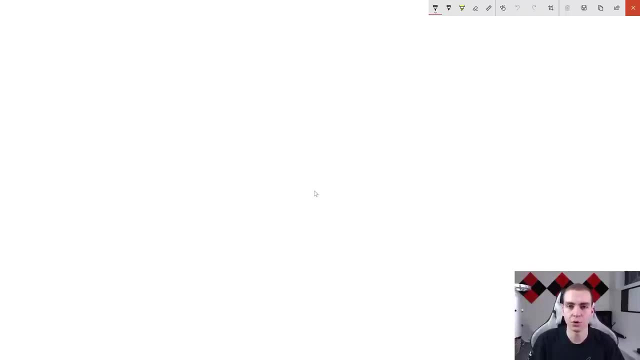 something called bag of words, in terms of how we can kind of encode and pre process text into integers. Now, obviously I'm not the first person to come up with this. bag of words is a very famous- almost I want to say- algorithm or method of converting textual. 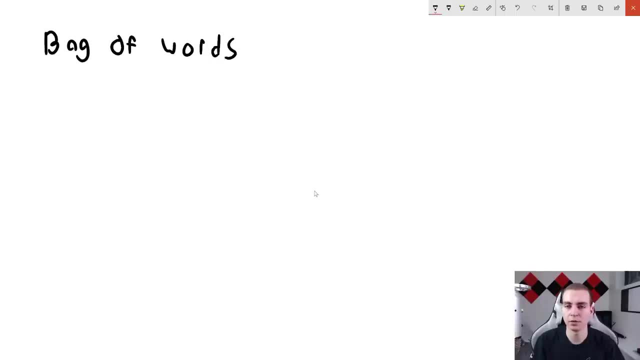 data to numeric data, although it is pretty flawed and it only really works for, say, very simple tasks, And we're going to understand why in a second. So we're going to call this bag of words. Essentially, what bag of words says is what we're going to do, is we're going 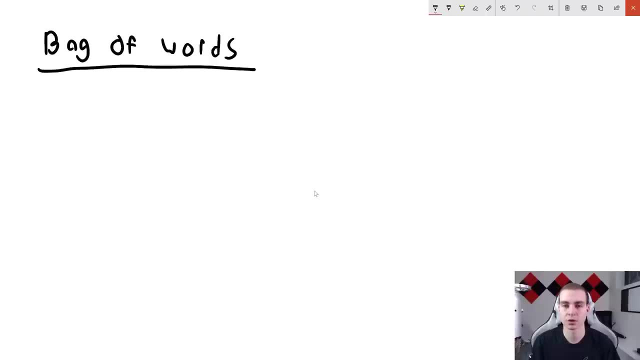 to look at our entire training data set. right, because we're going to be turning our training data set into a form the network can understand And we're going to create a dictionary lookup of the vocabulary. Now, what I mean by that is we're going to say that every single unique 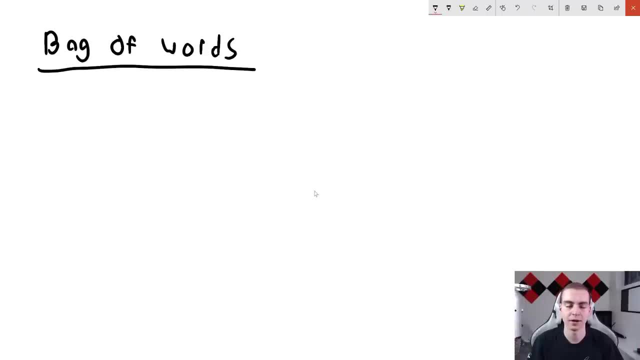 word in our data set is the vocabulary right. That's the amount of words that the model is expected to understand, Because we're, you know, going to show all those words to the model And we're going to say that every single one of these words, so every single one of these words in the 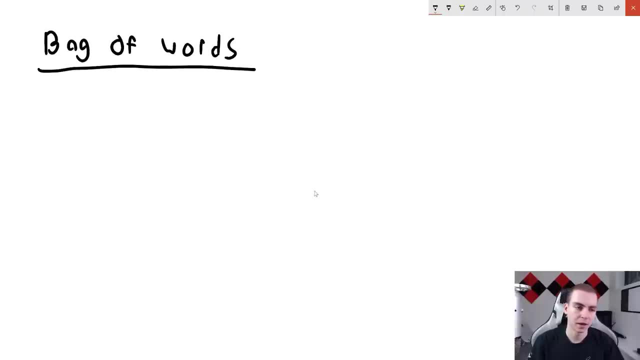 vocabulary is going to be placed in a dictionary And beside that we're going to have some integer that represents it. So, for example, maybe the vocabulary of our data set is the words: you know: I a, maybe, Tim, maybe, day me right. we're gonna have a bunch of arbitrary. 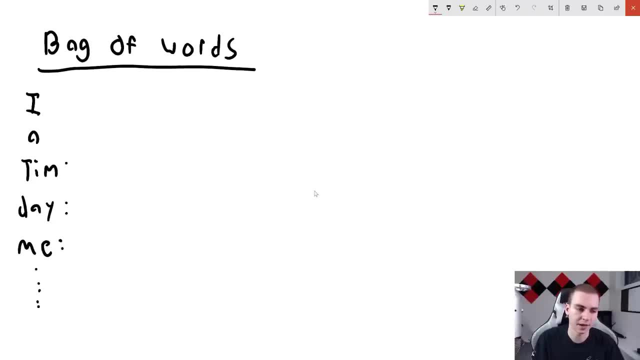 words. I'll just put dot dot dot to show that this kind of goes to the length of the vocabulary And every single one of these words will be placed in a dictionary which we're just going to call, kind of our lookup table or word index table, And we're going to have a number that 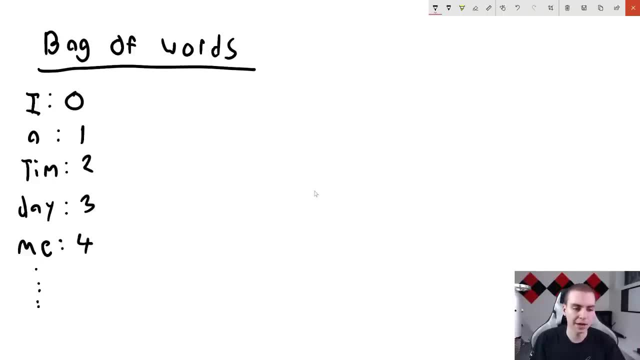 represents every single one of them. So you can imagine that in very large data sets, we're going to have, you know, 10s of 1000s, of 100s of 1000s, sometimes even maybe millions of different words, and they're all going to be encoded by different integers. Now 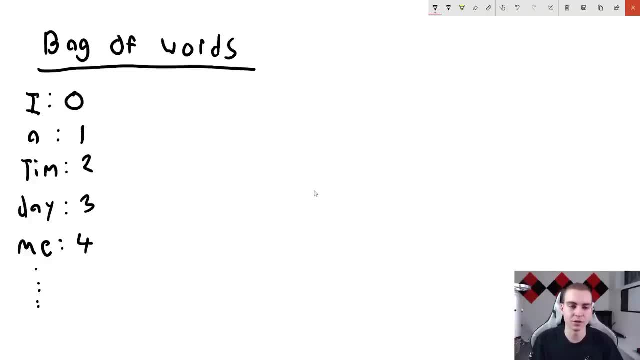 the reason we call this bag of words is because what we're actually going to do when we look at a sentence is we're only going to keep track of the words that are present and the frequency of those words, And, in fact, what we'll do well is we'll create what we call a bag And whenever we see a word appears, 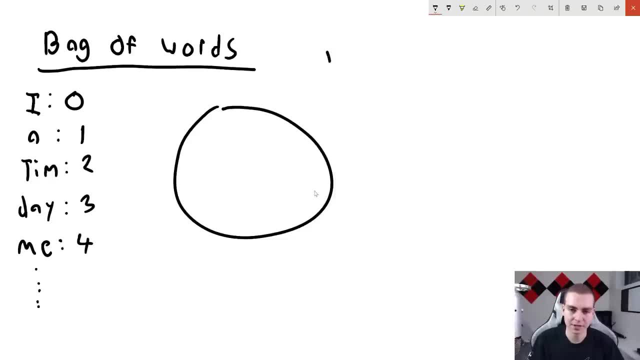 we'll simply add its number into the bag. So if I have a sentence- like you know, I am Tim day day- I'm just going to do like a random sentence, like that- then what we're going to do is, every time we see a word, we're going to take its number and throw it into. 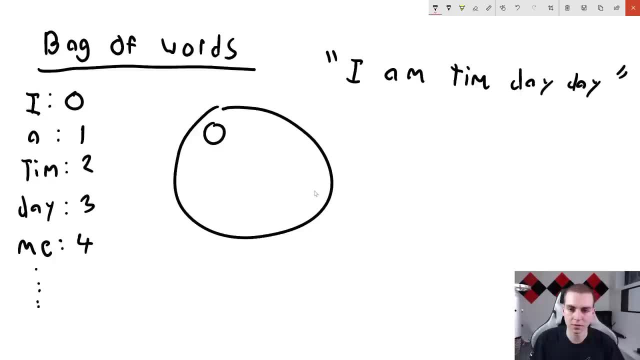 the bag. So we're going to say, Alright, I, that's zero, and that's one, Tim, that's two, day, that's three, that's three again, and notice that what's happening here is we're losing. 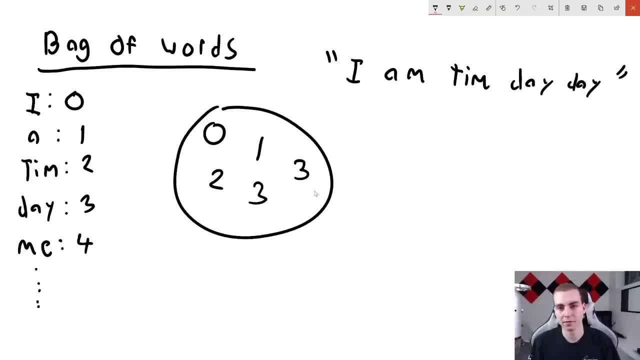 the ordering of these words, But we're just keeping track of the frequency. Now there's lots of different ways to kind of format how we want to do bag of words, But this is the basic idea. I'm not going to go too far in because we're not actually really going to. 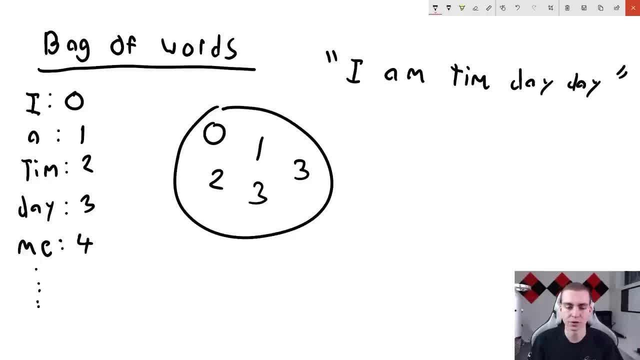 use this technique, But essentially you lose the ordering in which words appear and you just keep track of the frequency and what words appear. So this can be very useful. when you're looking, you know you're doing very simple tasks where the presence of a certain 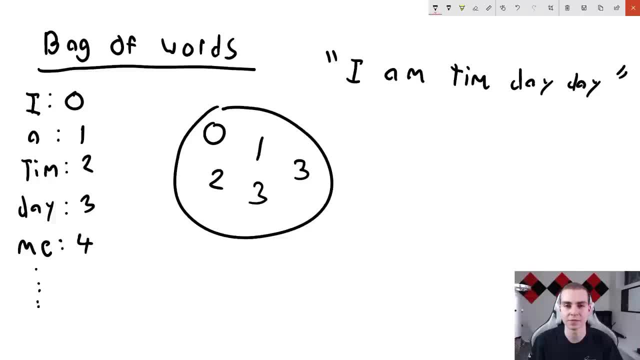 word will really influence the kind of type of sentence that it is or the meaning that you're going to get from it. But when we're looking at more complex input where, you know, different words have different meanings depending on where they are in a sentence, this is a. 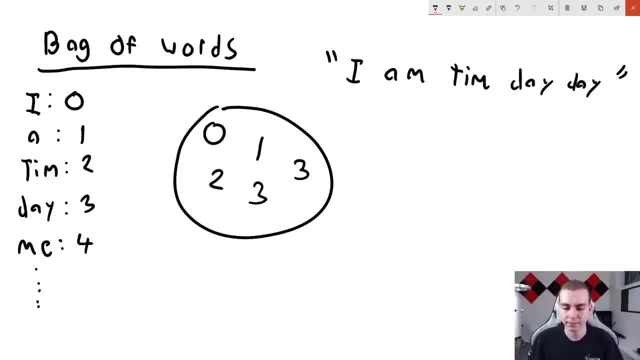 pretty flawed way to encode this data. Now, I won't go much further into this. this is not the exact way the bag of words works, But I just wanted to show you kind of an idea here, which is we just encode every single unique word by an integer And then we don't even really 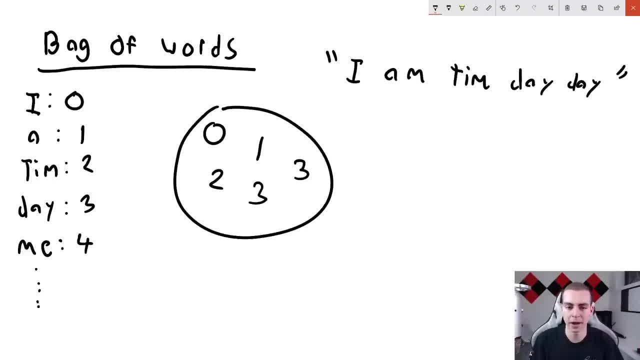 care about where these words are. we just throw them into a bag And we say, Alright, you know, this is our bag, right here, that I'm doing the arrow to. we'll just throw in three as many times as you know the word day appears. we'll throw in one as many times. 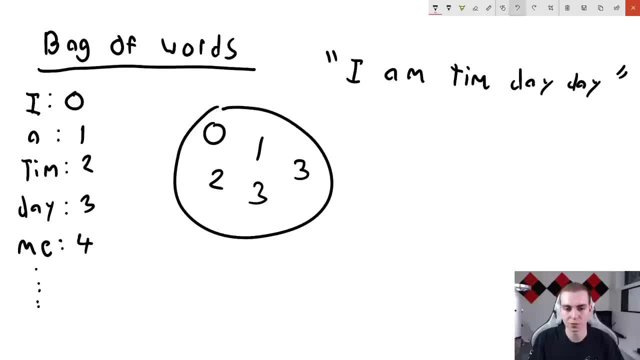 as the word I guess am appears, and so on and so forth. And then what will happen is we'll feed this bag to our neural network in some form, depending on the network that we're using, And it will just look at and say, Okay, so I have all these different numbers. that means these: 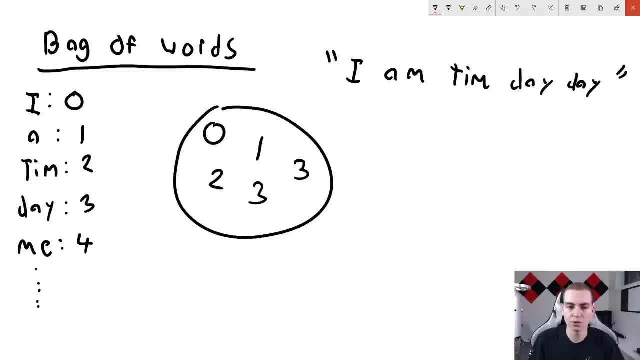 words are present and try to do something with it. Now I'm going to show you a few examples of where this kind of breaks down, But just understand that this is how this works. This is the first technique, called bag of words, which, again, we will not be using. So what? 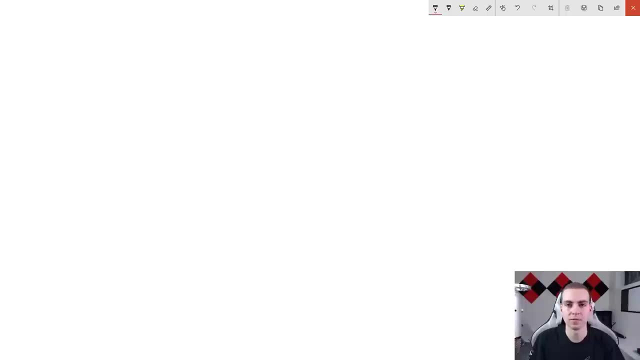 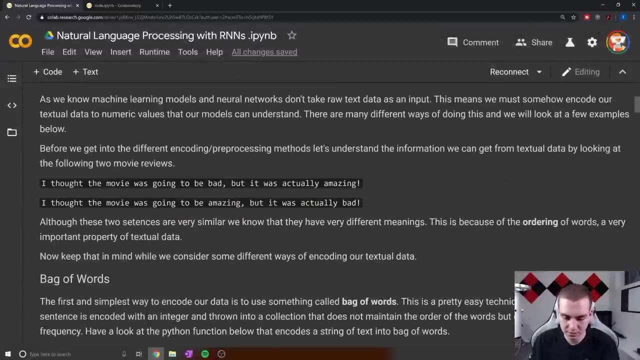 happens when we have a sentence where the same word conveys a very different meaning. right, And I'm actually- I think I have an example on the slides here that I'll go into- Yes, so like this. Okay, so for our bag of words technique, which we can kind of see here and maybe we'll go, 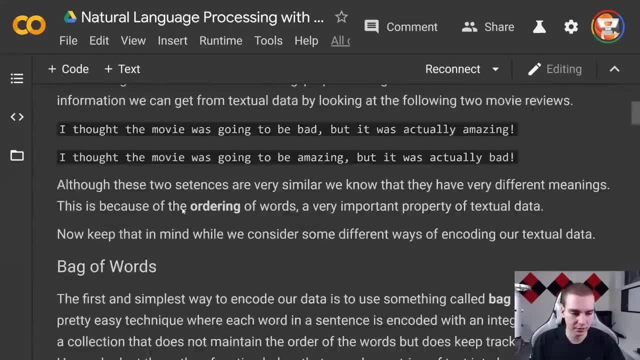 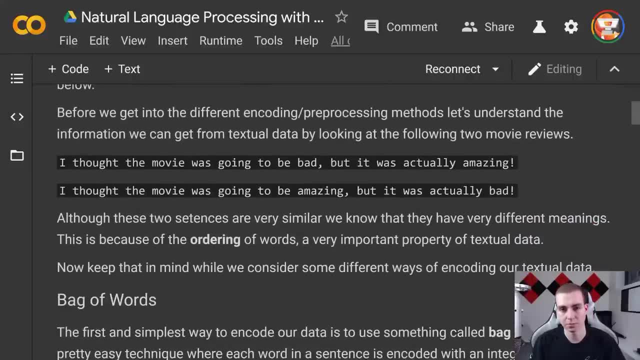 through it. Let's consider the two sentences. Where are they here? I thought the movie was going to be bad, but it was actually amazing. And I thought the movie was going to be amazing, but it was actually bad, Right? So consider these two sentences Now. I know you guys already. 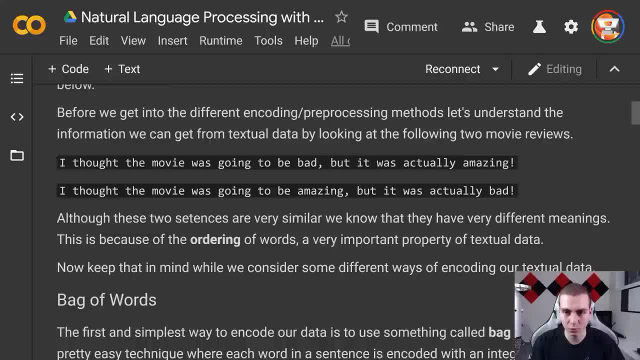 know what I'm going to get at, But essentially, these sentences use the exact same words. In fact, they use the exact same number of words, the exact same words in total, And well, they have a very different meaning. Meaning, with our bag of words technique, we're actually going to encode these two sentences. 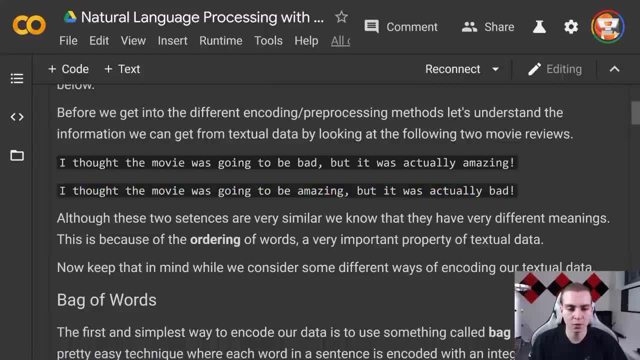 using the exact same representation Because, remember, all we do is we care about the frequency and what words appear, but we don't care about where they appear. So we end up losing that meaning from the sentence. because the sentence. I thought the movie was going to be bad, but 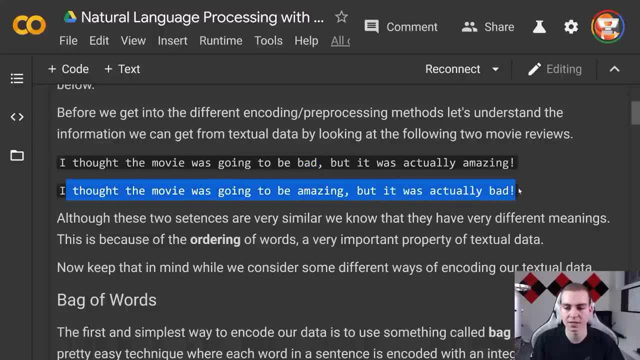 it was actually amazing- is encoded and represented by the same thing as this sentences, So that you know, obviously is an issue, That's a flaw And that's one of the reasons why bag of words is not very good to use, Because we lose the context of the words within the 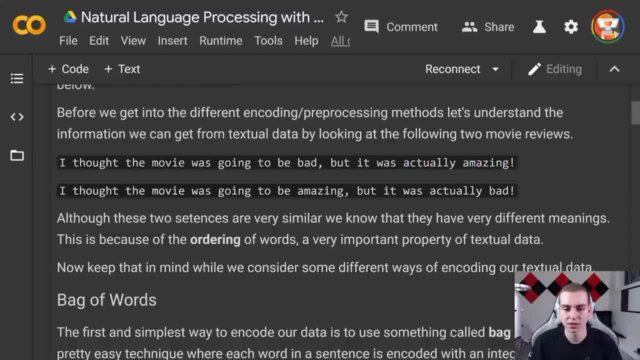 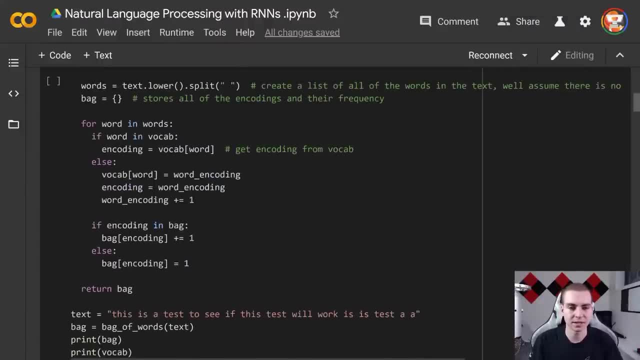 sentence. we just pick up the frequency and the fact that these words exist. So that's the first technique. that's called bag of words. I've actually written a little function here that does this for us. This is not really the exact way that we would write a bag of. 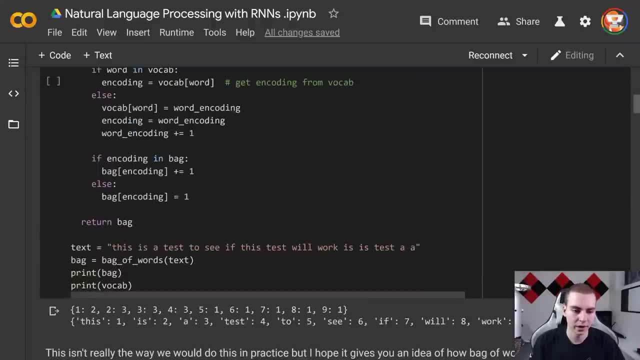 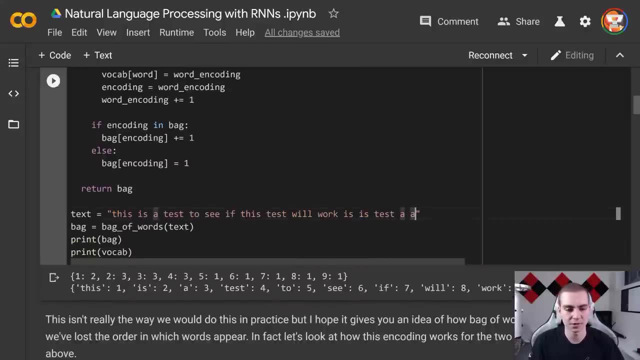 words function. But you kind of get the idea that when I have a text, this is a test to see if this test will work, is test a. I just did a bunch of random stuff So we can see what I'm doing is printing out. 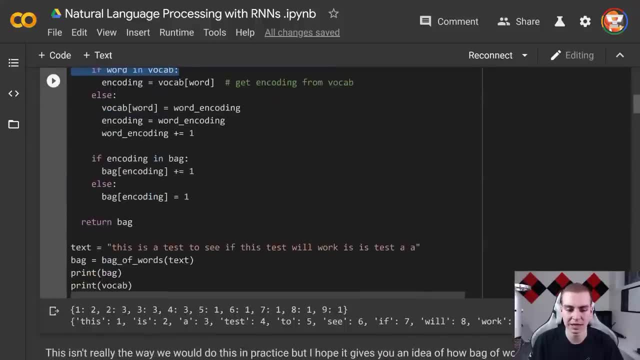 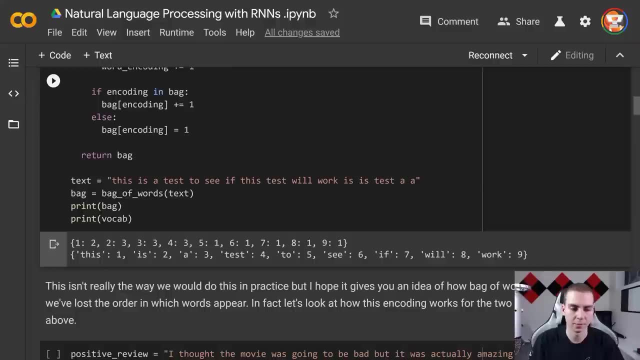 the bag which I get from this function And you guys can look at this if you kind of want to see how this works. And essentially what it tells us is: the word one appears two times, Yes, the word two appears three times. the word three appears three times word four. 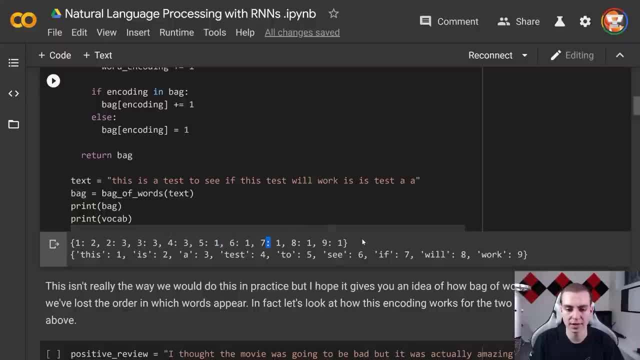 appears three times 51617 once, so on. That's the information we get from our bag, right from that encoding. And then if we look up here, this is our vocabulary. So this stands for one is is, two is three, so on, And you can kind of get the idea from that, So that 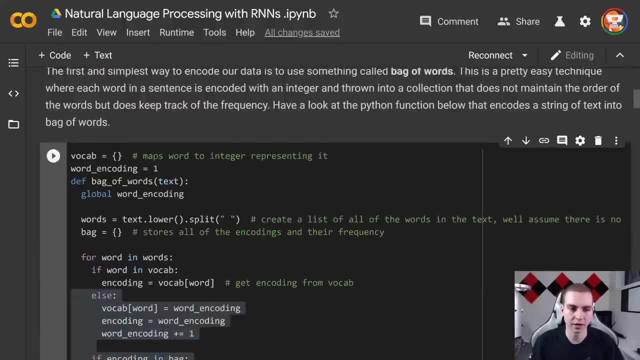 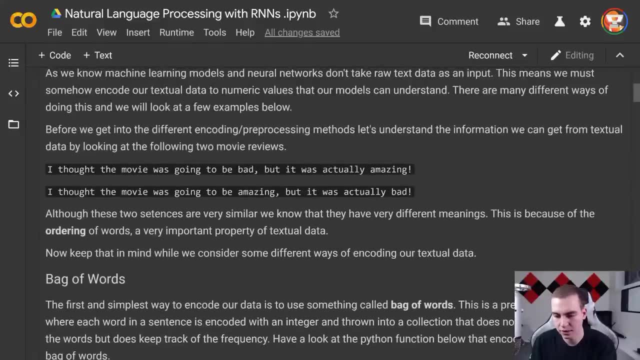 is how we would use bag of words, right, If we didn't encoding kind of like this. that's what that does, And that's one way of encoding it. Now I'm going to go back and we'll talk about another method here as well. actually a few more methods before we get into anything further. Alright, 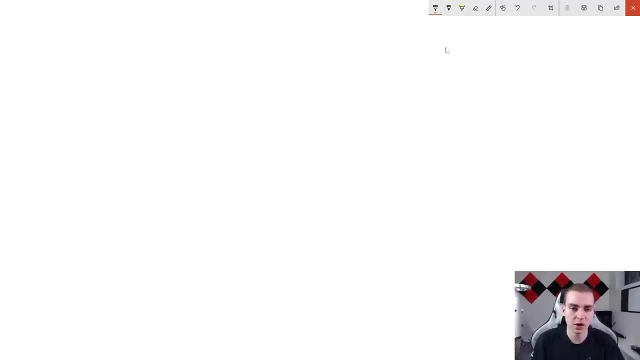 so I'm sure a lot of you were looking at the previous example I did And you saw the fact that what I did was completely remove the idea of kind of sequence or ordering of words, right, And what I did was just throw everything in a bag And I said, Alright, we're just 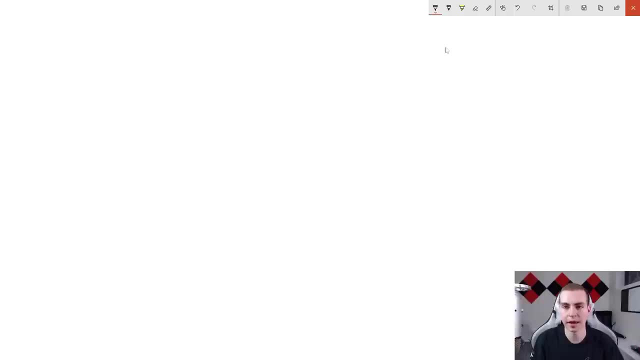 going to keep track of the fact that we have, you know, three A's right. we're going to have four does or seven Tim's right, And we're going to just going to lose the fact that you know words come after one each other. we're going to lose their ordering. 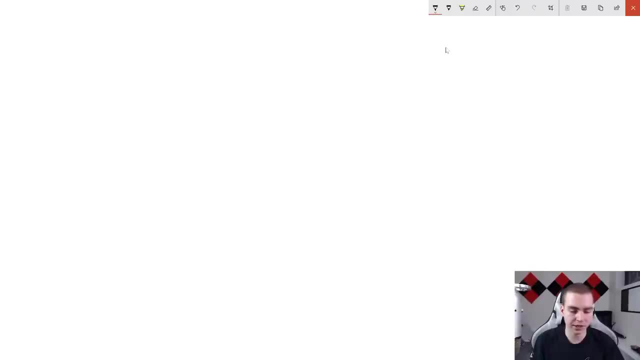 in the sentence And that's how we're going to encode it. And I'm sure a lot of you were saying: Well, why don't we just not lose the ordering of those words? we'll just encode every single word with an integer and just leave it in its space where it would have. 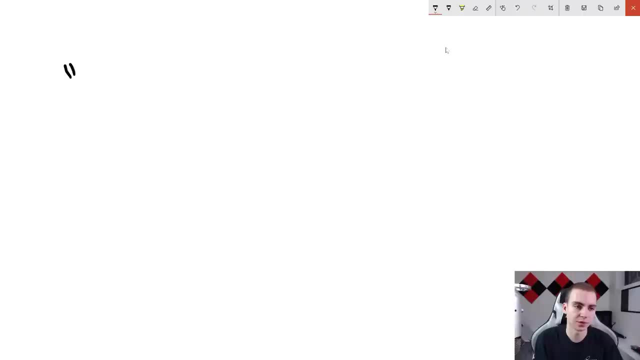 been in the original string. Okay, good idea. So what you're telling me to do is something like this: you know, Tim is here. will be our sentence. Let's say, we encode the word Tim with zero is as well: Here's one, here's two. And then that means our translation goes 012.. And that means right. 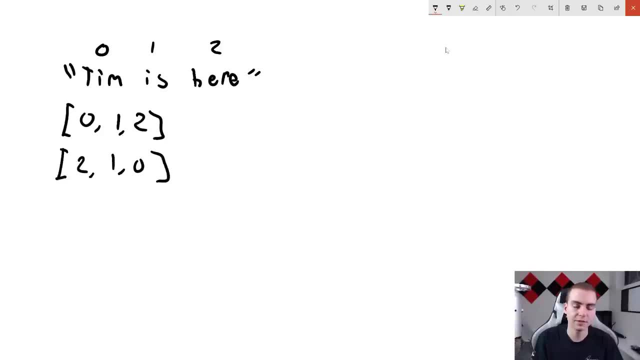 if we have a translation, say like 210,, even though these use the exact same number of words and exact same representation for all these words, well, this is a different sentence And our model should be able to tell that, because these words come in a different order. 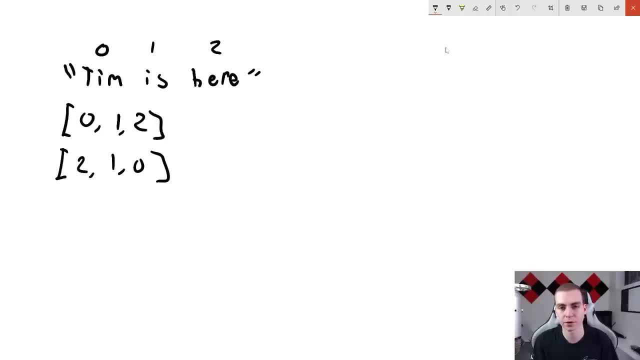 And to you good point if you made that point. but I'm going to discuss where this falls apart as well and why we're not going to use this method. So, although this does solve the problem I talked about previously, where we're going to kind of lose out on the context of a word, 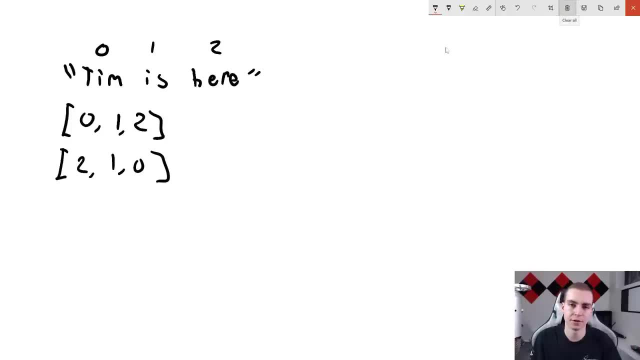 there still is a lot of issues with this, And they come especially when you're dealing with very large vocabularies. Now let's take an example where we actually have a vocabulary of, say, 100,000 words And we know that that means we're going to have to have 100,000. 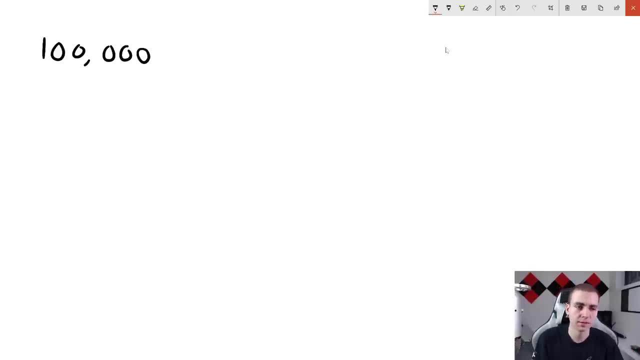 unique mappings from words to integers. So let's say our mappings are something like this: One maps to the string happy, the word happy right To maps, to sound right. And let's say that the string 100,000, or the number 100,000 maps to the word I don't know. 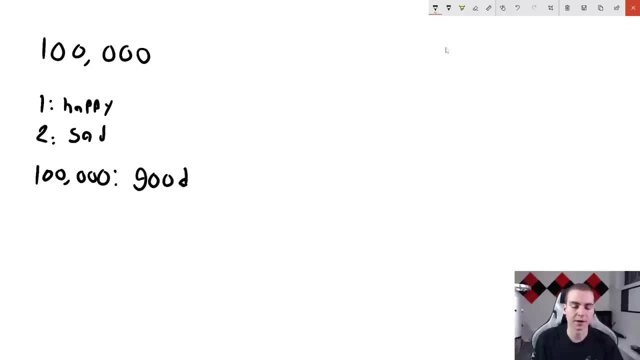 let's say good. Now we know as humans, by kind of just thinking about, let's consider the fact that we're going to try to classify sentences as a positive or negative, So sentiment analysis- that the words happy and good- in that regard, you know, sentiment analysis are probably 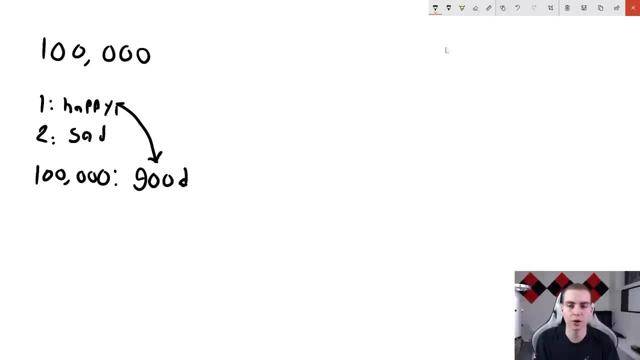 pretty similar words, right? And then if we were going to group these words, we'd probably put them in a similar group. we classify them as similar words. we could probably interchange them in a sentence, We could change the meaning, a whole ton. I mean, it might, but it might not as well. And 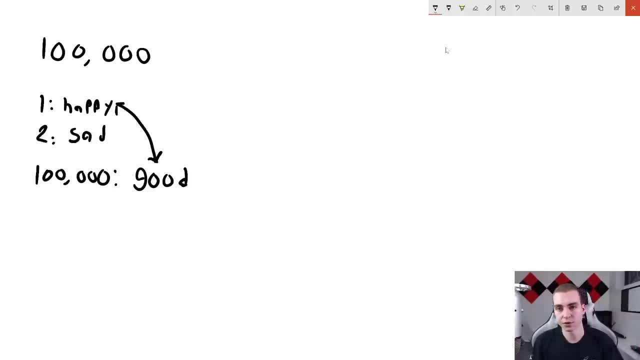 that we could say: these are kind of similar, But our model or our encoder right- whatever we're doing to translate our text into integers here- has decided that 100,000 is going to represent good and one is going to represent happy And well, there's an issue with that. 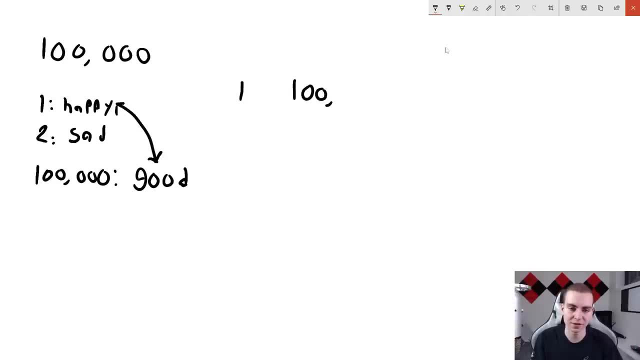 because that means when we pass in something like one or 100,000, to our model, it's gonna have a very difficult time determining the fact that one and 100,000, although they're 99,900, and 999, kind of units apart- are actually very similar words, And that's the issue. we 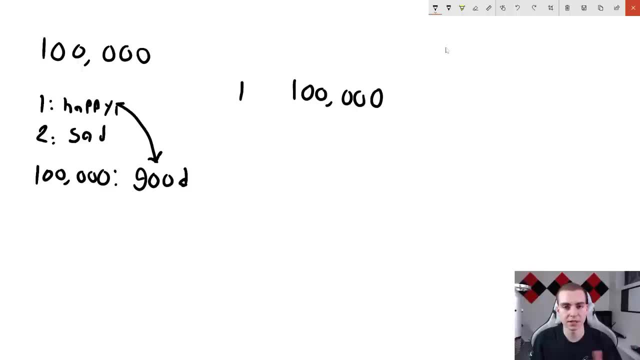 get into when we do something like this is that the numbers we decide to pick to represent each word are very important And we don't really have a way of being able to look at words, group them and saying, Okay, well, we need to put all of the happy words in the 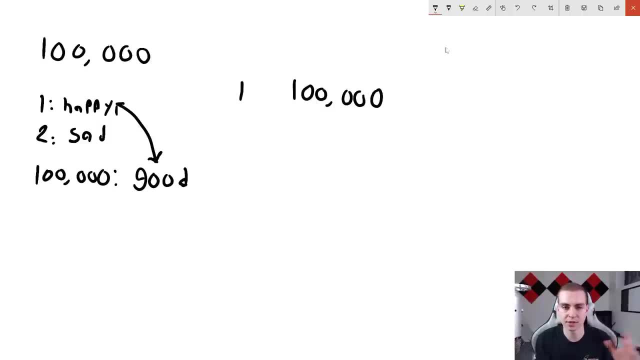 range like zero to 100. All of the like adjectives in this range. we don't really have a way to do that, And this gets even harder for our model when we have these arbitrary mappings right Like two in between, where two is very close to one right. Yet these words are complete. 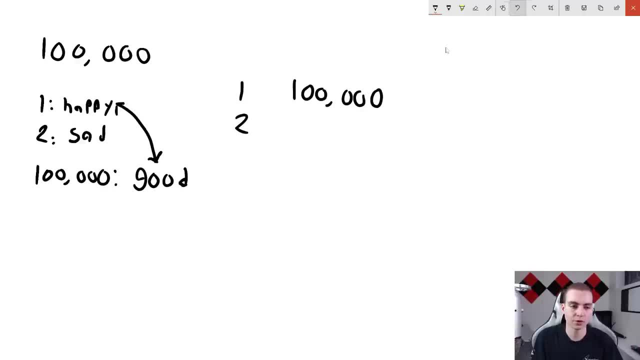 opposites. In fact I'd say they're probably polar opposites. our model- trying to learn that the difference between one and two is actually way larger than the difference between one and 100,000- is going to be very difficult, And say it's even able to do that as soon. 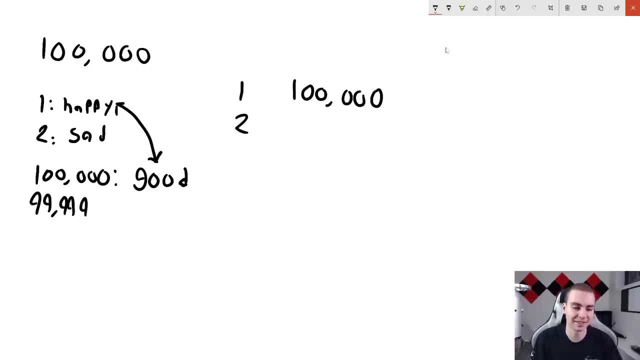 as we throw in the mapping 999,900, we put that as bad. Well, now it gets even more difficult because it's now like: okay, well, if the range is this big, then that means these words are actually very similar. 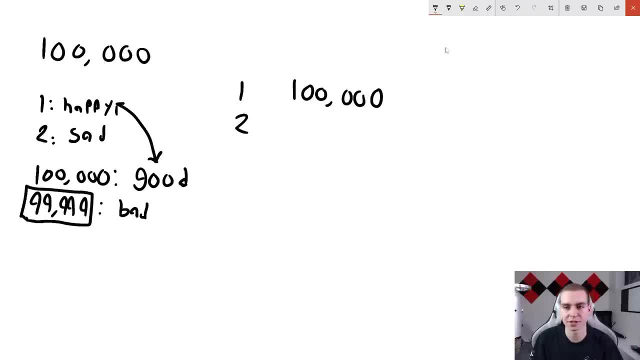 But then you throw another word in here like this, and it messes up the entire system. So that's kind of what I want to show. is that that's where this breaks apart on these large vocabularies, And that's why I'm going to introduce us now to another concept called 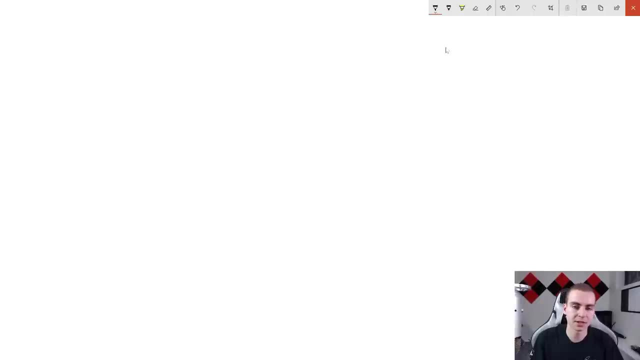 word embeddings. Now, what word embeddings does is essentially try to find a way to represent words that are similar, using very similar numbers. And, in fact, what a word embedding is actually going to do- I'll talk about this more in detail as we go on- is classify, or 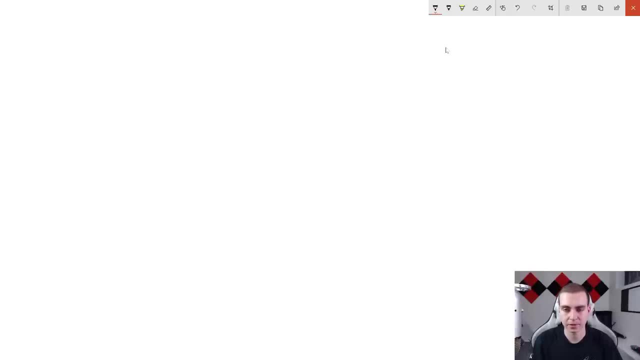 translate one of our words into a vector And that vector is going to have some you know n amount of dimensions. usually we're going to use something like 64, maybe 128 dimensions for each vector, And every single component of that vector will kind of tell us what group. 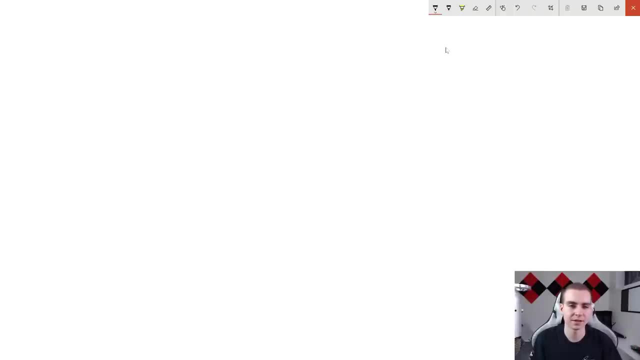 it belongs to or how similar it is to other words. So let me give you an idea of what I mean. So we're going to create something called a word embeddings. Now don't ask why it's called embeddings. I don't know the exact reason, but I believe it's to have has to. 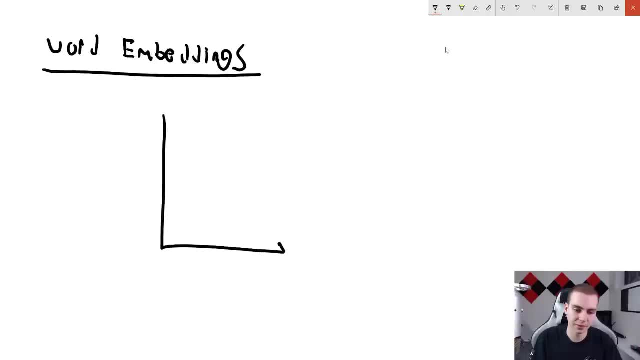 do something with the fact that they're vectors. And let's just say we have a 3d plane like this And we've already kind of looked at what vectors are before, So I'll skip over explaining them, And what we're going to do is take some word. So let's say we have the word good And instead of 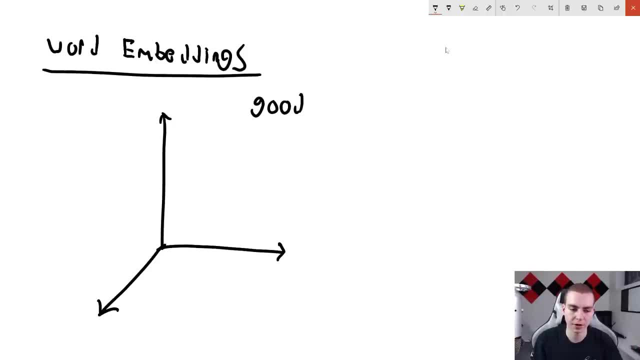 picking some integer to represent it. we're going to pick some vector, which means we're going to draw some vector in this 3d space. Actually, let's make this a different color. Let's make this vector say red, like this: And this vector represents this word good, 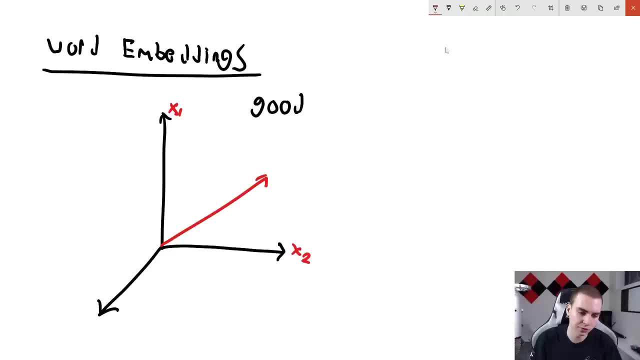 And in this case we'll say we have x one, x two, x three as our dimensions, which means that every single word in our data set will be represented by three coordinates. So one vector with three different dimensions, where we have x one, x two and x three And our 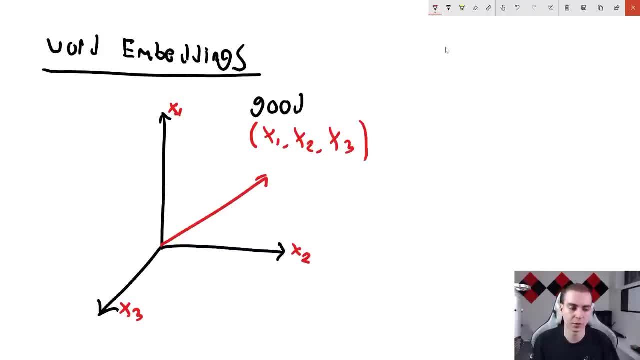 hope is that, by using this word embeddings layer- and we'll talk about how it accomplishes this in a second- is that we can have vectors that represent very similar, words being very similar, which means that you know if we have the vector, good, here we're going to. 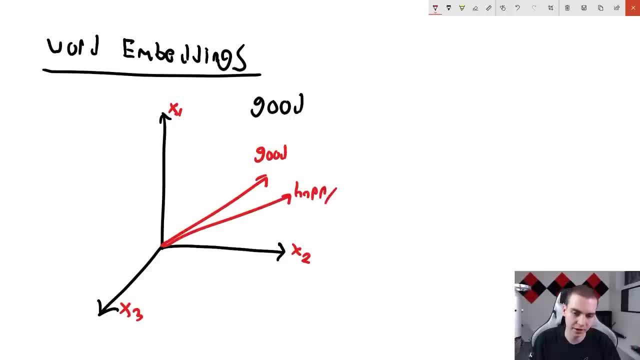 have a vector. good here we would hope the vector happy from our previous example right will be a vector that points in a similar direction to it. that is kind of a similar looking thing where the angle between these two vectors right and maybe I'll draw it. 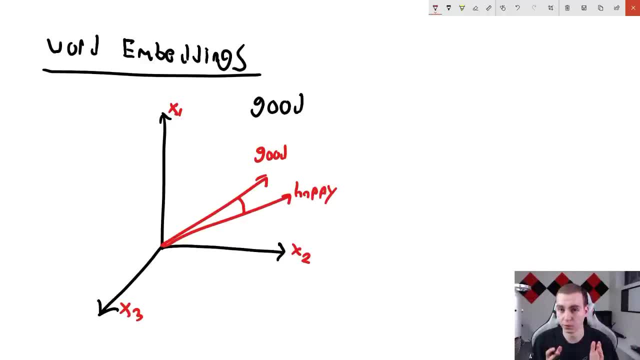 here, So we can see is small, so that we know that these words are similar. And then we would hope that if we had a word that was much different, maybe say like the word bad, that that would point in a different direction the vector that represents it and that that 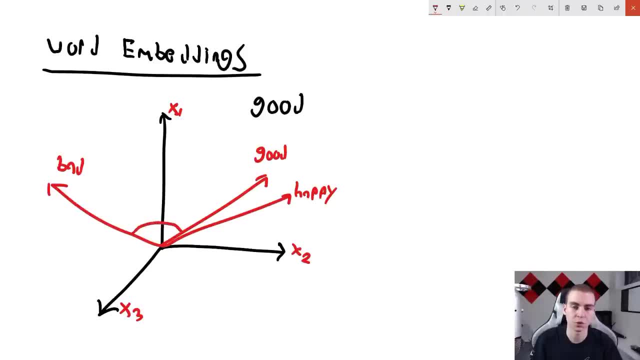 would tell our model, because the angle between these two vectors is so big that it's going to be big that these are very different words right Now. in theory, does the embedding word layer work like this? you know, not always, but this is what it's trying to do, is essentially. 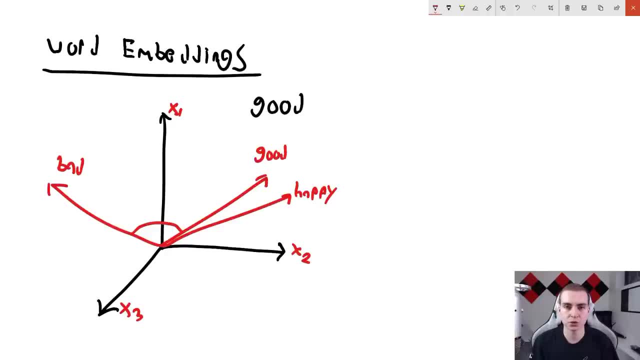 pick some representation in a vector form for each word And then these vectors- we hope, if they're similar words are going to be pointing in a very similar direction And that's kind of the best explanation of a word. embeddings layer. I can give you Now how. 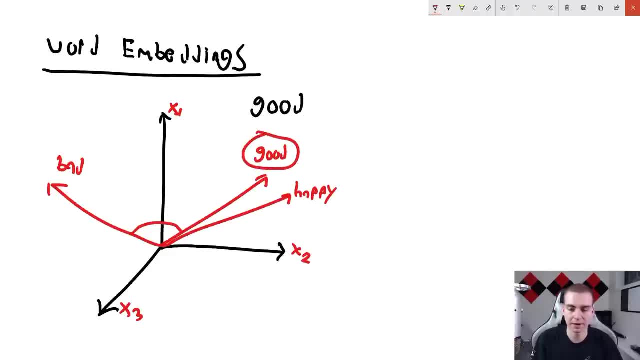 do we do this, though? How do we actually, you know, go from word to vector and have that be meaningful? Well, this is actually what we call a layer, So word embeddings is actually a layer, And it's something we're going to add to our model, And that means that this actually learns the. 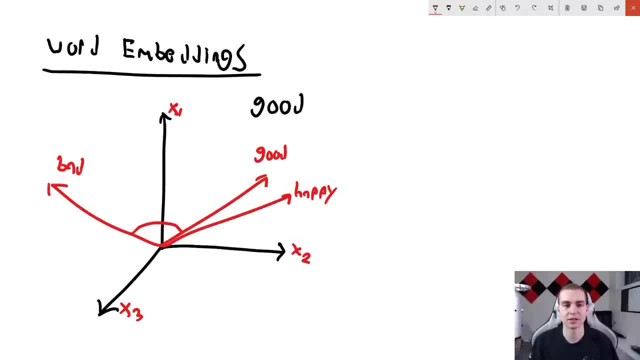 embeddings for our words. And the way it does that is by trying to kind of pick out context in the sentence and determine, based on where a word is in a sentence, kind of what it means, and then encodes it. doing that. Now, I know that's kind of a rough explanation to give. 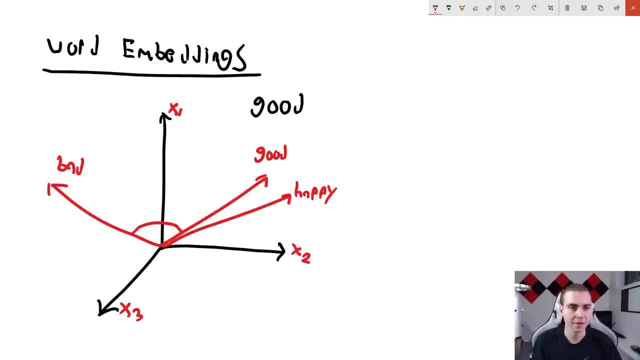 to you guys. I don't want to go too far into word embeddings in terms of the math because I don't want to get you know, waste our time or get too complicated if we don't need to, But just understand that our 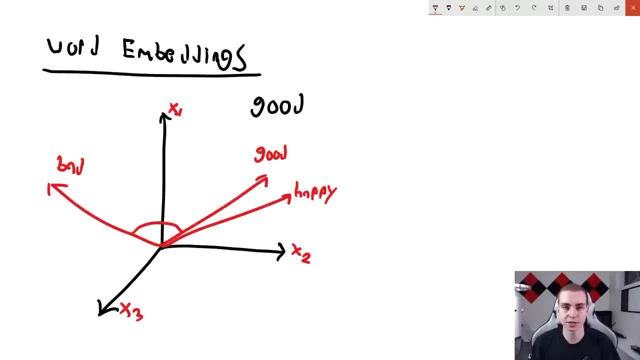 word embeddings are actually trained and that the model actually learns these word embeddings as it goes, And we hope that by the time it's looked at enough training data it's determined really good ways to represent all of our different words so that they make. 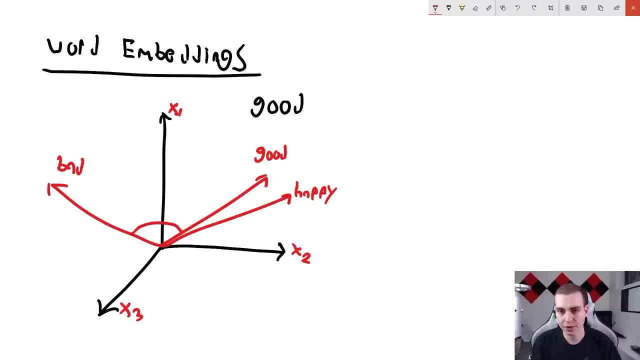 sense to our model in the further layers, And we can use pre trained word embedding layers if we'd like, just like we use that pre trained convolutional base in the previous section, And we might actually end up doing that. Actually, probably not in this tutorial, but it is something to consider that you can't. 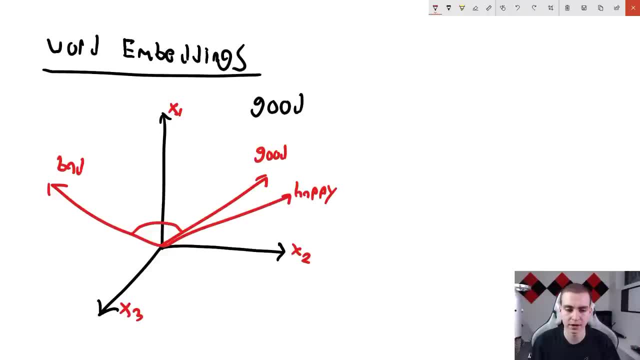 do that. So that's how word embeddings work. This is how we encode textual data, And this is why it's so important that we kind of consider the way that we pass information to our neural network, because it makes a huge difference. Okay, so now that we've talked about kind, 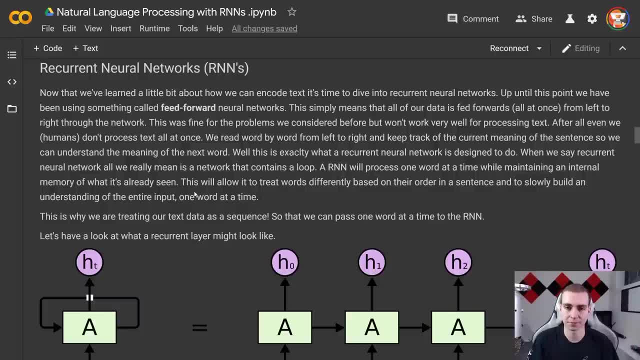 of the form that we need to get our data in before we can pass it further in the neural network, right before it can get past that embedding layer, before it can get put in, put into any dense neurons, before we can even really do any math with it. we need to turn. 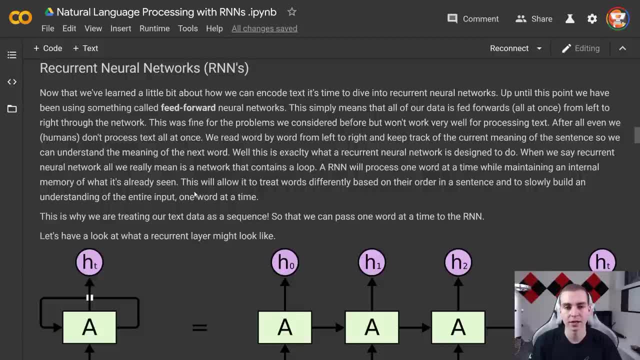 it into numbers, right? So let's talk about that. So let's talk about the process of processing textual data. So, now that we know that it's time to talk about recurrent neural networks, Now, recurrent neural networks are the type of networks we use when we process textual data. Typically, you don't. 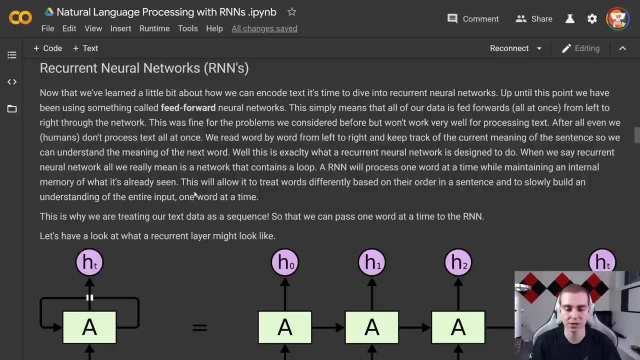 always have to use these, but they are just the best for natural language processing And that's why they're kind of their own class. right Now, the fundamental difference between a recurrent neural network and something like a dense neural network or a convolutional 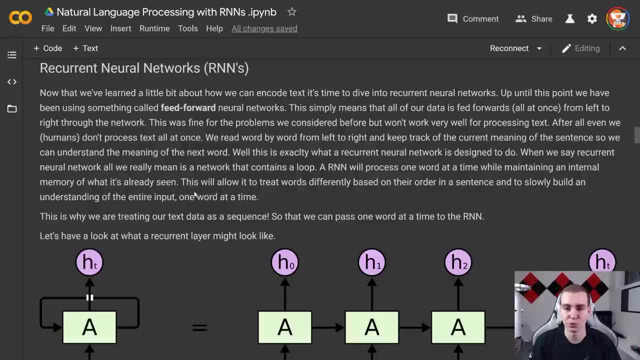 neural network is the fact that it contains an internal loop. Now, what this really means is that the recurrent neural network does not process our entire data at once, So it doesn't process the entire training example or the entire input to the model at once. what it does is processes it at different time steps. 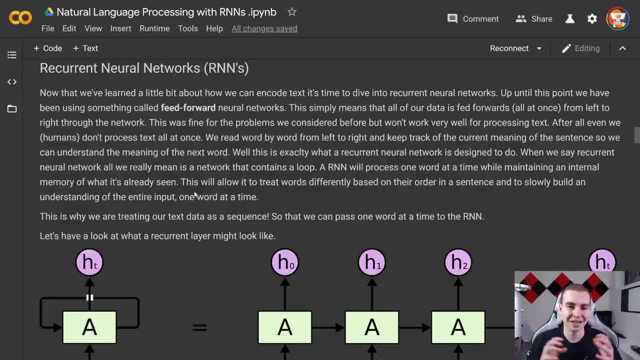 and maintains what we call an internal memory and kind of an internal state, so that when it looks at a new input it will remember what it's seen previously and treat that input based on kind of the context or the understanding it's already developed. Now I understand. 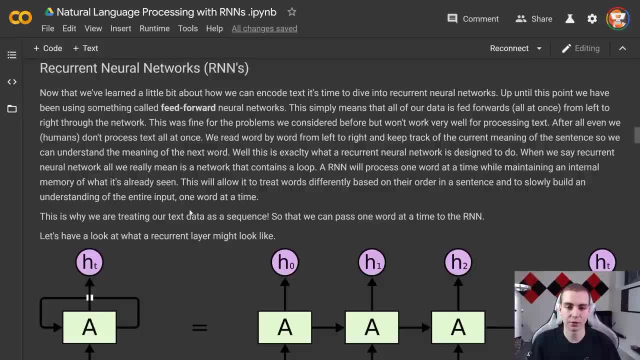 that this doesn't make any sense right now, But with a dense neural network, or the neural networks we looked at so far, we call those something called called feed forward neural networks. What that means is we give all of our data to it at once And we pass that data from left to right, or I guess for you guys. 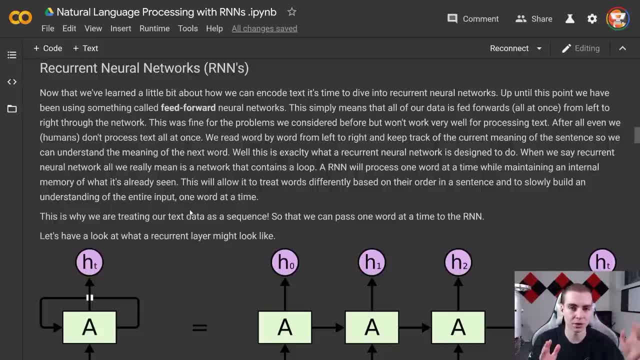 from left to right. So we give all of the information. you know we would pass those through the convolutional layer to start. maybe we have passed them through dense neurons, but they get given all of the info And then that information gets translated through the 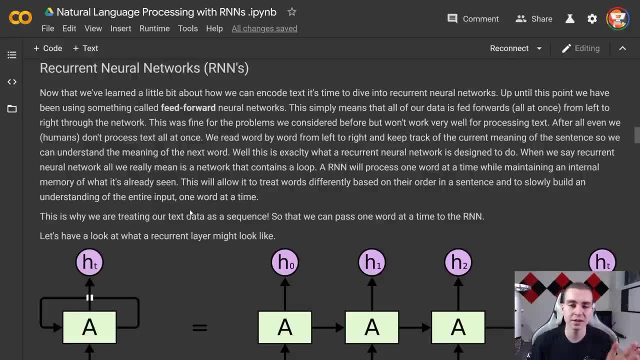 network to the very end, again from left to right, Whereas here, with recurrent neural networks, we actually have a loop which means that we don't feed the entire textual data at once. we actually feed one word at a time. it processes. 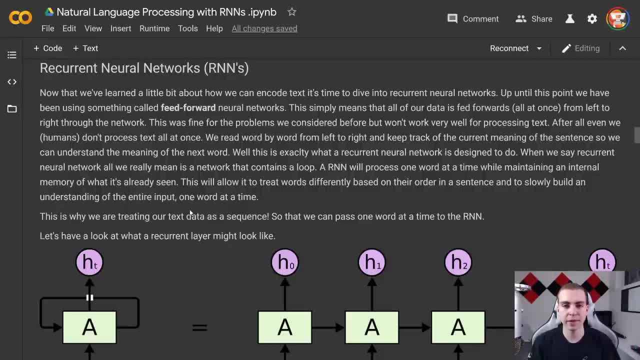 that word, generates some output based on that word and uses the internal memory state that is keeping track of to do that as part of the calculation. So, essentially, the reason we do this is because, just like humans, when we, you know, look at text, we don't just take. 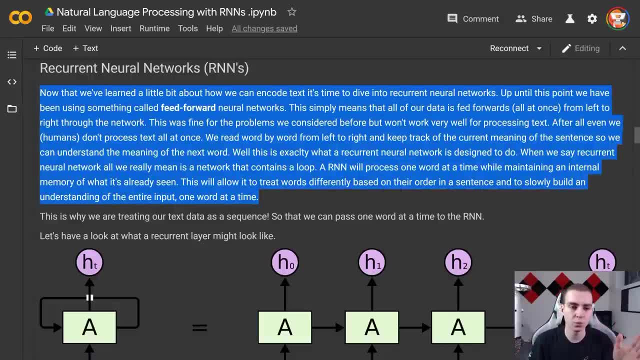 a photo of this text and process it all at once. We read it left to right, word to word, And, based on the words that we've already read, we start to slowly develop an understanding of what we're reading, right, If I just read: 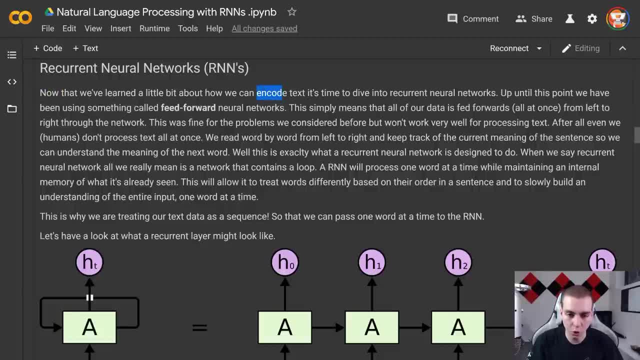 the word now, that doesn't mean much to me. if I just read the word in code, that doesn't mean much, Whereas if I read the entire sentence- now that we've learned a little bit about how we can encode text- I start to develop an understanding about what this next word. 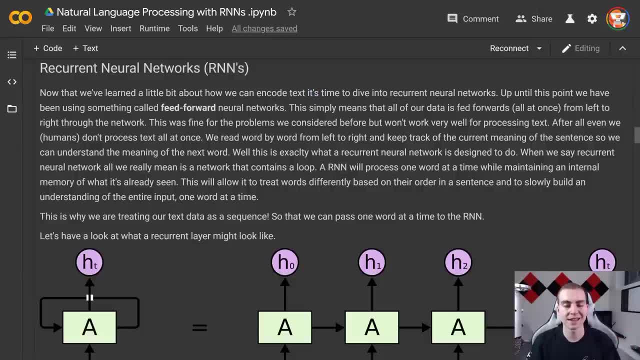 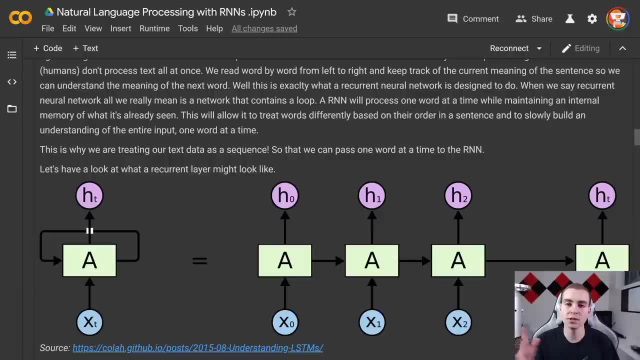 means based on the previous words before it. right- And that's kind of the point here- is that this is what a recurrent neural networks going to do for us: it's going to read one word at a time and slowly start building up its 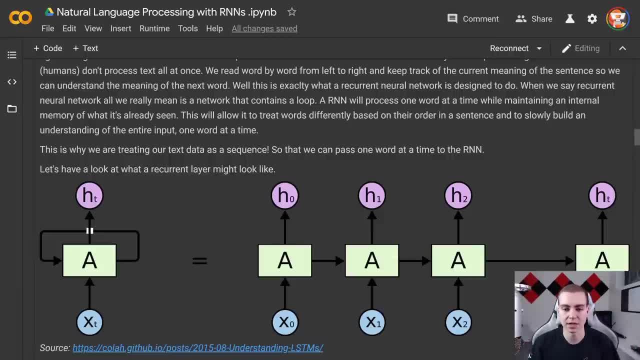 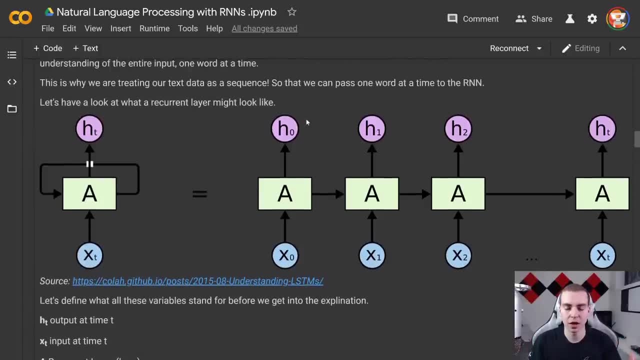 understanding of what the entire textual data means. And this works in kind of a more complicated sense than that. we'll draw it out a little bit, But this is kind of what would happen if we on, I guess, unraveled a recurrent layer, because recurrent neural network, yes, it. 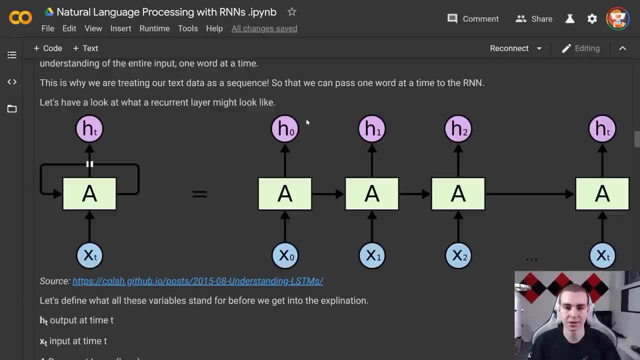 has a loop in it, But really the recurrent aspect of a neural network is the layer that implements this recurrent function functionality with a loop. Essentially, what we can see here is that if we're saying x is our input and h is our output, x, t is going to be our input at time t, whereas ht is going. 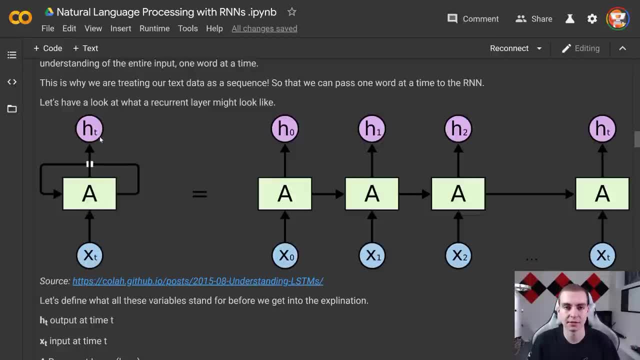 to be our output at time t if we had a text of, say, length four, so four words, like we've encoded them into integers Now. at this point, the first input at time zero will be the first word into our network, right, or the first word that this layer is going. 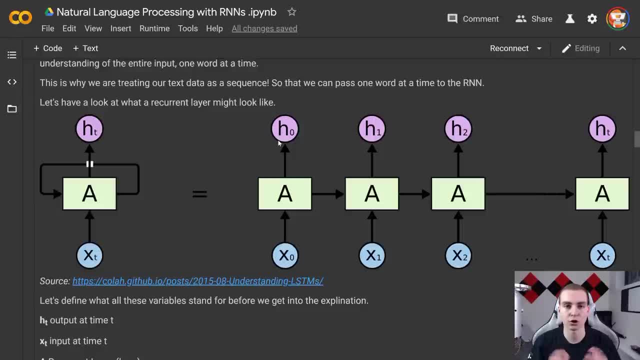 to see, And the output at that time is going to be our current understanding Of the entire text, after looking at just that one word. Next, what we're going to do is process input, one which will be the next word in the sentence, But we're going to use 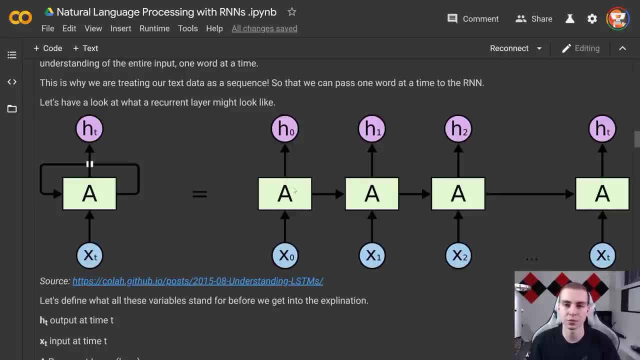 the output from the previous kind of computation or the previous iteration to do this. So we're going to process this word in combination with what we've already seen and then have a new output which hopefully should now give us an understanding of what those two words. 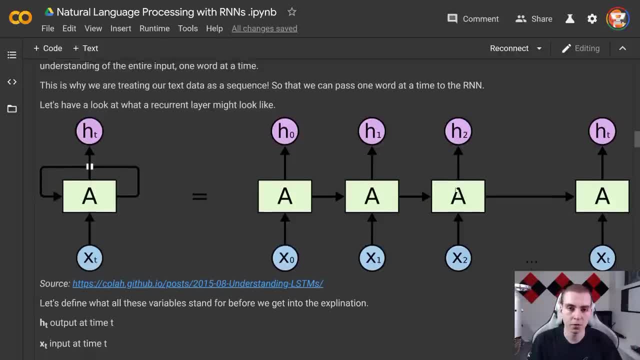 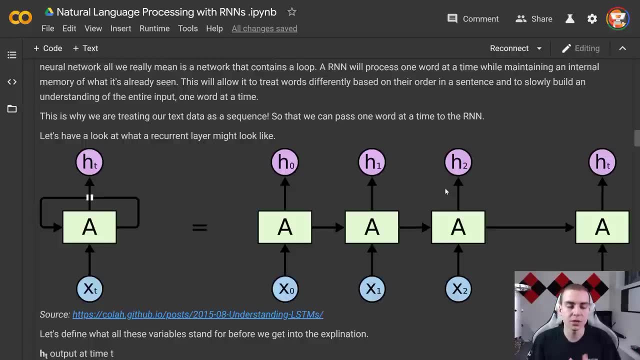 mean. Next, we'll go to the third word and so forth And slowly start building our understanding of what the entire textual data means by building it up one by one. The reason we don't pass the entire sequence at once is because it's 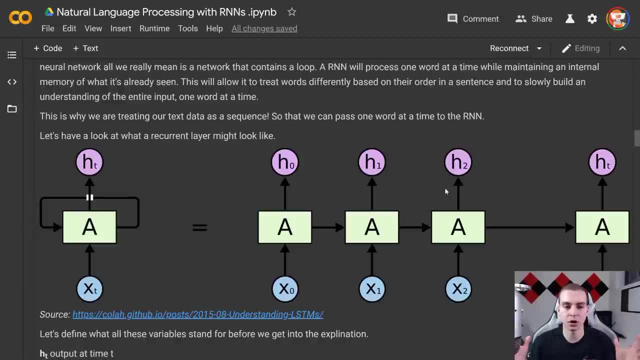 very, very difficult to just kind of look at this huge blob of integers and figure out what the entire thing means, If we can do it one by one and understand the meaning of specific words based on the words that have come before it and start learning those patterns. 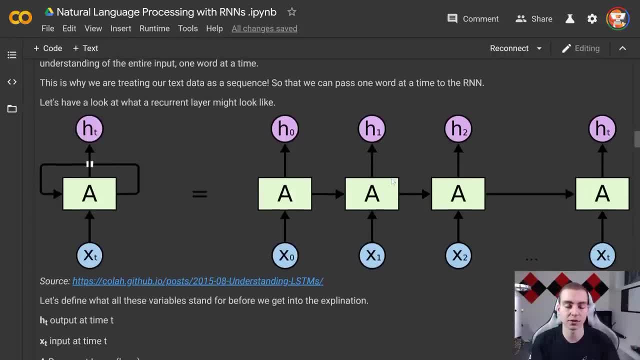 that's going to be a lot easier for a neural network to deal with than just passing it all at once, looking at it and trying to get some output, And that's why we have these recurrent layers. there's a few different types of them. 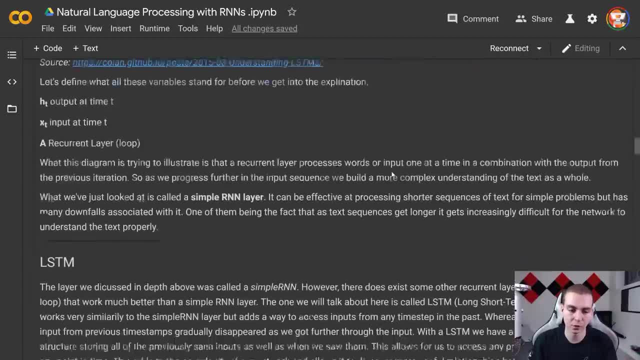 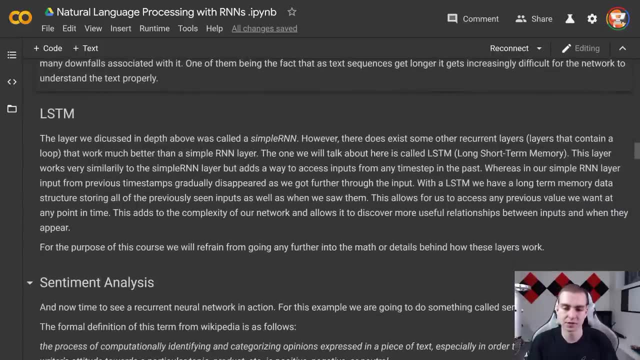 And I'm going to go through them And then we'll talk a little bit more in depth of how they work. So the first one is called long, short term memory And actually, in fact, before we get into this, let's let's talk about just a first, like a simple layer. so 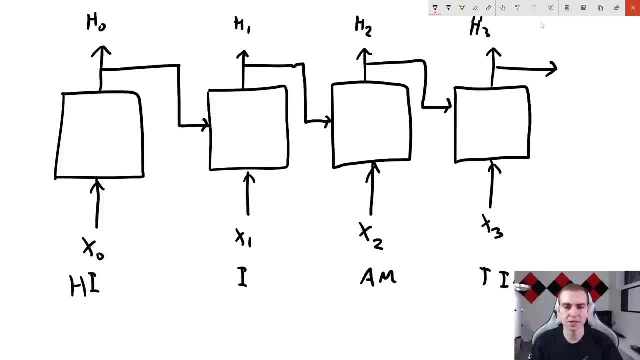 that we kind of have a reference point before going here. Okay, so this is kind of the example I want to use here to illustrate how a recurrent neural network works in a more- I don't know- teaching style, rather than what I was doing before. 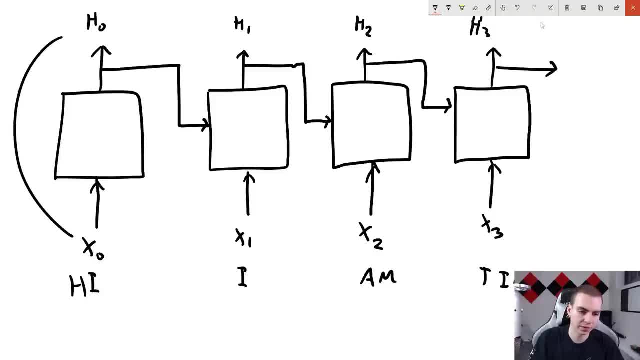 So essentially, the way that this works is that this whole thing that I'm drawing here right, all of this circle stuff, is really one layer, And what I'm doing right now is breaking this layer apart and showing you kind of how this works in a series of steps. 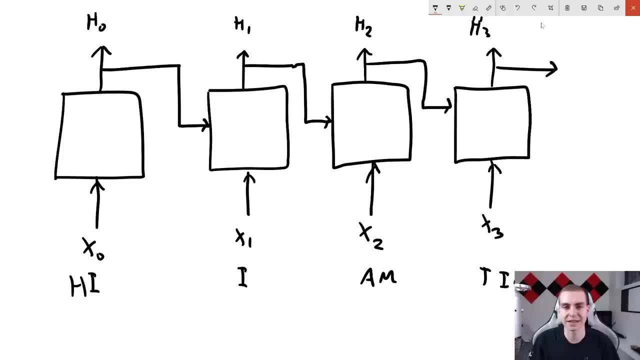 So, rather than passing all the information at once, we're going to pass it as a sequence, which means that we're going to have all these different words and we're going to pass them one at a time, to the kind of to the layer right to this recurrent layer. So we're going 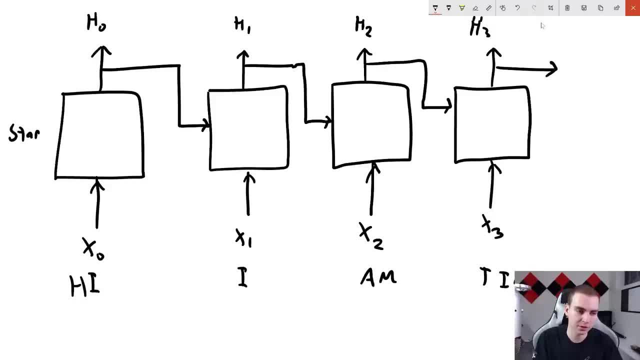 to start from this left side over here. So let's write. you know, start over here at time step zero, that's what zero means. So time step is just. you know the order. In this case, this is the. 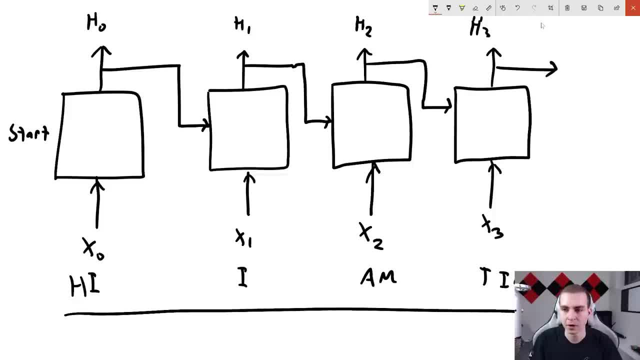 first word. So let's say we have the sentence: Hi, I am Tim. right, We've broken these down into vectors. they've been turned into their numbers. I'm just writing them here So we can kind of see what I mean in like a natural language. And they are the input to this recurrent. 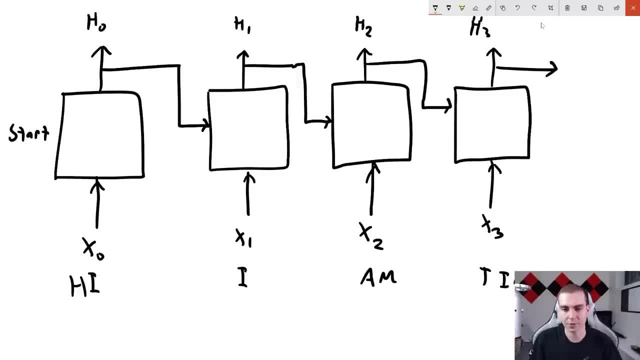 layer. So all of our different words, right, that's how many kind of little cells we're going to draw. here is how many words we have In this sequence that we're talking about. So in this case we have four, right four words. 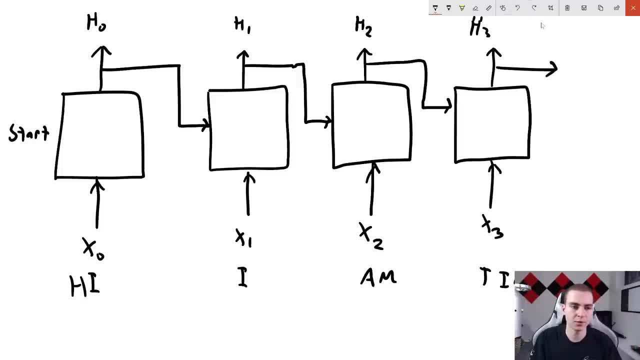 So that's why I've drawn four cells to illustrate that. Now what we do is that time step zero. the internal state of this layer is nothing, there's no previous output, we haven't seen anything yet, which means that this first kind of cell, which is what I'm looking at, 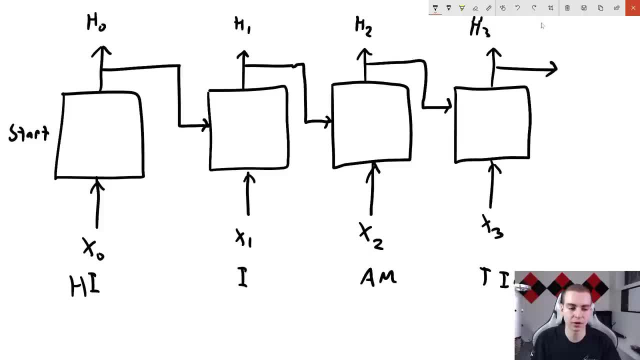 right here. what I'm drawing in this first cell is only going to look and consider this first word and kind of make some prediction about it and do something with it. we're going to pass Hi to this cell- some math is going to go on in here- And then what it's going to do. 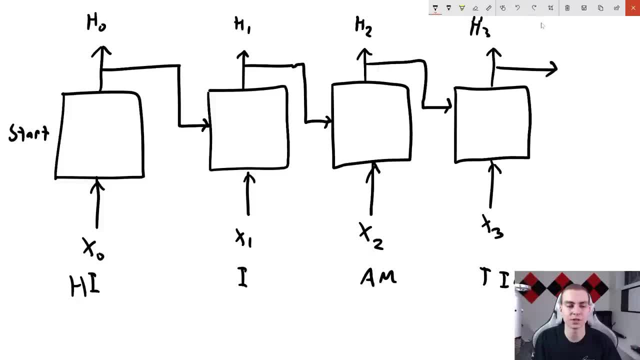 is. it's going to output some value which you know tells us something about the word high right, some numeric value. we're not going to talk about what that is, but it's going to. there's gonna be some output. Now, what happens is after the cell has finished. 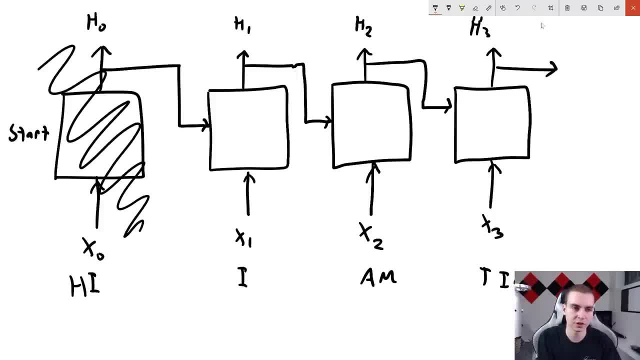 processing this. so right, so this one's done. this is completed. h zero the outputs. there we'll do a checkmark to say that that's done. it's finished processing. this output gets fed into actually the same thing Again. we're kind of just keeping track of it And now what we do is we process the next. 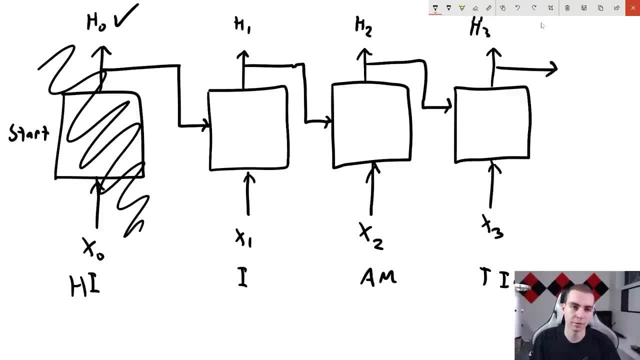 input, which is I, and we use the output from the previous cell to process this and understand what it means. So now, technically, we should have some output from the previous cell, So from whatever high was right. we do some analysis on the word I. we kind of combine these things. 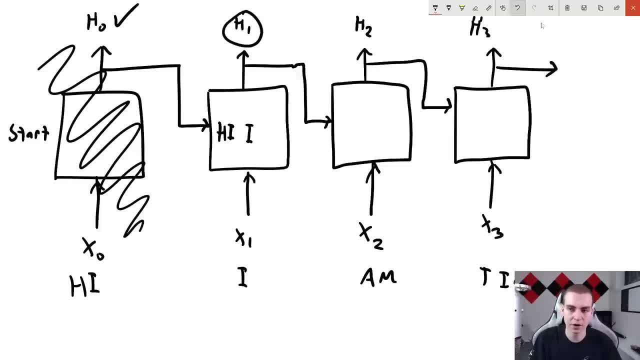 together, And that's the output of this cell- is our understanding of not only the current input but the previous input with the current input. So we're slowly kind of building up our understanding of what this word I means, based on the words we saw before. And that's the point I'm trying. 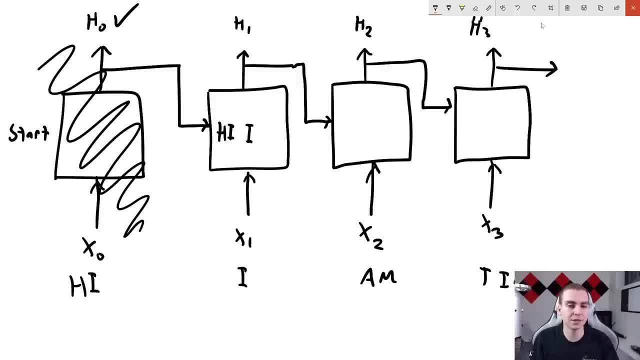 to get at is that this network uses what it's seen previously to understand the next thing that it sees. it's building a context. it's trying to understand not only the word but what the word means, you know, in relation to what's come before it. So that's what's. 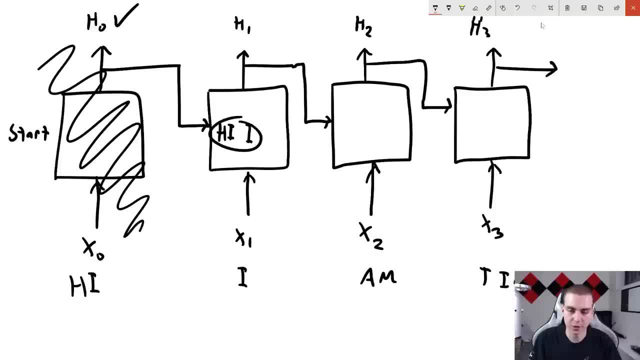 happening here. So then, this output here: right, we get some output, We finish this, we get some output. h1, h1 is passed into here, And now we have the understanding of what high and I means. And we add: am like that we do some kind of computations, we 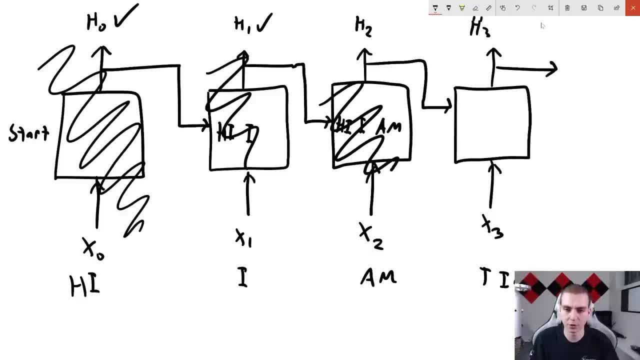 build an understanding of what the sentences, and then we get the output h2, that passes to h3. And now, finally, we have this final output, h3,, which is going to understand, hopefully, what this entire thing means. Now, this is good. 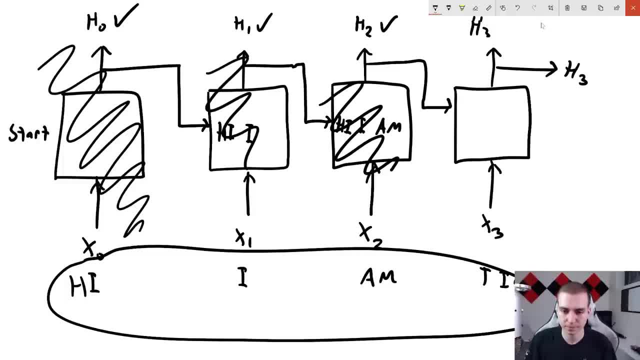 This works fairly well And this is called a simple RNN layer, which means that all we do is we take the output from the previous cell or the previous iteration, because really all of these cells is just an iteration, almost in a for loop right based on all the different. 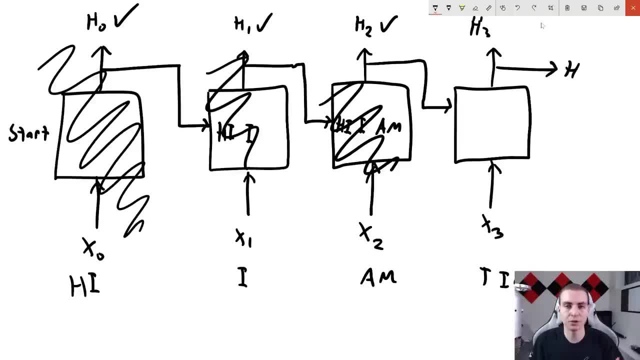 words in our sequence And we slowly start building to that understanding as we go through the entire sequence. Now, the only issue with this is that, as we have a very long sequence, so sequences of length, say 100, or 150. 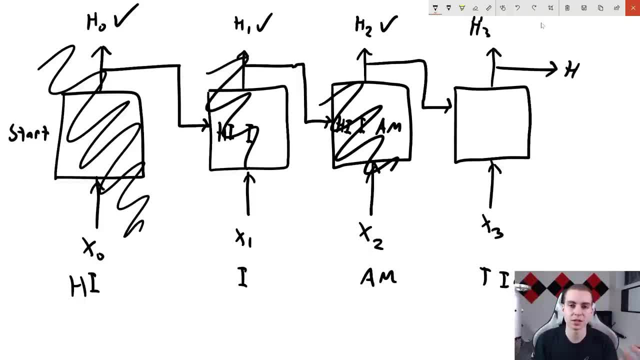 The beginning of those sequences starts to kind of get lost as we go through this, because, remember, all we're doing, right is the output from h2 is really a combination of the output from h0 and h1.. And then there's a new word that we've looked at and h3 is now a combination. 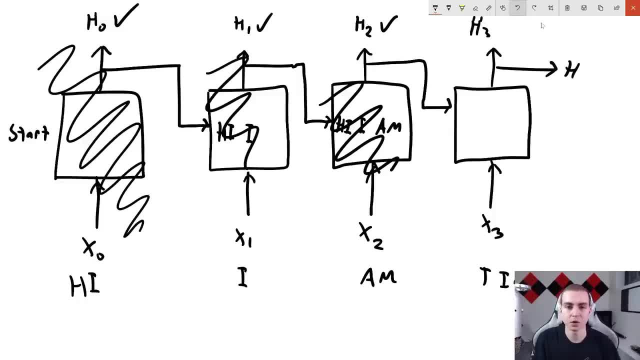 of everything before it and this new word. So it becomes increasingly difficult for our model to actually build a really good understanding of the text in general when the sequence gets long, because it's hard for it to remember what it's seen At the very beginning, because that is now so insignificant. there's been so many outputs. 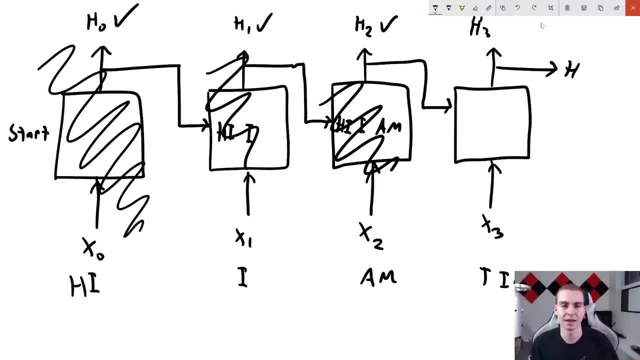 tacked on to that that it's hard for it to go back in and see that. if that makes any sense. Okay, so what I'm going to do now is try to explain the next layer we're going to look at, which is called LSTM. So the previous layer. we just looked at the recurrent layer. 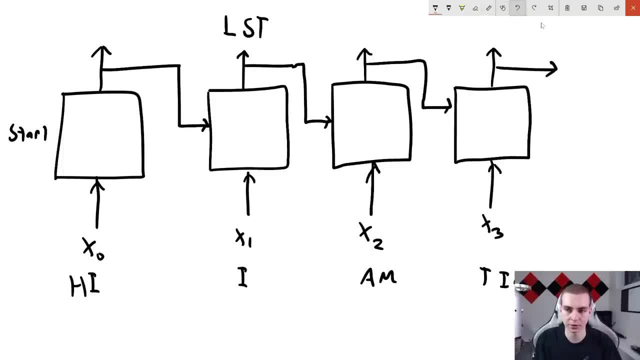 was called a simple RNN layer. So simple recurrent neural network layer, whatever you want to call it right, simple recurrent layer. Now we're going to talk about the layer which is LSTM, which stands for long, short term memory. 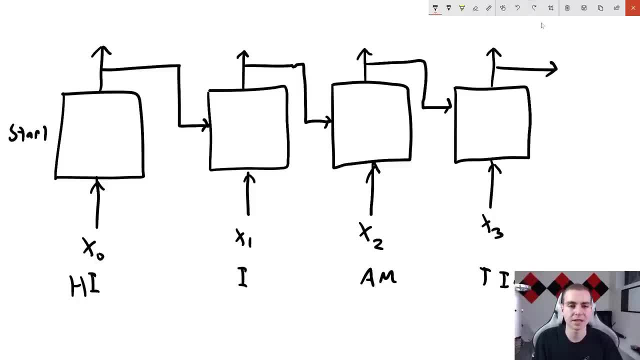 Now long and short are hyphenated together, But essentially what we're doing- and it just gets a little bit more complex, but I won't go into the math- is we add another component that keeps track of the internal state. So right now, the only thing that we 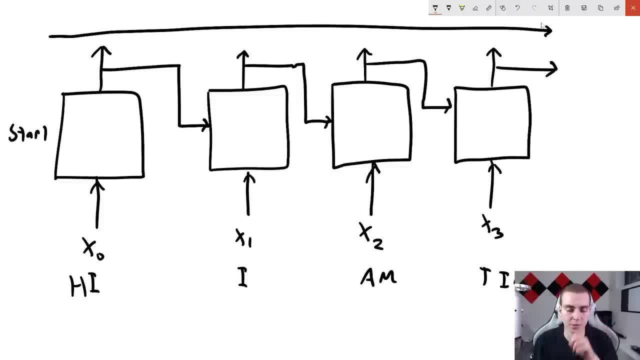 were tracking as kind of our internal state, as the memory for this model was the previous output. So whatever the previous output was, so for example, at time zero here there was no previous output, So there was nothing being kept in this model, But at 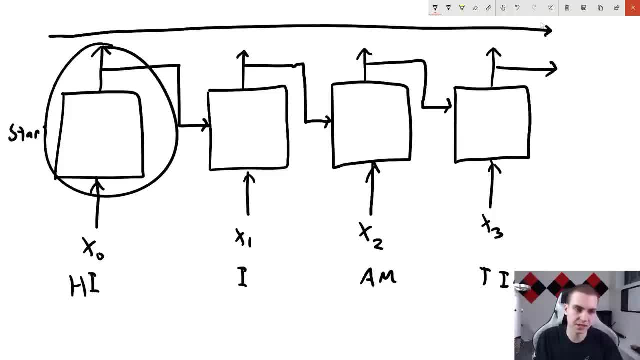 time one, the output from this cell right here was what we were storing, And then at cell two, the only thing we were storing was the output at time one right, And we've lost now the output from time zero. what we're adding in long short term, memory is an ability. 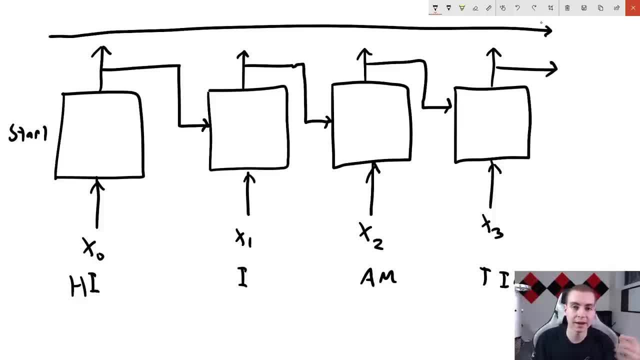 to access the output from any previous state at any point in the future when we want it, And what this means is that, rather than just keeping track of the previous output, we're adding all of the outputs that we've seen so far into what I'm going to call my little. 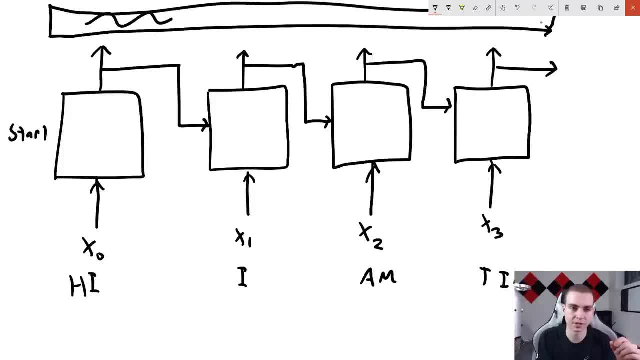 kind of conveyor belt. it's going to run at the top up here. I know it's kind of hard to see, but it's just what I'm highlighting. It's almost just like a lookup table that can tell us the output at any previous cell that we want, So we can kind of add things. 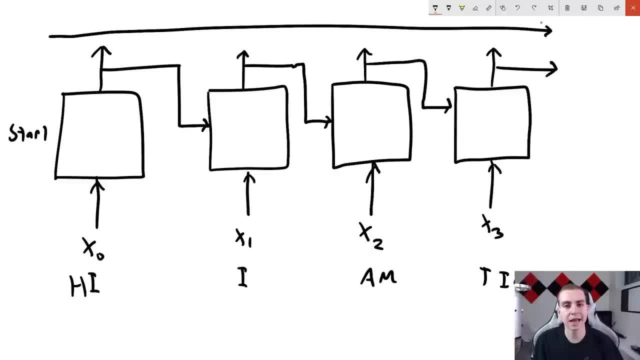 to this conveyor belt, we can pull things off, we can look at them, And this just adds a little bit of complexity to the model. it allows us to not just remember the last state, but look anywhere at any point in time, which can be useful. 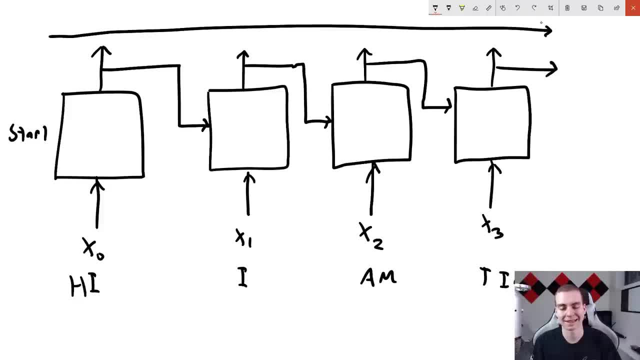 Now I don't want to go into much more depth about exactly how this works, But essentially you know, just think about the idea that as the sequence gets very long, it's pretty easy to forget the things we saw at the beginning. So if we can keep track of some of the things, 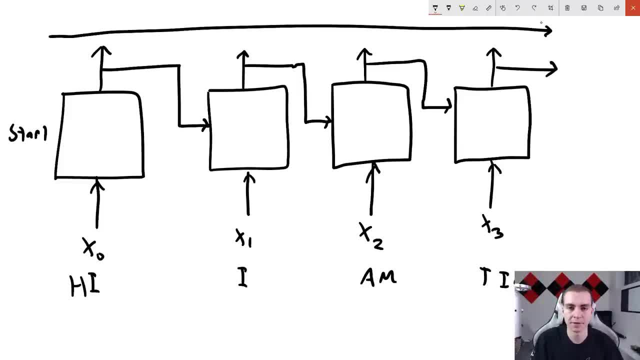 we've seen at the beginning and some of the things in between on this little conveyor belt and we can access them whenever we want. then that's going to make this probably a much more useful layer. right, we can look at the first sentence and the last sentence. 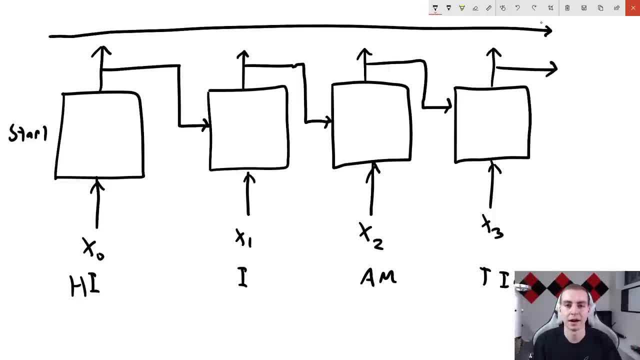 of a big piece of text at any point that we want And say, Okay, you know, this tells us x about the meaning of this text, right? So that's what this LSTM does. Again, I don't want to go too far. we've already spent a lot of time. 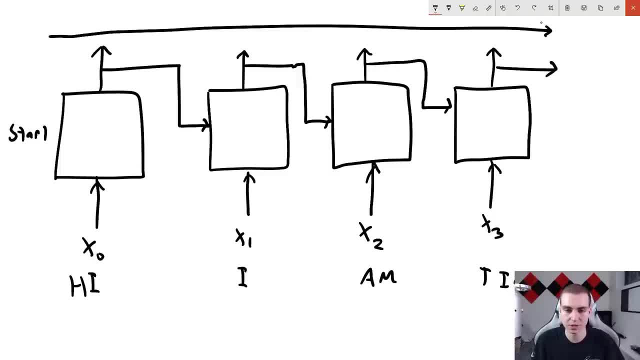 kind of covering, you know, recurrent layers and how this works. Anyways, if you do want to look it up, some great mathematical definitions again- I will source everything at the bottom of this document So you can go there. But again, that's LSTM: long short term memory. 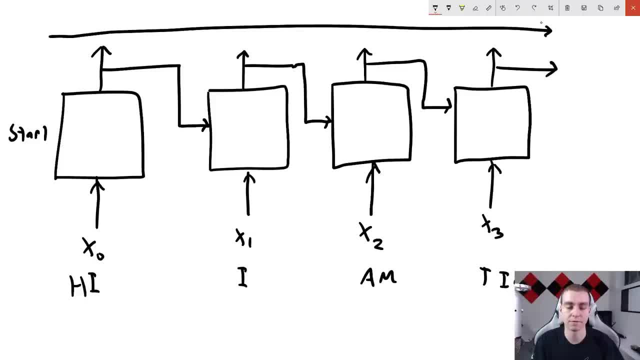 that's what we're going to use for some of our examples, although simple RNN does work fairly well for shorter length sequences. And again, remember, we're going to use a lot of our examples here. we're going to use a lot of our examples here. we're going to use a lot of our examples. here we're going. 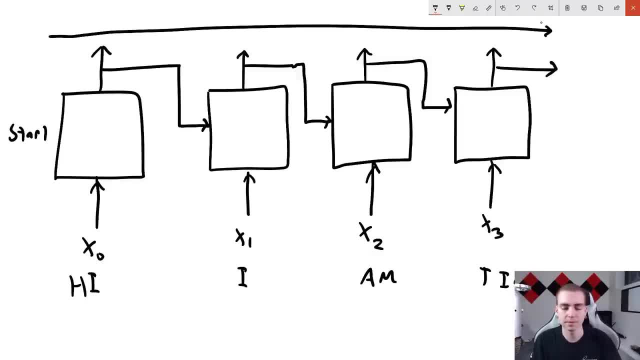 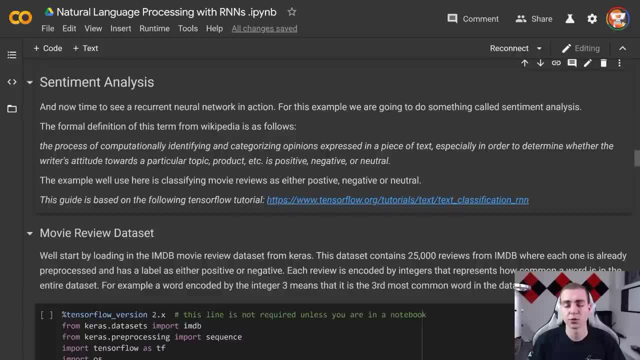 we're treating our text as a sequence now, or we're going to feed each word into the recurrent layer and it's going to slowly start to develop an understanding as it reads through each word right and processes that Okay. so now we are on to our first example. 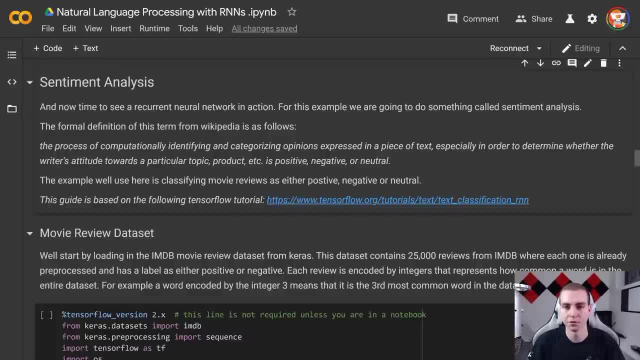 where we're going to be performing sentiment analysis on movie reviews to determine whether they are positive reviews or negative reviews. Now we already know what sentiment means. That's essentially what I just described. So, picking up, you know whether a block of 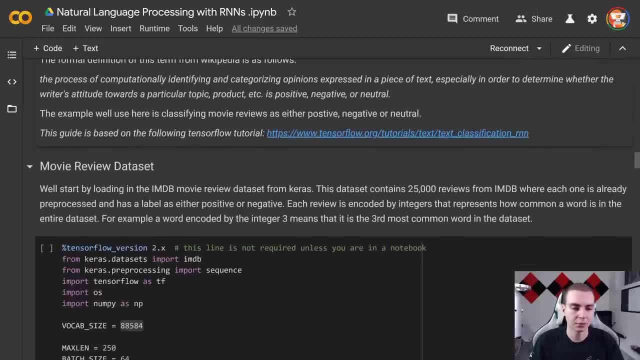 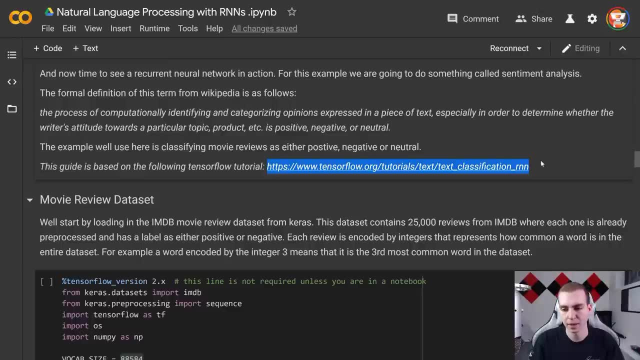 text is considered positive or negative And for this example, we're going to be using- we're going to be using the movie review data sets. Now, as per usual, this is based off of this TensorFlow tutorial slash guide. I found this one kind of confusing to follow. 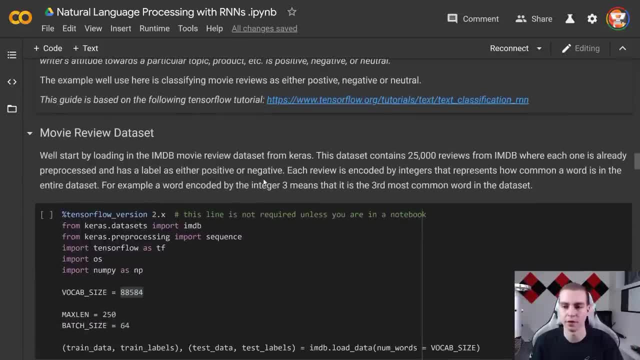 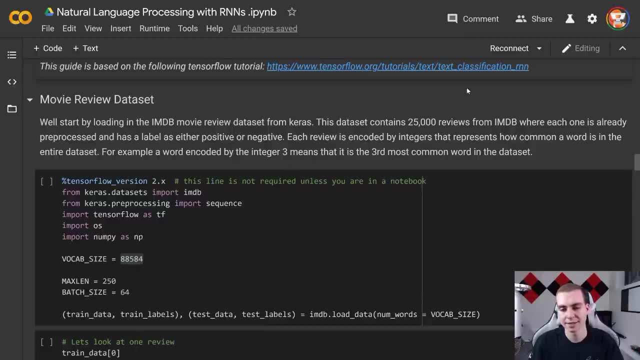 on the TensorFlow website, But obviously you can follow along with that if you don't prefer that version over mine. But anyways, we're going to be talking about the movie review data set. So this data set is straight from Kara's and it contains 25,000 reviews. 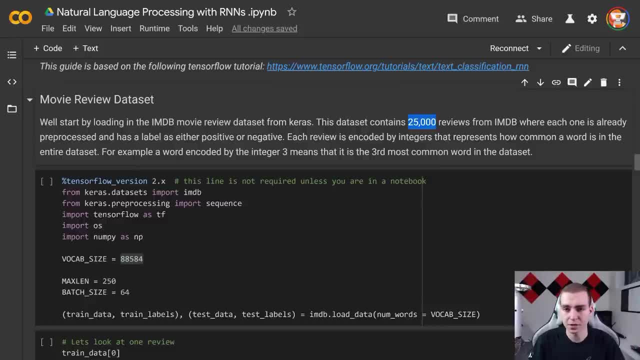 which are already pre processed and labeled. Now what that means for us is that every single word is actually already encoded by an integer, And in fact they've done kind of a clever encoding system where what they've done is said: if a character is encoded by, say, integer. 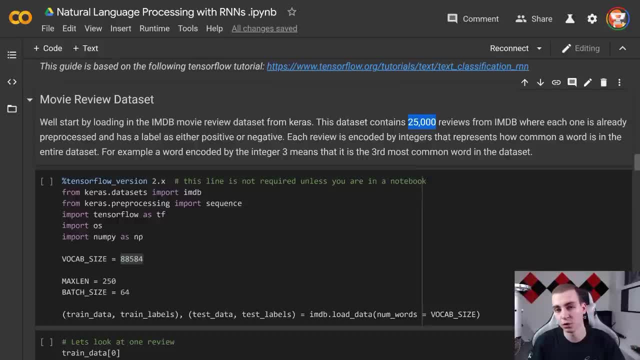 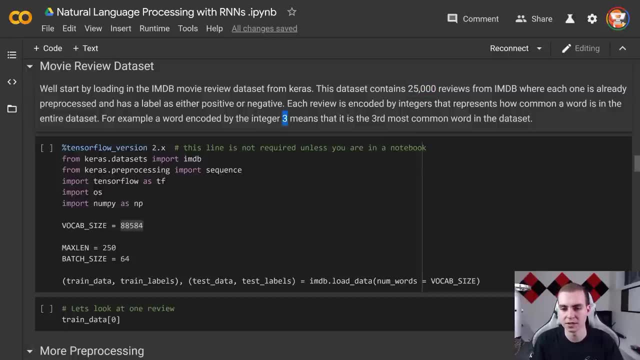 zero. that represents how common that word is in the entire data set. So if an integer was encoded by or non integer, a word was encoded by integer three, that would mean that it is the third most common word in the data set. And in this specific data set we 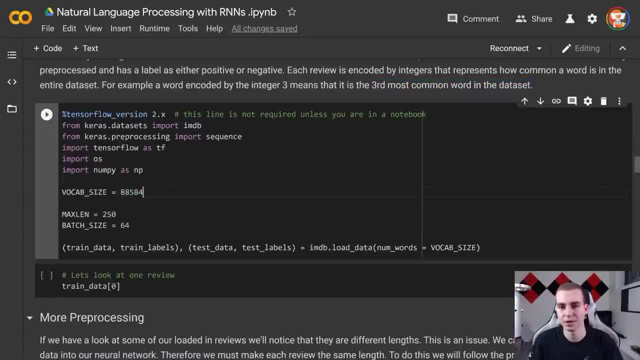 have vocabulary size of 88,584 unique words, which means that some of the words that we've encoded are actually encoded by an integer zero. So if an integer is something that was classified as this, so 88,584 would be the least common word in. 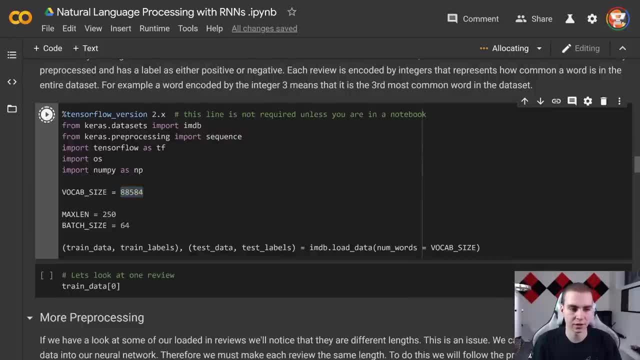 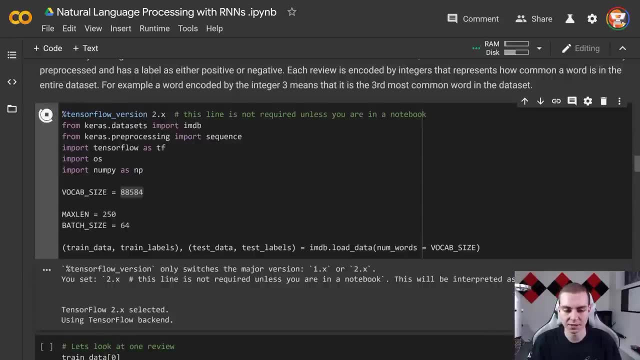 the data set. So something to keep in mind. we're going to load in the data set and do our imports just by hitting run here And, as I've mentioned previously, you know I'm not going to be typing this stuff out. it's just kind of a waste of time. I don't have 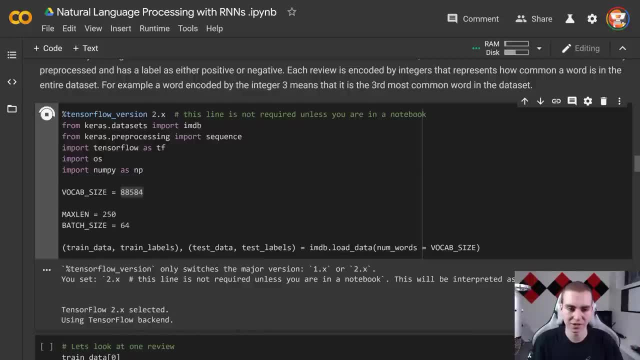 all the syntax memorized. I would never expect you guys to memorize this either, But what I will do is obviously walk through the code step by step and make sure you understand why it is that we have what we have here. Okay, 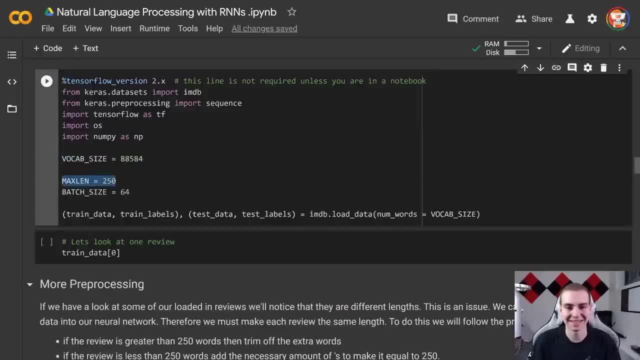 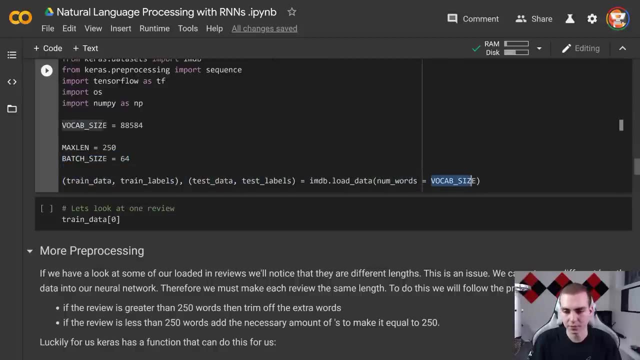 so what we've done is define the vocabulary size, the max length of a review and the batch size. Now what we've done is just loaded in our data set by defining the vocabulary size. So this is just the words that will include, So in this case, all of them. we have trained. 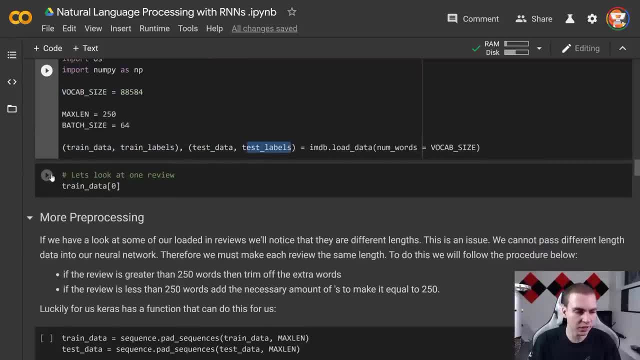 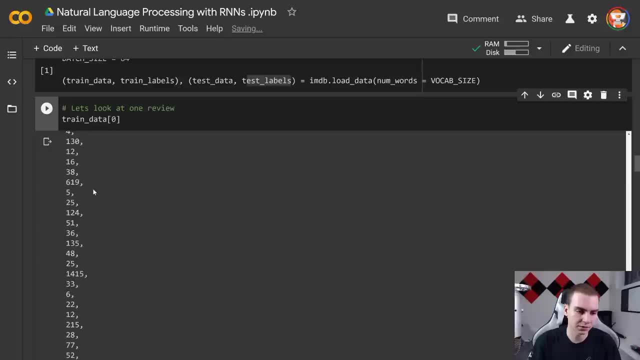 data, train labels, test data, test labels- And we can look at a review and see what it looks like by doing something like this. So this is an example of our first review. we can see kind of the different encodings for all of these words And this is what it looks. 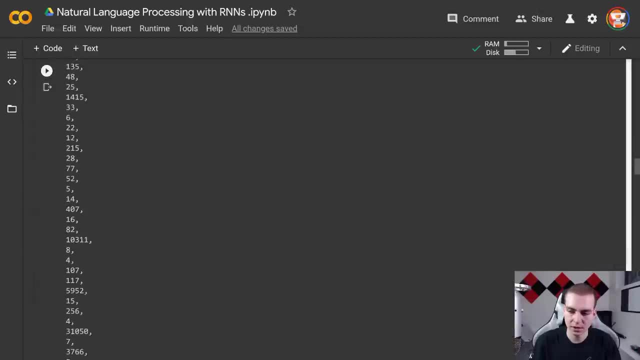 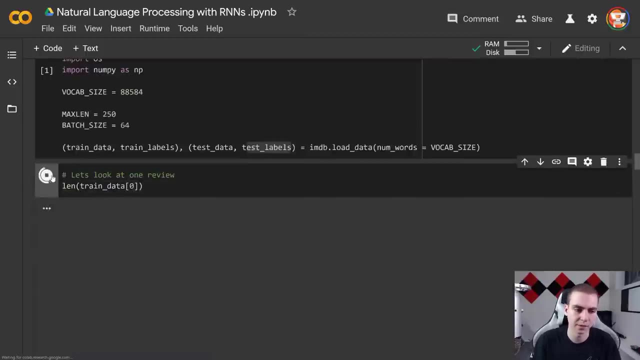 like they're already in integer form Now, just to give you a little bit of a preview. now, just something to note here is that the length of our reviews are not unique. So if I do the length of train data, I guess I wouldn't say unique, but I mean they're. 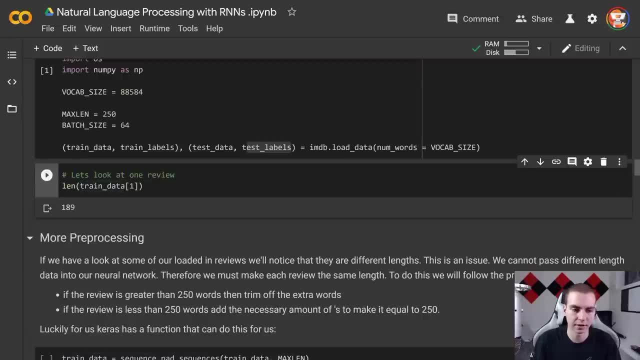 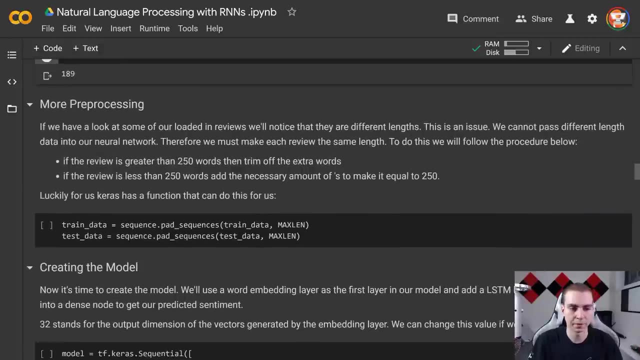 just all different. So the length of train data zero is different than the land of train data one right. So that's something to consider As we go through this and something we're actually going to have to handle. Okay, so more pre processing. So this is what I was. 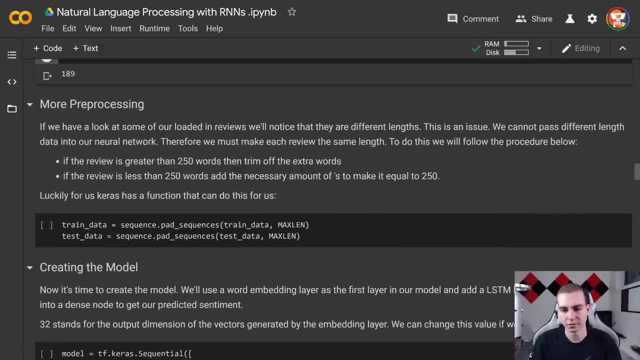 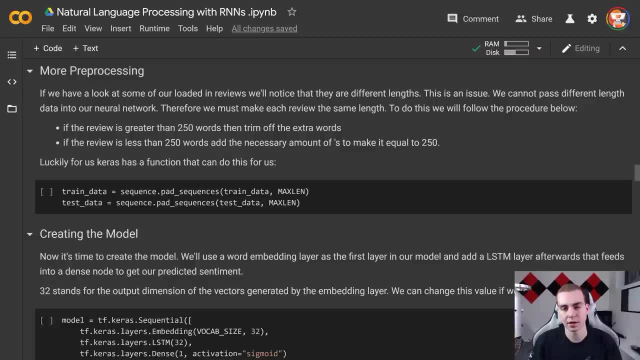 talking about. If you have a look at our loaded interviews, we'll notice they're of different lengths. this is an issue: we cannot pass different length data into our neural network, which is true. Therefore, we must make each review the same length. Okay, so what we're going to do for now is we're actually 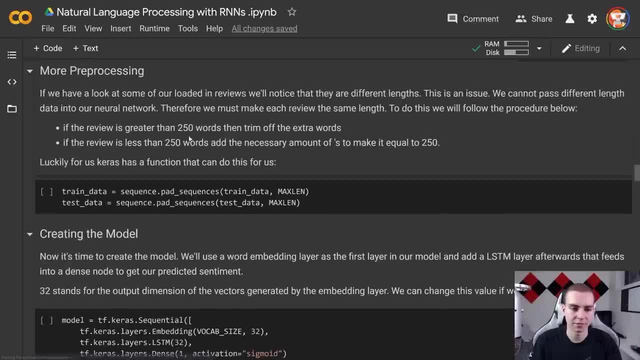 going to pad our sequences Now. what that means is we're going to follow this kind of step that I've talked about here. So if the review is greater than 250 words, we will trim off extra words. if the review is less than 250 words, we'll add the necessary amount. 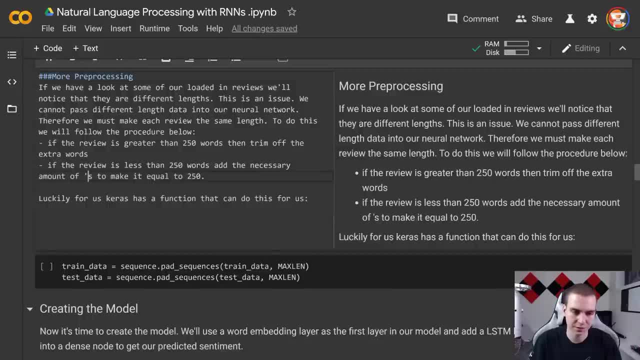 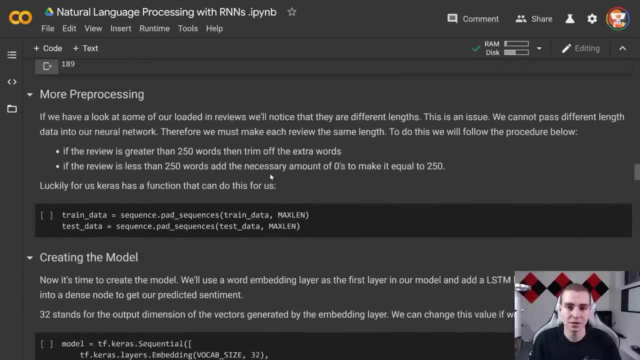 of this should actually be zeros in here. let's fix this of zeros to make it equal to 250.. So what that means is we're essentially going to add some kind of padding to our review. so in this case, I believe we're actually going to pad to the left side, which means 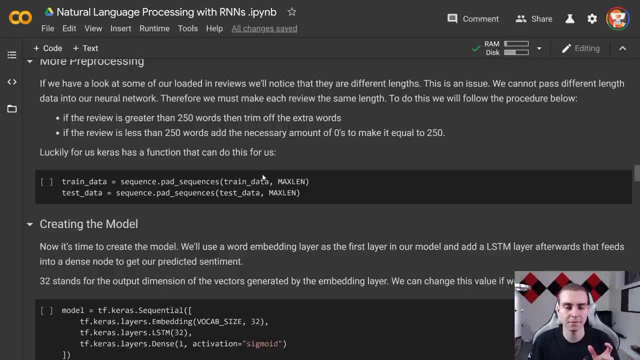 that say we have a review of length, you know 200, we're going to add 50, just kind of blank words which will represent, with the index zero to the left side of the review, to make it the necessary length. So that's, that's good, We'll do that. So if we look at train 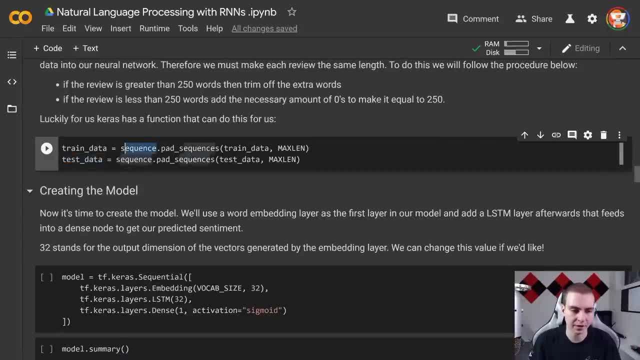 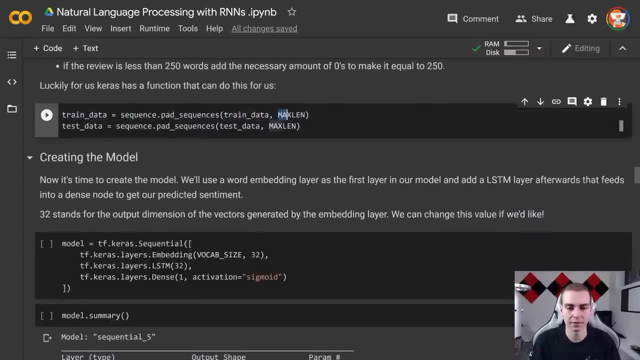 our index, And then we're going to add a new index to our index, And then we're going to say sequence, dot pad sequences, train data, and then we define the length that we want to pad it to. So that's what this will do. it will perform these steps that we've already. 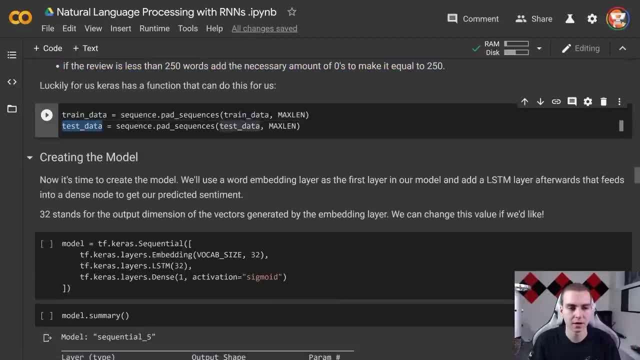 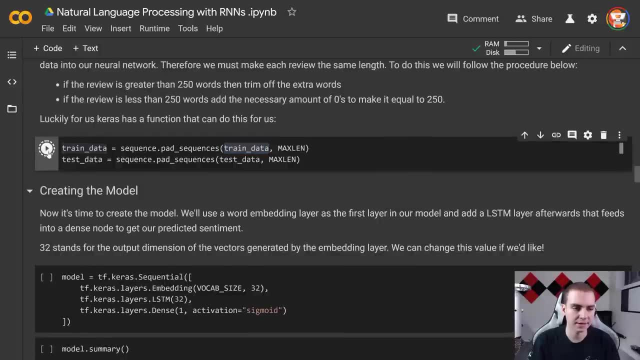 talked about, And again, we're just going to assign test data and train data to you know, whatever this does for us, we pass the entire thing. it'll pad all of them for us at once. Okay, so let's run that. And then let's just have a look at, say, train data. 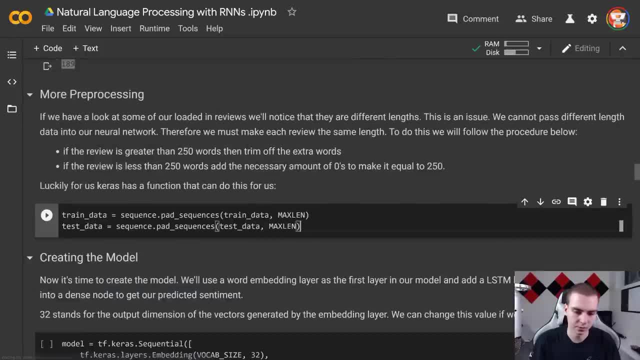 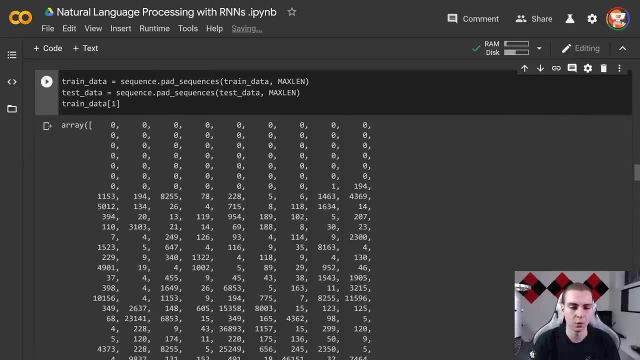 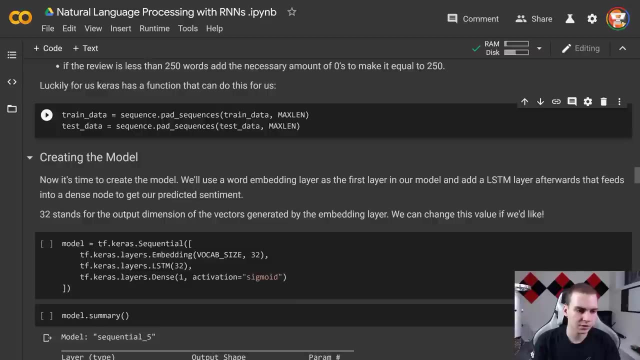 one now, because, remember, this was like 189.. Right, So if we look at train data, so train underscore data, one like that, we can see that as an array with a bunch of zeros before, because that is the padding that we've employed to make it the correct length. Okay, so that's. 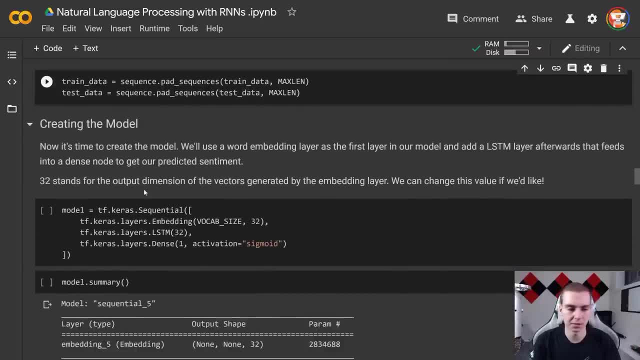 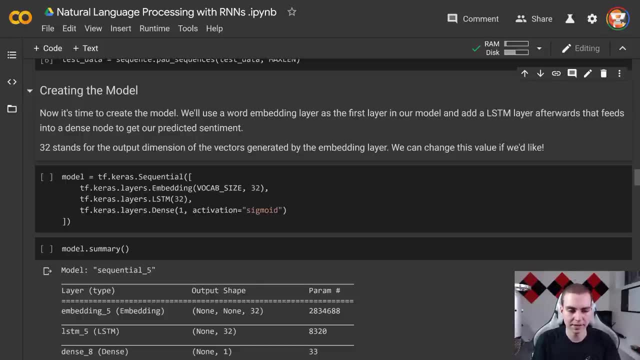 padding. That's something that we're probably gonna have to do most of the time when we feed something to our neural networks. Alright, so the next step is actually to create the model. Now, this model is pretty straightforward. we have an embedding layer and LSTM in a dense 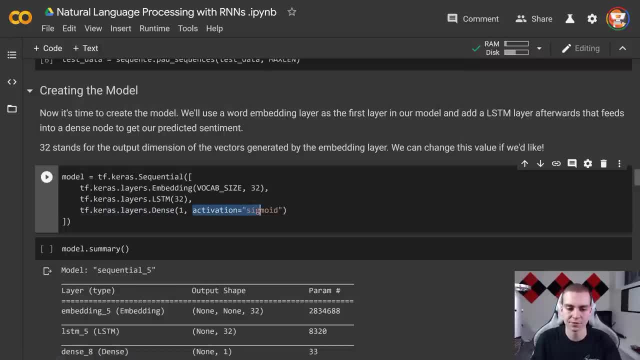 layer here. So the reason we've done dense with the activation function of sigmoid at the end is because we're trying to pretty much predict the sentiment of this right, which means that if we have the sentiment between zero and one, then if a number is greater than 0.5, we could classify. 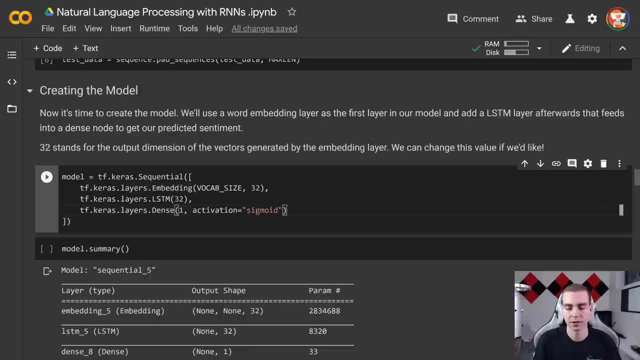 that as a positive review, And if it's less than 0.5, or equal, you know whatever you want to set the bounds at, then we can say that's a negative review. So sigmoid, as we probably might recall, squishes our values between zero and one. So whatever the value, 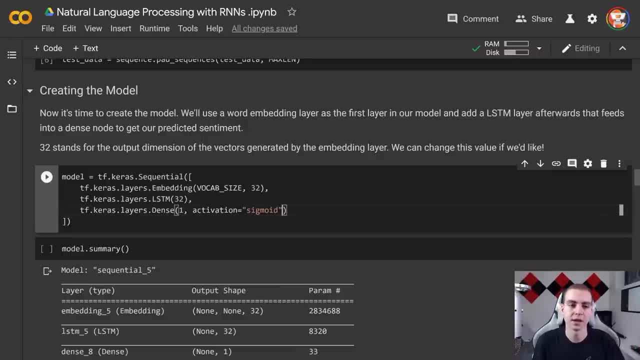 is at the end of the network will be between zero and one, which means that you know we can make the accurate prediction. Now here, the reason we have the embedding Larry, like well, we've already pre processed our review- is even though we've pre processed this with these integers and they are a bit 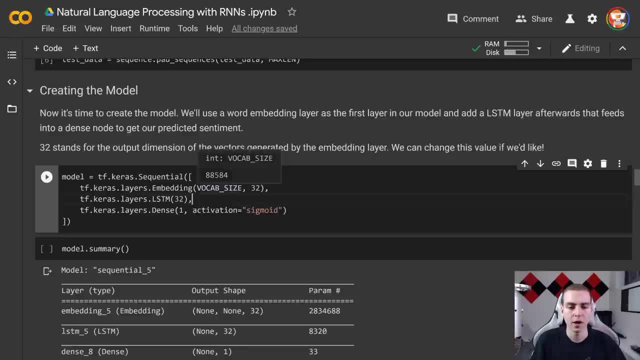 more meaningful than just our random lookup table that we've talked about before. we still want to pass that to an embedding layer which is going to find a way more meaningful representation for those numbers than just their integer values already. So it's going to create those. 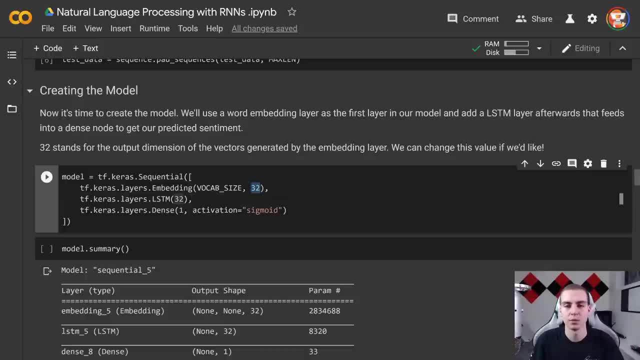 vectors for us, And this 32 is denoting the fact that we're going to make the output of every single one of our embeddings or vectors that we're going to use to create those vectors. So we're going to create those vectors for us, And this 32 is denoting the fact that. 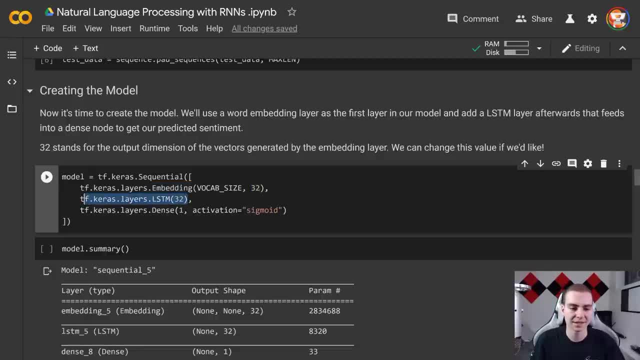 are created 32 dimensions, which means that when we pass them to the LSTM layer, we need to tell the LSTM layer it's going to have 32 dimensions for every single word, which is what we're doing, And this will implement that long, short term memory process we talked. 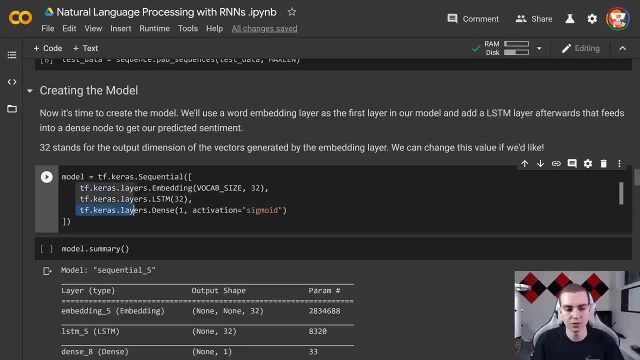 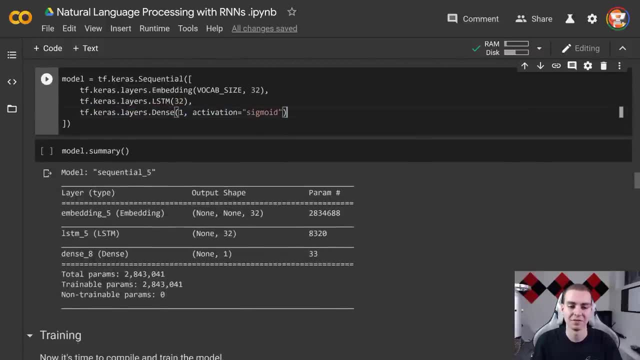 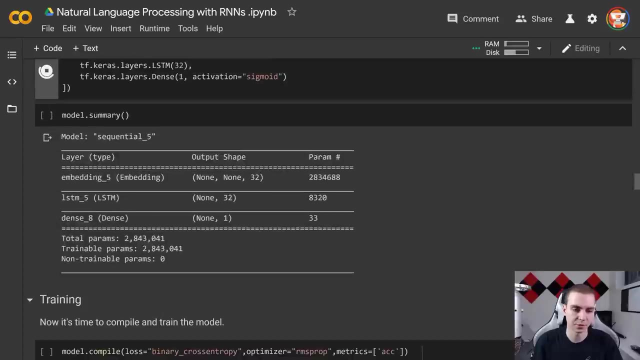 about before and output the final output to tf, dot, keras, dot layers, dot, dense, which will tell us: you know that's what. this is right. It'll make the prediction. So that's what this model is. We can see. let's give this a second to run. here the model summary, which is already printed out: 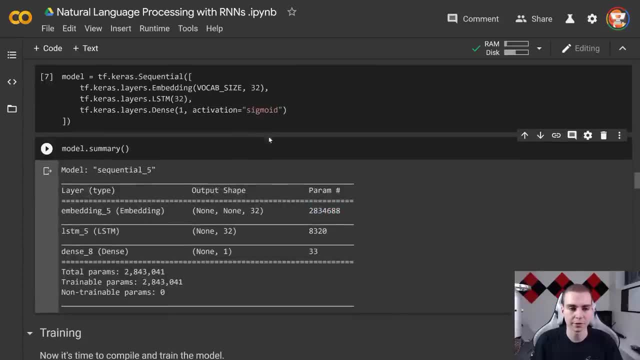 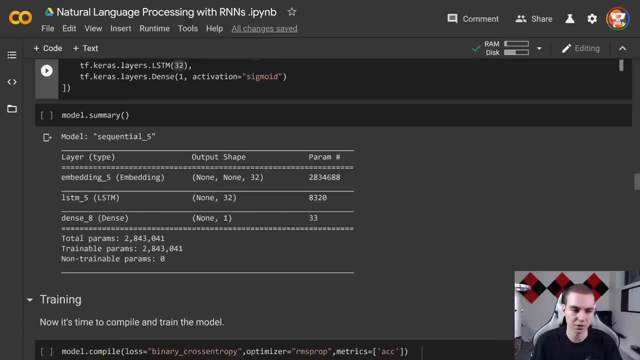 we can look at the fact that the embedding layer actually has the most amount of parameters, because essentially it's trying to figure out, you know, all these different numbers. how can we convert that into a tensor of 32 dimensions, which is not that easy to do? 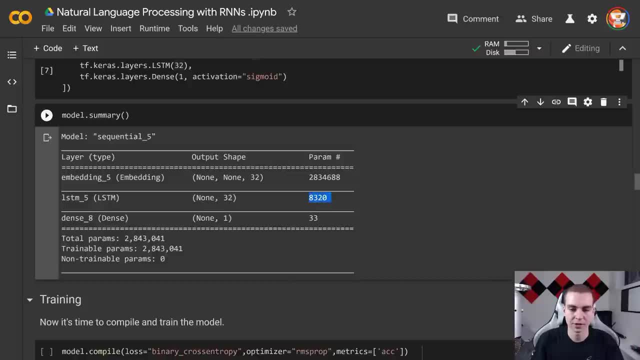 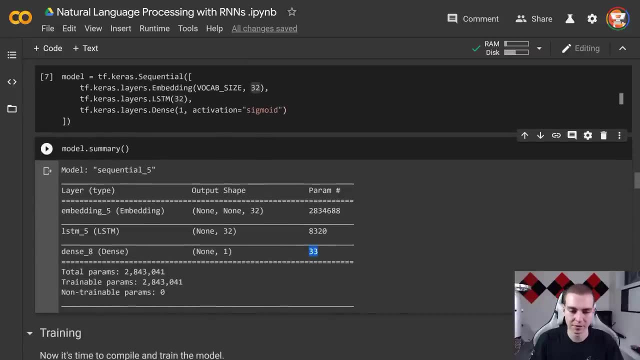 And this is going to be the major aspect that's being trained. And then we have our LSTM layer. we can see the parameters there And our final dense layer, which is eight, getting 33 parameters. That's because the output from every single one of these dimensions 32 plus a bias node. 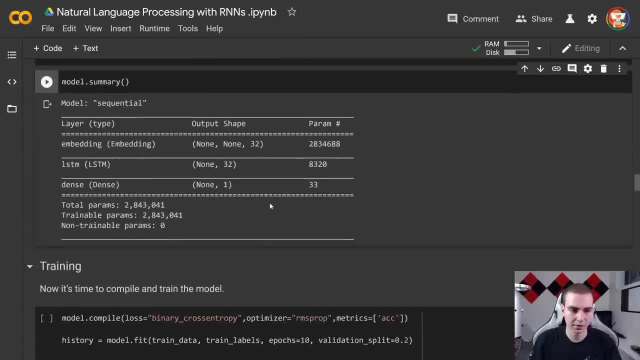 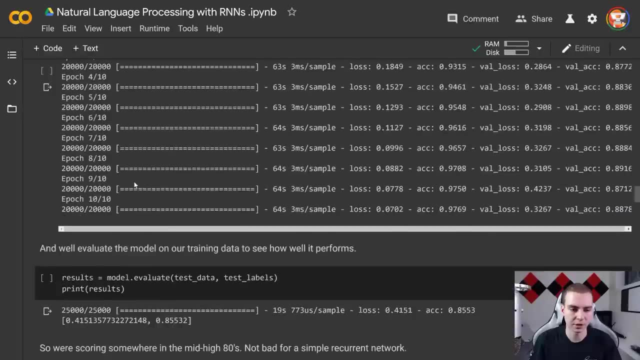 right that we need. So that's what we'll get there. You can see model dot summary. we get the sequential model. Okay, so training. So now it's time to compile and train the model. you can see, I've already trained mine. what I'm going to say here is: if you want, 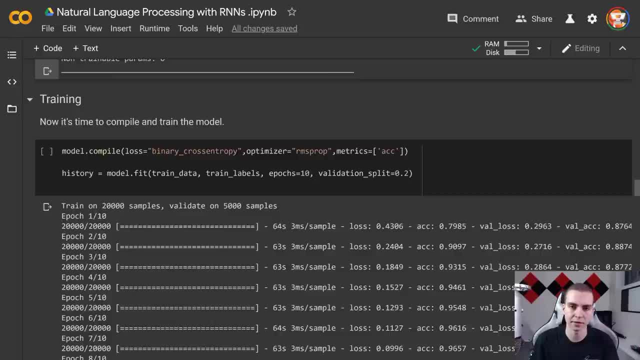 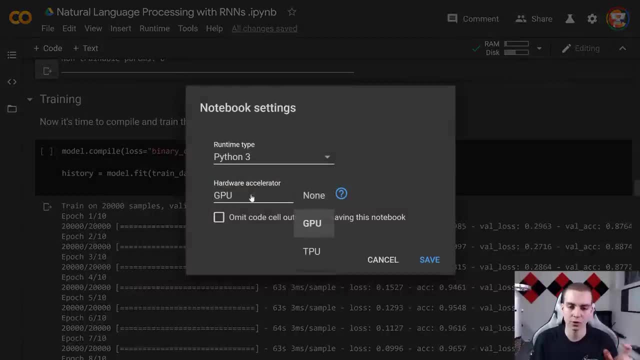 to speed up your training- because this will actually take a second, and we'll talk about why we pick these things in a minute- is go to runtime, change runtime type and add a hardware accelerator of GPU. What this will allow you to do is utilize a GPU while you're. 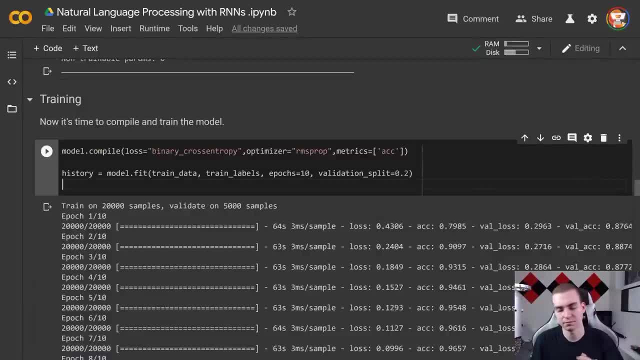 training, which should speed up your training. So we're going to go ahead and do that. So we're going to go ahead and do our training by about 10 to 20 times. So I probably should have mentioned that beforehand, But you can do that, And please do for these examples. 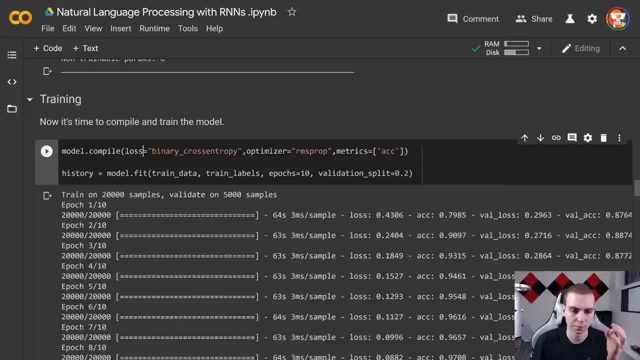 So model dot compile, Alright. so we're compiling our model. we're picking the loss function as binary cross entropy. The reason we're picking this is because this is going to essentially tell us how far away we are from the correct probability right, Because we have two different. 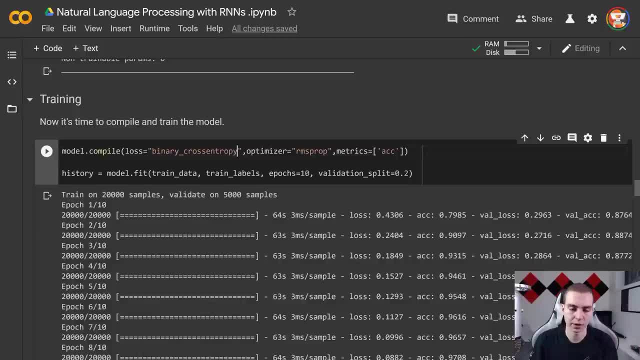 things we could be predicting. So you know either zero or one, so positive or negative. So this will give us a correct loss For that kind of problem that we've talked about before. the optimizer: we're gonna use RMS prop again. I'm not going to discuss all the different optimizers. you can look 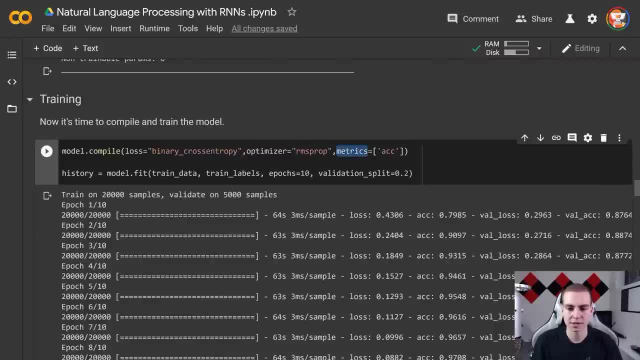 them up if you care that much about what they do, And we're going to use metrics as ACC. One thing I will say is the optimizer is not crazy important For this one. you could use Adam if you wanted to, and it would still work fine. My usual go to is just use the. 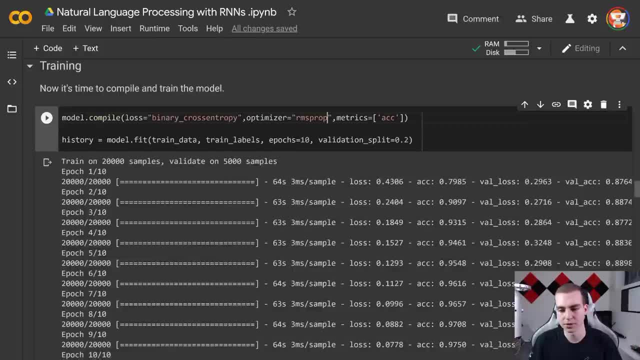 atom optimizer, unless you think there's a better one to use. But anyways, that's something to mention. Okay, so finally, we will fit the model. we've looked at the syntax a lot before, So let's go ahead and do that. So we're going to go ahead and do that, So let's. 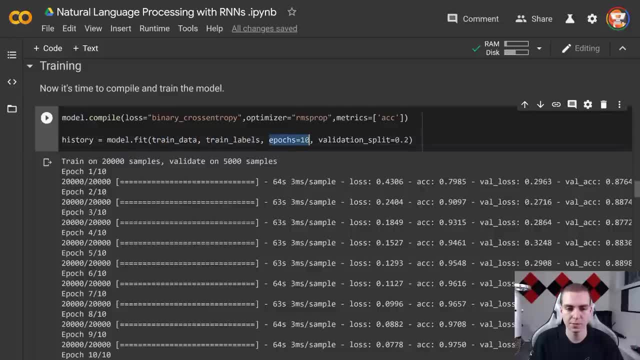 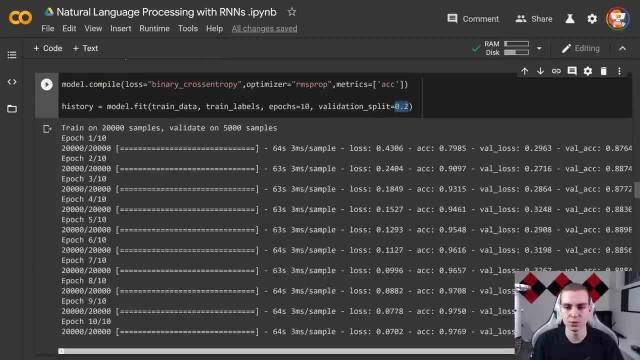 model that fit. we have the training data, the training labels, the epochs, and we'll do a validation split of 20%. So that's what 0.2 stands for, which means that what we're going to be doing is using 20% of the training data to actually evaluate and validate the. 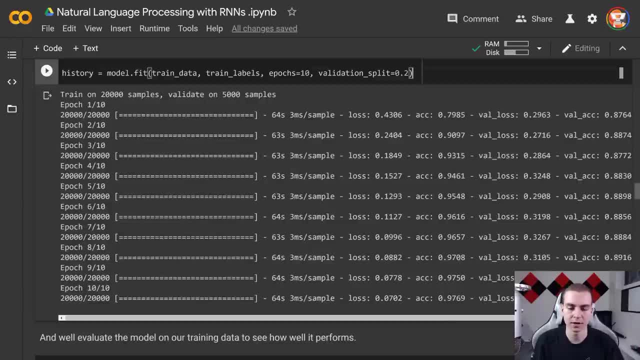 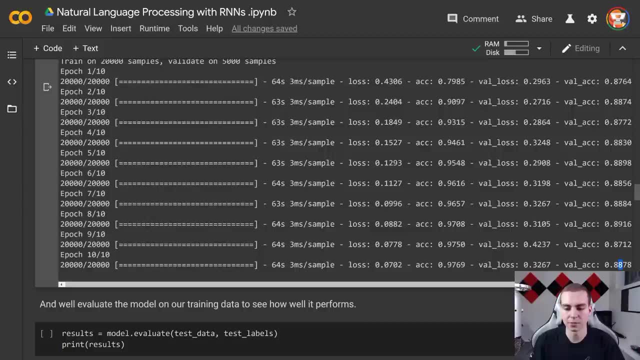 model as we go through And we can see that after training- which I've already done and you guys are welcome to obviously do on your own computer- we kind of stall at an evaluation accuracy of about 88%, Whereas the model actually gets overfit to about 97- 98%. So what this? 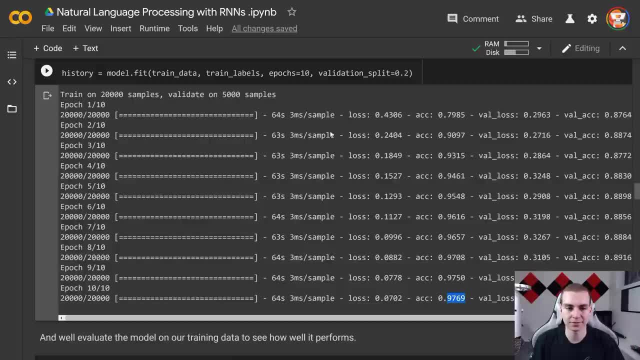 is telling us essentially is that we don't have enough training data And that, after we've even done just one epoch, we're pretty much stuck on the same validation accuracy and that there's something that needs to change in the model to make it better. But for now, 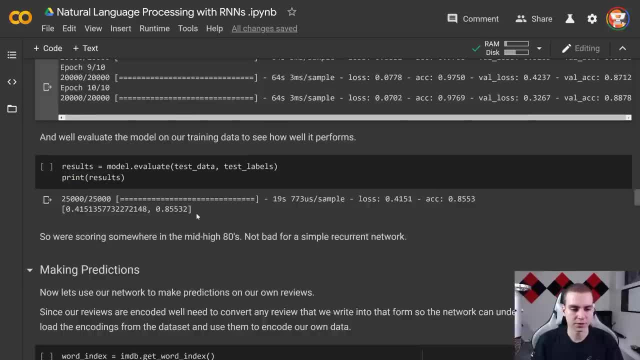 that's fine, we'll leave it the way that. it is Okay. so now we can look at the results. I've already did the results here, just to again speed up some time, but we'll do the evaluation on our test data and test labels to get a more accurate kind of result here. 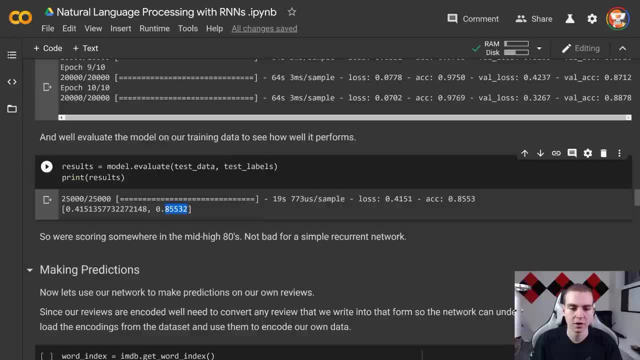 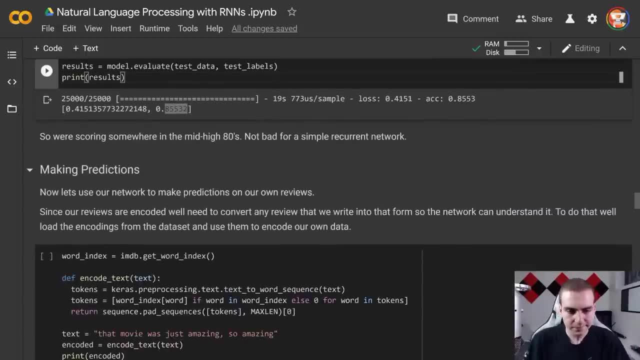 And that tells us we have an accuracy of about 85 point 5%, Which you know isn't going to be great, but it's decent considering that we didn't really write that much code to get to the point that we're at right now. Okay, so that's what we're getting the models been. 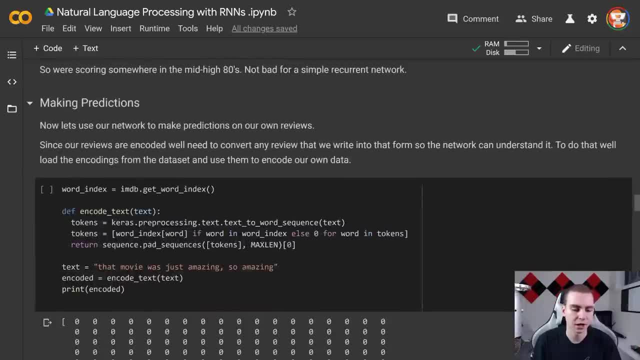 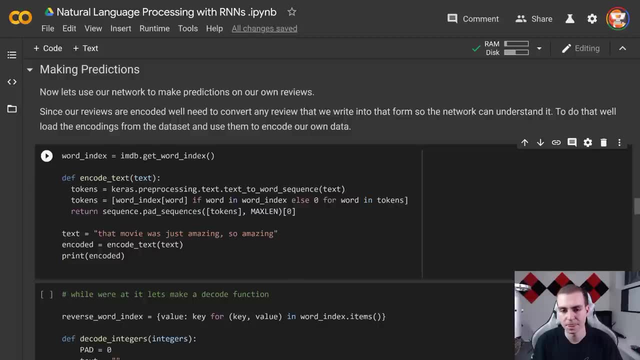 trained Again, it's not too complicated, And now we're on to making predictions. So the idea is that now we've trained our model and we want to actually use it to make a prediction on some kind of movie review. So, since our data was pre processed when we gave it to 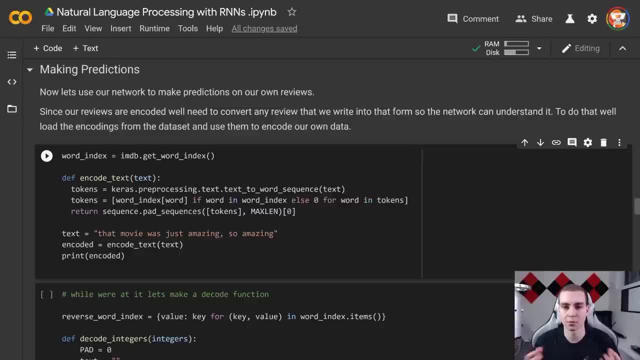 the model. that means we actually need to process anything we want to make a prediction on in the exact same way. we need to use the same lookup. We need to use the exact same lookup table. we need to encode it. you know precisely the same. Otherwise, when we give 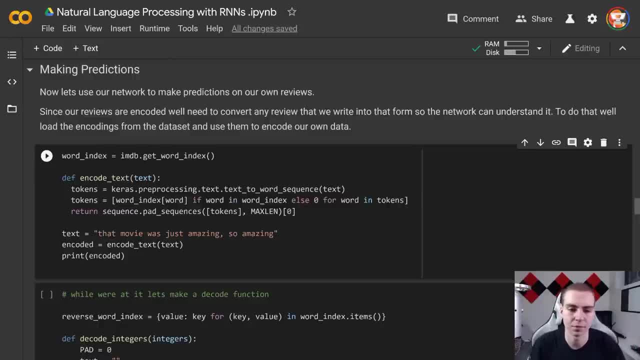 it to the model, it's going to think that the words are different and it's not going to make an accurate prediction. So what I've done here is I've made a function that will encode any text into what do you call it? the proper pre processed kind of integers, right? 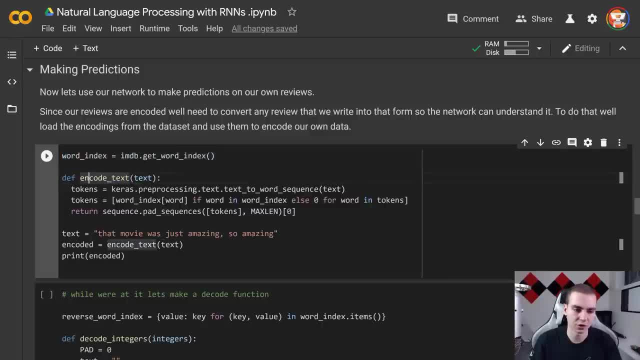 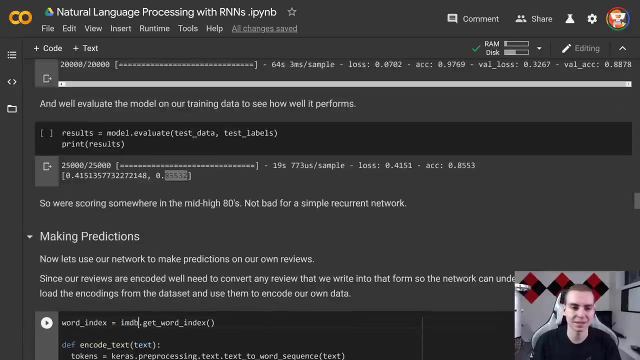 Just like our training data was pre processed. That's what this function is going to do for us is pre process some line of text. So what I've done is actually got in the lookup table. So essentially the mappings from IBM, IB, IMDb- I could read that properly from that data set that. 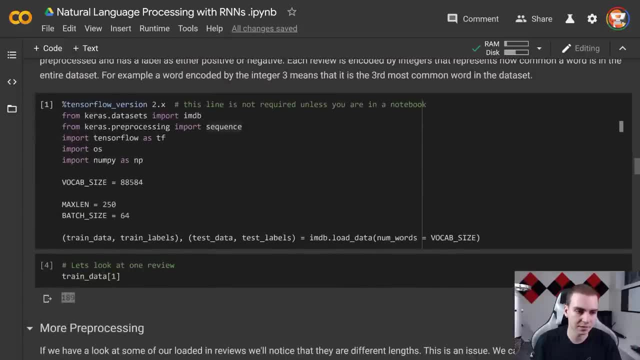 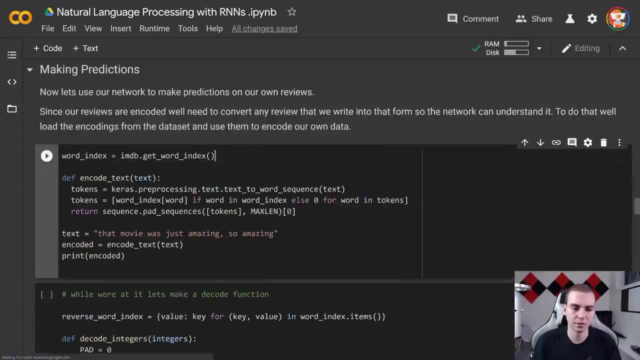 we loaded earlier. So let me go see if I can find where I defined IMDb. You can see up here. So Kara's dot data sets import IMDb. Just like we loaded it in, we can also actually get all the word indexes or that map. we can actually print this out if we want to look. 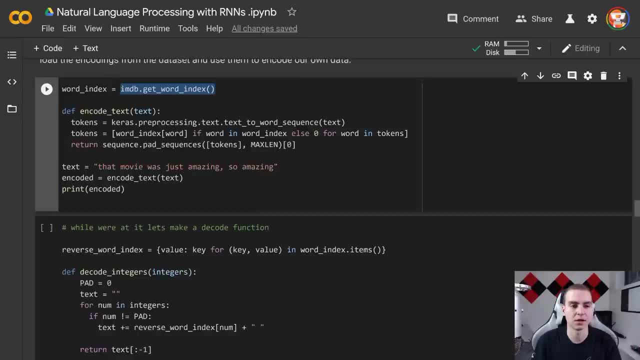 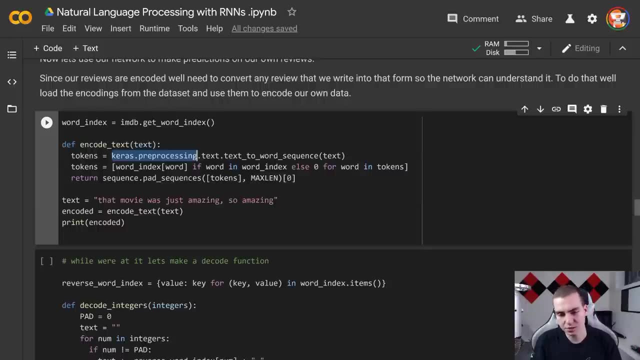 at what it is after. But anyways, we have that mapping, which means that all we need to do is Kara's pre processing dot text, dot text to word sequence. what this means is: give given some text, convert all that text into what we call tokens, which are just the individual words themselves. And then what? 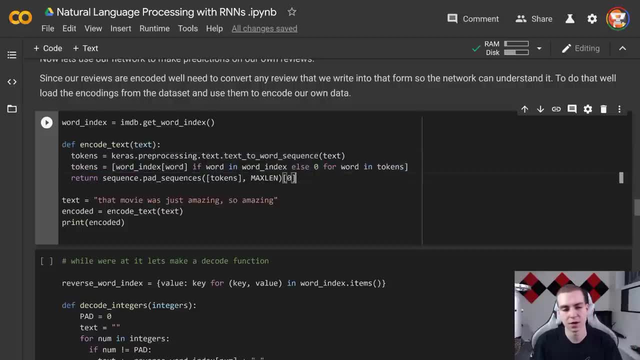 we're going to do is just use a kind of for loop inside of here that says word index at word, if word in word, index l zero for word and tokens. Now what this means is essentially if the word that's in these tokens now is in our mapping. so in that vocabulary of 88,000. 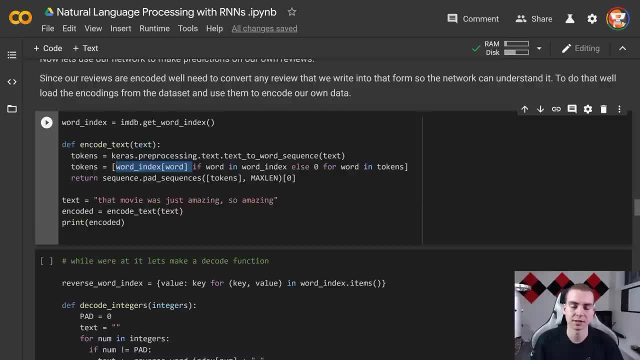 words, then what we'll do is replace its location in the list with that specific word or with that specific integer that represents it. Otherwise we'll put zero just to stand for you know, we don't know what this character is, And then what we'll do is return sequence. 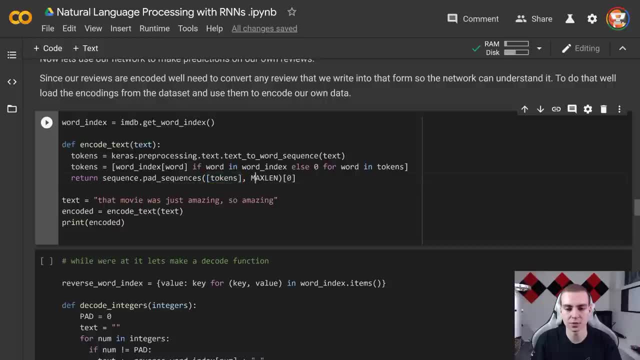 dot pad sequences And we'll pad this token sequence and just return- actually the first index here. The reason we're doing that is because this pad sequences works on a list of sequences, so multiple sequences, So we need to put this inside a list. 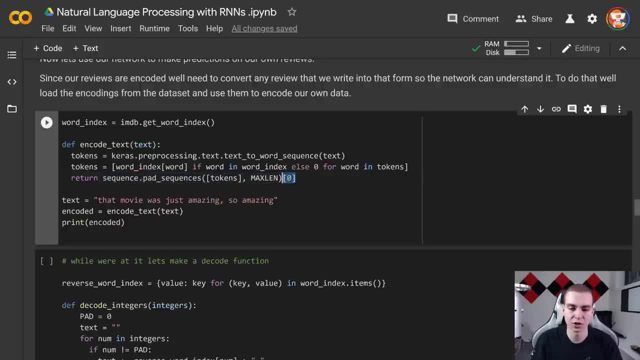 Which means that this is going to return to us a list of lists. So we just obviously want the first entry, because we only want, you know, that one sequence that we padded. So that's how this works. Sorry, that's a bit of a mouthful to explain, But you guys. 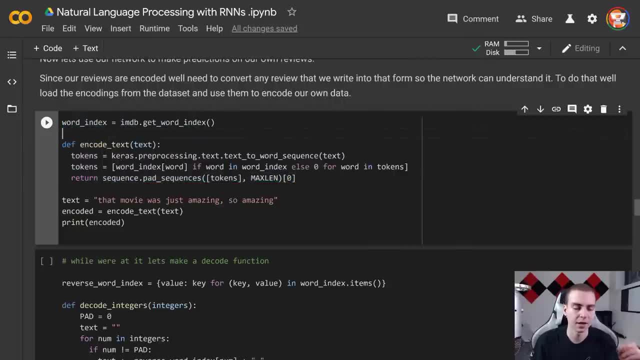 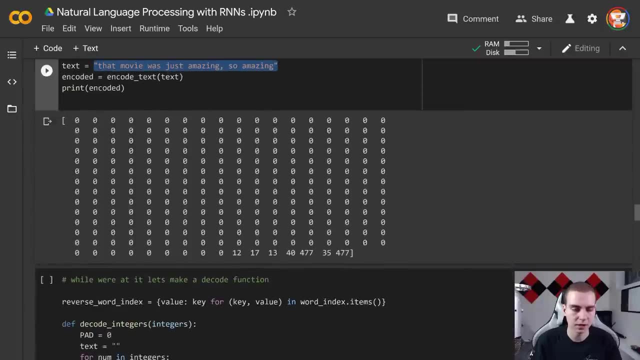 can run through and print this stuff out if you want to see how all of it works specifically. But yeah, so we can run this cell and have a look at what this actually does for us on some sample text. So that movie was just amazing, So amazing. We can see we get the output that. 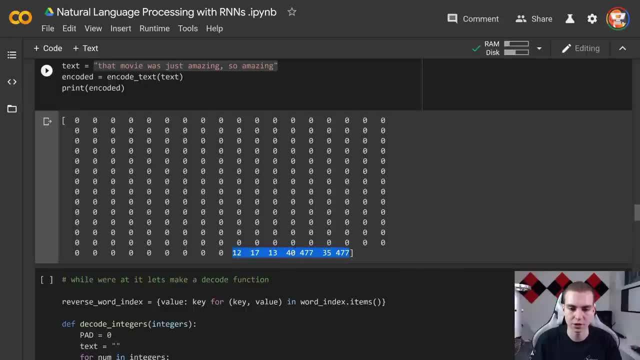 we were kind of expecting. So integer, encoded words down here and then a bunch of zeros just for all the padding. Now, while we're doing this, we're going to go ahead and run this. So we're going to go ahead and run this. So we're going to go ahead and run this. 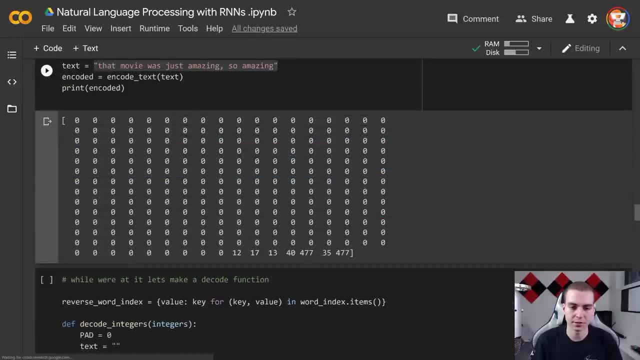 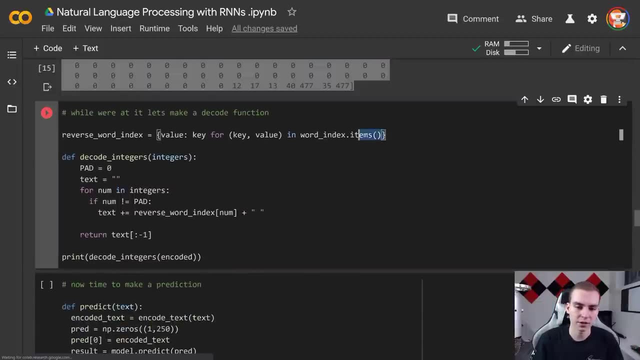 Now, while we're at it, I decided: why not? why don't we make a decode function so that if we have any movie review like this that's in the integer form, we can decode that into the text value? So the way we're going to do that is start by reversing the word index. 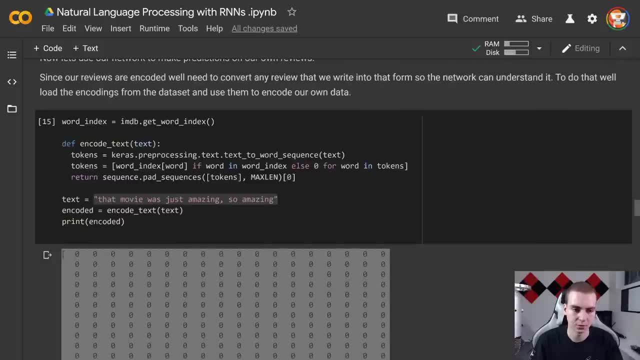 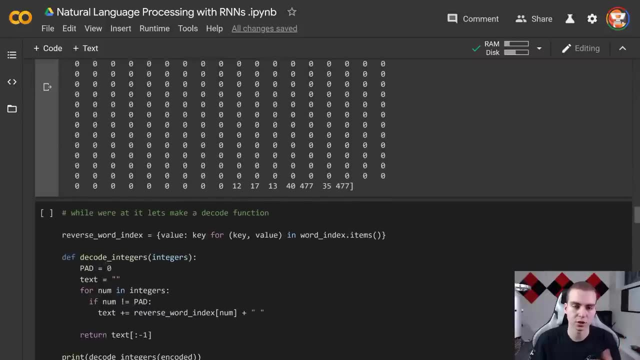 that we just created. Now, the reason for that is the word index we looked at, which is this: right goes from word to integer. But we actually now want to go from integer to word so that we can actually translate a sentence right. So what I've done is made. 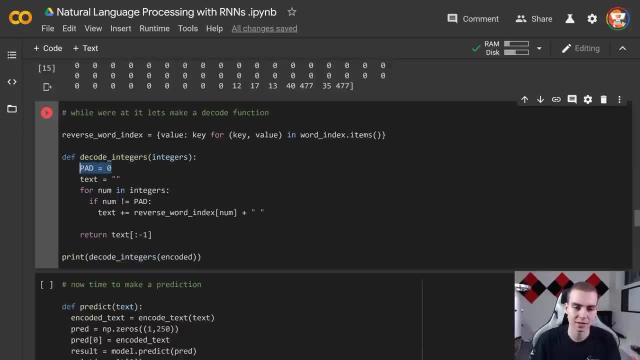 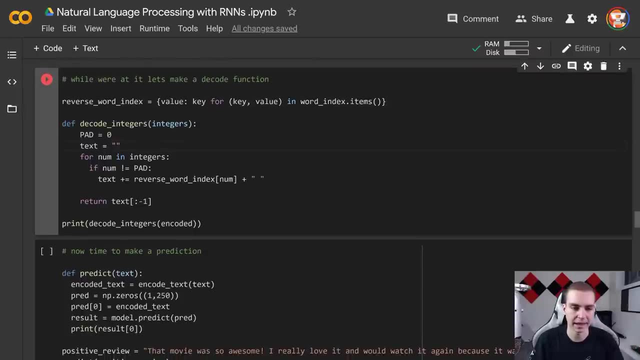 this decode integers function. we've set the padding key as zero, which means that if we see zero, that's really just means you know nothing's there. we're going to create a text string which we're going to add to. then I'm going to say: 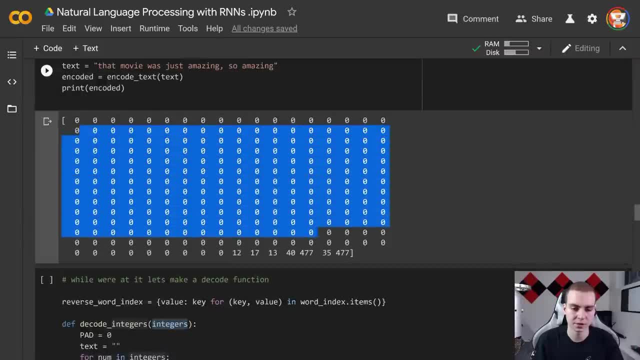 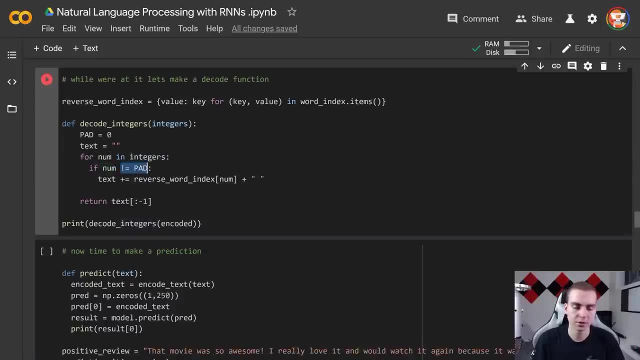 for num in integers. integers is our input, which will be a list that looks something like this, or an array, whatever you want to call it. we're gonna say: if number does not equal pad, so essentially, if the number is not zero, right, it's not padding, then 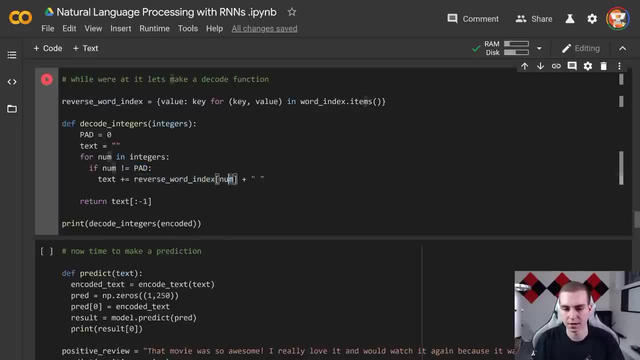 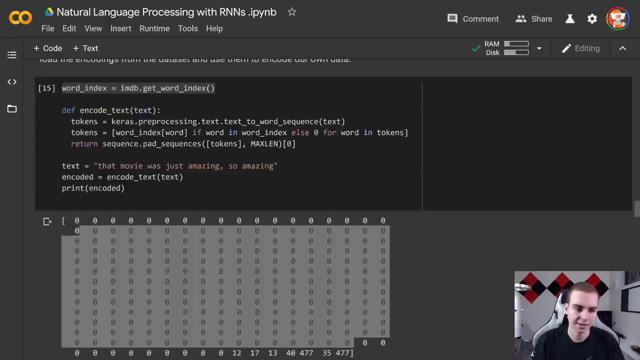 what we'll do is add the lookup of reverse word index num, So whatever that number is- into this new string plus a space, and then just return text colon, negative one, which means return everything except the last space that we would have added. And then, if I print the decode integers, we can see that this encoded thing 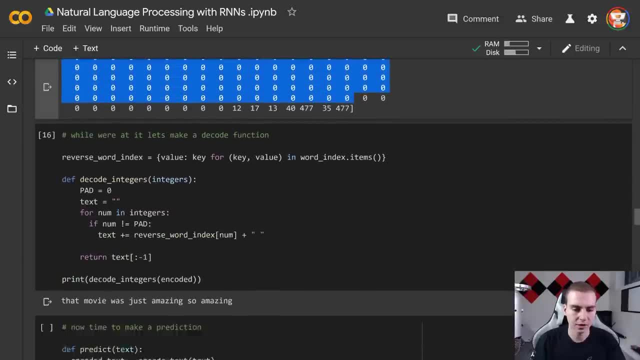 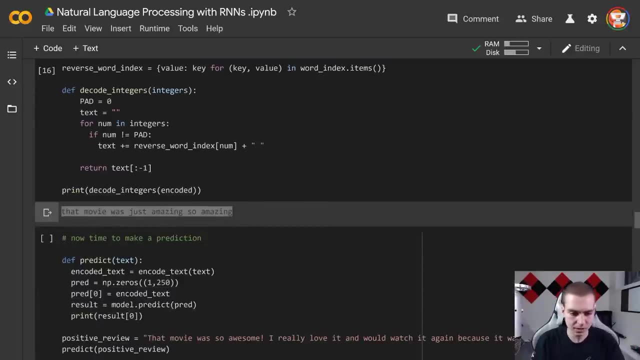 that we have before, which looks like this: gets encoded by the string. that movie was just amazing, So may sorry, not encoded- decoded because this was the encoded form. So that's how that works, Okay, so now it's time to actually make a prediction, So I've written: 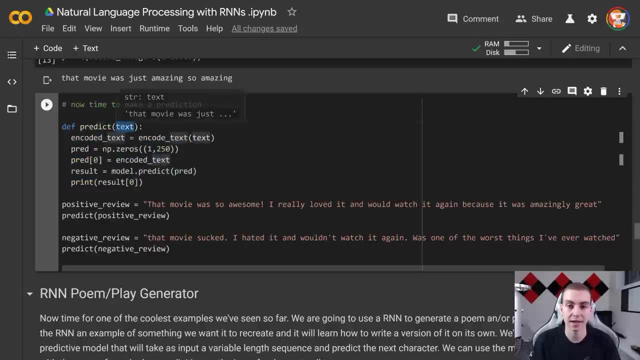 a function here that will make a prediction on some piece of text, as the movie reveals- and I'm going to do a movie review for us And I'll just walk us through quickly how this works. then I'll show us the actual output from our model. you know, making predictions. 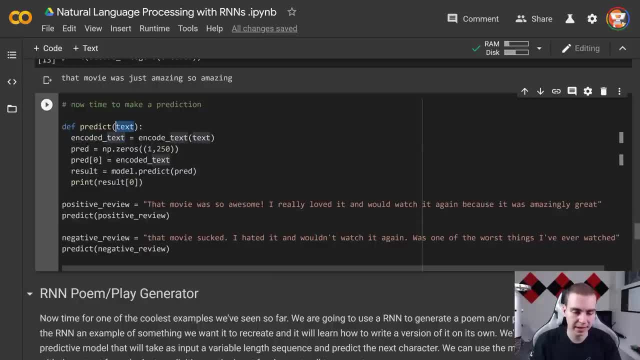 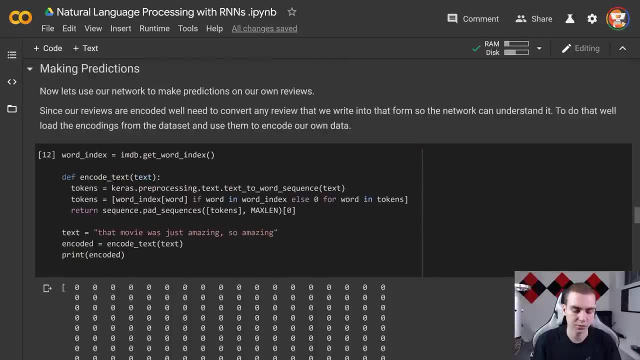 like this. So what we say is: we'll take some parameter text, which will be our movie review, And we're going to encode that text using the encode text function we've created above. So just this one right here. that essentially takes our sequence of you know words we'd 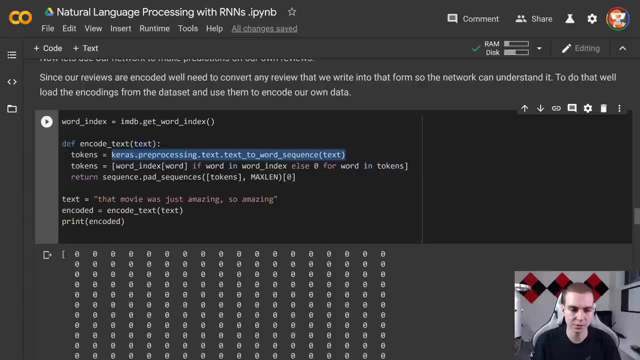 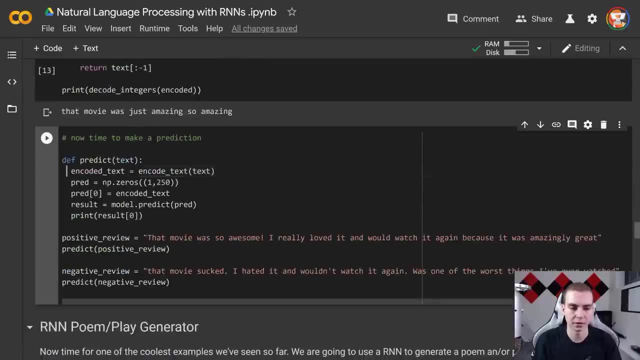 get the pre processing, So turn that into a sequence. remove all the spaces, whatnot you know. get the words, then we turn those into the integers. we pad that, we return that. So here we have our proper pre process text. then what we do is we create a blank. 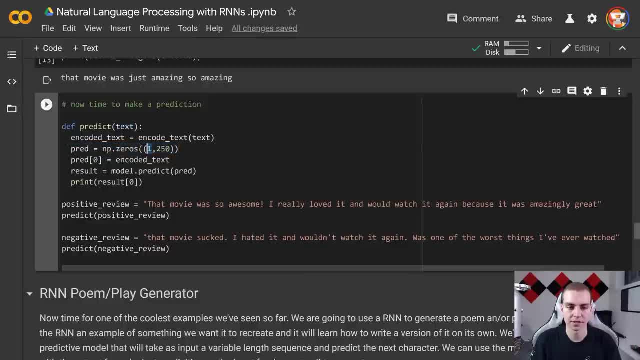 NumPy array that is just a bunch of zeros. that's in the form one to 50, or in that shape. Now, the reason I'm putting that in that shape is because the shape that our model expects is something 250,, which means some number of entries and then 250 integers representing 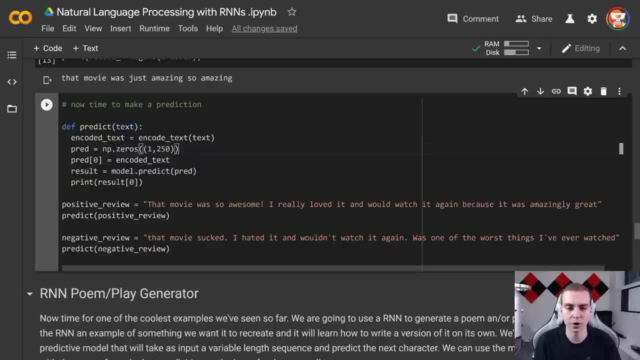 each word right, because that's the length of movie review is what we've told. the model is length 250.. So that's the length of the review. then what we do is we put pred zero. so that's what's up here equals the encoded text. So we just essentially insert our one. 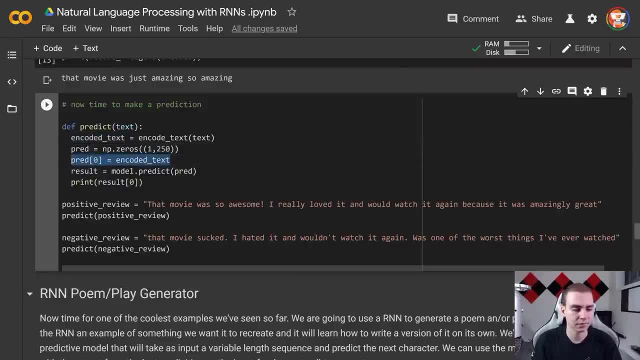 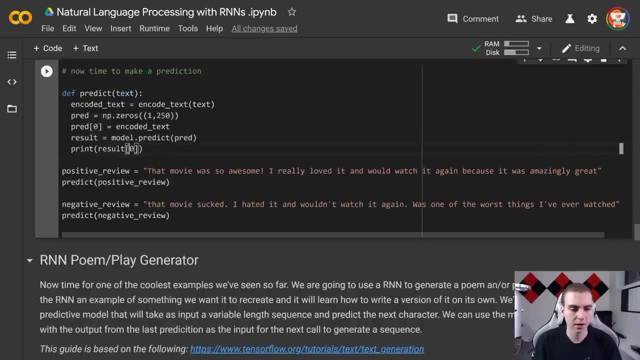 entry into this, this array we've created. then what we do is say model dot, predict on that array and just return and print the result zero. Now, that's pretty much all there is to it. I mean, that's how it works. The reason we're doing result zero is because 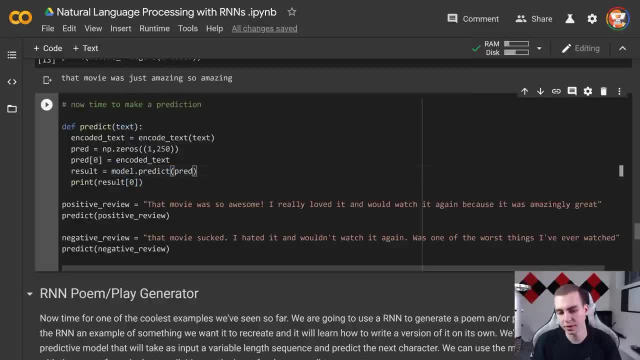 again, model is optimized To predict on multiple things, which means, like I would have to do, you know, list of encoded text, which is kind of what I've done by just doing this prediction lines here, which means it's going to return to me an array of arrays. So if I want the first prediction, 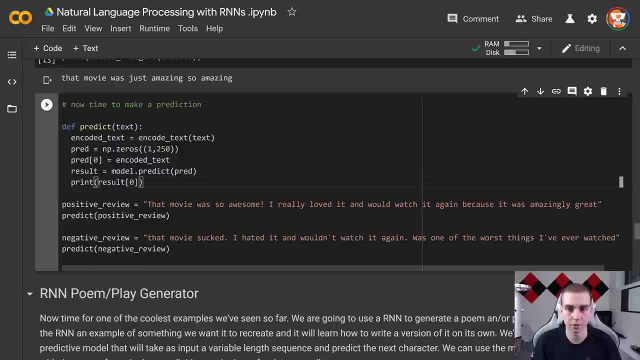 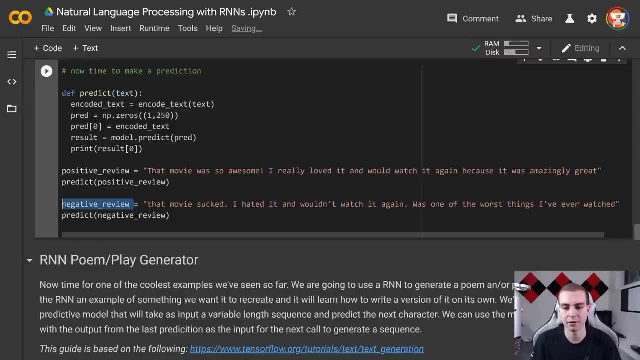 I need to index zero, because that will give me the prediction for our first and only entry. Alright, so I hope that makes sense. Now we have a positive review of written and a negative review, And we're just going to compare the analysis on both of them. So that movie was 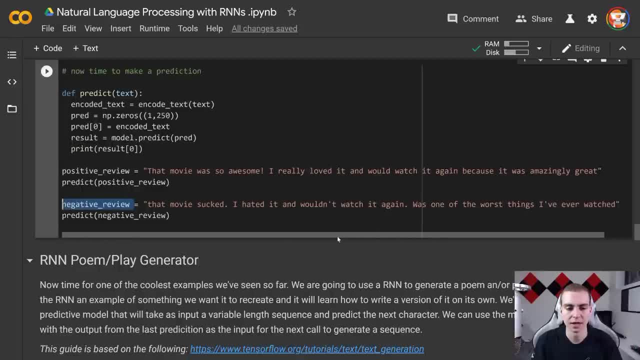 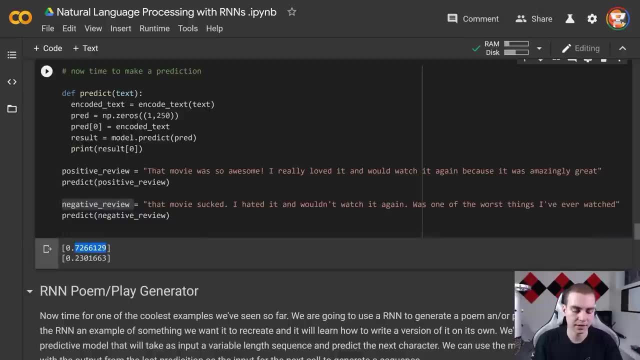 so awesome. I really loved it. I would watch it again because it was amazingly great. And then that movie sucked. I hated it and wouldn't watch it again, was one of the worst things I've ever watched. So let's look at this now And we can see. the first one gets predicted at 72% positive, whereas 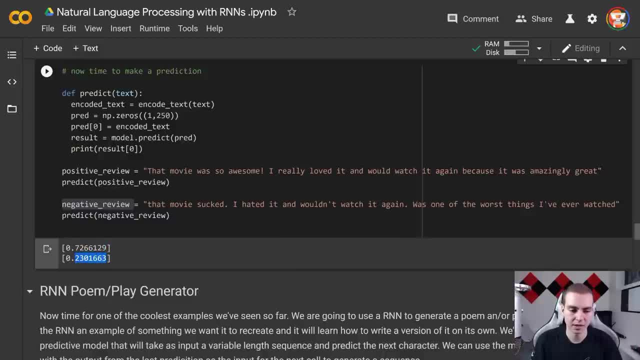 the other one is 23% positive. So essentially what that means is that you know if the lower the number, the more negative we're predicting it is, the higher the number, the more positive we're predicting it is. if we wanted to not just print out this value And instead what 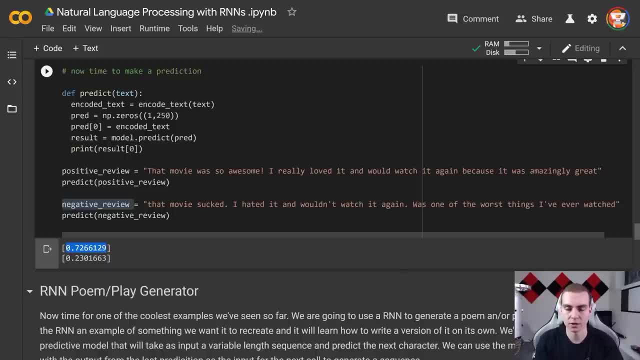 we wanted to do was print out, you know, positive or negative. we could just make a little. if it says: if this number is greater than 0.5, say positive. otherwise say not, say negative. right, And I just want to show you that changing these reviews ever so slightly actually makes. 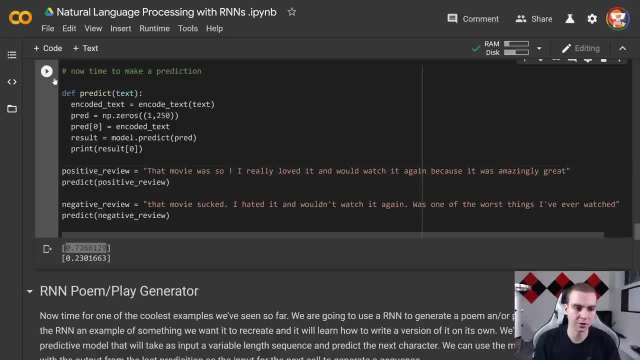 a big difference. So if I remove the word awesome, so that movie was so- and then I run this, you can see that oh, wow, this actually increases and goes up to 84%, Right, So the presence of certain words in certain locations actually makes a big difference, And especially 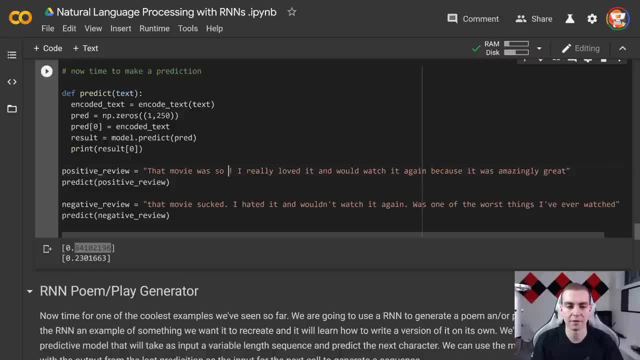 when we have a shorter length review, right, If we have a logger length review won't make that big of a difference. But even the removal of a few words here- and let's see so the removing the word awesome- changed it by almost like 10% Right Now. 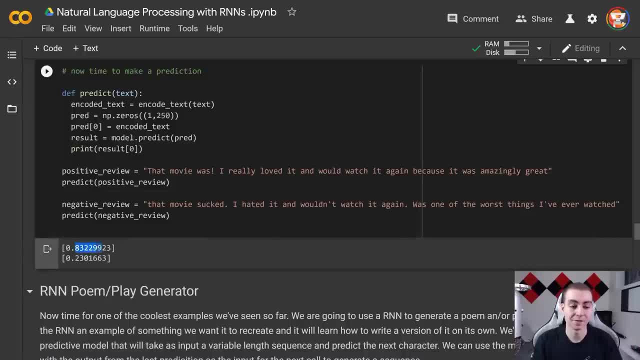 if I move so let's see if that makes a bigger difference. It makes a very little difference because it's learned, at least the model right, that the word so doesn't really make a huge impact into the type of review, Whereas if I remove the word I, let's see if that makes. 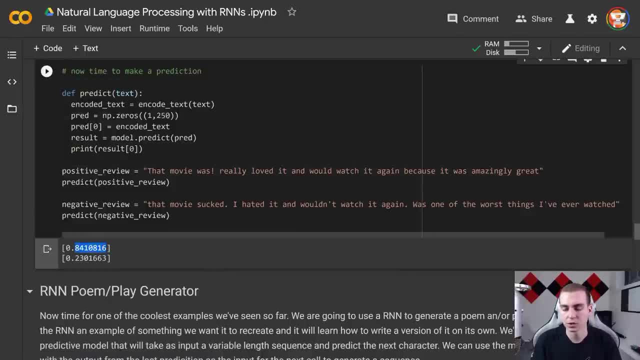 a big impact? Probably not right now. it goes back up to 84.. So that's cool And that's something to play with is removing certain words and seeing how much impact those actually carry. And even if I just add the word great, like would great. 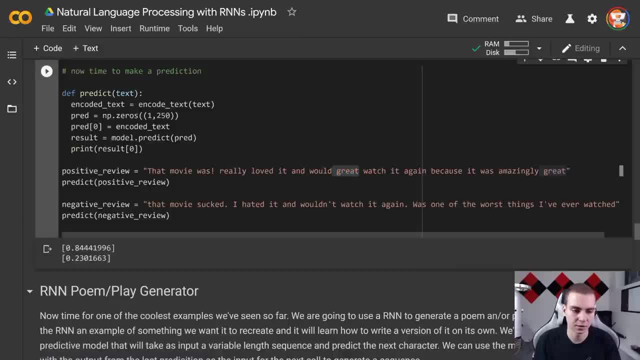 watch it again just in the middle of the sentence doesn't have to make any sense. Let's look at this here: Oh boom, we increase like a little bit right. And let's say: if I add this movie, you really suck. Let's see if that makes a difference. No, that just reduces. 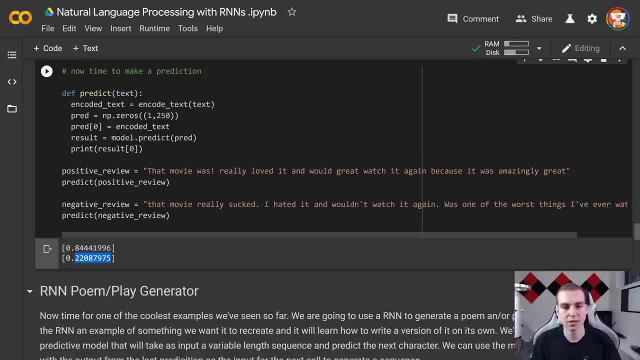 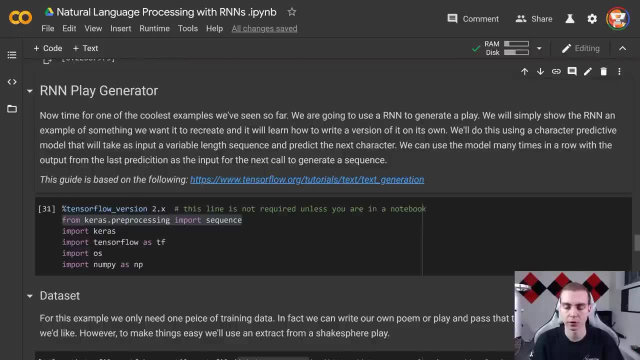 it like a tiny bit. So something cool, something to play with. Anyways, now let's move on to the next example. So now we're on to our last and final example, which is going to be creating a recurrent neural network play generator. 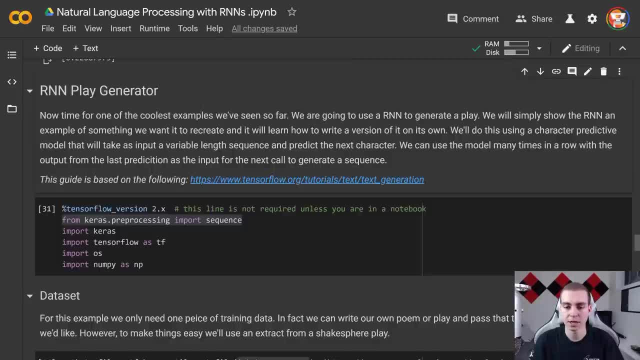 Now this is going to be the first kind of neural network we've done. that's actually going to be creating something for us, But essentially what we're going to do is make a model that's capable of predicting the next character in a sequence, So we're going to give it some 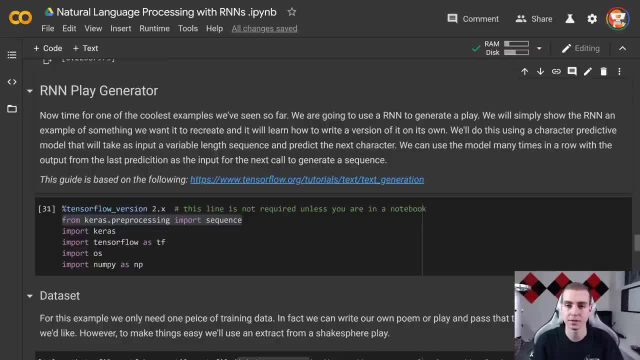 sequence as an input And what it's going to do is just simply predict the most likely next character. Now, there's quite a bit that's going to go into this, But the way we're going to use this to predict a play is we're going to train the model on a bunch of sequences. 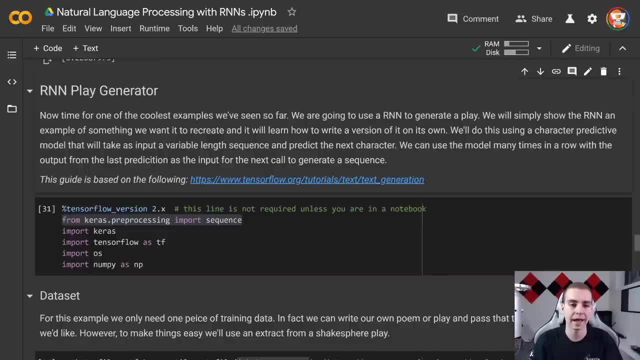 of texts from the play Romeo and Juliet. And then we're going to have it So that we're going to ask the model. we'll give it some starting prompt, some string to start with, And that'll be the first thing we pass to it. it will predict to us what the most likely 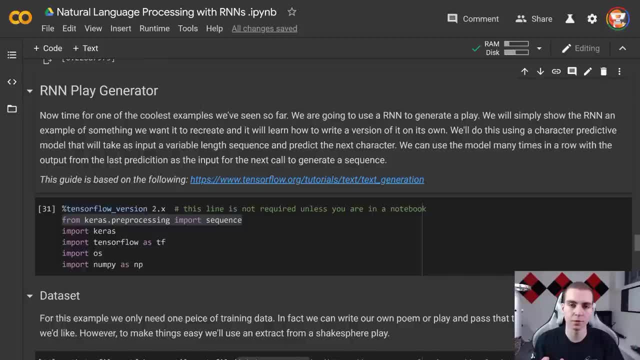 next character for that sequence is, And we'll take the output from the model and feed it as the input again to the model and keep predicting sequence of characters. So keep predicting the next character from the previous output as many times as we want to generate an entire. 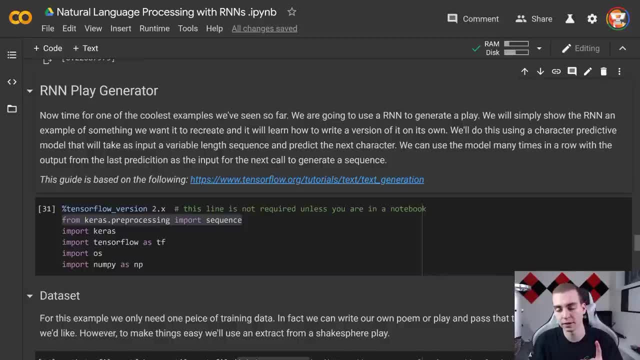 play. So we're going to have this neural network that's capable of predicting one letter at a time and we're going to end up generating an entire play for us by running it multiple times on the previous output from the last iteration. Now, that's kind of the problem. That's what 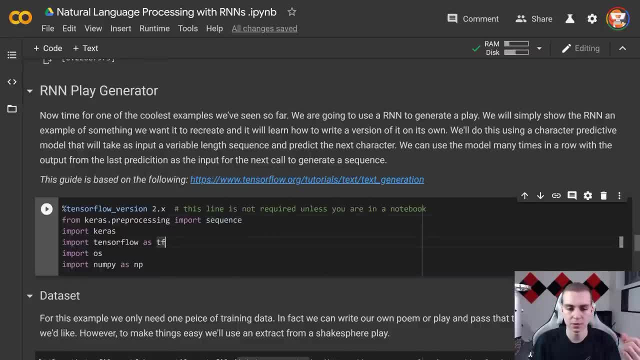 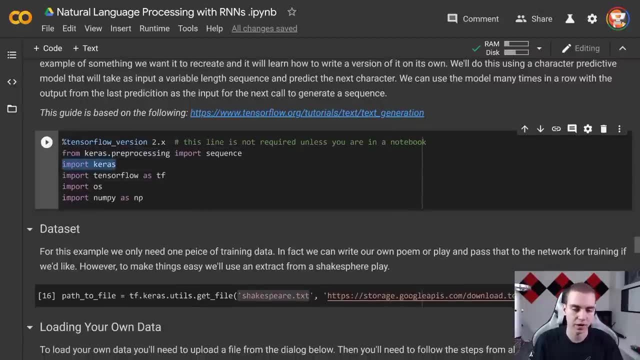 we're trying to solve. So let's go ahead and get into it and talk about what's involved in doing this. So the first thing we're going to do, obviously, is our imports. So from Kara's dot pre processing, import sequence, import Kara's. we need TensorFlow, NumPy and OS. 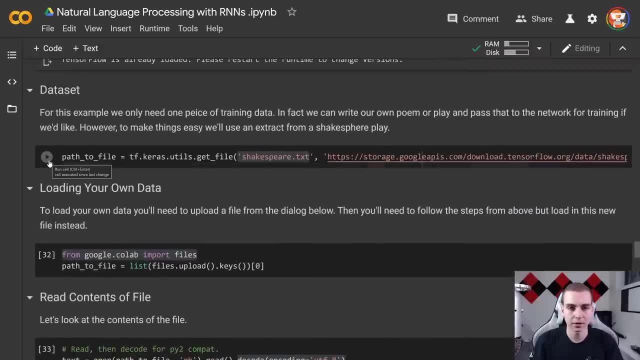 So we'll load that in, And now what we're going to do is download the file, So the data set for Romeo and Juliet, which we can get by using this line here. So Kara's has this utils thing which will allow us to get a. 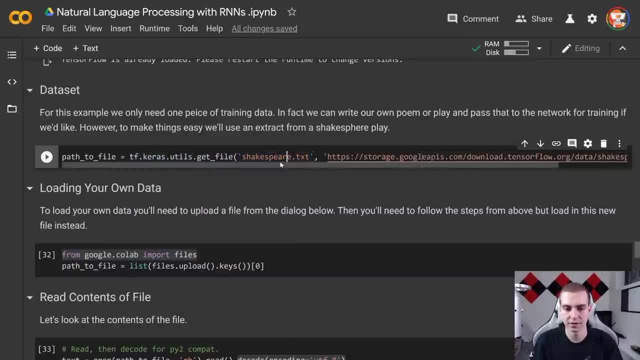 file, save it as whatever we want. In this case, we're going to save it as Shakespeare dot txt, And we're going to get that from this link. Now, I believe this is just some like shared drive that we have access to from Kara's, So we'll load that in here And then. 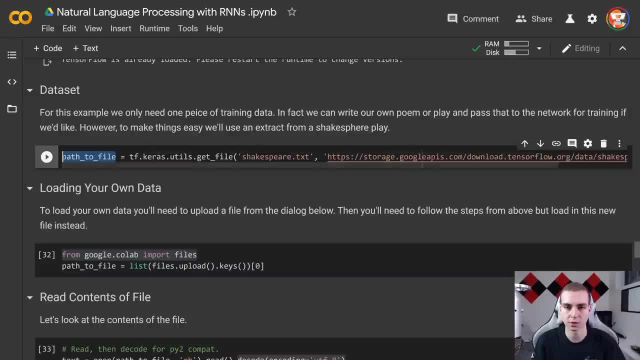 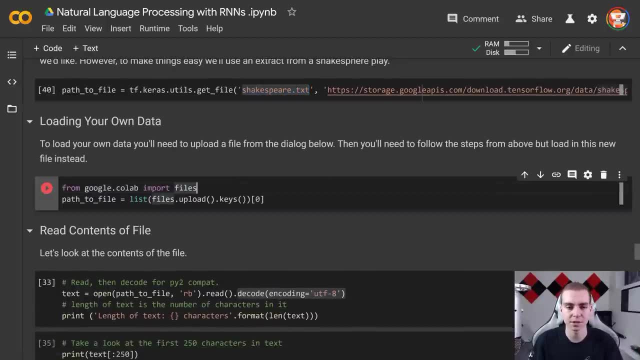 this will simply give us the path on this machine- Because, remember, this is Google Collaboratory- to this text file. Now, if you want, you can actually load in your own text data, So we don't necessarily need to use the Shakespeare play, we can use anything we want. In fact, an example: 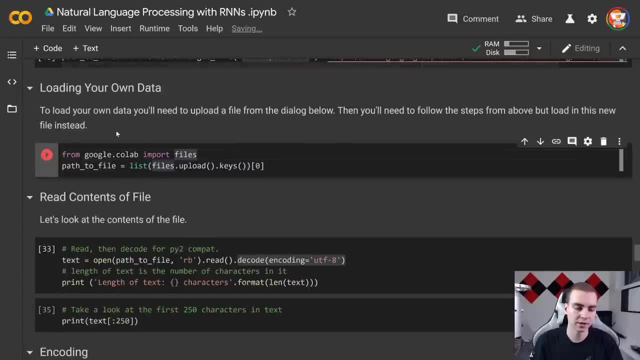 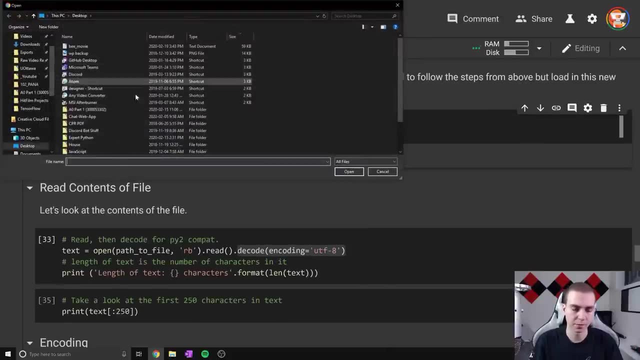 that I'll show later is using the B movie script. But the way you do that is run this block of code here And you'll see that it pops up this thing for choose files. just choose a file from your local computer, And then what that will do is just save this on. 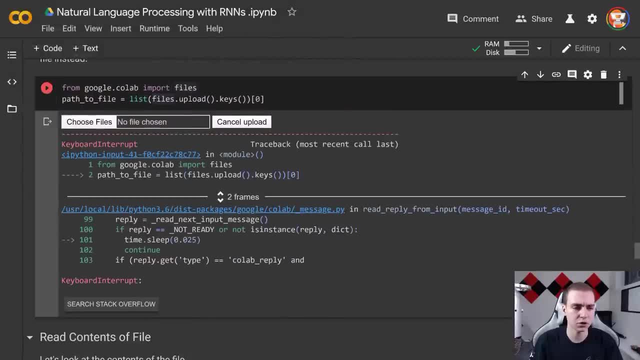 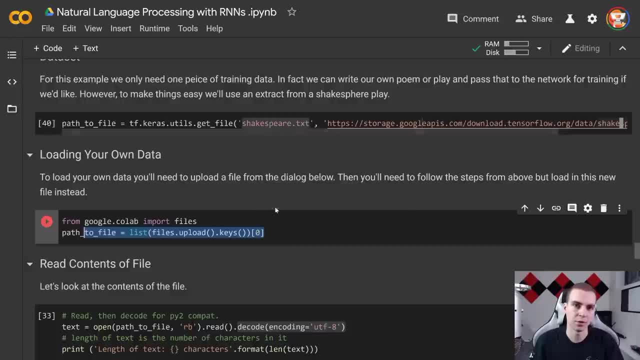 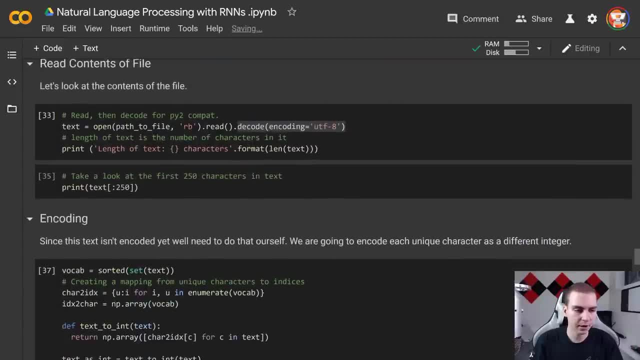 txt, But otherwise you can load in your own file. Now, after we do that, what we want to do is actually open this file. So remember, that was just saving the path to it. So we'll open that file in RB mode, which is read bytes mode, I believe. And then we're going to say: 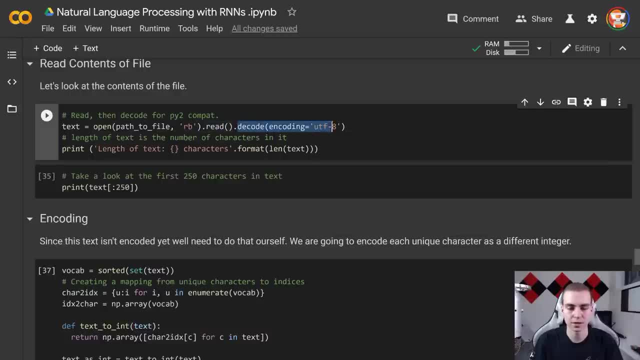 dot read. So we're going to read that in as an entire string, we're going to decode that into UTF eight format And then we're just printing the length of the text or the amount of character characters in the text. So if we do that, we can see we have the length of the text. 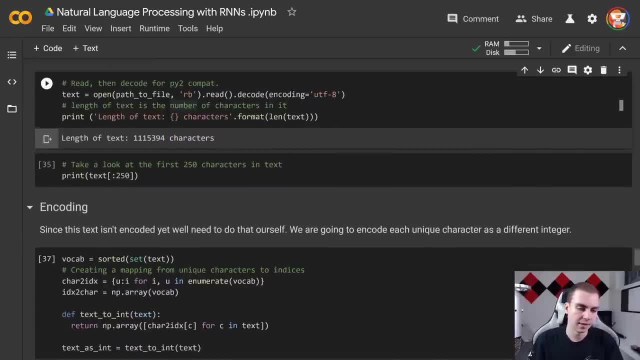 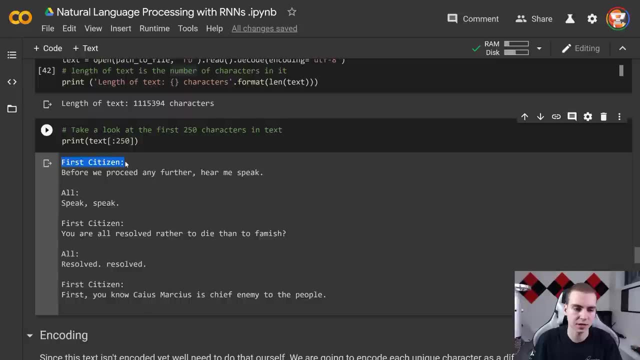 is 1.1 million characters approximately, And then we can have a look at the first 250 characters by doing this, So we can see that this is kind of what the plate looks like. we have whoever's speaking colon, then some line whoever's speaking colon, some line and. 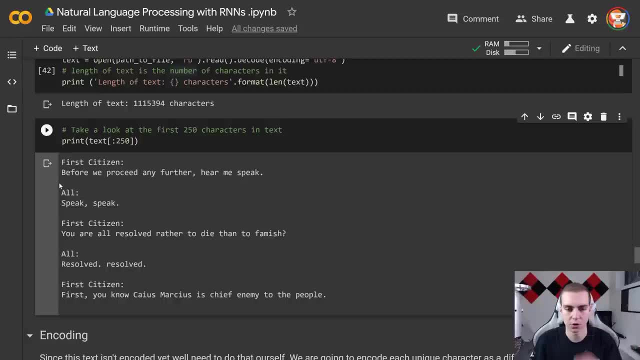 there's all these break lines, So backslash ends, which are telling us: you know, go to the next line, right. So it's going to be important because we're going to hope that our neural network will be able to predict things like break lines. 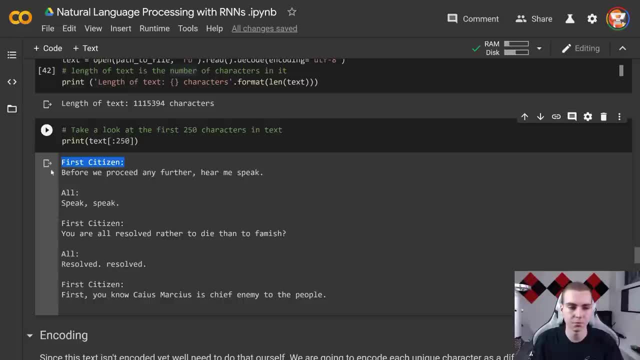 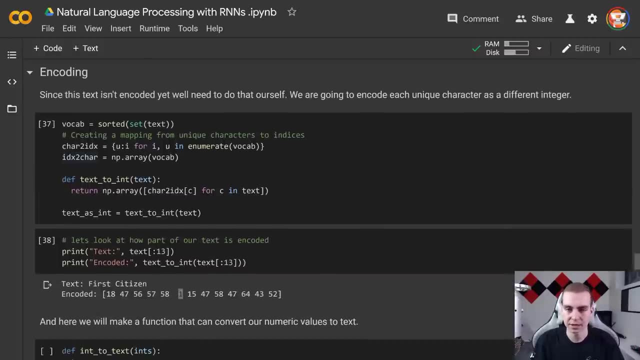 and spaces and even this kind of format, as we teach it more and get further in. But now it's time to talk about encoding. So obviously all of this text is in text form. it's not pre process for us, which means we need to pre process it and encode it as integers before. 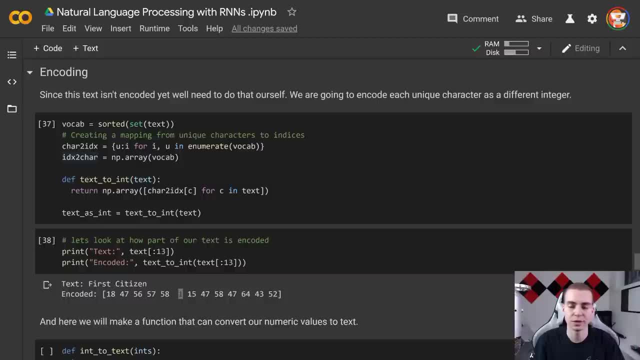 we can move forward Now. fortunately for us, this problem is actually a little bit easier than the problem we discussed earlier with encoding words, because what we're going to do is simply encode each character in the text with an integer. Now you can imagine. 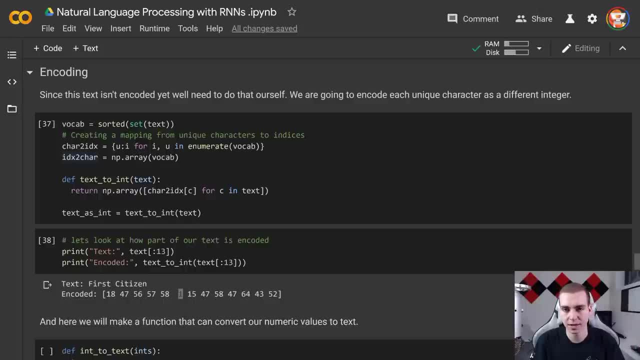 why this makes it so hard. It's because the text is a lot more complex. it's a lot more. this easier because there really is a finite set of characters, Whereas there's kind of indefinite or, you know, I guess, infinite amount of words that could be created. So 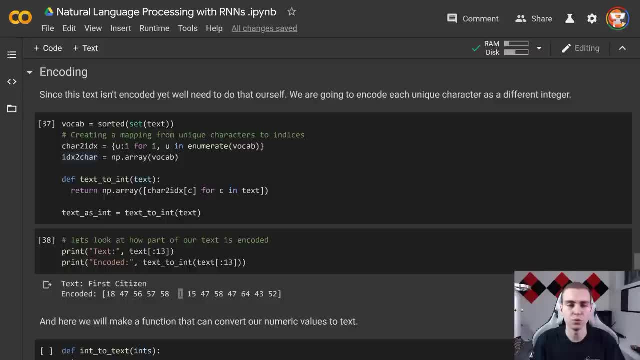 we're not really going to run into the problem where, you know, two words are encoded with such different, or two characters are encoded with such different integers that it makes it difficult for the model to understand. because I mean, we can look at what the value of vocab. 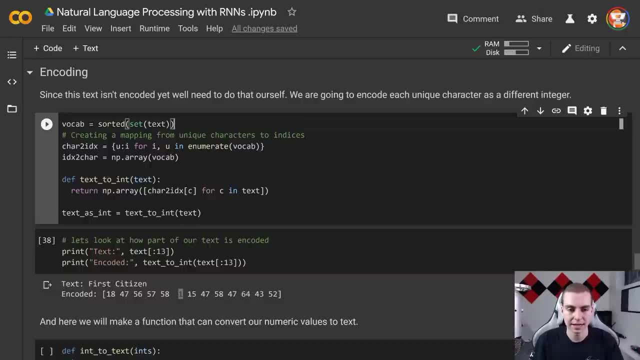 is here. we're only going to have so many characters in the text, And for characters it just doesn't matter as much, because you know, an R isn't like super meaningful compared to an A. So we can kind of encode in a simple format, which is what we're going to do. So 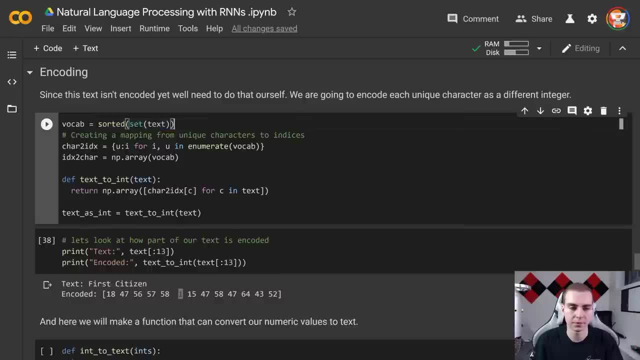 essentially, we need to figure out how many unique characters are in our vocabulary. So to do that, we're going to say: vocab equals sorted set text. this will sort all of the unique characters in the text, And then what we're going to do is create a mapping from 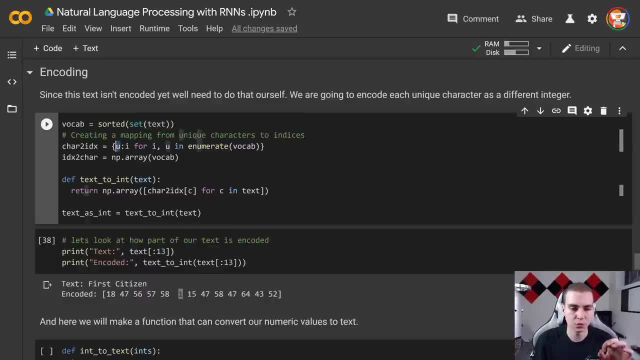 unique characters to in these indices. So essentially we're going to say UI for IU in a new enumerate vocabulary. what this will do is give us essentially zero, whatever the string is one, whatever the string is to, whatever the string is, for every single letter or character in our vocabulary. 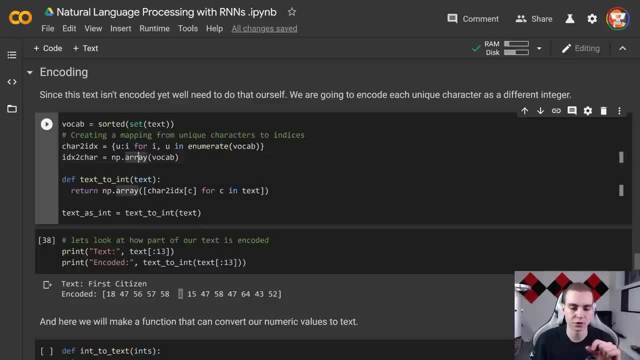 which will allow us to create this mapping, And then what we'll do is just turn this initial vocabulary into a list or into an array, So we can just use the index at which a letter appears as the reverse mapping, So going from index to letter rather than letter to index. 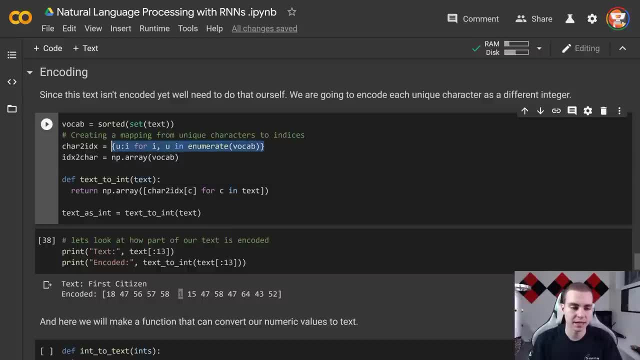 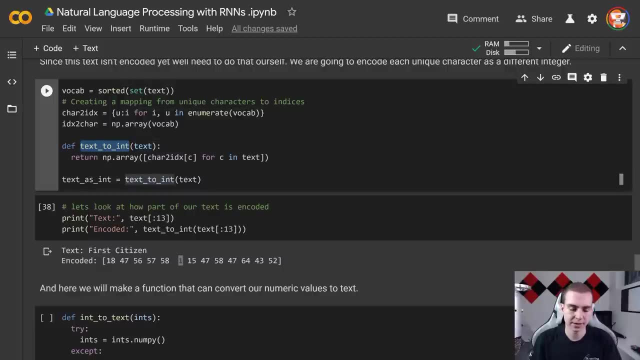 which is what this one's doing here. Next, I've just written a function that takes some text and converts that to an int or the int representation for it, just to make it a little bit easier for us as we get later on in the tutorial. So we're just going to say np, dot, array of in this case, and we're 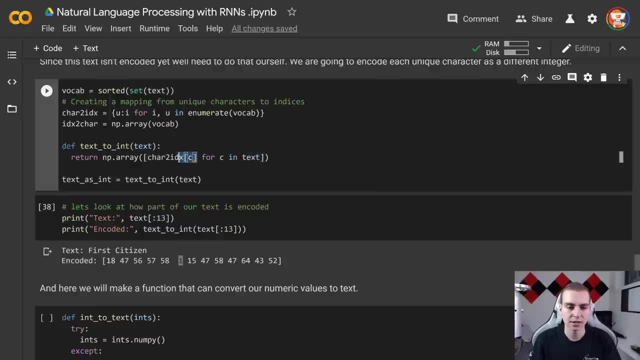 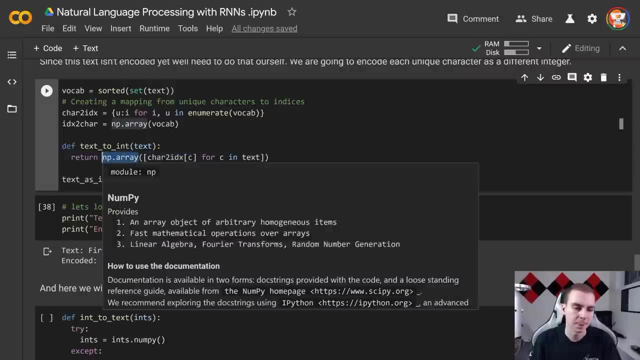 just going to convert every single character in our text into its integer representation by just referencing that character and putting that in a list here and then obviously converting that to NumPy array. So then, if we wanted to have a look at how this works, we can say: 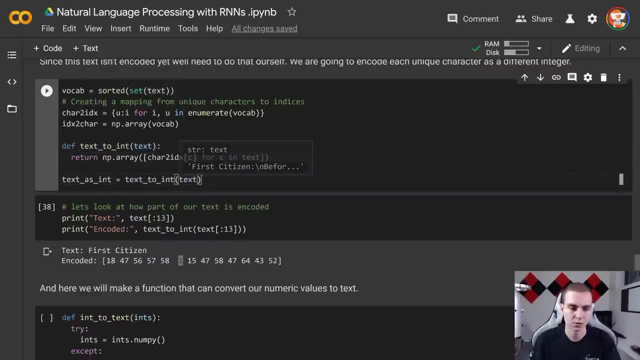 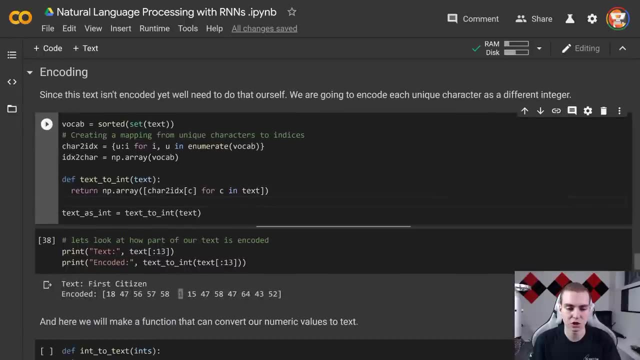 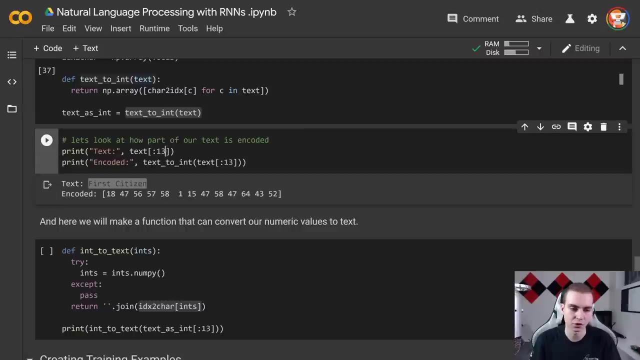 text, as int equals text to int text. So remember, text is that entire loaded file that we had above here. So we're just going to convert that to its integer representation entirely using this function, And now we can look at how this works down here. So we can see that the text first citizen, which is: 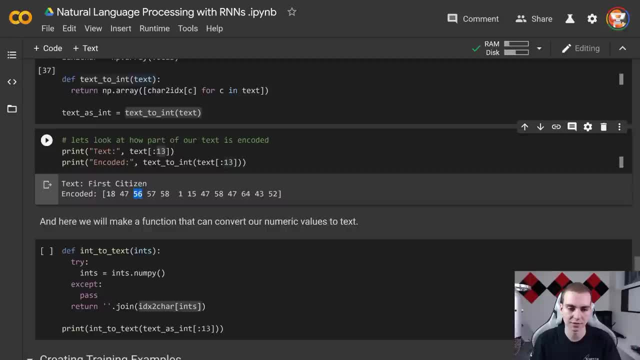 the first 13 letters is encoded by 184756, 5758. One, and obviously each character has its own encoding and you can go through and kind of figure out what they are based on the ones that are repeated, right? So that is how that works. 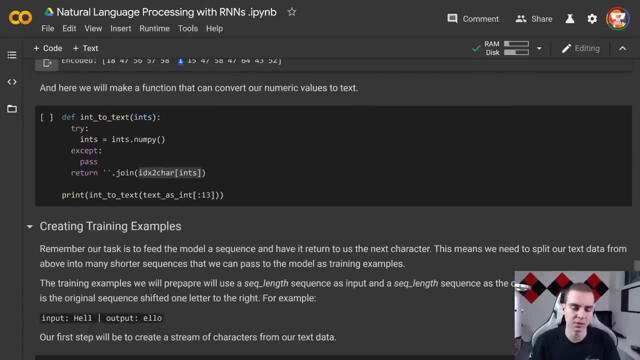 Now I figured while we were at it we might as well write a function that goes the other way. So into text. reason I'm trying to convert this to a NumPy array first is just because we're going to be passing in different objects potentially in here. So if it's not already, 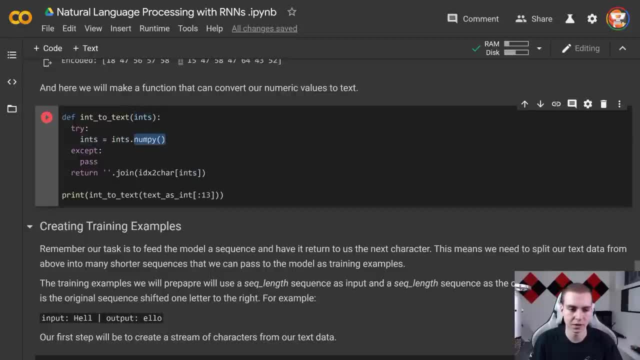 a NumPy array. it needs to be a NumPy array, which is kind of what this is doing. Otherwise we're just going to pass on that. we don't need to convert it to NumPy array if it already is one. we can just join all of the characters from this list into here. So that's essentially. 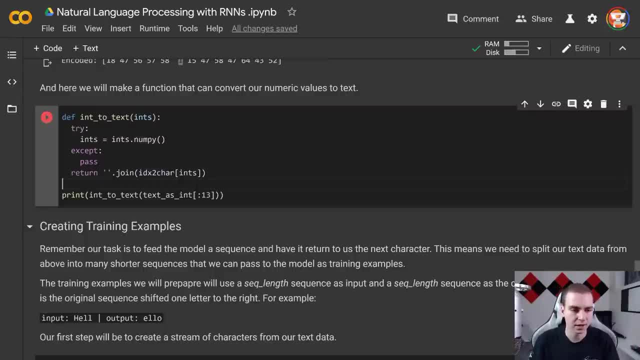 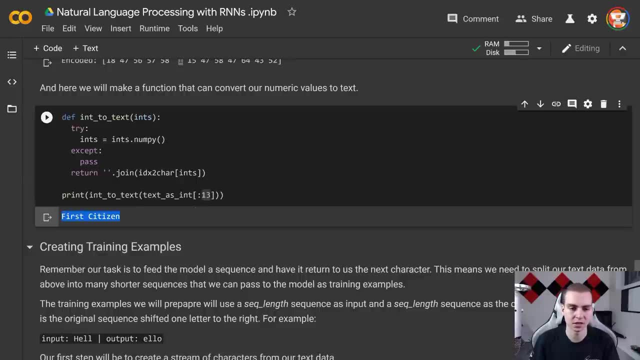 what this is. This is doing for us. it just joining into text And then we can see. if we go into text Texas in colon 13,. that translates that back to us for citizen. I mean, you can look more into this function if you want, but it's not that complicated, Okay, so now that we have 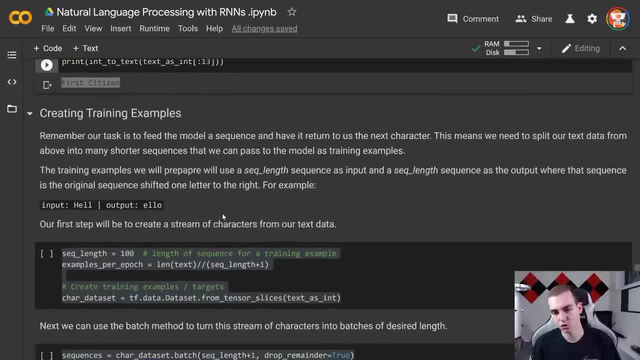 all this text encoded as integers. what we need to do is create some training examples. it's not really feasible to just pass the entire- you know 1.1 million characters to our model at once for training. we need to split that up into something that's meaningful. 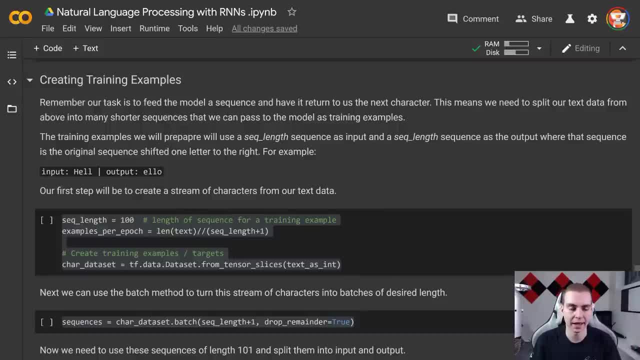 So what we're actually going to be doing is creating training examples where we have the first, where the training input right, so the input value is going to be some sequence of some length. we'll pick the sequence length. in this case, we're actually going to pick. 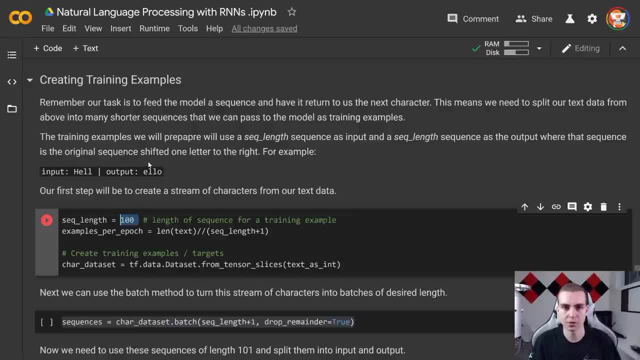 100.. And then the output or the expected output. So I guess, like the label for that training example is going to be the exact same sequence, shifted right by one character. So essentially I put a good example here. our input will be something like hell right, And then our 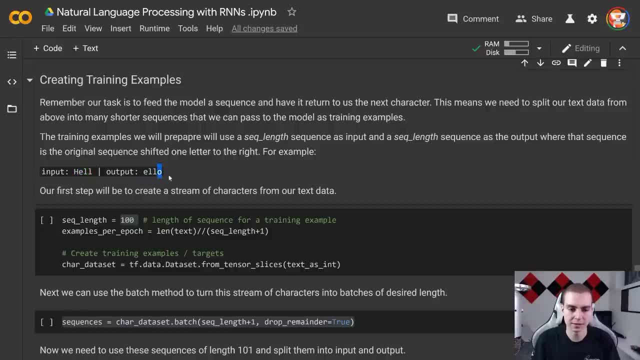 output will be ELL. So what it's going to do is predict this last character, essentially, And these are what our training examples are going to look like. So the entire beginning sequence and then the output sequence should be that beginning sequence minus the first. 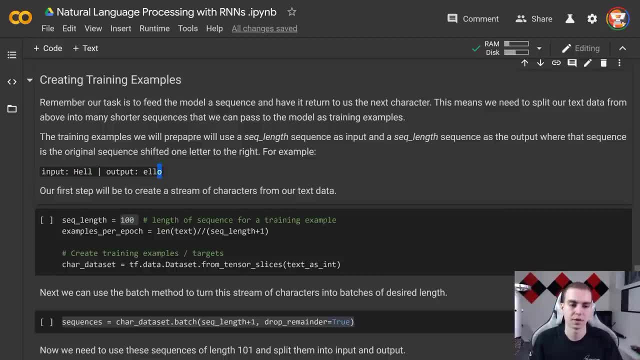 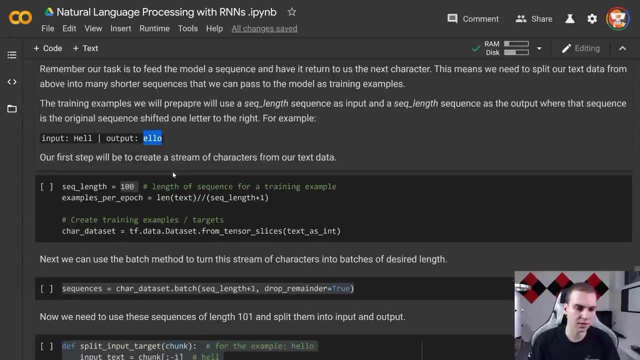 letter, but tack on what the last letter should be, So that this way we can look at some input sequence and then predict that output sequence, you know, plus a character, right, Okay, so that's how that works. So now we're gonna do is define a sequence length of 100,. 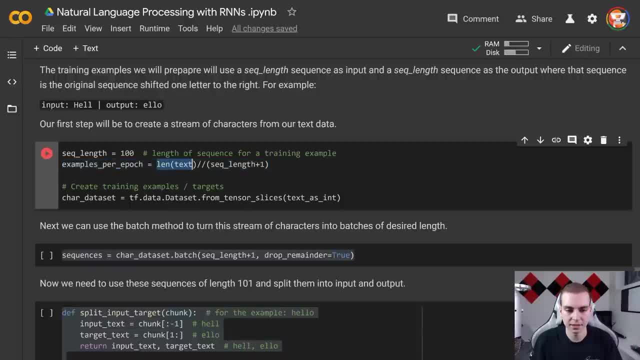 we're going to say the amount of examples per epoch is going to be the length of the text divided by the sequence length plus one. The reason we're doing this is because, for every training example, we need to create a sequence input that's 100 characters long, And we need to create a sequence output that's 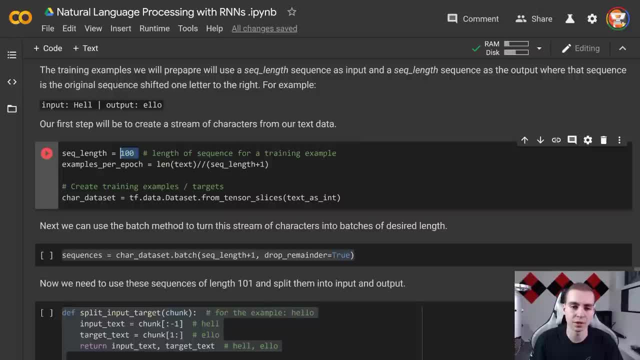 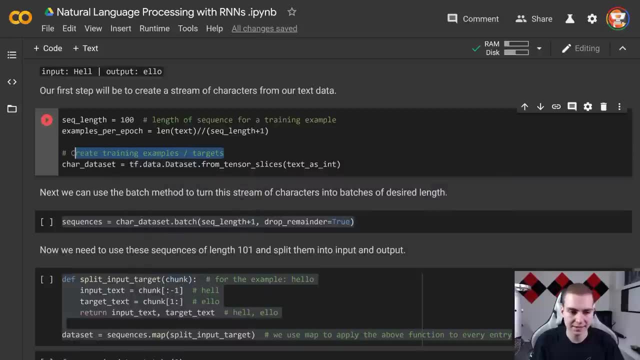 100 characters long, which means that we need to have 101 characters that we use for every training example. right? Hopefully that would make sense. So what this next line here is going to do is convert our entire string data set into characters, And it's actually going to allow us to have a stream of characters. 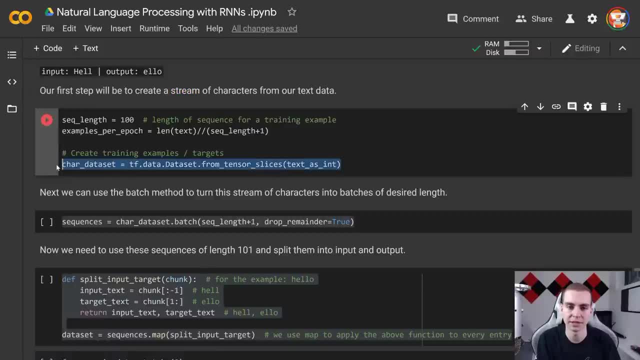 which means that it's going to essentially contain, you know, 1.1 million characters inside of this tf dot data set object from tensor slices. That's what that's doing Next. So let's run this and make sure this works. All right, what we're going to do is say sequences. 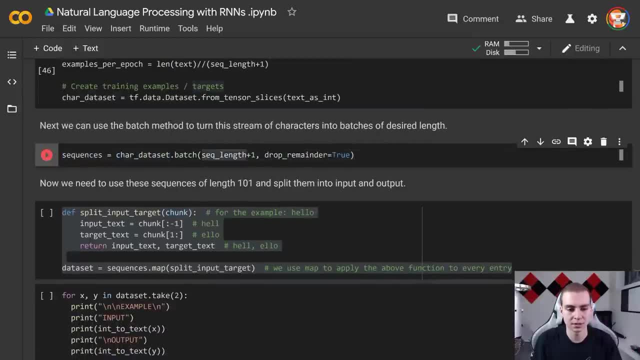 is equal to char data set dot. batch sequence length is the length of each batch, So in this case, one to one and then drop remainder means, Let's say that we have, you know, 105 characters in our text will, since we need sequences of 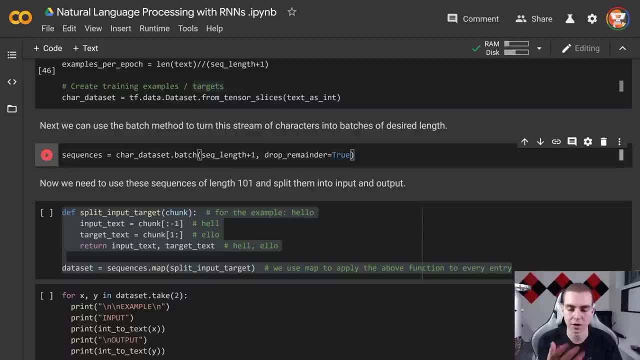 length 101, we'll just drop the last four characters of our text because we can't even put those into a batch. So that's what this is doing for us is going to take our entire character data set here that we've created and batch it into length of 101. And then 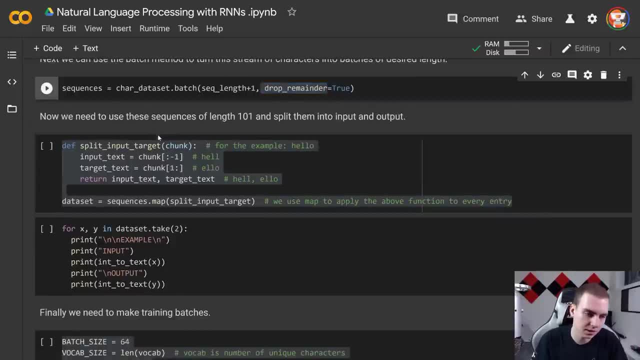 just drop the remainder. So that's what we're going to do here. sequences does now split input, target. What this is going to do, essentially, is just create those training examples that we needed. So taking this, the sequences of 101 length, and converting them into the input and target text, and I'll show you how they. 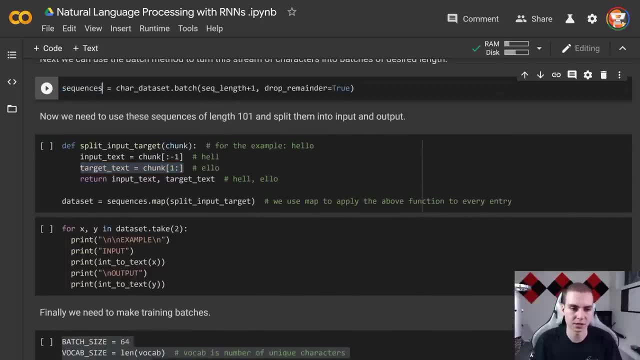 work in a second. we can do this: convert the sequences to that by just mapping them to this function. So that's what this function does. So if we say sequences, dot, map and we put this function here, that means every single sequence will have this operation applied. 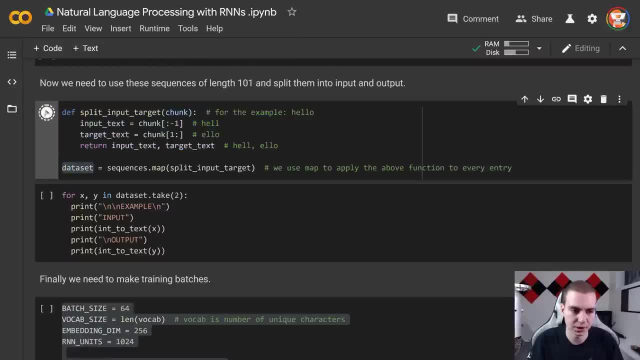 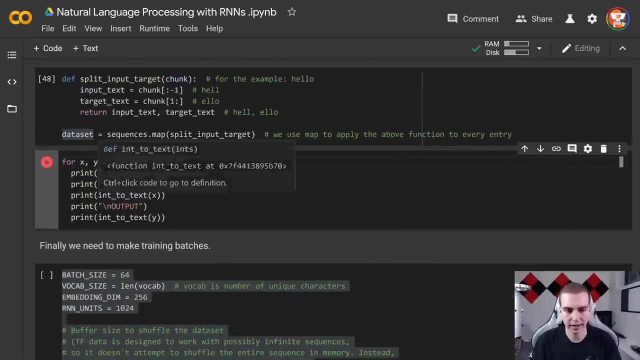 to it And that will be stored inside this data set. object are, I guess you'd say object, but we'll also just say that's it's going to be. you know the variable right? So if we want to look at an example of how this works, we can kind. 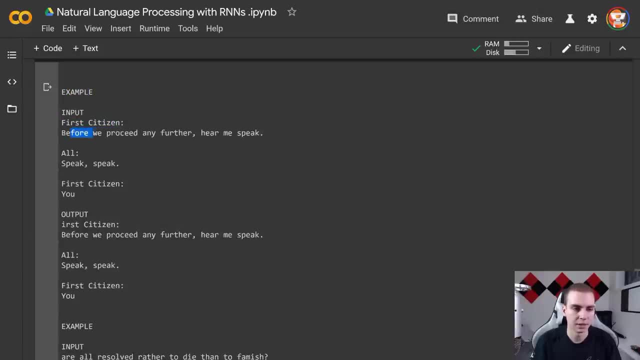 of see. so, just as example, the input will be first citizen, before we proceed any further, hear me: speak, all, speak. speak first citizen. you and the output. notice the first character is gone. certs that I in the last character is actually just a space here, Whereas here: 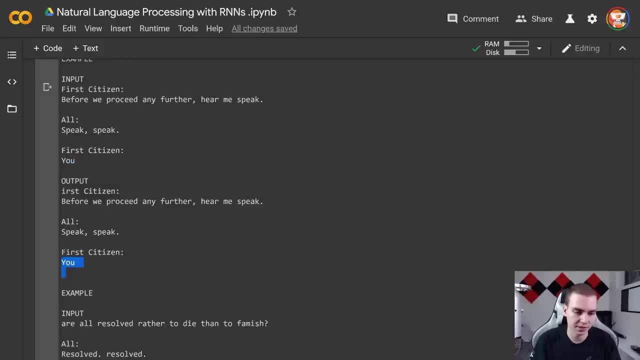 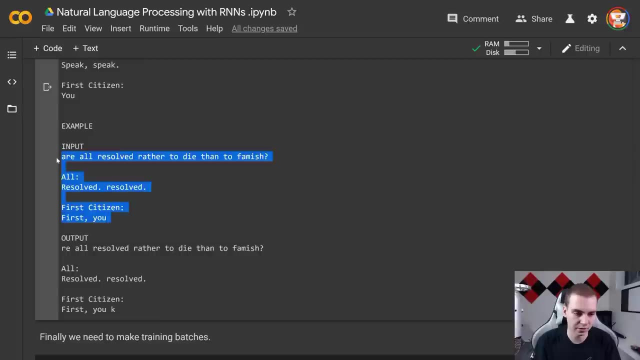 it didn't have a space where you can see there's no space Here, there is a space. that's kind of what I'm trying to highlight for you. The next example: we get our all resolved value to die rather than famine, whatever it goes to here, right, And then you can see here: 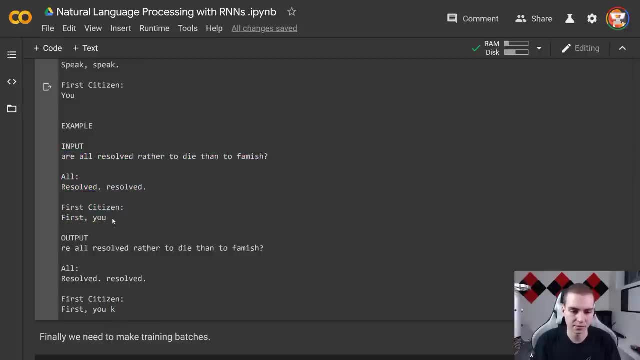 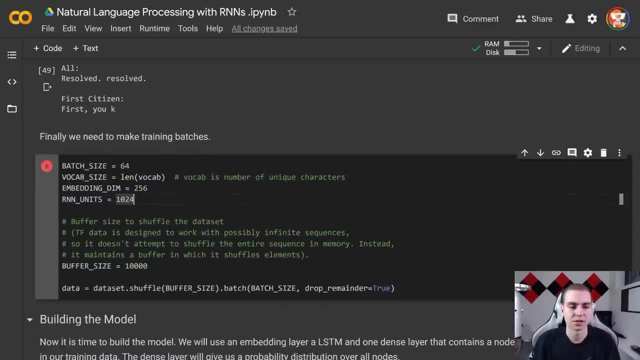 we omit that a and the next letter is actually a K. right, that's added in there. So that's how that works. Okay, so next we need to make training batches. So we're going to say the batch size equals 64.. The vocabulary size is the length of the vocabulary which, if 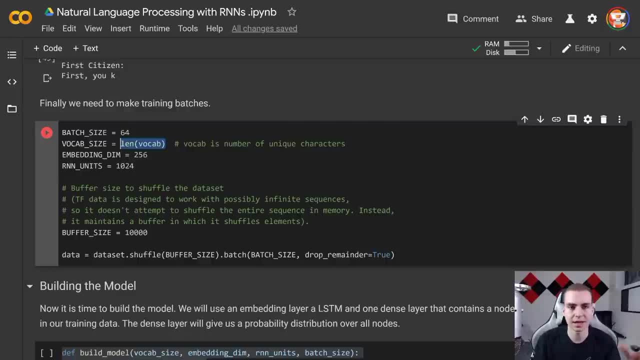 you remember, all the way back up to the top of the code, was the set or the sorted set of the text, which essentially told us how many unique characters are in there. The embedding dimension is 256, the RNN units is 1024.. And the buffer size is 10,000.. What we're going? 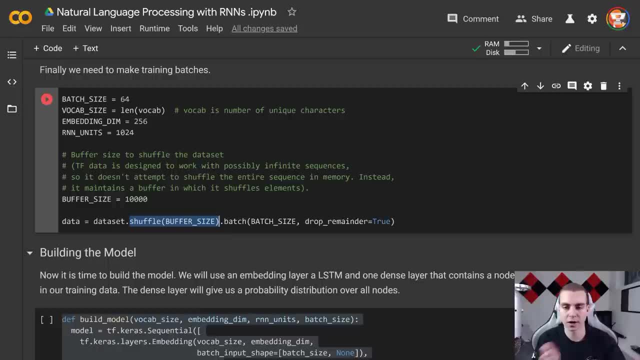 to do now is create a data set that shuffled. So we're going to switch around all these sequences so they don't get shown in the proper order, which we actually don't want, And I'm going to batch them by the batch size. So if we haven't kind of gone over what batching, 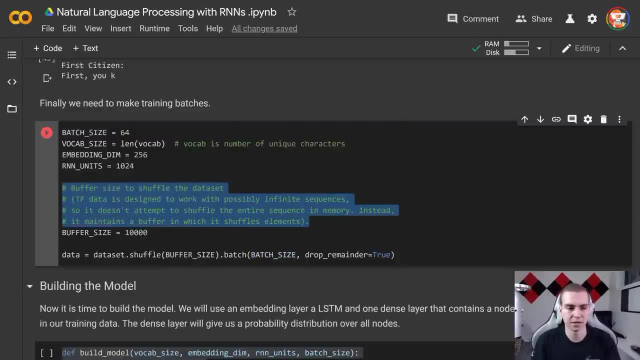 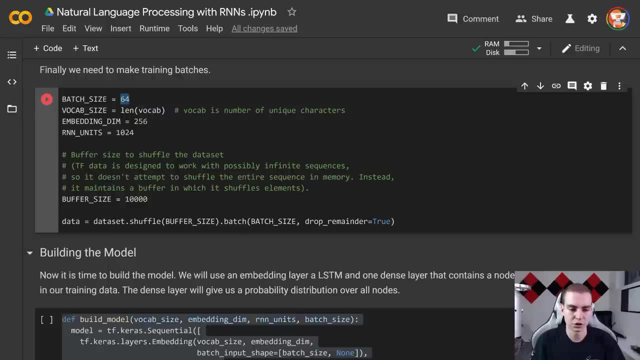 and all this does before. I mean you can read these comments as a straight from the TensorFlow documentation. What we want to do is we're going to go ahead, and we're going to go ahead, and we're going to do is feed our model 64 batches of data at a time. So what we're going to do is shuffle. 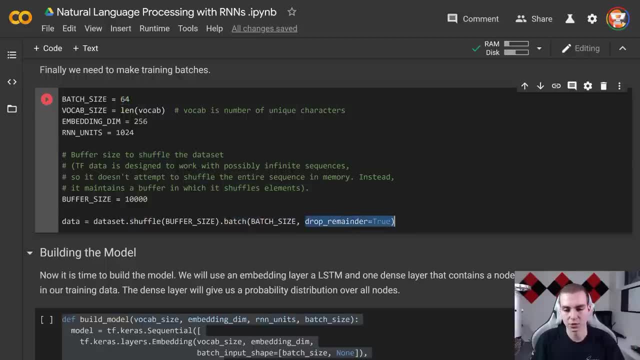 all the data, batch it into that size And then again drop the remainder. if there's not enough batches- which is what we'll do- We're going to define the embedding dimension, which is essentially how big we want every single vector to represent. our words are in. 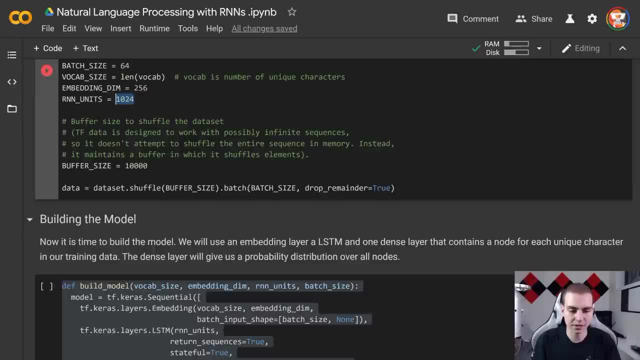 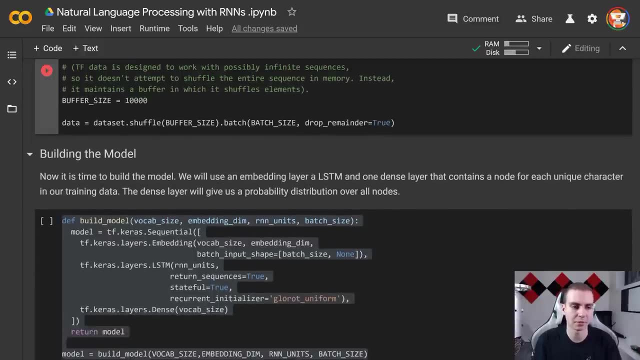 the embedding layer and then the RNN units. I won't really discuss what that is right now, But that's essentially how many it's hard to really just. I'm just going to omit that for right now because I don't want to butcher an explanation. It's not that important. 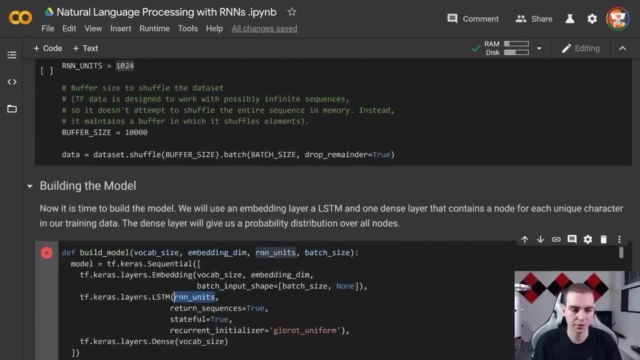 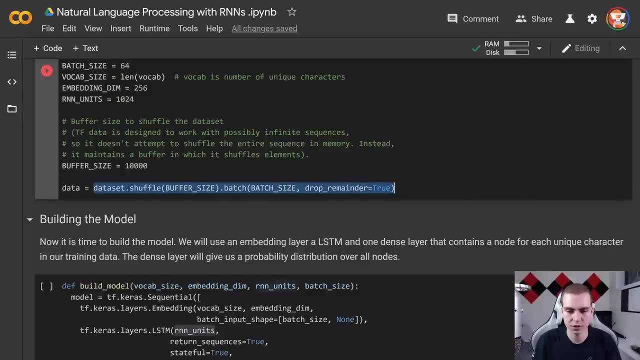 Anyways. okay, so now we're going to go down to building the model. So we've kind of set these parameters up here- remember what those are? we've batched and we've shuffled the data set And again, that's how this works. You can print it out if you want to see what. 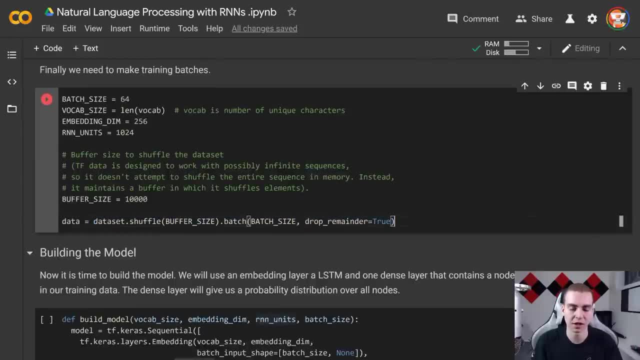 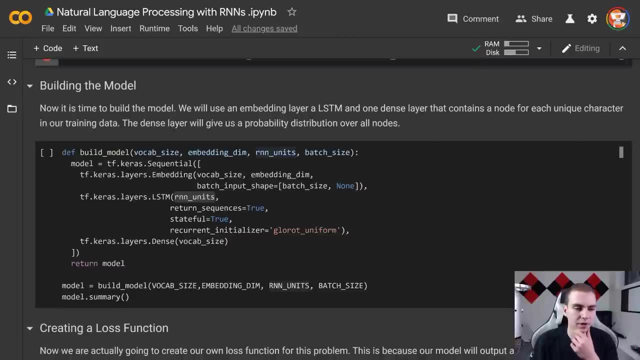 a batch actually looks like, But essentially it's just 64 entries of those sequences, right? So 64 different training examples is what a batch of that is. Alright. so now we go down here and we're going to say build model. we're actually making a function that's going to return to us a built model. 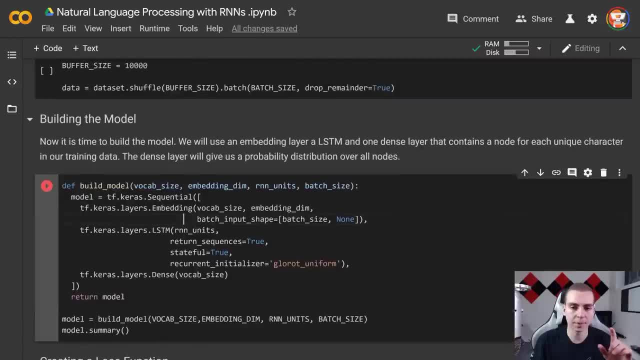 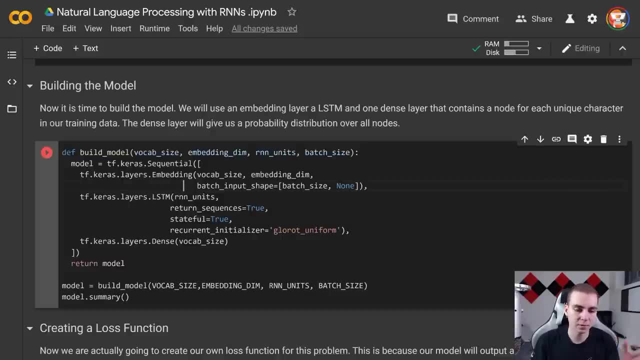 The reason for this is because right now we're going to pass the model batches of size 64 for training, right, But what we're going to do later is save this model and then we're going to patch, pass it batches of one pieces of, you know, training, whatever data, so that 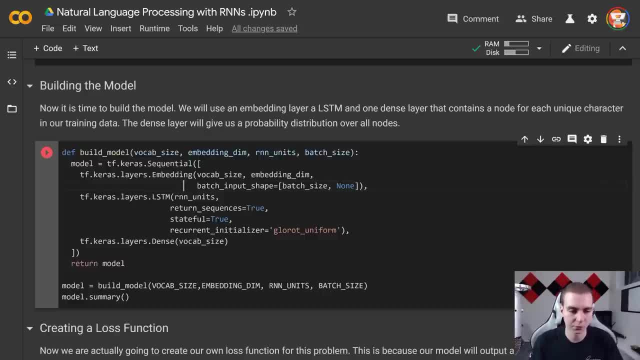 it can actually make a prediction on just one piece of data, because, for right now, what it's going to do is: takes a batch size of 64, it's gonna take 64.. training examples and return to a 64 outputs. That's what this model is going to be built. 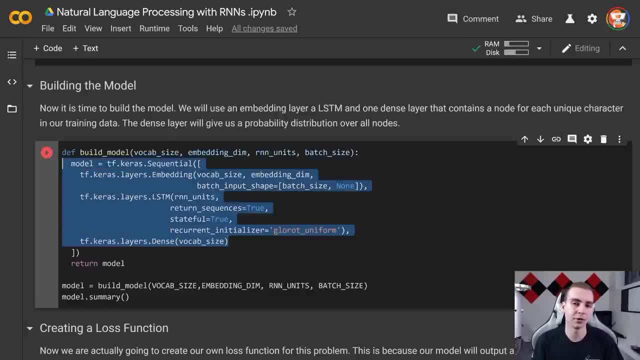 to do the way we build it now to start, But later on we're going to rebuild the model using the same parameters that we've saved and trained for the model, but change it to just be a batch size of one, so that that way we can get one prediction for one input. 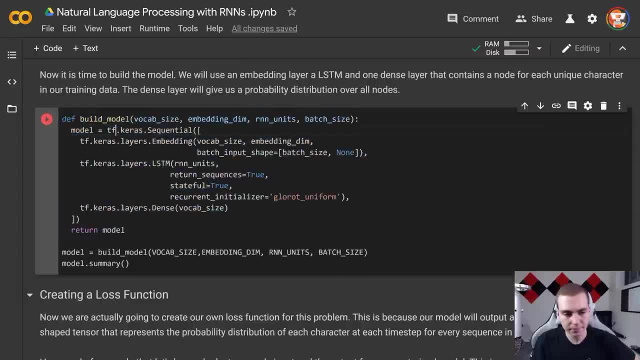 sequence, right. So that's why I'm creating this build model function. Now in here it's going to have the vocabulary sizes, first argument. the embedding dimension, which remember was 56, as a second argument. but also, these are the parameters up here, right? And then we're. 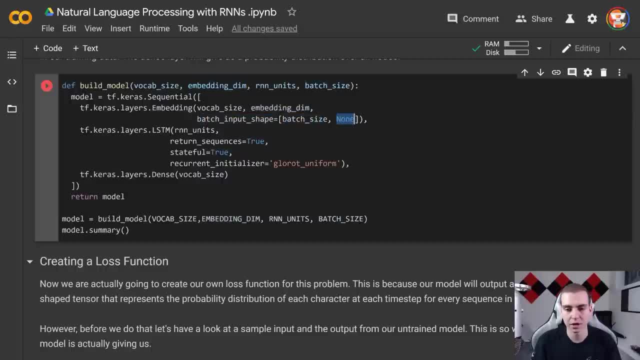 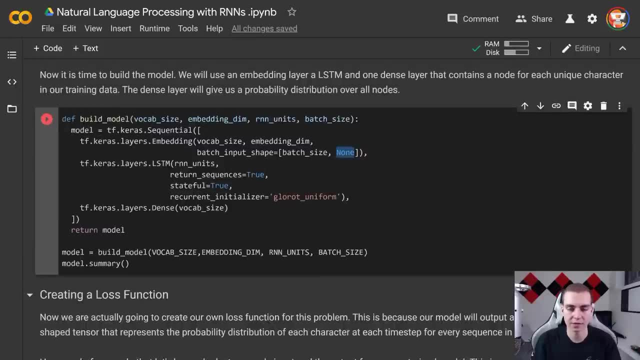 going to define the batch size. as you know, batch size none. what this none means is we don't know how long the sequences are going to be in each batch. all we know is that we're going to have 64 entries in each batch, And then of those 64 entries, so training examples. 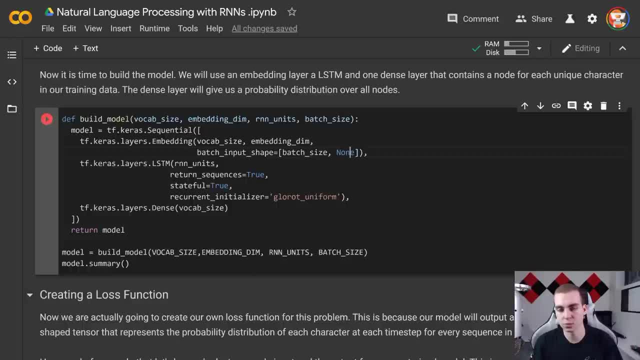 right, we don't know how long each one will be, Although in our case, we're going to use ones that are length 100.. But when we actually use the model to make predictions, we're going to use a bunch of them and we don't know how long the sequence is going to be that 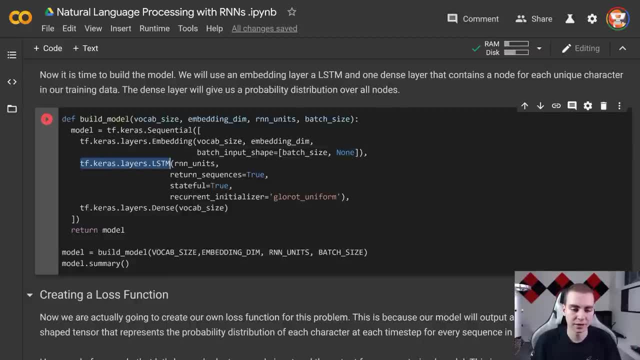 we input, so we leave this none. Next, we'll make an LSTM layer, which is long, short term memory, RNN units, which is 1024.. Which, again, I don't really want to explain but you can look up if you want. return sequences means return the intermediate stage at every step. 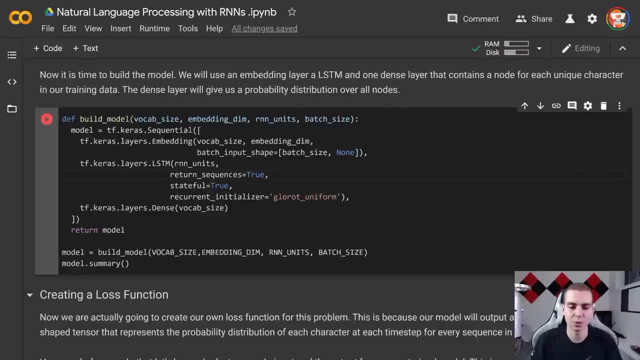 The reason we're doing this is because we want to look at what the models seeing at the intermediate steps, not just the final stage. So if you leave this as false and you don't set this to true, what happens is this: LSTM just returns one output that tells us what the model kind of found at the very last time. 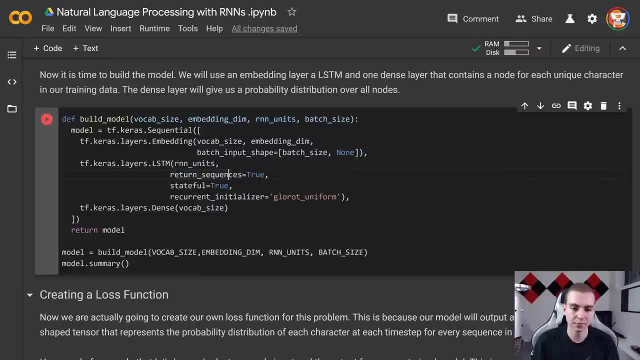 step, But we actually want the output at every single time step for this specific model, And that's why we're setting this true stateful. I'm not going to talk about that one right now. That's something you can look up if you want. And then recurrent initializer is just. 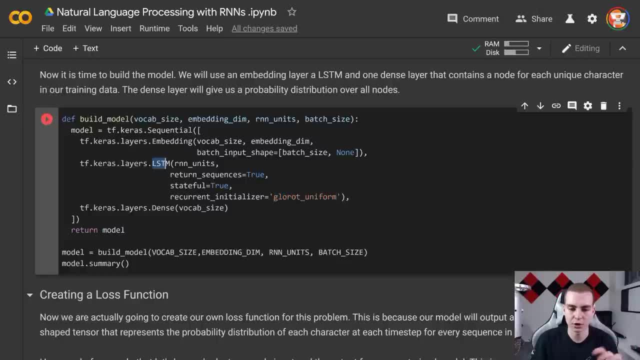 what these values are going to start at In the LSTM. we're just picking this because this is what TensorFlow is, kind of said is a good default to pick. I won't go into more depth about that Again, things that you can look up more if you want. Finally, we have 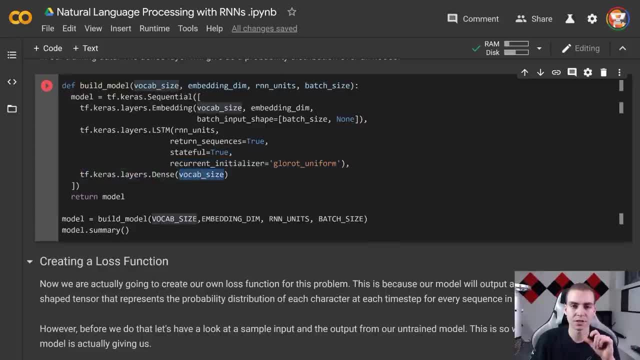 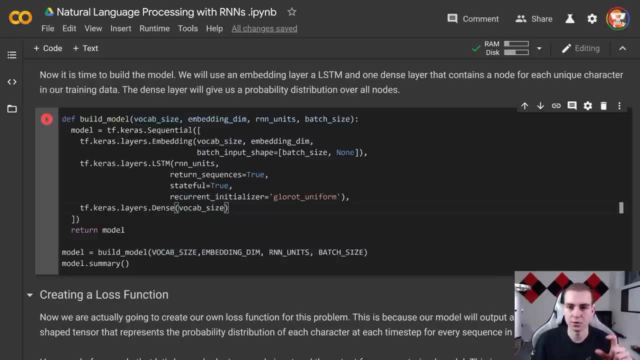 a dense layer which is going to contain the amount of vocabulary size notes. The reason we're doing this is because we want the final layer to have the amount of nodes in it equal to the amount of characters in the vocabulary. This way, every single one of those nodes 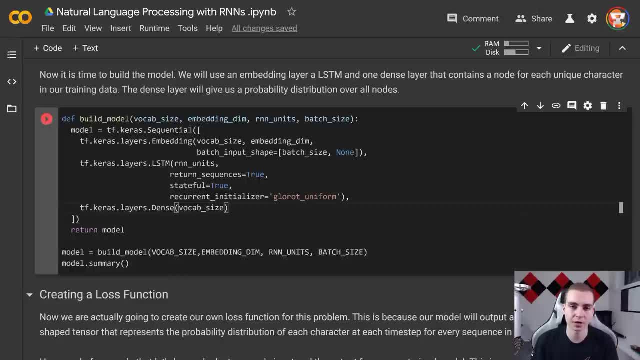 can represent a probability distribution that that character comes next. So all of those nodes value some sum together should give us the value of one. And that's going to allow us to look at that last layer as a predictive layer where it's telling us the probability that these characters come next. We've discussed how that's worked previously. 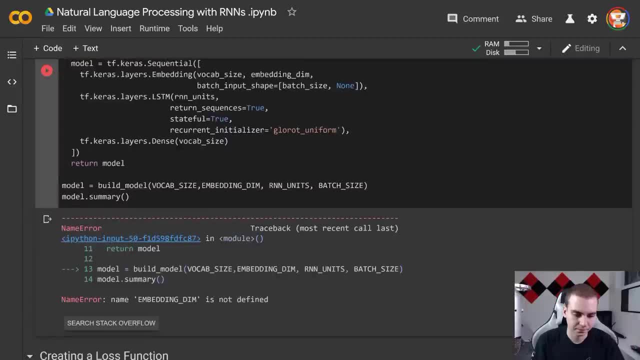 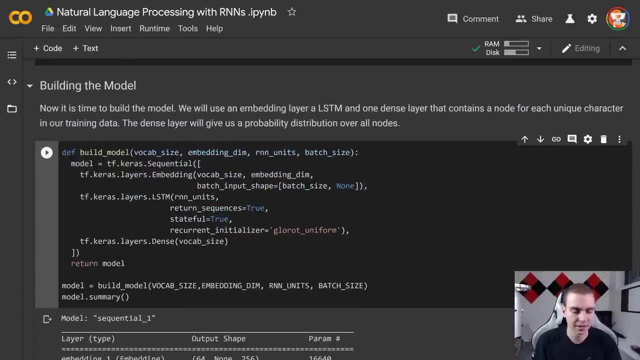 with other neural networks. So let's run this now. Name embedding dim is not defined, which I mean believes I have not ran this yet, So now we run that and we should be good. So if we look at the model summary, we can see we have. 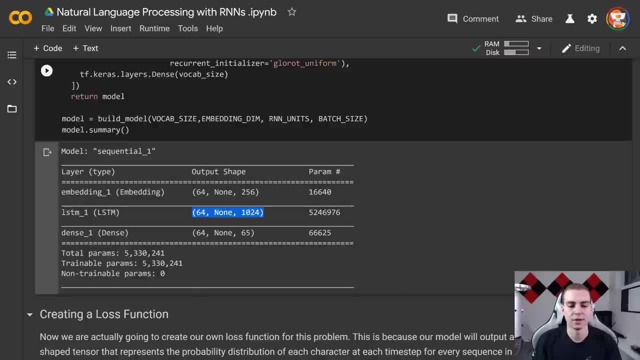 our initial embedding layer, we have our LSTM And then we have our dense layer at the end. Now, notice 64 is the batch size, right? That's the initial shape. None is the length of the sequence, which we don't know, And then this is going to be just the output. 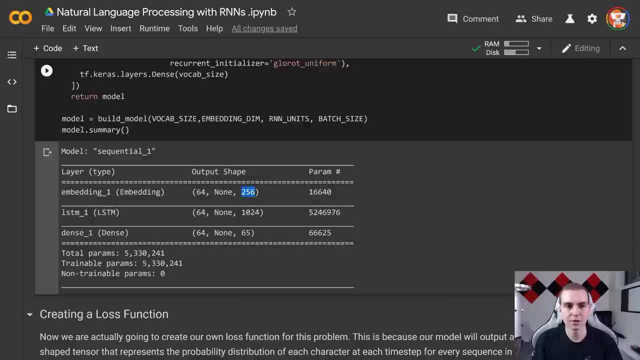 dimension, or sorry, this is the amount of values in the vector, right? So we're going to start with 256, we'll just do 1024 units in the LSTM, And then 65 stands for the amount of nodes, because that is the length of the sequence. 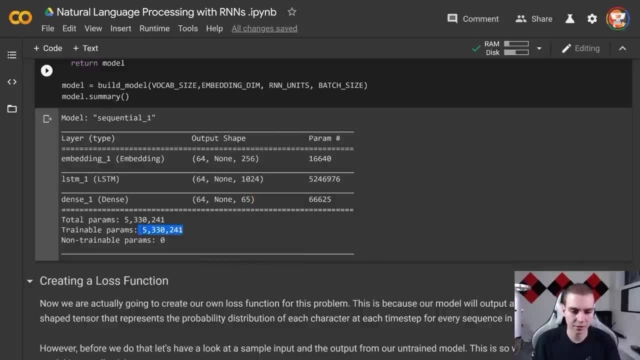 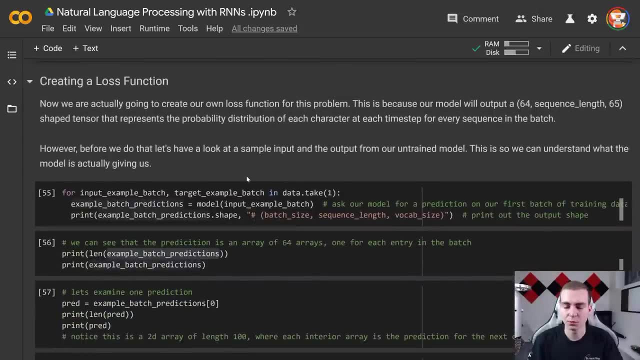 All right, so combined, that's how many trainable parameters we get. you can see each of them for each layer, And now it's time to move on to the next section. Okay, so now we're moving on to the next step of the tutorial, which is creating a loss function to compile. 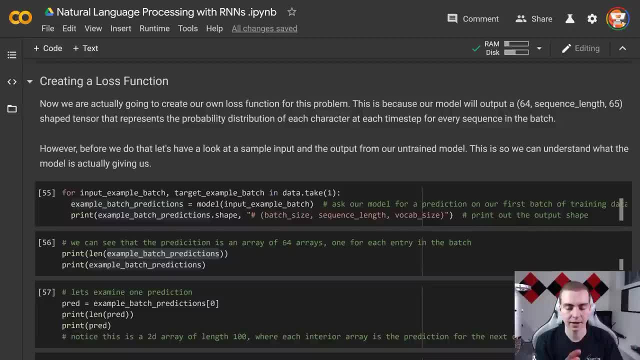 our model with Now. I'll talk about why we need to do this in a second, But I first want to explore the output shape of our model. So remember, the input to our model is something that is of length 64, because we're going to have batches of 64 training examples. So 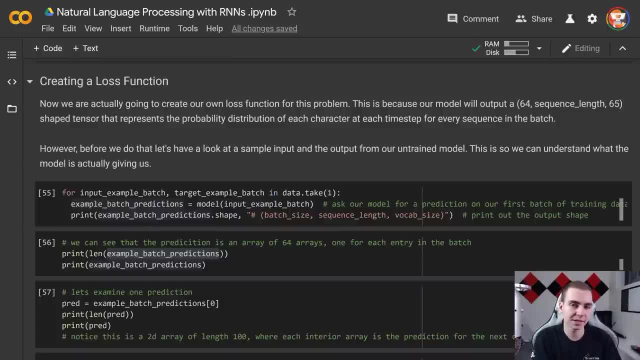 every time we feed our model, we're going to give it 64 training examples. Now, what those training examples are are sequences of length 100. That's what I want you to remember. we're passing 64 entries that are all of length 100 into the model as its training data, right. 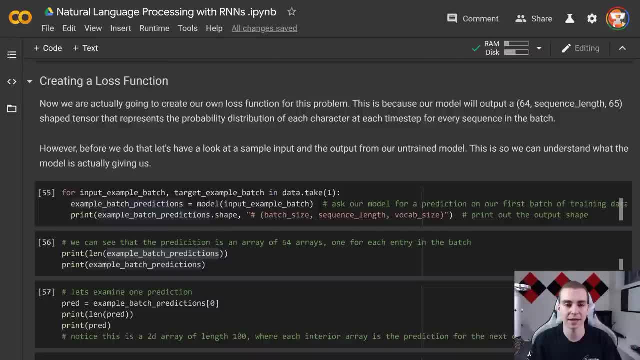 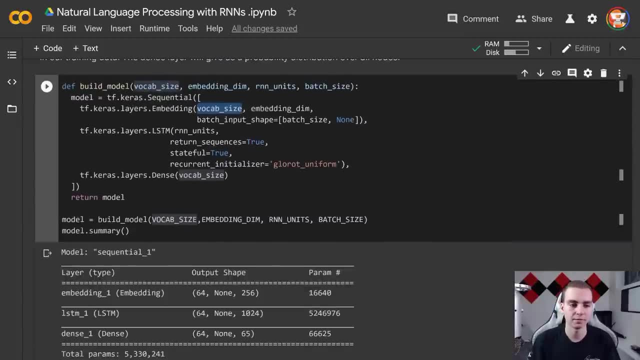 But sometimes, and when we make predictions with the model later on we'll be passing it. just one entry that is of some variable length, right, And that's why we've created it, this build model function, so that we can build this model using the parameters. 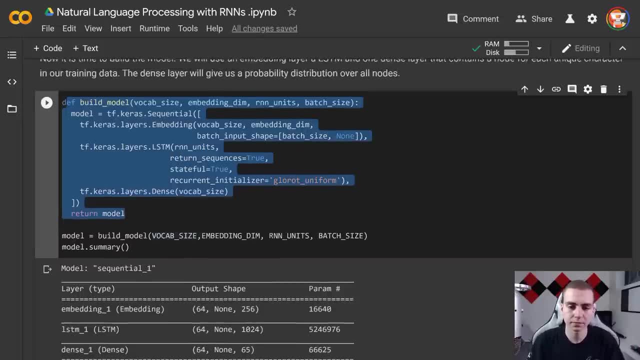 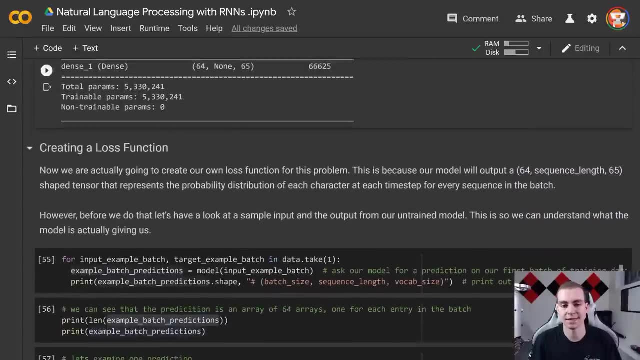 that we've saved. later on, once we train the model and it can expect a different input shape- right, Because when we're training it, it's going to be given a different shape than we're actually testing with it. Now what I want to do is explore the output of 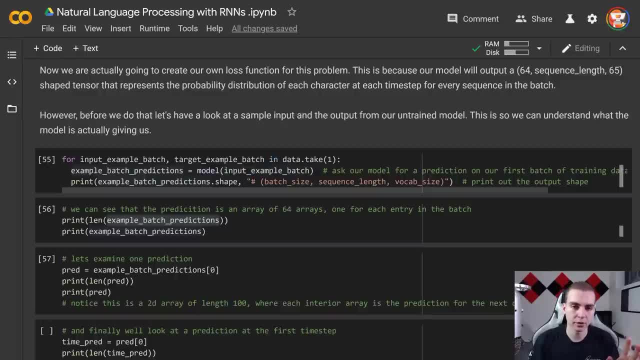 this model, though at the current point in time. So we've created a model that accepts a batch of 64 training examples that are of length 100.. So let's just look at what we're going to get, what the output is from the final layer. Give this a second to run. we. 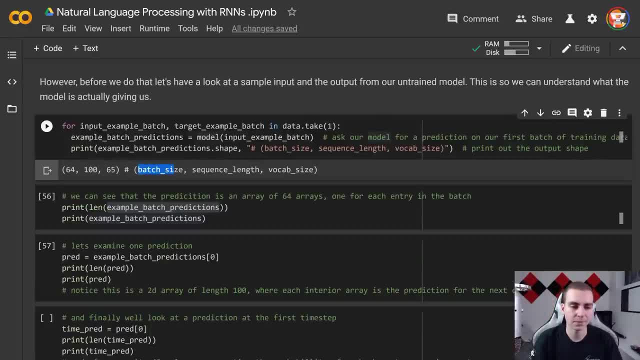 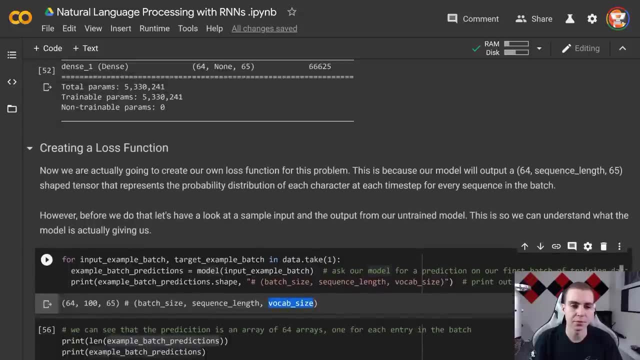 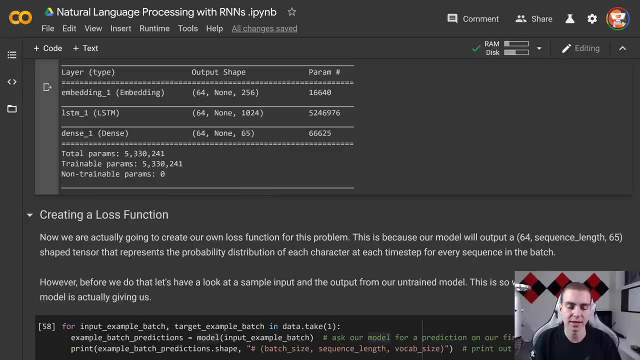 get 64, 165.. And that represents the batch size, the sequence length and the vocabulary size. Now, the reason for this is we have to remember that when we create a dense layer, as our last layer that has 65 nodes, every prediction is going to contain 65 numbers. 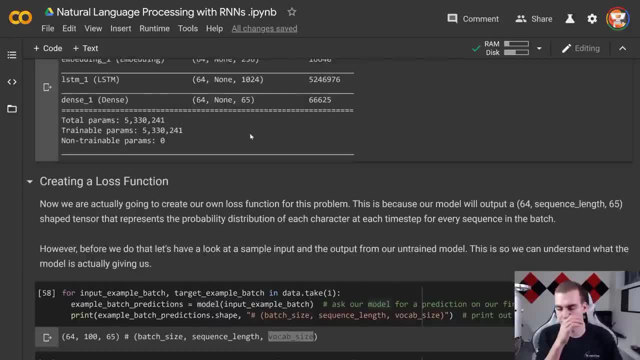 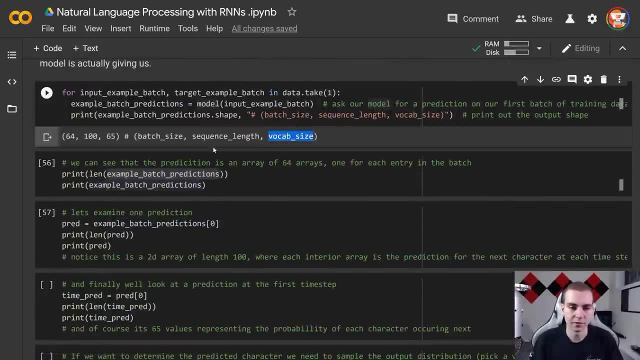 And that's going to be the probability of every one of those characters occurring. right, that's what that does at the last one for us. So obviously, our last dimension is going to be 65.. For the vocabulary size, This is the sequence length, And that's about I just 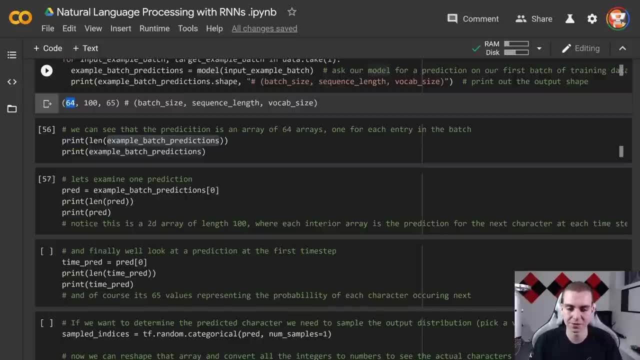 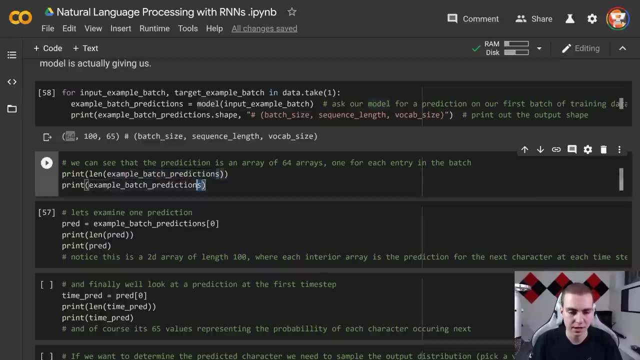 want to make sure this is really clear before we keep going. Otherwise it's gonna get very confusing very quickly. So what I want to do now is actually look at the length of the example batch predictions and just print them out and look at what they actually are. 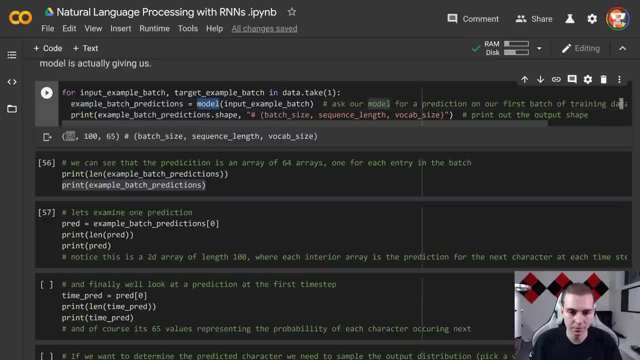 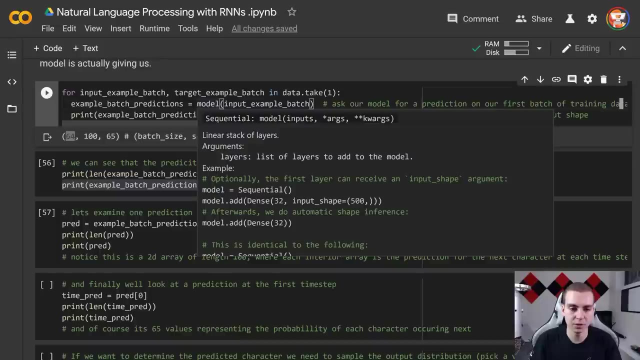 So example, batch predictions- is what happens when I use my model on some random input example actually, well, one from my data set with when it's not trained. So I can actually use my model before it's trained with random weights and random biases and parameters by simply using model And 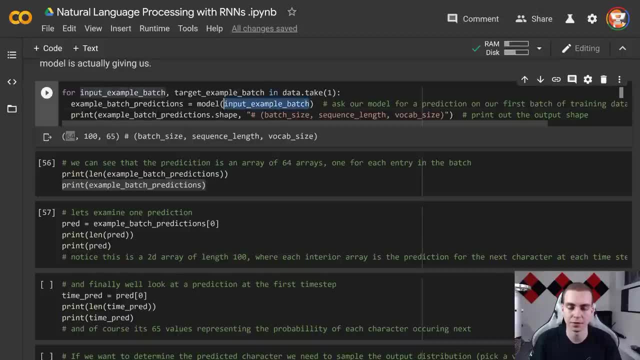 then I can put the little brackets like this and just pass in some example that I want to get a prediction for. So that's what I'm going to do. I'm going to give it the first batch And it can even. it shows me the shape of this batch: 64, 100,. I'm going to pass that. 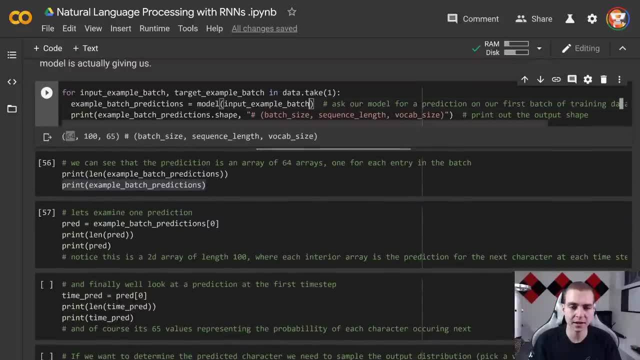 to the model And it's going to give us a prediction for that, And in fact, it's actually going to give us a prediction for every single element in the batch right, every single training example in the batch it's going to give us a prediction for. So let's look. 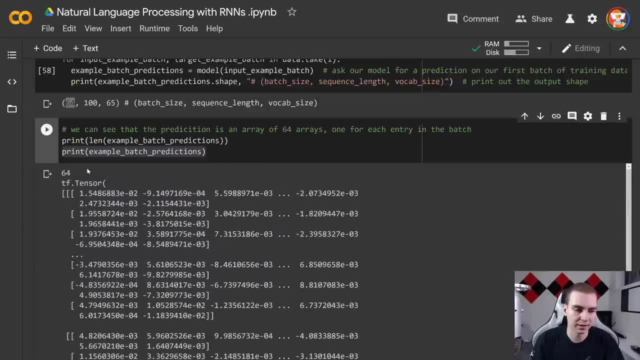 at what those predictions are. So this is what we get. we get a length 64, tensor right, And then inside of here, we get a list inside of a list, or an array inside of an array with all of these different predictions. So we'll stop there For this. like explaining this. 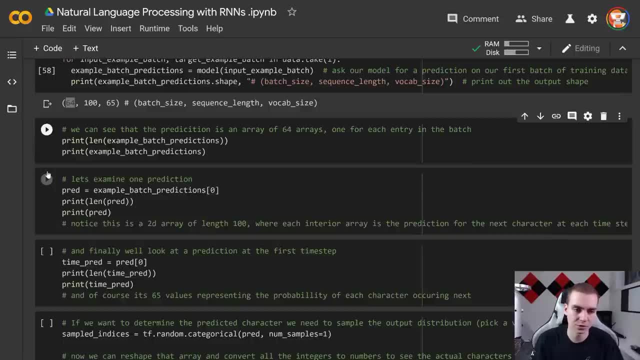 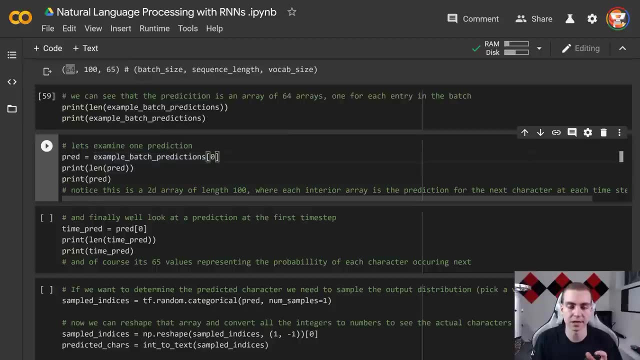 aspect here. But you can see we're getting 64 different predictions because we're going to say there's 64 elements in the batch. Now let's look at one prediction, So let's look at the very first prediction for, say, the first element in the batch, right? So let's 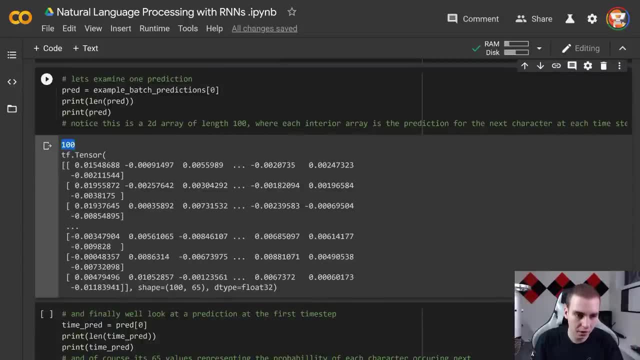 do that here And we see now that we get a length, 100, tensor, and that this is what it looks like, there's still another layer inside And in fact we can see that there's another nested layer here, right another nested array inside of this array. So the 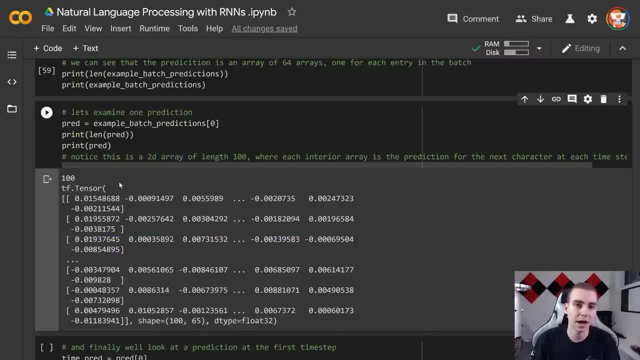 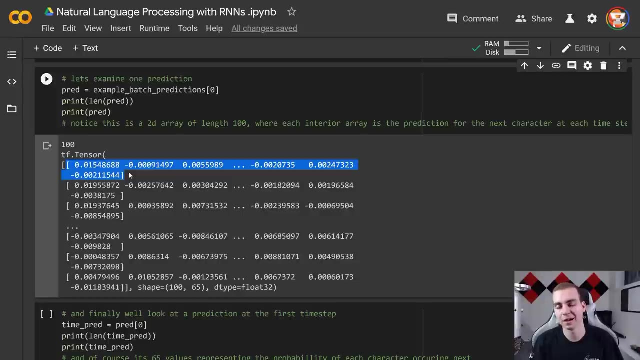 reason for this is because, at every single time step, which means the length of the sequence, right, because, remember, our recurrent neural network is going to feed one at a time, every word in the sequence. in this case, our sequences are length 100.. At every time step, we're actually saving that output as a, as a prediction. 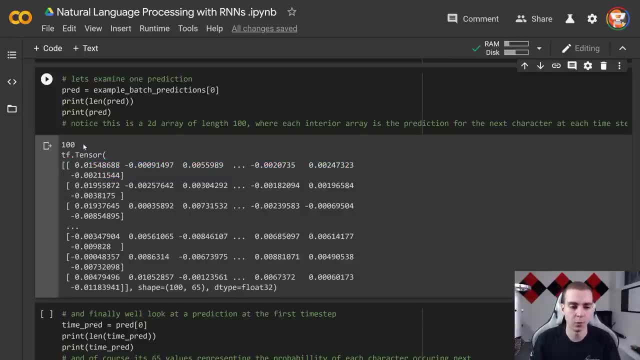 right And we're we're passing that back, So we can see that for one batch one training- sorry, not one batch one training- example- we get 100 outputs, And these outputs are in some shape. we'll talk about what those are in a second. So that's something to remember. 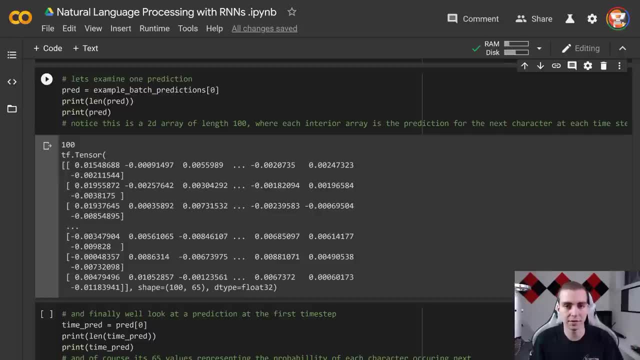 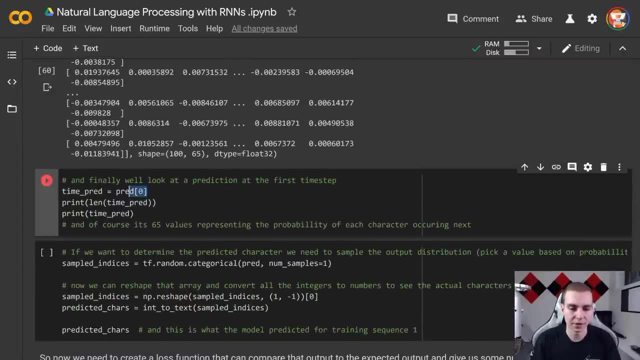 that for every single training example, we get, whatever the length of that training example was- outputs, because that's the way that this model works. And then, finally, we look at the prediction at just the very first time step. So this is 100 different time steps. 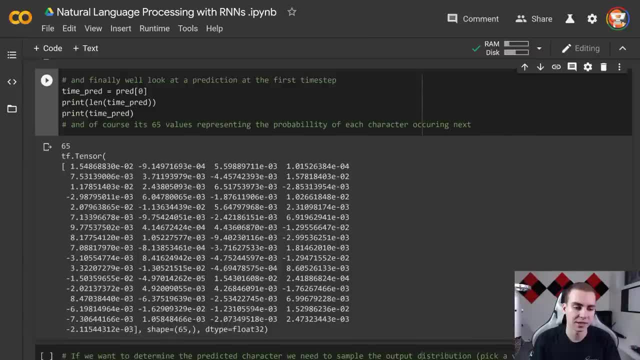 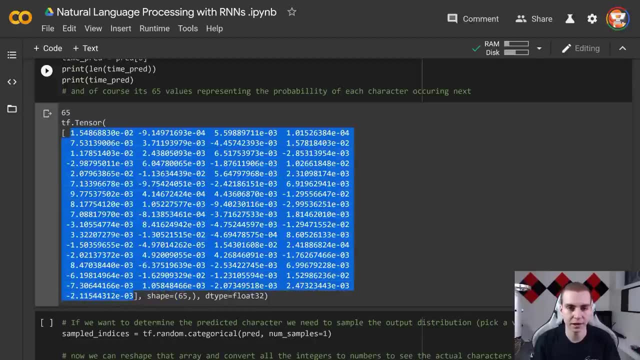 So let's look at the first time step and see what that prediction is. And we can see that now we get a tensor of length 65. And this is telling us the probability of every single character occurring next at the first time step. So that's what I wanted to show you. 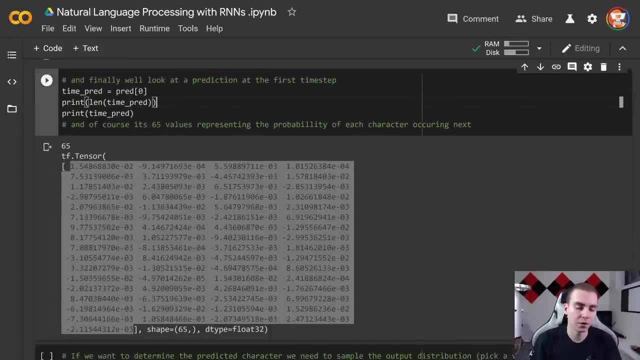 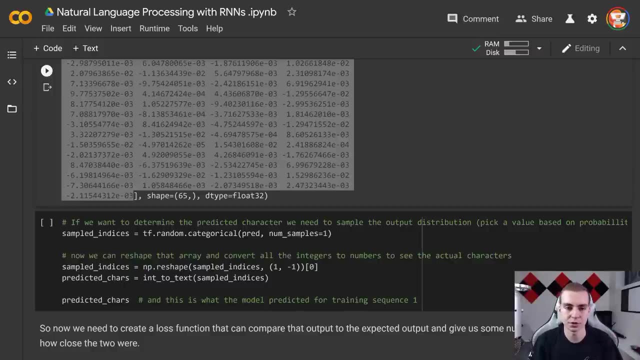 To walk through is showing you what's actually outputted from the model, the current way that it works, And that's why we need to actually make our own loss function to be able to determine how you know good our models performing when it outputs something ridiculous that looks. 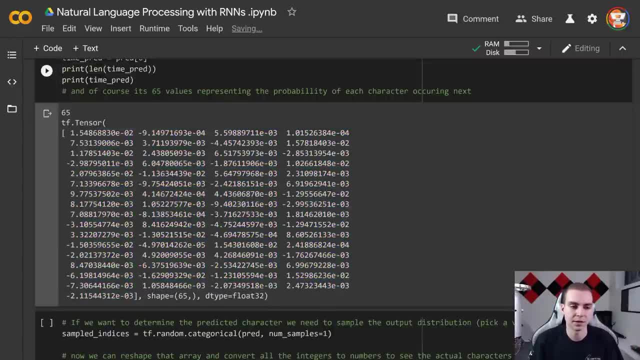 like this, because there is no just built in loss function in TensorFlow that can look at a three dimensional nested array of probabilities over you know the vocabulary size and tell us how different the two things are. So we need to make our own model And then, lastly, during our final 근, we have up to 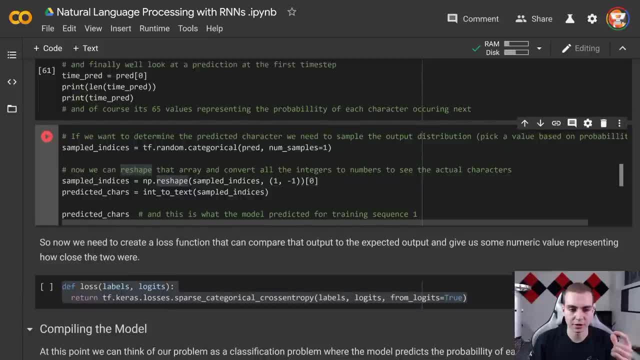 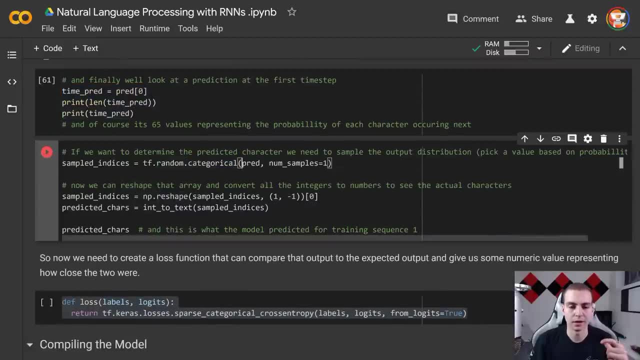 loss function. So if we want to determine the predicted character from this array, so we'll go there. now what we can do is get the categorical. with this call, we can sample the categorical distribution And that will tell us the predicted character. So what I? 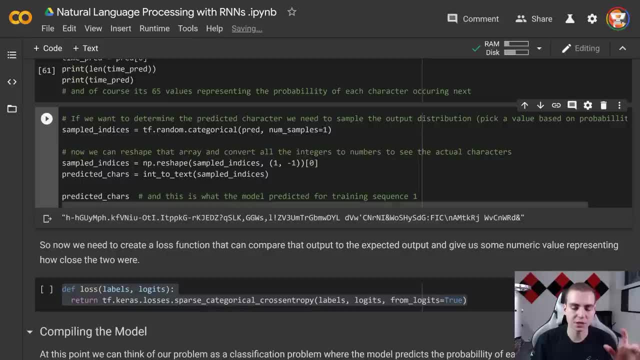 mean is: let's just look at this and then we'll explain this. So, since our model works on random weights and biases right now, we haven't trained it yet. this is actually all of the predicted characters that it had. So, at every time step, at the first time step. 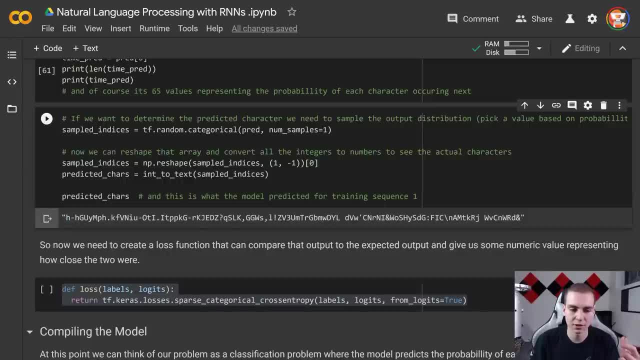 it predicted h, then a predicted hyphen, then h, then g, then you, and so on, so forth. you get the point right. So what we're doing to get this value is we're going to sample the prediction. So at this, this is just the first time step. actually- we're sample the 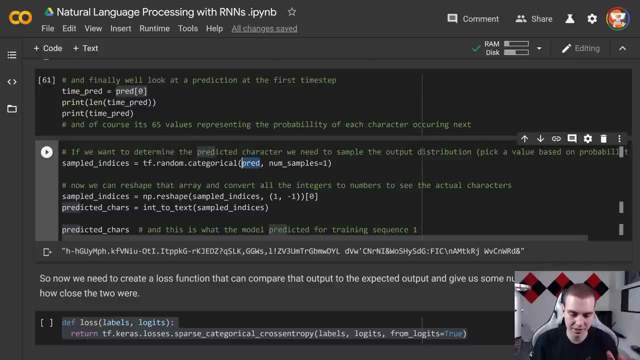 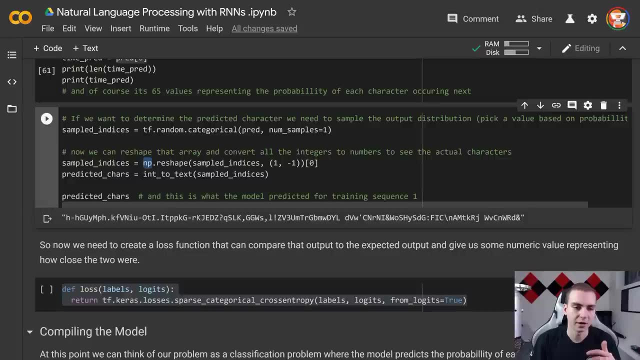 prediction. Actually, no, sorry, we're sampling every timestamp, my bad there. we're gonna say sampled indices equals np, dot reshapes or just reshapes- shaping this, just changing the shape of it. we're gonna say predicted characters equals. 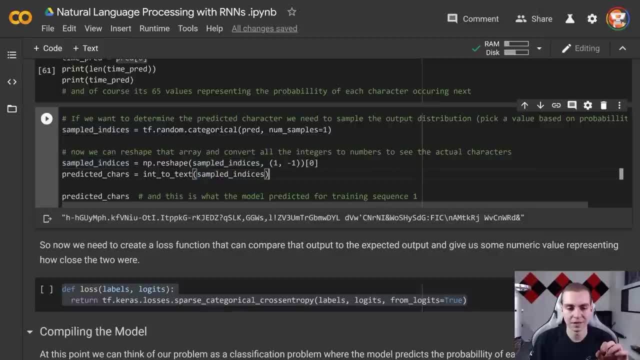 int to text sampled indices. So it's I really it's hard to explain all this if you guys don't have a statistics kind of background, a little bit to talk about why we're sampling and not just taking the argument max value of like this array, because you would think 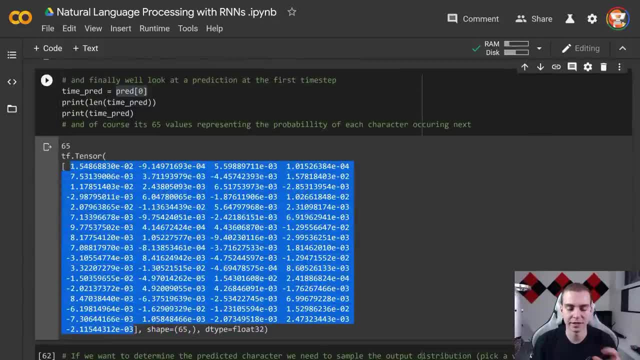 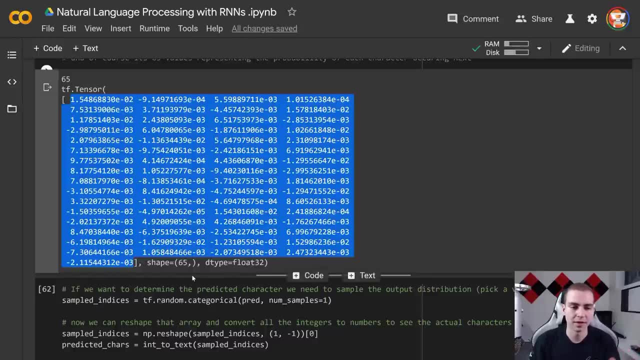 that what we'll do is just take the one that has the highest probability out of here, And that will be the index of the next predicted character. There's some issues with doing that for the loss function, just because if we do that, then what that means is we're going to kind of get stuck in an infinite loop, almost where. 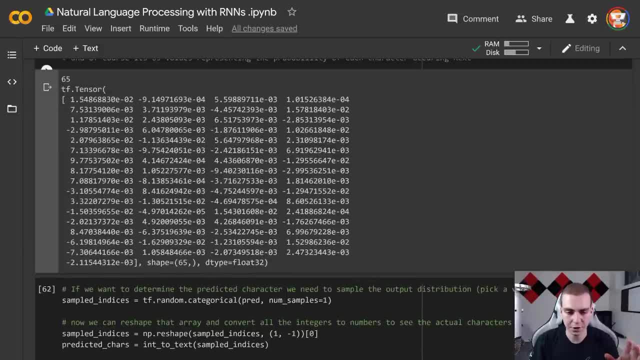 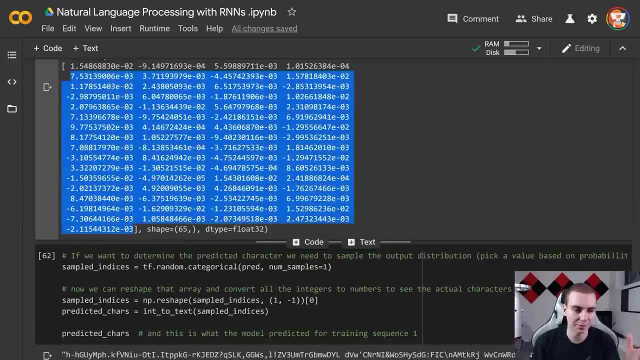 we just keep accepting the biggest character. So what we'll do is pick a character based on this probability distribution, kind of. Yeah, again it's hard, It's called sampling the distribution. You can look that up if you don't know what that means. But sampling. 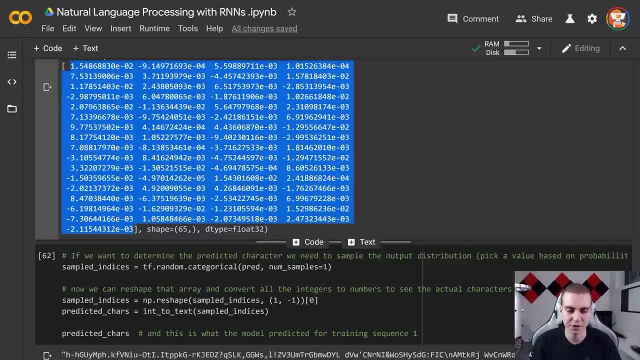 is just like trying to pick a character based on a probability distribution. It doesn't guarantee that the character with the highest probability is going to be picked. it just uses those probabilities to pick it. I hope that makes sense. I know that was like a really rambly definition. 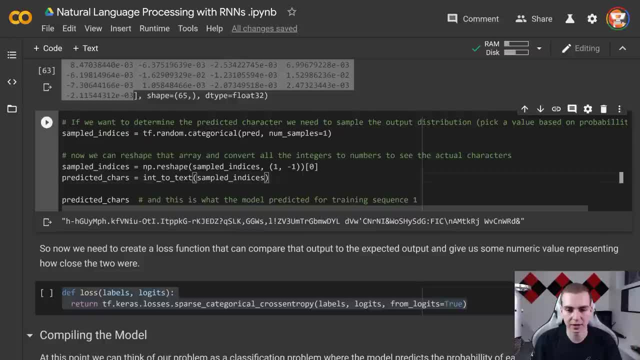 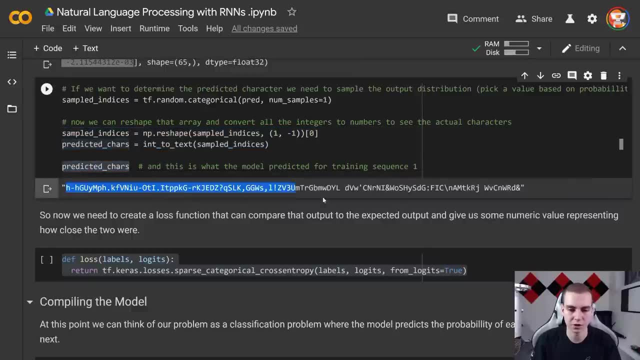 but that's the best I can do. So here we reshape the array and convert all the integers to numbers to see the actual characters. So that's what these two lines are doing here, And then I'm just showing the predicted characters by showing you this, And you know the character. 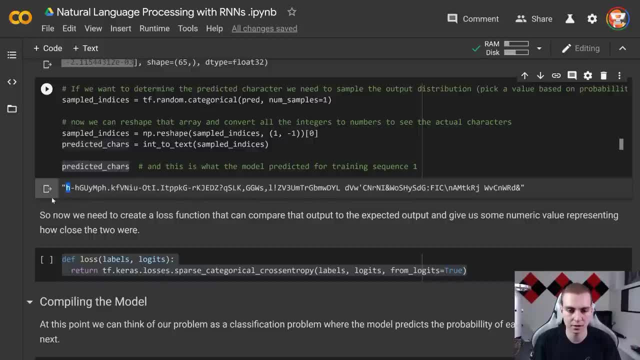 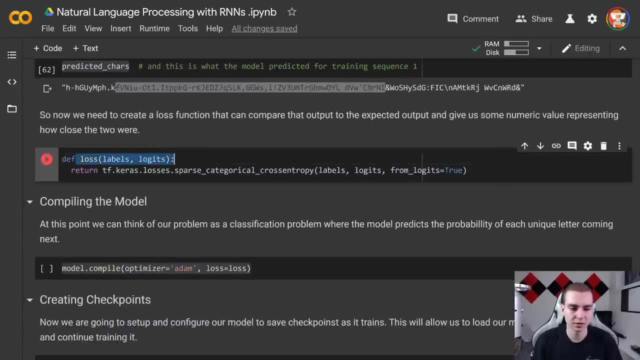 here is what was predicted at time: step zero to be the next character, and so on. Okay, so now we can create a loss function that actually handles this for us. So this is the loss function that we have. Keras has like a built in one that we can utilize, which is what we're doing. But what? 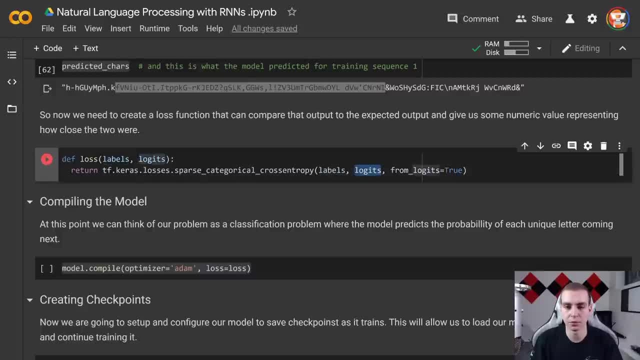 this is going to do is take all the labels and all of the probability distributions, which is what this is- logits- I'm not going to talk about that really- And we'll compute a loss on those. So, how different or how similar those two things are, Remember the goal of 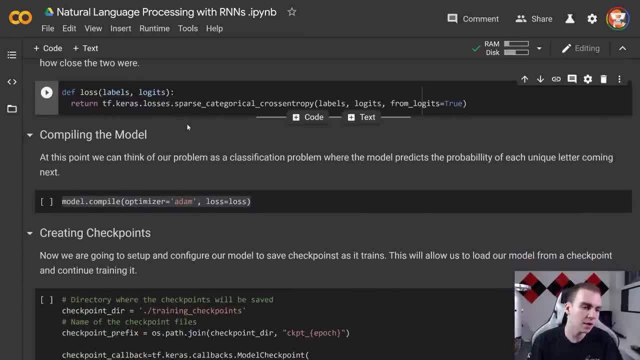 our algorithm in the neural network is to reduce the loss, right, Okay. so next we're going to compile the model, which we'll do here. So we're going to compile the model with the atom optimizer and the loss function as loss. 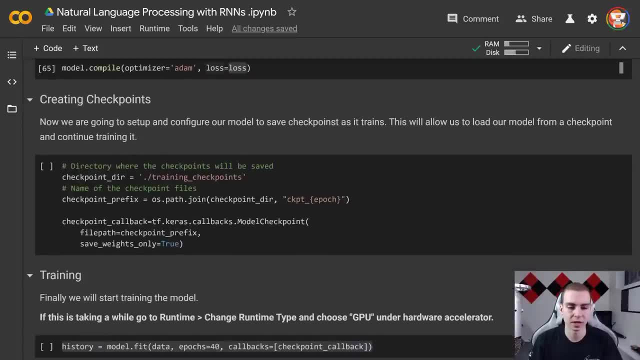 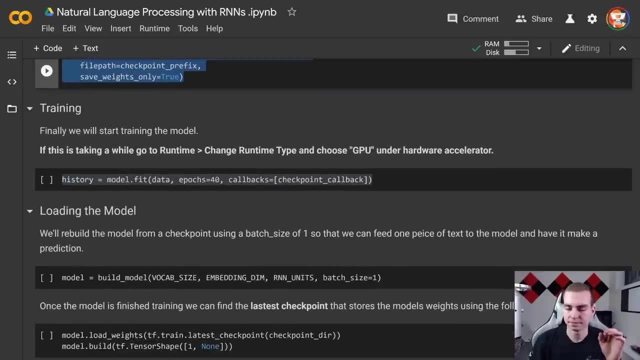 Which we defined here, And now we're going to set up some checkpoints. I'm not going to talk about how these work. you can kind of just read through this, if you want- And then we're going to train the model. Remember to start your GPU hardware accelerator under. 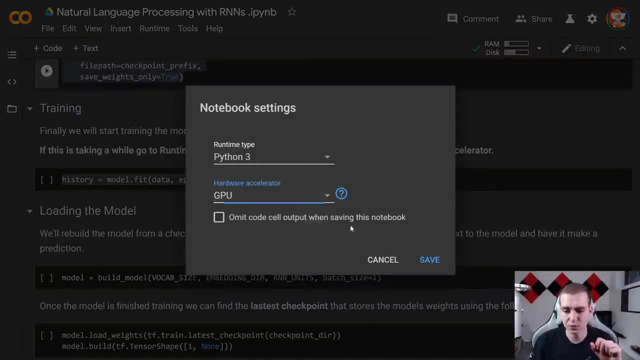 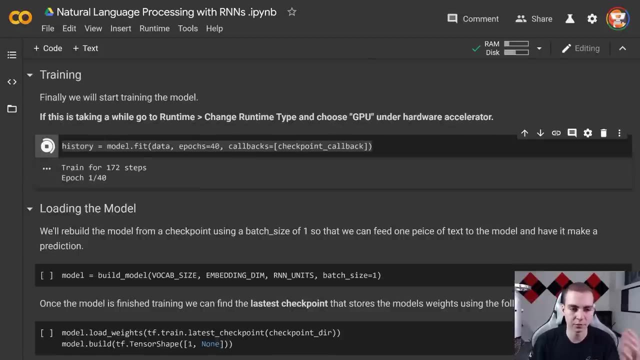 runtime change, runtime type GPU, because if you do not, then this is going to be very slow. But once you do that, you can train the model. I've already trained it. But if we go through this training we can see it's going to say train for 172 steps And then 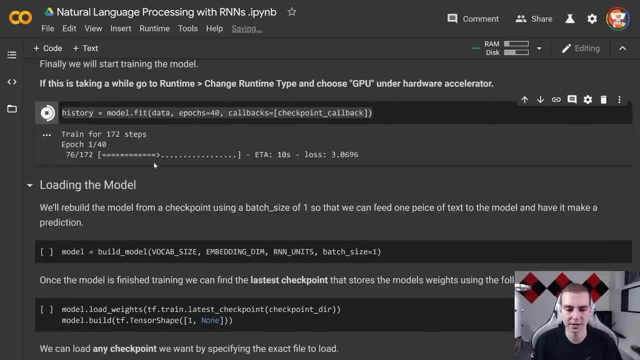 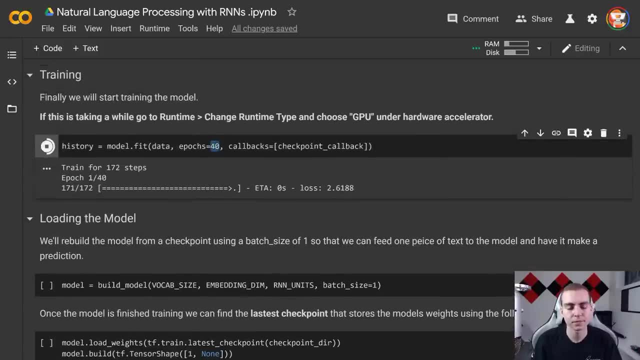 it's going to take about. you know, 30 seconds per epoch, probably, maybe a little bit less than that, And the more epochs you run this for, the better it will get. this is a different. we're not likely going to overfit here, So we can run this for, like, say, 100 epochs. 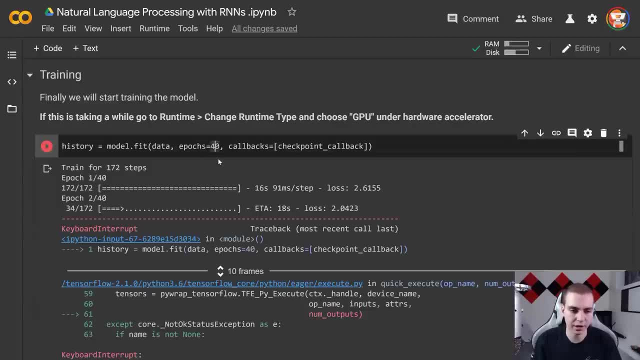 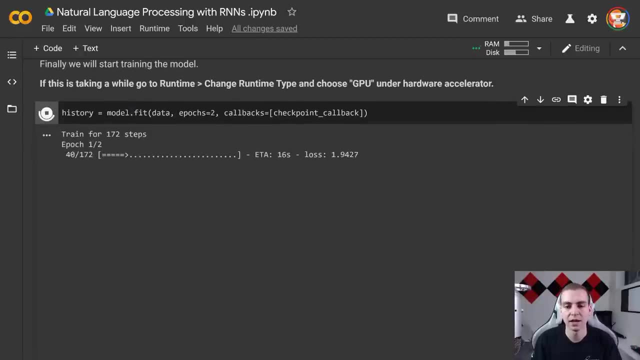 if we wanted to. for our case, let's actually start by just training this on, let's say, two epochs, just to see how it does, And then we'll train it on like 1020, 4050, and compare the results. But you'll notice, the more epochs the better it's going to get. But just like 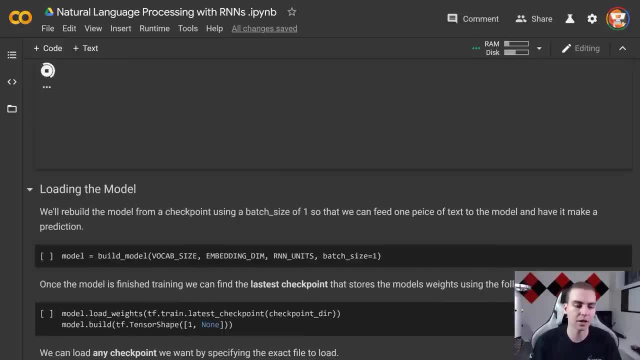 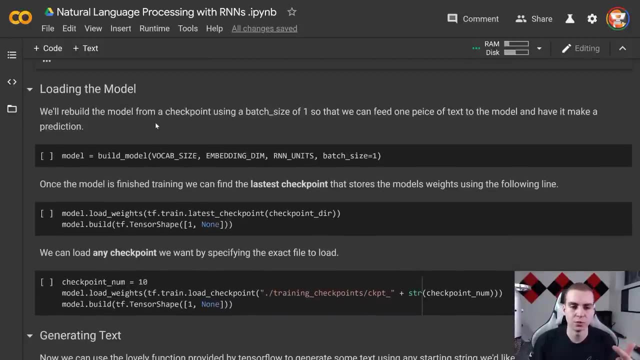 for our case, we'll start with two and then we'll work our way through it And then we'll work our way up. So while that trains, we'll actually explain the next aspect of this without running the code. So, essentially, what we need to do after we've trained the model of 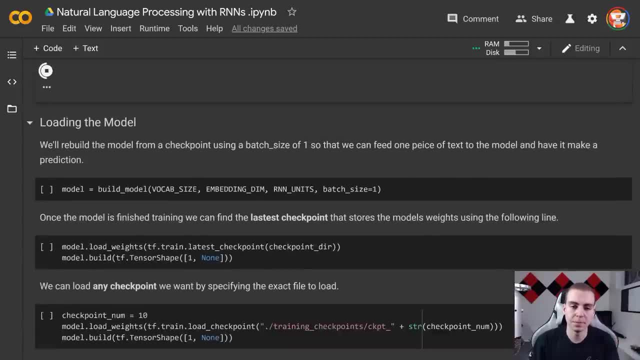 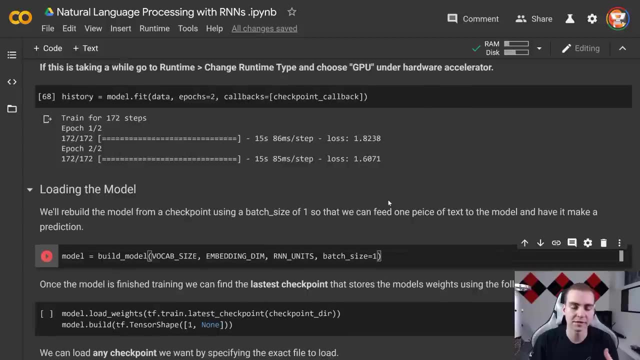 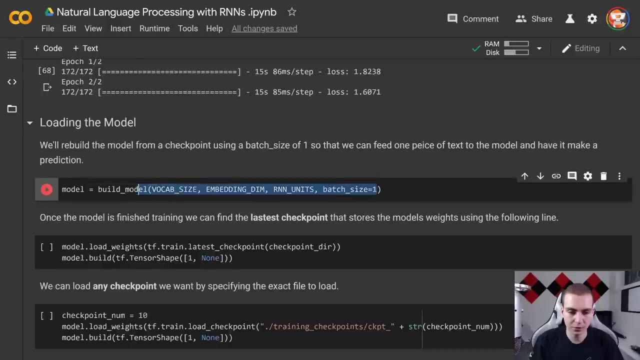 initialize the weights and biases. we need to rebuild it using a new batch size of one. So remember, the initial batch size was 64, which means that we'd have to pass it 64 inputs or sequences for it to work properly. But now what I've done is I'm going to rebuild. 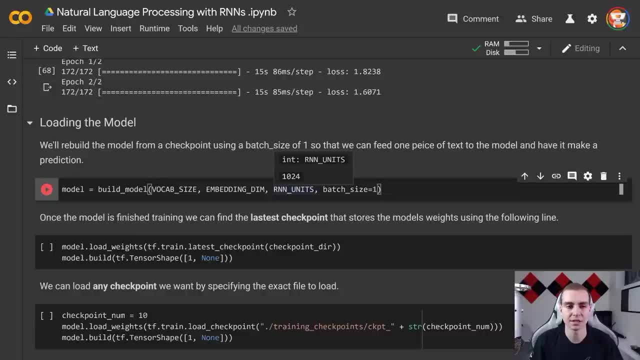 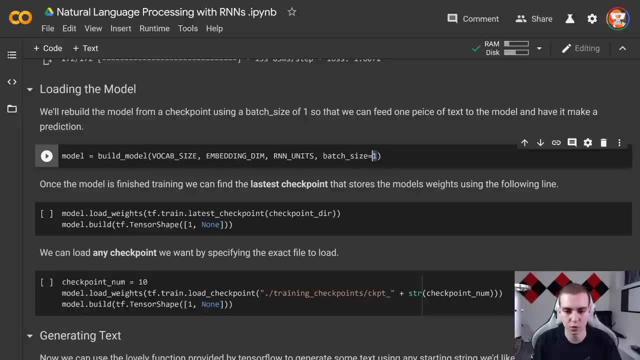 the model and change it to a batch size of one, So that we can just pass it some sequence of whatever length we want, and it will work. So if we run this, we've rebuilt the model with batch size one. that's the only thing. 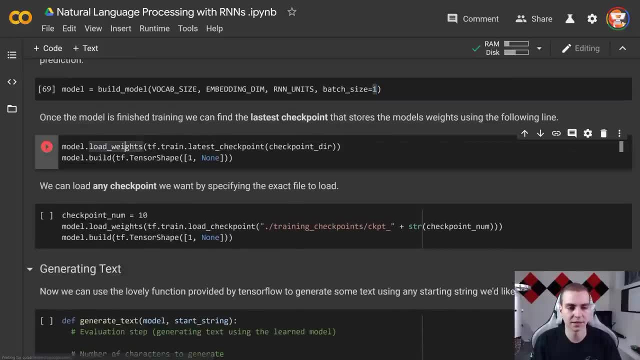 we've changed And now what I can do is load the weights by saying model dot, load weights tf, dot, train, dot, latest checkpoint, checkpoint directory, and then build the model using the tensor shape one. none, I know sounds strange. This is how we do this: rebuild the model one. 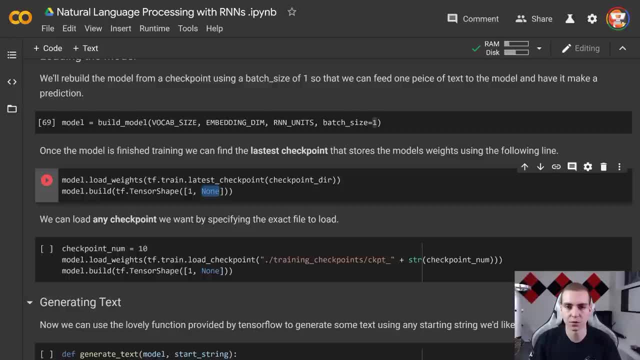 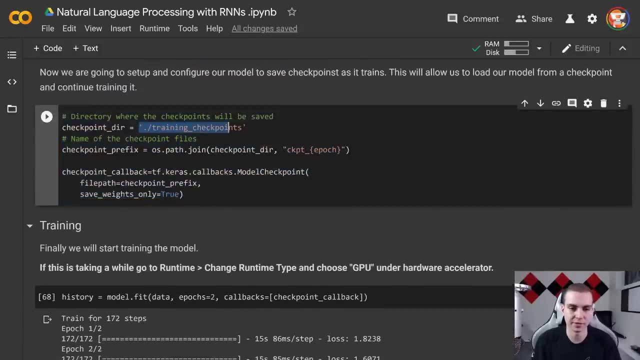 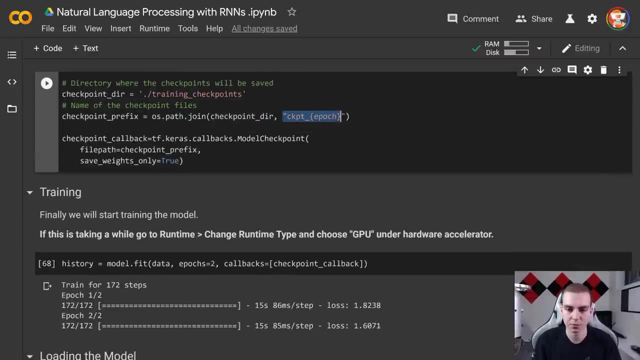 none. It's just saying expect the input one and then none means we don't know what the next dimension length will be. But here checkpoint directory is just: we've defined where on our computer we're going to save these TensorFlow checkpoints. This is just saying this is the 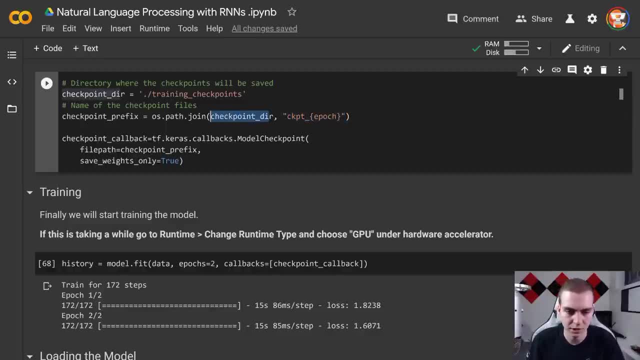 was the prefix we're going to save the checkpoint with. So we're going to do the checkpoint directory And then checkpoint epoch, where epoch will stand for, obviously, whatever epoch we're on. So we'll save checkpoint here. we'll save a checkpoint. 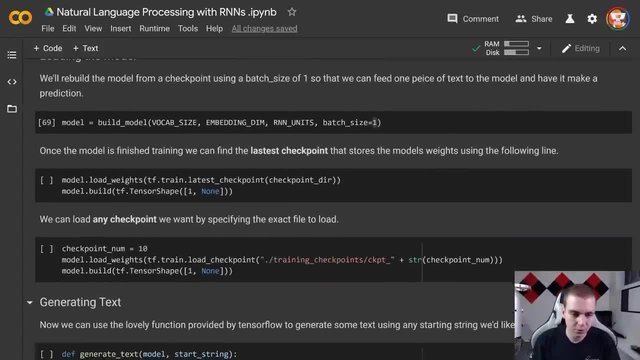 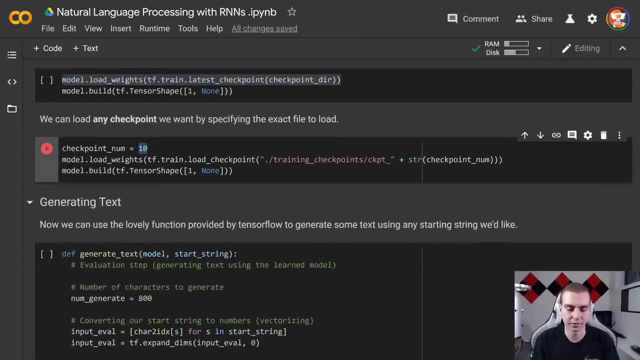 At epoch one checkpoint, at epoch two to get the latest checkpoint. we do this And then if we wanted to load any intermediate checkpoint, say like checkpoint 10, which is what I've defined here- we can use this block of code down here And I've just hardwired the checkpoint. 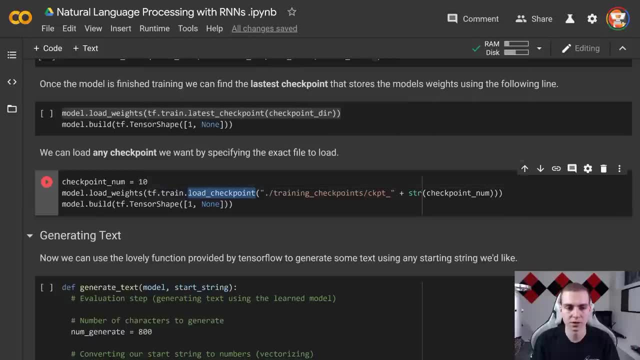 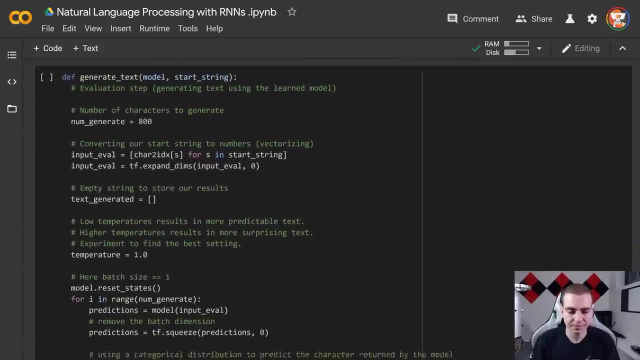 that I'm loading by saying tf, dot, train dot, load checkpoint, whereas this one just gets the most recent. So we'll get the most recent, which should be checkpoint two for me, And then what we're going to do is generate the text. So this function, I'll dig into it in. 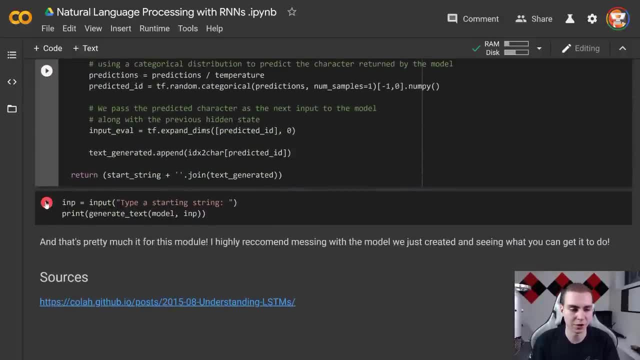 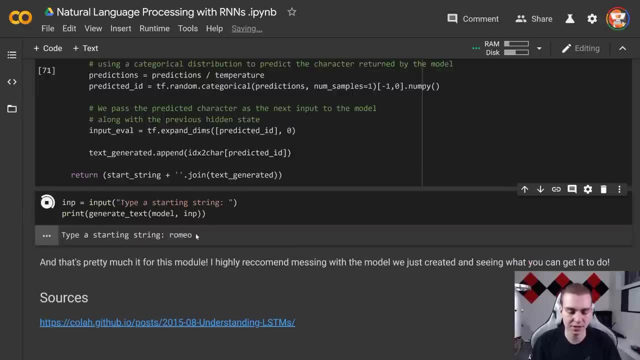 a second. I'll show you how this works, because I feel like we've done a lot of work for not very many results right now, And I'm just going to type in the string Romeo and just show you that when I do this, we give it a second And it will actually generate an output sequence. 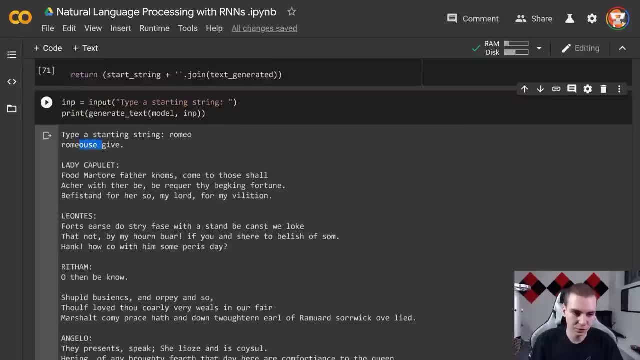 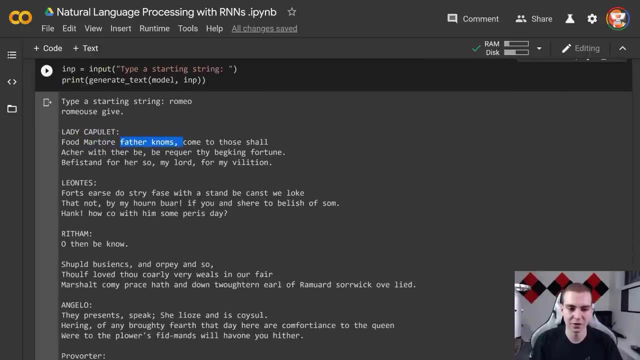 like this. So we have Romeo us give. this is the beginning of our sequence that says: lady Capulet, food Marathon, father gnomes, come to those shall write. so it's like pseudo English. Most of it are like kind of proper words, But again this is because we trained it on. 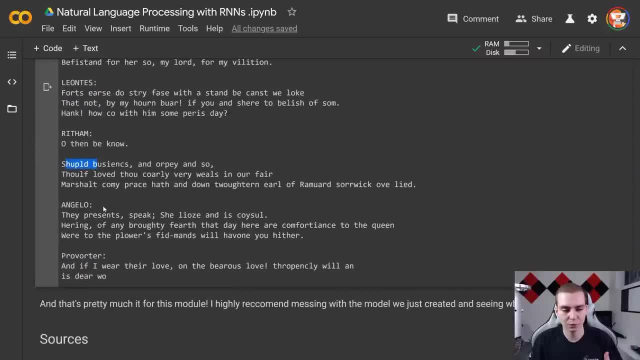 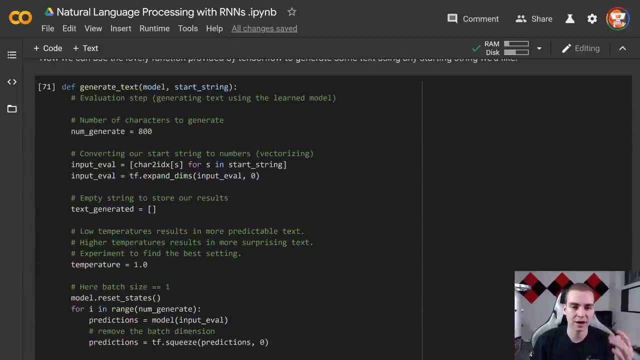 just two epochs. So I'll talk about how we build this in a second. But if you want it a better output for this part, then you would train this on more epochs. So now let's talk about how I actually generated that output. So we rebuilt the model to accept a batch size of 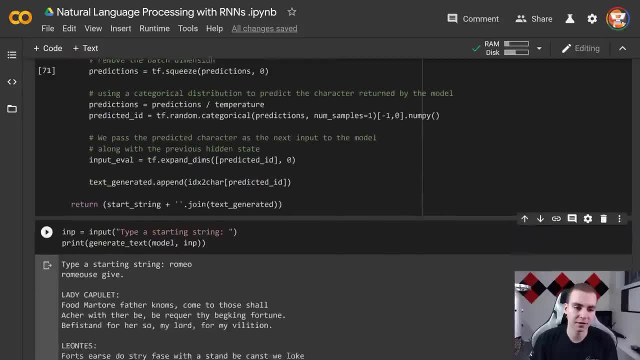 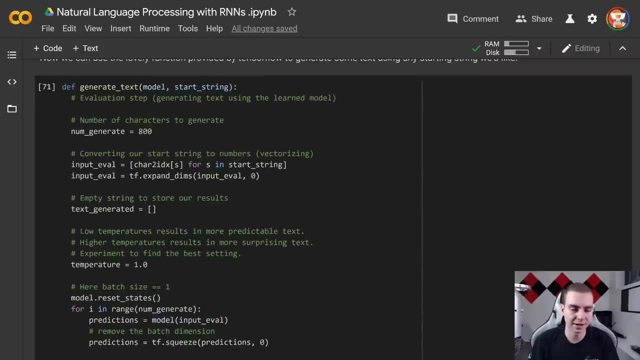 one, which means that I can pass it a sequence of any length, And, in fact, what I start by doing is passing the sequence that I've typed in here, which was Romeo. then what that does is we run this function generate text. I just stole this from TensorFlow, his website, like. 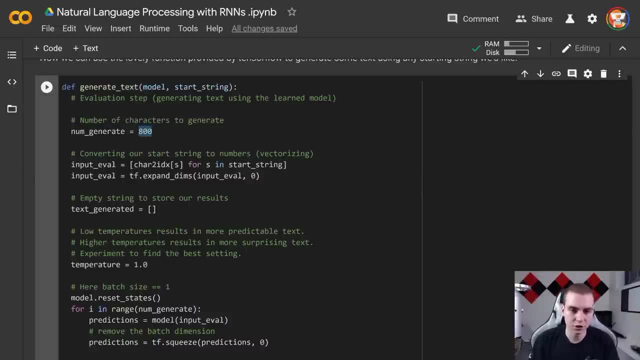 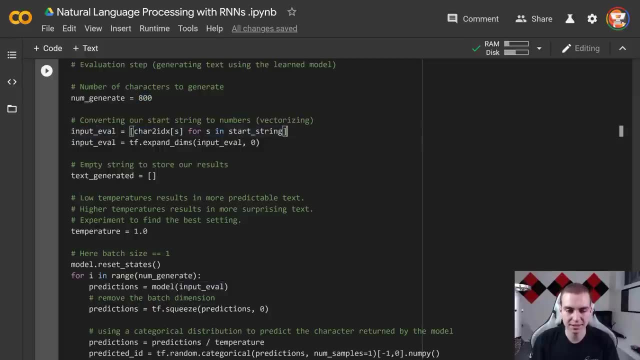 I've stolen almost all of this code. And then we say: the number of characters to generate is 800.. The input evaluation, which is now like we need to pre process this text again so that this works properly. we could use my little function or we can just write this: 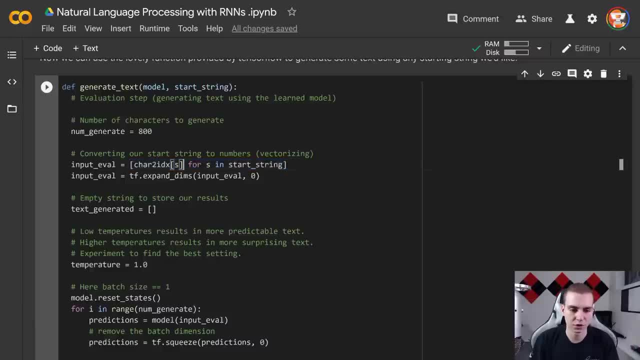 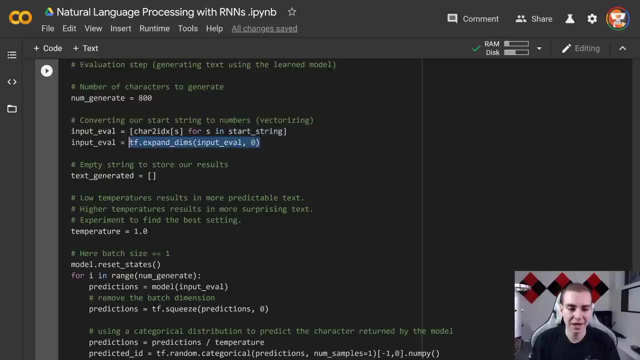 line of code here which does what the function that I wrote does for us. So char to ID x, s for s and start string. start string is what we typed in in that case, Romeo, then what we're going to do is expand the dimensions So essentially turn just a little bit of. 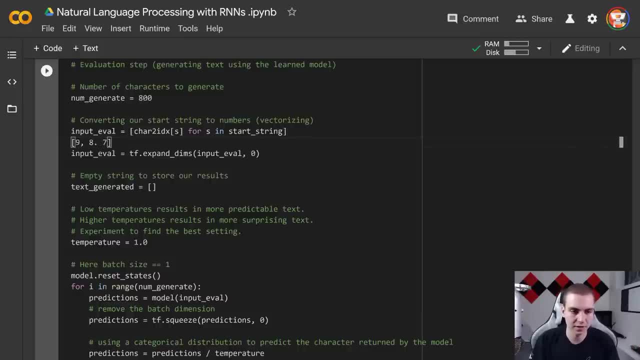 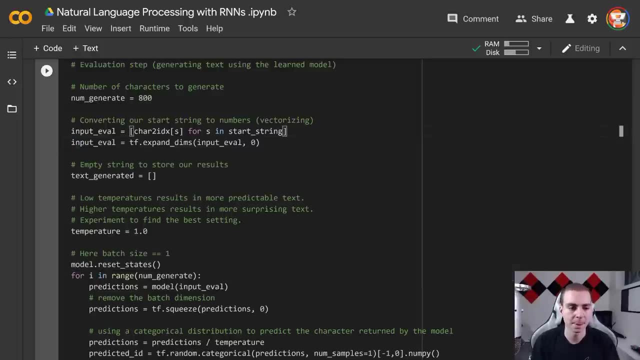 list like this that has all these numbers, the 987, into a double list like this or just a nested list, because that's what it's expecting as the input- one batch, one entry. then what we do is we're going to say the string that we want to store because we want to print. 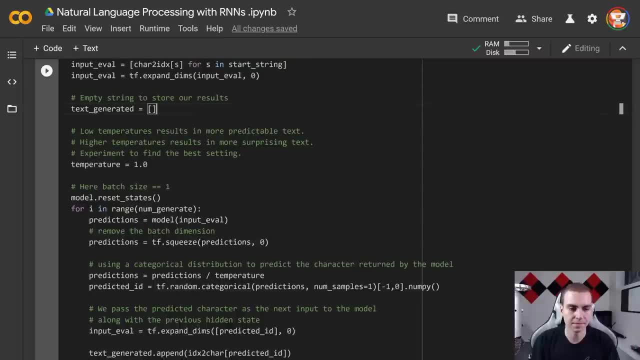 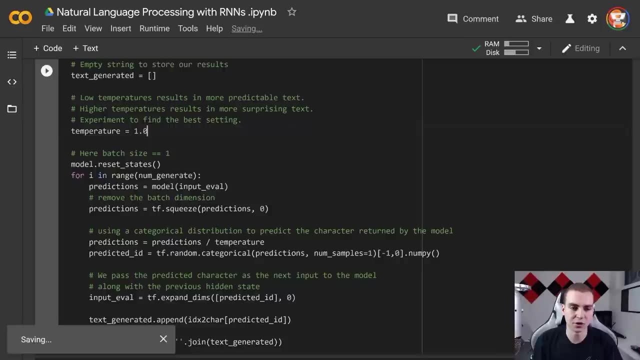 this out at the end, right, we'll put in this text: generated list. temperature equals 1.0,. what this will allow us to do is if we change this value to be higher. I mean, you can read the comment here, right: low temperature results in more predictable text. higher temperature. 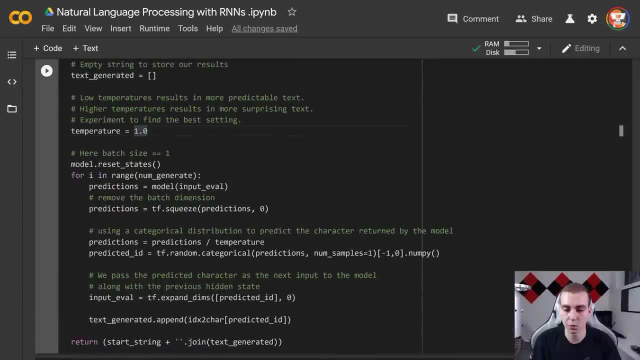 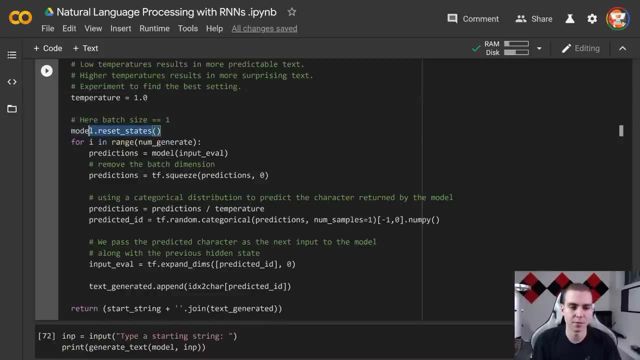 results in more surprising text. So this is just a parameter to mess with if you want. you don't necessarily need it, And I would like I've just left mine at one for now. we're going to start by resetting the states of the model. This is because when we rebuild, 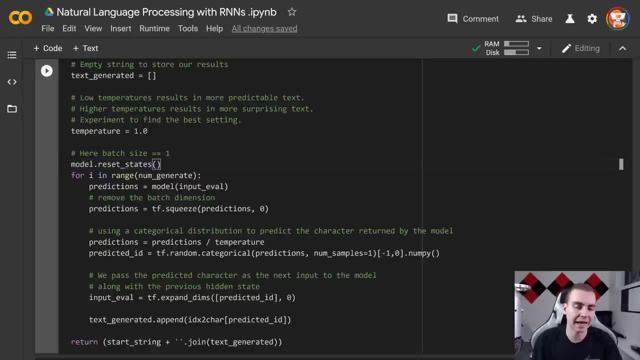 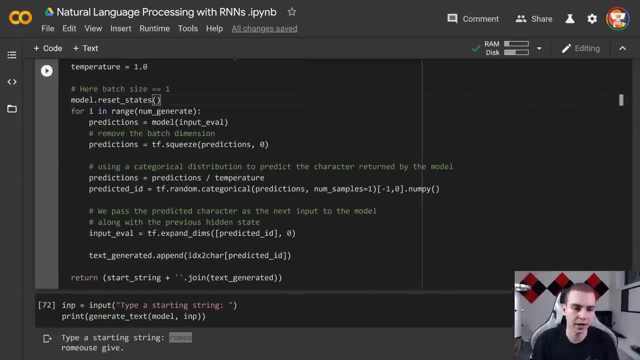 the model, it's going to have stored the last state that it remembered when it was training. So we need to clear that before we pass new input text to it And we say for I in range num generate, which means however many characters we want to generate, which is 800. Here what? 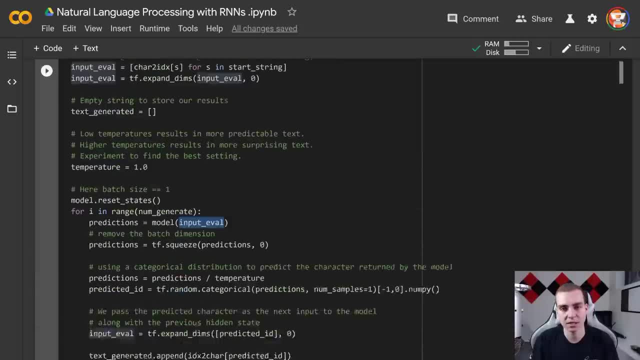 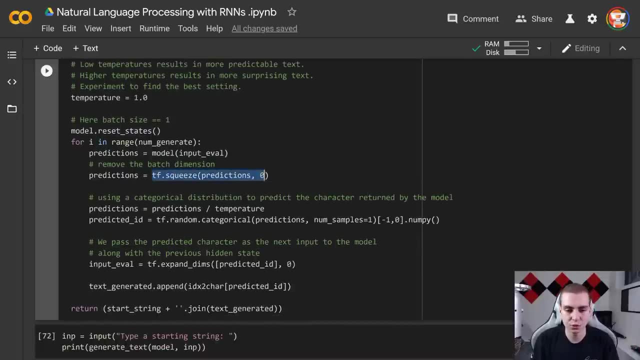 we're going to do is say: predictions equals model input of Val. that's going to start as the start string that's encoded right. And then what we're going to do is say: predictions equals tf dot squeeze, prediction zero. what this does is take our predictions, which is going to be in a nested list, and just removes. 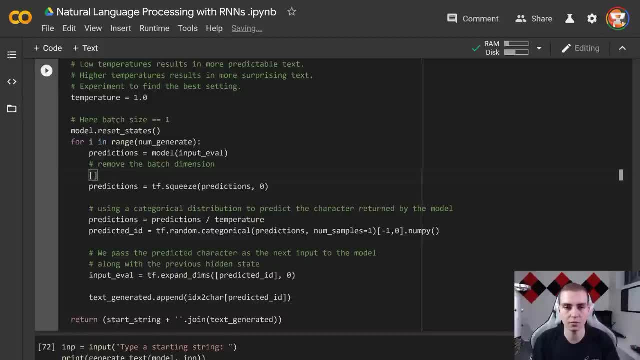 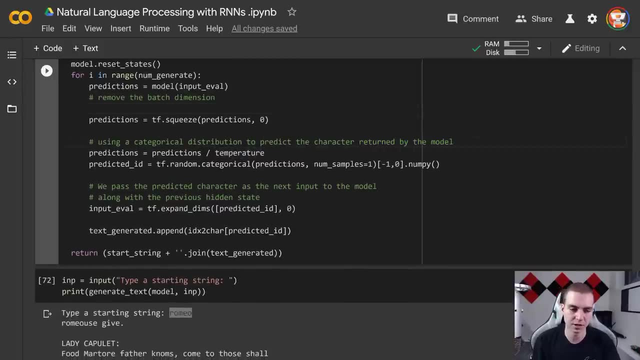 that exterior dimension. So we just have the predictions that we want. we don't have that extra dimension that we need to index again. And then we're going to say, using a categorical distribution to predict the character returned by the model. that's what it writes here. 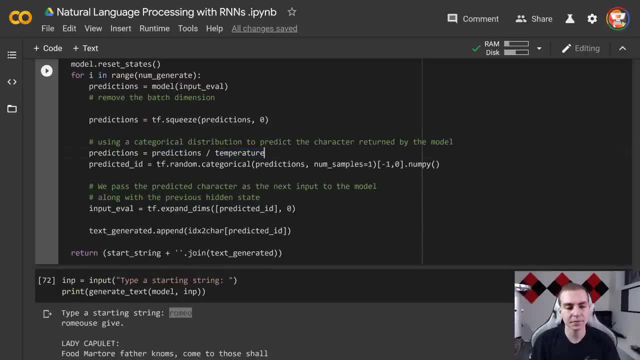 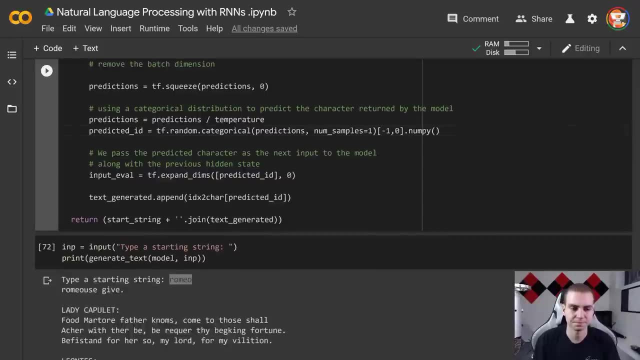 will divide by the temperature. if it's one, that's not going to do anything. So we're going to say: predicted ID: equals will sample whatever the output was from the model, which is what this is doing, And then we're going to take that output, So the predicted ID. 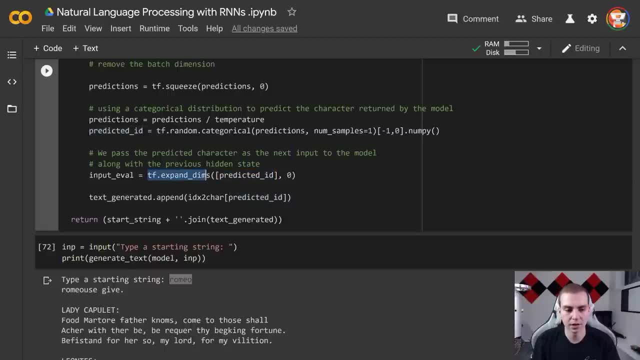 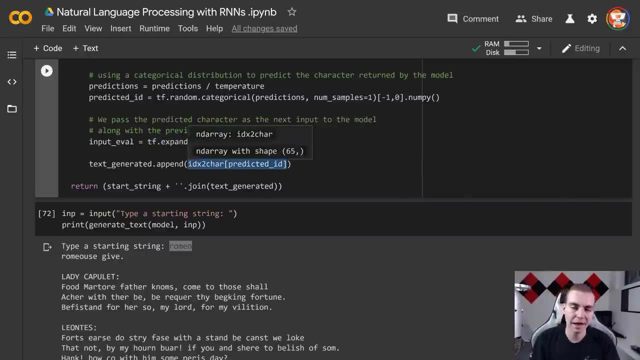 and we're going to add that to the input evaluation. And then what we're going to say is: text generated, dot append, and we're going to convert the text that are integers now back into a string and return all of this. Now, I know this seems like a lot. 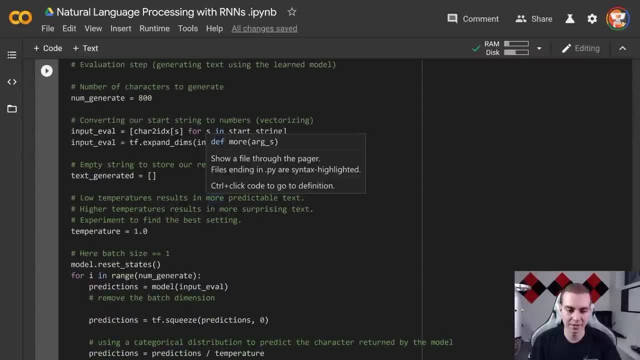 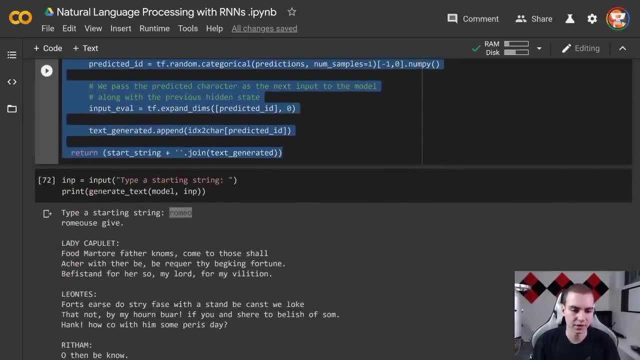 Again, this is just given to us by TensorFlow to you know, create this aspect. you can read through the comments yourself if you want to understand it more, but I think that was a decent explanation of what this is doing. So, yeah, that is how we can generate you. 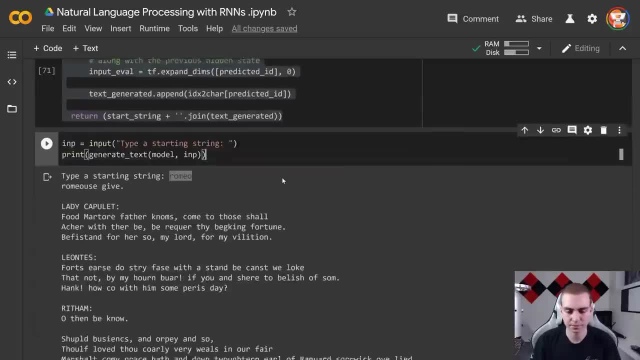 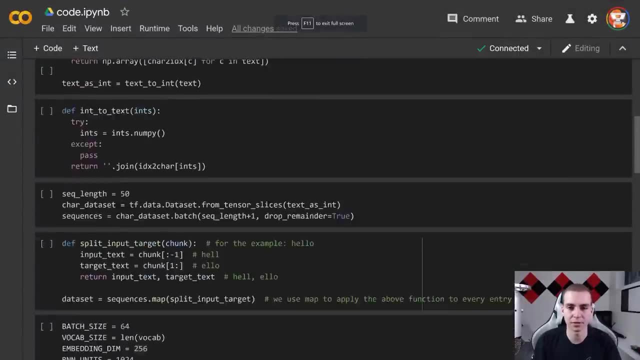 know sequences using recurrent neural network. Now what I'm going to do is go to my other window here where I've actually typed all the code just in full, and do a quick summary of everything that we've done, just because there was a lot that went on, And then from 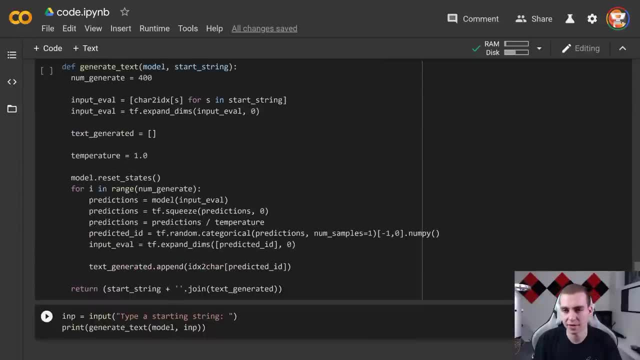 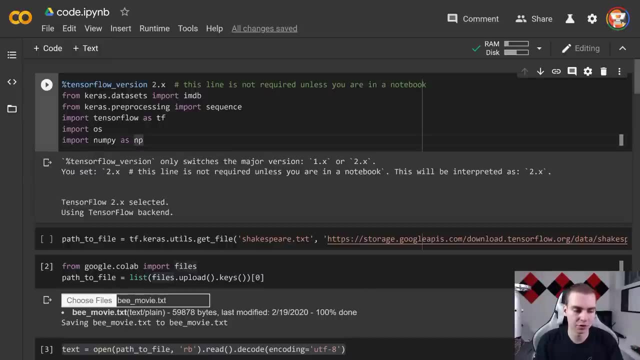 there. I'm actually going to train this on a B movie script and show you kind of how that works in comparison to the Romeo and Juliet. Okay, so what I'm in now is just the exact same notebook we have before, but I've just pretty much copied all the text in here, Or it's the exact same. 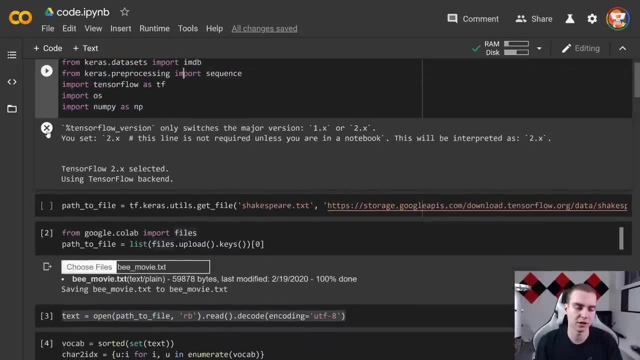 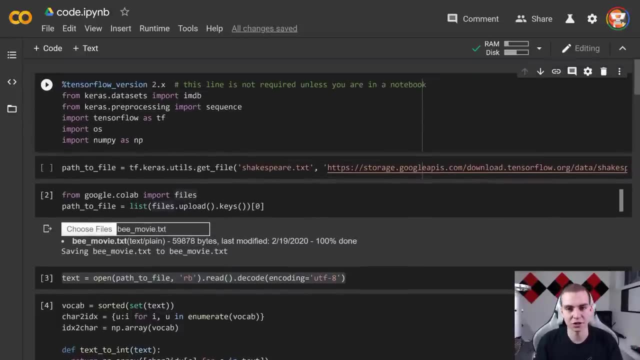 code we had before, So we just don't have all that other text in between. So I can kind of do a short summary of what we did as well as show you how this worked when I trained it on the B movie script. So I did mention I was going to show you that I'm not lying. 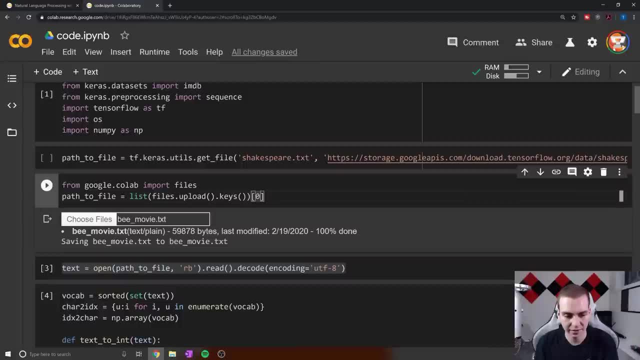 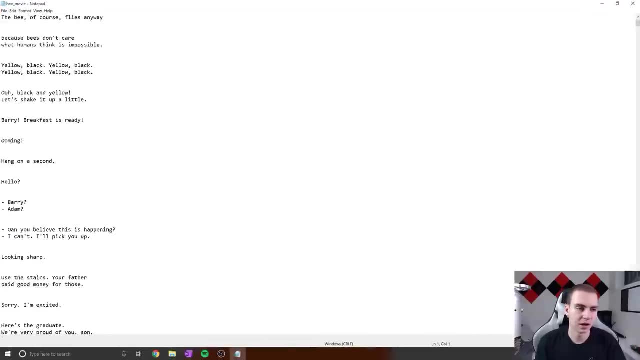 I will show. you can see, I've got B movie dot txt loaded in here And in fact actually I'm going to show you this script first, to show you what it looks like. So this is going to show you what the B movie script looks like. You can see it just like a long you. 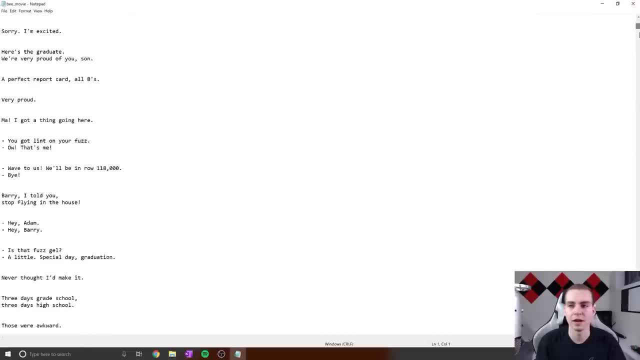 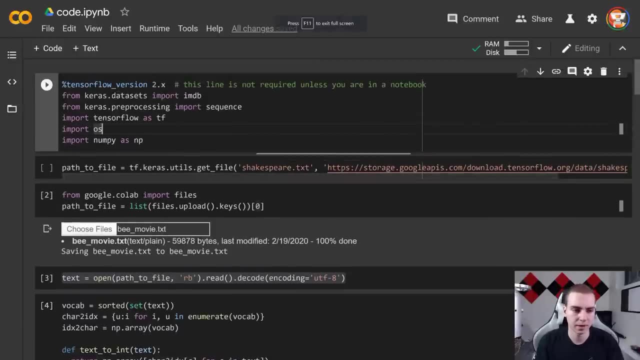 know. script of text. I just downloaded this for free off the internet And it's actually not as long as the Romeo and Juliet play, So we're not going to get as good of results from our model, But it should hopefully be okay. So we just start and I'm just gonna. 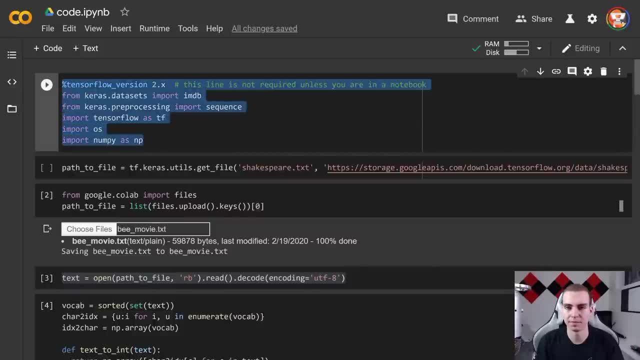 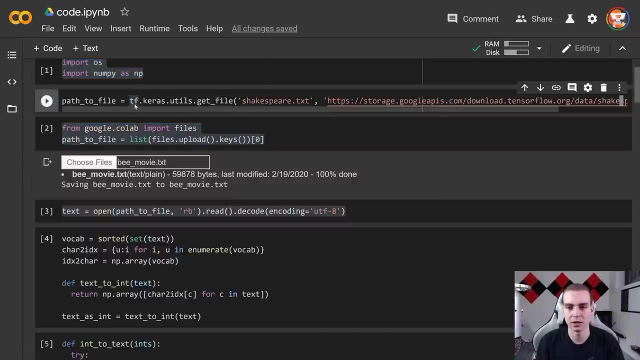 do a brief summary And then I'll show you the results from the B movie script, just so that people that are confused maybe have something that wraps it up. here We're doing our imports. I don't think I need to explain that. this part up here is just loading in your file. 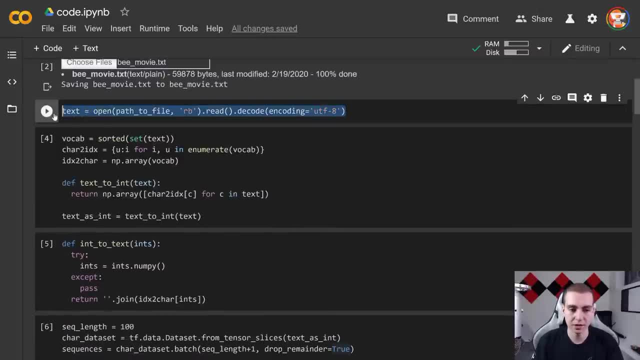 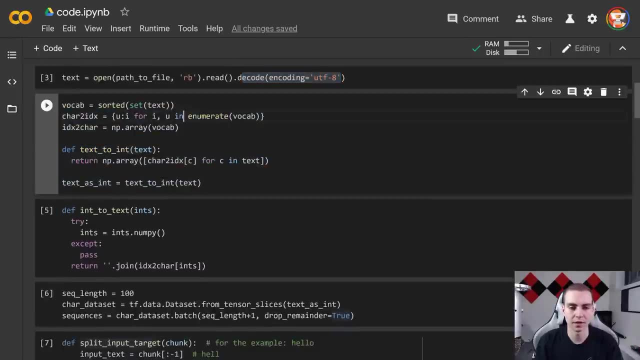 Again, I don't think I need to explain that. Then we're actually going to read the file, So open it from our directory, decode it into UTF Eight. we're going to create a vocabulary and encode all of the text that's inside of. 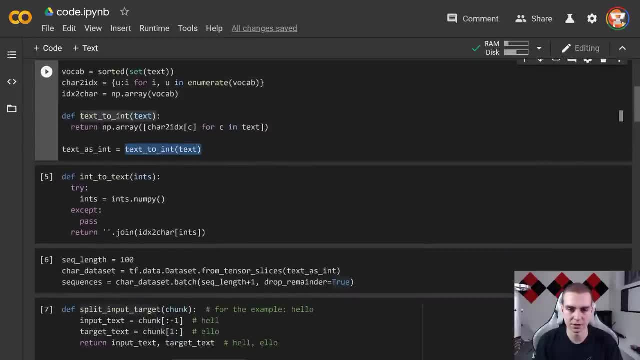 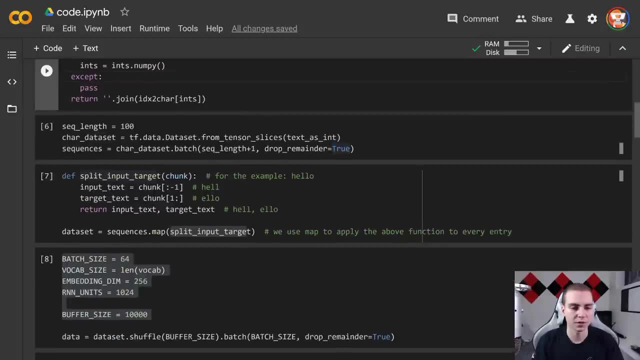 this file, Then what we're going to do is turn all of that text out into, you know, the encoded version. we're writing a function here that goes the other way around, So from into to tax, not from text to int. we're going to define the sequence length that we want. 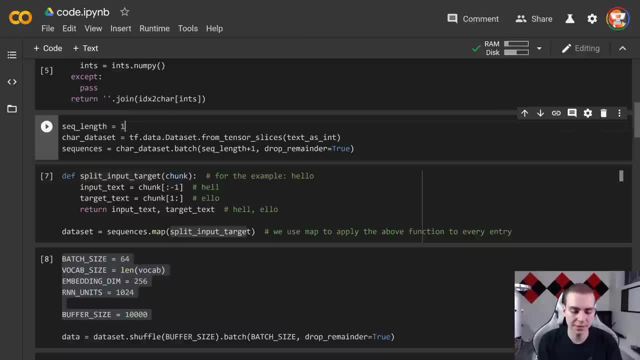 to train with, which will be sequence length of 100,. you can decrease this value if you want. you go 50.. 20, it doesn't really matter, it's up to you. It just that's going to determine how. 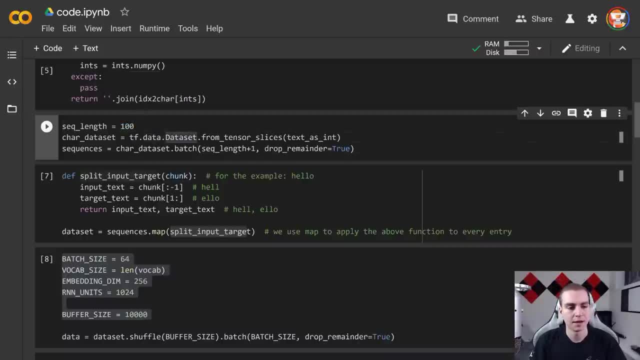 many training examples you're going to have. right is the sequence length. Next, what we're going to do is create a character data set from a tensor- slices from text as int. what this is going to do is just convert our entire text- that's now an integer array- into a bunch. 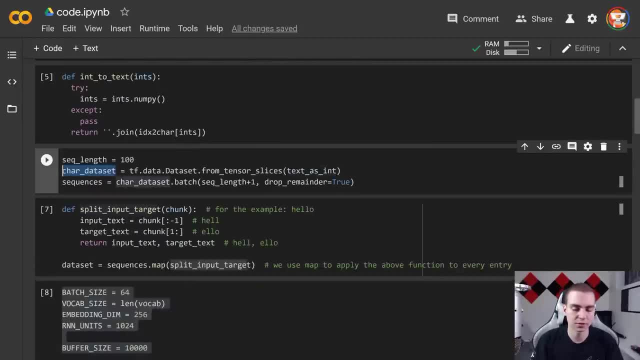 of slices of characters. So that's what this is doing here. So are not slices what I'm saying. you're just going to convert, like split, that entire array into just characters, like that's pretty much it. So that's what we're going to do. So we're going to create. 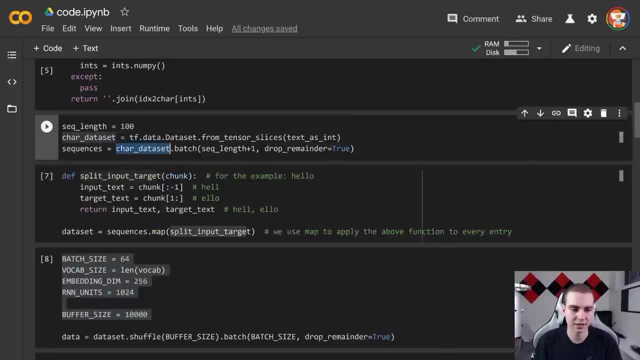 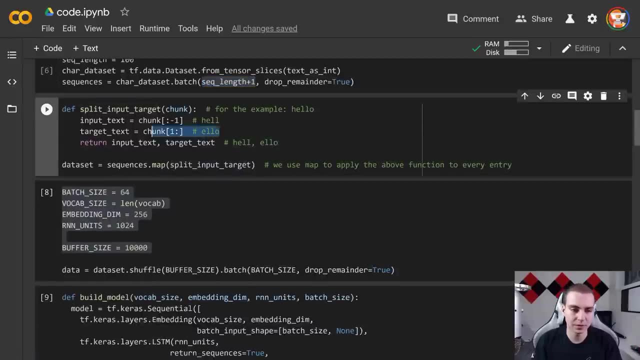 a data set, And then we're going to say: sequences equals char, data set, dot batch, which now is going to take all those characters and batch them in lengths of 101.. What we're going to do then is split all of that into the training examples. So, like this, right he ll, and. 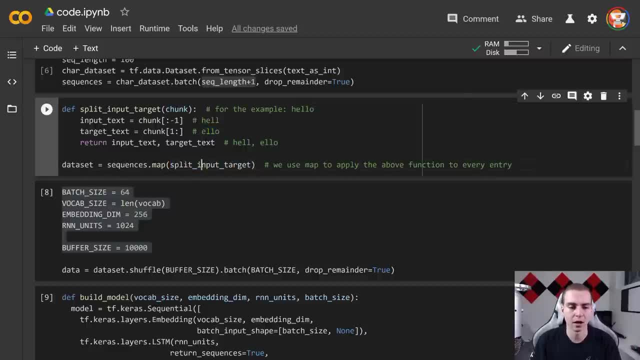 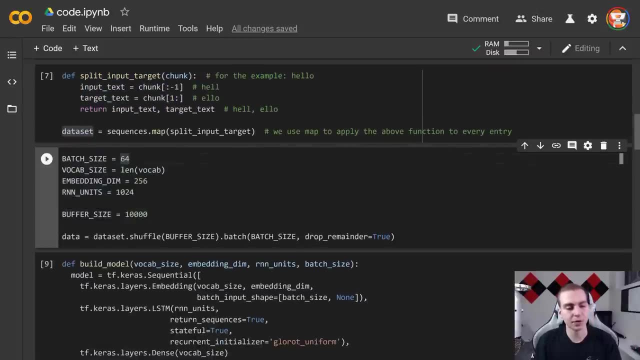 then he ll. we're going to map this function to sequences, which means we're going to apply this to every single sequence and store that in data set. then we're going to find the parameters for our initial network. we're going to shuffle the data set. 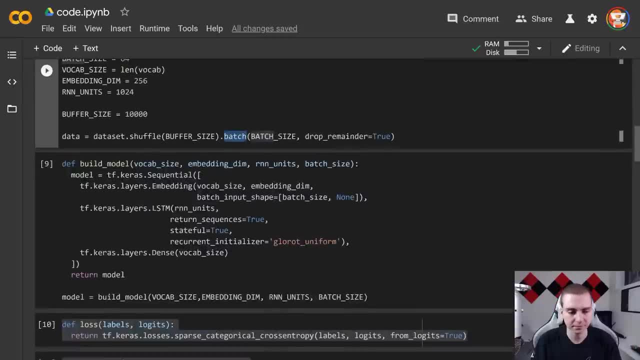 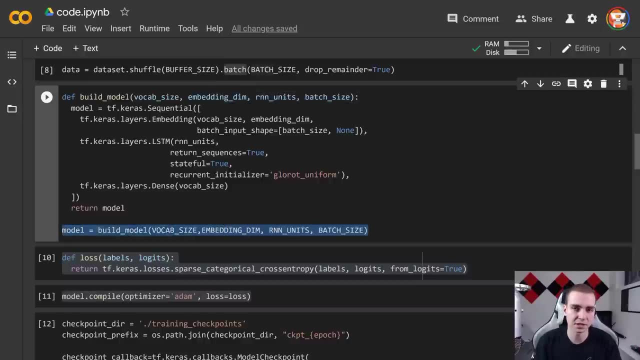 And batch that into now- 64 training examples, then we're going to make the function that builds the model, which I've already discussed. we're going to actually build the model starting with a batch size of 64, we're going to create our loss function, compile the model set. 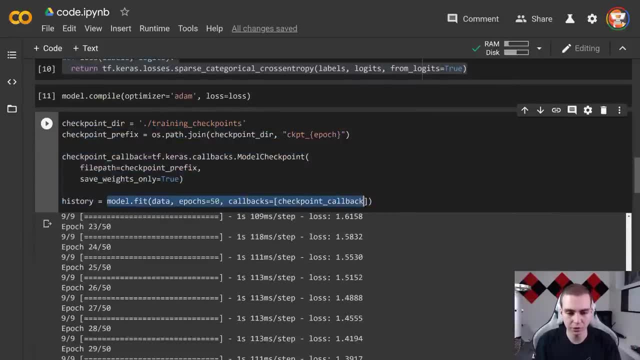 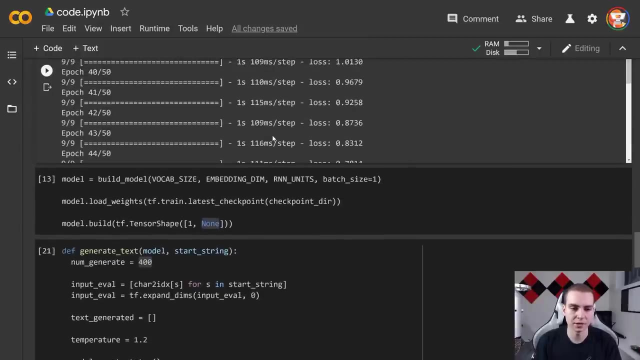 our checkpoints for saving and then train the model and make sure that we say checkpoint callback as the checkpoint callback for the model, which means it's going to save every epoch the weights that the model had computed at that epoch. So after we do that, then our models train. So we've trained the model. you can see I 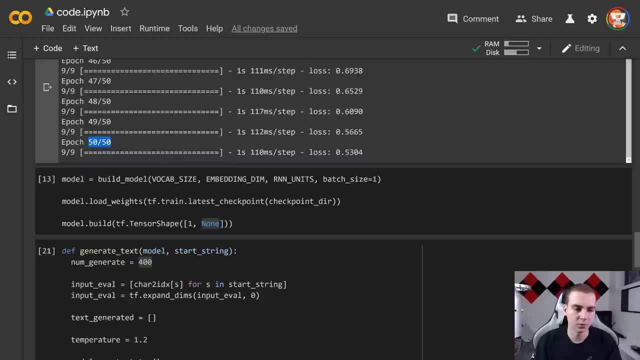 trained this on 50 epochs for the B movie script. And then we're going to do is build the model now with a batch size of one, So we can pass one example to it and get a prediction. we're going to load the most recent weights into our model from the checkpoint directory. 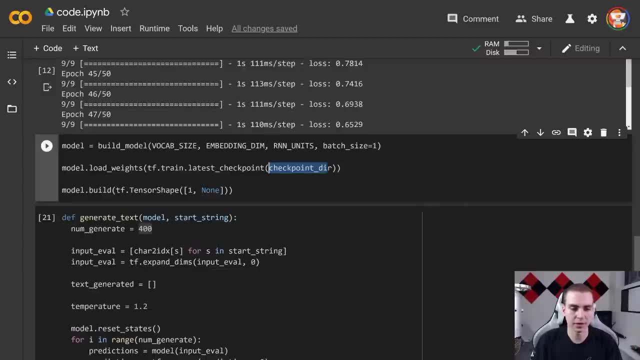 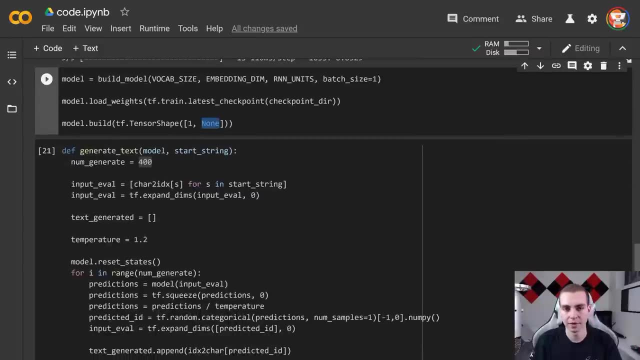 that we defined above, And then what we're going to do is build the model and tell it to expect the shape one none as its initial input. Now, none just means we don't know what that value is going to be, But we know that we're gonna have one entry, Alright. so now, 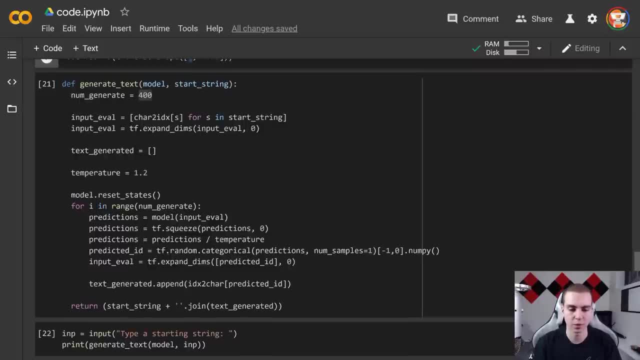 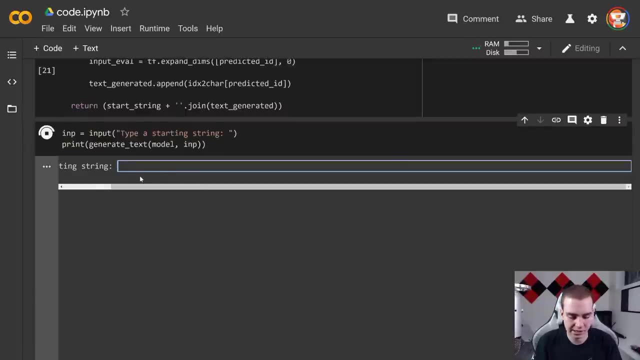 we have this generate text method or function here, which I've already kind of went through how that works, And then we can see that if I type in input string, so we type, you know, input string, let's say of Hello and hit enter, we'll watch, and we can see that the 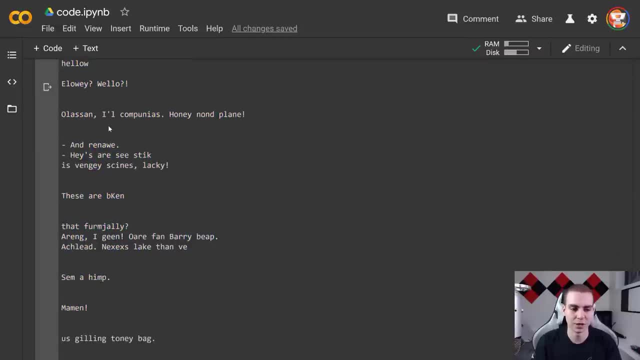 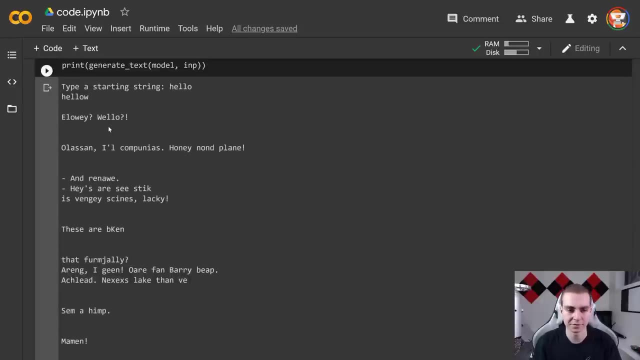 B movie. you know, trained model comes up with its output here. Now, unfortunately, the B movie script does not work as well as Romeo and Juliet. That's just because Romeo and Juliet is a much longer model piece of text. It's much better. It's formatted a lot nicer and more predictable, But yeah. 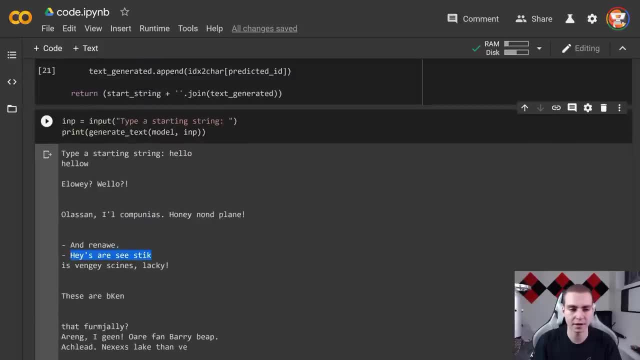 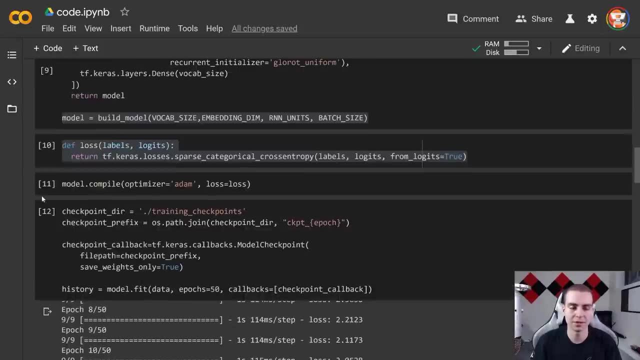 you kind of get the idea here And it's kind of cool to see how this performs on different data. So I would highly recommend that you guys find some training data that you could give this other than just the Romeo and Juliet, or maybe even try another play or something. 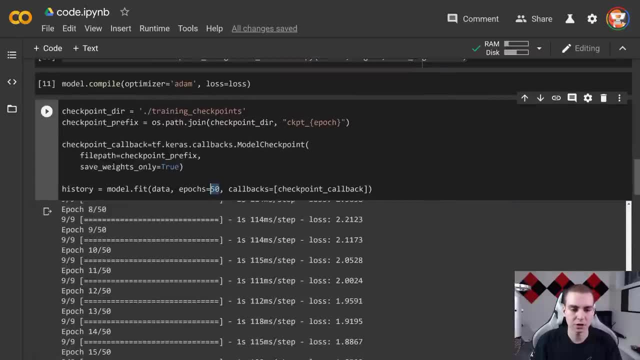 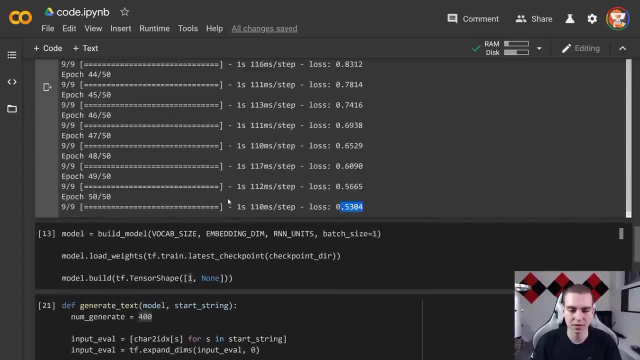 and see what you can get out of it. Also, quick side note: to make your model better, increase the amount of epochs here. Ideally you want this loss to be as low as possible. you can see mine was still actually moving down at epoch 50, you will reach a point where the amount of epochs won't make a difference. 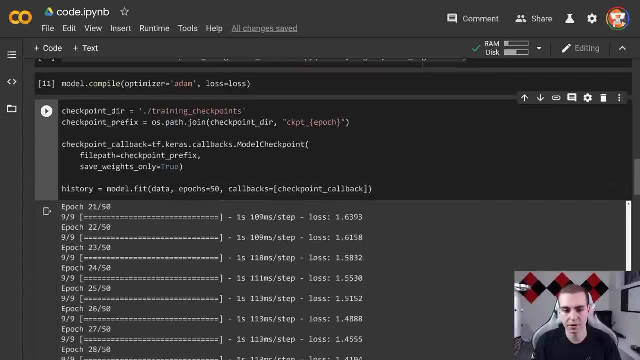 Although with models like this, the more epochs typically the better, because it's difficult for it to kind of overfit, because all you want it to do really is just kind of learn how the language works and then be able to replicate that to you almost right. So that's. 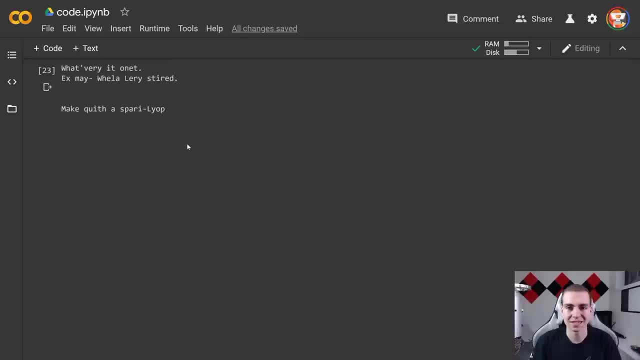 kind of the idea here And, with that being said, I'm going to say that this section is probably done. Now, I know this was a long, probably confusing section for a lot of you, But this is. you know what happens when you start getting into some more complex things. 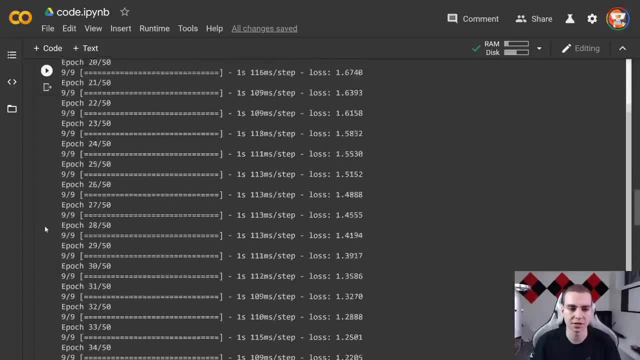 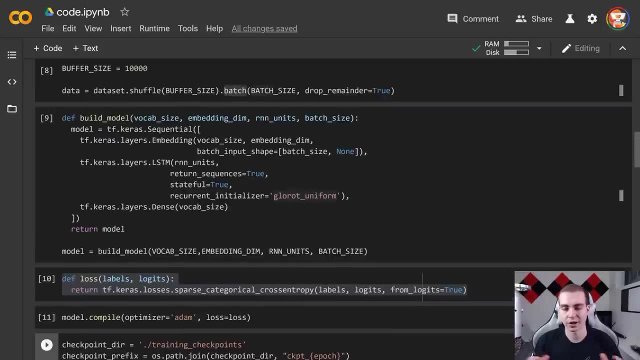 in machine learning. it's very difficult to kind of grasp and understand all these concepts in an hour of me just explaining them. What I try to do in these videos is introduce you to the syntax, show you how to get a working, you know, kind of prototype and hopefully 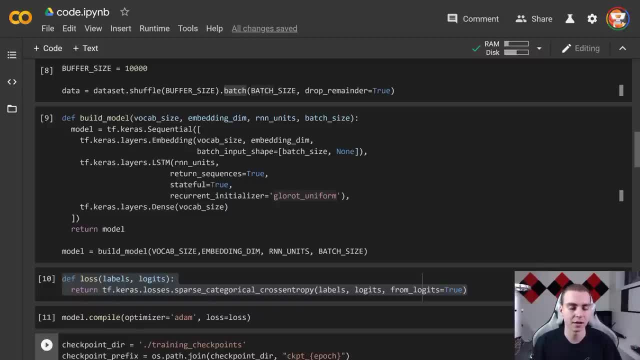 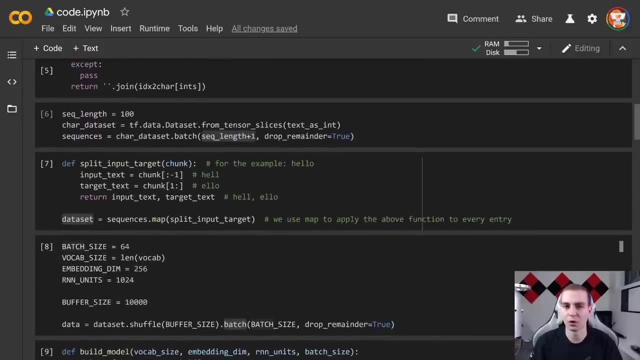 give you enough knowledge to the fact where, if you're confused by something that I said, you can go and you can look that up And you can figure out kind of the more important details for yourself, because I really just I can't go into all you know the extremes. 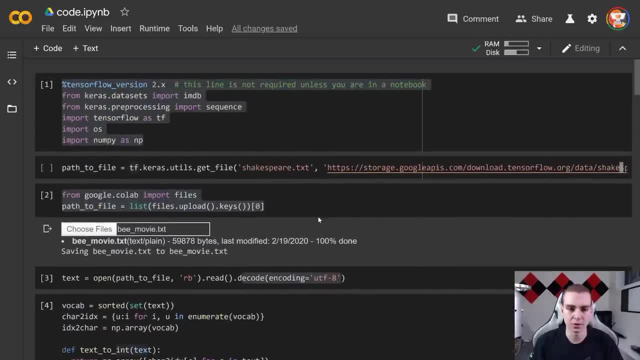 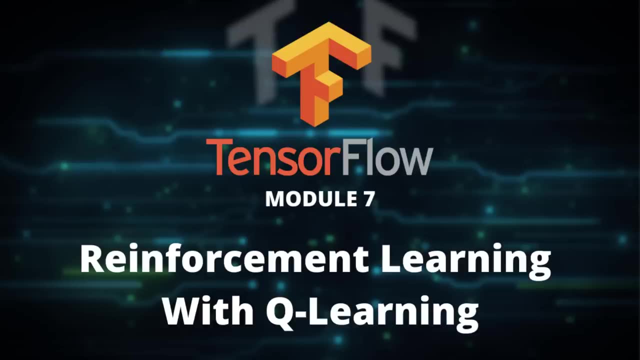 in these videos. So, anyways, that has been this section. I hope you guys found this video helpful. I hope you guys enjoyed doing this. I thought this was pretty cool And in the next section we're gonna be talking about reinforcement learning. Hello everyone, and 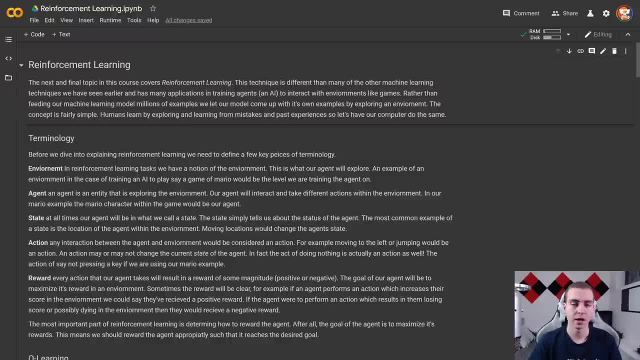 welcome to the next module in this course on reinforcement learning. So what we're gonna be doing in this module is talking about another technique in machine learning called reinforcement learning. Now, if you remember, at the very beginning of this course, which I know for, 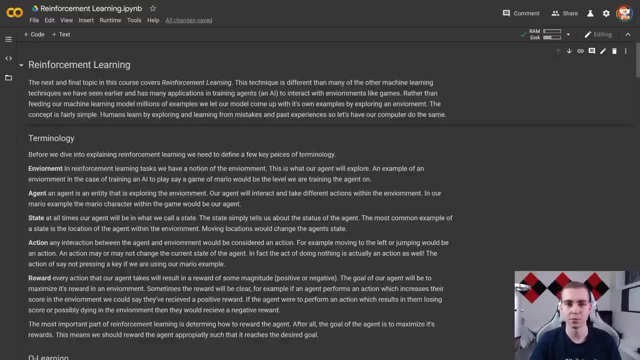 you guys is probably at like six hours ago. at this point we did briefly discuss what reinforcement learning was. Now I'll go through a recap here just to make sure everyone's clear on it. But essentially reinforcement learning is kind of the strategy and machine learning. 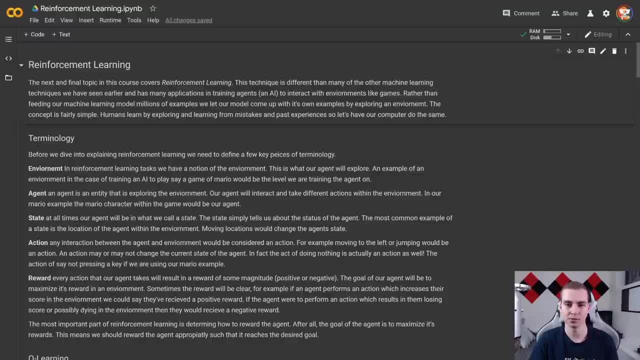 where, rather than feeding a ton of data and a ton of examples to our model, we let the model- or in this case, we're going to call it agent- actually come up with these examples itself, And we do this by letting an agent explore an environment. Now, essentially, 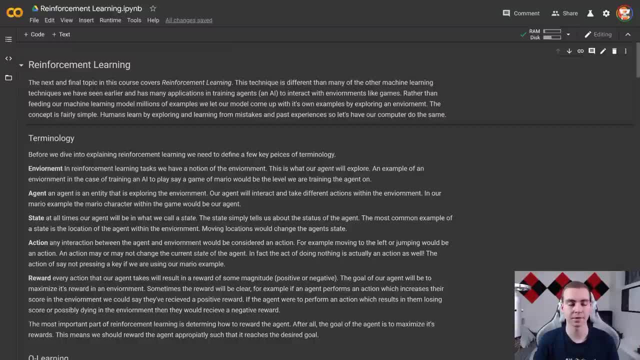 the concept here is: just like humans, the way that we learn to do something, say like play a game, is by actually doing it. we get put in the environment, we try to do it And then, you know, we'll make mistakes, we'll encounter. 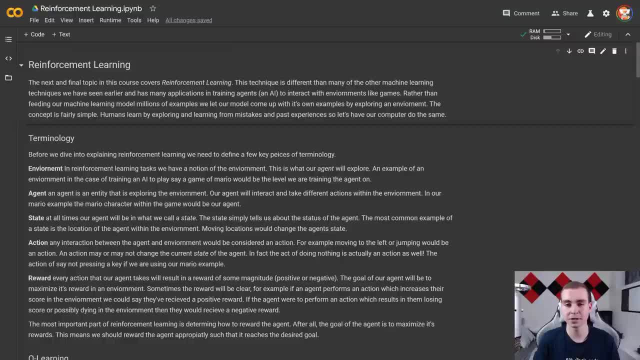 different things. we'll see what goes correctly And based on those experiences, we learn and we figure out the correct things to do. A very basic example is: you know, say we play a game And when we go left we fell off a cliff or something right. Next time we play. 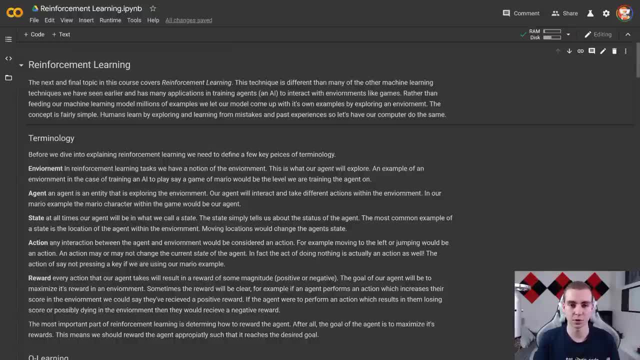 that game and we get to that point, we're probably not going to go left because we're going to remember the fact that that was bad and hence learned from our mistakes. So that's kind of the idea here with reinforcement learning. I'm going to go through exactly how this works. 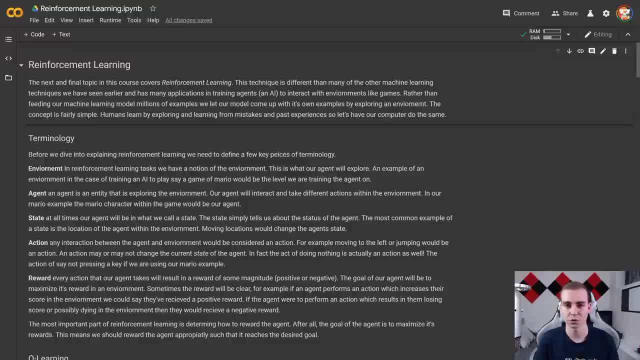 and give some better examples and some math- The implementations we're going to use, but I just want to make this clear that there's a lot of different types of reinforcement learning. In this example, we're just going to be talking about something called Q learning And I'm going to keep this module shorter. 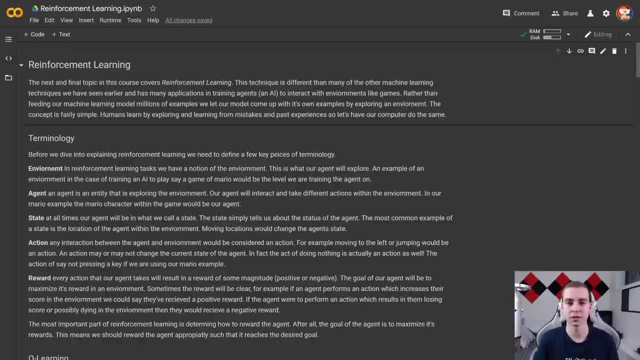 compared to the other ones, Because this field of AI- machine learning- is pretty complex and can get pretty difficult pretty quickly, So it's something that's maybe a more advanced topic for some of you guys. Alright, so anyways, now we need to define some terminology before. 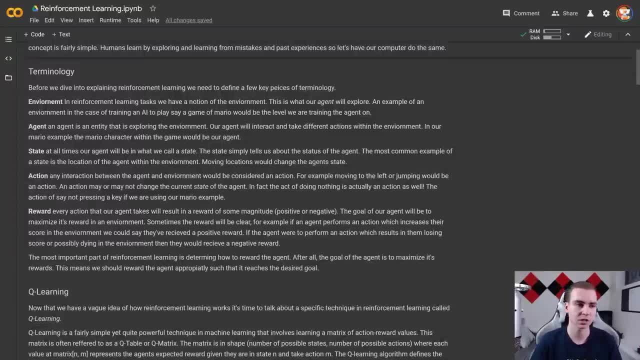 I can even start really explaining the technique we're going to use and how this works. So we have something called an environment agent, state action and reward, And I'm hoping that some of you guys will remember this from the very beginning. But environment is essentially what we're trying. 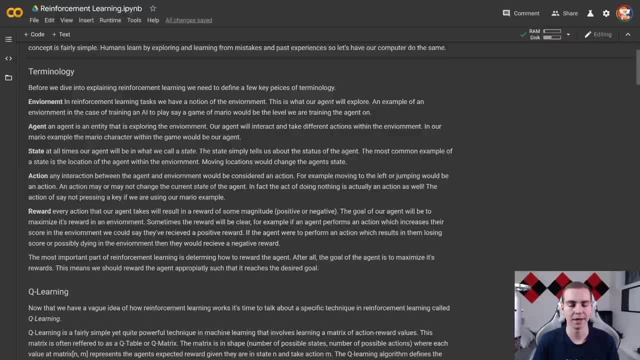 to solve or what we're trying to do. So in reinforcement learning, we have this notion of an agent, and the agent is what's going to explore the environment. So if we're thinking about reinforcement learning when it comes to, say, training in AI to play a game, well, 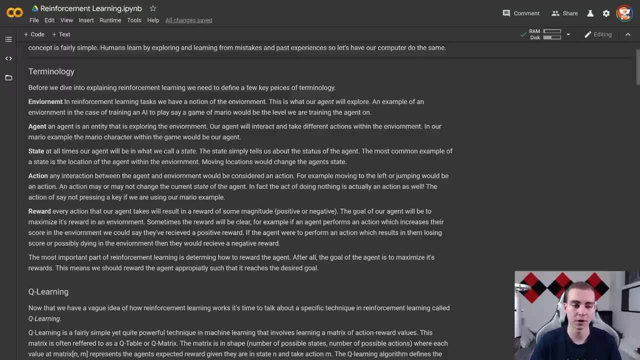 in that instance, say we're talking about Mario, the agent would be Mario, as that is the thing that's moving around and exploring our environment, And the environment would be the level in which we're playing in. So you know, in another example maybe, in the example we're going to use below, we're actually 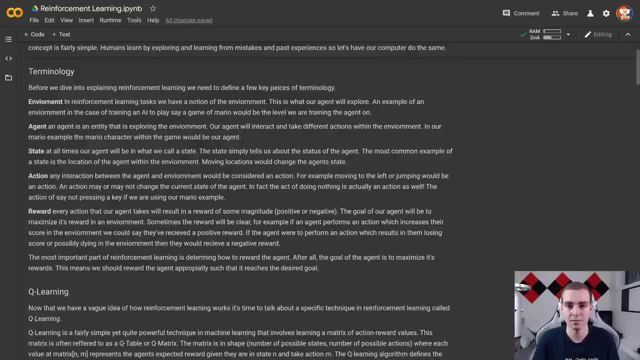 going to be kind of in almost a maze. So the environment is going to be the maze and the agent is going to be the character or the entity, or whatever you want to call it, that's exploring that maze. So it's pretty. it's usually pretty intuitive to come up with what. 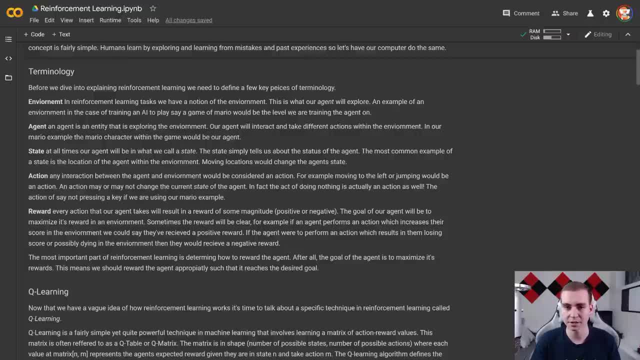 the environment and the agent are, Although in some more complex examples it might not always be clear, But just understand that reinforcement learning deals with an agent- something exploring an environment- and a very common application of reinforcement learning is in training AI is on how to play games, And it's actually very interesting what they've. 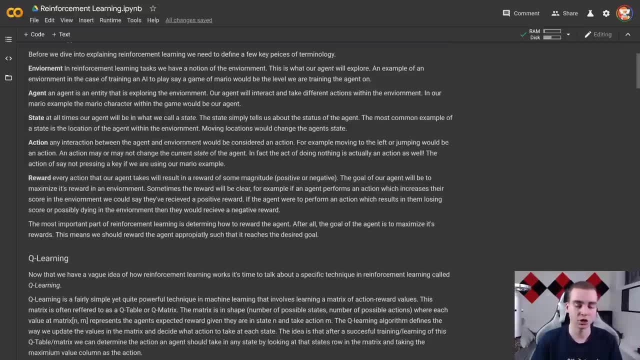 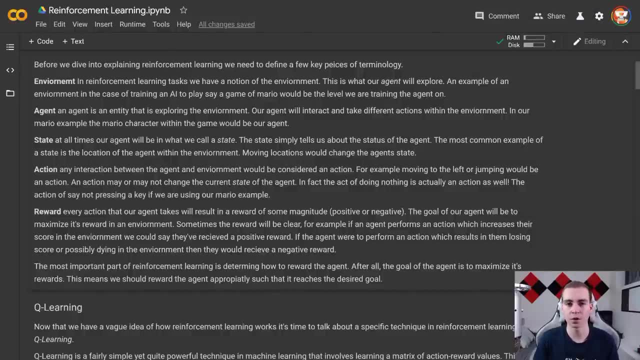 been able to do in that field recently. Okay, so we have environments and agent. hopefully that makes sense. The next thing to talk about is state. So essentially, the state is where you are in the environment. So obviously inside of the environment we can have many. 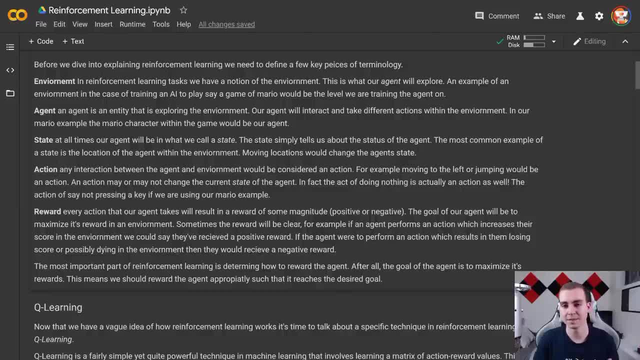 different states and a state could also be associated with the- you know- agent itself. So we're going to say the agent is in a specific state whenever it is in some part of the environment. Now, in the case of our game, the state that an agent would be in would 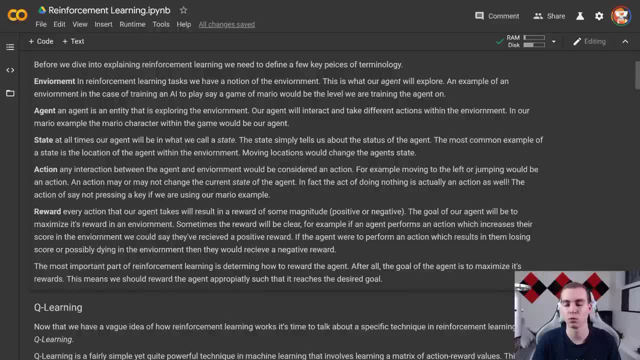 be their position in the level. say, if they're at, you know x, y coordinates like 1020, they would be at state or in state 1020. That's kind of how we think about states Now, obviously. 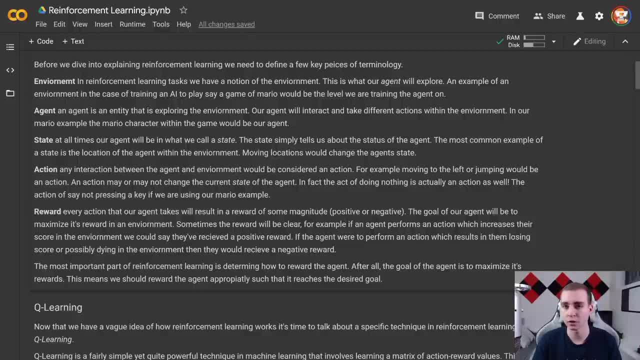 state can be applied in some different instances as well. We're playing, say, maybe, a turn based game. you know, actually that's not really a great example. I'm trying to think of something where the state wouldn't necessarily be a position. 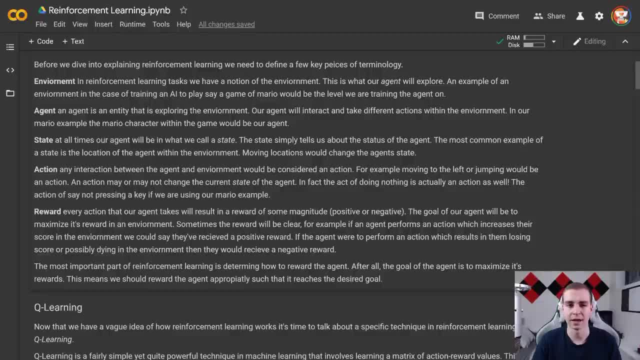 maybe if you're playing a game where you have like health or something like that And part of the states might be the health of the character. This can get complicated depending on what you're trying to do, But just understand the notion that for most of our examples state: 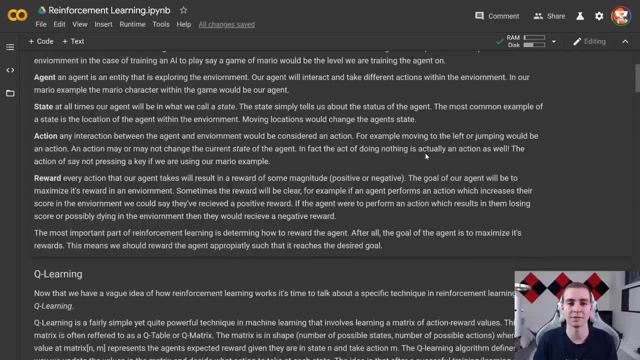 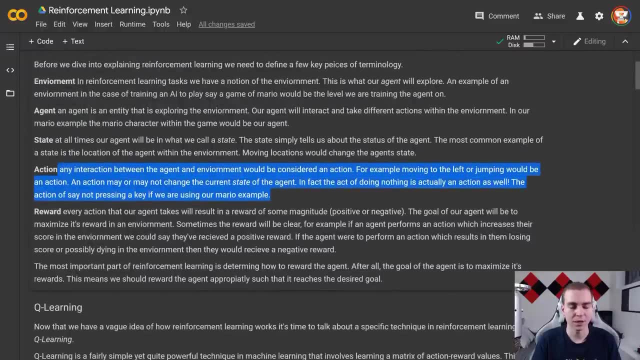 is simply going to be location, although it really is just kind of telling us information about where the agent is and its status in the environment. So next we have this notion of an action. So in reinforcement learning, our agent is exploring the environment. it's. 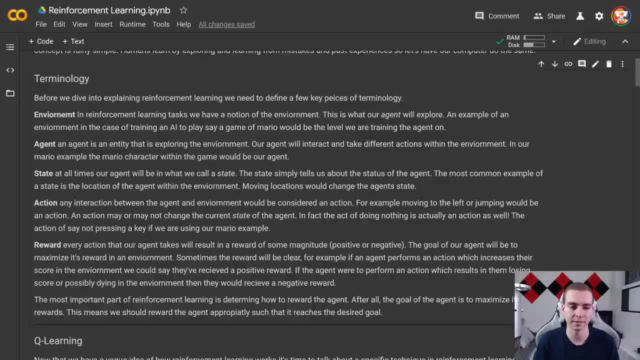 trying to figure out the best way or how to accomplish some kind of goal in the environment And the way that it interacts with the environment is with something called actions. Now actions could be, say, moving the left arrow key right, moving to the left in the environment moving. 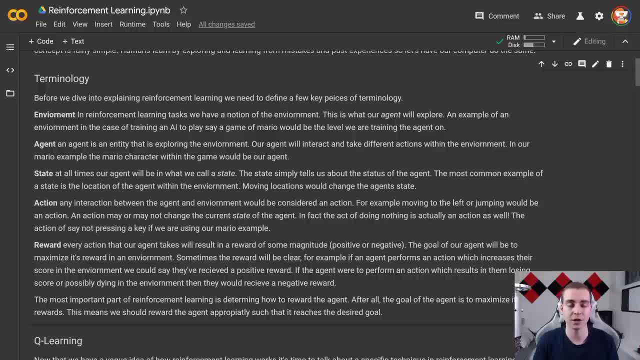 to the right. it could be something like jumping in an action can actually be not doing something at all. So when we say, you know, agent performed action, that could really mean that the action and that maybe time step was that they didn't do something right, that they didn't do anything. 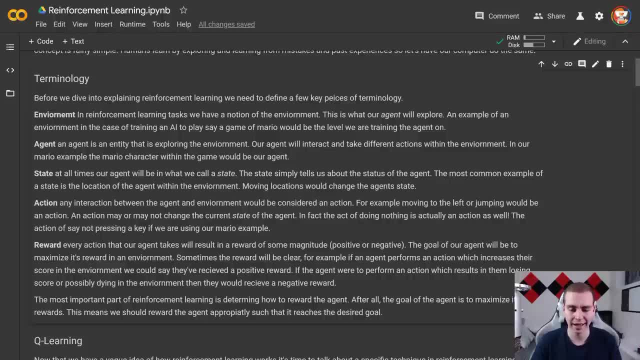 that was their action. So that's kind of the idea of action. In the example of our Mario one, which I keep going back to, an action would be something like jumping, And typically actions will change the state of our entity or our agent, although they might not necessarily do that, In fact. 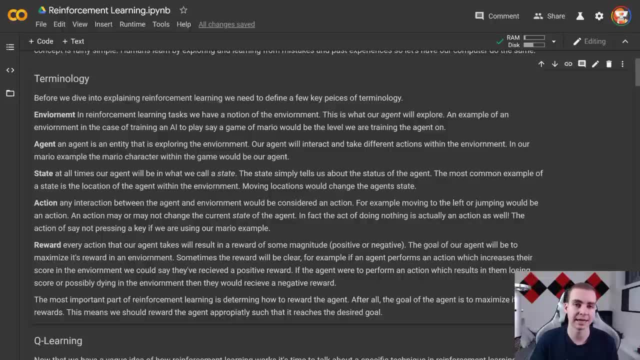 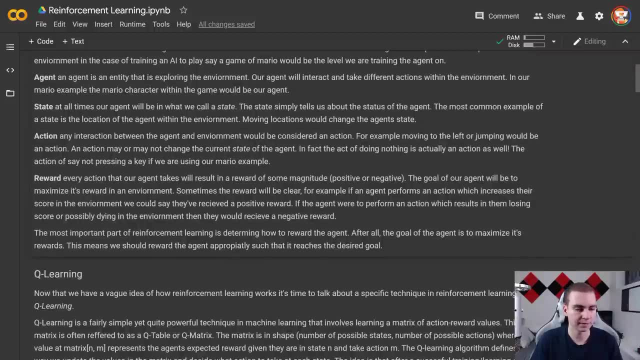 we will observe, with a lot of the different actions, that we could actually be in the same state after performing that action. Alright, so now we're on to the last part, which is actually the most important to understand, And this is reward. So reward is actually what our agent is trying to maximize while it is in the environment. 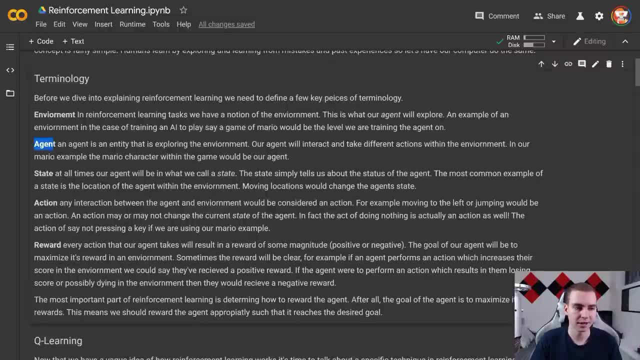 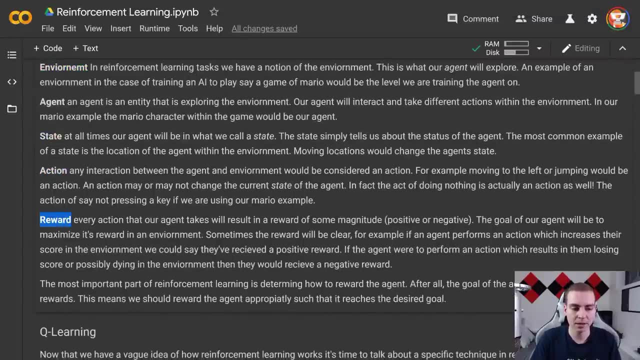 So the goal of reinforcement learning is to have this agent navigate this environment, go through a bunch of the different states of it and determine which actions maximize the reward at every given state. So essentially, the goal of our agent is to maximize a reward. 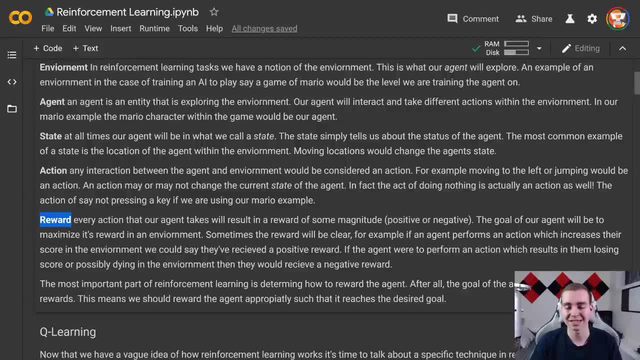 But what is a reward? Well, after every action that's taken, the agent will receive a reward. Now, this is something that us, as the programmer, need to come up with. The reason we need to do this is because we need to tell the agent when it's performing well and when it's performing. 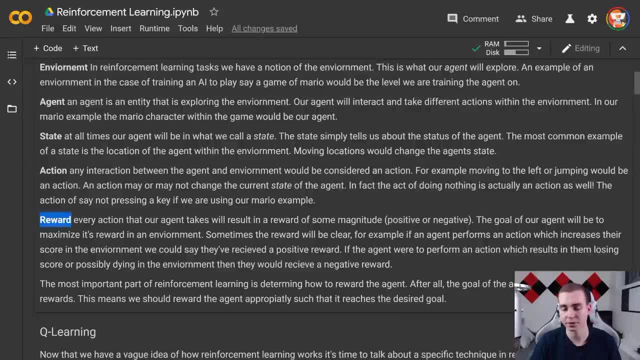 poorly And just like we had like a loss function in neural networks when we were using those before. this is almost like our loss function. you know the higher this number is, the more reward the agent gets. the better the lower the reward. you know it's not as good it's. 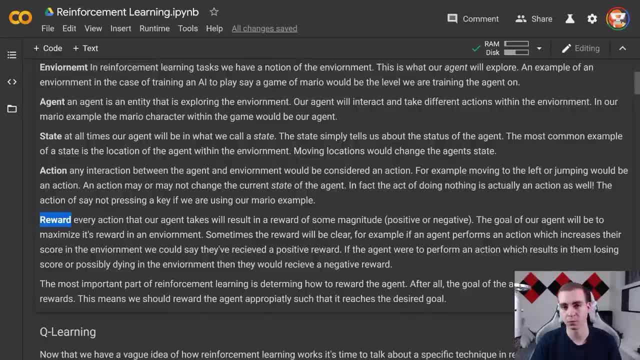 not doing as well. So that's how we kind of monitor and assess performance for our agents is by determining The almost average amount of reward that they're able to achieve And their goal is really to. you know, it's almost an optimization problem where they're trying to maximize this reward. 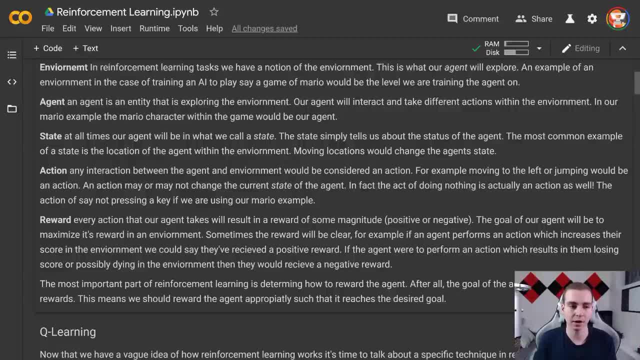 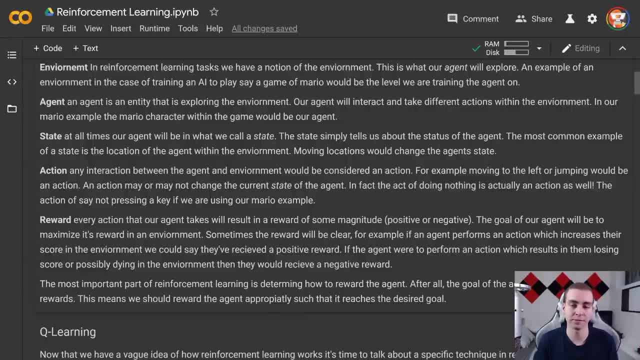 that we don't like, say, like dying or like jumping in the wrong spot, we could give it a negative reward. to try to influence it to not do that, And our goal, you know, when we train these agents, is for them to get the most reward, and we hope that they're going. 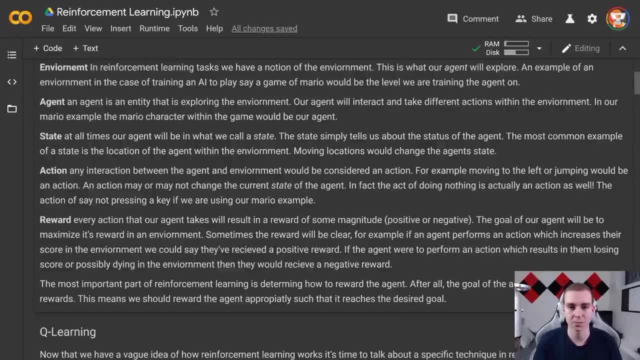 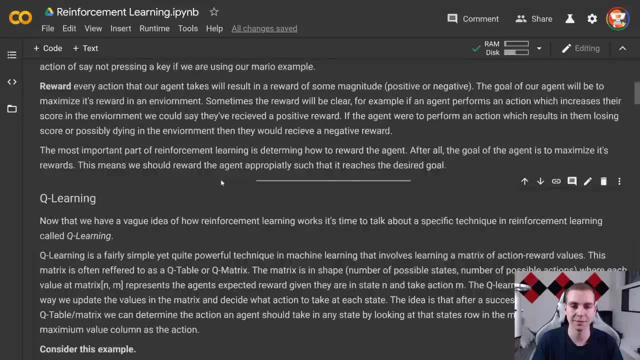 to learn the optimal route through a level or through some environment that will maximize that reward for them. Okay, so now I'm going to talk about a technique called q learning, which is actually just an algorithm that we're going to use to implement this idea of reinforcement. 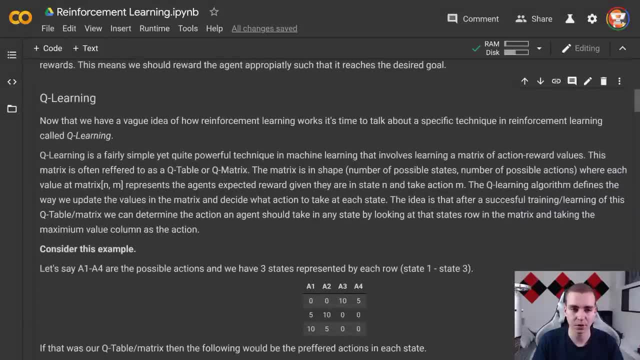 learning. we're not going to get into anything too crazy in this last module because this is meant to be more of an introduction into the kind of field of reinforcement learning than anything else. But Q learning is the most basic way to implement reinforcement learning, at least that I have discovered, And essentially what Q learning is, and I 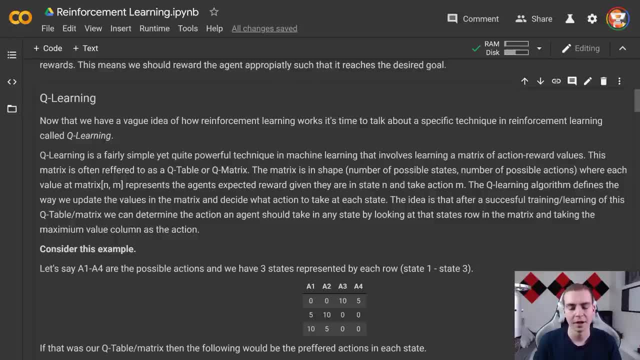 don't actually really know why they call it Q, although I should probably know that is creating some kind of table or matrix like data structure. it's going to contain, as the what is it, I guess, the rows, every single state, and as the columns, every single action. 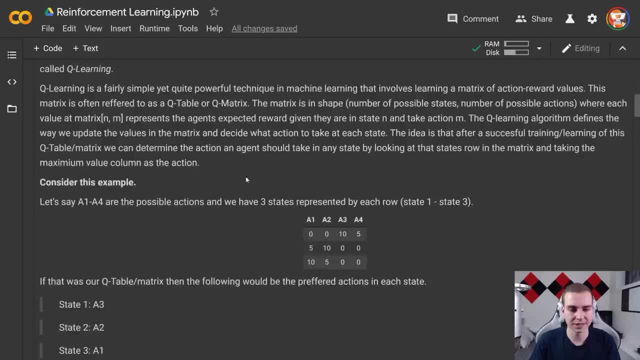 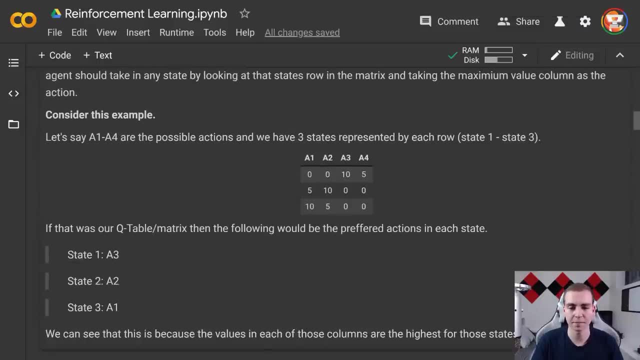 that could be taken in all of those different states. So for an example here- and we'll do one on kind of the whiteboard later on if we can get there- But here we can see that this is kind of my cue table And what I'm saying is that we have a one, a, two a. 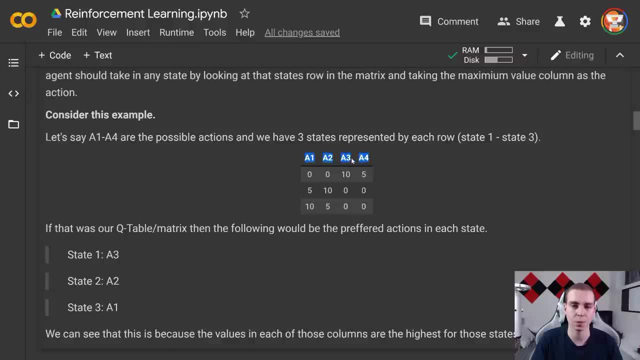 three, a four as all the possible actions that could be performed in any Q table, And what I'm saying is that we have a one, a two, a three, a four as all the possible actions that could be performed in any. 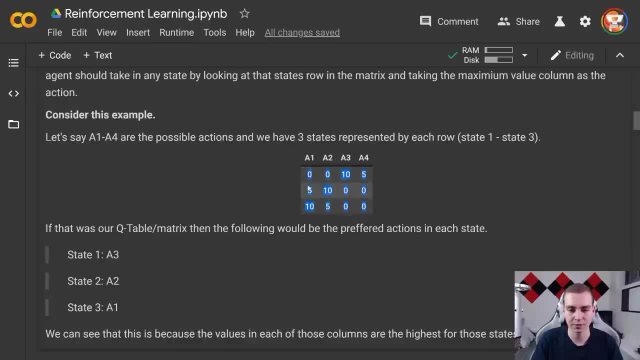 given state And we have three states, denoted by the fact that we have three rows, and the numbers in this, this table, is Q. what do they call it? Q matrix, Q table, whatever you want to call it. the numbers that are present here represent what the predicted reward will. 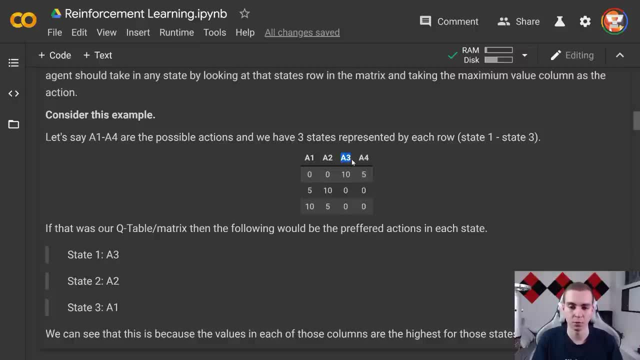 be given that we take an action, whatever this action is in this state. So I'm not sure if this is making sense to you guys, But essentially, if we're saying that row zero is state zero, action to a two, this value tells us what reward we should expect to get If we take this action. while 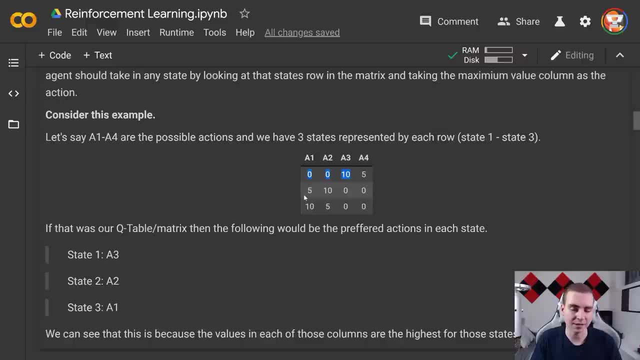 we're in this state. That's what that is trying to tell us. That's what that means. Same thing here in you know, state two, we can see that the optimal action to take would be action two, because that has the highest reward for this state, And that's what this table is. 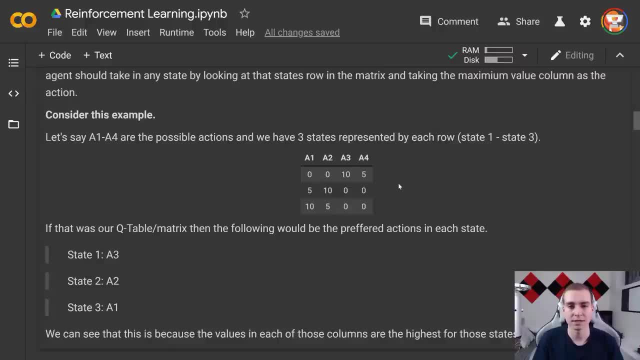 that we're going to try to generate, with this technique called Q learning, a table that can tell us, given any state with the predict, predicted reward will be for any action that we take. And we're going to generate this table by exploring the environment many different times and updating these values according. 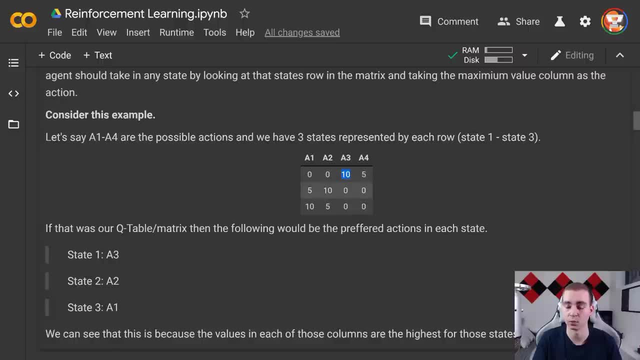 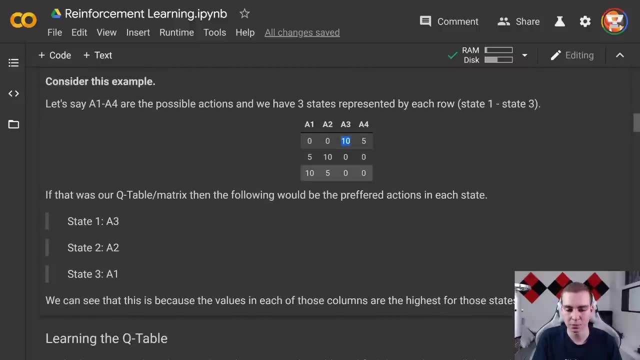 to what we kind of see or what the agencies in the environment and the rewards that receives for any given action in any given state, And we'll talk about how we're going to update that later, But this is the basic premise. So that is kind of Q learning I'm going to 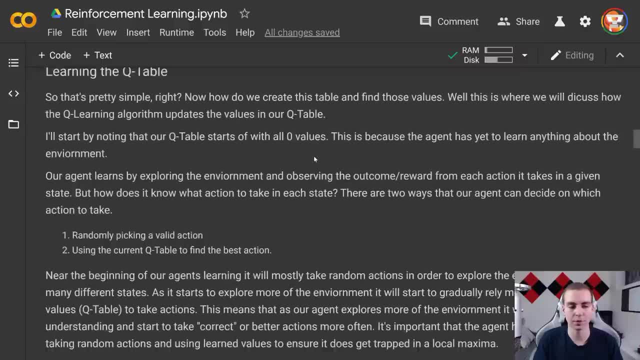 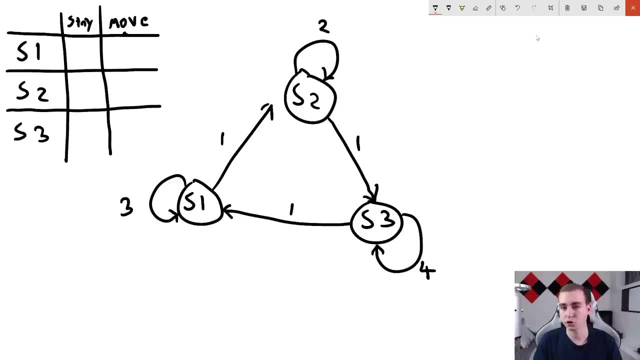 hop on the whiteboard now And we'll do a more in depth example, But then we're going to talk about how we actually learned this Q table that I just discussed. Okay, so I've drawn a pretty basic example right now that I'm going to try to use to. 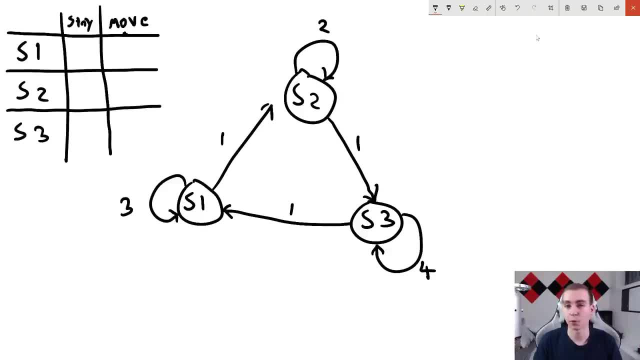 illustrate the idea of Q learning and talk about some problems with it and how we can kind of combat those as we learn more about how Q learning works. But the idea here is that we currently have three states and why what is happening? Why was that happening? 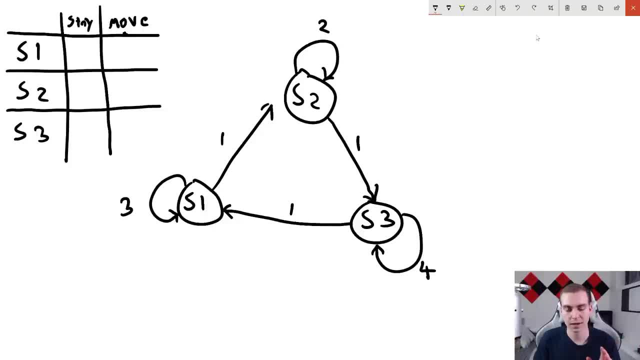 up at the top, I don't know. Anyways, the idea is we have three states: s1,, s2, and s3. And at each state we have two possible actions that can be taken. we can either stay in this. 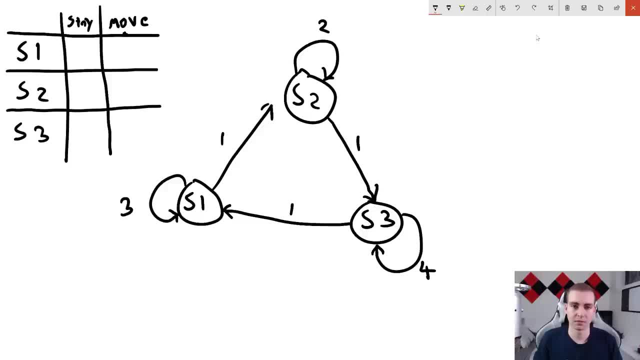 state or we can move. Now what I've done is kind of just written some integers here that represent the reward that we're going to get or that the agent is going to get, such that it takes that action in a given state. So if we take the action here in s1, right of moving, then we will. 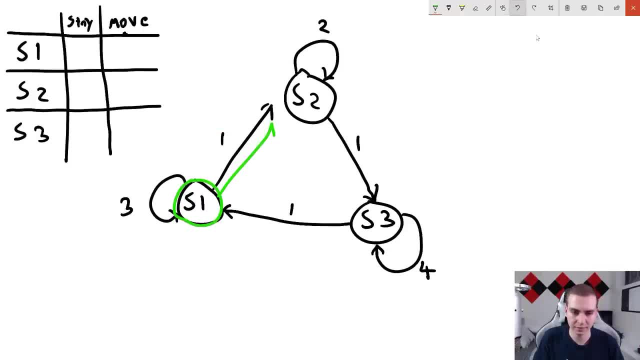 receive a reward of one, because that's what we've written here- is the reward that we get for moving, Whereas if we stay we'll get a reward of three. you know same concept here: if we stay, we get to, if we move, we get one, and I think you understand the point. 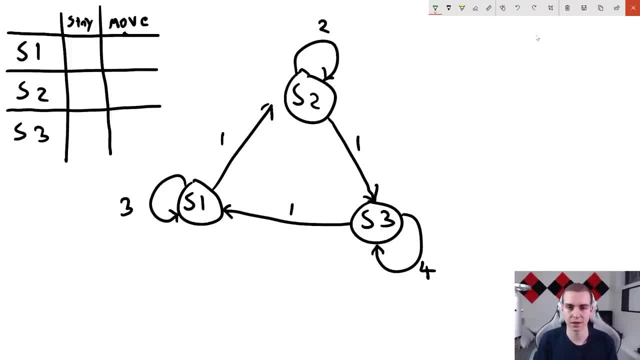 So the goal of our agent, to remember, is to maximize its reward in the environment, And what we're going to call the environment is this, right here the environment is essentially defines the number of states, the number of actions, and you know the way that the agent 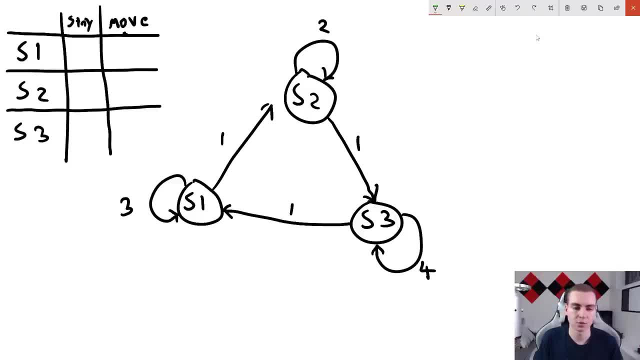 can interact with these states and these actions. So in this case, the agent can interact with the states by taking actions that change its state right. So that's what we're getting out with this. Now, what I want to do is show you how we use this cue table, or learn this. 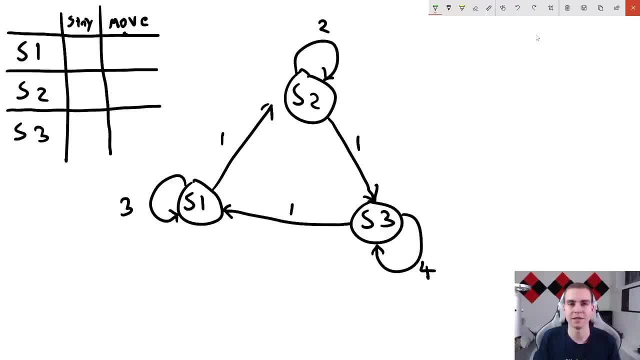 cue table To come up with kind of the almost you know the model, like the machine learning model that we're going to use. So essentially what we would want to have here is we want to have a kind of pattern in this table that allows our agent to receive the maximum reward. So 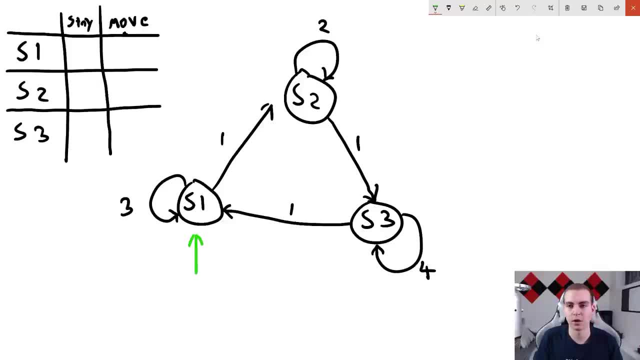 in this case, we're going to say that our agent will start at state s1. And obviously whenever we're doing this reinforcement learning, we need to have some kind of start state that the agent will start in. this could be a random state, it could change. 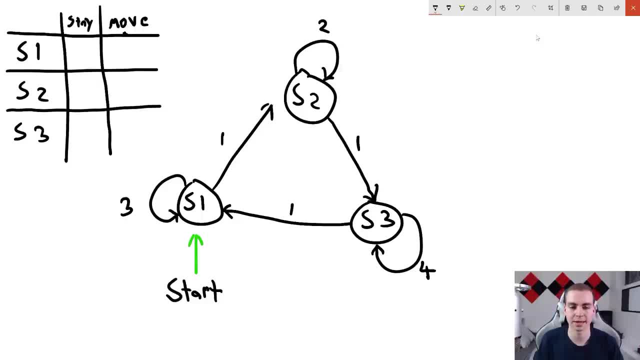 But it doesn't just start in some state. So in this case we're going to say it starts at s1.. Now, when we're in s1, the agent has two things that it can do. it can stay in the current state and receive a reward of three, or it can move and receive a reward. 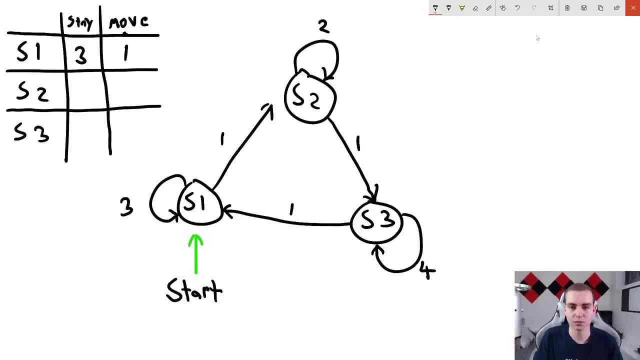 of one right If we get to s2,. in this state, what can we do? we can stay, which means we receive a reward of two, or we can move, which means we get a reward of one. And same thing for s3,: we can stay, we get a reward of four and we can move, we get a reward of one. So 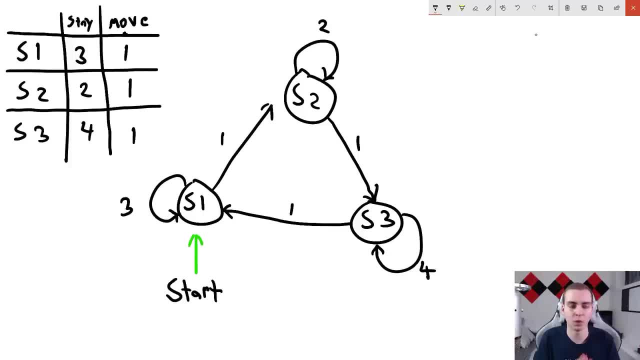 now, right now, if we had just ran this one time and have the agent stay in each state like start, in each unique state, this is what the queue table we would get would look like, Because after looking at this just one time, starting in each state, what the agent would 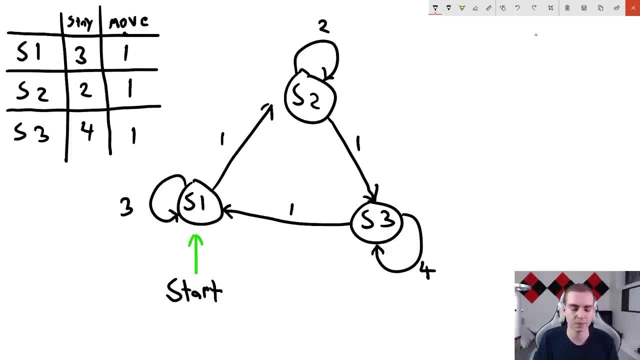 be able to, or I guess two times, because it would have to try each action. Let's say we had the agent start in each state twice, So it started in s1 twice, it started s2 twice and it started in s3 twice And every time it started there it tried one of the different. 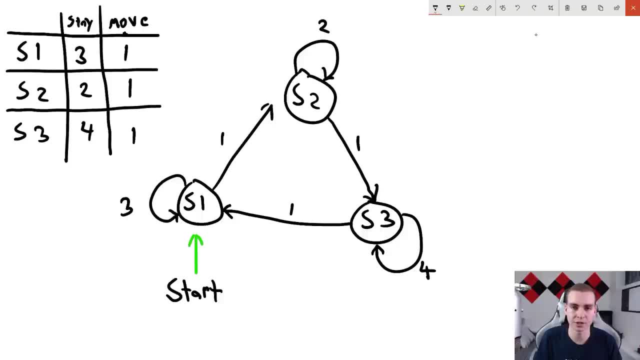 actions. So when it started in s1, it tried moving once and then it tried staying once. we would have a queue table that looks like this, because what would happen is we would update values in our queue table to represent the reward we received when we took that action from. 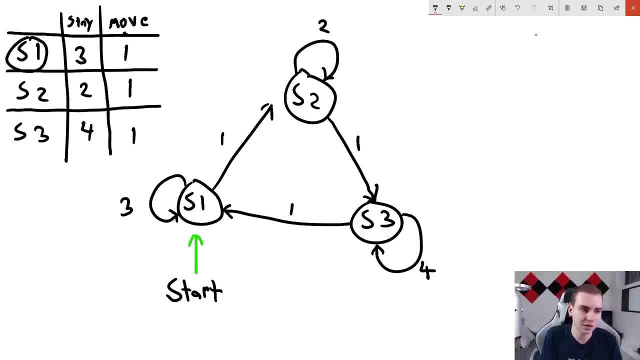 that state. So we can see here that when we're in state s1, and we decided to stay, what we did is we wrote a three inside of the stay column because that is how much reward we received when we moved right. Same thing for state two when we moved for state two. 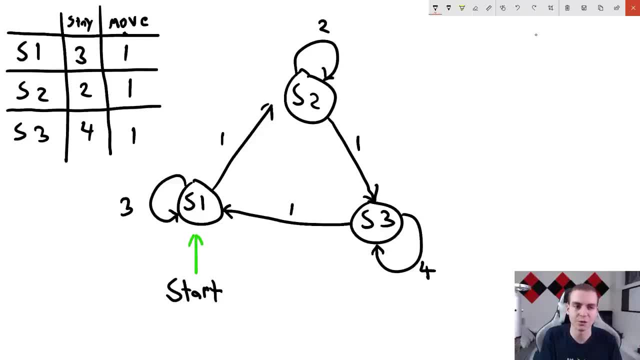 or have, I guess, sorry, stayed. when we stayed in state two, we received a reward of two. same thing for four. Now this is okay, right? This tells us, kind of you know, the optimal move to make in any state to receive the maximum reward. But what if we introduce the idea? 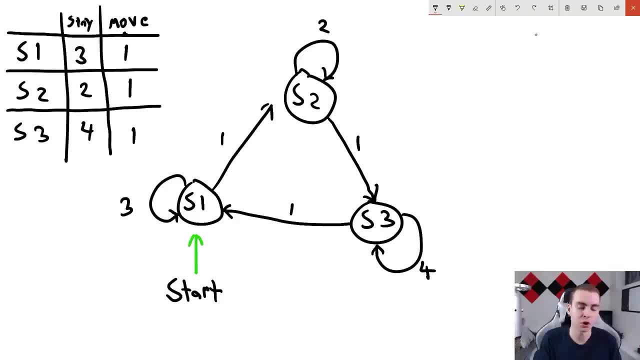 that you know our agent. we want it to receive the maximum total reward possible, right? So if it's in state one, ideally we'd like it to move to state two and then move to states three and then just stay in state three because it will receive the maximum. total reward possible, right? So if it's in state one, ideally we'd like it to move to state two and then move to state three, because it will receive the maximum total reward possible, right? So if it's in state two, it would receive the maximum total reward. 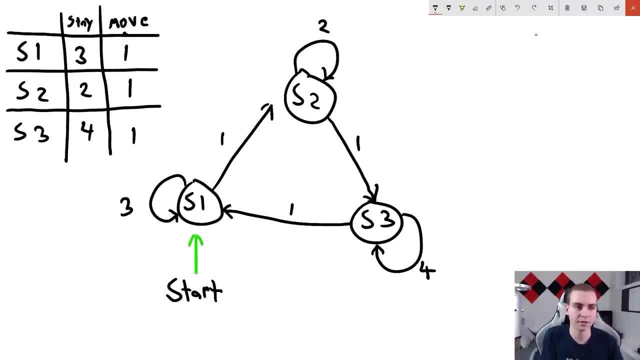 possible right? So if it's in state two, it would receive the maximum total reward possible. Well, with the current table that we've developed, if we just follow this and we look at the table, we say, Okay, if we want to use this queue learning table now to you know move. 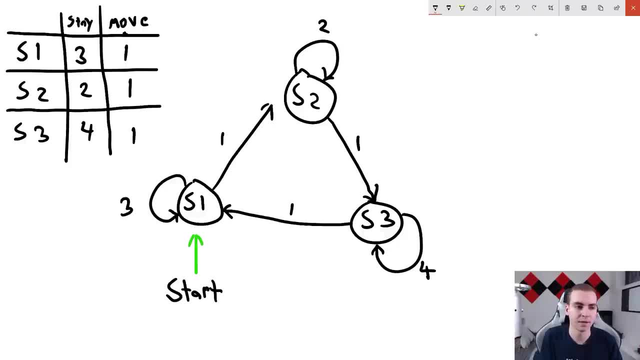 an agent around our level, what we'll do is we'll say: Okay, what state is it in? if it's in state two, we'll do stay, because that's the highest reward that we have in this table. if that's the approach we use, then we can see that if our- you know- agents start in 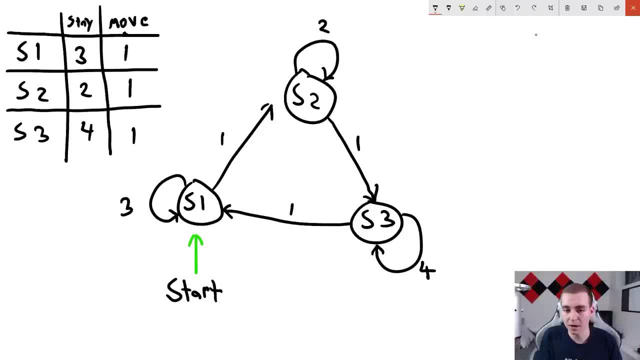 state one or state two, it would stay in what we call a local minima because it's not able to kind of realize from this state that it can move any further and receive a much greater reward right. And that's kind of the concept we're going to talk about as we implement and you 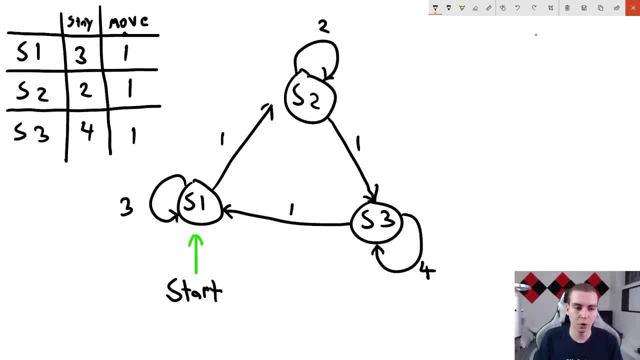 know, discuss further how Q learning works, But hopefully this gives you a little bit of insight into what we do with this table. Essentially, when we're updating these table values is when we're exploring this environments. when we explore this environment and we start. 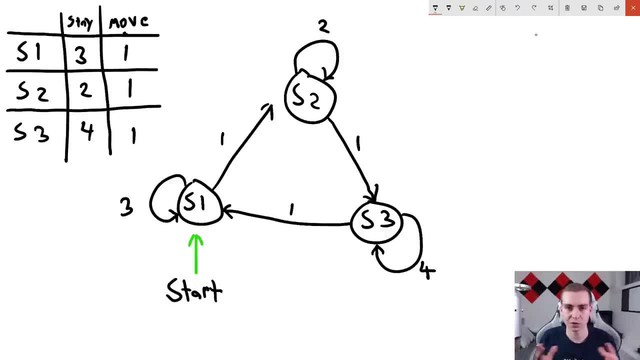 in a state. when we take an action to another state, we observe the reward that we got from going there And we observe the state that we changed to right. So we observe the fact that in state one, when we go to state two, we receive the reward of one And what we 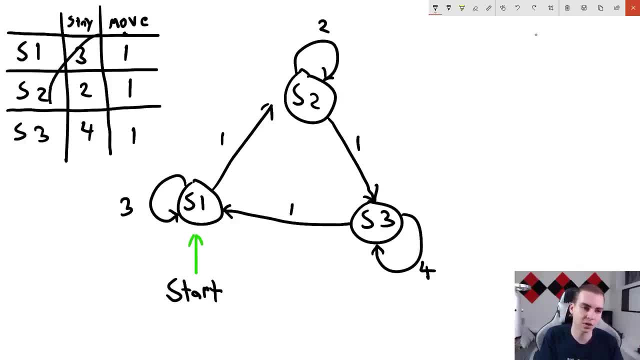 do is we take that observation and we use it to update this cue table, And the goal is that, at the end of all of these observations- and there could be millions of them- that we have a cue table that tells us the optimal action to take in any single state. So we're. 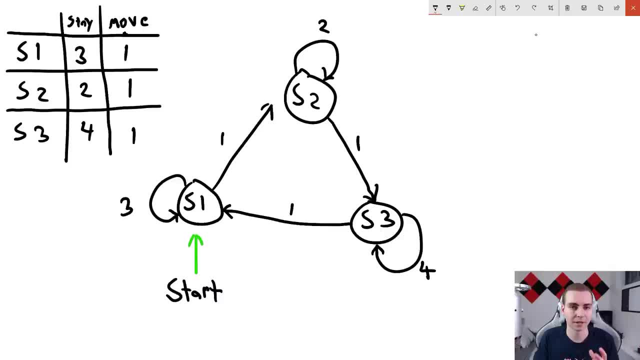 actually hard coding this kind of mapping that essentially just tells us, given any state, all you have to do is look up in this table, look at all of the actions that could be taken and just take the maximum action or the reward that's supposed to give, I guess, the action. 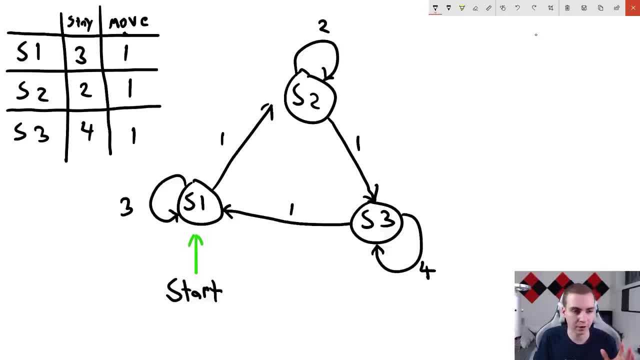 that's supposed to give the maximum reward And if we were to follow that on this, we can see we get stuck in the local minima, which is why we're going to introduce a lot of other concepts. So our reinforcement learning model and Q learning we have to implement. 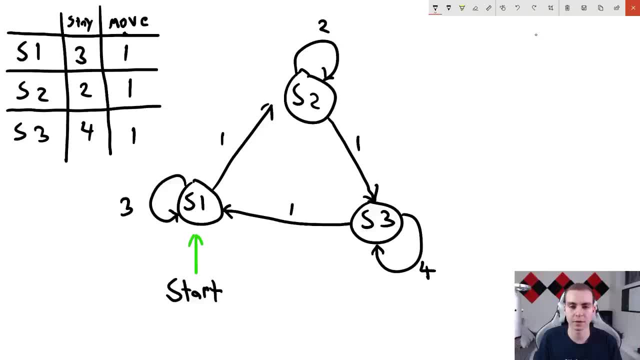 the concept of being able to explore the environment, not based on previous experiences. right, Because if we just tell our model, okay, what we're going to do is we're going to start in all these different states. we're going to start in the start state and just start. 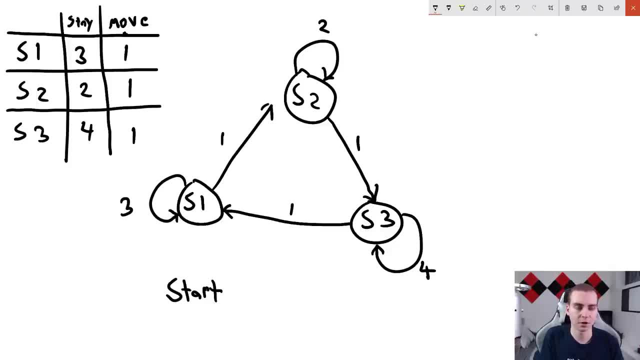 navigating around. If we update our model immediately or update our cue table immediately and put this three here for stay, we can almost guarantee that, since this three is here when our model is training, right If it's using this cue table to determine what state to. 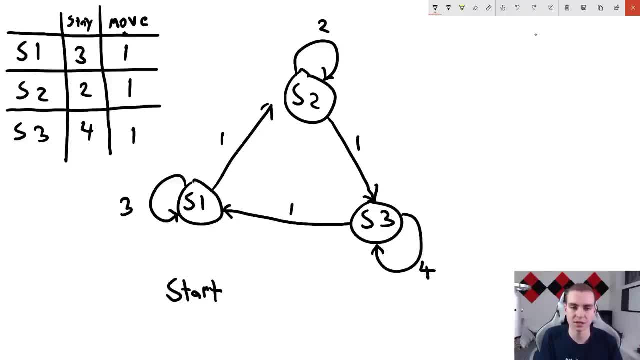 move to next, when it's training and determining what to do, it just always going to stay, which means we'll never get a chance to even see what we could have gotten to at s3.. So we need to kind of introduce some concept. 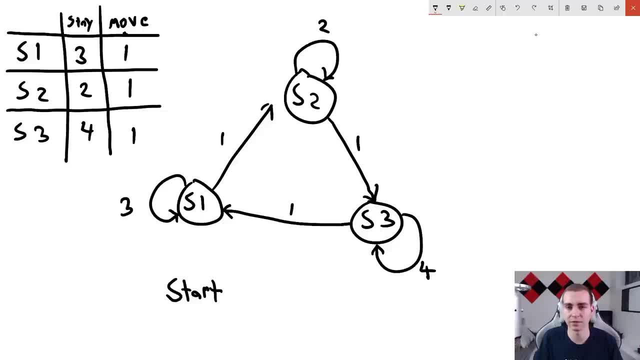 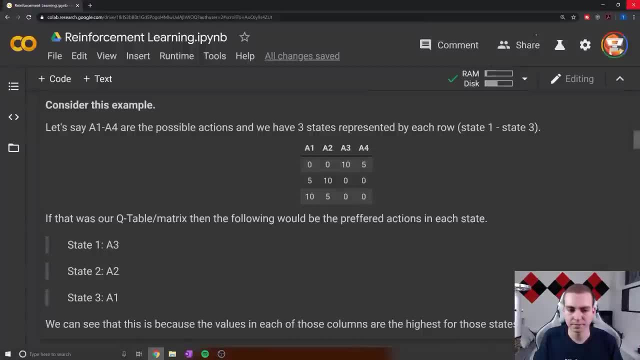 of taking random actions and being able to explore the environment more freely before starting to look at these Q values and use that for the training. So I'm actually going to go back to my slides now to make sure I don't get lost, because I think I was starting. 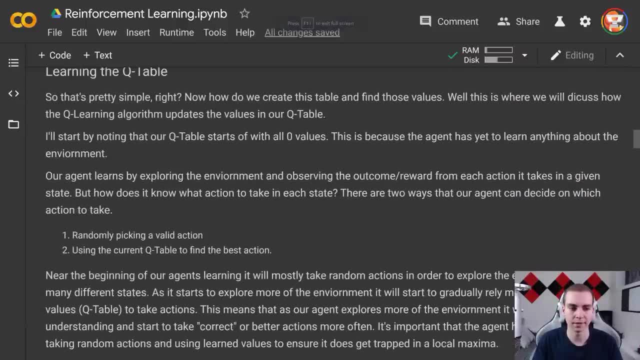 to ramble a little bit there. So we're going to now talk about learning the cue table. So essentially I showed you how we use that cue table which is given some state. we just look that state up in the cue table and then determine what the maximum reward we could. 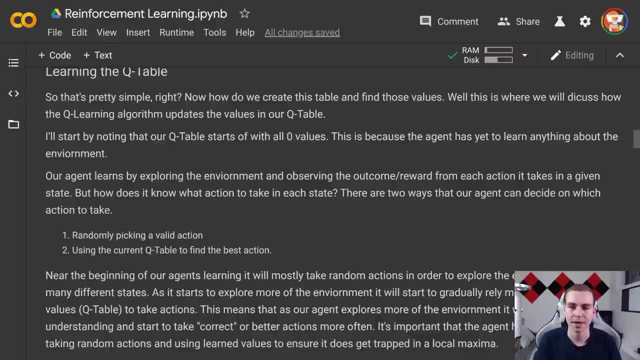 get by taking. you know some action is and then take that action, And that's how we would use the cue table later on when we're actually using the model. But when we're learning the cue table, that's not necessarily what we want to do. we don't want to explore the environment. 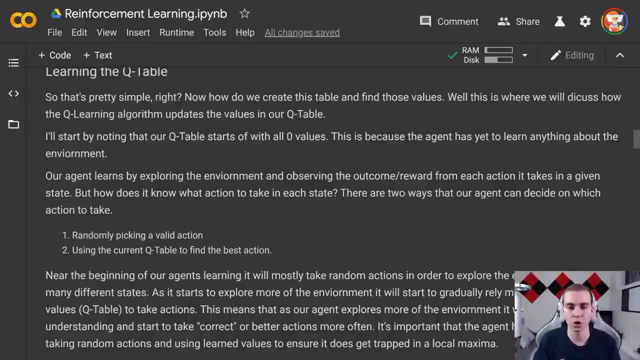 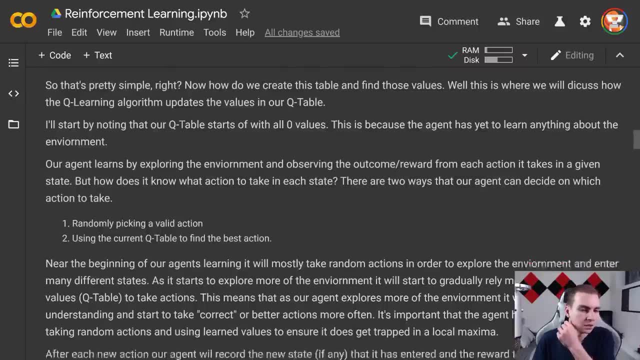 by just taking the maximum reward we've seen so far and just always going that direction. we need to make sure that we're exploring an a different way and learning the correct values for the cue table. So essentially, our agent learns by exploring the environment and observing the outcome. slash reward from each action. 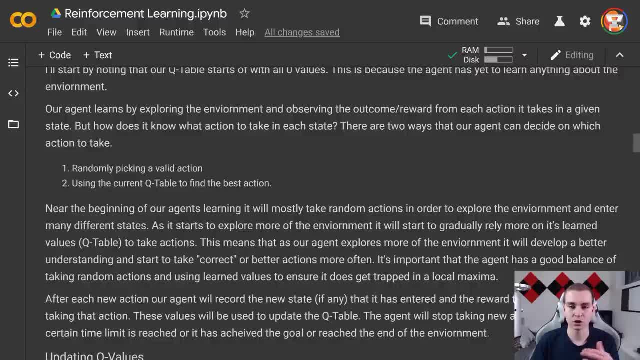 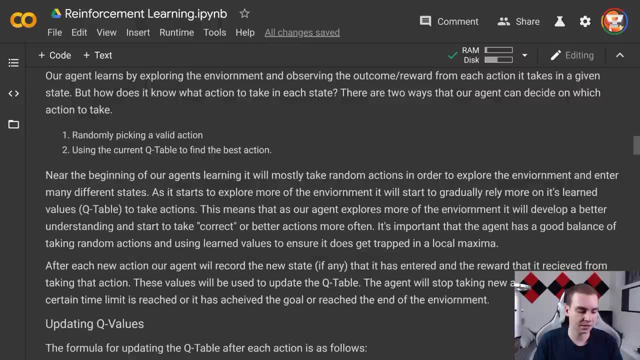 it takes in a given state, which we've already said. but how does it know what actions taken each state when it's learning? That's the question I need to answer for you now. Well, there's two ways of doing this. our agent can essentially, you know, use the current. 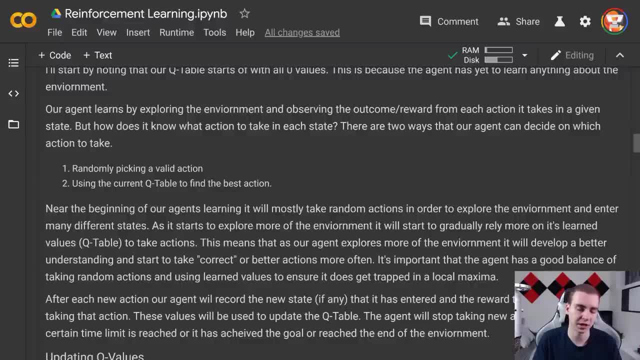 cue table to find the best action, which is kind of what I just discussed. So taking, looking at the cue table, looking at the state and just taking the highest reward, or it can randomly pick a valid action And our goal is going to be, when we create this, cue learning. 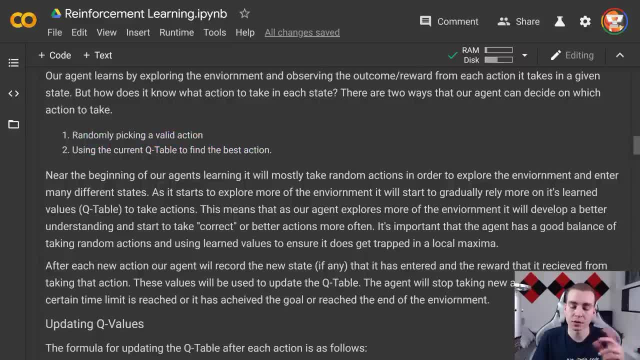 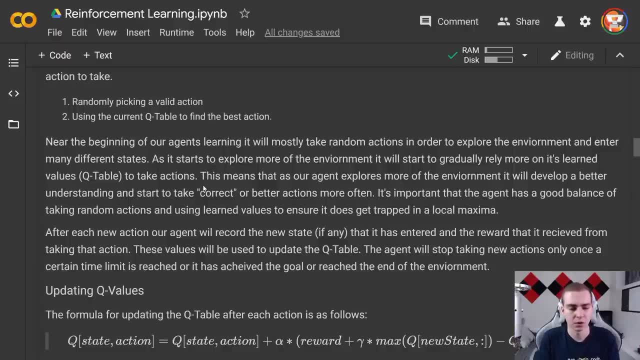 algorithm to have a really great balance of these two, where sometimes we use the cue table to find the best action and sometimes we take a random action. So that is one thing, But now I'm just going to talk about this formula for how we actually update cue values. 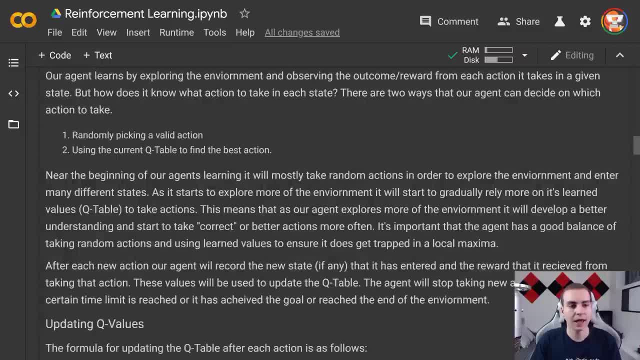 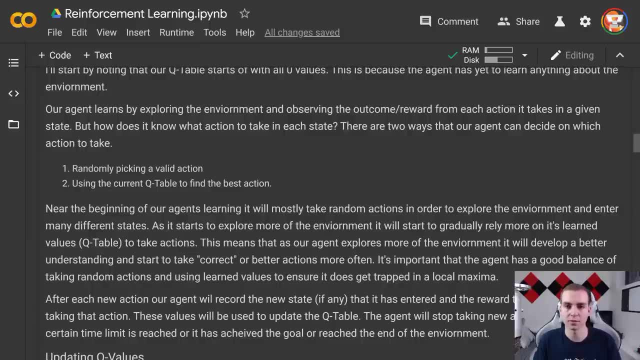 So, obviously, what's going to end up happening in our cue learning is we're going to have an agent that's going to be in the learning stage exploring the environment and having all these actions and all these rewards and all these observations happening And it's 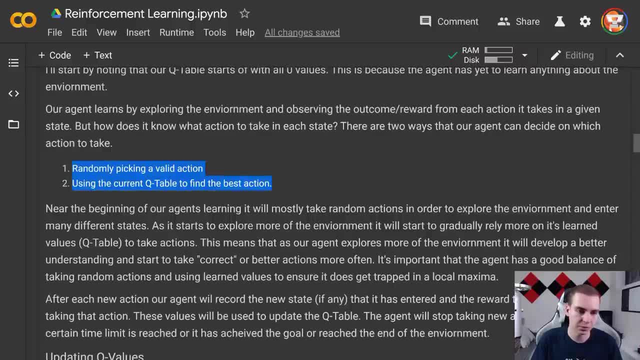 going to be moving around the environment by following one of these two kind of principles: randomly picking a valid action or using the current cue table to find the best action. When it gets into a new state and it, you know, moves from state to state, it's going. 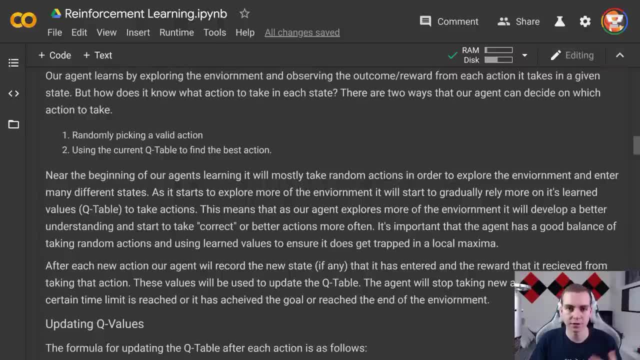 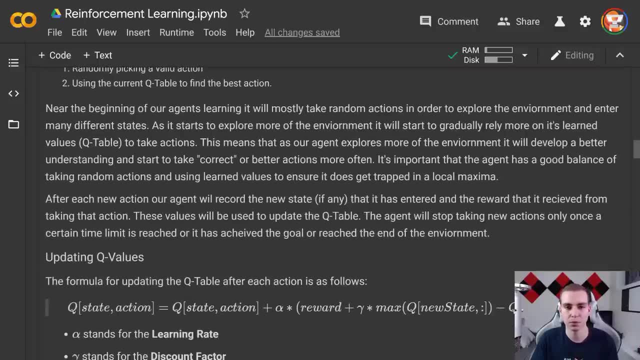 to keep updating this cue table telling it. you know, this is what I've learned about the environment. I think this is a better move. we're going to update this value, But how does it do that in a way that's going to make sense, because we can't just put 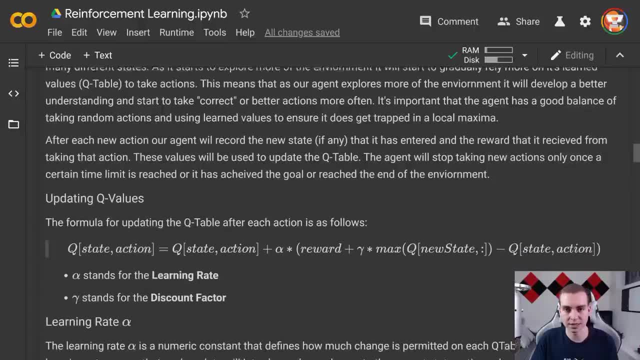 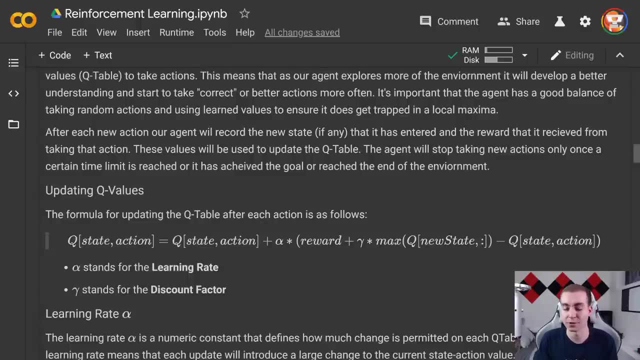 you know the maximum value we got for moving. Otherwise we're going to run into that issue which I just talked about, where we get stuck in that local maxima right. I'm not sure if I called it minimum before, But anyways. 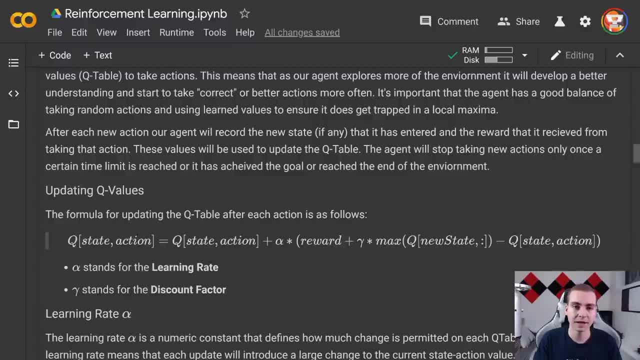 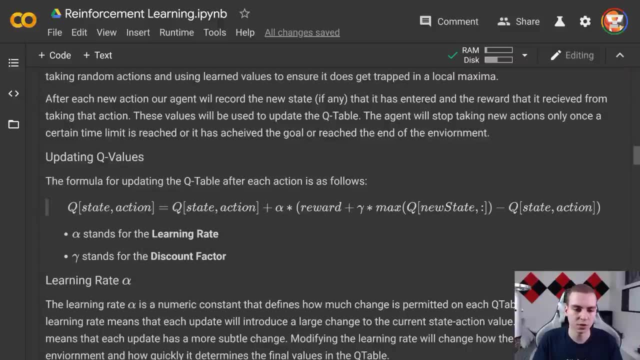 it's local maxima where we see this high reward, But that's preventing us, if we keep taking that action, from reaching a potentially high reward in a different state. So the formula that we actually use to update the cue table is this: So q state action equals q state. 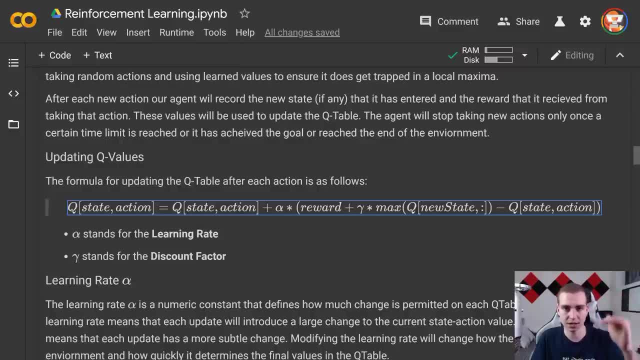 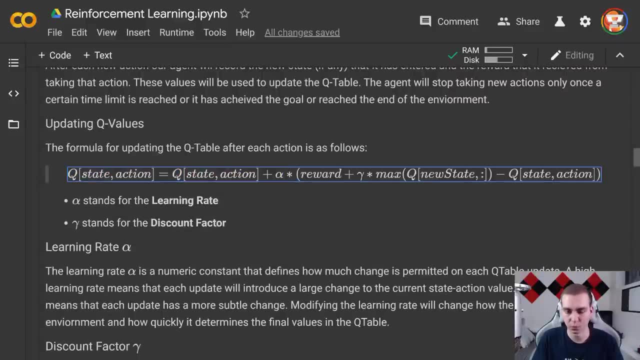 action and the state action is just referencing first the rows for the state and then the action as the column plus alpha times, and then this is all in brackets, right. reward plus: I believe this is gamma times max q of new states minus q state action. So what the heck does this mean? What are 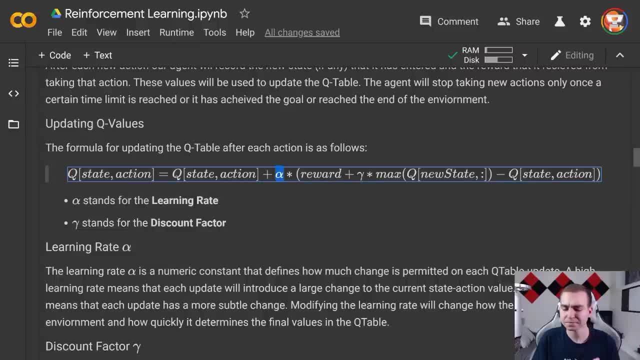 these constants? What is all this? we're going to talk about the constants in a minute, but I want to. Yeah, I want to explain this formula actually, So let's Okay. well, I guess we'll go through the constants. it's hard to go through a complicated math formula, So a stands. 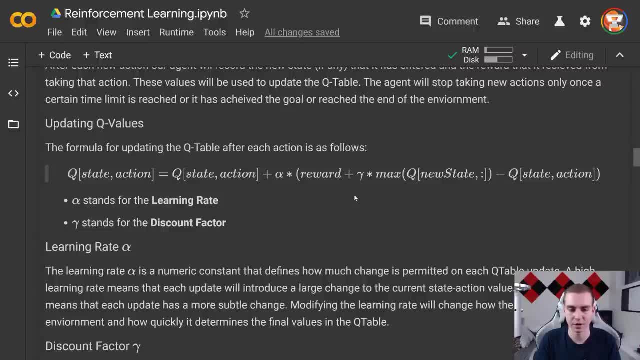 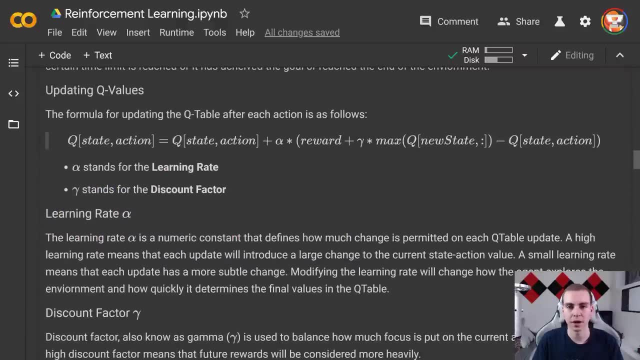 for the learning rate and gamma stands for the discount factor. So alpha learning rate, gamma discount factor. Now, what is the learning rate? Well, this is a little blurb on what this is, But essentially, the learning rate ensures that we don't update. 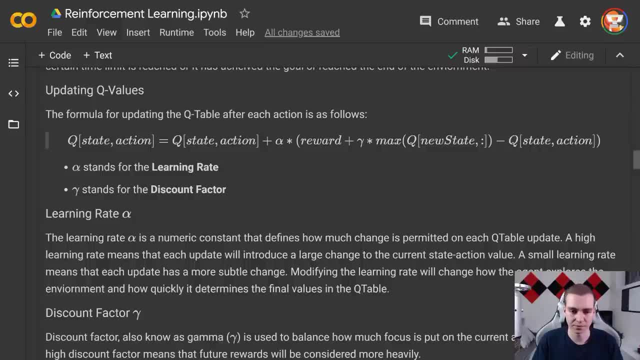 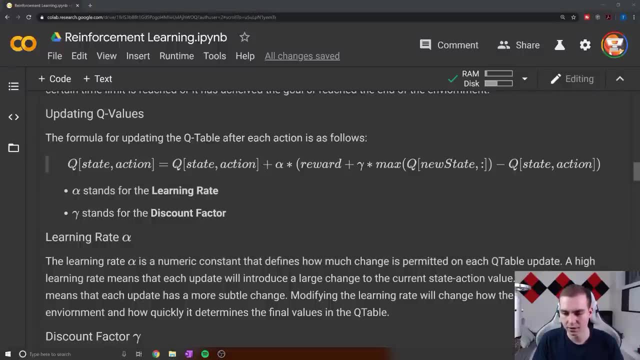 our cue table too much on every observation. So before, right when I was showing you like this: if we can go back to my Windows Ink, why is this not working? I guess I'm just not patient enough. Before, when I was showing you all I did when I took an action, was I. 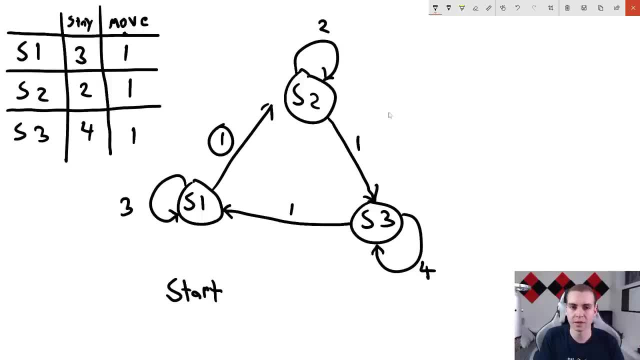 looked at the reward that I got from taking that action And I just put that in my cue table right Now. obviously, that is not an optimal approach to do this, Because that means that in the instance where we hit state one well, I'm not going to be able to get. 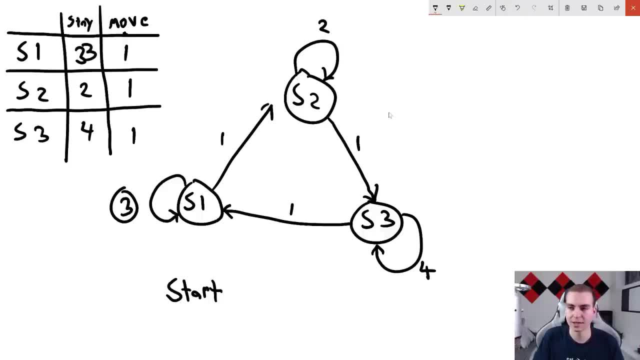 to this reward of four, because I'm going to throw that, you know, three in here and I'm just going to keep taking that action. We need to, you know, hopefully make this move, action actually have a higher value than stay, So that next time we're in state one. 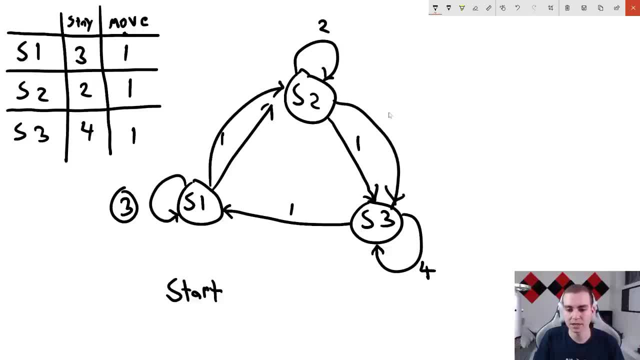 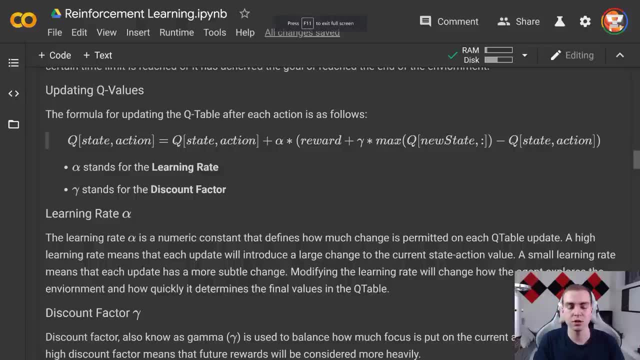 we consider the fact that we can move to state two and then move to state three to optimize our reward. Well, the learning rate is one thing that helps us kind of accomplish this behavior. Essentially, what it is telling us- and this is usually a decimal value right- is how. 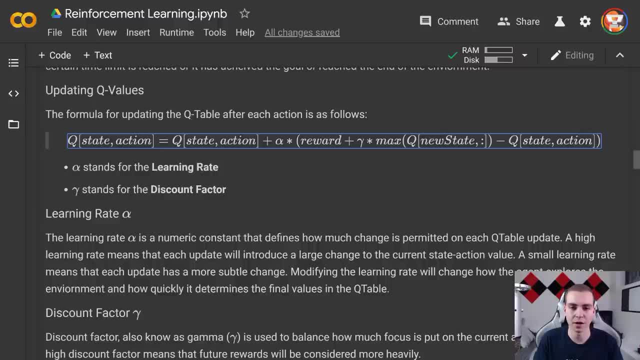 much. we're allowed to update every single cue value by on every single action or every single observation. So if we just use the approach before, then we're only going to need to observe, given the amount of states and the amount of actions, and we'll be able. 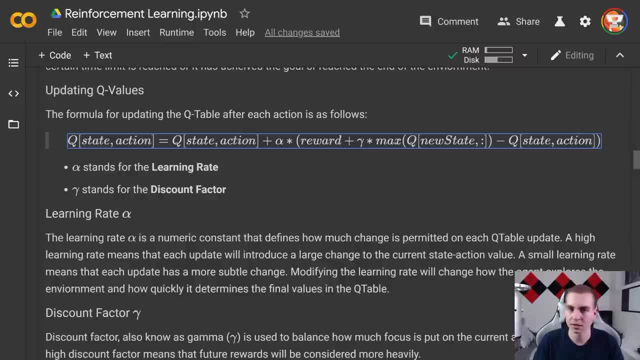 to completely fill in the cue table. So in our case, if we had like three states and three actions, we could, you know, nine iterations. we'd be able to fill the entire cue table right. So the learning rate means that it's going to just update a little bit slower. 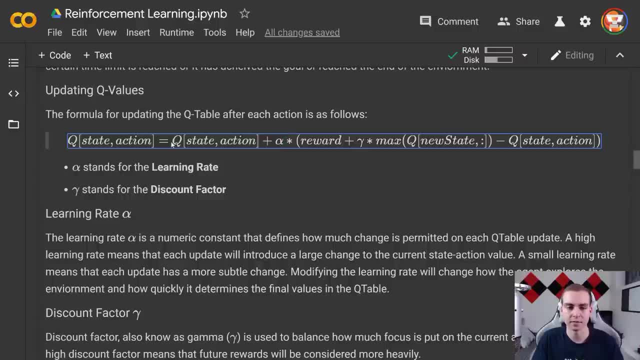 and essentially change the value in the cue table very slightly. So you can see that what we're doing is taking the current value of the cue table, so whatever is already there, And then what we're going to do is add some value here, And this value that we add is: 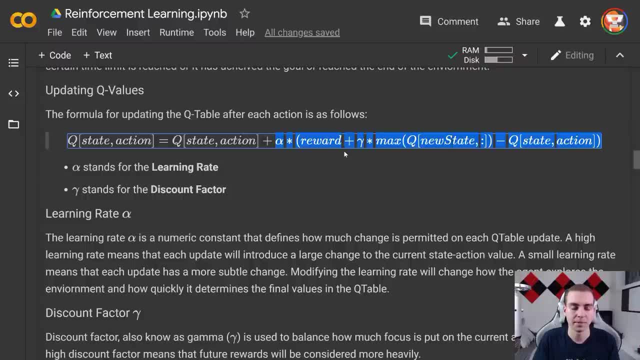 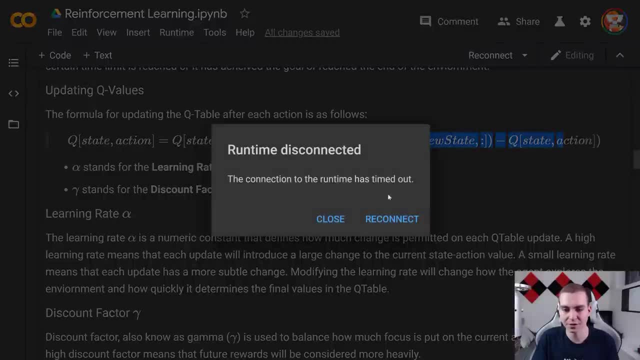 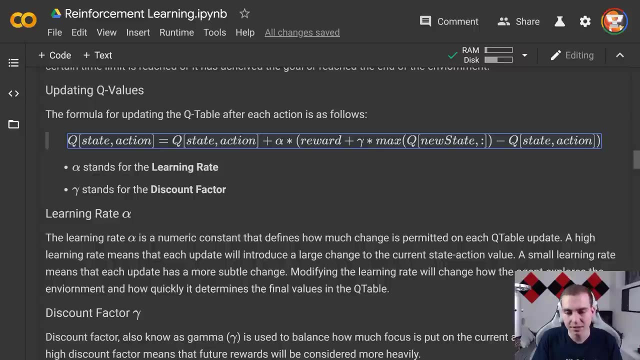 either going to be positive or negative, essentially telling us, you know, whether we should take this new action or whether we shouldn't take this new action. Now, the way that this kind of value is calculated right is obviously: our alpha is multiplied this by this, but we have the reward plus, in this case, gamma. 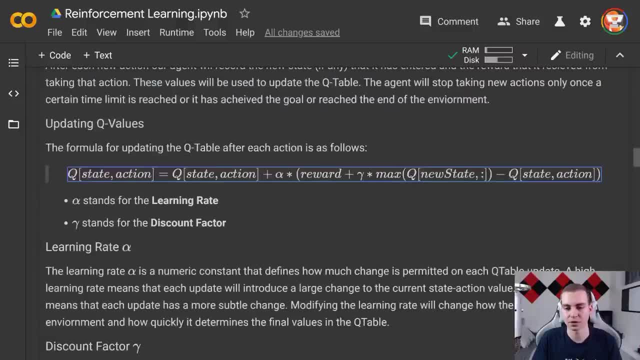 which is just going to actually be the discount factor- And I'll talk about how that works in a second- of the maximum of the new state we moved into. Now what this means is find the maximum reward that we could receive in the new state by taking any action and multiply. 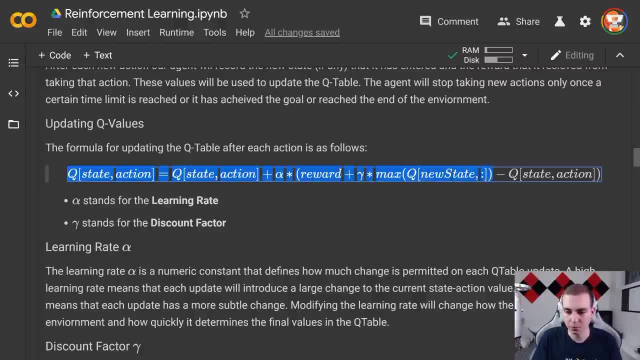 that by what we call the discount factor. What this part of the formula is trying to do is exactly what I've kind of been talking about: try to look forward and say, Okay, so I know, if I take this action in this state, I receive this amount of reward, but I need 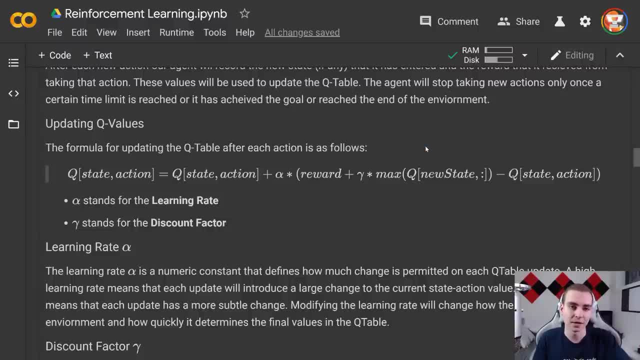 to factor in the reward I could receive in the next state so that I can determine the best place to move to. That's kind of what this max and this gamma are trying to do for us. So this discount factor- whatever you want to call it- it's trying to factor in. 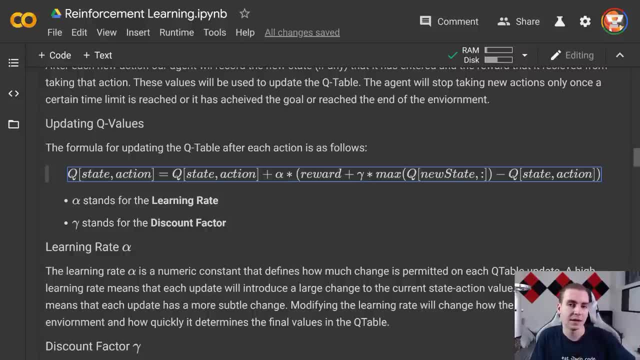 a little bit about what we could get from the next state, And so what we do is we subtract from this the state and action. This is just to make sure that we're adding what the difference was in. you know what we get from this versus. 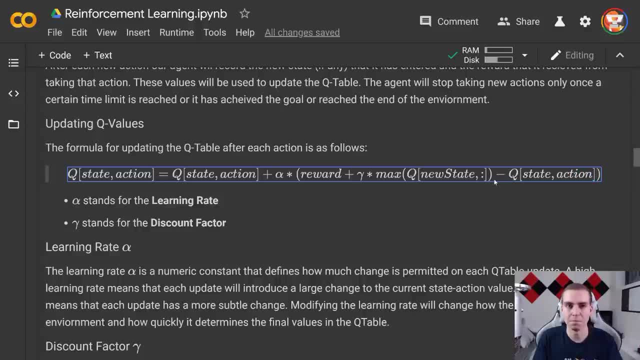 what the current value is, and not like multiplying these values crazily. I mean, you can look into more of the math here and plug in like some values later And you'll see how this kind of works. But this is the basic formula And I feel like I explained that in depth enough, Okay so, 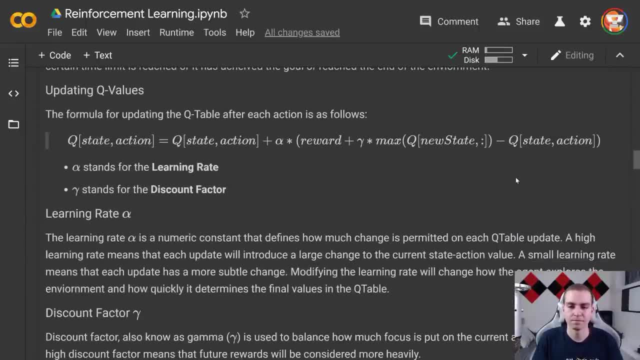 now that we've done that and we've updated this, we've learned kind of how we update the cells and how this works. I could go back to the whiteboard and draw it out, But I feel like that makes enough sense. We're going to look at what the next state is. we're going 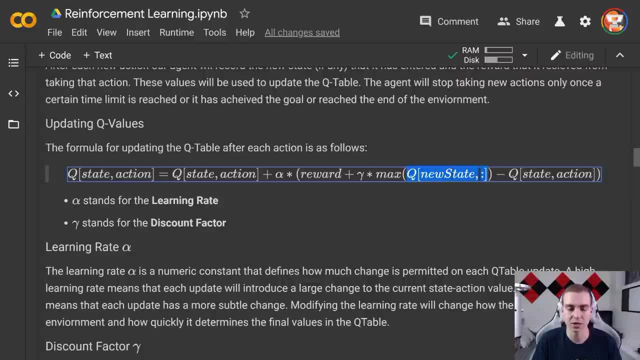 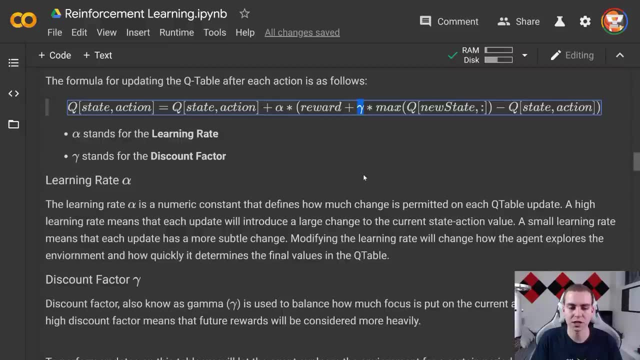 to factor that into our calculation. we have this learning rate, which tells us essentially how much we can update each cell value by, And we have this- what do you call it here? discount factor, which essentially tries to kind of define the balance between finding 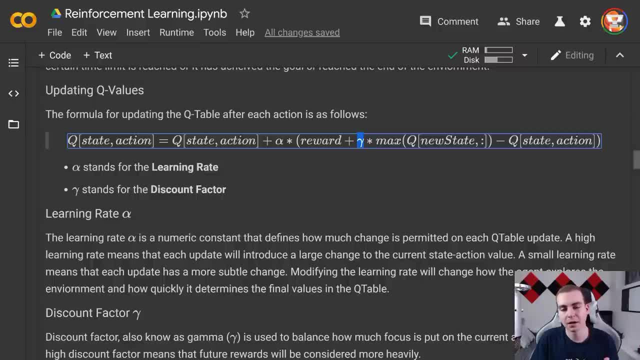 really good rewards in our current state and finding the rewards in the future state. So the higher this value is, the more we're going to look towards the future. the lower it is, the more we're going to focus completely on our current reward right And obviously, 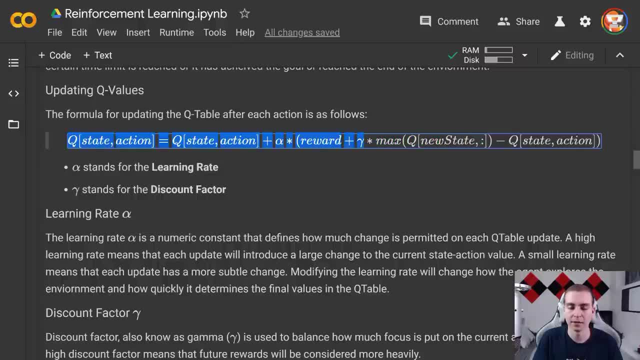 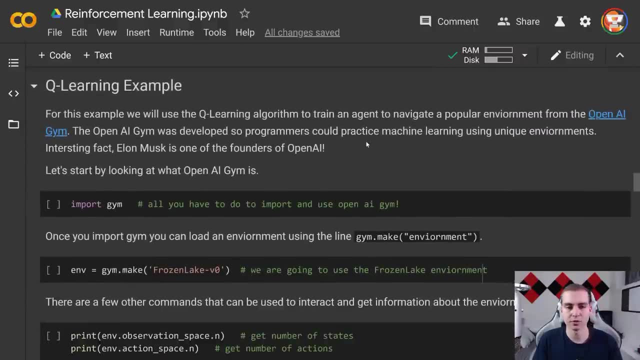 that makes sense, because we're going to add the maximum value, And if we're multiplying that by a lower number, that means we're going to consider that less than a, And if that was greater, awesome, Okay. So now that we kind of understand that, I want. 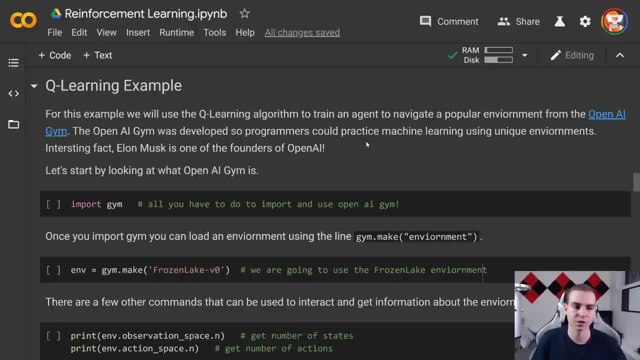 to move on to a Q learning example, And what we're going to do for this example is actually use something called the open AI gym. I just need to throw my drawing tablet away right there so that we can get started, But open AI gym is actually a really interesting kind. 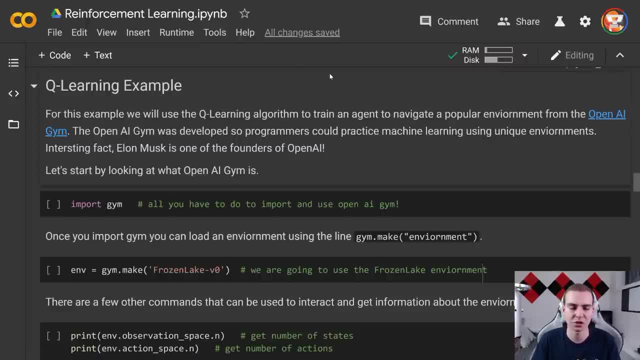 of module- I don't even- actually- I don't even really know the way to describe it- almost tool. there's actually developed by open AI- you know, coincidentally, by the name- which is founded by Elon Musk and someone else. So he's actually, you know, made this kind of- I don't really 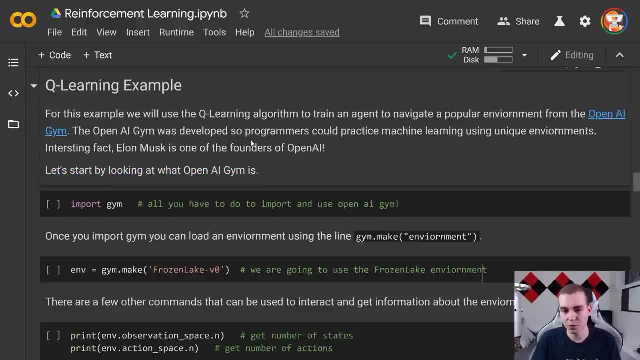 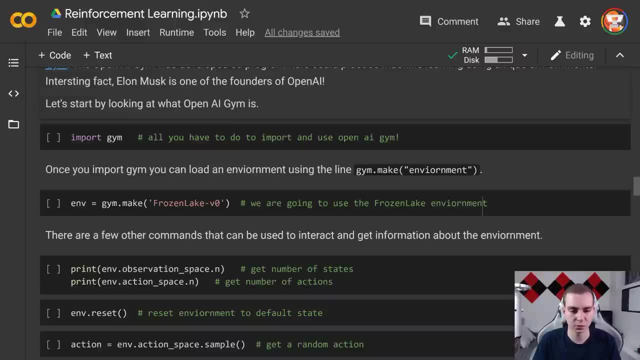 don't know the word to describe it. I almost want to say tool that allows programmers to work with these really cool gym environments and train reinforcement learning models. So you'll see how this works in a second, But essentially there's a ton of graphical environments. 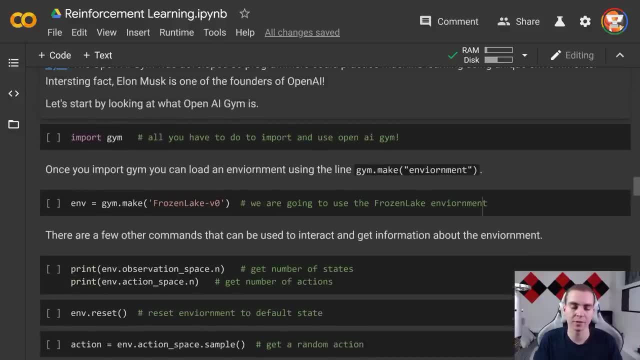 that have very easy interfaces to use, So like moving characters around them, that you're allowed to experiment with completely for free as a programmer, to try to, you know, make some cool reinforcement learning models. That's what open AI is, So that's kind of. 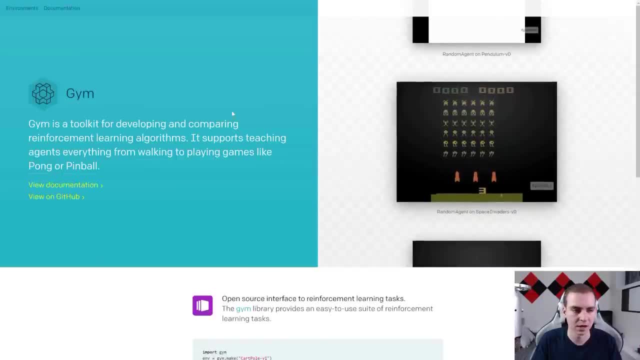 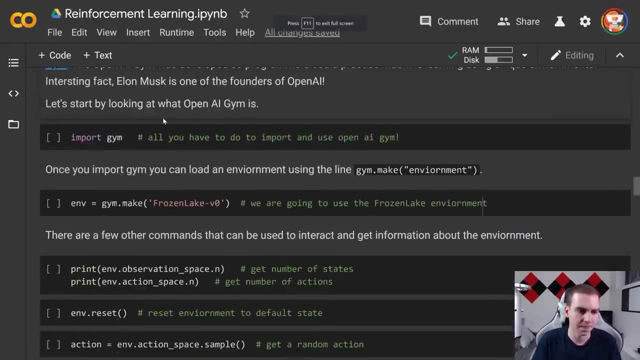 what open AI gym is And you can look at it. I mean, we'll click on it here actually to see what it is. you can see, Jim, there's all these different Atari environments And it's just a way to kind of train reinforcement learning models. Alright, so now we're going. 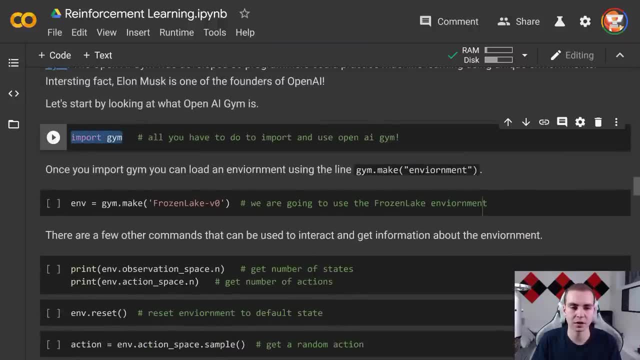 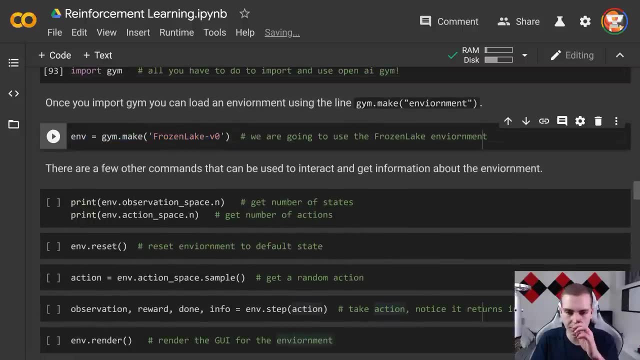 to start by just importing Jim. if you're in Collaboratory, there's nothing you need to do here. If you're in your own thing, you're gonna have to pip install Jim, And then what we're gonna do is make this frozen like v zero gym. So essentially, what this does is: 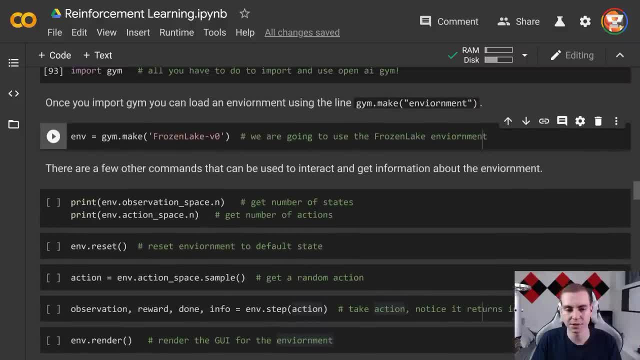 just set up the environment that we're going to use Now. I'll talk more about what this environment is. later We're going to talk about how Jim works, because we are going to be using this throughout the thing. So the open AI gym is meant for reinforcement learning And essentially what it has is. 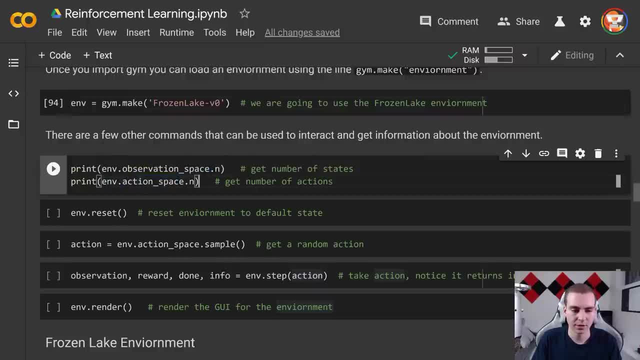 an observation space and an action space for every environment. Now, the observation space is what we call our environment, right, And that will tell us the amount of states that exist in this environment. Now, in our case, we're going to be using kind of like a maze. 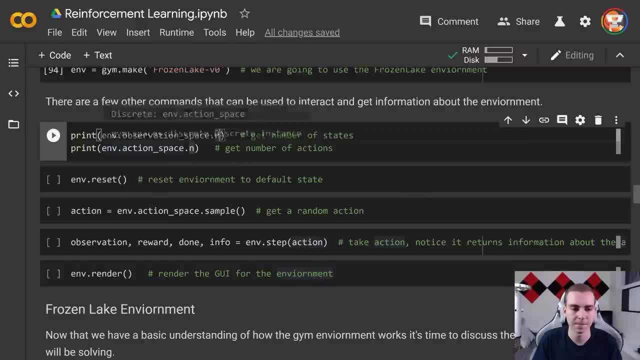 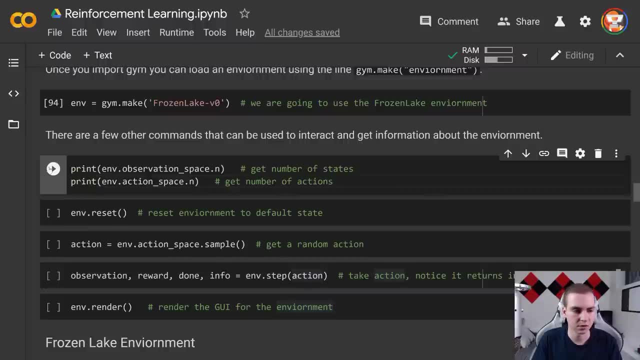 like thing, which I'll show you in a second. So you understand why we get the values we do. Action space tells us how many actions we can take when we do the dot n at any given state. So if we print this out, we get 16. 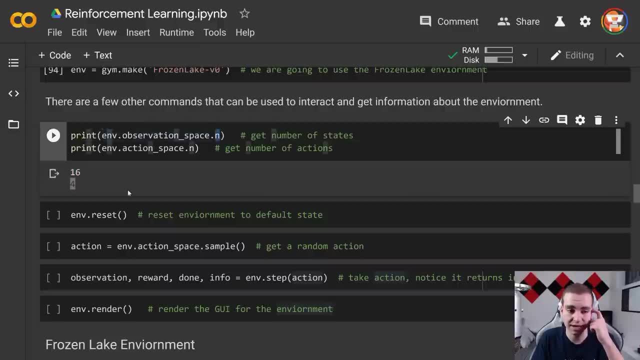 and four representing the observation space. In other words, the number of states is 16.. And the amount of actions we can take in every single state is four. Now, in this case, these actions are gonna be left down, up and right, But yes, now Env dot reset. So essentially, 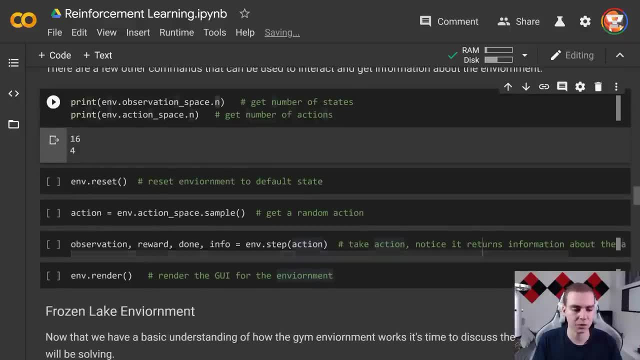 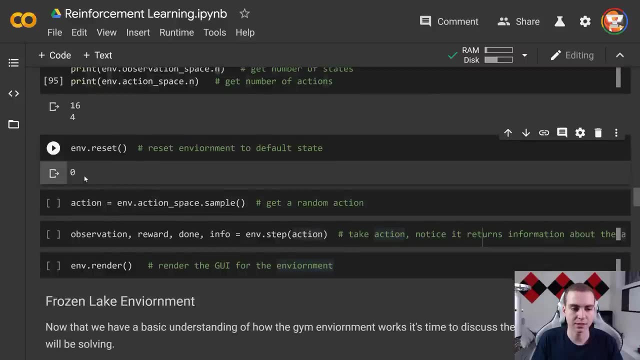 we have some commands that allow us to move around the environment, which are actually down here, if we want to reset the environment and start back in the beginning- So we're going to go back to the start state- then we do Env dot reset. you can see this actually. 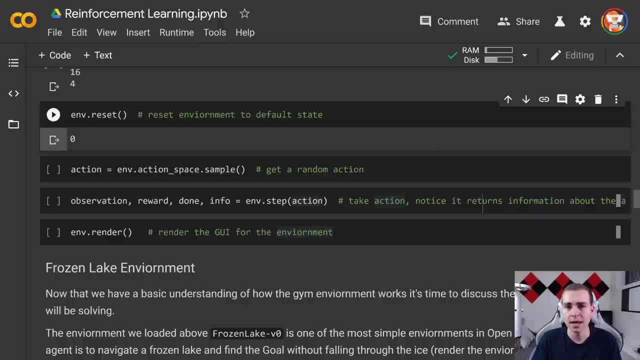 returns to us the starting state, which obviously is going to be zero. Now we also have the ability to take a random action or select a random action from the action space. So what this line does right here is say of the action space, so of all the commands, that 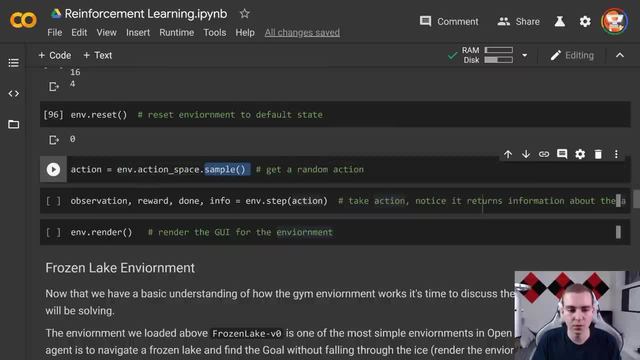 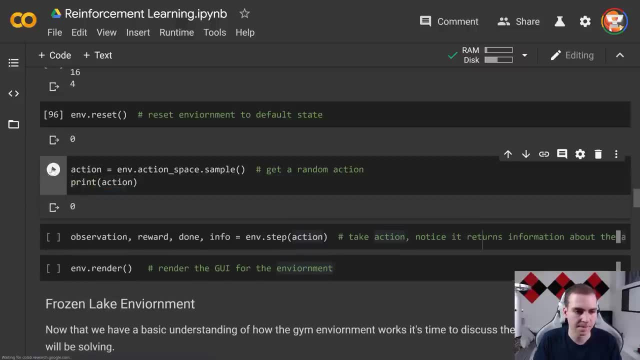 are. there are all the actions we could take. pick a random one and return that. So if you do that, actually let's just print action and see what this is. you'll see we get zero two right. So we get zero two, three, four, five, six, six, seven, eight, nine, 10,, 10,. 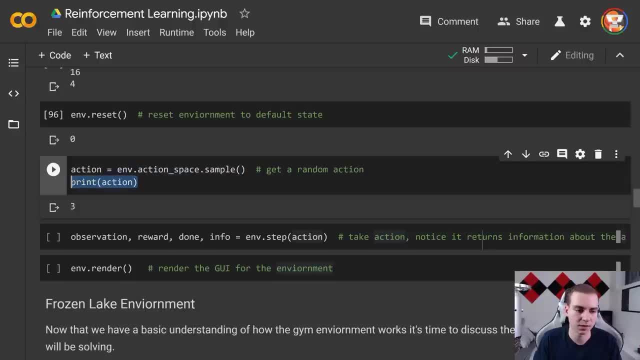 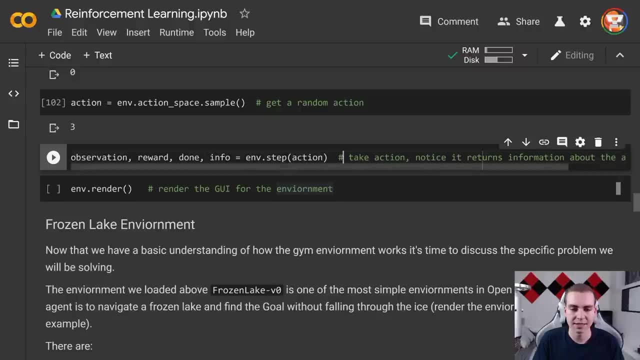 right, it just gives us a random action that is valid from the action space. Alright. next, what we have is this: Env? dot step in action. Now, what this does is take whatever action we have, which in this case is three, and perform that in the environment. So tell our. 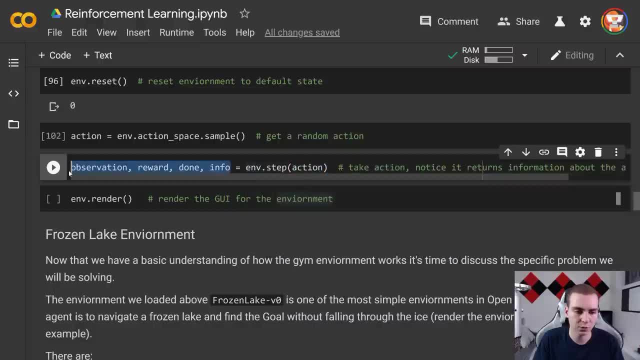 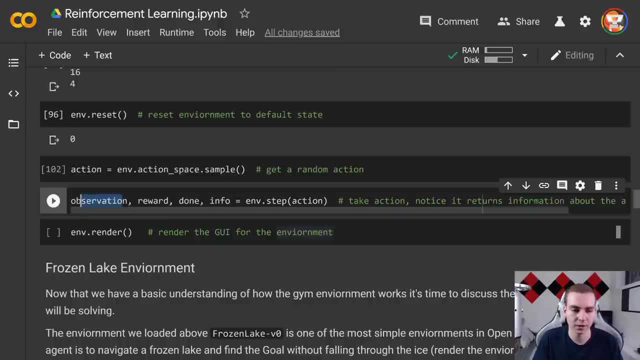 agent to take this action in the environment and return to us a bunch of information. So the first thing is the observation, which essentially means: what state do we move into next? So I could call this new source state. reward is: what reward did we receive by taking that action? So this will. 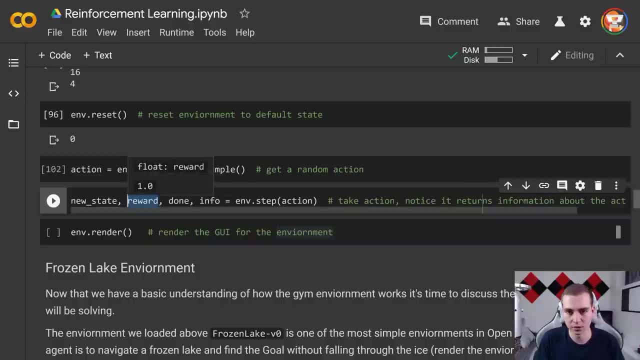 be some value right in our. in this case, the reward is either one or zero, But that's not that important to understand. And then we have a bool of done which tells us: did we lose the game Or did we win the game, Yes or no, So true? So if this is true, what this? 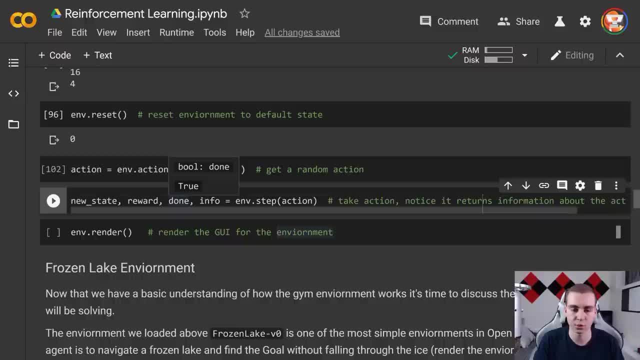 means is we need to reset the environment because our agent either lost or one and is no longer in a valid state in the environment. Info gives you us a little bit of information that's not showing me anything here. we're not going to use info throughout this, but 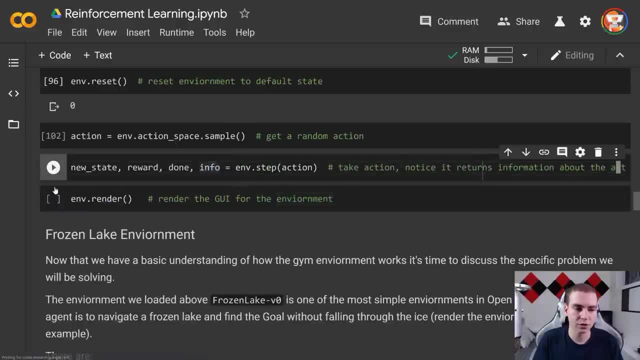 figured. I'd let you know that Now env dot render, I'll actually render this for you and show you renders, a graphical user interface that shows you the environment. Now, if you use this while you're training, so you actually watch the agent do the training, which is. 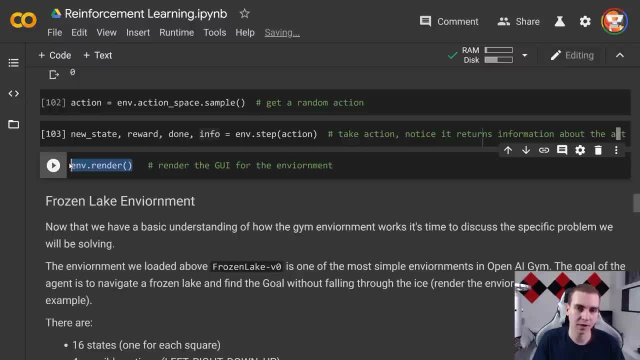 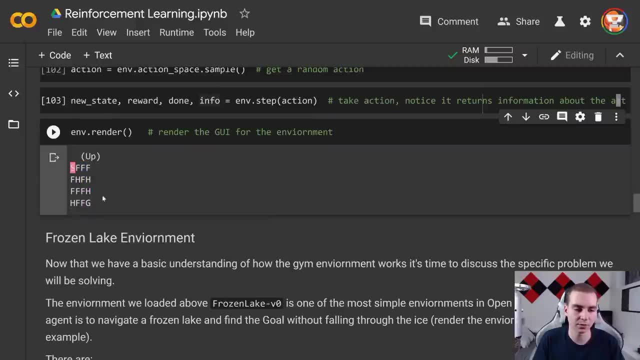 what you can do with this. it slows it down drastically, like probably by you know, 10 or 20 times, because it actually needs to draw the stuff on the screen. But you know you can use it if you want. So this is what our frozen lake example looks like. you can see. 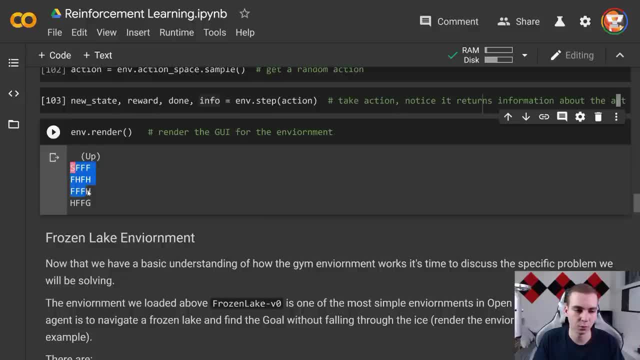 that the highlighted square is where our agent is, And in this case we have four different blocks. We have s, f, h and g, So s stands for start, f stands for frozen. This is a frozen lake, And the goal is to navigate to the goal without falling in one of the holes which 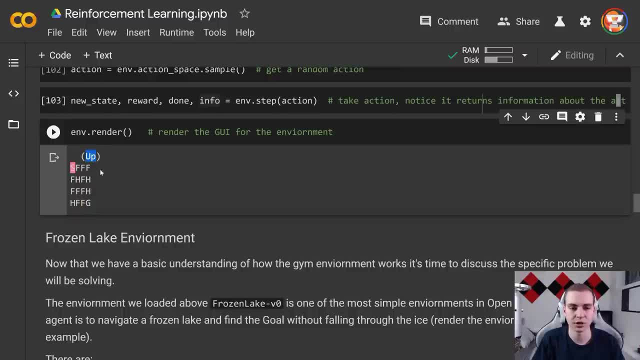 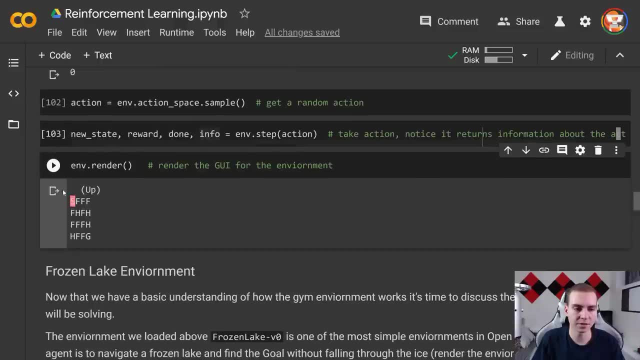 is represented by H, And this here tells us the action that we just took. Now I guess the starting action is up, because that's zero, I believe, But yes, so if we run this a bunch of times, we'll see this updating. 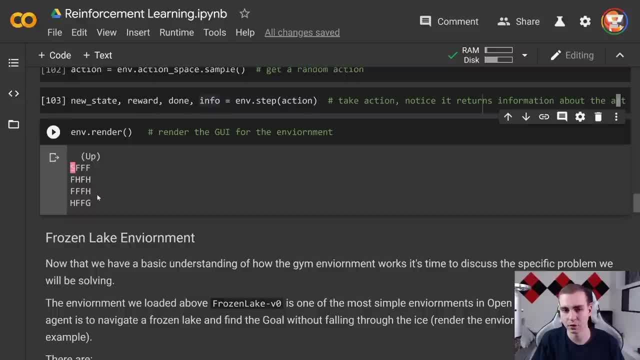 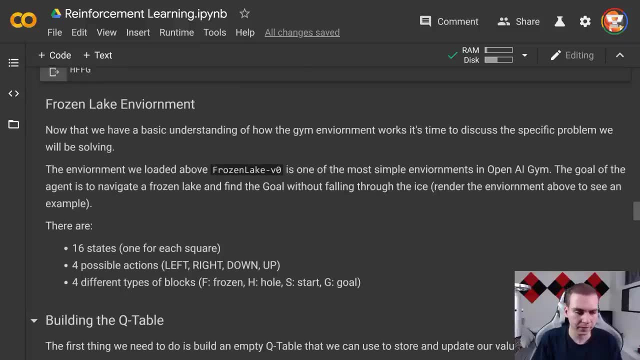 Unfortunately doesn't work very well in Google Collaboratory, the, the GUIs, But if you did this in your own command line and, you like, did some different steps and rounded it all out, you would see this working properly. Okay, so now we're on to talking about the frozen lake environment. 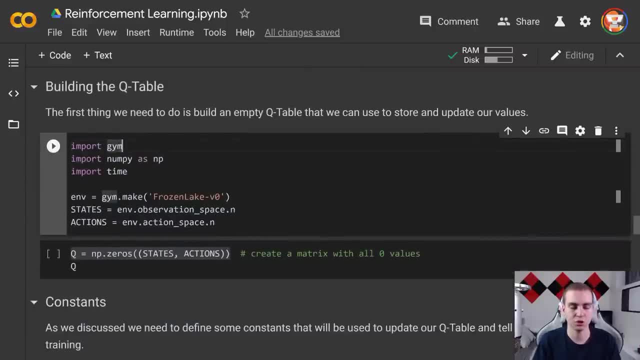 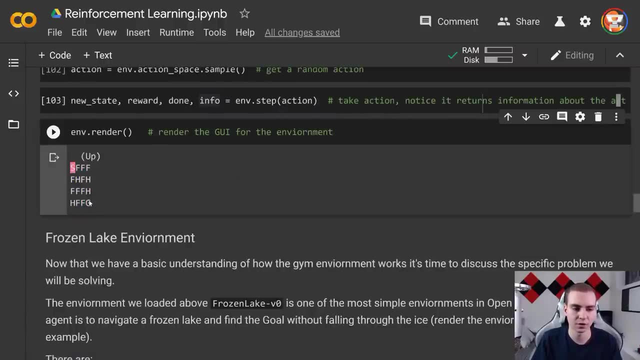 which is kind of what I just did. So now we're just going to move to the example where we actually implement Q learning to essentially solve the problem. how can we train an AI to navigate this environment and get to the start, to the goal? How can we do that? Well, 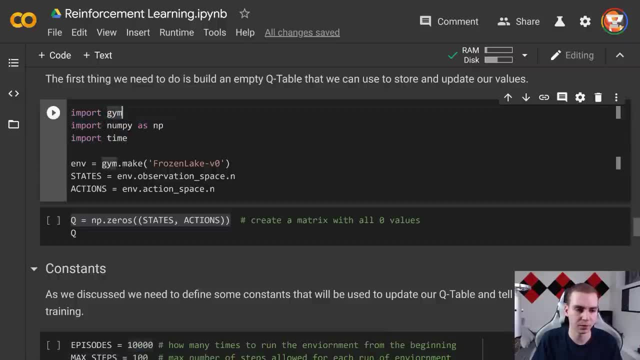 we're gonna use Q learning, So let's start. So the first thing we need to do is import Jim, import numpy and create some constants here. So we'll do that. we're going to say the amount of states is equal to the line I showed you before. So Env dot observation space, dot n actions. 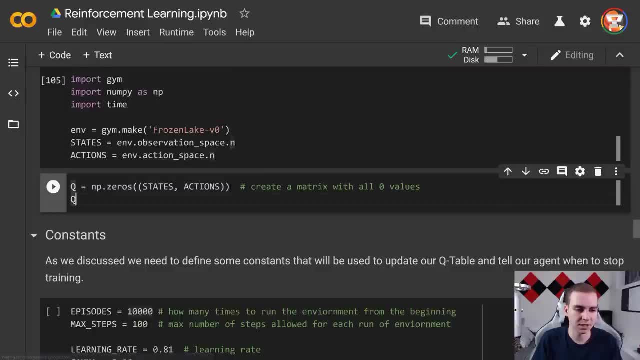 is equal to Env dot action space n. And then we're going to say q is equal to np dot zeros, states and actions. So something I guess I forgot to mention is when we initialize the queue table, we just initialize all blank values or zero values, Because obviously 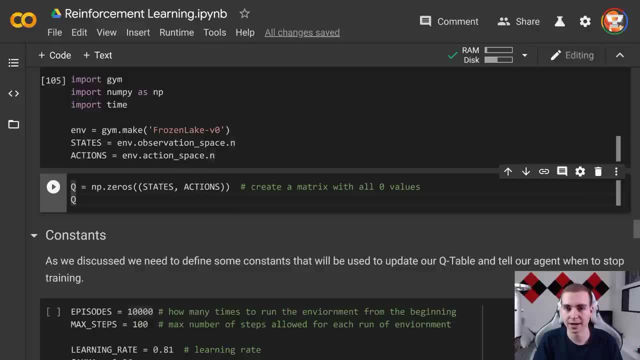 at the beginning of our learning. our model or agent doesn't know anything about the environment yet, So we just leave those all blank, Which means we're going to more likely be taking random actions at the beginning of our training, trying to explore the environment space more, And then as we get further on and 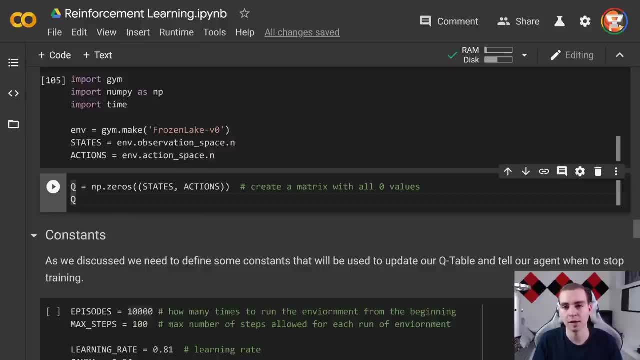 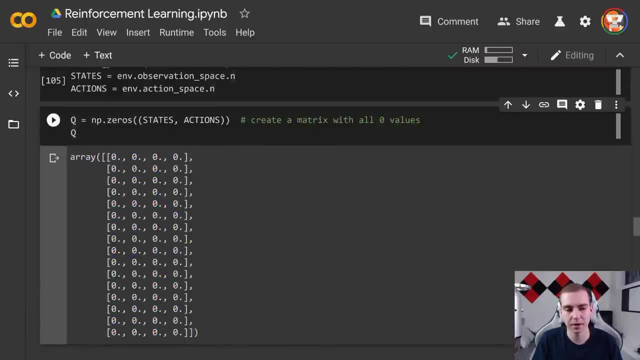 learn more about the environment. those actions will likely be more calculated based on the queue table values. So we print this out. we can see this is the array that we get. we've had to be build a 16 by four. I guess, not array. Well, I guess this technically. 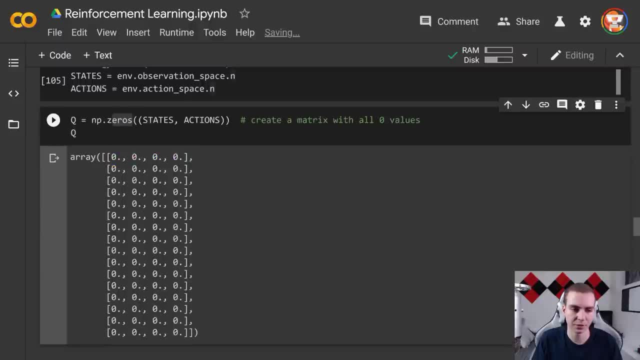 is an array queue and we'll call it matrix 16 by four. So every single row represents a state and every single column represents an action that could be done in the next row. So we're going to be taking random actions at the beginning of our training, trying to 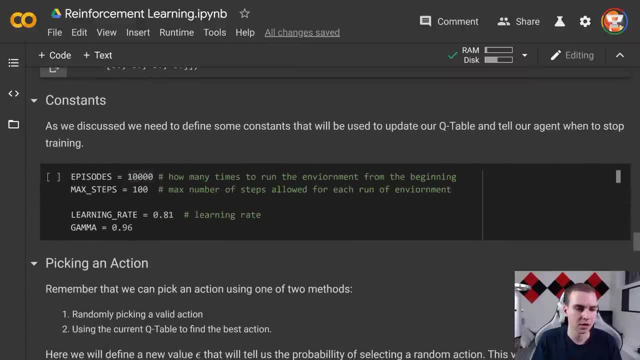 capture the graves ofims And we're going to call them 16 by four. So at the top of our code we're going to say: let's run some nursing class And this will bring in an order list of revenues, In this case where our agent is now. let's say, every year I have eight. 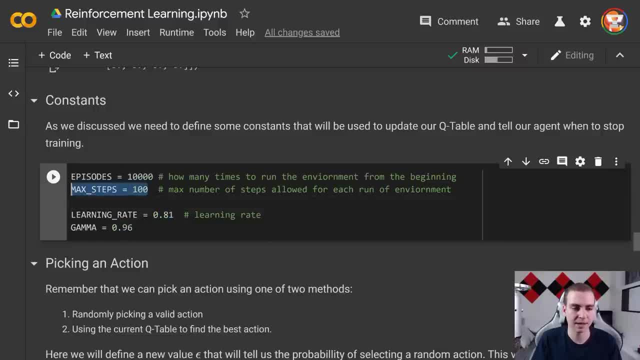 shower head And in was our agent conditions, And then also the pins for each step. so as they pass through each step, the really, really important thing to know is that everything that we say is so important to explain should be explained, all the actions. So we want to remember before we introduce our property. we want to make sure that removing integer addresses from each step is warranted, and then we need a certain value for each person every time we pass through a new state to thatECH keyings. just like a long ago, we 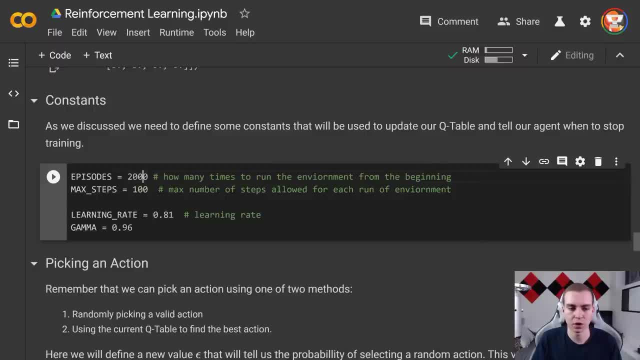 can define an initial value data and then we can define some remote indexing like this: many episodes you want to train your agent on. So how many times do you want it to run around and explore the environment? That's what episode stands for. Max steps essentially says Okay. 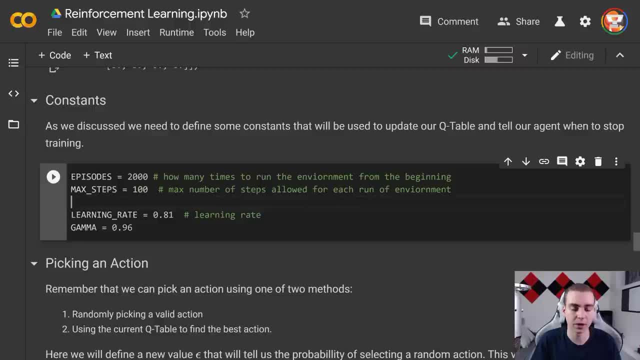 so if we're in the environment and we're kind of navigating and moving around, we haven't died yet. how many steps are we going to let the agent take before we cut it off? Because what could happen is we could just bounce in between two different states indefinitely. So we need to make sure we 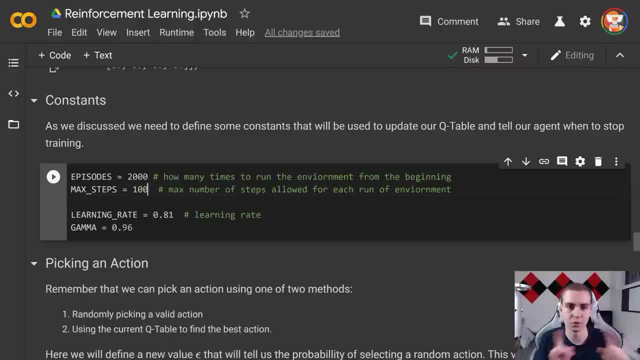 have a max steps so that at some point, if the agent is just doing the same thing, we can, you know, end that, or if it's like going in circles, we can end that and start again with different, you know- Q values. Alright, so episodes. yeah, we already talked about that learning rate. 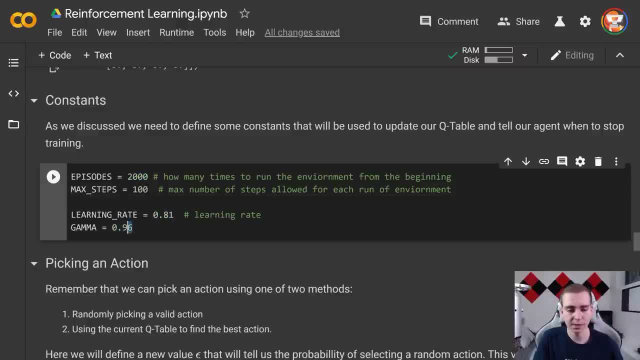 we know what that is gamma, we know what that is mess with these values. as we go through you'll see the difference it makes in our training. I've actually included a graph down below So we'll talk about that kind of show us the outcome of our training. but learning rate. 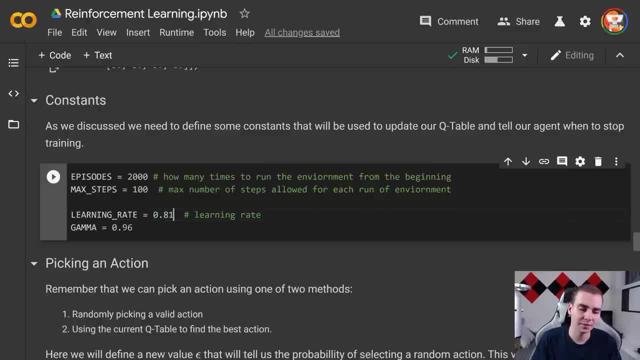 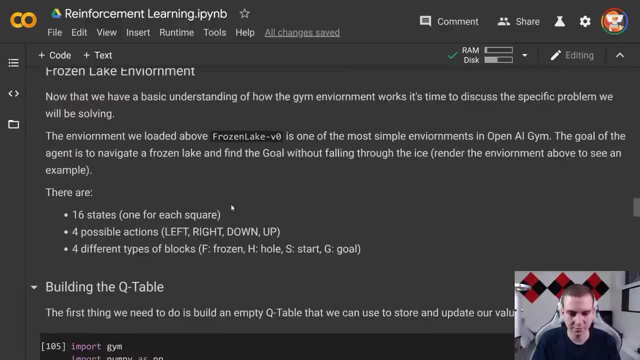 the higher this is, the faster I believe that learns. yes, So a high learning rate means that each update will introduce larger change to the current state. So yeah, so that makes sense, based on the equation as well. Just wanted to make sure that I wasn't going crazy there, So let's run this constant block to make. 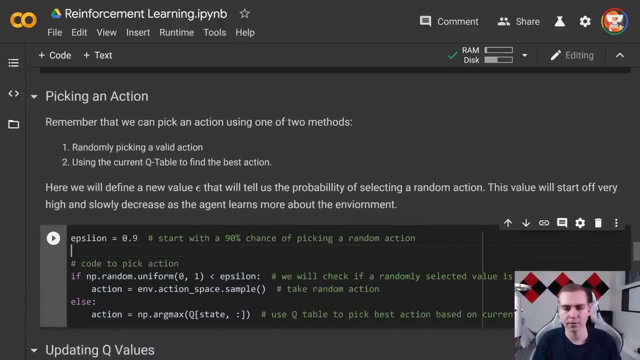 sure, And now we're going to talk about picking an action. So remember how I said- and I actually wrote them down here- there's essentially two things we can do at every- what do we call it- step right. We can randomly pick a valid action, or we can use the current queue table to find 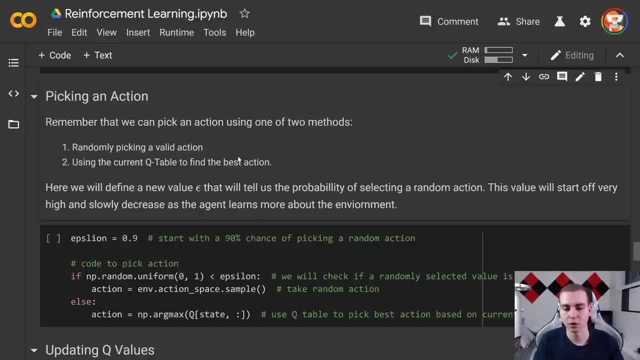 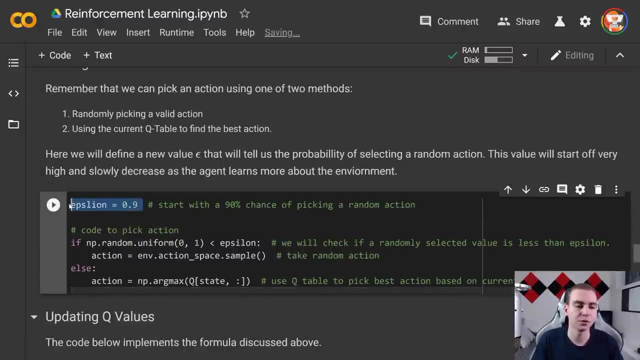 the best action. So how do we actually implement that into our open AI gym? Well, I just wanted to write a little codeblock here to show you the exact code that will do this for us. So we're going to introduce this new concept or this new can, almost call it constant, called epsilon, And I 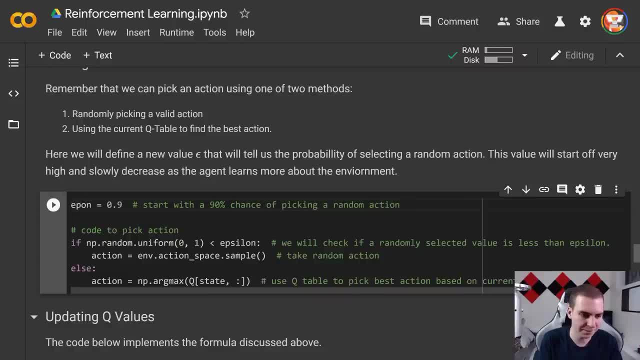 think epsilon- I think I spelled this wrong- Hep, So long, yeah, that should be how you spell it. So we're gonna start. the epsilon value essentially tells us the percentage chance that we're going to pick a random action. So here we're gonna use a 90% Epsilon. 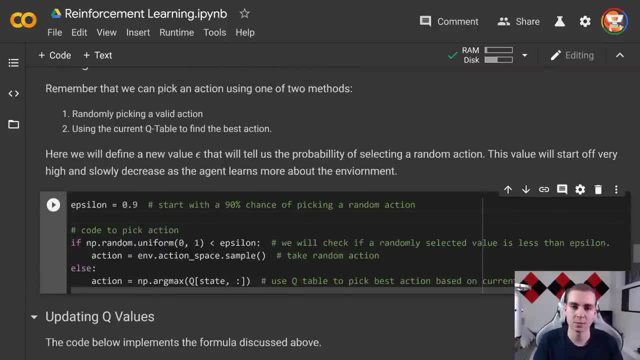 which essentially means that every time we take an action, there's gonna be a 90% chance that's random and 10% chance that we look at the cue table to make that action. Now we'll reduce this epsilon value as we train so that our model will start being able to explore you. 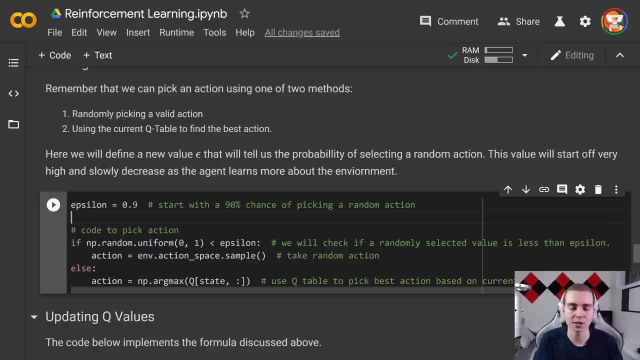 know as much as it possibly can in the environment by just taking random actions, And then, after we have enough observations and we've explored the environment enough, we'll start to slowly decrease the epsilon so that it hopefully finds a more optimal route for things to do. 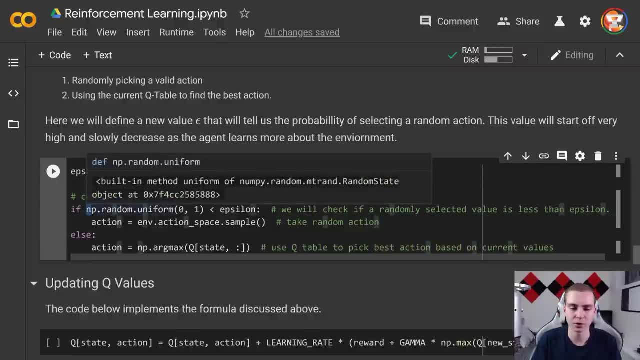 Now the way we do this is we save np dot, random dot, uniform 01, which essentially means pick a random value between zero and one is less than epsilon and up Solon like that's. I think I'm gonna have to change some other stuff, But we'll see that action equals env. 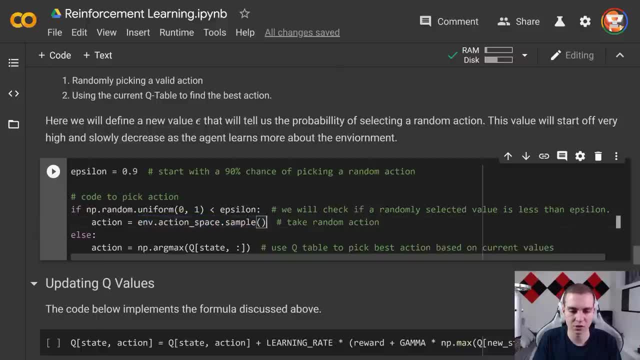 dot action space Sample. So take a random action. that's what this means. store what that action is in here. Otherwise we're going to take the argument max of the state row in the cue table. So what this means is so our argument. 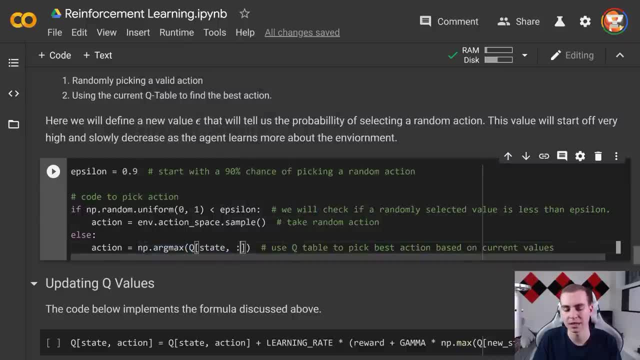 arbitrary. It's in in the middle, so put in theücht. So what this two takes is we're means is find the maximum value in the Q table and tell us what row it's in, So that way we know what action to take. So if we're in row, I guess not. sorry, not row column for. 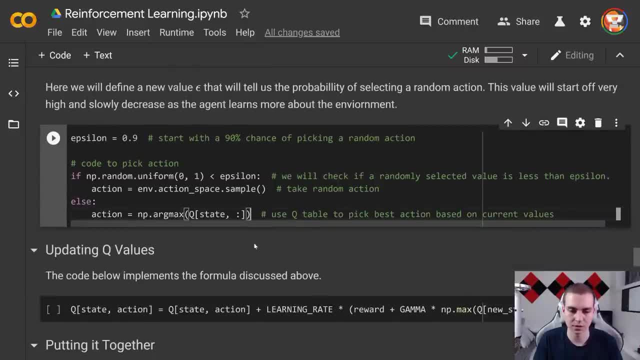 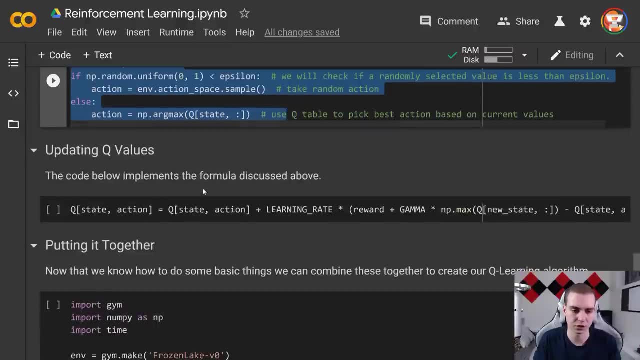 in column one. you know that's the maximum value. take action one. that's what this is saying. So using the Q table to pick the best action. Alright, so we don't need to run this, because this is just going to be which. I just wrote that to show you. Now how do we update? 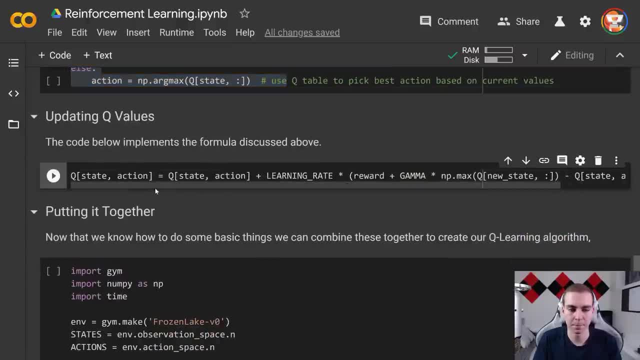 the Q values. Well, this is just following the equation that I showed above. So this is the line of code that does this. I just want to write it out So you guys could see exactly what each line is doing and kind of explore it for yourself. But essentially, 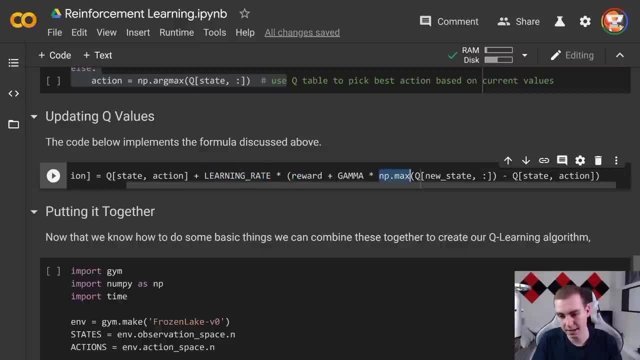 you get the point. you know you have your learning rate, reward gamma. take the max, So NP dot max does the same thing as a max function in Python. this is going to take the max value, not the argument max, from the next state, right, the new state that we moved. 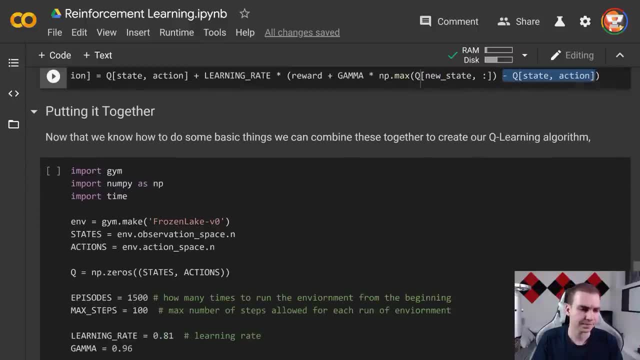 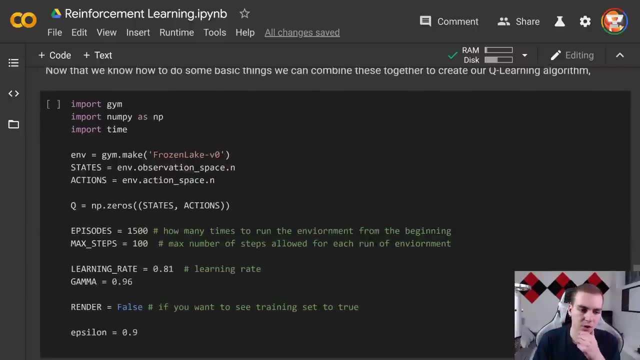 into and then subtracting, obviously, the Q state action. Alright, so putting it all together. So now we're actually going to show how we can train and create this Q table and then use that Q table. So this is the pretty much all. 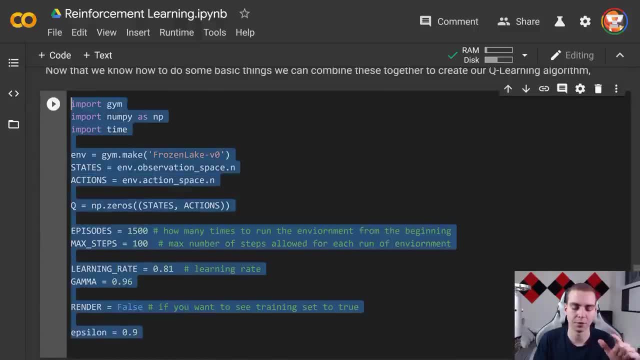 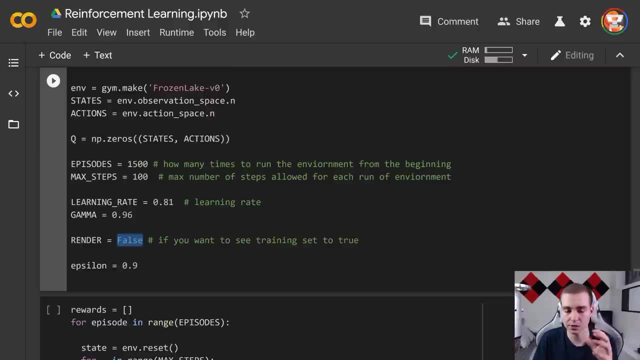 this code that I have. we've already actually written at least this block here. that's why I put it in its own block. So just all the constants. I've included this render constant to tell us whether we want to draw the environment or not. in this case, I'm gonna leave it false. 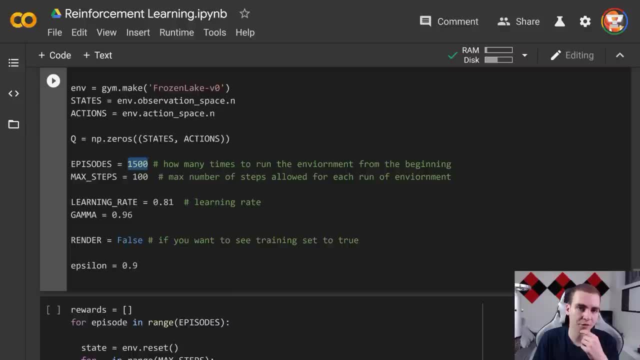 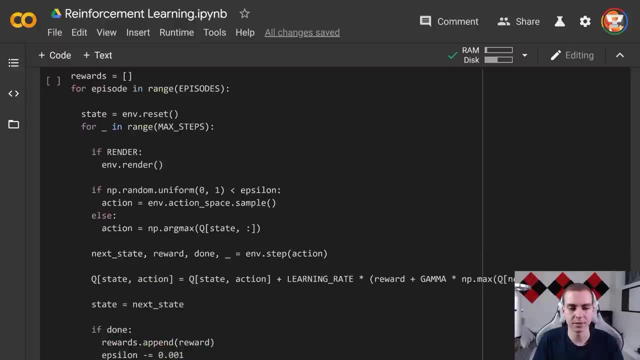 but you can make it true if you want episodes. I've left at 1500.. For this, if you want to make your model better, typically you train it on more episodes, But that's up to you. And now we're gonna get into the big chunk of code which I'm going to talk about. So 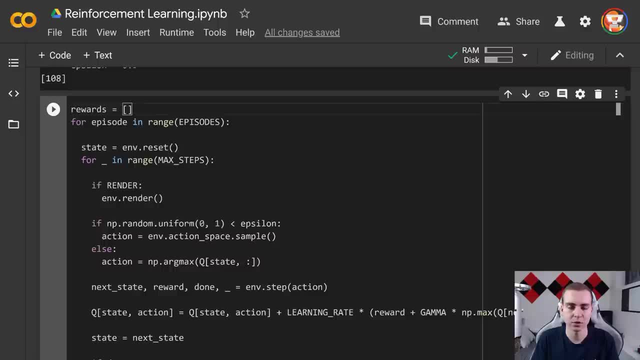 what this is going to do. we're gonna have a rewards list which is actually just going to store all the rewards we see, just so I can graph that later for you guys. then we're going to say for episode, in range episodes. So this is just telling us, you know, for every episode, let's do the steps. I'm about. 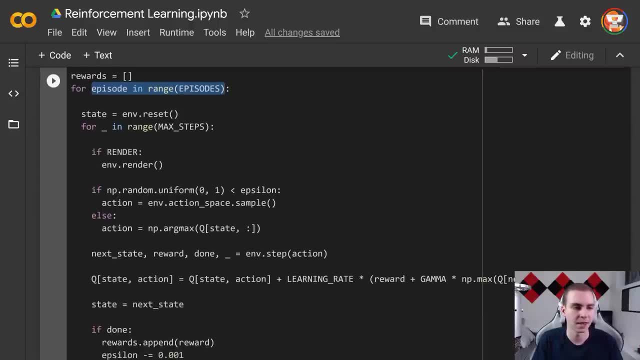 to do So: maximum amount of episodes, which is our training length. essentially we're going to reset the state, obviously, which makes sense. So state equals in V, dot reset, which will give us the starting state we're going to say for underscore in range, max steps. 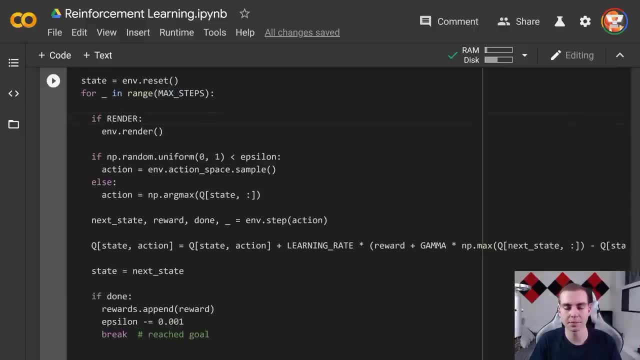 which means, okay, we're going to do. you know, we're going to explore the environment up to maximum steps. we do have a done here which will actually break the loop if we've reached the goal, which we'll talk about further. So the first: 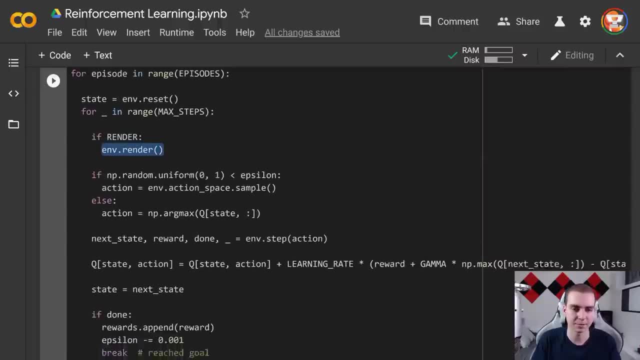 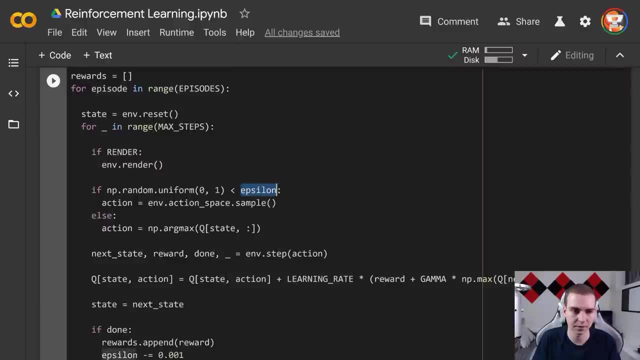 thing we're gonna do is say: if render, you know, render the environment, that's pretty straightforward, Otherwise let's take an action. So for each time step we need to take an action. So epsilon, I think, is spelled correctly here. Yeah, believe that's right. 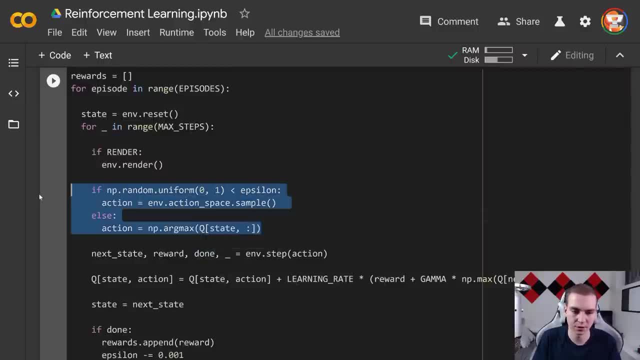 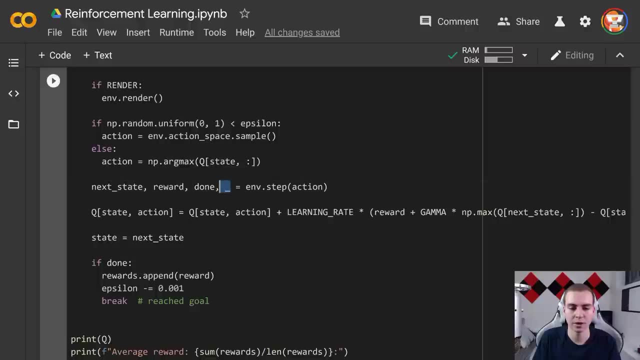 So I'm gonna say: action equals EMV dot action space. this is already the code we've looked at. And then what we're gonna say is: next state reward done underscore equals EMV dot step action. we've put an underscore here because we don't really care about this in. 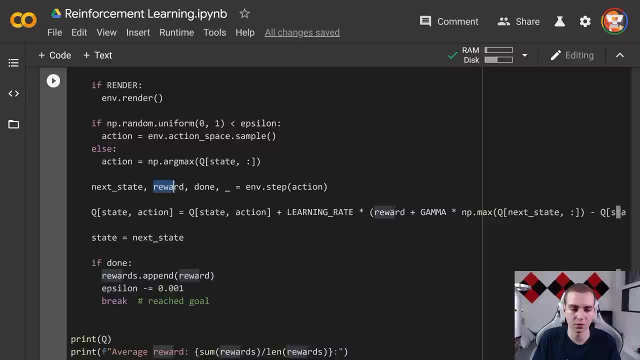 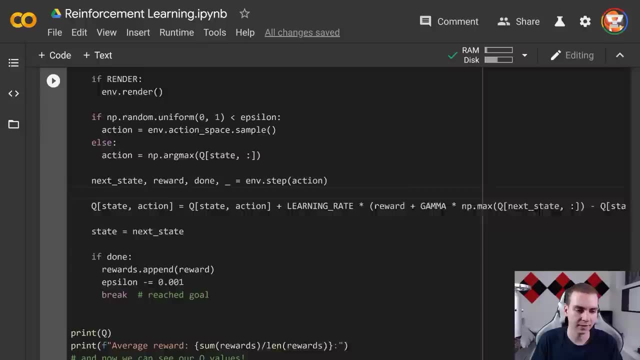 info value So I'm not going to store it. But we do care about what the next state will be, the reward from that action, and if we were done or not, So we take that action. that's what does this EMV dot step. And then what we do is say q state action. we just 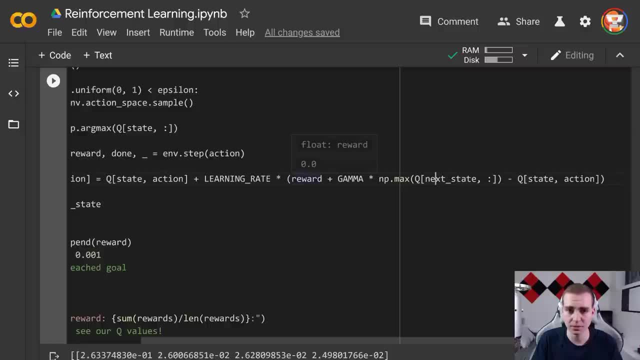 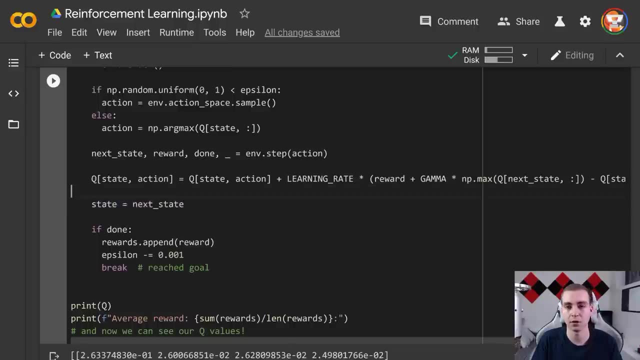 update the Q value using the formula that we've talked about. So this is the formula. you can look at it more in depth if you want, But based on whatever the reward is. you know, that's how we're going to update those Q values And after a lot of training we should have 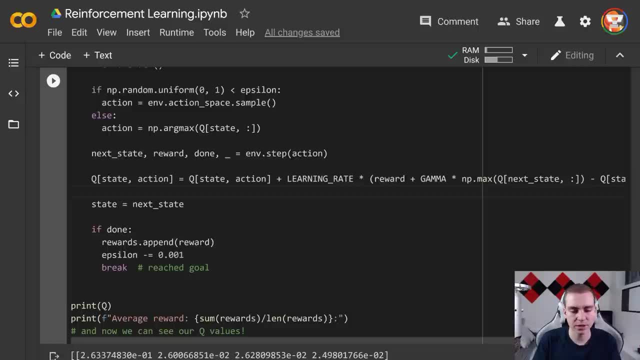 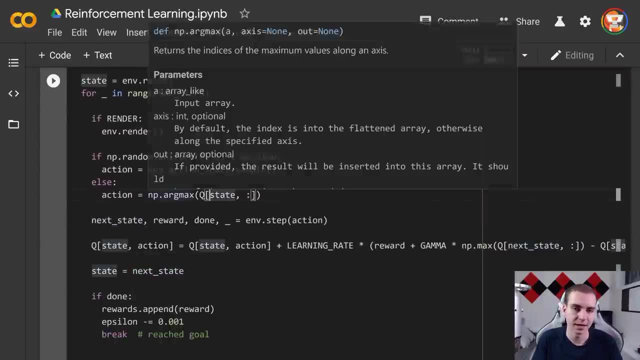 some decent Q values in there, All right. So then we set the value of the action and the current state to be the next state, so that when we run this time step again now, our agent is in the next state and can start exploring the environment again in this current 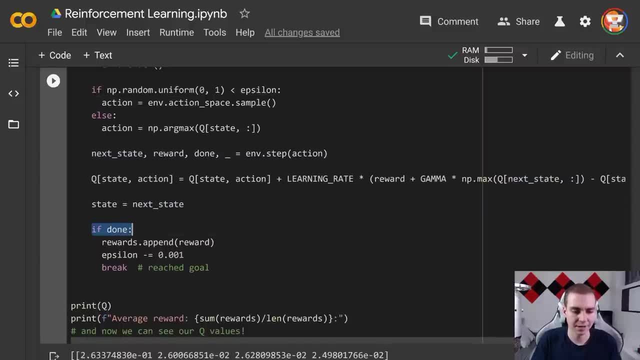 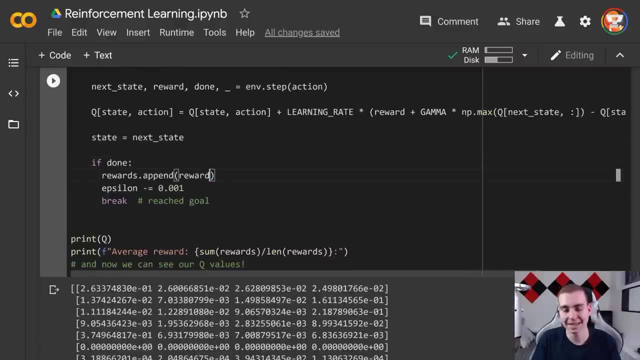 you know, iteration, almost, if that makes sense. So then we say: if done so, essentially if the agent died or if they lost or whatever it was, we're going to append whatever reward they got from their last step into the rewards up here. And it's worthy of noting that the 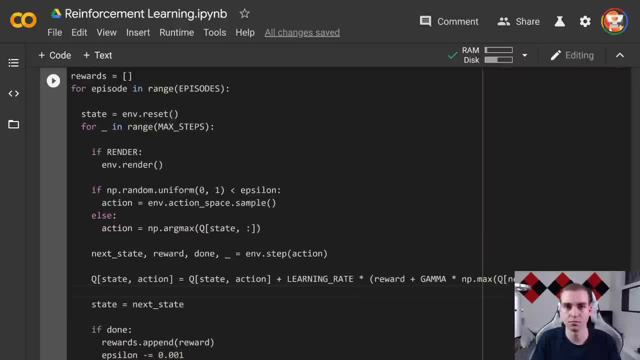 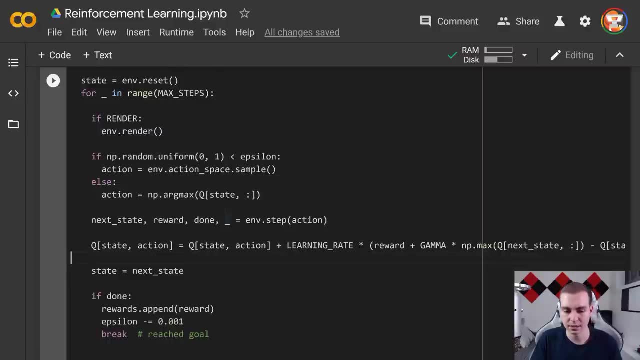 way the rewards work here is you get one reward If you move to a valid block and you get the zero reward if you die. So every time we move to a valid spot we get one, otherwise we get zero. I'm pretty sure that's the way it works. 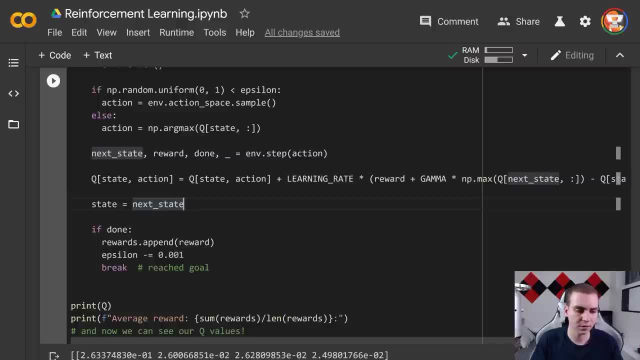 at least, But that's something that's important to note. So then, what we're going to do is reduce the epsilon if we die by just a fraction of an amount- you know, 0.001, just so we slowly start decreasing the epsilon and moving in the correct direction. And then we're going. 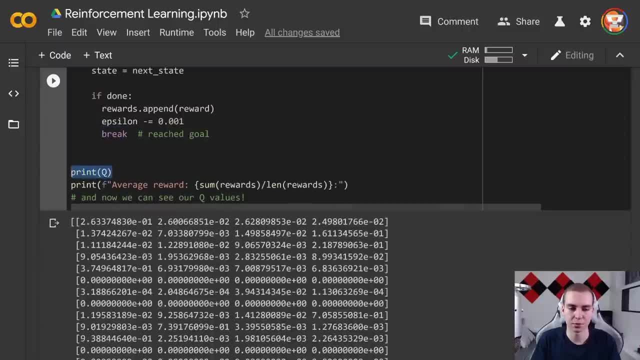 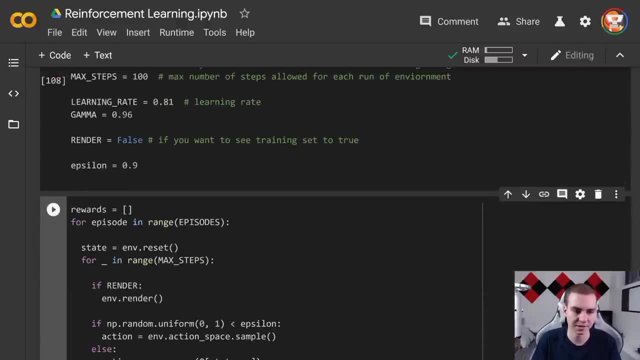 to break because we've reached the goals, print the cue table and then print the average reward. Now this takes a second to train. Like you know a few seconds really. that one is pretty fast because I've set this at was 1500. But if you want, you can set this at, say, 10,000, wait another, you know. 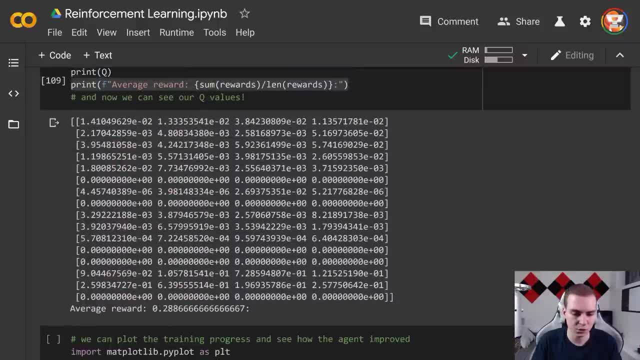 few minutes or whatever, and then see how much better you can do. So we can see that after that, I received an average reward of 0.288866667,. this is actually what the cue table values look like. So all these decimal values, after all these updates, I just decide. 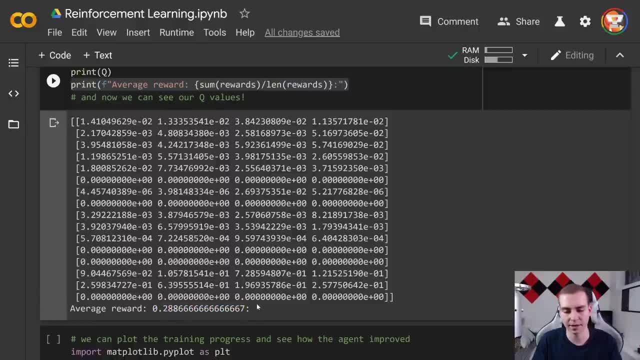 to print them out And I just want to show you the average reward so that we can compare that to what we can get from here. So, for instance, if you want to get a score, you can, you know- to what we can get from testing or this graph. So now I'm just going to graph this And we're 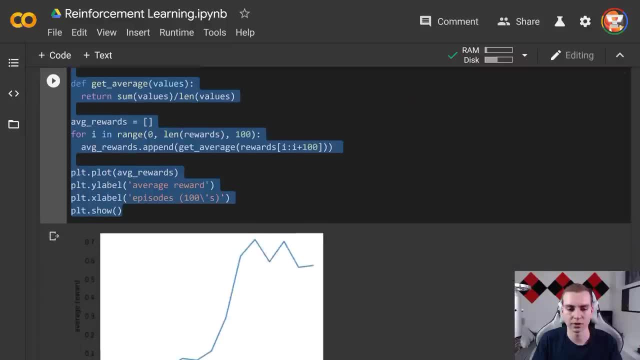 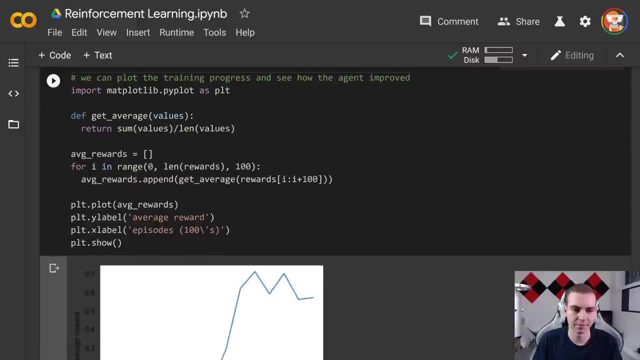 going to see. this is what the graph, so you don't have to really understand this code if you don't want to. but this is just graphing the average reward over 100 steps from the beginning to the end. So essentially I've been, I've calculated the average of every. 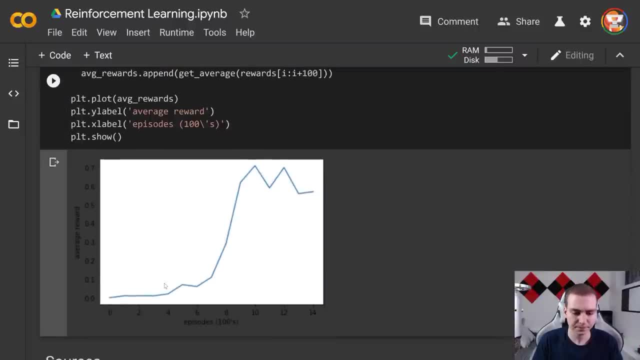 100 episodes and then just graph this on here, we can see that we start off very poorly in terms of reward because the epsilon value is quite high, which means that we're taking, you know, random actions pretty much all the time. So if we're taking a bunch of random, 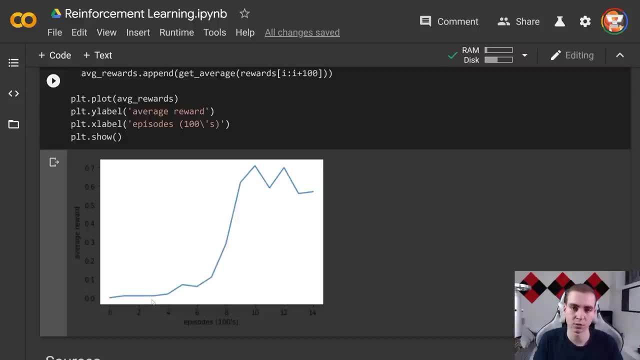 actions. obviously, chances are we're probably going to die a lot, we're probably going to get rewards of zeros quite frequently, And then, after we get to about 600 episodes, you can see that six actually represents 600. Because this is in hundreds, we start to slowly. 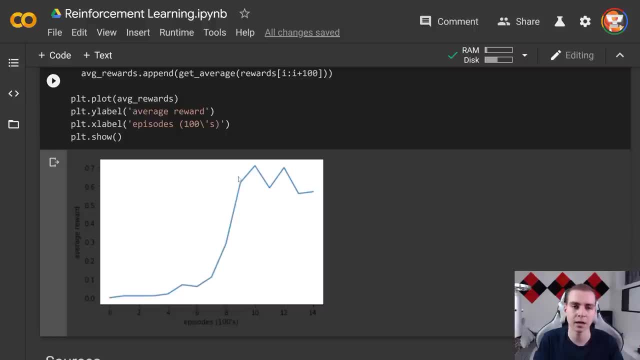 increase. And then actually we go on a crazy increase here where we start to take values more frequently. So the epsilon is increasing right. And then after we get here we kind of level off And I this does show a slight decline. But I guarantee you, if we were to, 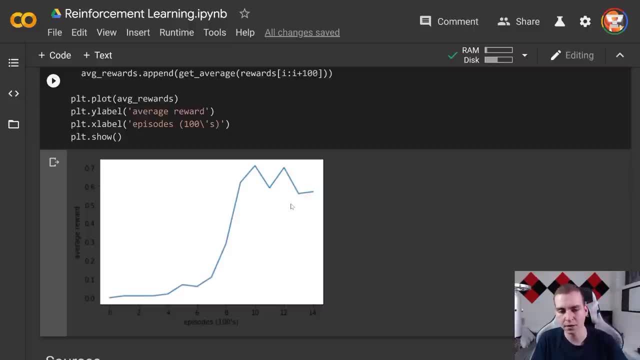 run this for you know, like 15,000, it would just go up and down and bob up and down, And that's just because, even though we have increased the epsilon, there is still a chance that we take a random action and, you know, gets your reward. So that is pretty much it for. 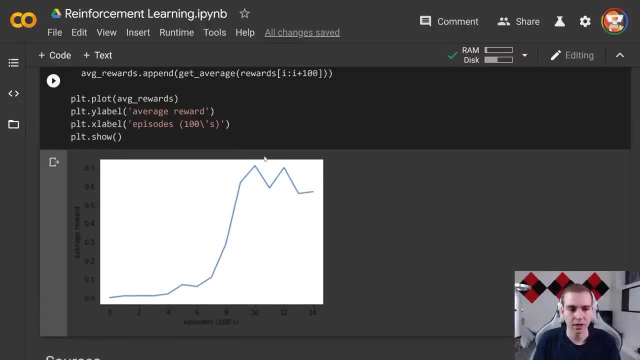 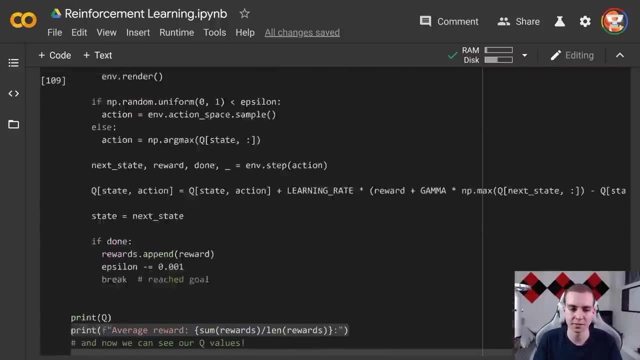 this cue learning example And I mean that's pretty straightforward To use the cue table If you actually wanted to say, you know, watch the agent move around the thing. I'm going to leave that to you guys, Because if you can follow what I've just done in here and 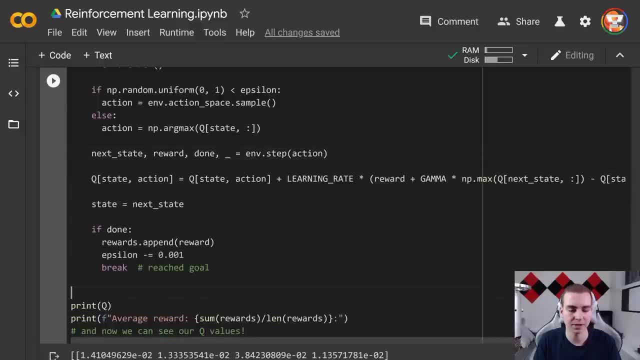 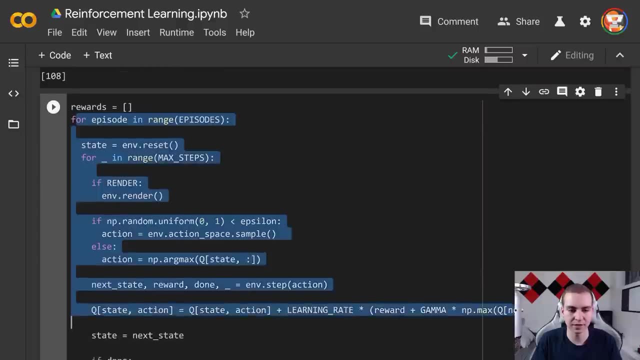 understand this. it's actually quite easy to use the cue table And I think as a lot of times like a final, almost. like you know, trust in you guys. you can figure out how to do that. The hint is essentially: do exactly what I've done in here, except don't update. 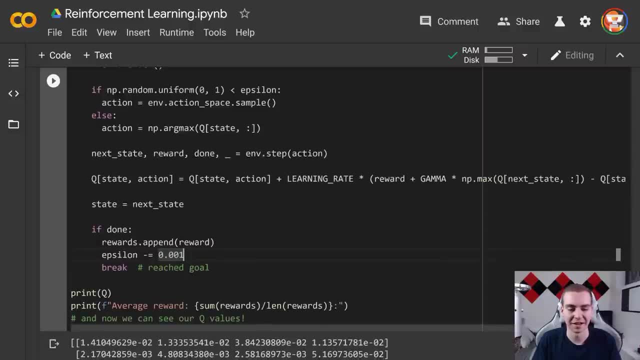 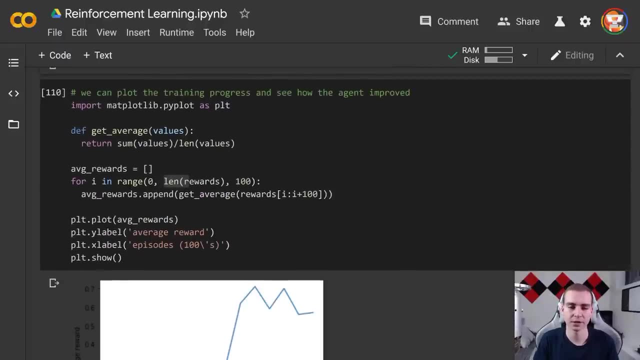 the cue table values. just use the cue table values already And that's you know pretty much all there is to cue learning. So this has been the reinforcement learning module for this TensorFlow course, which actually is the last module in this series. Now I hope. 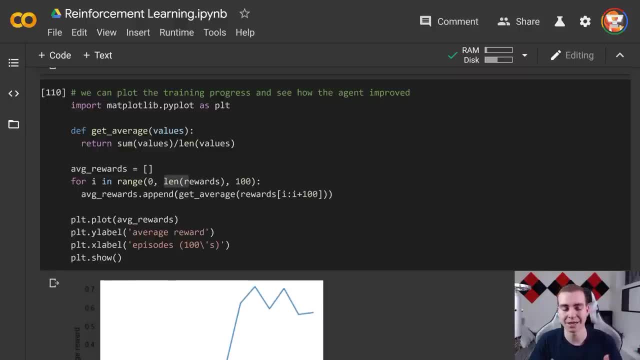 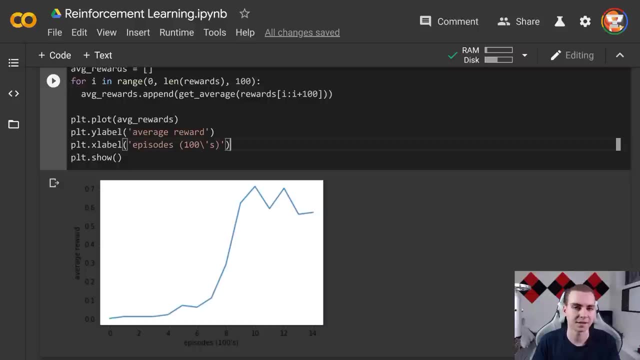 you guys have enjoyed up until this point. just an emphasis Again: this was really just an introduction to reinforcement learning this technique in this process. The problem itself is not very interesting and not you know the best way to do things. 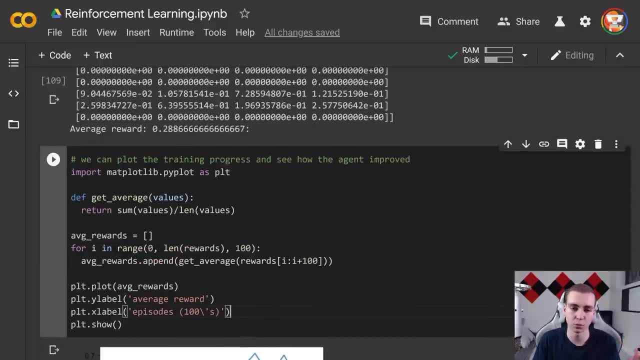 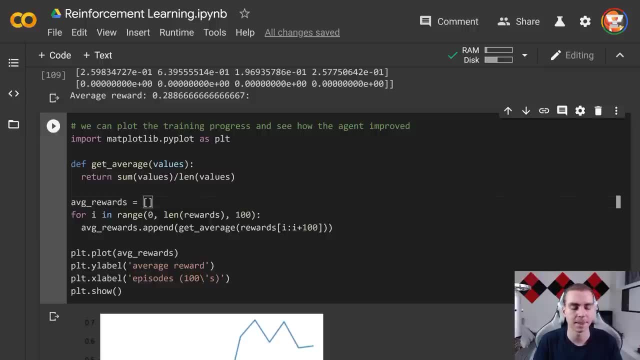 is not the most powerful. it's just to get you thinking about how reinforcement learning works And potentially, if you'd like to look into that more, there's a ton of different resources and you know things you can look at in terms of reinforcement learning. So 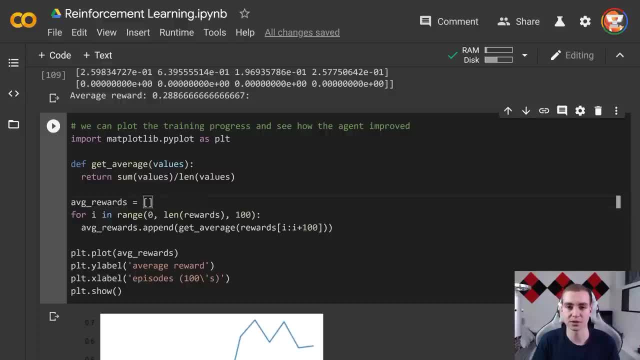 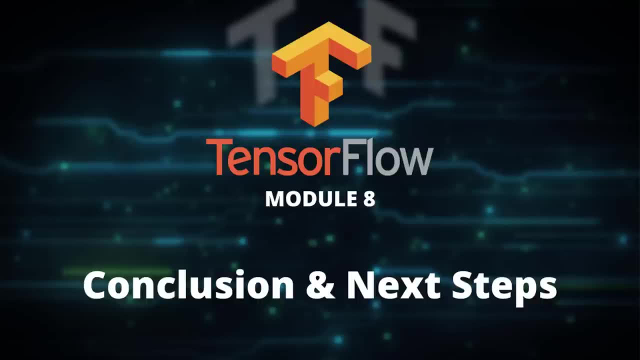 that being said, that has been this module, And now we're going to move into the conclusion. we'll talk about some next steps and some more things that you guys can look at to improve your machine learning skills. So, finally, after about seven hours of course, content. 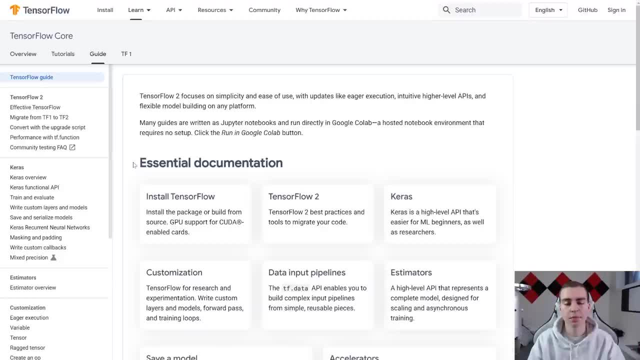 we have reached the conclusion of this course. Now what I'm going to do in this last brief short section is just explain to you where you can go for some next steps and some further learning with TensorFlow and machine learning, artificial intelligence in general. Now what? 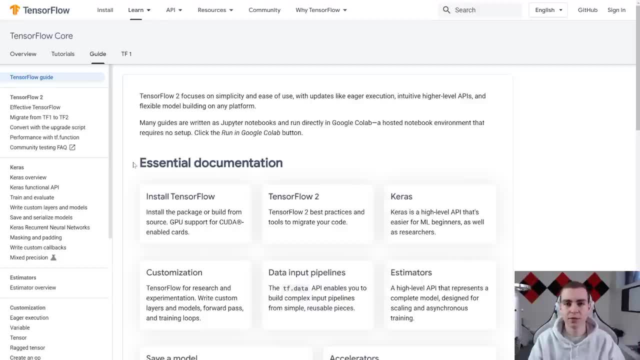 I'm going to be recommending to you guys is that we look at the TensorFlow website, because they have some amazing guides and resources on here, And, in fact, a lot of the examples that we used in our notebooks were based off of, or exactly the same as, the original TensorFlow. 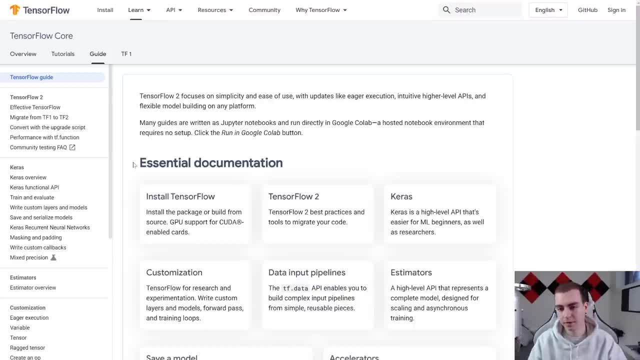 guide. The code that they have is just very good. They're very good and easy to understand. examples And, in terms of learning, I find that these guides are great for people that want to get in quickly, see the examples and then go and do some research on their own time and understand. 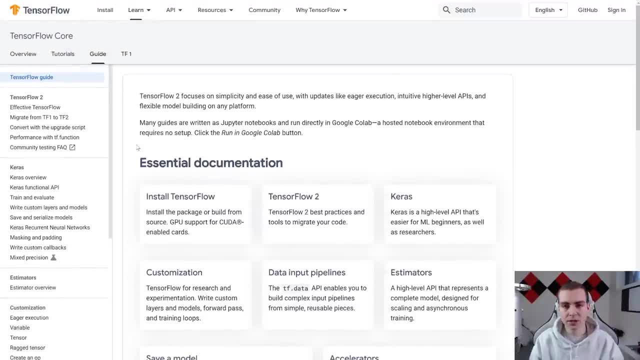 why they work. So if you're looking for some further steps at this point in time, you have gained a very general and broad knowledge of machine learning and AI. you have some basic skills in a lot of the different areas And hopefully this has introduced you to a 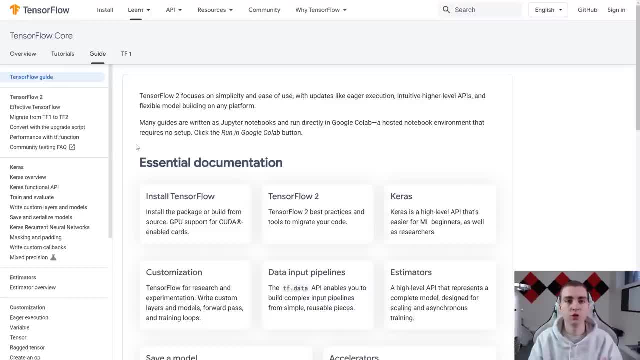 bunch of different concepts And the possibilities of what you are able to do using modules like TensorFlow. Now what I'm going to suggest to all of you is that if you find a specific area of machine learning or AI that you are very interested in, that you would dial in on that area and focus most. 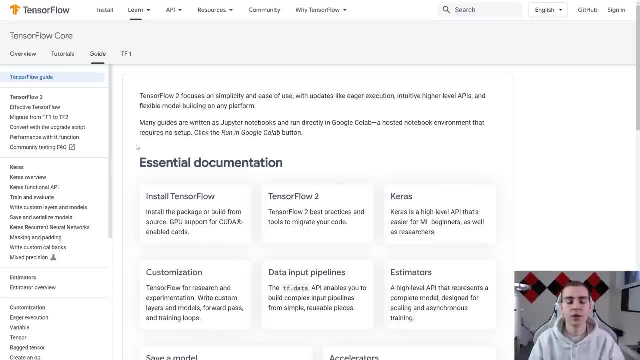 of your time into learning that. that is because when you get to a point in machine learning and AI where you really get specific and pick one kind of strain or one kind of area, it gets very interesting very quickly And you can devote most of your time to getting as 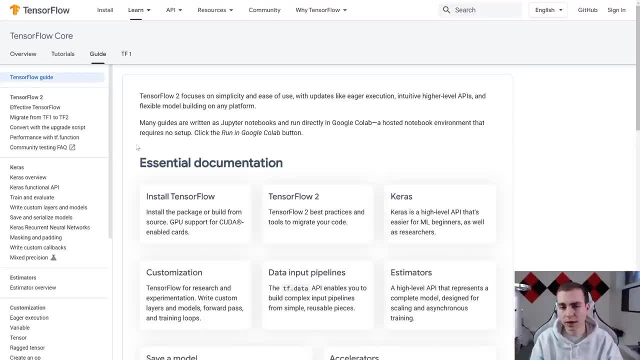 deep as possible And that specific topic, and that's something that's really cool. And most people that are experts in AI or machine learning field typically have one area of specialization. Now, if you're someone who doesn't care to specialize an area or you just want to play around and 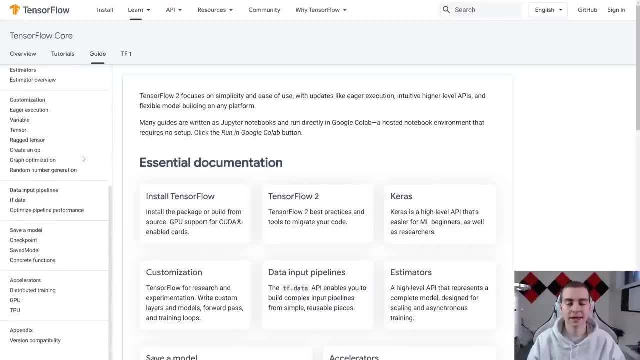 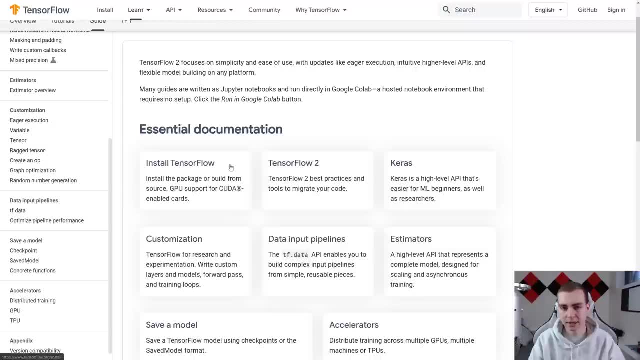 see some different things. the TensorFlow website is great to really get kind of a general introduction to a lot of different areas and be able to kind of use this code, tweak it a little bit on your own and implement it into your own projects. And, in fact, the next.